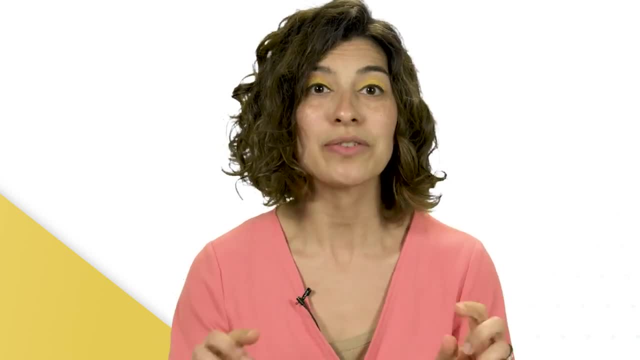 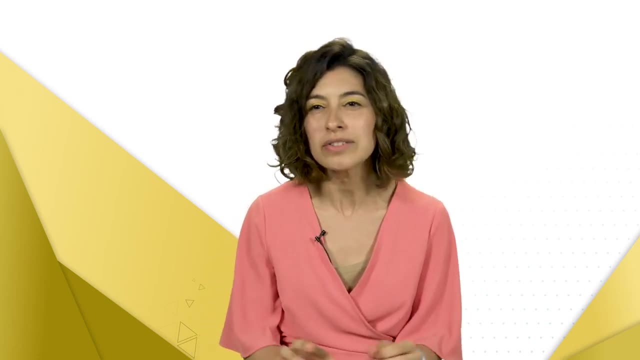 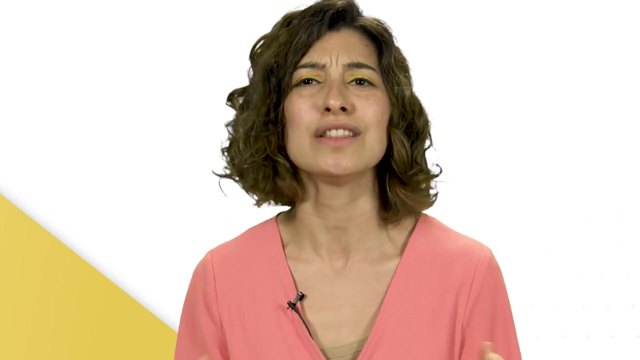 sense and a need to explore the potential of a particular mathematical algorithm can express thoughts numerically is part of this knack for patterns. We humans are pattern searchers and mathematics is the ultimate expression of our conquest of patterns. The word mathematics comes from mathema that relates to gaining knowledge. 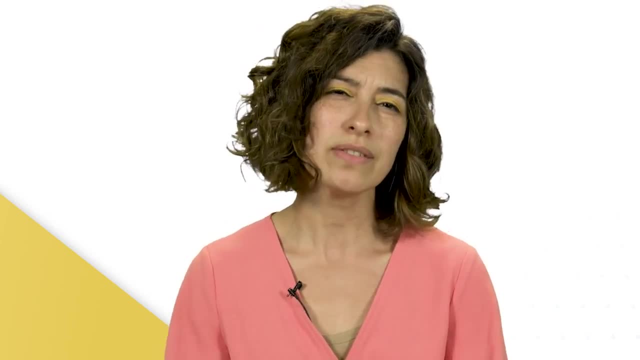 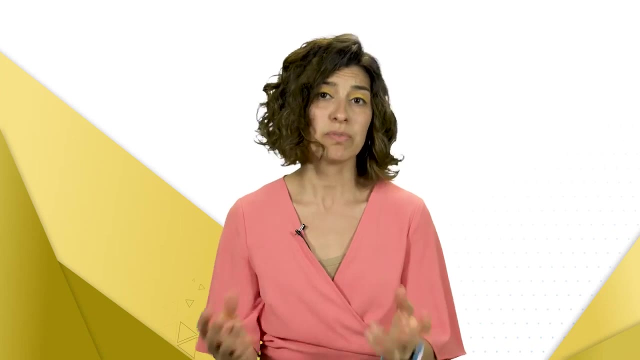 to really knowing something. Patterns, rhythm, beauty and the pleasure that comes from those are a very human thing. People specialize on how they deal with patterns. Some paint it, dance it, sing it, drum, it feel them cause patterns in others. 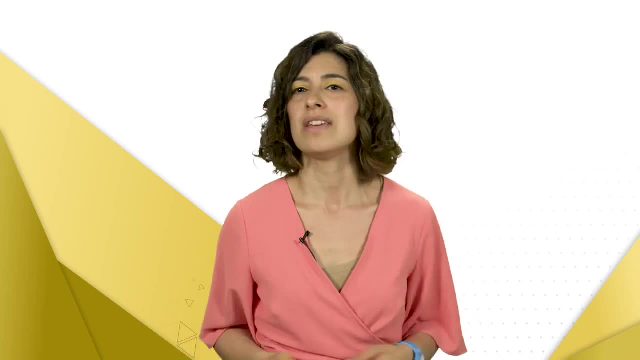 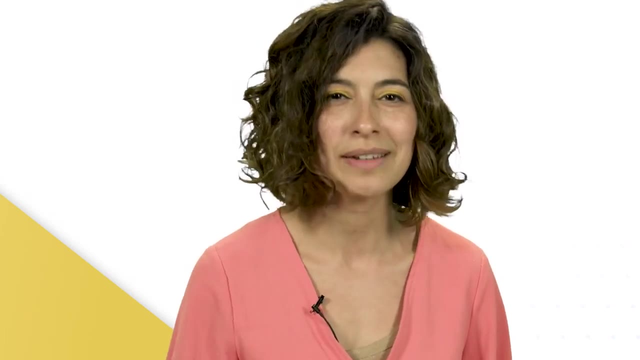 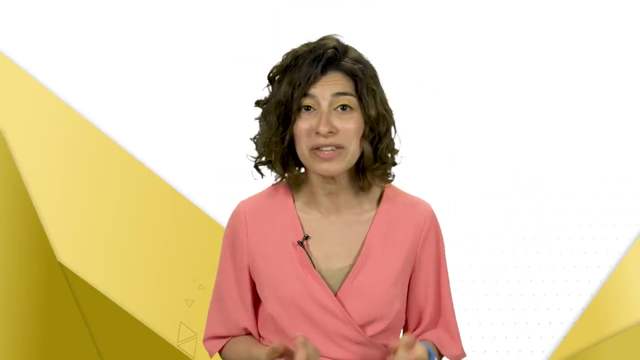 via words, code, laughter medicine, others, even without a physical context. Being a mathematician, observing patterns, seeking the rule behind them, being able to know things for sure, proving that a rule works, Also being baffled by the mysteries of patterns is all part of being human. It is the process of studying. 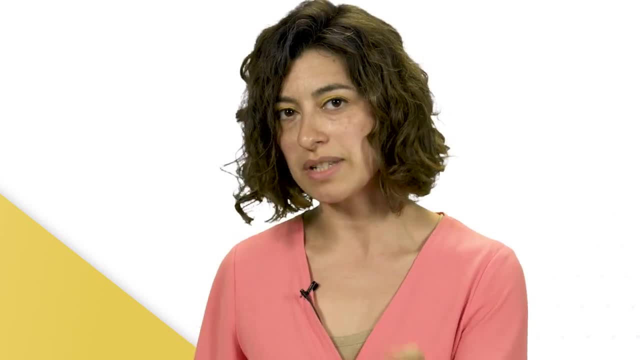 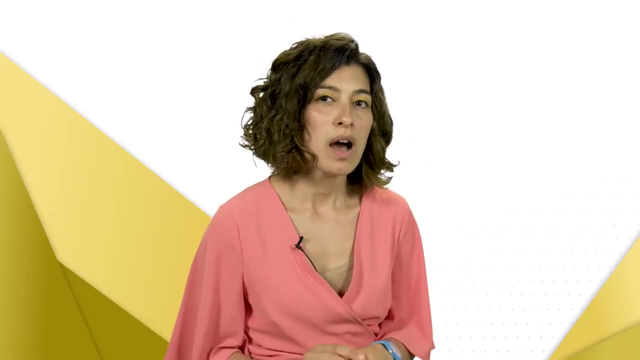 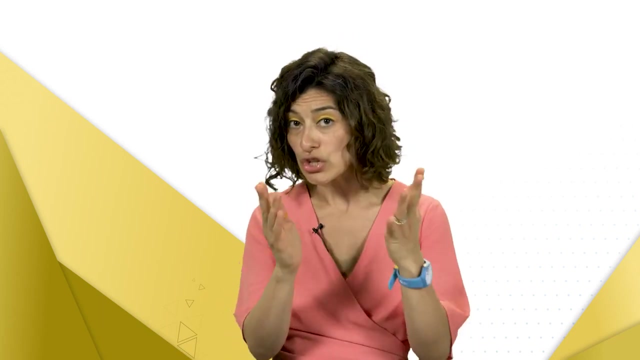 patterns that we nowadays call mathematics, But deep down we are all mathematicians. Some of the mathematics we cover here may be familiar to you. other parts may seem outlandish, but we keep it all linked to computing situations and we invite you to always place the maths we learn in the context. 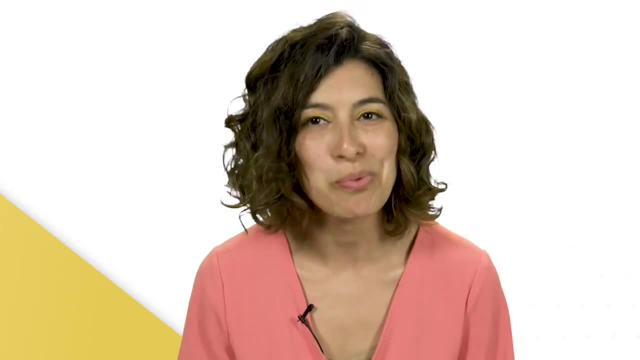 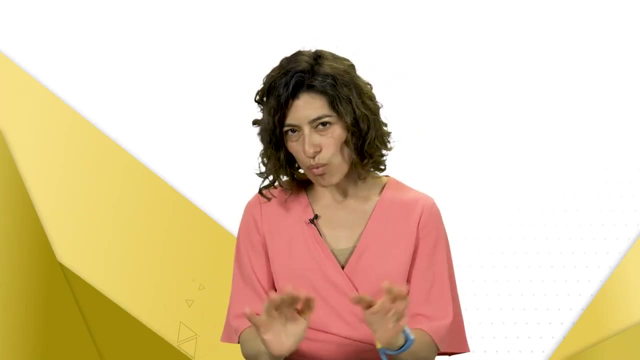 of a theme or a problem in computing. We will support you on that journey too. But what have I got in store for you? This module is designed as a walking and climbing journey. We are in it together, and I have prepared the way You are going. 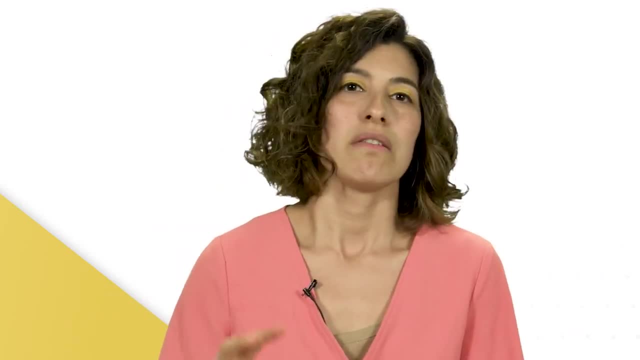 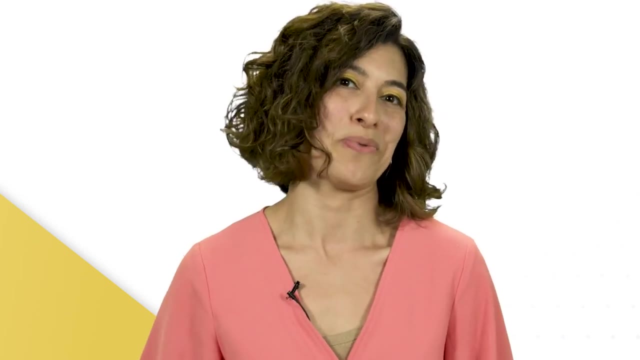 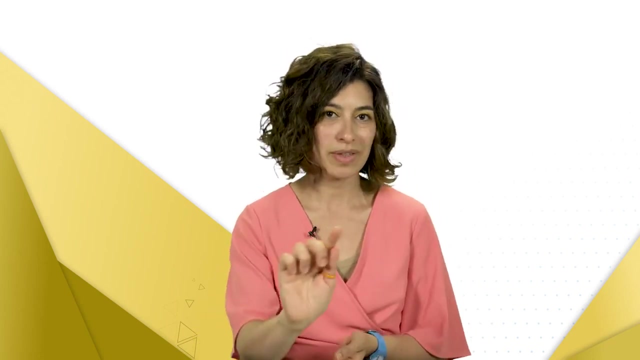 along the same path with enough room for you to do your own footsteps. but you are to do the walking and you all can talk along the way. I'll point out some beautiful bits on the landscape. You will have options to go off the track sometimes, but within sight. 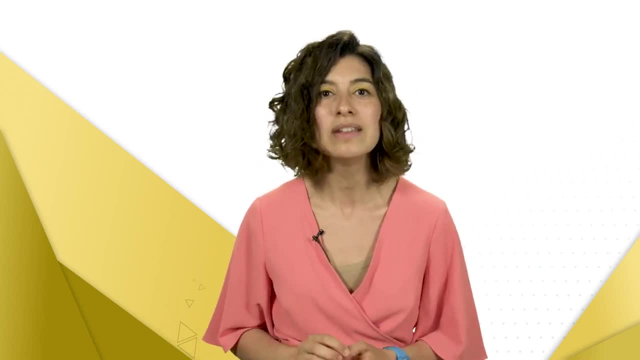 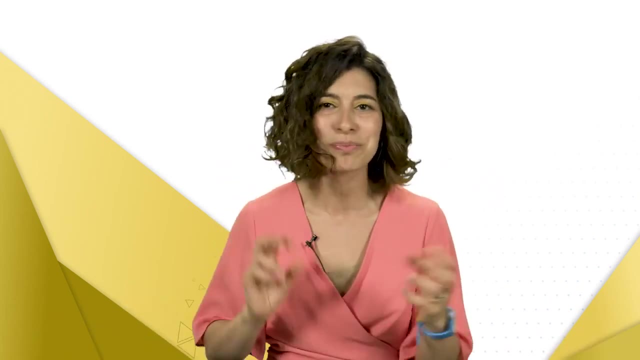 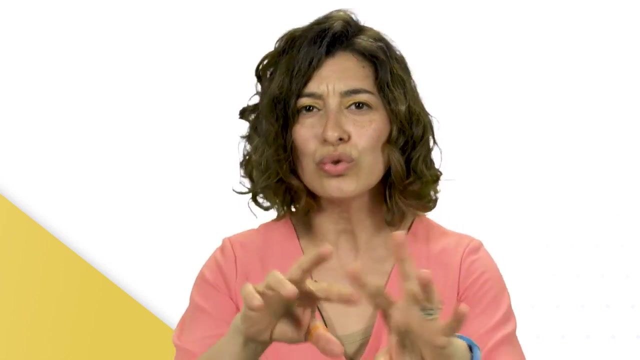 of the journey. You can stop and have a breathe and then race back in. You can also talk along the way. I hope you also point out to all of us when you find a new flower tree or special rock along the way. The videos that contain examples were made thinking about you stopping the video. 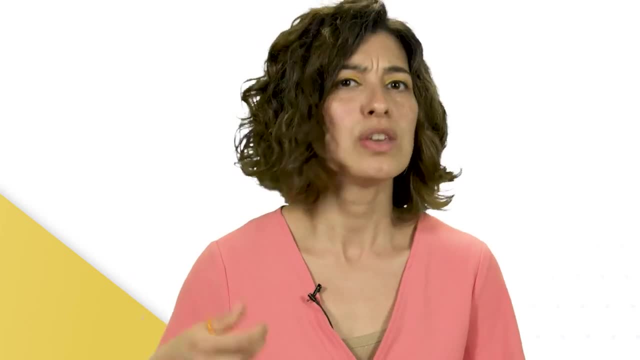 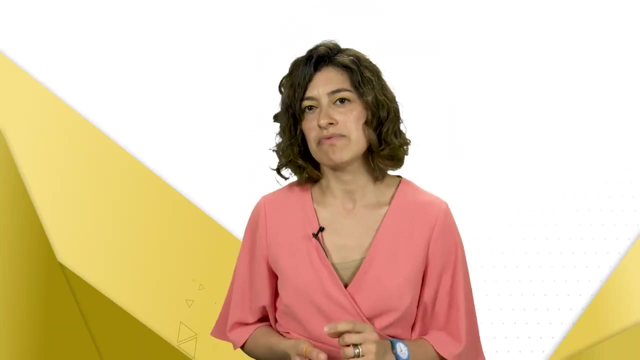 and working through the example yourself with good old fashioned pen and paper before you check against my results. Don't be tricked by the need to be right all the time. The surprise of being wrong and learning from it is a very valuable experience. 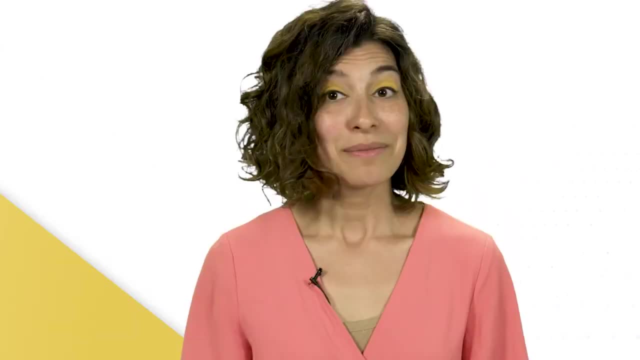 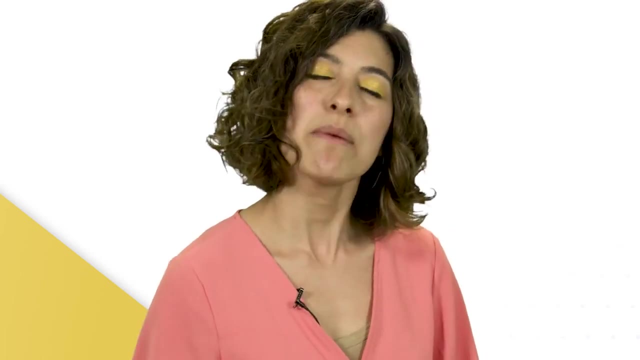 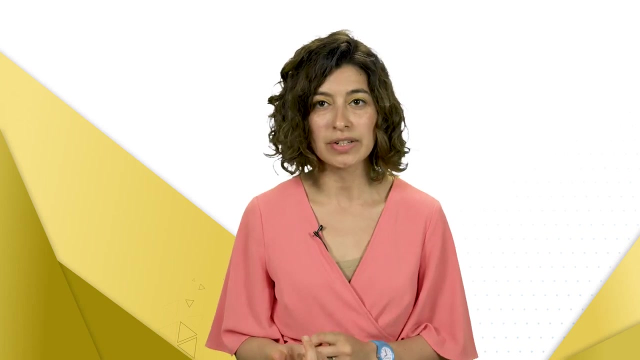 So enjoy it and learn. Sometimes you will be asked to read something in advance or think of a problem or revise a topic before a lecture. Do it and bring your own notes and thoughts- questions- with you. You need a scientific calculator that is not your computer or your. 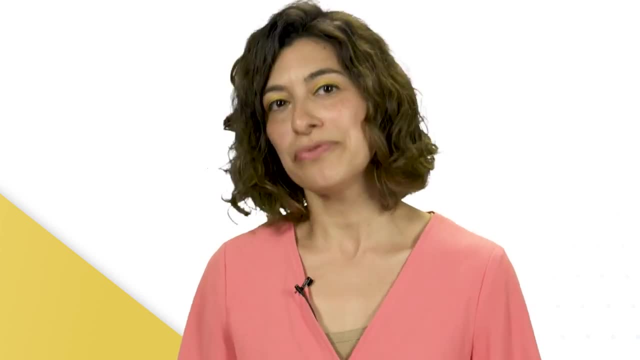 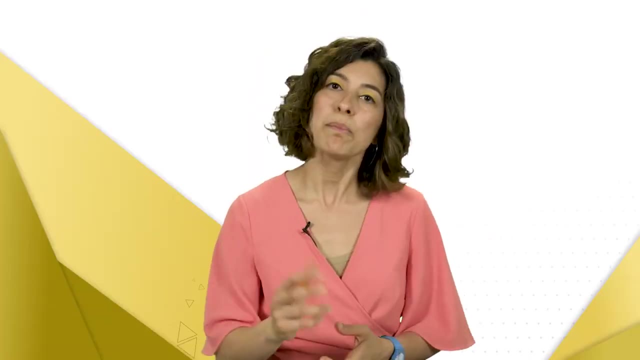 phone After each video. do attempt the formative quizzes as soon as possible to understand if you need to revisit the videos or if you can progress to the next one. I hope you have a great day. The point of the formative quizzes is for you to get feedback on your learning, so do. 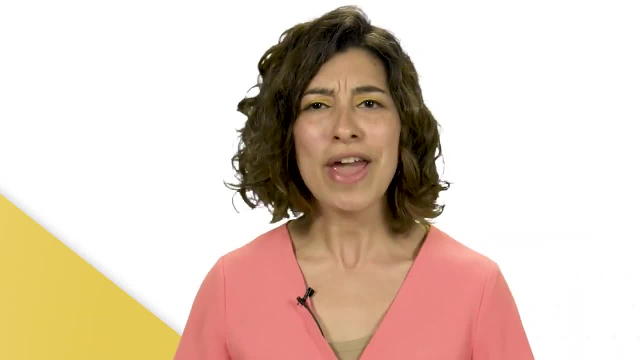 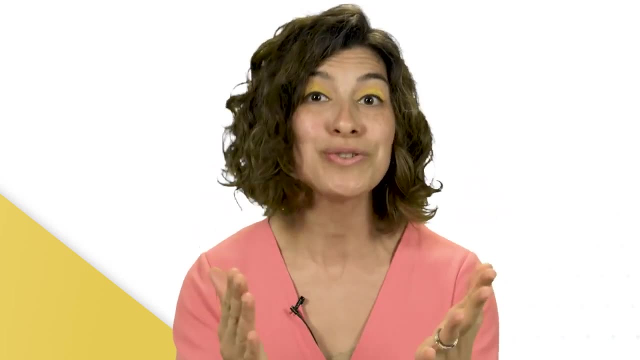 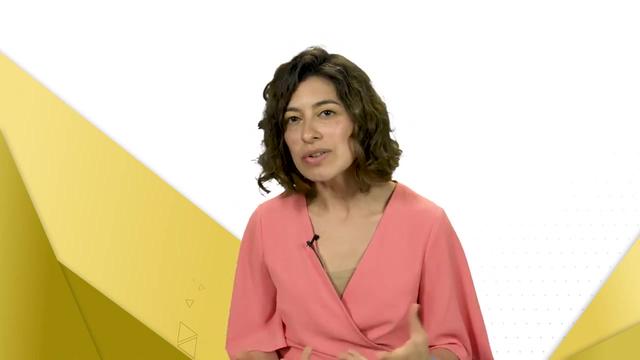 attempt it early on and as often as you need. Embrace the difficulties as learning moments and share your questions and thoughts in the discussion forum. We want you to succeed. There will be tasks with problem solving elements and some peer reviews. You are encouraged. 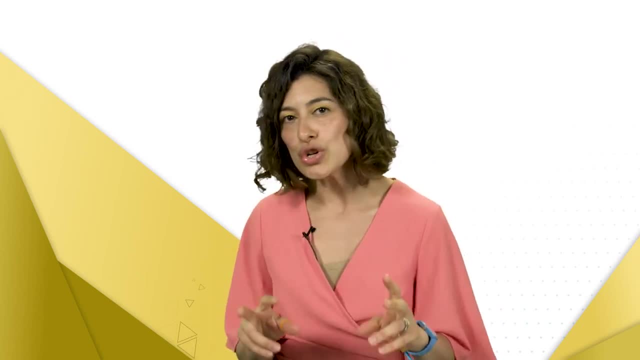 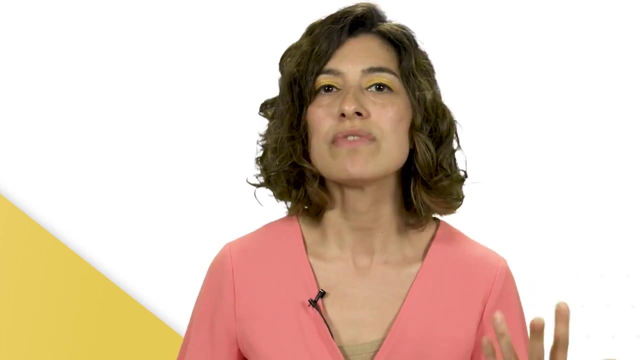 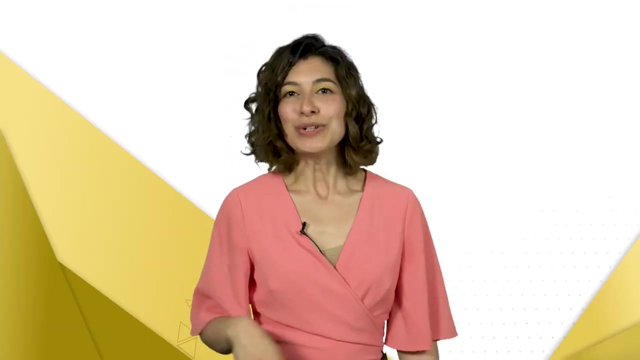 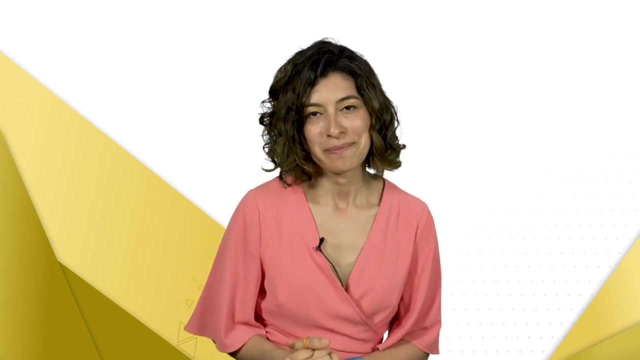 to discuss some elements of these tasks in the forum. to make sure you understand the assignment, There will be at least one summative quiz per topic that may contain questions that require you having completed previous tasks in order to be able to answer. We will look at numbers, functions, geometry, linear algebra and simple probability. 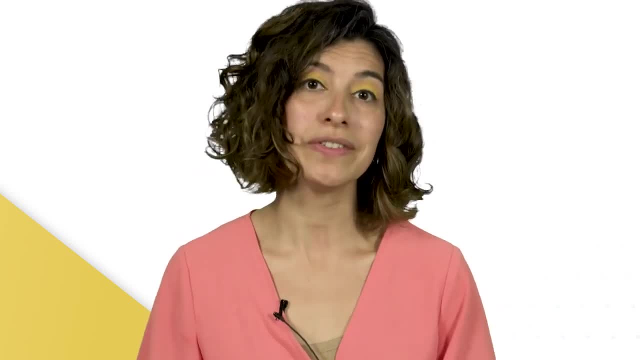 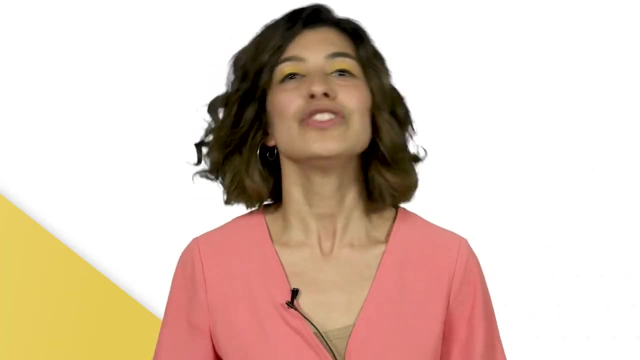 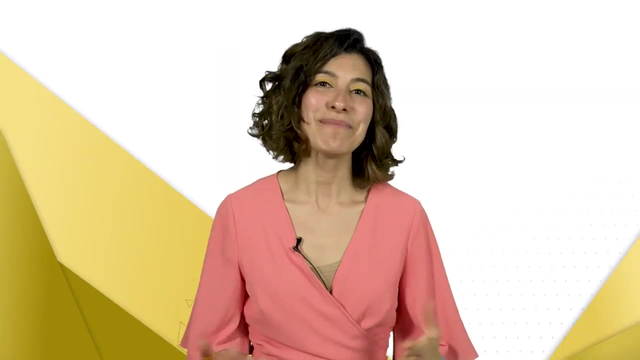 Numbers will include binary and other bases, as well as sequences and series. In functions we will look at graphs, but also at calculus. In geometry and linear algebra we will go through triangles, vectors and matrices. Come along with us in this journey and enjoy the module. 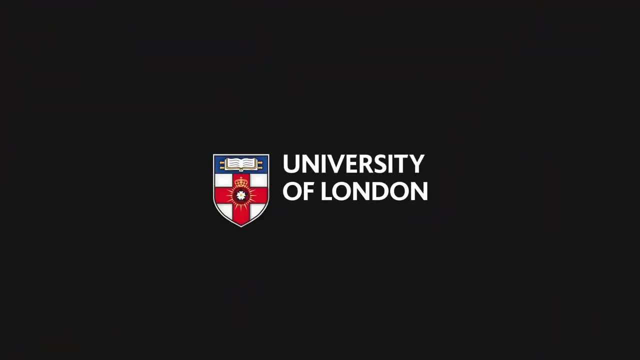 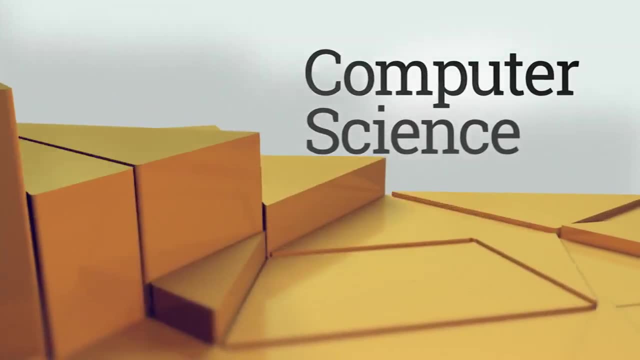 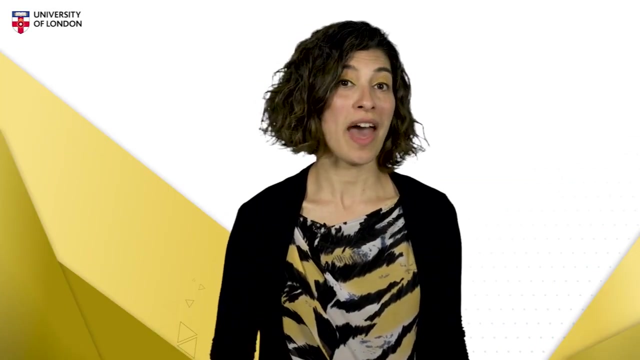 Have you ever wondered how computers work at the very lowest level? Yes, they do, But how do they work at the very lowest level? Well, the answer is simple: They work at the very lowest level. How do they work at the very lowest level? 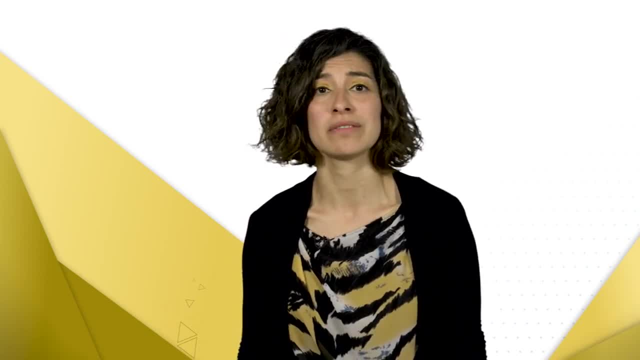 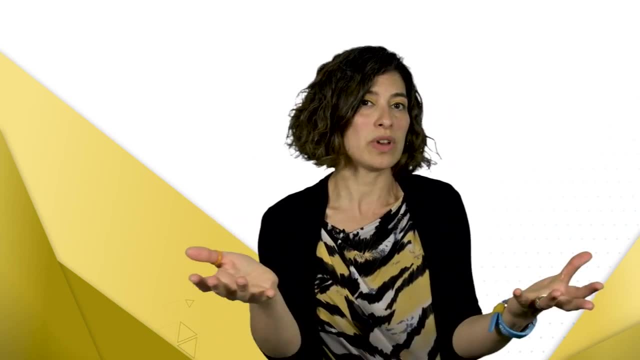 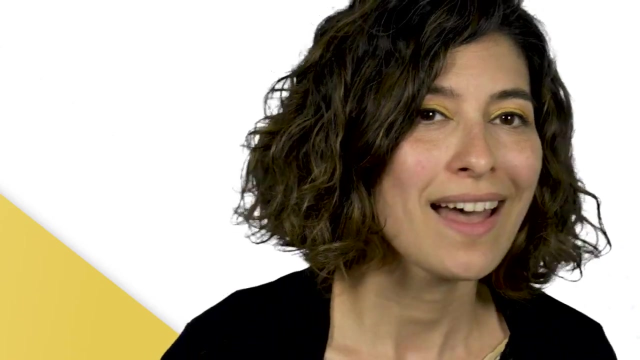 Well, how is the input of information that you enter by either touching a screen or typing on a keyboard used inside a machine to be computed into an action such as opening a website, playing music or even just adding up numbers? In computing? everything is number. 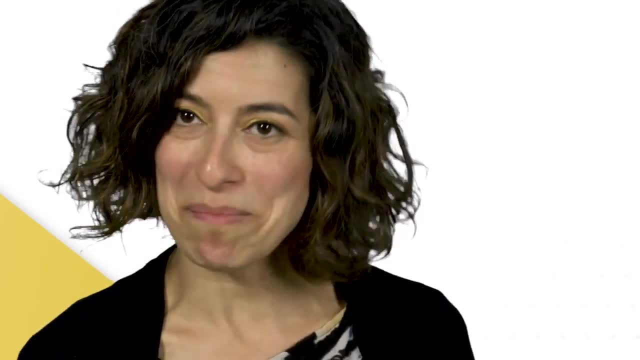 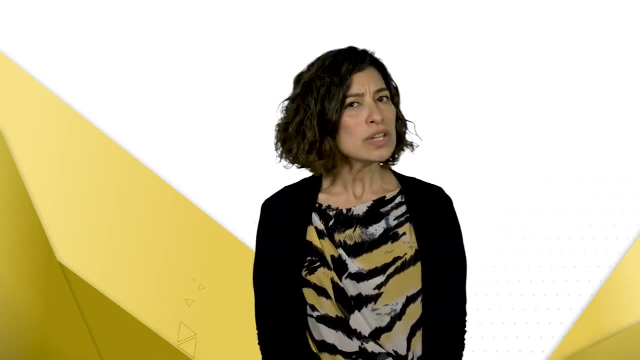 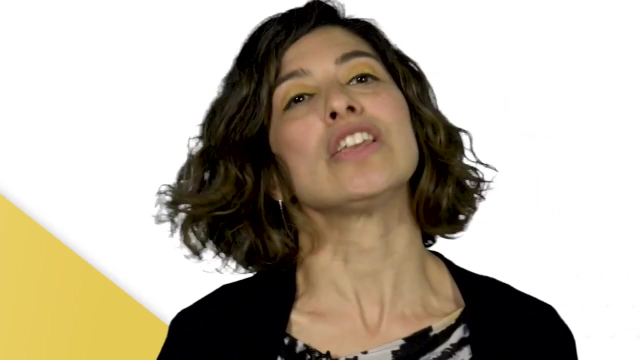 Everything is treated as a number and it all boils down to comparing and operating with zeros and ones. But how? And do you need to know all about this low-level process all the time? Fortunately, the answer to that question is no. You can abstract from it, but it will save you a lot of bother if you have a sense of. 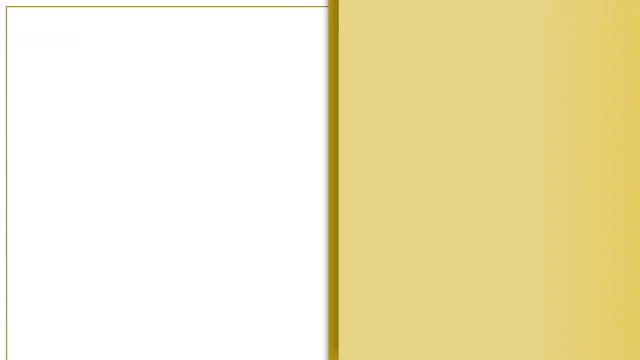 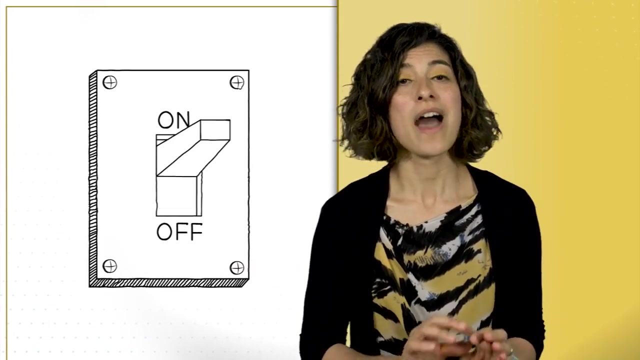 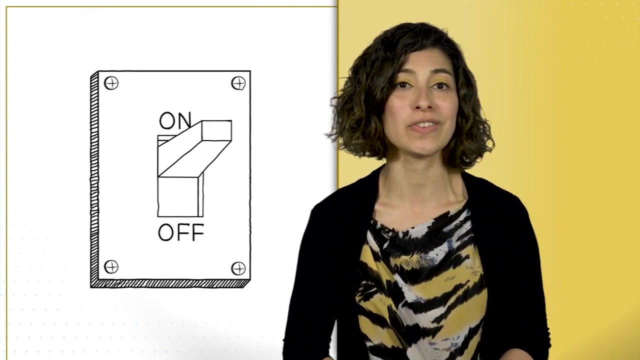 how it works, And here's an idea. A light switch is either on or off and at the very basic level there are many switches inside a computer, And operations that involve the on and off state of switches make the whole magic of computing work. 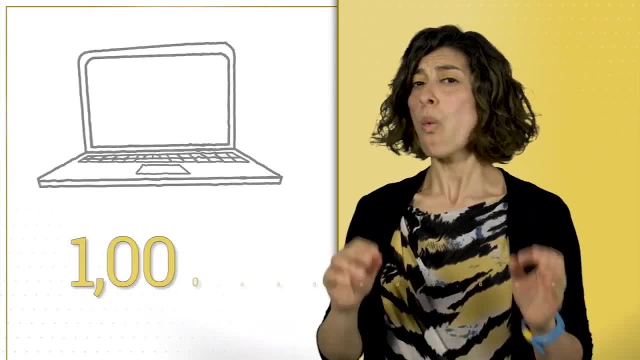 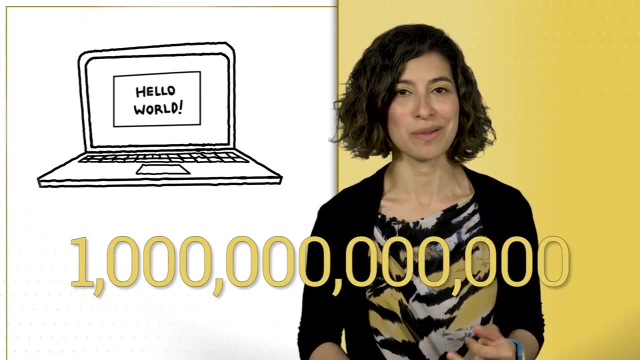 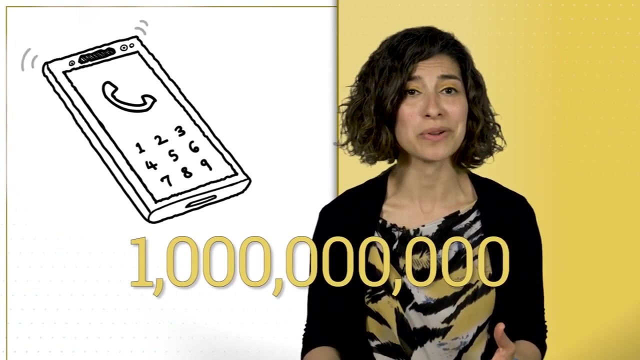 Here's how many switches are inside each type of computer. There's one billion switches inside a laptop- I used a long scale for naming numbers with large numbers of zeros- And there's one thousand million switches inside a smartphone. Two million switches inside a computer. 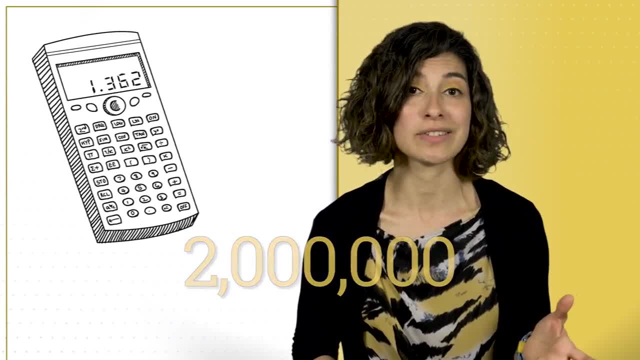 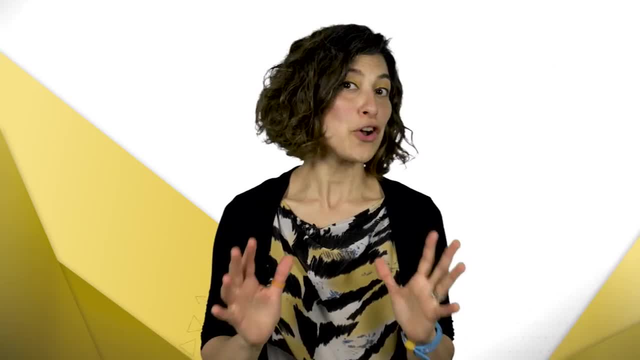 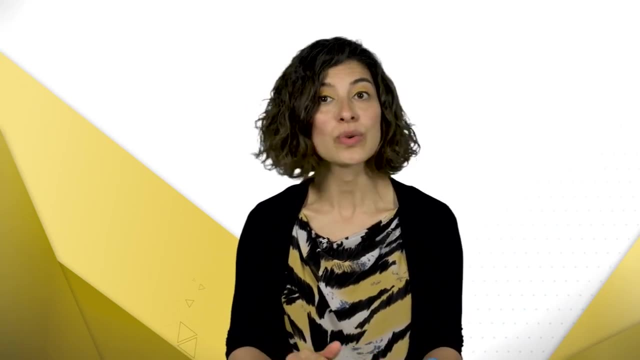 Two million switches inside a scientific calculator. By the way, you are going to need one for this course. Now I've got a job for you. Go and find out what I mean by switches. I wanted to go and find out what is at the hardware level that makes the computations. 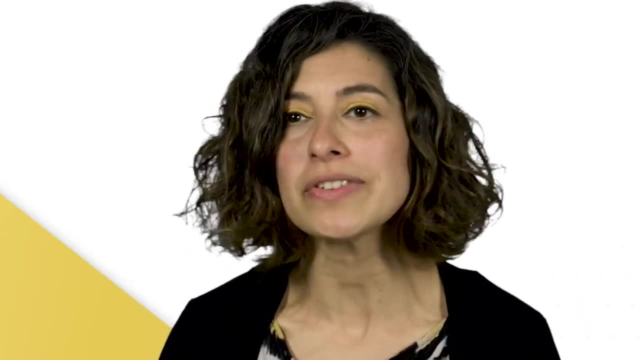 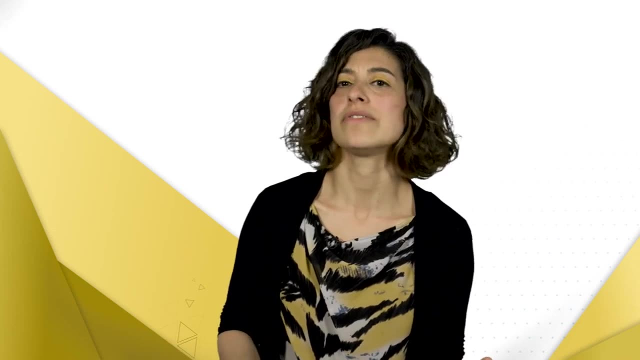 inside a computer. Go to the lowest, simplest level you can and discuss with your peers in the discussion forum on the following lessons: Bye, What other devices have switches? You go and find out which everyday gadgets and devices have it and how many. 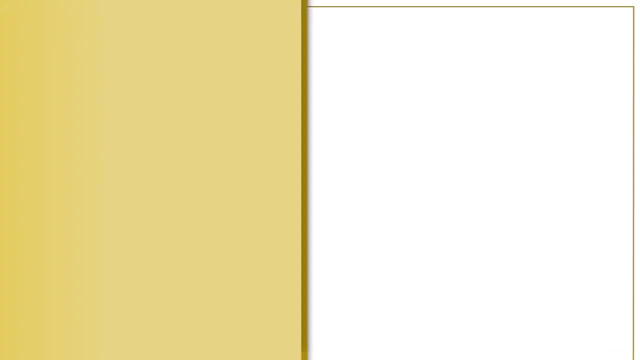 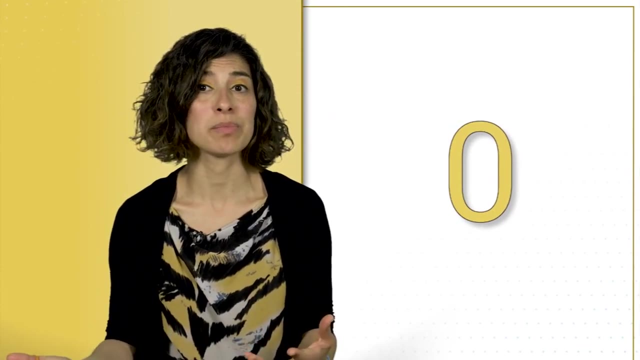 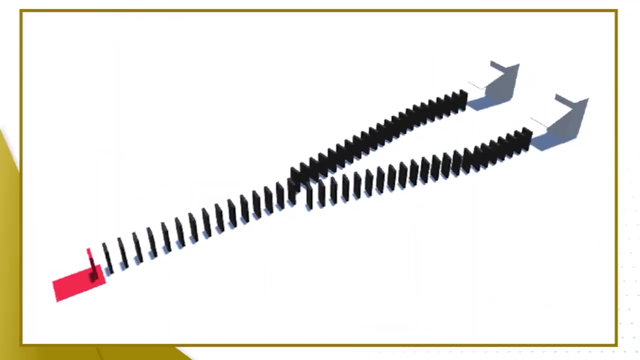 Bring back your findings to the discussion forum. Basically, on equals one, off equals zero. And here's one example of these switches in action. I do nothing- zero and nothing happens. So input zero gives output zero. I push it so it is an input of one and at the end I have an output of one. 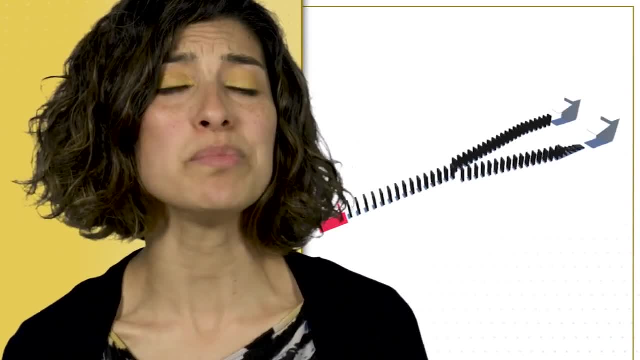 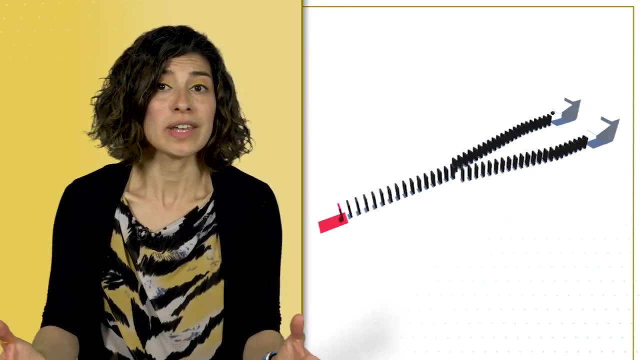 We can do operations with these switches and in a full computing degree. you study them as logic gates and create a computer. If you fancy it, you can buy kits of connectable logic gates and build your own devices. Or if you're like me, 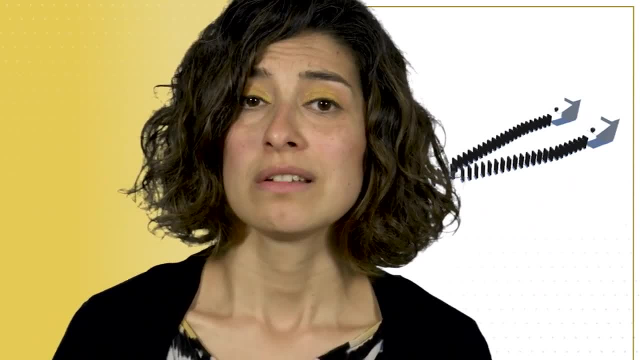 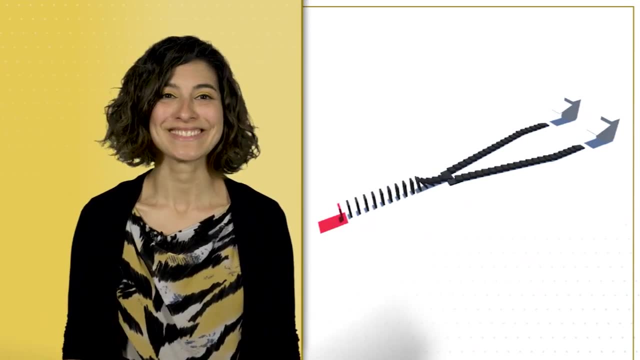 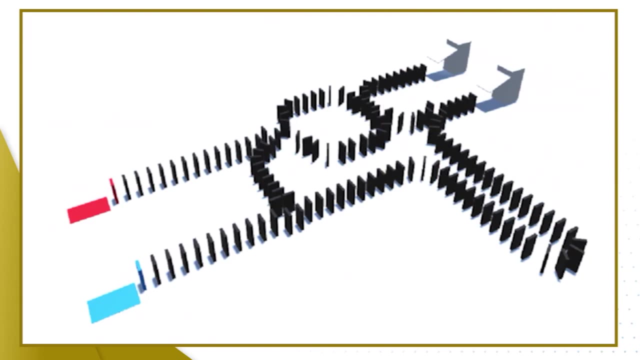 and like doing things from scratch. you can build a simple computer using rods and spindles or Lego parts or even dominoes. And here's a simple calculator. It performs the addition of two numbers. It adds zero plus zero, zero plus one. 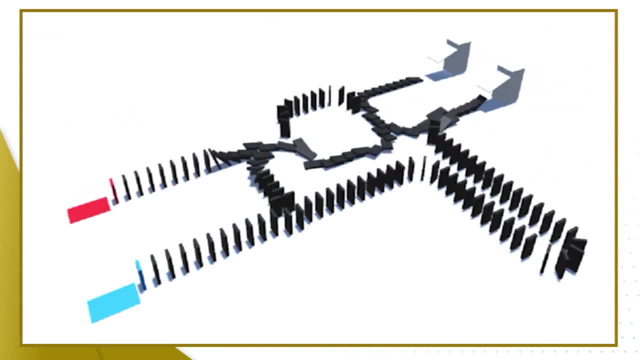 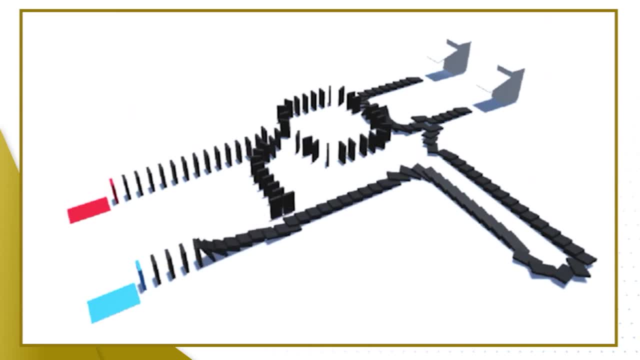 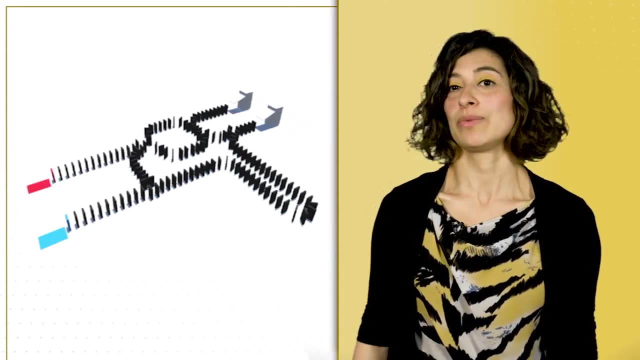 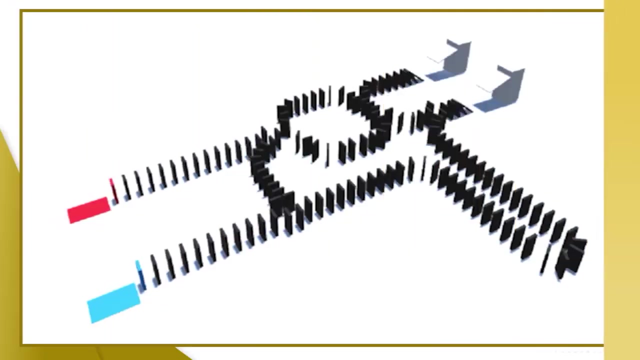 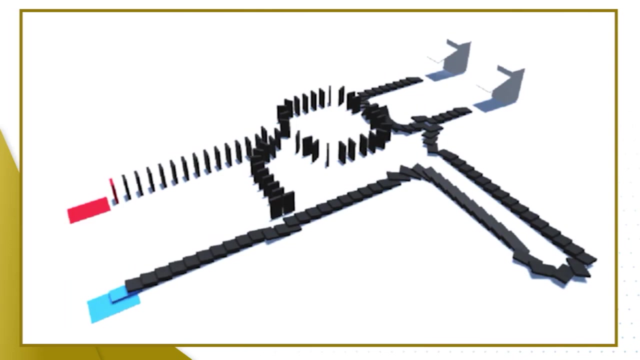 one plus zero and one plus one. I know you are really impressed with this level of calculation, But bear with me. We add up one plus one here. Well, one plus one is two, But we've got one hour, one output with nothing and one output with one. 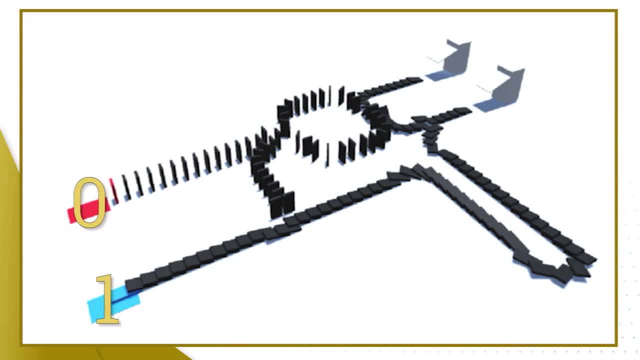 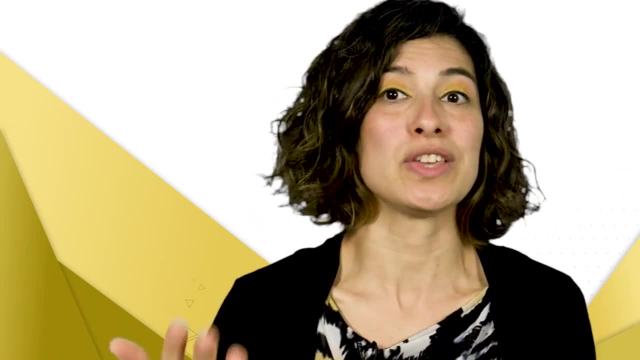 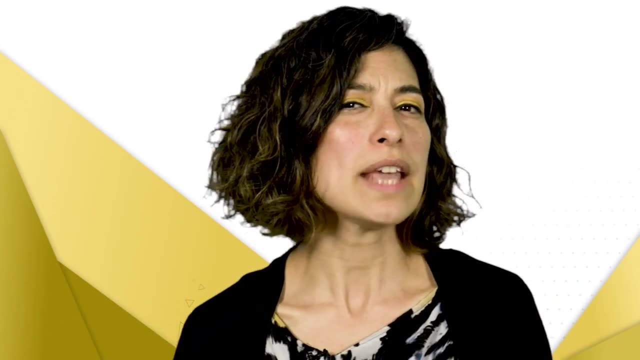 How is this two? In other words, what is the meaning of each of these outputs? They are like symbols to represent numbers. just like you and I use 35, three, five to mean three tens plus five ones. So the outputs have a value of ones and twos. 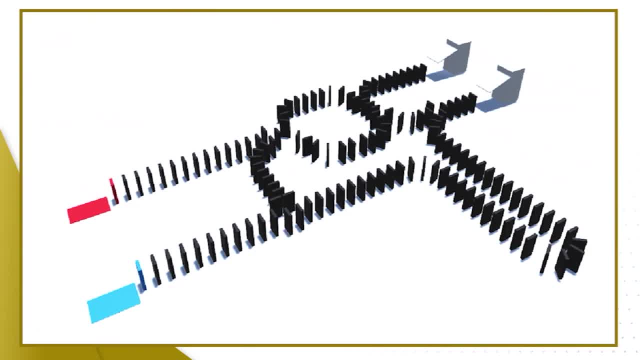 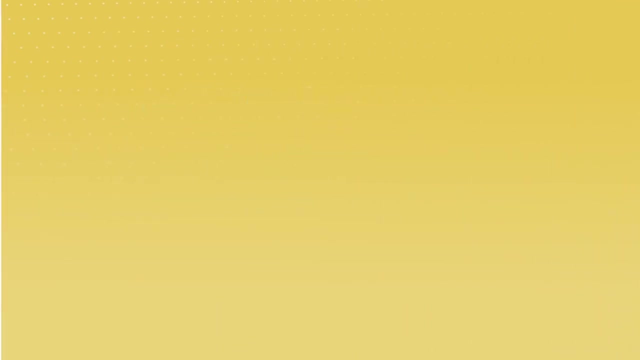 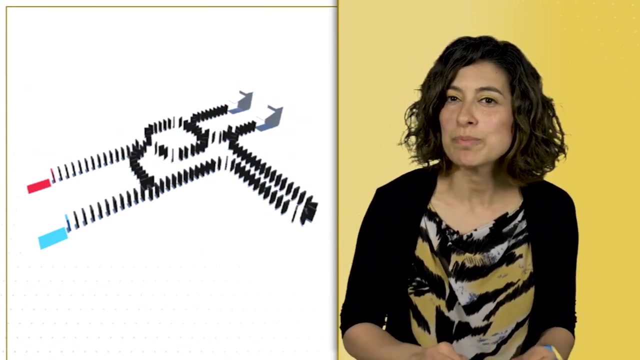 Let's have you deciphering this, Study this image carefully and when you think you've got it, give your answer in the InVideo quiz. Okay, some of you got it. The inputs are units, either zero or one. the output on the left is worth one if it's on. 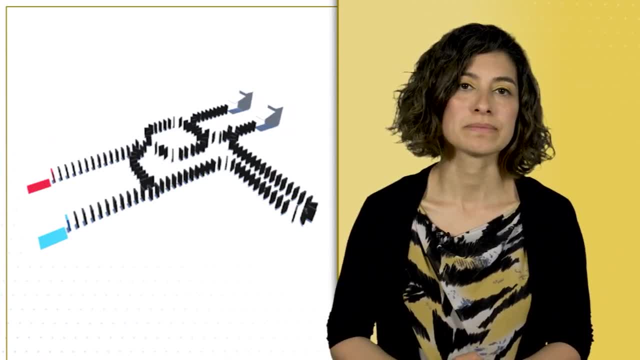 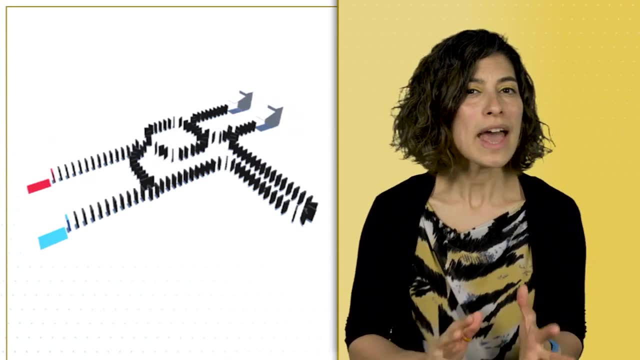 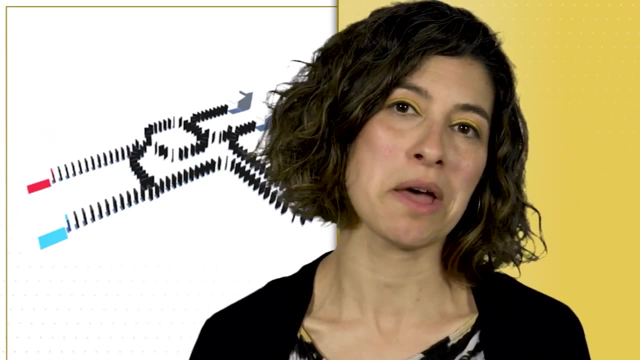 or zero if it's off. so either zero or one. The output on the right is worth two if on, zero if off. So the left is for ones and the right is for twos. Together the two outputs can make the numbers. 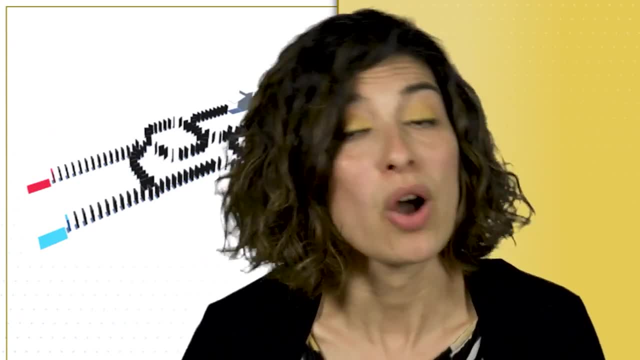 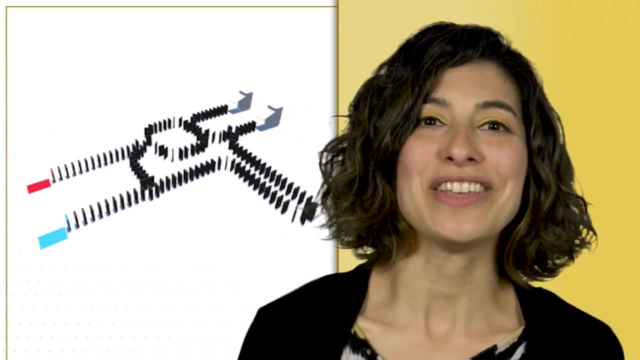 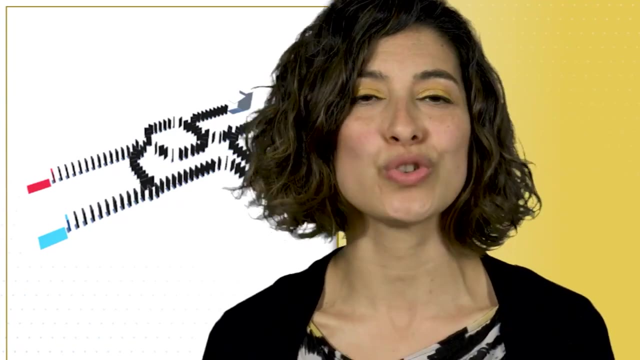 zero, one, two and three, Although in this calculation, we never get an output of three. as a result, The clever thing is to code numbers using zeros and ones in positions that are worth one or two. It takes about 148 dominoes for this operation. 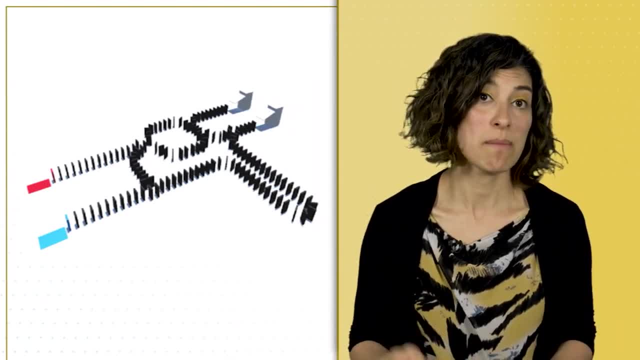 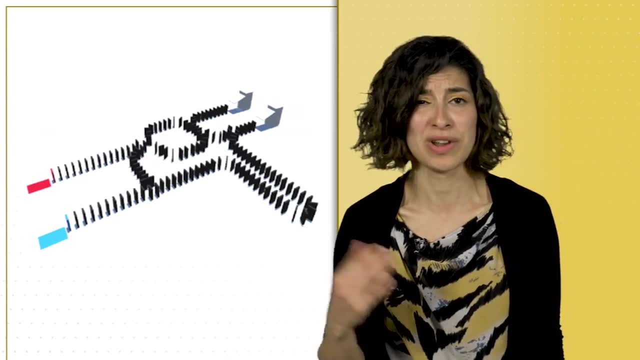 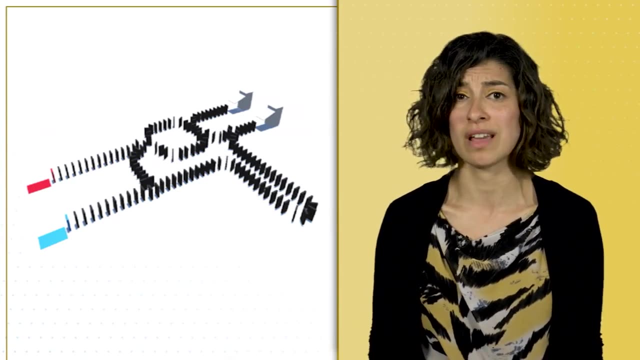 Adding up two two-digit numbers in this fashion, made of zeros and ones, only takes about 10,000 dominoes. So you can imagine the trillions of dominoes needed to to mimic a smartphone And imagine how long computations like the ones 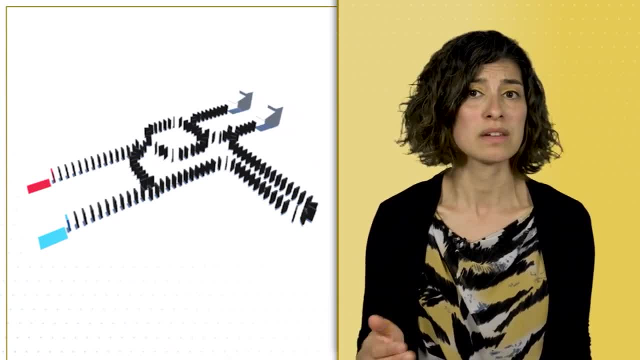 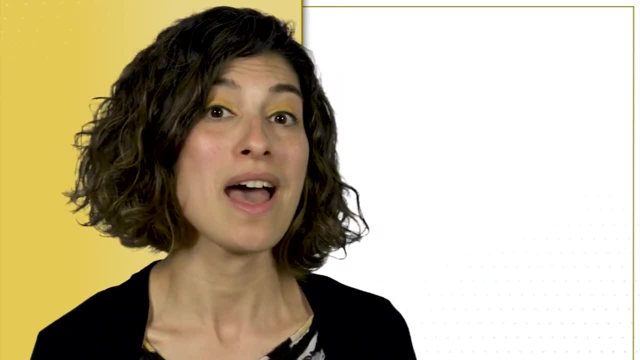 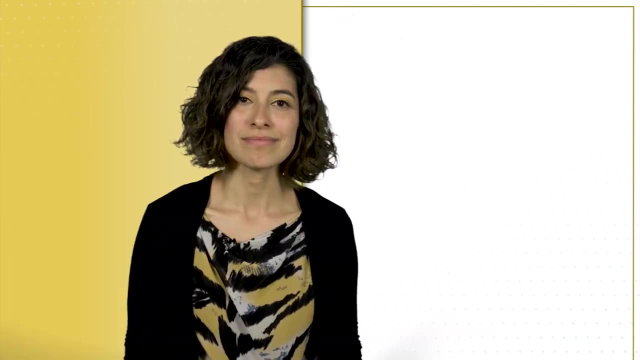 performed by a smartphone would take if mimicked in dominoes. I invite you to go and visit your nearest science museum and learn about the initial computers and then predecessor mechanical calculators. The key element in a computer is the ability to have a device that makes decisions under logical rules. 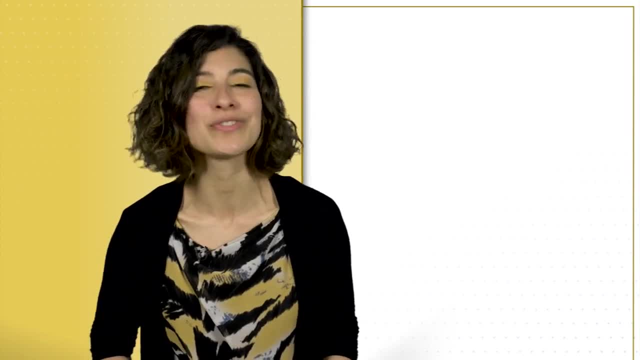 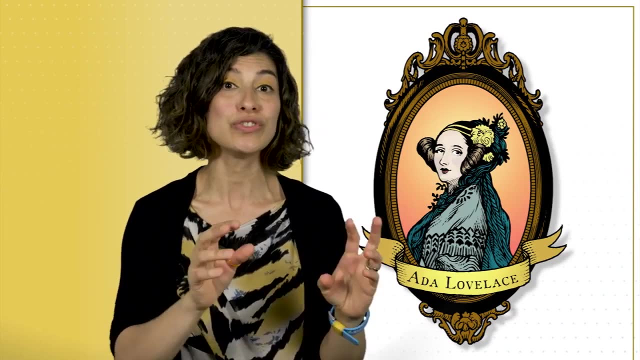 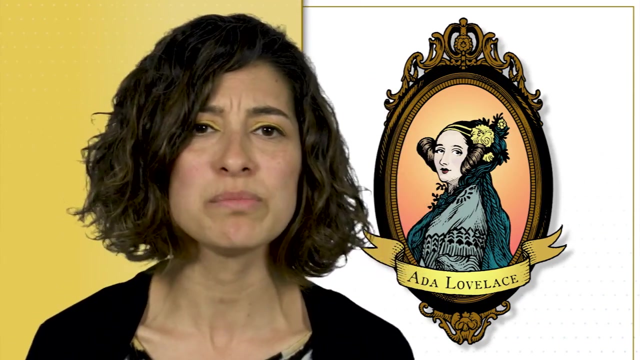 And the first person to come up with such a device was Ada Lovelace, who made the jump from mechanical calculating devices to digital computation. And how does this relate to light switches and to how computers really work, And why am I talking to you about this? 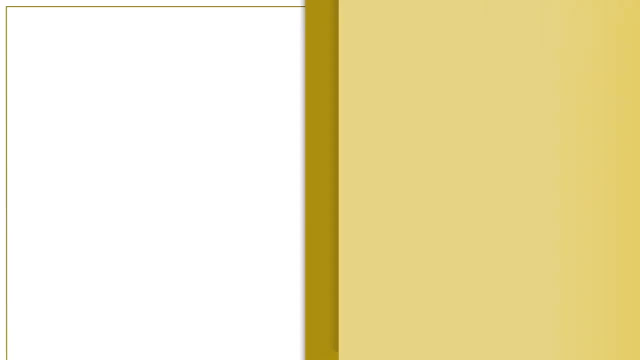 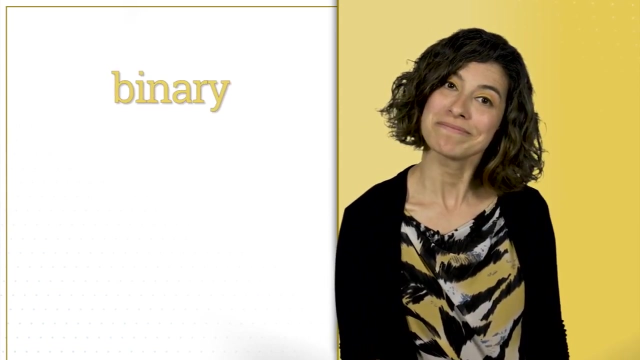 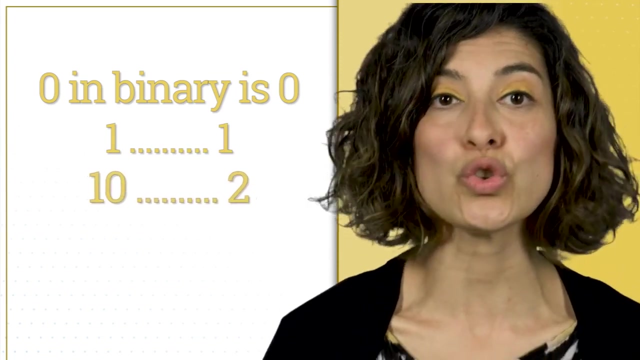 in a mathematics module. Back to the code I mentioned earlier. as you may have realized, it's called binary. Zero in binary is zero, One in binary is one. One. zero in binary is two One, one in binary is three, and so on. 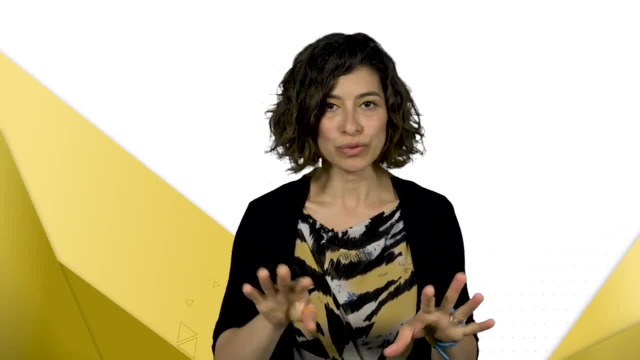 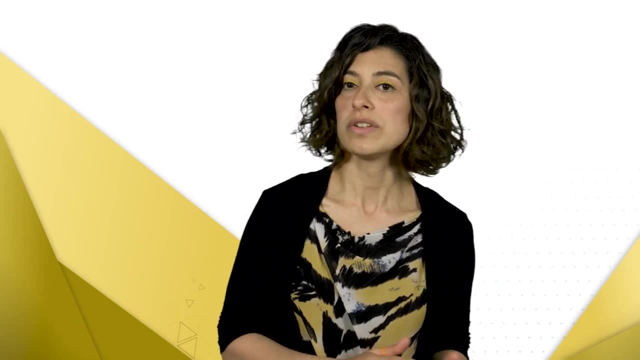 Well, how to make the next numbers. We will study this. in this section We will look at steps to make the conversion of everyday numbers to binary and to other number systems. We will use it in the context of hiding secret messages in science. 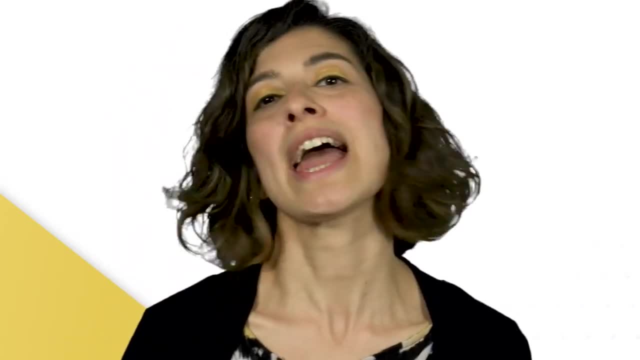 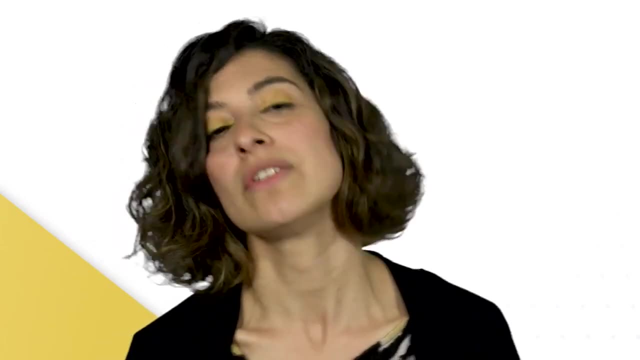 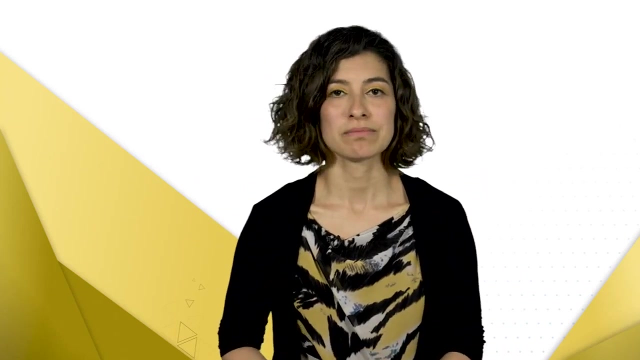 We will use it to hide images and using encryption to guarantee secure exchange of messages. Online banking and other secure websites. use encryption to protect sensitive information. Throughout this topic, bear in mind these two problems: Concealing a message in an image and encryption of secret messages. 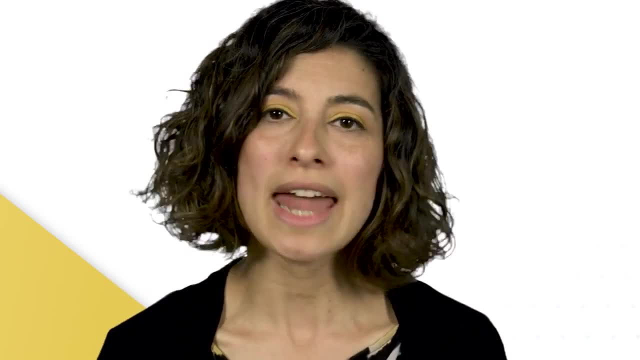 Think of them from the point of view of computer science and how we implement it. think of them from the point of view of computer science and how we implement it. think of them from the point of view of computer science and how we implement it. 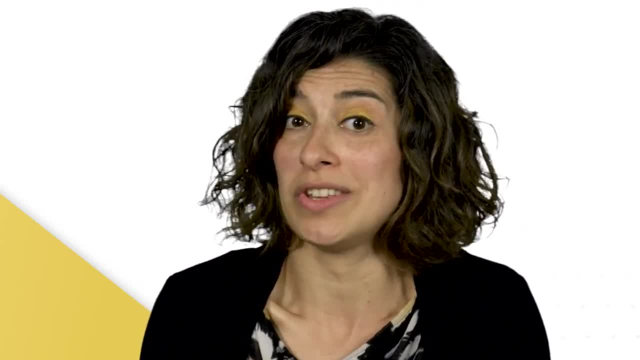 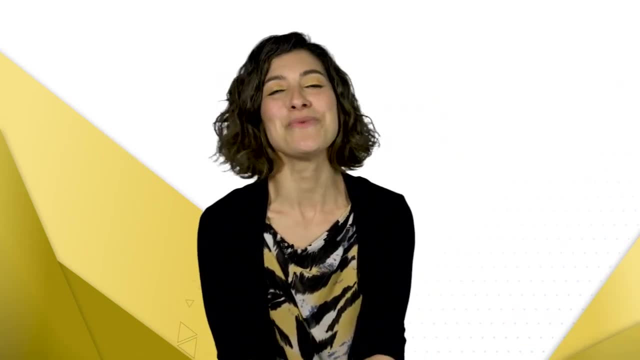 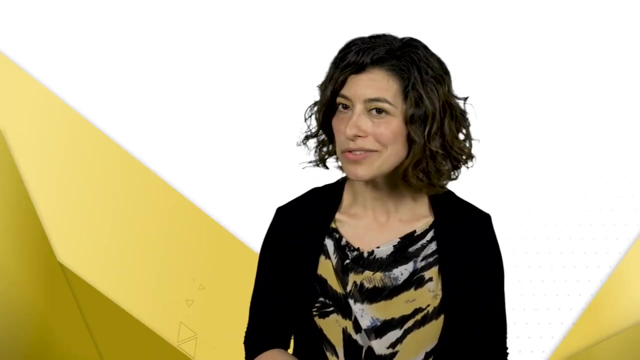 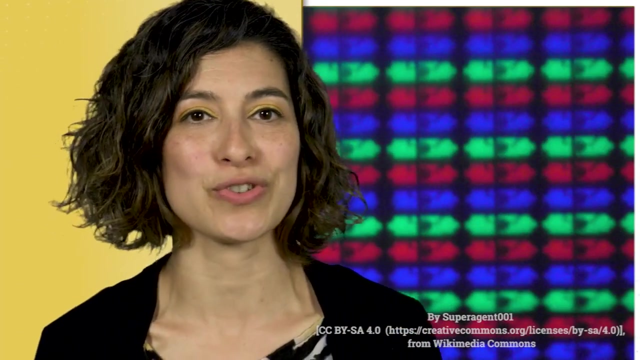 computationally to send messages using the Internet. If you are brand new to computing, panic not. We will prepare you with the tools you need. Let me tell you more about these two problems. Everything is number, and so are pictures. The quality of a picture is usually rated on its resolution. 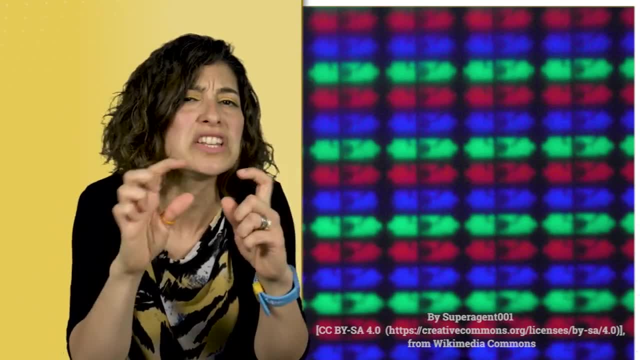 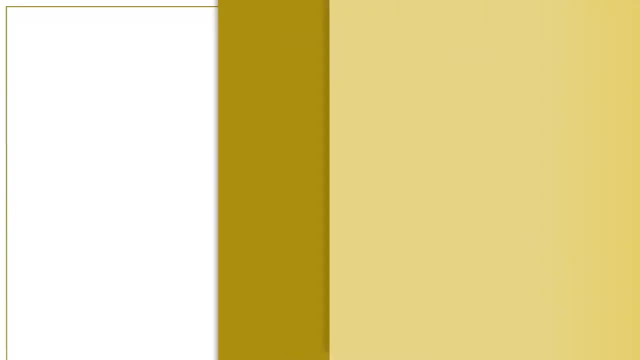 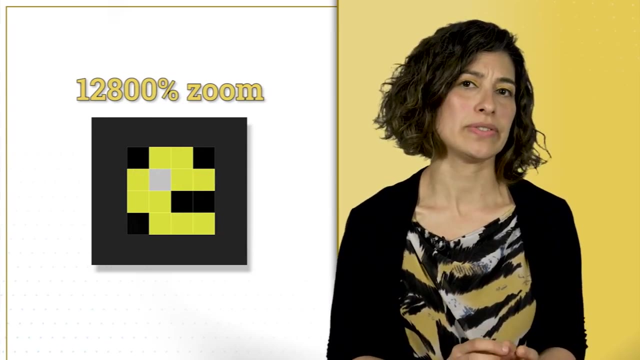 that is the number of pixels, the number of little squares made of one single shade of color that make up the whole picture. A small image like this one already needs 16 pixels, and that means at least 48 numbers to convey the pixel information. 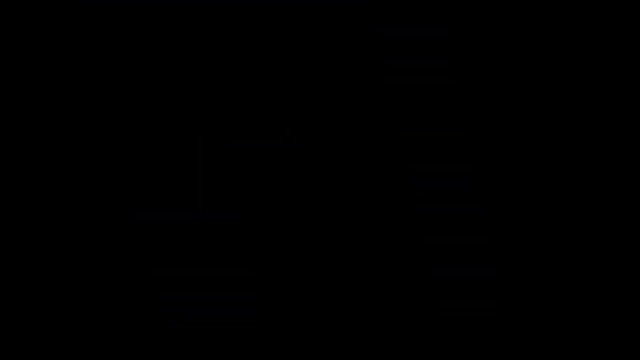 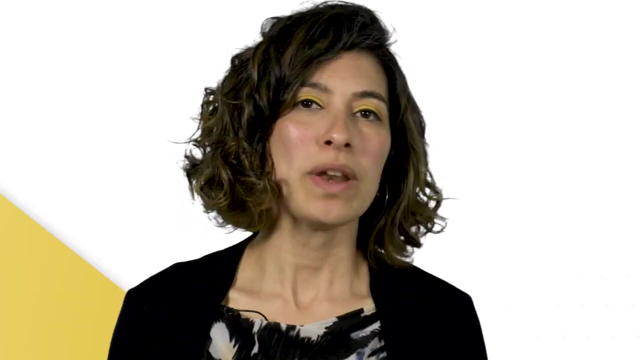 and that means at least 48 numbers to convey the pixel information. Let's look at the numbers that describe the color of a pixel. Let's look at the numbers that describe the color of a pixel. When making a web page, we write HTML instructions. 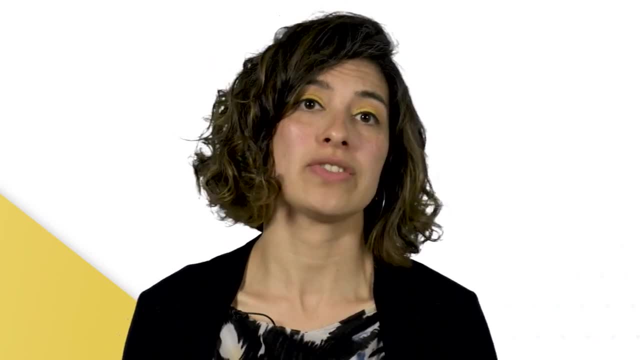 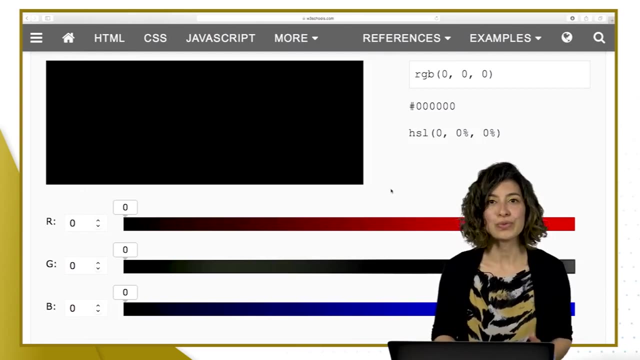 When making a web page, we write HTML instructions to give color information to parts of the page. Let's look at the W3Schools website. I'll show you the tools for color coding. One of them is this one here: the RGB calculator. 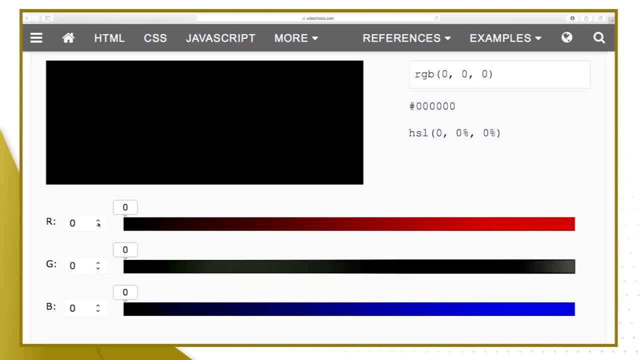 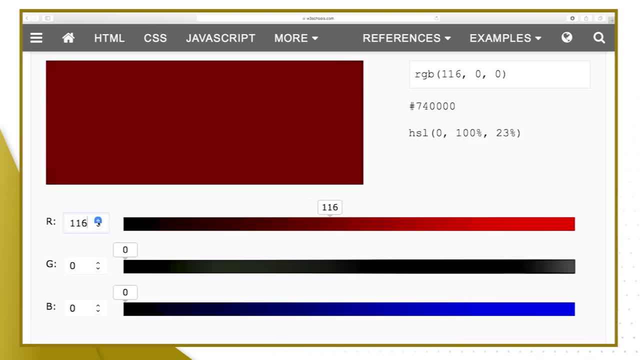 I've got black at the moment, color black And I'm going to go for red. It's not probably the best choice for a whole web page, but anyway. It's not probably the best choice for a whole web page, but anyway. 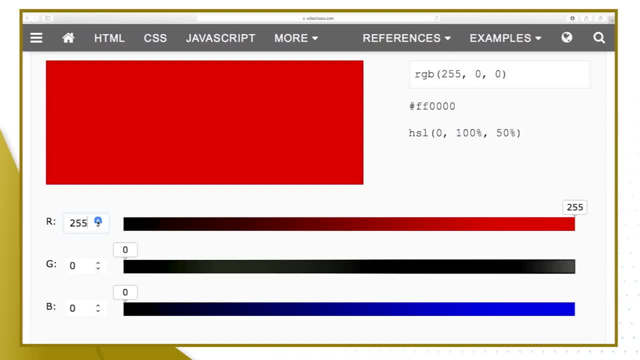 It's not probably the best choice for a whole web page, but anyway, Why not? Why not? So full red, 255 red. So full red, 255 red. And if I want to make the page say yellow, 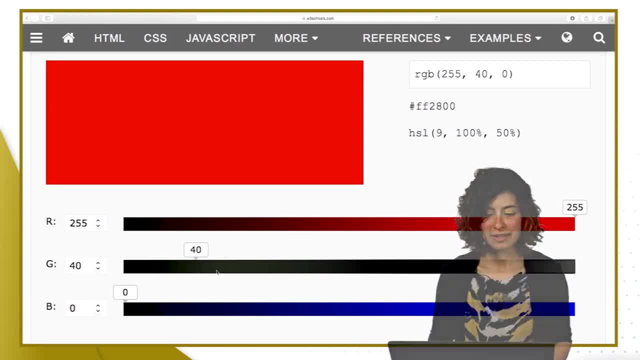 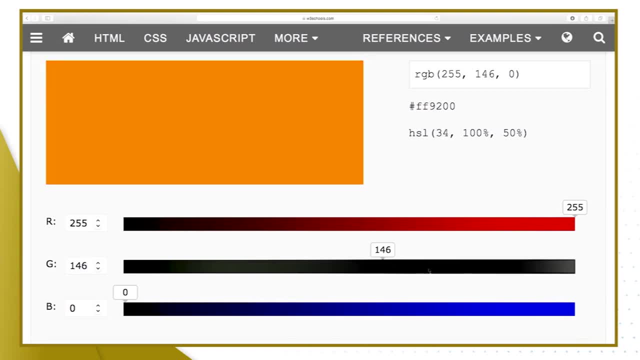 surprisingly, I'll just keep adding green. You see it's turning a little bit orange. That's quite a nice shade. More and more green And yellower- almost the color of my dress, And yellower- almost the color of my dress. 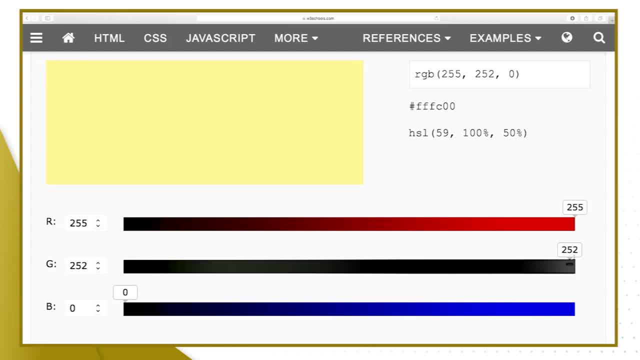 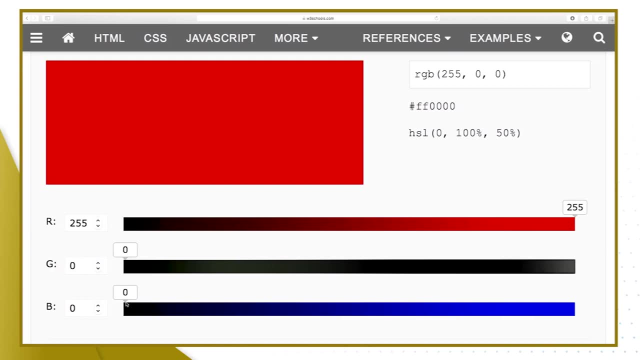 And then top top yellow, And then top top yellow, And then top top yellow. Wow, Okay. so lots of red, lots of green got yellow. But we could instead, let's play with blue. We've got red full on, let's add a bit of blue. What's happening? Oh a shade. 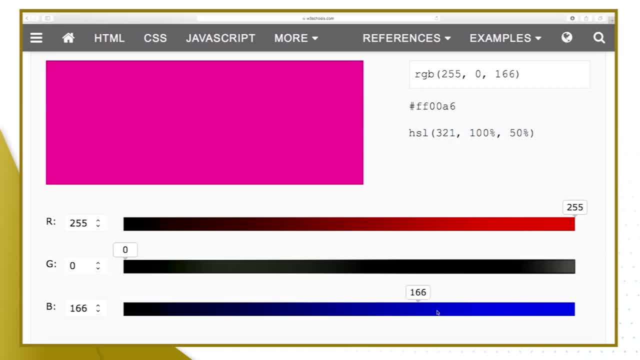 of pink. As we increase that blue, we get closer and closer to magenta. we get a magenta colour Right, And there's other combinations we can have. So here's different shades And as I put more and more of these colours I've got a nice pale pink And all in increasing. 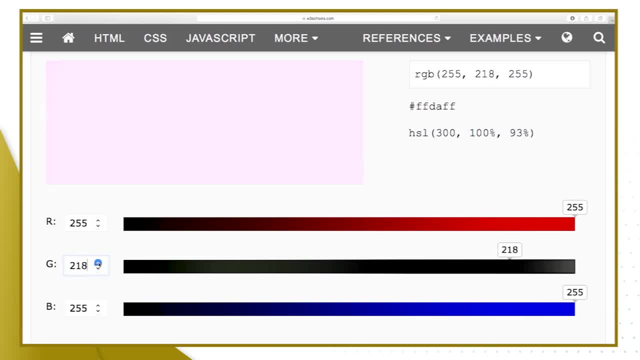 Guess what's happening, Guess what we're going to get. With zero in all colours, we have black. With 255 on each colour, we have blue, The full spectrum of light. So we will tap into these numbers to hide secret messages inside images. We're. 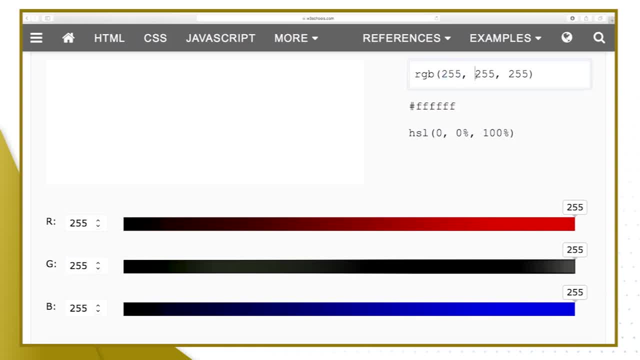 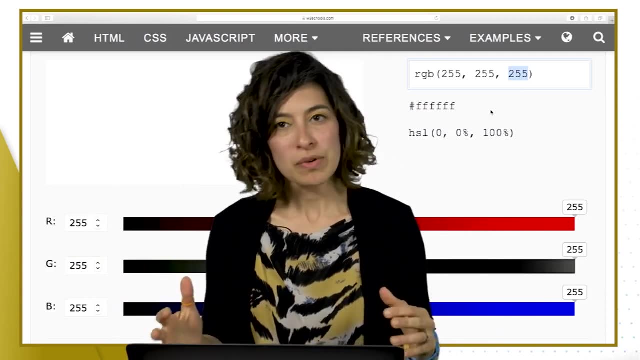 going to tap into the colour of red, the colour of green, the colour of blue to hide the colour of another image. So we're going to use these numbers for the colour values and some of their properties to hide the message. As we go through the lessons, I want you to get thinking on how. 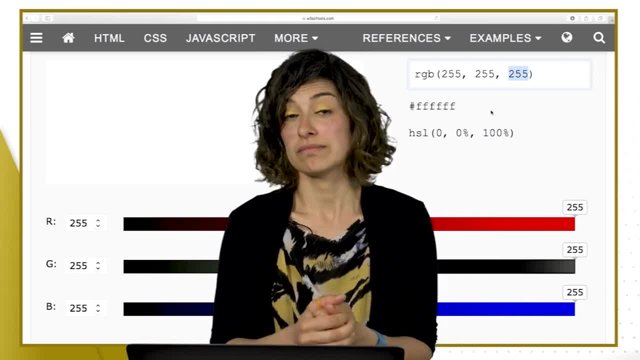 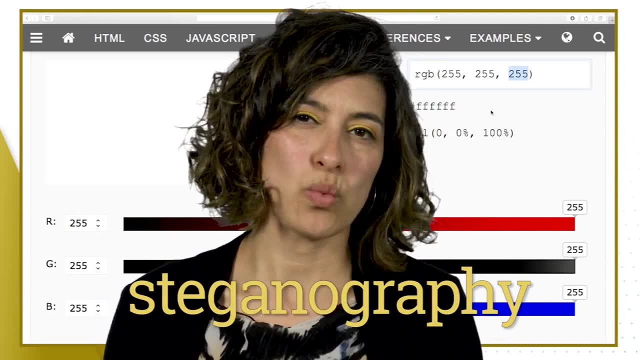 you will use these numbers to hide the message. that could even be another image. This is called steganography: hiding secret information within a public, non-secret image or text or data. I invite you to play with it And remember to hit the like button. Thank you so much for. 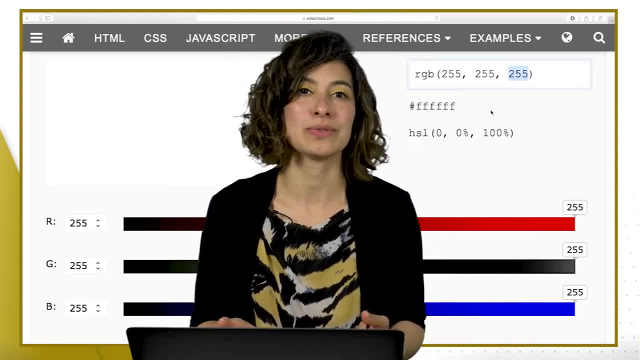 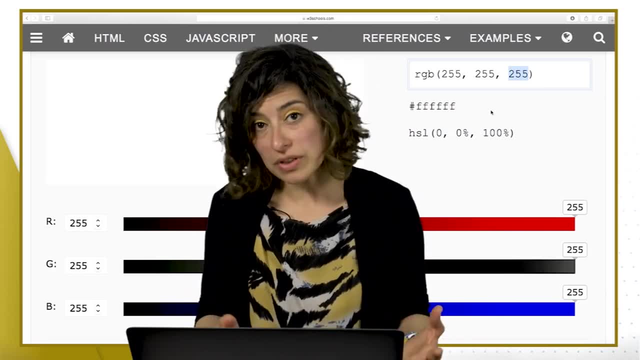 watching. See you next time, Bye, Bye, bye. images and pixel colour values. you can use the W3Schools website as a starting point. You can discuss in the forum how you think the colour codes can be used for steganography. 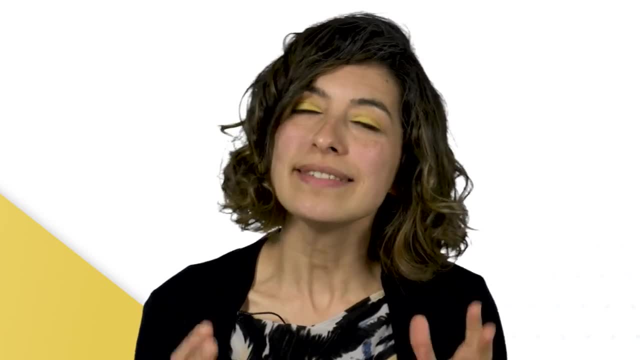 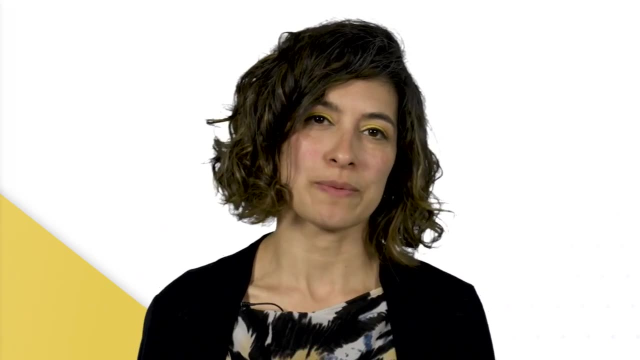 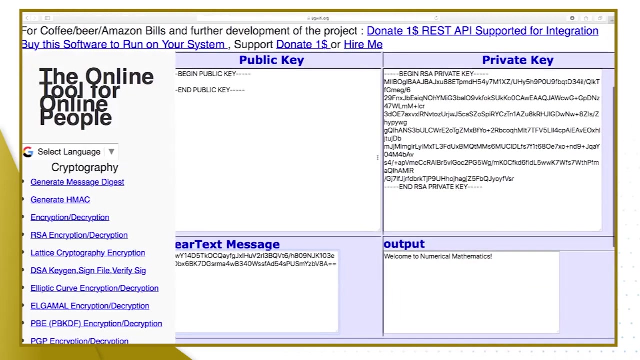 A great step up from concealing is encryption, where the secret message is scrambled so it cannot be read without the key that unscrambles the message. I have a secret message I received which is here in this box, and I have my private. 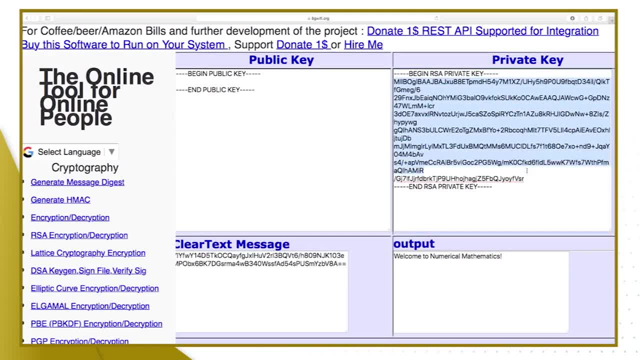 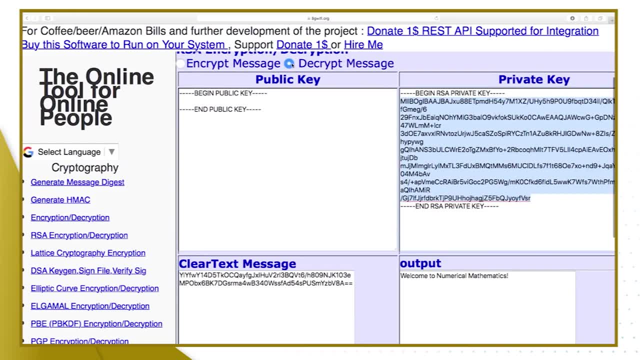 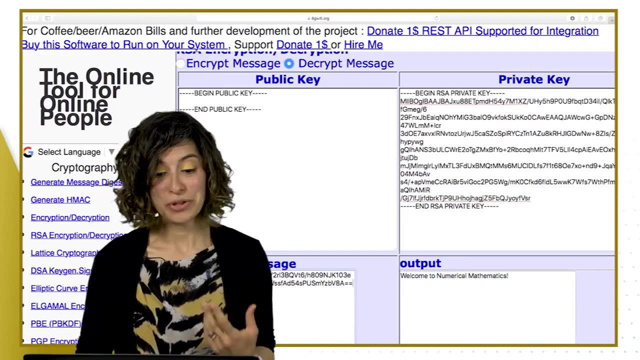 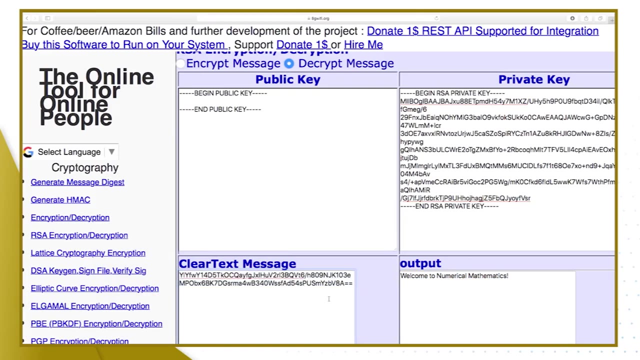 key- this really large one over here- and the output: so the real message that's been decrypted. I press there is actually Welcome to Numerical Mathematics, so it doesn't look anything like the message I received. OK, OK, To encrypt a message I only need a public key, so I don't need that private key at all. 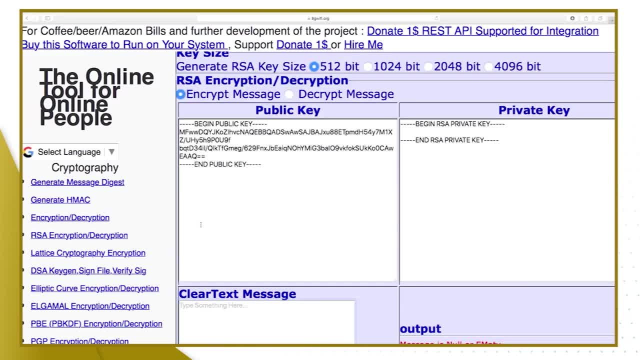 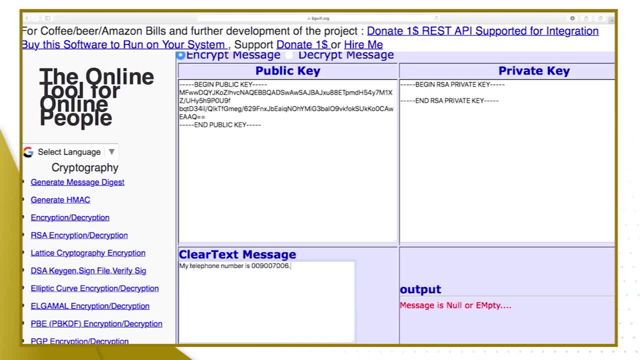 My public key is this: So I've got my public key. I'm going to encrypt a message and the message is: My telephone number is 009 007 006, and on that box there the output. I've got the encrypted. 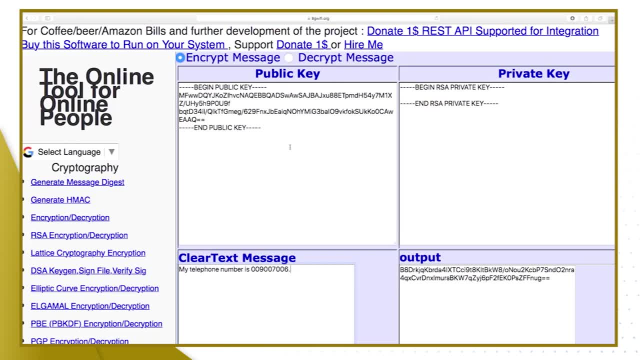 message. So I use the public key to encrypt. here's the output, and if I were to give this to you and you had the private key, you would then read my telephone number. Without the private key, it's not possible to extract the real meaning of the message. 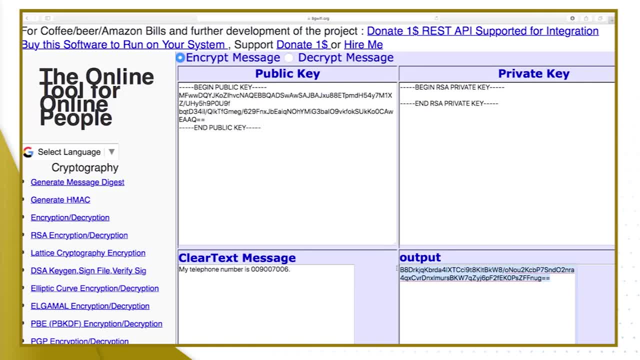 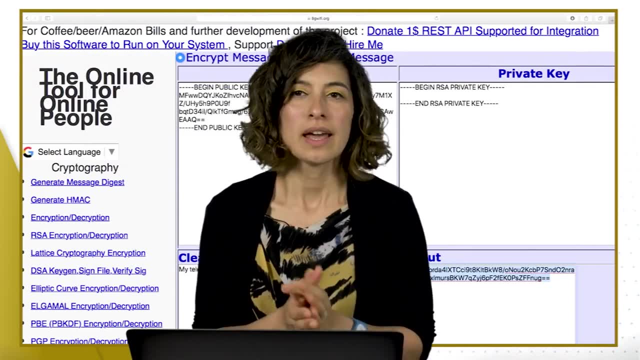 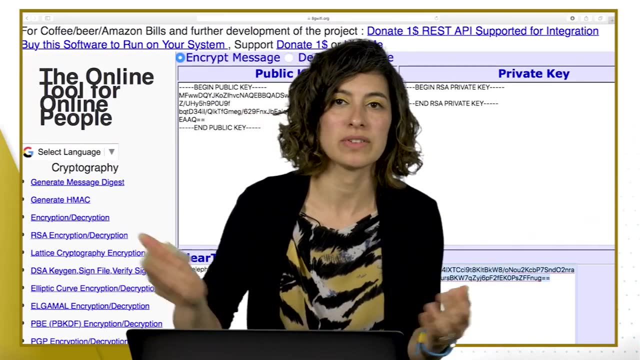 and we're going to look at a simplified version of this method later on. So the point is, you can send me safe messages if you have my public key, And usually that is a huge, huge, huge number that is not easy to factorise, as in finding, 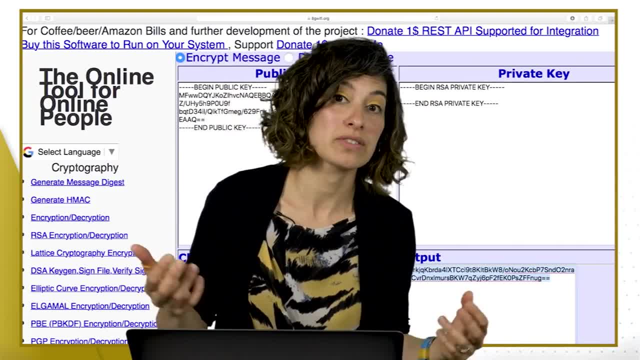 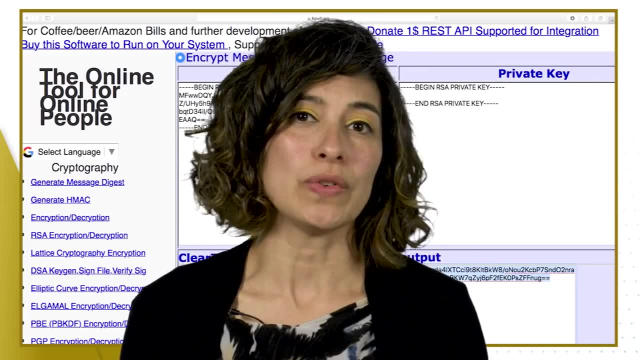 numbers that divide into it, and my private key is a number that factorises in that sort of. You will see later all the details. This method uses as a public key two prime numbers multiplied, two huge, huge prime numbers. 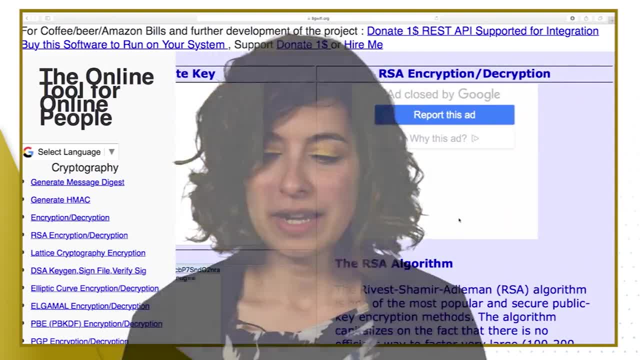 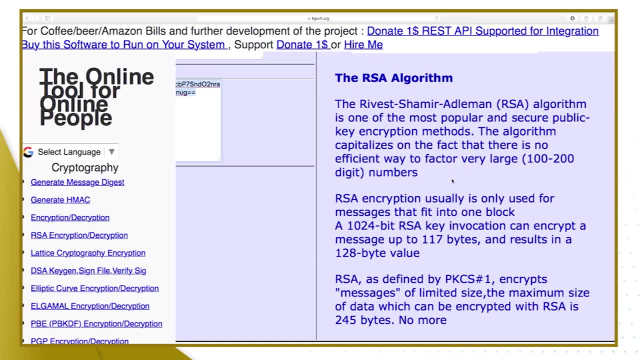 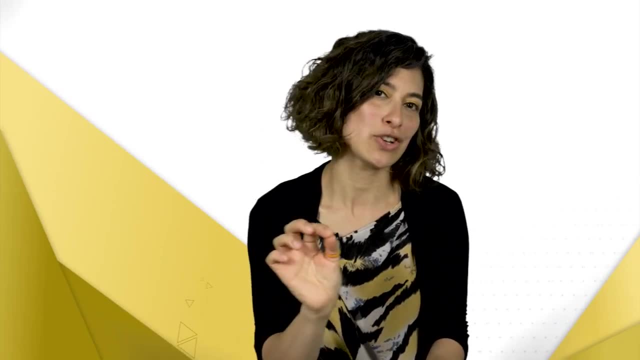 and that gives a huge number And as a reminder Here on the website, it does tell you we're looking at numbers that have around 100-200 digits. The private key will have a connection to one of the primes and with that number I 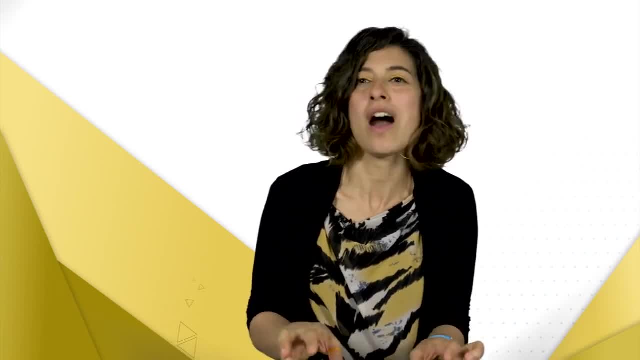 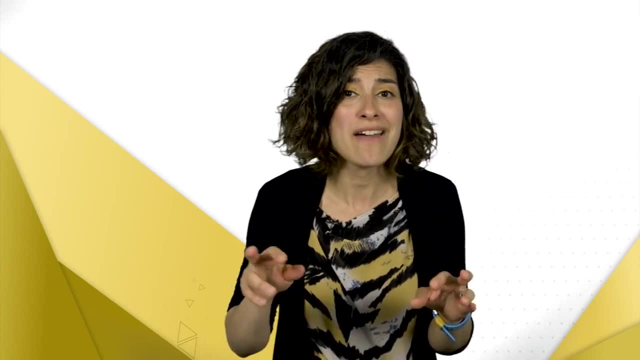 can decipher the message, But it's computationally too hard for someone else to work it out and it may take forever. I mean the forever of everyone's life on this planet. So here's the private key. You can't see it when you're online. 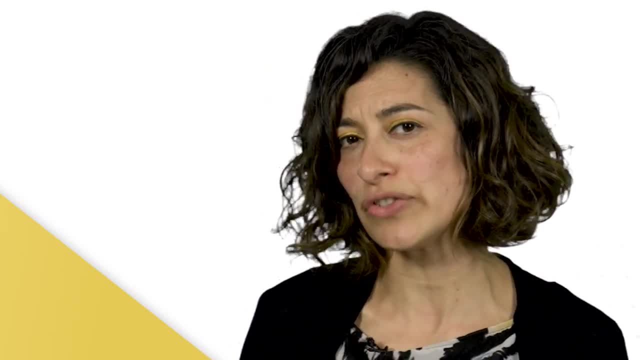 You can't see it when you're in a watchЯB. You can see it when you're in a watchYB. It's the perfect match. But it's a recurring data that can be used any time of the day, But we don't care whether it's around 200,, 400, or even 500 digits. 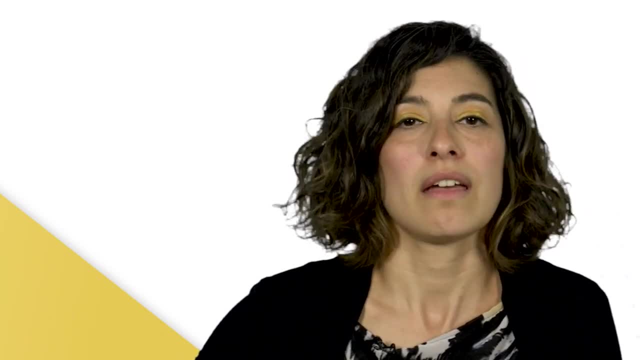 I mean, it depends on the amount of data you have, but it depends on how the public key is being used. So, if you want to be able to use it, the private key is the most important, And if you want to use it when it's at all, or when you want to use it as a personal, 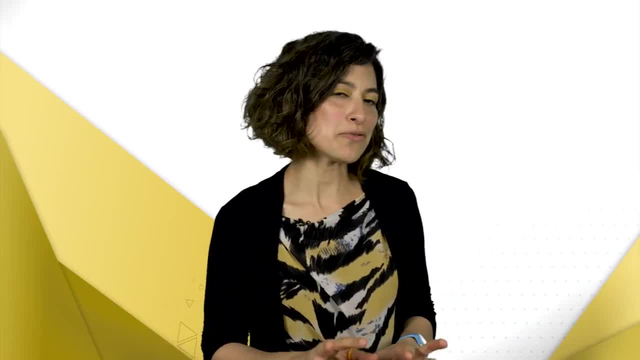 security. the private key is the most important. But what about when you're not using it? You can use it for other things, such as paying for your mobile. cash is different from steganography. In steganography, people see an image or a text. that it's normal. 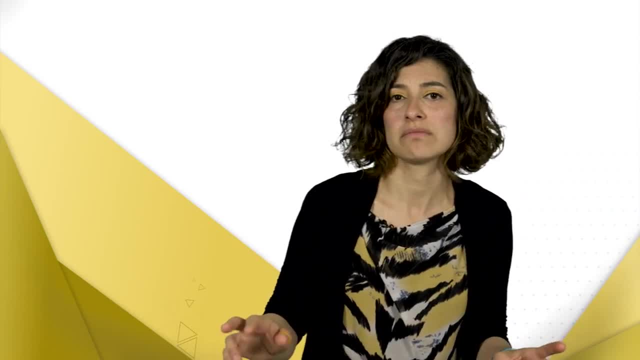 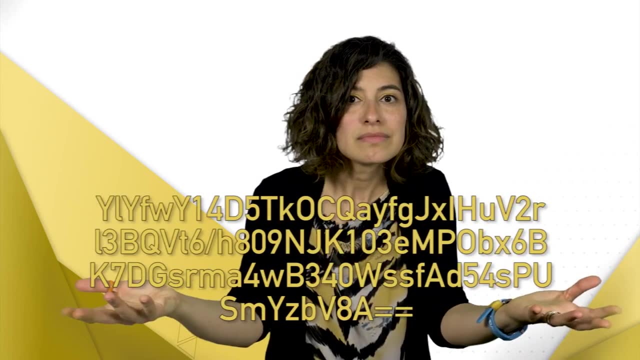 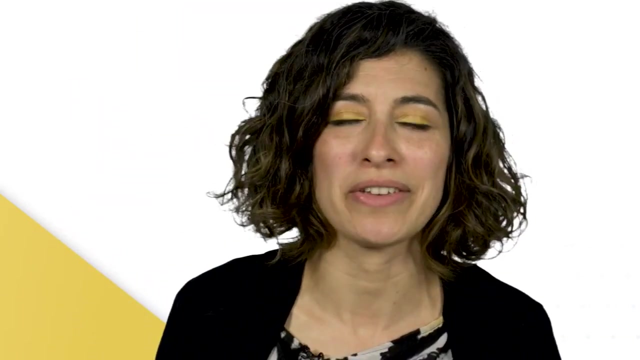 and there's no reason to suspect there is a secret message in it. In encryption, a message may look unreadable, such as Sherlock Holmes was famous for using both- usually some sort of anagram of an encoded message, though. read like a real word. But let's leave Sherlock. 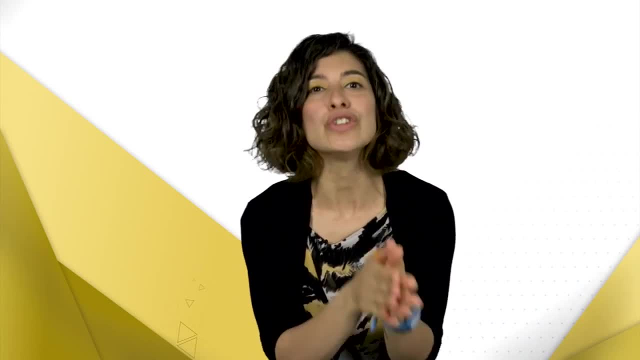 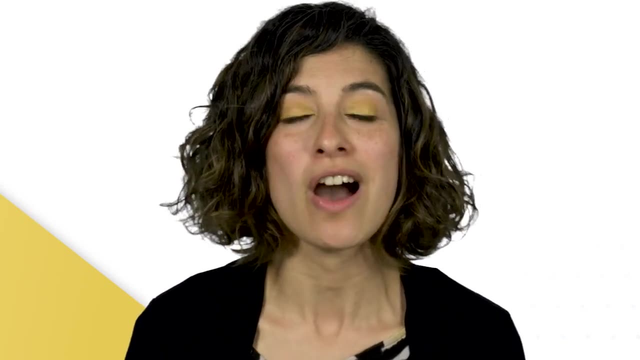 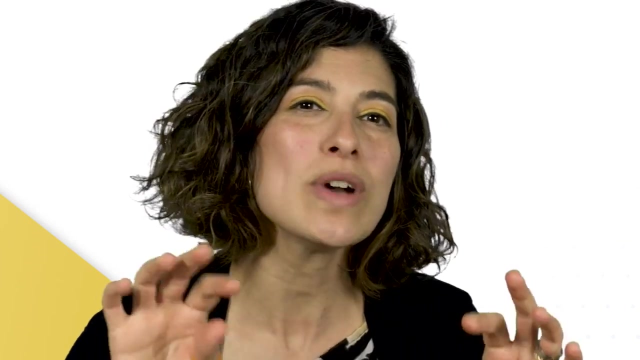 in the books, shall we? The information is converted into a code. The most secure system in classic computing relies on properties of prime numbers, specifically on how hard it is to find prime numbers that divide into a given number if this number is very large. 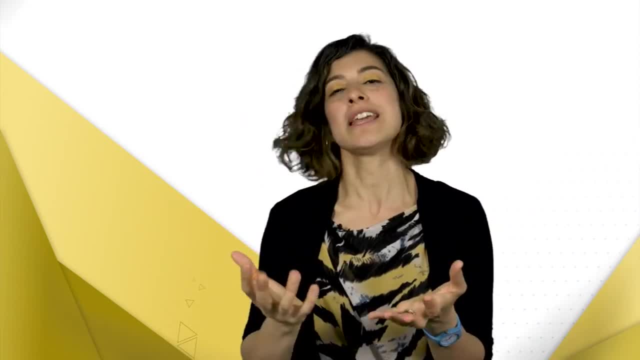 This means that finding the correct key to unscramble the encryption system in a timely fashion is extremely unlikely. Doing it in a way that makes it difficult to find the correct key to unscramble the encryption system in a timely fashion is extremely unlikely. 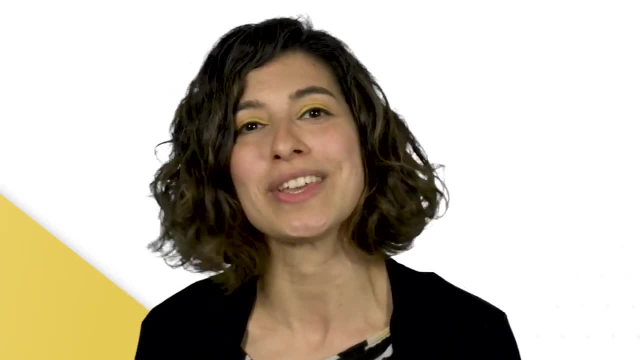 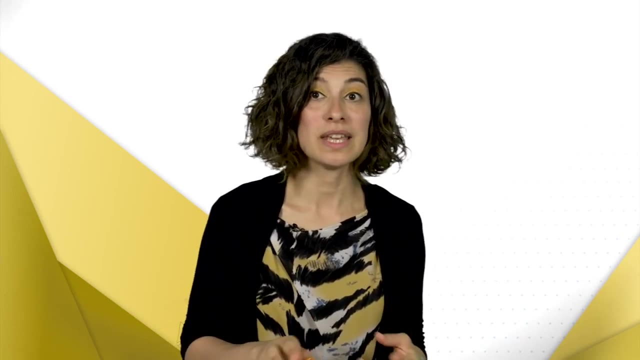 Doing it in a way that makes it difficult to find the correct key to unscramble the encryption system in a timely fashion is extremely unlikely. Doing it in a systematic manner is impossible using classic computers. We will ease your knowledge of working with integers, in particular prime numbers. these will be key for modular arithmetic and encryption. 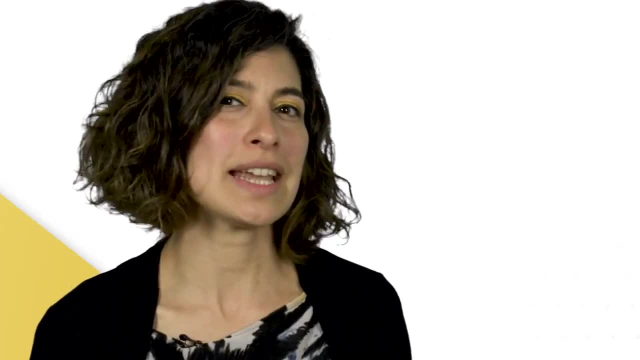 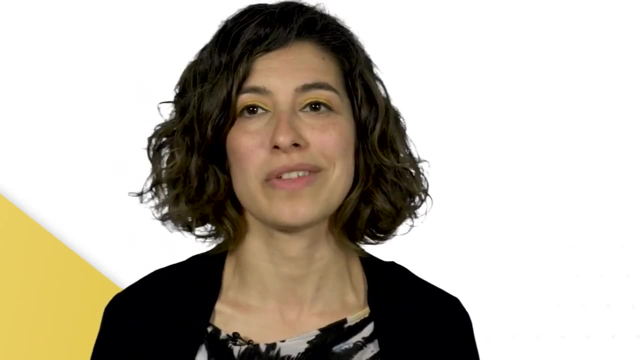 as well as decimals and fractions. Every technique you learn can be systematised and you will be invited to write informal algorithms for all of them If you want to take it further. always bear in mind implementing such algorithms in a programming environment. 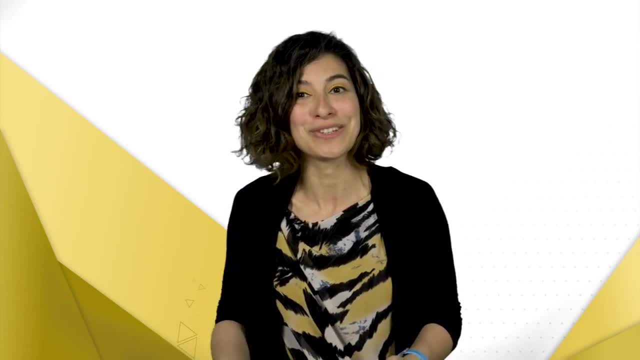 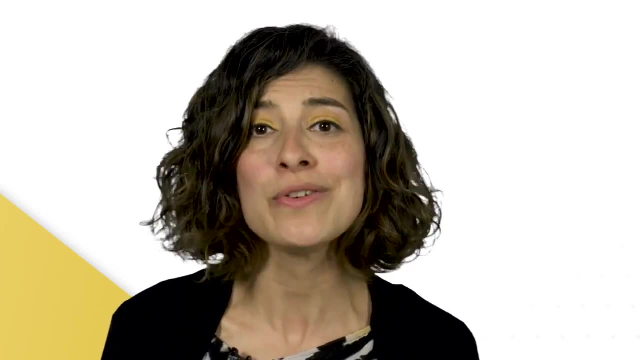 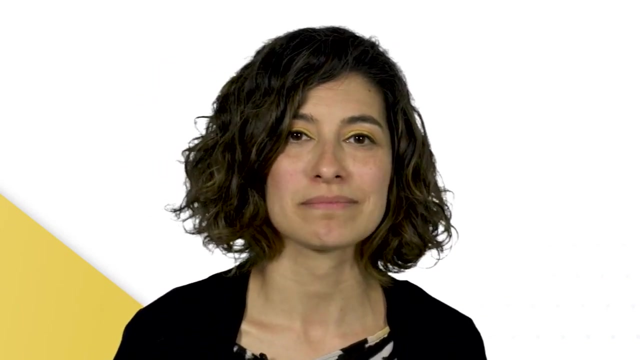 You will not be required to use the programming language you are learning or use it as an opportunity to learn one. Programming is outside the scope of this module, but the purpose of this topic is to prepare you for when you use number basis and modular arithmetic in computing. 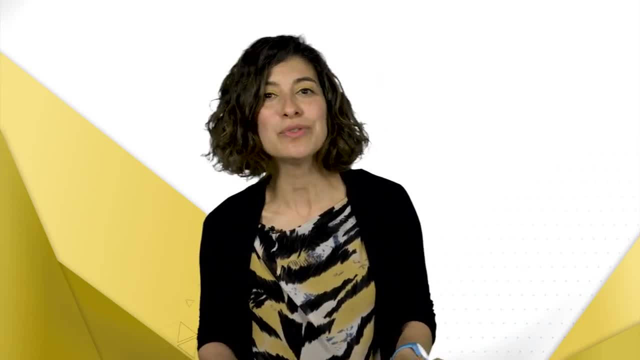 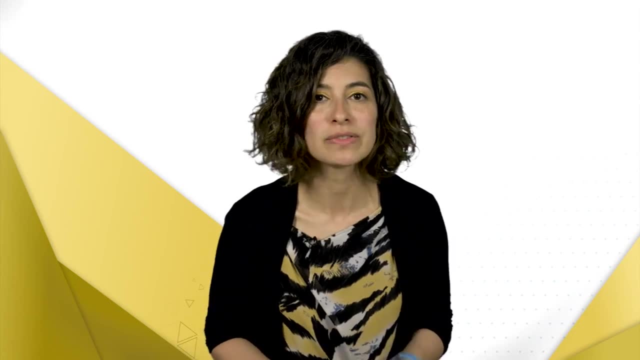 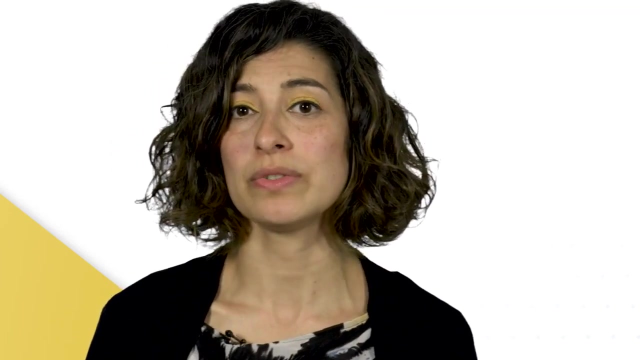 In these first two weeks- topic 1,- you will aim to build the mathematical skills to tackle the following problems: Steganography using images, Encrypting using images using prime numbers. You will implement a simple instance of these problems using the tools in our platform. Don't worry if you are absolutely brand new to 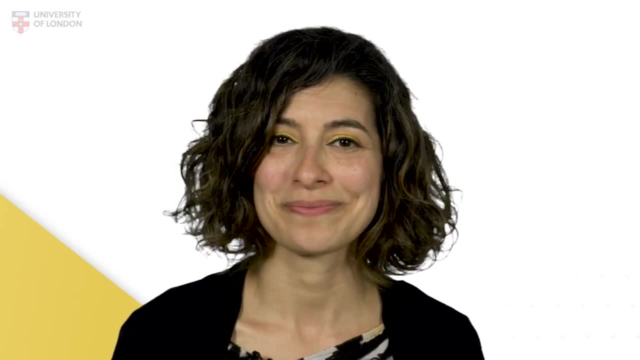 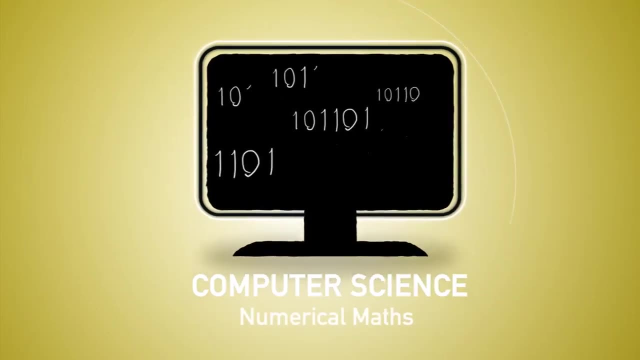 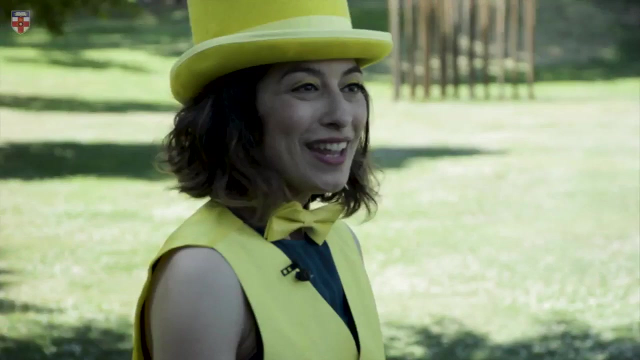 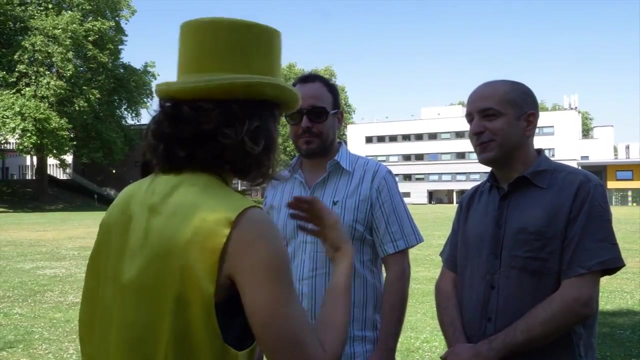 computing. we have design tools to support you. Good morning, good morning, good morning. Oh, lovely to meet you. You are Nancy, Jack Peter And I'm Sarah. I am a mind reader. I'm going to read your mind, but I will ask for your. 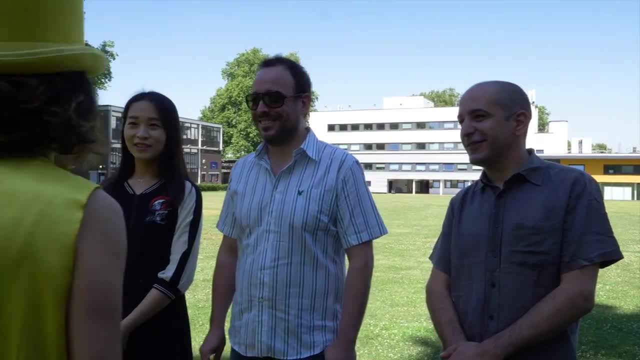 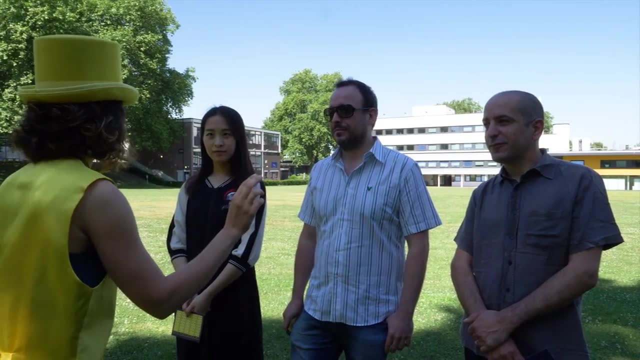 permission, I'll go. a nod of consent. Good, I try to be polite, I try very hard, So I need you to think very hard of the day of your birthday. Just the date, Forget the year and the month, which is a day between 1 and. 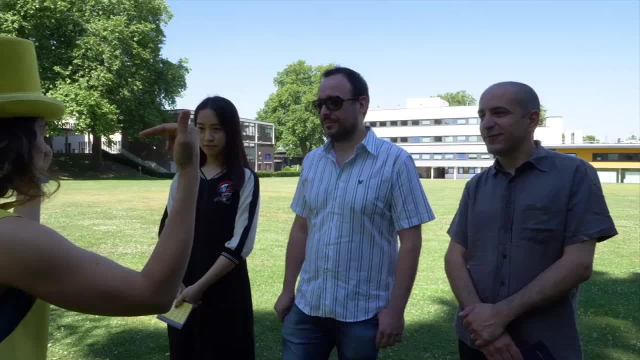 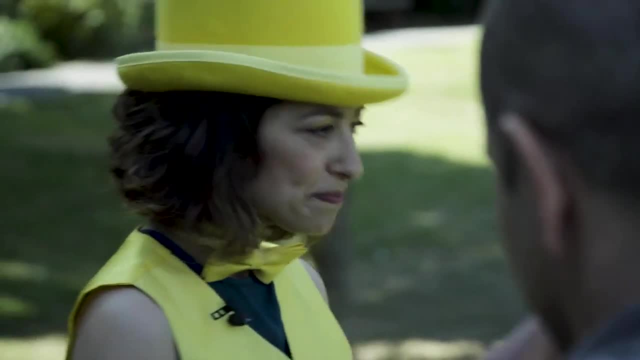 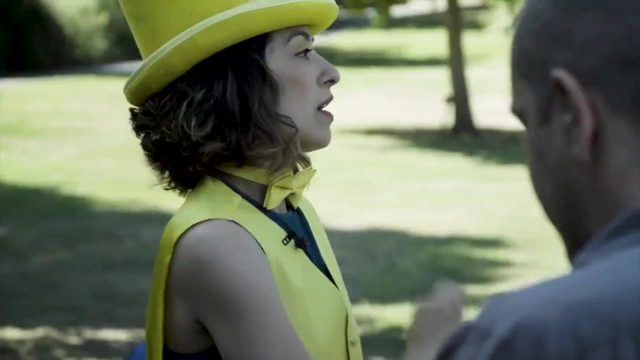 31,. right Now, beam it to me. You're too good, I'm seeing too many numbers. Let's narrow it down. You've got a magic card in your hand and that magic card has boxes that says card 4,, card 3,, da-da-da-da, all to card zero. Scan those cards. 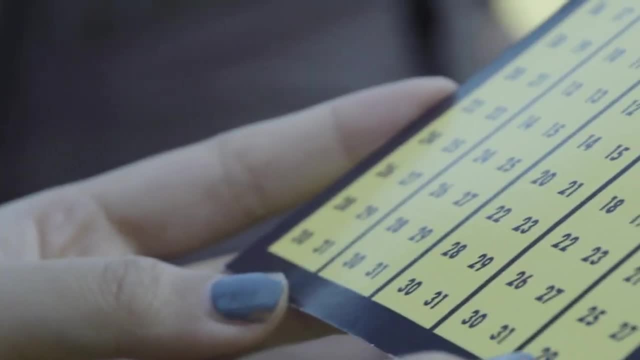 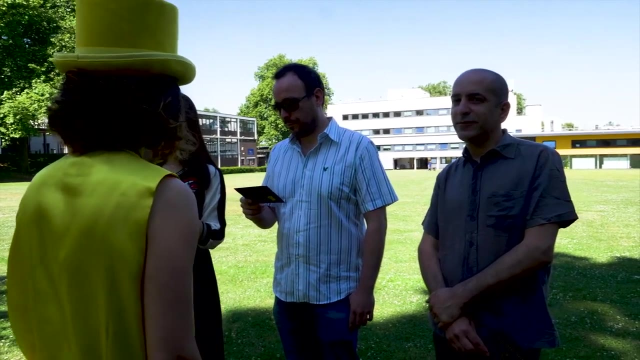 Okay, Okay, And tell me all the cards that have your date. Okay, If there's more than one, I need to know all of them And I will ask you in order- and try very hard not to tell me the date of your birthday, just the card numbers. Okay, You ready. 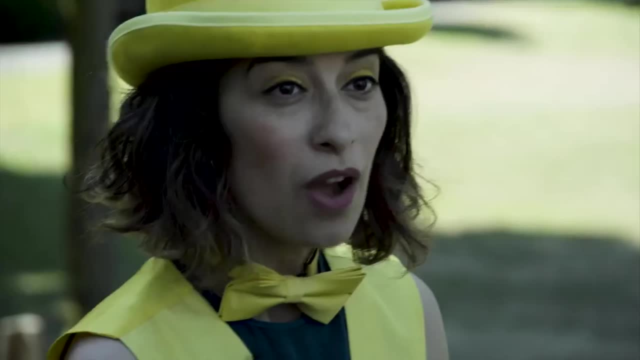 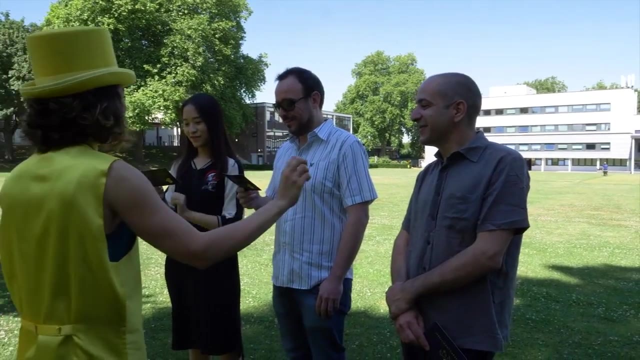 Mm-hmm, Lovely Peter. One and zero, Only one and zero, Peter. Yes, I can feel some vibration in my hat. No, Okay, That's a lovely, lovely number, prime number. Let me hang on to that thought, Jack. 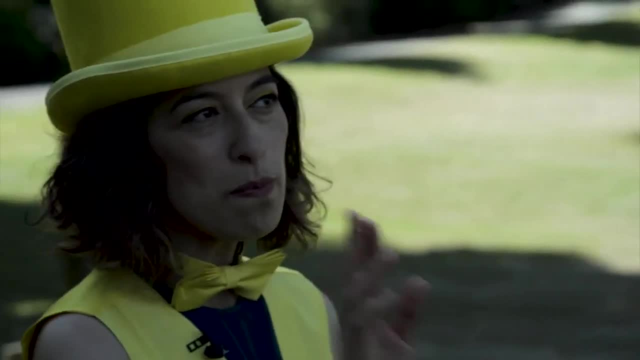 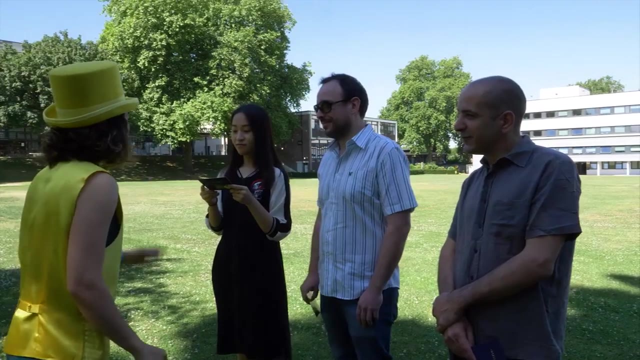 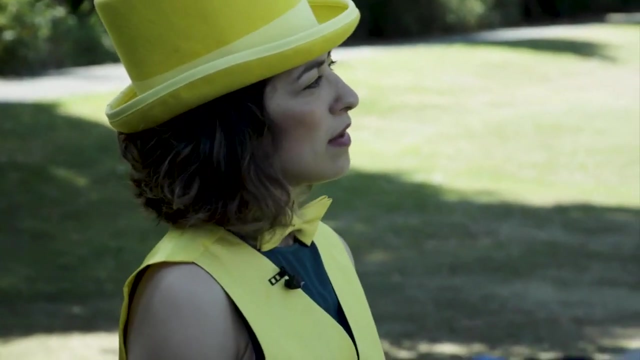 Zero two and four. Zero two and four. So you're missing card one and three on purpose. Yeah, Yeah, And yours, Nancy, Zero one and a three. Zero one and a three. So we've got prime numbers. We got to number three, Peter is. 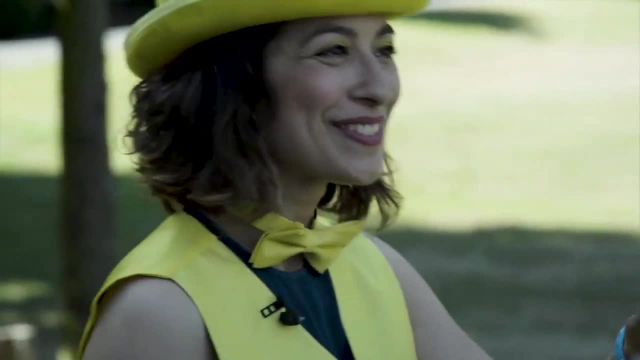 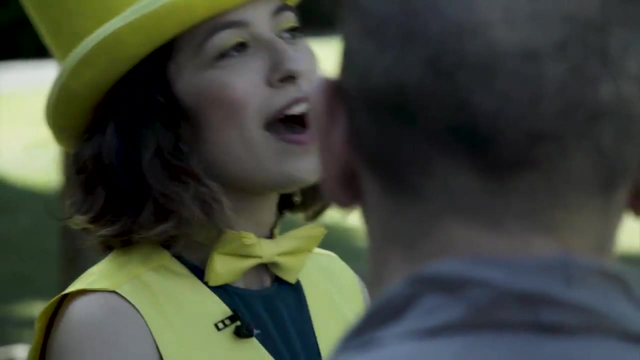 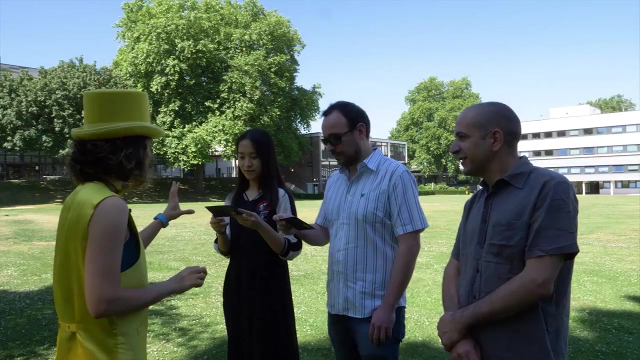 on the third Correct, Jack, tell me again what were the card numbers? The card numbers are zero, two and four. Okay, Exactly, zero, two and four. ah ah, ah, we got multiple three, but a multiple seven is 21, is that right? yes, and yours is prime number 11, is that right? 11, yes, thank you. 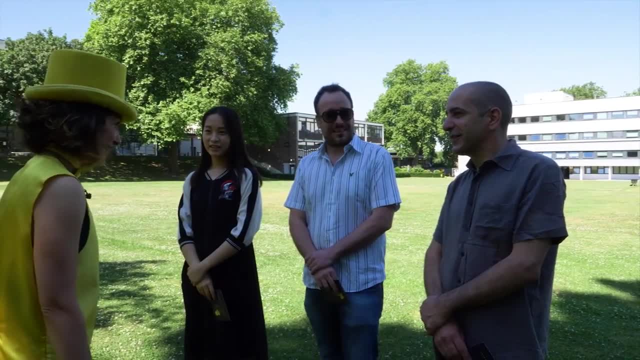 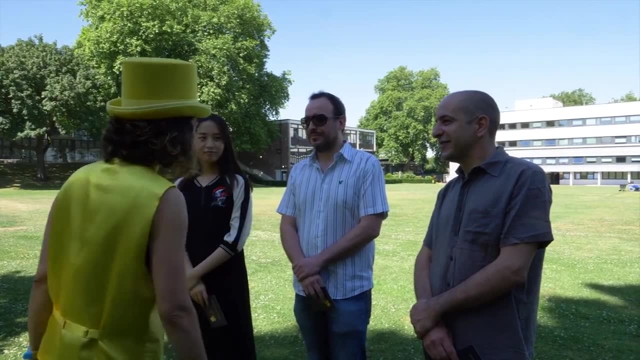 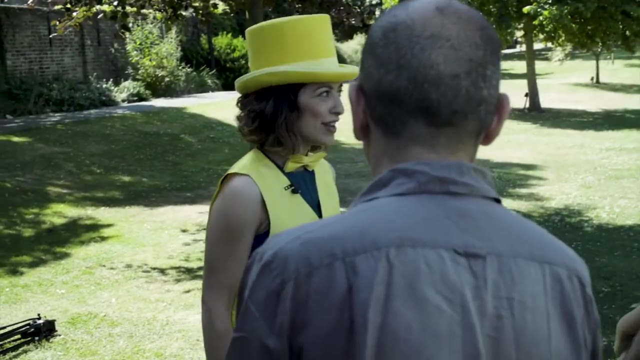 very much. now, how did I read your mind? did I really do it as in? did you actually beam your number into my mind? and you know my hat did? is his trick? or we're University here and and I'm a maths lecturer, or did I use some? 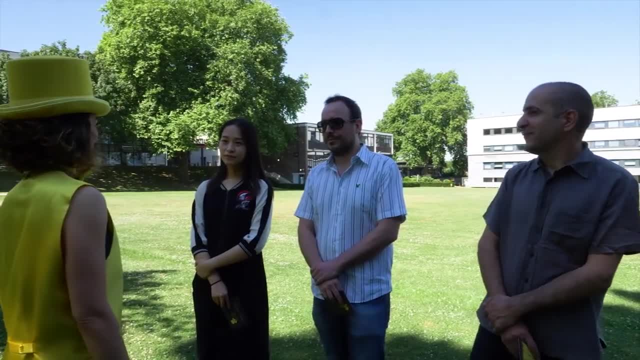 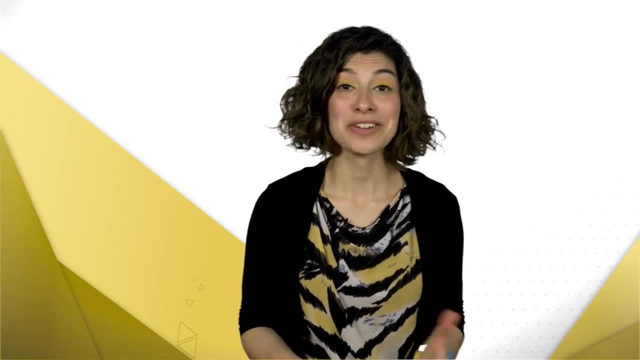 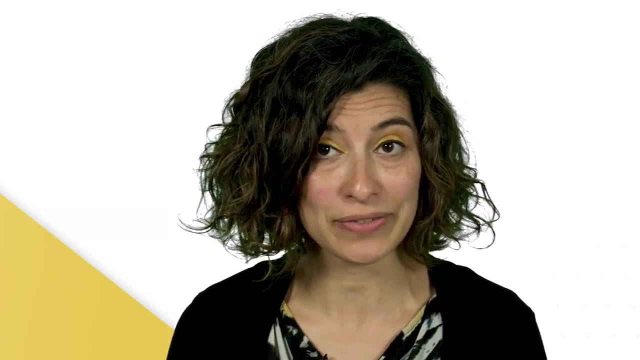 mathematics or science to do this. what do you think? how did I read their minds? actually, I made the audience give me their birthday in code, a code made of card numbers, and I used maths to decode it. take a moment to examine the magic mind reading cards closely. 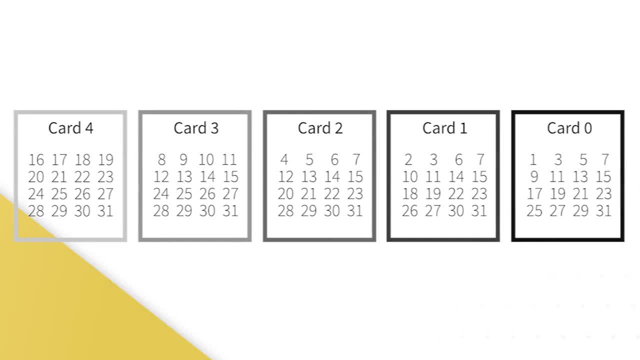 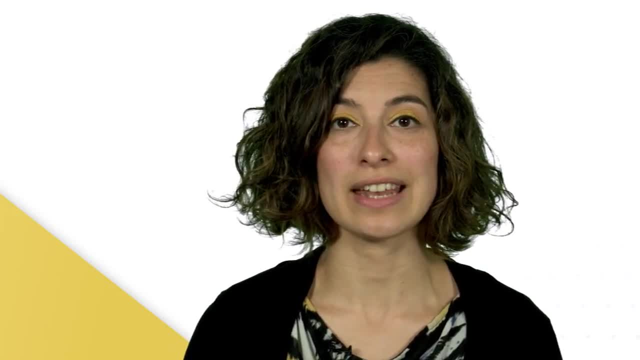 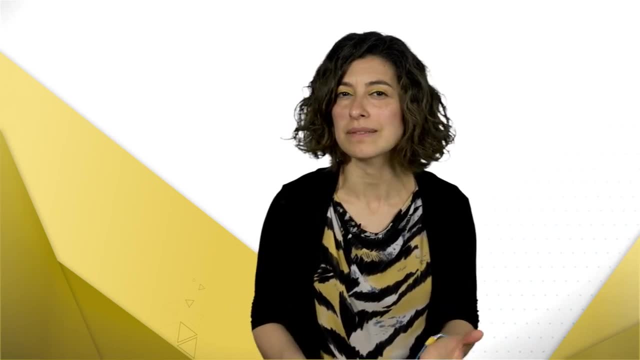 later. you can use the discussion forum at any stage to discuss your thoughts or even investigate some patterns together, not that all the cards have exactly the same number of dates on them. sixteen, why sixteen? and why did I number the cards from zero to four instead ofCome with us and read them? 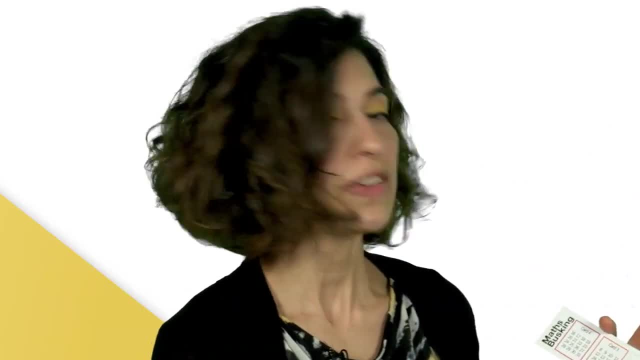 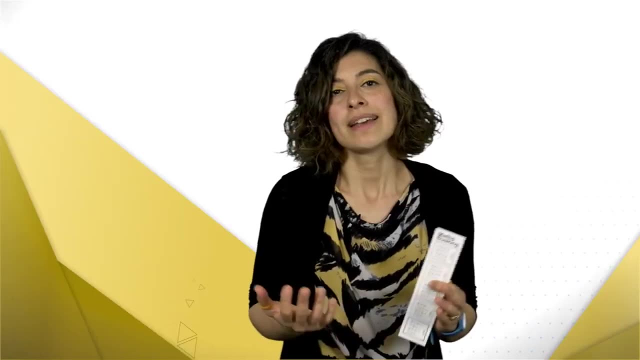 after understood everything, look around you, look around you hear the disc is mushroom. don't call others. one can everywhere elope with the calculation choice instead of 1 to 5.. Notice that some cards have consecutive numbers in them. But what is the pattern? And does this matter at all? It doesn't give you the method I used to. 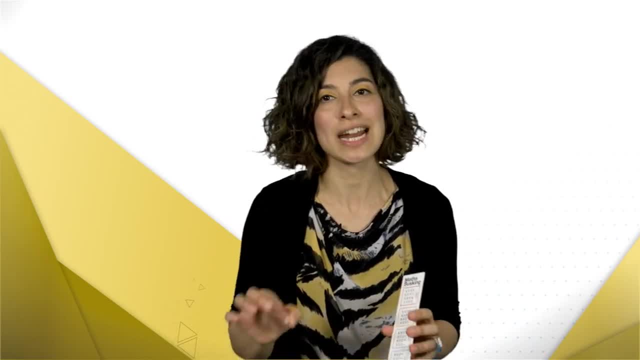 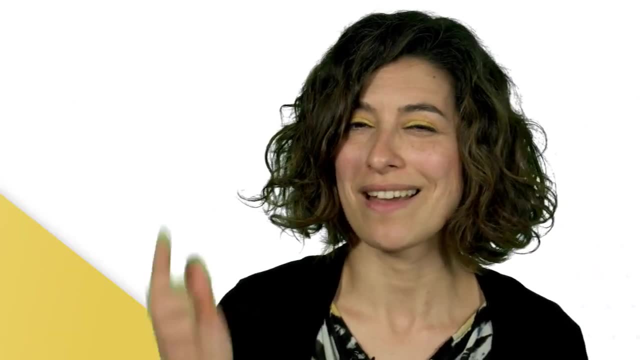 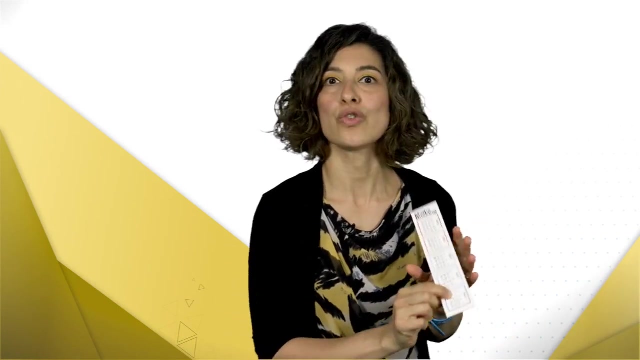 uncover Alvin and his birthdays. but if you study these characteristics, you will gain further knowledge and understanding of the system behind it. But try this, Read my mind. I'm thinking of the date that is on card 4, on card 3 and on card 0- only, Of course. 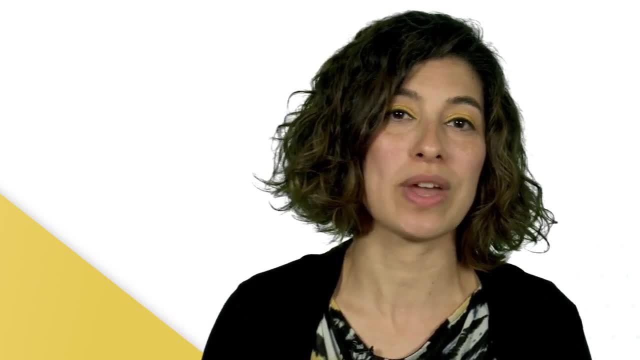 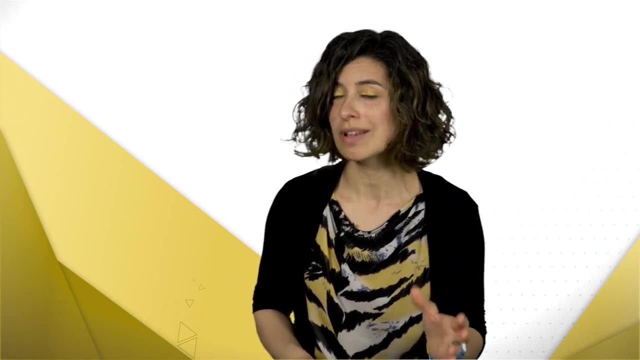 you can look at all possible combinations, but again, that will not give you any insight to the system behind it. It will just get you an answer. If you try to understand what is going on, you will crack the code. Now I'll guide you through the mind-reading. 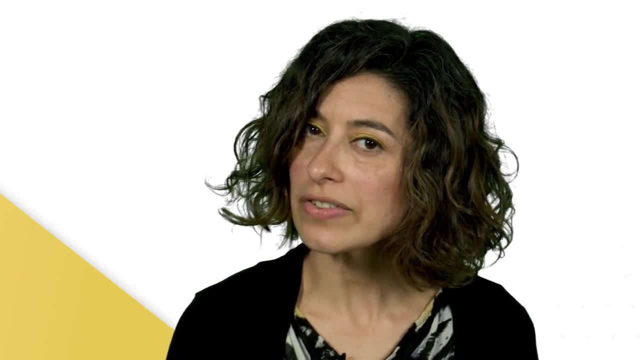 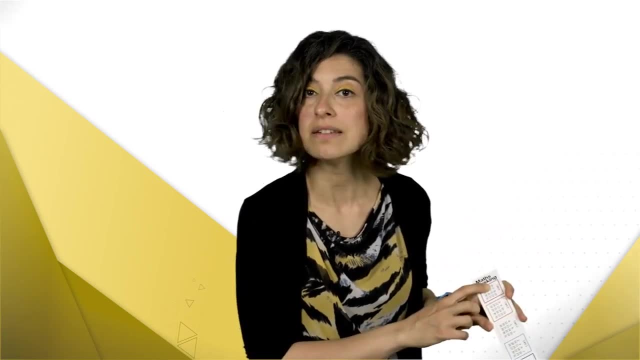 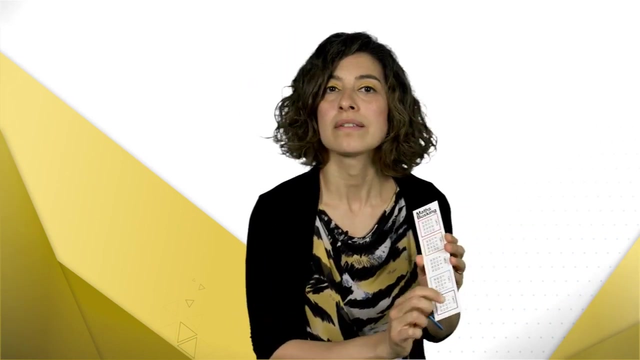 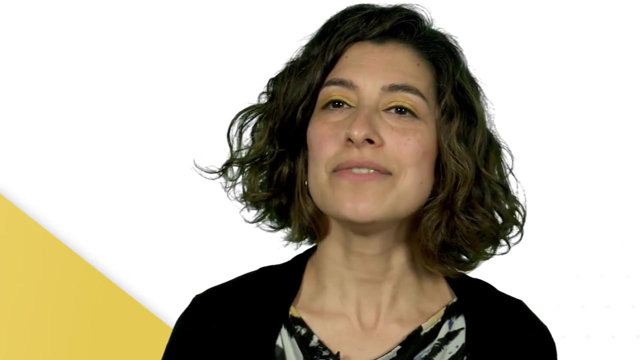 process. Note down the first number that appears on each of the selected cards. The first number listed in card 4 is 16.. The first on card 3 is 8.. And on card 0, it's 1.. But how can we use the numbers 16,, 8 and 1 to make my date? Let's leave this question. 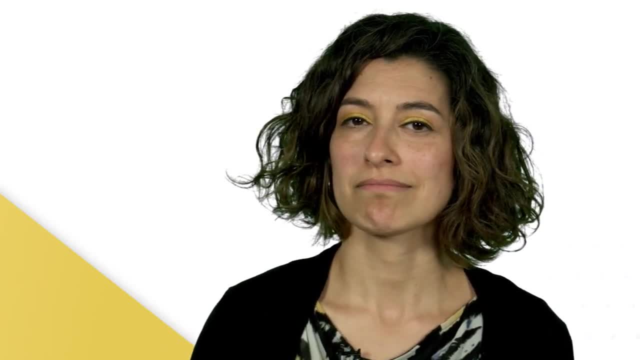 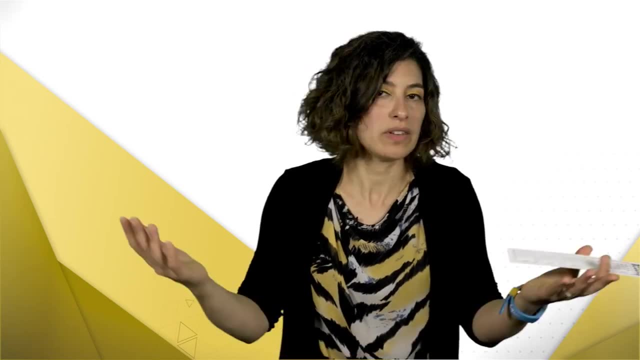 for a bit, and we'll come back to it later. Let's try this approach with the number you select. Write your selected number. It's a number between 1 and 32.. And then you write the number you select. And then you write the number. 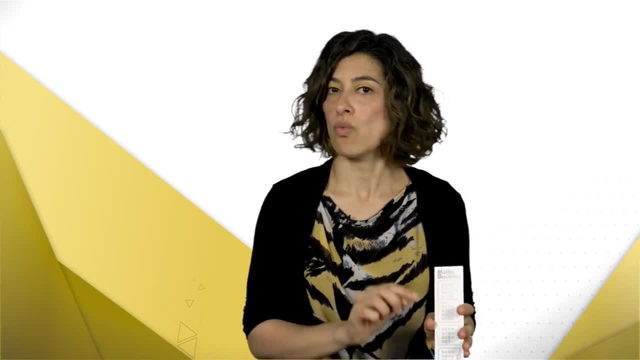 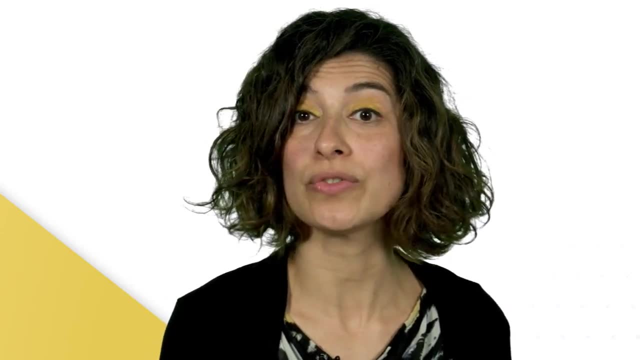 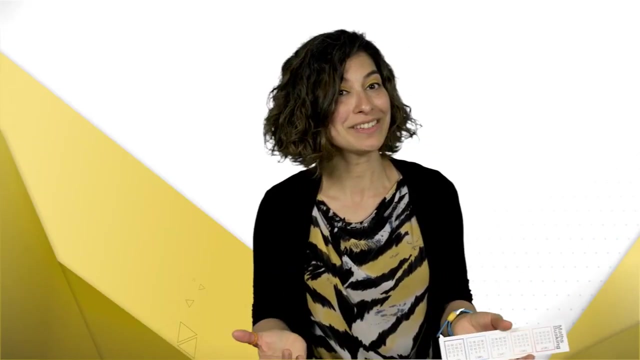 within 31.. And note down all the cards where it features. I mean all of them. Write down the first number featuring on each of those cards. Compare the date and those special numbers. Any thoughts, Any ideas? Feel free to pause the video now. 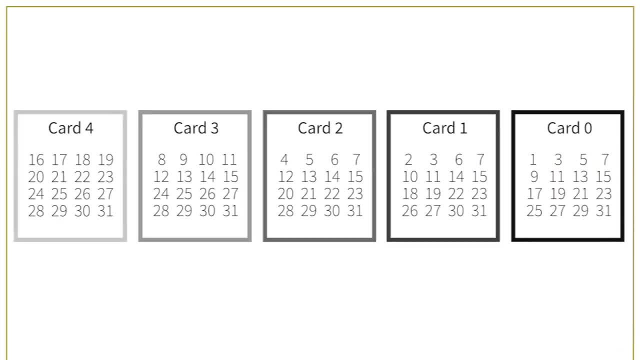 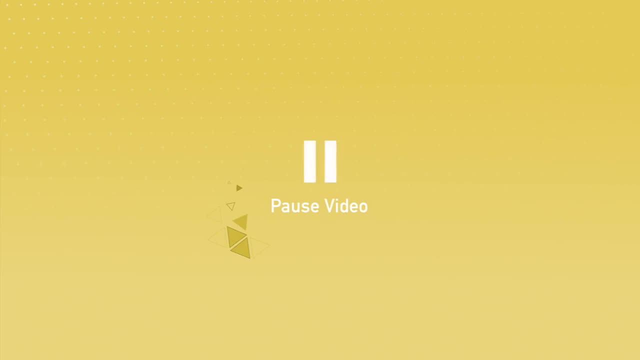 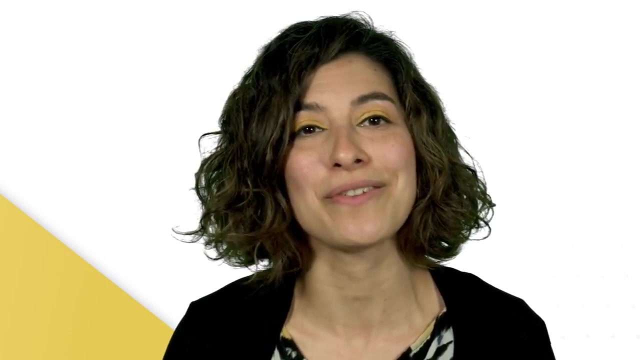 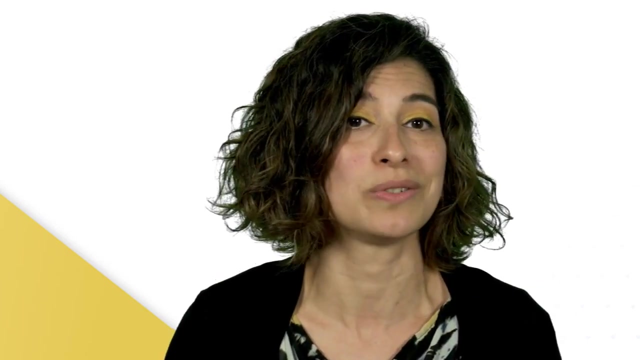 and work through some examples until you crack it. I don't want to rob you of the delight of discovery. In fact, anything you discover becomes a memory, with an emotion and with many more dimensions and connections than something you read or are told. So, throughout this course, any investment you put into understanding and discovering, 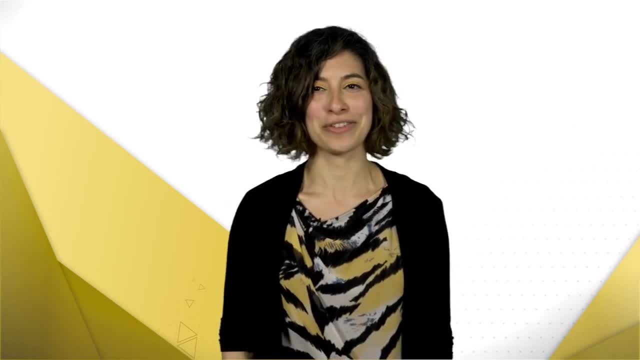 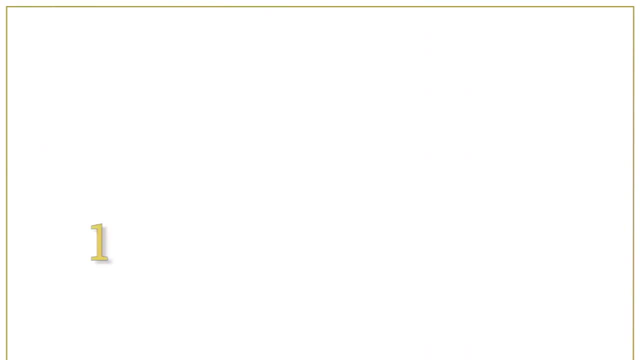 will pay off, especially if you experience a bit of healthy struggle. OK then, so back to my example. Sixteen plus eight plus one makes twenty-five. and let's check that twenty-five is in exactly those cards and no other. Could it be just coincidence? 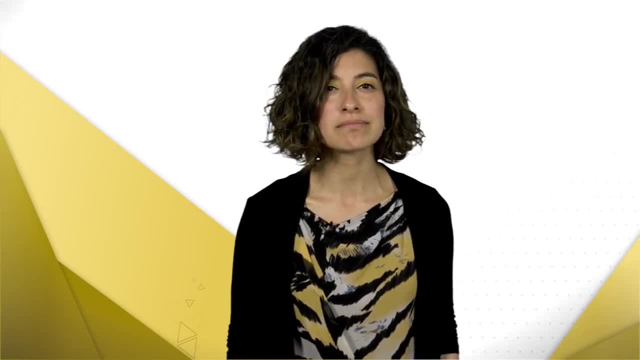 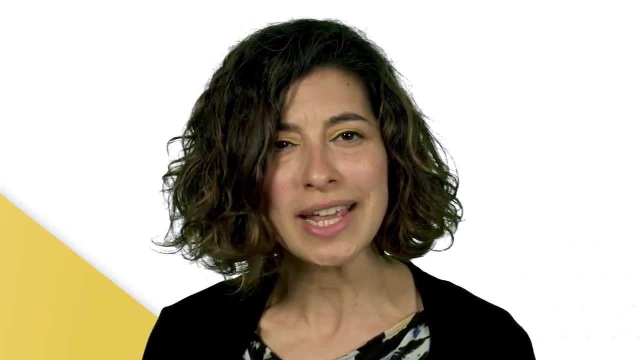 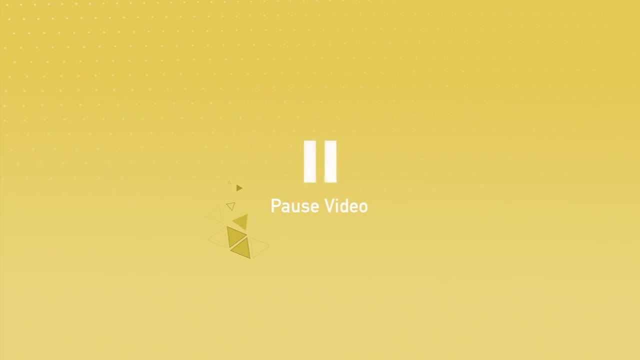 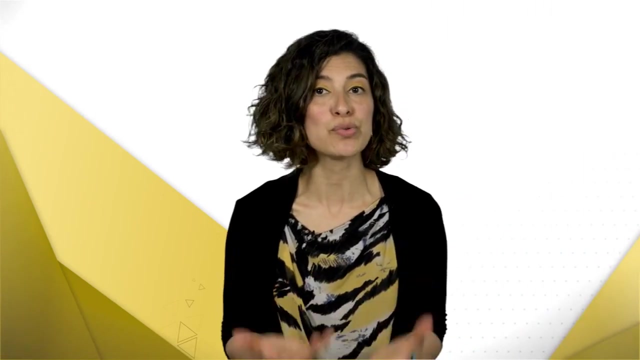 Adding up the first number in the cards, resulting in the secret number. Well, we have a theory. now We can test it. Or, better still, you can test it. Do it again with other numbers Once you get data that confirms the theory. you need a proof that it will always work. 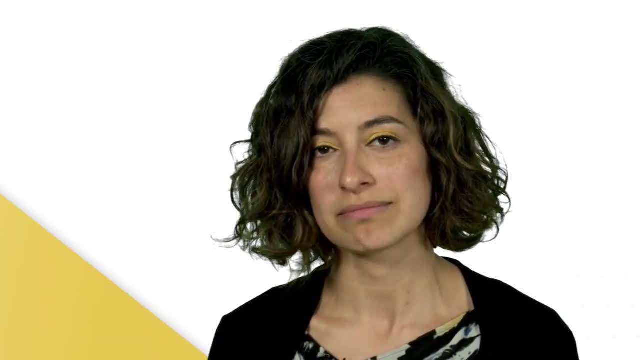 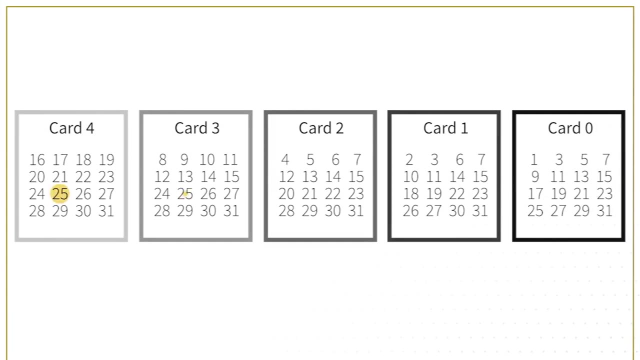 In mathematics. such a proof is an explanation. and here it comes: The way the mind-reading cards code the date of the birthday is the same we used in our domino computer binary. The first numbers of the cards are one, two, four, eight and sixteen. 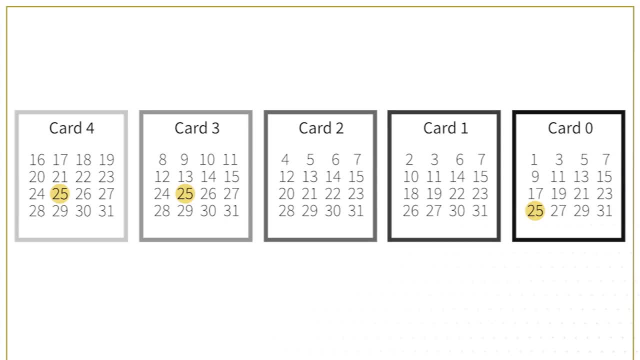 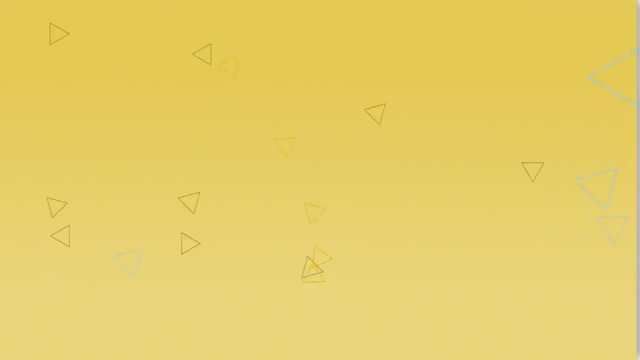 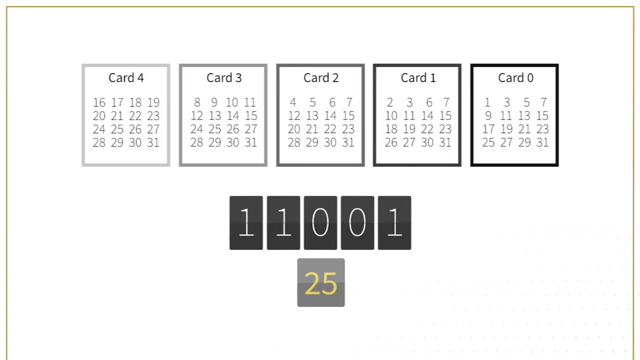 They're all doubling numbers. They are powers of two, Two to the zero, two to the one, two squared, two cubed, two to the power of four To write twenty-five. in binary we write one, one, zero, zero, one. where each one stands, 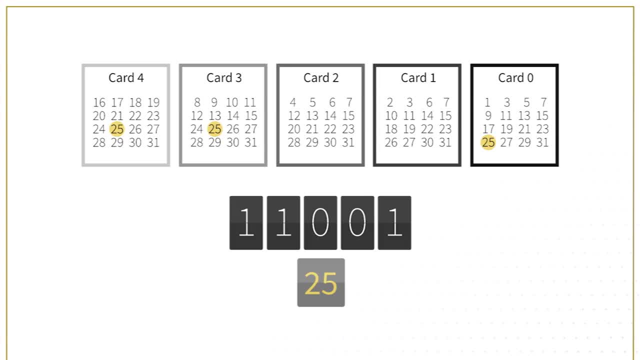 for twenty-five being on a card and zero stands for not being on that card. So from left to right we have card four, card three, card two, card one, card zero, And we write one for being on card four, one for being on card three, zero for not being. 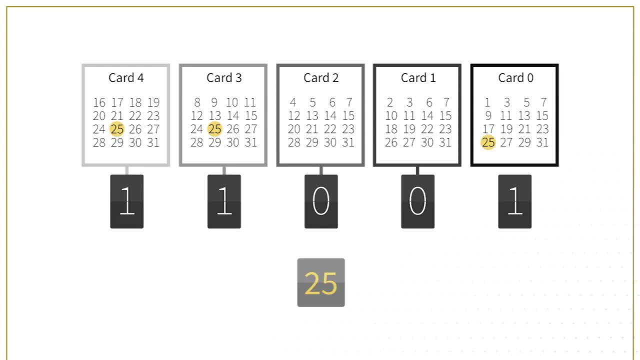 on card two, zero for not being on card one and one for being on card zero. The worth of these positions are sixteen, eight, four, five, six, seven, eight, nine, ten. So if there is a one in a position, we add the corresponding worth. 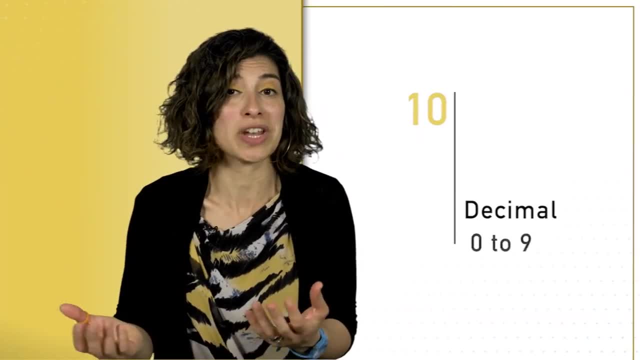 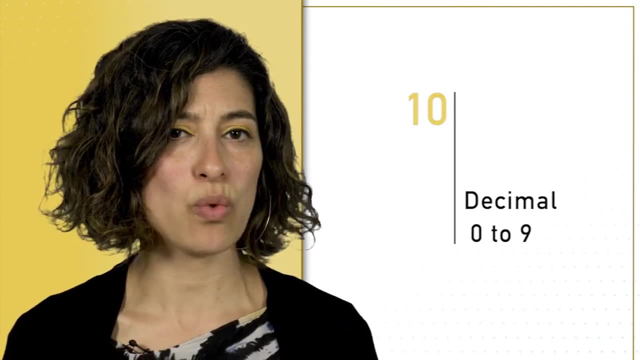 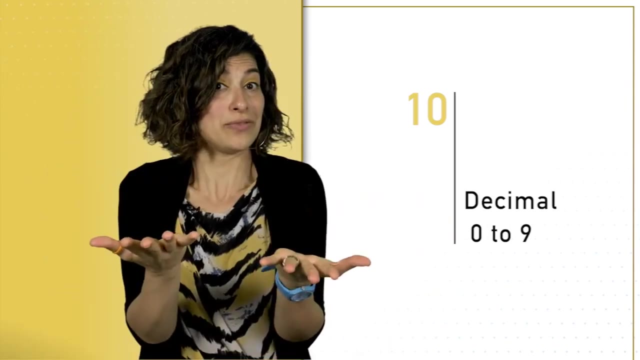 In everyday life, we use the decimal system using digits zero to nine, Ten digits in total. The number twenty-five uses five in the position that is worth one and uses two in the position that is worth ten. It is very likely that the reason behind using ten digits is that the number twenty-five 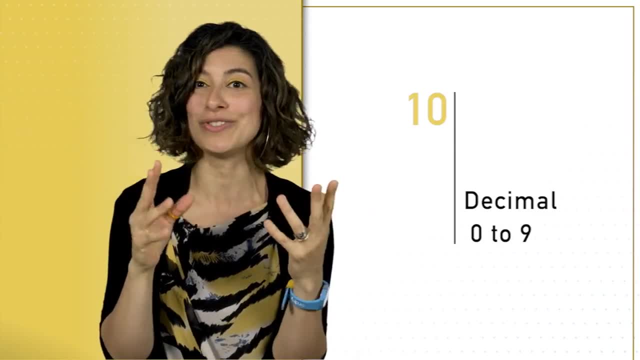 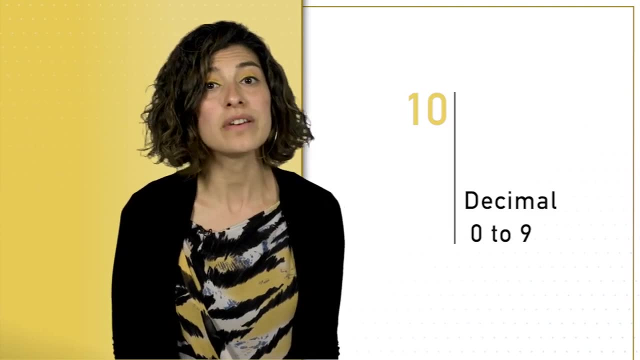 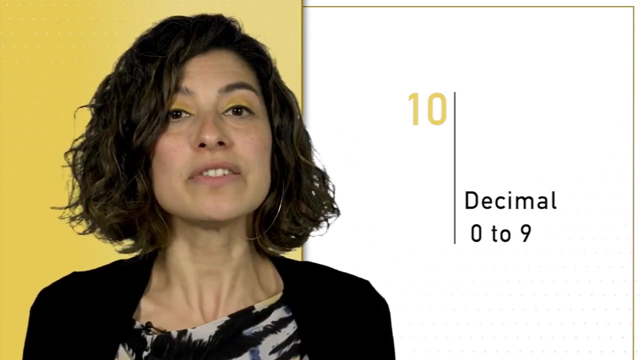 is the number of fingers humans usually have in their hands. The decimal system is also called base ten. The worth of each position is called the place value. The place values in decimal go up by a factor of ten. it's always the base number starting. 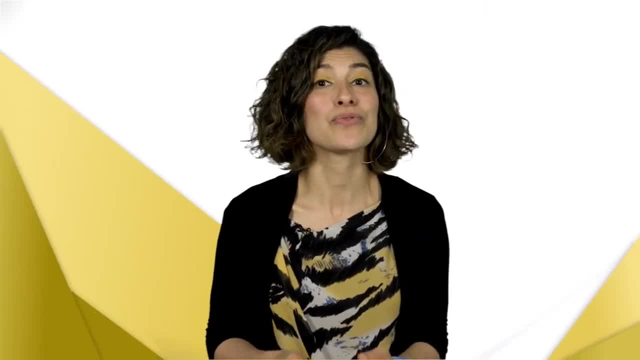 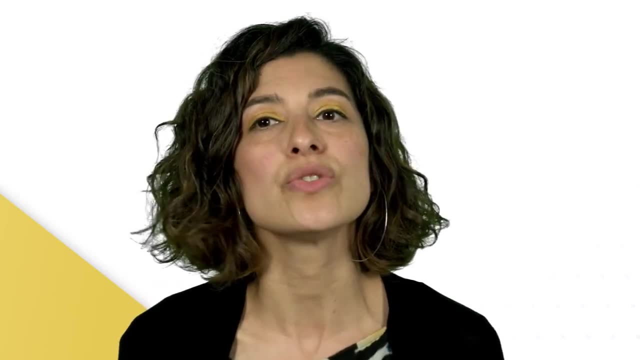 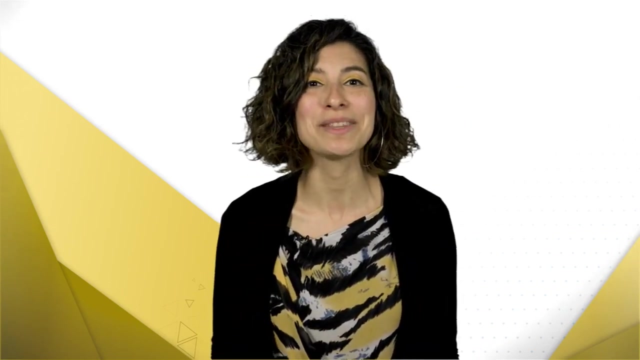 from one. We read place value from right to left, with the rightmost place value being one, Then ten, then hundred and so on. The digits- a word that comes from the Latin word for fingers- are multiplied by the place value in order to know the total value. 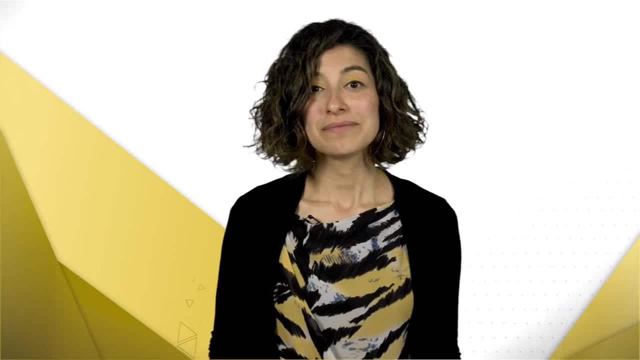 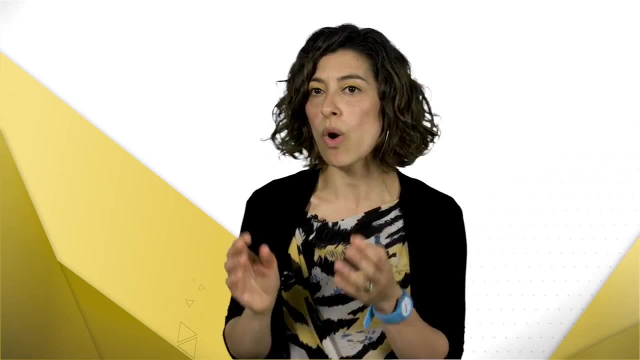 We use this recipe for any number base. The key idea in number bases is that the base number is how many digits are used, and the place values start in one on the right hand side and the next place value on the left goes up by a factor of the base. 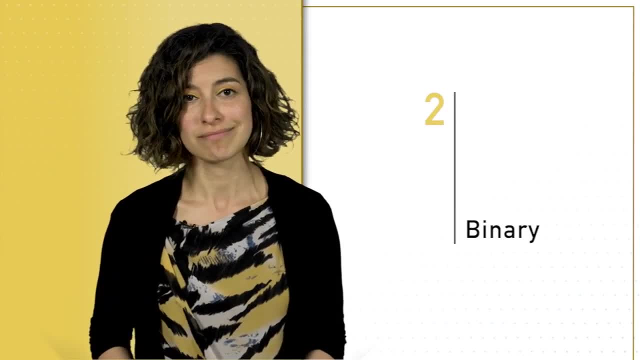 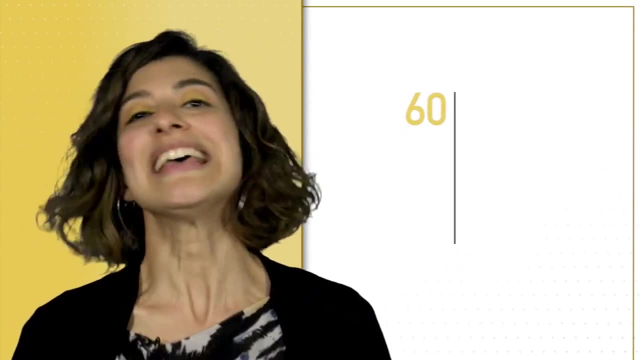 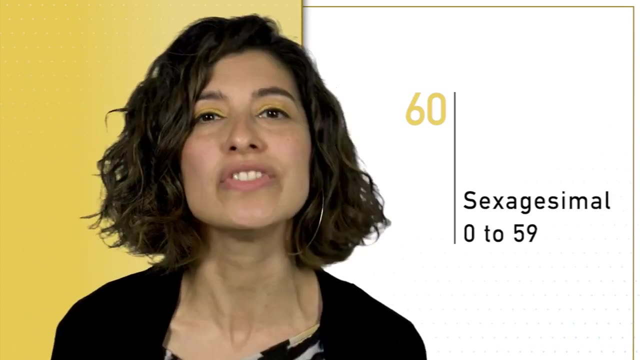 So base number is one. Base two, called binary, has two digits, zero to one. The place values are powers of two. Base sixty, called sexagesimal, has sixty digits, from zero to fifty-nine, and the place values are powers of sixty, and so on. 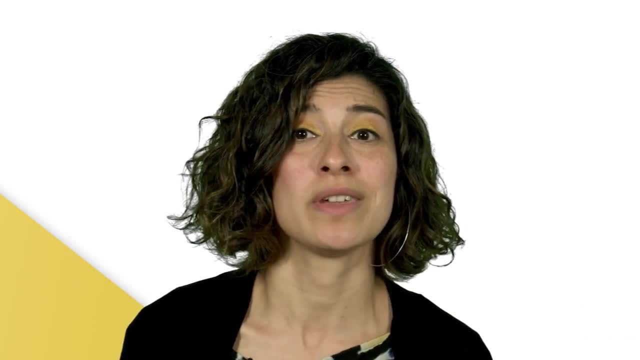 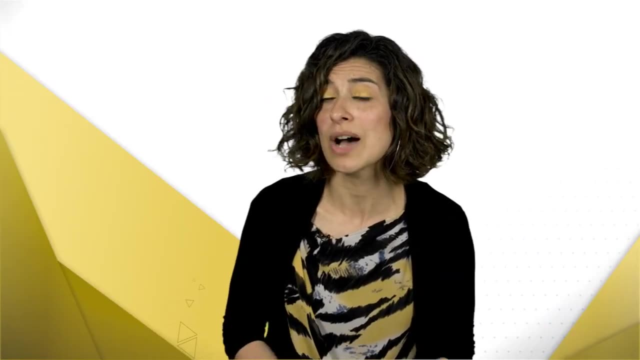 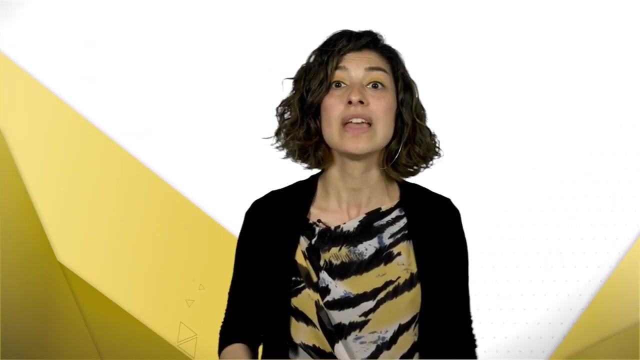 But base numbers aren't a modern thing. They have been along with us as humans since the time we started organising counting for larger numbers. Number bases allow us to use only a small number of symbols to write an unlimited quantity of numbers in a systematic fashion. 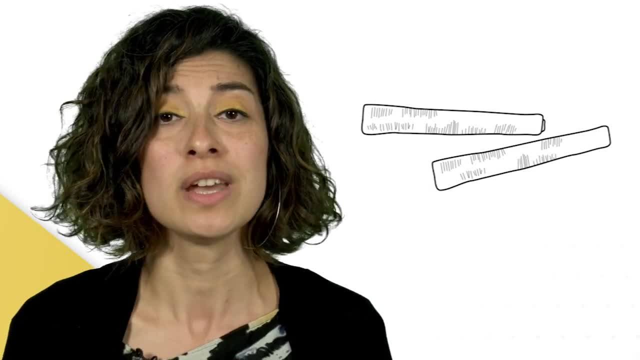 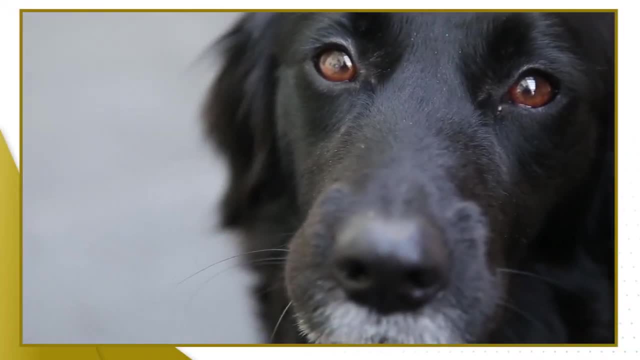 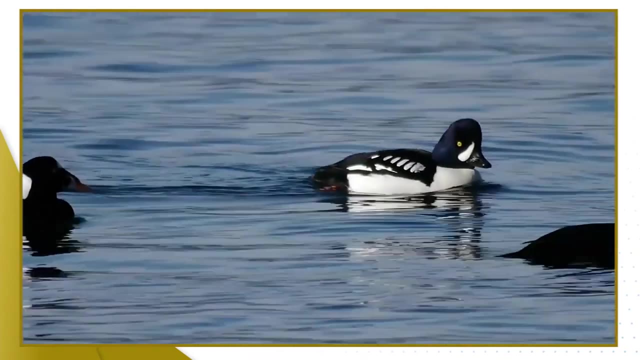 It is a huge leap from carving notches on a bone to keep track of how many sheep you keep. A number sense is not exclusive to humans. Many mammals and birds have a number sense, and there is evidence that shows such animals being able to distinguish quantities of one, two, three, four, five, six, seven, eight. 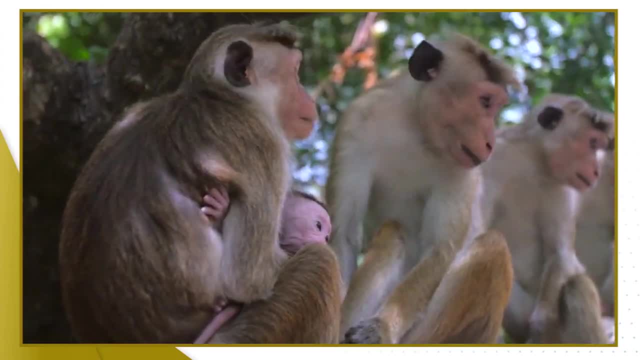 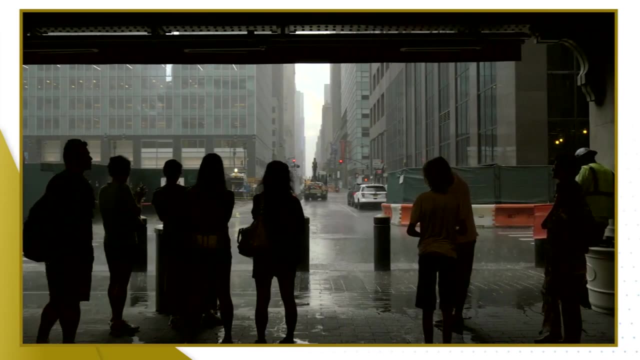 five, some three, four and some four, and an ability to compare larger quantities or even fractional quantities such as half, quarter and three-quarters. But we humans are a species that took that number also further and have mental and physical 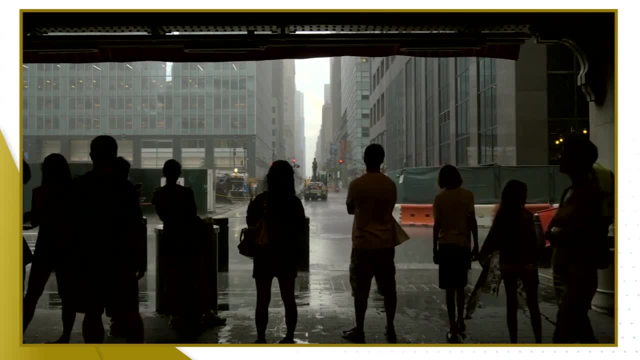 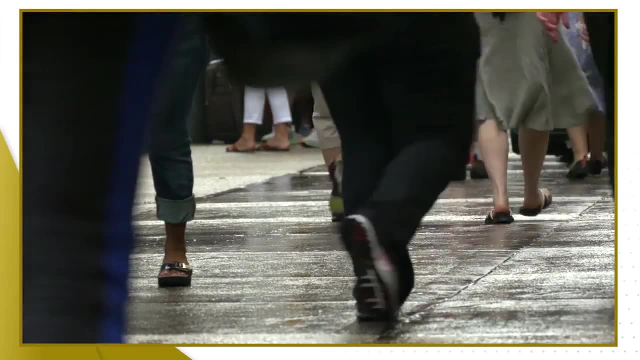 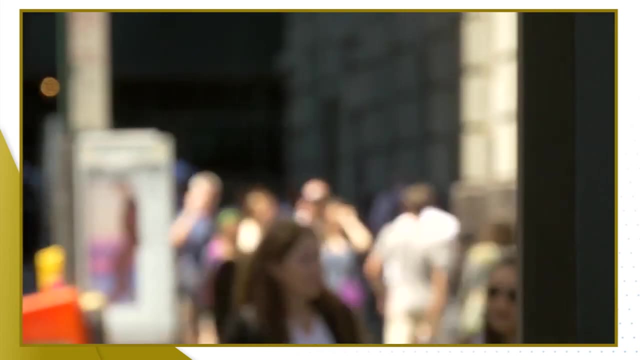 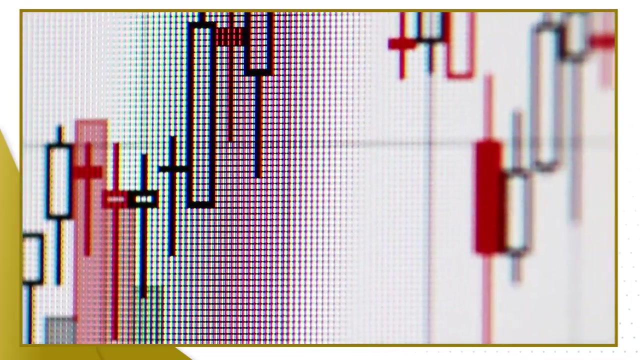 representations of counting numbers, including without the concept of coming to nothing and infinity. Our species has cultural needs that require precision, so we need a system to note down numbers, making sense of them and doing sophisticated operations with them. We develop routines, algorithms to add up, subtract, multiply, divide, to keep track. 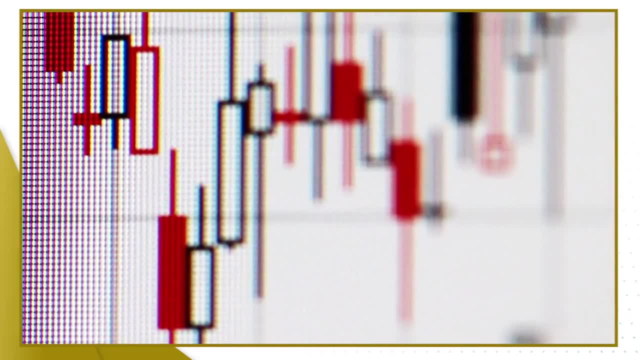 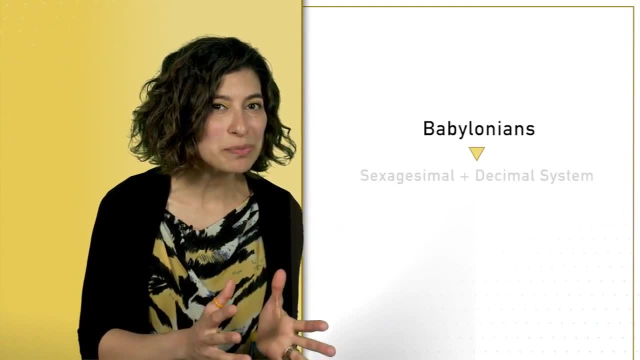 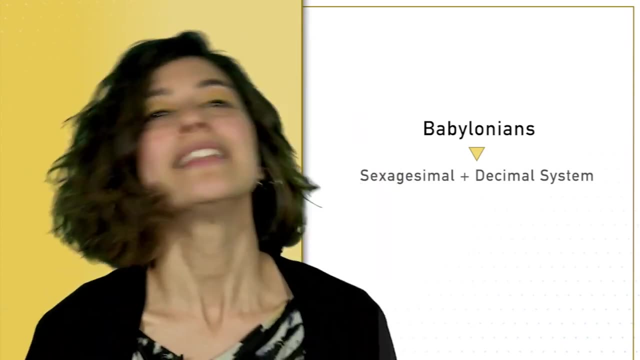 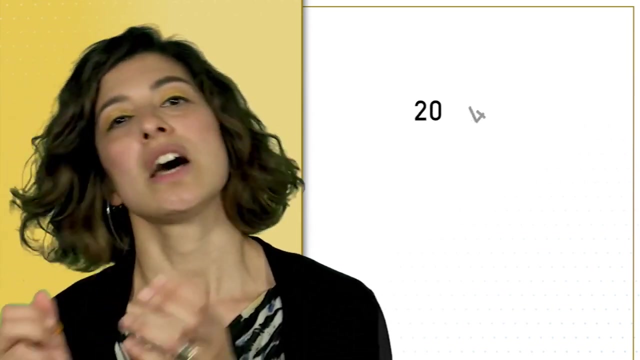 of money and goods when trading. Today we still employ mathematicians and computer scientists to work in trading. Babylonians used the sexagesimal system combined with decimal base 10 to make numbers up to 59, the digits. These digits were then used in place values that are worth powers of 60. In sexagesimal, 20,, 4,, 59. 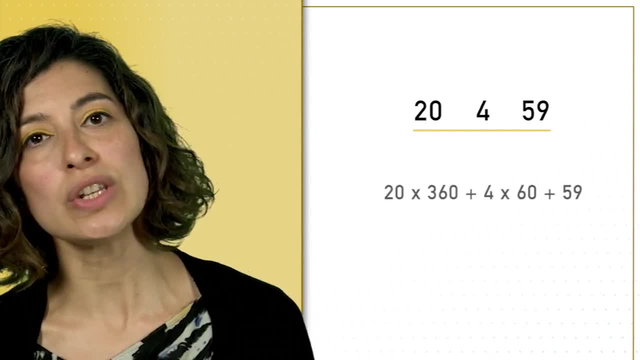 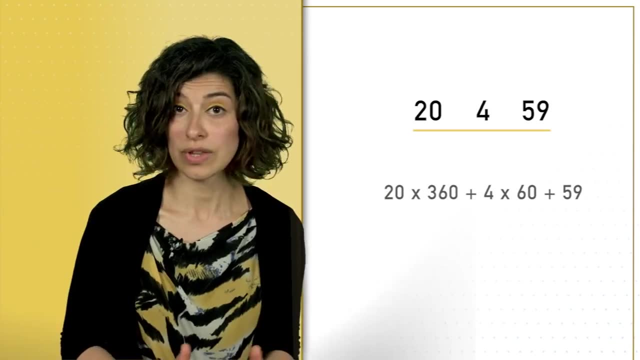 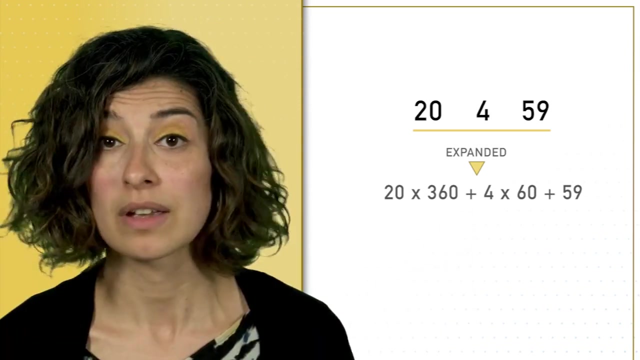 means, from the right to the left, 59 units, 4 times 60 and 20 times 360, all added up. So the expanded form of this number is 20 times 360 plus 4 times 60 plus 69.. And note we write from left to right, from the largest place value to the. 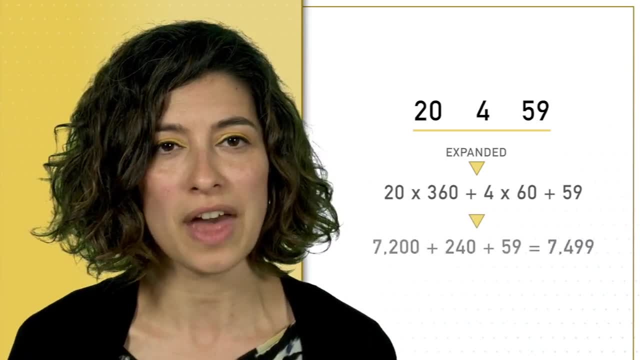 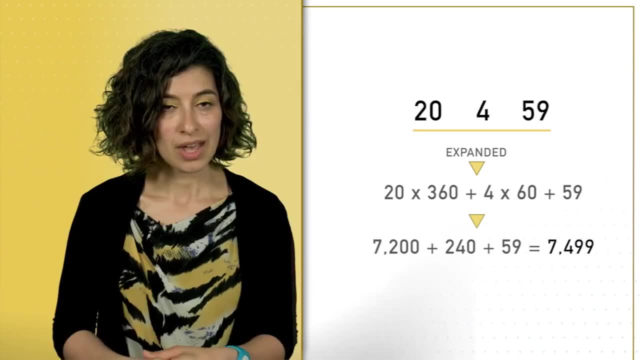 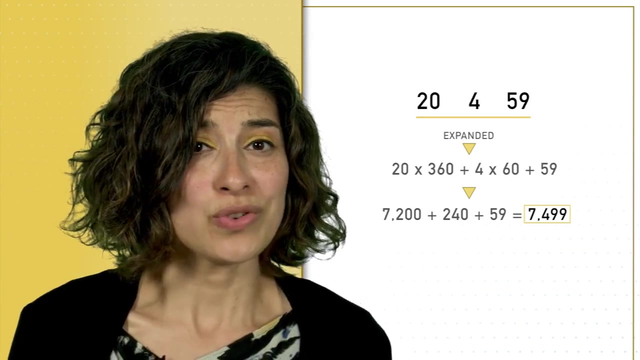 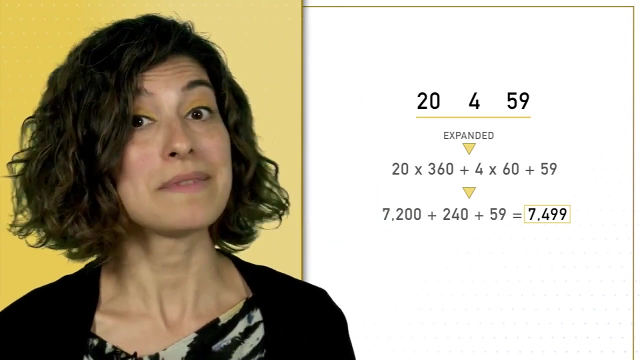 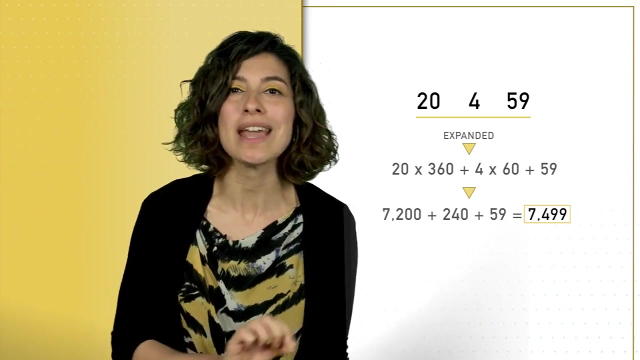 smallest, and this equals to 7200 plus 240 plus 59, which equals 7,499 in decimal. Now are you wondering if the Babylonians had 60 different symbols for the digits 0 to 59? Yes and no. The genius of it is that they used two symbols only to make all the digits. They used clay tablets. 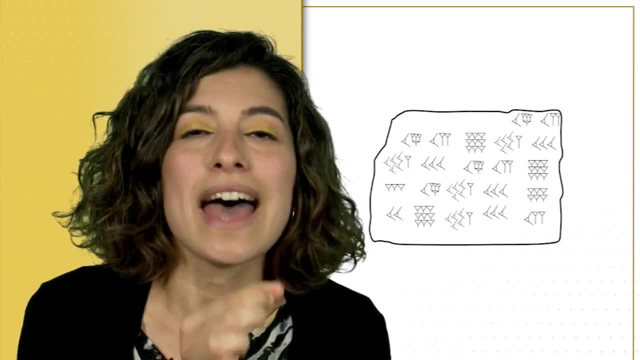 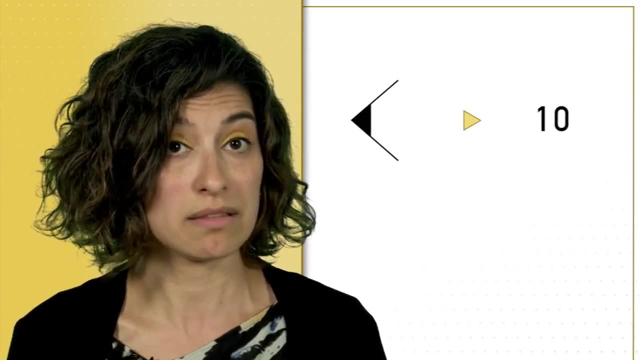 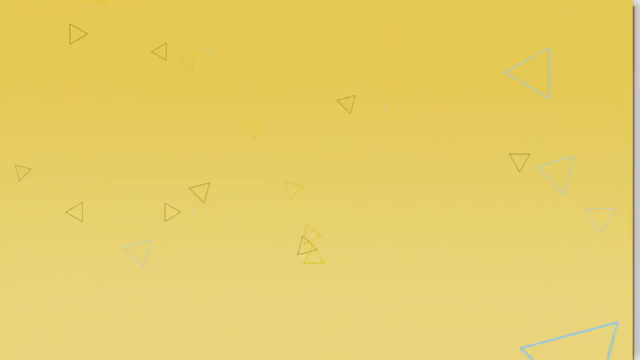 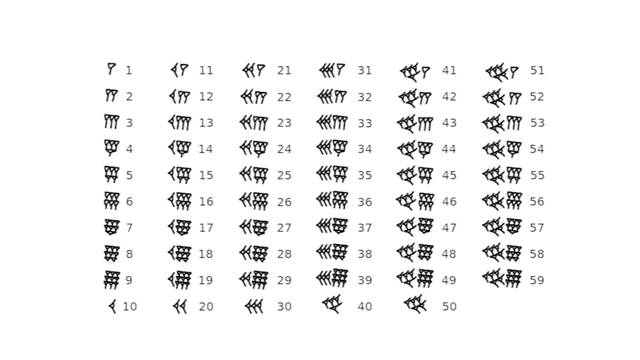 and a stylus- really just a stick- and pressed the stylus on the fresh clay to make marks like this for 10 and like this for 1.. And using base-10, they organized the marks like in this picture And this allowed them to make astronomical calculations. I mean both as in large numbers. 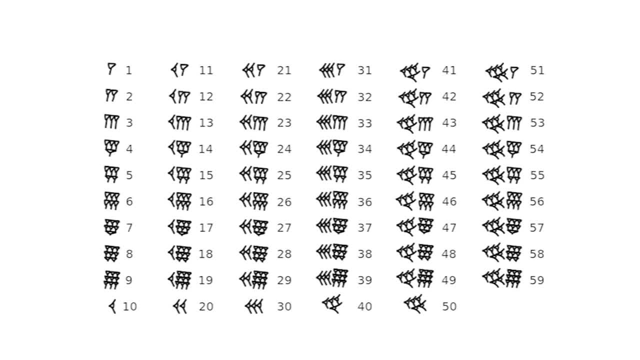 and also as in tracking the movements of the bodies observed in the sky. The motivation for this system may be that to observe the sky, it is handy to divide a circle into many small equal parts. 60 is a number with many factors. It can be divided by 1,, 2,, 3,, 4,, 5, 6,, 10,, 12,, 15,, 20,, 30,, 60, which is 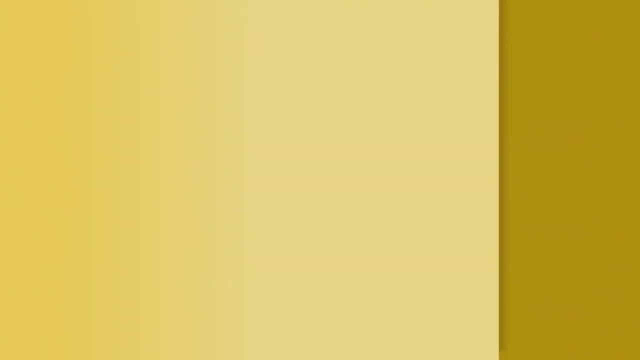 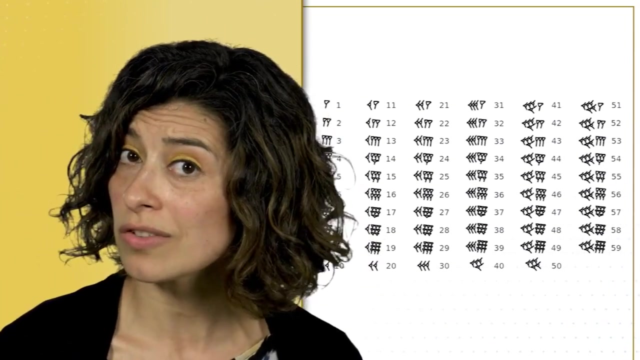 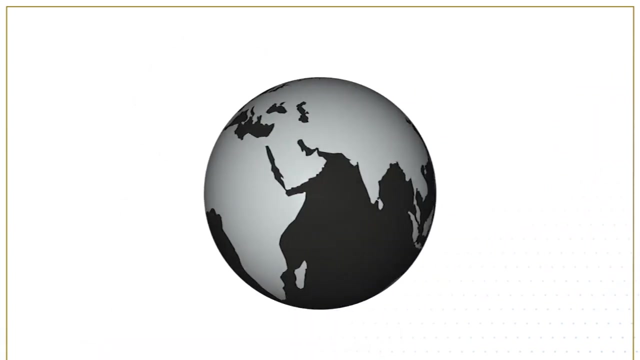 handy when we work out fractions of the denominator 60. This was a very sophisticated system and Babylonians calculated with fractions, not just whole numbers. Looking around cultures across the world, there is evidence of even other number systems. The Pomeranians used the vigesimal system, that is, base-20.. Although Europe primarily uses decimal, 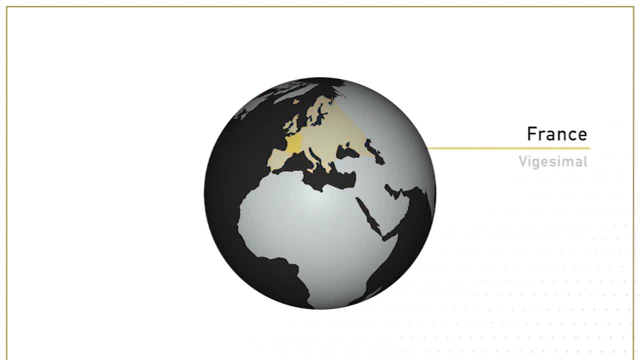 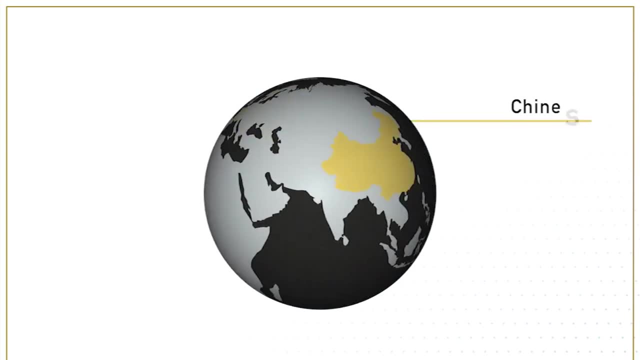 systems. in France there is evidence of using vigesimal, as the French word for 80 is 4, twenties 80. The Chinese number system is decimal, but with the added feature that a symbol for the place value is written after the digit as a reminder for the expanded form. For example, 193 is written as the equivalent. 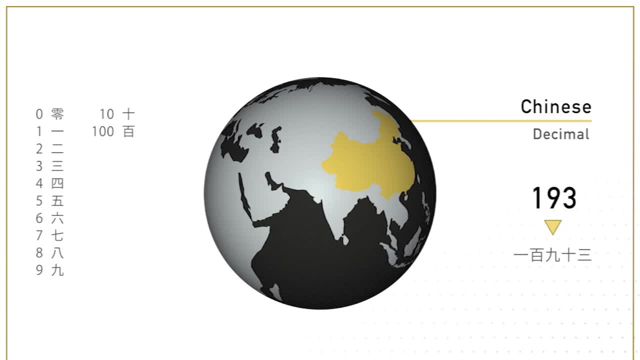 equivalent of 1,, 100,, 9,, 10,, 3,, with 110 being a symbol for the place value, 1,, 9, and 3 being digits. If that sounds really long, join me in appreciating a language fit for. 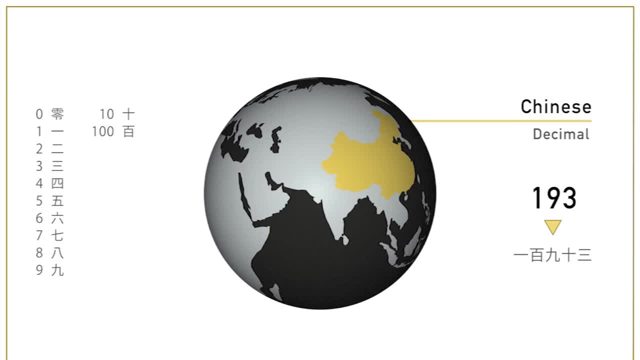 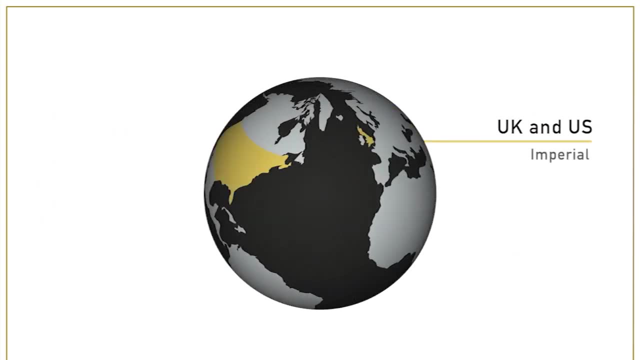 computation. The sounds for number words are shorter than the corresponding English words. In Britain and the US, the imperial system of measures uses bases 8,, 12,, 14, and 16, as they are: 12 inches in a foot, 16 ounces in a pound, 14 pounds in a stone, 8 pints in 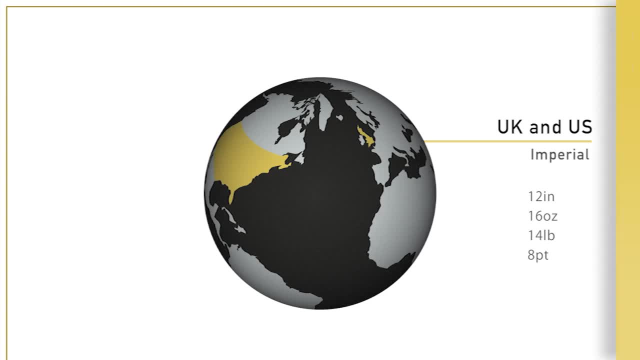 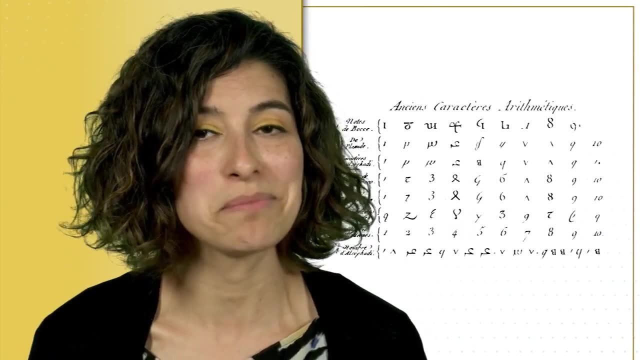 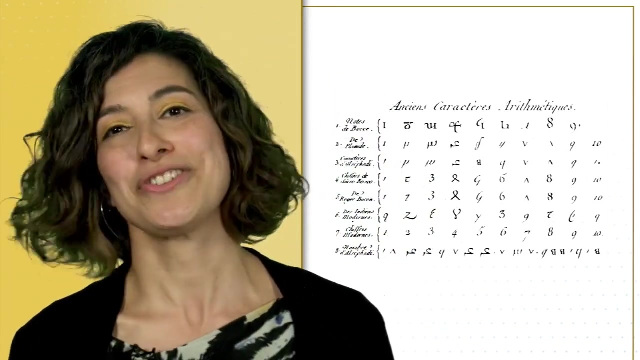 a gallon all side by side with decimal. Now the digits we use today in the decimal system come from the Hindu-Arabic numerals. The trading in the Mediterranean gave Europe access to the number of digits in the decimal system. It gave Europe access to a much more sophisticated number system, positional and fit for efficient. 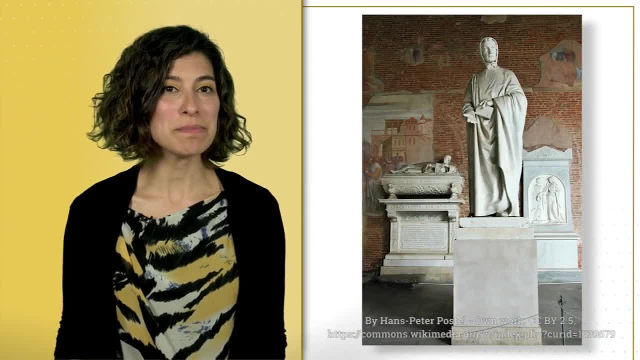 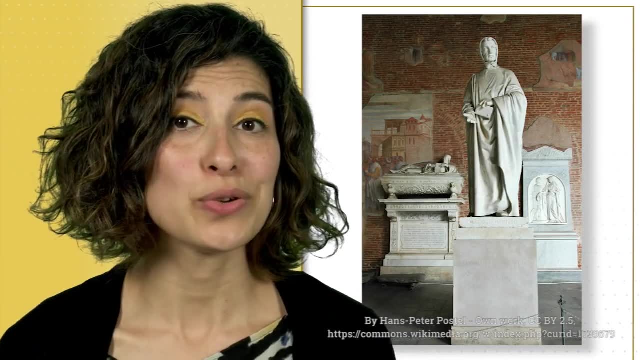 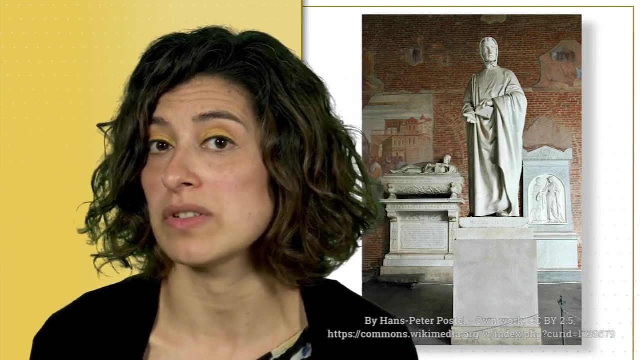 arithmetic. In the 1200s, Leonardo di Pisa, also known as Fibonacci, and himself the son of a trader, popularized these numbers. Until then, in Europe, the Roman numerals were used, and these were not suitable for speedy calculations. as the system is not positional, I mean to 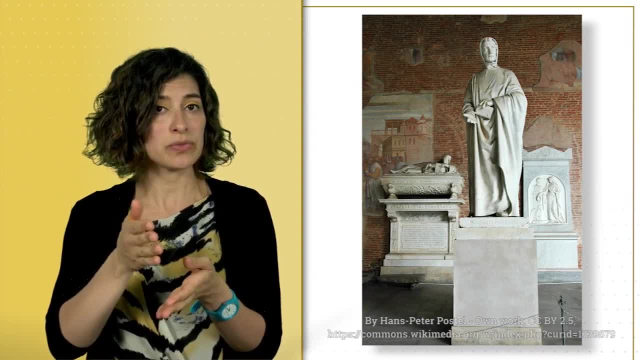 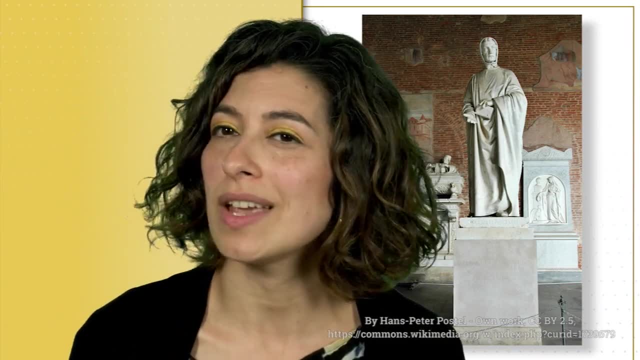 add 16 and 43,. we add the units 6 plus 3 to give 9, and the 10. We add the numbers 1 plus 4 to give 5, and get 59.. With Roman numerals it takes longer as the numbers in each place value are not so clear. 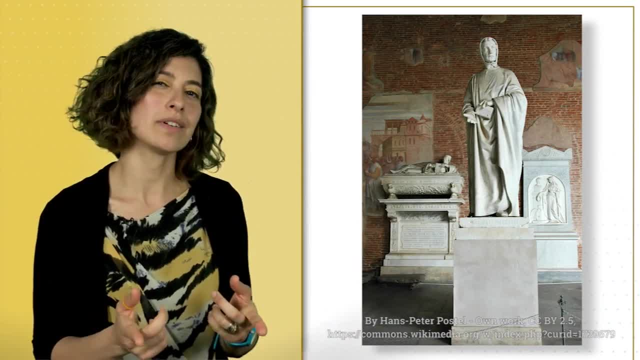 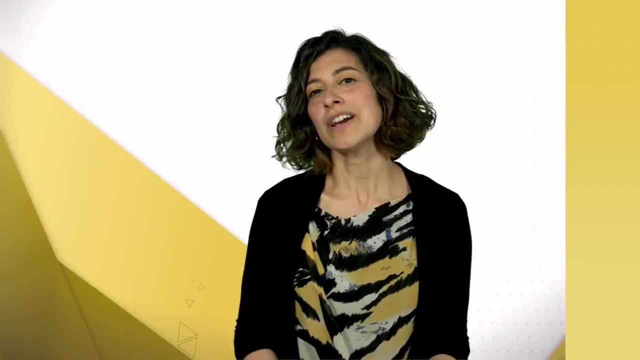 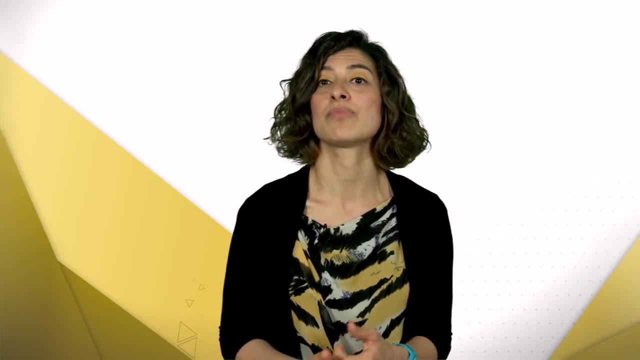 We still measure time using other bases. What bases are these? I invite you to investigate grey codes, as these are variations of straight binary system but have additional properties. We will not cover it in this topic, but it is of interest for any computer scientist. 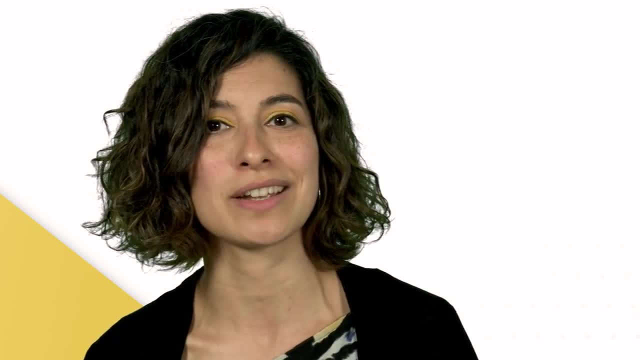 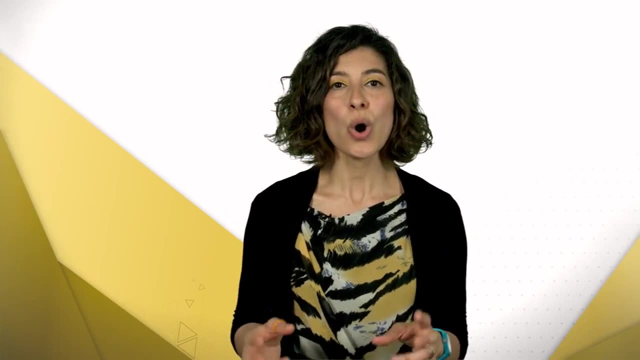 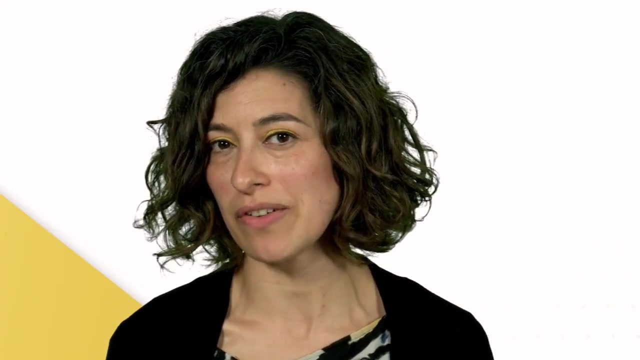 wanting to use number systems and error-correcting codes in making physical devices. It surprisingly comes up in the disentanglement puzzles called Bagnaudier. In the next lessons we will look at number systems of base- 2,, 8,, 16, and will perform. 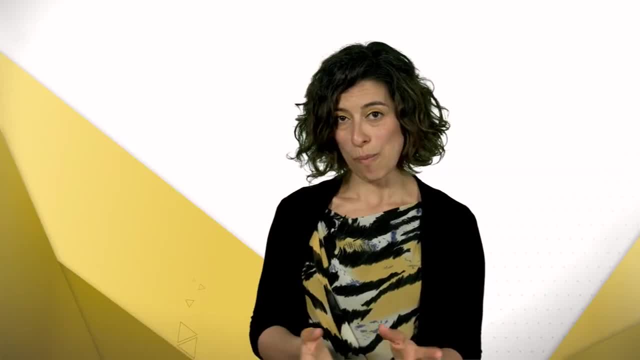 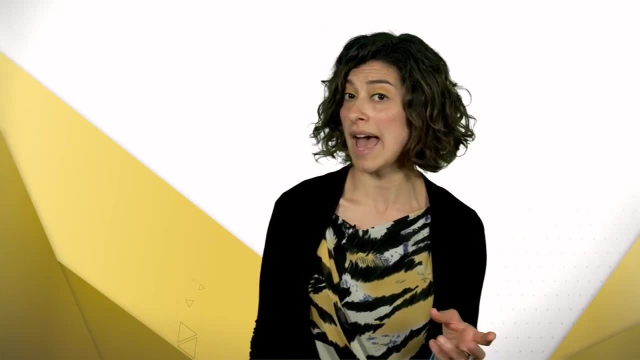 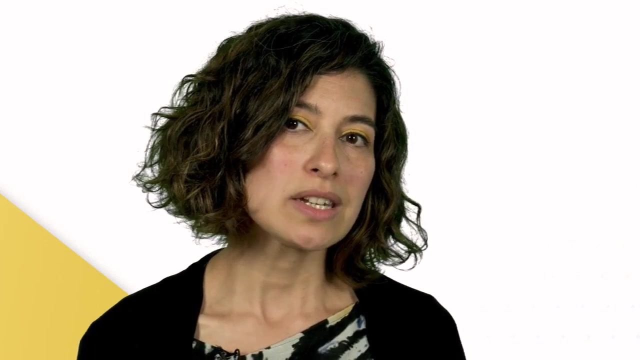 arithmetic operations in these bases To warm up, refresh your memory of how you learned to perform addition, subtraction, multiplication and division by hand back when you were a child. We will also look at fractional numbers- that is, between 0 and 1, and how we work with. 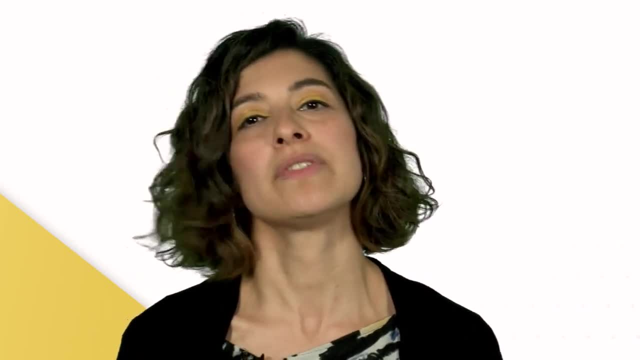 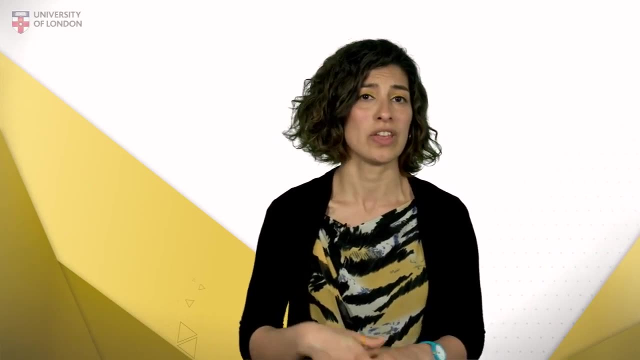 their digital expansion and their fraction representation. So go ahead and revise how to operate with fractions and turn digital expansions such as 0.25, into the fraction representation. Subtitles by the Amaraorg community. Subtitles by the Amaraorg community. 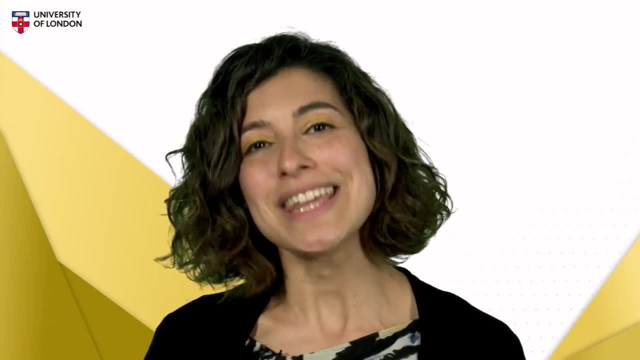 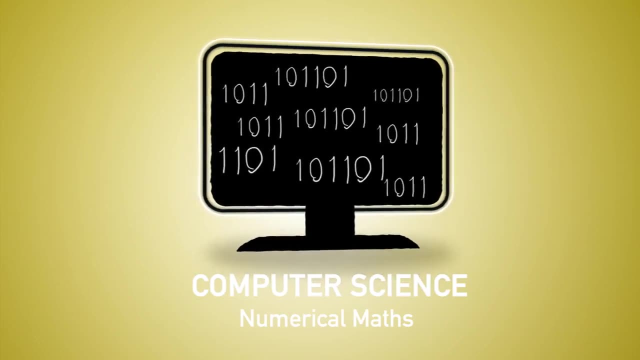 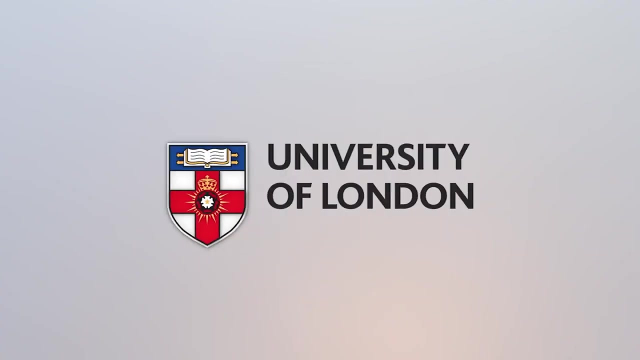 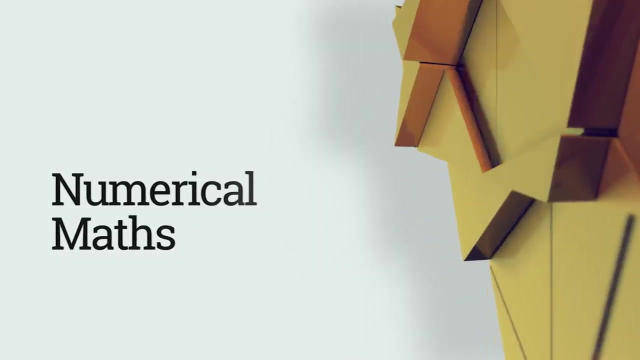 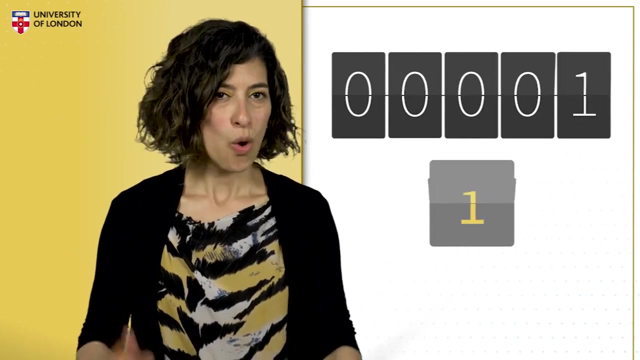 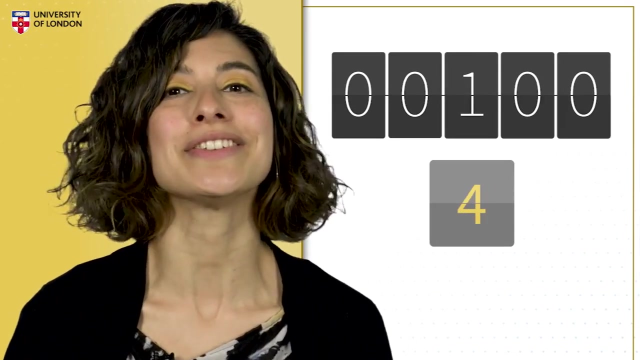 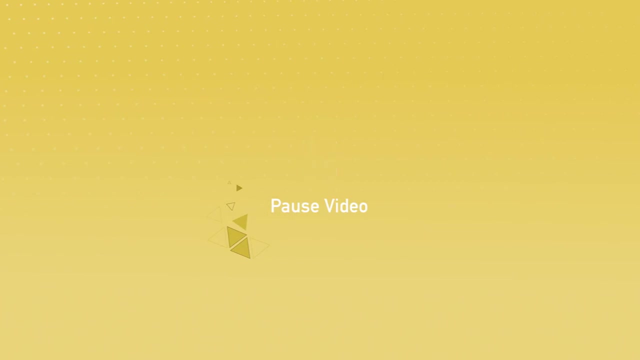 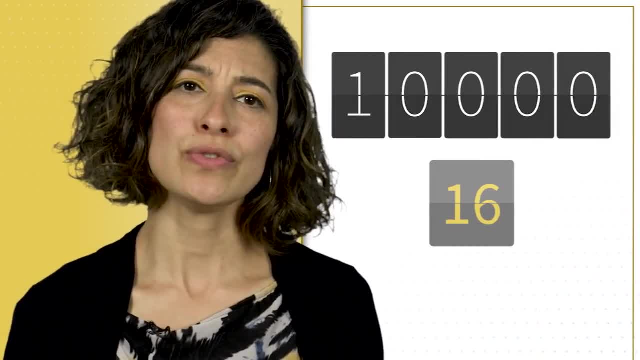 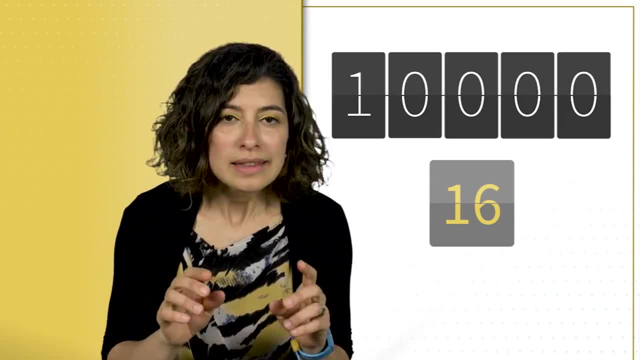 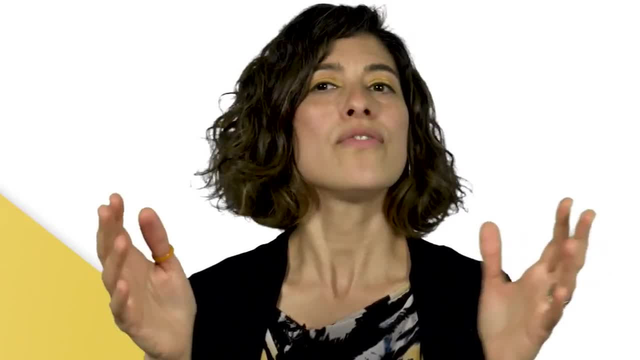 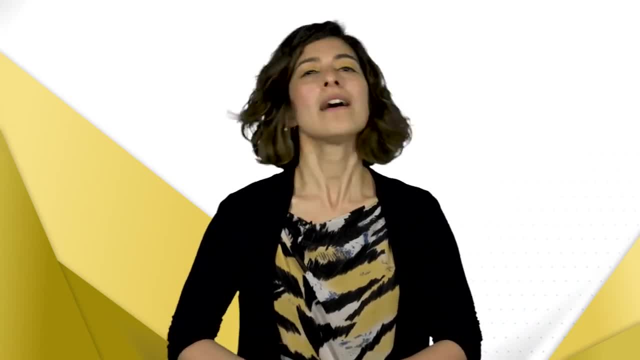 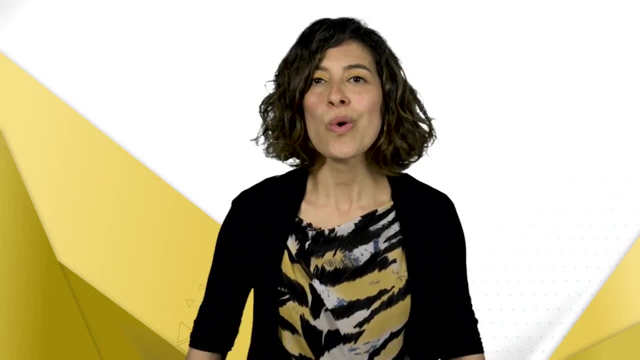 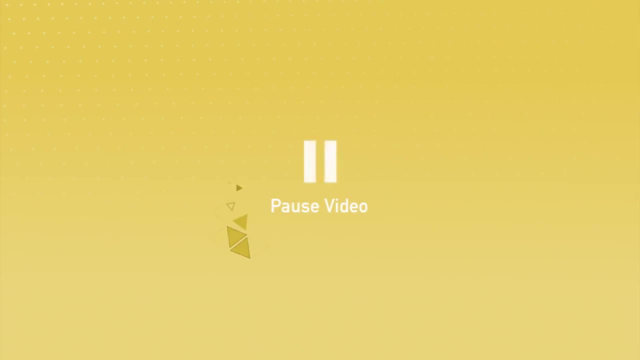 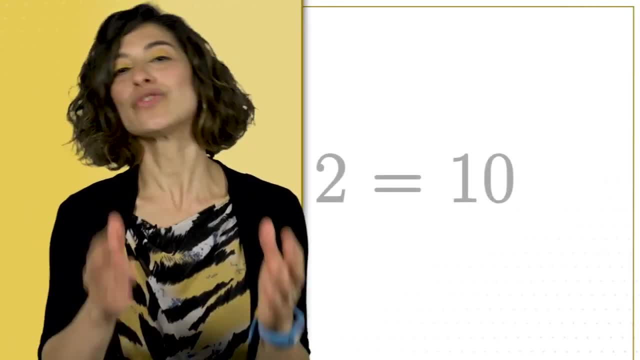 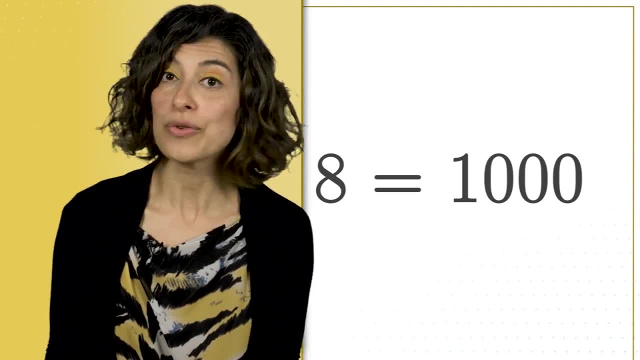 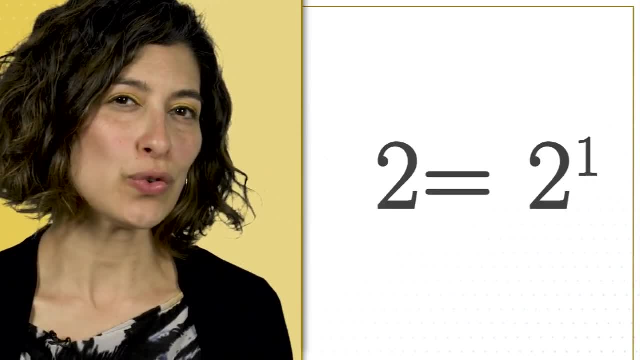 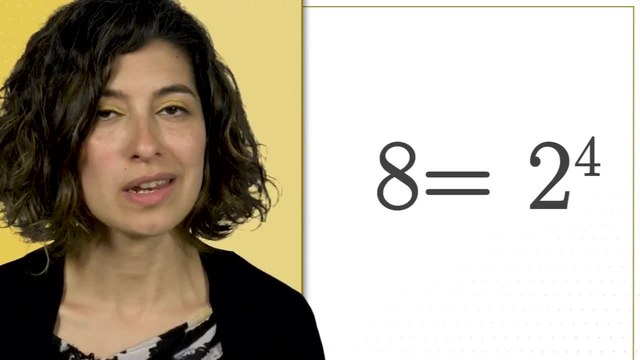 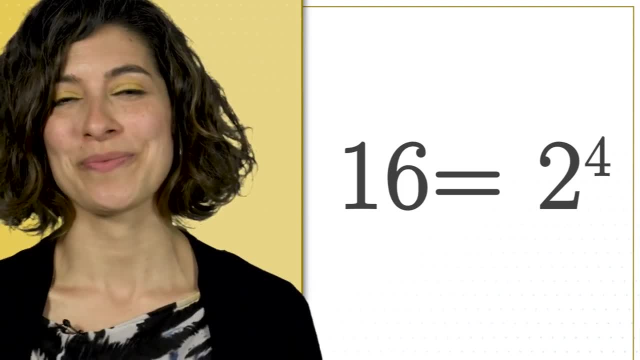 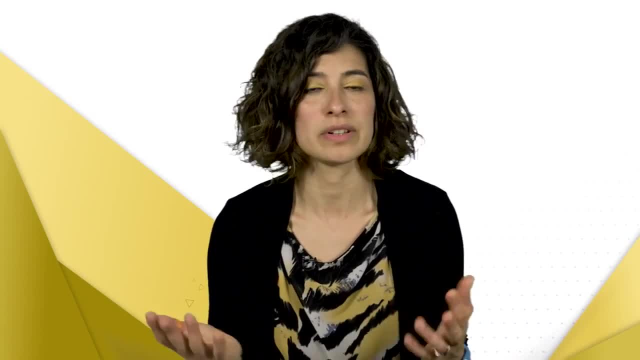 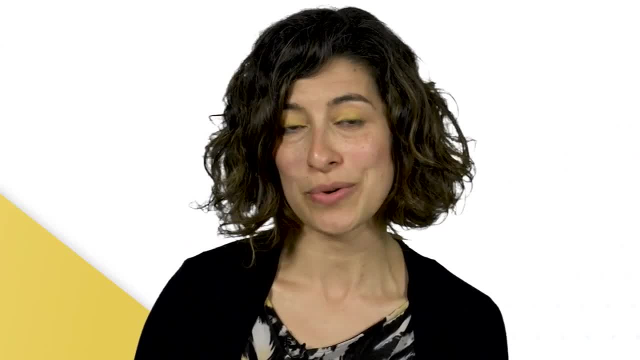 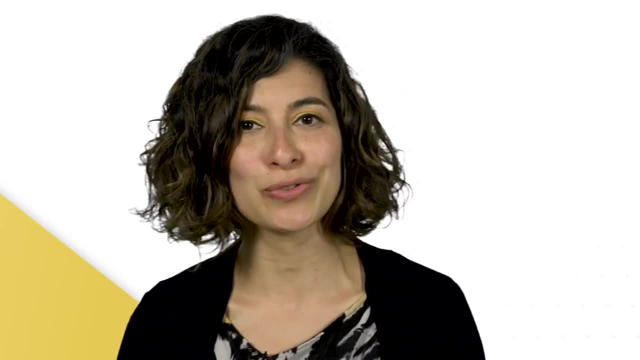 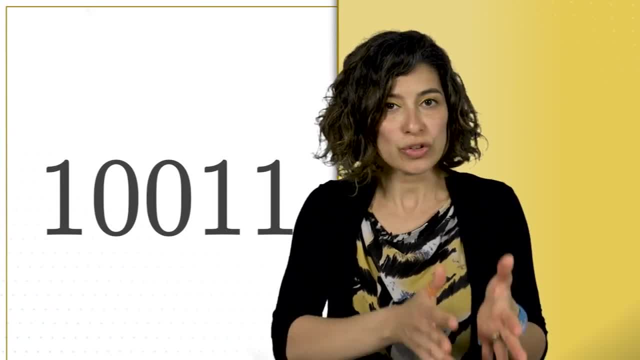 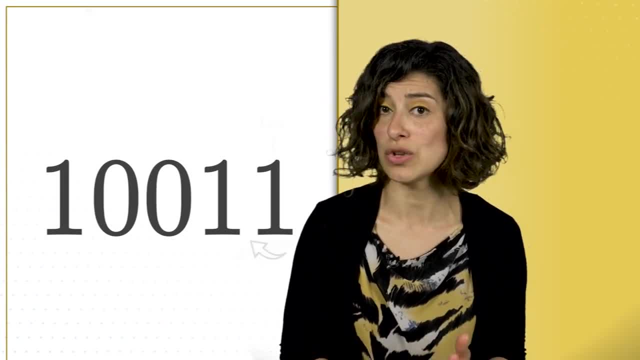 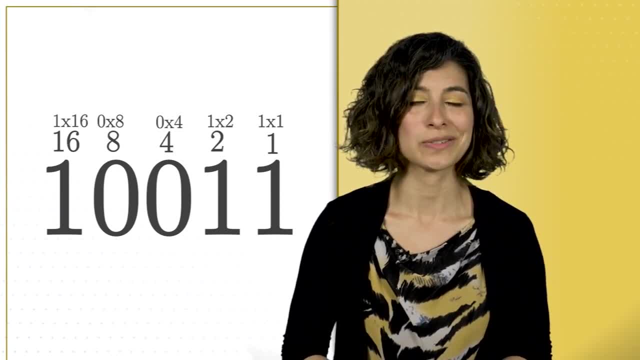 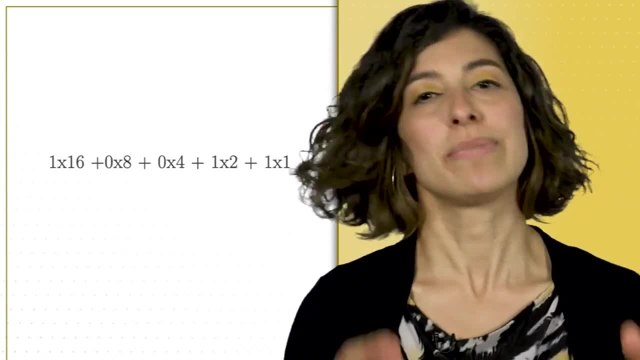 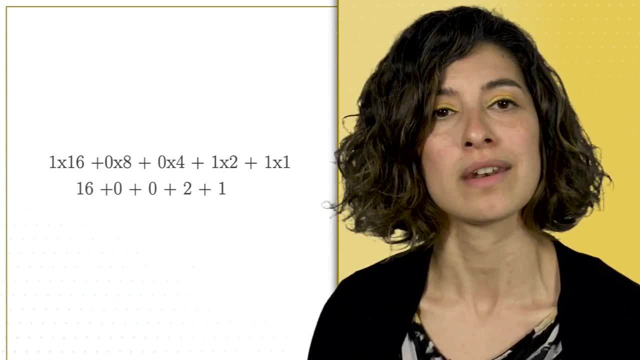 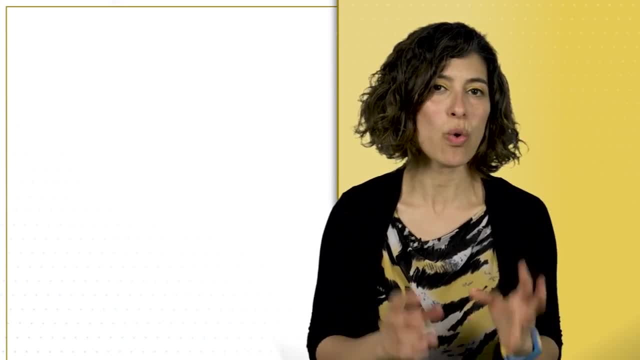 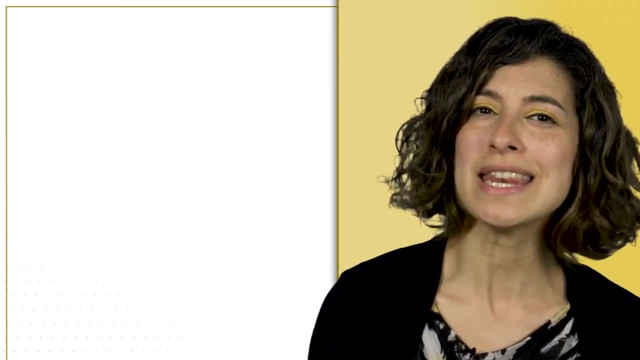 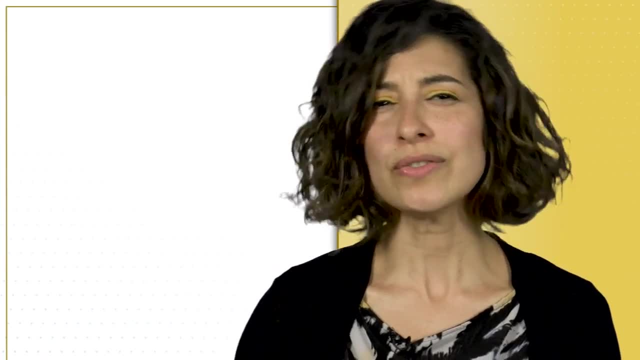 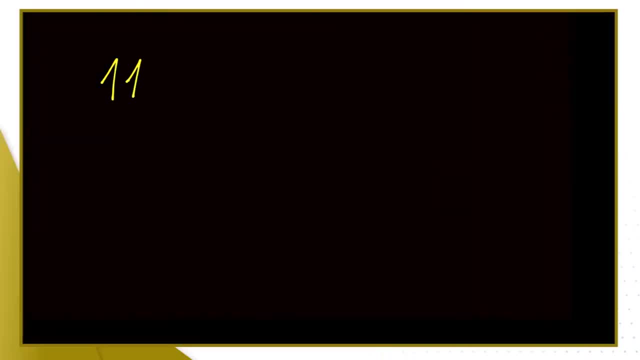 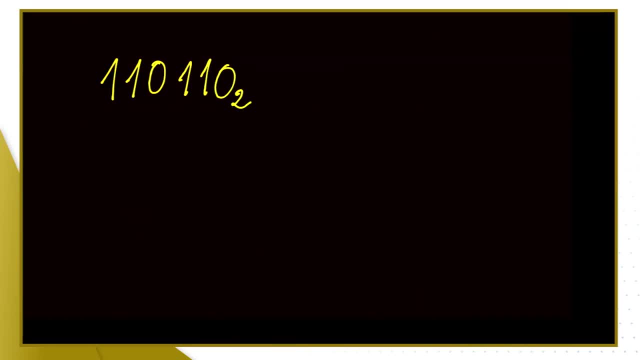 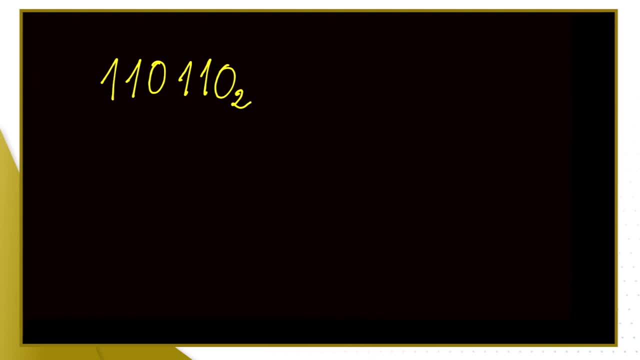 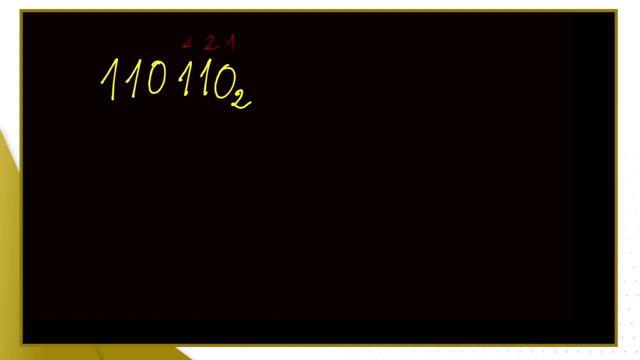 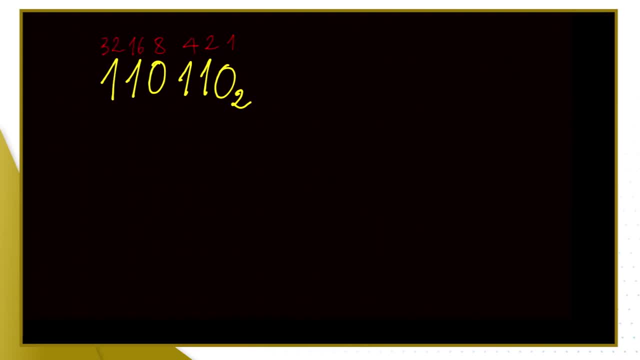 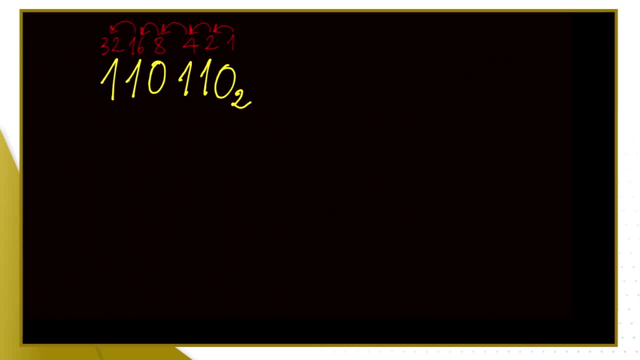 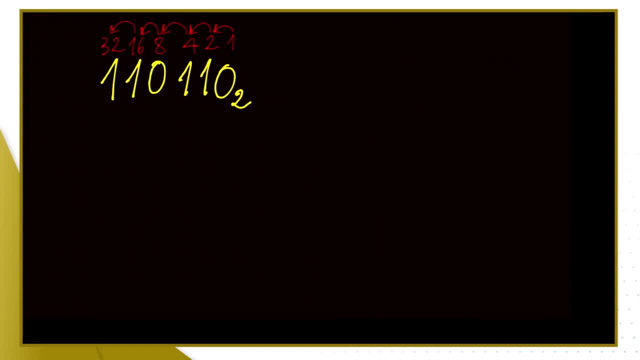 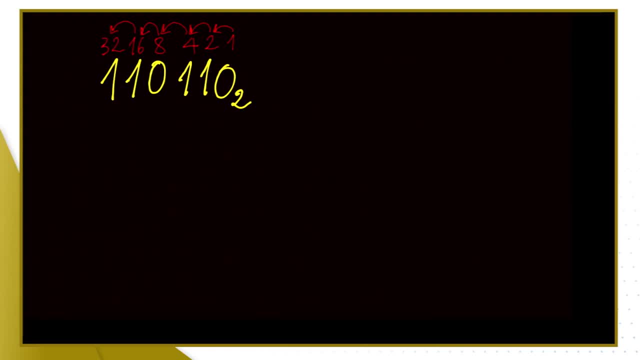 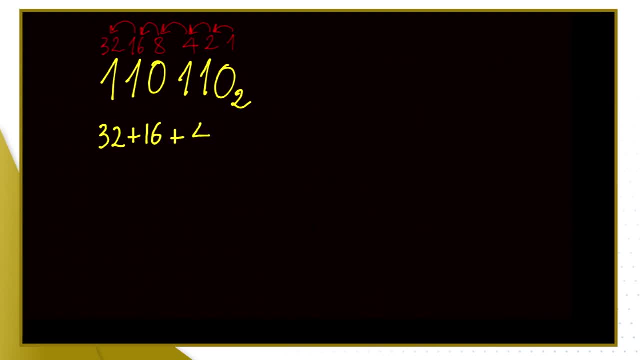 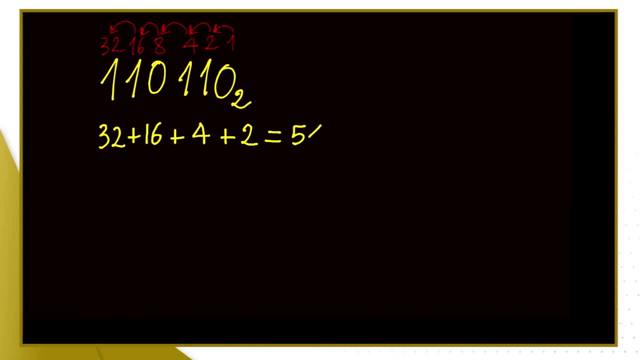 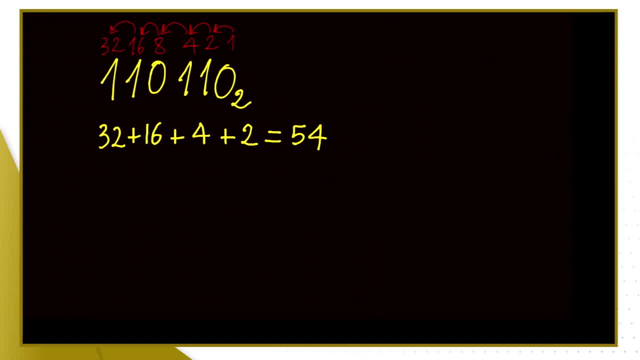 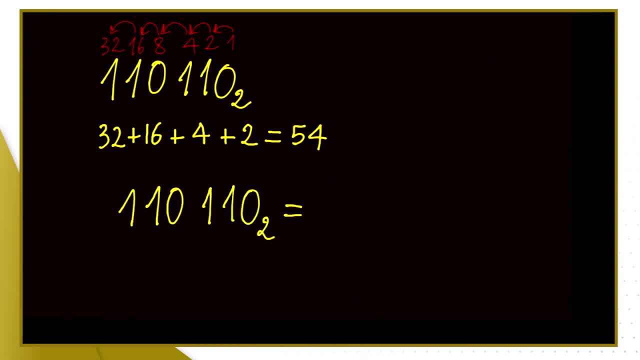 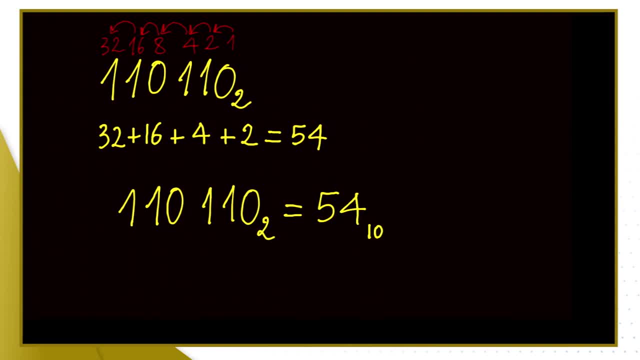 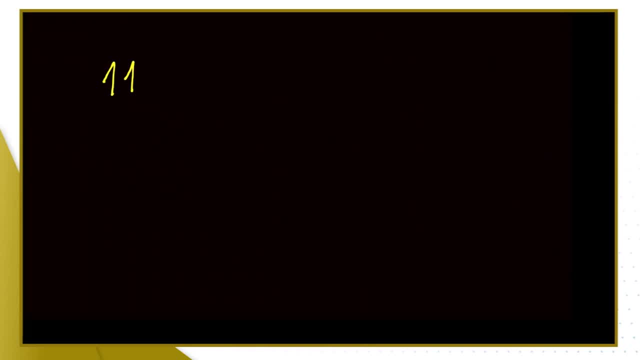 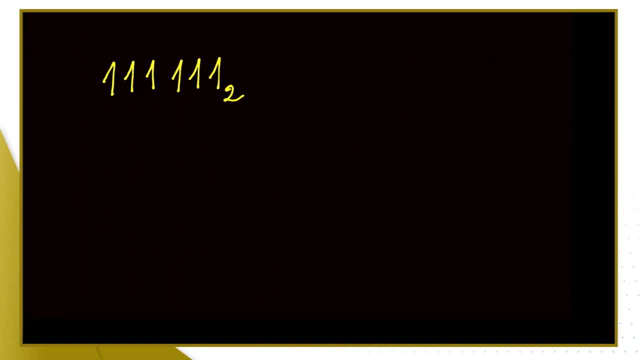 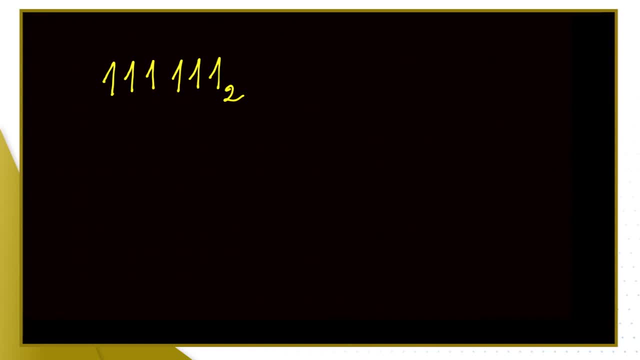 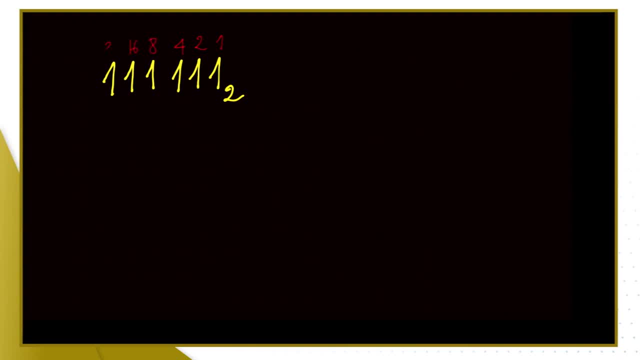 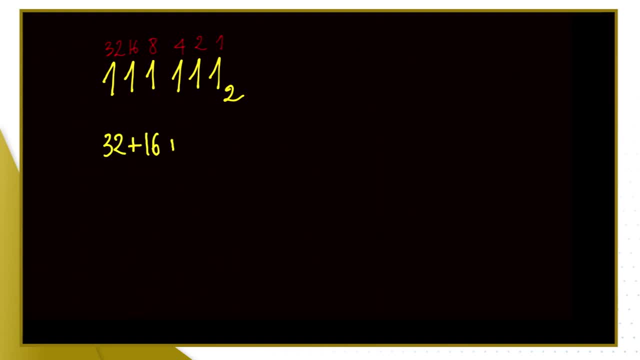 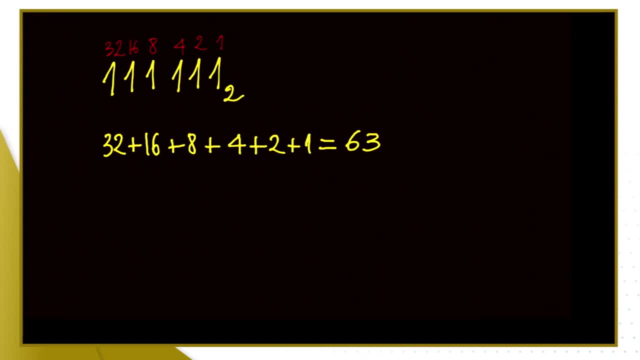 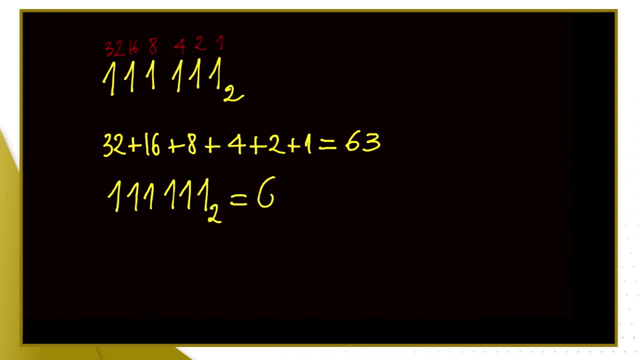 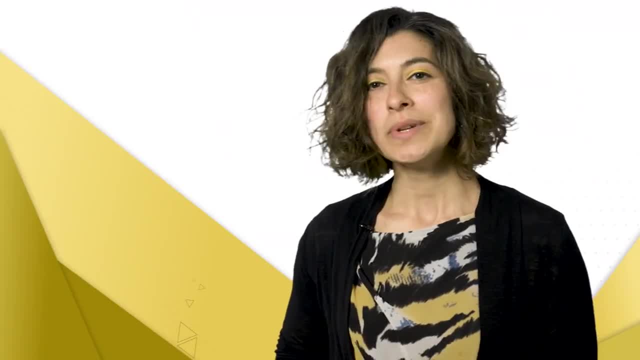 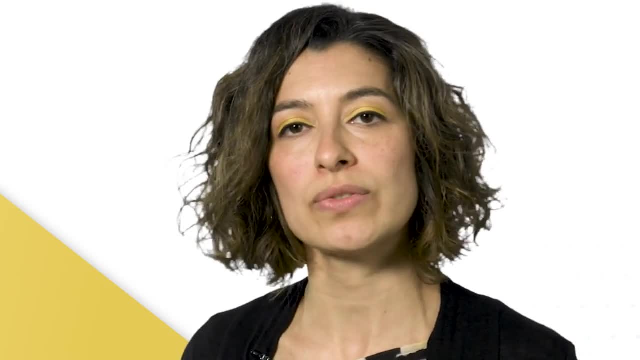 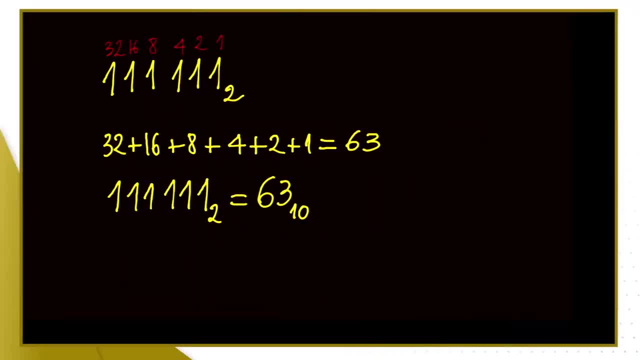 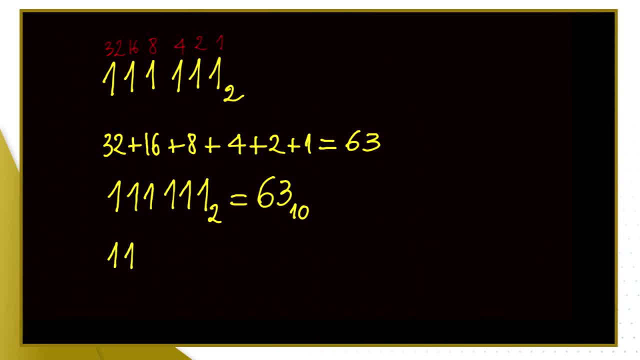 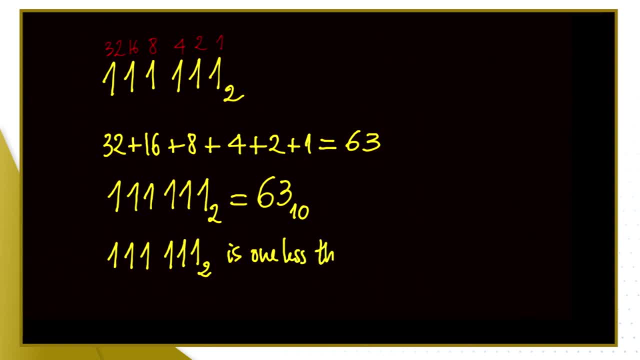 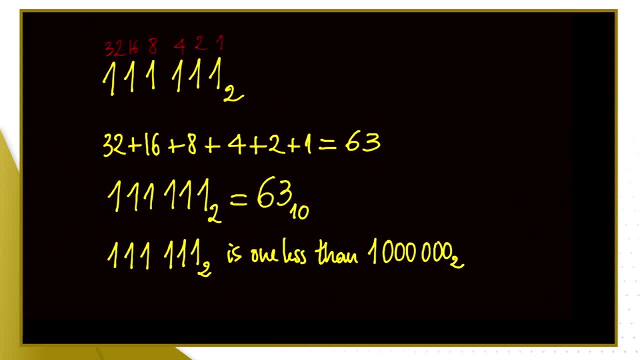 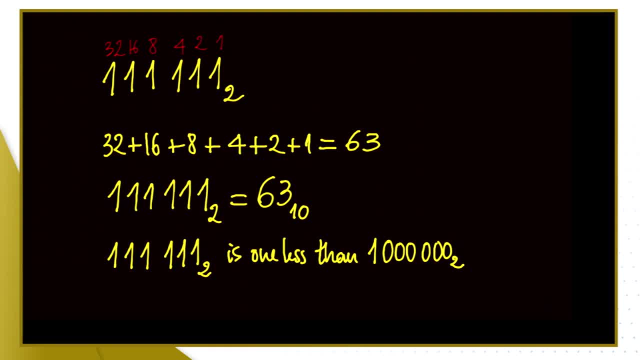 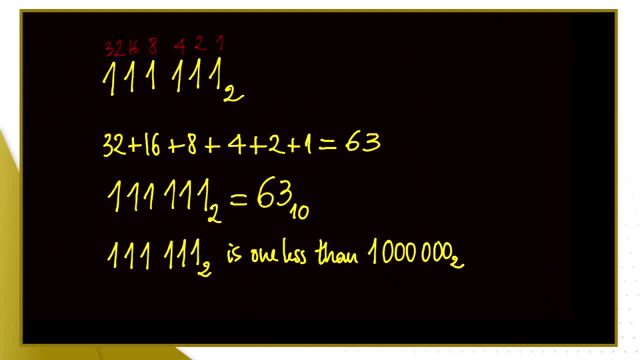 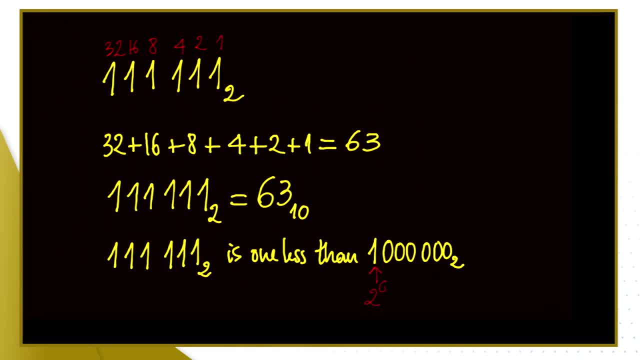 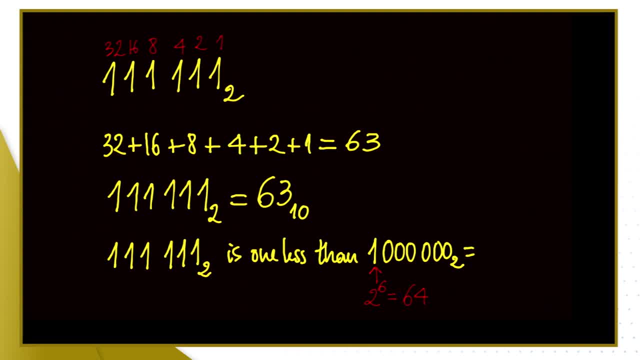 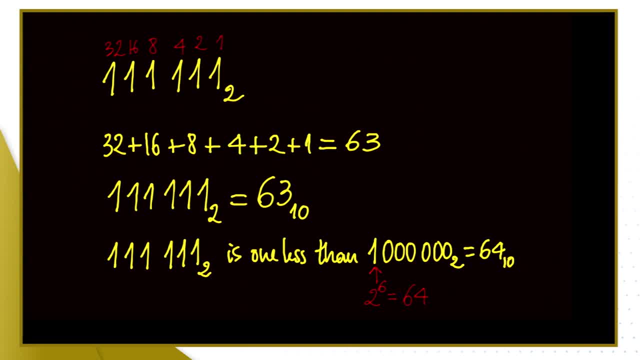 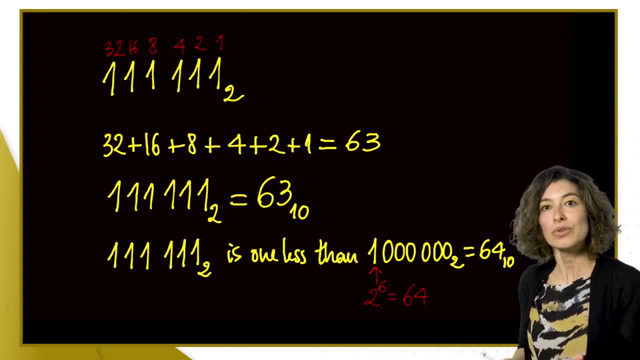 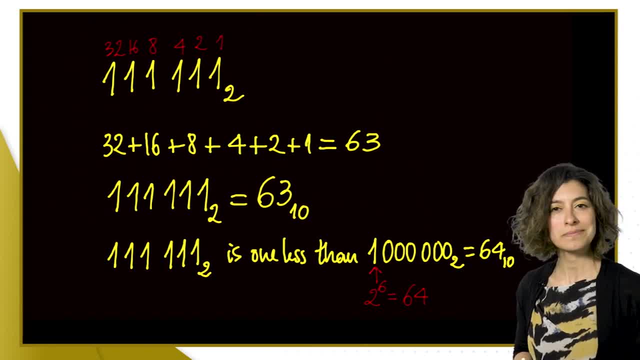 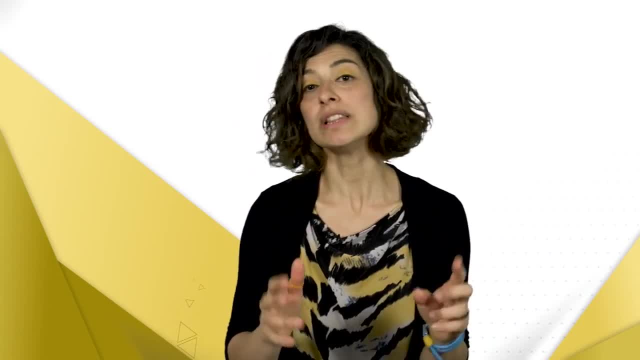 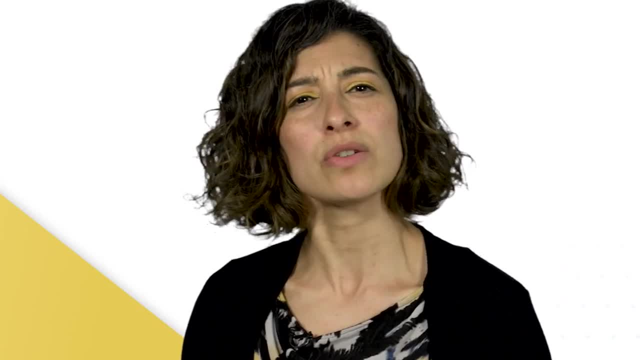 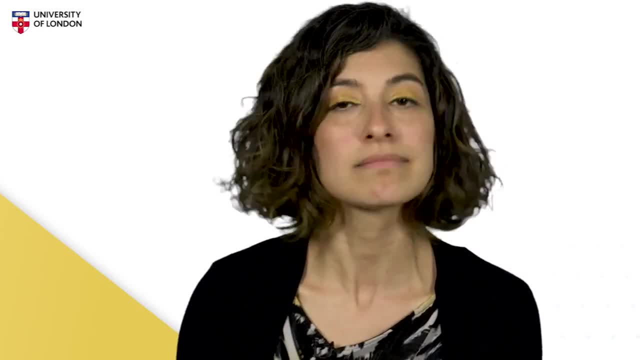 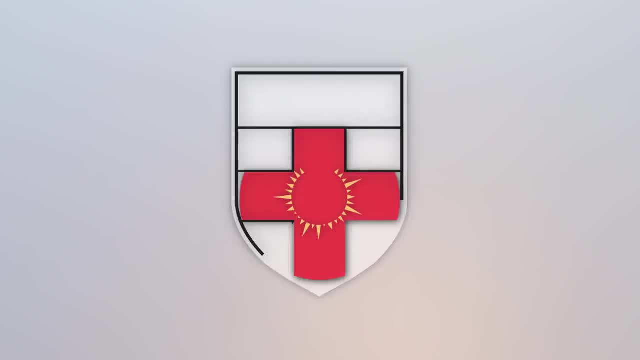 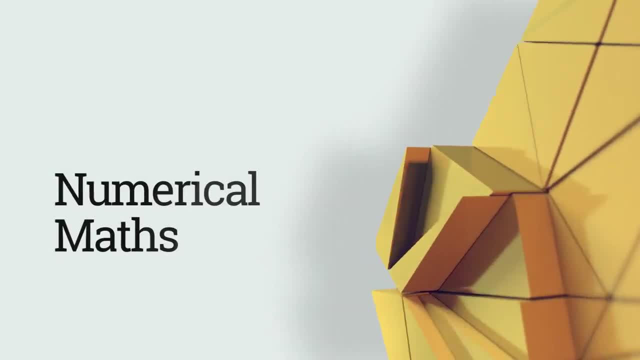 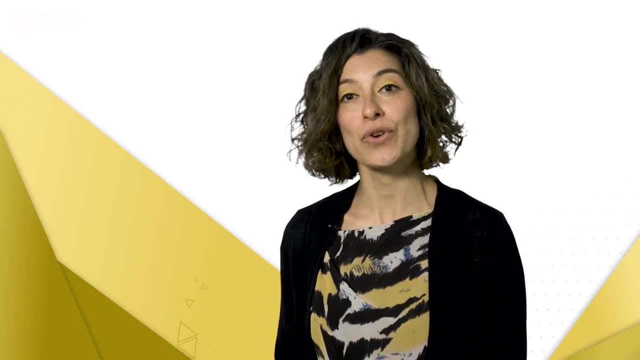 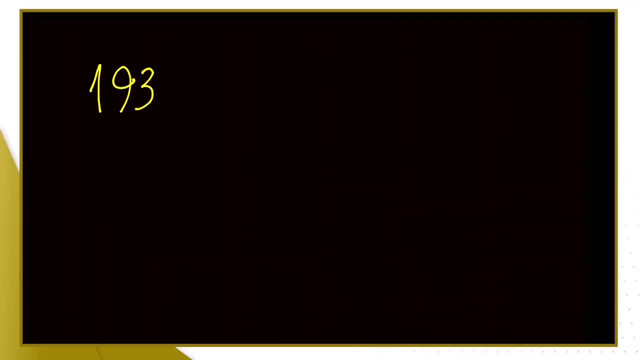 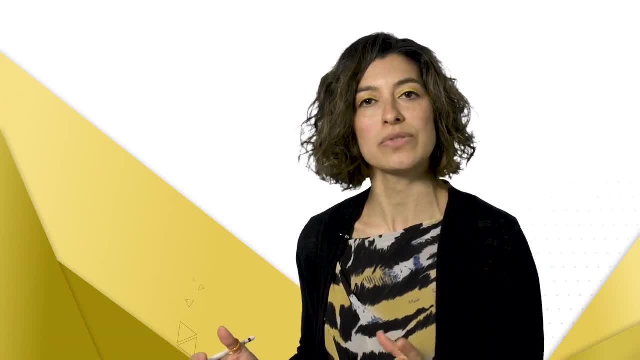 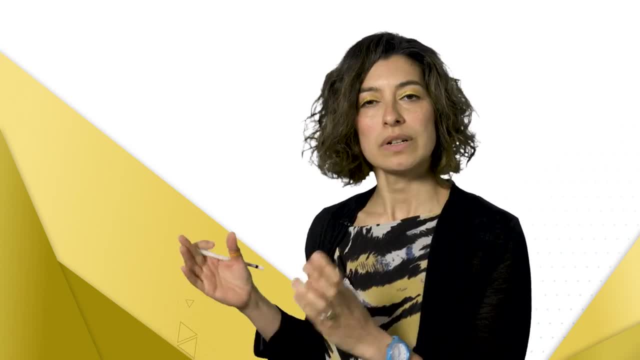 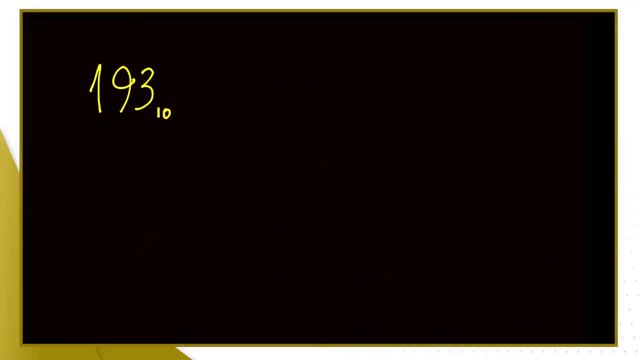 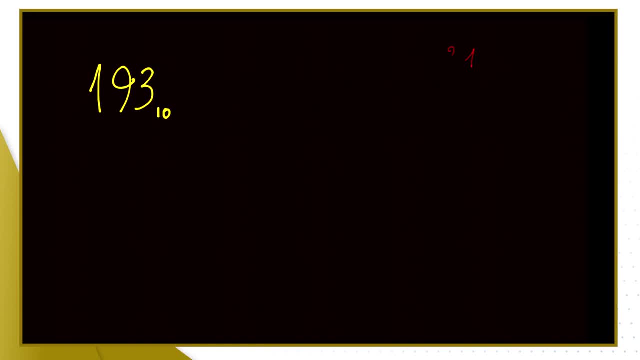 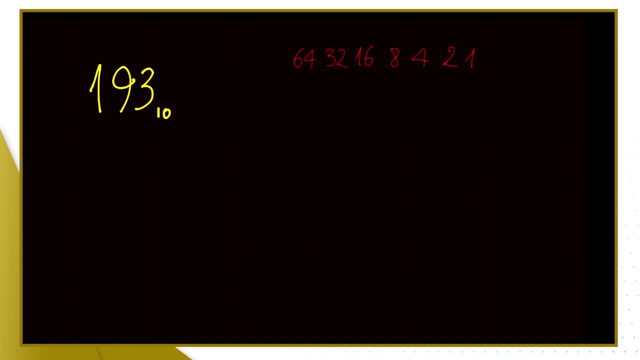 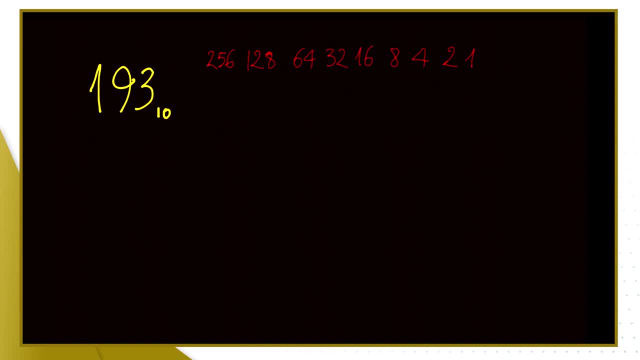 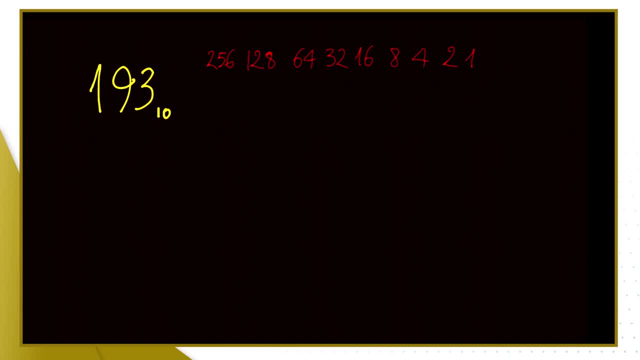 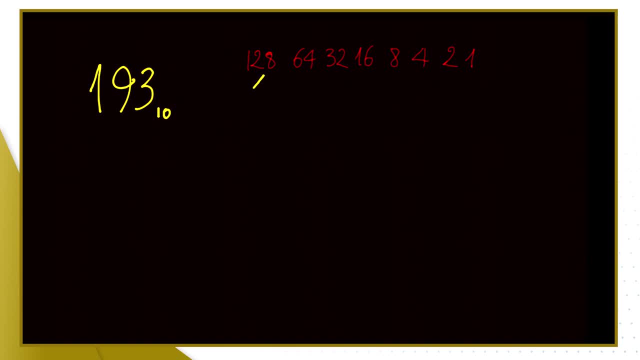 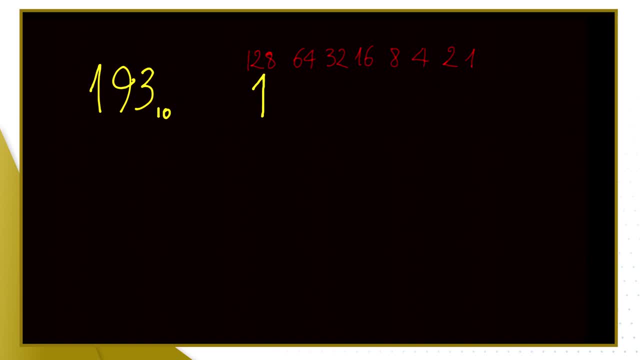 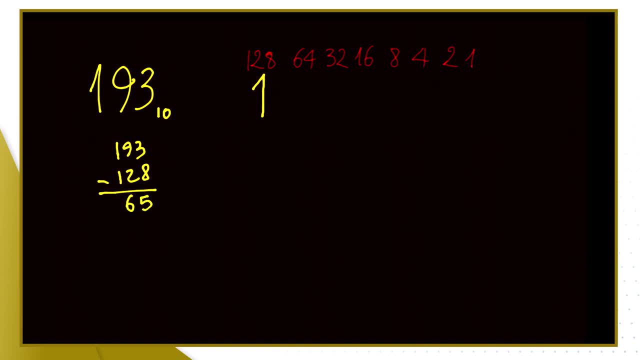 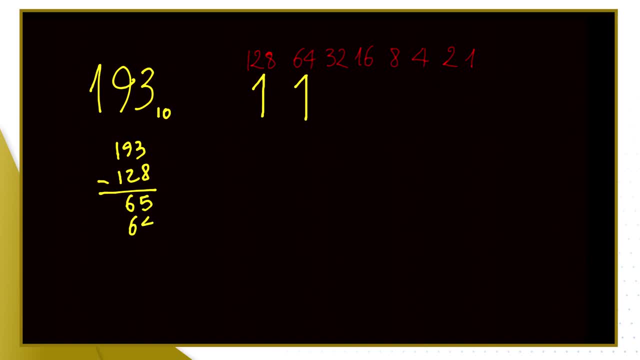 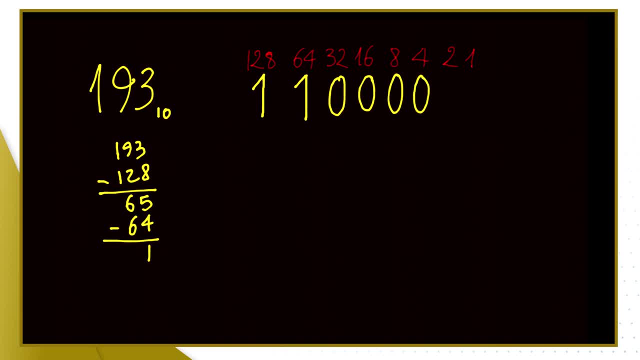 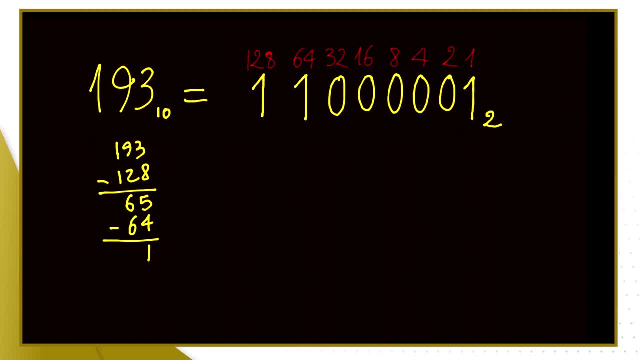 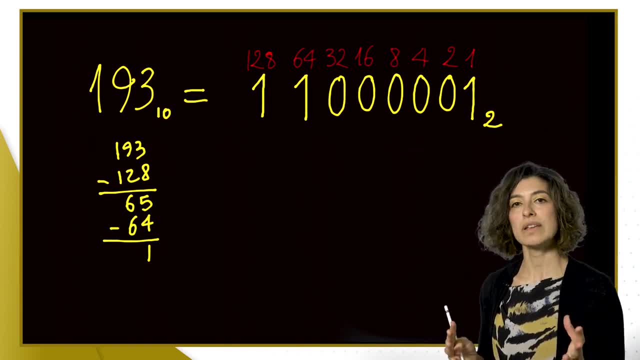 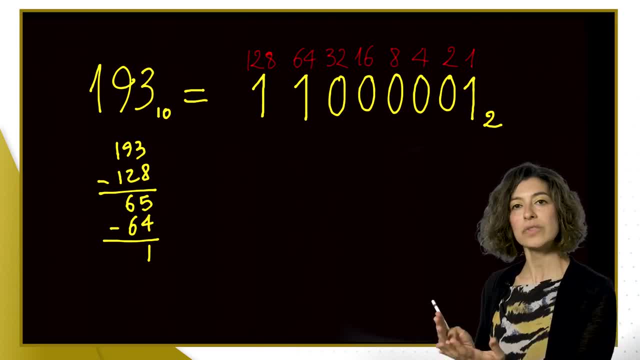 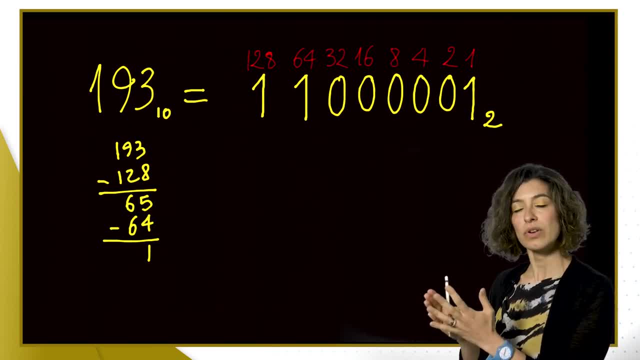 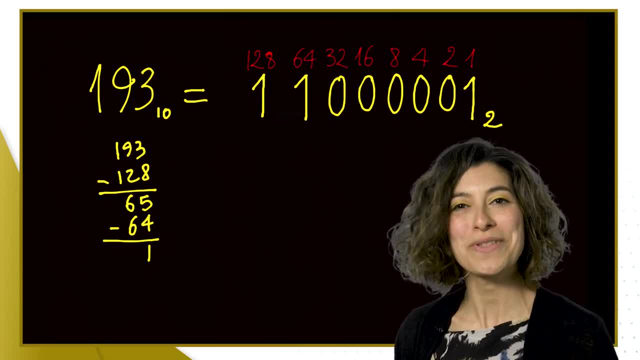 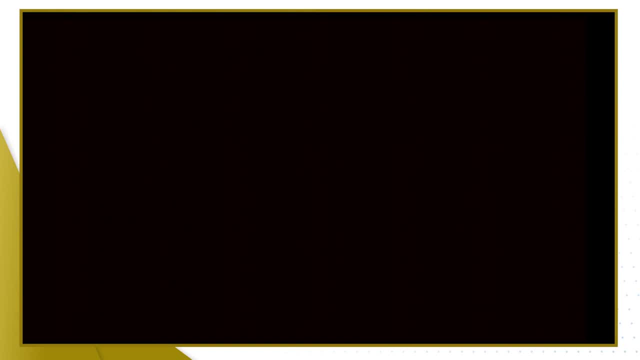 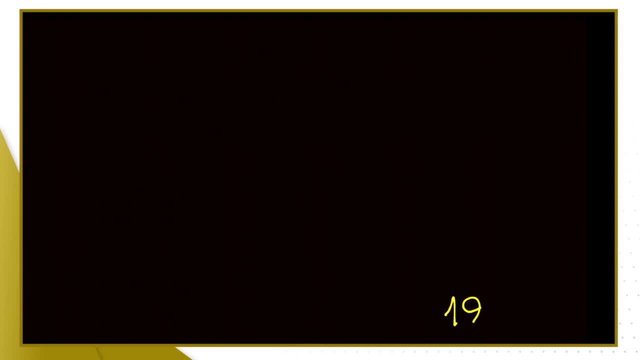 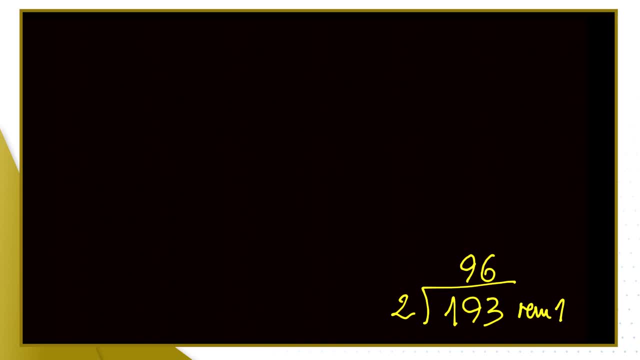 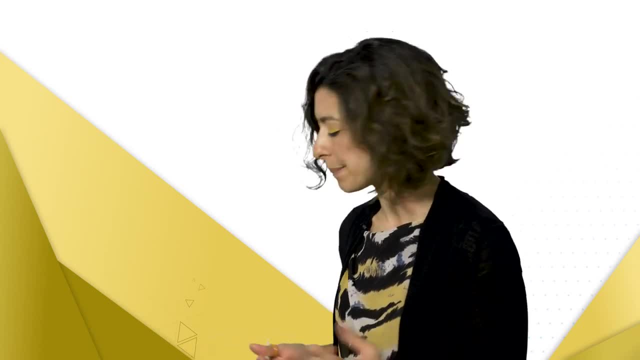 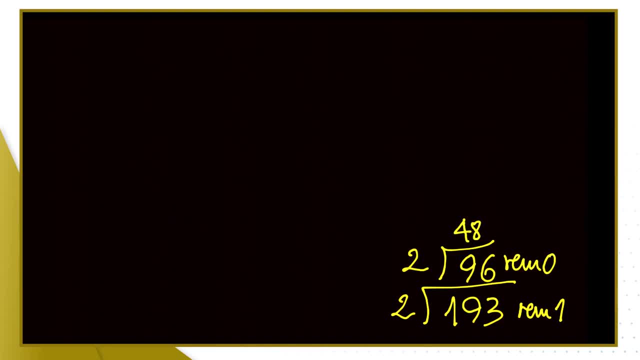 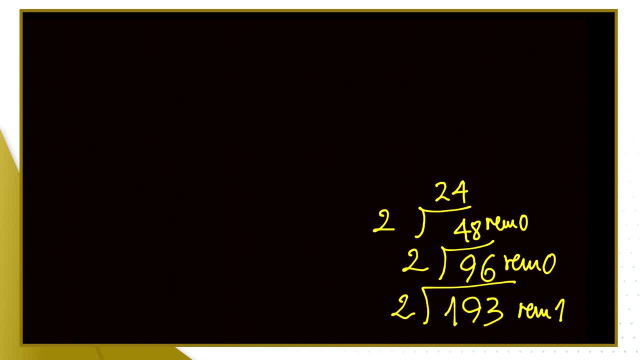 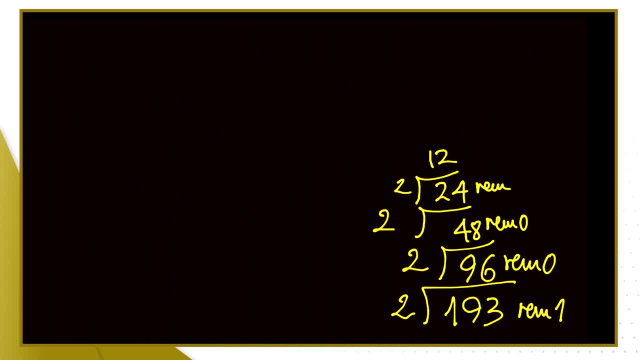 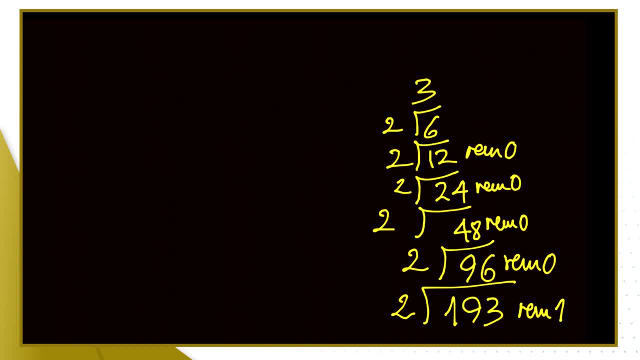 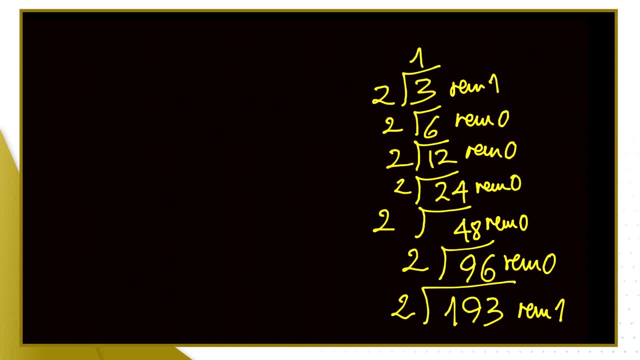 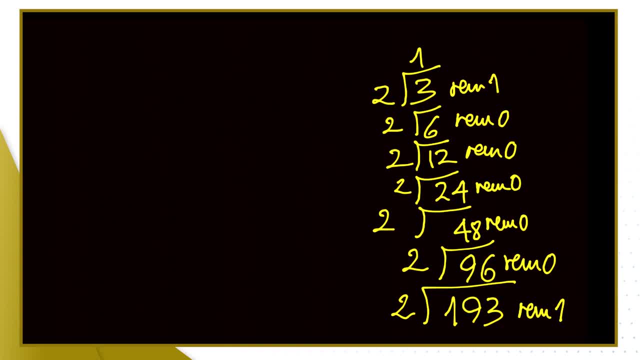 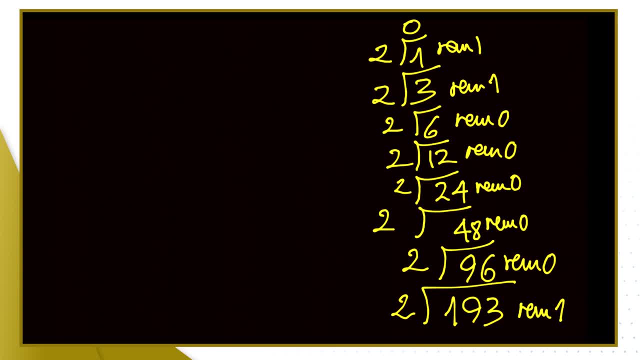 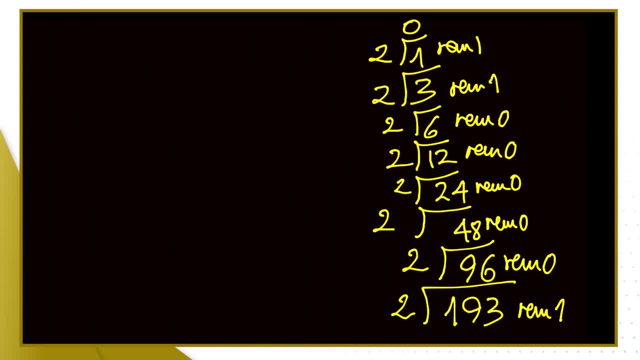 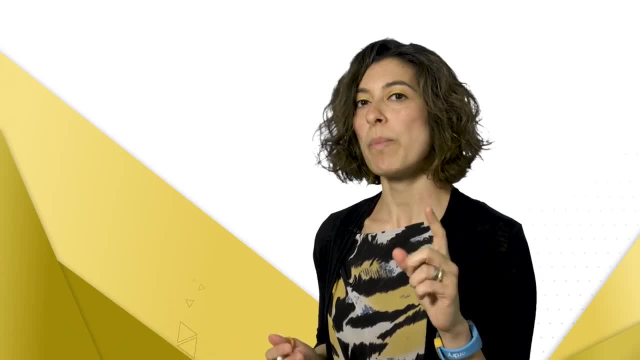 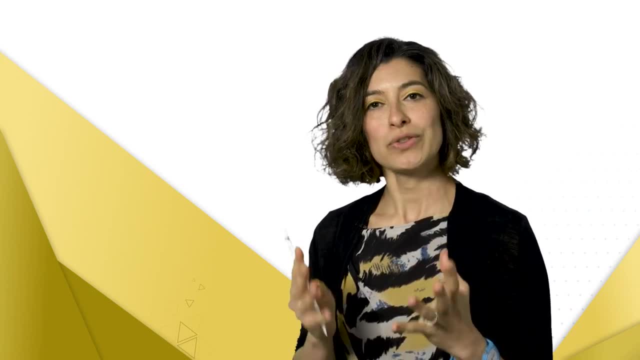 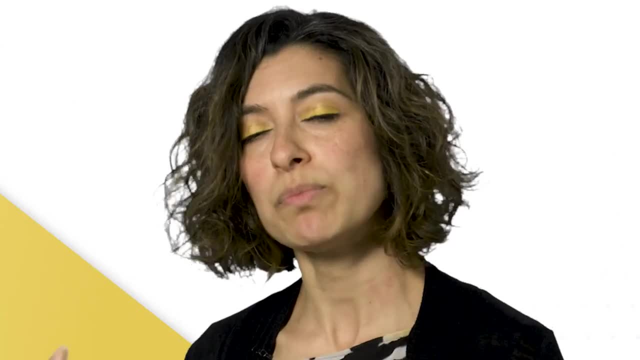 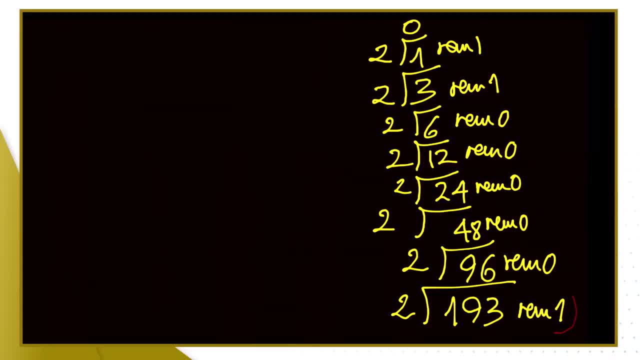 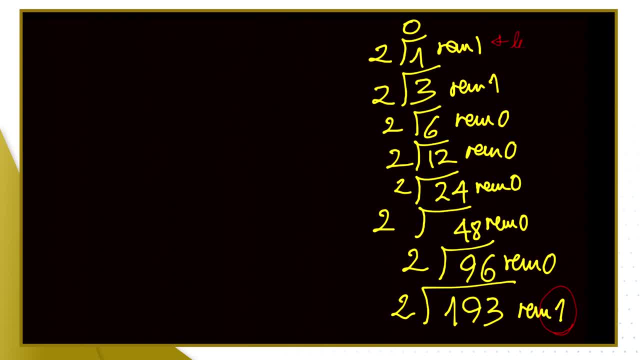 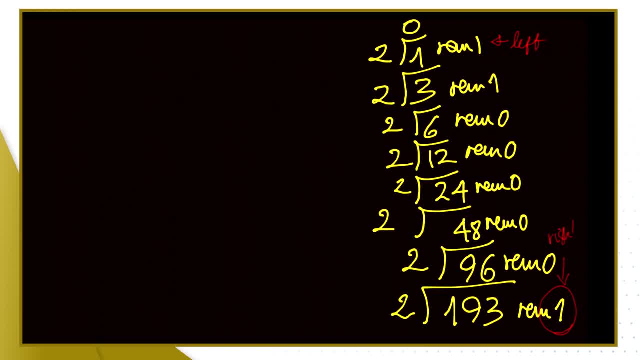 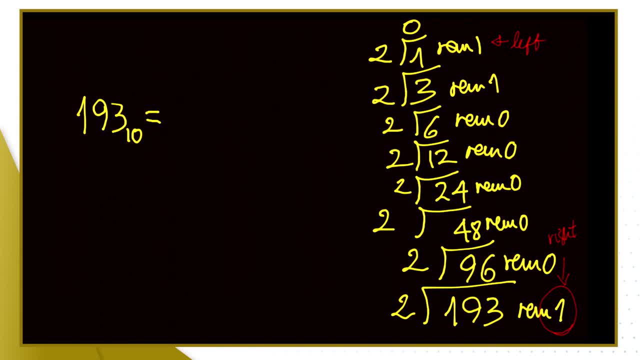 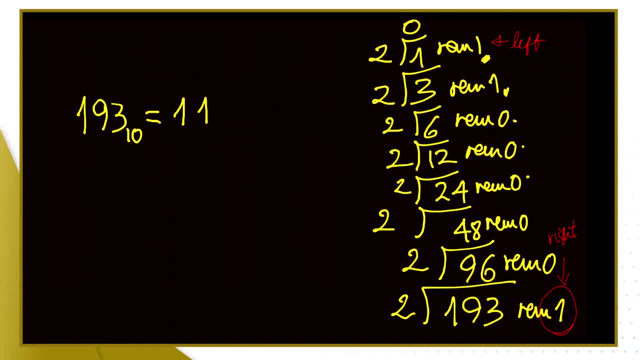 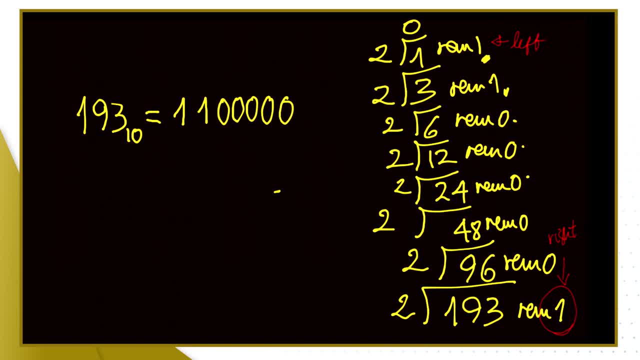 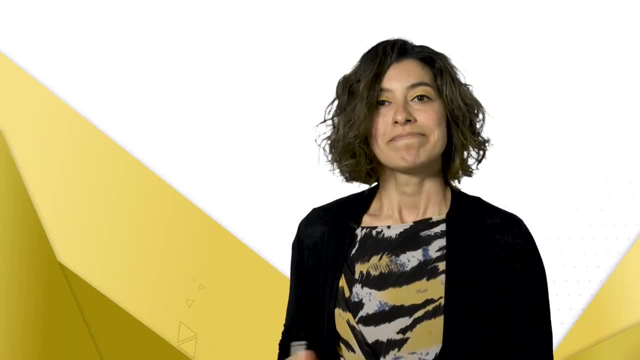 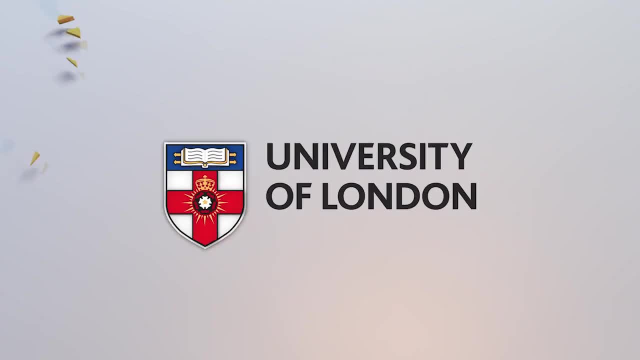 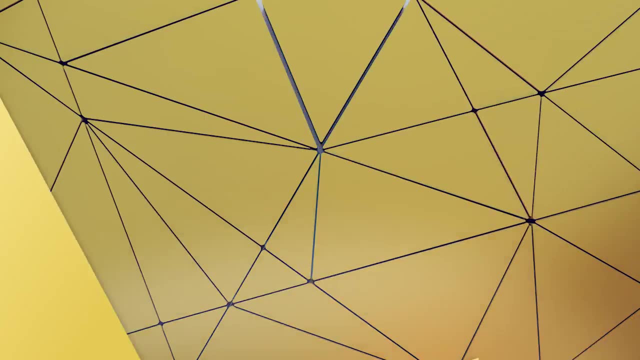 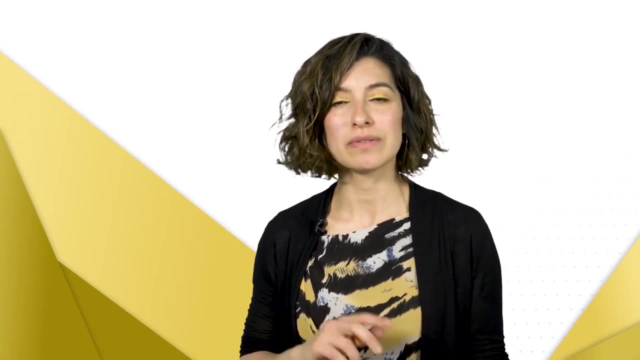 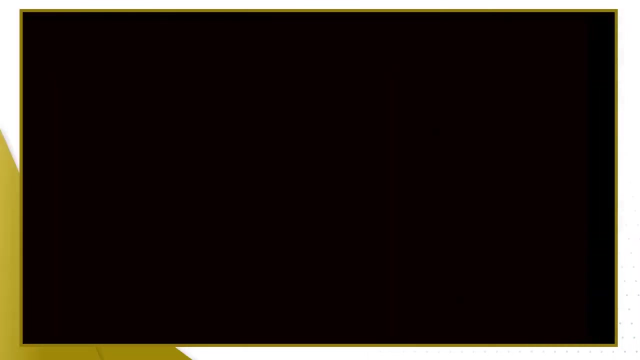 Subtitles by the Amaraorg community. You've worked with integers in binary and decimal to and fro. We're going to look at numbers that aren't integers. numbers with a fractional part, Say we've got 1101.101,. that's what I mean by fractional part. 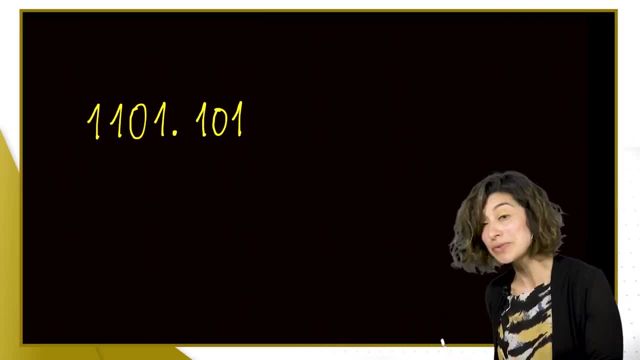 There is a point which we usually call a decimal point, but it's not a decimal point because we're working in binary, the fractional point, And these guys over here are the non-integer part. Now, what's their place value? What are they worth? 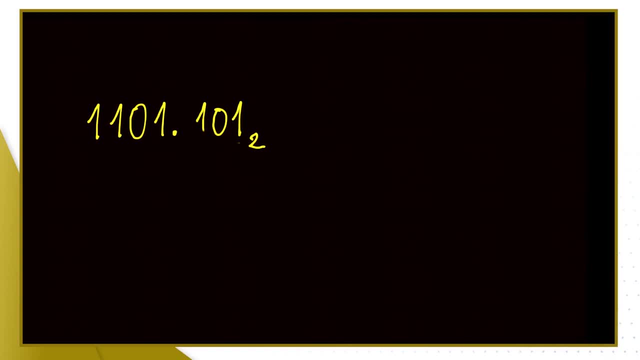 Similarly to what we did with the integer part, we're going to write the place values above the digits. So we've got 1,, 2,, 4, and 8.. And the way we work those out, we start in 1,, we double, double, doubled. 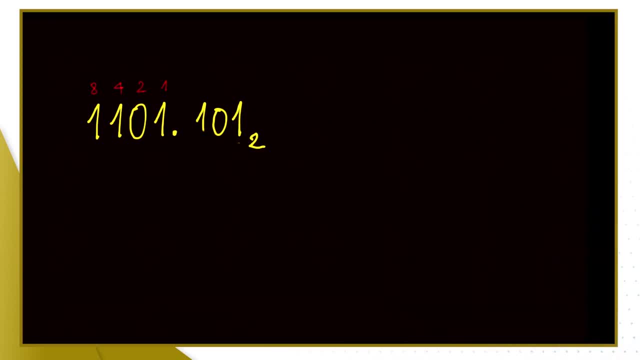 To go into the fractional part, we're going to divide by 2 every time. So 1 divided by 2, we've got a half, which is 0.5, and then we've got 0.25, and we've 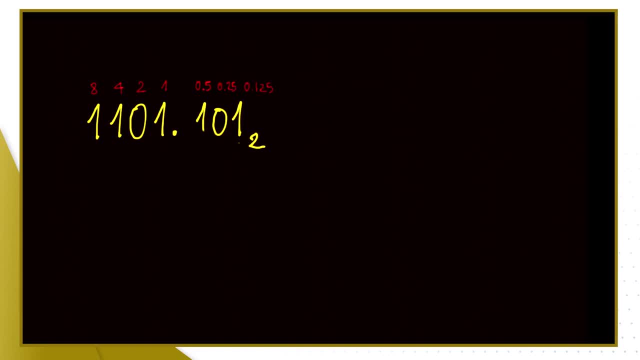 got 0.125.. We can write these as fractions, which I'm going to write above it, and I encourage you to do so. That's a half, that's a quarter and that's an eighth. We can write it as well as powers of 2.. 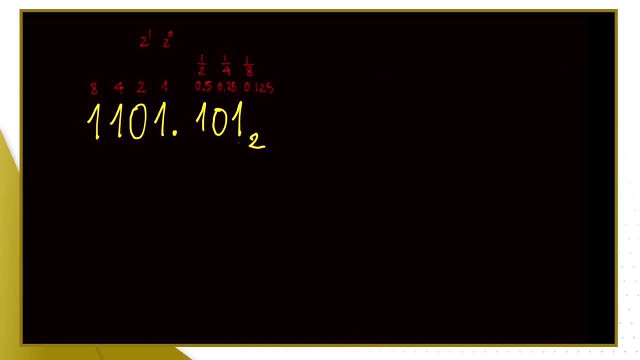 Let's do it: 2 to the 0 there, 2 to the 1,, 2 to the 2,, 2 to the 3, and 2 to the minus 1,, 2 to the minus 2,, 2 to the minus 3.. 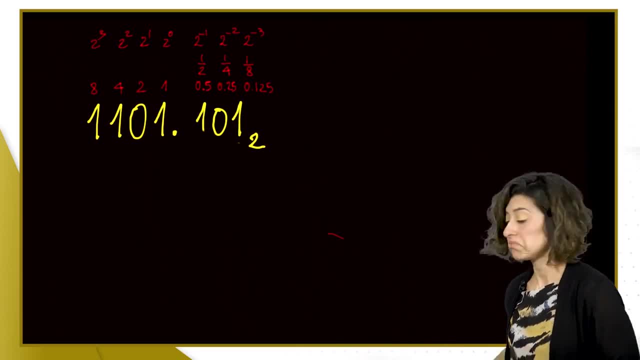 Now, how do we now calculate this number into decimal? As before, when you've got a 1, you add the place value. When you've got a 0, just ignore it. Let's do it. I'm going to add up the place values that have a 1.. 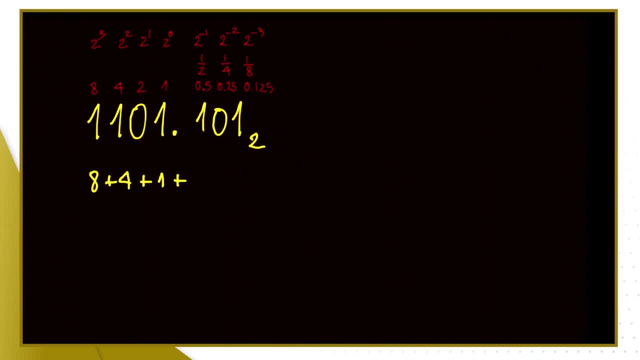 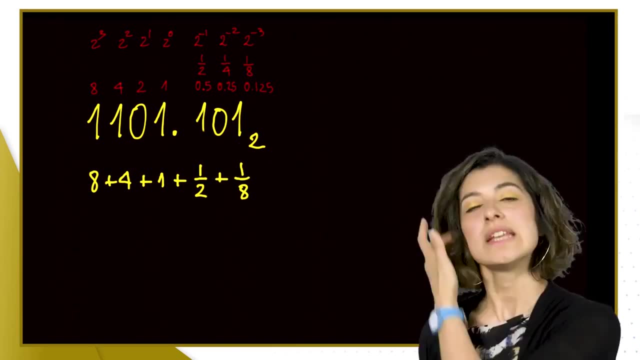 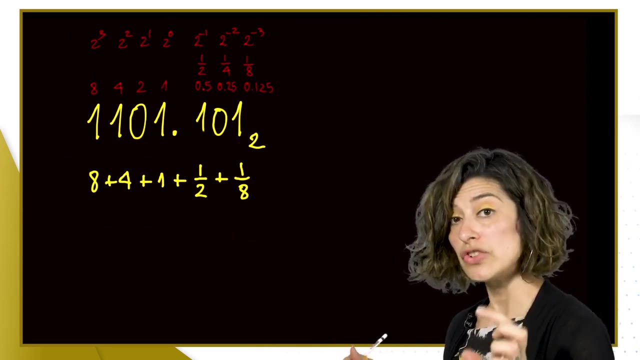 So 8 plus 4 plus 1, plus the half and plus the 1 eighth. Because we want this written in decimal and we want the decimal expansion with a fractional part, let's add up as digital expansion of the numbers. So we've got 8 plus 4 plus 1.. 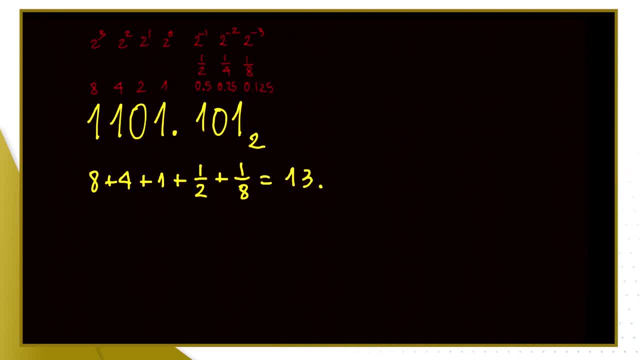 We've got 13.. And then we've got a 1 half, which is 0.5, and 1 eighth, which was 0.125.. And that adds up to 13.625, and that is 1, 1, 0, 1, 0.101 in binary. 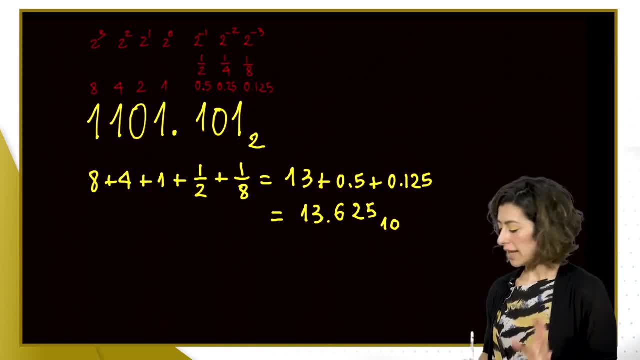 Now just reminding you again that in place value the fractional part, so this number in decimal, 13.62.. That's a half 0.625,. I will never say 13.625, never, unless I want to refer to 625 thousandths. 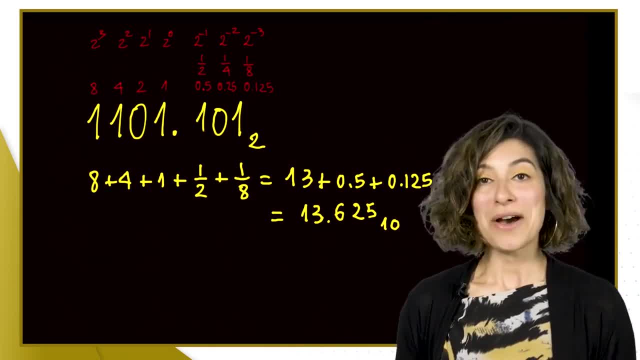 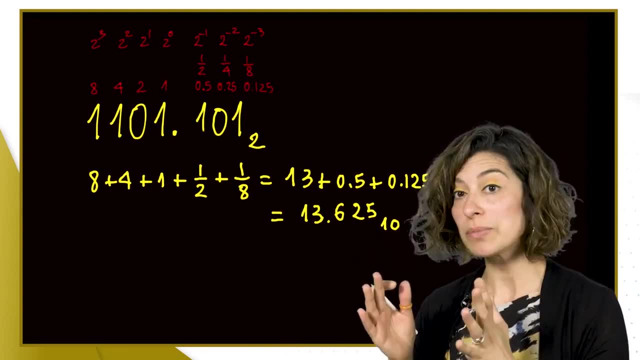 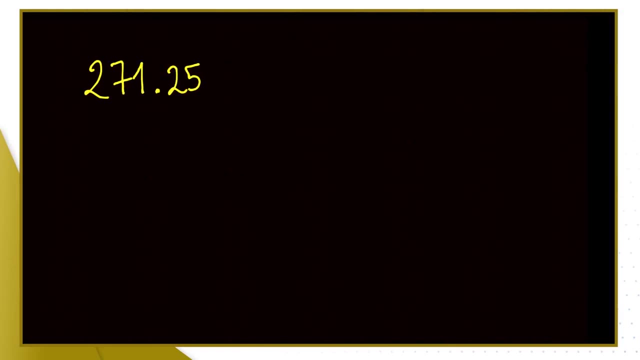 But let's simply call it 13.625.. Now that was binary to decimal. for fractional numbers, Let's do the other way around. Let's do from decimal to binary. Say, my number is 271.25.. That's my decimal number. 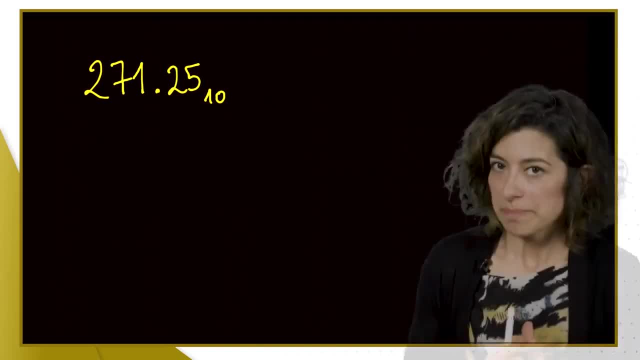 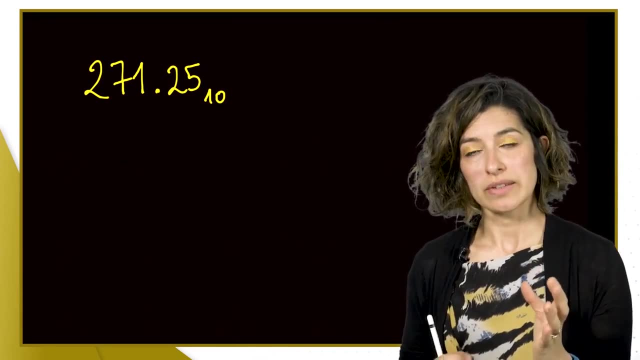 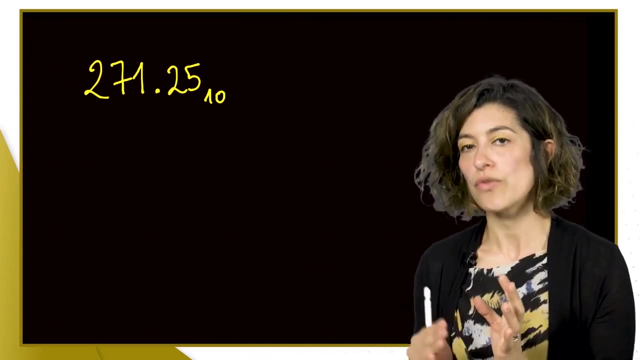 I've got to write this in binary. Here's the algorithm For the integer part. you've seen that we divide by 2 and keep note of the remainders. That's how we transform an integer number from decimal to binary. You divide by 2, over and over again. When you have a fractional part of the number, we're not going to divide by 2.. We're going to multiply by 2, and, instead of taking the remainder, we're going to take the integer part of that result. We're going to multiply by 2, and instead of taking the remainder, we're going to take. 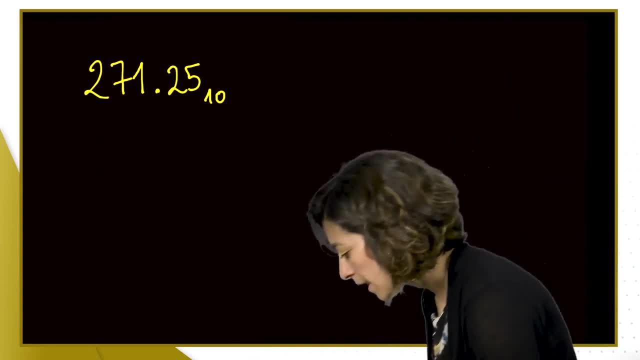 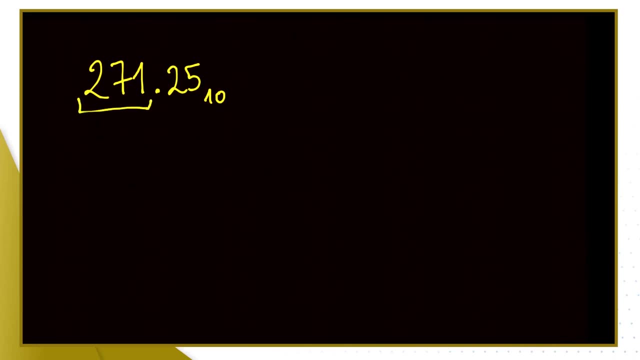 the integer part of that result I'll show you. So this number 271.25, the 271, you know how to do that one in binary, so I'm going to ignore it for now. I'm going to focus on writing the 0.25, writing that in binary. 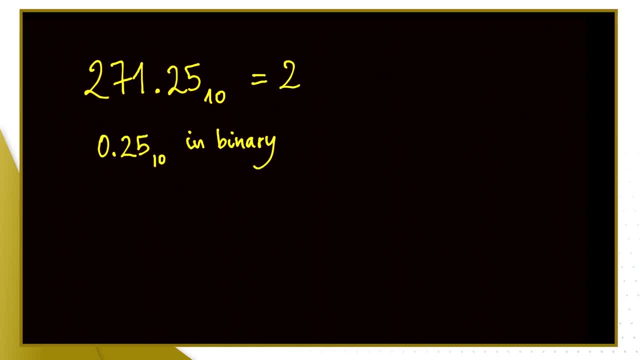 So in other words, we always separate the number into integer plus fractional, And we have two separate algorithms for that. So for 0.25, I will consecutively multiply by 2.. Now, 0.25 times 2 is 0.5.. 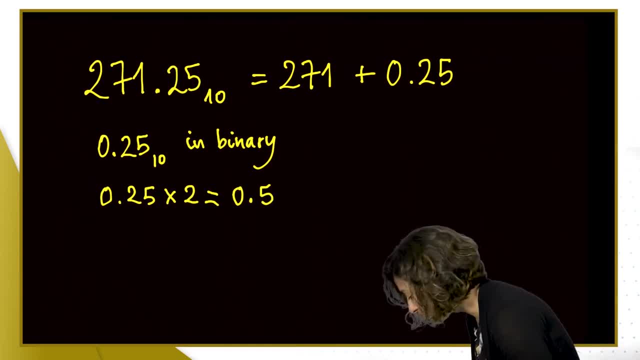 The integer part is 0.. So that integer part 0, is my first fractional digit. So that is going to be 0.0.. That's the first digit Did just now. Now I look at what I've done. 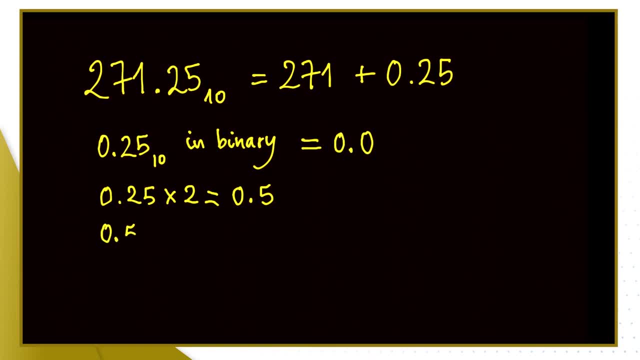 I look at what's left. So 0.5 times by 2 again I get 1. And 1, the integer part is 1, so that is going to be my next digit that appears there, And the next thing to do is to take away that integer part and see what's left. 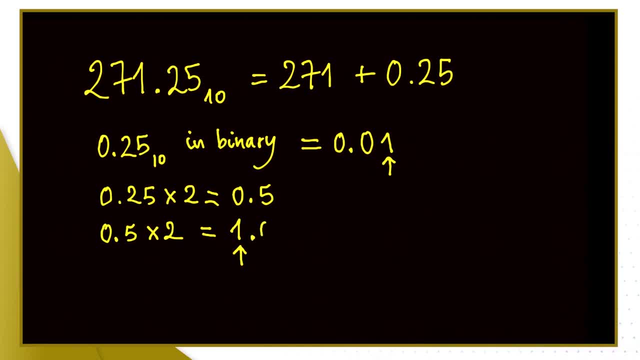 Well, in this case there's nothing left, because 1 is the same as 1.000000.. So when you take away the 1, all you have is 0. So you would finish the algorithm there. So we stop, as the result is an integer. 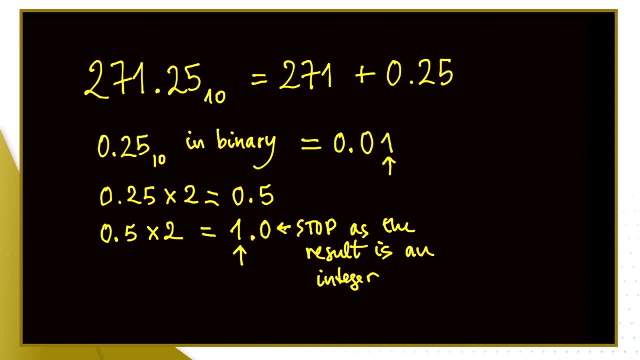 That means that 0.25 is 0.01 in binary, which is not very surprising if you think about the place value. The place value for that 0 is 1.5.. The place value for that 0 is 1.5.. 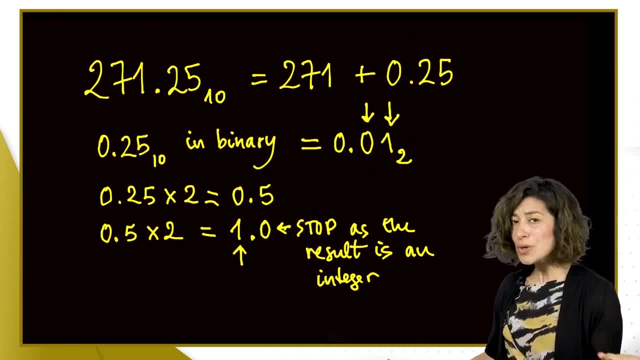 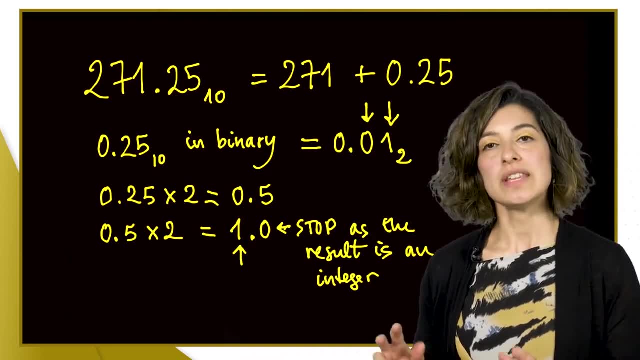 The place value for that 0 is 1.5.. The place value for that 1 is 1.25.. And 1.25 is 0.25.. So, bang on, it's correct. We've calculated the fractional part of this number in binary. 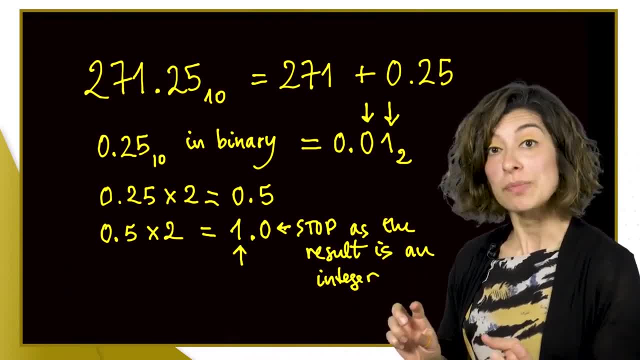 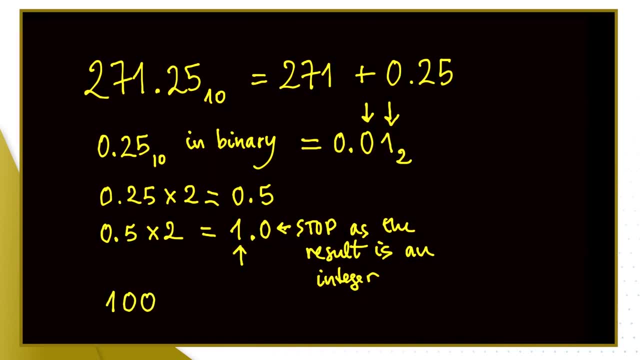 Let's now put it together with the binary translation of the integer part. So 271 is 1, 0, 0, 0, 0, 1, 1, 1, 1, which I haven't calculated. 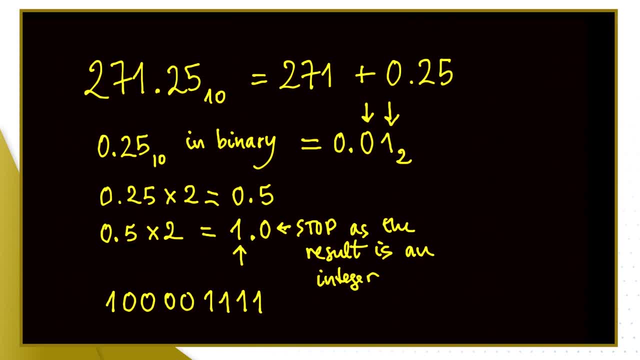 Here, but you now know how to calculate. So that is 271 into binary And then dot the 0, 1 that we calculated here for the fractional part, So that in binary is 271, 2, 5.. Just to recap: we separate the integer part and the fractional part of the number. 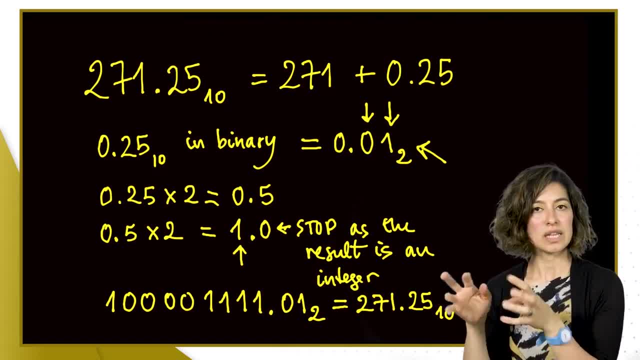 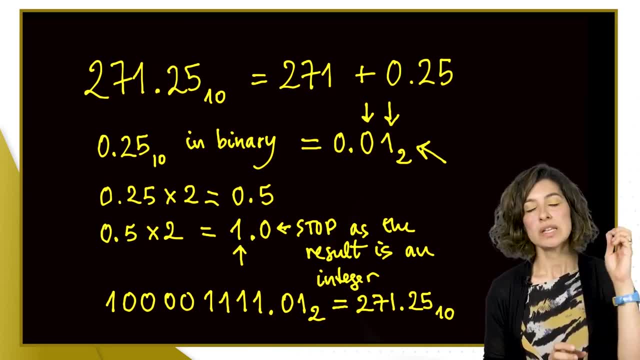 Use the division algorithm to calculate the integer part into binary. For the fractional part, which is the new bit we've done here, you keep multiplying by 2. Take the integer part of that result as your binary digit And keep doubling what's left over and over again. 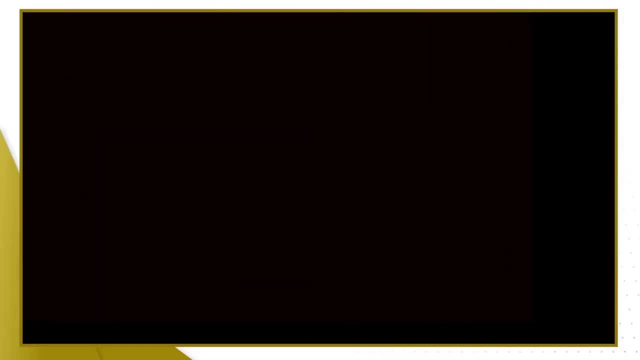 Let's just do one more example. Say our number is now 0.75.. That's a number, a decimal number, fractional. How do we do this into binary Once again? we take the number, we double it, And 0.75 times 2 is 1.5.. 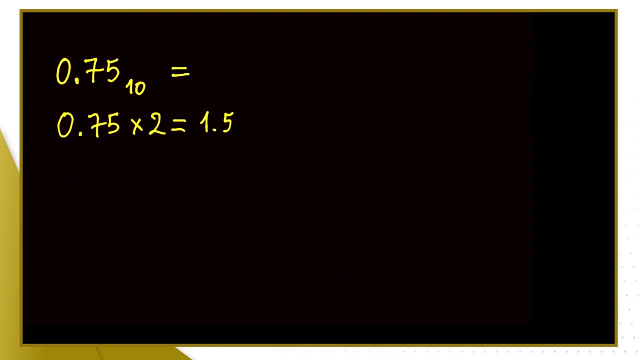 The integer part of this result is 1.. So that's the first fractional digit, that's 1.. Now I'm going to take away that integer part, So that's 1.5.. I'm going to take away the integer part, which is just the fractional part, 0.5.. 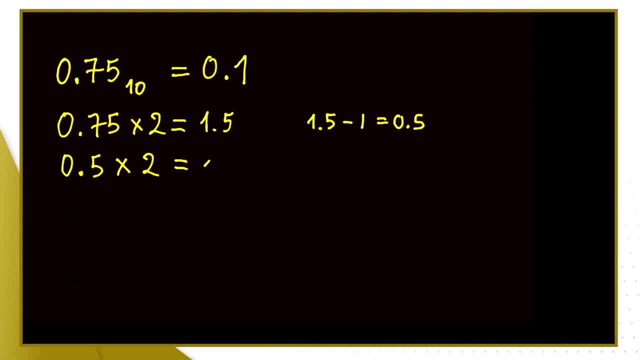 And I will double that 0.5.. That gives me 1.. So that's the other digit, And again we don't have any more fractional part left. So this is an integer Stop. So we stop, And therefore 0.75.. 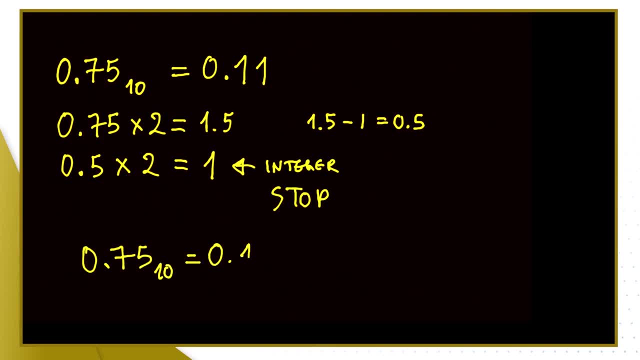 0.75.. 0.25 is written as 0.11 in binary And, looking at the place value, each of these ones corresponds to the fractional place values of 1.5 and 1.25.. And 1.5 plus 1.25 is 0.5 plus 0.25, which is 0.75.. 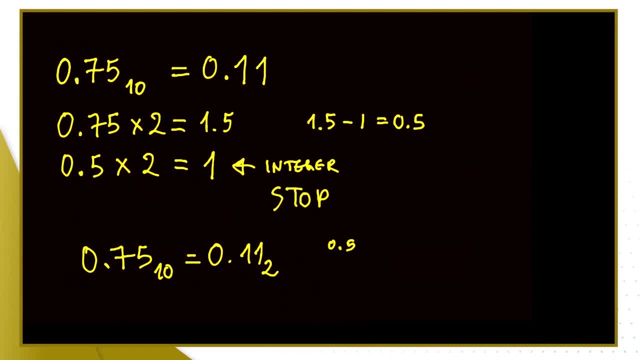 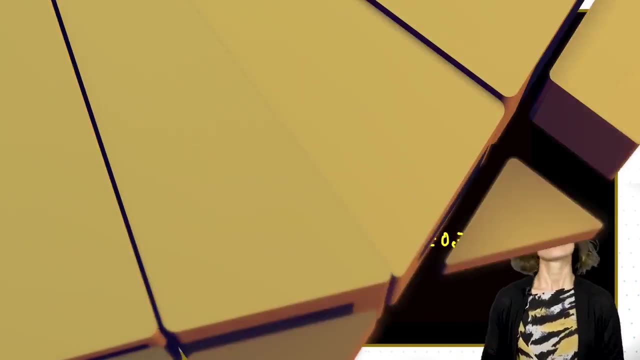 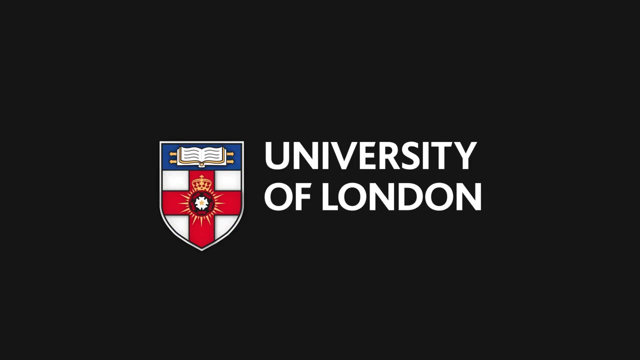 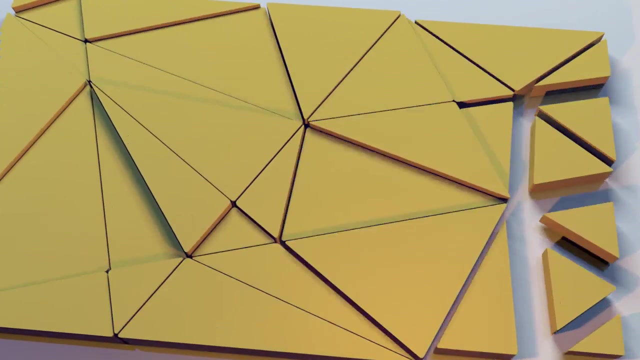 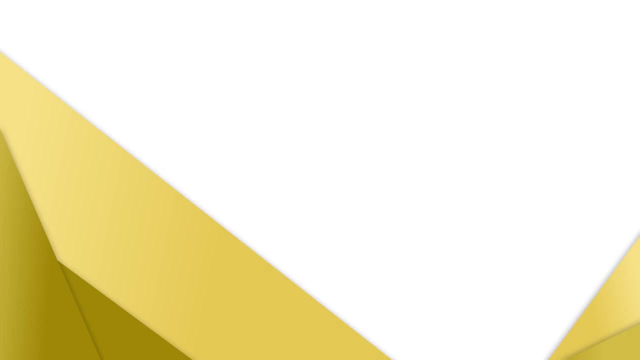 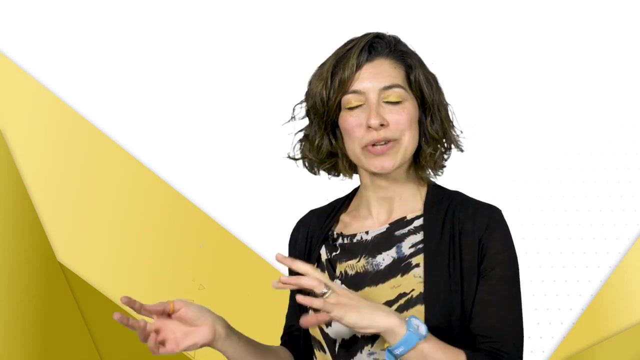 So it all adds up. So 0.5 add with 0.25 is 0.75.. Just to double check that we make sense of the calculations and the results we obtained, We looked at fractional numbers and how we translate between binary and decimal for those. 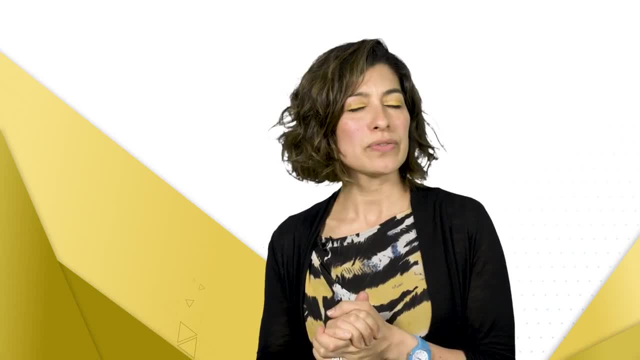 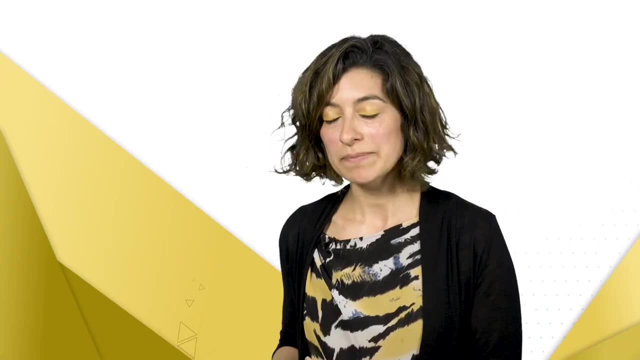 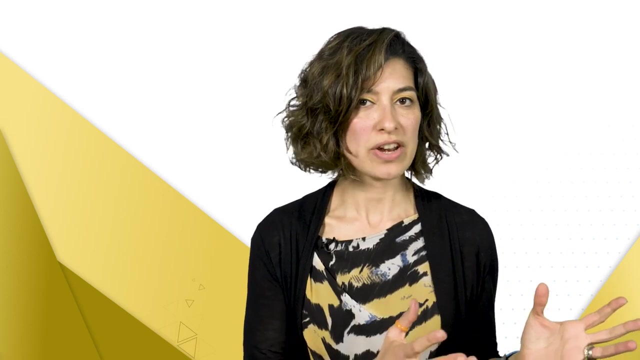 types of numbers. You may have asked yourself: are there more types of numbers than the fractional numbers we saw just before? There are mainly two types. You have the numbers that are rational and numbers that are irrational. I'll show you what I mean. 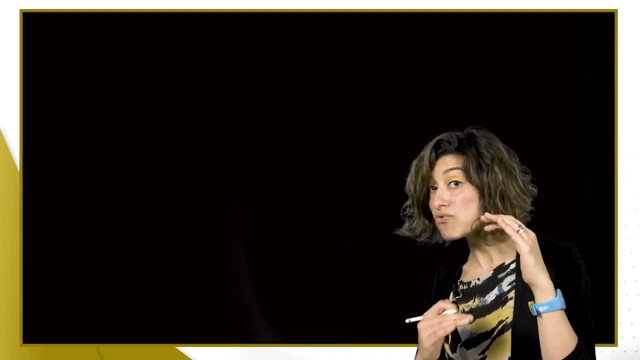 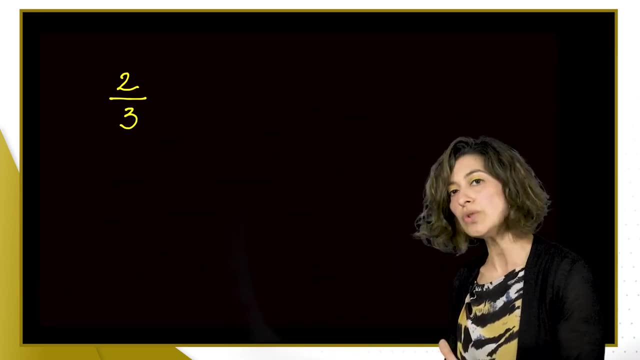 A rational number is a. It is a number that can be written as a ratio, So something like a fraction, like two-thirds. it is a rational number because the two numbers I'm using in this fraction are integers. The two is an integer, the three is an integer. 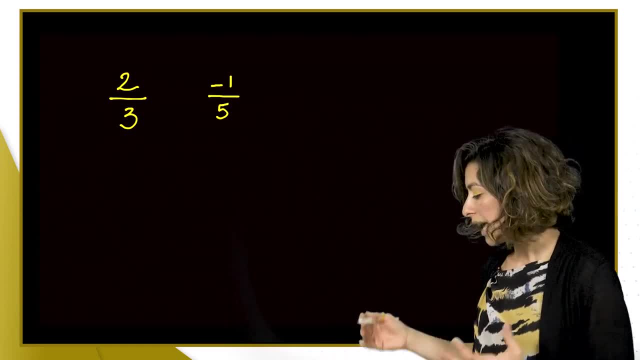 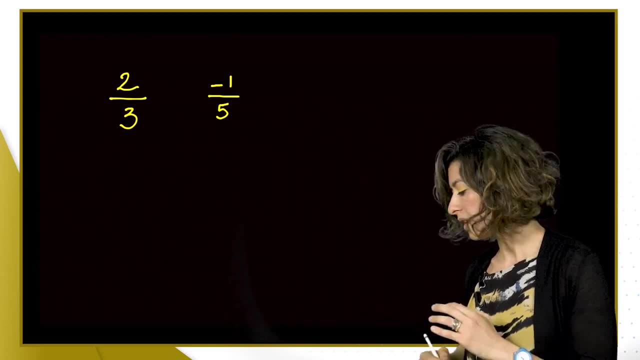 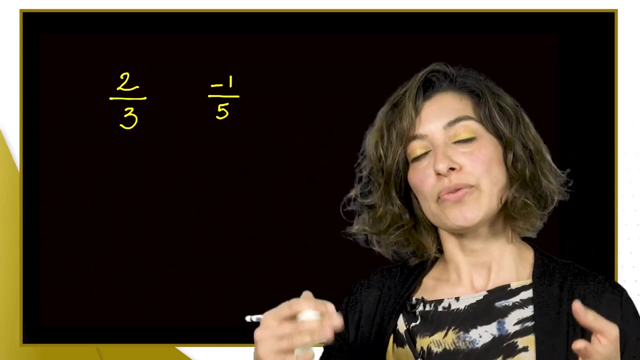 Minus one-fifth is also a rational number And traditionally we write: if the number is negative, the top number, the numerator, will be negative and we keep the denominator, the bottom number, positive. They are written as fractions, but of course every fraction can be written in a digital. 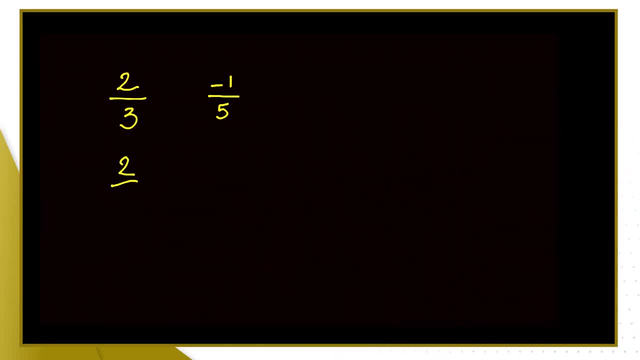 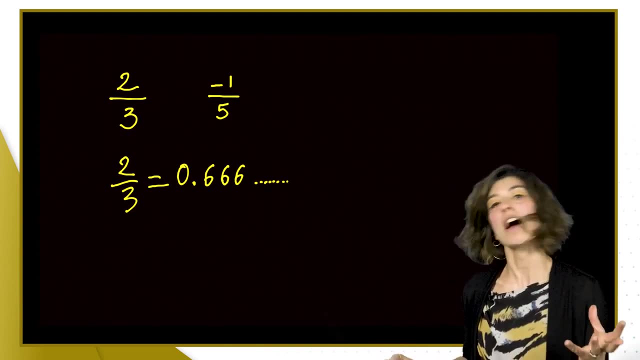 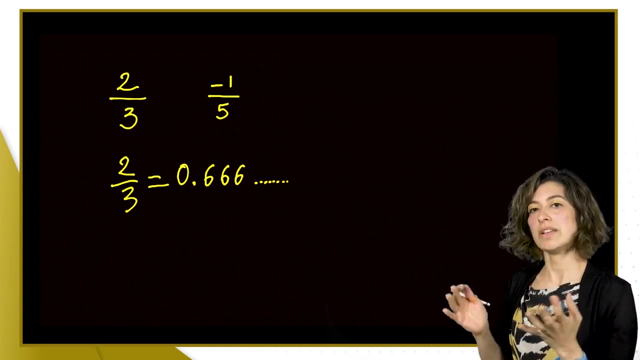 expansion. So two-thirds is zero point six, six, six and so on. It's a recurring decimal, we call it. The digital expansion of this number has a pattern that is repeated, is a six that repeats over and over again. 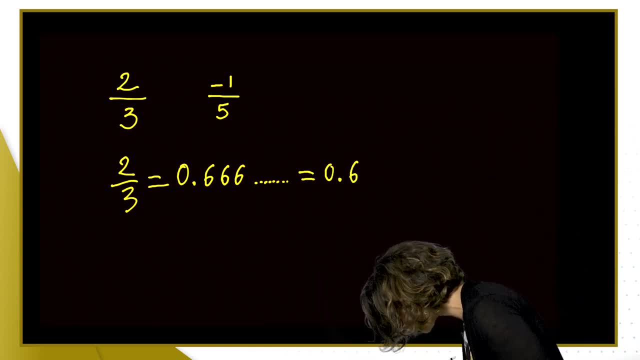 So we write this as zero point six over and over again. So we write this as zero point six over and over again, With that dot on top that says: I repeat the six to infinity. The minus one-fifth is minus zero point two. 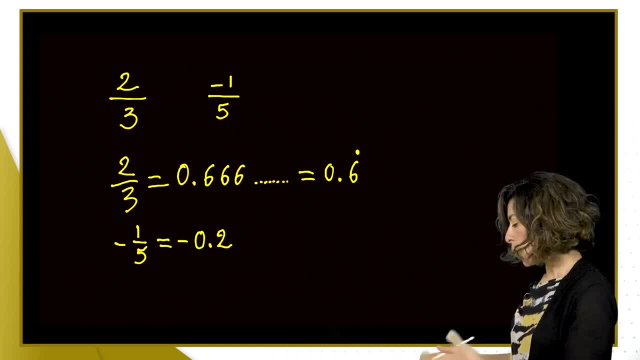 They're both rational numbers. they both have a digital expansion. One of them has a repeating digital expansion, the other a finite expansion. So this is finite And this is repeating. The cool thing is every fraction, every rational number, when you write it down as 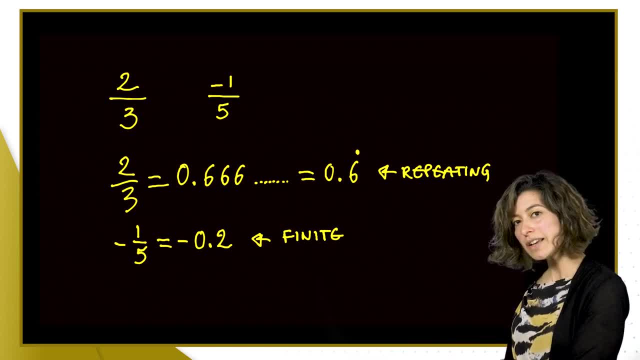 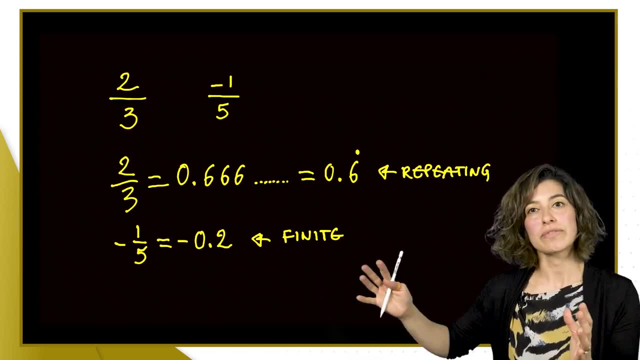 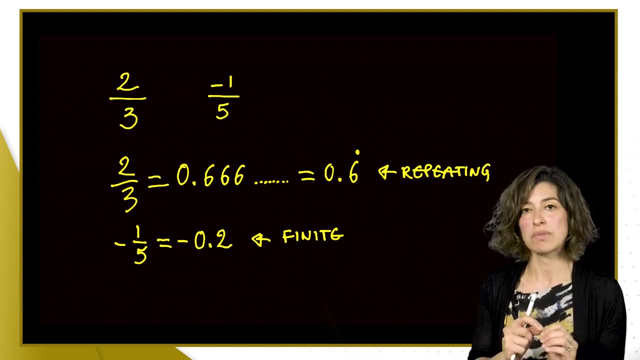 a digital expansion. you either have a finite expansion or a repeating expansion, That's it. If the number you're working with goes on forever without a repeating pattern, then it is an irrational number And that means it cannot be written. It cannot be written as a nice fraction with integer numbers. 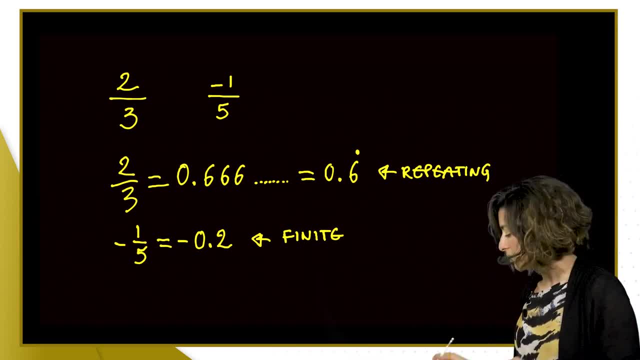 It cannot. And examples of that number. you are familiar with numbers like root two, the square root of two and any number with a root, even numbers that you probably came across as pi, e and so on. lots of constants, numbers that cannot be written as a fraction. 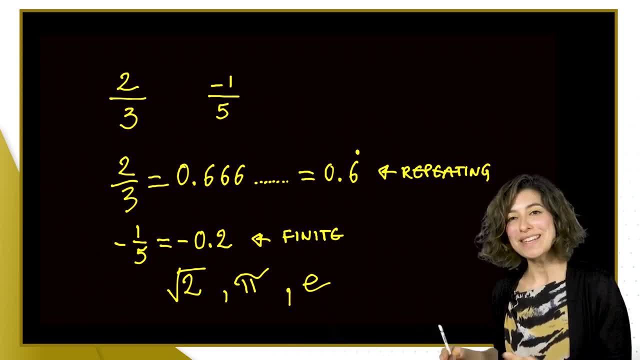 Now the point of this is: in binary, you will also meet digital expansions that are finite or recurring, And I'm just going to show you how to do that. And I'm just going to show you how to do that, But you should also look at one example here, so that you are familiar with what happens. 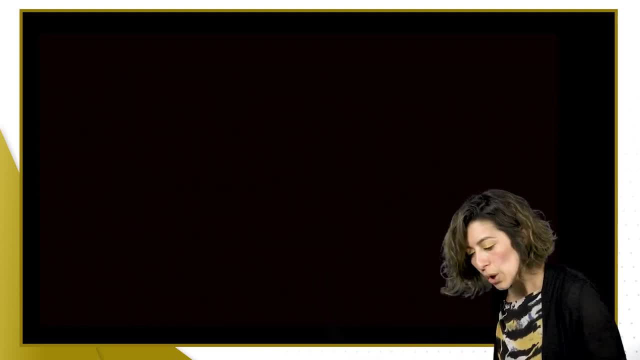 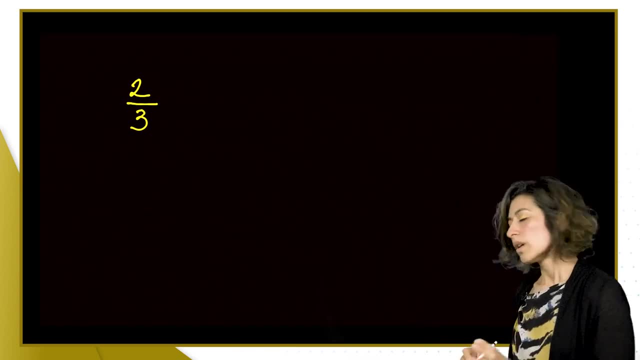 when you meet such a number. So, going back to the number, two thirds, I want to write this in binary. OK, So we already know that the number is 0.6, recurring in decimal. In binary, we can approach it in several ways. 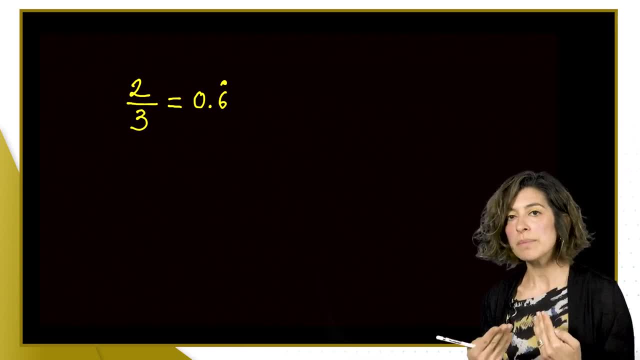 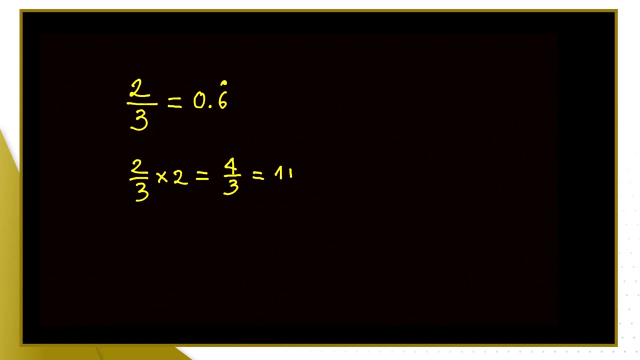 Remember the algorithm we just looked. You keep doubling the number and gather the integer part as the digit. That's what we're going to do. So 2 thirds times by 2, that is 4 thirds. 4 thirds is more than 1, that is 1 plus 1 third. The 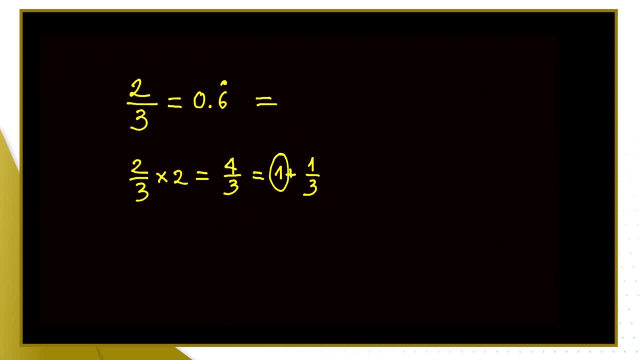 integer part is that one. so that is going to be the first binary digit. And now the 1 third is the fractional part. so we take the 1- 3rd, we times it by 2, and now I have 2 thirds, which is less than 1, so this is a number like zero. 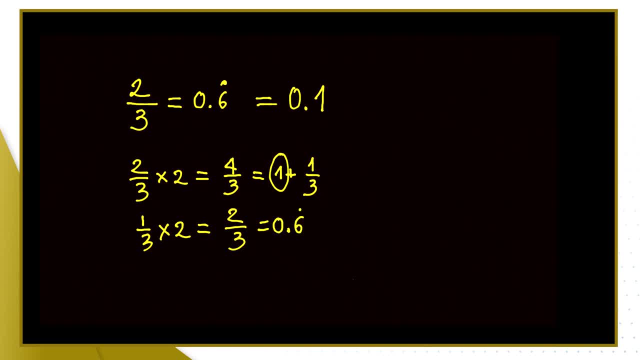 point, something we know: it's 0.6 recurring, so the integer part is the digit we're gonna put there. Now we would carry on doubling the number 0.6 recurring, which is our 2 thirds, and double. 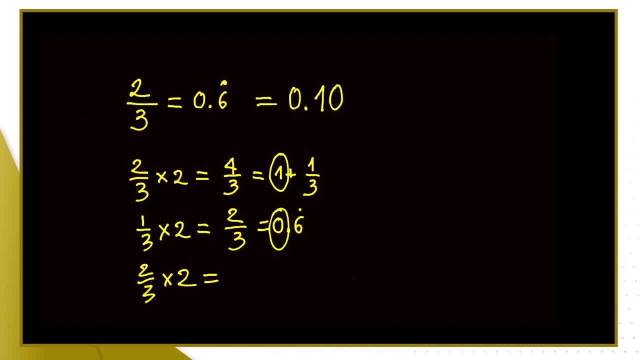 See, And hang on. we have seen this before because that's the first line of our calculation. So we are repeating, we're back there, we're on a loop. That means that if we carry on doing that calculation over and, over and over again, 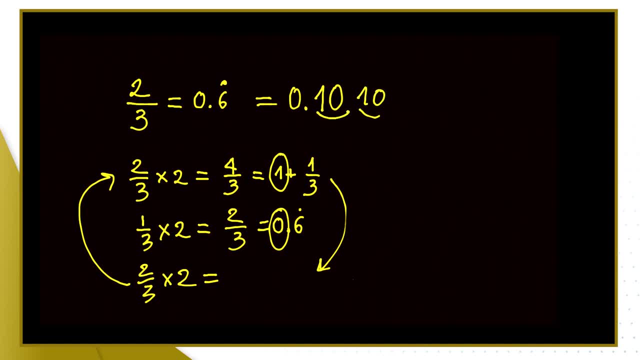 we're going to have that one zero repeated over and over again, forever. In other words, two thirds is written as a recurring digital expansion. in decimal, that's the 0.66666, or in binary, is 0.101010, repeating over and over again. 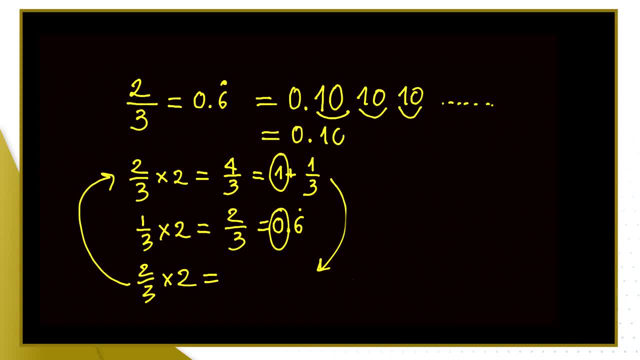 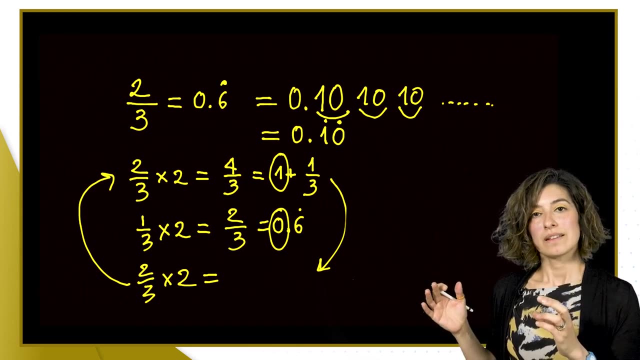 So I'm going to write this as 0.10, with a dot at the beginning of the period and a dot at the end of the period. So if you are working with a recurring digital expansion in binary, then you're going to have to carry on doing that calculation over and over again forever. 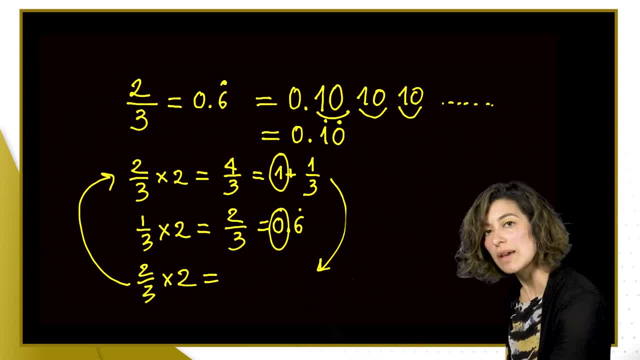 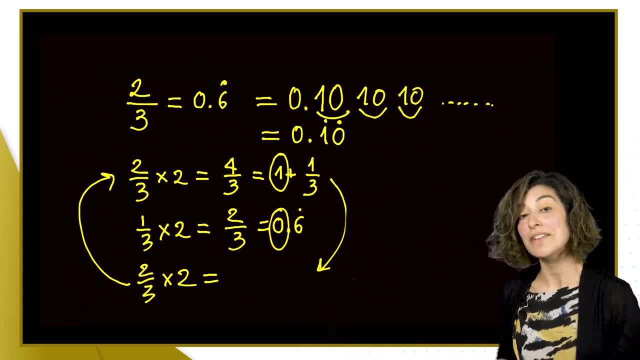 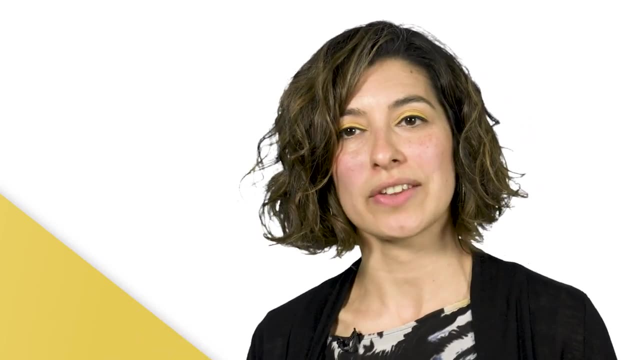 At some point your calculations will look the same, will follow the same pattern. You'll have a recurring set of calculations that creates that repeating pattern. This is how you know that you have such an example. We are using fractions and digital expansions to represent a number. 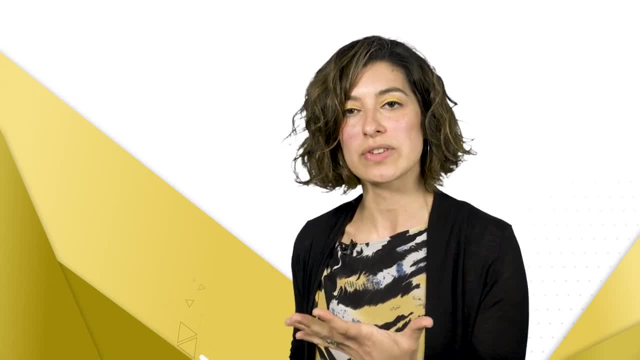 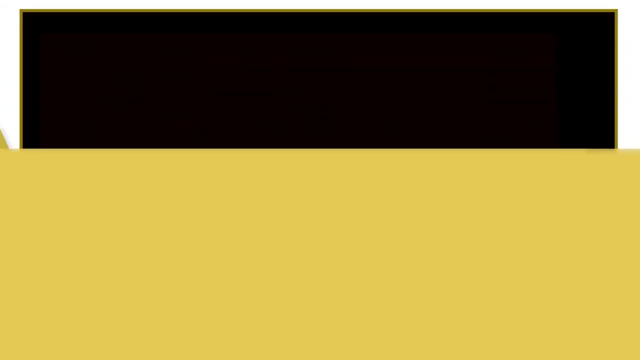 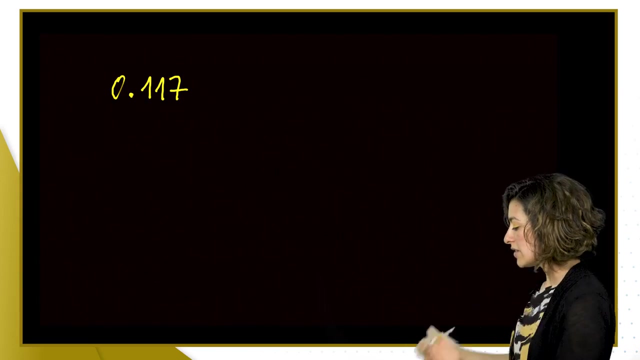 I'm going to go through the process of transforming a digital expansion in decimal into a fraction, so we know how to handle it. Say, the number in decimal is 0.117.. This number can be written as a fraction. we know it has a finite digital expansion. 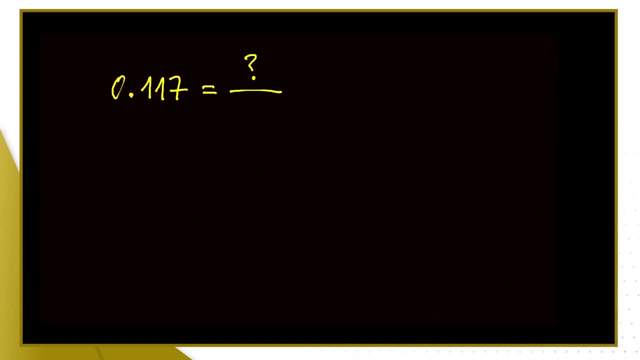 therefore, it can be written as a fraction with two numbers: a numerator and a denominator. How do we work them out? Here's what we do: I'm going to call this number x, just for convenience, and I'm going to multiply this number by x. 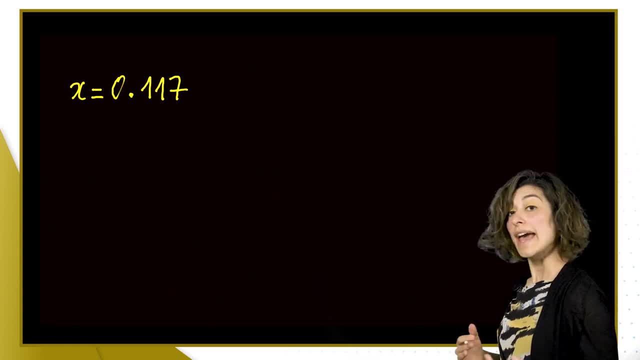 I'm going to multiply this number by 10, over and over again, until I have no fractional part. So if I do 10x, I get 1.17.. If I do 100x, I get 1.17.. 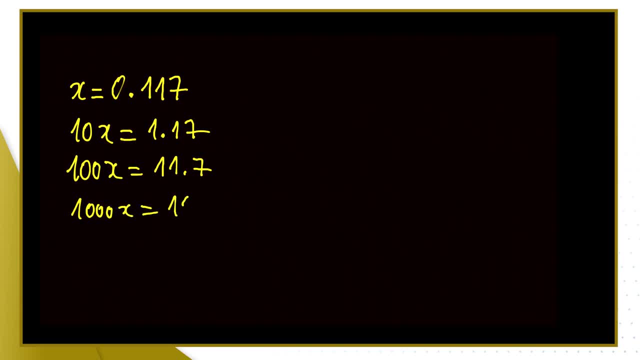 If I do 1000x, I get 1.17.. That's the number I want. In fact, you could have worked out that it was enough to multiply by a thousand straight away. So what do I do From here to get the fraction for x? I divide both sides of the equation by a thousand. 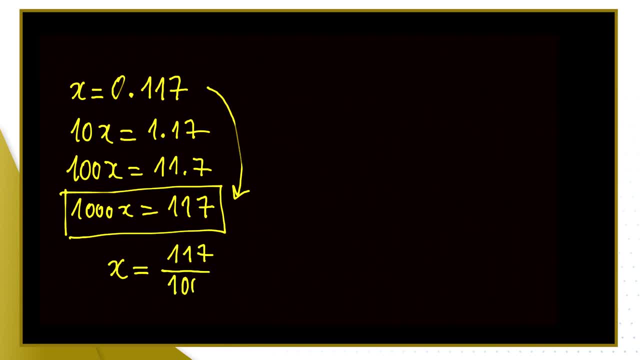 So I've got 1.17 divided by 1000, and that's the fraction that represents that digital expansion. Is this in lowest terms, Is this fraction in the simplest way as in: are there common factors between 117 and 1000?? 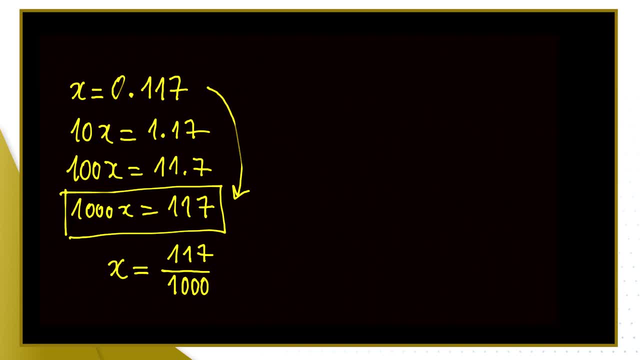 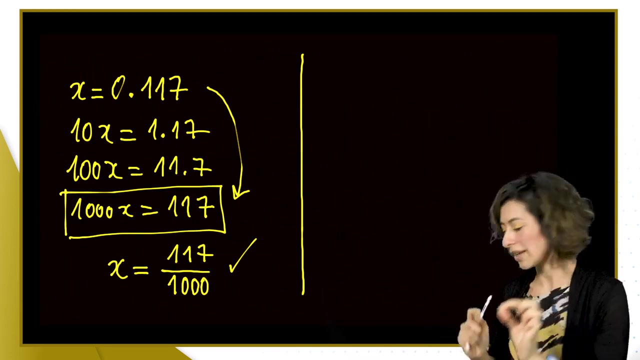 Not in this case. 1.17 is a multiple of 3 and a multiple of 13,, and the denominator doesn't have those factors. so this is in their lowest terms. But I'm going to do another example a little bit similar, but this time it's going to be a number with a repeating digital expansion. 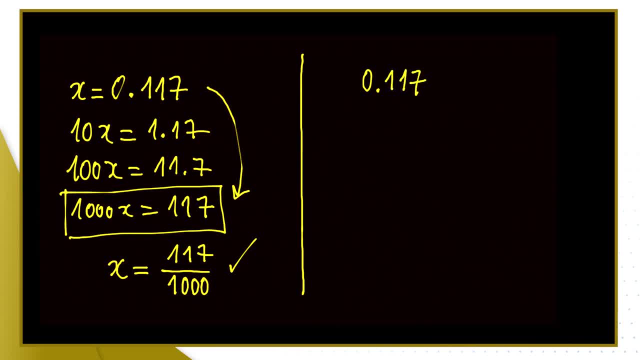 And I'm going to keep it very similar to that. one Say: the pattern that repeats is the 117.. So, in other words, what I mean by this is 0.117117117 and so on. That's what I mean. That's my number. 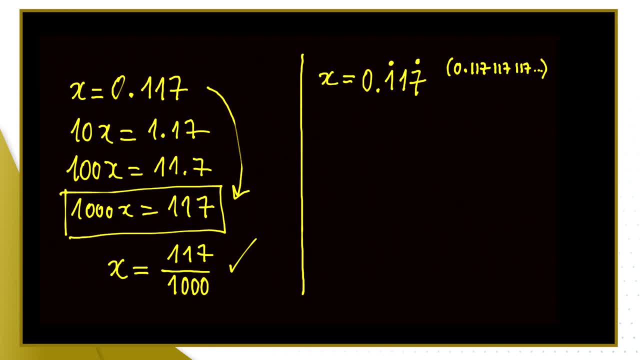 I'm going to call it x again for convenience, And what I want to do now is to multiply x by a power of 10 until the fractional part is exactly the same As the fractional part I have here on x. So if I multiply this number by 1000, I'm going to shift 117 to the integer part of the number. 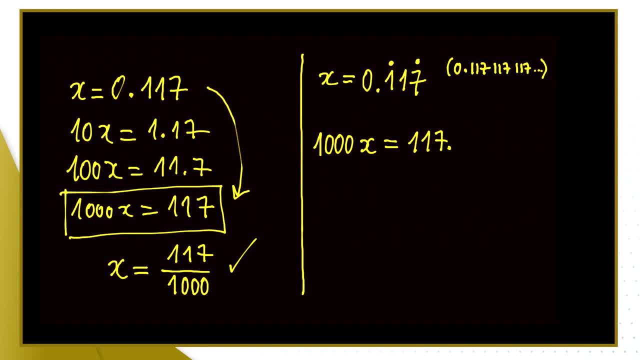 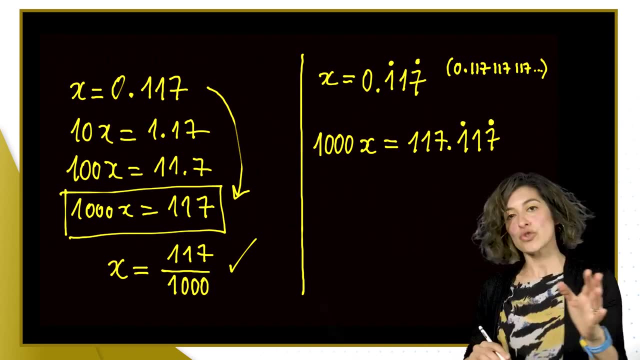 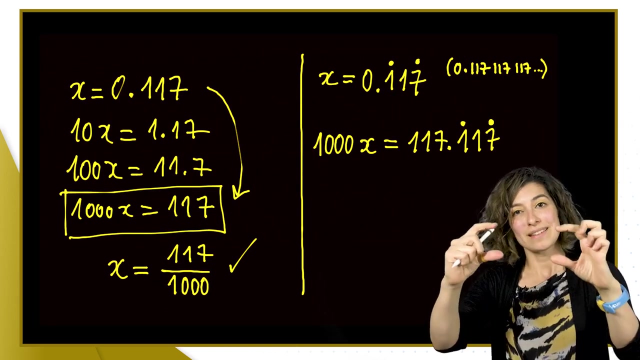 But because it has a repeating digital expansion, the 117117 will keep repeating on the fractional part. So I still have that and I will avoid writing forever by putting the dots on top. Okay, And now here's a trick: Because the two numbers, the x and the 1000x, have the same fractional part, I can subtract them to obtain an integer number. 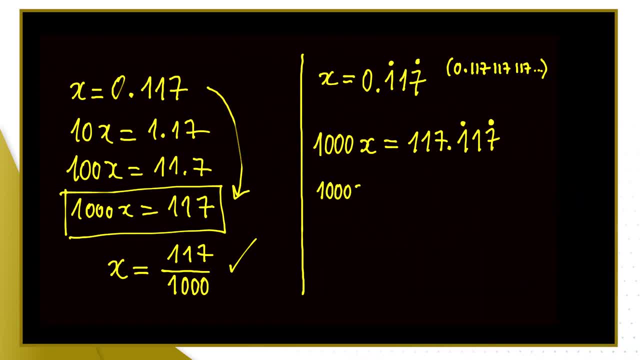 So if I subtract, as in I do, 1000x, take away the x, that means I'm doing 117.117 recurring And I'm going to take away 0.117.. And that means these guys subtract and I've got 117 left. 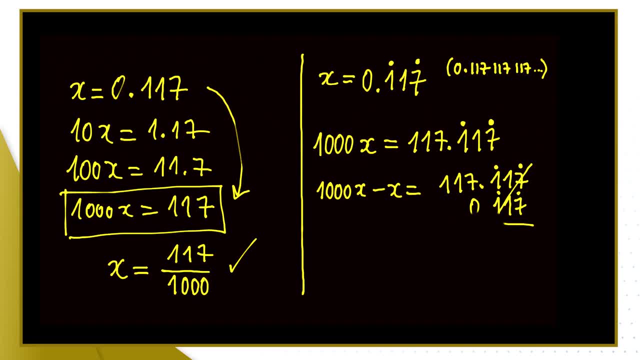 Okay, So the result is 117, which is just the integer part. Okay, And now, on this side, how many multiples of x do I have? Well, I had 1000 of x. Take away 1 of x. 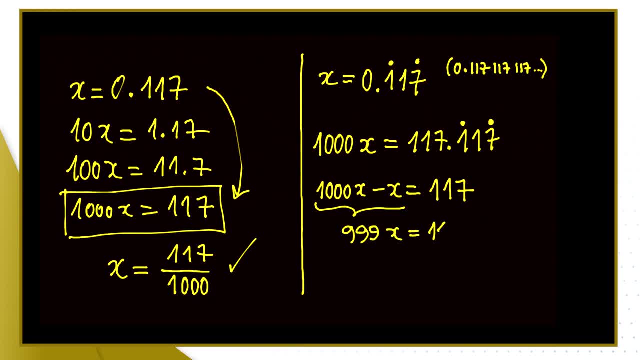 I've got 999 of x, Okay, And that's 117.. And now to get the fraction for my number, I divide everything by 999.. And here I am, And 117 divides by 9.. 117 divided by 9 gives us 13, divided by 111.. 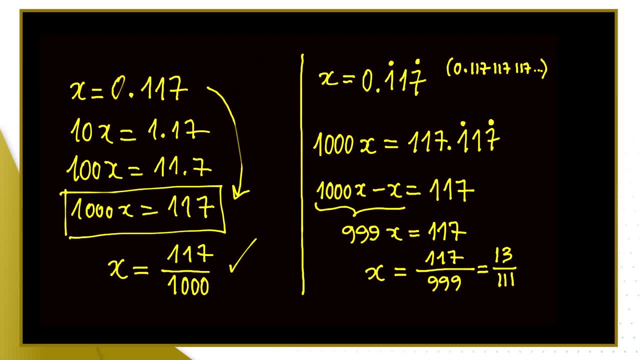 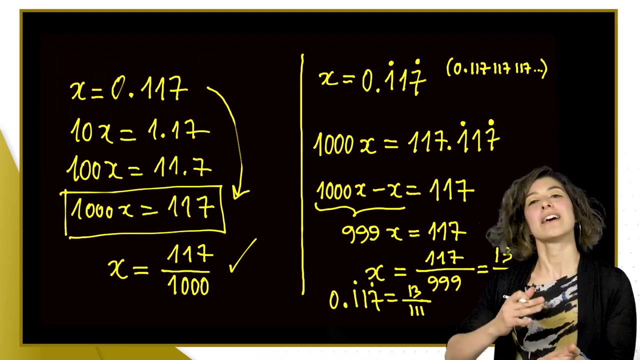 So that is the fraction that represents my recurring decimal, Or my recurring digital expansion, 0.117.. So, in other words, 0.117 equals 13 over. Now I wanted to note that there is a way of knowing whether a fraction is going to have a finite expansion or is going to have a repeating fraction. 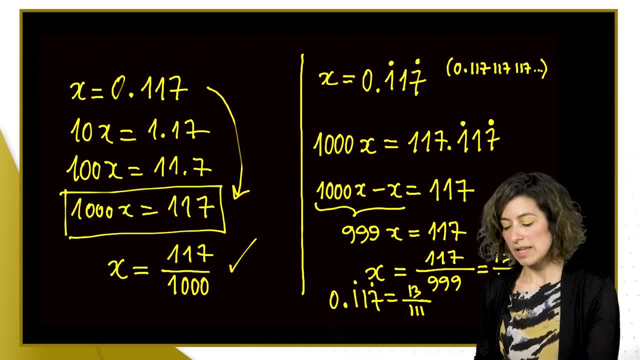 Or it's going to have a repeating expansion. It's to do with the denominator of that fraction. So in the examples we saw we've got the two numbers here side by side And in that first example I have a finite digital expansion. 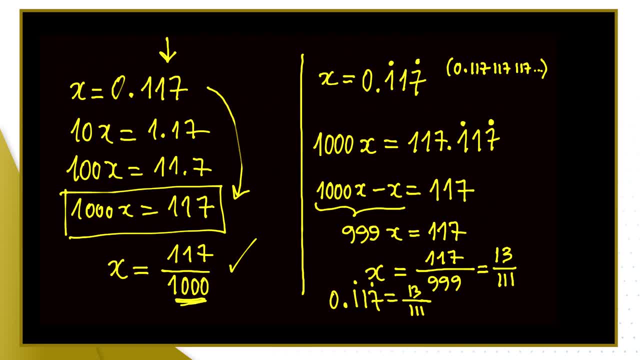 And look what the denominator is. The denominator of this fraction is 1000,, which is divisible by 2 and by 5.. On the second example, where I have the repeating fractional expansion, the denominator of the fraction is 111.. Which is not divisible by 2, and is not divisible by 5.. 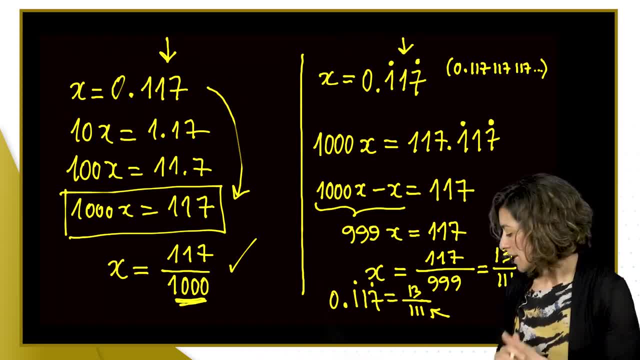 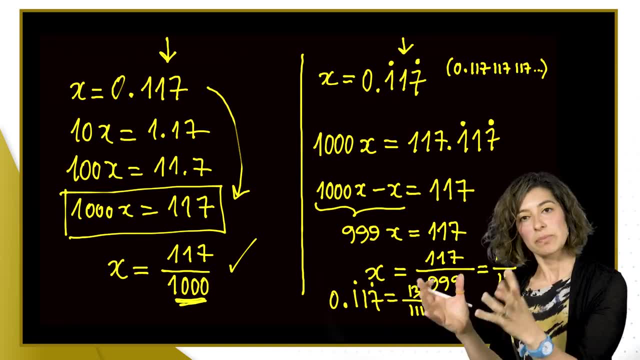 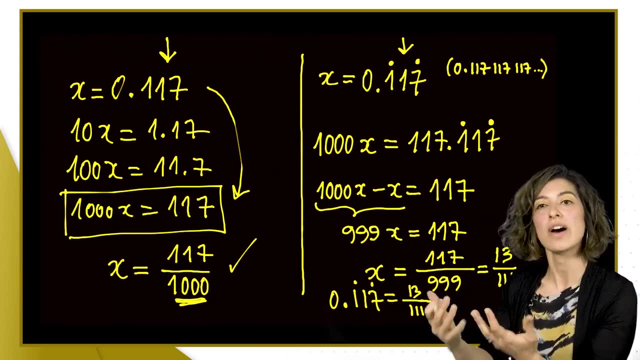 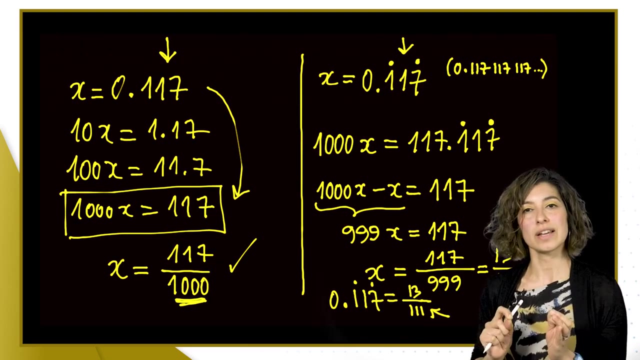 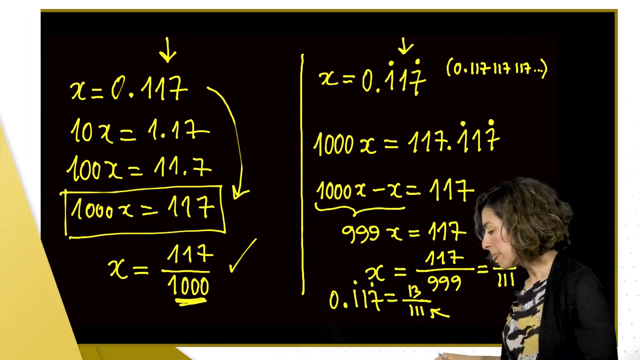 So when I'm working in base 10, in decimal, the fractions that will give me a finite expansion have a denominator that is a multiple of 2, or a multiple of 5, or a multiple of both. Any other fraction where the denominator is not divisible by 2 or not divisible by 5, will give rise to a recurring decimal. 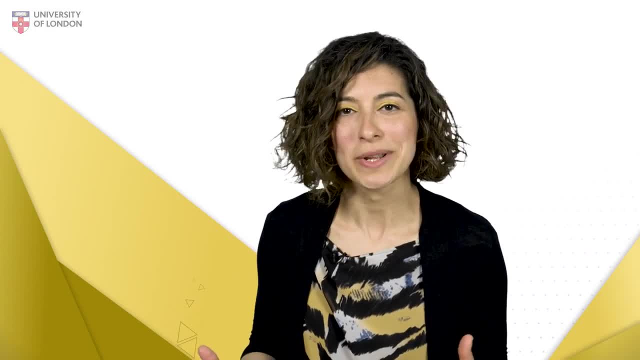 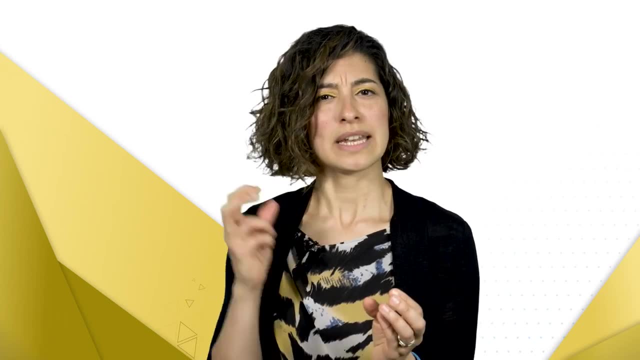 We saw the algorithm to write fractional numbers in binary. Now we multiplied the number by 2 and took the integer part to get the digit for the digital expansion. Why do we do that? Why do we multiply by 2?? Why do we multiply by 2?? 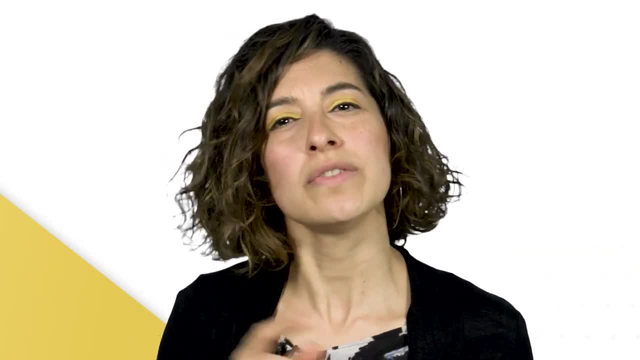 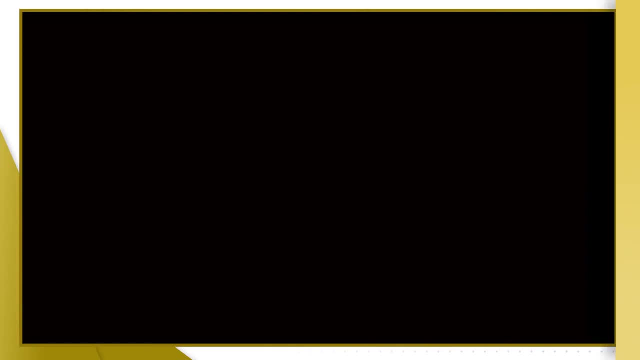 When, for the integer part of the number, we do division by 2 and take remainders. We're going to look at why that is. It is to do with the place values. Say we have the binary number 0.1011.. 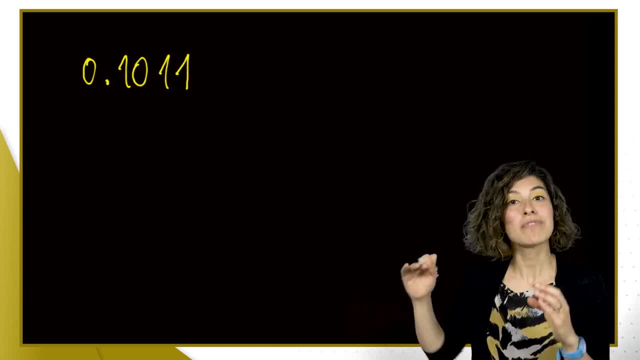 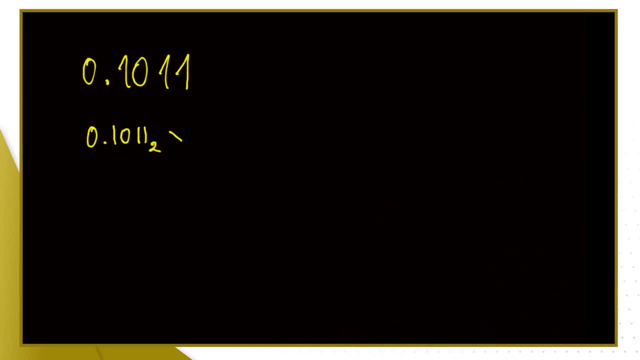 That's a number in binary. Although the number is in binary, I'm going to run the algorithm first to observe what is happening. So the algorithm says: multiply this number by 2.. Now, if I multiply this number by 2, because this is in binary- multiplying by 2 means I'm going to shift the place values. 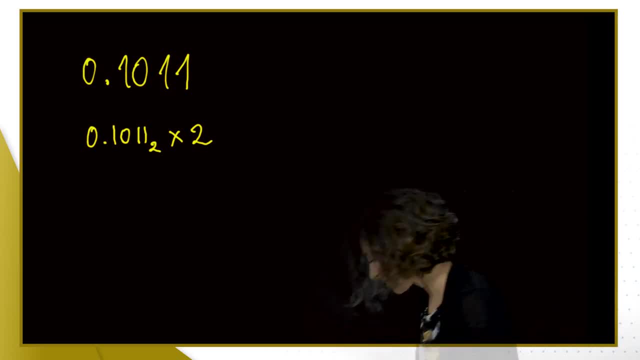 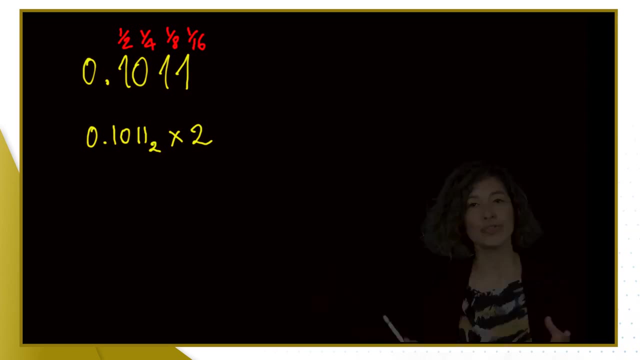 Let's look at the place values of the number to start with. This is for the place value of 1, half, 1 quarter, 1 eighth, 1 over 16.. And so multiplying by 2 is going to shift the place values. 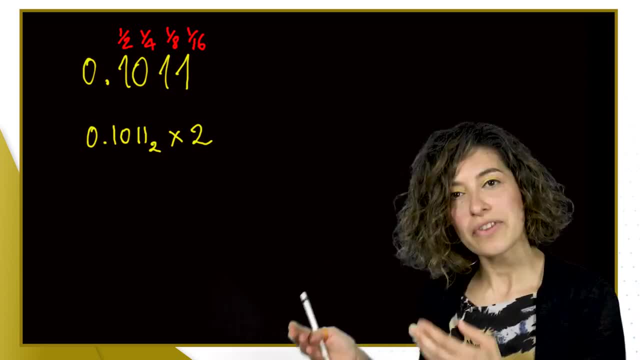 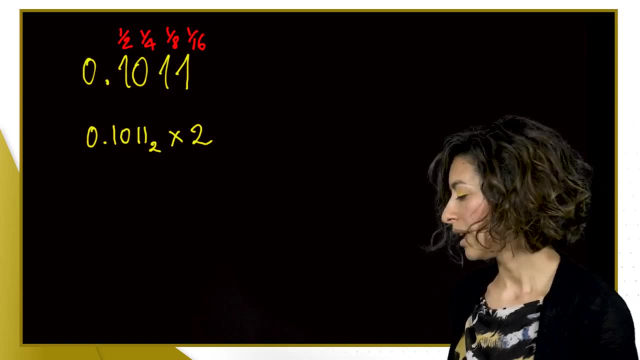 It's going to double all of them. The first 1 that appears there for place value 1 half is going to become the digit for place value 1.. The 0 for place value quarter is going to become the digit for place value 1 half, and so on. 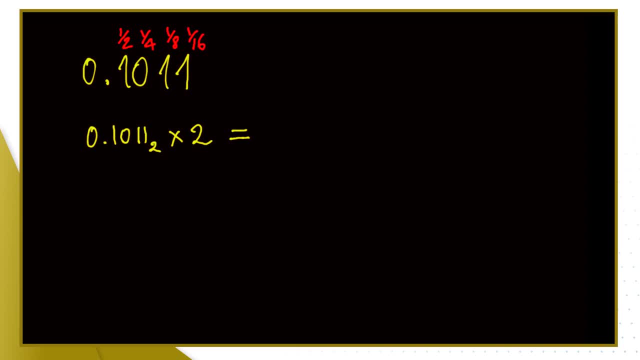 So what I mean is that this number multiplied by 2 is going to be 1.011 in binary And the algorithm said: let's take the integer part And that's going to become the first digit of the expansion. So that should be the first digit. 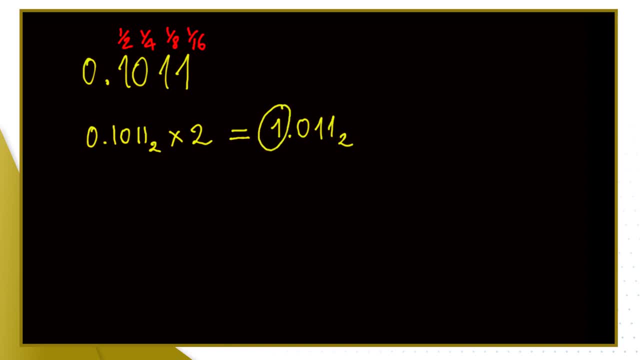 And that is true. And that is the first digit, because that was the digit for place value 1 half. And now we double the number, It became the integer part, And the algorithm says: take the integer part away and keep just the fractional. 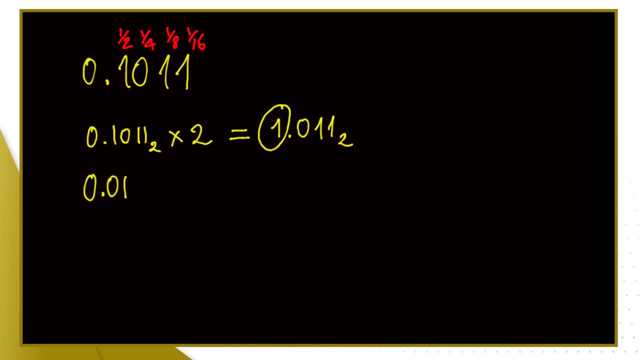 So we would then have 0.011 in binary And we would double it again. Again, doubling is going to shift all the place values. So we have 0.11 in binary. The integer part is 0. And that 0 came from the place value of 1 quarter from the initial number. 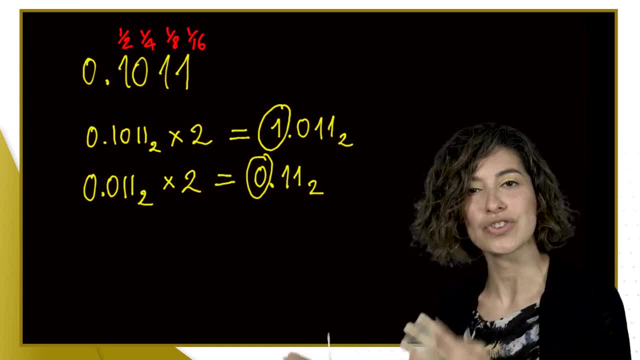 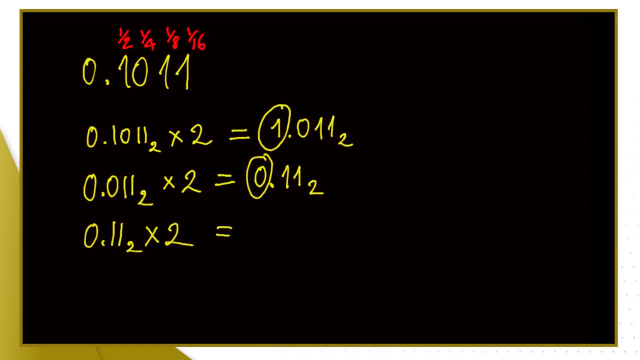 Because by now we multiply by 2 twice. So we shifted the digit two places And we keep going. We double it again. There's going to be 1.1 in binary. That integer part is the third digit. That's the third digit of the expansion. 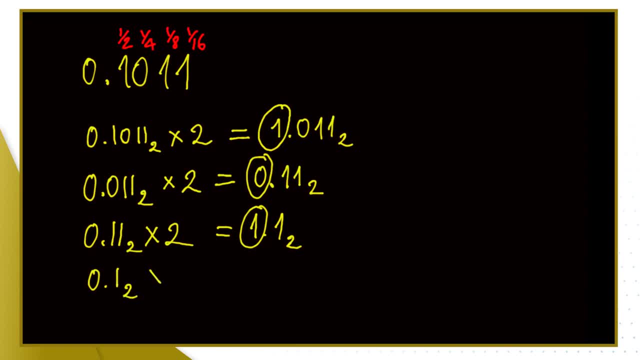 Take away the integer part, We get 0.1 in binary. Multiply by 2. That means 1.0 in binary. The integer part is 1, which is the last digit. And we know to stop, because as you remove the integer part, you're left with 0. 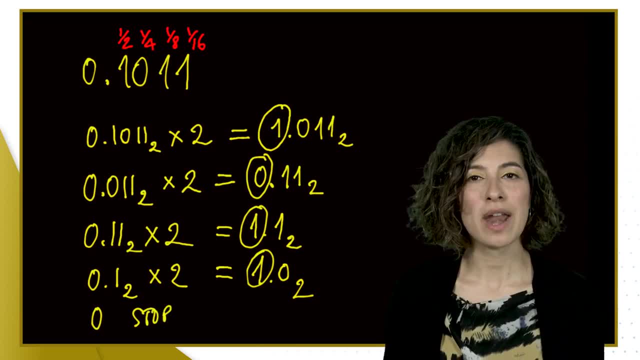 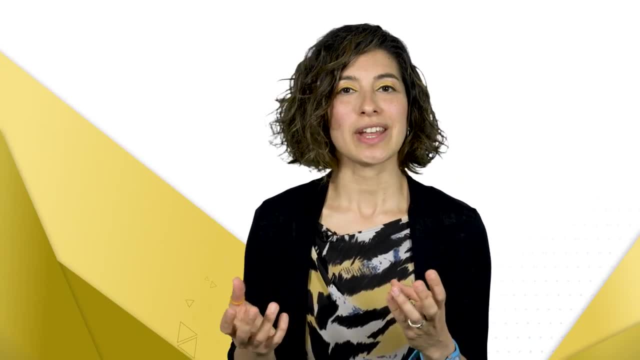 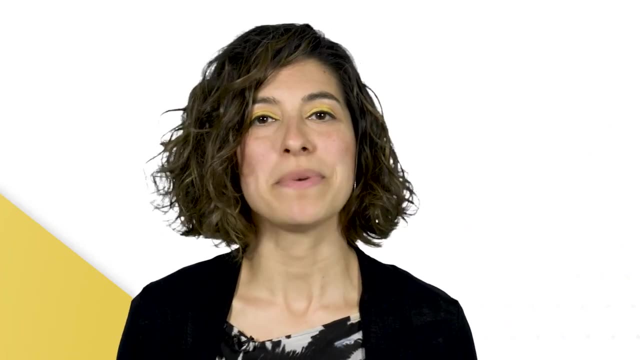 So we stop. I hope this example gives you a better idea of why the algorithm works In decimal. we know that looking at the digital expansion of a number, you can tell whether the number is rational or irrational. Rational numbers are numbers that can be written as a fraction. 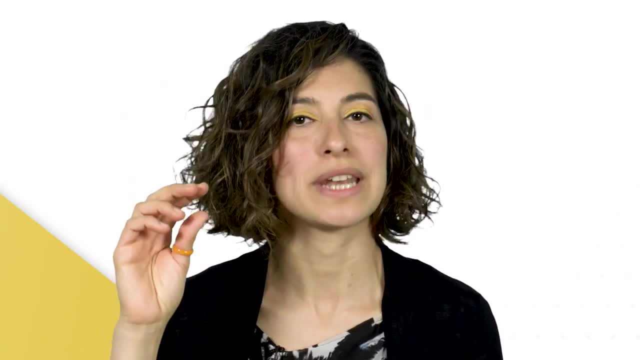 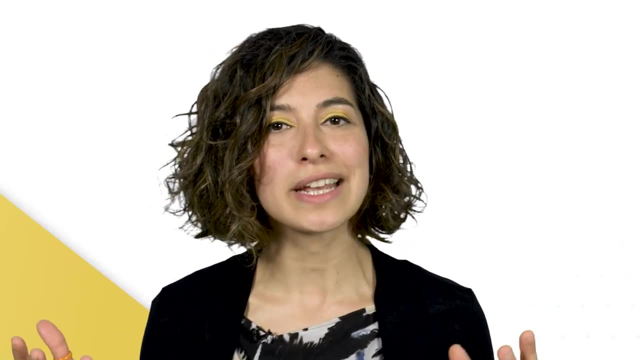 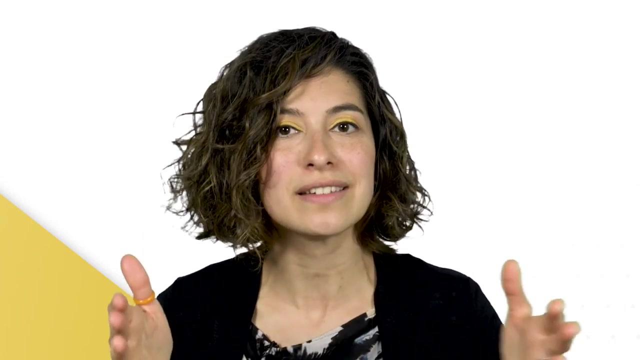 with whole numbers as numerator and denominator. If, instead of using a fraction, we want to use the digital expansion of the number, can we tell if the number is rational or irrational? Yes, we can, Because all rational numbers have either a finite digital expansion. 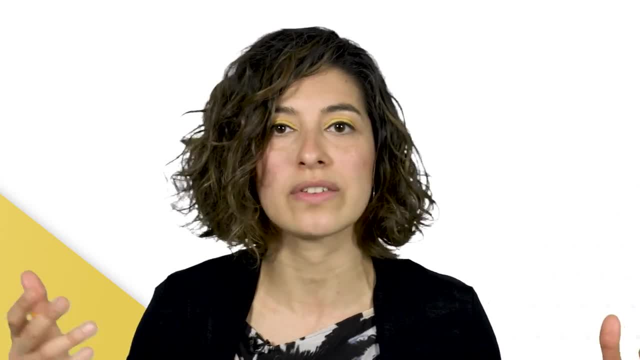 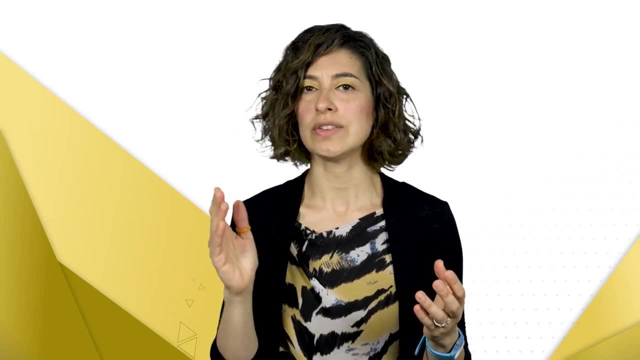 like 0.5, or 0.62, or they have a recurring digital expansion, Like when you do 1 third in your calculator you see 0.33333, or you can just write a 0.3 with a dot on top. 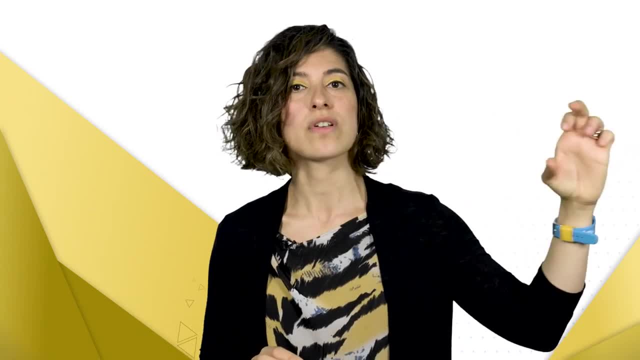 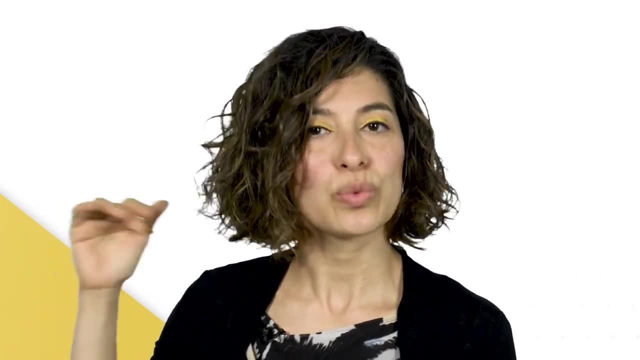 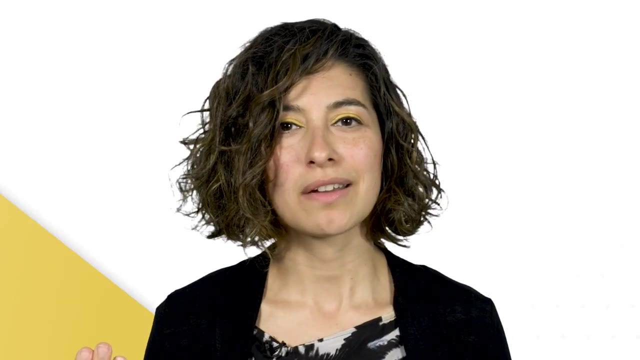 to say that that is a 3. that is going to repeat over and over again. Now those are the two types of rational numbers and they all are written as fractions, as we saw the method earlier on. What about binary? What happens with rational numbers? when you write them in binary or irrational numbers. when you write them in binary- Surprisingly or not, maybe you're already guessing- the same is true If the number is rational, if the number can be written as a fraction, with integer, numerator and denominator. 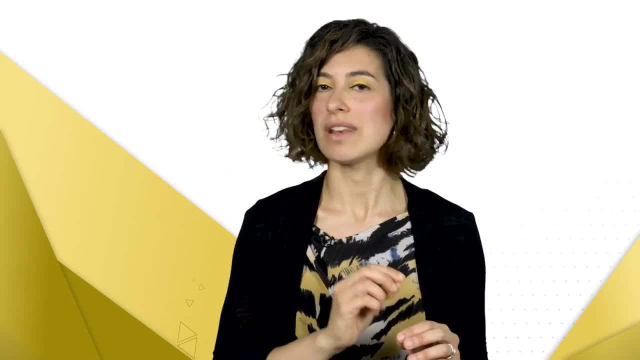 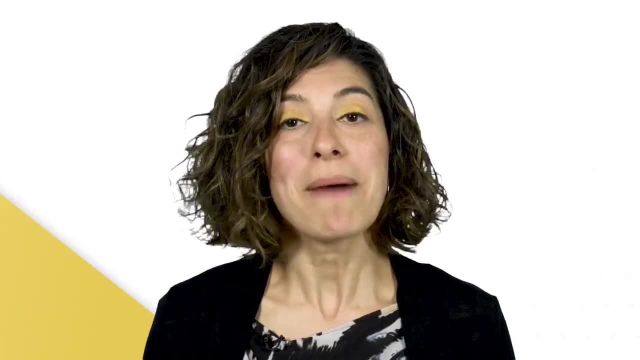 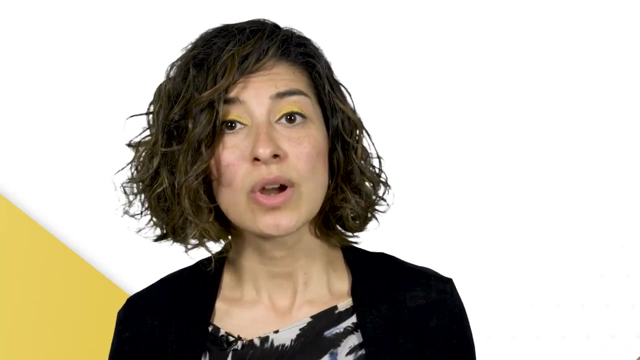 then the digital expansion, no matter which base you write it on, it will be either finite or recurring. It might happen that a number can have a finite expansion in one base but a recurring expansion on the different, or have recurring expansions on both but with different periods. 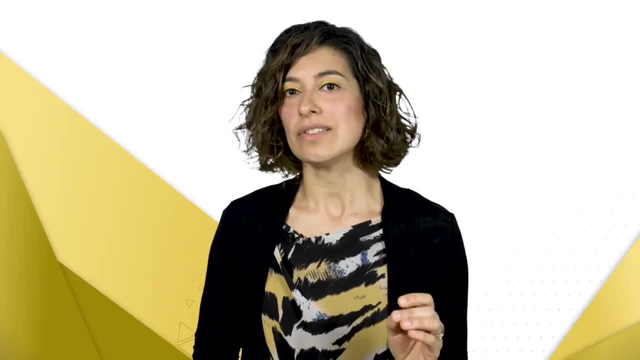 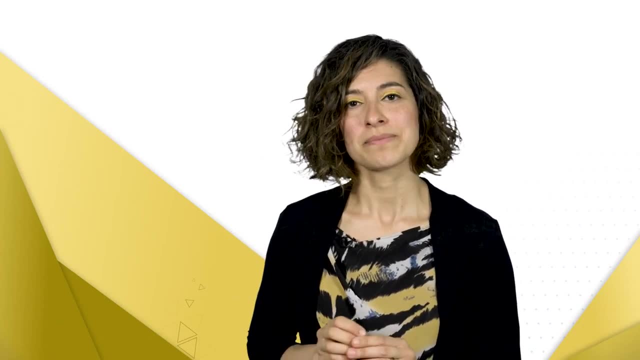 with different patterns of repetition. The key to deciding whether it's going to be finite or recurring is to do with the denominator of that fraction. I'm not going to go into too much detail, but I want to lift the veil of this to you so you know what to expect. 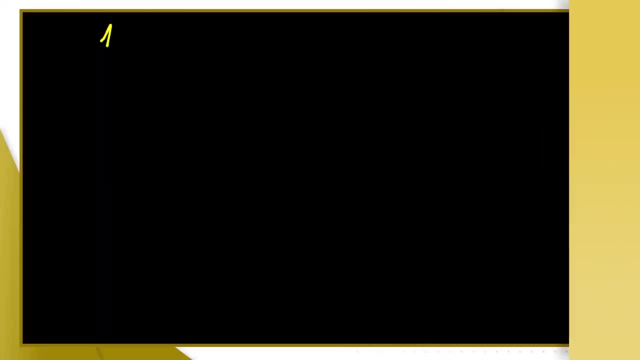 when you're working with these numbers. Let's look at 1 over 6.. 1 over 6 is less than 1, therefore the first binary digit, the integer part, is going to be 0.. Now I'm going to double this number. 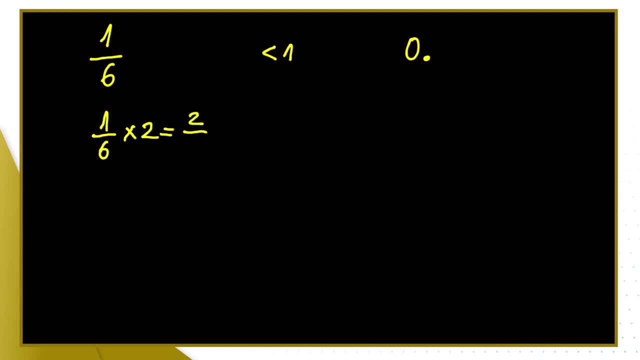 1 over 6 times 2, which is 2 over 6,, which is 1 third. 1 third is still less than 1, so the first fractional binary will be 0.. So digit 0 there. digit 0 there. 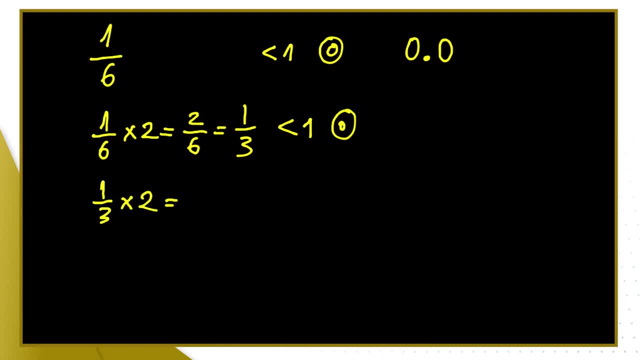 Now take 1 third and double it. That's 2 thirds. That is still less than 1, so I got another 0.. Then 2 thirds, double it. I got 4 thirds, which is 1 plus 1 third. 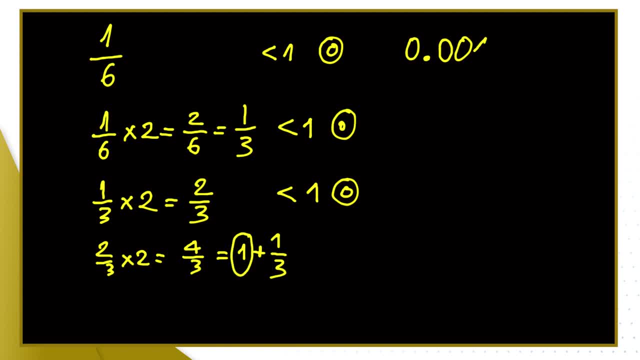 And that the integer part is 1, that's the digit I'm going to put there And I'm going to take the fractional part and double it again. Now, at this stage, you realise that that 1 third times 2. 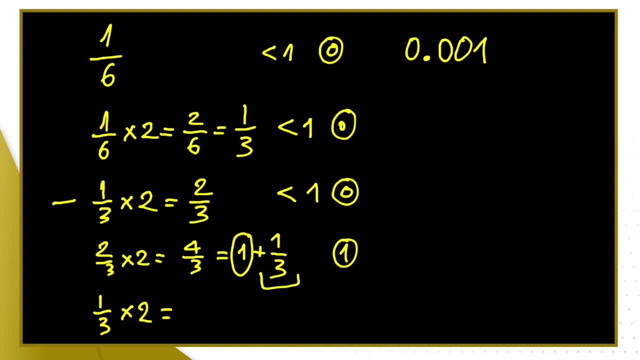 is what I've got there, So we're going to have this part repeating. So that is 1 over 6 as a fraction. that is written in decimal. It has a binary fractional expansion of 0.001, with 0.01 repeating. 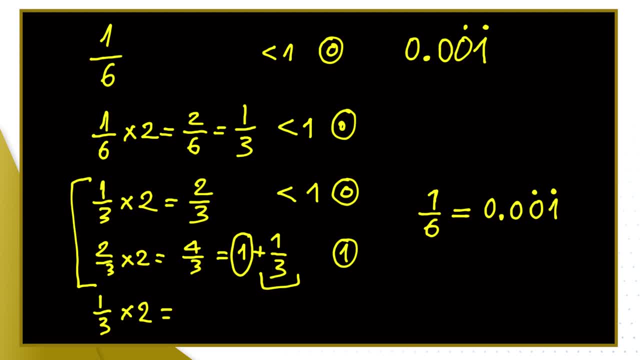 Now there's 2 things I want to draw your attention for. First, there is a period, There is a repeating pattern, And second, there is an initial part before the repetition starts. Now, this initial 0 comes from the fact that the 6. 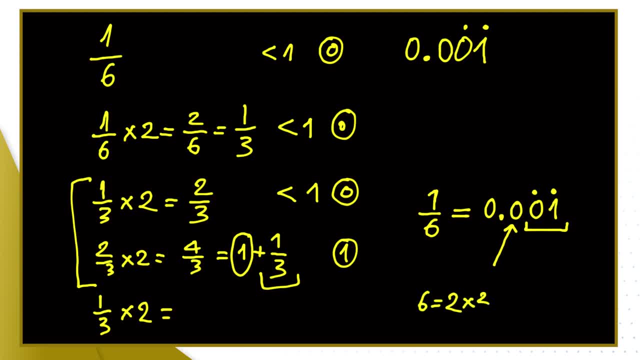 being the denominator 6 is 2 times 3.. The fact that we have a 2, which is a factor of the base base 2, means that I've got that initial 0, meaning I've got that initial non-repeating part. 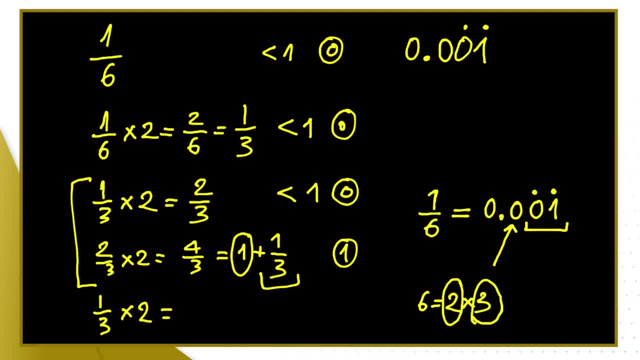 Then the fact that I've got a 3 as a factor of 6 means that I will have a repeating pattern. Now, why does 3 give us a repeating pattern? Because 3 has no common factors with the base. 3 has no common factors with 2,. 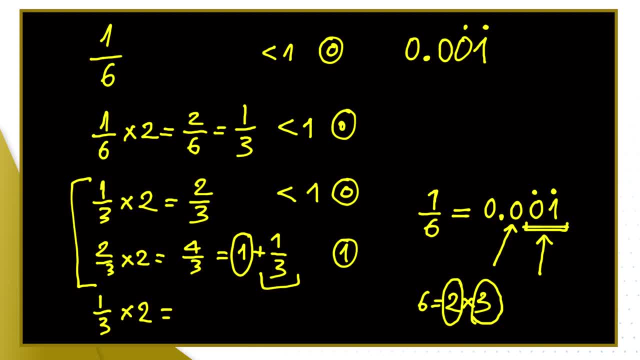 so I will have a periodic expansion. I've got that 2 that is a factor of the base, so I will have, say, a delay until the period begins And these considerations I made here about the denominator of the fraction and the relationship to the factors of the base. 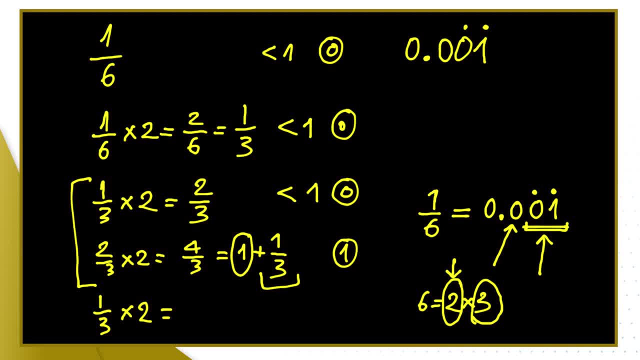 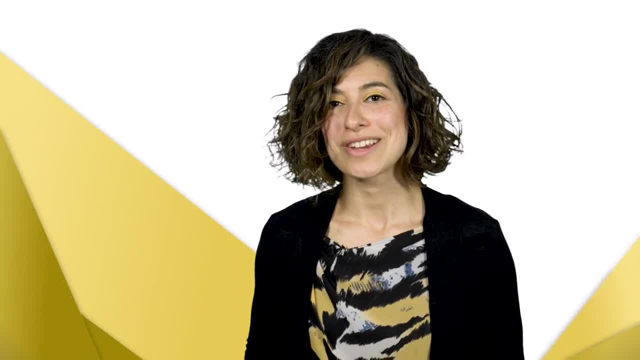 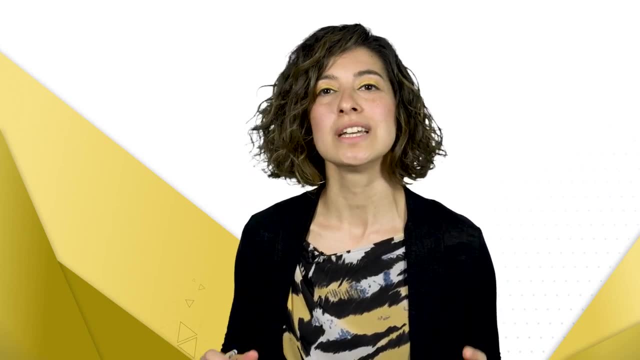 are essentially the bits that decide what the fractional expansion of a number looks like in a given base. Have a play with more fractions and gain an idea of how it works. If you have powers of 2 in the denominator, you will have a finite digital expansion in binary. 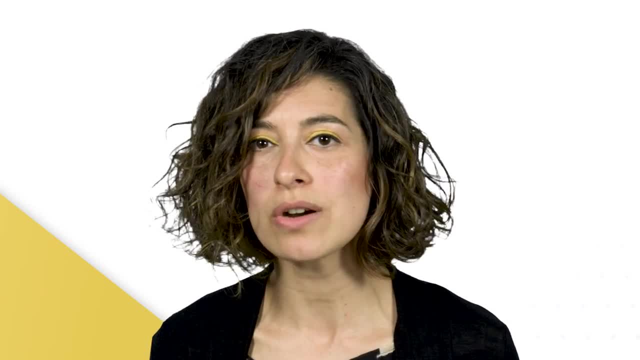 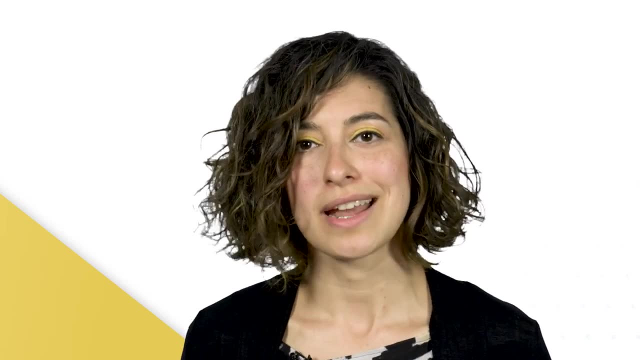 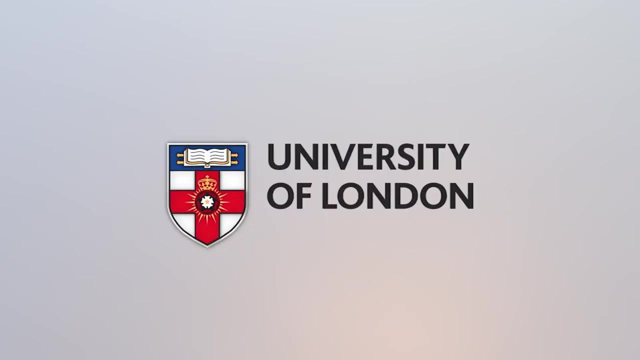 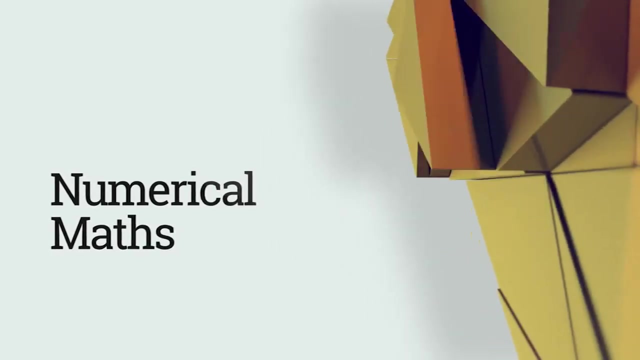 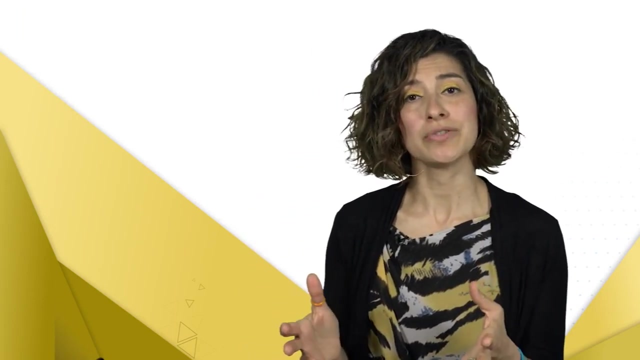 If the number you have there isn't a power of 2, if it's a power of 2 times something else, or just no 2s at all, it will be a recurring decimal. In this lesson we looked at number systems and we focused on binary. 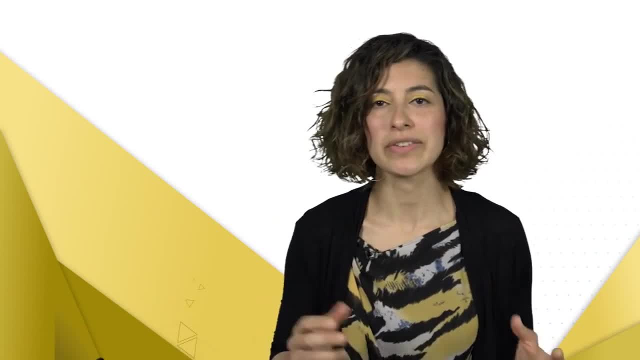 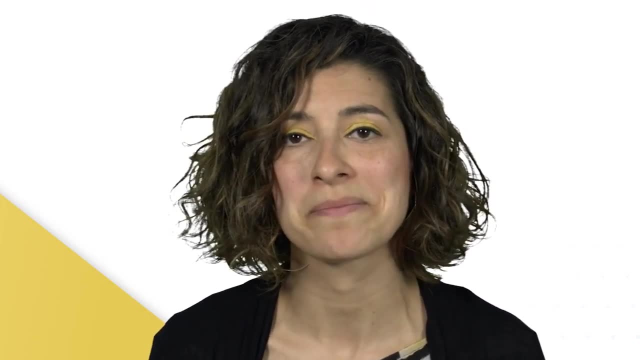 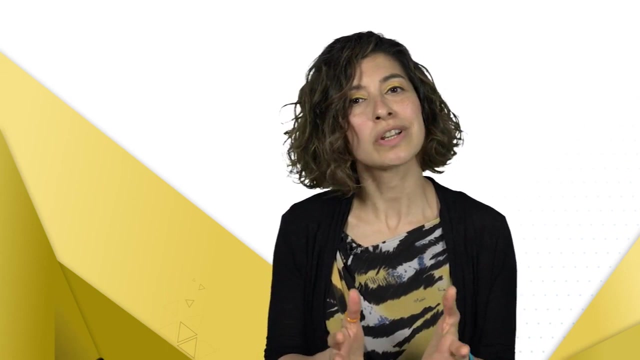 both converting decimal to binary and binary to decimal. We looked as well at rational and irrational numbers, how they are represented both in decimal and in binary. Now I would like you to get ready for operations in binary. That only requires you to recap. 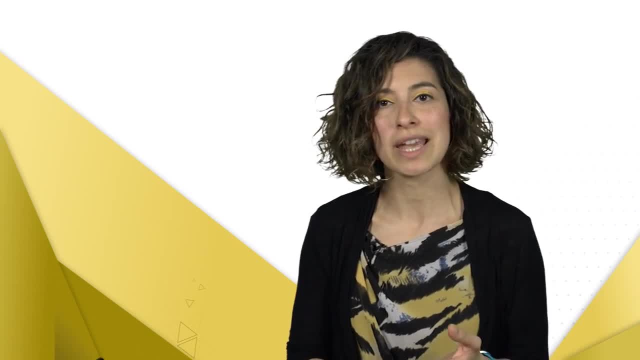 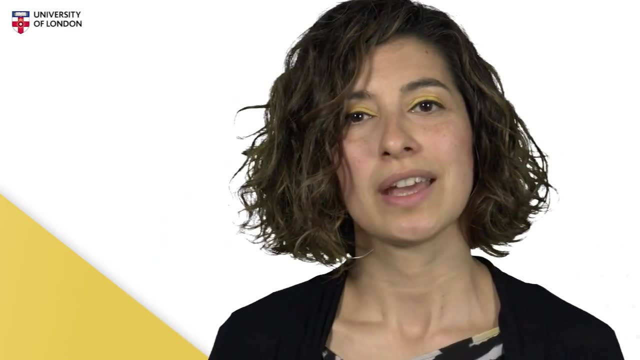 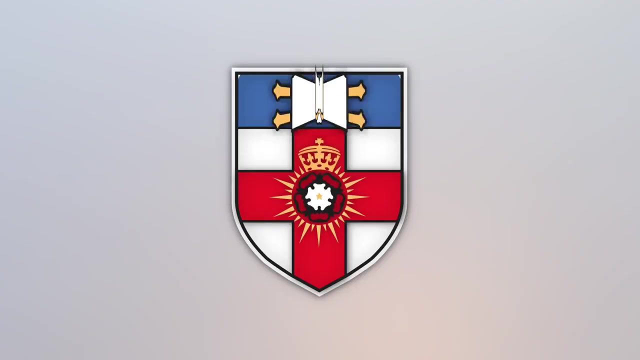 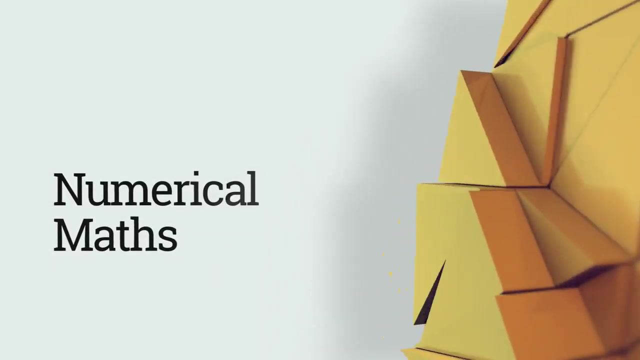 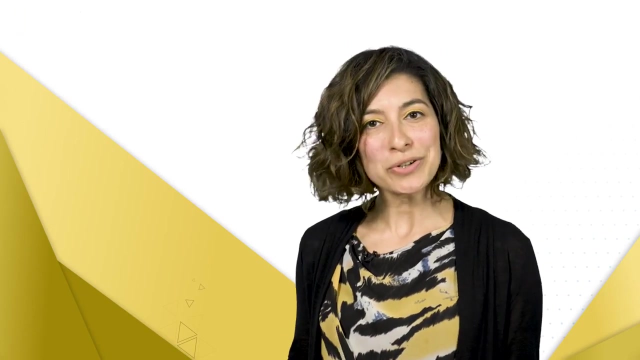 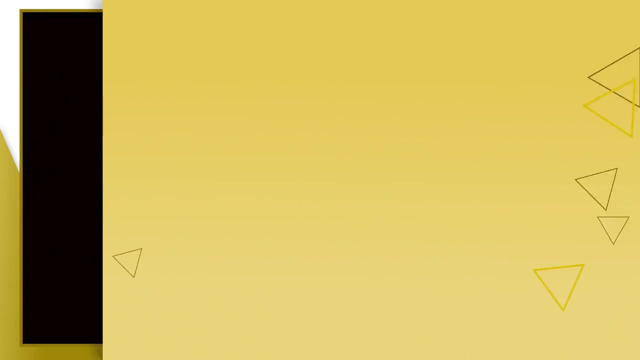 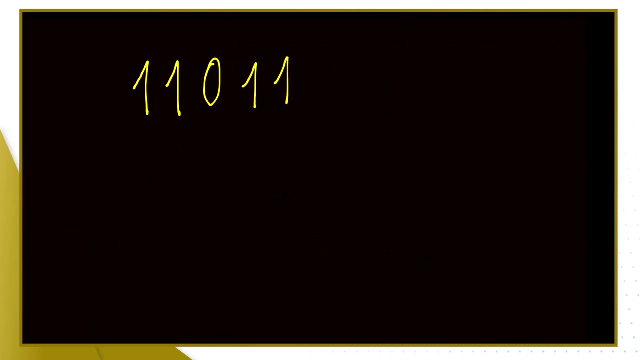 how you've learned to do addition, subtraction and multiplication back in primary school. So go and revise that, those really handwritten algorithms, and get ready for the next lesson. Subtitles by the Amaraorg community. We're going to do it old school style. 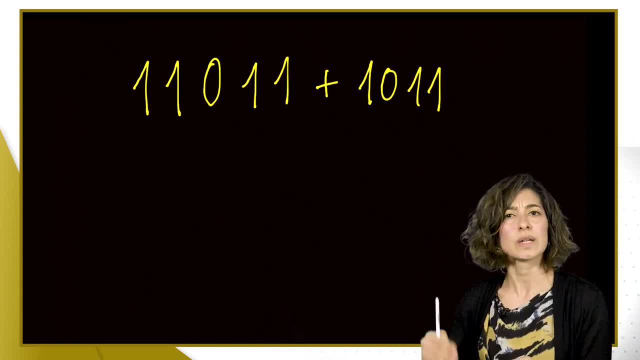 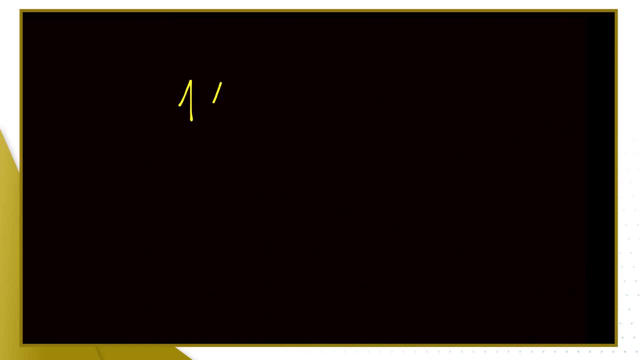 We're going to write the numbers one on top of the other and do the algorithm column by column, like you learn how to add up numbers back in primary school: 1, 1, 0, 1, 1.. Now we're going to write the numbers lined up. 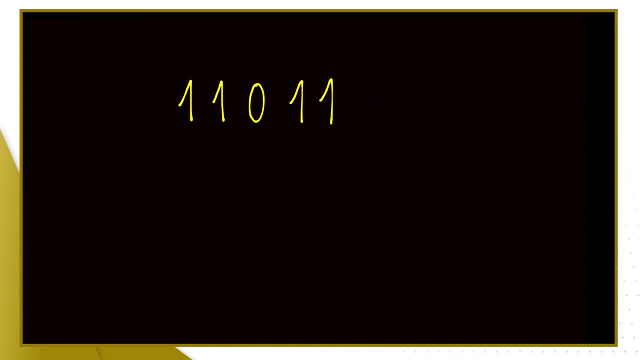 with the place values correctly aligned, So 1, 0, 1, 1 underneath Our long line adding it up. And we have to keep in mind going in between binary and decimal for some of the minor calculations going on. 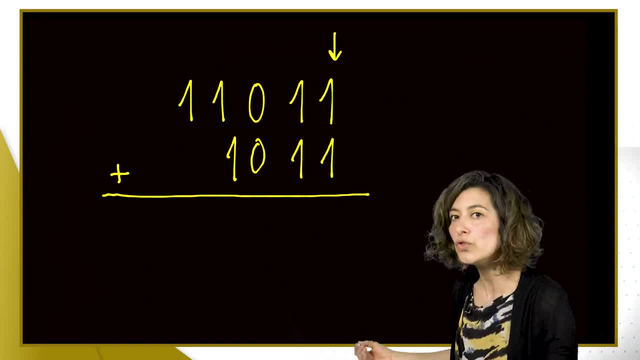 So what I mean is first column 1 plus 1, that is 2.. 2 in binary is 1, 0. Hang on, how do we do this? Where do we write the numbers? No problem, so 1 plus 1 is 2.. 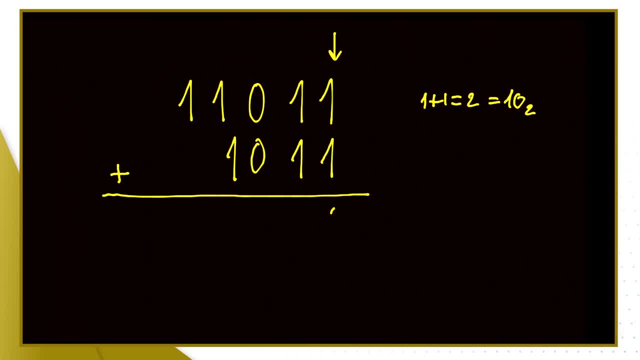 That is 1, 0 in binary. We need to put a 0 here and the 1 would kind of go there, but we can't really write it there because that is going to be for the result of the column. So what we do, we're going to carry that digit. 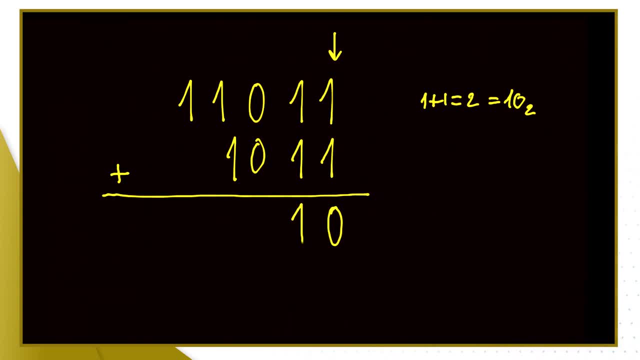 and we're going to put it at the top of the column. So I'm going to rub that one off and I'm going to write it over there, because really that 1 is from the next place value, So we put it on the column for the next place value. 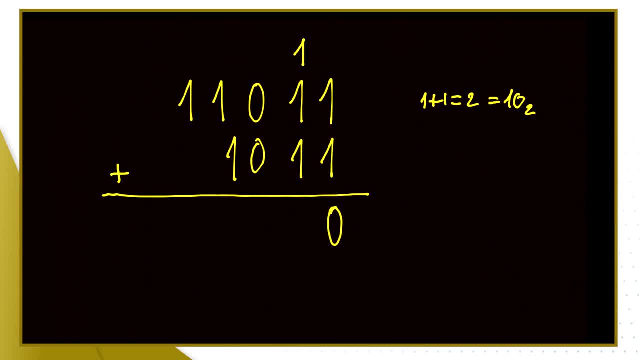 And now we proceed. So we're now on the second column. We're going to add up the 1 with the 1 with the 1.. So 1 plus 1 plus 1 is 3.. And 3 is 1, 1 in binary. 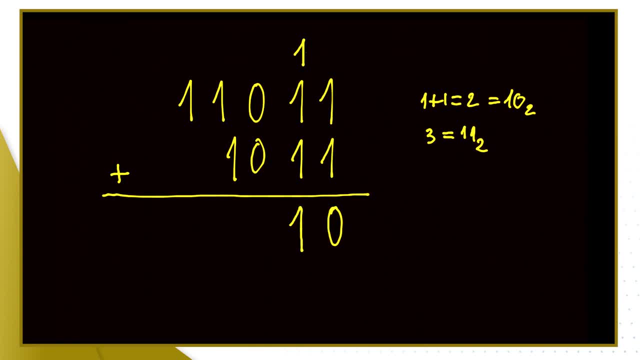 Again, we need the 1 over here And the other 1. that is for the next place value. we'll put it on top. Now we add up the numbers in that column: 1 plus 0 plus 0, that's just 1.. 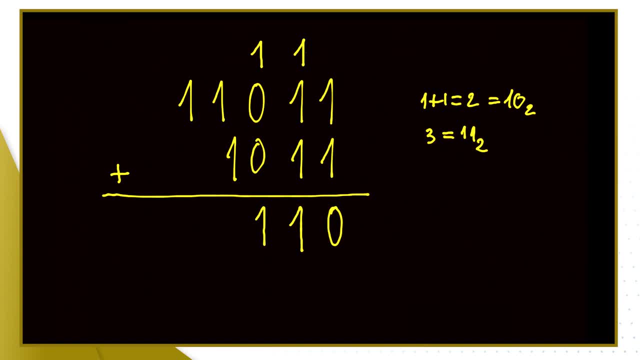 No numbers to carry. And then 1 plus 1 again is 2.. 2 is 1, 0,, so 0 here, And the 1 for the next place value goes on top of the next column. And now 1, 1 is 2, so it's 1, 0 again. 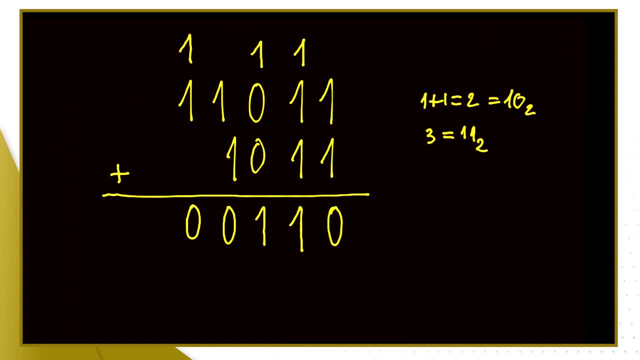 And we'll put the 0 there and we're going to put the 1 in the next column, So we just put it on the next place. value Done, Okay. So what do we write? We write: the result of our sum is that: 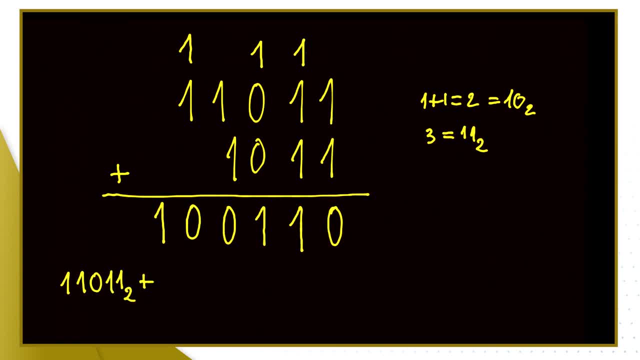 1, 1, 0, 1, 1 in binary added with 1, 0, 1, 1 in binary equals 1, 0, 0, 1, 1, 0 in binary. 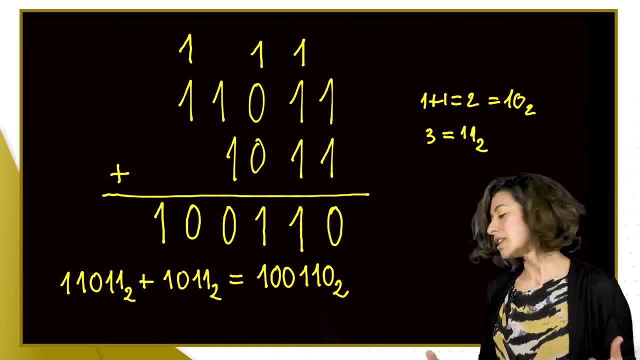 And when you get used to doing this, you'll be a lot faster than converting binary to decimal of the both numbers at the map and then convert it back to binary. That is a long way. It's much better to learn how to manipulate the numbers in binary and get confident with it. 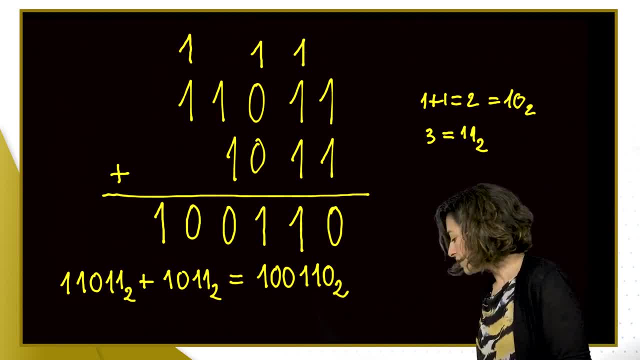 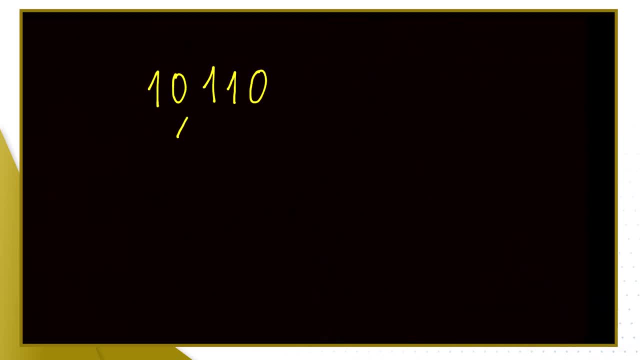 Let's do another example of addition in binary. Let's do 1, 0, 1, 1, 0 added with a string of 1s- Those there, You can anticipate that there might be loads of carries. Let's see: 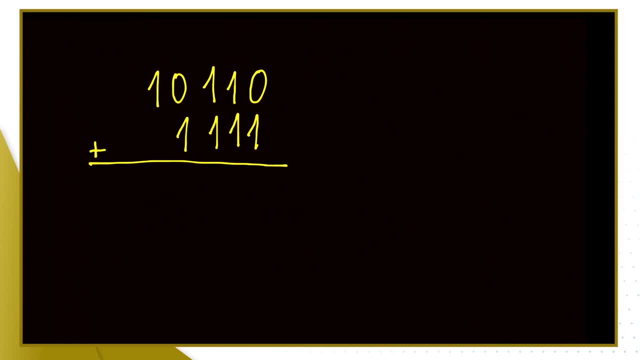 So first column Column for the place value: 1. 0 plus 1 is 1.. No problem. Now here, 1 plus 1 is 2.. 2 is 1, 0. So we're going to write 0 here and 1 carried over there. 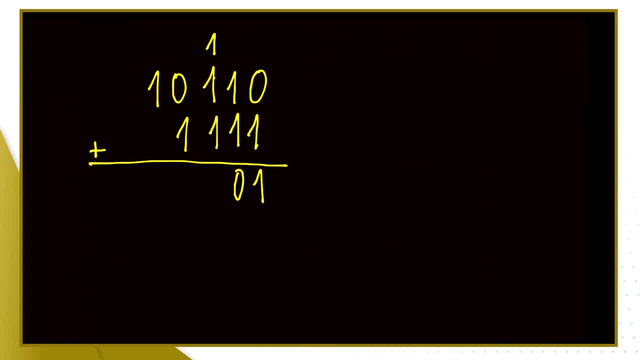 Now, 1 plus 1 plus 1 is 3.. That's 1, 1.. So 1 here and the next 1 there. 1 plus 1 is 2.. 2 is 1, 0.. So 0 there and 1 over there. 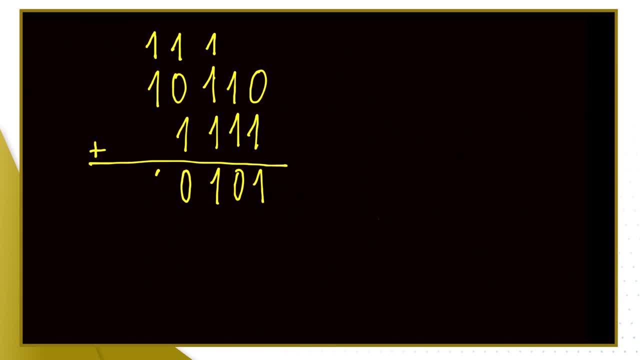 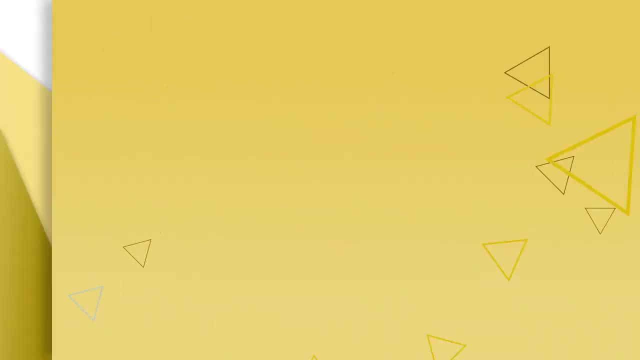 1 and 1 adds to 2,, which is 1, 0. And there we go, So 1, 0, 1, 1, 0 in binary added with 1, 1, 1, 1 in binary is 1, 0, 0, 1, 0, 1 in binary. 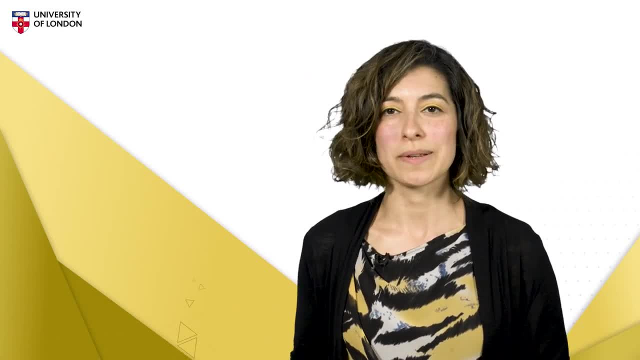 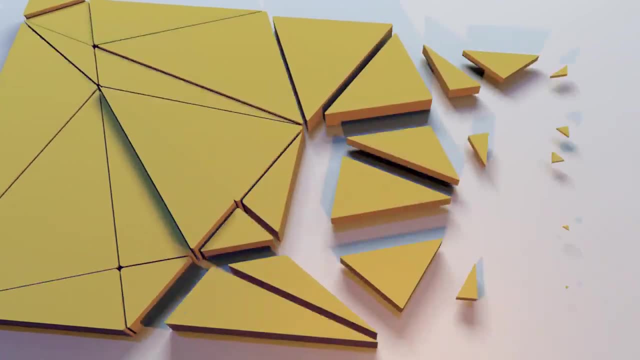 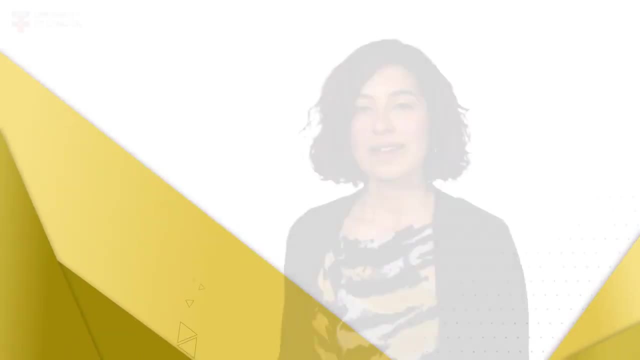 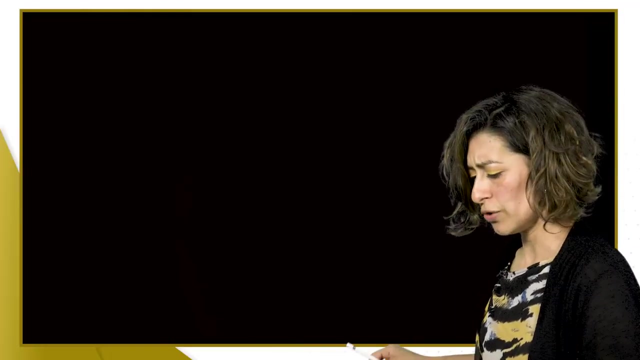 So that's how you perform addition purely in binary. Now we're going to look at subtraction in binary. Let's do the following: Let's do 1, 0, 1, 0, 0, 0,. take away 1, 0, 0, 0, 1.. 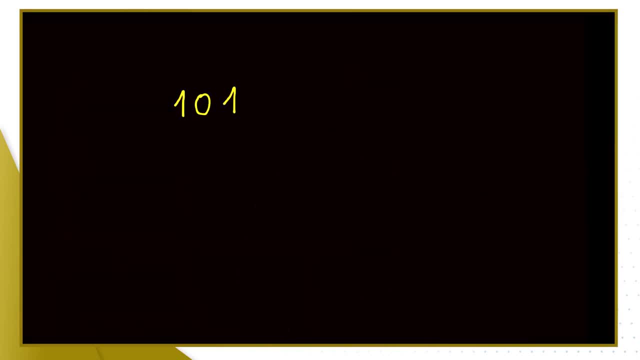 I'm just going to write it down. So we do 1, 0, 1, 0, 0, 0, take away 1, 0, 0, 0, 1.. It's very important to line up the numbers in the correct columns of place value. 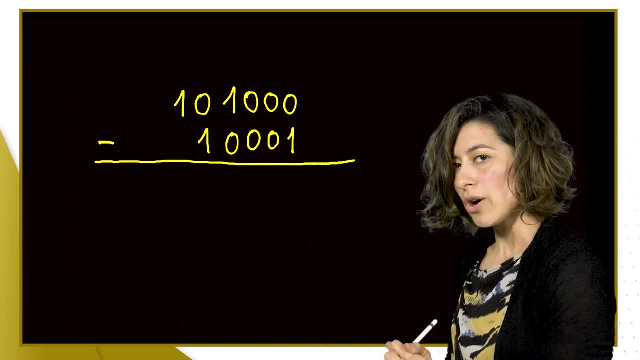 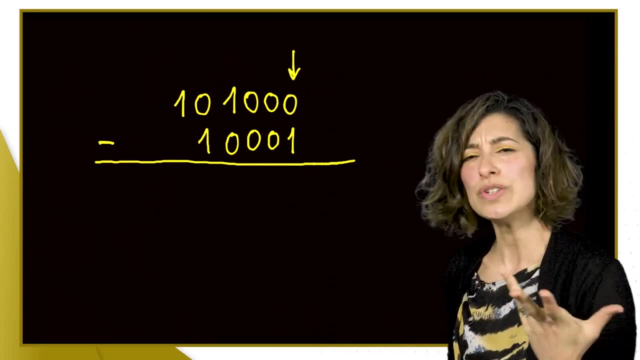 We're going to subtract. Looking at it column by column, There's immediately a little problem, isn't it? Look at the first column there: 0, take away 1.. How do we do that? Do you remember how we did that? 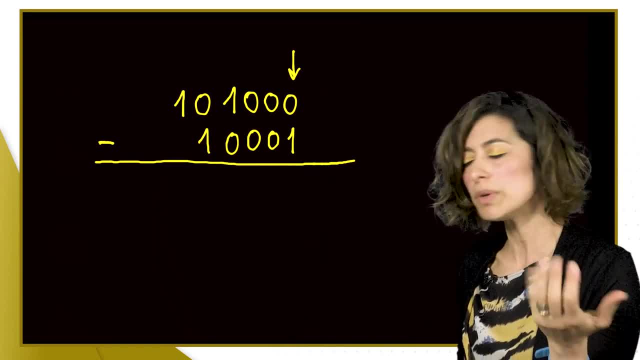 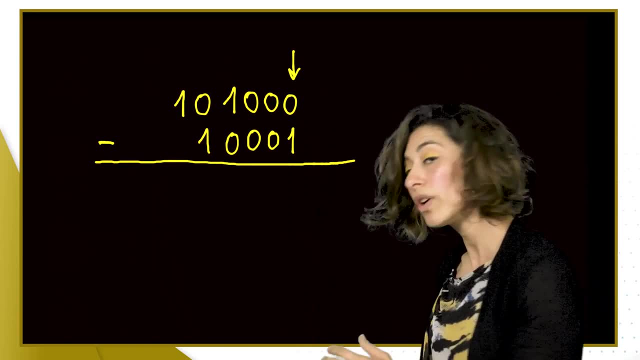 How you did that in primary school. for decimal numbers, You had to borrow, Because 0 is too small to take away 1.. You had to borrow. Where are we going to borrow from? Well, we're going to borrow from the bigger place- files next to it. 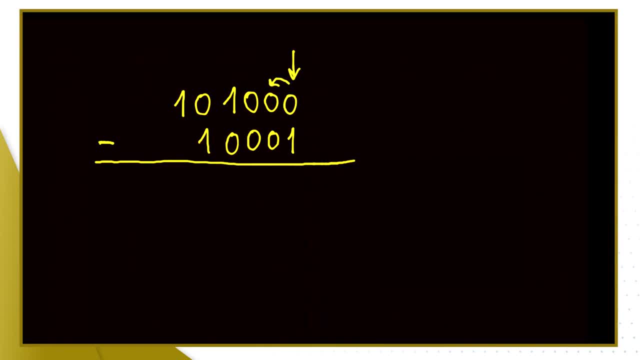 The thing is we've got a 0 just there, which you can't borrow anything from there, and another 1. So we're going to have to borrow from a lot of place values. What I mean is we're going to look at this part of the number here. 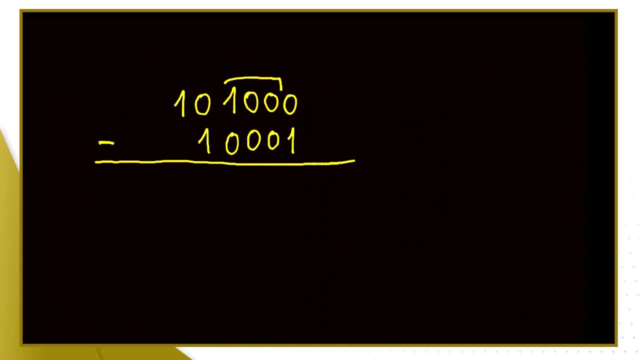 1, 0, 0,. 1, 0, 0 can be written as 1, 1, add 1.. That means we're going to replace the 1, 0, 0 by just 1, 1.. 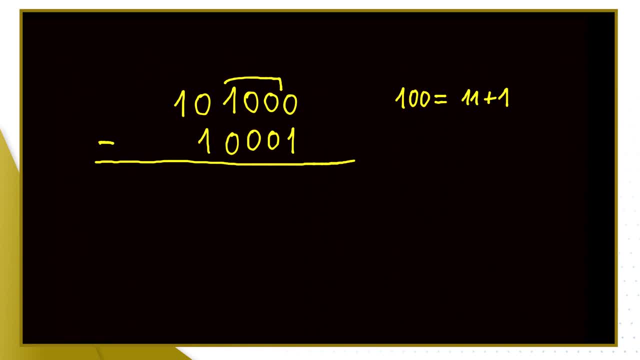 And we're going to borrow that extra 1 to the first column. This way, We're going to cross that 1, 0, 0 out And we're going to replace it with 1, 1.. Like I did here on the side. 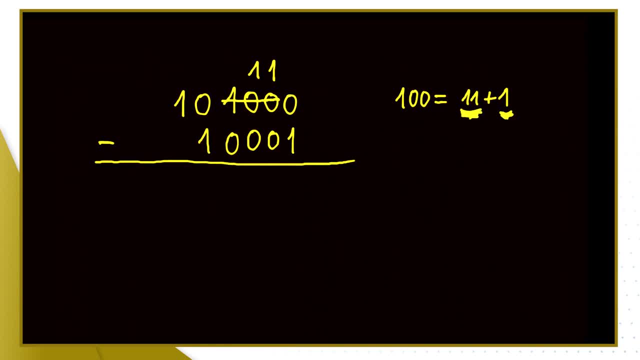 And this one here is going to be borrowed to the smaller place value, So this 0 becomes 1, 0. That's 2.. Now we do 1, 0, take away 1.. 1, 0, take away 1.. 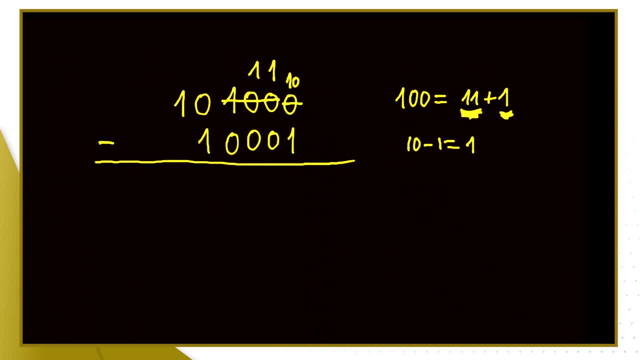 That's 2 minus 1.. So that is 1.. That means that 1, 0, take away 1 is 1.. And now I look at the next column. I've got 1, take away 0.. 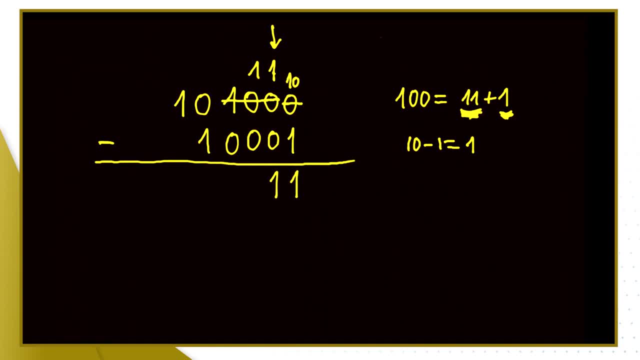 That's fine. 1, take away 0 is just 1.. Next column: 1, take away 0, also just 1.. Next column: actually I haven't got anything there because I should have put a 0 there. 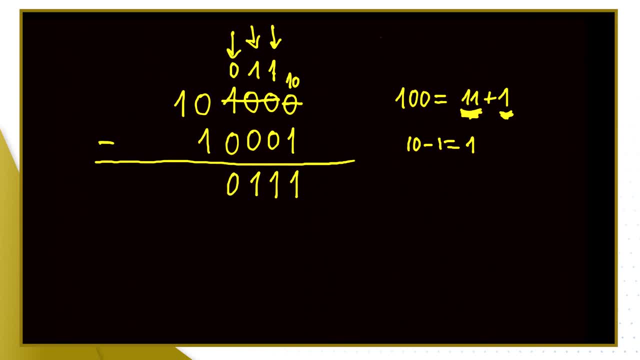 I've got 0, take away 0.. That's just 0.. Next column: I've got 0, take away 1.. 0, take away 1.. Same problem as before, but not an issue, because we can borrow. 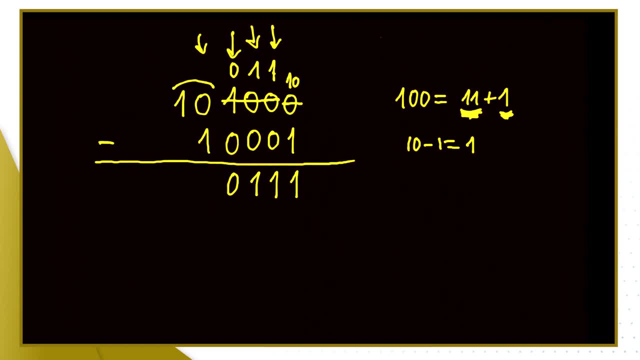 And in fact we've got 1, 0,. take away 1.. That is 1.. That's it. That means that 1, 0, 1, 0, 0, 0, take away 1, 0, 0, 0, 1 is 1, 0, 1, 1, 1 in binary. 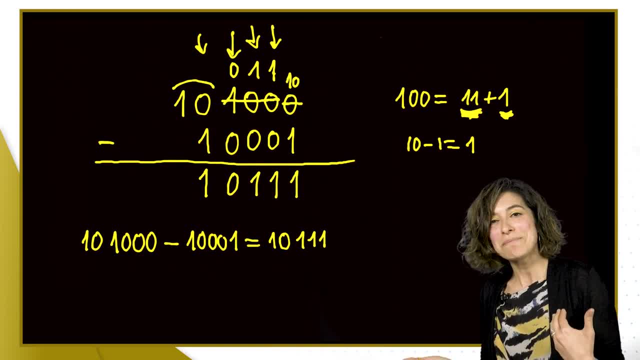 Now we can check if this is right or not. Let's do the addition in binary backwards to see if we've got the right sum. So if we add these up we should get the big guy. So let's do it here on the side. 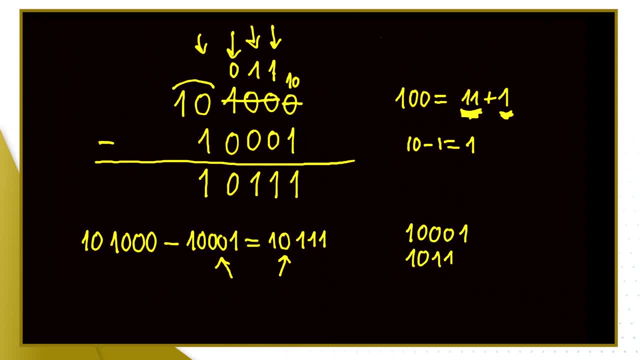 1, 0, 0, 0, 1.. 1, 0, 1, 1, 1.. Let's add it up: 1 and 1 is 2,, which is 0, 1.. 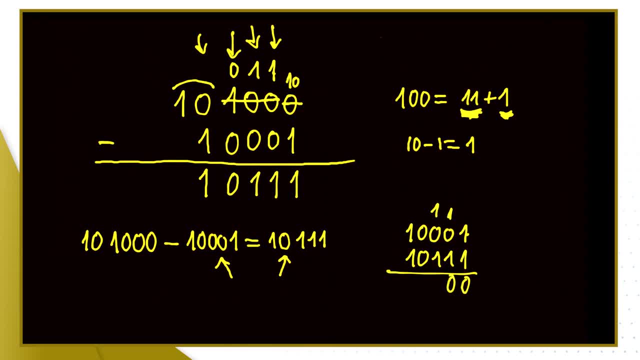 1 and 1 is 2,, which is 0, 1.. 1 and 1 is 2,, which is 0, 1.. 1 plus 0 plus 0 is just 1.. 1 plus 1 is 2,, which is 1, 0.. 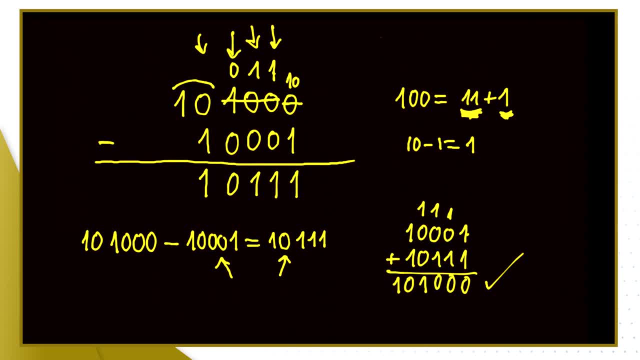 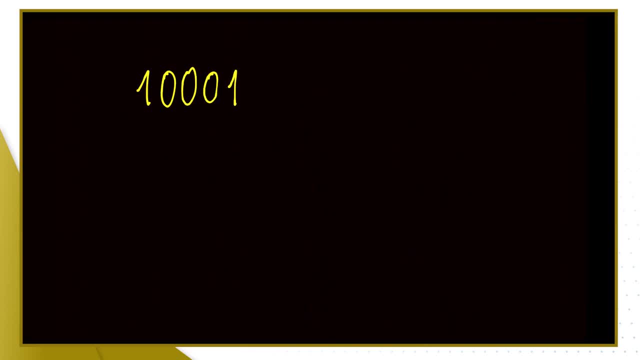 And that is the number we started with, so correct. Next, let's do 1, 0, 0, 0, 1, take away 1, 1, 1.. So 1, take away 1 is just 0.. 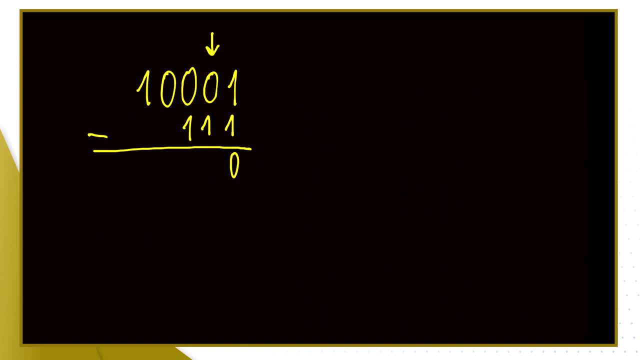 The next place value, we've got 0, take away 1, which we can't do. So anyway we've got to borrow And again we're going to borrow from that number of greater place value. So again we observe the 1, 0,, 0,, 1.. 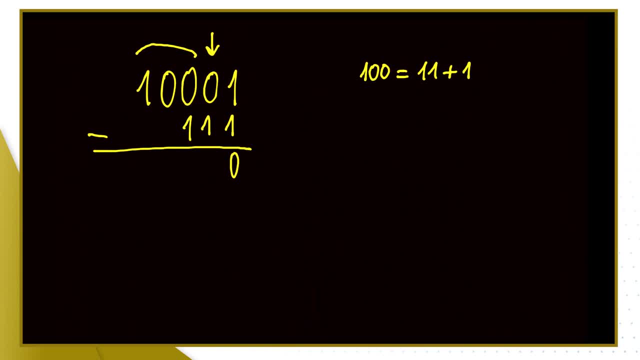 0 is 1, 1, add 1.. So we're going to replace that 1, 0, 0 by 1, 1.. And we're going to replace this 0 here that was too small- by 1, 0.. 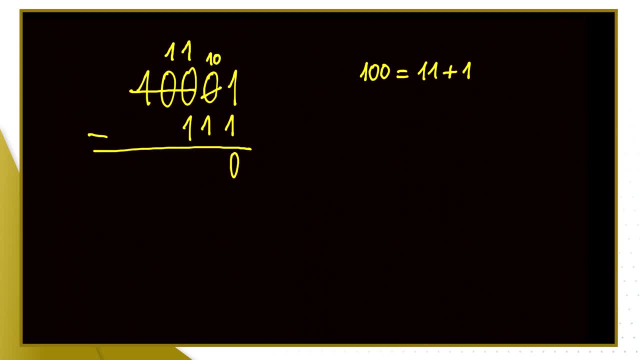 That's where the borrowing is taking place. And now we do 1,, 0,, which is 2.. Take away 1,, that's 1.. And now 1,. take away 1, is just 0.. 1,, this 1 here, take away 0, is just 1.. 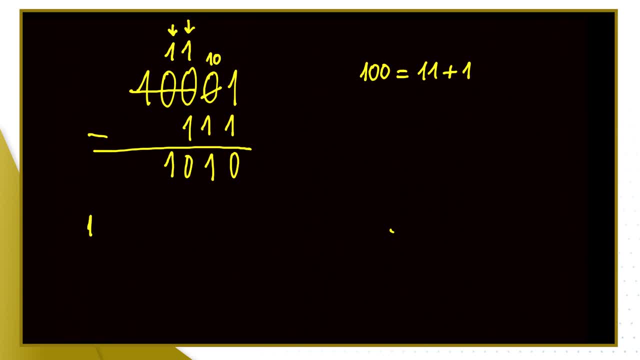 And over here we have nothing. so we're done: 1, 0, 0, 0, 1,. take away 1, 1, 1 is 1, 0, 1, 0.. 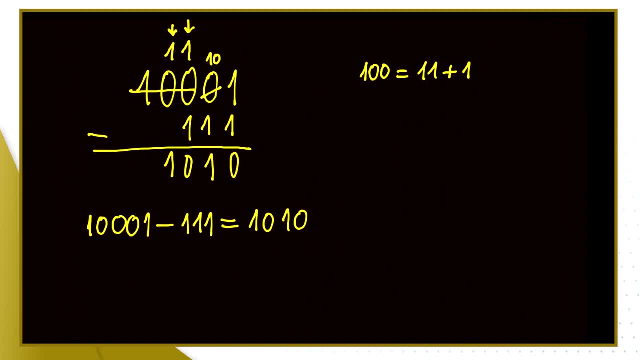 And let's check that we did the right sums. Just add up the 1, 0, 1, 0 with 1, 1, 1.. And 1, 1, 0, 1, 0, 1, 0,, which is the number we started with. 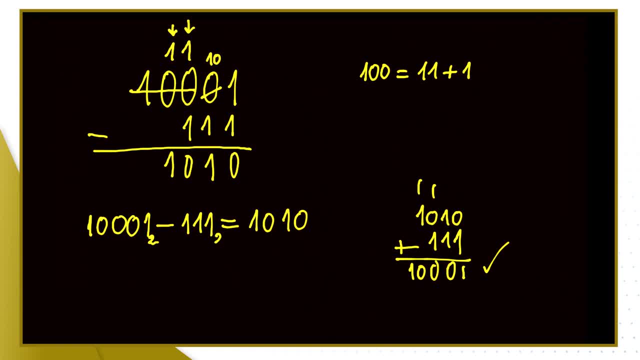 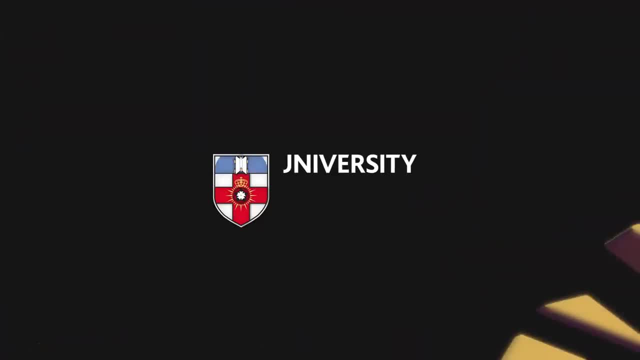 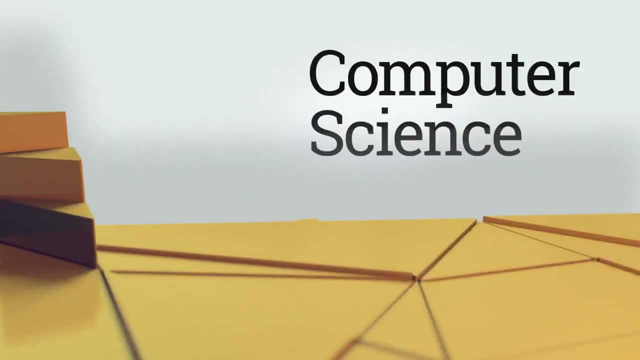 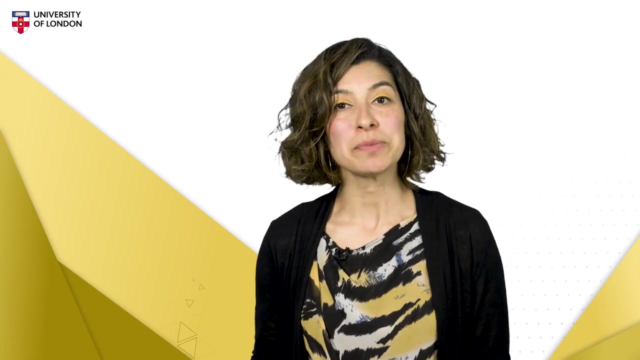 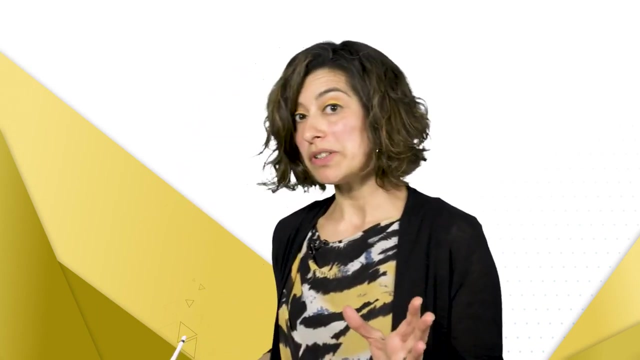 So it is correct. Let's see who's here And there we are. subtraction in binary. We're now going to multiply numbers in binary. Let's look at a simple multiplication first. Say we're doing 1, 1, 0, 1.. 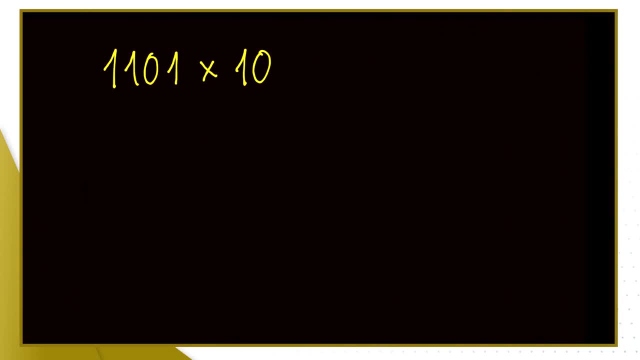 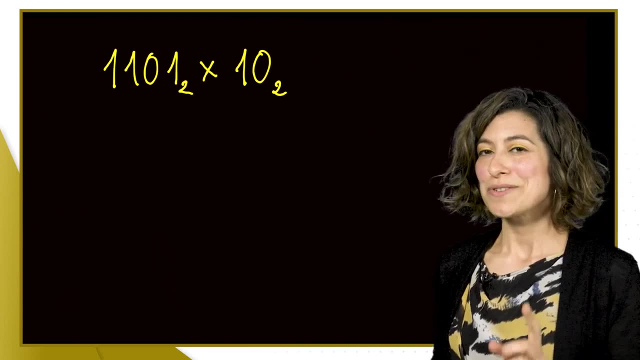 And I just want to multiply that by 1, 0.. It's not 10, it's 1, 0.. And that is all in binary. I talked about 10 just as a reminder of how would we do this in decimal. 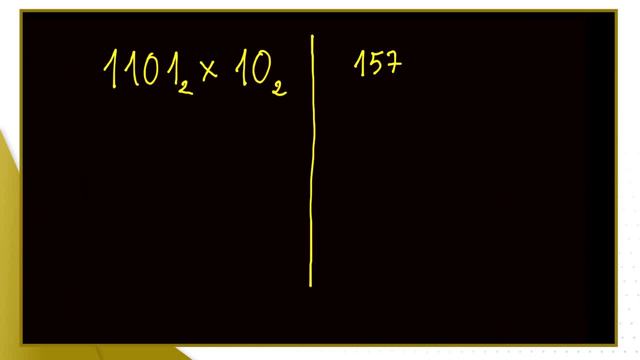 I'm going to do it on the side. If you have 157 and you were going to multiply by 10,, this is a proper 10.. By 10, you would just increase All the place values by a factor of 10.. 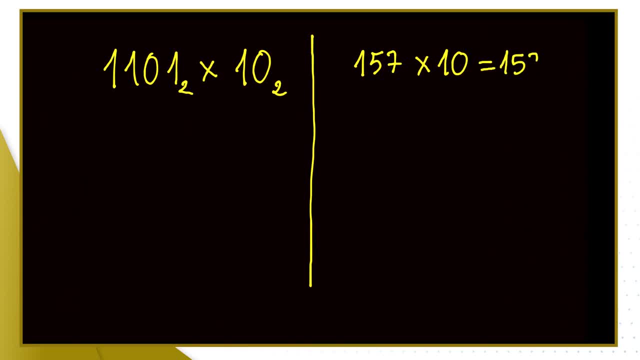 So you would just do 1, 5, 7, 0.. As in the 7 is now goes from being in the place values for the units to the place value of the tens. The 5 goes from being the place values for the tens to being the place values for the hundreds. 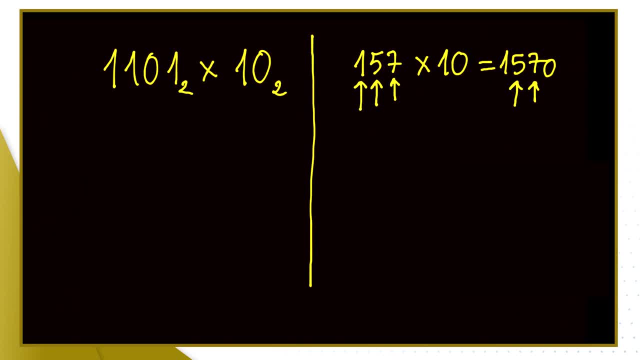 And that 1 goes from being the place value for the hundreds to the place value for the thousands And you stick a 0 in the units place value. So that's what you do in decimal. Now back to binary. This 1, 0 means 2.. 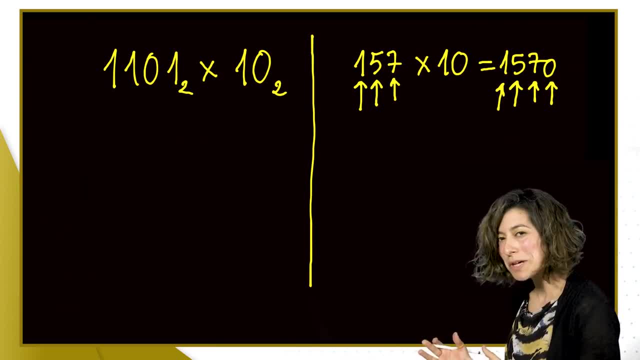 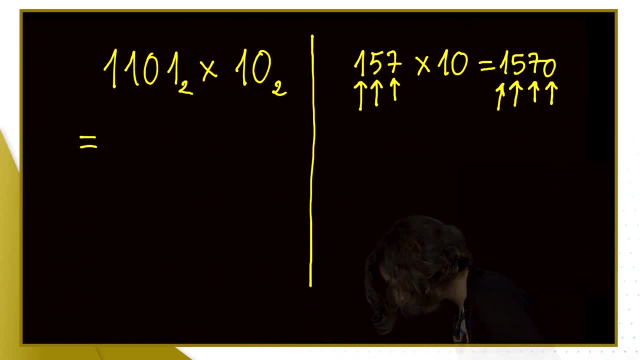 But it has the same idea as multiplying by 10 in decimal. It's that you shift the number 1 place value to the left. So that means it is 1, 1, 0, 1, 0 in binary. 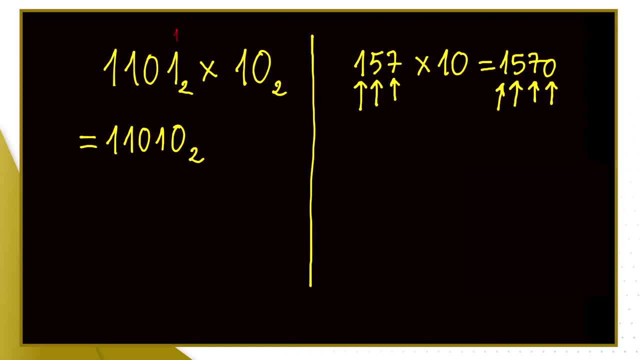 This one is a place value for 1.. So it becomes a digit on the place value for 2s. This 0 is a place value for 2s. It goes to the place values for 4s. This one place value for 4s becomes place value for 8s. 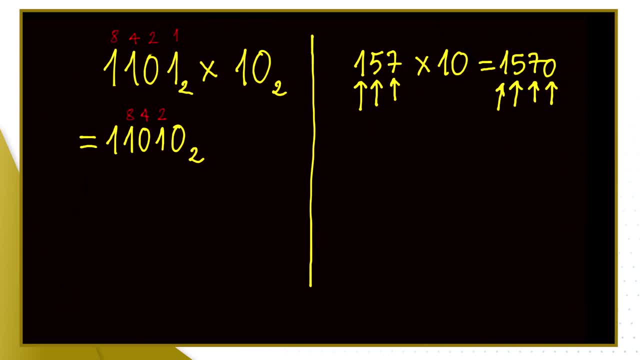 And the 1 on the place values for 8s becomes the 1 on the place values for 16s. So that's what happens, And I put a 0 on the empty space for the place values for 1.. So this is what happens when you multiply by 1, 0 in binary. 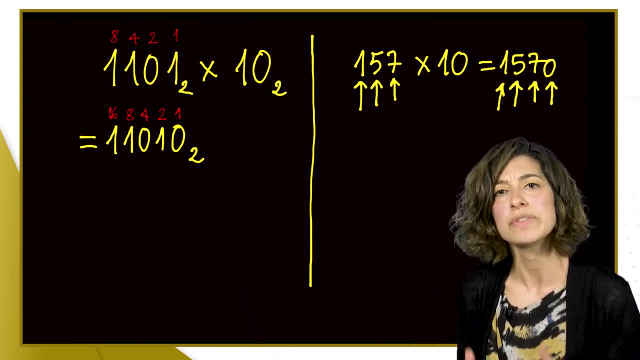 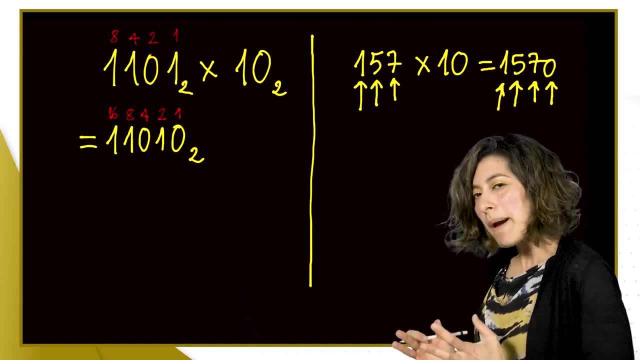 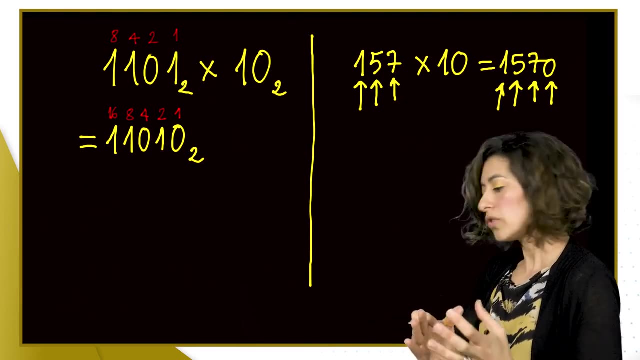 When you multiply by 2 in binary, When you double numbers in binary, If you double it again you're going to shift the digits again 1 place value. So multiplying by powers of 2 in binary just shifts the number place values to the left. 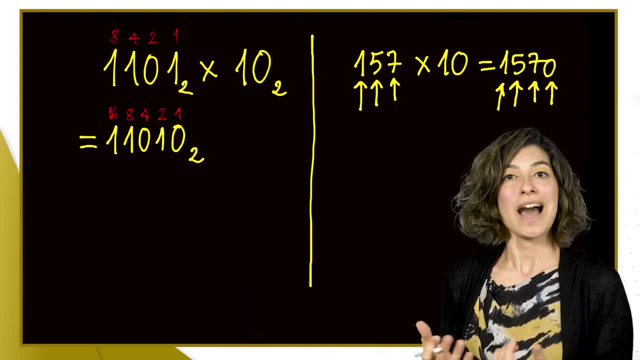 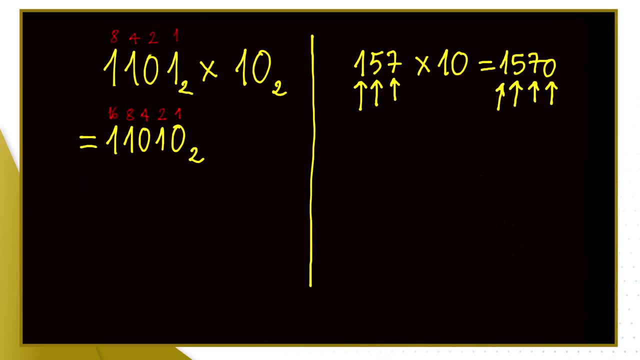 So this is the main idea: to understand how multiplication works in binary. It's a lot easier to multiply in binary than it is to multiply in decimal- actually, I'll show you how. So let's look at doing a little bit more complicated multiplication. 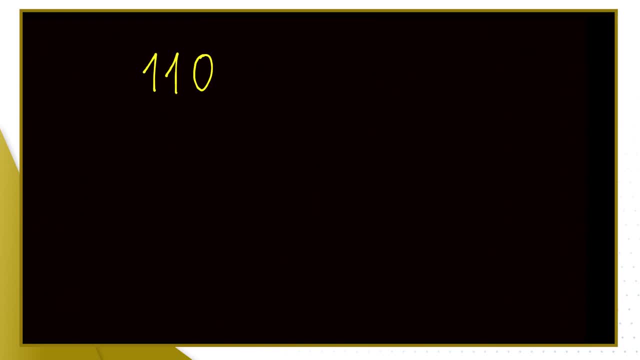 Say we're doing 1, 1, 0, 1. Put another 1. Multiply by 1, 0, 1.. We can do the algorithm in this way. But let's see what we should expect. The multiply here: 1, 0, 1.. 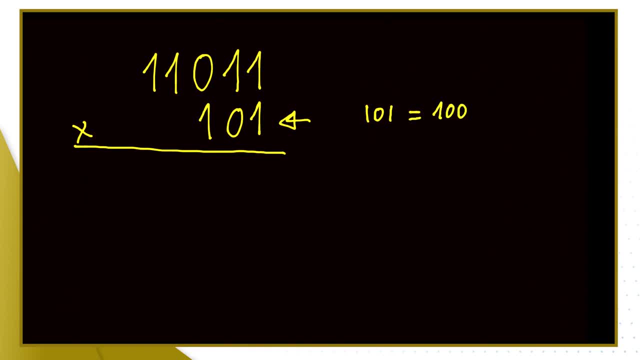 1, 0, 1 just means 1, 0, 0, add 1.. And multiply a number by 1 changes nothing, just repeats the same number. Multiplying the number by 1, 0, 0 is going to shift all the digits. 2 places to the left. 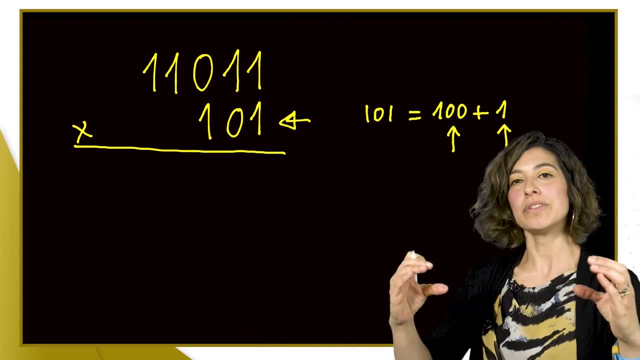 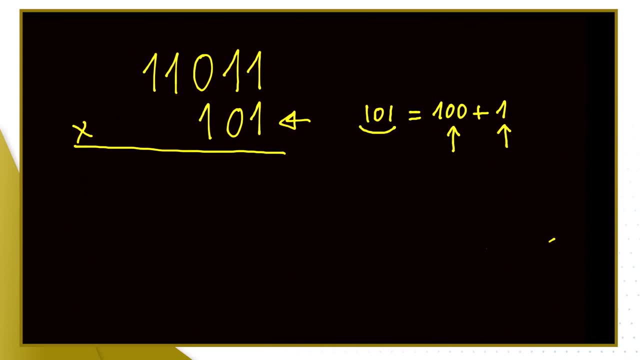 So basically, what we're going to do is we're going to add a copy of the number, with a copy of the number shifted 2 places to the left. That's always going to happen. Multiplying by 1, 0, 1 is going to be multiply 1, 1, 0, 1, 1 by this guy. 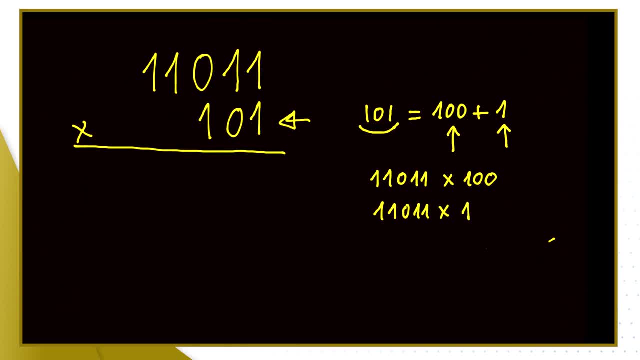 And multiply 1, 1, 0, 1, 1 by 1.. And then add the results, So 1, 1, 0, 1, 1, with two zeros at the end. And this is just a copy of its own. 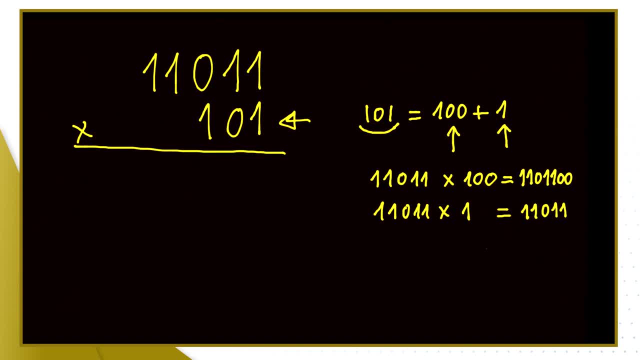 Now I haven't lined up the place values correctly there. I'm going to try and do it now. So 1, 1, 0,, 1 and 1. And then adding these guys up will be That's what we should expect. 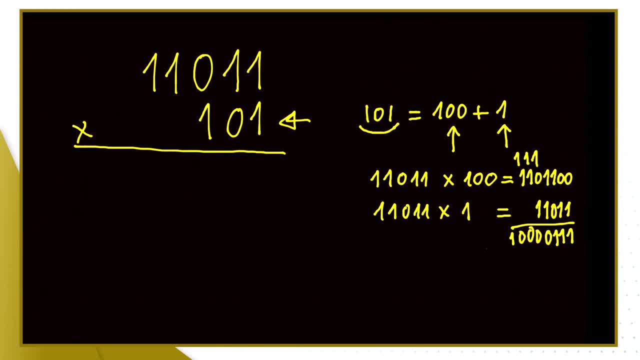 But I'm going to do that again on the main calculation here. So I mean, let's do it here. So I multiply this top number by this first one, And that means just repeating the top number. So 1, 1, 0, 1, 1.. 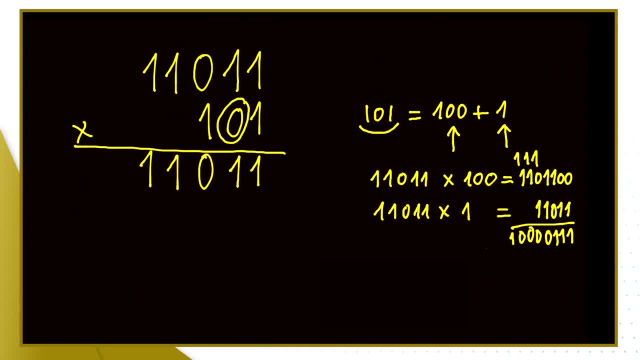 Now, this zero here means just leave another place value blank. So I'm going to leave that place value blank And then multiply by this one. here It's going to be copy the number again, but starting from here. Okay, So I'm going to do 1, 1, 0,, 1 and 1.. 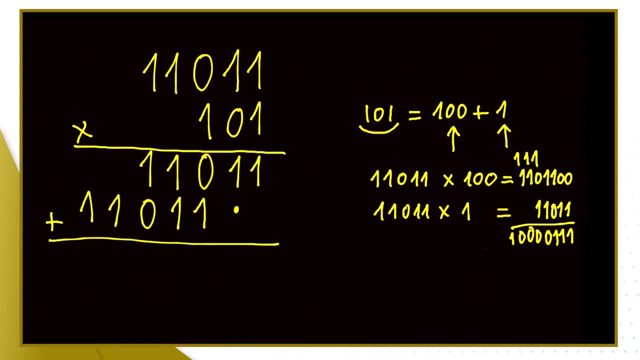 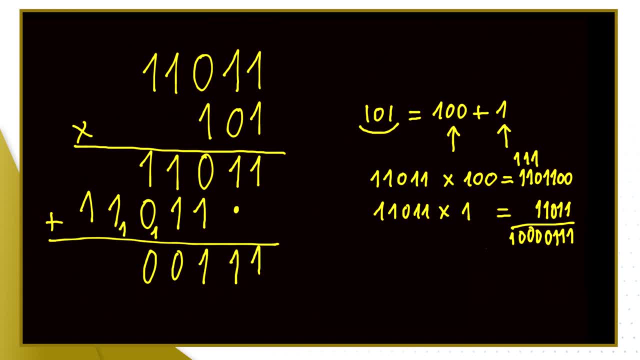 1 plus 1 is 1, 0. Another 1 there, 1 plus 1 is 1, 0. So I put another 1 there And 1 plus 1, 1, 0. And I've got it. 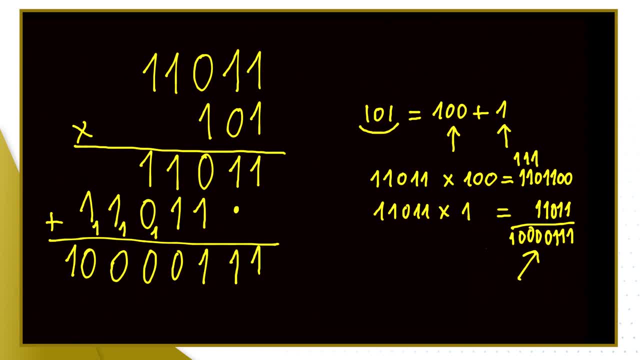 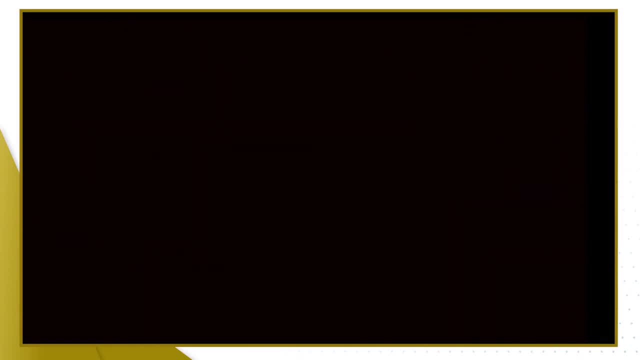 Which is what we had predicted over there. Now we're just going to do one more example to see if we nail it. Okay, So I've got 1, 0, 1, 1, 1.. Multiply by 1, 1.. 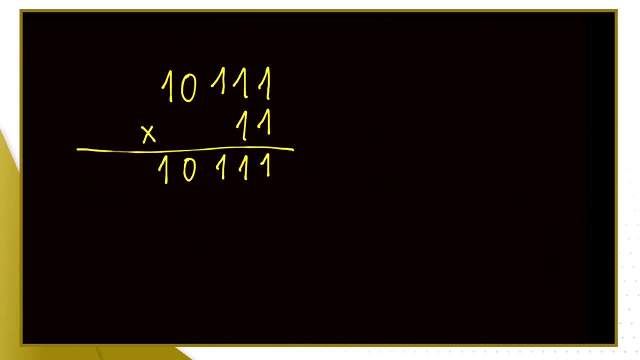 So copy the top number. And now for the second one here, copy the number again, but one place value shifted to the left. So 1, 1, 1, 0, 1.. Add them all up. 1 plus 1 is 2, which is 1, 0.. 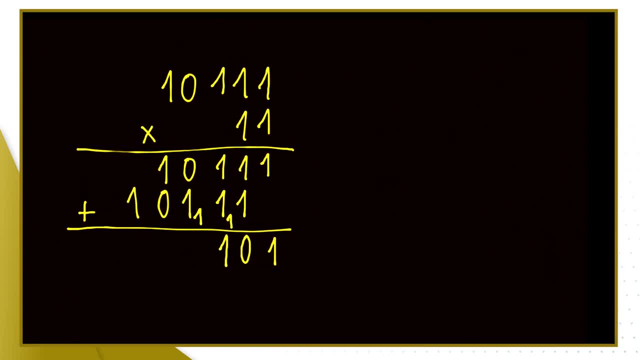 1 plus 1 plus 1 is 3, which is 1, 1.. So carry, 1 plus 1 is 2, which is 1, 0.. So 0 there and a 1 there. 1 plus 1 is 2, which is 1, 0.. 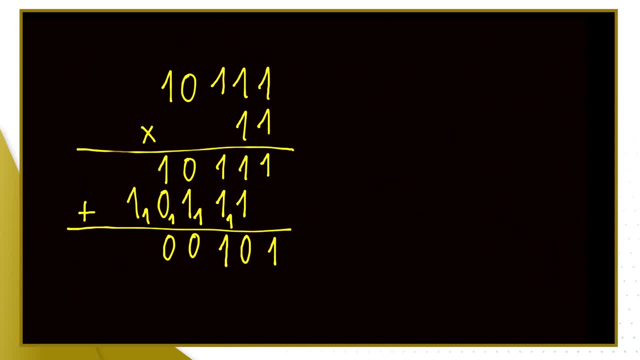 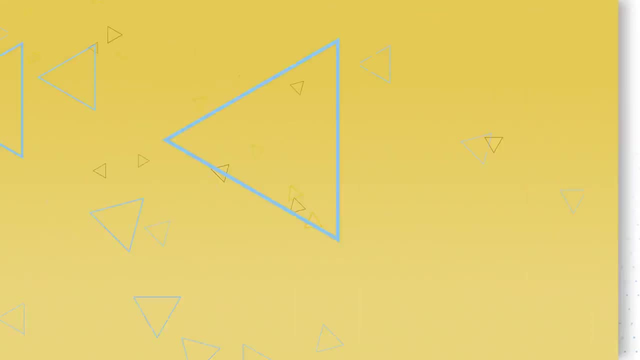 And I put that one there. 1 plus 1 is 2, which is 1, 0. So the result: 1, 0, 1, 1, 1 in binary times 1, 1 in binary equals 1, 0, 0, 0, 1, 0, 1 in binary. 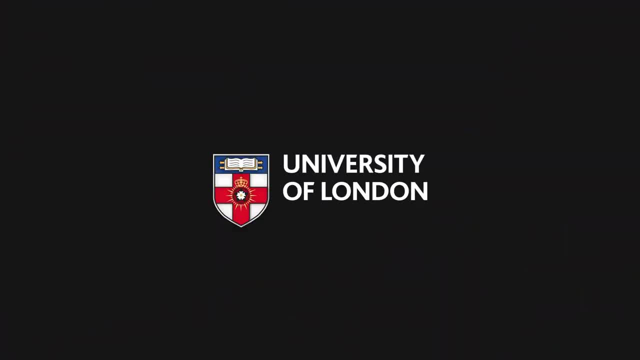 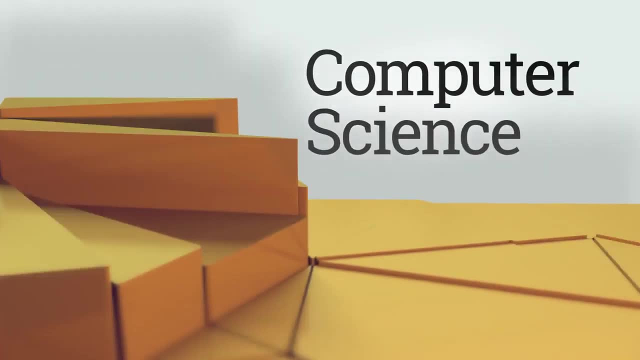 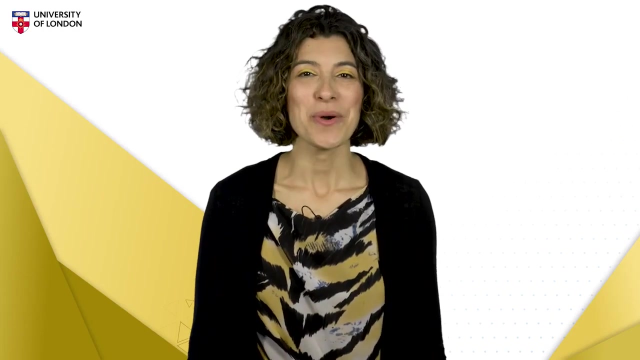 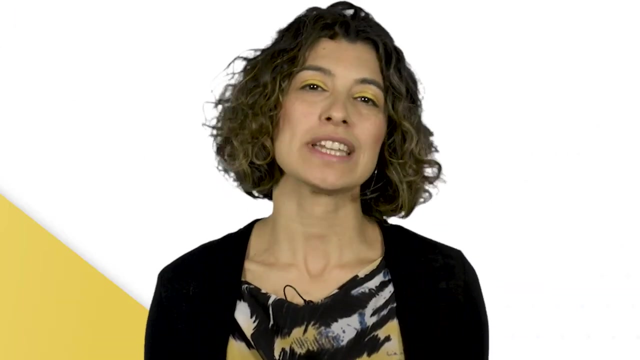 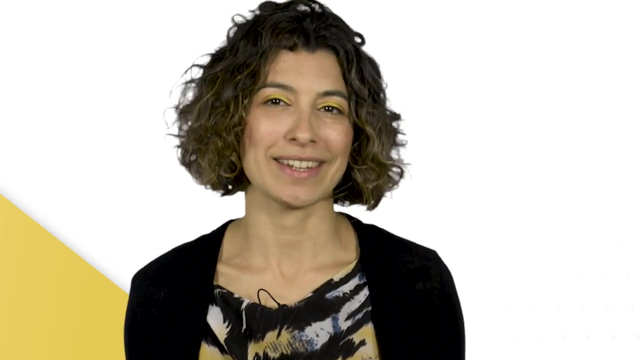 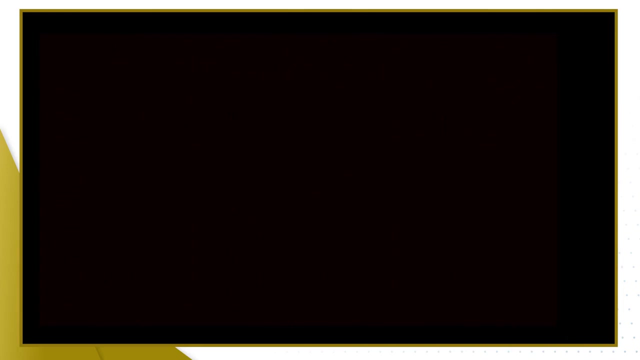 And that's done. Hello, there We're looking at some examples of your work in writing the algorithms. Let's look at converting between decimal and binary. We're going to write the algorithm alongside looking at an example. We have the binary number 1, 0, 1, 1, 1 and we're going to convert it to decimal. 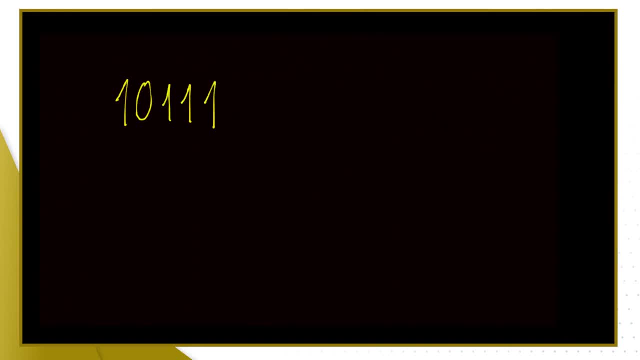 1, 0, 1, 1, 1.. We're going to convert this number to decimal. We look through the place values which are right here. So place values 1,, 2,, 4,, 8,, 16.. 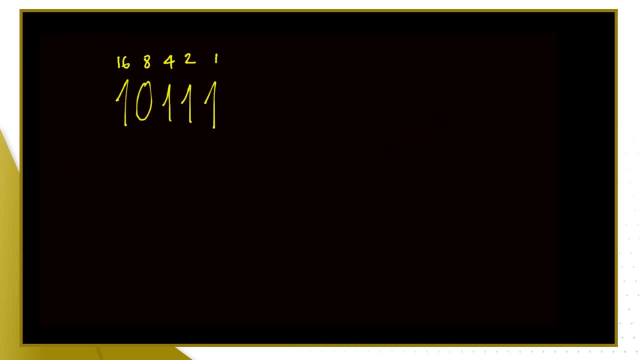 We're going to do that in general for our algorithm. Let's focus on that example. For the conversion, All we have to do is to add up a place value when we have a 1. That's all we do. So we have that decision there to do. 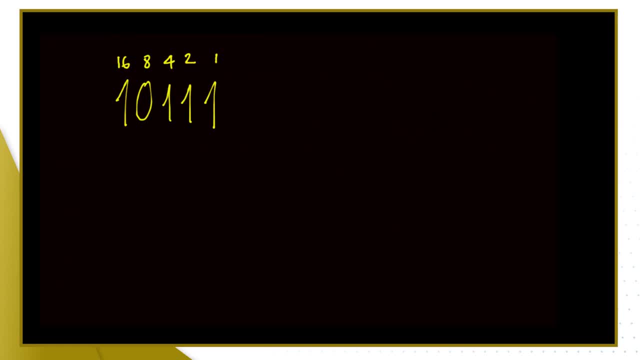 So let's bear that in mind. so we write that step, that decision, in the algorithm. So in this example we're going to add up the 16, the 4, the 2 and the 1. So we're going to need a container to hold that sum. 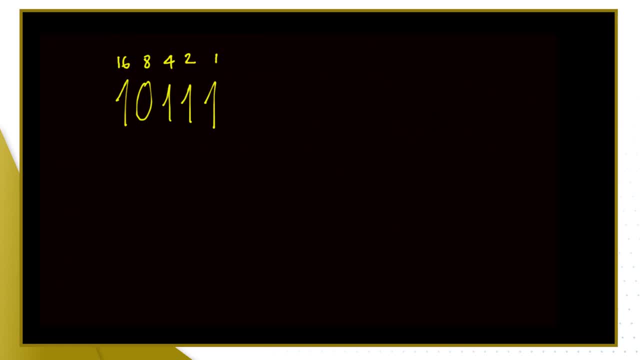 And we're going to do it on a loop. Now it might help if you picture that we have these values on a bit of paper. We're going to have a mental bit of paper to hold the value of a number. That it's like a variable. 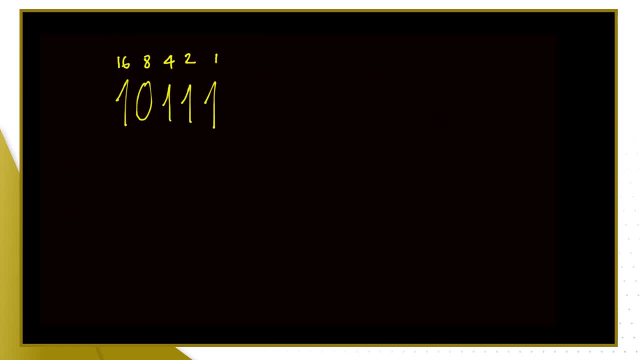 So let's bear that in mind as we go along. So, to start with, we need to know which place value we begin. I want to start with the largest place value. I want to start On the left of the number. I want to start on the place value 16 here. 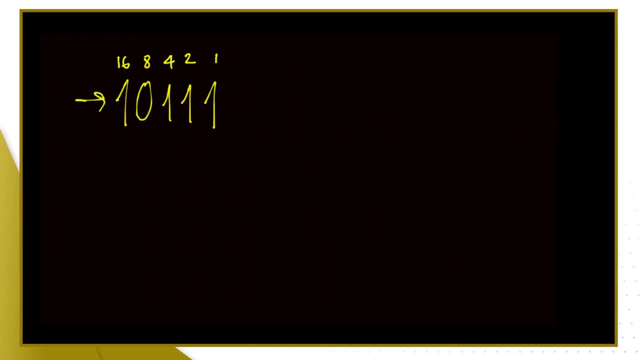 So how do I know where to start? I want to start on that place value 16.. I need to know how many digits I've got. So the first thing is work out how many digits we have. Count the digits of the number. 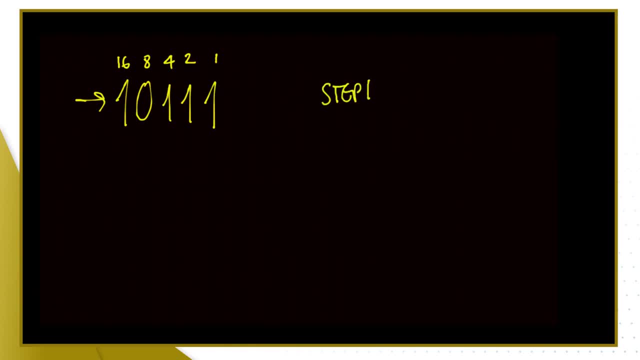 So our first step is going to be as simple as count the number of digits. Okay, Okay, Count the number of digits. Now we count, but it's not enough to count. We need to hold that value in the variable, Which is like a bit of paper, if you want. 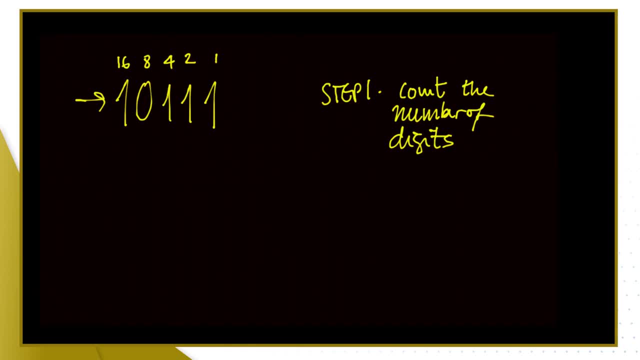 Or a little box. Where are we going to keep that? We're going to call n this value. Okay, So Make big: N equals to this number. I am using a rather informal language here, And it's fine. We are precise about the things. we need to be precise. 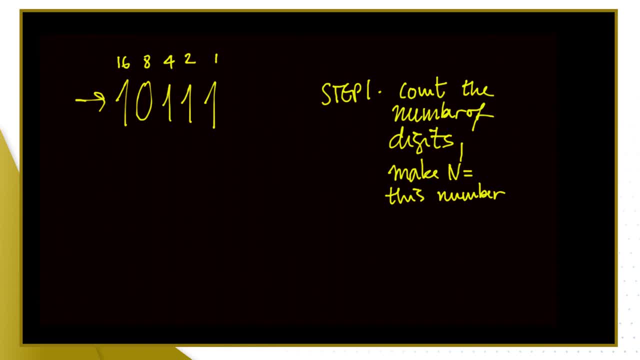 And the other parts. we can be quite informal in our algorithm. This is not a formal algorithm class, Right? So we do that In our case. we count how many digits We have: 1,, 2,, 3,, 4,, 5 digits. 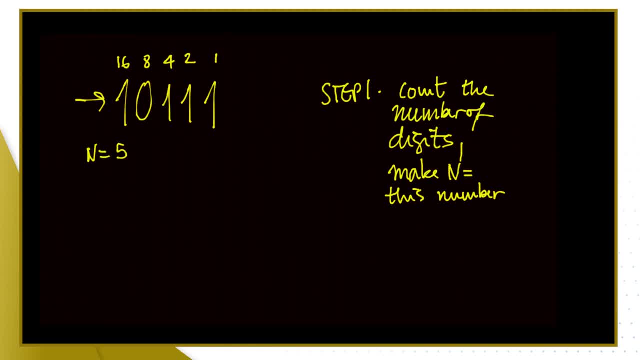 Our n is 5.. Okay, And how does that help with what we're going to do next? We're going to start with the large place value. In our example, the large place value is the 1 on place value 16.. How does 16 relate to that? n equals 5?. 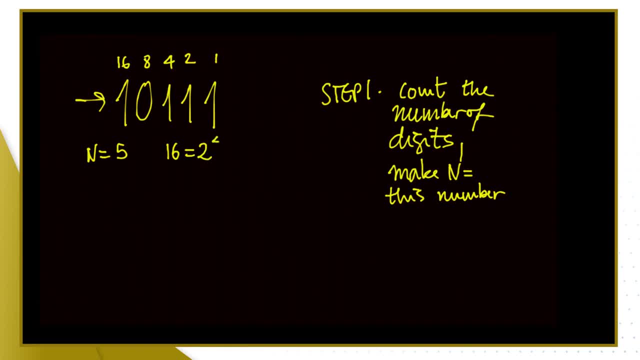 16 is 2 to the power of 4.. It's 1 less than the 5.. That means the first place value we're going to add is the 2 to the power 9.. 2 to the power, not n, but n minus 1.. 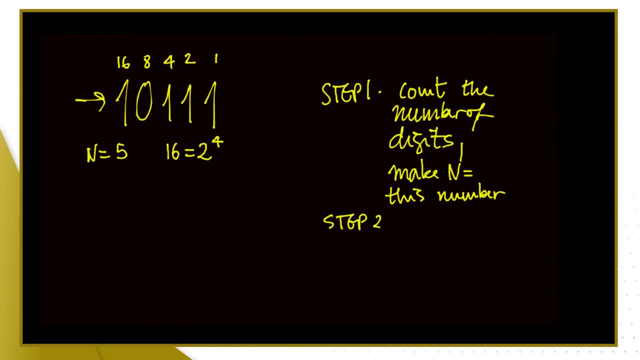 So I'll say, on step 2, for now, We're going to add up the value of 2 to the power of n minus 1.. But you are screaming over there Adding where We need a container, don't we? We need another variable to hold the sum. 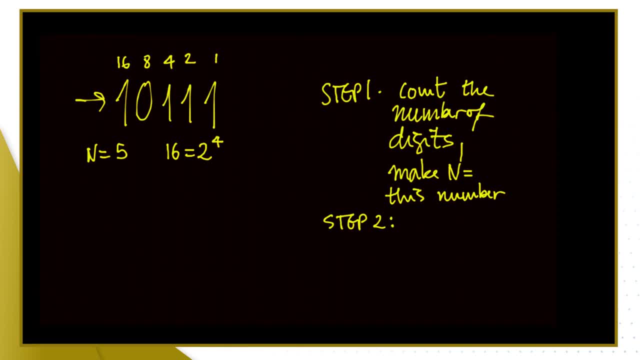 So step 2 is actually going to be: Make a variable sum. Make a variable sum And it's going to be an integer variable Sum And we're going to restart it. Well, we're going to start it with value equals 0.. 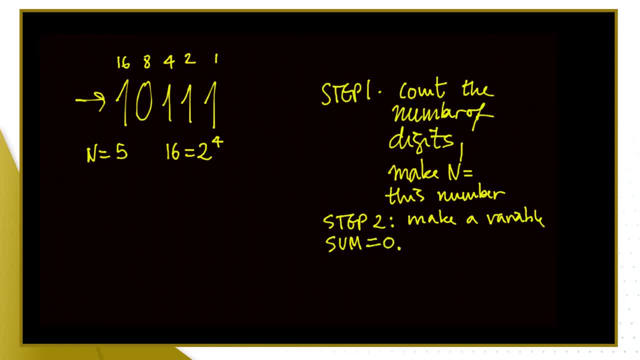 Okay, That's 0.. And now we've got a container. We're going to put in there the first digit. Well, not quite the digit. What we want to put in there is the place value of that leftmost digit. So 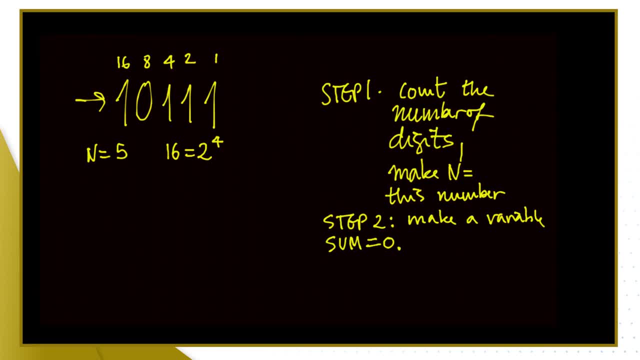 In that case it's 2 to the 4.. We want 2 to the n minus 1.. So step 3 is going to be: Make sum equals to the sum you had there, Which was 0, but it doesn't matter. 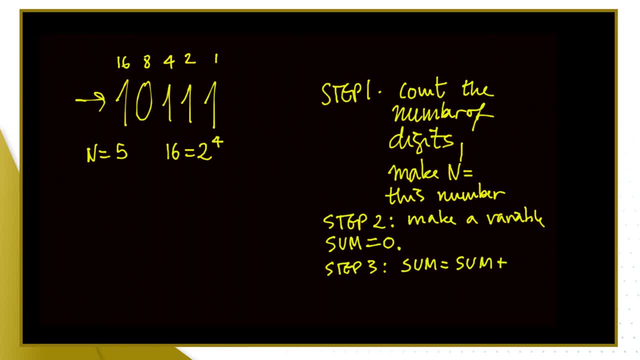 Add 2 to the power of n minus 1.. 2 to the n minus 1.. Great, We got our first little bit in the In our room, In our routine. Now Some of you might be thinking, Shouldn't I multiply that place value by the value of the digits? 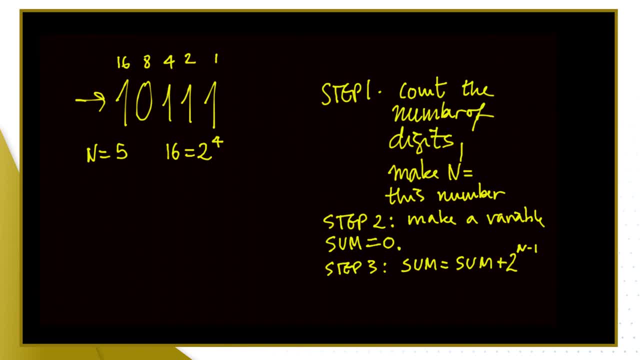 Yes, you are right, We would do digit times the place value. But remember, This is the first time we're doing it. The first digit is the first one You find We're not going to do Run through all the possible zeros into infinity. 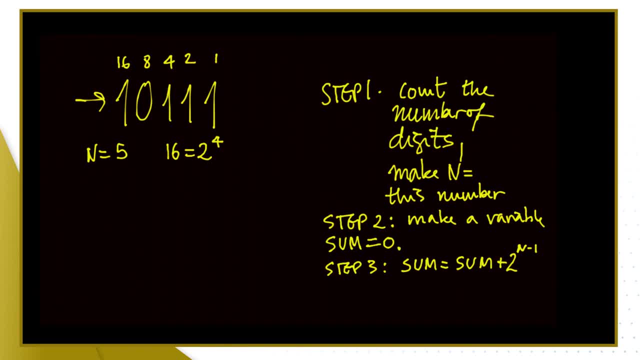 We are going to start with 1.. So in this first step we can skip that. But you might be saying, Shouldn't we future proof this step And have a multiplication by the digits? Let's come back to this thought. So step 3 so far is this way: 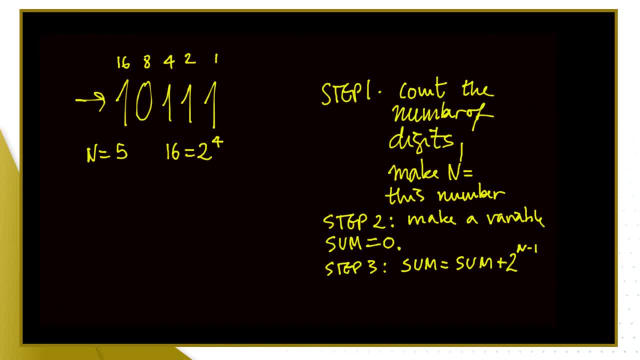 And now we want to move to the next digit. Move to the next digit. How do I do that? We can say Move to the next digit. Let's try and write that down. Move To the next digit. To the right. 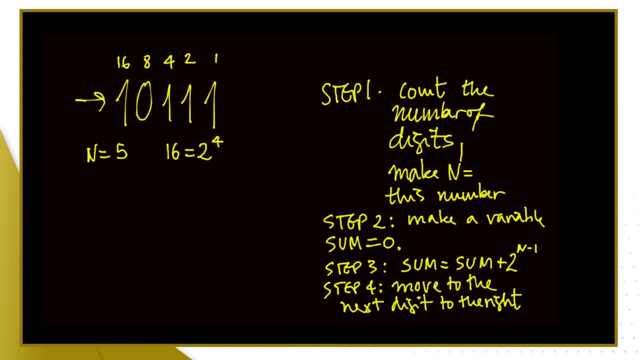 Okay, We can do that. That means we now would be on our example, We would be on place value 8. Which we have a 0. And then what would we do? We would do Because I've got a 0.. 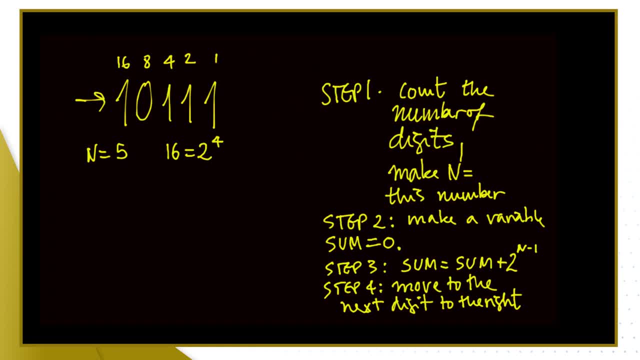 I've got nothing to add to my sum. If I had a 1. I would add again the place value. Okay, We wouldn't do that. So we need to decide, We need to check what that digit is. So our next step: 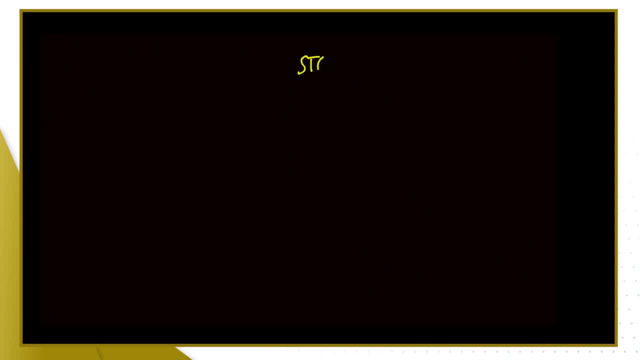 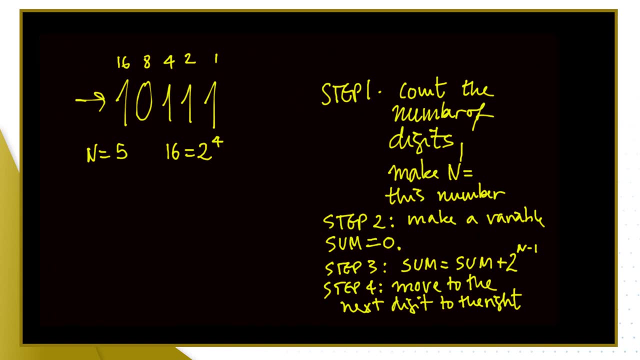 Which I'm going to write. Let's say step 5. We would say: Let's have a look there. What do we say If the digit is 0. Do nothing. If the digit is 1. Add the place value. 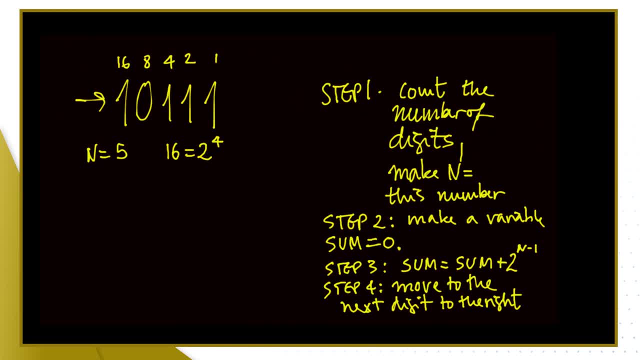 Okay, Now do we know what the place value is? The place value needs to be the other power of 2., A smaller power. So it looks like we have to update our place value holder, Which I think it's enough to use n. 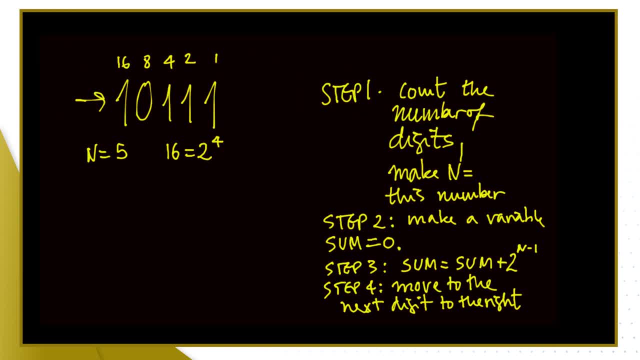 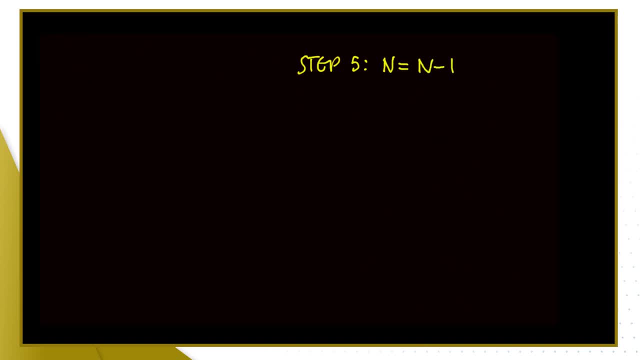 The number of digits And now say I was on the last digit, I want to now go to the next one. So I'm going to say I'm going to make n be 1 less. And now Let's see. 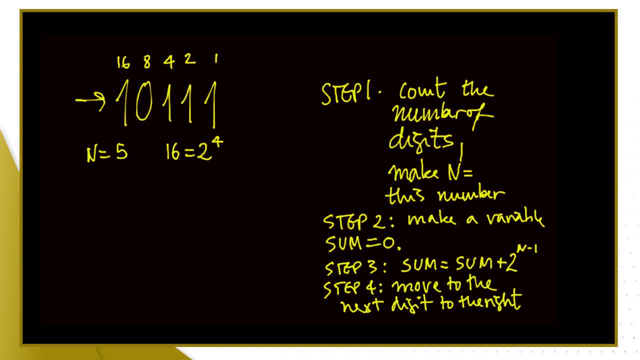 Could we use the steps we had before? Could we go back to step 3. And say the sum is going to be the previous sum Plus the next power of 2.. We could do that, But we did say that we only do that. 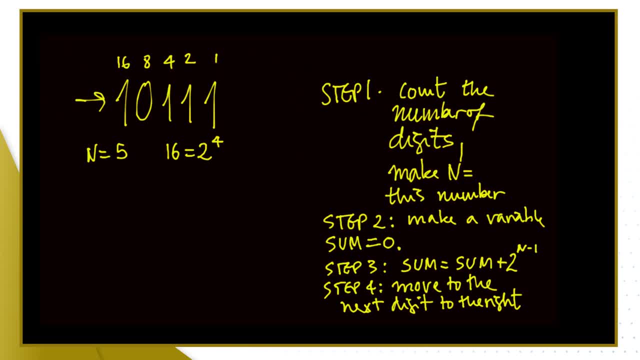 If the digit is a 1. If the digit is a 0. We don't go there. So it looks like we need to redo that step 3.. And have an if. If the digit is a 1.. Do this. 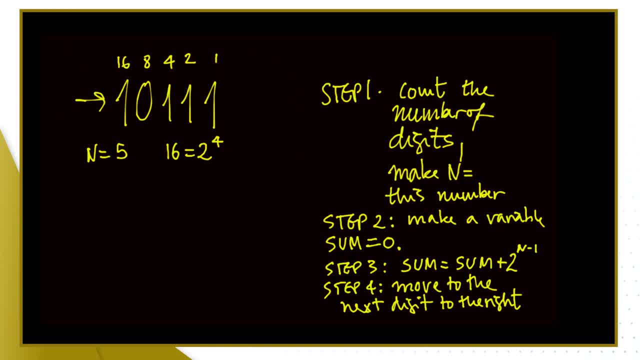 If the digit is 0. Just carry on to the next digit. But you are probably thinking: Have we got a way of keeping hold of digits? Not yet. We're going to need a container for the current digits, So we're going to have to go back. 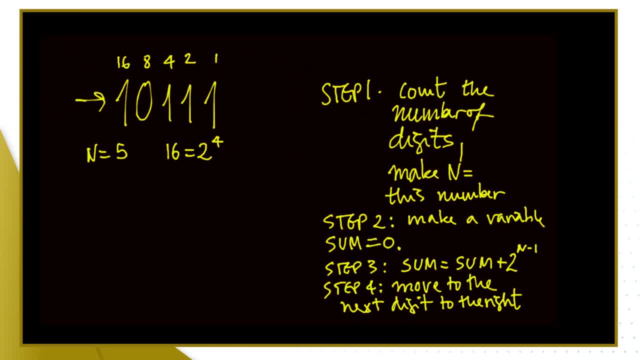 And let's see: On step 1. We did: We count the number of digits. We made n to be the number of digits. Okay, On step 2. We said: make a variable sum equals 0. That's fine. 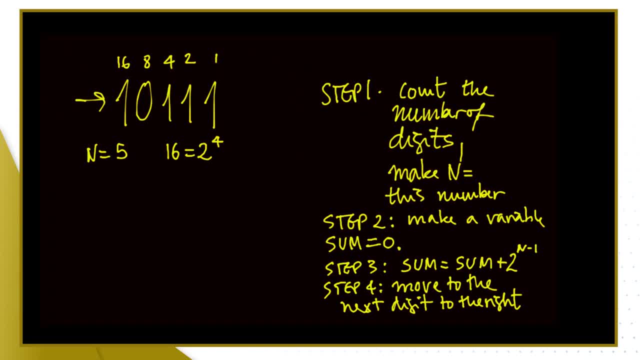 But we also need to make A digit variable. So I'm going to change. Feels like we need to make a digit variable Here: Digit Equals 1.. On that first step, So say, make variables: Sum equals 0.. 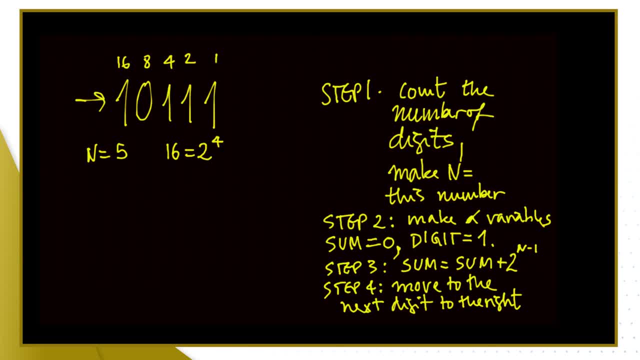 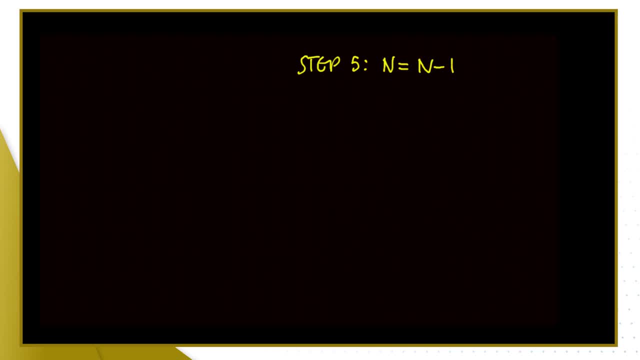 And digit equals 1.. Okay, Maybe that works. So Let's see On step 5.. n equals n minus 1.. So we moved A digit. We now need to go Where We need to go to the step. 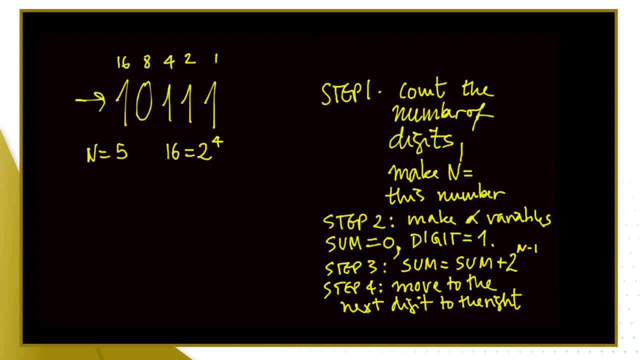 3. But we need to read The next digit. So On step 4. We say: Move to the next digit To the right, So we have Okay, Into Value, Into variable, So We have. 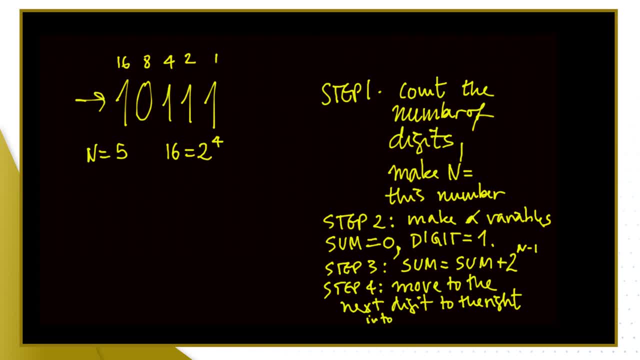 Okay, Into Value, Into Variable, So Digit. Okay, We're kind of reading That, And then We can go back to step 3.. Okay, So on step 5.. We can say Step 6.. 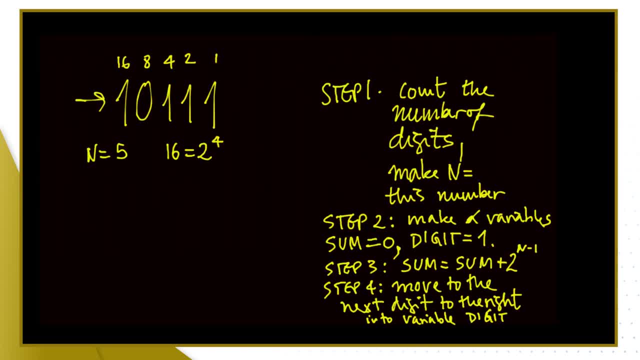 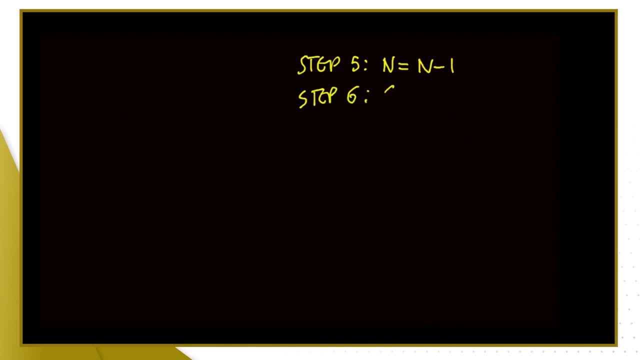 Is Go To Step 3.. And now What happens on step 3.? On step 3. It says: Do the sum, But we only do 1. And 2. And 3.. 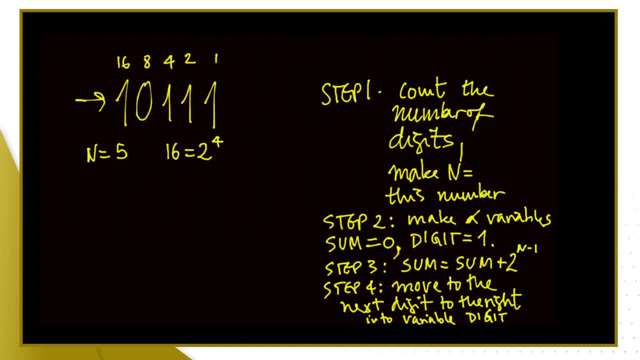 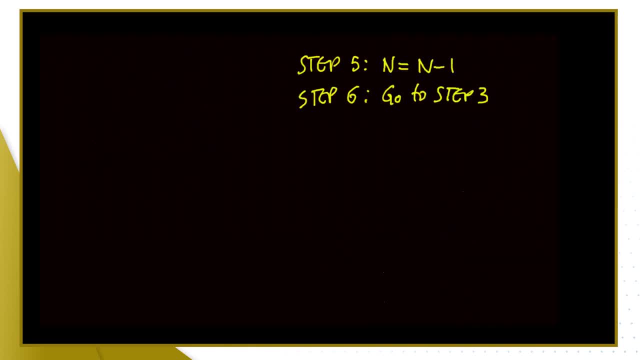 And 4. And 5. And 6. And 7. And 8. And 9. And 10. And 11. And 12. And 13. And. 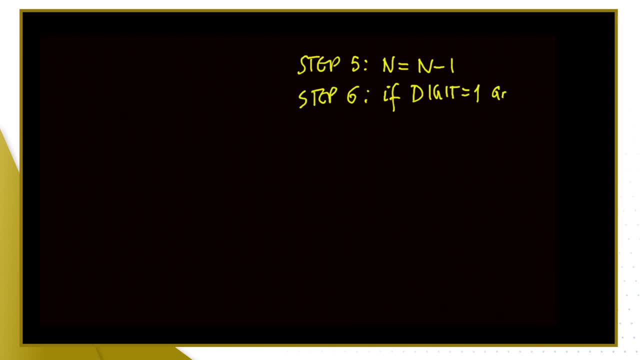 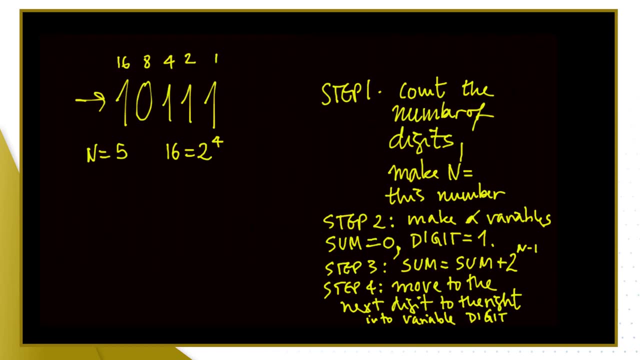 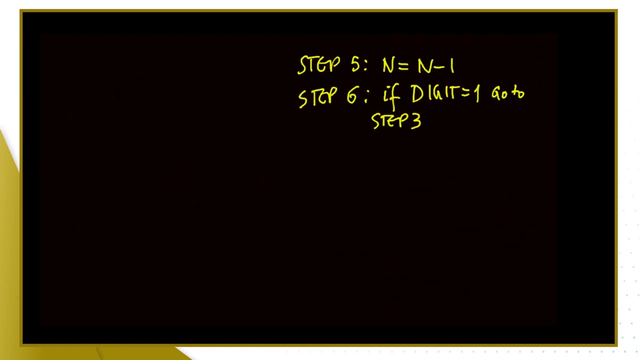 14. And 15. And 16. And 17. And 18. And 19. And 20. And 21. And 22. And 23. And 24.. 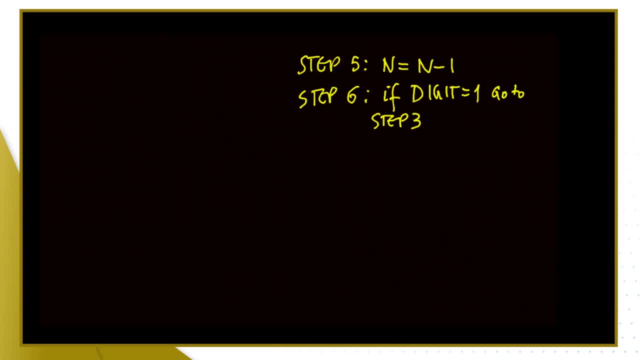 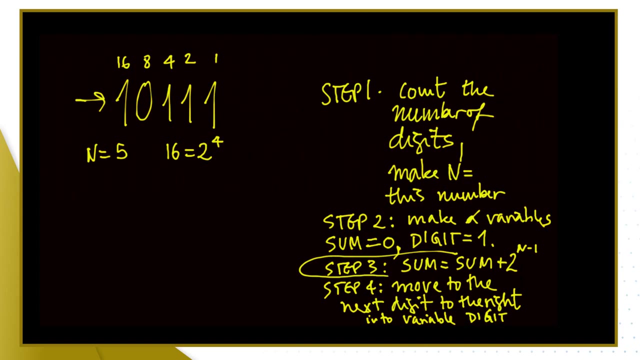 And 25. And 26. And 27. And 28. And 29. And 30. And 31. And 32. And 33. And 34. And. 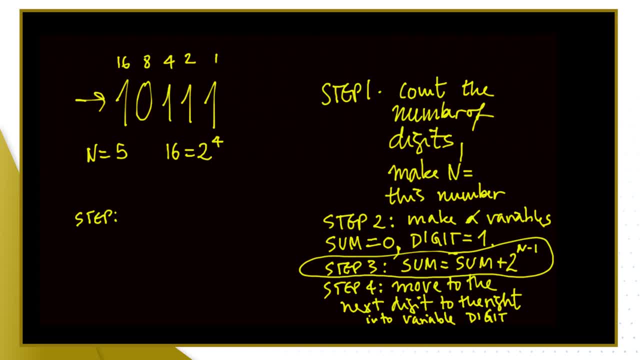 35. And 36. And 37. And 38. And 39. And 40. And 41. And 42. And 43. And 44. And 45.. 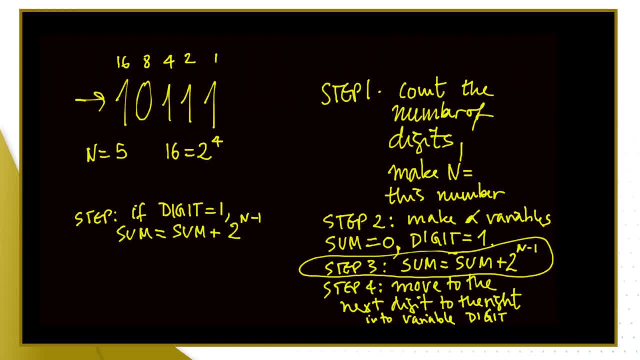 And 46. And 47. And 48. And 49. And 50. And 51. And 52. And 53. And 54. And 55. And. 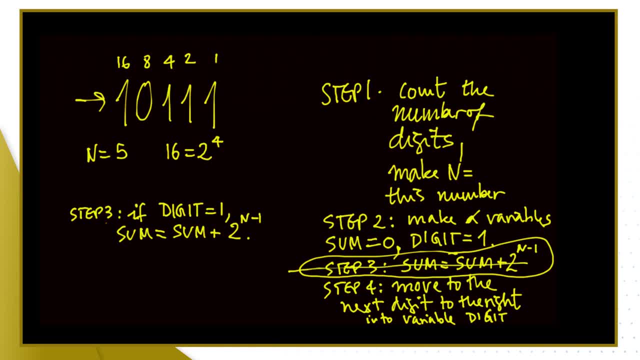 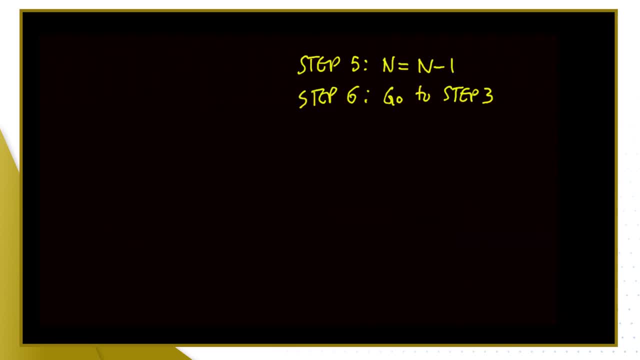 56. And 57. And 58. And 59. And 60. And 61. And 62. And 63. And 62. And 63. And 64.. 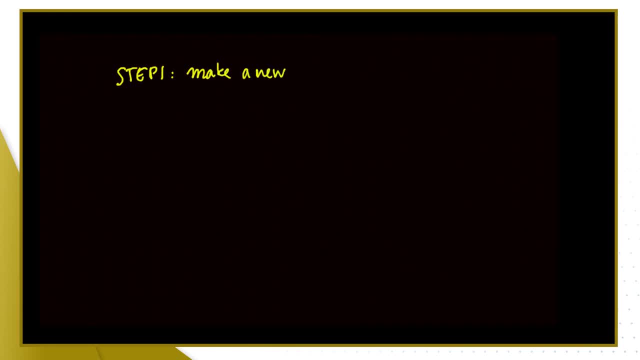 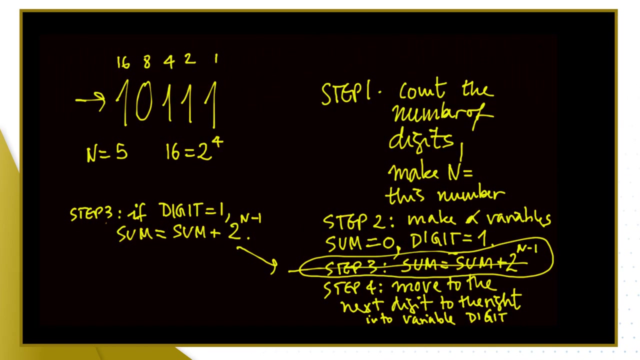 And 65. And 66. And 67. And 68. And 69. And 70. And 71. And 72. And 73. And 74. And. 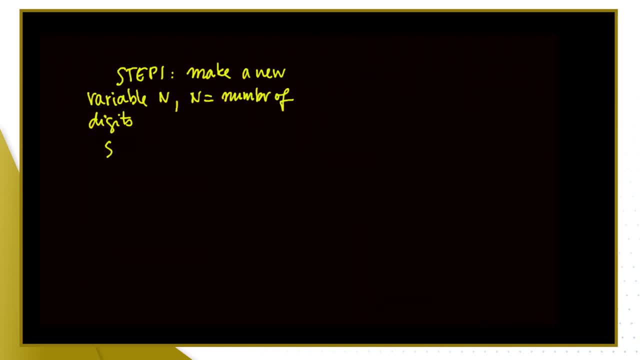 75. And 76. And 77. And 78. And 79. And 80. And 81. And 82. And 83. And 84. And 85.. 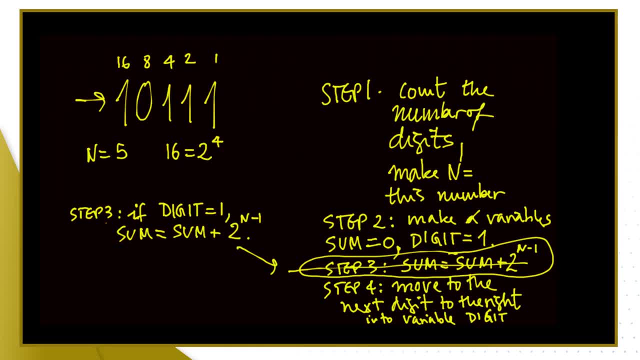 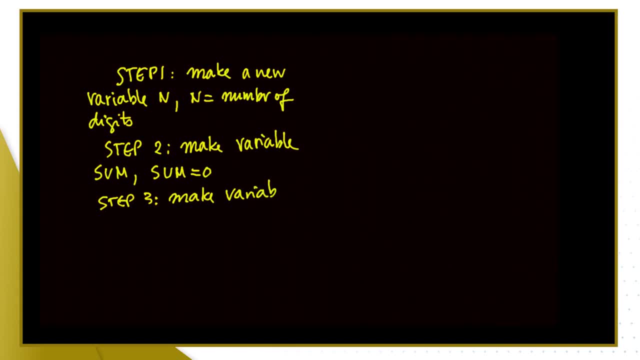 And 86. And 87. And 88. And 89. And 90. And 92. And 83. And 92. St 83. And 94. And. 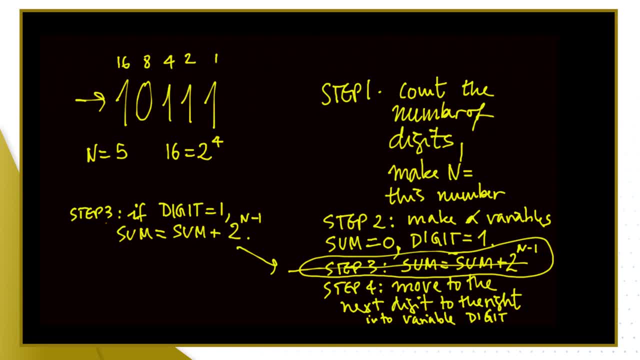 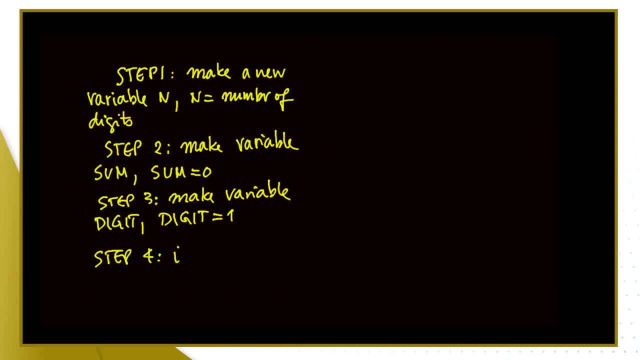 94, 85. And 80. And 96. 85. And 69. And 97. And 98. And ct. the correct power of 2, else we don't need to say else, because else just move on. What happens, moving on? 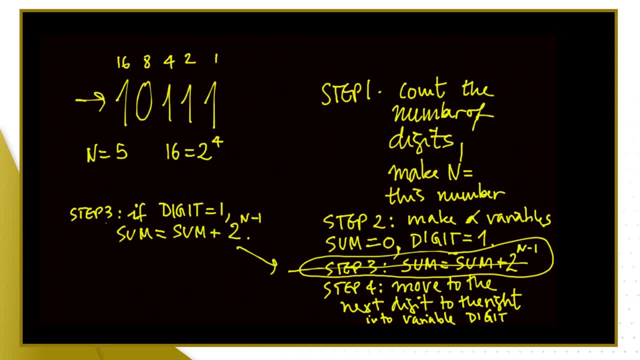 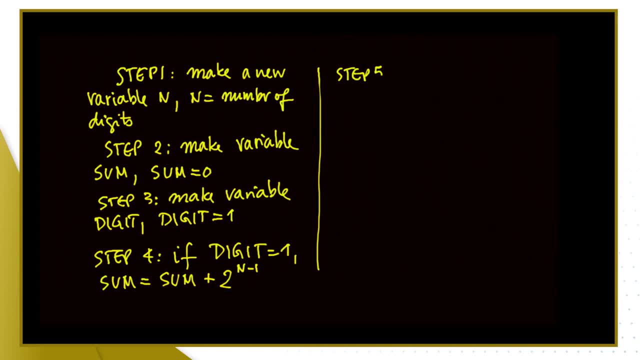 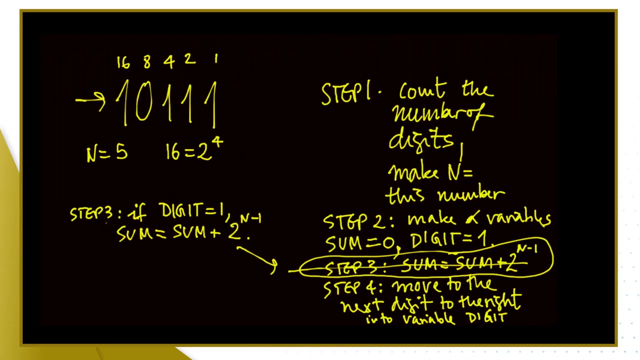 Moving on means go to the next digit. so we're gonna write that step, which is now going to be step 5: move to the next digit, to the right. move to the next digit to the right. store it in the digit that's the variable digit. and now it says: 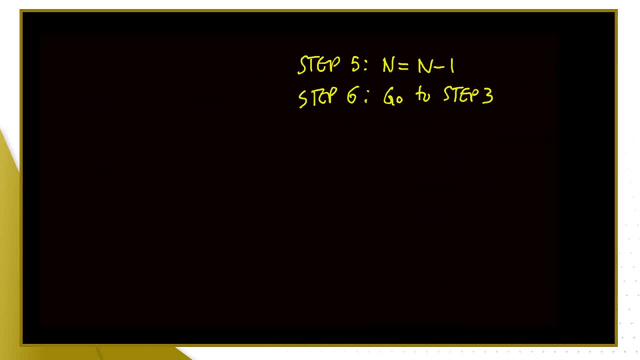 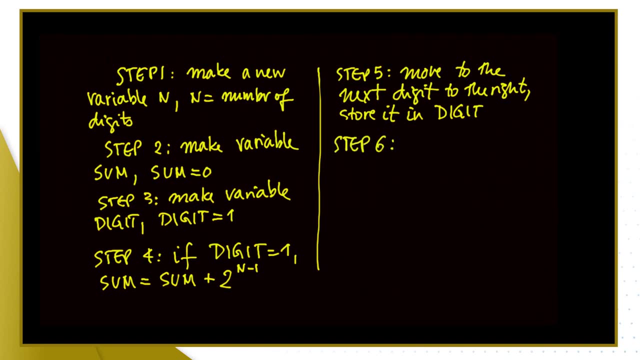 we should go. we now should decrease n and then go to step 3, so step 6 will be: decrease n, so n equals n minus 1, and then the next step will be go to the loop, which now is step 4. go to step 4. 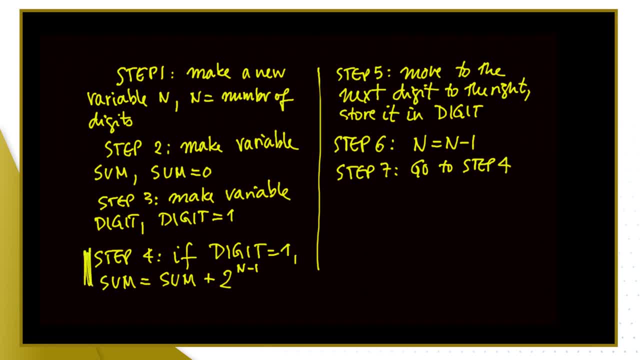 step 4 here. okay, if it's one added, if otherwise, then move on, decrease the n. okay, and now it looks pretty cool. does this work? Is this a good algorithm? Does it stop? Not, so far, we have when do? 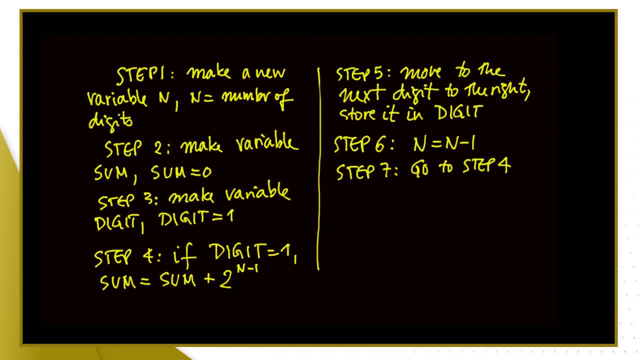 we stop. We stop when we run out of digits. we run out of digits when n is 1. okay, so we need to stop. we need to put an if statement somewhere saying let's stop when n is 1, when we do the final. 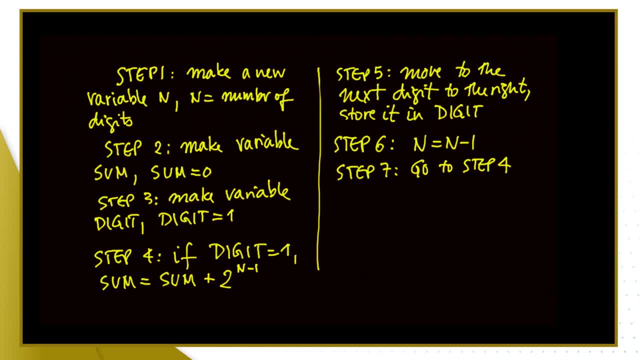 round. okay. so what do we do Here? what we do is we say: go to step 4. we should say if, if n is 1, we still want to run the cycle. so if n is 0, we want to stop. 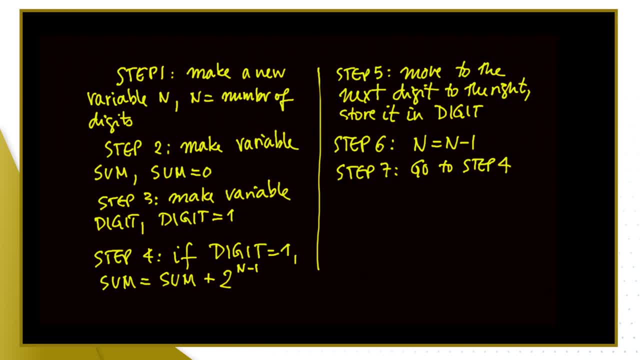 so we're going to change this statement here and we're going to say, instead of go to step 4, we're going to say: if n equals 0, we want to stop. so I'm going to leave some space for what we're going to. 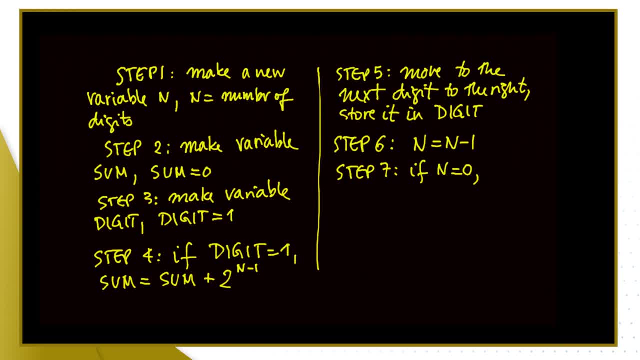 say we stop, because if we stop we need to print out the value of the number, and the value is sum and and then stop. okay, so if n is 0, output the message value in binary equals. print out the value of the variable. so equals sum. okay, and then stop. 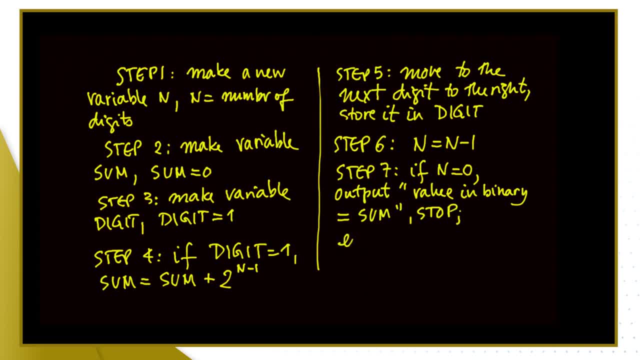 else if n is not 0, else that means n is 1 or more. we still go to step 4, okay, so let's run this by hand now, right? so step 1: make a new variable, n. n is number of digits. our number was 1: 0. 1, 1. 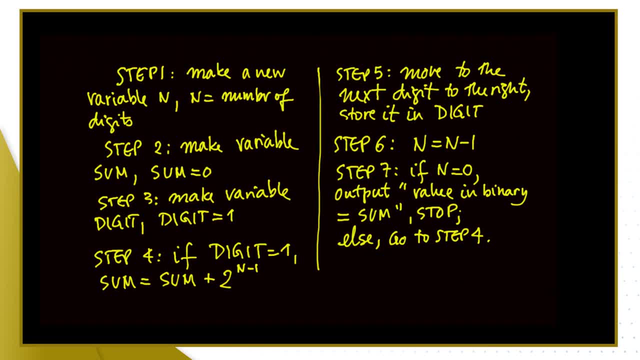 1, so the number of digits n is 5, and the number of digits n is 5,. okay, make my variable sum equals 0,, that's fine, and my variable digits equal 1,. that's great, and that's because I'm the beginning of the. 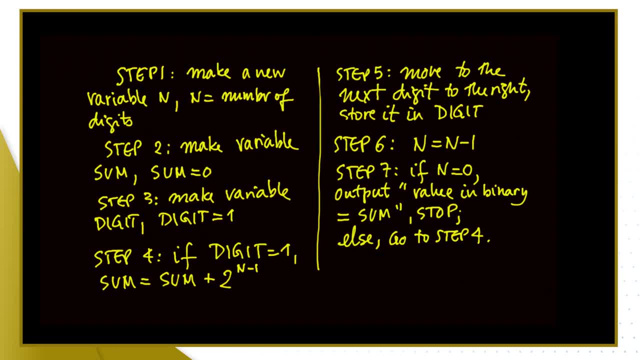 number 1, 0, 1, 1, 1,. now step 4. if the digit is 1, which it is, do the sum. so sum is now the value I had there, which was 0, add 2 to the power of 4, because. 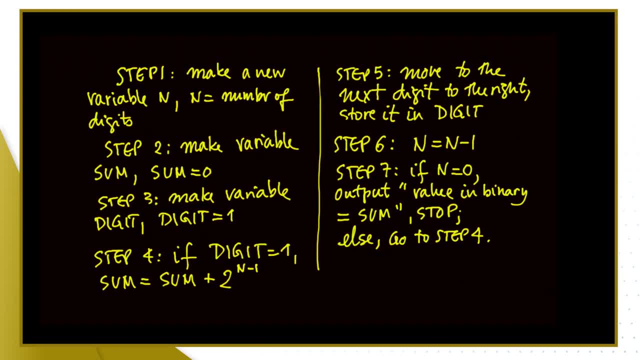 it's 5 minus 1, so 2 to the 4, great, so let's go and do the next step and then, step 5, move to the next digit to the right. so that's now. the digit equals 0. so now my digit equals 0. and step 6 decrease the n, so n is now 4. 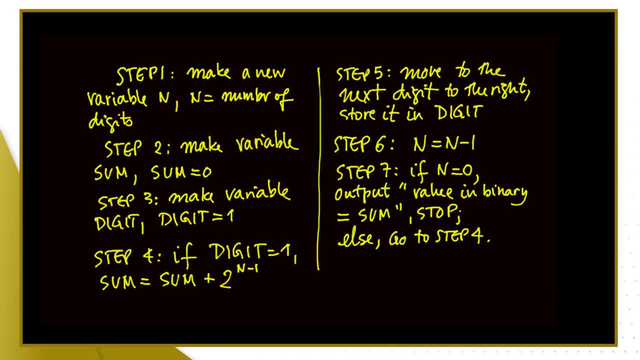 great. and if n is 0, which is not else, got step 4. step 4 digit is 1. no, it's not. so move on step 5. move to the next digit to the right, and next digit is a. 1. store it on. the variable digit is now 1. great decrease. the n n is 3. if n is 0: no, 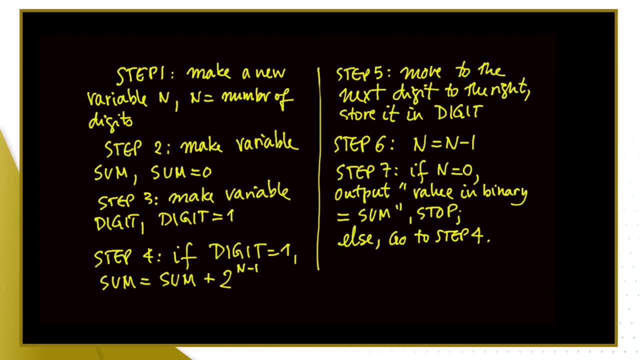 n is not 0, so, goto, step 4 digit is 1. yes, it is. update the sum. the sum is now what I had before: 2 to the 4. add 2 to the square because it's 2 to the n minus 3. and then, if x is 7, it's 1. so it's now 2 to the 4. so that's 2 to the square because it's 2 to the n minus. 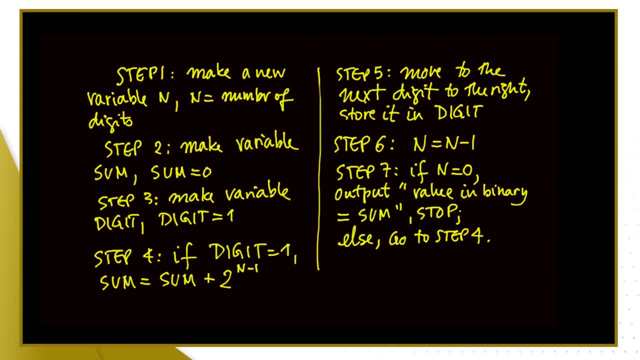 1 and n is 3, great. and then step 5 move to the next digit. so there's another one that is coming, and step 6: decrease the n. n is 2, and then step 7. if n is 0, no, it's not. so go to step 4. step 4 if 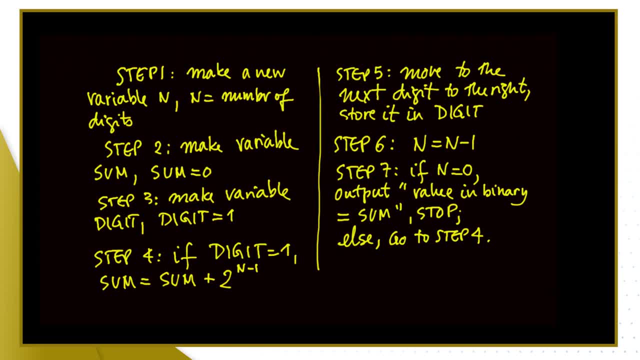 digit is 1, which it is do the sum. so sum is what i had there before. add 2 to the n minus 1. n is 2, so it's 2 to the 1, and then step 5, move to the next digit. next digit is a 1 and step 6 decrease. 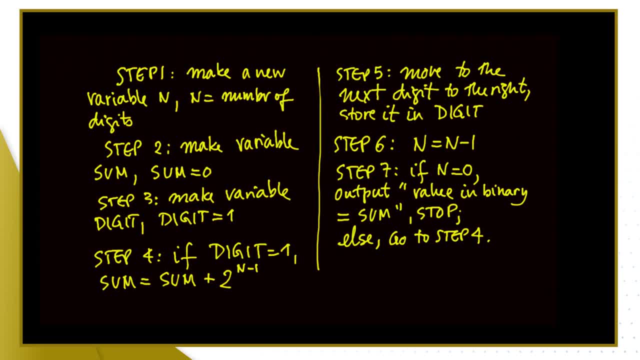 the n. n is now 1 and if n is 0, no, it's not step 4. step 4 digit is 1. add the sum, so sum now is what i had there before and now add 2 to the 1 less than the n, so 2 to the 0 and step 5. move to the 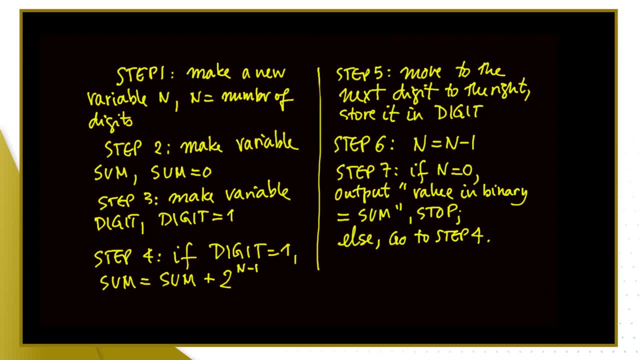 next digit to the right. there is no digit to write yes. so it feels that we should fix the algorithm and say there, if there's nowhere else to move, we should stop. so the instructions i put on step 7 should be on step 5 and i'm showing you the how we improve our algorithm as we run it. i'm not expecting you. 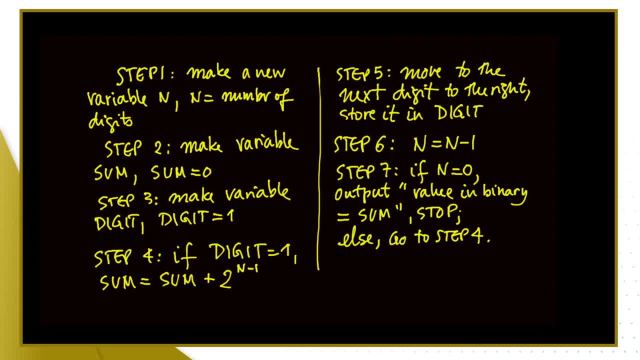 to write the algorithm neat first time round. it's a trial and improvement process, so we need to go back and fix what we've written, and we're going to do it here as well. so it feels that the right place to uh to have a stop instruction is on. move on step 5. move to the next digit. 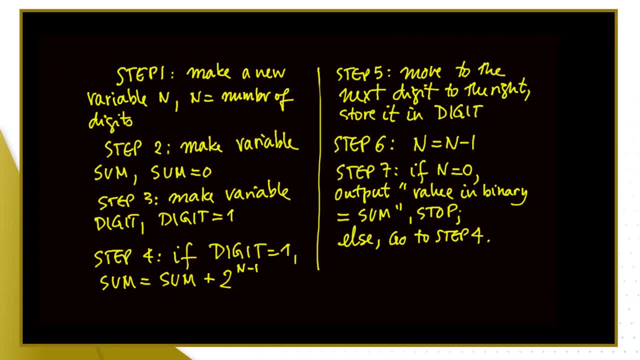 to the right and store it in digits. so we need to have there an instruction: if n is 0, we would output. we're going to change that instruction there and we're going to say: if n is 1, we now need to output the results. output. 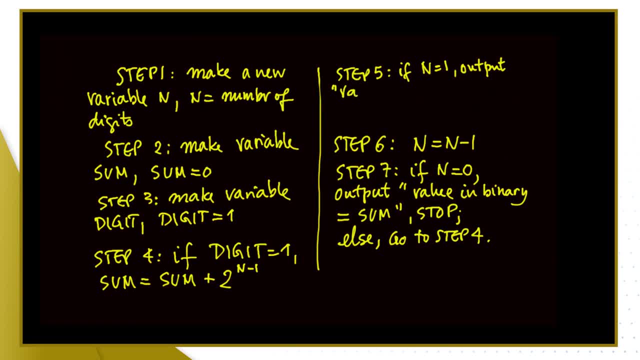 value in value in decimal equals sum and we stop, else else we need to move to the next digit, okay, else move to the next digit and then store it in digits. okay, and that we're going to tidy up. that means that on step four we have to select the time variable. so let's say he auf. 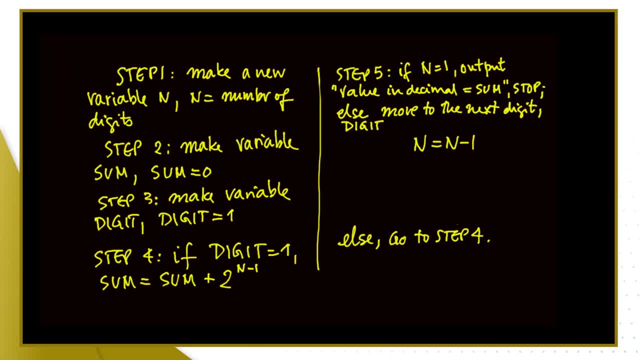 on step one, wesch, and we need to make the n equals n minus one on the same step. okay, and then on step six, which we only run if we still get a digit to go, we do go to step four. Now, does that make sense with our example? 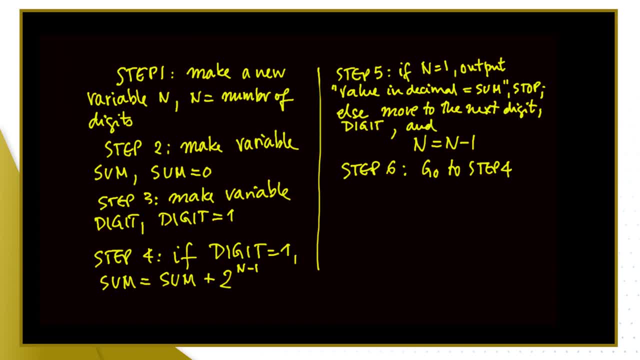 Yes. so where were we? We were at the point where we had n equals one. if n equals one output, and we had done the sum, we had a total sum. if n is one, we output the value. so at this point we print the value in decimal. 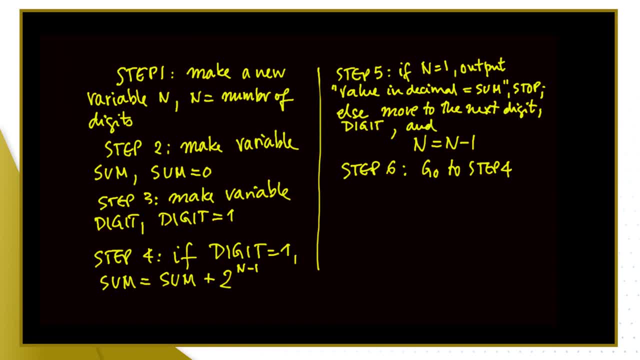 and then we do the sum. we had 16 plus 4 plus 2, which was 22,. that's what we accumulated on the variable sum and we stop. Okay, great, did I change what we've done before? No, because every time we got to this stage in the other steps. 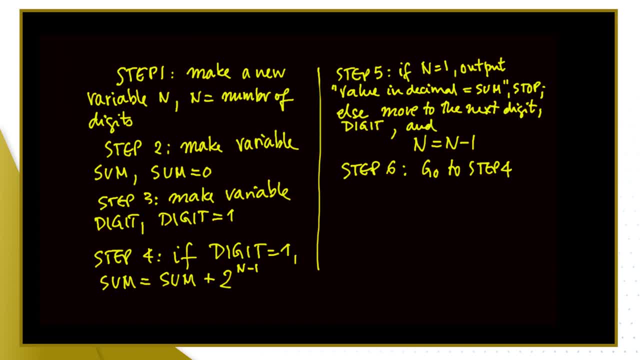 n was bigger than one, and so we could carry on doing the sum. Okay, so here's one example of an algorithm you could run to do the conversion from binary to decimal. What things could be different? There are many ways of writing the same algorithm. 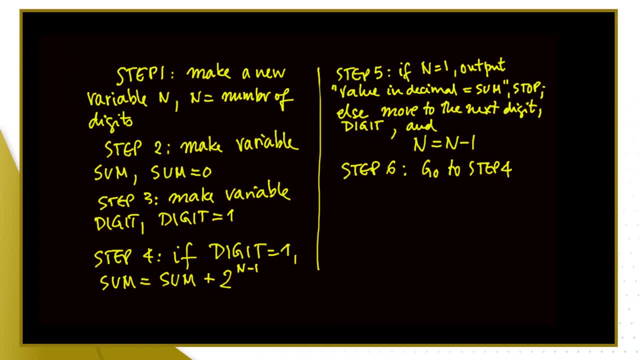 but one thing we could change is that in this algorithm, when we do the sum equals sum plus a power of two, we could have done a weighted sum instead of having it. if digit equals one, we do the sum, and if digit equals zero, go somewhere else. 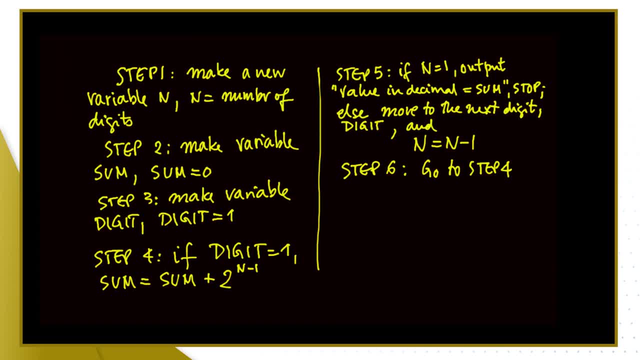 instead of that we could have done: sum equals sum plus the digit times the power of two, and if the digit digit is zero, then that means you're not adding anything. If the digit is one, you're adding the power of two, So that is an alternative which means you don't need to have ifs There's. 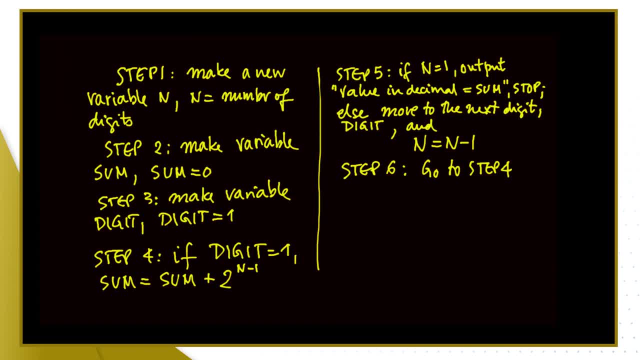 different ways of solving the same problem. Another approach could be starting from the rightmost digit. You could start from the one on the right and then go up in your powers of two You could. So you could invert the cycle and you could still say: now instead. 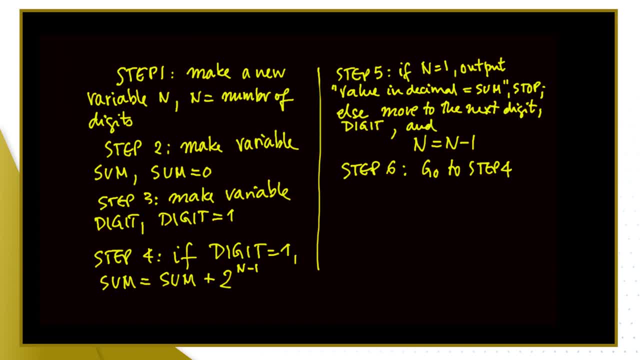 of decreasing the n, as we did, you could increase the n, So pretty much a similar structure as we had written just now. but instead of having n equals n minus one in your increment, in your decrement we would increase n. We would start from n equals one and then n equals. 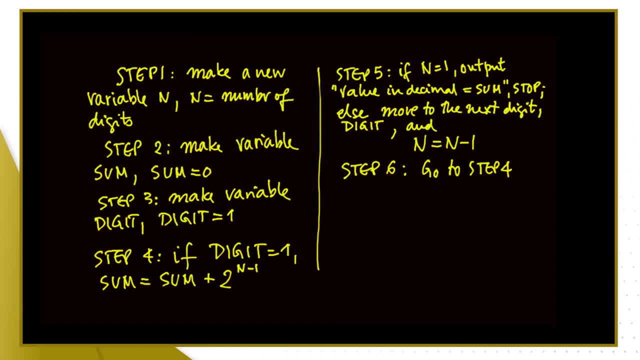 n plus one and so on. But then how do you know you stop? Well, same way You stop because you count the digits to start with And you run this cycle that many times. So that's another way. There is still another. 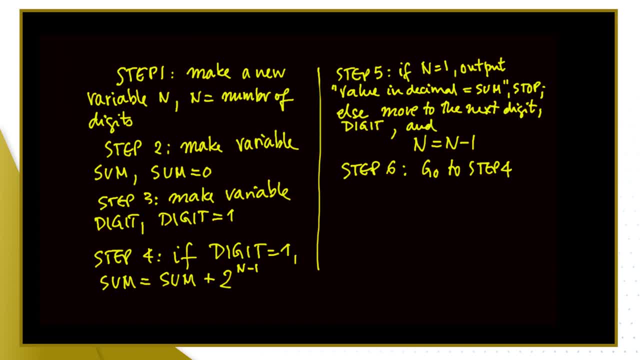 way, which I'm not going to write in algorithm form, but I want to write the algebraic reason for it. So, instead of adding a power of two in every cycle, you could add the digit and then times it by two, And so you add a digit and double the result, And that is a lot more. 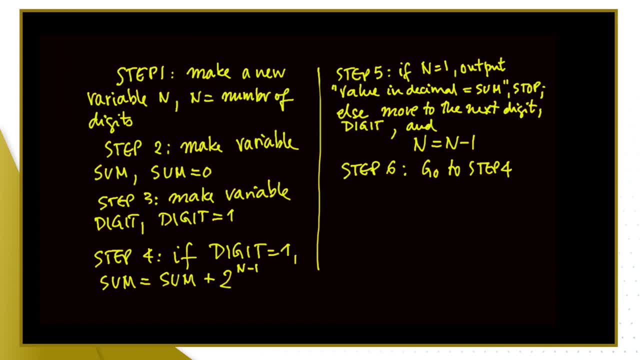 efficient because you are not calculating powers of two. You are doubling every time, which, if you remember that a machine level doubling is just putting a zero at the end of a binary number. It's a very easy operation compared to multiplication. So back to this idea. We can do a new algorithm where the variable sum is going to store the 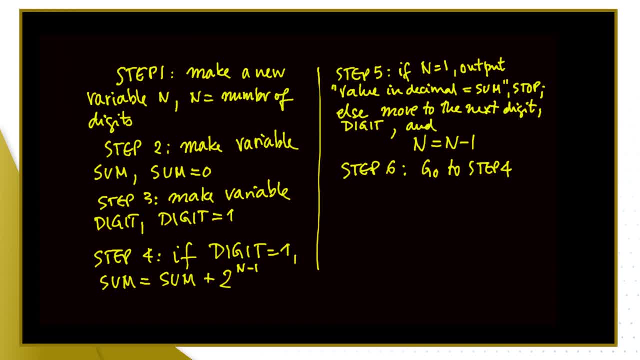 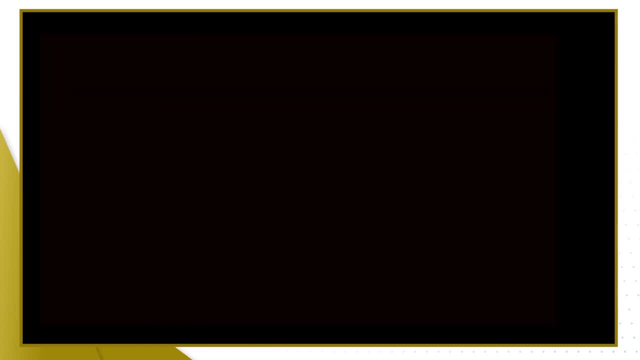 new digit, Then you double the sum, and then you add a new digit, and then you double the sum and you carry on going like this. So I'm going to write the algebra of that And that's a very elegant way of doing it. So, for our example, where we have five digits, our number is this: 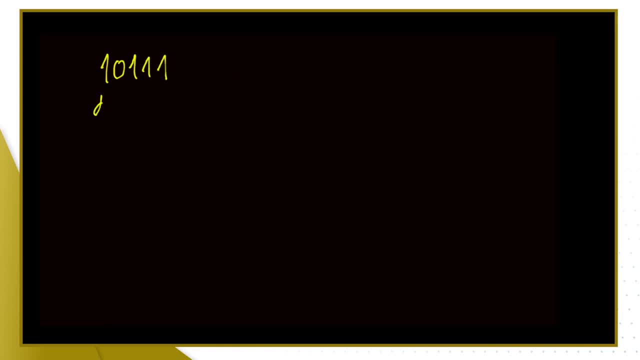 one. I'm going to call the digits digit four, digit three, digit two, digit one and digit zero, in that order. But the expanded form of this number is going to be the number of digit four, two to the power of four, plus digit three, two cubed plus digit two, two. 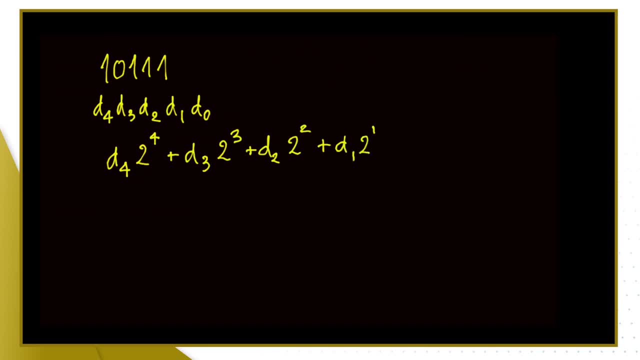 squared plus digit one. two to the one plus digit zero. two to the zero. So this is the expanded form of that number And I can have a two, multiplying for most of it and decreasing the power. So this is what happens. 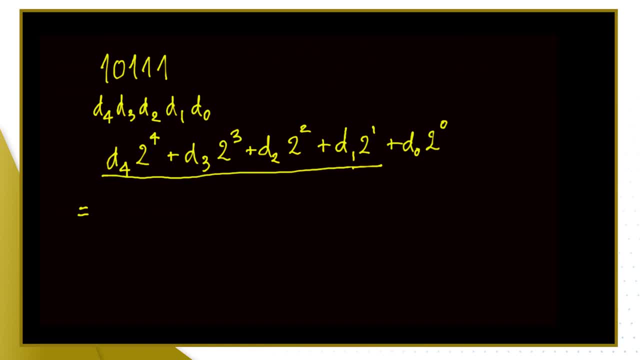 But here it's a multiple of two. I've got a two on each fact on each term, So I do two times. And then, instead of having d four, two to the power four, I'm going to have d four, two cubed, Because the two outside the bracket and the two cubed multiply out to 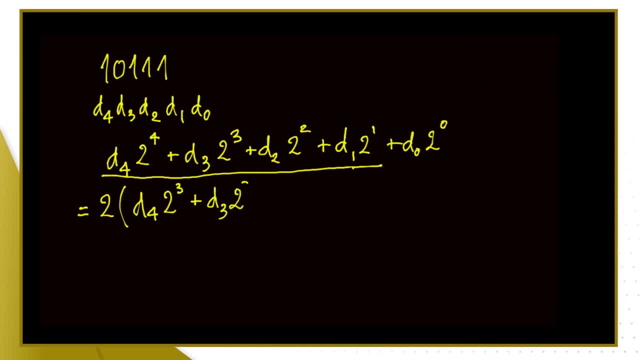 two to the four. Then I have d three, two squared, plus d two, two to the one Plus d one, And then outside the bracket I've got d zero. two to the zero. Two to zero is just one. And now inside the bracket I can do the same idea. I put everything from d four to d two. 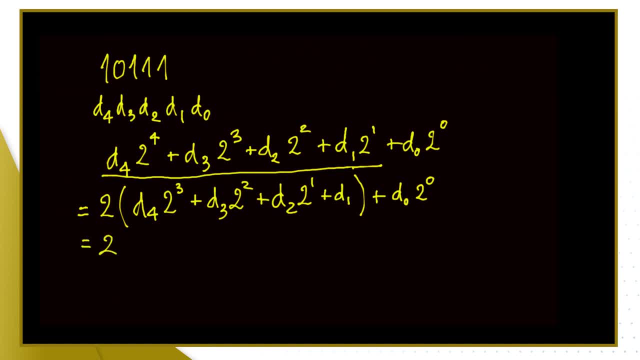 in the brackets with a factor of two out. So it's two, two d four. two squared plus d three. two to the one plus d five. That's two squared plus d three. two to the one plus d five. All right, 코�. 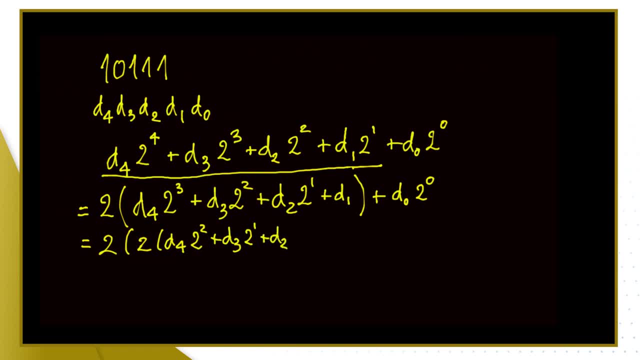 plus d2, 2 to the. I'm just going to write d2,. could have written 2 to the 0, but I don't need to plus d1 there and I'm going to get rid of that 2 to the 0, because it's just 1,. 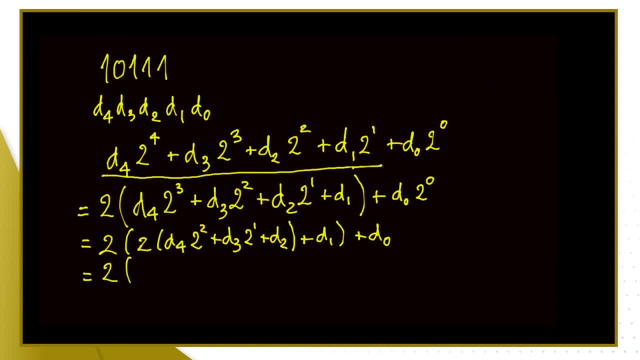 and I keep doing this. so the bracket there is going to be 2, and now bracket d4,: 2 to the 1, plus d3, and then plus the d2,. close the bracket plus the d1,. close the bracket plus the d0,. 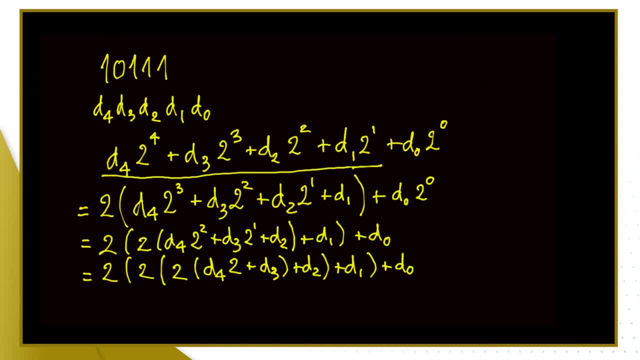 we can check if the brackets are right. let's do some colouring. let's do some colouring I've got. these are red brackets, that's great. these here are yellow brackets, that's cool. and the other ones are white brackets. that works okay. so let's do one more. 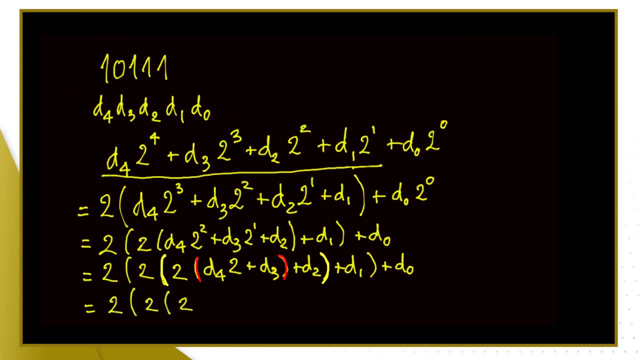 one more level means 2, bracket, 2 bracket, and now I've got 2 d4 plus d3 plus d2 plus d1 plus d0.. I didn't add any brackets, but I just rewrote that d42 as a 2 times a thing, That means this: 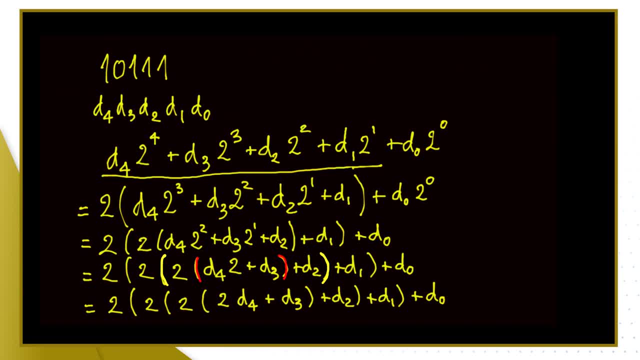 nested sequence of brackets. it's how I can build this sum in the way I said earlier. So if I start with a sum that is d4, so the digit is kept in sum, and then the next round you double it, you do this double sum and then the next time you run the loop you do. 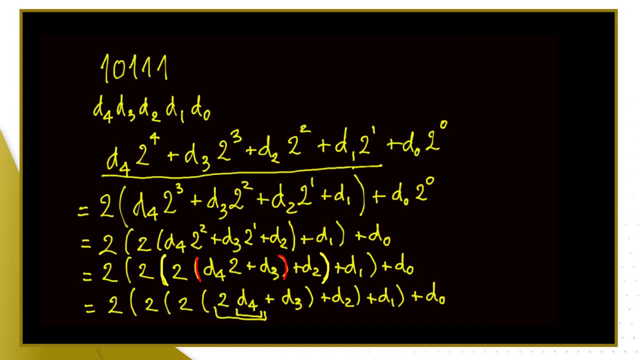 add the digit which gives you this set of brackets, and then you double it, which means that 2 multiplying for the bracket, and so on. So that is the most. in my view it's the most elegant way of doing this conversion. 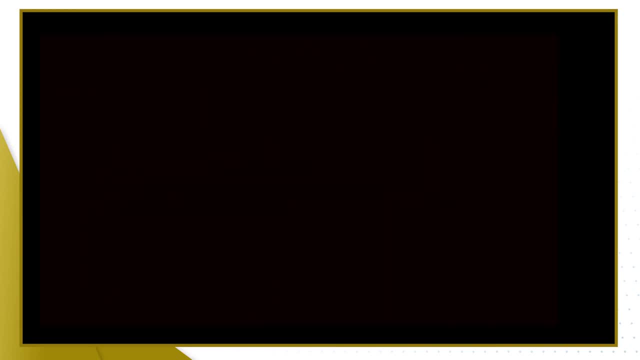 from binary to decimal. So now let's look at the other aspect. Let's write the algorithm for converting from decimal to binary. We're going to use the division algorithm. So to convert 38, which is a decimal number, into binary, we divide 38 by 2.. 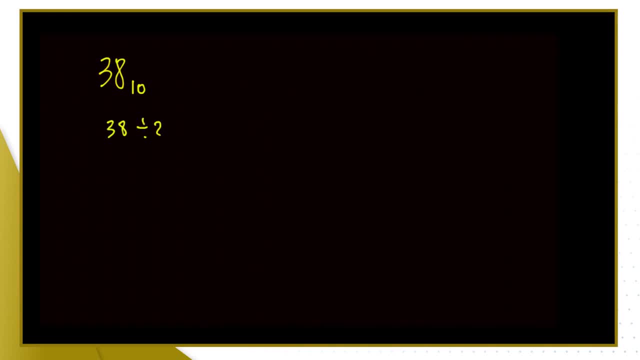 Okay, so we start: 38 divided by 2. That's 19. Remainder 0.. Then we do 19 divided by 2. That's 9. Remainder 1.. 9 divided by 2.. 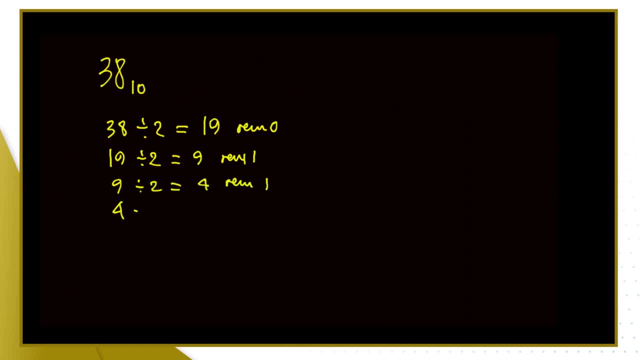 That's 4.. Remainder 1.. 4 divided by 2 is 2.. Remainder 0.. 2 divided by 2 is 1.. Remainder 0.. And then 1 divided by 2 is 0.. 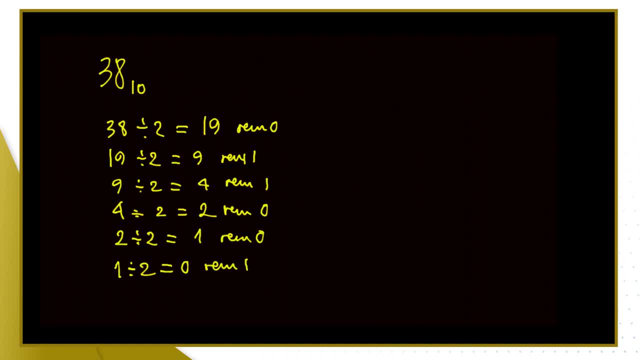 Remainder 1.. I've just done that example so that we tap into that to write the generic algorithm. So what's important? first we need the number, which is n, and we need the digits. The digits, they're going to be our binary digits. 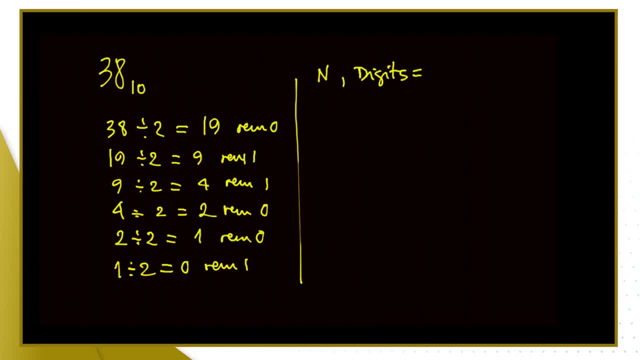 I'm going to start with an empty word there, So this is going to be the empty word: Empty word. okay, We have the number saved in the variable n. We have the digits containing just an empty word. We have the number saved in the variable n. 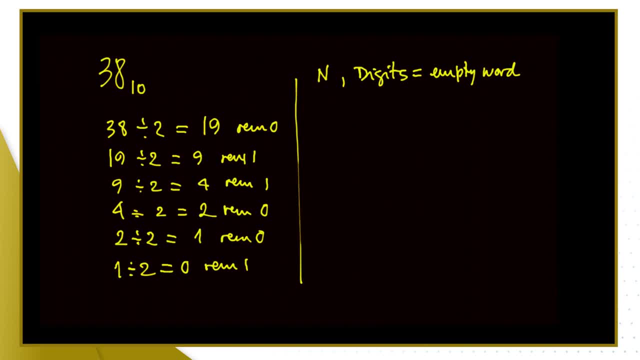 We have the digits containing just an empty word And then every time we do a division and capture a remainder, we're going to save the new remainder in that word. Let's call q the integer part of the division of the number. So it's going to be the integer division of n by 2, okay. 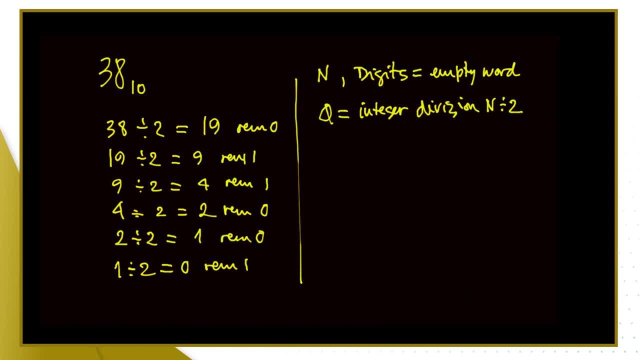 So the integer part, And now we need to extract the remainder. To extract the remainder, we're going to need the integer part. We're going to need the integer part. To extract the remainder, we do the number minus twice the q. okay, 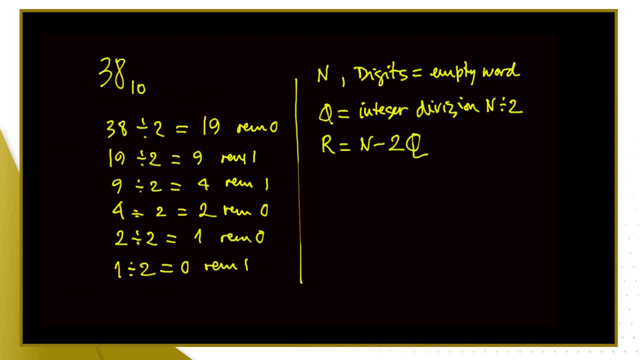 The number minus twice what we've got. That's our remainder. I call it r, So the remainder is our digit. okay, And now we're going to carry on doing the division. So let's make n equal to our q. n is our q now. 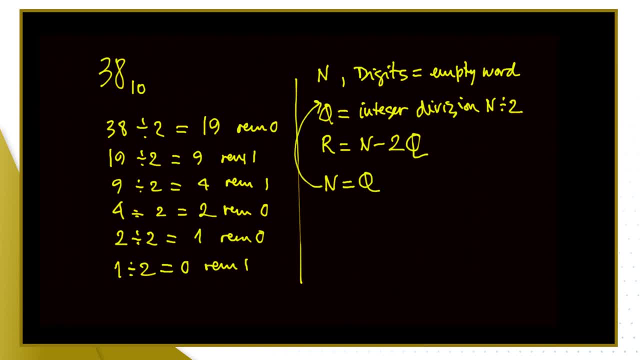 And we just loop. We should just now loop up there, But you've noticed We're not keeping track of the digits. We need to save the digits, So we need somewhere to say let's write the digit r to the left of the word digits. okay, 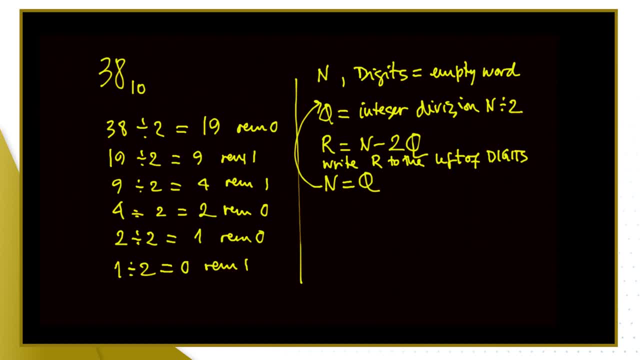 That's how we keep track of the digits. Now, did we do it the right way around? Is it left or right? So let's look at our example. The first remainder, It's going to be the The rightmost digits, And the last one is the leftmost. 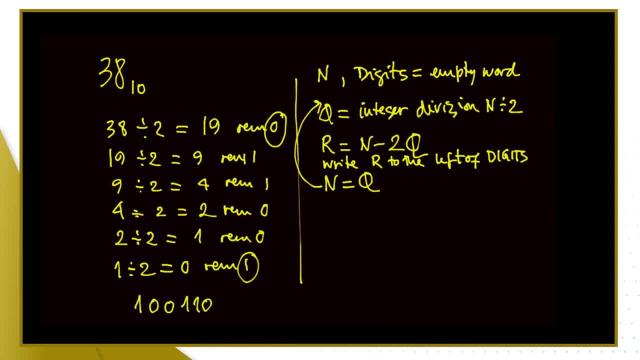 So the number in binary is going to be like this And we went that way. So every new digit is written to the left of the digits we had so far. okay, So those are the steps And we can write that into step one, step two, step three, step four, step five. 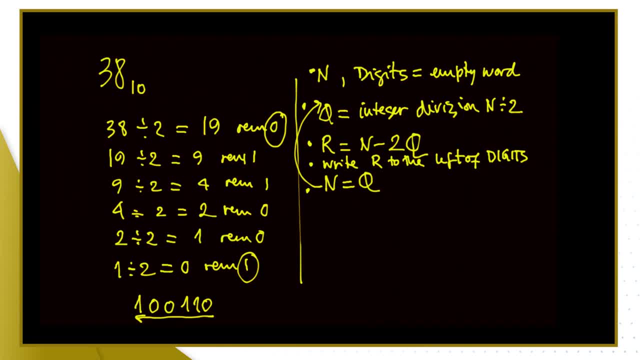 How do we stop? We stop. Let's look at our sums. We stop when we had quotient zero. If the quotient is zero, we stop And we have to print out the value. So that means that here I would say, if q is zero, we print digits and stop. 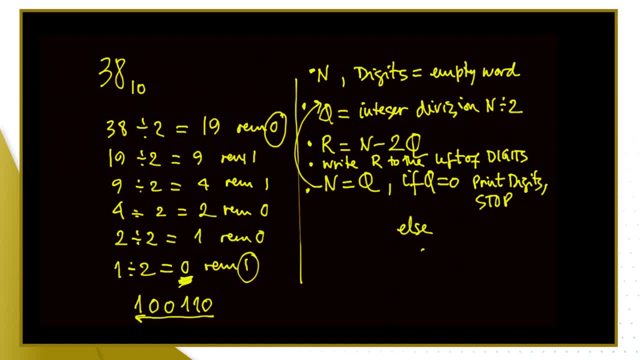 Else we have to go back there. okay, How do we do that? You can name all these steps into step one, step two, step three, step four, step five, and redirect here on the else to step two. okay, We have an algorithm that stops. 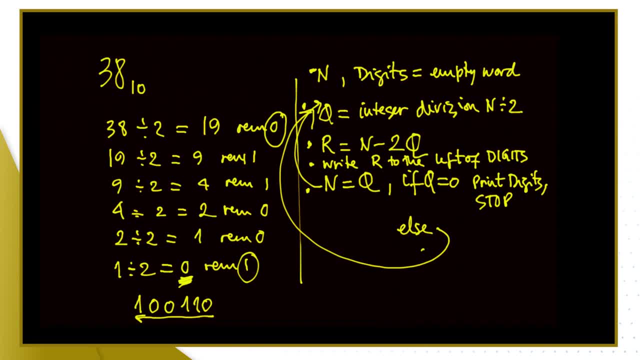 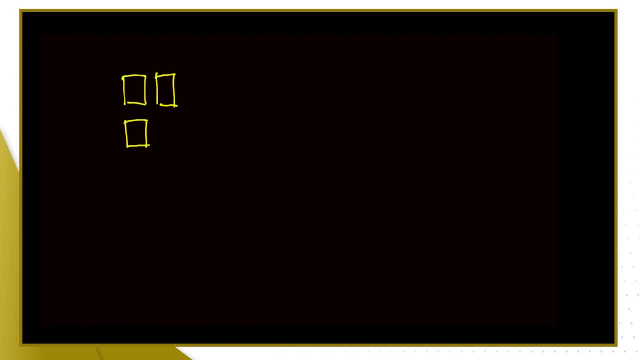 I'll just give you a very brief overview of task two. On task two, you are to write algorithms of adding up two, Two, Two, Two in binary. Two digit numbers in binary. Two digit numbers in binary. You are to do subtraction as well and multiplication. 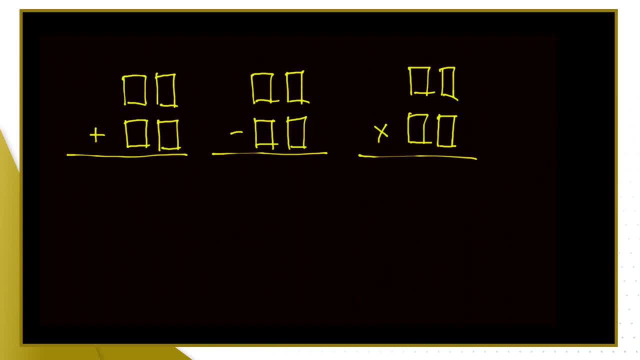 Put in boxes for all the digits we need to account for, And the main thing to consider is that if you're adding these two numbers, it's all very good. if it's one with zero or zero with one, You only get. You get one answer there. 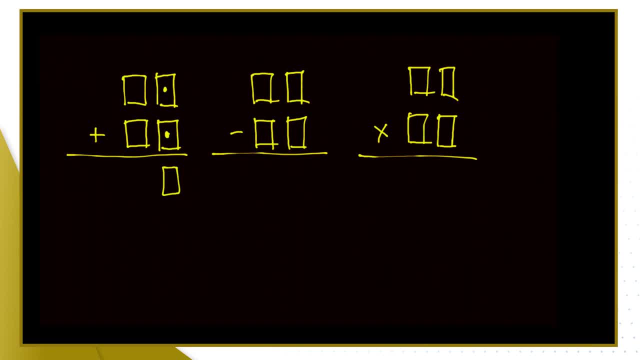 But you need to account that if you have one plus one, one, zero, Yes, Wow, zero as an answer, which means you need to have a zero here and a one that it's carried. so you need to take into account that you need to have a variable for carries. okay, so that's a pointer. 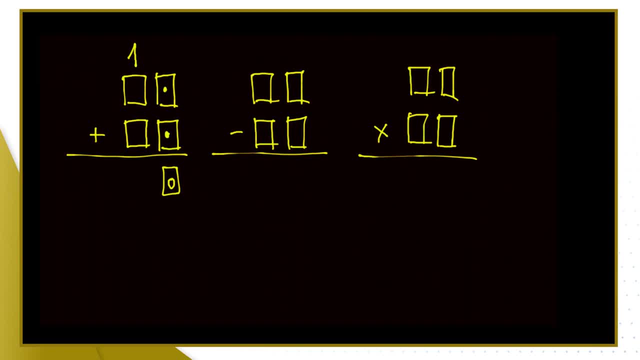 there on. on subtraction, you need to take into account the borrowing that goes on. if this digit here is too small for this one, meaning if you've got a zero here on top and a one below, then you will need to borrow from over there. so there will be. you will need to change the digits of. 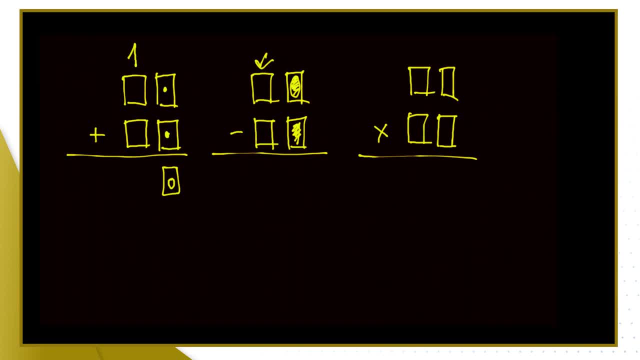 the numbers as you go along with multiplication, we need to take into account that the results are going to be here, possibly like this: and then when you multiply this guy here by the top number, you'll move place value. so you need to take into account that. okay, so you're not going to write anything there, but you're going to move place value. 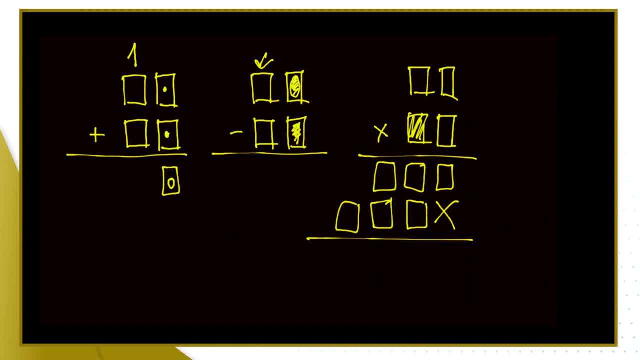 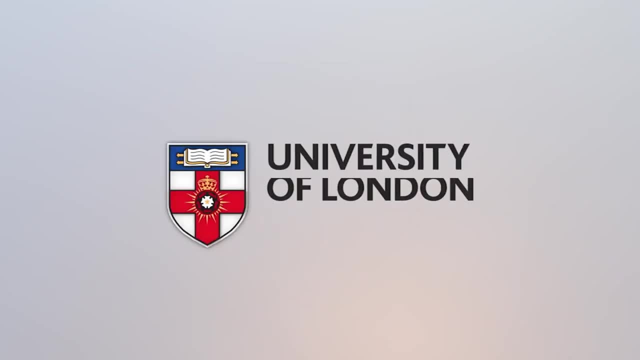 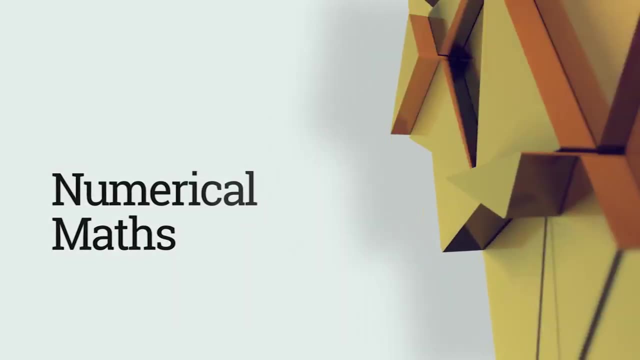 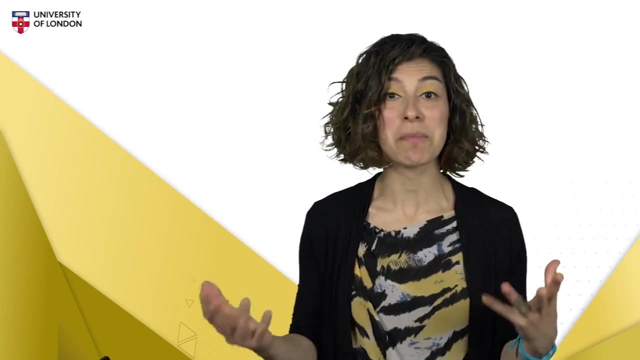 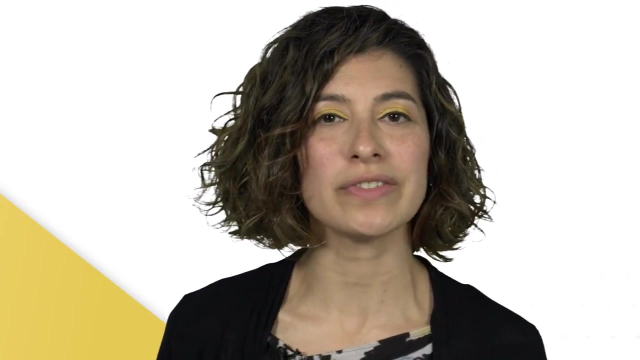 so that's a few pointers of what your algorithms need to take into account. we've now looked at operations in binary, and you know how to add, subtract and multiply numbers in binary. you are now to write down the algorithms for these operations using two two-digit numbers. 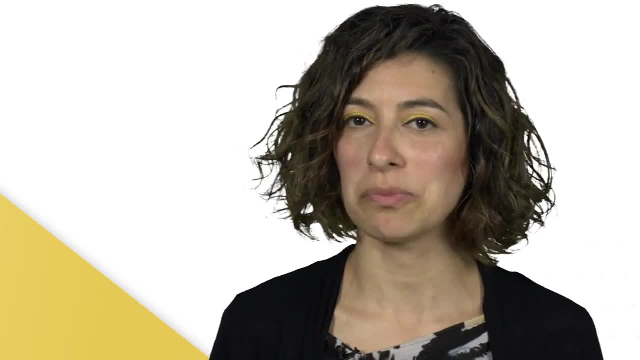 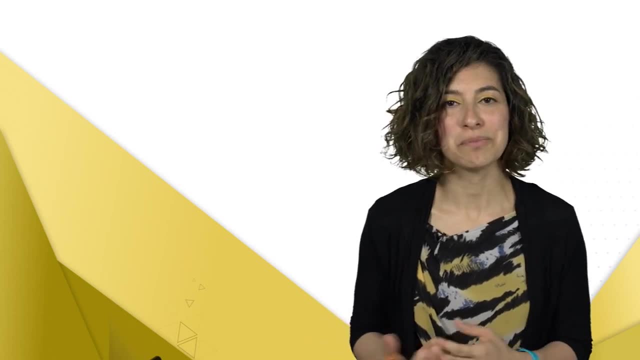 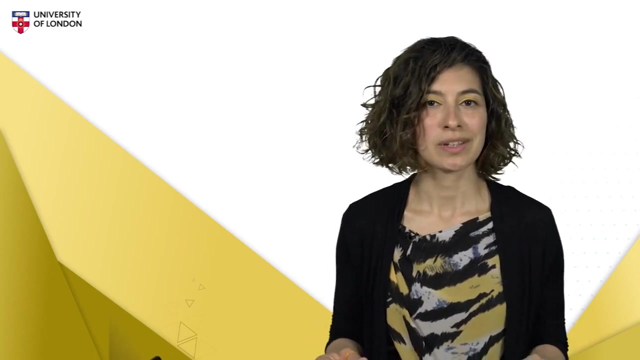 and I would like you to write it the best you can, as much detail as you can, as close as to a computer scientist as you can, as to how this fits in computing. keep an eye out for logic, as these tools together will allow you to build your own simple computer. 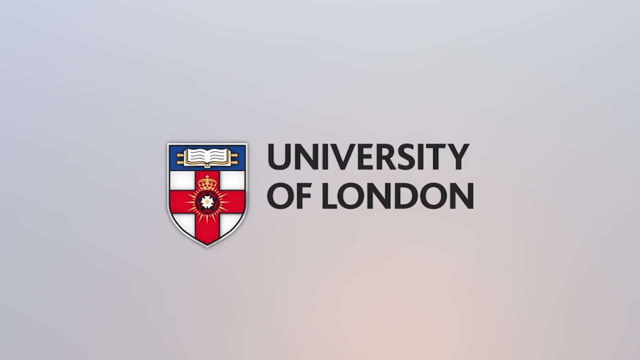 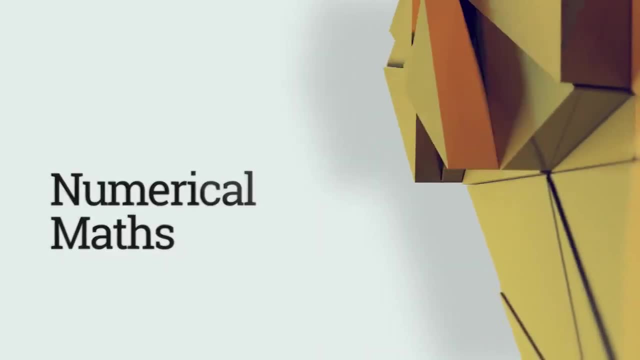 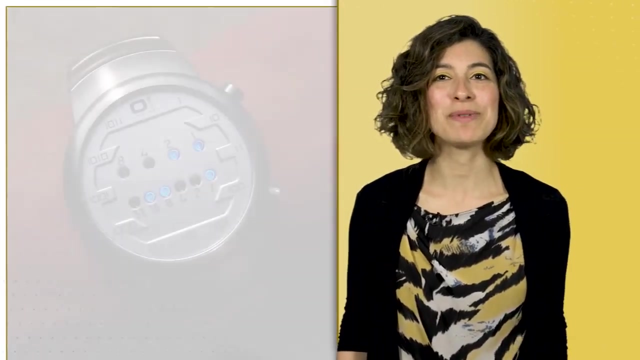 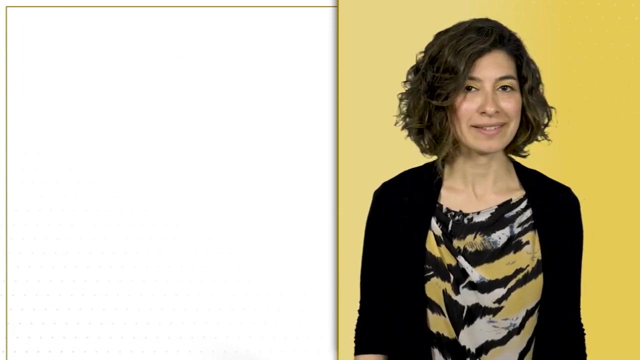 you now do binary back to front and some of you may be dreaming of making a binary clock. we will work through the details of two more bases: base 8 and 16. I would like you to focus on generalizing these examples and then we will move on to the next step, which is to create a binary clock. we will work through the details of two more bases: base 8 and 16. I would like you to focus on generalizing this example. 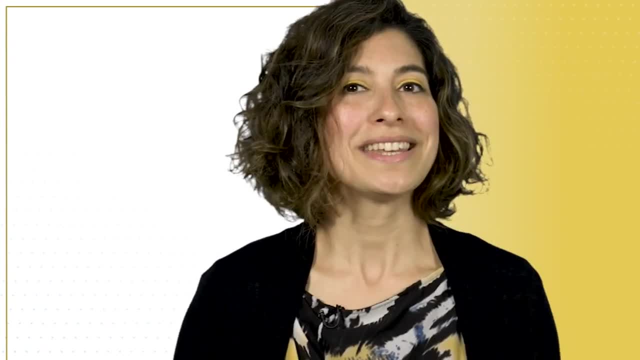 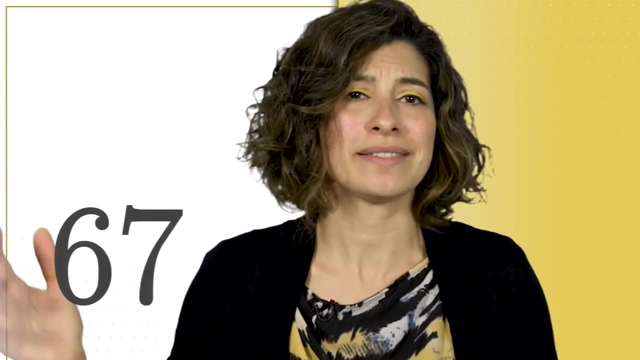 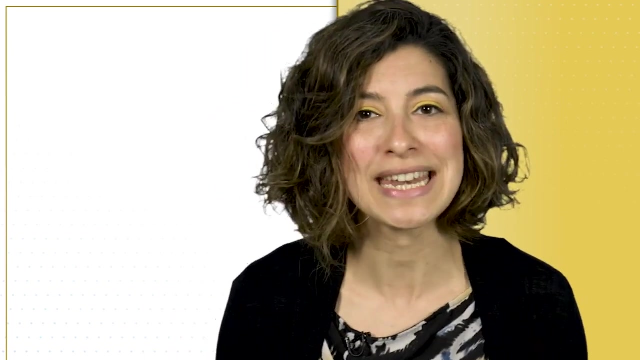 on to working with any other base. I mean, I want you to think about how you use base 3, base 4, base 67, any base. so follow these examples and make your own notes and form your own theory of how to write numbers and perform arithmetic in any 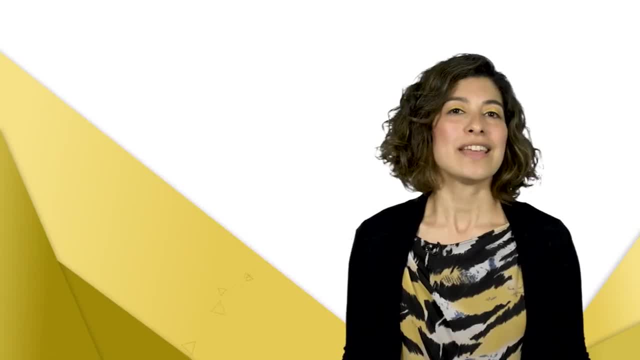 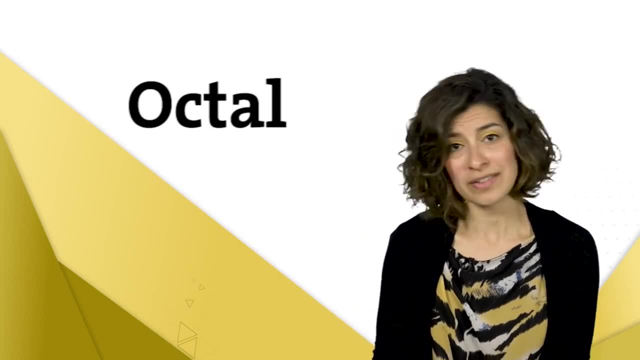 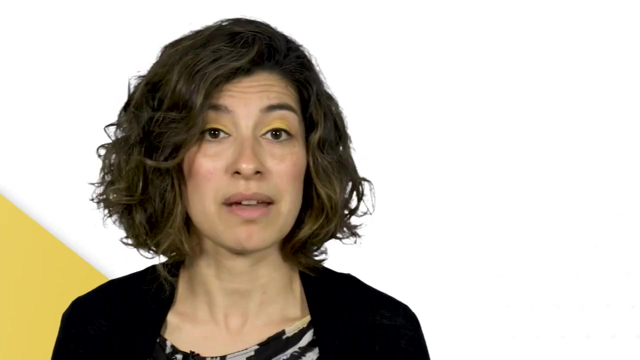 other base base. 8 is also called octal, from the Greek word for eight. they are octal from the Greek word for eight. they are octal from the Greek word for eight. they are 8 digits and these are 0, 1, 2, 3, 4, 5, 6 & 7. but what are the place values I mean? 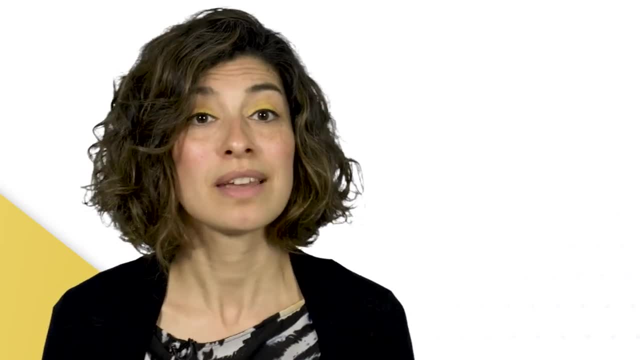 8 digits and these are 0, 1, 2, 3, 4, 5, 6 & 7. but what are the place values? I mean 8 digits and these are 0, 1, 2, 3, 4, 5, 6 & 7, but what are the place values? I mean, say the first three place values. you can answer that in. 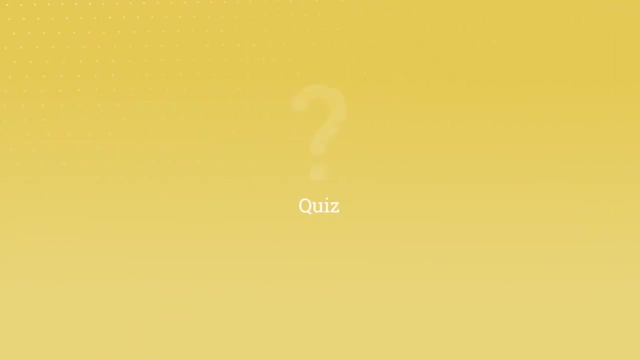 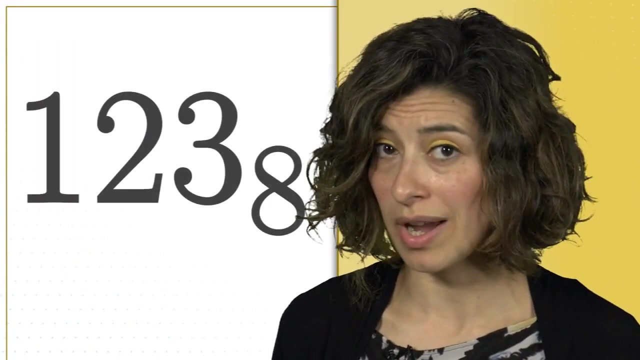 say the first three place values. you can answer that in. say the first three place values. you can answer that in the in video quiz. the octal number one, two, three, which I. the octal number one, two, three, which I. the octal number one, two, three, which I will write: one, two, three, with a little. 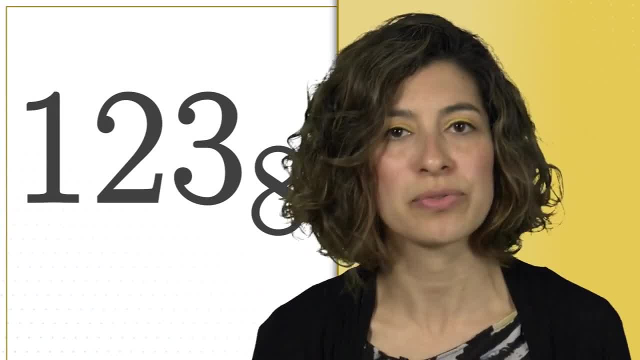 will write one, two, three with a little. will write one, two, three with a little. eight for avoidance of doubt. this is the eight for avoidance of doubt. this is the eight for avoidance of doubt. this is the subscript, subscript, subscript, which means that is written. base 8: this: 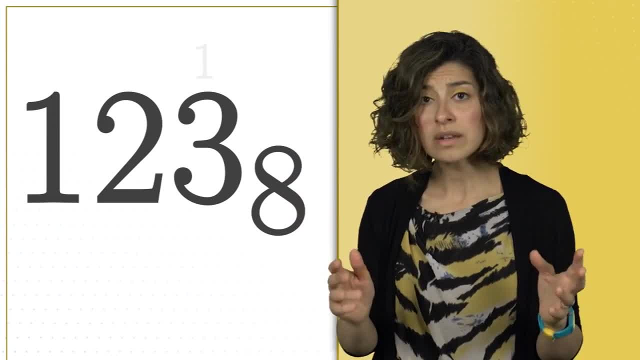 which means that is written base 8. this, which means that is written base 8. this number uses three place values worth 1. number uses three place values worth 1. number uses three place values worth 1, 8 & 64. as we start with a place value, 1 on. 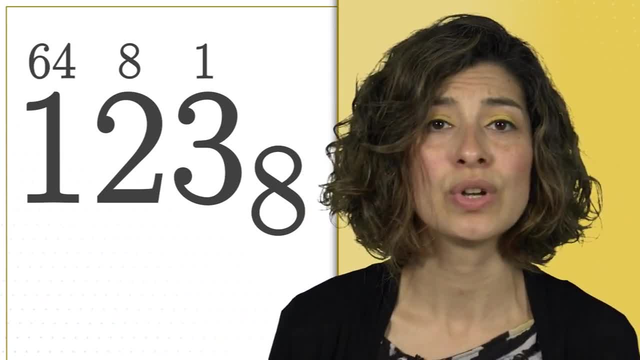 8 & 64. as we start with a place value 1 on 8 & 64. as we start with a place value 1 on the right and multiply by 8 to get to the right, and multiply by 8 to get to the right, and multiply by 8 to get to the next place value to the left, the. 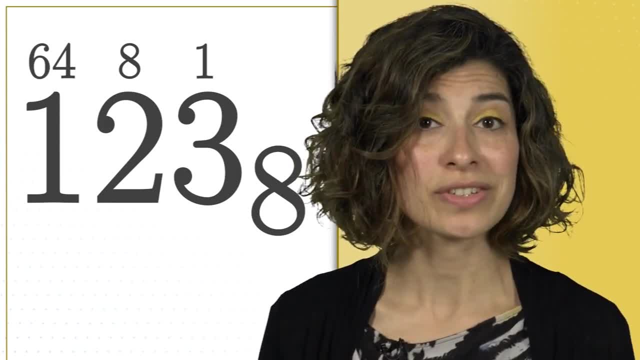 the next place value to the left. the the next place value to the left. the place values are consecutive powers of place values are consecutive. powers of place values are consecutive powers of 8 starting from 1. the digit 3 is for units. 8 starting from 1. the digit 3 is for units. 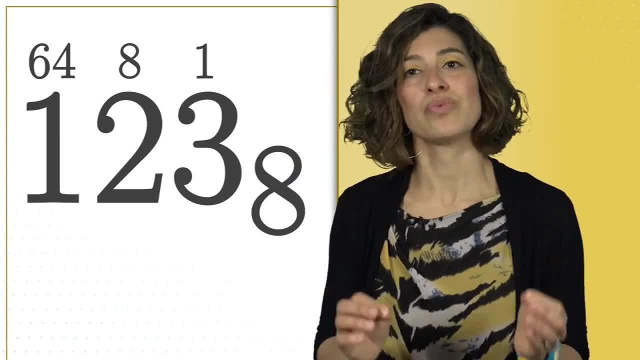 8, starting from 1, the digit 3 is for units, the digit 2 is for 8 and the digit 1. the digit 2 is for 8 and the digit 1, the digit 2 is for 8 and the digit 1 is for 64. we use this to write the. 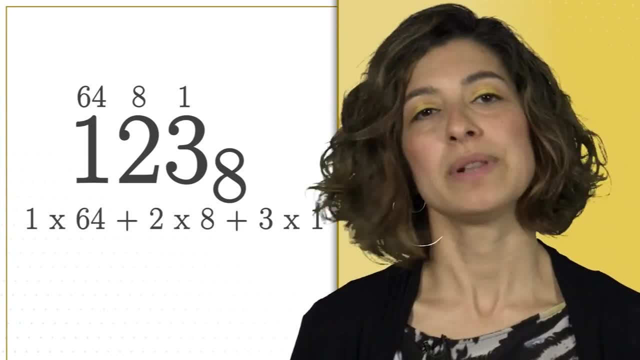 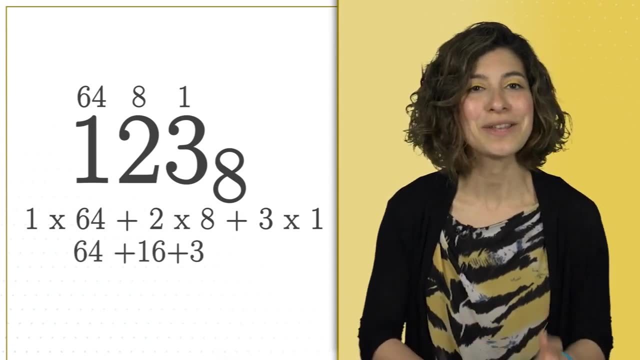 is for 64. we use this to write the is for 64. we use this to write the expanded form: 1 times 64 plus 2 times 8. expanded form: 1 times 64 plus 2 times 8. expanded form: 1 times 64 plus 2 times 8 plus 3 times 1, which gives 64 plus 16. 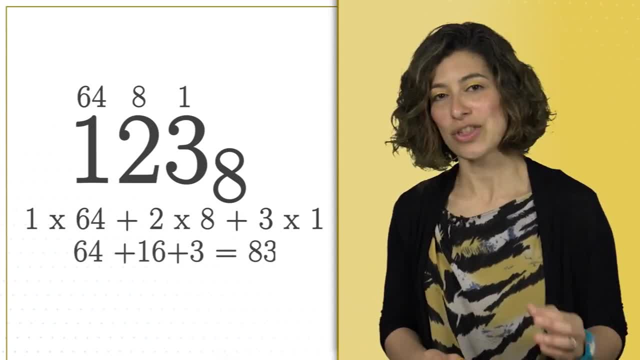 plus 3 times 1, which gives 64 plus 16 plus 3 times 1, which gives 64 plus 16 plus 3 and totals 83, and that means plus 3 and totals 83, and that means plus 3 and totals 83, and that means that 1, 2, 3 in octal is written as 83 in. 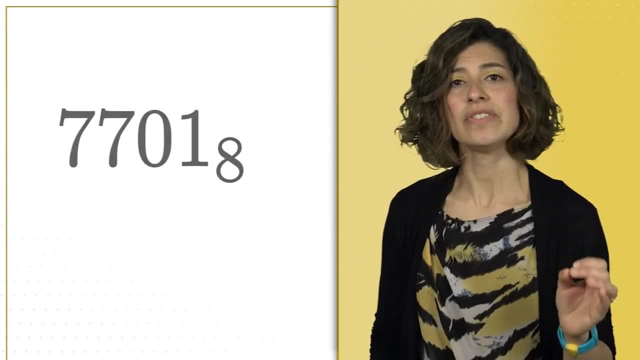 that 1, 2, 3 in octal is written as 83, in that 1, 2, 3 in octal is written as 83 in decimal. the number decimal, the number decimal, the number 7, 7, 0, 1 in octal uses 4 place values. 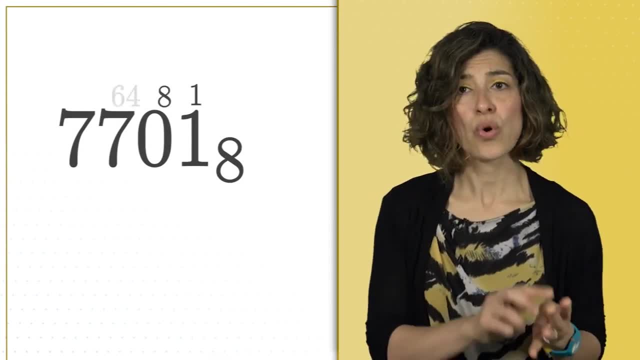 7, 7, 0, 1 in octal. uses 4 place values: 7, 7 0, 1 in octal. uses 4 place values worth 1, 8, 64 and 512. the first 4 worth 1, 8, 64 and 512: the first 4. 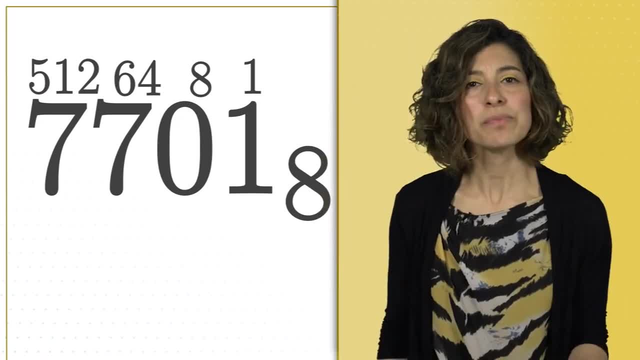 worth 1, 8, 64 and 512. the first 4 powers of 8. the leftmost 7 is on the powers of 8. the leftmost 7 is on the powers of 8. the leftmost 7 is on the position for 8 cubed, so 512. the next. 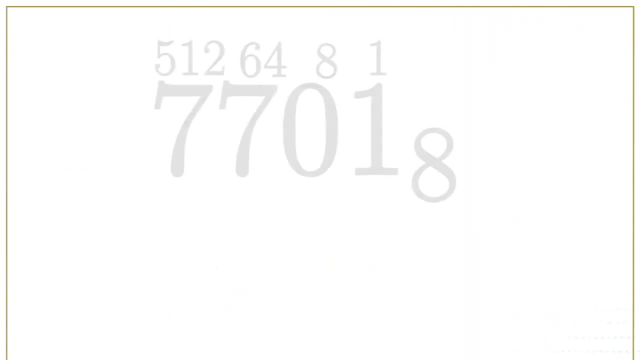 position for 8 cubed so 512. the next position for 8 cubed so 512. the next 7 on the 64s, the 0 on the 8 and the 1 on. 7 on the 64s, the 0 on the 8 and the 1 on. 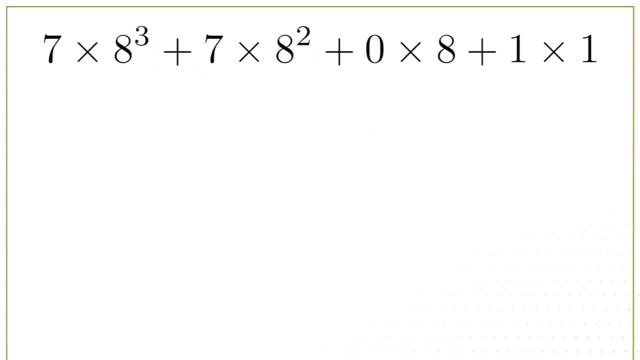 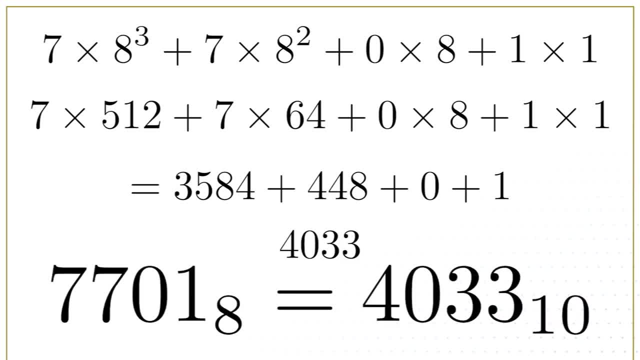 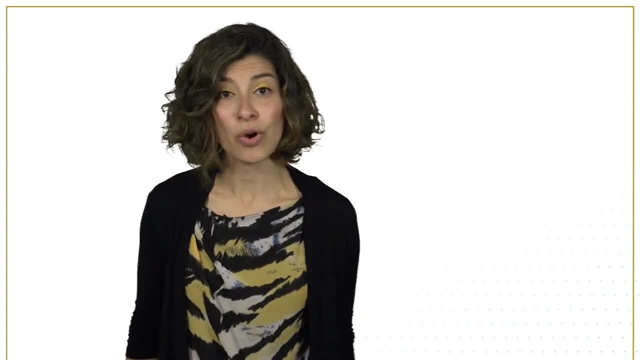 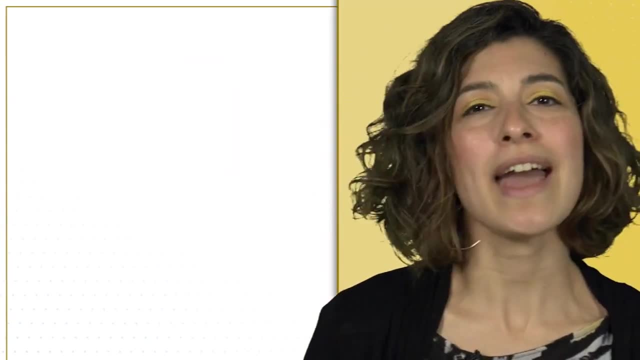 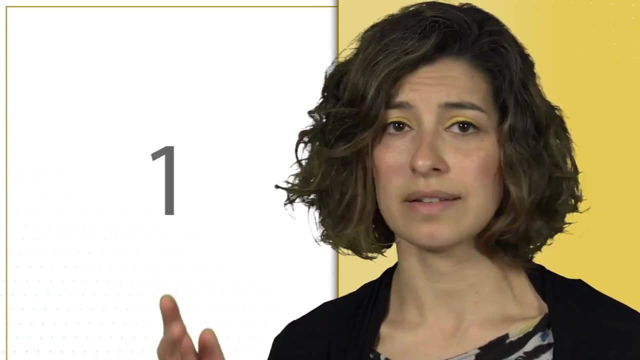 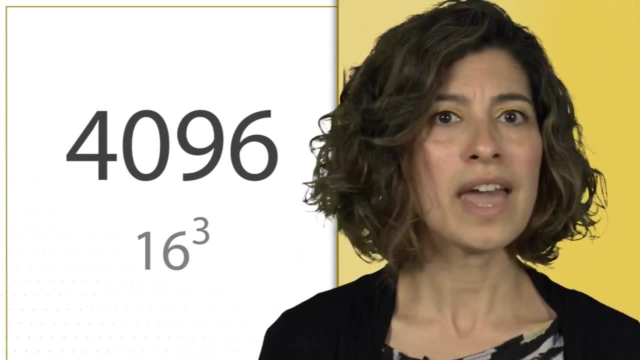 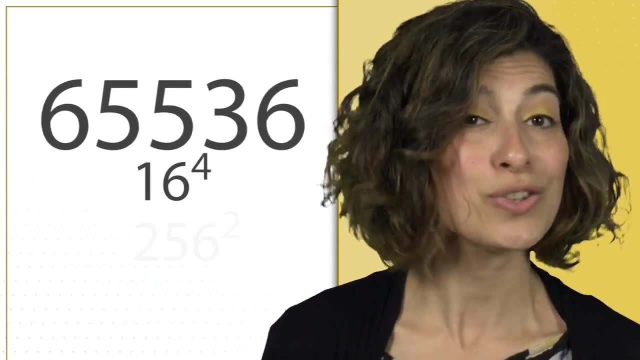 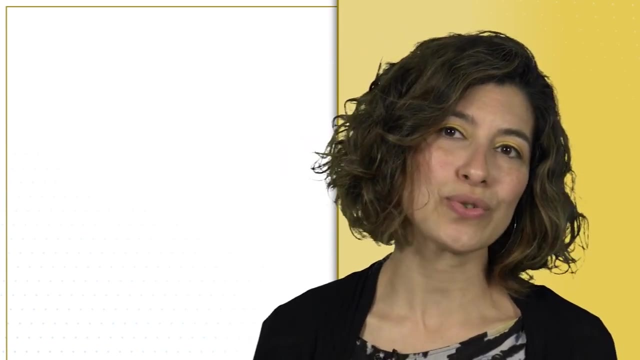 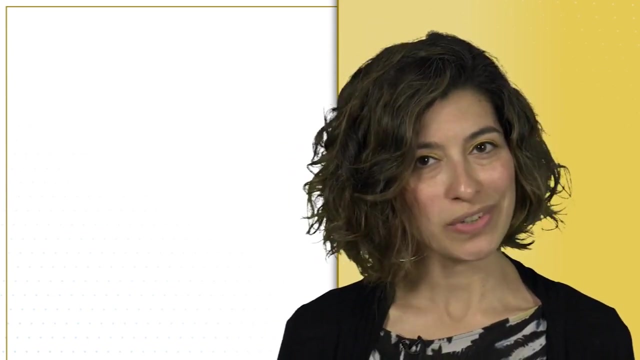 1096, which is 16, cubed, then 65,536, which is 16 to the power of 4, but also 256 squared, and so on. in the in video quiz I asked you to relate powers of two, powers of eight and powers of sixteen. later we will see why this is important. 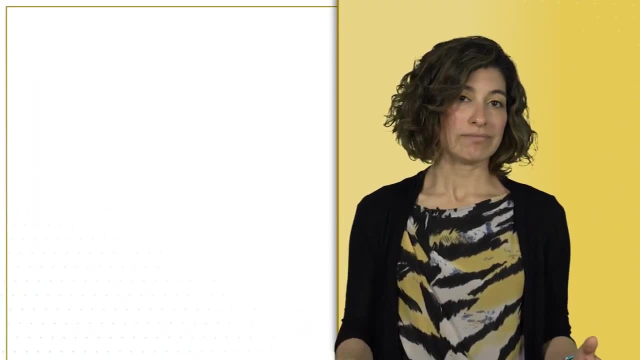 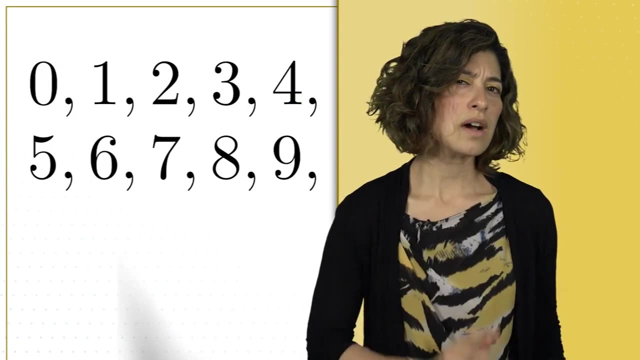 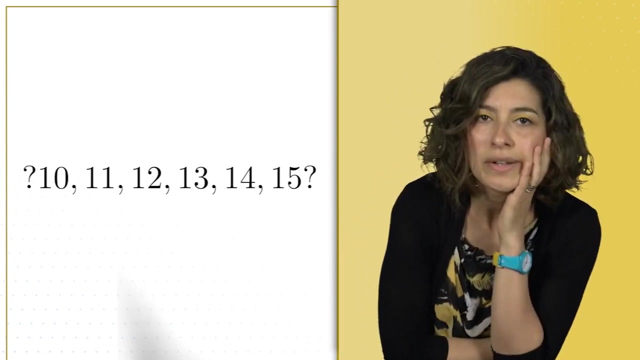 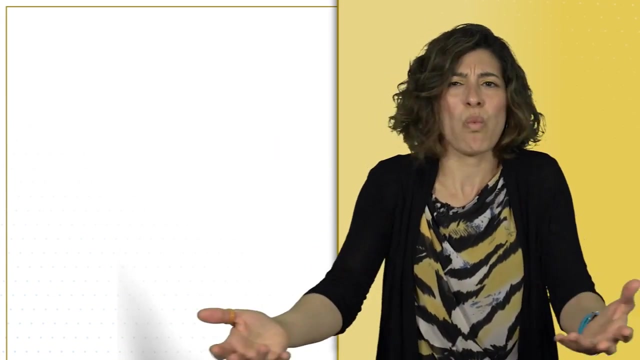 with base 16. we need 16 digits. that's great. we can go zero, one, two, three, four, five, six, seven, eight, nine, but we can't go 10, 11, 12, 13, 14, 15. well, we can, like the Babylonians did, but that would be very confusing. you know what does one, one, one. 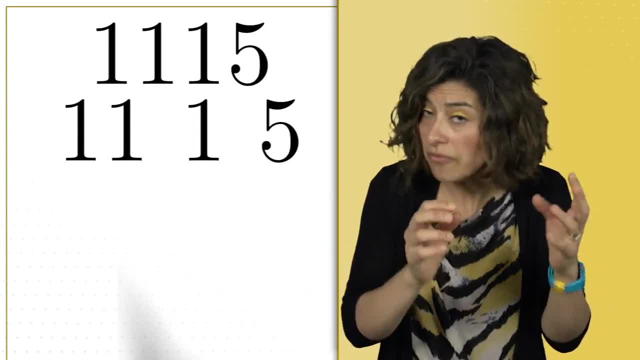 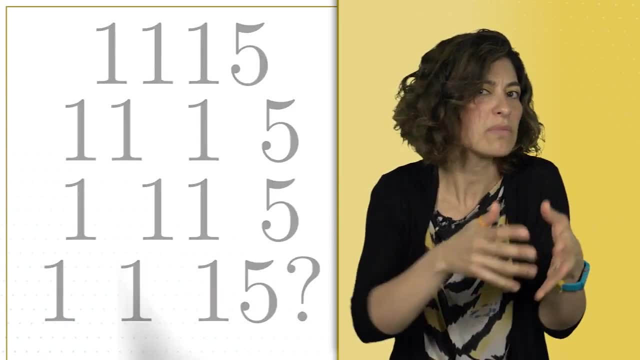 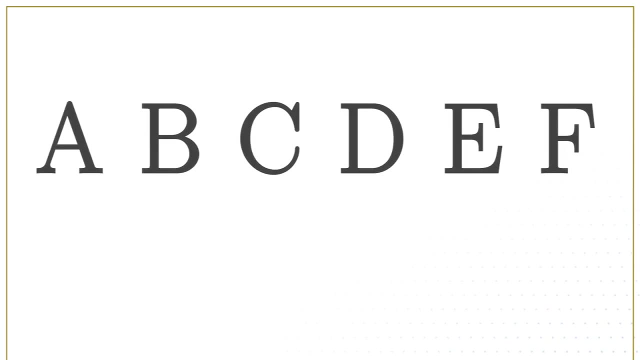 five mean? does it mean one one, 5,, really? Or 1, 11, 5? Or 11, 15? Or something else? To remove this ambiguity, we use symbols A, B, C, D, E and F. 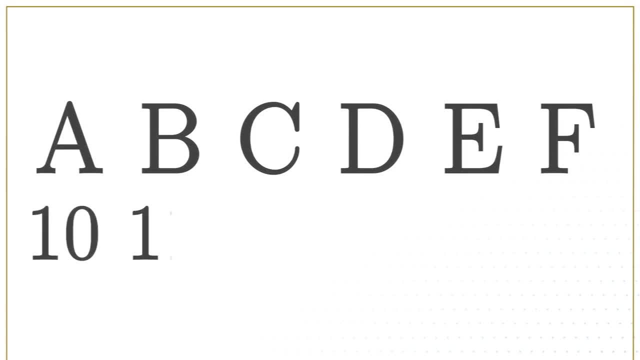 to stand for the numbers 10, 11,, 12, 13,, 14, 15, respectively. So 11, 15 is BF in hexadecimal and 1, 1, 15 is 1, 1F. 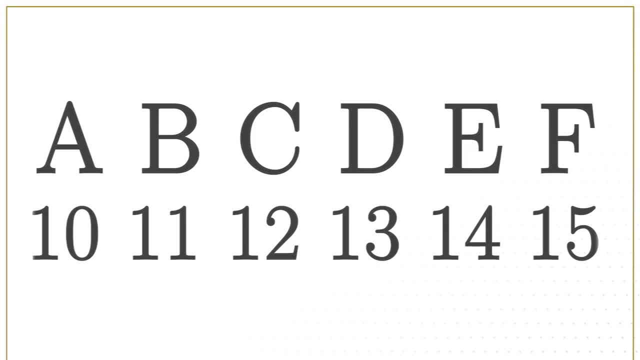 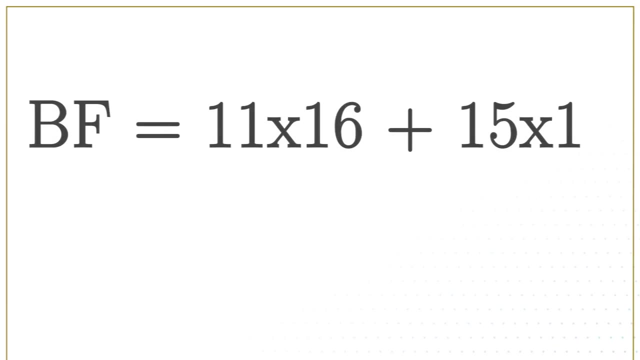 Let's look at the value of these numbers. You know how it goes. We have to note down the place values. Follow me on this one. We write the place values and write the number in the expanded form. So BF equals 11 for B times 16.. 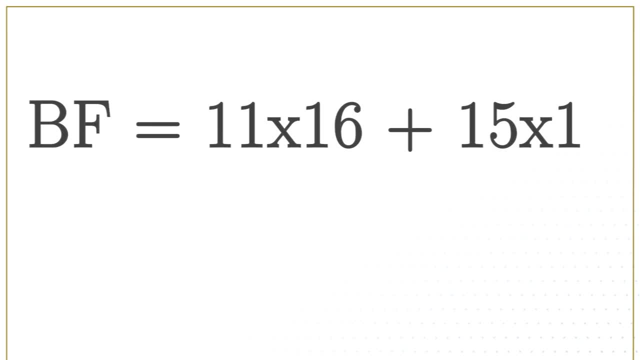 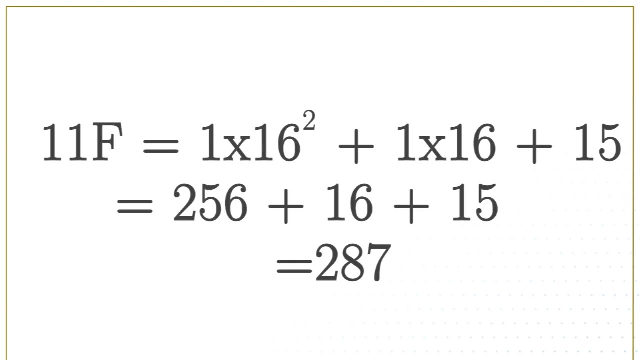 Plus 15 for F times 1.. And that gives 176 plus 15,, which totals 191.. As to 1, 1F, that is 1 times 16 squared plus 1 times 16, plus 15 times 1,. 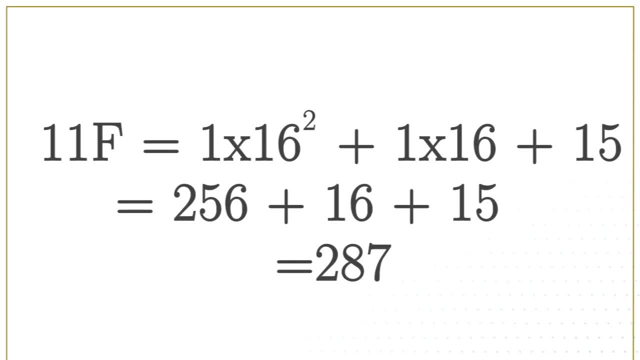 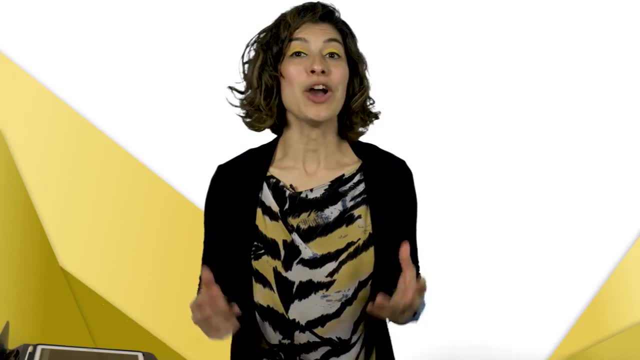 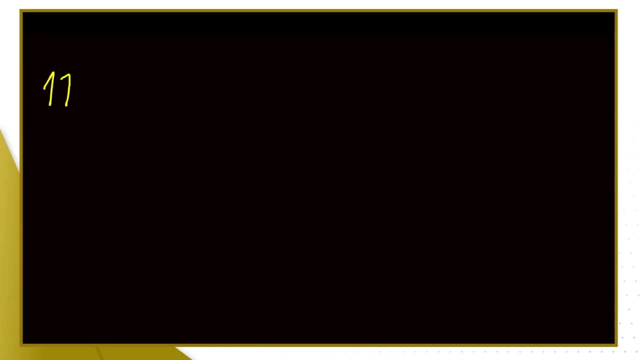 which equals 256 plus 16 plus 15 and totals 287.. Very different numbers. Let's see all of this in action with two examples. Let's write the number 179.. That's a decimal number. Let's write this into octal. 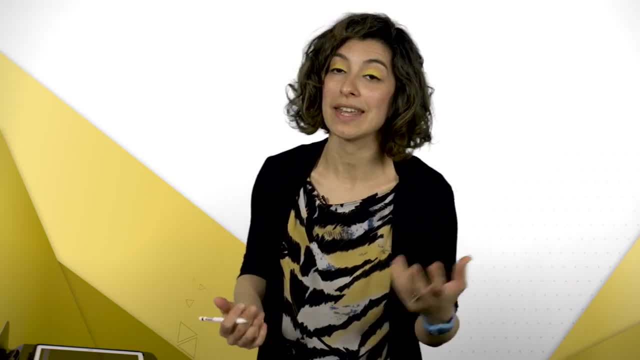 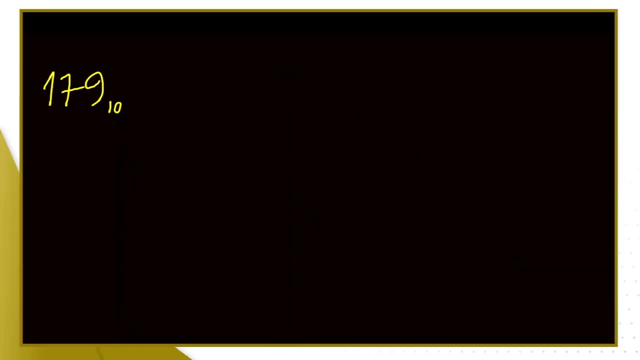 We're going to use the division algorithm, We're going to divide by 8, over and over again, and taking note of the remainders, And those will be the digits of the number in octal. So, on our calculator, 179 divided by 8, that is 22.. 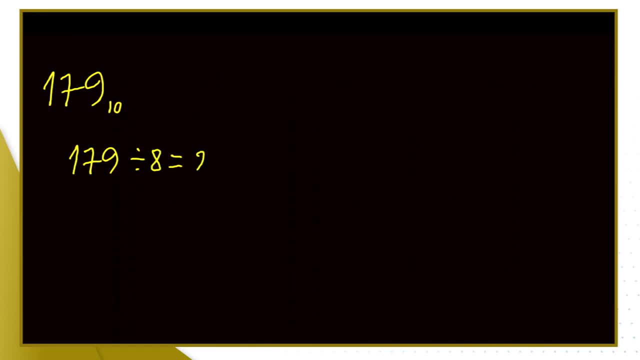 179 divided by 8, that is 22,. integer part. Let's work out the remainder. So we take the 22 times by the base, which is 8.. We got 176.. That, taken away from 179, leaves remainder 3.. 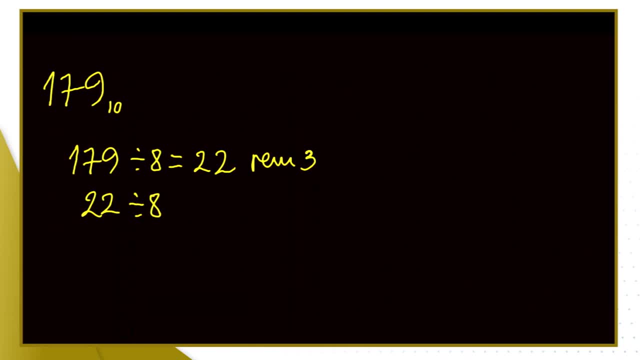 And now we divide the 22 by 8.. 22 divided by 8.. Yeah, We got 2., We got 2.. And the remainder will be 2 times 8,, which is 16.. 16 to 22 is 6.. 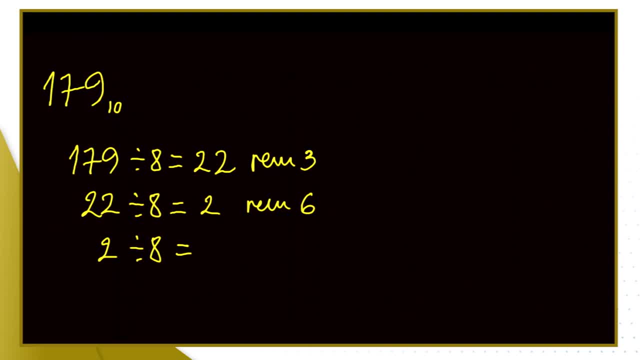 And now we divide 2 by 8, which is 0, remainder 2.. The first remainder is the rightmost digit, so the number is 263 in octal. We could, instead of using the division algorithm, match the powers of 8,. 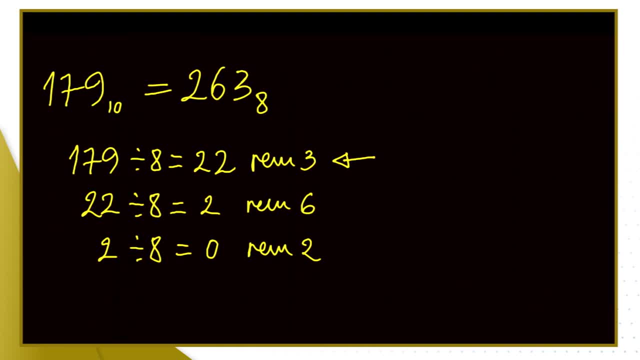 which is really essentially what we've done here. But let's look how that seems. You would write: the powers of 8.. 1, 8, 8 times 8, 64.. And the next one: 64 times 8, 512.. 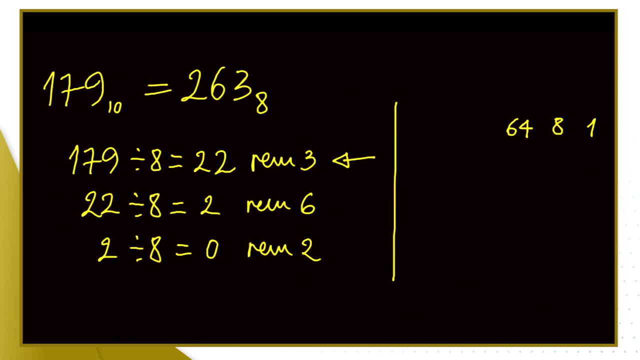 512 is too large for 179, so we don't need it. And now we would write 179 as multiples of these powers And then add up, And then add them all up. So how many 64s go into 179?? 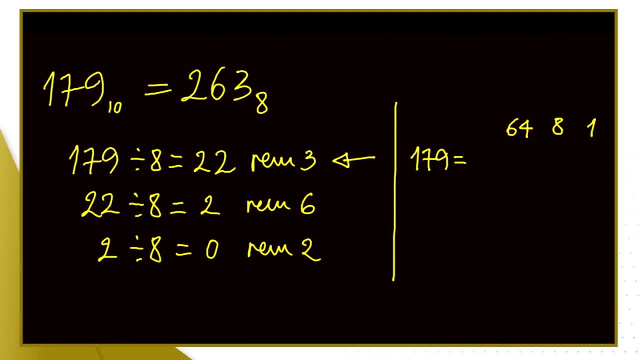 Well, 179 divided by 64. That is 2, 64s, And let's see how much is left now. So 64 times 2 is 128. We do 179. take away that 128.. We've got 1,, we've got 5.. 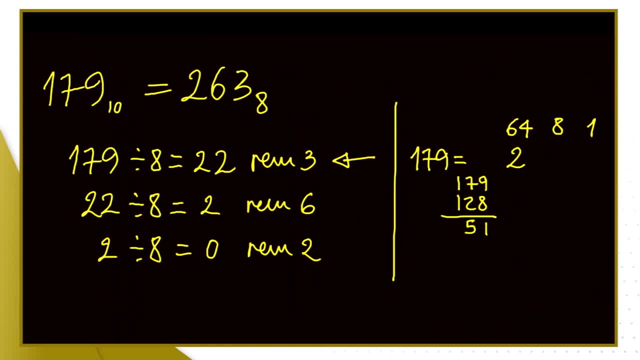 So we've got 51 left. We need to make 51 out of 8.. How many 8s? Well, we've got now 51 divided by 8. That's integer part 6.. 6 times 8, 48.. 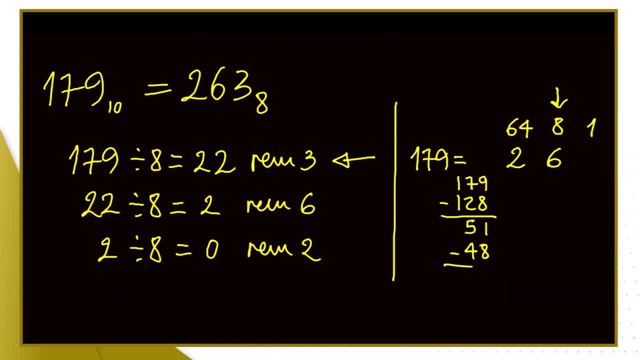 So we've got 51. take away the 48. And we are left with 3. And so 3 ones make the rest of the number. Of course we get the same result as we got using the other method, And we're essentially doing divisions by 8.. 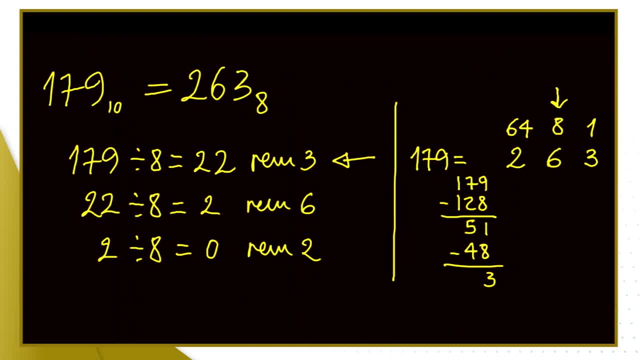 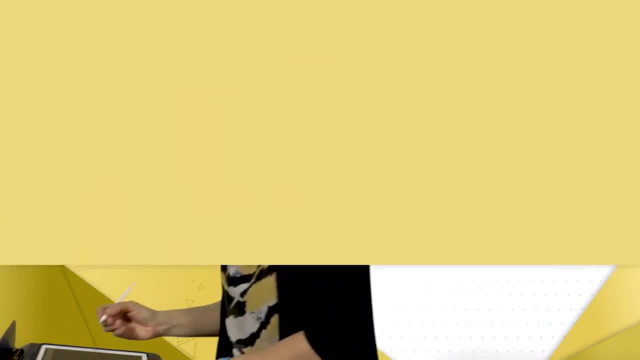 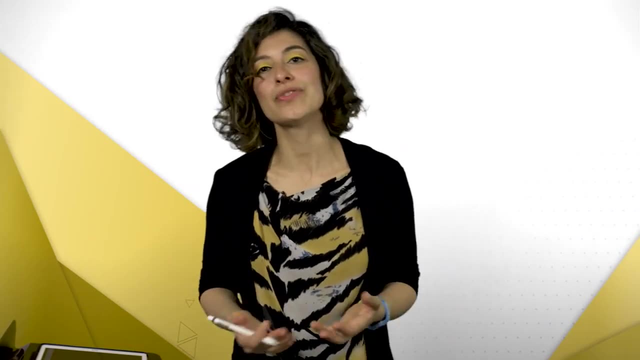 But in this case we're doing divisions by 64, and then by 8, and then by 1.. Let's now look at an example. in hexadecimal We're going to write the same number- 179,, in hexadecimal. Hexadecimal is based 16, so we're going to divide by 16, over and over again. 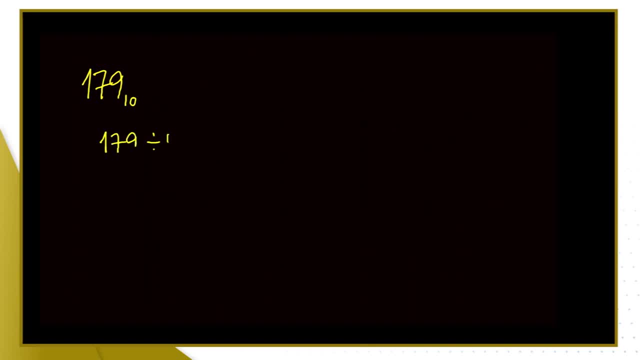 So we're going to do 179 divided by 16. And it does speed up stuff if we use the calculator. Divide by 16. And that is 11.. And let's work out the remainder: We do 16 times 11,, which is actually 176.. 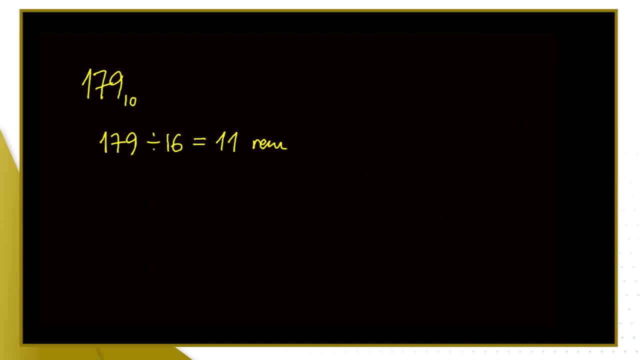 We should know that 176.. So 179 minus 176 is remainder 3.. And now we do 11 divided by 16, which is 0 remainder 11.. So the remainders have to be up to 16, but never 16.. 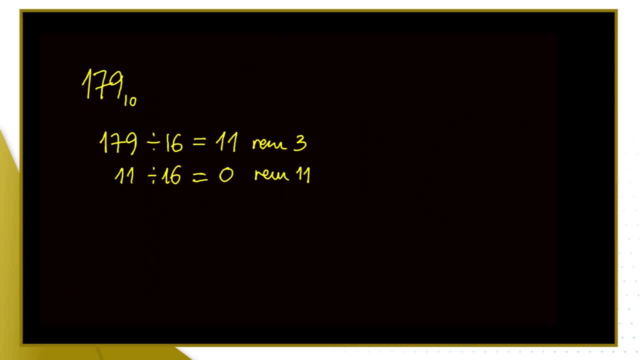 Right. So here's our result, Here are our digits. So if we don't remember what is A, B and C, 9 is the last numerical digit. A is 10.. B is 11. C is 12, and so on. 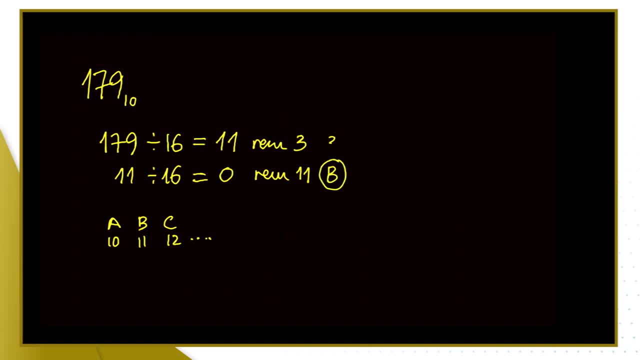 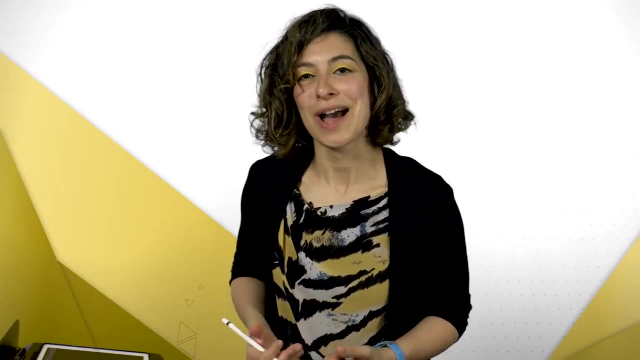 Well, this is going to be a B And this is a 3. So our number- remember the first remainder- is the rightmost digit. So we have B3 in hexadecimal. Let's also look at how we could do this with approximating by powers of 16.. 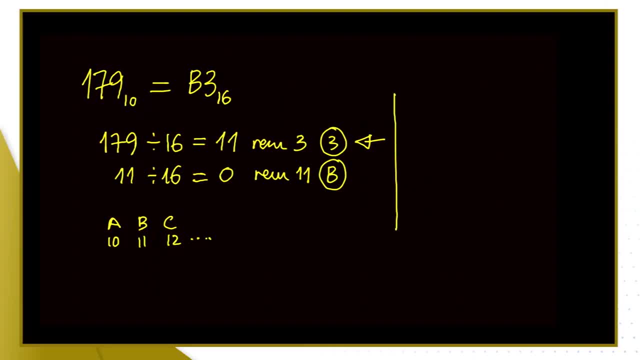 In this case, it's very, very close to what we did. We start with 1. 16. 16 squared is 256. And we make 179 using these numbers. 256 is too large. We're not going to need. 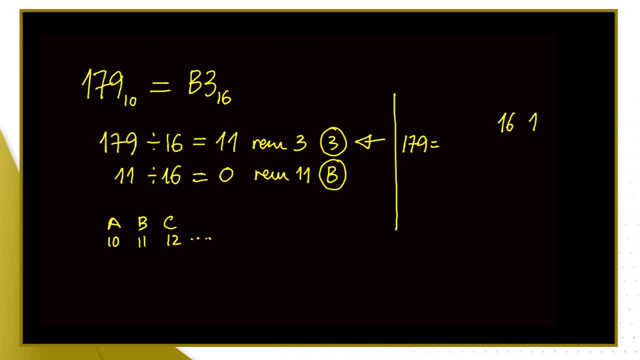 So the question is how many 16s fit into 179?? Well, we would do 179 divided by 16, which we've done for the previous calculation. So it's going to be 11 16s, And then we have remainder 3.. 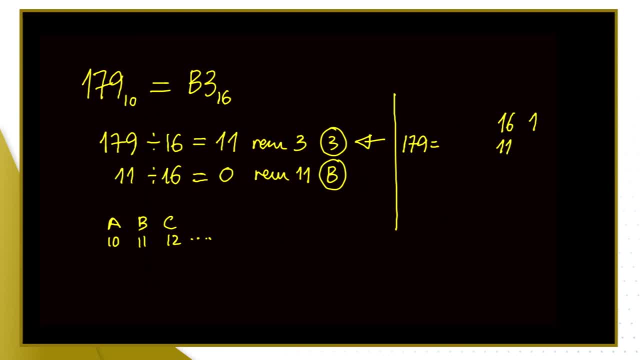 So 11, 16s, 16 times 11, 176.. So we got remainder 3.. And that 3 is made of three 1s. So, like we did before, this is a B, That's a 3.. 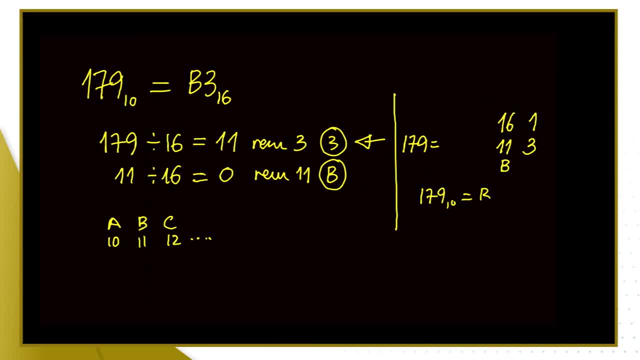 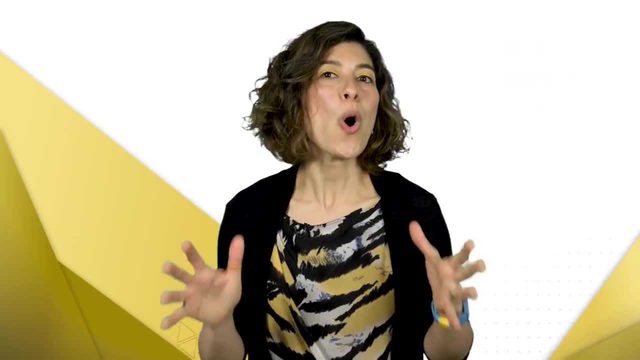 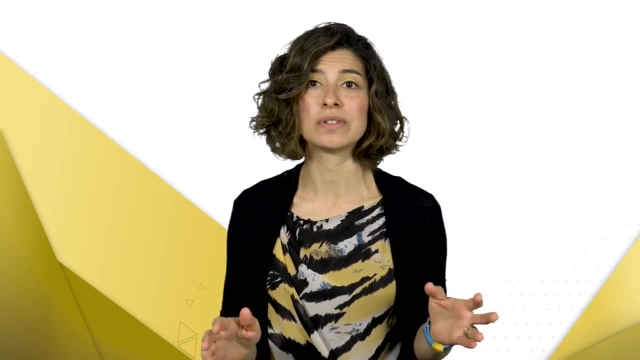 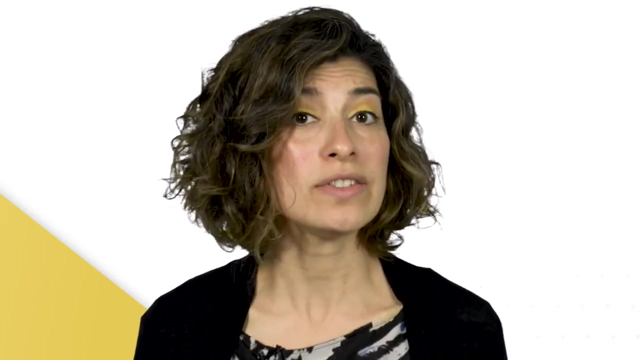 So 179 is B3 in hexadecimal. You have now all the tools to work in any number base. We just looked at the place values for octal and hexadecimal And we can translate between these bases and decimal. Octal uses 8 digits, from 0 to 7.. 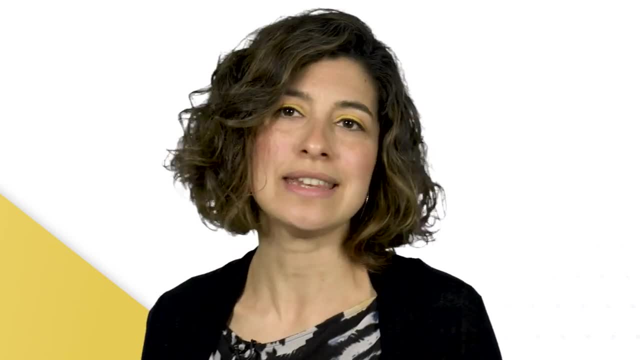 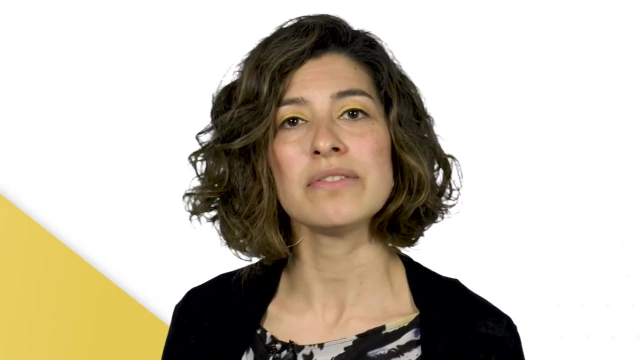 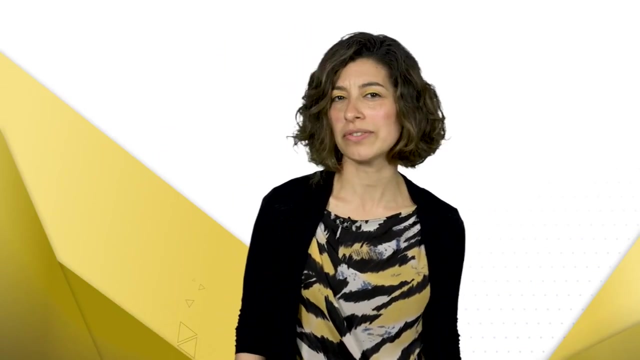 And hexadecimal requires 16 digits. So we use all the digits 0 to 9, followed by letters A to F to mean the values from 10 to 15.. Next we will look at fractional numbers. Have a think of what the place values should be. 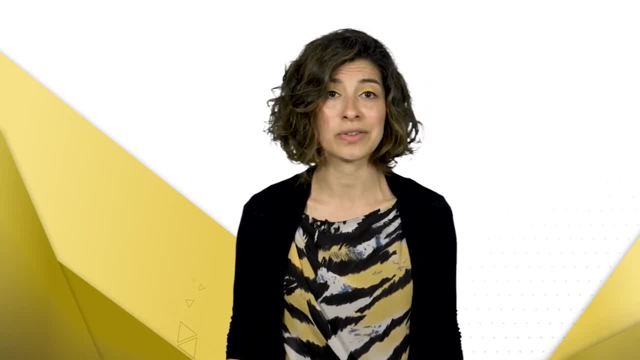 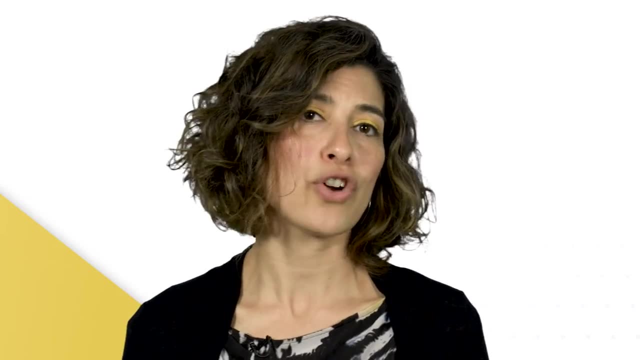 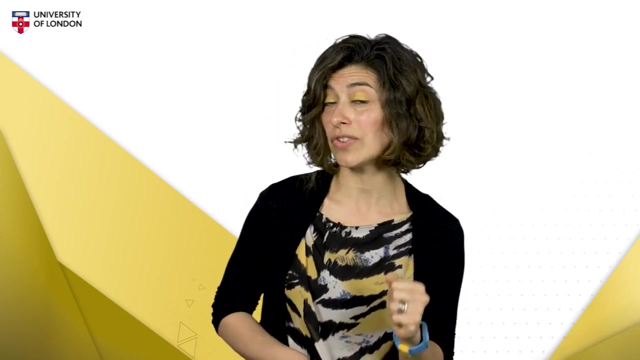 for fractional numbers written in octal and hexadecimal To fully appreciate the upcoming videos. start extending the algorithms for operations in binary into these new bases. And I asked you to think about steganography. I haven't forgotten that, So let's get started. 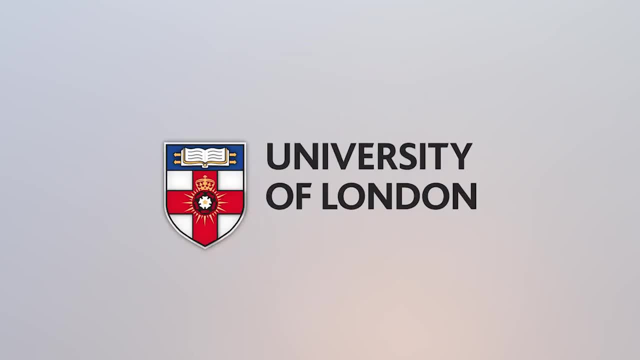 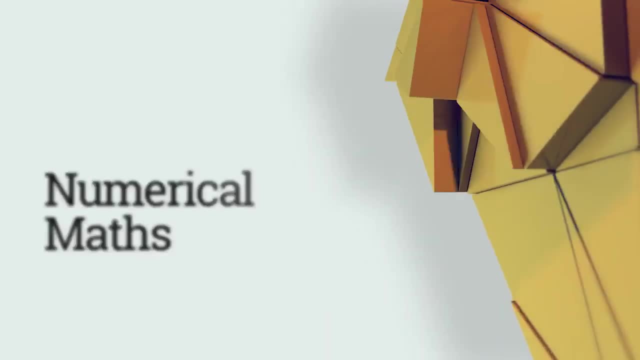 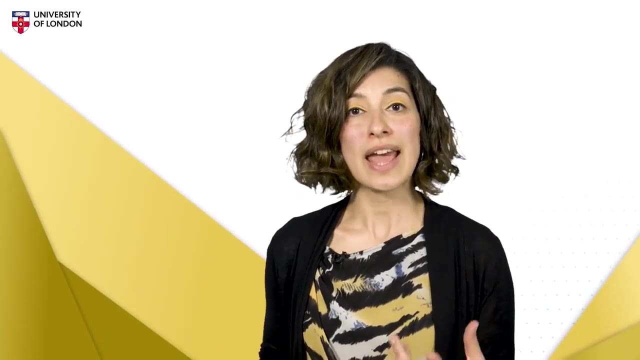 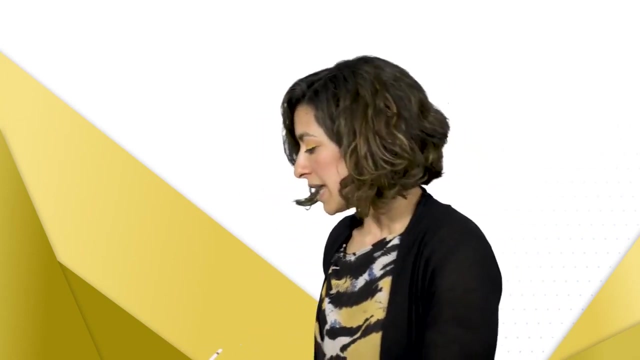 We're now looking at how to work with fractional numbers in hexadecimal and octal. Let's remind ourselves of the place values in octal. The integer place values start with 1, and then multiply by 8,, multiply by 8 again. 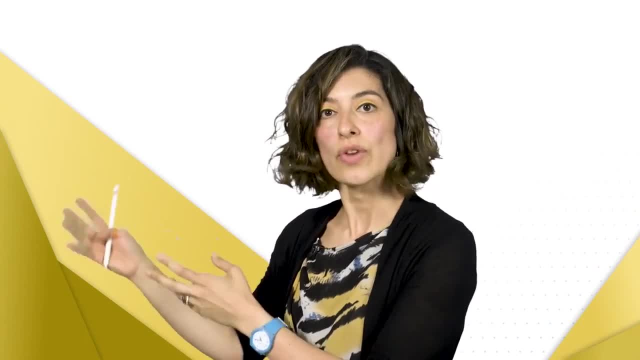 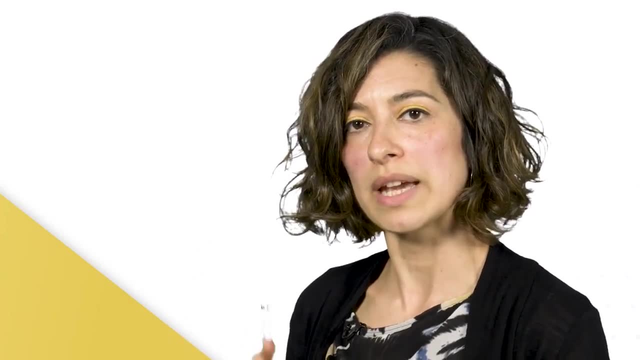 so 1,, 8,, 64, and so on For the fractional part, like we did in binary, we start dividing by the base. So we're going to divide 1 by 8, and then divide by 8,. 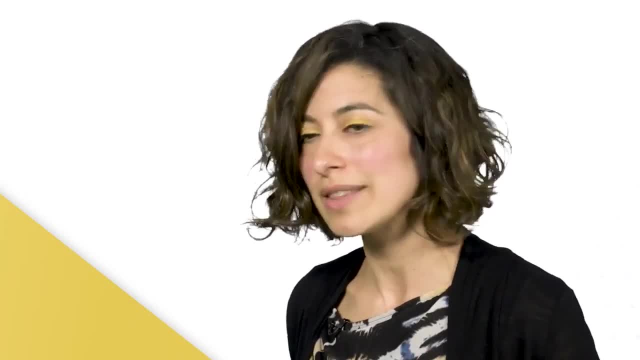 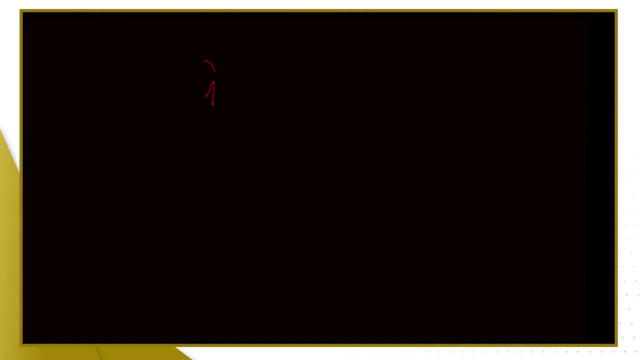 and divide by 8, and so on to get all the fractional place values. I'll write this down. So the integer place values we wrote 1, and then 8, and then 64, and if you carry on. 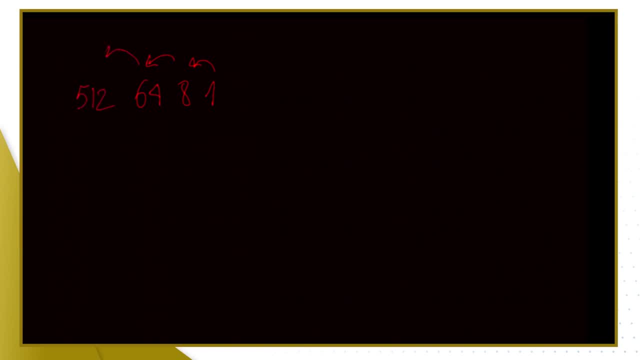 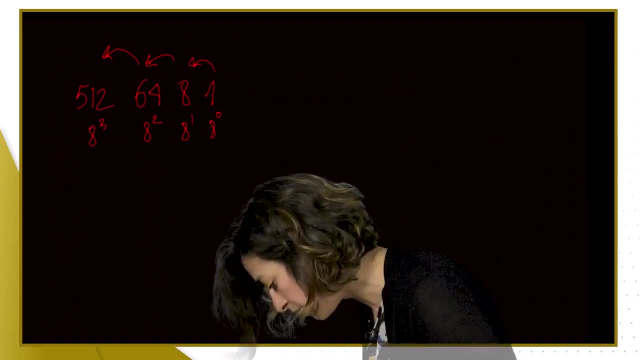 you would get to 512.. Just reminding ourselves that these are powers of 8.. So, 8 to the 0,, 8 to the 1, 8, squared, 8 cubed Gets really big with powers of 8, doesn't it. 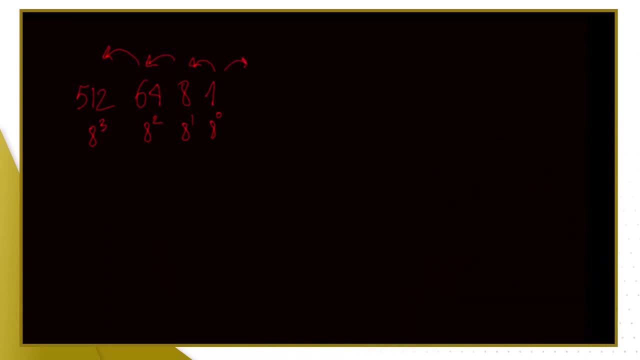 For the fractional part, we're going to divide by 8.. So we're looking at 1 eighth, then 1 over 64, and 1 over 512.. The powers: 8 to the minus 1,, 8 to the minus 2,. 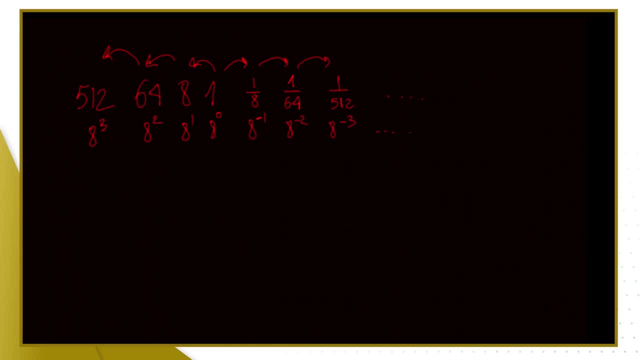 8 to the minus 3, and so on. I'm just going to write what these guys are in decimal. So 1 eighth is 0.125, 1 over 64, we're looking at 0.015625,. 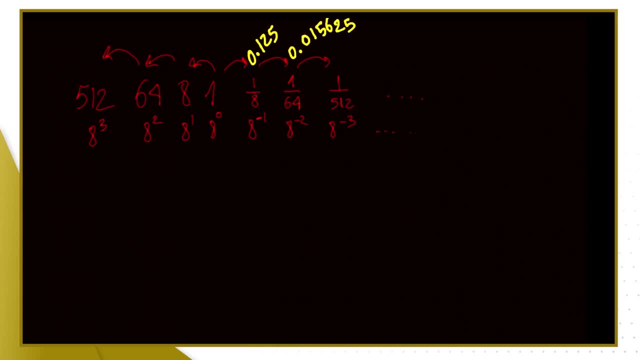 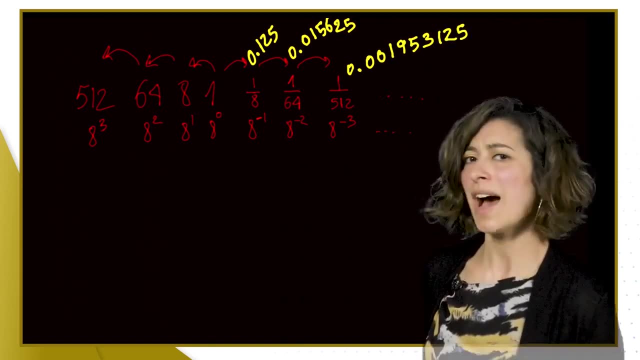 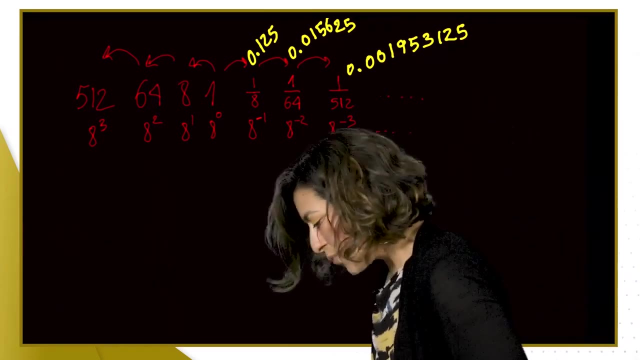 and the 1 over 512, 0.001953125.. I'm somehow feeling a little bit discouraged of adding these numbers by hand, but hey, that's what calculators are for. So we're going to look at an example of how to translate a number that is in octal into decimal. 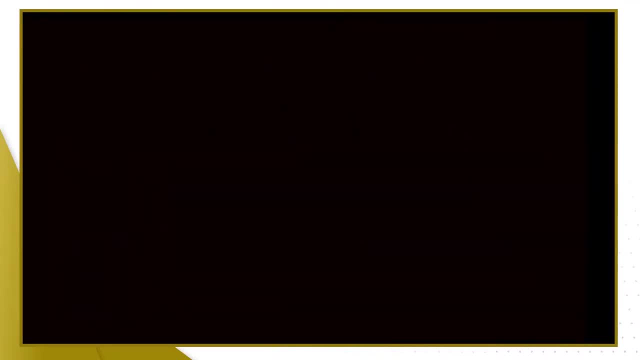 So there we go. Say our number is 0.72,. this is a fractional number in octal. that's our reminder there, with a little 8.. This means that the 7 is in the place value for the 1 over 8,. 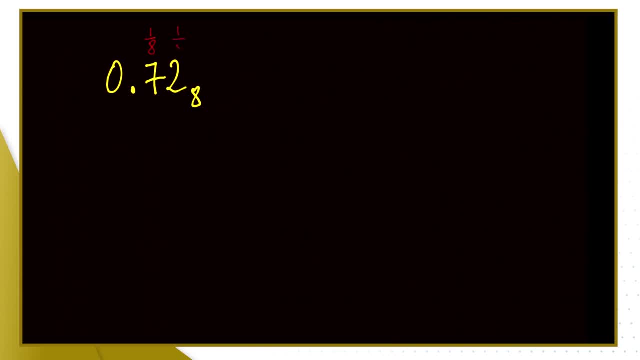 and the 2 is in the place value for the 1 over 8 squared. So all I'm going to do is to say I've got 7 of that lot of 1 eighths and I've got 2 of that lot of 1 over 8 squared. 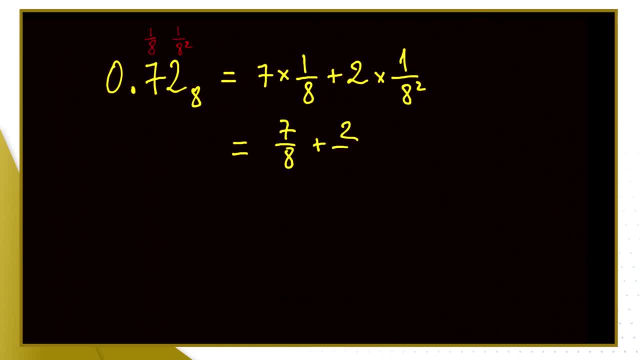 So I've got 7 eighths plus 2 over 64, and adding it all up that's 29 over 32, which is 0.90625 in decimal. So that is fractional octal to decimal. Let's do the reverse now. 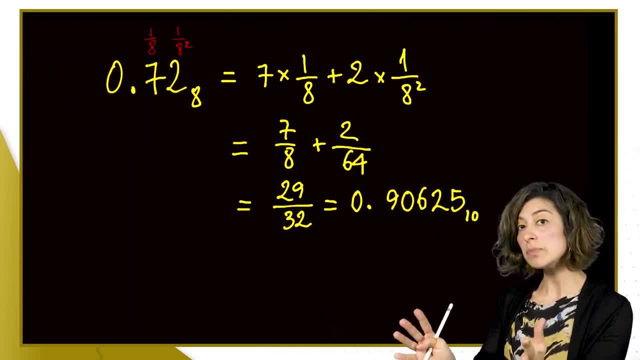 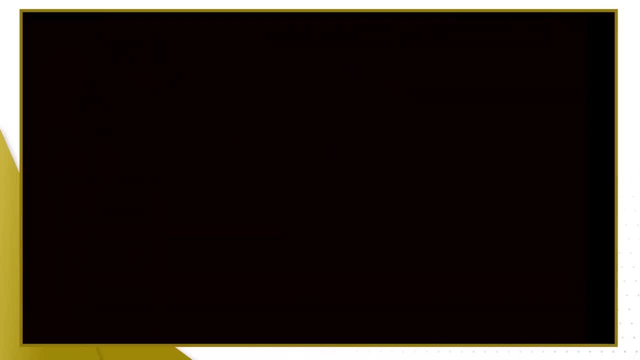 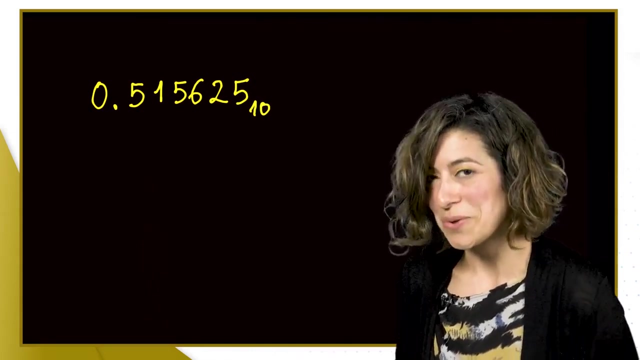 Let's look at a fractional decimal number and write it in as a fractional in octal, Say, we've got the number 0.515625, that's our decimal nice and long. I feel discouraged to compare this number to the powers of 8,. 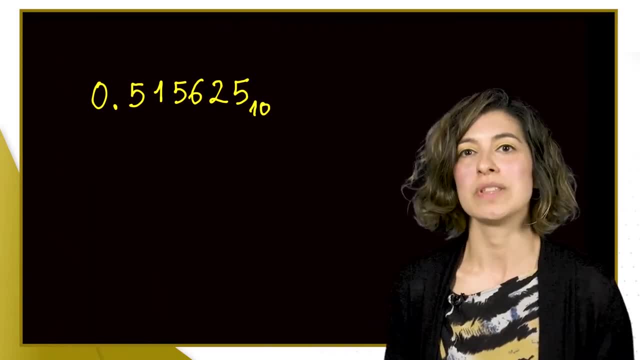 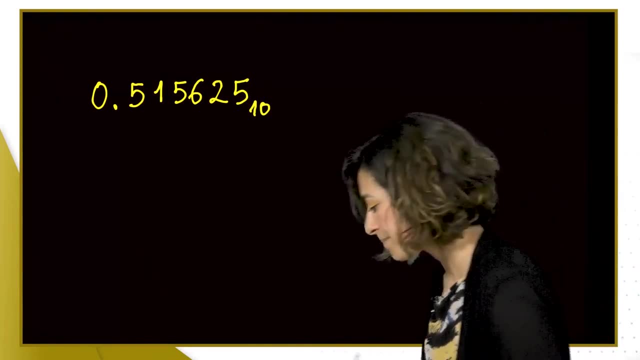 the negative powers of 8,. so we're just going to do the algorithm of just multiplying by 8 over and over again and taking the integer part as the digit. Let's do that. So 0.515625 times 8,. 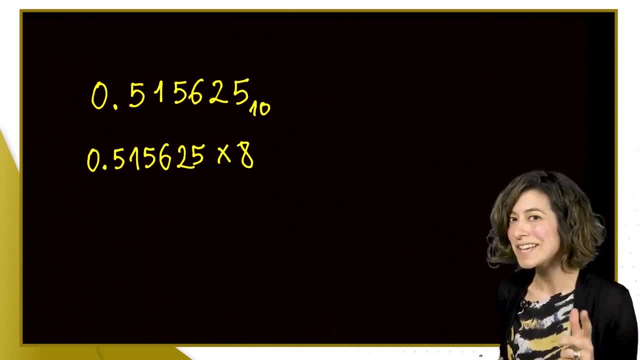 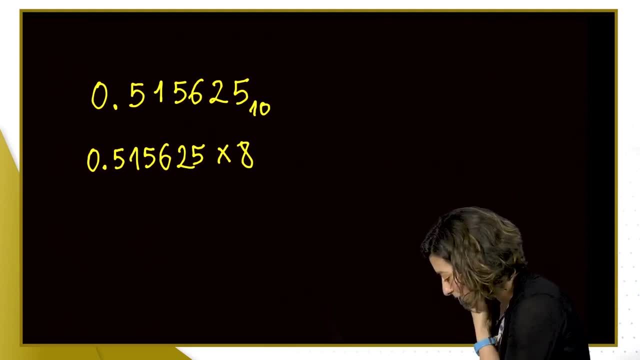 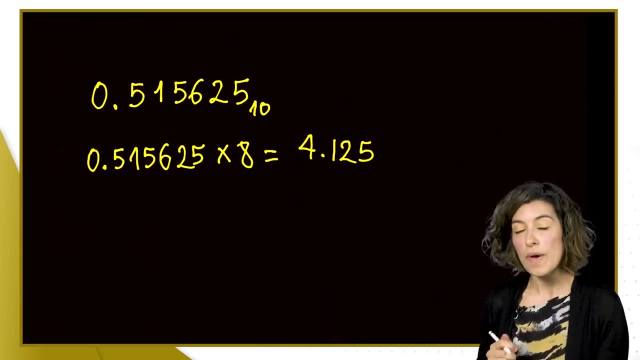 and we're doing times 8, because that is octal. in binary we multiply by 2, in octal we multiply by 8.. Calculator says 4.125, now the integer part of this result is 4, that's going to be our first fractional digit. 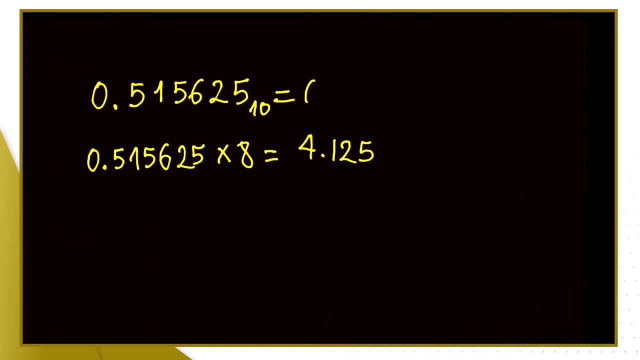 in octal, So 0.4, and that 4 comes from that integer part. Now remember what we did in binary: we took away that integer part and worked with what was left, the fractional part. So from here we take away the 4,. 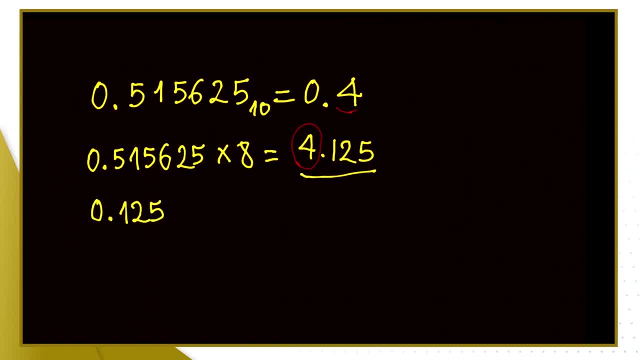 which means 0.125, that's what we're left with. And now multiply by 8.. Multiply by 8, and, surprise, surprise, we get 1!. So that is the next octal digit, And we stop, because this one has no fractional part. 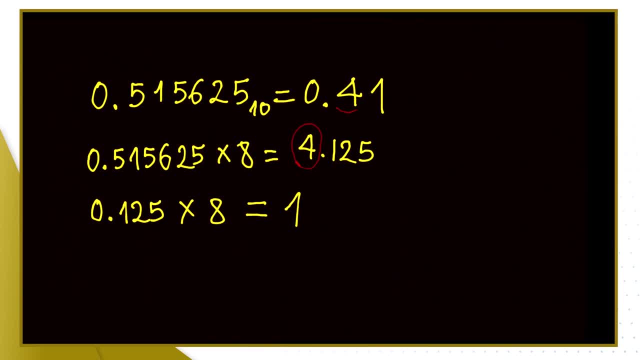 so actually it's an integer number. So integer and we stop. Yeah, I'm relieved I don't have to do more multiplications of 8 here, I'll stop, and so this is my number in octals, Just a reminder. 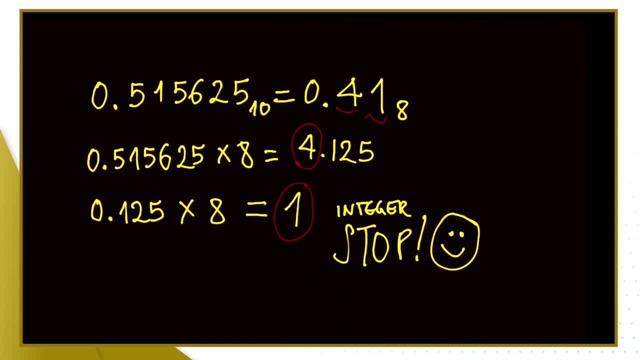 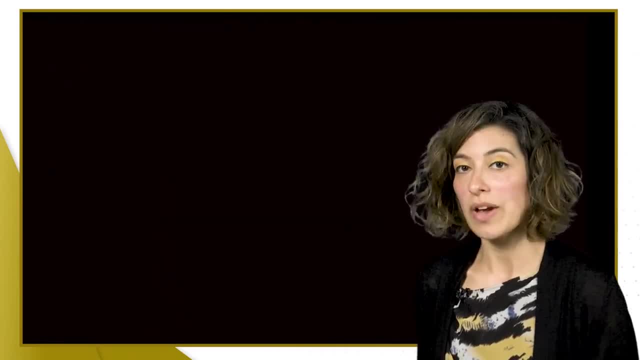 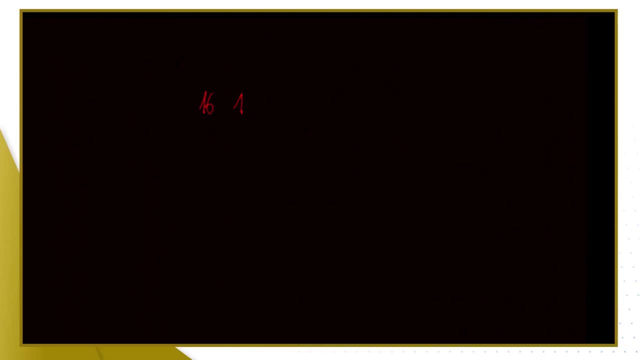 where that one came from. that one there became that one there. Okay, Let's look at hexadecimal next. Just a reminder: hexadecimal place values are powers of 16, we'll write them. So we have 1,, 16, and then 16 squared. 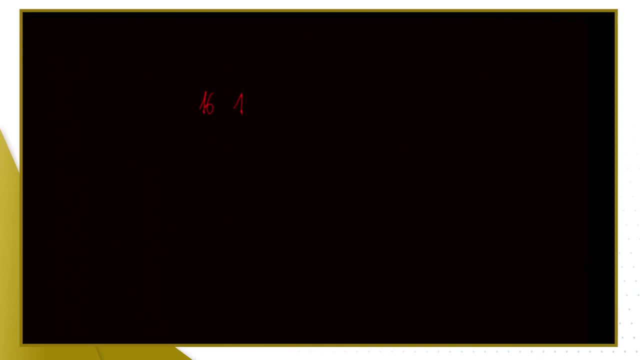 which, you'll remind yourself, 16 squared is 256.. 16 cubed 4096.. Those are the integer ones. so that's 16 to the power of 0,, 16 to the 1,, 16 squared 16 to the cube. 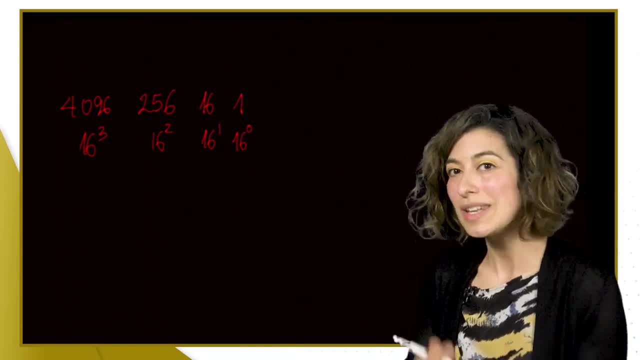 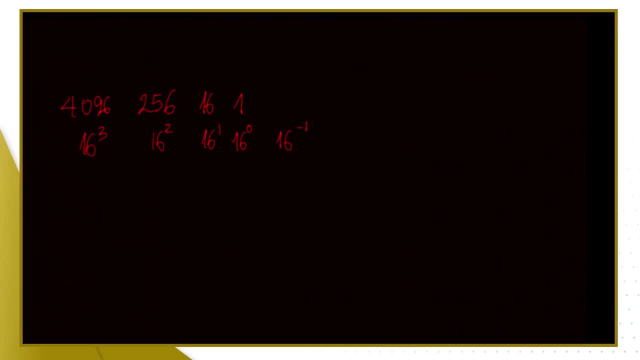 We're going to need the fractional parts with the negative powers of 16 for this bit. So we're going to divide by 16, so 16 to the minus 1, which is 1 over 16, that writes down as a decimal as 0.625.. 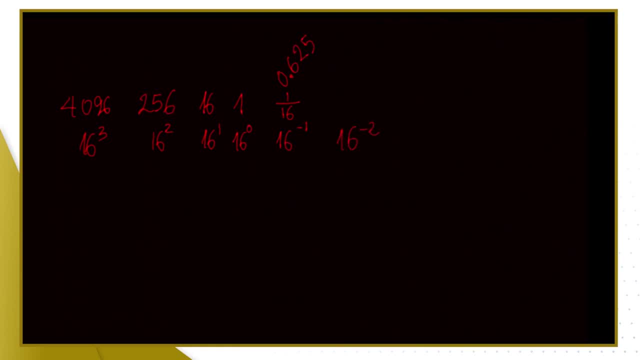 Next, 16 to the minus 2,, which is 1 over 256.. Calculator says we get 0.003906250, and just carry on like that: 16 to the minus 3, and so on. So these are the place values. 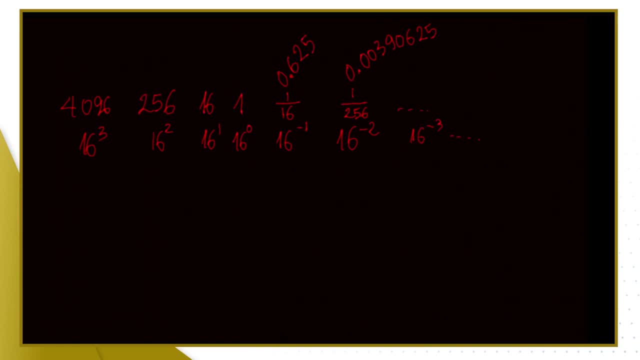 So for fractional numbers in hexadecimal, we're going to work with these place values here. Let's look at an example. Right, let's transform this number here, 0.9b, which is a hexadecimal number. Let's remind ourselves what these b's and a's and so on mean. 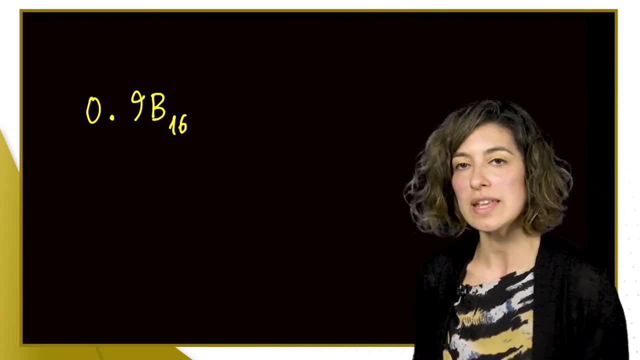 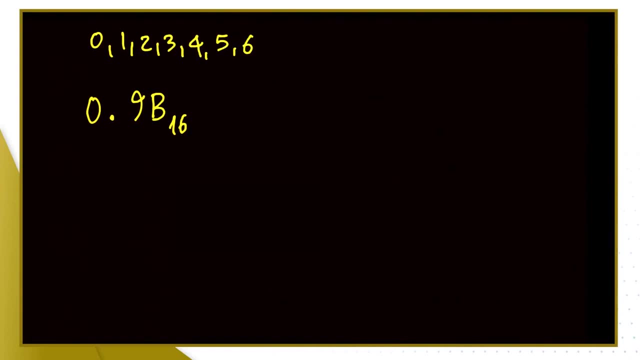 The digits in hexadecimal. we have 16 digits which we need to work with, and those are 0,, 1,, 2,, 3,, 4,, 5, 6,, 7,, 8,, 9,. 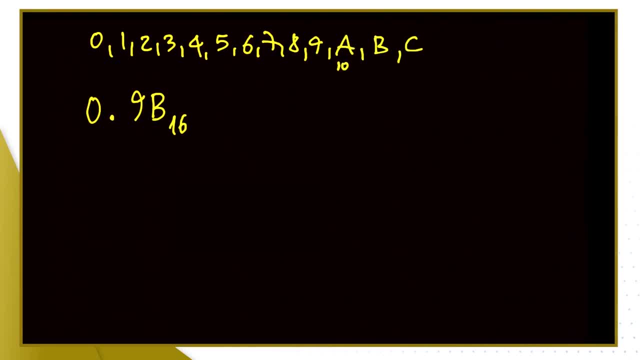 and then a for 10,, b for 11,, so 10, 11,, 12,, d for 13,, e for 14,, f for 15.. That's it Now. I recommend that when you do your working. 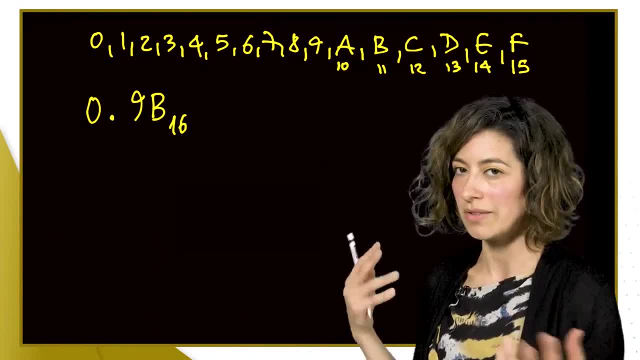 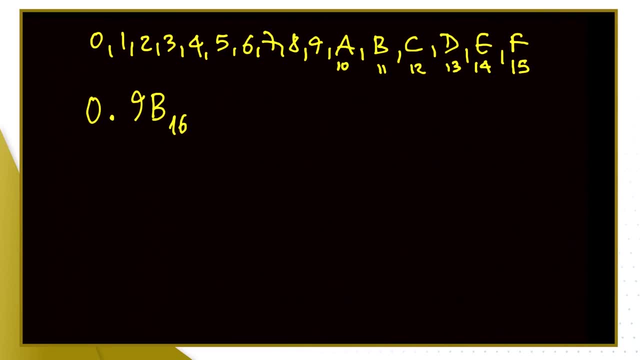 write at the top of the page the digits so you don't confuse what a, b, c and d and so on are worth. There we are on the top line, So we're going to write what the place values are and we're going to work out what this number is in decimal that way. 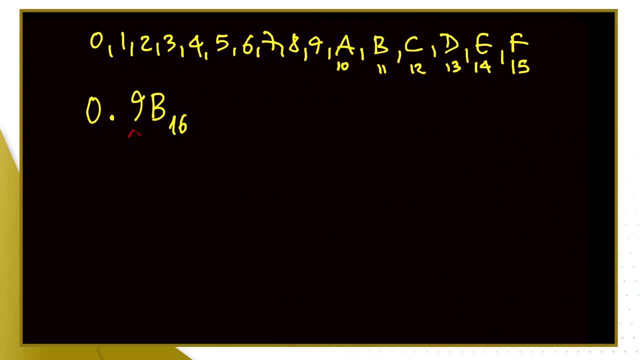 So we just did this. The 9 stands for the 1 over 16, and that b is on the position for the 1 over 256. That means that this number is 9 times 1 over 16, plus 11 times 1 over 256. 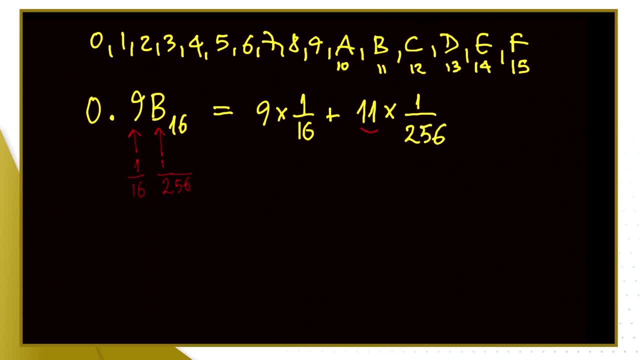 And just a reminder again, this 11 here is because of the b and this 9 here is the other digit on the original number. So calculator to the rescue: adding up these numbers, it comes out to 155 over 256,. 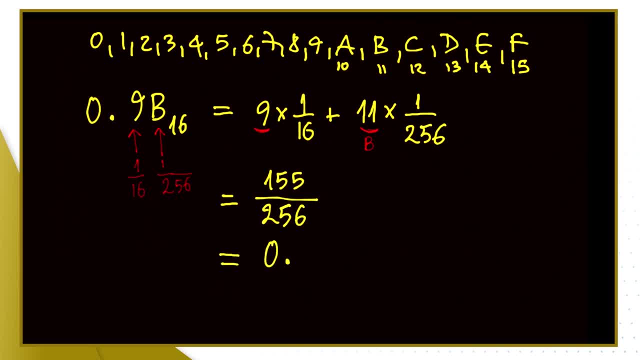 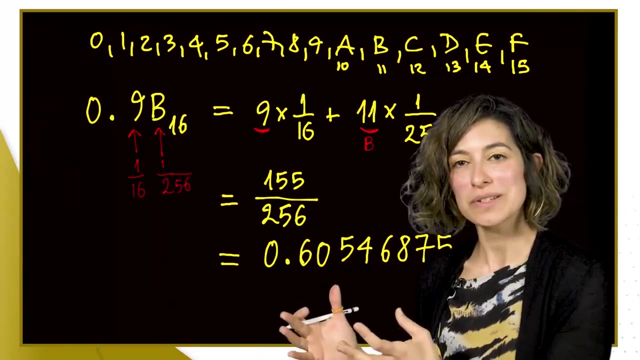 which is no more, no less than 0.60546875.. And that is in decimal. Now if your number had an integer part and a fractional part, you work out what the integer part is in hexadecimal doing the division by 16. 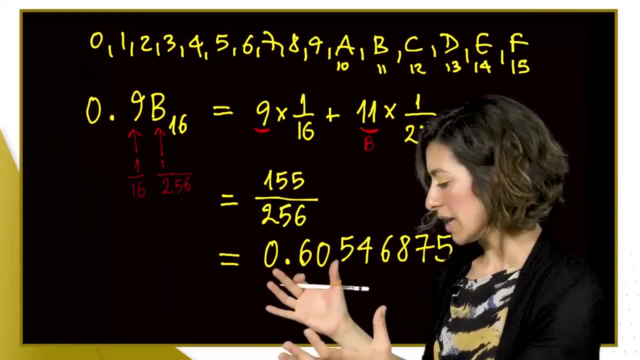 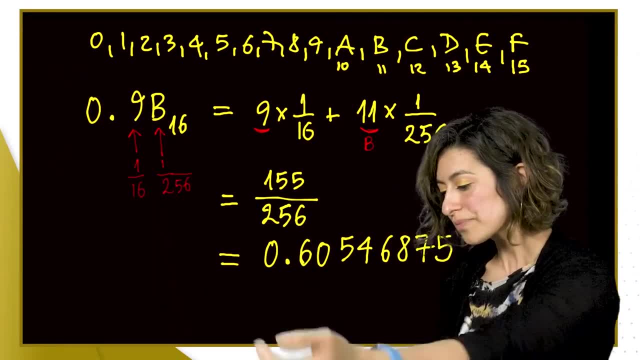 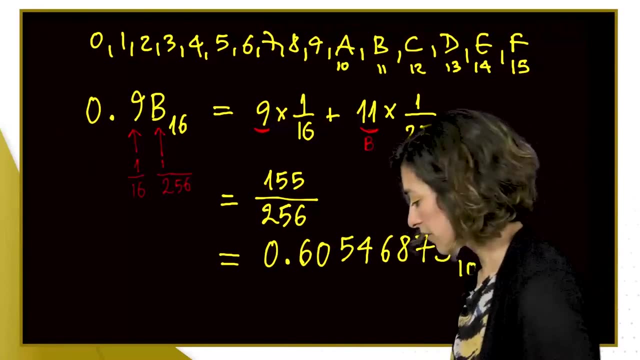 and take the remainders algorithm. Work out the fractional part using the algorithm I'm going to show you now, which is the other way around: Multiply by 16 and take the integer part as the digits. So the example I've got for us is: 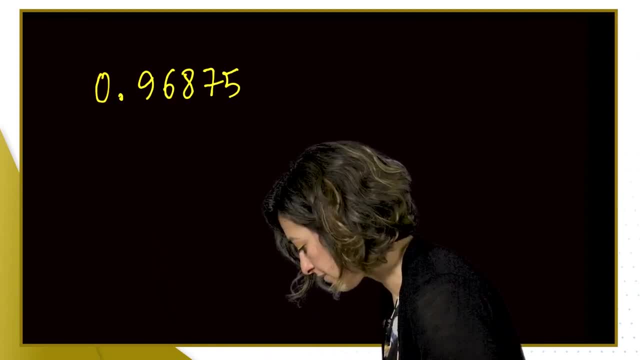 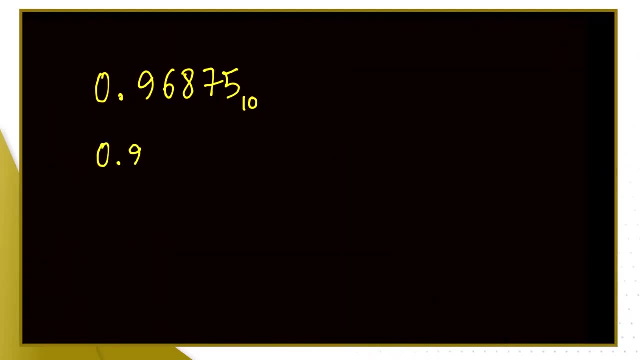 0.96875.. That's a decimal number. We want to write this in hexadecimal. We're going to start by multiplying by 16, because that's the base Base: 16.. Multiply that and we get 15.5, precisely. 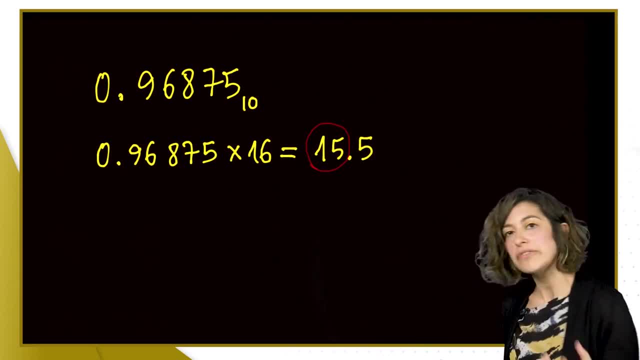 And this is the integer part. This is going to be our first hexadecimal digit. Now, remember, 15 in hexadecimal is f, So we're going to write it here: 0.f, That f on that 15.. From 15.5 here. 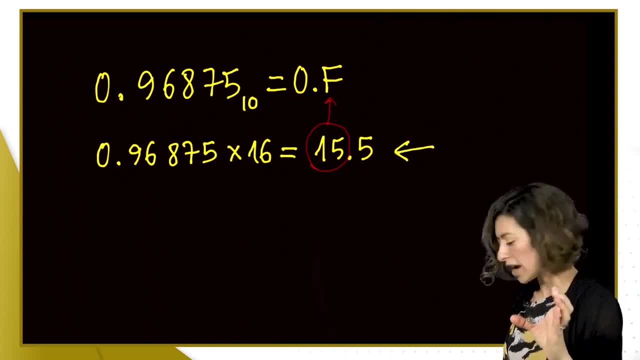 we're going to take away the 15 and just work with the fractional part, So 0.5.. And then we multiply by 16. And that is 8.. 8 is going to be the next digit And we stop. 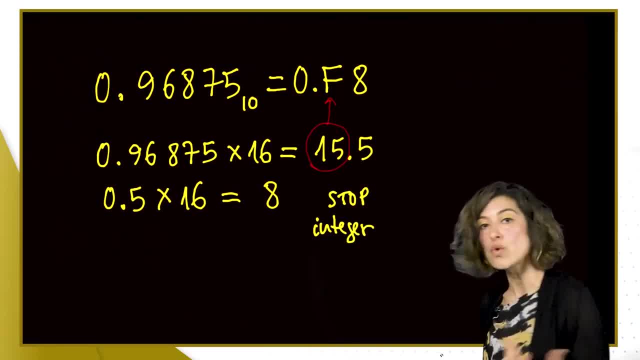 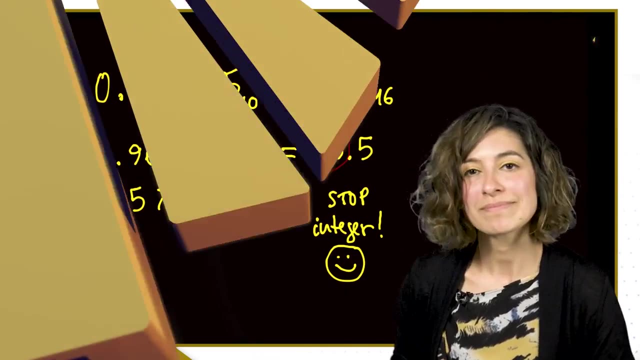 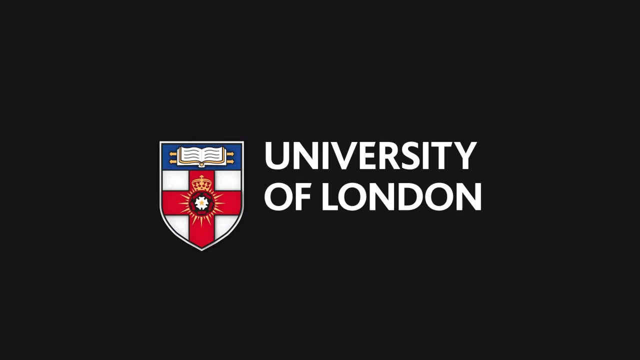 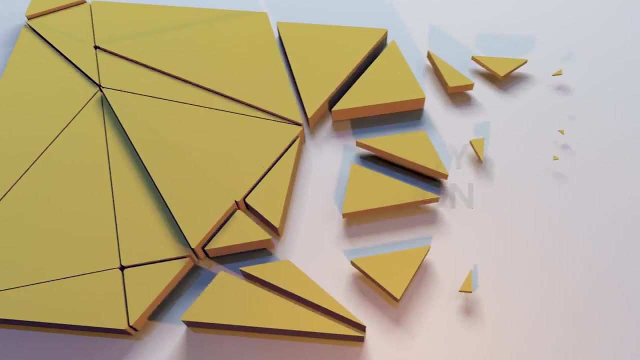 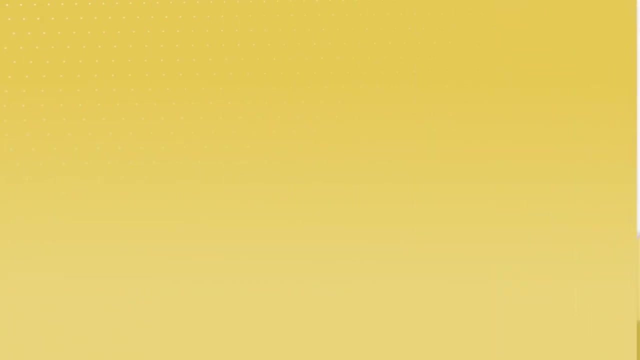 because 8 is an integer, There's no fractional part. to continue, Yeah, I'm still happy. So that means that that fractional number in decimal is written as 0.f8 in hexadecimal. Earlier, when you played with powers of 2,, 8 and 16,. 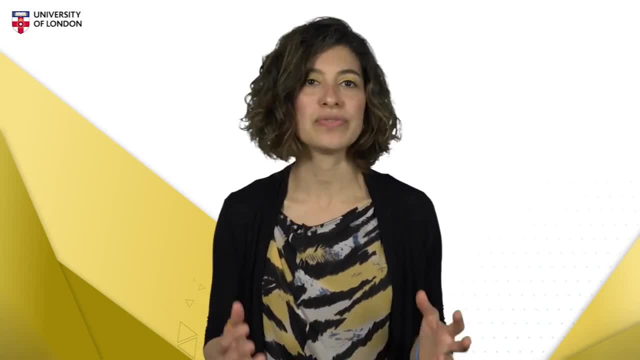 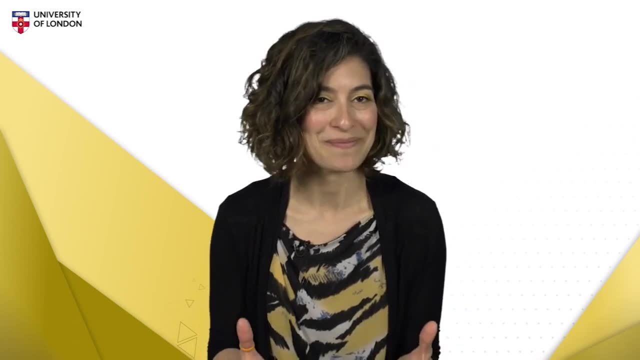 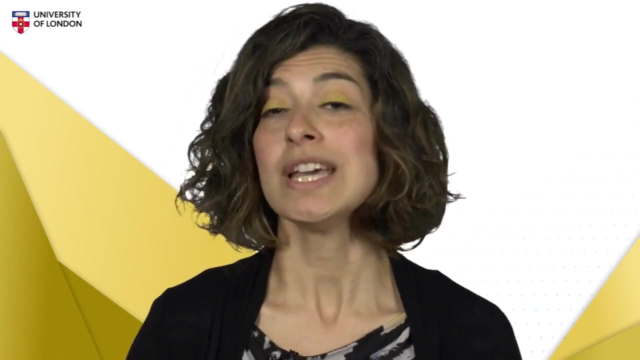 you probably noticed that there is a pattern between powers of 2 and powers of 8. And a pattern between powers of 2 and powers of 16.. We will use that pattern to move between binary and octal. We will use it too. 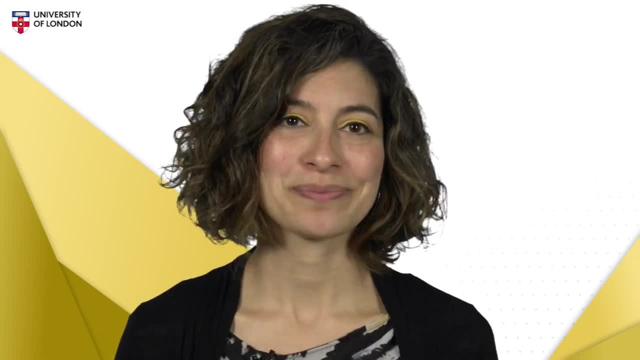 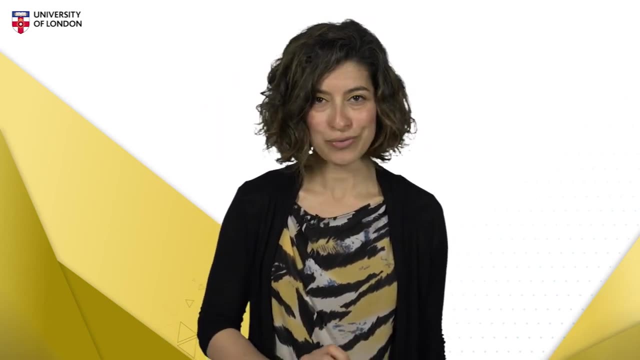 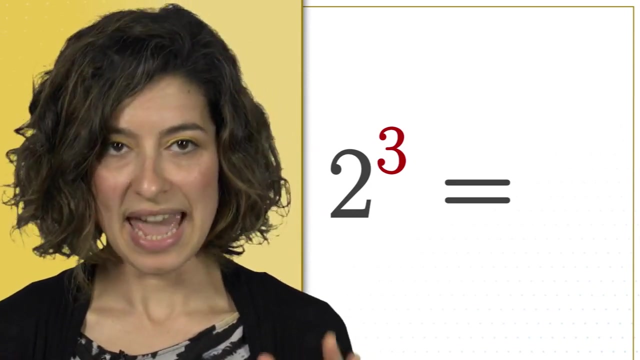 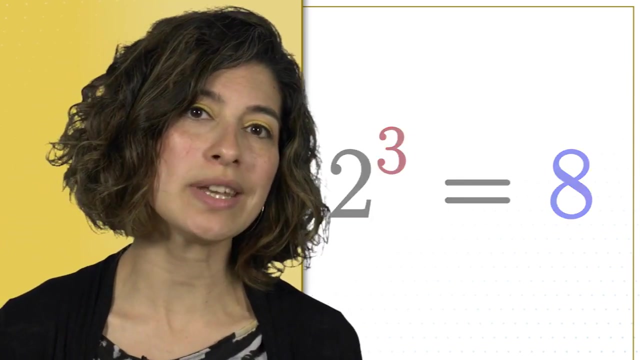 to move between binary and hexadecimal And between hexadecimal and octal via binary without going through decimal. The key thing to note is that 2 cubed is 8. And that means that one octal digit can be expressed as a binary number using up to three digits. 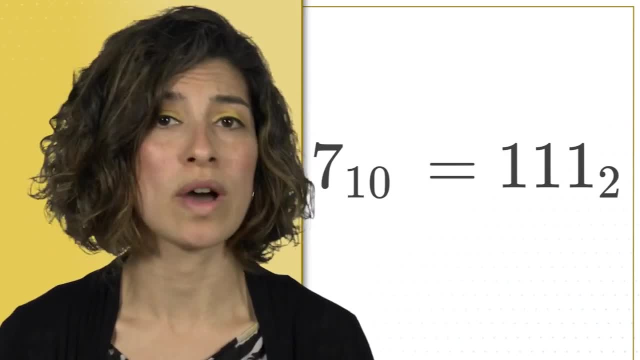 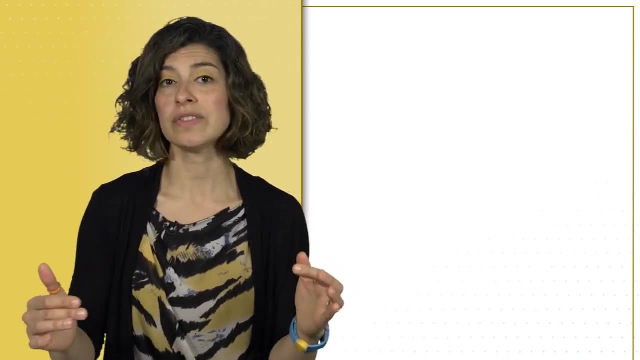 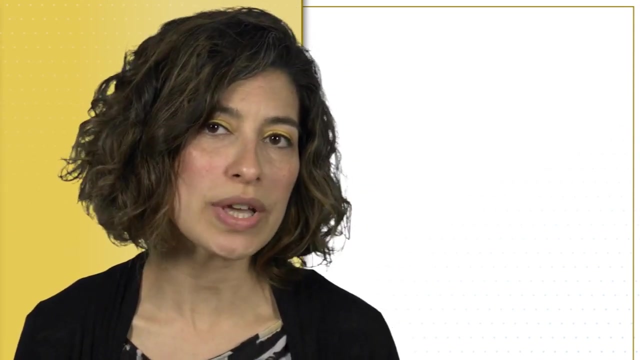 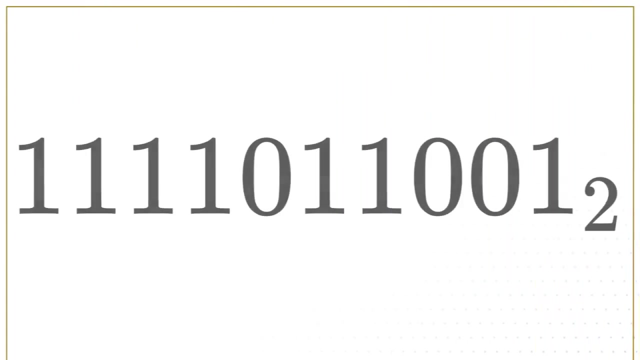 Note that 7 in decimal is 111 in binary. Take this moment to write the octal digits 0 to 7 as three-digit binary numbers. Answer in the in-video quiz with your results. Let's write the number 1111011001. 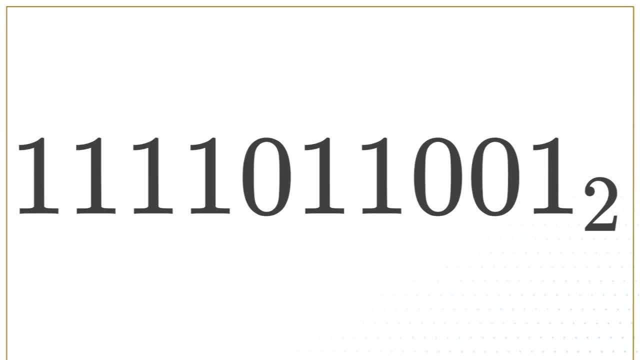 the binary number. in octal We count a number of digits. There's 10 binary digits- And starting from the smallest place value, the right-hand side, we group the digits in threes. So we start with a 1,, a 111,. 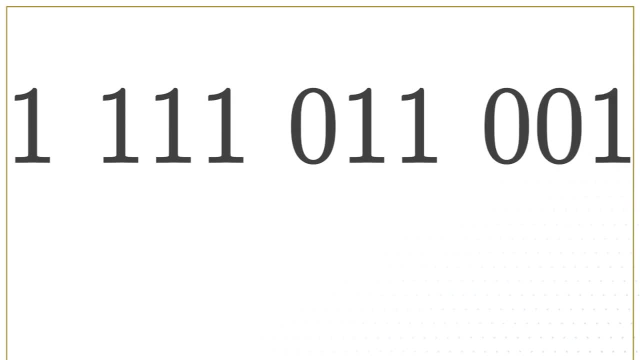 a 011, and a 001.. And now take each group of three binary digits as a number of its own right, So 1, a 111,, then 011,, then 001.. And write these individual numbers in decimal, which is exactly one octal digit. 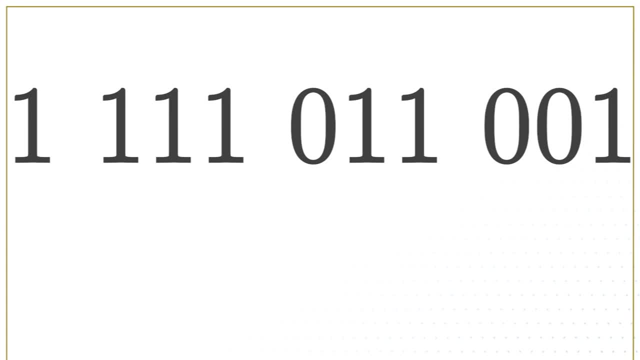 It is possible because they have at most three digits. That gives 1,, then 7,, then 3, and then 1.. And these numbers are the digits in octal, giving 1, 111, 011.. 011, 001 binary. 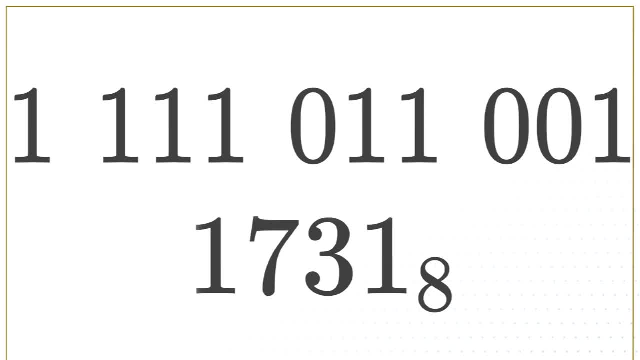 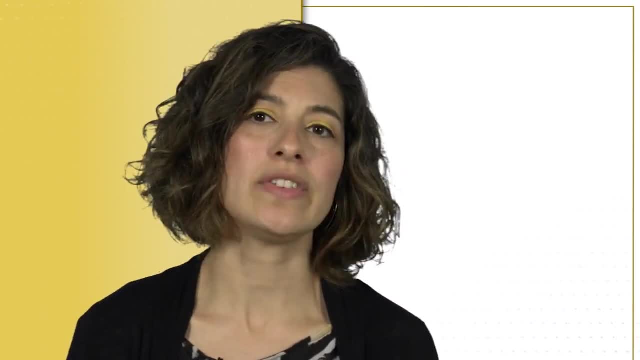 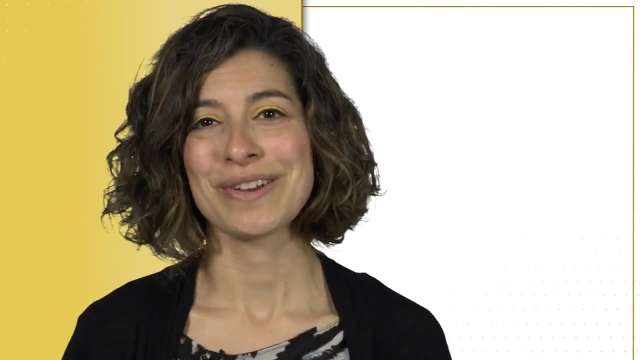 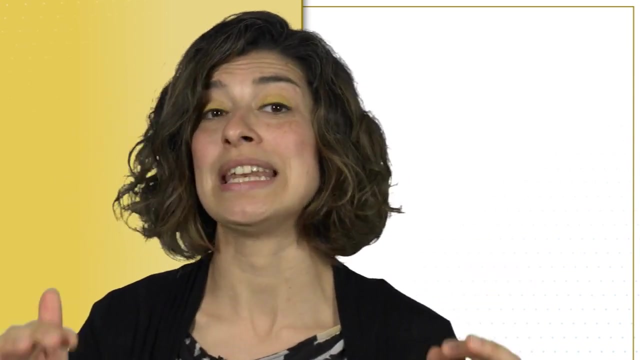 written as 1731 in octal. In short, we group the binary digits in threes and replace each group of three digits as one octal digit, which is the decimal conversion of the three-digit binary number, using the same conversion you used in the in-video quiz earlier on. 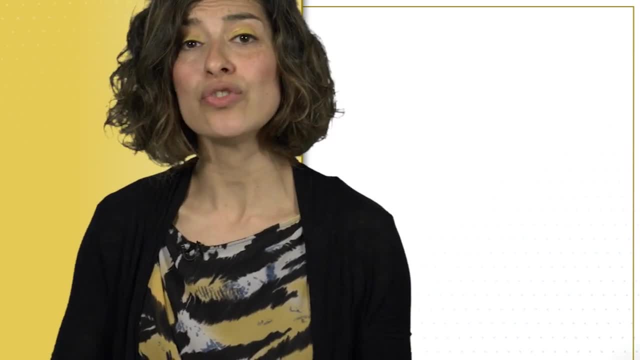 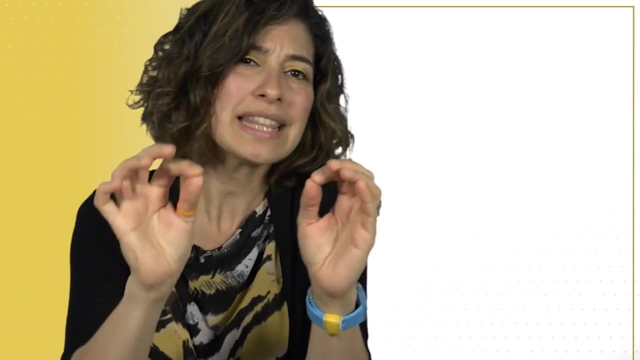 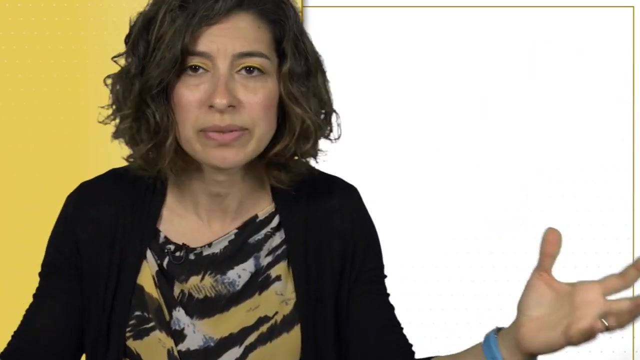 Remember that the whole point of this section is to do a direct conversion without converting to decimal. But we use decimal only at the level of groups of three digits to do immediate octal, rather than converting the whole binary number to decimal and then the whole decimal number to octal. 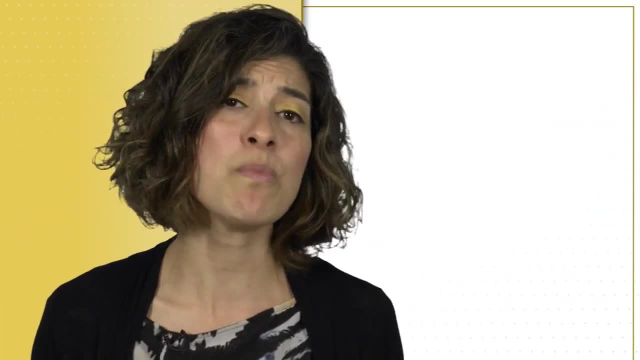 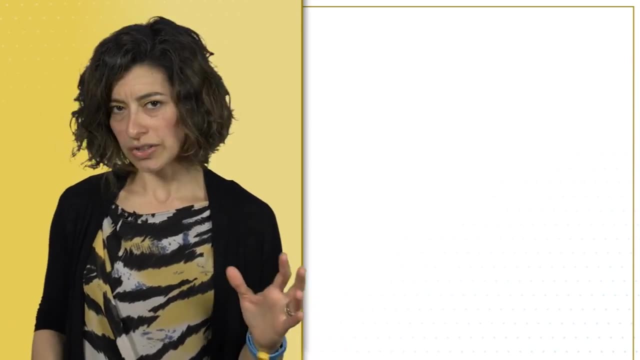 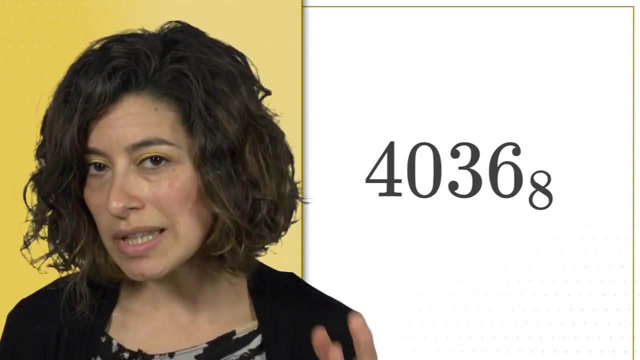 You can try the two methods and appreciate how much quicker and elegant the direct binary to octal method is. Let's start now with an octal number- 4036.. And let's transform it into binary using the idea of one octal digit. 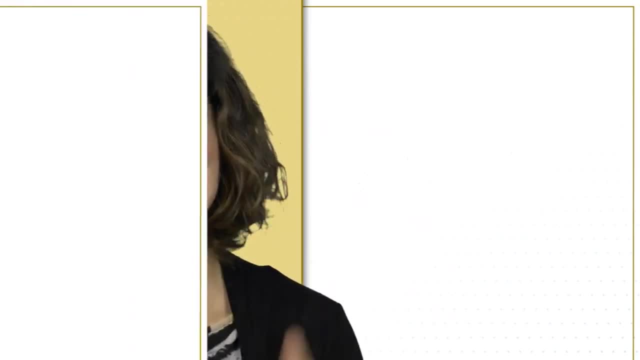 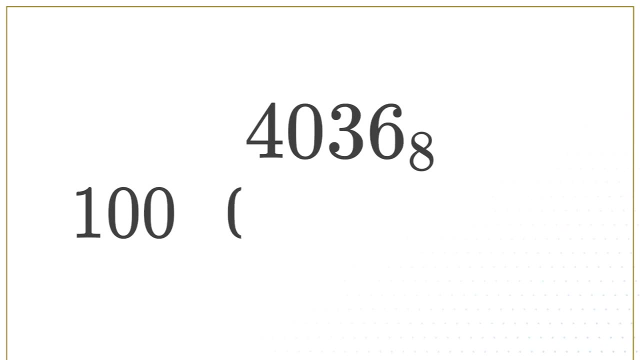 being a three-digit binary number. So 4 is 100,, 0 is 0, but we need to write it as 000 because we need to have three digits. 3 is 11,, so we do 011.. 6 is 110.. 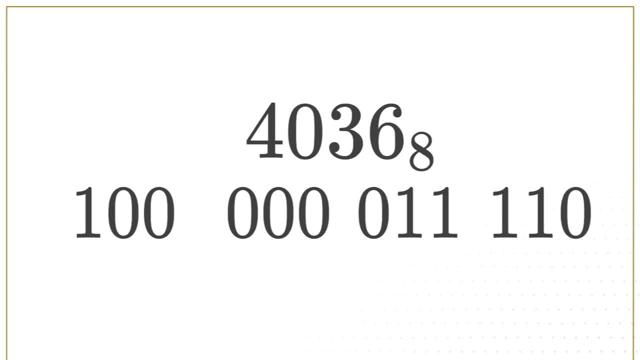 And now we write the binary strings in the same order: 100, 000, 011, 110, and we have that 4036 in octal is written in binary as 100, 000, 011, 110.. 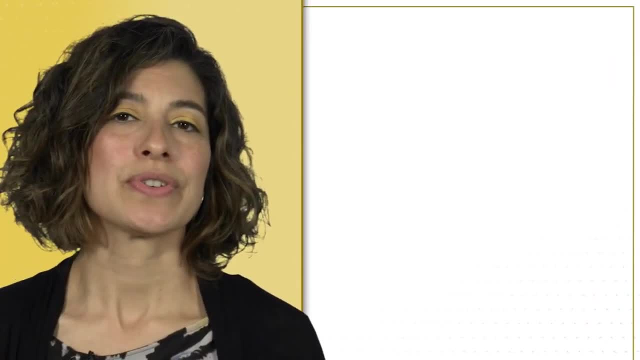 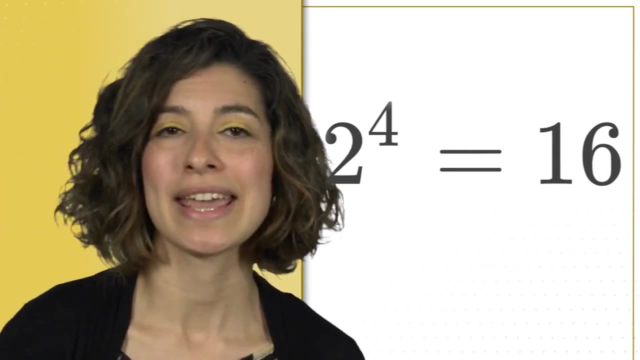 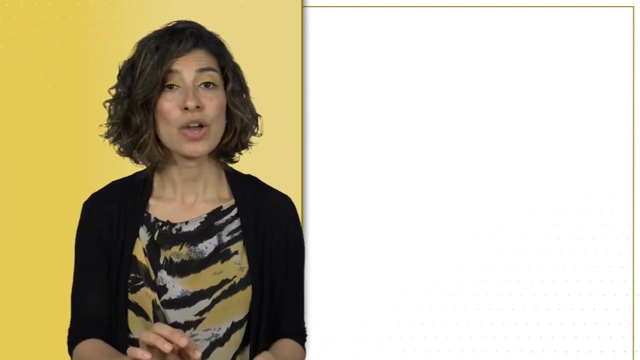 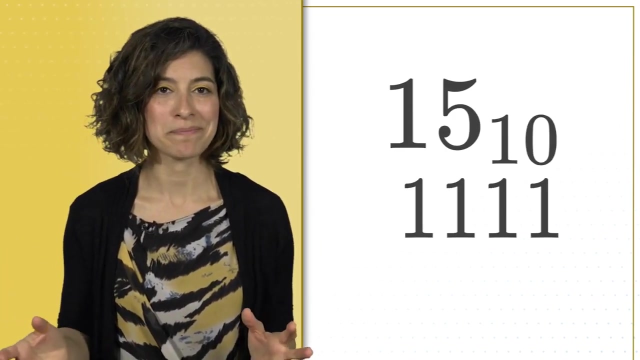 And we're done. The key thing to note is that 2 to the power of 4 is 16, and that means that one hexadecimal digit can be expressed using up to four-digit binary number. Note that 15 in decimal writes as 1111 in binary. 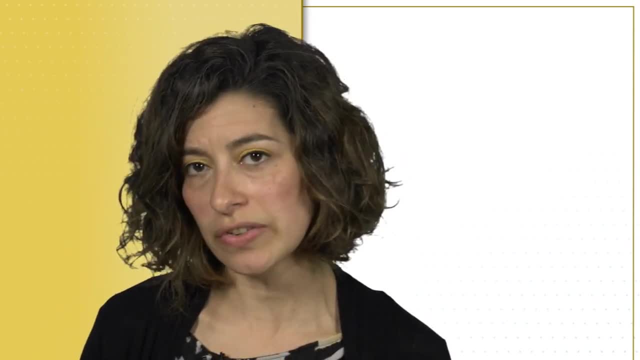 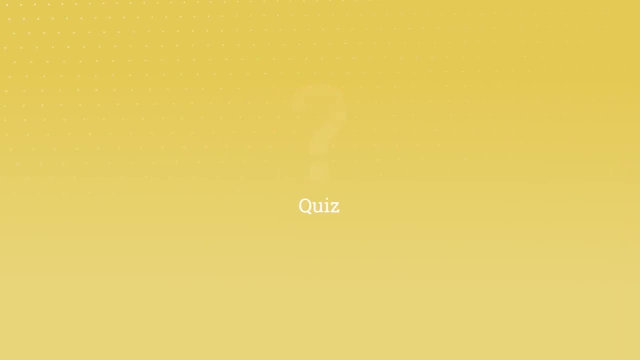 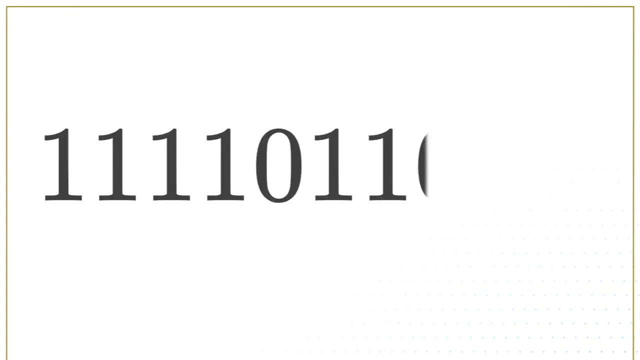 Take this moment to write the hexadecimal digits 0 to 9,, 8 to f, 8 to f as four-digit binary numbers. Let's write the number 1, 111, 011, 001.. That means we have 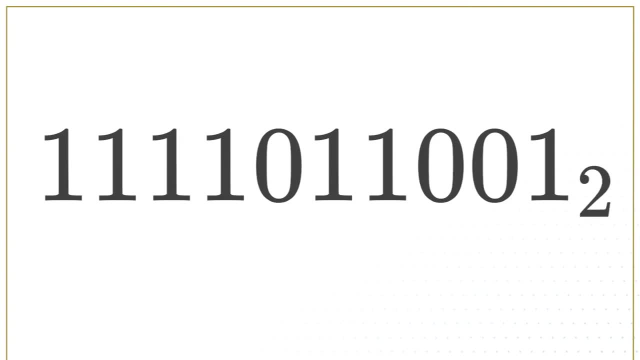 11, 1101, 1001.. And now we take each group of four binary digits as a number of its own right- We have 11, 1101,, then 1101,, then 1001, and write these individual numbers in decimal. 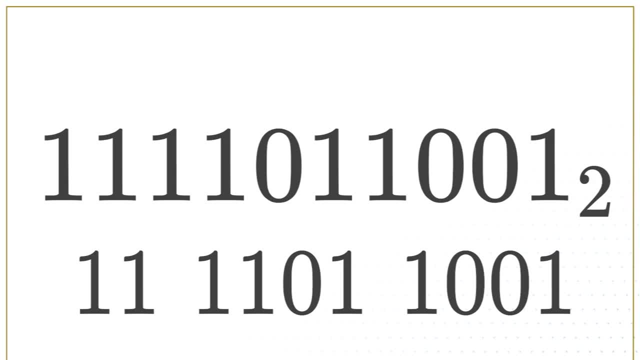 and then as one hexadecimal digit, And it is possible because they have at most four digits. So we get 3,, then d for 13,, then 9.. And these numbers are the digits in hexadecimal, given that 1,, 111,. 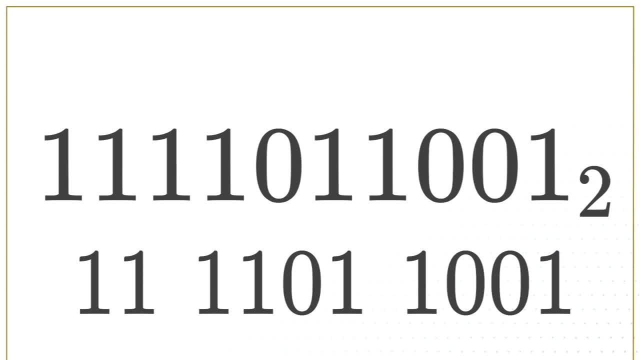 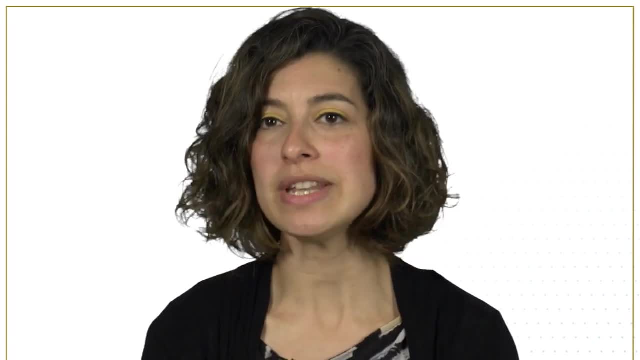 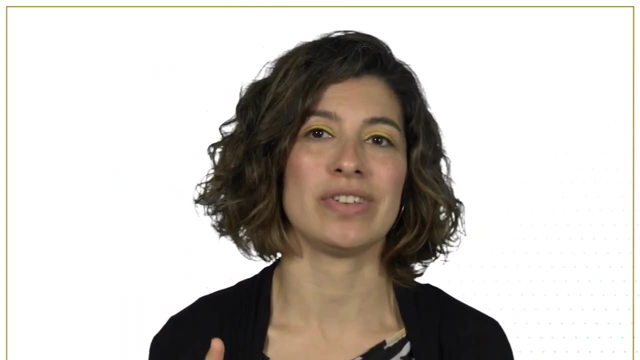 011, 001 in binary is written in hexadecimal as 3d9.. In short, we group the binary digits in fours and replace each group of four digits as one hexadecimal digit, which is the decimal conversion of the four-digit binary number. 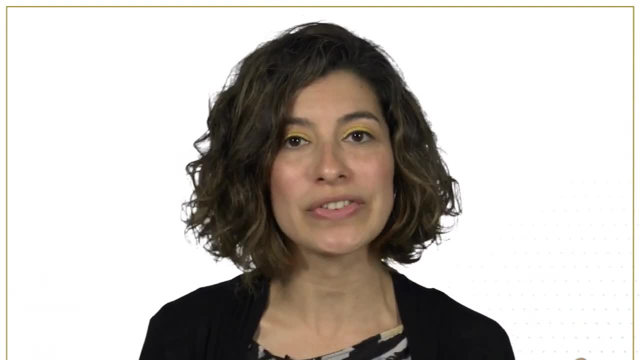 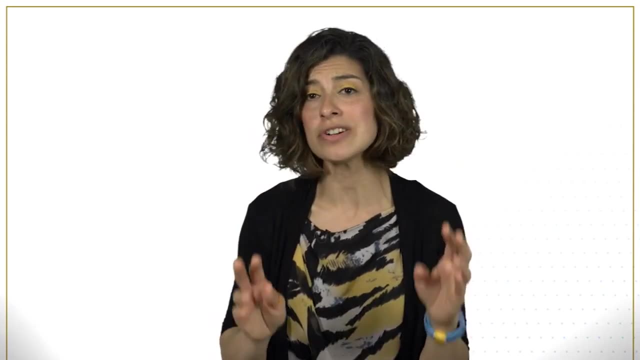 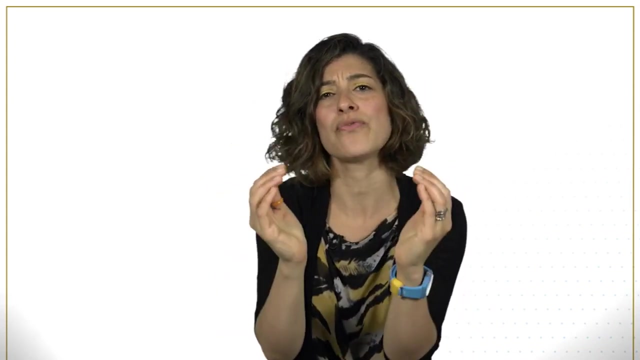 using the same conversion you used in the InVideo quiz earlier. Again, remember that the whole point of this section is to do a direct conversion without converting to decimal. But we use decimal only at the level of groups of four digits to do immediate hexadecimal. 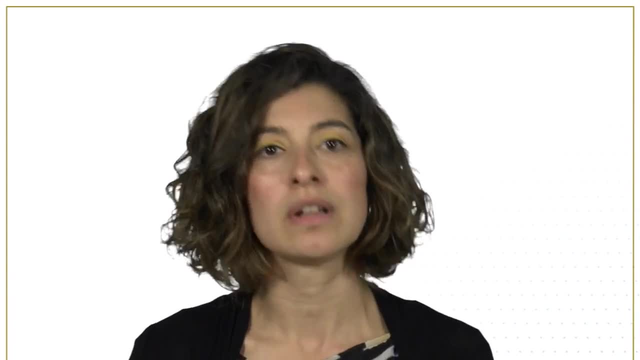 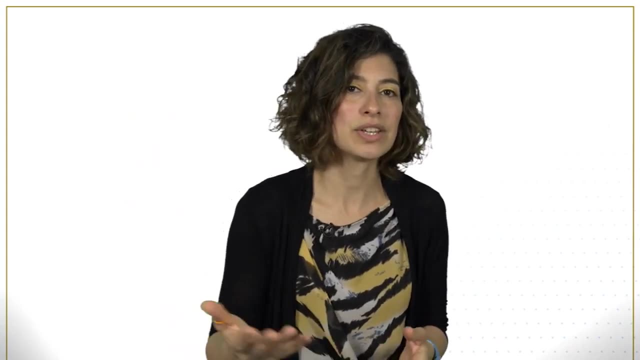 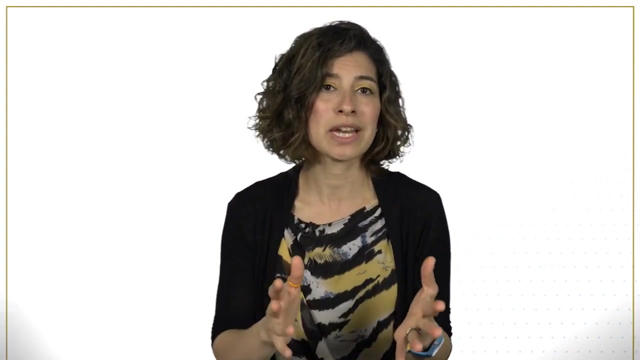 rather than converting the whole binary number to decimal and then the whole decimal number to hexadecimal. Like I said earlier, you can try the two methods and appreciate how much quicker and elegant it is to do the direct binary to hexadecimal conversion. Let's start now with a hexadecimal number. 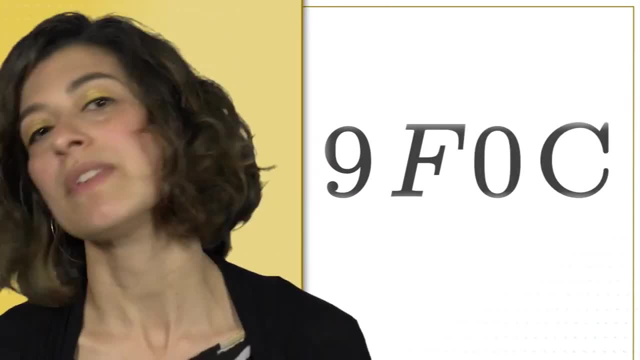 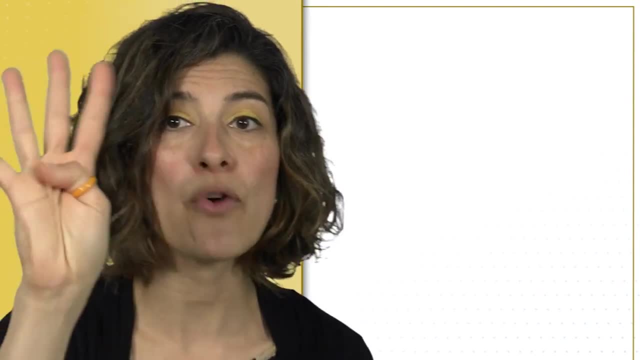 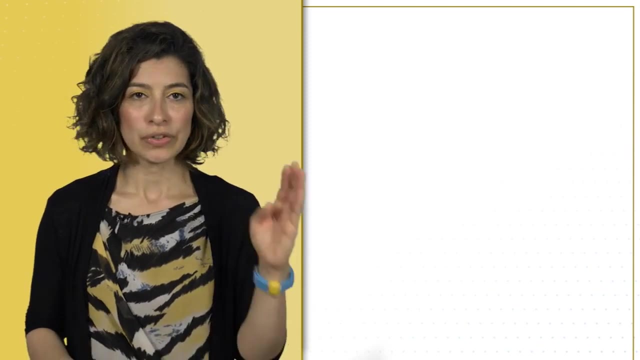 9F0C and let's transform it into binary using the idea of one hexadecimal digit being a four-digit binary number. So let's write each hexadecimal digit as a four-digit binary number. So 9 is 1001, F. 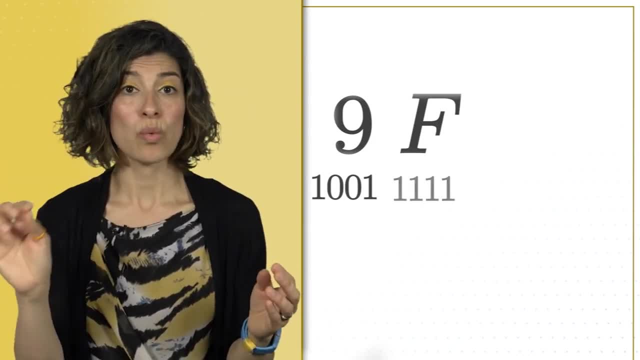 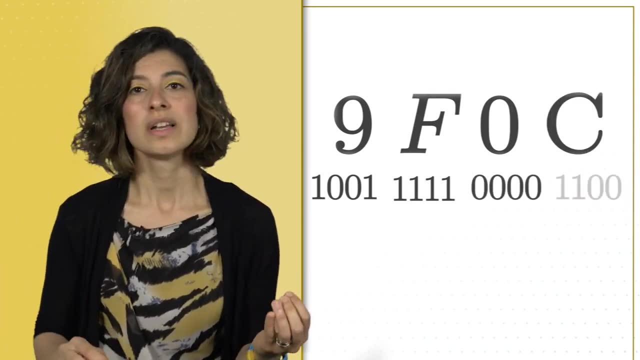 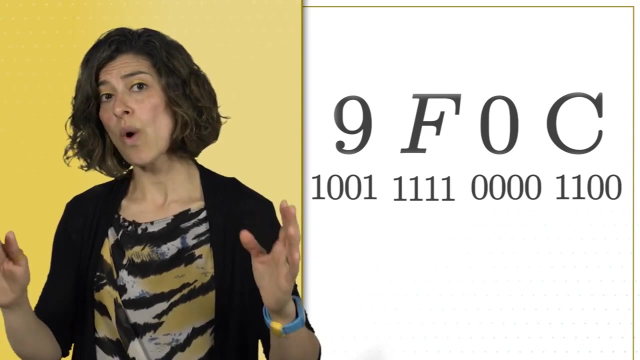 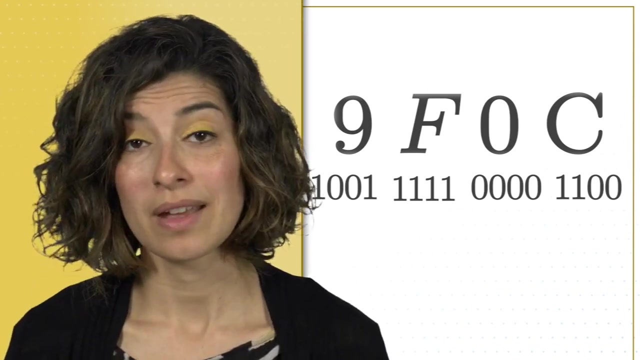 which is 15, is 1111,, 0 is 001,, for example, we write 0000, and C, which is 12, is 11001.. And now we write the binary strings in the same order, and so 1001,, 1111,, 0000,, 1101.. 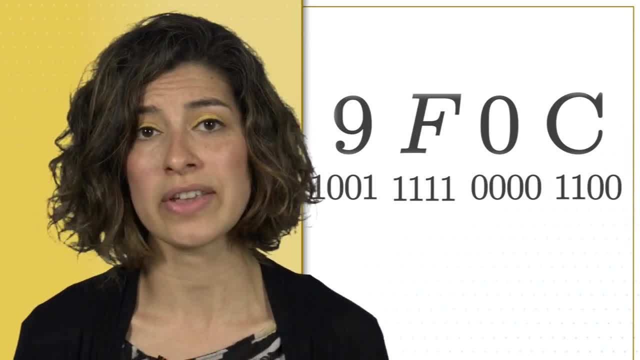 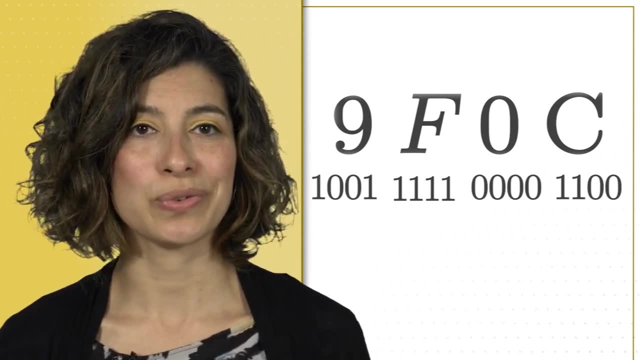 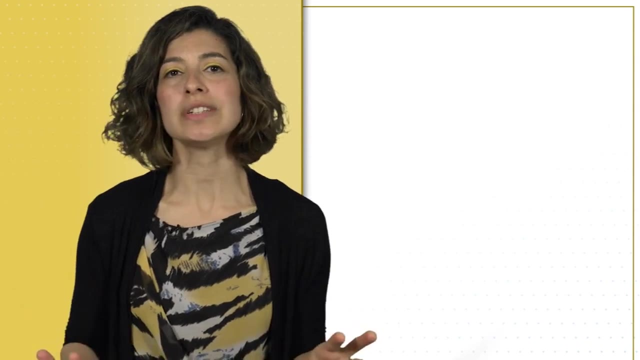 And we have that 9F0C. the hexadecimal number is written in binary as 1001, 1111, 0000, 1101.. And we're done To translate between octal and hexadecimal. we go via binary at digit level. 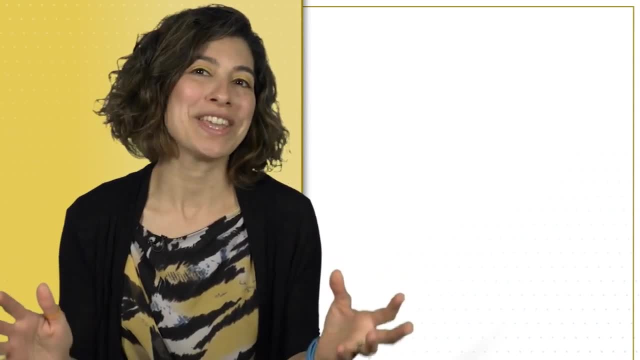 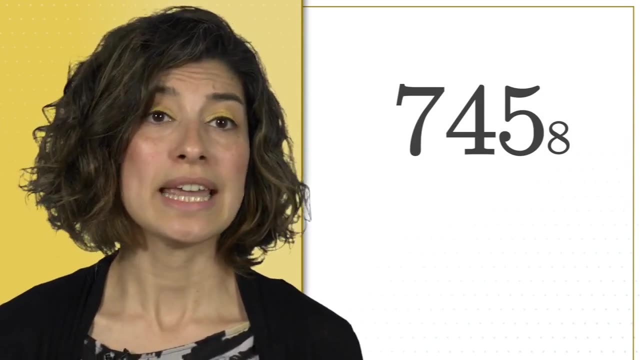 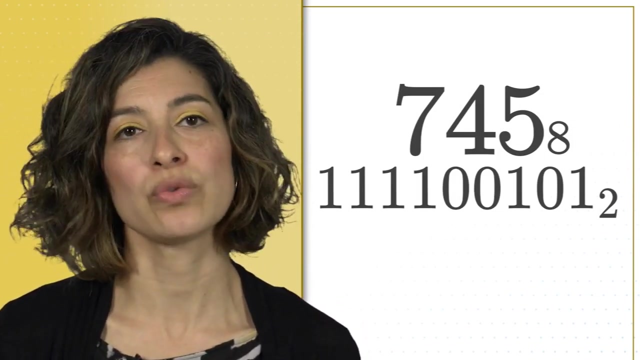 It is really only a regrouping of digits. We use the methods we have just covered. So 745 in octal is 111, 100, 101 in binary, because 7 is 111, 4 is 100,. 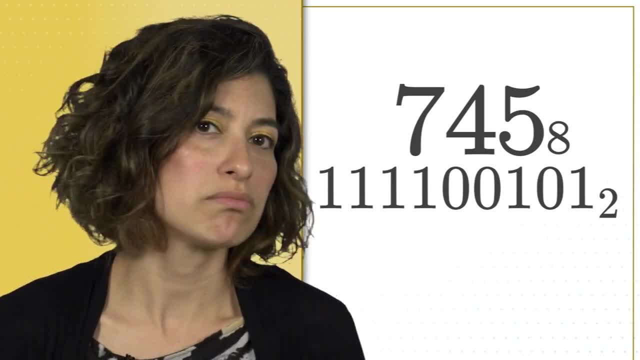 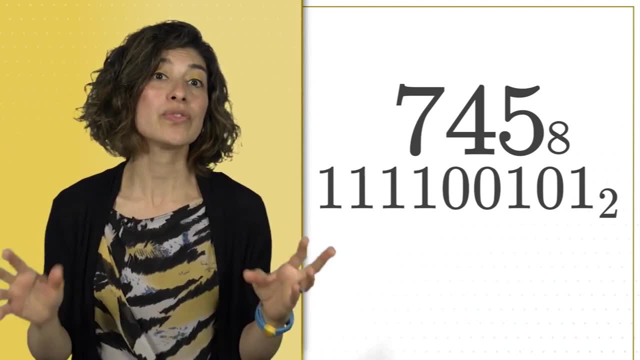 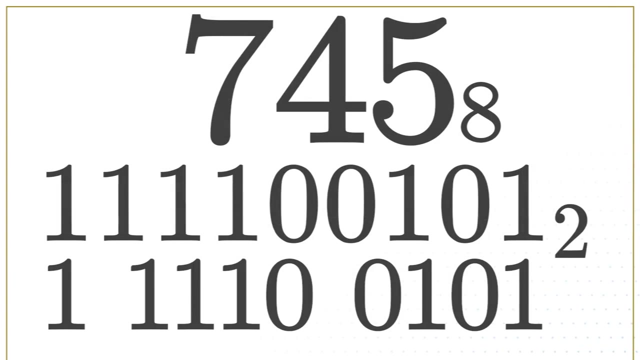 and 5 is 101.. So 111,, 100, 101.. And now we regroup all these binary digits as fours, giving 1, 1110, 0101 in binary. Remember we start with the smallest place value for the grouping. 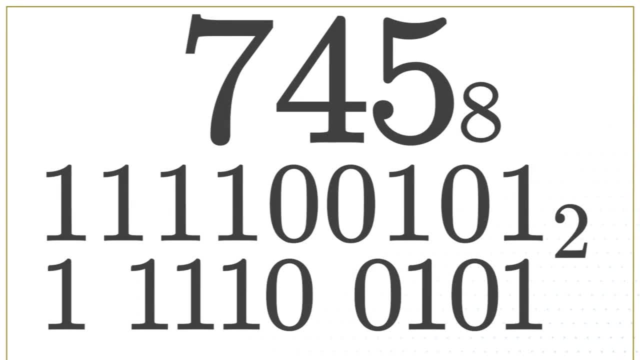 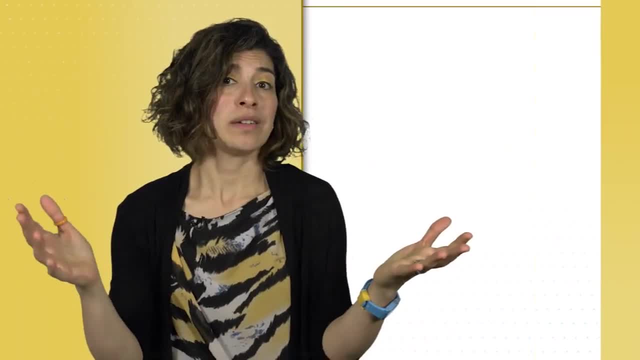 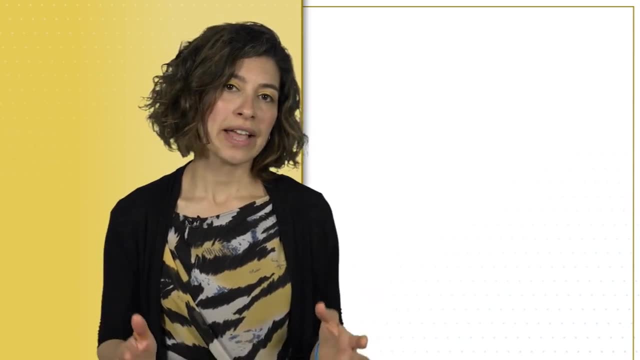 And get writing these groups of digits into a hex each. Now we know that 1 in hex is 1, 1110 in hex is E, 0101 in hex is 5.. And we write them one after the other and get. 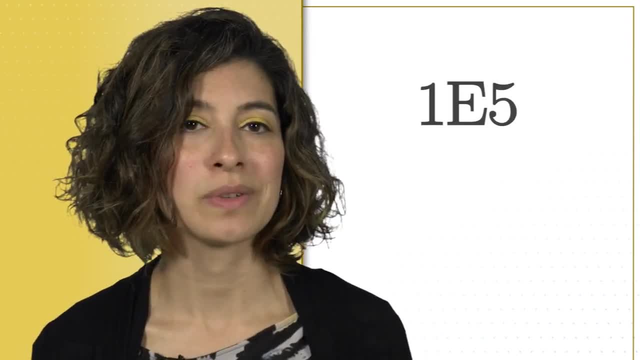 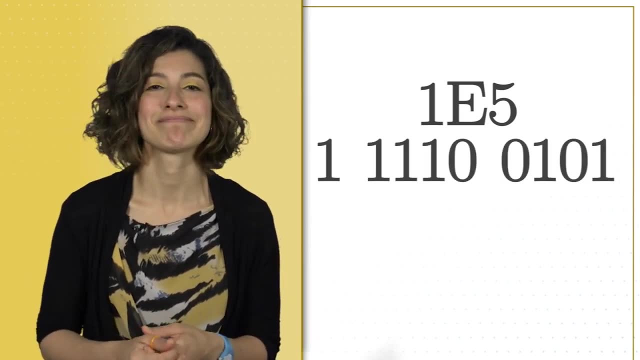 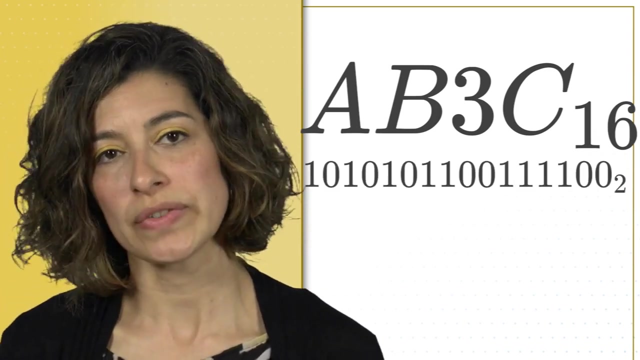 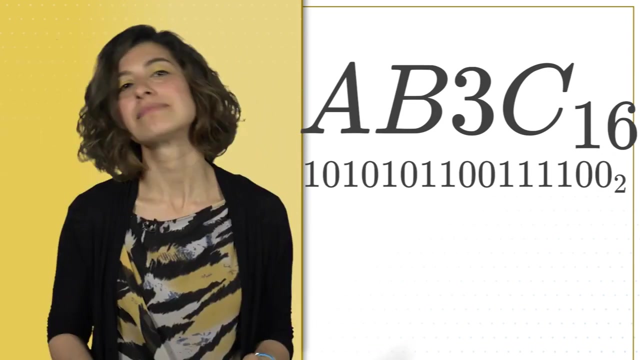 1E5 in hexadecimal, which equals 1, 1110, 0101 in binary. Easy peasy. AB3C is 1010, 1011, 0011, 1100 in binary, Because A is 1010,. 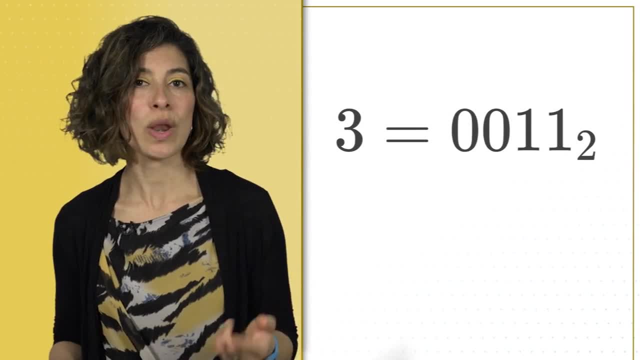 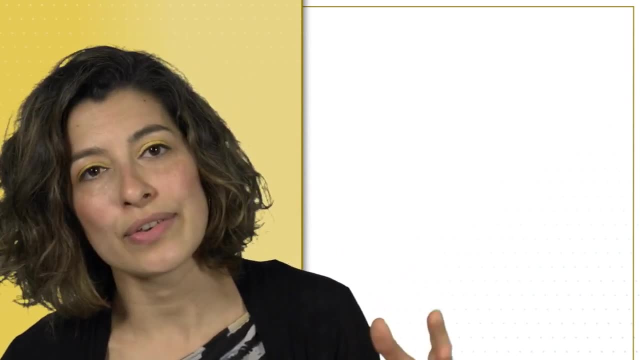 B is 1011,, 3 is 0011, and C is 1100.. And yes, we need the leading zeros, making 3 as 0011, and not just 11, because we need to stick to the length of 4.. 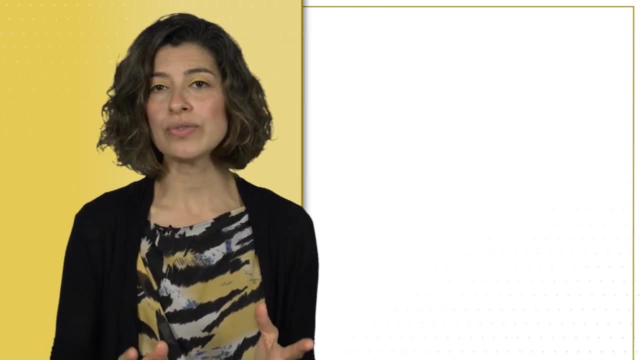 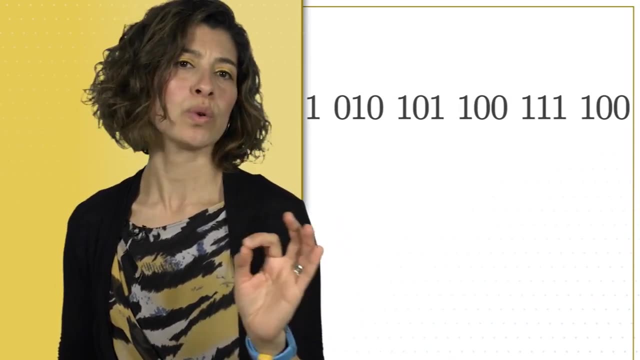 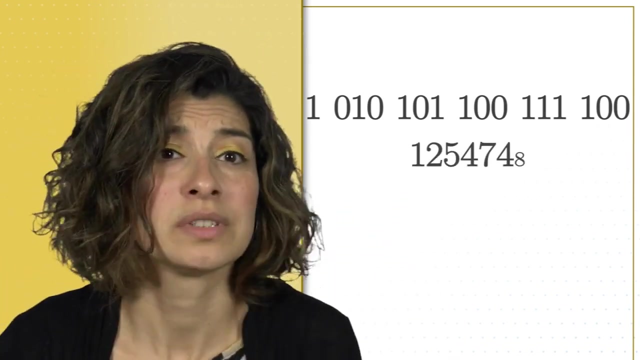 So now we regroup these digits in trios And we have 1, 010, 101,, 100,, 111, and 100.. And we write these guys in decimal, which is octal, And we get 125474 in octal. 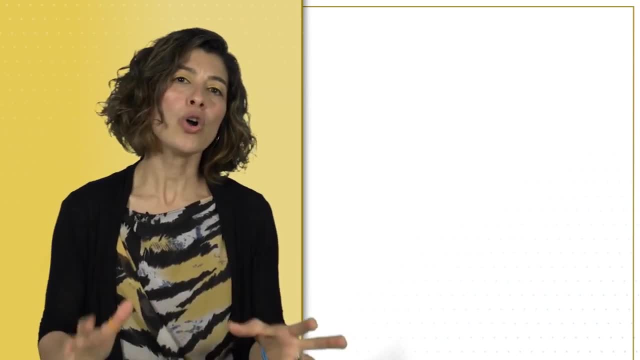 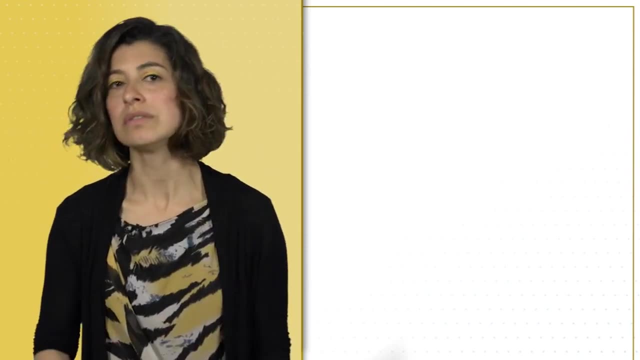 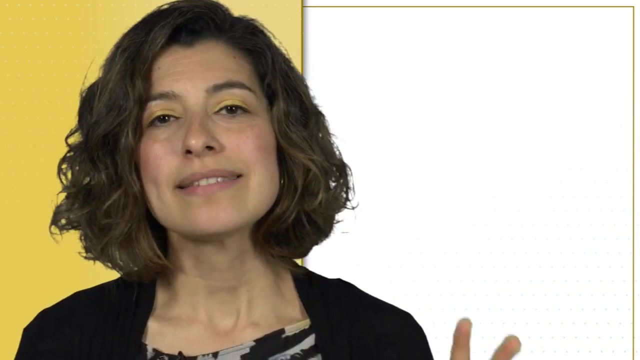 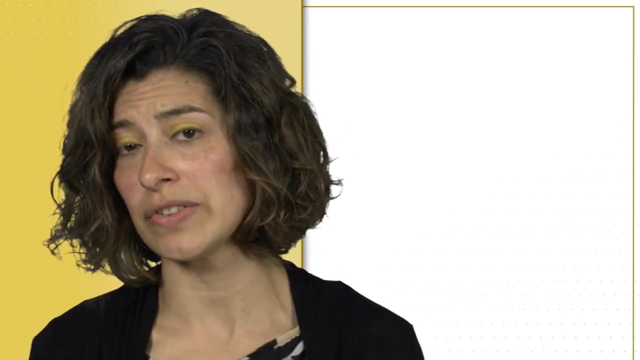 And we're done. The whole idea is 1 octal 3 bits, 1 hexadecimal 4 bits, And I'm using bits as binary places. The same algorithm applies to fractional numbers, but we have to think carefully of how to group the digits. 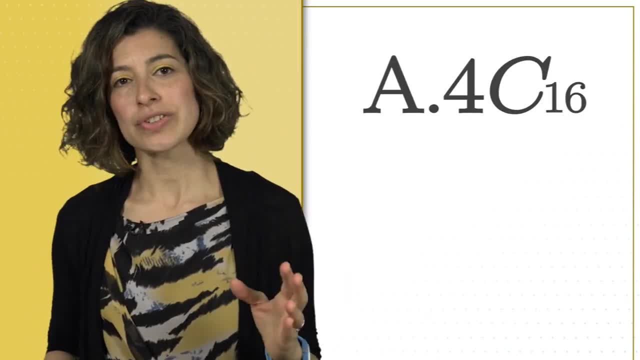 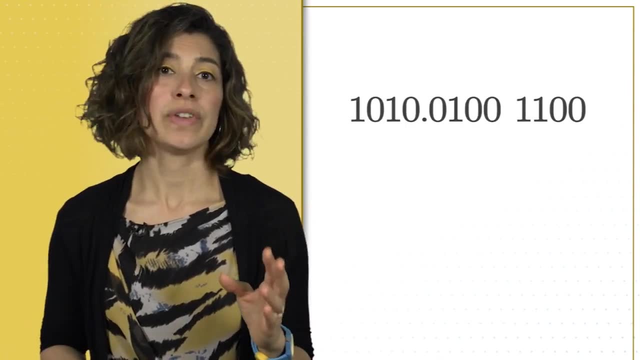 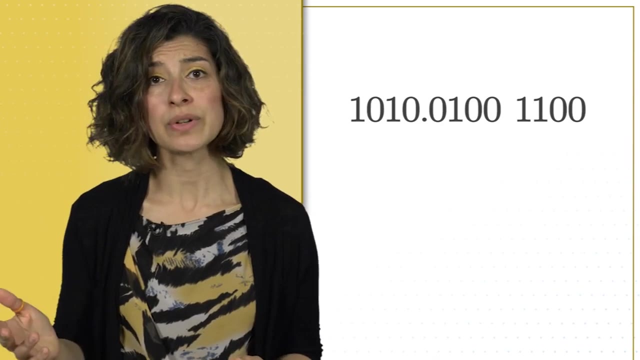 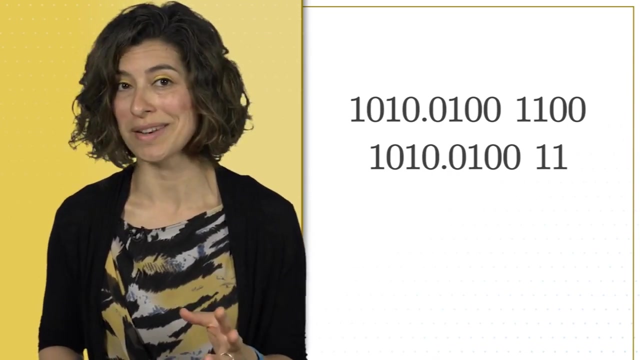 Let's look at some examples. A dot 4C in hexadecimal. Let's convert it to binary: 1010 dot 01001100.. We're going to tidy up the zeros at the end: 1010 dot 010011.. 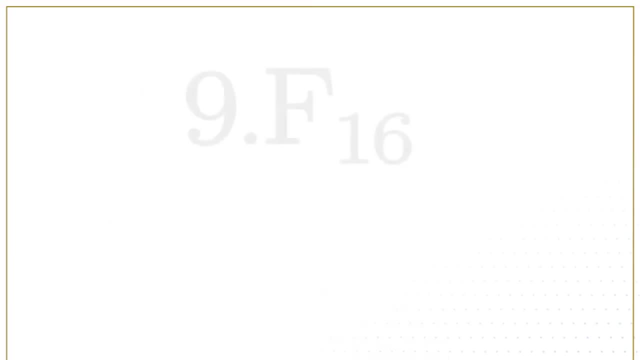 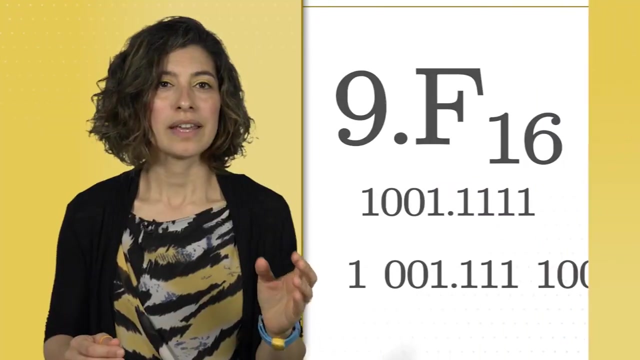 Let's do another one: 9 dot F. Let's convert this hexadecimal into octal: It's 1001 dot 1111.. Then 1001 dot 111100.. And notice how the grouping was done here, Giving 11 dot 74 in octal. 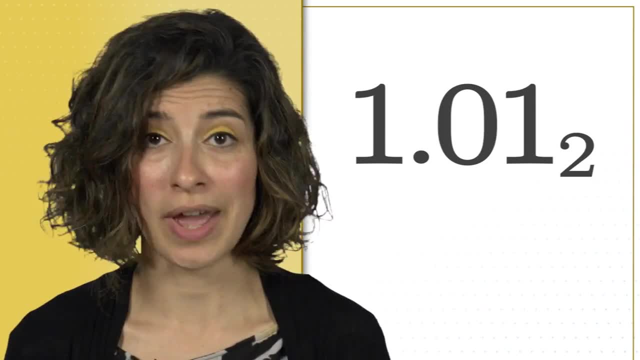 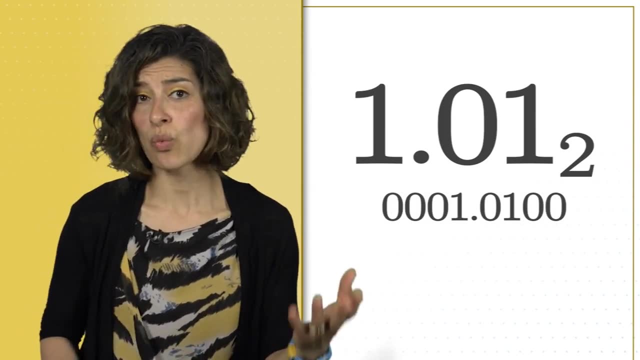 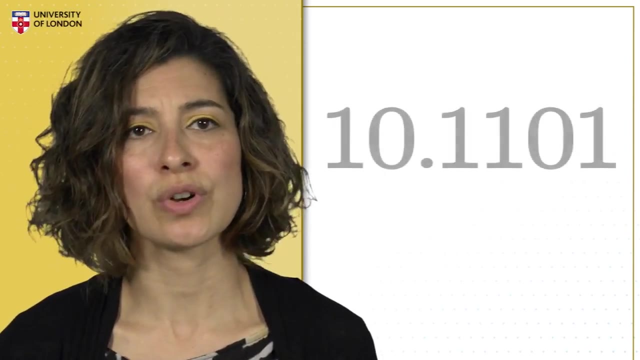 Let's do the binary 1 dot 01 into hexadecimal. We write 0001 dot 0100.. And that is 1 dot 4 in hexadecimal. Let's do 10 dot 1101, a binary number into octal. 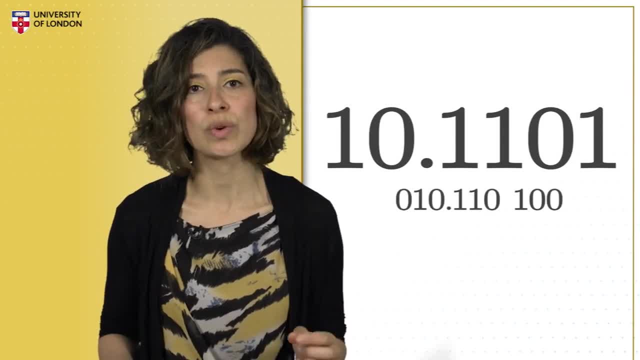 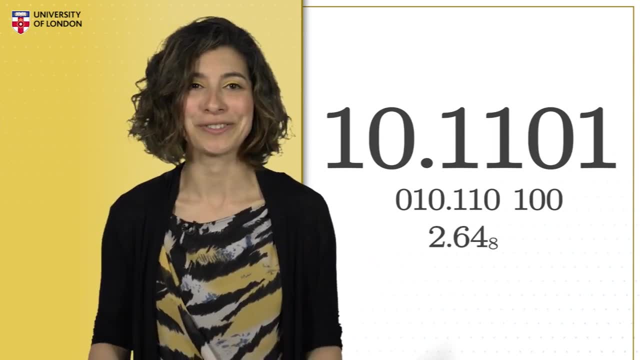 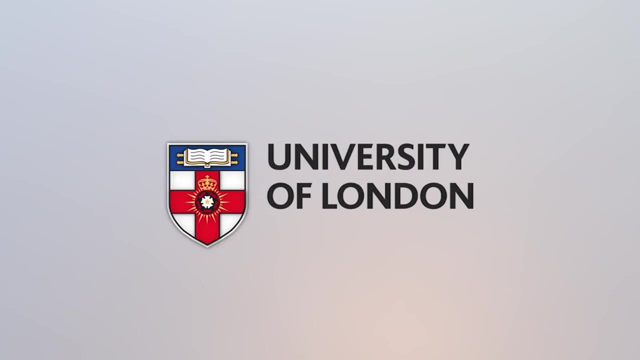 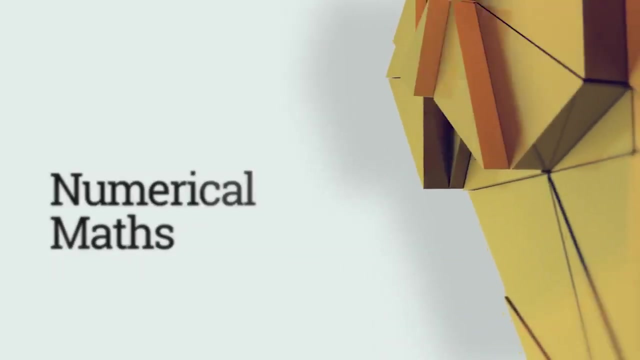 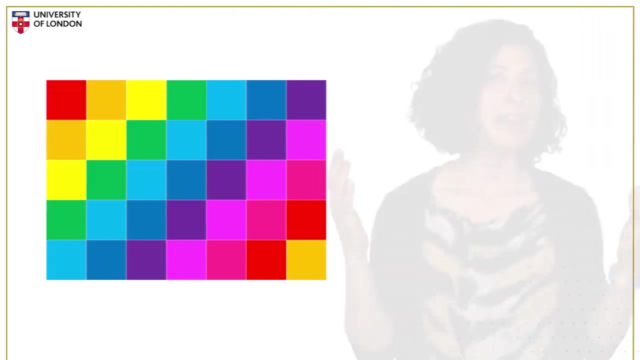 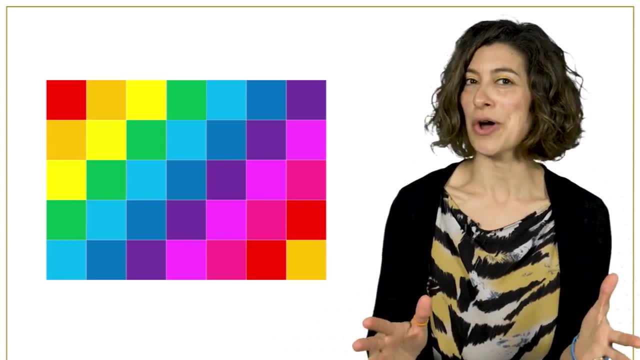 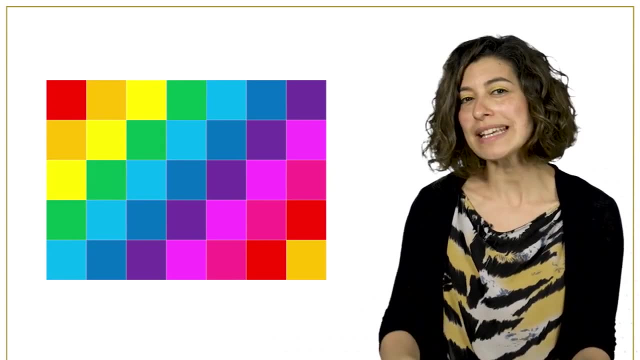 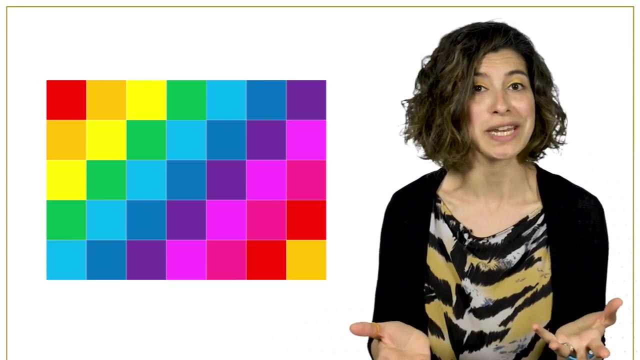 Can you see? Probably not. I'm not talking about a deeper artistic meaning or a metaphor. I'm talking about concealing a message within the information that makes this picture render on your screen. Everything is number, And this image is made of numbers. 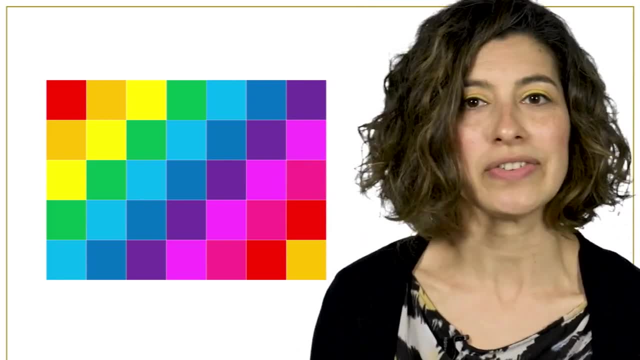 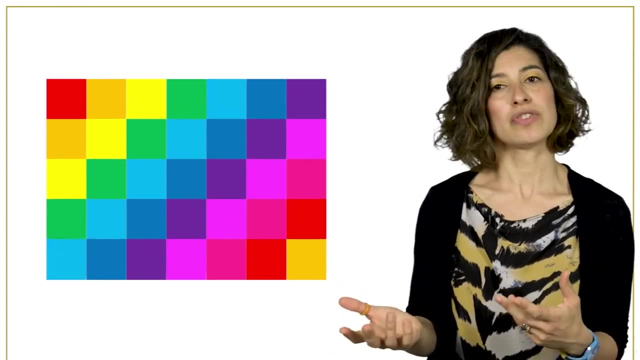 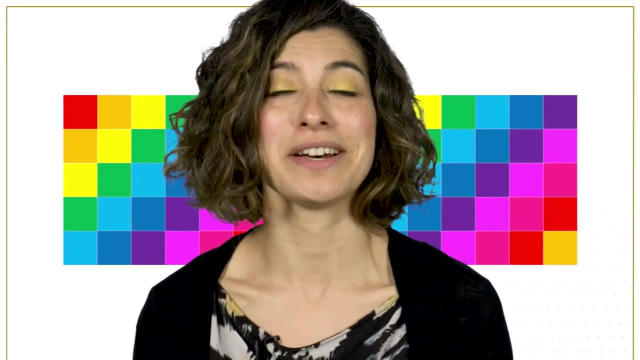 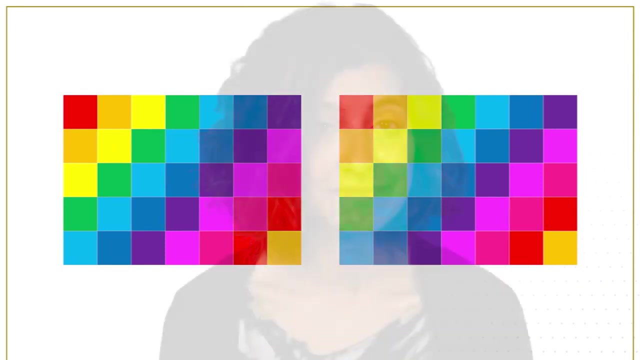 that describe each pixel. The process consists of using the pixel information to conceal a message. This is the image before the message was concealed, And now let's look at both of them side by side. Can you now tell what the message is? No, 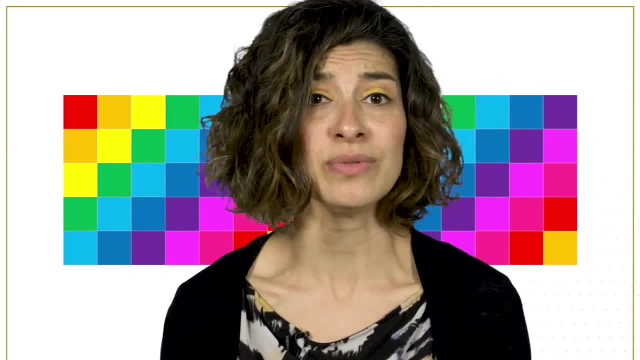 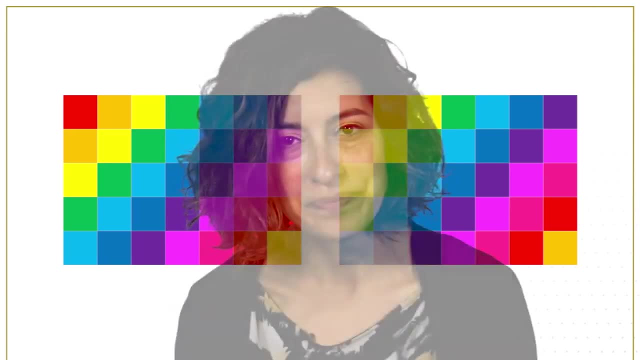 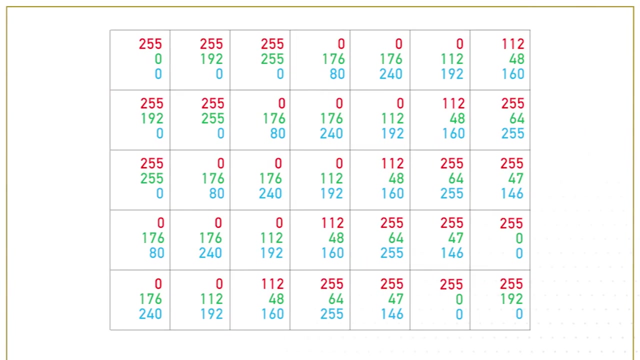 Do you suspect something is hidden in it? I don't. The main idea is to use the color codes to hide the message, And these are the RGB codes of the original image. On each row we got a red, green and blue color value. 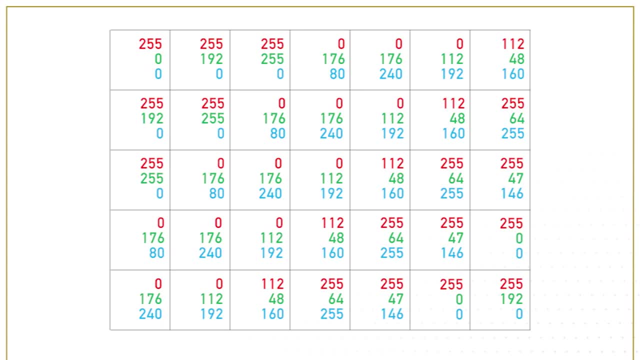 And we go along all the columns and we complete the row, Then we go to the next row, and so on. So we've got on the first row, we've got 25500.. That's one pixel. 255920.. That's another pixel on that row. 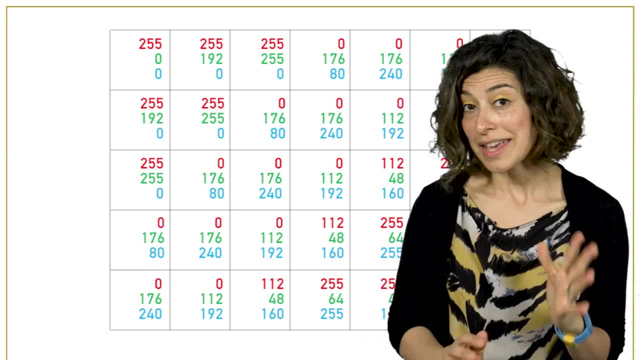 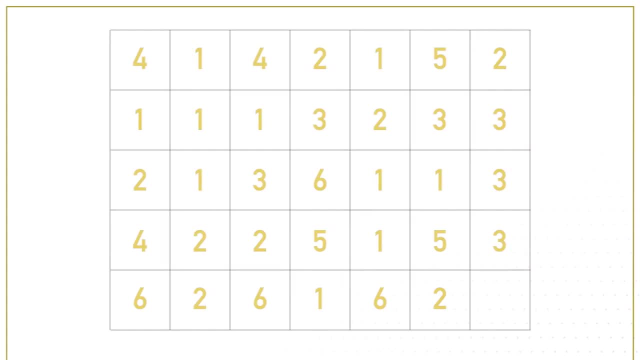 And so on, and so on, and so on. Here is the secret message. I haven't told you how the message was created. I'll go into that later. The idea is to fit the numbers of the message in each pixel. So we group the numbers in the message. 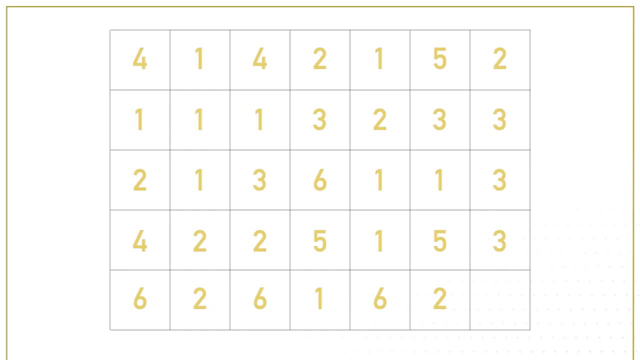 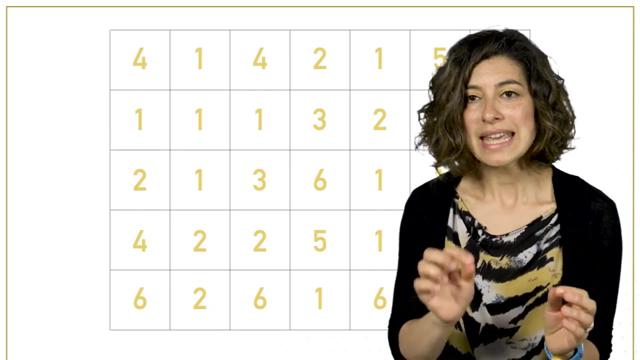 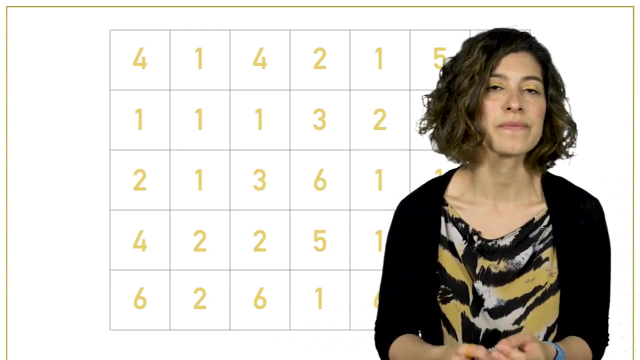 in rows with seven numbers on each row. as we have seven pixels in each row Like this- And here is the clever bit- Each pixel has three numbers: for red, green and blue colors. For RGB colors, The numbers in the secret message. 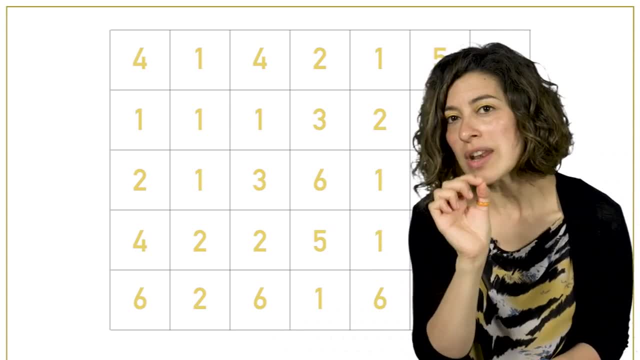 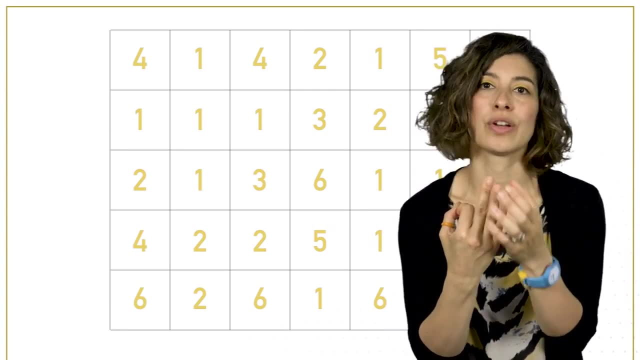 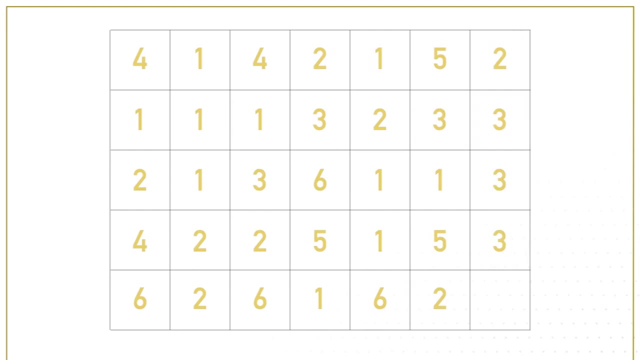 go up to six, So we can write each number in binary using three digits, And then we hide each binary digit in one color code: Red, green, blue. I'll show you how We write the first message number into a three-digit binary number. 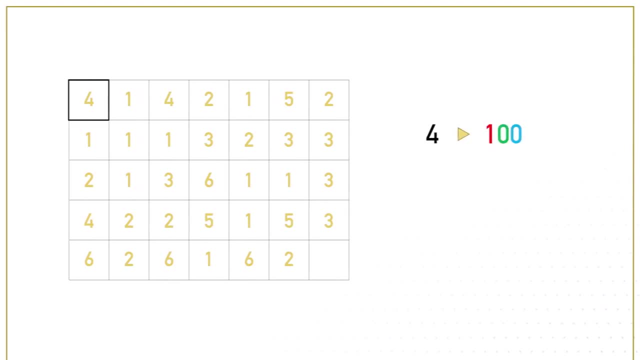 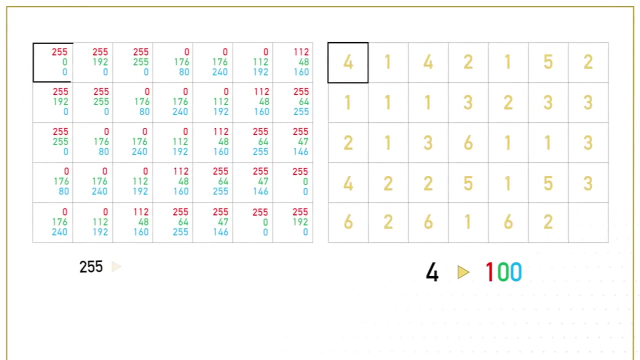 So four is 100.. And we hide the digit one in the red value of the pixel, the second digit zero in the green value of the pixel, the third digit zero in the blue of the pixel. 255 is an eight-digit binary. 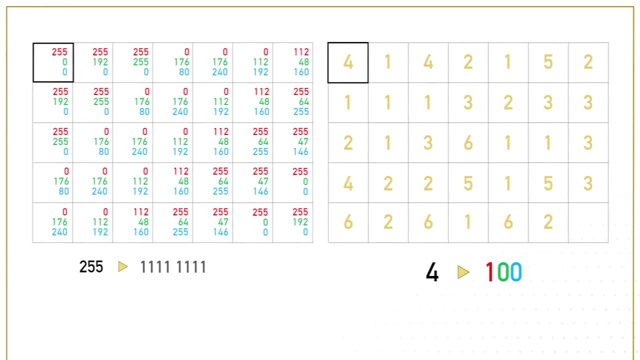 It's 1111, 1111.. And we replace the rightmost digit by the one giving the same number: 1111, 1111.. It's the same number. in this instance, Zero is an eight-digit binary: 0000, 0000.. 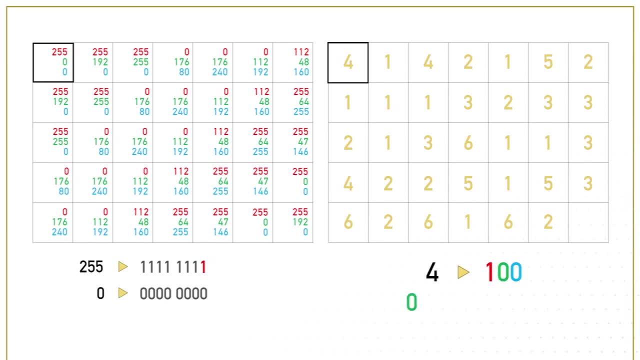 And we replace the rightmost digit by the zero of the message giving 0000, 0000.. So far they all look the same. With the other zero, still an eight-digit binary with eight zeros, And we replace the rightmost digit. 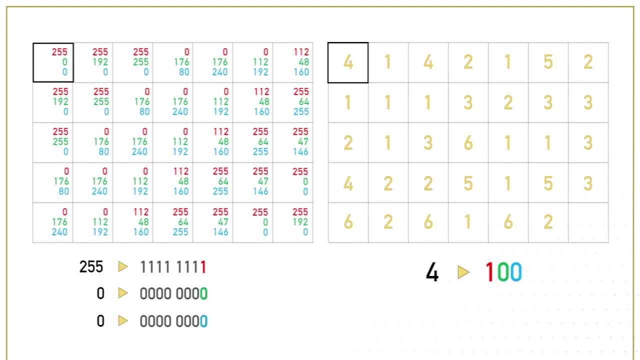 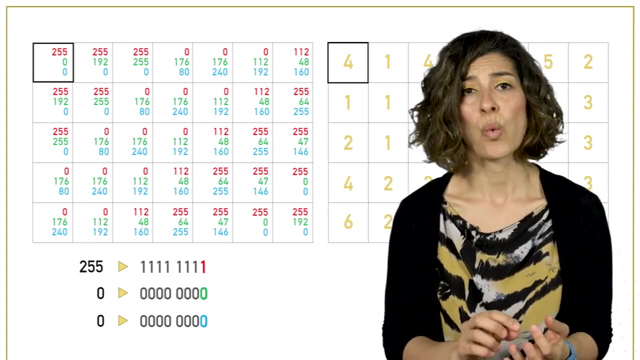 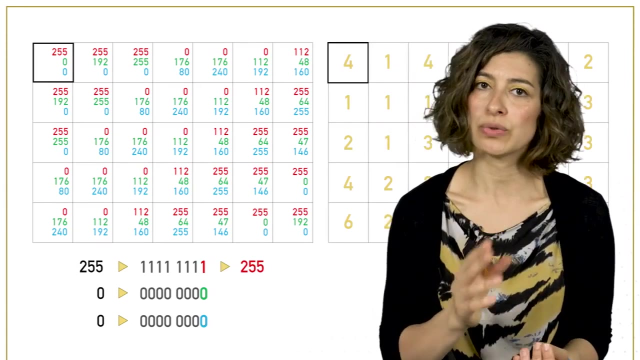 by the zero, giving another array of eight zeros. That means that the first pixel has codes for red: 1111, 1111,, which is 255.. Green will be 0000, 0000.. Which is value of zero. 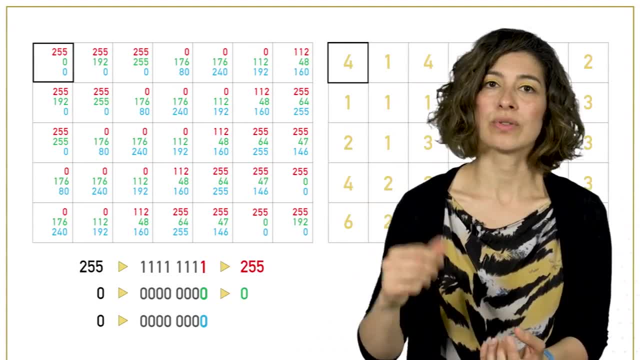 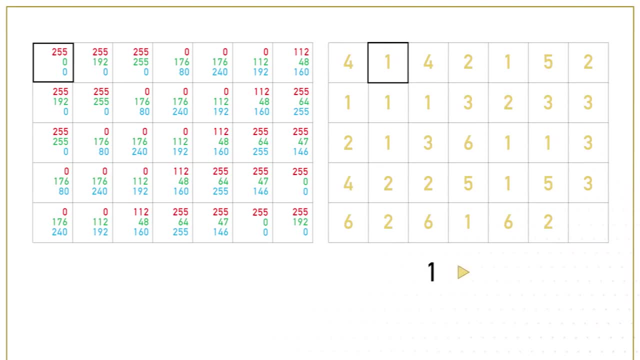 And blue: 0000, 0000.. Which is zero. For the second number from the message one, we write it as 001. in binary, We use the first digit, zero. for the red value of the pixel, The second digit, which is zero. 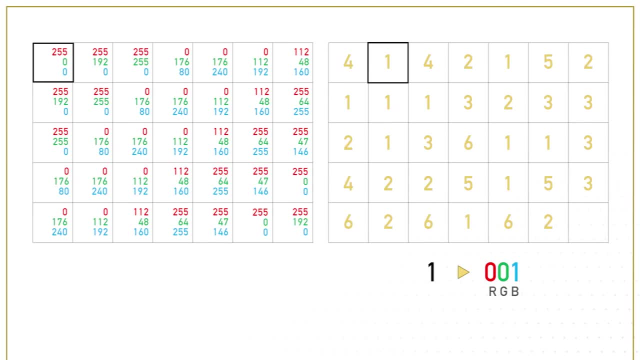 in the green value of the pixel. The third digit one in the blue value of the pixel, So 255 is the eight-digit binary: 1111, 1111.. We replace the rightmost digit by the zero, giving 1111, 1110.. 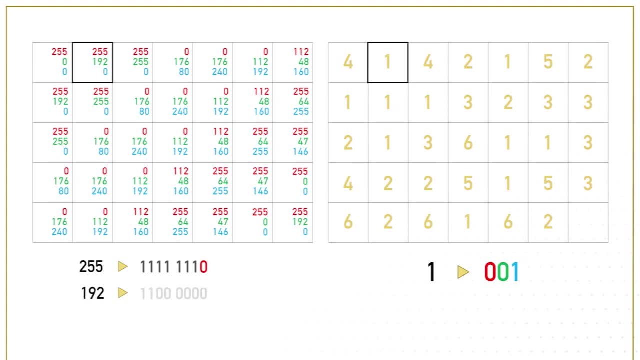 192 in binary is 1100, 0000.. Eight digits And we replace the rightmost digit by the zero, giving 1100, 0000.. Zero in binary will be eight zeros And we replace the rightmost digit by the one. 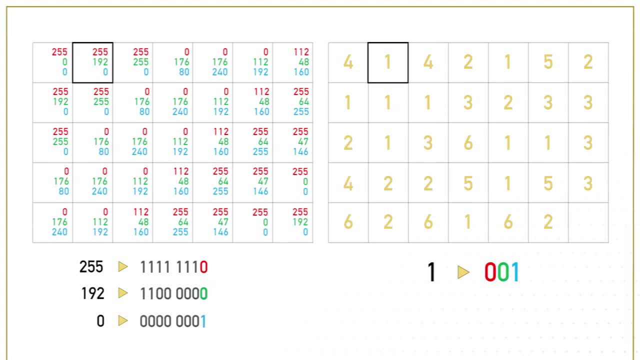 giving 0000, 0001.. So the second pixel becomes a pixel with color codes red, 1111, 1110, which is 254.. Green, 1100, 0000,, which is 192.. And blue, 0000, 0001,. 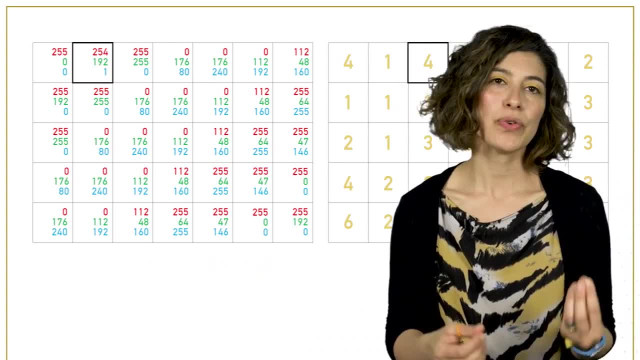 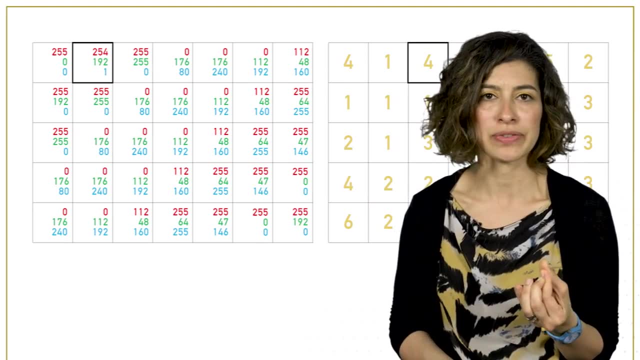 which is one. The third number from the message is four, which is 100.. And we're going to use the first digit, one in the red value of the pixel. The second digit, zero, in the green value of the pixel. 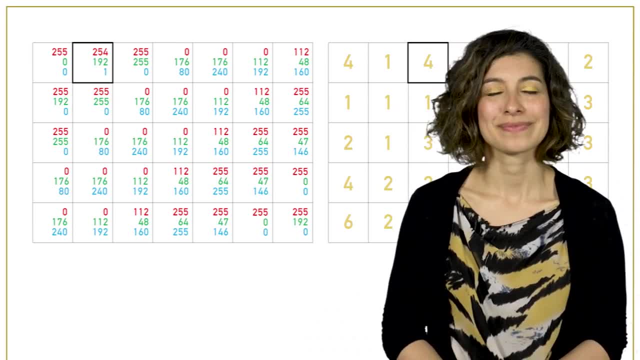 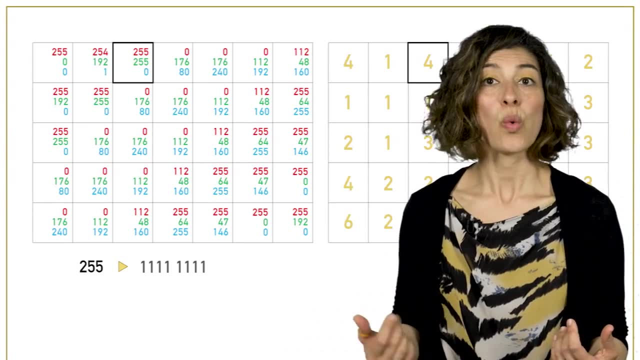 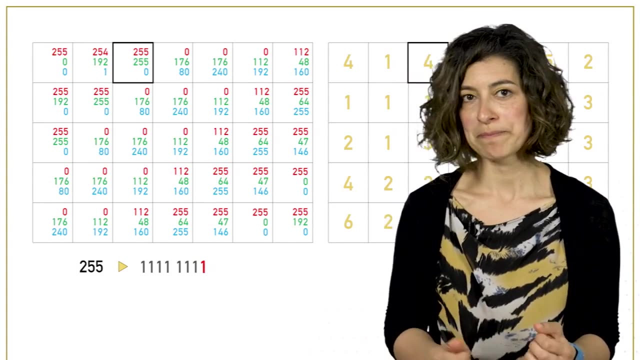 And the third digit, zero in the blue value of the pixel, And again 255, is the eight-digit binary: 1111, 1111.. And we replace the rightmost digit by the one giving 1111, 1111.. 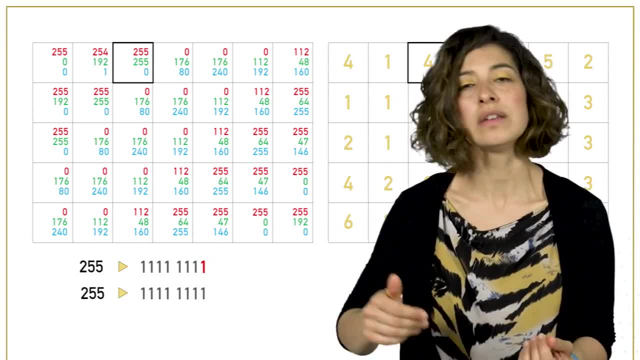 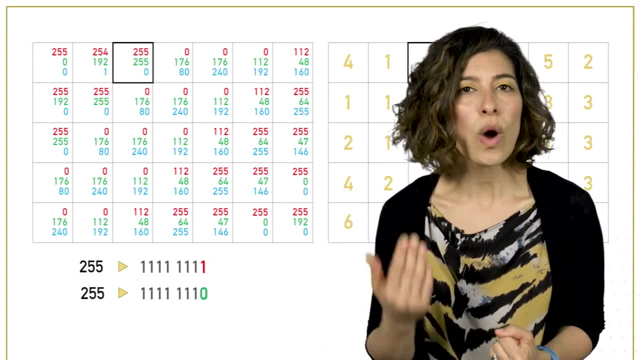 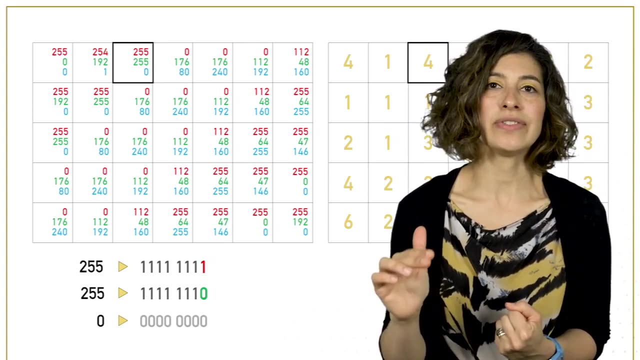 For green, 255 is 1111, 1111.. And we replace the rightmost digit by the zero, giving 1111, 1110.. For blue, zero is the eight-digit binary: 0000.. 0000.. 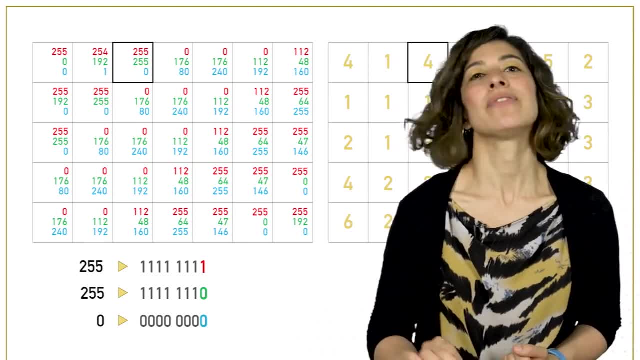 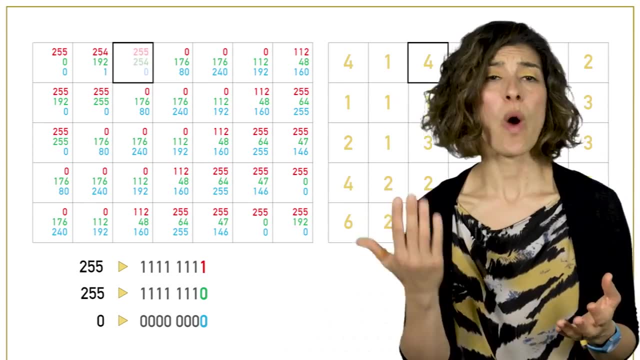 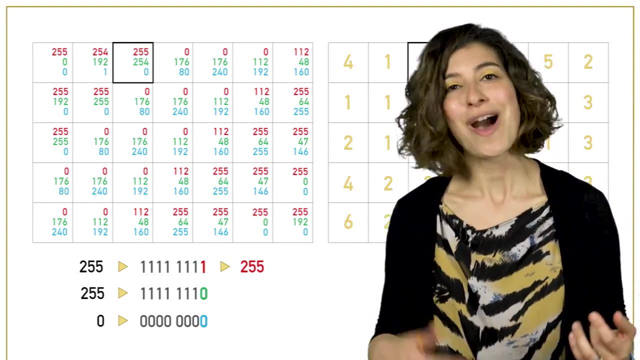 And we replace the rightmost digit by the zero, giving 0000, 0000.. So the third pixel becomes red- 1111, 1111,, which is 255.. Green- 1111, 1110,, which is 254.. 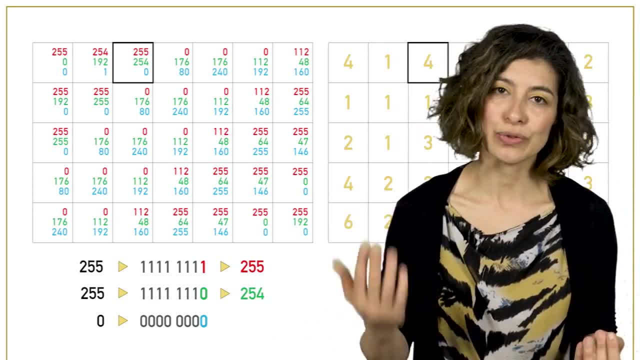 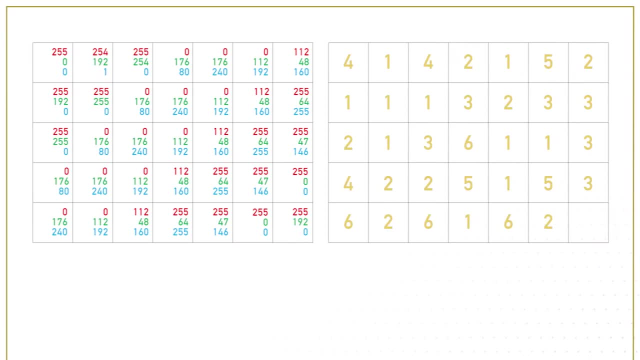 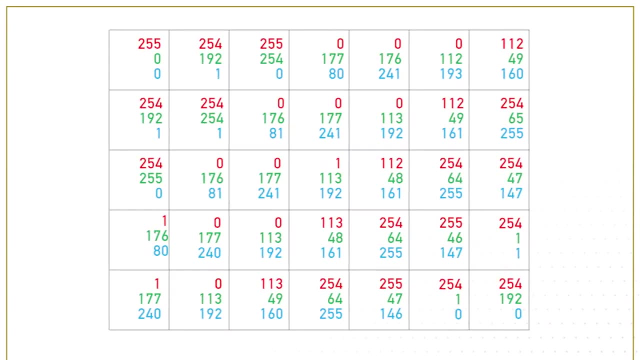 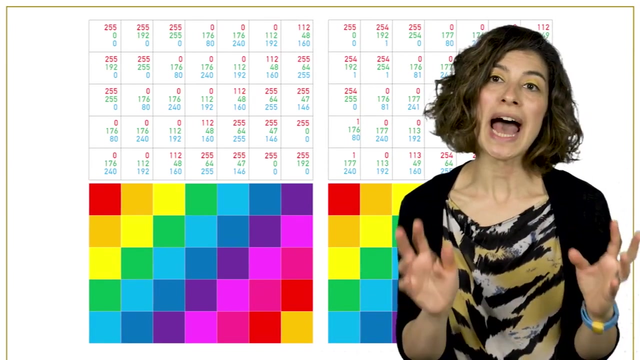 And blue 0000,, 0000,, which is zero, And so on. The final image with the message hiding it has the pixel information as follows And looks pretty much like the original. Now to recover the message, we undo the process. 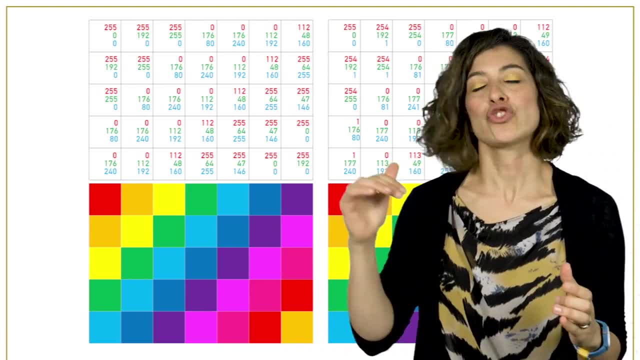 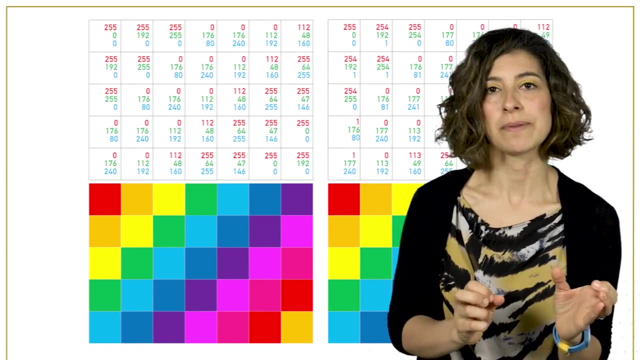 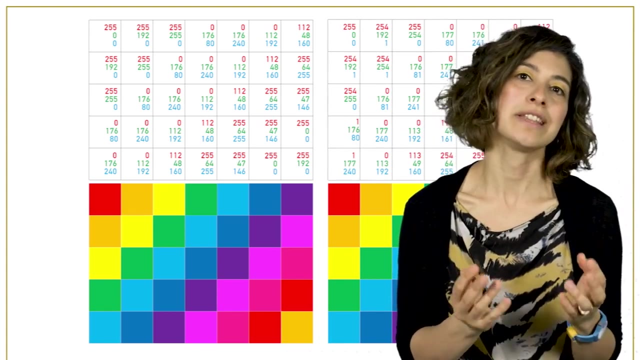 We write the caller codes in binary, extract the rightmost digit and use three consecutive digits to write a number in binary. Then translate this number in binary to decimal. We will have recovered the message intact And it will be this one, just like we started. 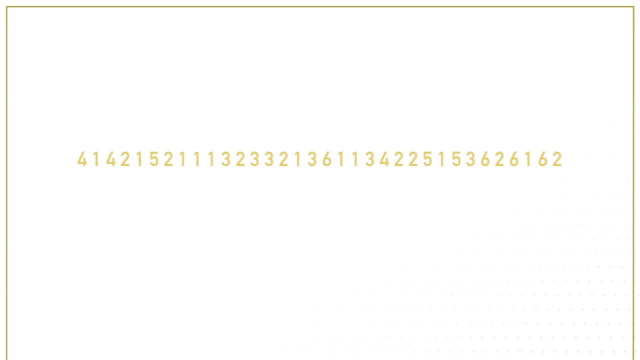 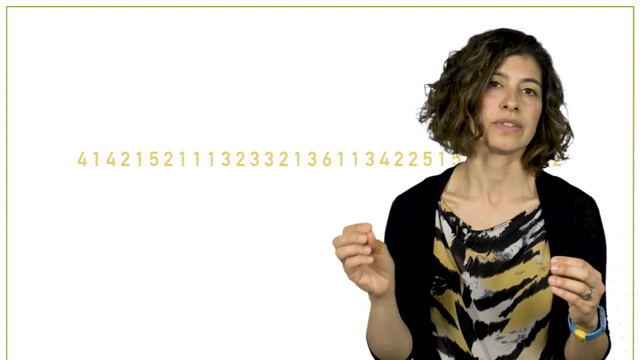 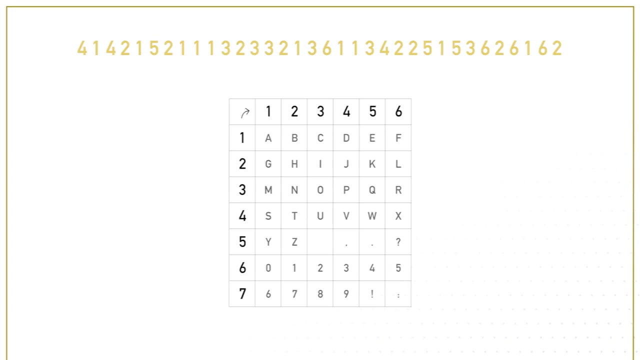 You can try it yourself. The secret message was created by mapping the characters and the numbers. I used this table And then we group the numbers in the message in pairs so we can recover the characters and read the message below. The same concept can be used. 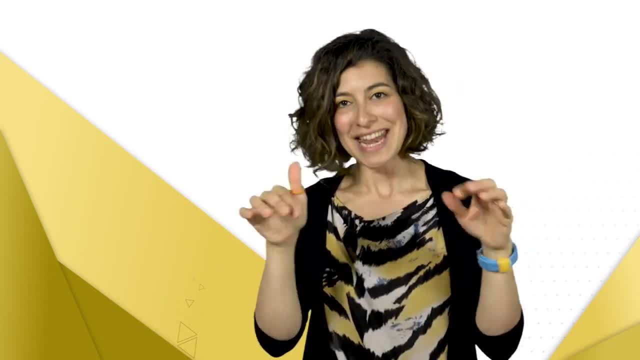 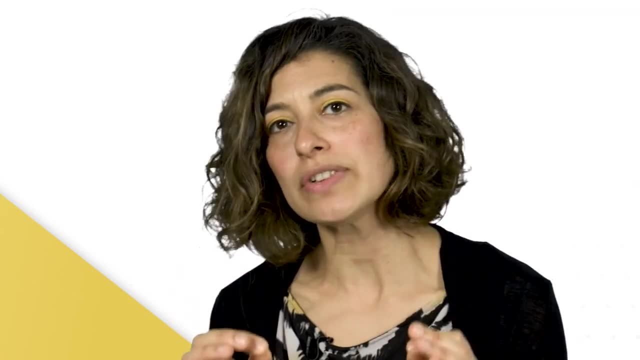 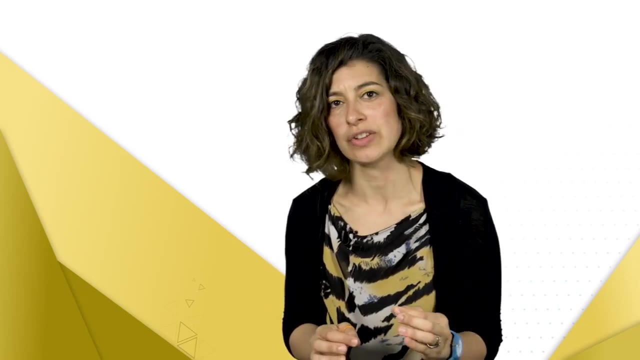 to hide an image inside an image. We're not going to use a table of letters This time. we're going to hide a pixel caller code inside a pixel caller code. In the example we just saw, we used the unit digits of the binary number for each caller. 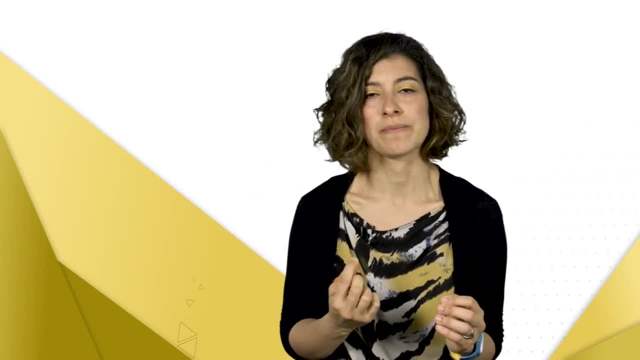 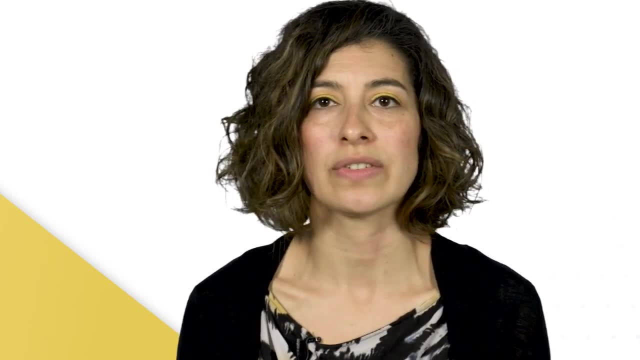 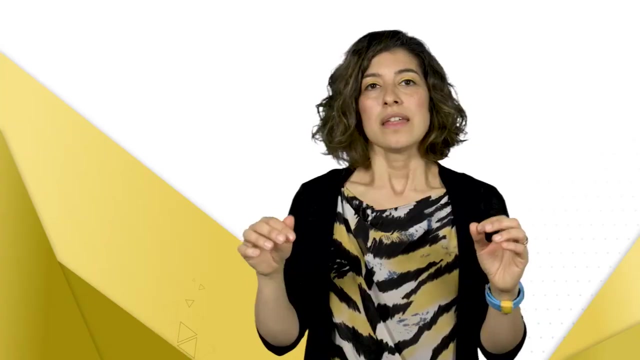 to hide one binary digit of the hidden message. Now, in this new process, we will use the least significant binary digits of the caller to hide the caller code for the hidden image. Let's see how many we need to use. This will be the process you will follow. 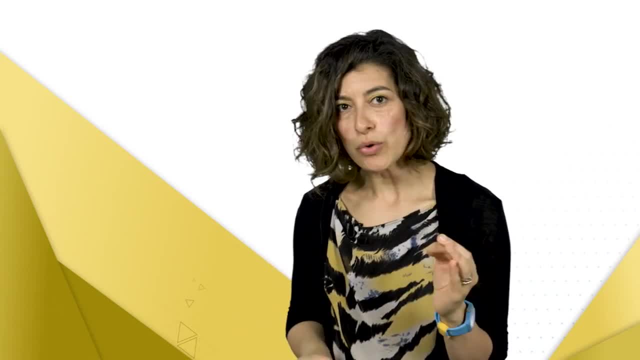 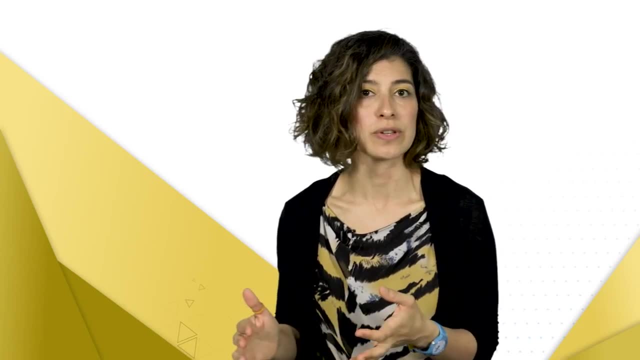 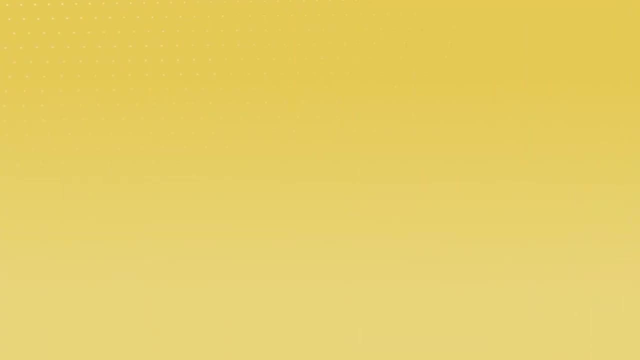 for the next task. To make the most of this video, I suggest you pause it during the calculations and try it for yourself before seeing my solution. Here is the process, both in binary and in hexadecimal. Let's do binary first. Say I wanted to hide. 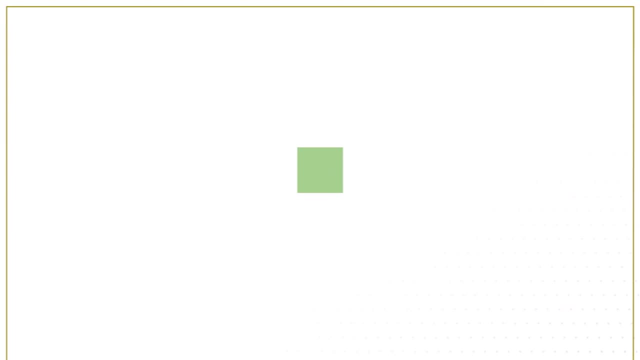 the pixel information: 162,, 200,, 140 on the pixel, with codes 255,, 150,, 20.. This is the code for the original image. We do it in this way. The red of the original image is 255,. 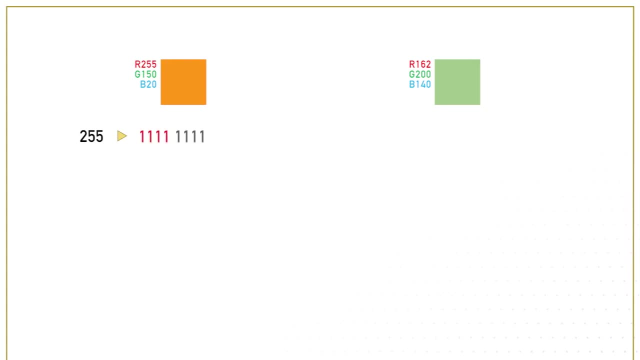 which is 1111, 1111. in binary, The least significant digits are 1111,, which we will ignore. The red of the hidden image is 162,, which is 1010, 0010 in binary, The most significant digits. 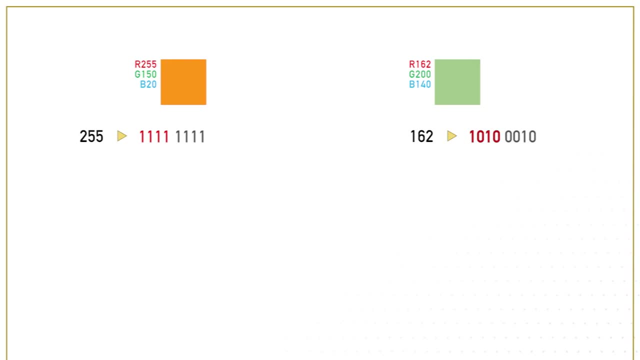 the leading digits are 1010.. The new red value will be 1111, 1010.. So we took the most significant digits of both callers but made the digits of the hidden caller of less significance. That means we put them at the end of the number. 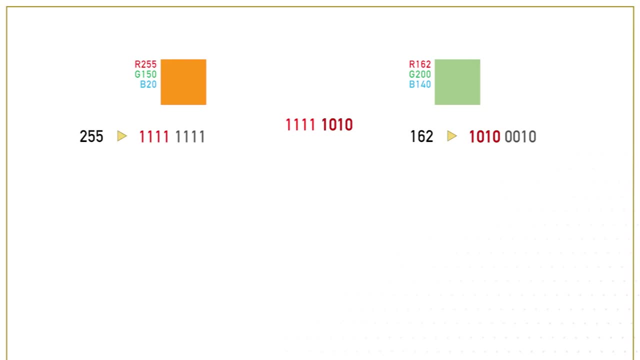 So red will have the value 1111, 1010,, which is 250.. Let's do it for green. The green of the original image is 150,, which is 1001, 0110. in binary, The least significant digits. 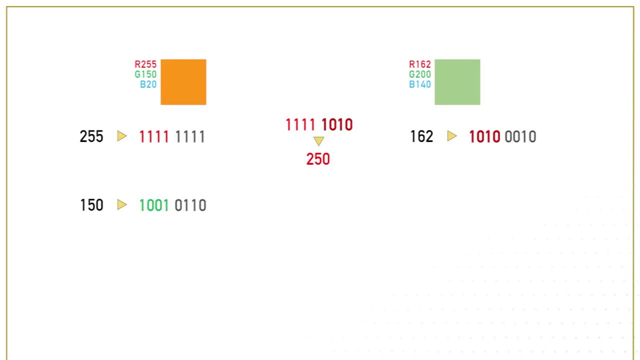 are 0110,, which we will ignore. The green of the hidden image is 200, which is 1100, 1000. in binary, The most significant digits are 1100.. So the new green value will be 1001, 1100.. 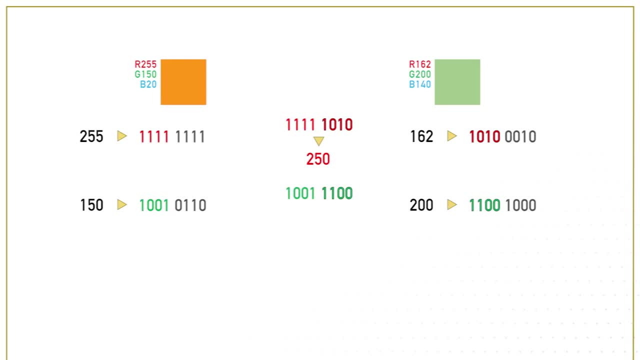 So we took the most significant digits of both callers but made the digits of the hidden caller of least significance. So the green color code will be 1001, 1100, which is 156.. The blue of the original message is 20,. 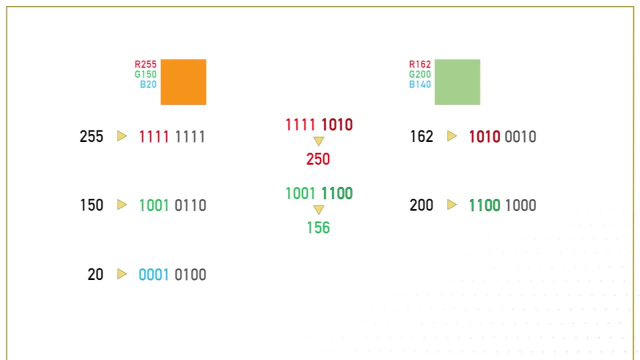 which is 0001, 0100 in binary. The least significant digits are 0100,, which we will ignore, And the blue of the hidden image is 140,, which is 1000, 1100 in binary, The most significant digits. 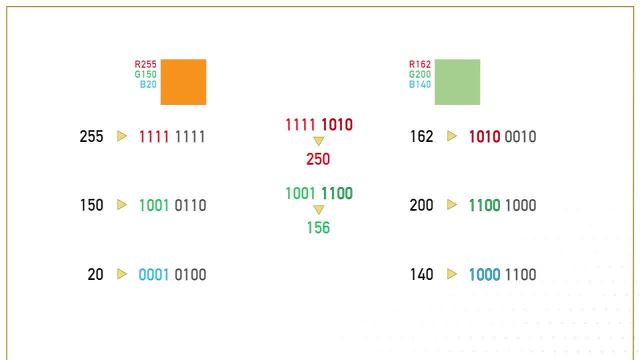 are 1000.. So the new blue value will be 0001, 1000.. We took the most significant digits of both callers but made the digits of the hidden caller of least significance, So the blue color value will be 0001,. 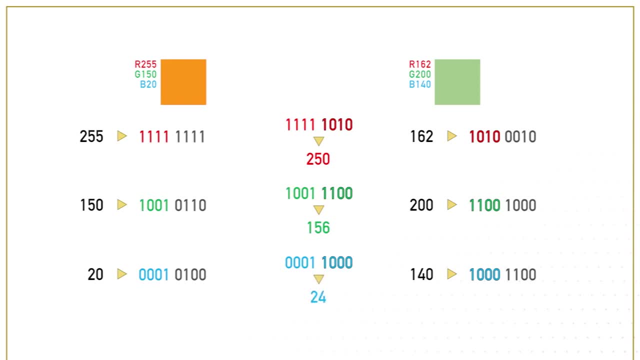 1000,, which is 24.. So the pixel of the image that contains the hidden image has RGB codes 250,, 156, 24.. These two shades are very similar. Can you tell the difference between the shade of the original image? 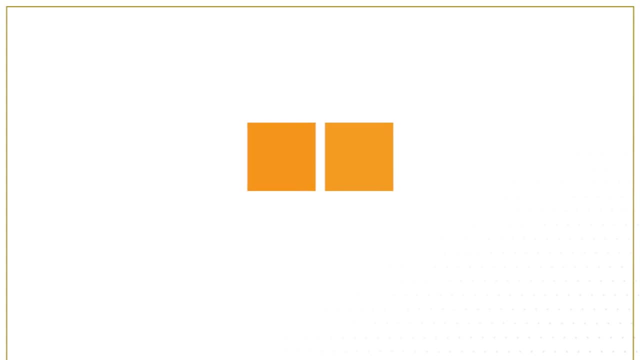 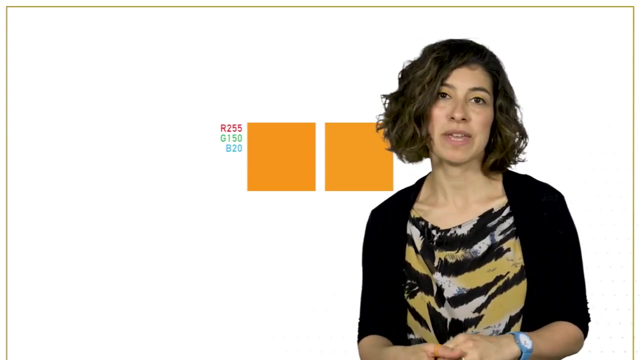 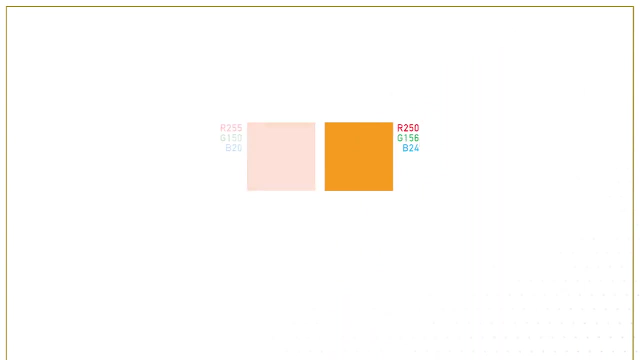 and the shade of the image. with a hidden pixel, The difference is very subtle And we would do this process for every pixel of the image. How well can the secret image be retrieved? Let's see. Let's do the inverse process For a pixel with RGB values. 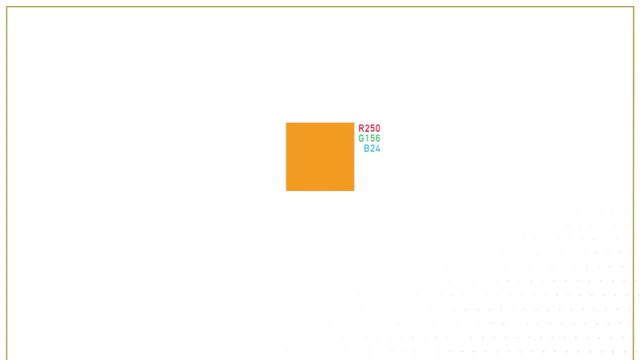 of 250,, 156, and 24,. this is from the image that has an image hiding inside. the red code is 250,, which is 11,, 11,, 10, 10. in binary, The least significant digits are 1010.. 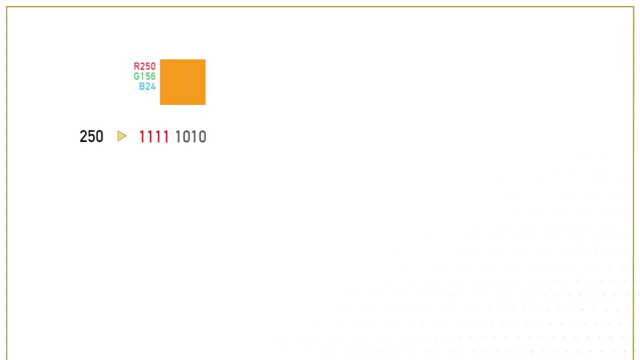 That is where the hidden image is. We use these to be the leading digits of the hidden color value. So we write 1010 0000.. We then convert this number, 1010 0000, to decimal, which gives us 160.. 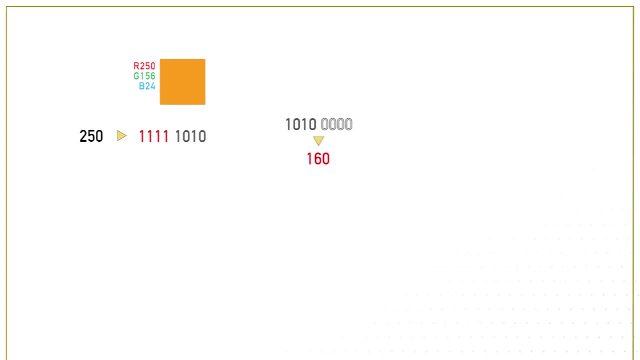 And so the hidden value for red is 160.. For the green code, which is 156,, written as 1001, 111, 1001, 1000 in binary, the least significant digits are 1100.. That's where the hidden image is. 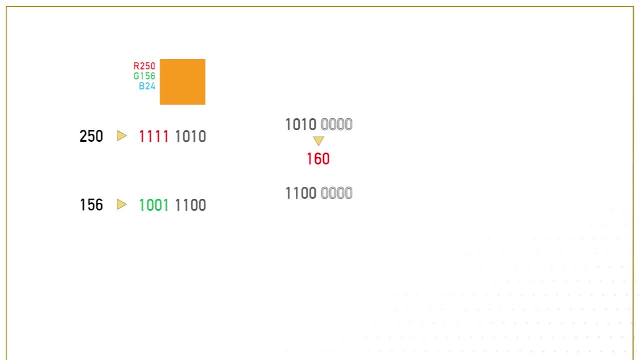 The hidden color value is 1100.. And we put four zeros at the end, So 1100 0000.. We convert this number to decimal, So 1100 0000 is 192.. And that is the hidden value for green. For blue, we have 24.. This is 0001, 1000. in binary, The least significant digits are: 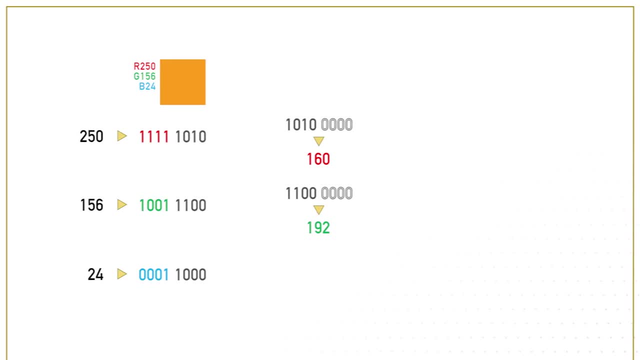 1000.. So the hidden color value is going to be 1000, with four zeros at the end. So 1000, 00, 00, 00.. We convert this number to decimal and we get 128.. The hidden color value for: 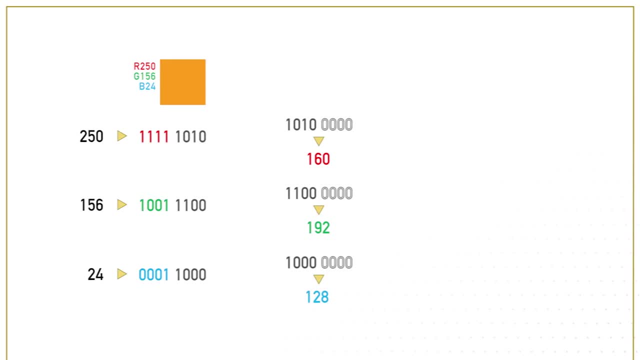 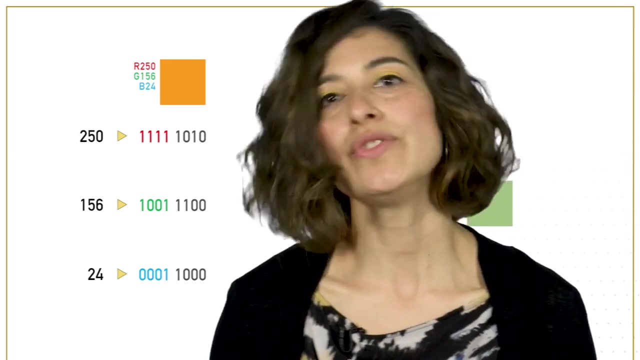 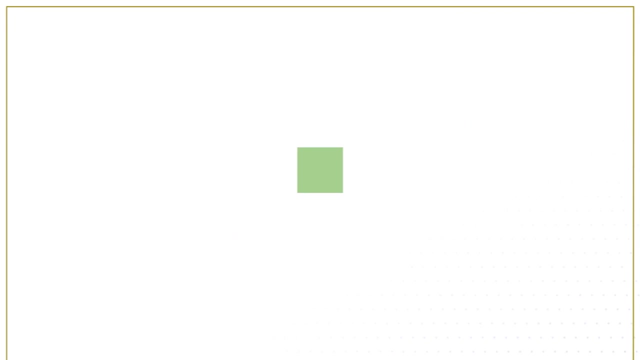 blue is 128. So the RGB color values for the hidden pixel are 160,, 192,, 128.. Now let's do this process in hexadecimal. Say, I wanted to hide the pixel information, the RGB code 162,, 200,, 140- on the pixel with RGB code 255,, 150, and. 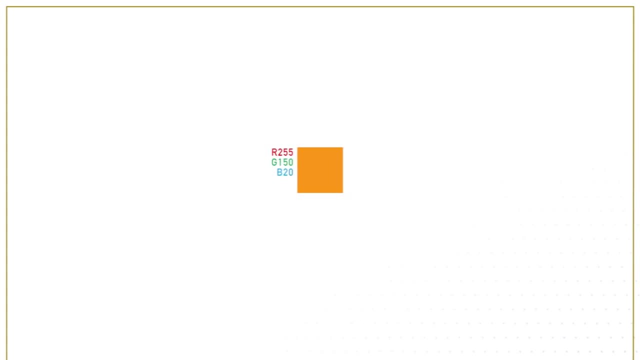 20.. So this is the one from the original image. We do it in this way. It is the same process, but we're doing it in hex. The red of the original image is 255, which in hexadecimal is FF. The least significant digit is F, which we will ignore. The red of the hidden image is: 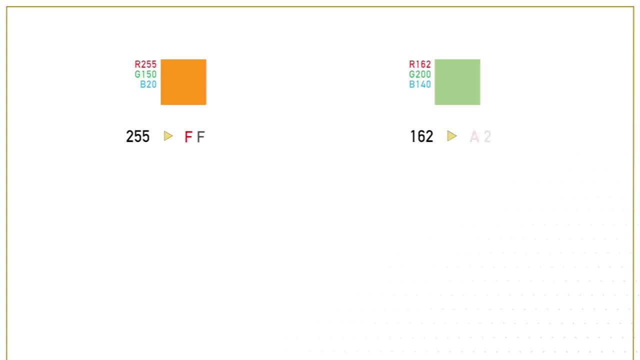 162, which in hexadecimal is A2.. The most significant digit is A, So the new red value will be FA. So we took the most significant digits of both colors but made the digits of the hidden color of less significance, So the red value will be FA, which is 250.. For the green: the green of the original message. 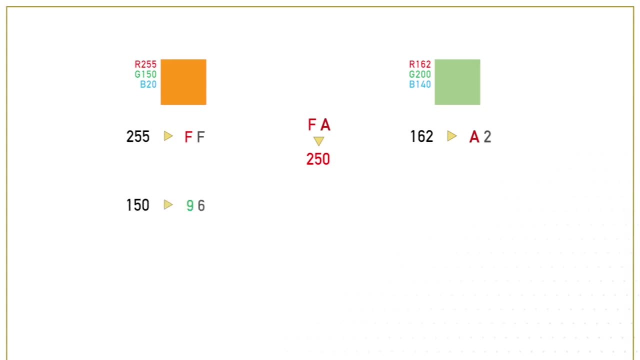 is 150,, which is 96 in hex. The least significant digit is 6,, which we will ignore, And the green of the hidden image is 200, written as C8 in hex. The most significant digit is C, So the new green value will be 9C. We took the most significant digits of both colors, but 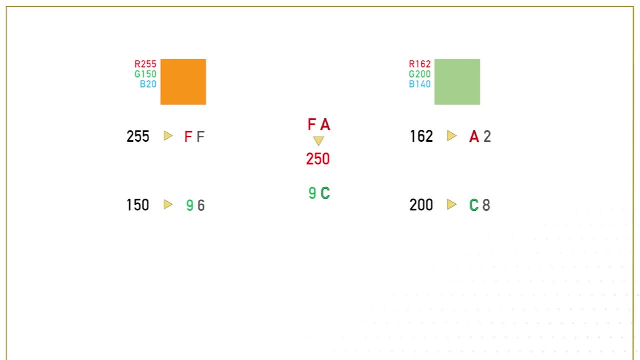 made the digits of the hidden color of less significance, So the green color code will be 9C, which is 156.. The blue of the original message is 20,, which is 14 in hex. The least significant digit is 4,, which once again we will ignore, And the blue of the hidden. 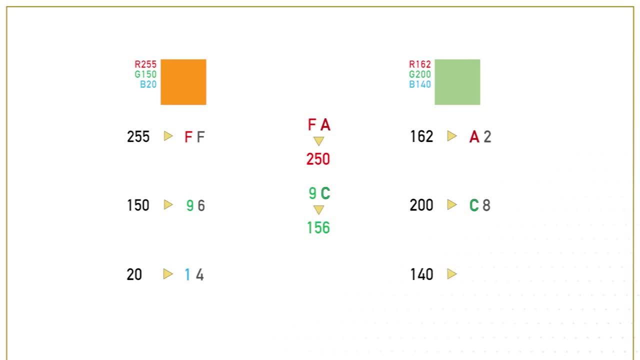 image is 140,, which is 8C. in hex, The most significant digit is 8.. The new blue value will be 18.. We took the most significant digits of both colors, but made the digits of the hidden color of less significance. 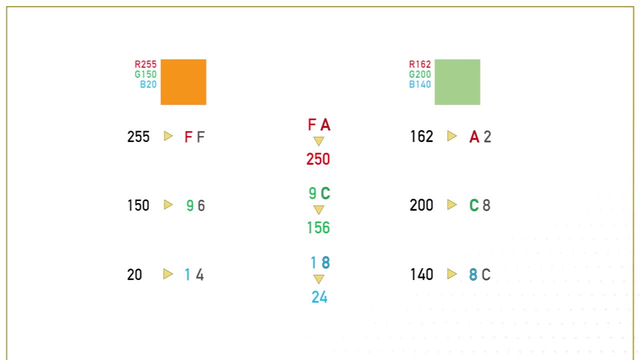 The least significant digit is 118 in hex, which is 24.. That means that the pixel of the image that contains the hidden image has RGB codes 250, 156, 24.. The two shades are very similar. Can you tell the difference? 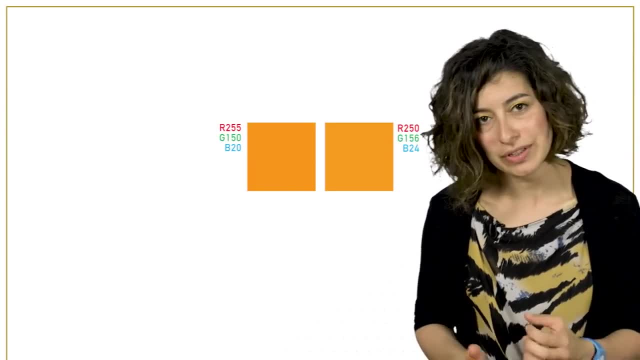 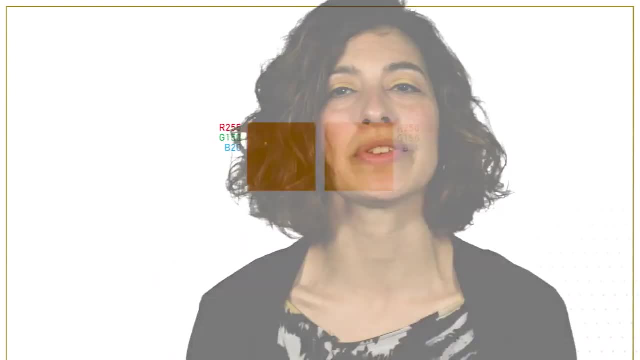 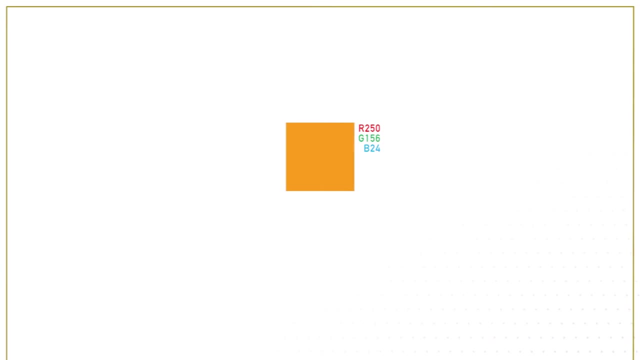 And we would do this process twice For every pixel of the image To retrieve the hidden image. we go pixel by pixel. once again, Let's take the pixel with RGB values 250,, 156,, 24,, which was the end result of the process we've just followed. 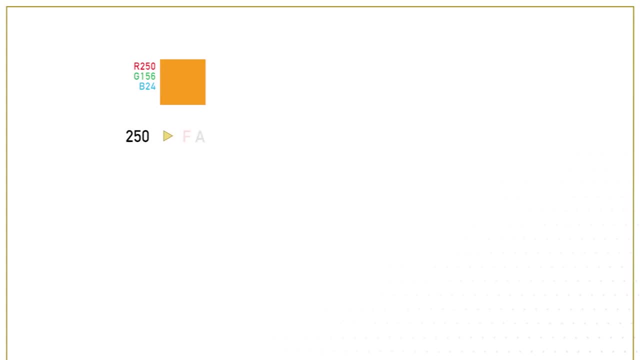 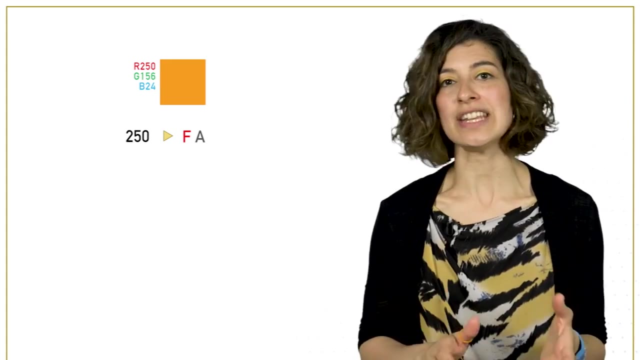 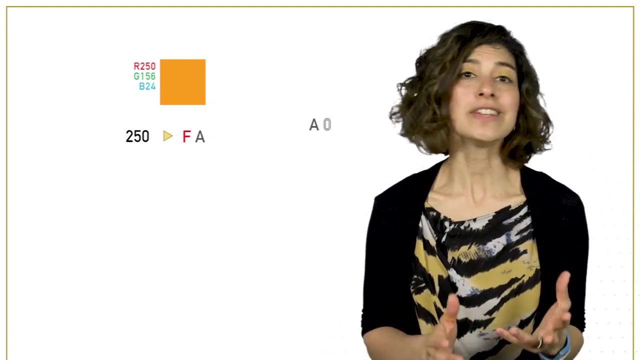 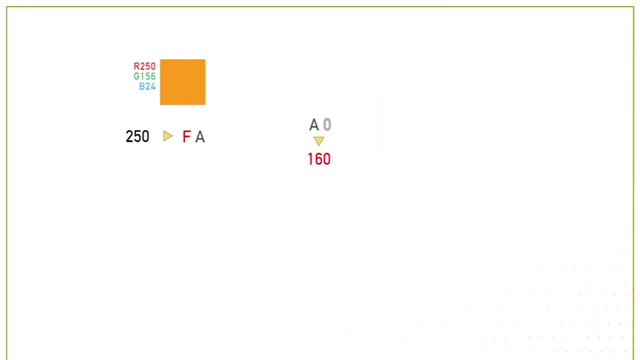 The red is 250, which is FA. in hex, The least significant digit is A. We use this as the leading digit of the hidden color value, which in this case is A0. Converting A0 to decimal gives us the hidden value of 160 for red. 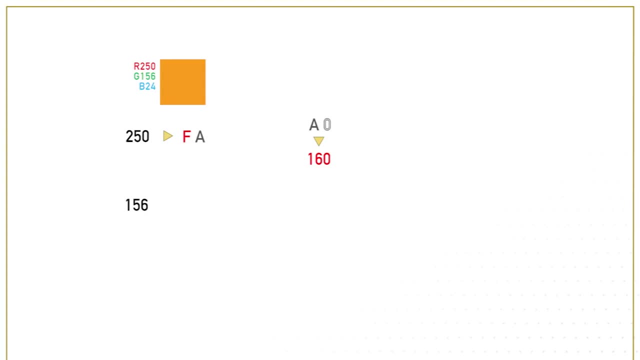 Let's look at green. The code is 156, which is 9C. in hex, The least significant digit is C, so the hidden color value becomes C0.. Converting C0 to decimal gives us the hidden value of 192 for green. 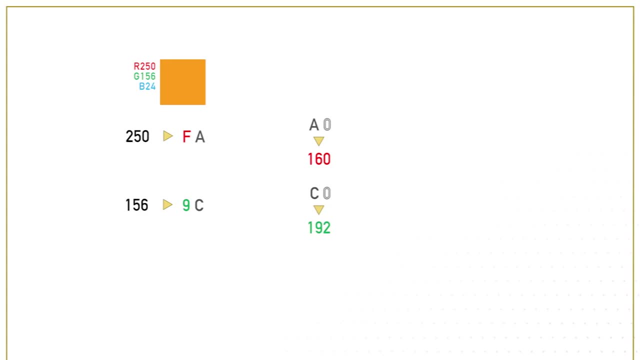 As to blue, the value 24 is 1: 8. in hex, the least significant digit is 8, and so the hidden color value is 8: 0.. We convert 8: 0 to decimal, giving us a hidden color value of 128 for blue. 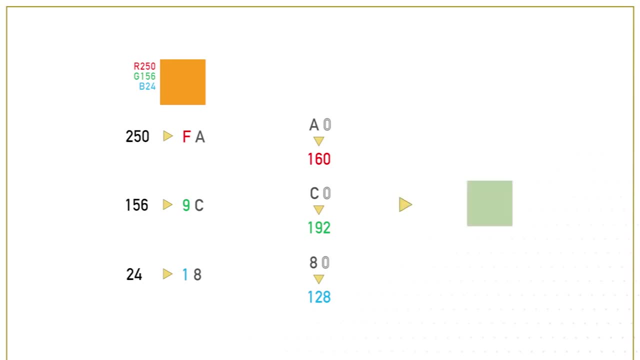 So the hidden color value we just recovered is RGB 160, 192, 128.. Compare these RGB color values to the color values of the original image. There is a slight difference, but it's not that much. Here's an example of an image and the secret image. 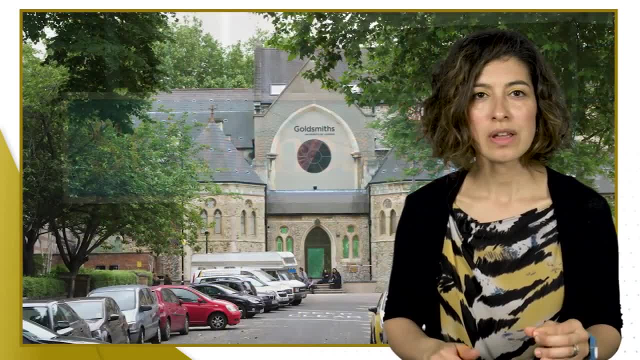 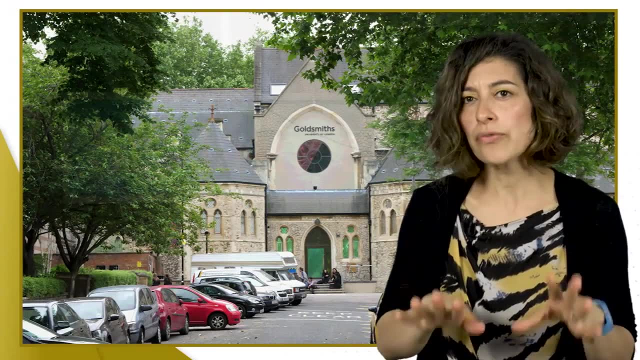 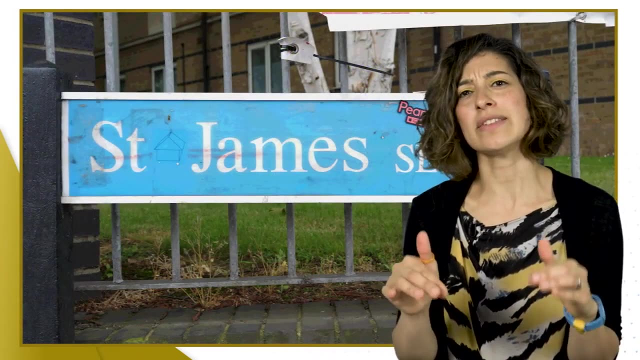 After hiding the secret image, the original image changes to this. It's not that different. When we follow the extraction process, the secret image comes out like this: It's not exactly the same as we started, but it's close enough to tell what it is. 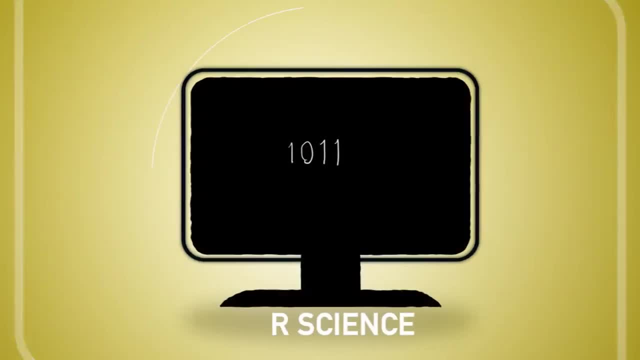 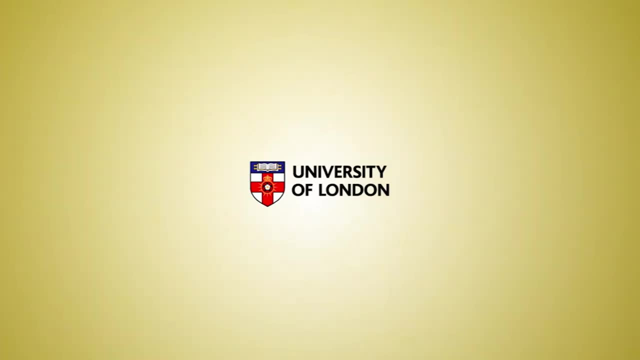 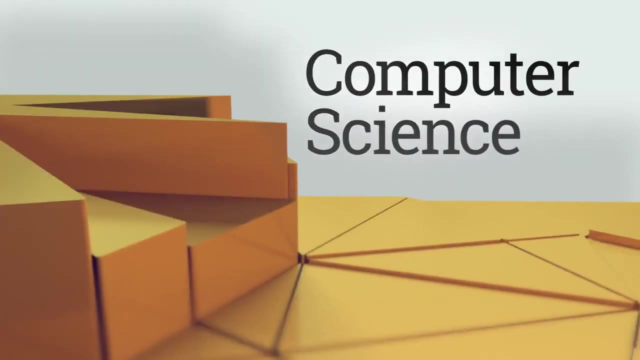 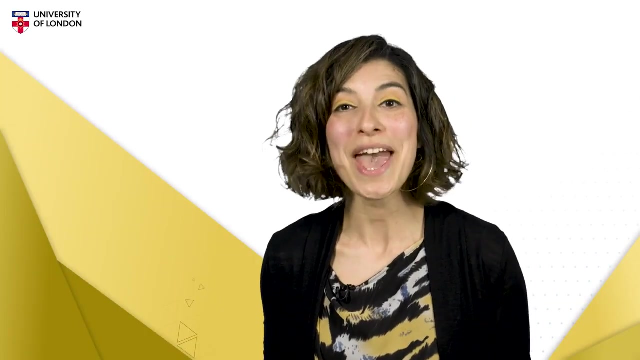 To Modify the image we use our. this time we need to try to modify the image First. we remove the hidden color values by clicking the News icon. when we click the News icon- Great news- We can perform arithmetic in octal and hexadecimal too. 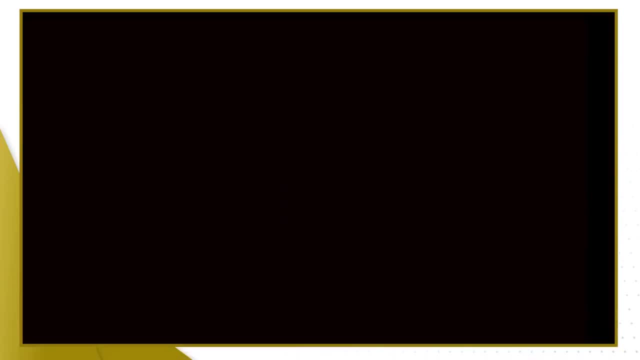 I'll show you. Say, we're adding up the octal numbers 7, 1, with 6, 5.. We're going to put them in columns, like we did with binary. So 7, 1,, 6, 5, all lined up. 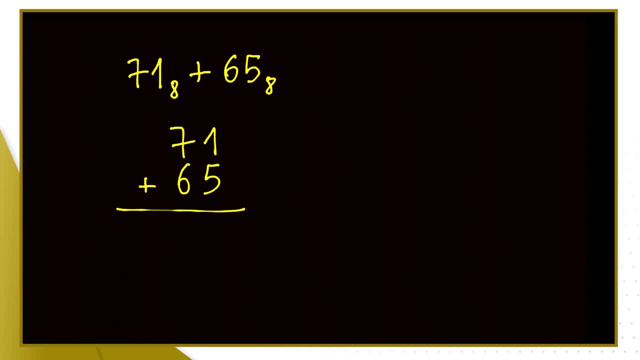 We're adding up these numbers column by column. So over here, 1 plus 5 is 6.. 6 is still less than 8, which is our base 8.. So it is a valid digit, so 6.. Then 7 plus 6, that's more than 8.. 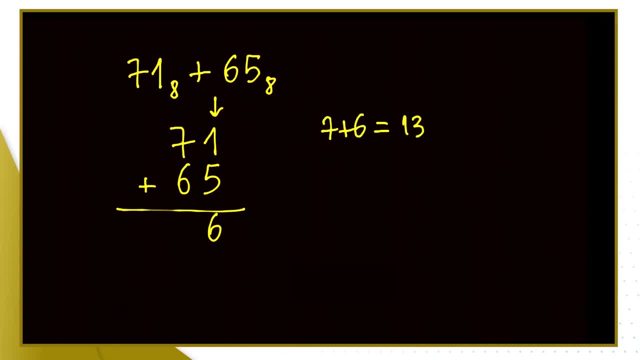 So 7 plus 6, it's a 13. And 13 in octal it's written as OK. let's work it out: It's 8 plus 5.. So that means it's going to be a 1 and a 5 in octal. 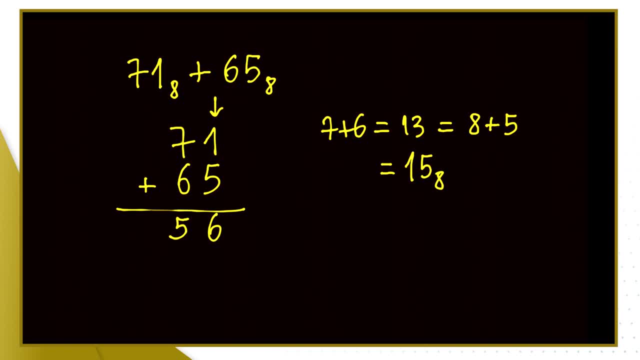 So we write a 5 here and we take 1.. That 1 is going to carry to the next place value, which just happens to be empty, and therefore we just write it there. So the result is 1, 5, 6 in octal. 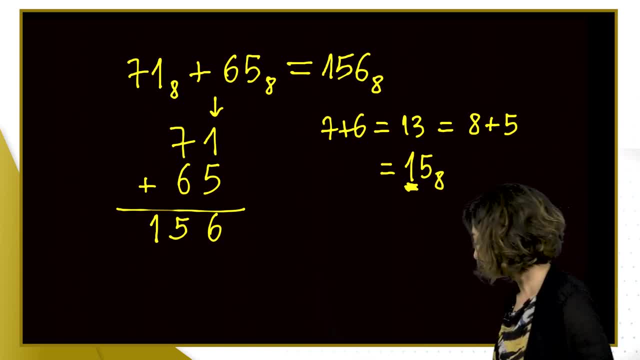 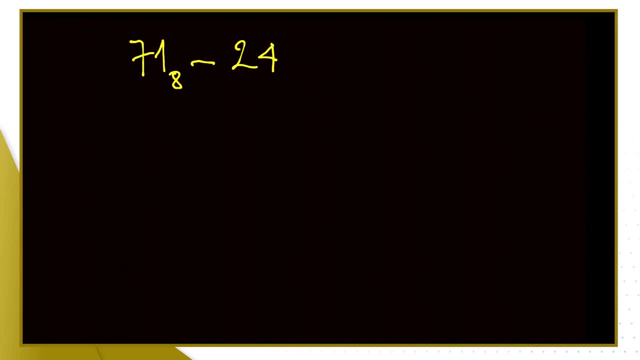 That's what it adds up to. Let's do a subtraction In a similar fashion: 7, 1 in octal, take away 2, 4 in octal. We line them up. We leave some space at the top for borrowing. 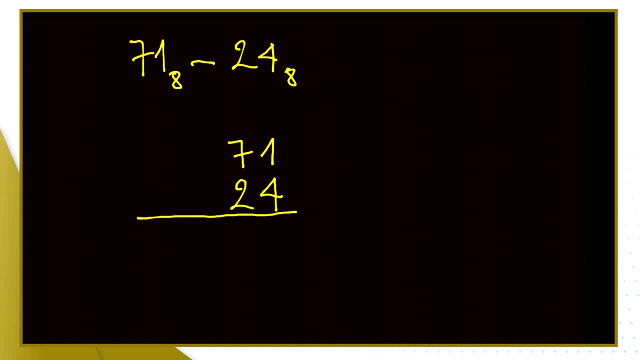 We're borrowing digits if needed and replacing some of the place values, So we start with 1 take away 4.. We can't do it straight away- 1 take away 4, because 1 is too small. So we're going to look at here. 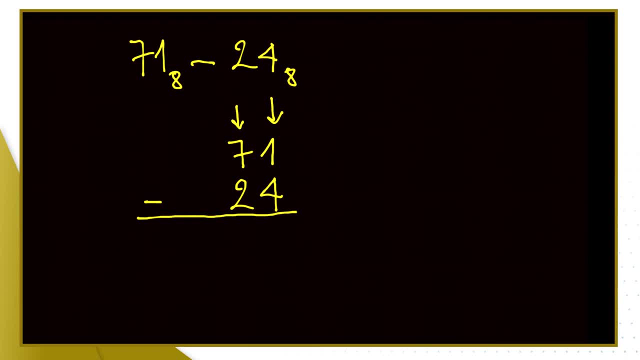 We've got 7.. We're going to borrow 1 from that place value, because 7 is 6 plus 1.. So we're going to leave a 6 there. We're going to borrow 1 over here, meaning we're going to replace that with a 6, and. 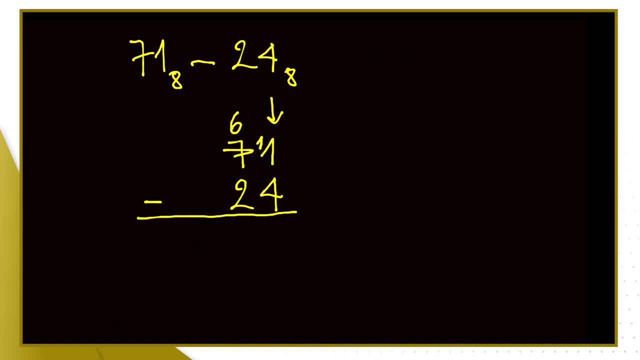 we're going to put a 1 in octal. So we've got 1, 1. take away 1, 4.. I'll just rewrite that more neatly, So that 1 there becomes a 1, 1.. And now we do 1, 1 in octal. take away 4.. 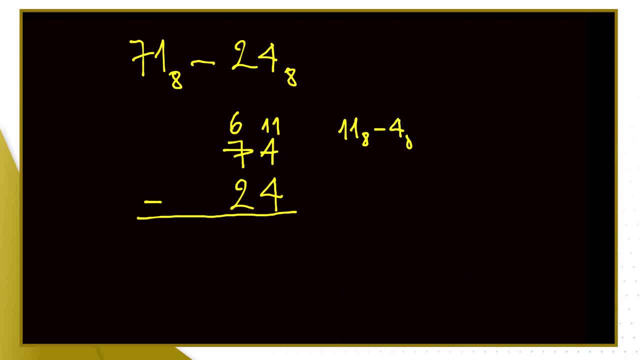 1, 1 in octal. take away 4 in octal. Let's remind ourselves what 1, 1 means: It's 8 plus 1.. And now take away 4.. And so we've got 9. take away 4, which is 5.. 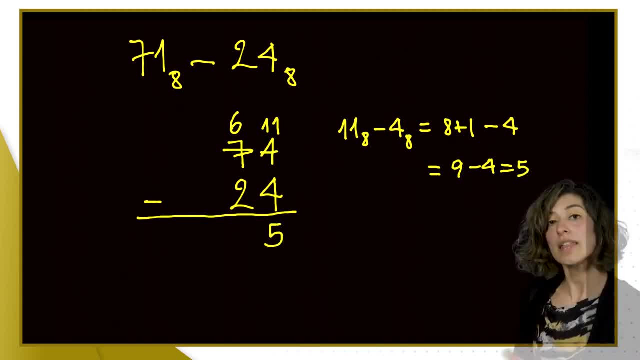 Therefore, we've got a 5 there. Okay, And now we move on to the next place value. We've got 6 take away 2.. So here's 6 take away 2, and that is 4 in octal. 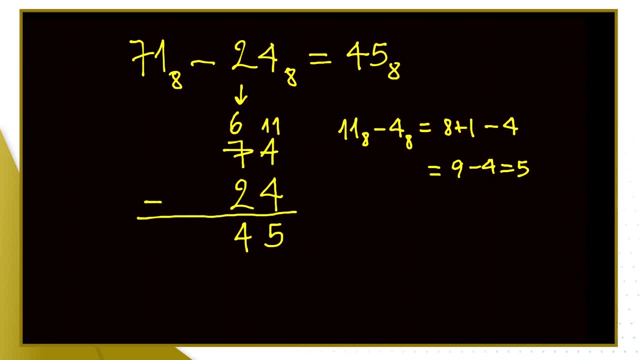 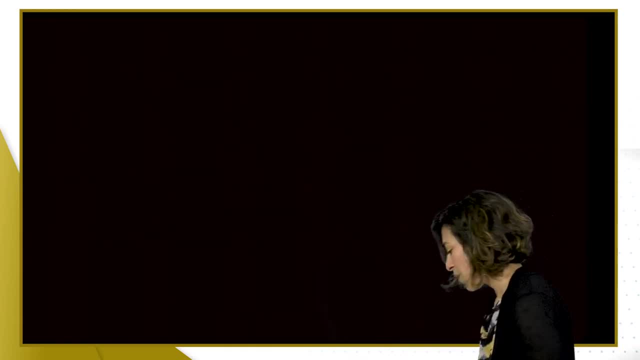 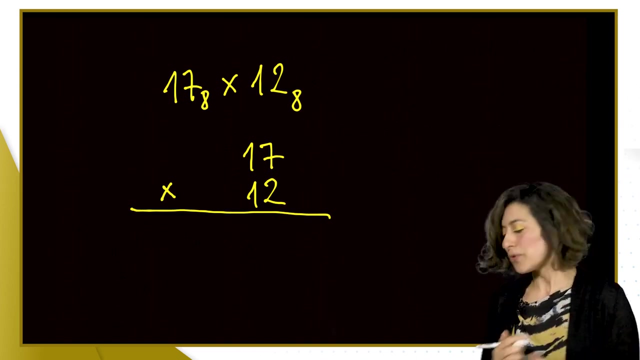 So the result is 4, 5 in octal Multiplication, next Multiplying 1, 7 in octal by 1, 2 in octal, Minding them up, Okay. So we're going to do like before. 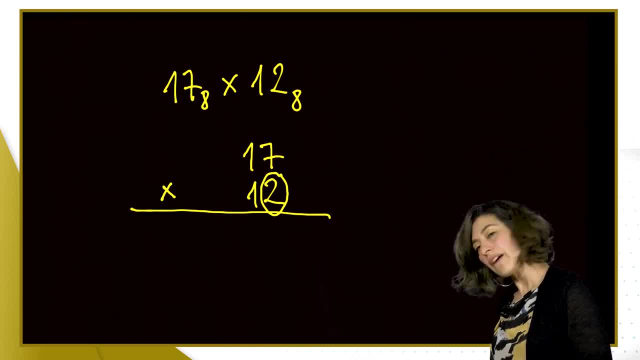 We multiply this 2 by the 1,, 7. Write the result over here. And then we multiply this 1 by the 1,, 7.. Write the result here: Shifted 1 place value. That's what I'm going to do. 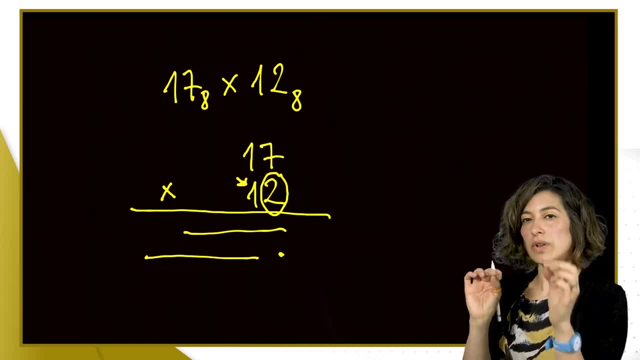 But we're going to have to go back and forth with decimal to interpret the multiplication digit by digit. in decimal, in octal, I'll show you. Okay, Right, So 2 times 7.. 2 times 7 is 14.. 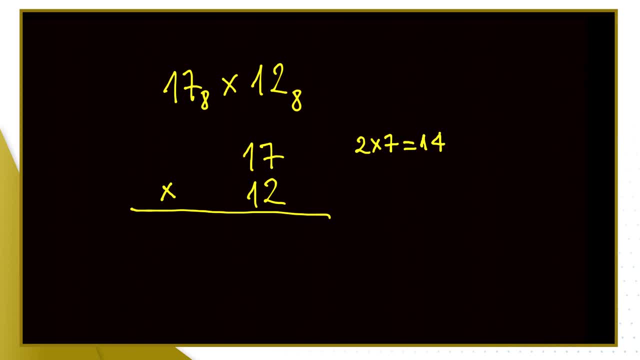 Now, 14 is not a number we can use in octal straightaway. We need to convert to octal. It's greater than 7.. So this is 8 add 6. Which makes 1 in octal And 6 in octal. 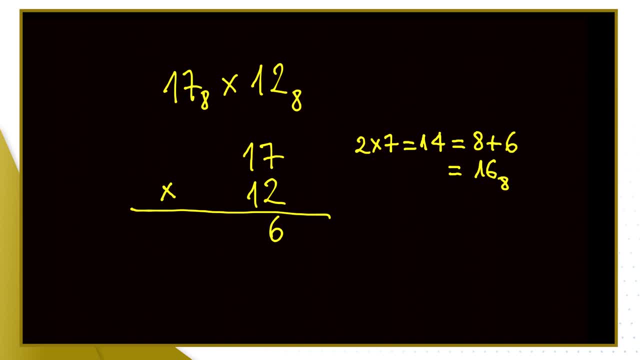 So we put the 6 here And we have a 1 that is going to hang around there. Now we do 2 times the 1., This 2 times that 1., Which is just 2.. And we do that 2 added with this 1.. 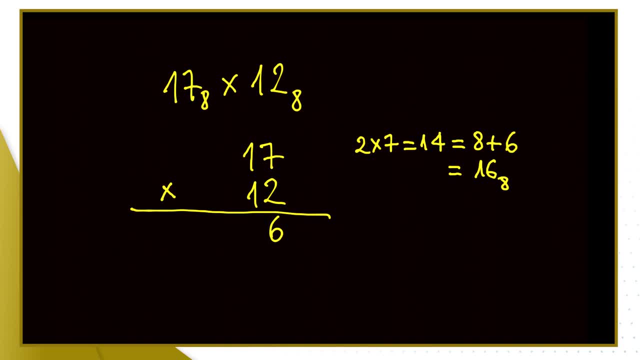 It's going to be 3.. 3.. Now We're going to multiply, We're going to shift things: one place value And we're going to do 1 times 7., Which is 7. And 1 times 1.. 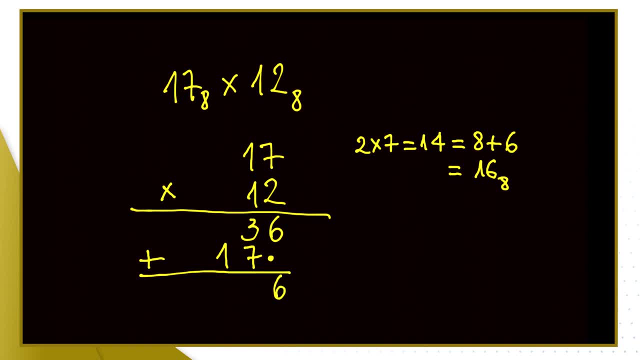 Which is 1. And add them up So we've got 6.. 3 plus 7 is 10.. 10 in octal is 8 plus. So 8 plus 2 means it's 1, 2 in octal. 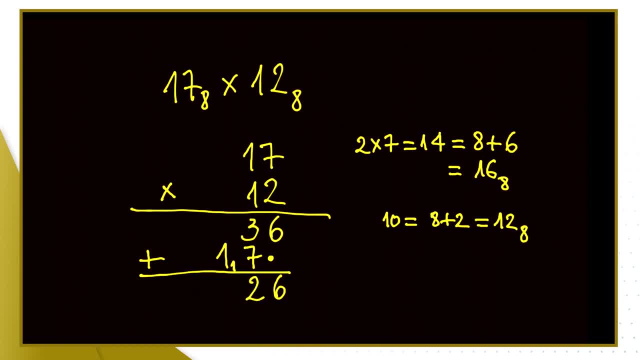 So put the 2 here And carry the 1 over there, And now 1 plus 1 is 2. Which is valid in octal. So that means 2, 2, 6 in octal. And now let's look at the similar operations in hexadecimal. 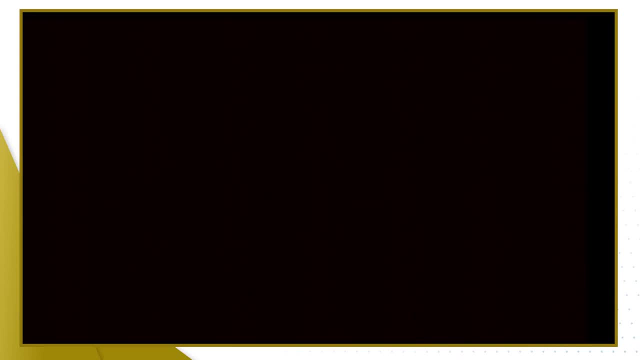 We're going to add up two numbers in hexadecimal. We're going to have the number AB in hexadecimal Added with 2, 5 in hexadecimal. Let's just remind ourselves what the letters mean. So after 9 comes, 10 is A. 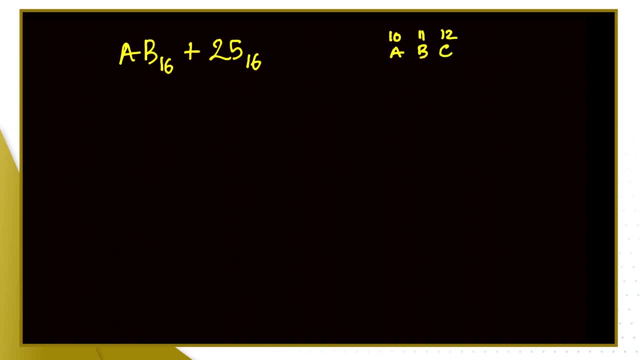 11 is B, C is 12.. D is 13.. E is 14.. F, F is 15.. And we're going to line up the numbers as before: AB 2, 5.. Add them up. We're going to do column by column. 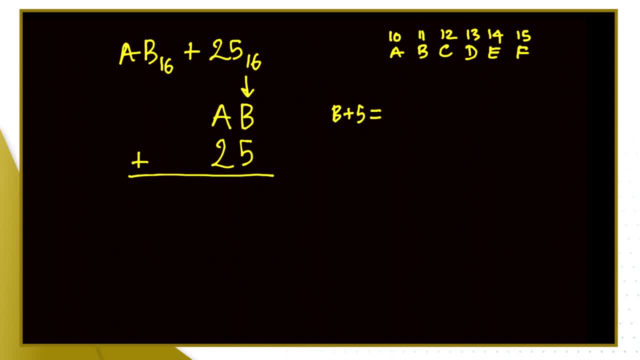 We've got B plus 5.. B plus 5. We're looking at 11 at 5.. That is 16. And 16 in hexadecimal is going to be 1: 0.. So I'm going to write 0 here. 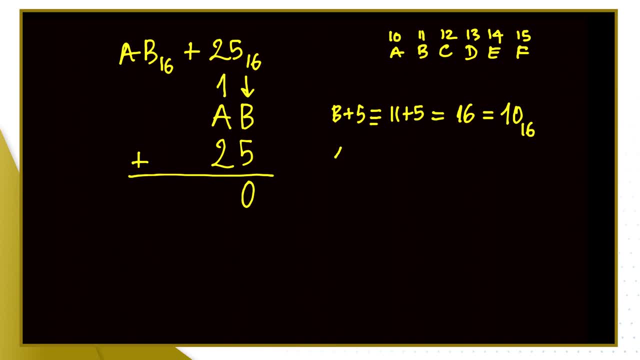 And 1 on that column. And now I need to add up the 1 with the A with the 2. And that is 1 plus 10, because A is 10 plus 2.. That makes it 13.. And 13 is the digit D in hexadecimal. 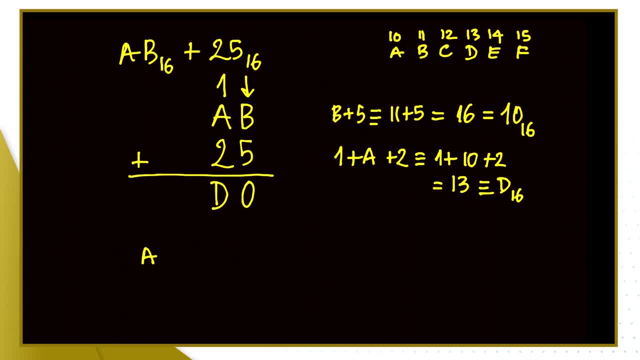 So I'll write D there. So that means that AB in hexadecimal Add 2, 5 in hexadecimal equals D, 0 in hexadecimal. And in a similar fashion we're going to do a subtraction. We have AB in hexadecimal. Take away 1 F in hexadecimal. 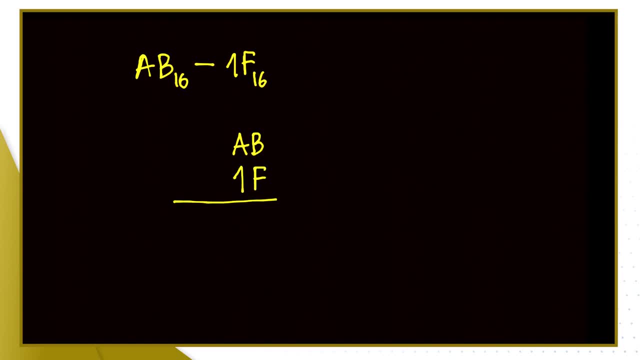 So AB and 1 F all lined up, Take away. So, column by column, we're going to B, take away F. Now let's remind ourselves again: B stands for 11. B is 11. And F is 15.. We can't really do 11, take away 15.. 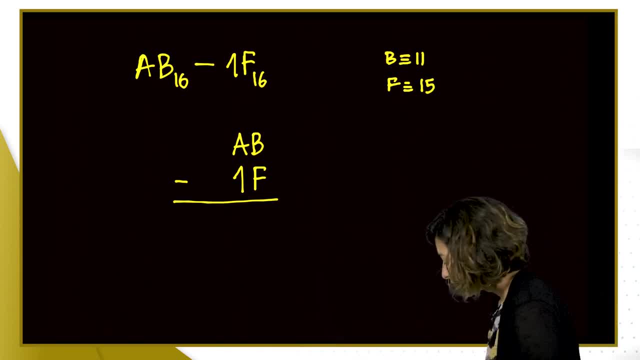 We're going to have to borrow from the next column, So A is worth 10.. So we're going to say: A which is 10 is the same as 9 plus 1.. So we're going to replace that A by a 9.. 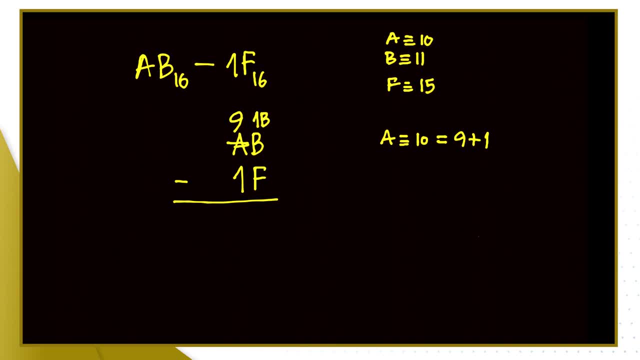 And we're going to put 1 B in this column. And now 1 B in hexadecimal means 16. add 11 from the B, That's 27.. And then 1 B take away F means 27, take away 15.. 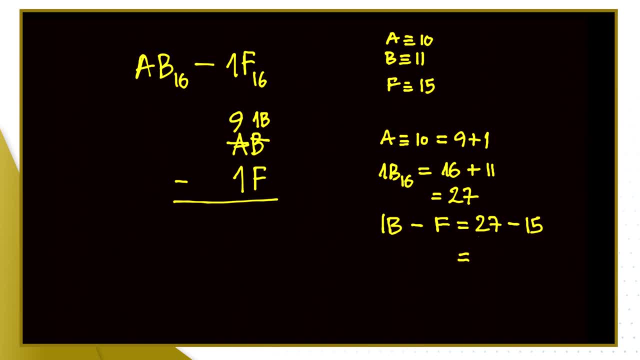 Because F is 15. And that gives us 12. as a result, 12 is letter C in hexadecimal. That means I've got C there, And now all I'm left to do is 9. take away 1, which is 8.. 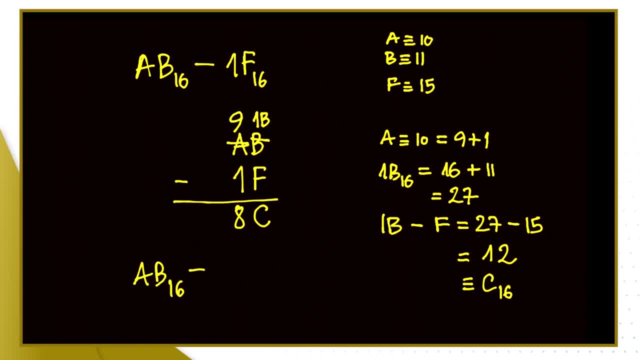 That means that A- B in hexadecimal. take away 1 F in hexadecimal equals 8 C in hexadecimal. One more, We've got a multiplication All right. So A- B in hexadecimal times 1: 1 in hexadecimal A B 1: 1.. 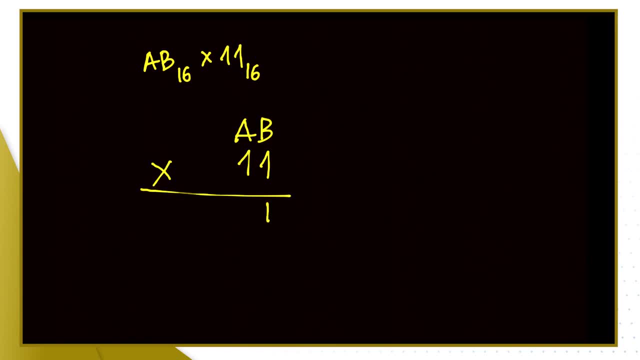 Let's multiply. So we're going to do 1 times B, which is B, 1 times A, which is A, And then we're going to write 1 times B, which is B, here And A, And add them up, So B. 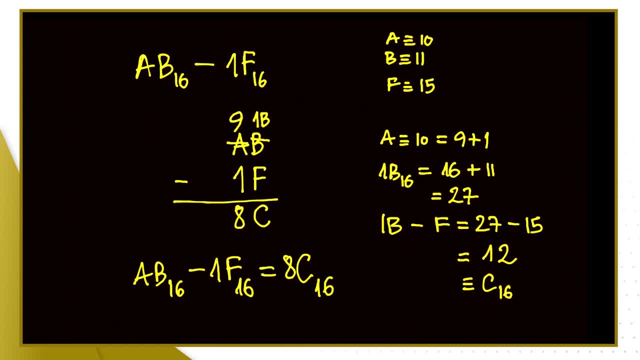 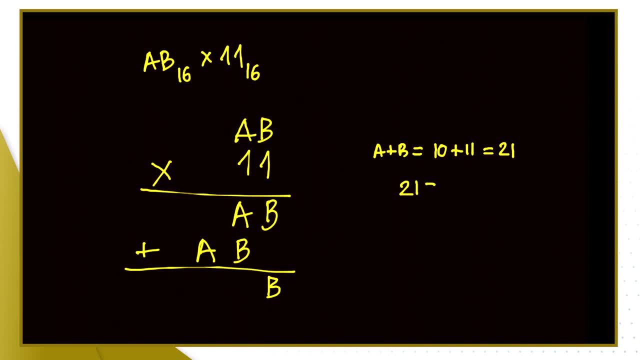 A plus B. A plus B is 10 plus 11, which is 21.. And 21 is 16 plus 5, which makes it 1, 5 in hexadecimal. And put a little 1 there, And now we do A plus 1, which is B. 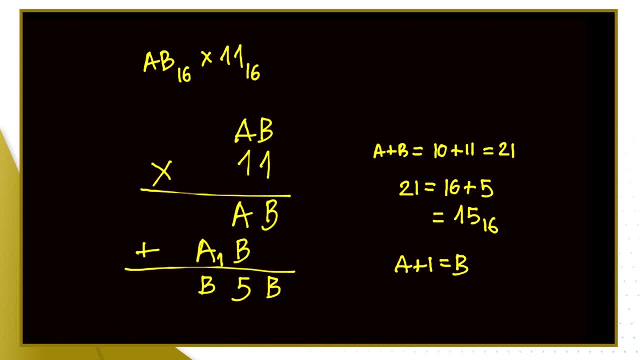 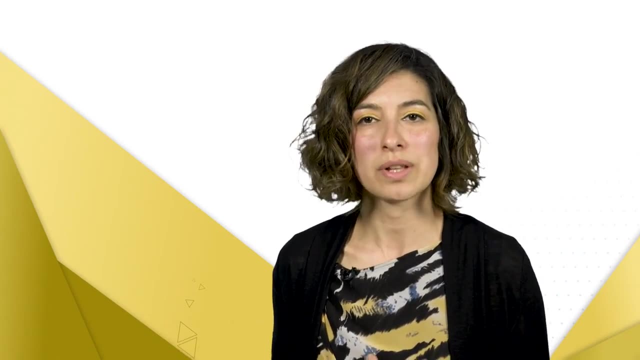 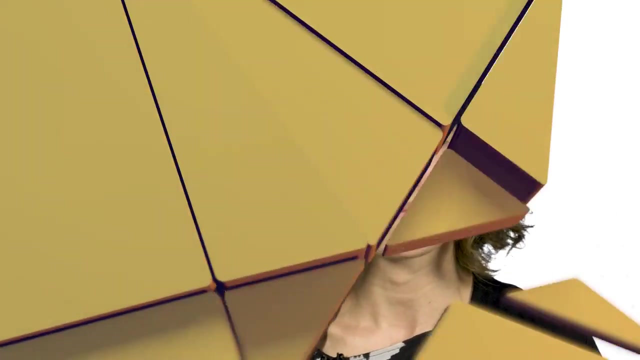 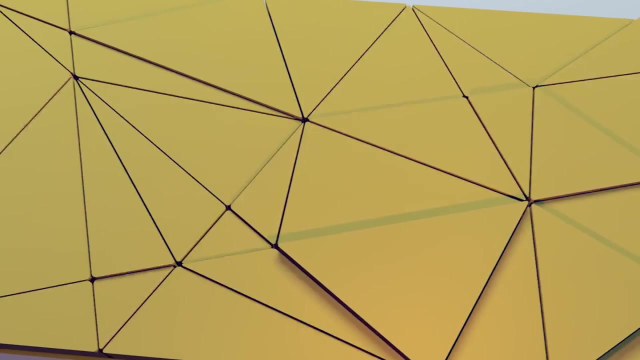 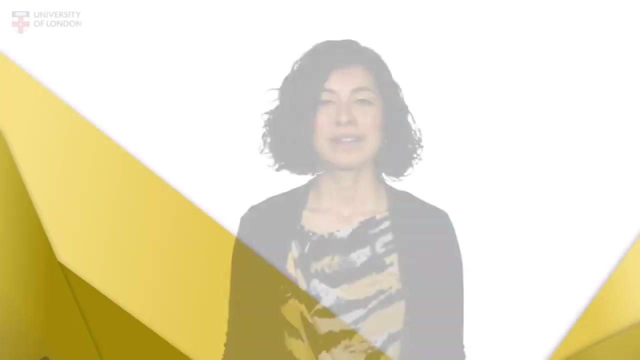 So A plus 1 is just B And the result of this sum is B 5 B in hexadecimal. So we can use the same ideas of adding, subtracting and multiplying from decimal and binary into octal and hexadecimal. You can even extend it to other number bases. 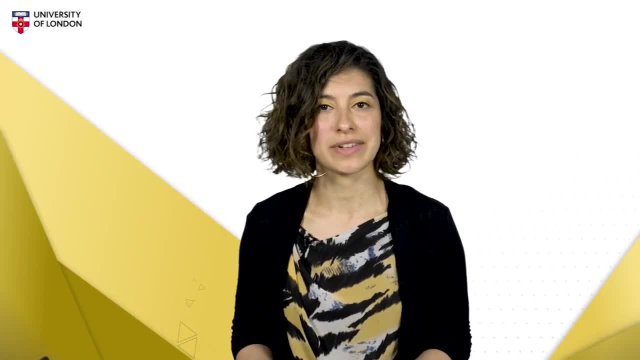 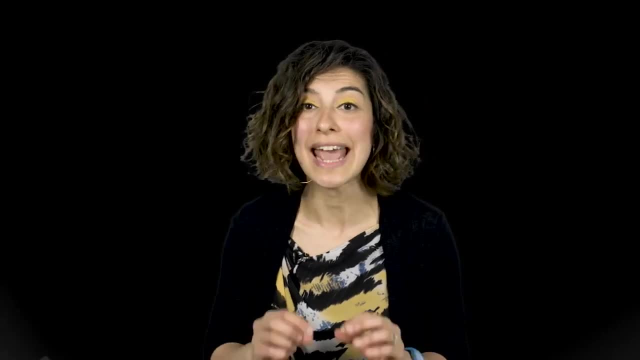 We have worked in great detail: Binary, octal and hexadecimal. I just want to show you a few examples of how we extend the same techniques into working in any base. The main thing to bear in mind is that in, say, base 3, we're using digits from 0,, 1, and 2.. 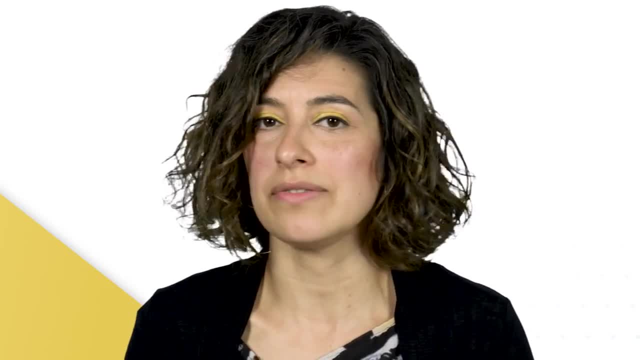 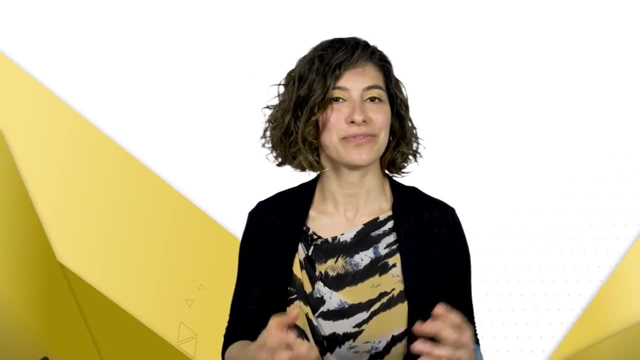 So digits up to 3. If it's base 5,, 0,, 1,, 2,, 4.. Base 60, up to 59, and so on. That means that when we are converting from decimal to any base, say base 3,. 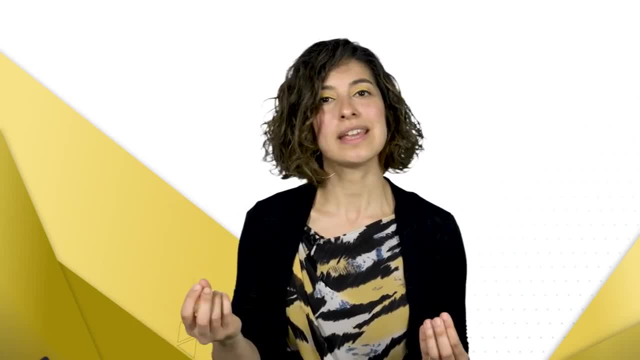 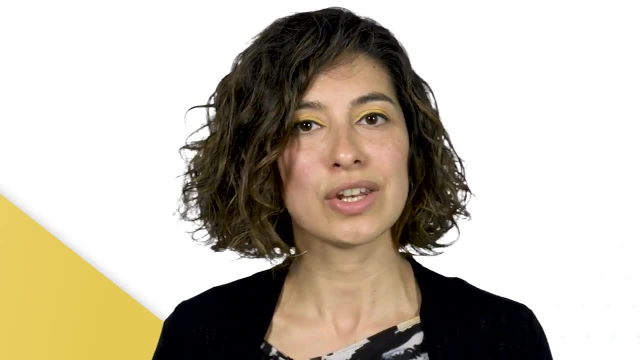 we keep dividing over and over again By 3 and taking note of the remainders For the fractional part. we will multiply by 3 over and over again and take note of the integer part, And that's how we extend the algorithm to any base. 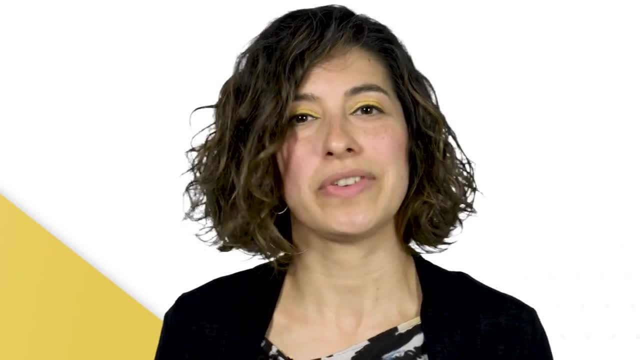 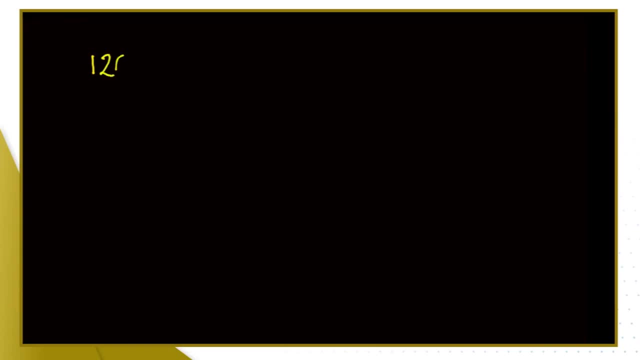 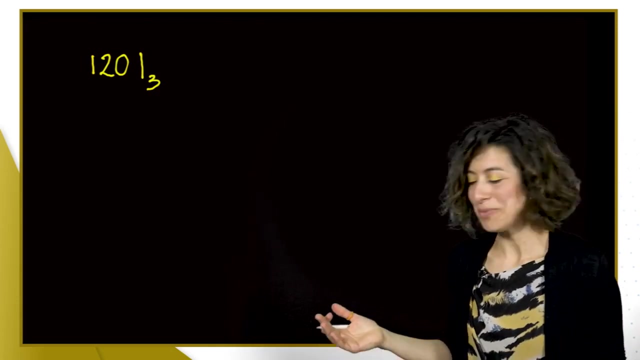 With operations, you'll see that it's very similar. I'll stop talking and I'll show you some examples. Say, we have 1201 in base 3.. What is this number in decimal? Well, base 3 is going to use place values that are powers of 3, starting from 1.. 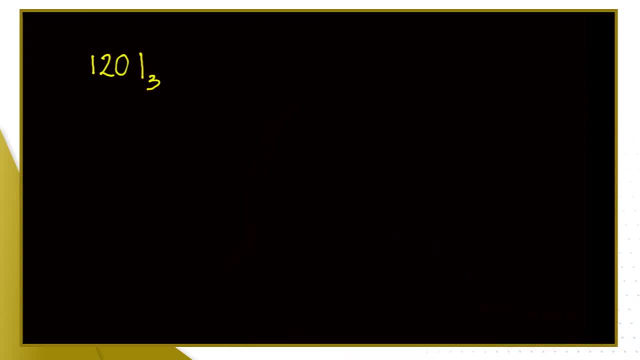 So we'll write those up As a reminder. we have 1,, 3,, 3 squared, which is 9,, and 3 cubed, which is 27.. That means we go straight to the expanded form, which is 1, the digit times the 27.. 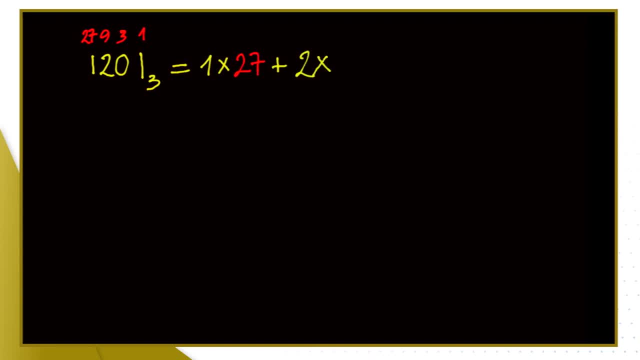 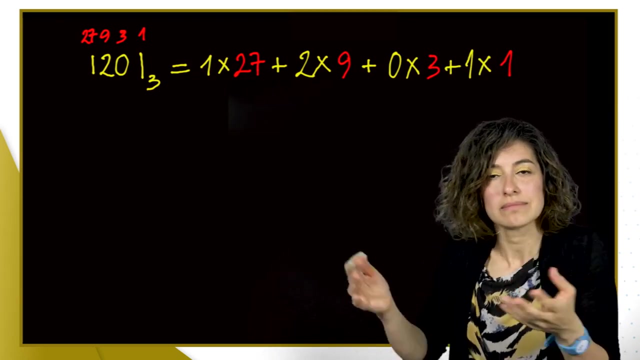 Plus 2, the digit times the place value 9.. Plus 0, times the place value 3.. Plus 1, times the place value 1.. And that was a number in ternary base 3, because the digits were 1201.. 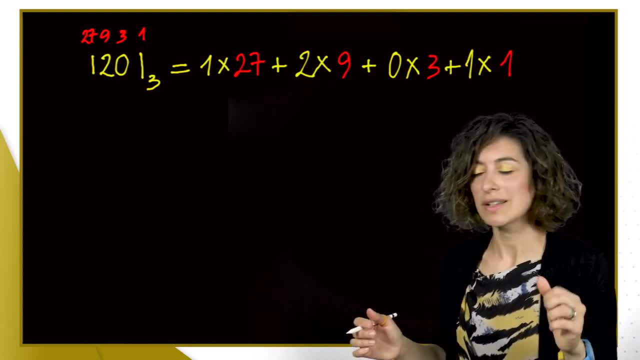 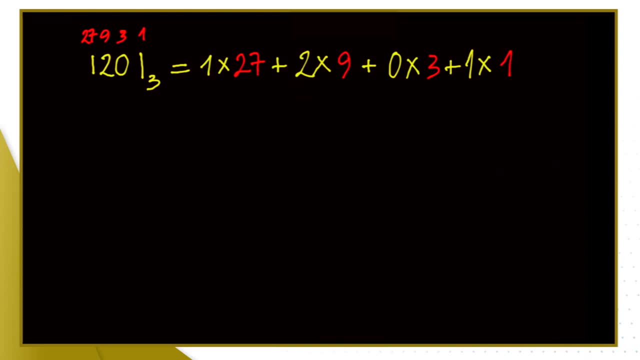 There were no digits 3 or greater. Now we have the expanded form. We just do the calculation and get on with it. So we've got 27 plus 18 plus 1. That makes t40, 46. And so 1201 in ternary is 46 in decimal. 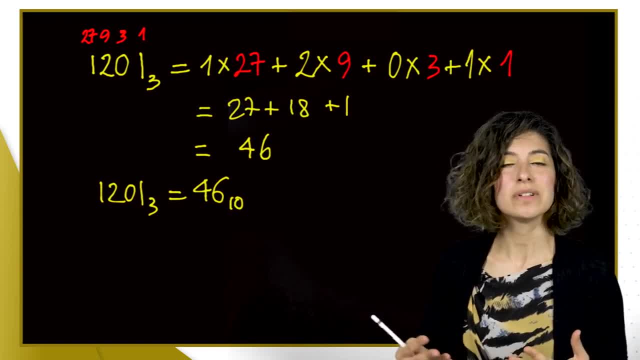 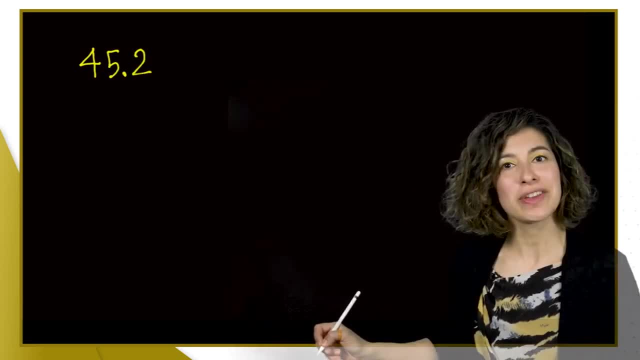 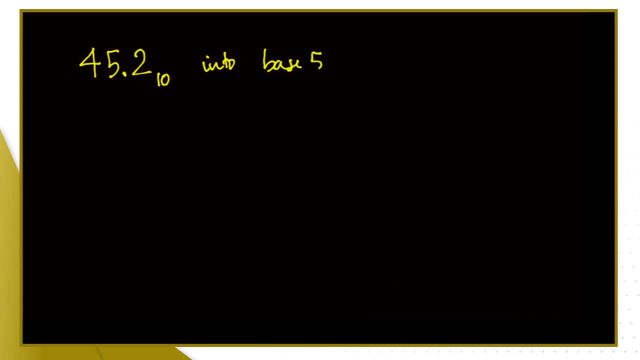 Let's look at changing from decimal to base 5.. Let's do 45.2.. 45.2.. I'm allowed to say 45 because it's decimal And we want to write this into base 5.. This is the division algorithm. 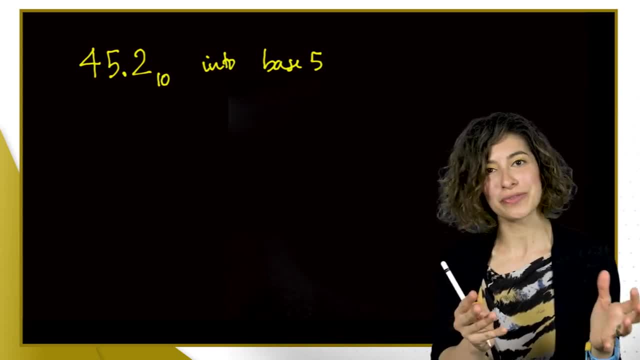 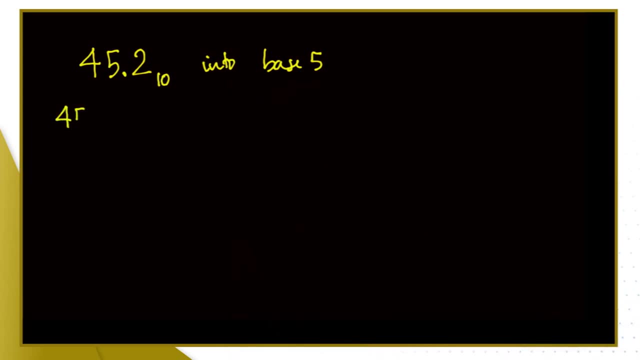 Well, kind of It is the division algorithm for the integer part, for the 45, and it's going to be the multiplication by 5 algorithm for the 0.2.. So let's do it separately. So 45, we're going to divide by 5, because it's base 5.. 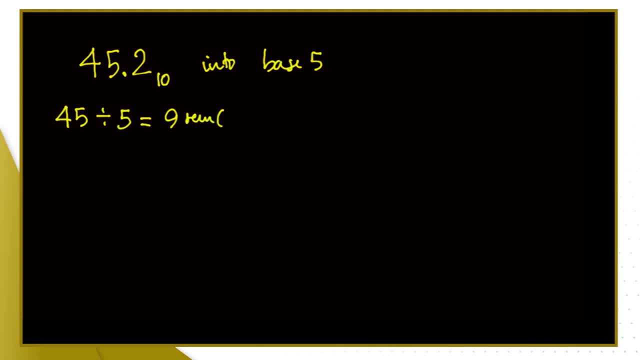 And that is 9 remainder 0.. And then 9 divided by 5, it's 1 remainder 4.. And then 1 divided by 5 is 0 remainder 1.. That gives me the digits for 45.. So 45 in decimal is written as: 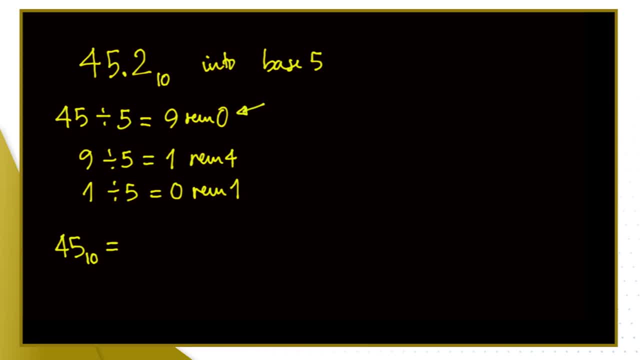 Remember, the first remainder is the. The left remainder is the rightmost digit, So the 1 is going to be the leftmost, So 140 in base 5.. Now let's do the fractional part, So 0.2 in decimal. 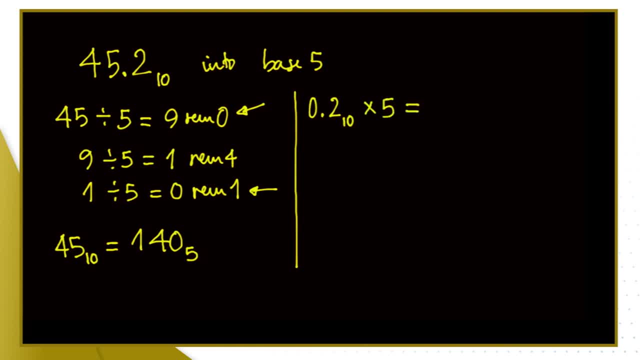 We're going to multiply that by 5.. 0.2 times 5 is 1.. 1 is the whole part, So that's going to be the first digit. We take away the 1, we have 0. And so we stop. 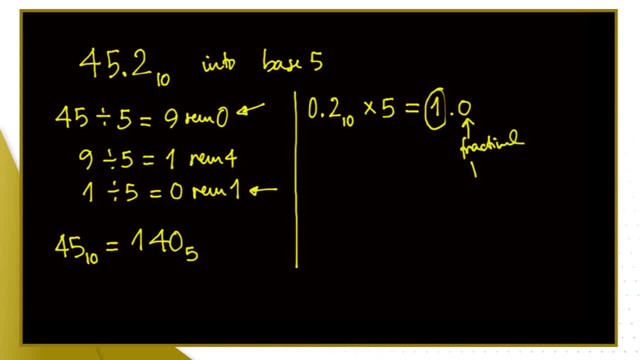 So this is Fractional. part is 0.. So we stop, And that means that 0.2 is going to be written as 0.1 in base 5. Which is OK, because 0.2 is a fifth. 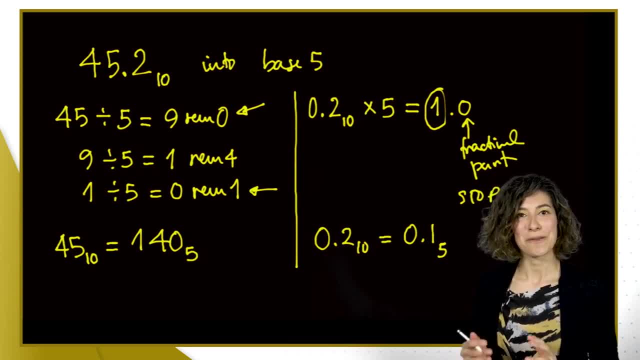 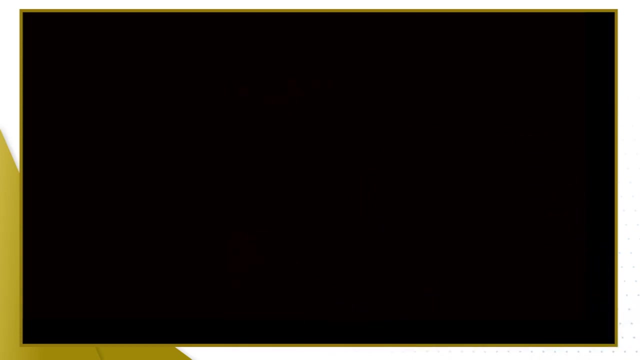 And 1. fifth is the first fractional place value for base 5.. So, putting it all together, 45.2 is 140.1 in base 5.. So let's look at an example of addition. Let's do addition in base 11.. 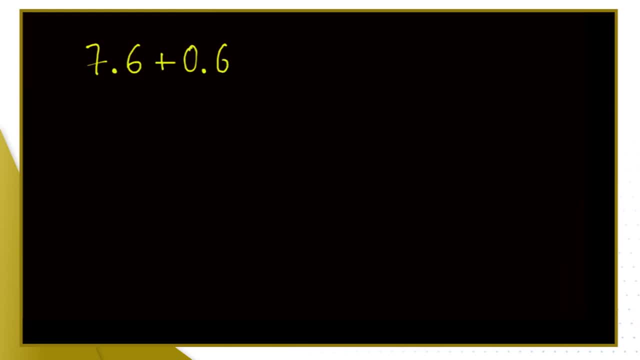 7.6. And 0.6 in base 11.. We're going to stack the numbers one on top of the other. Do the addition: 6 plus 6 is 12.. 12 is 1 more than our base. 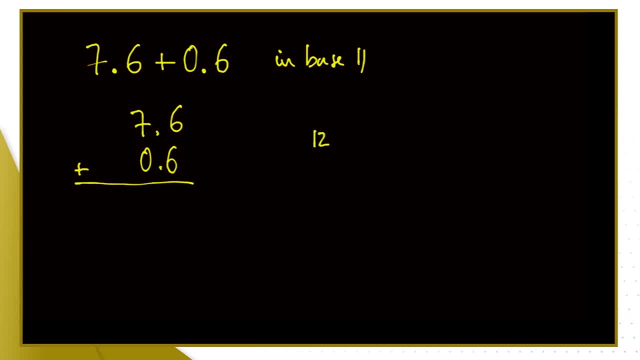 So 12 in base 11.. So 12 in base 11 is going to be 1.11 plus 1. So it's going to be 1.1.. That means I put a 1 here, the units one. 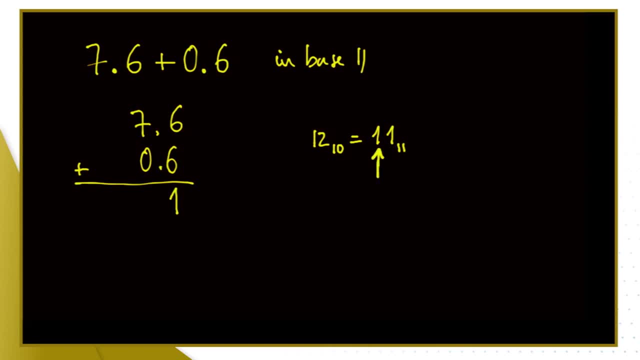 And this other one for the 11 place value is going to go there on top, And I've got 1 plus 7 plus 0. That makes it 8.. 8 is still less than 11.. So it's a number we're allowed to use. 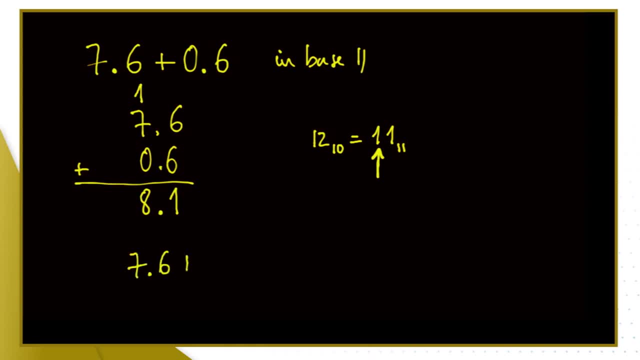 And there we go. The result of the sum is 7.6 plus 0.6 in base 11. It's 8.1 in base 11.. We're going to do subtraction now: Base 5.. 2.3, take away 1.4.. 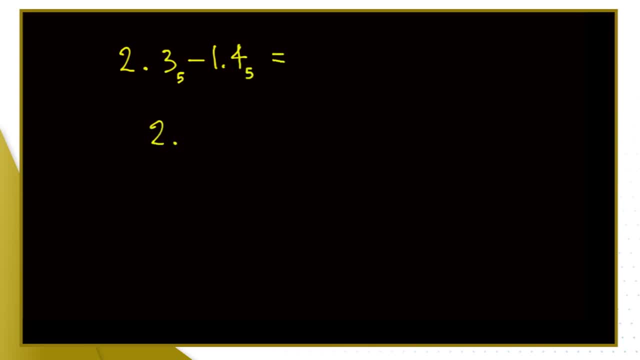 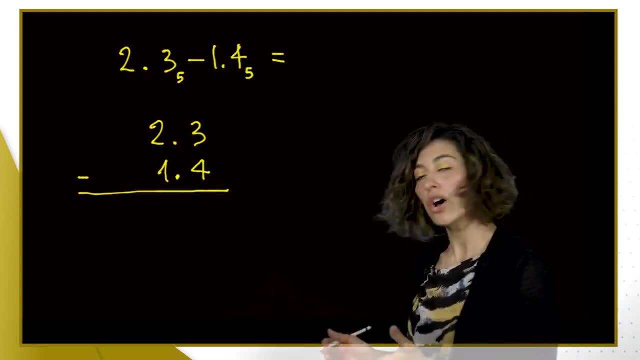 And that's base. 5. Stack the numbers one on top of the other. Place values aligned, We're going to subtract. And now we have, column by column, we've got 3. take away. 4. Too small? We're going to have to borrow. 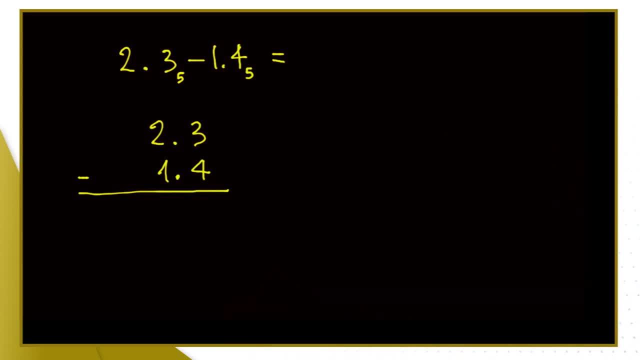 Now, what are we going to borrow? We have a 2.. We're going to split that. That's a 1 plus a 1.. We're going to lend it to the 3.. So I've got a 1.3 over there. 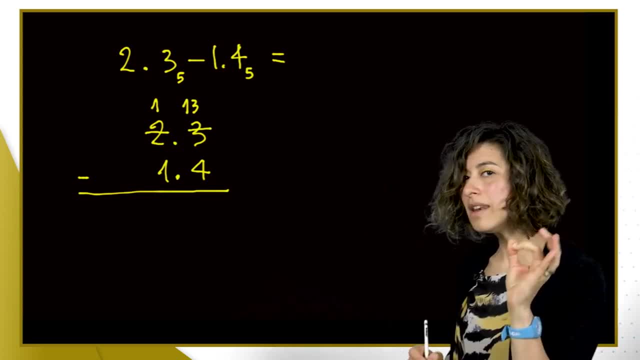 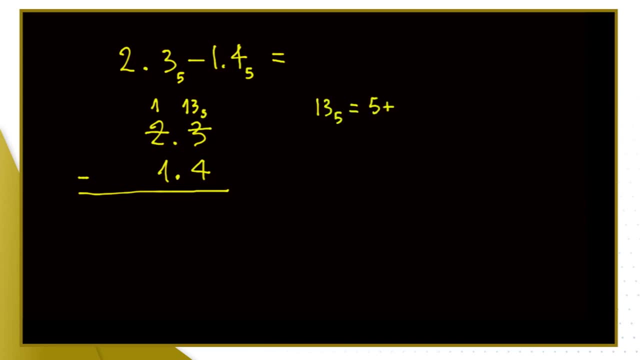 And now I have that 1.3, which is a 1.3 in base 5.. So it's a 1.3 in base 5.. What is that 1.3 in base 5 is 5 plus 3, which is 8.. 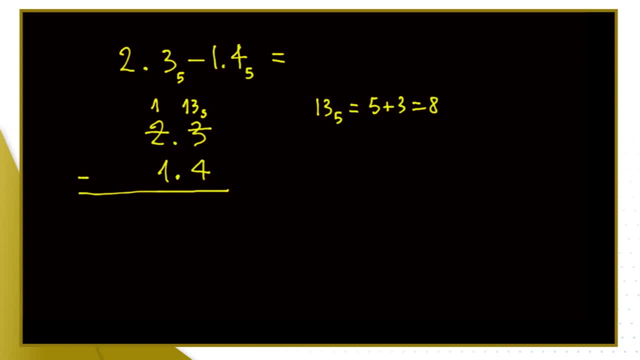 So really I'm doing 8, take away 4, which is 4.. And now the next column: I've got 1, take away 1, which is 0. And so the result is 0.4 in base 5.. 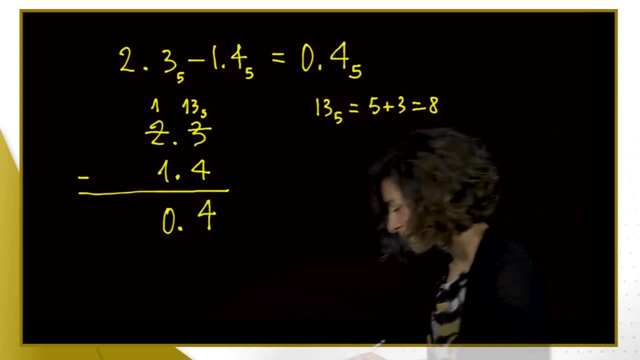 Does that work? We can always check. Let's add them up. If we do 1.4 add 0.4,, what do we get? 4 plus 4 is 8.. But 8 in base 5 is going to have to be written. 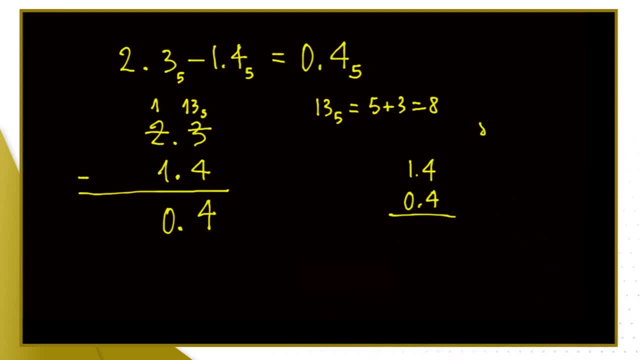 using the help of 5 plus 3.. So 8 is 5 plus 3, like we did earlier, And that means it's going to be a 1 on the place value of 5 and a 3 on the place value of 1.. 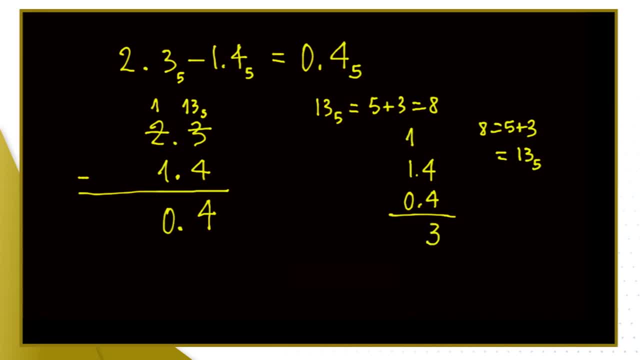 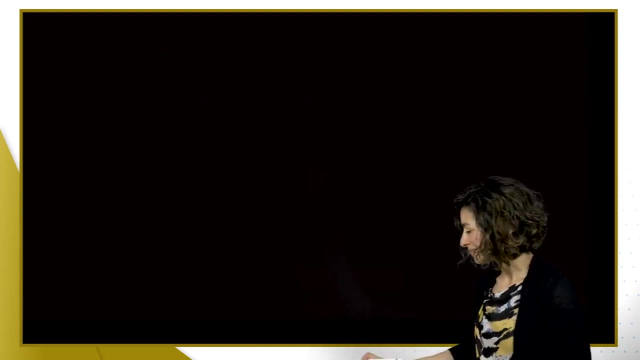 So I write the 3 here and the 1 on top, And now I add the 1 with the 1, which is a 2. And that's correct. Now let's look at one more example: Multiplication in base 7.. 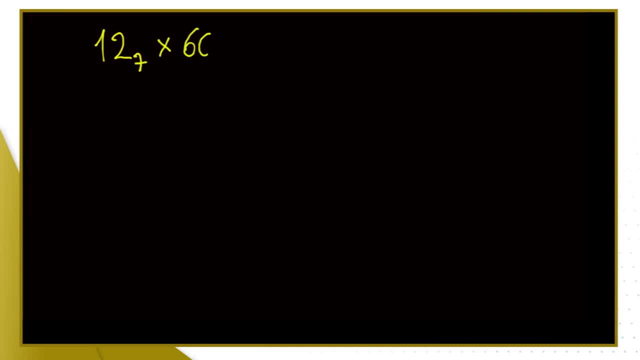 1, 2, base 7, times 6, 0, base 7.. Let's do it: 1, 2, 6, 0.. 0 times 2 is 0.. 0 times 1 is 0.. 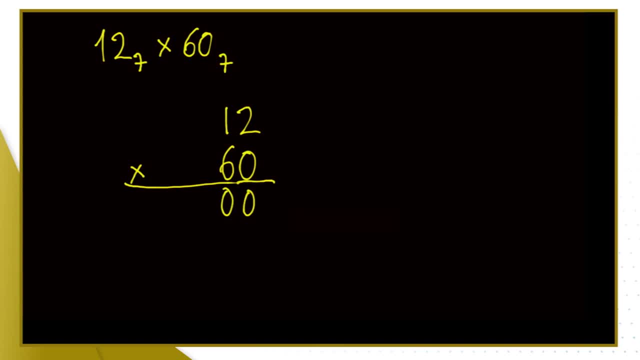 And now, 6 times 2 is 12.. 12, but 12,. what is that in base 7?? Well, let's split the 12.. There's a 7 plus something, So it is 7 plus 5.. 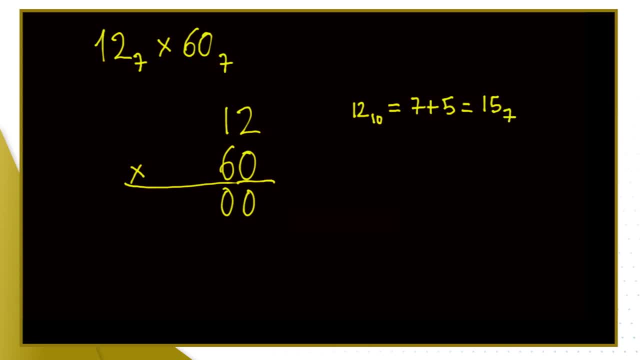 That makes it 1, 5 in base 7. So we do 5 here and the other one over there, And now 6 times 1 is 6.. Put it there And let's add everything up Column by column. 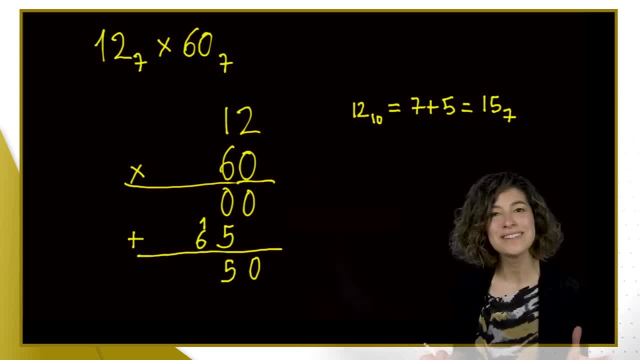 0, 5, and then 1 plus 6 is 7.. But 7 in base 7 is 1, 0. So 1, 0.. Note it down here on the side. 7 is written as 1, 0 in base 7.. 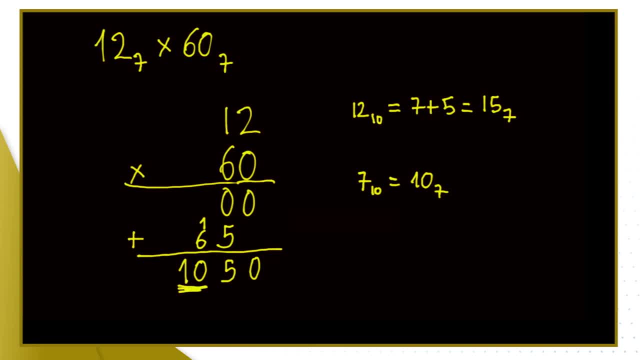 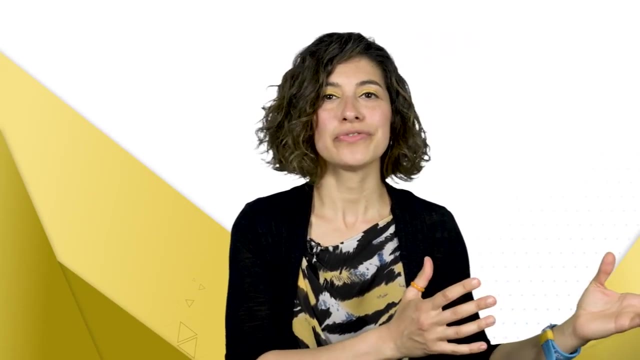 So that's what we did over here And therefore the result is 1, 0, 5, 0 in base 7.. And with these examples and with a little bit of revision of what we've done on all the other bases, 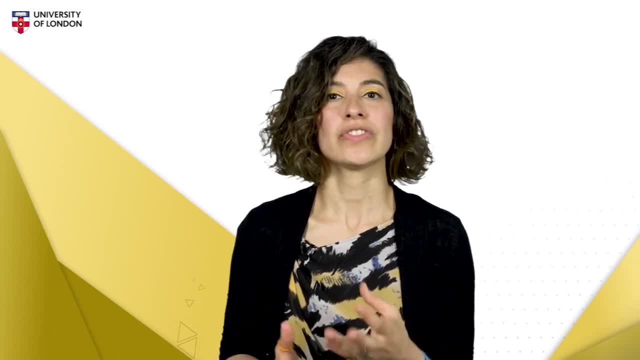 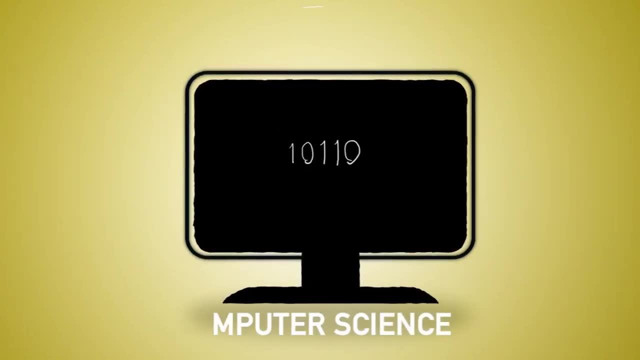 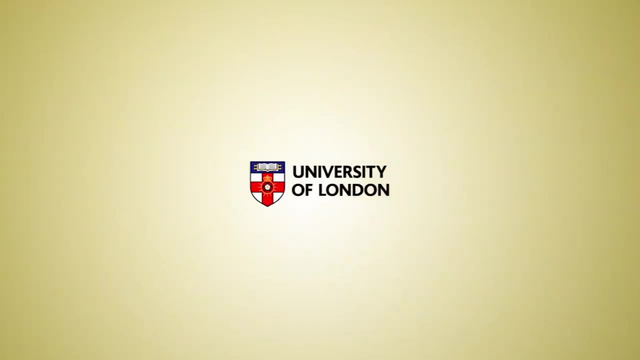 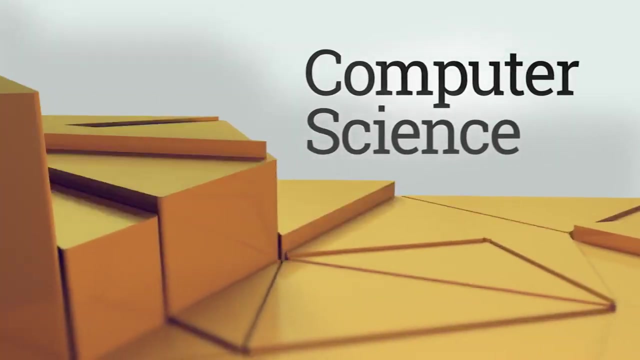 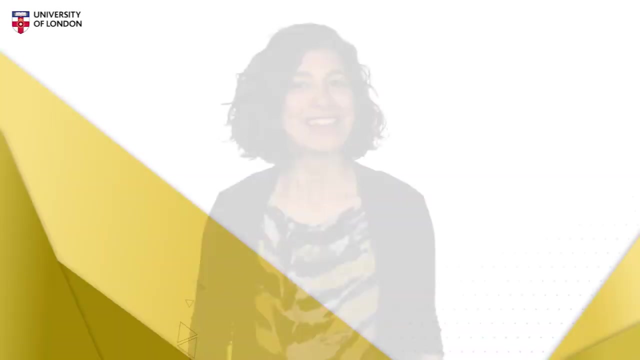 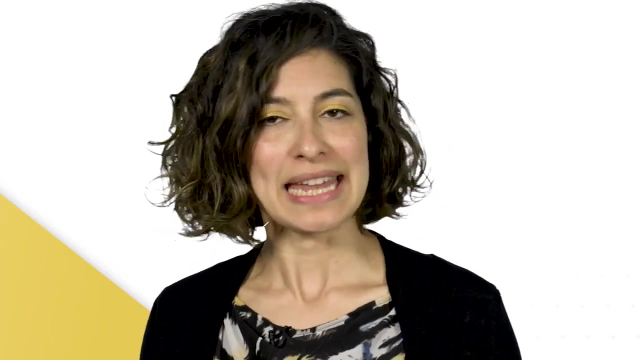 you should be able to perform base translation and operations in any number base. You have all the tools to operate with numbers in any base. You know the algorithms to convert between decimal and any base, Although we did it explicitly for binary, octal and hex. 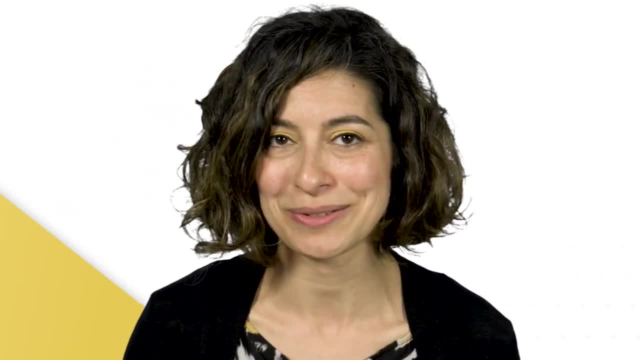 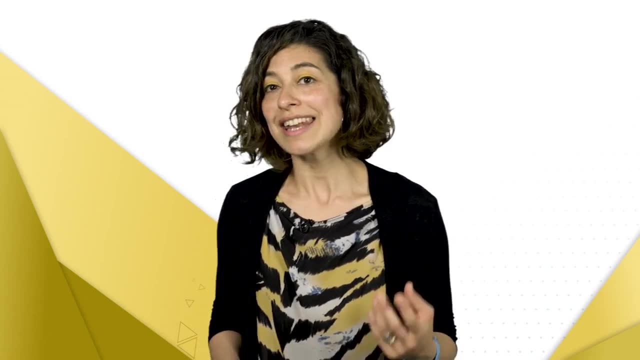 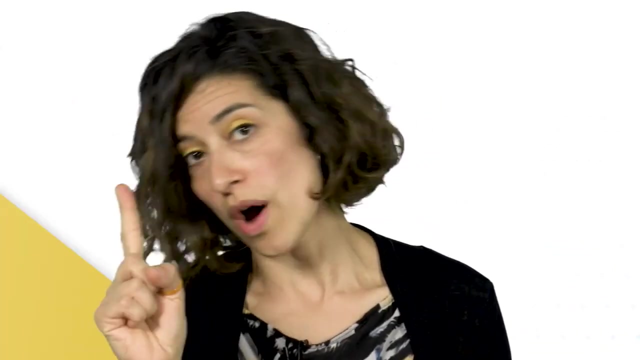 you wrote your own algorithms for any base. We looked at the special relationship binary has with octal and hexadecimal. One octal digit maps to three binary digits. One hexadecimal digit maps to three binary digits. One hexadecimal digit maps to four binary digits. 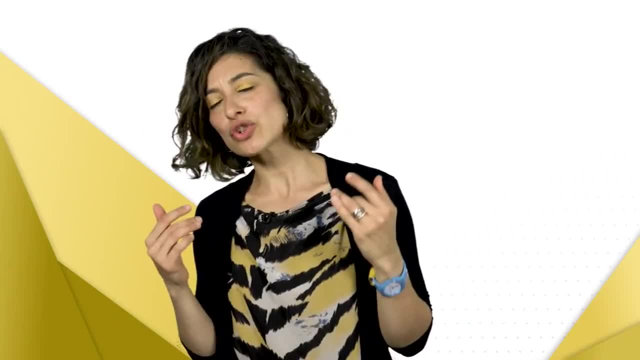 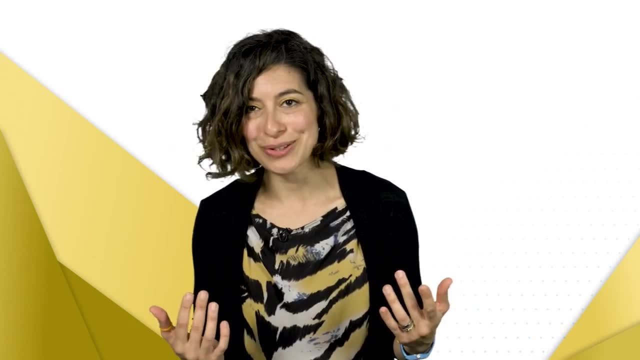 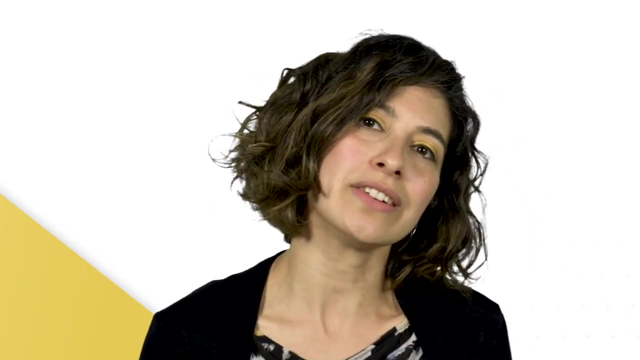 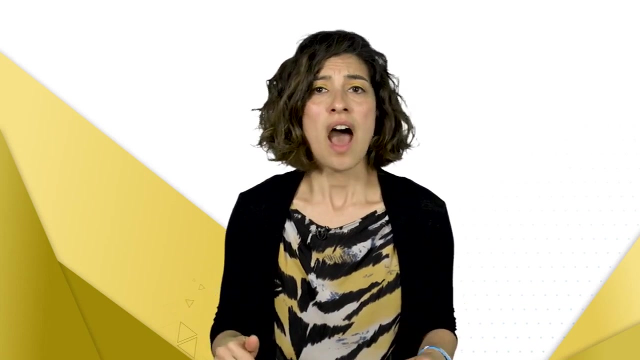 Hexadecimal maps to the way we describe colors, with 24-bit fitting into six hexadecimal place values. Go and find out more about ways of describing color. across the years and as technology advanced, You played with concepts of steganography and exercised the concept of manipulating pixels in an image. 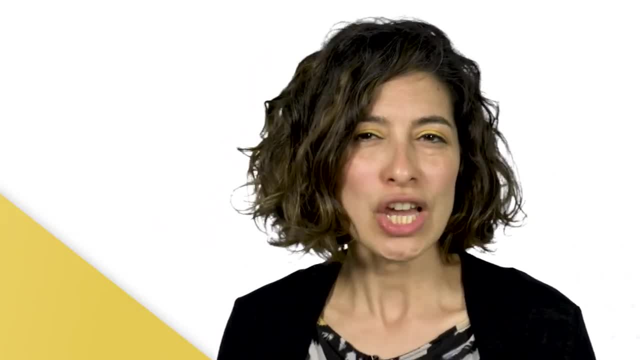 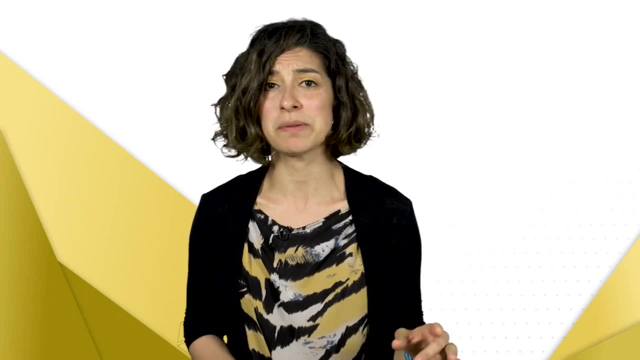 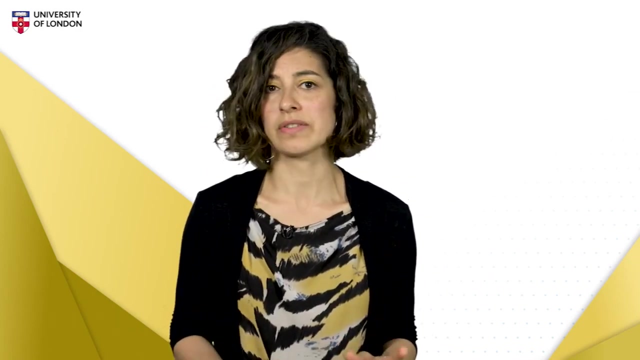 I hope you enjoyed the task and found in it an opportunity to deepening your understanding of numbers and number bases. Some of you have started implementing these ideas and algorithms of these lessons into a programming language, But remember, programming tasks are outside the scope of this module. 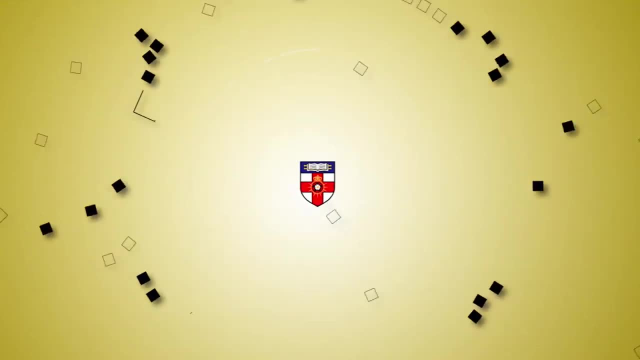 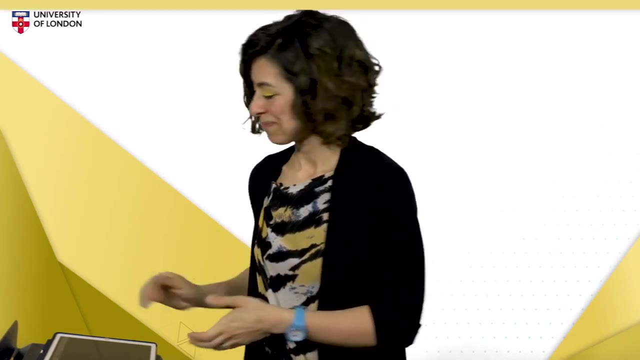 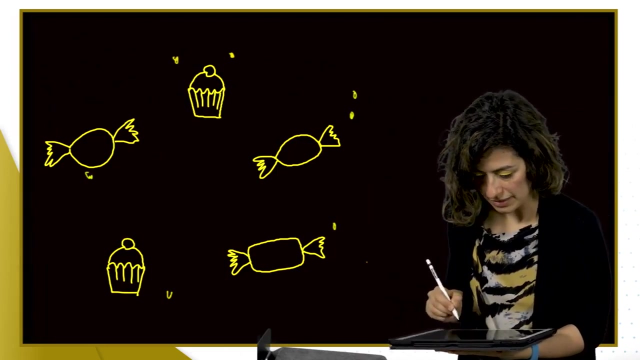 If you have any questions, please feel free to ask them in the comments. Thank you, Which sweet treat shall I have? Eena meena moena, might Baskalora bora bite Hooga booga bow. 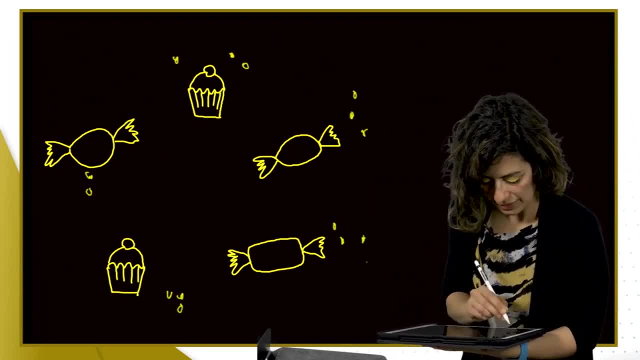 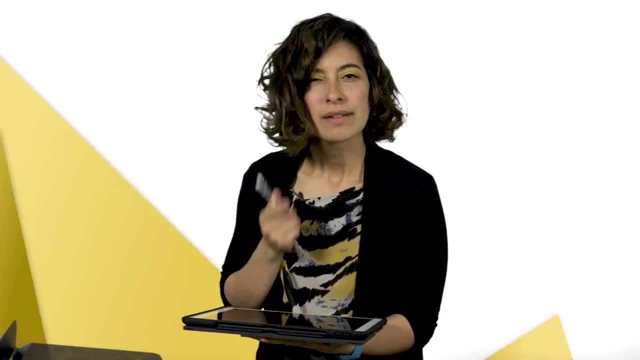 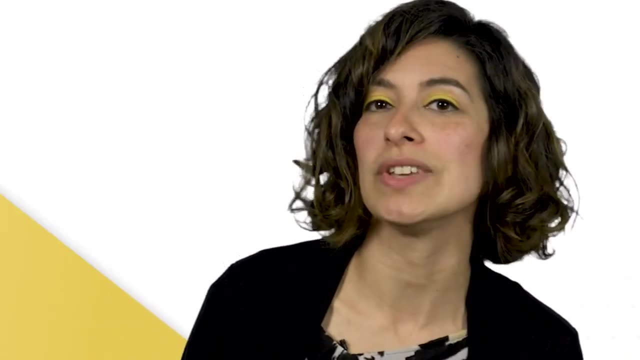 Eggs, butter, cheese, Bread, stick, stock, stone Dead out, Not that one. You probably know your own version of this song. Most cultures have their own selection rhymes of songs. I'm using it to eliminate the sweets one by one. 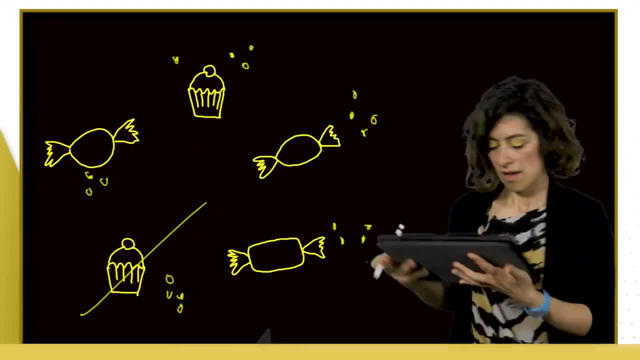 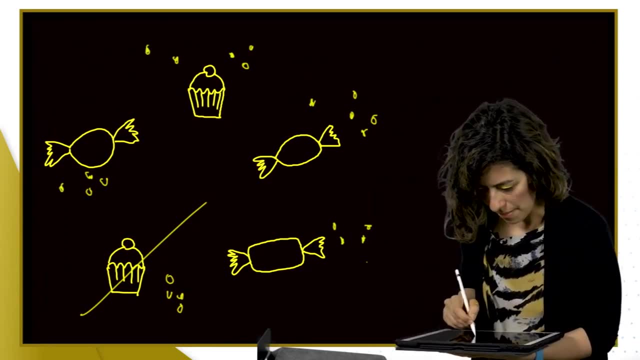 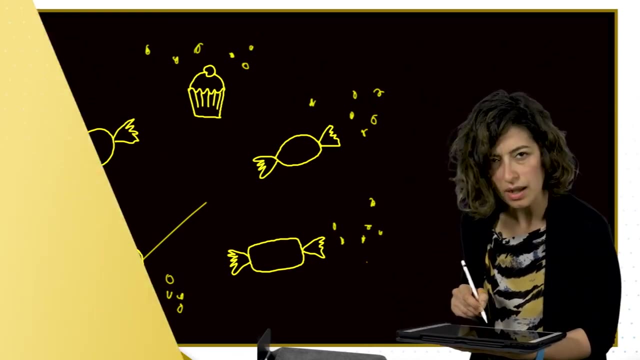 and I'll eat the last one. So I was here. so Eena, meena, moena, might Baskalora bora bite Hooga? Oh, I don't really need to do it this way. 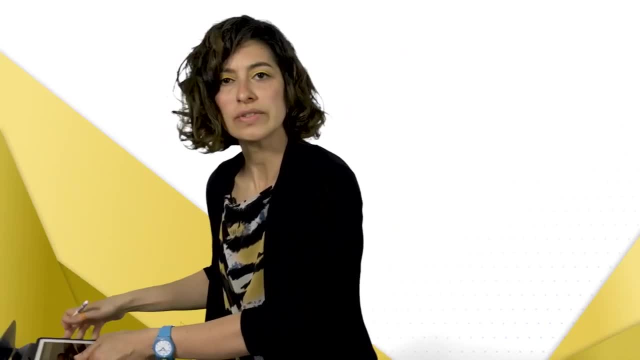 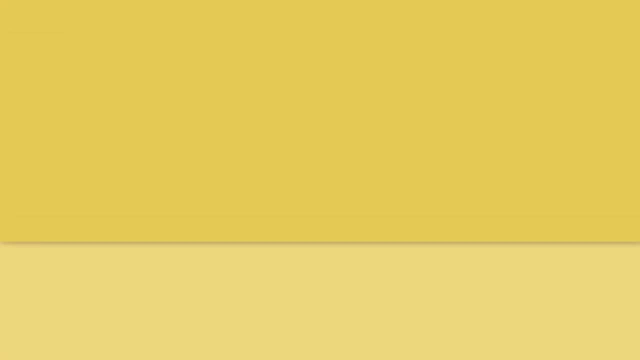 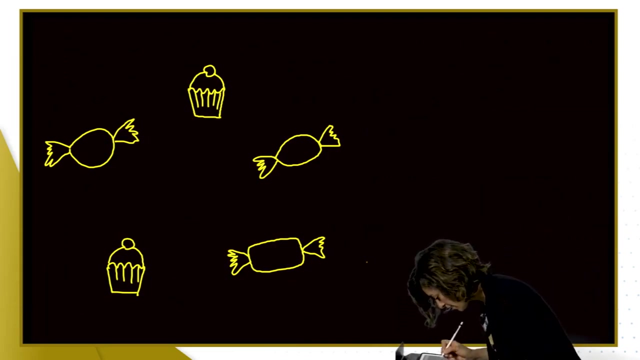 I can just count the sweets, Count the words and see how many times the sweets fit into that length. Let's look at that. There are 19 words in this rhyme, So it goes like this: I start on my cupcake, So I'm going to start here. 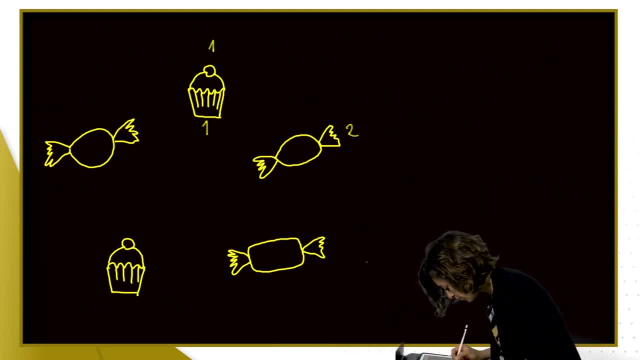 And I count one, two, three, four, five, six, seven, eight, nine, ten, eleven, twelve, thirteen, fourteen, fifteen, sixteen, seventeen, eighteen, nineteen. This one is out, So the fourth sweet is out. 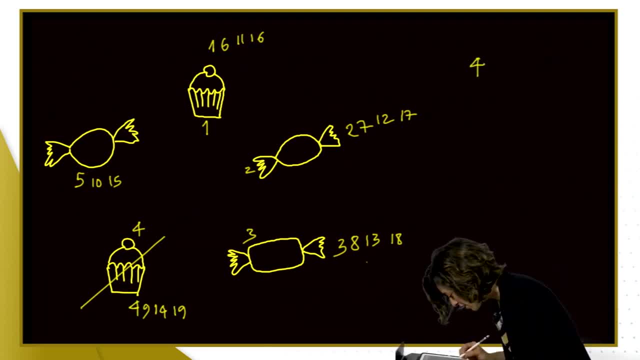 That's the one I eliminate, And then I'm going to start from the fifth. sweet So start. So this is, four is out. I start from the fifth, And now I go: one, two, three, four, five, six. 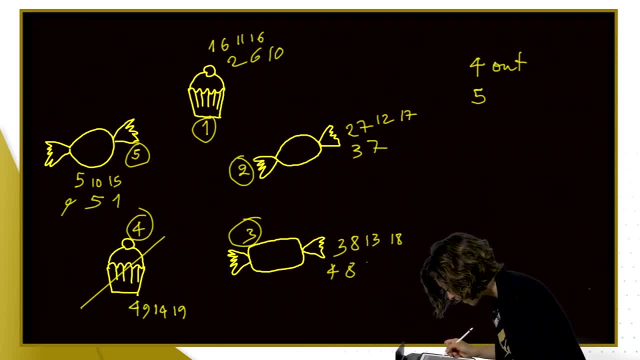 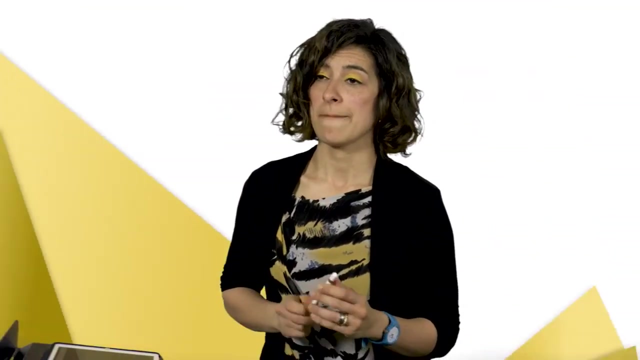 seven, eight, nine, ten, eleven, twelve, thirteen, fourteen, fifteen, sixteen, seventeen, eighteen, nineteen. So okay, this is out. So the two is out And I would start again on the third. sweet, That's going to take a long time. 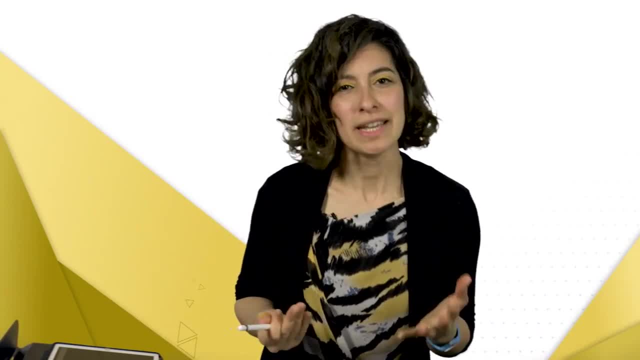 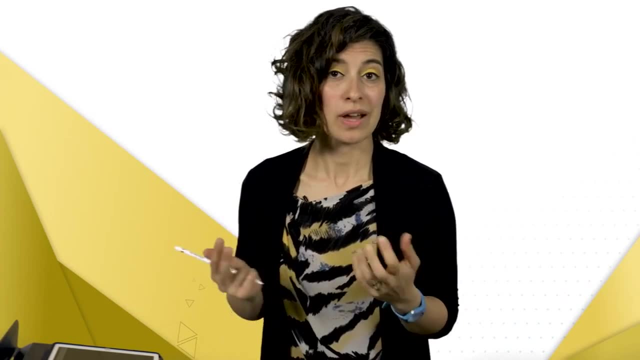 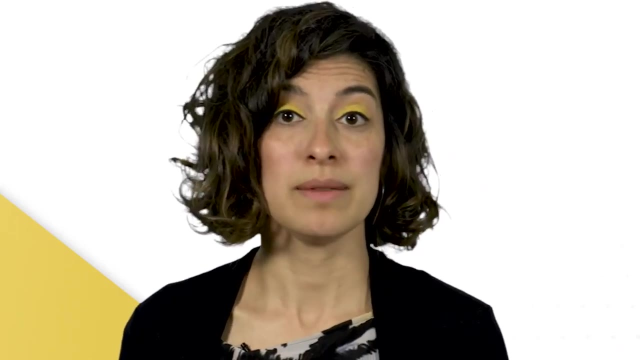 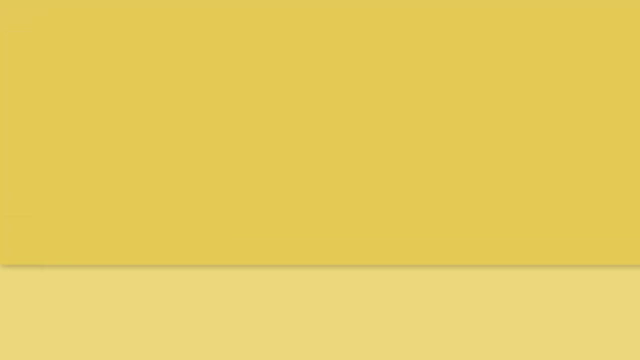 We can do better than that, Because really we're wrapping around the number nineteen around the number of sweets, Around five sweets. So that means that nineteen covers the five sweets three times, And then there's four more words to use, So the fourth, chocolate is out. 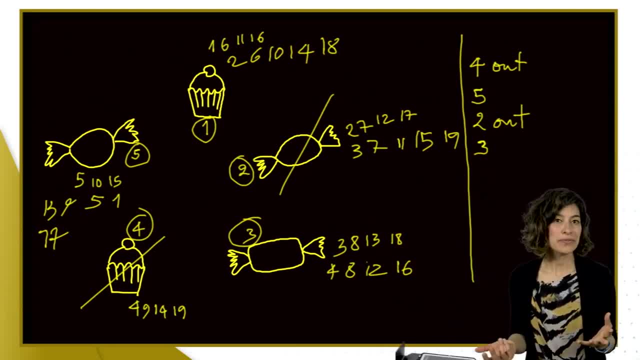 Yes, that's what we got. And then I start counting on the fifth, And I've got four chocolates to count over. Nineteen covers it four times, That's sixteen, And then there's three more words left. So the third chocolate after the fifth. 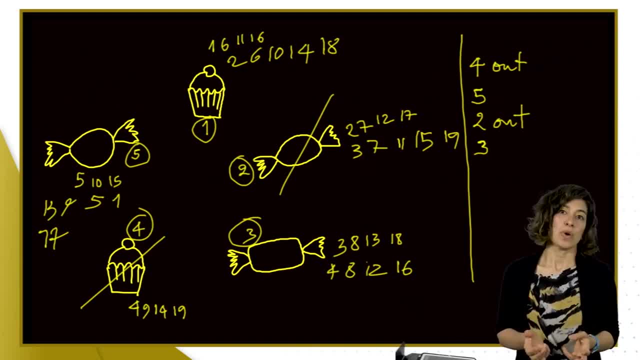 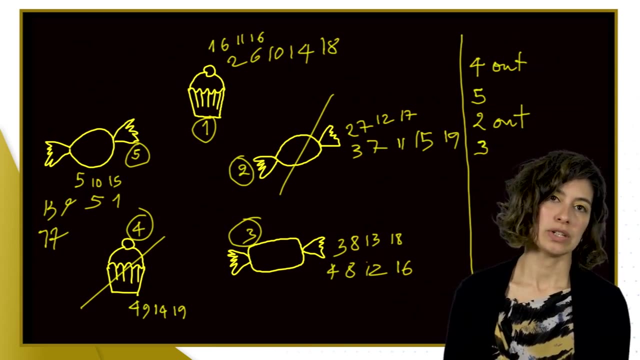 which is a third. that is number two, And that is out. Then I've got three chocolates left. I start on the third chocolate. Nineteen covers it six times. That makes eighteen, And then there's one word left, So the third chocolate is out. 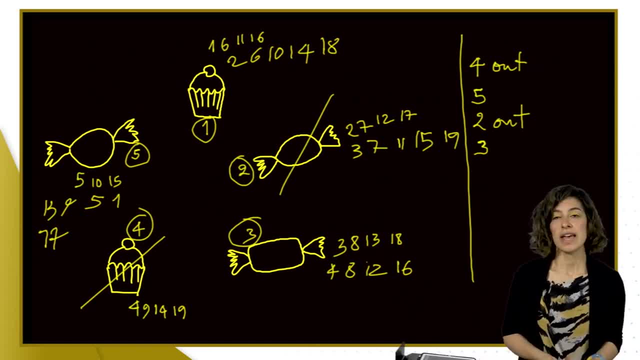 Then I'll do it again. I have two chocolates left. I start on the fifth And then I'll just go even and odd, even and odd, alternating between the fifth and the first, And the fifth is out, So I will eat the first sweet first. 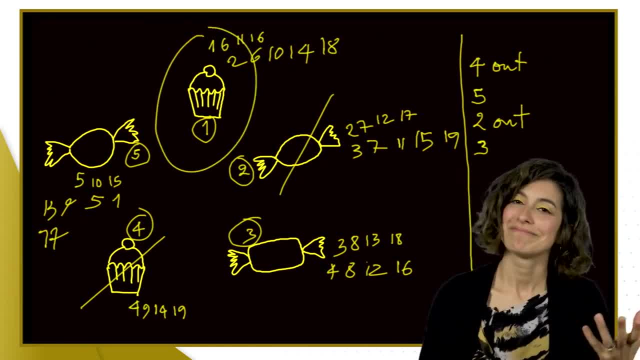 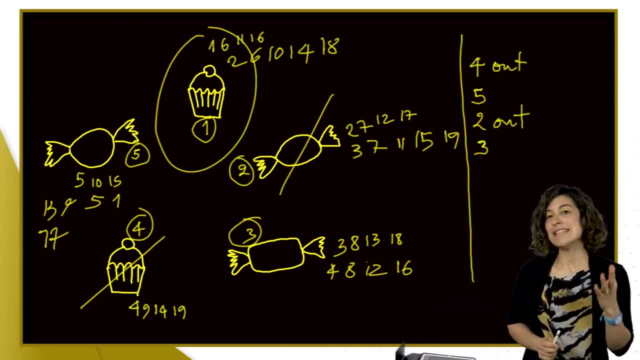 I'll eat my cupcake first. You can do it yourself with your treats And check my maths. So we really didn't need to do the counting around every time. What we needed was the remainder of the division of nineteen by how many sweets were left on the table. 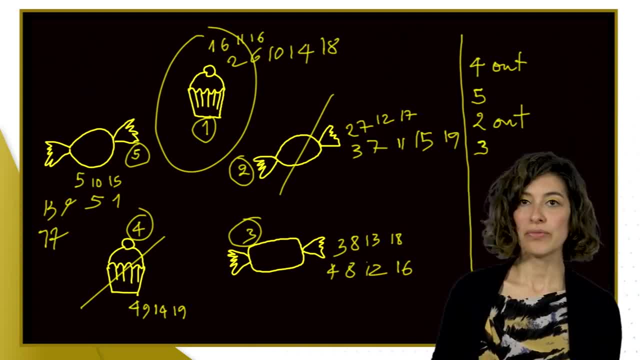 So nineteen divided by five is three, With the remainder four. So the fourth chocolate is out And I start on the fifth. So I've got the fifth, the first, the second and the third available. Then, starting on the fifth, I do nineteen divided by four. 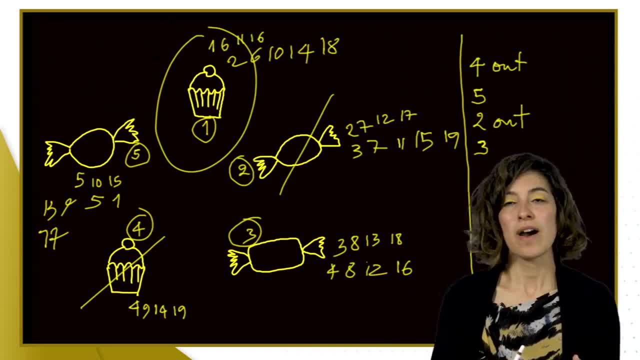 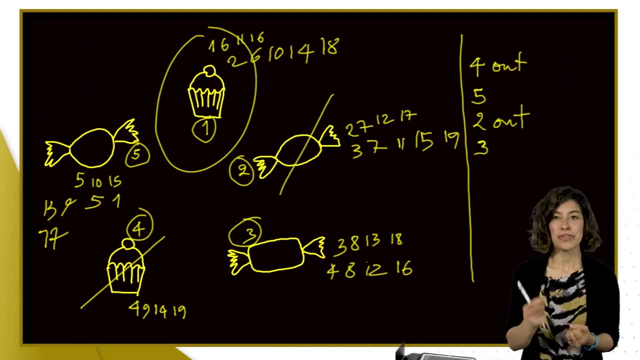 which is four, remainder three, And from five, one, two. the second is out. Then I start on the third chocolate, And I have the third, the fifth and the first. So nineteen divided by three is six with the remainder one. 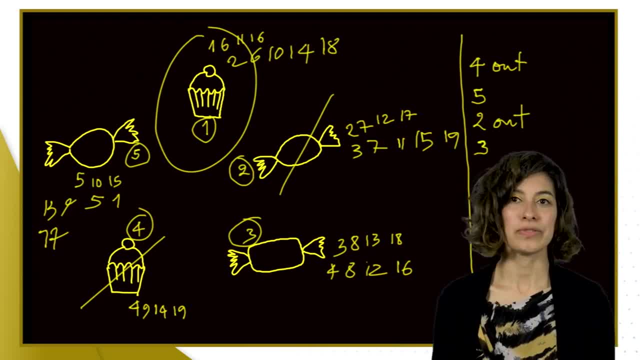 So the third chocolate is out. Then I start on the fifth chocolate. I've got the fifth and the first. Nineteen divided by two is nine with the remainder one. So the fifth chocolate is out, And so I will eat the first. 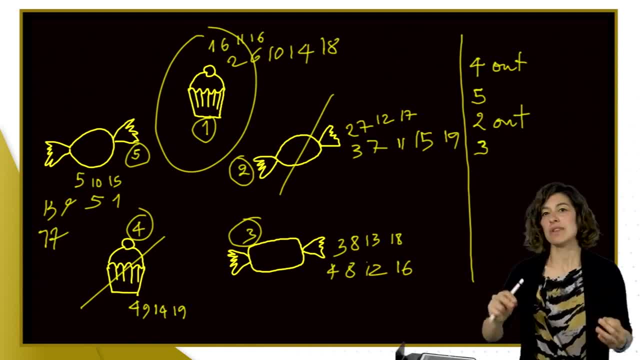 All we needed were the remainders. This wrapping around numbers and requiring only remainders of division is the core of what we do in modular arithmetic. You and I use it every day to work with hours and minutes and seconds. You see, twenty minutes after 1.56 pm. 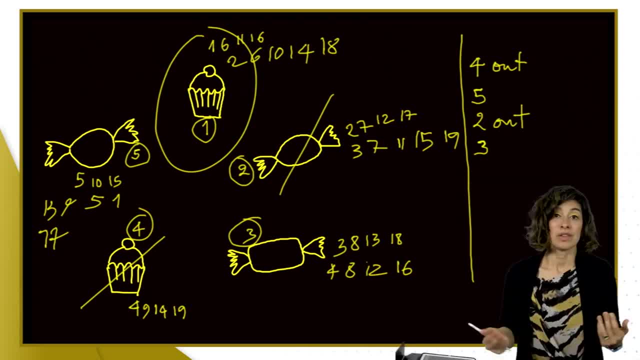 it's 2.16 pm, You add 56 minutes with 20 minutes, That makes 76 minutes And then you take away the 60 minutes, giving you 16 minutes past the hour And then that extra 60 minutes. 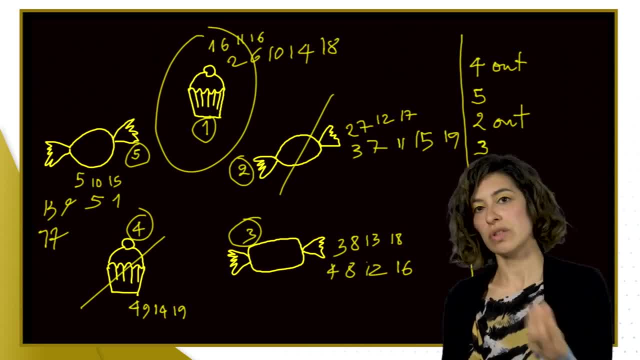 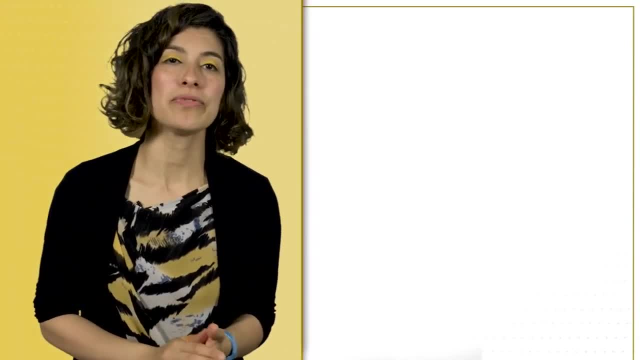 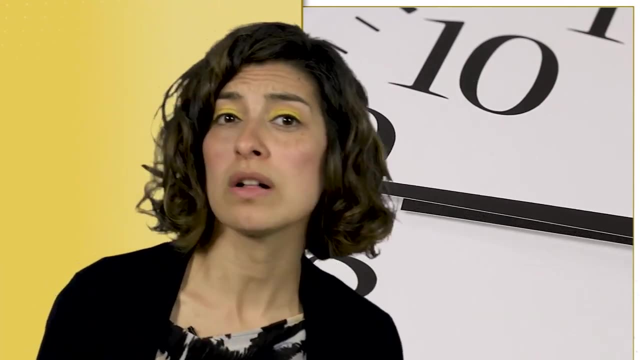 you convert into one more hour, So you add one to the 1 pm, making it 2.16 pm. Modular arithmetic is often referred to as clock arithmetic, But instead of working always with 60 minutes of 12-hour clock faces, 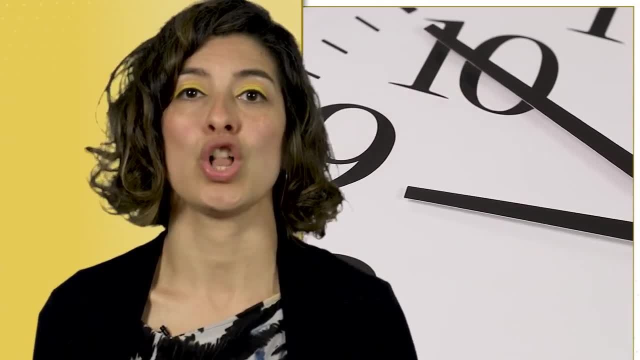 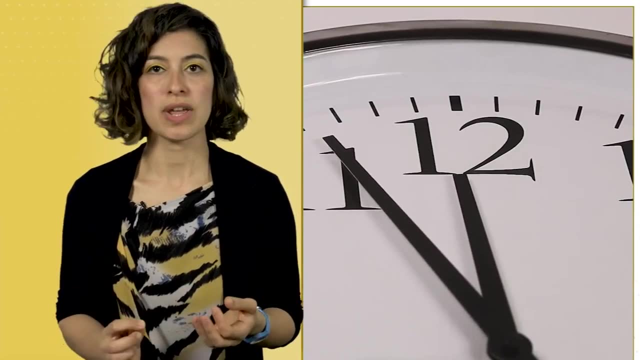 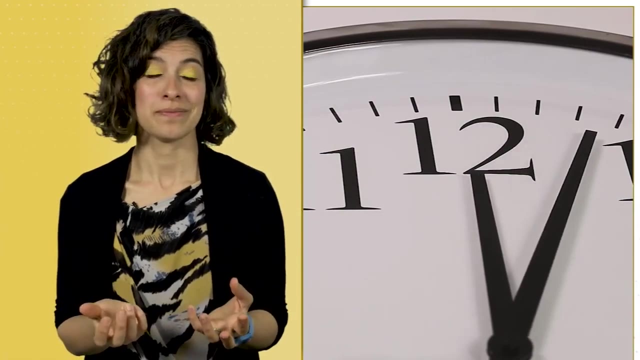 we work with the size of the clock we need for each problem With the chocolates we did: 19 divided by five equals three with remainder four. So here we were working with a clock face with five hours When we did clock arithmetic. 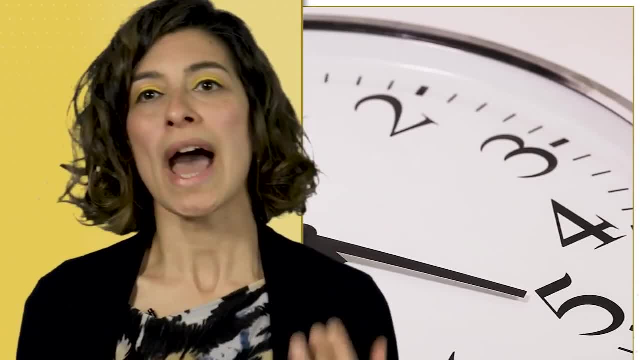 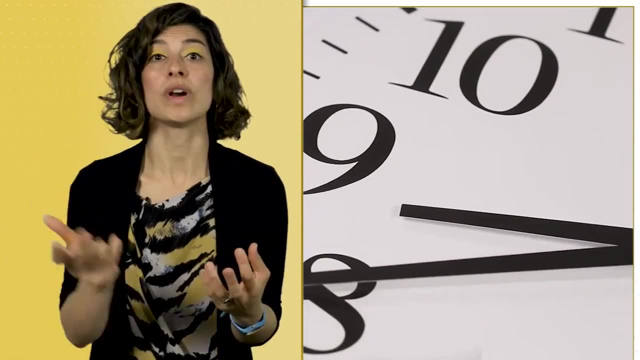 19 divided by four equals four, with remainder three. we actually want a clock face with four hours. 19 divided by three, which was 16, with remainder one. we were working on a clock face with three hours And 19 divided by two. 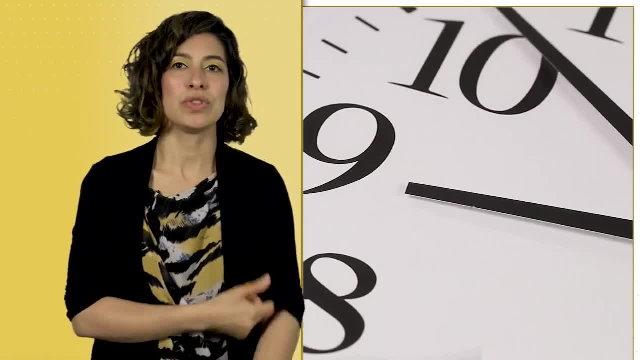 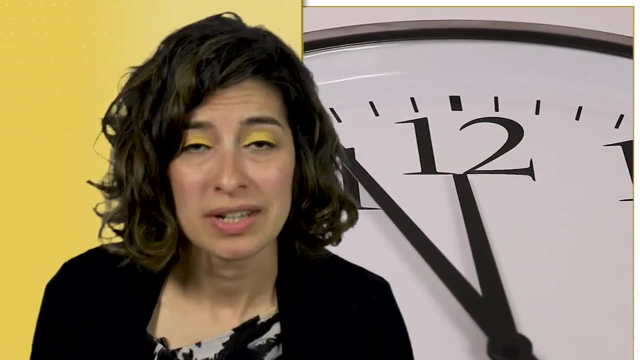 which is nine, with remainder one. we actually want a clock face with two hours. Well, the two-hour clock just highlights if the number we were working is even or odd. Like in binary, odd numbers end with a one and even numbers end with a zero. 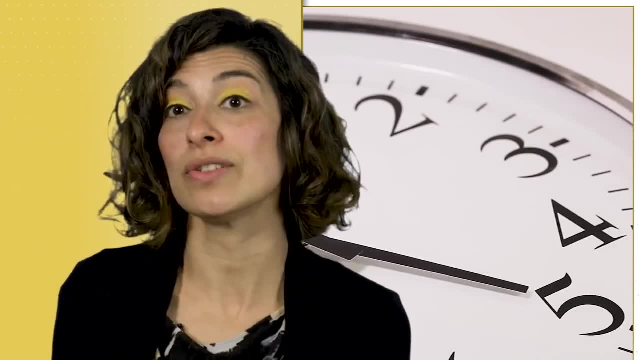 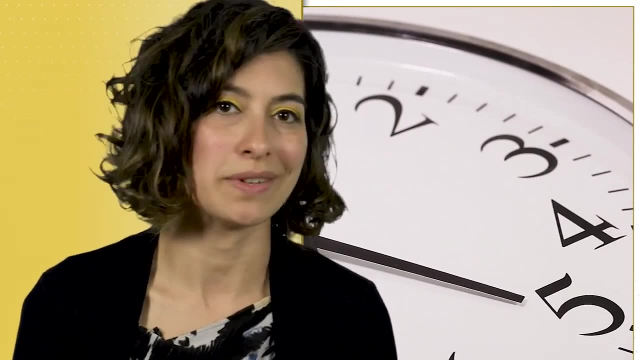 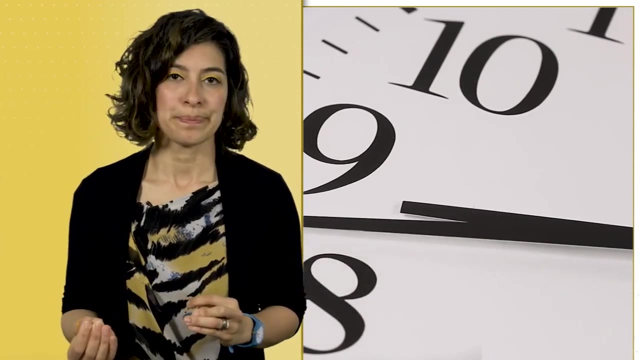 What's cool about this concept of working with remainders of division is that the rules of arithmetic are very similar to the ones with common numbers. What I mean is that 45 divided by four leaves remainder one, And that's because four times 11 is 44,. 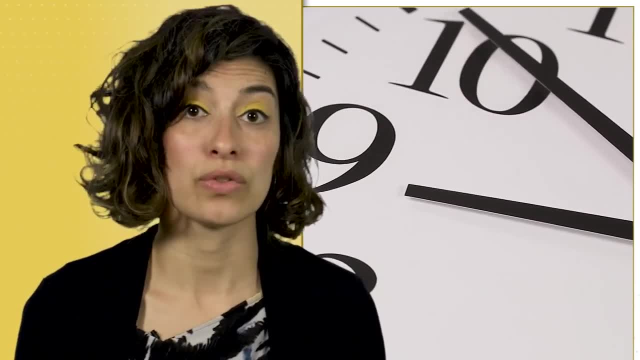 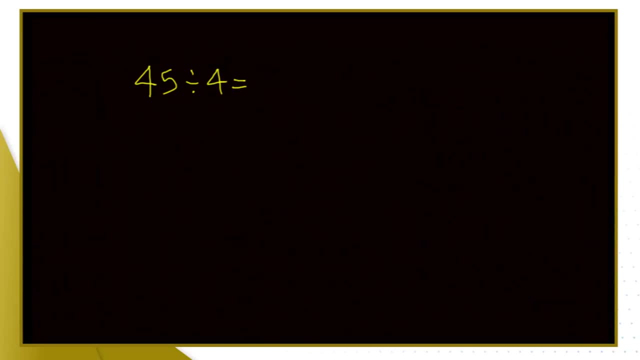 and that's the highest multiple of four fitting into 45. So the remainder is one. So 45 divided by four leaves remainder one, And 18 divided by four- I'm ignoring the integer part, for now- leaves remainder two, because four times four is 16,. 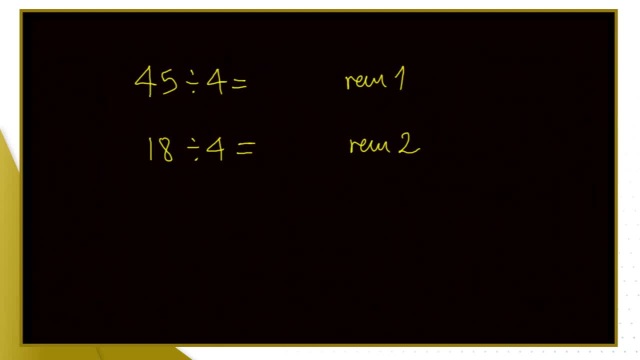 and then 16 to 18 is two, So that's remainder two. Now the cool thing about the rules of arithmetic here is that if I add 45 with 18, the remainder of that sum, when divided by four, is the same as adding. 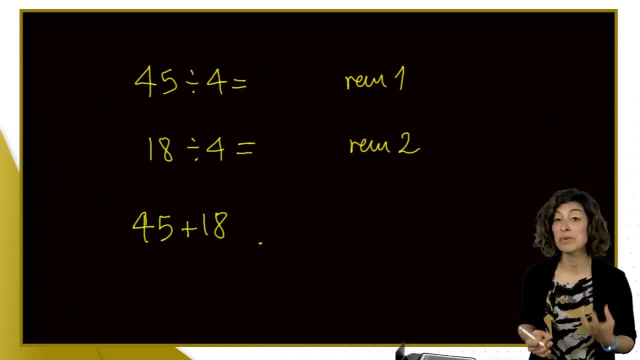 the remainder one and the remainder two. So it's going to be remainder three. So I don't need to add the numbers up, do the division by four and work out the remainder. I can just say: well, it's going to be the remainder. 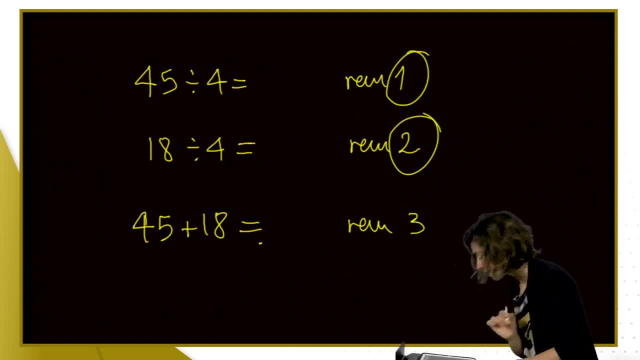 one from here plus two from there. I can add up the remainders, And that is one of the key properties we're going to tap into Now. this also works for multiplications. So 45 times 18,, 45 times 18,. 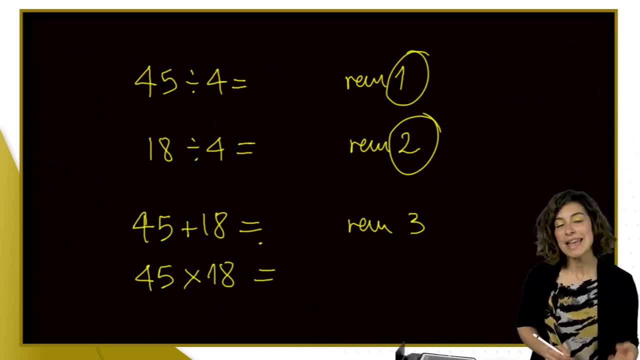 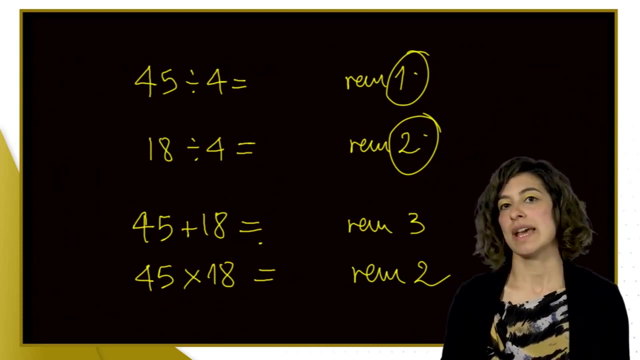 the remainder of division by four is the multiplication of the two remainders, So one times two. So the remainder is going to be two. Check for yourself. That means that if we are only interested in remainders, then we can work out remainders of smaller numbers. 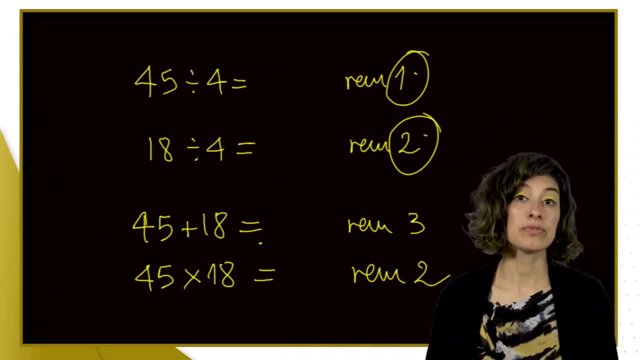 and then add, subtract and multiply remainders, provided we are working in the same size of clock. We're going to call that the modulus. Sometimes I call it mod. Now, this property does not extend to division, It is only for addition. 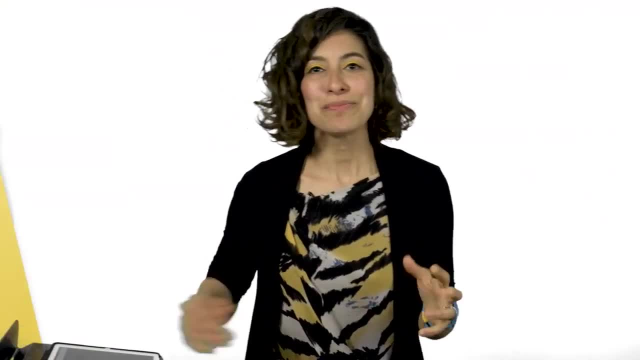 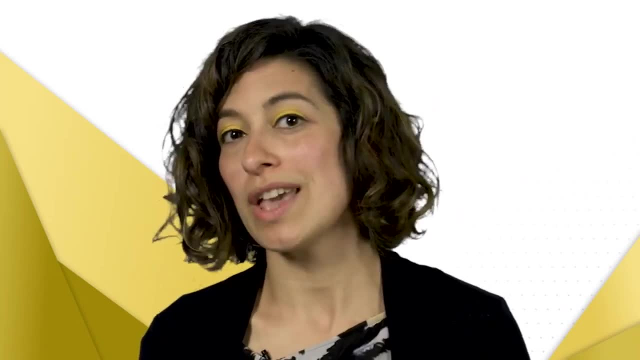 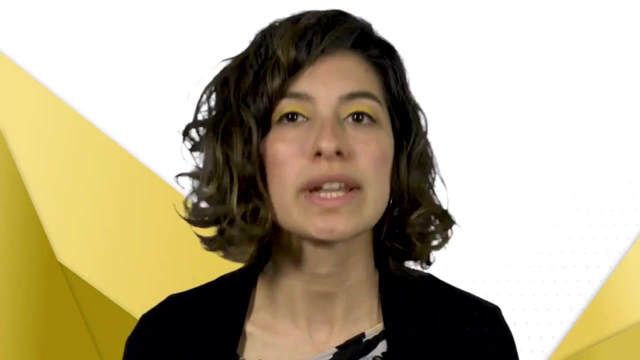 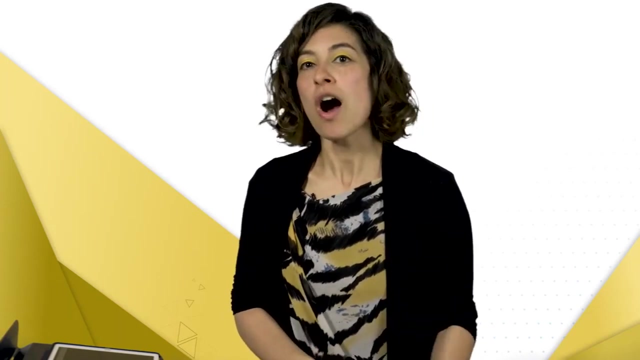 subtraction and multiplication From the first examples with suites, the pattern of numbers we keep eliminating looks random. One way of generating pseudo-random numbers for computing purposes employs modular arithmetic working with remainders. And one incredible use of modular arithmetic is the strongest form of encryption. 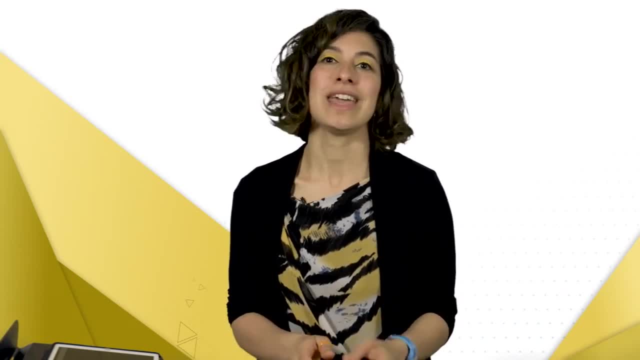 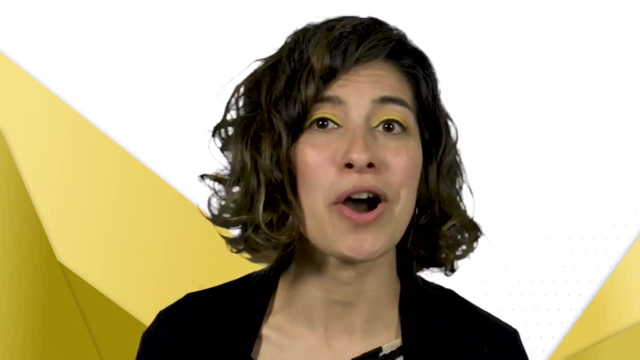 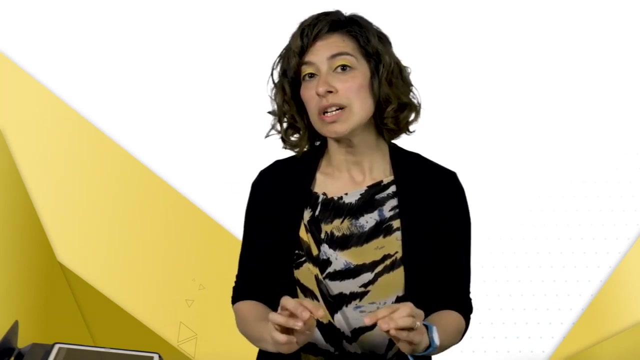 using classical computing, the RSA encryption that relies both on large prime numbers and modular arithmetic. RSA stands for the name of the mathematicians that developed it: Rivest, Shamir and Adelman. In this lesson, you will learn how to work. 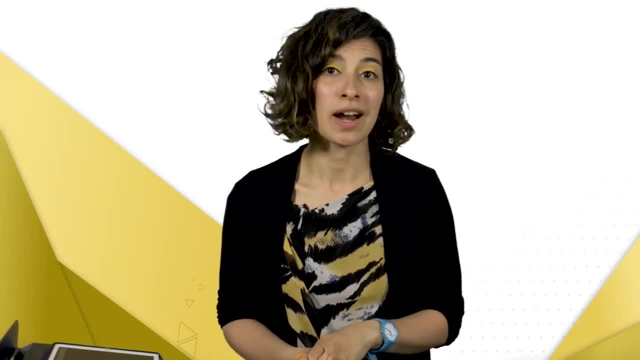 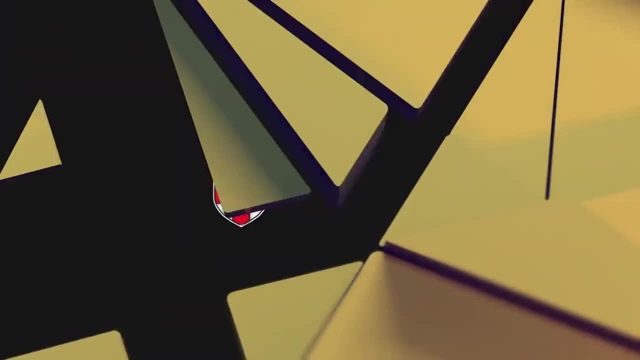 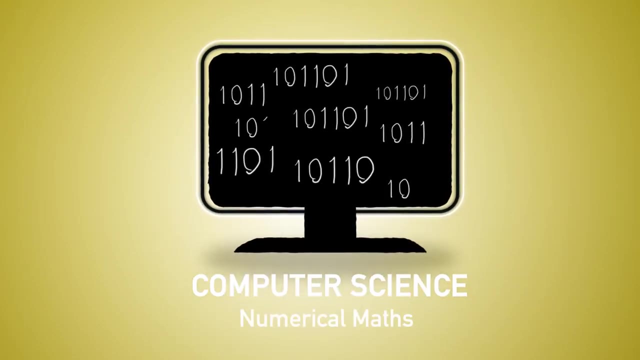 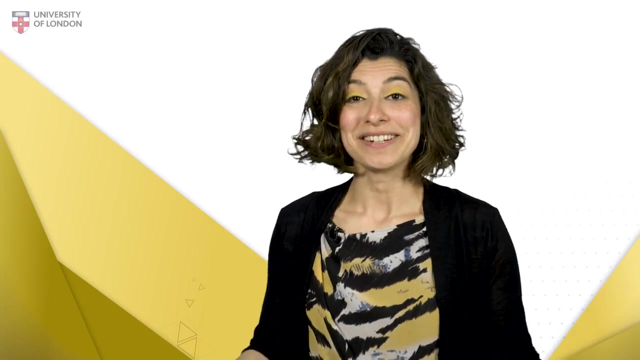 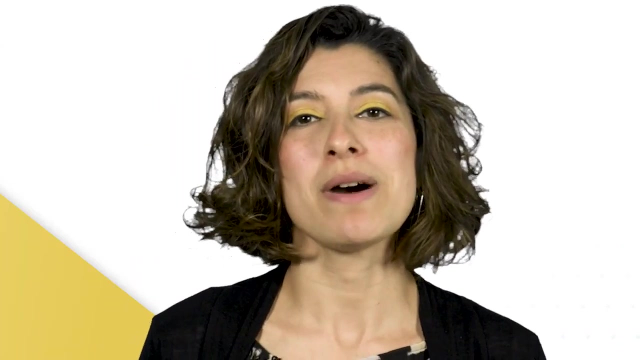 on encrypting and decrypting messages using the RSA algorithm. banking on modular arithmetic. Get ready for this adventure. Hi there. Let's look at more detail how to actually compute in modular arithmetic. The main thing to bear in mind is that we are working. 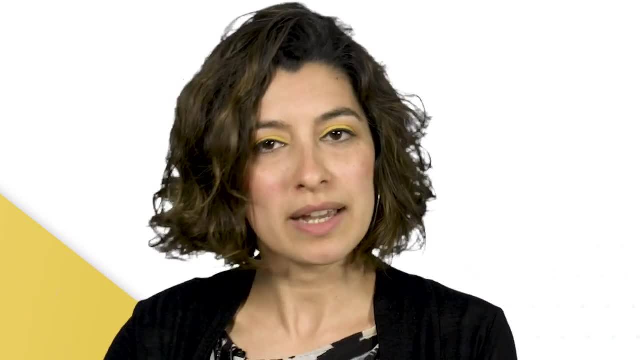 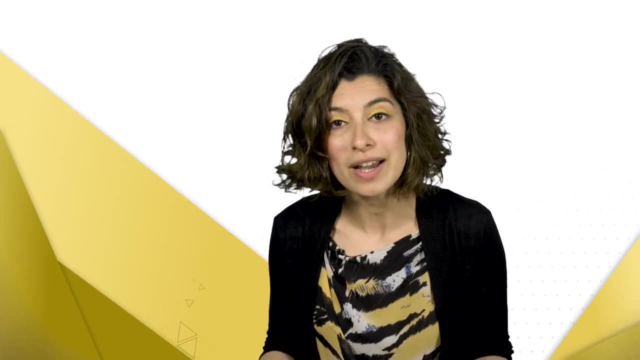 with the remainders of division by the number that is written after the mod. So when we work in mod 5, we are working with the remainders of division by 5.. Actually, the remainders can only be 0,, 1,, 2,, 3, or 4.. 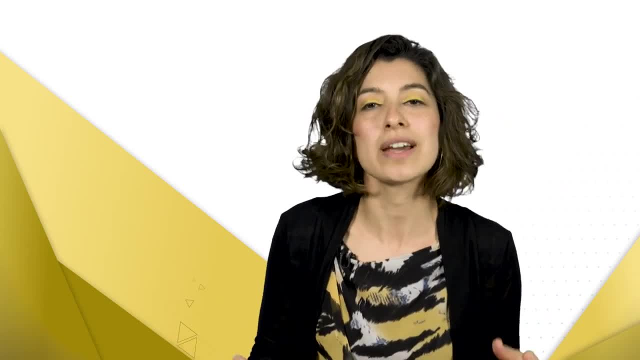 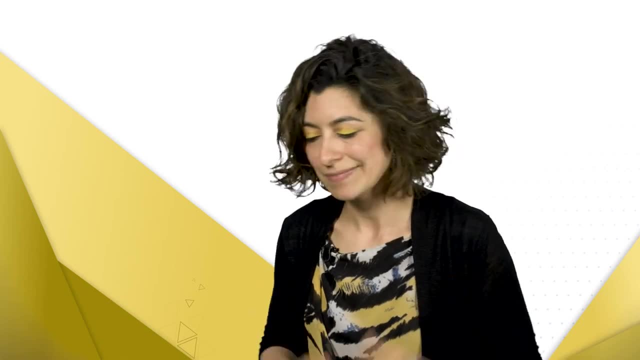 There's only 5 options. So every time we're working in mod 5, we're really boiling down every number to either 0,, 1,, 2,, 3, or 4.. I'm talking about 23.. I want to work out. 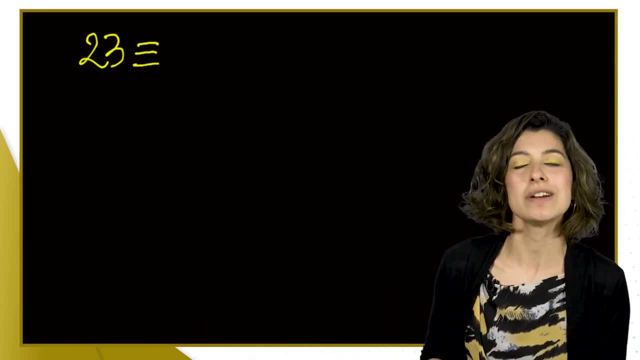 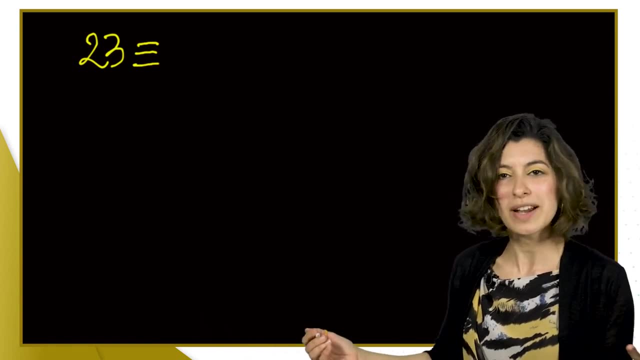 what is the smallest positive number that is congruent with 23 mod 5.. I'm actually saying: what's the remainder of 23 when divided by 5? That's really what I'm asking. Okay, So we want to work out what that guy here is. 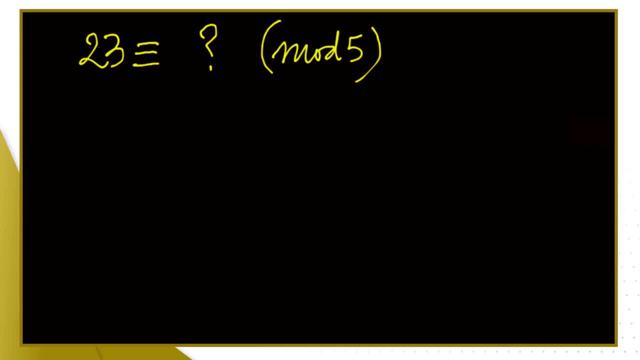 The way to do that. we do the division of 23 by 5. And we know that 23, the largest multiple of 5 that fits in 23 is 20.. So really we'll be doing: 23 is 20 plus some extra bit. 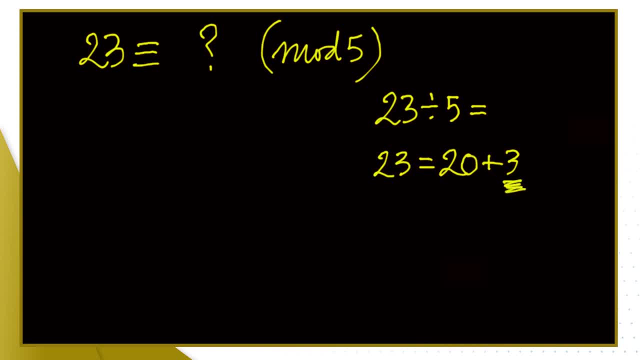 that it's a 3.. So 3 is that remainder. Now how do we do that? from the division itself? Well, 20 is 4 times 5.. So I've got 4 is the integer part of my division. 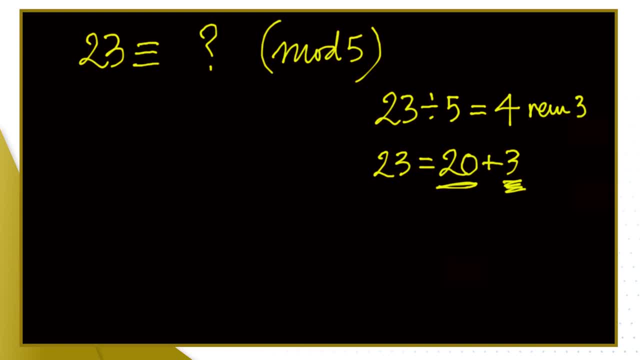 And then I've got my remainder 3.. So the answer to this is: 23 is congruent with 3 mod 5.. It sounds like I'm kind of complicating it by writing down all these expressions, But this is the meat and bones. 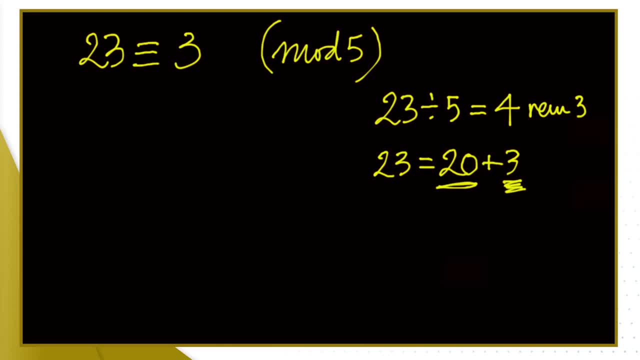 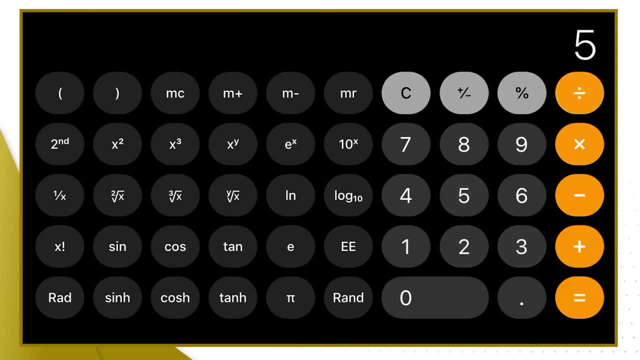 of what you've got to do every time you work with numbers in mod 5.. I'll show you in the calculator. So I'll write 23 divided by 5.. That gives you 4.6.. None of those numbers is the remainder. 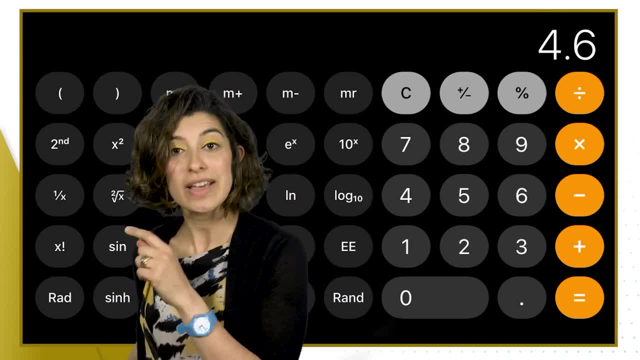 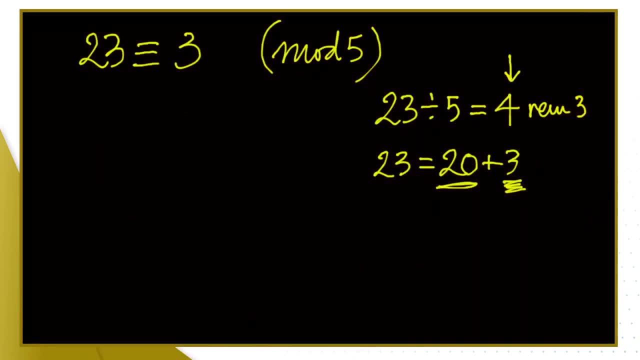 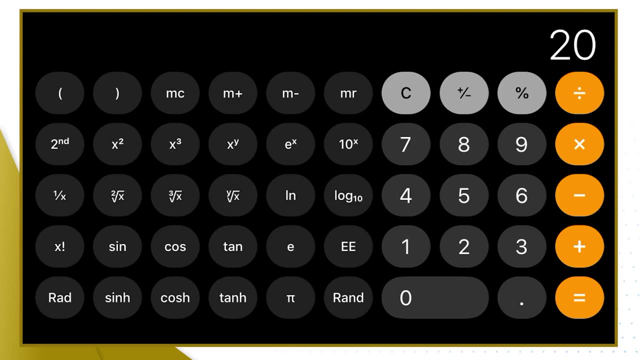 4 is the integer part of the division, as I had written on the board before. I'll show you again. OK, that's a 4 there, And now on the calculator I would do 4 times 5, which is the mod, which is 20.. 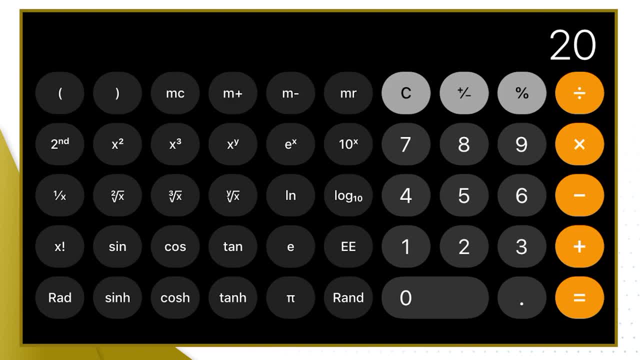 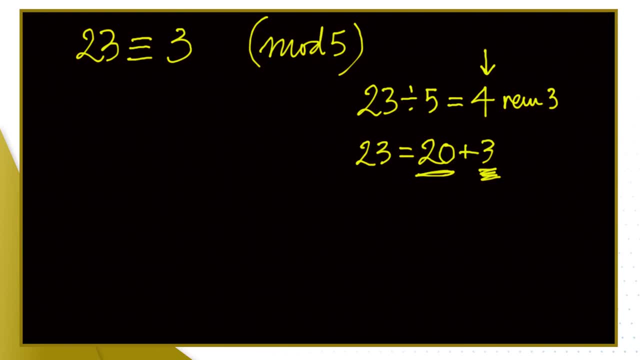 And then I'll do 23, take away 20, which is 3.. OK, so done. Now, on the back of this, I can get for free pretty much what. 28 is congruent with mod 5. So 28.. 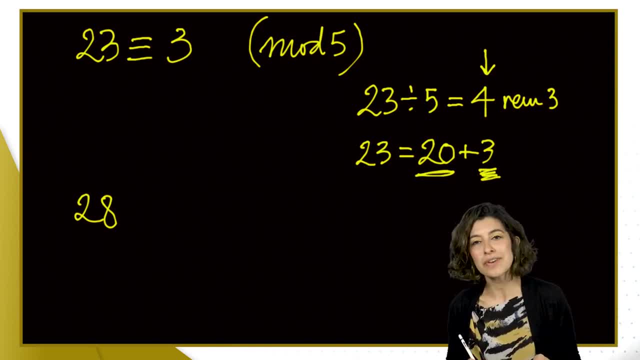 28 is just one more multiple of 5 away from 23.. So it's got the same remainder when divided by 5.. What I mean is that 28 is 23 add 5.. So really it's going to have the same. 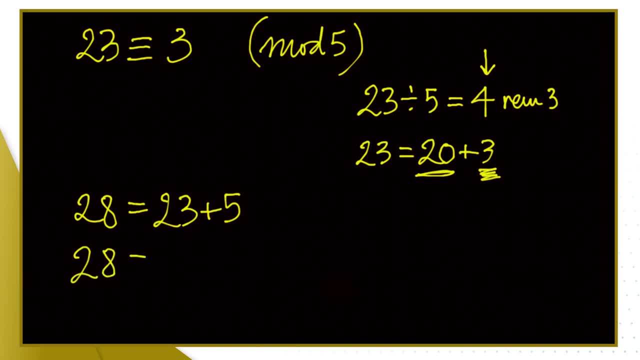 remainder when divided. So 28 is congruent with 23,, which is congruent with 3 mod 5.. And you can check that, You can sort out yourself by doing the calculation by writing 28 divided by 5.. Well really, 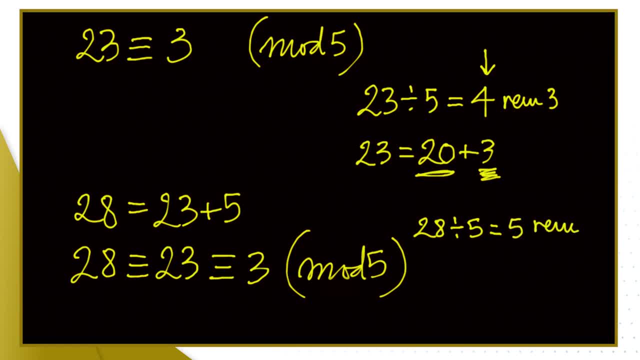 it's going to be 5 and some remainder, because 25 fits into 28.. And then you do 28. take away the 25, which is 3,, as we said, And job done. What about larger numbers? Can we bank on this idea? 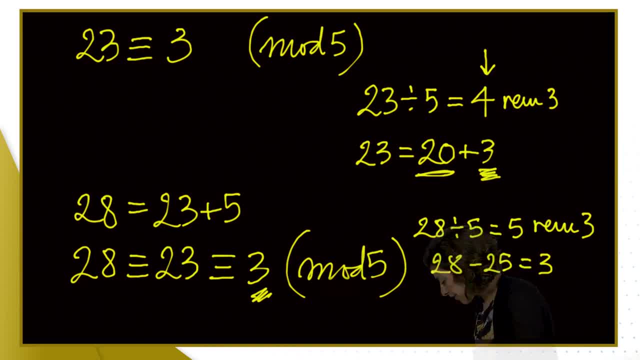 for larger numbers? Of course we do, If I had instead 128.. 128 is 100 on top of the 28. And 100 is itself a multiple of 5. So that's not going to change the remainder of the division. 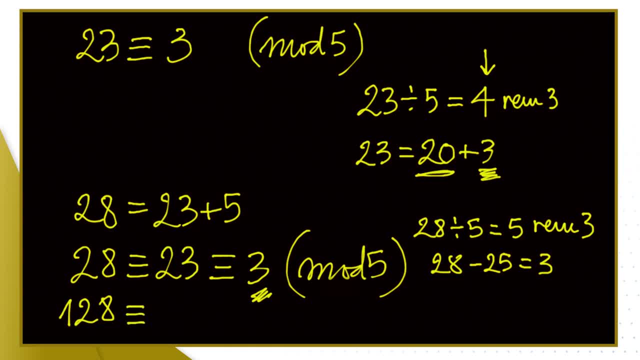 So 128 is still going to be congruent with 28 and congruent with 3 mod 5.. Now, in other words, the smallest positive number that is congruent with 128 mod 5 is still 3.. Let's look at another number. 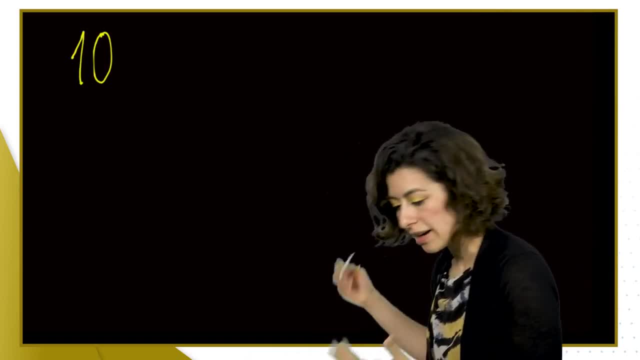 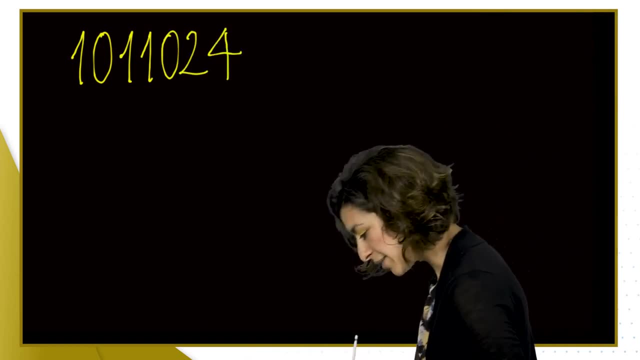 larger one. If I just write here a number I fancy, I don't know, 1011024.. I nearly tricked you to think we were doing binary, didn't I? OK, anyway, so that's that one. What is that congruent with mod 5?? 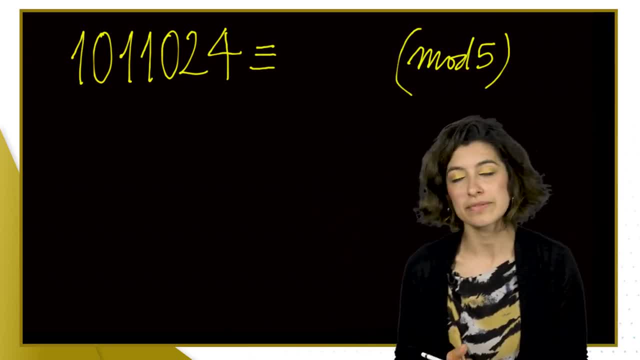 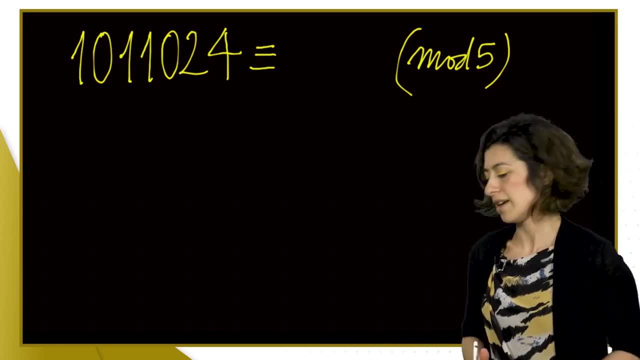 What is the smallest positive number that is congruent with this one mod 5?? Again, don't get fooled by the large number. It all boils down to the remainder of division by 5.. Fortunately, when we look at multiples of 5,. 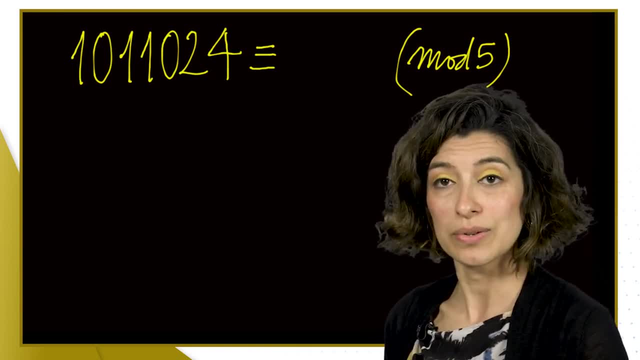 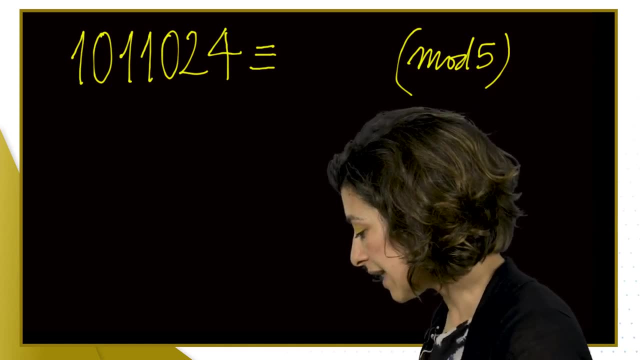 the last digit, the units digit, tells you whether the number is a multiple of 5 or not. If it ends in 0 or in 5, it is a multiple of 5.. This guy ends up in 4,, but the closest number. 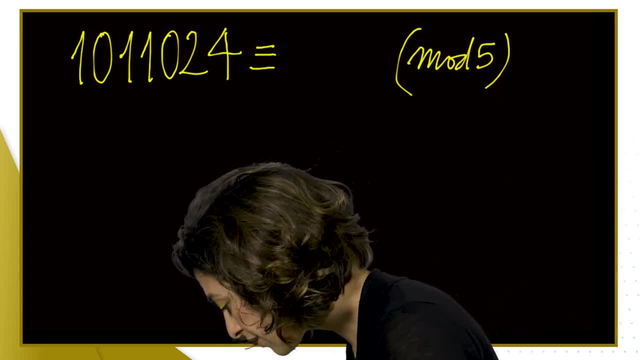 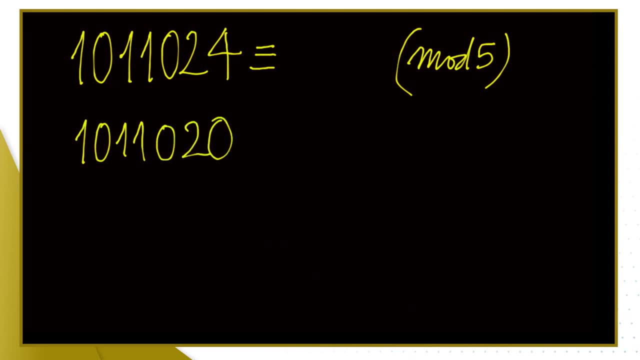 to it. that is, a multiple of 5 is going to be the guy that ends up with a 0. So 1011020 is the closest multiple of 5, so this number plus 4 is the number we started with. Therefore, the remainder. 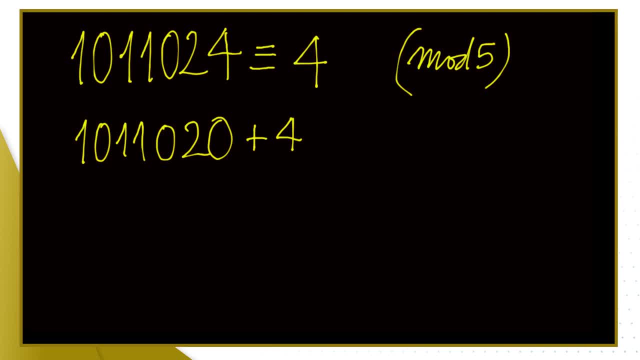 of the division by 5 is going to be that This means you can spare doing the whole division and in fact if you were to do the division you would be doing: divide that guy by 5, you have some integer part which I don't care about. 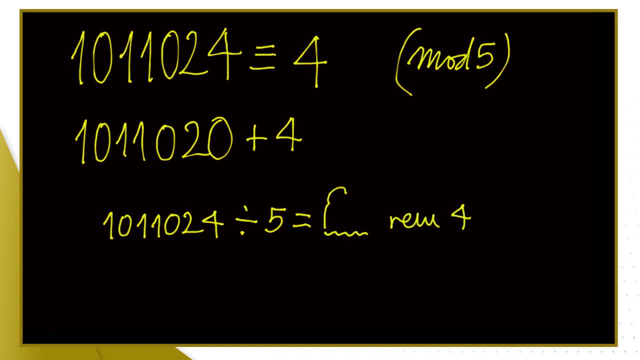 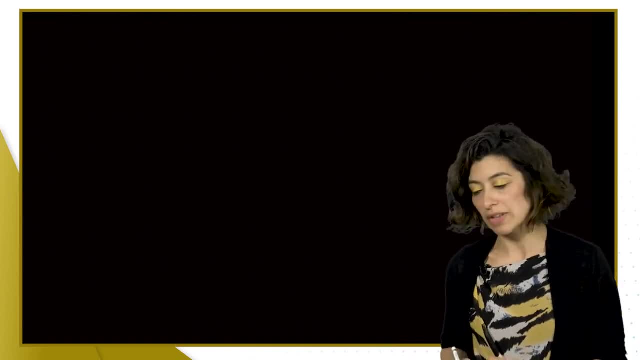 and you're going to have a remainder of 4.. You will get it, Just check it out with your calculator. okay, Let's have a taste of what mod 9 looks like. Again, mod 9,. how many remainders are you going to have? 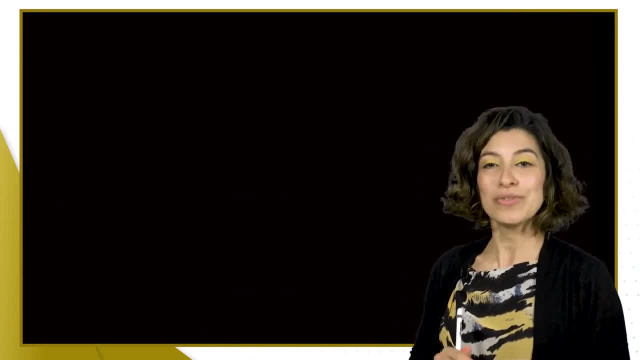 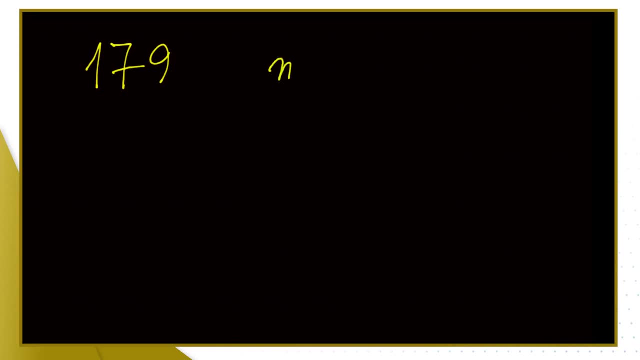 Yeah, I can hear you. 9 remainders from 0 to 8, that's all you're going to get. So if we're working with 179 mod 9, there's only 9 possibilities for that answer there. How do we get it? 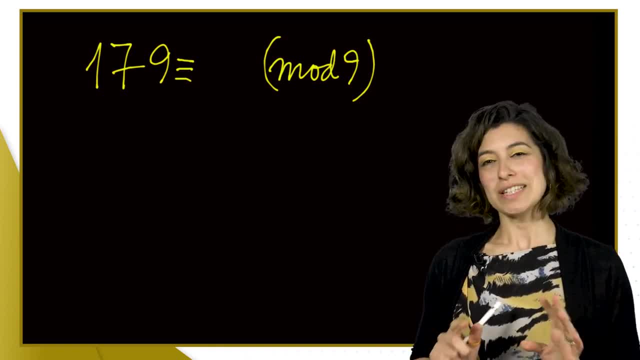 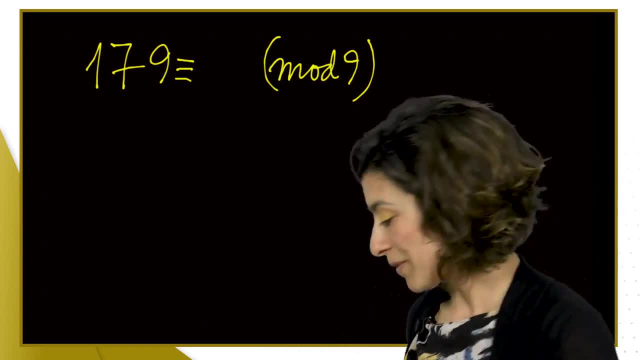 Now, mod 9 is one of my favorites because we got a little shortcut to work out the remainder. It is the thing you've learned in primary school of casting off 9s. yeah, So casting off 9s means you add up the digits. 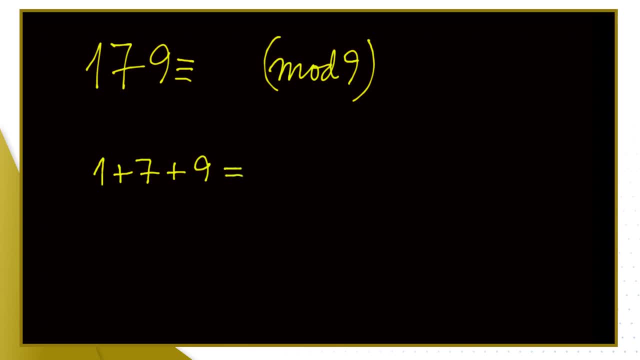 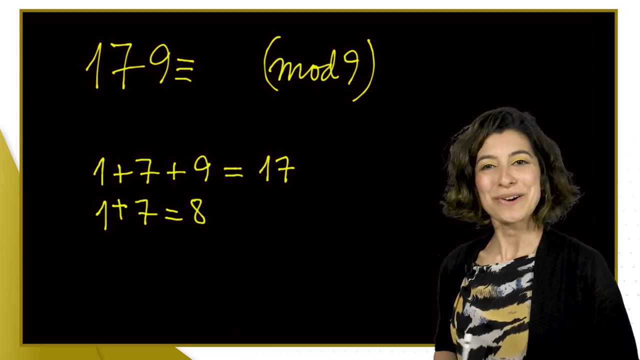 of the number and that brings us to 17.. The result is still a two-digit number. Let's add the digits again, That gives you 8.. So 8 is going to be the remainder of the division by 9. That means that it's going to get you. 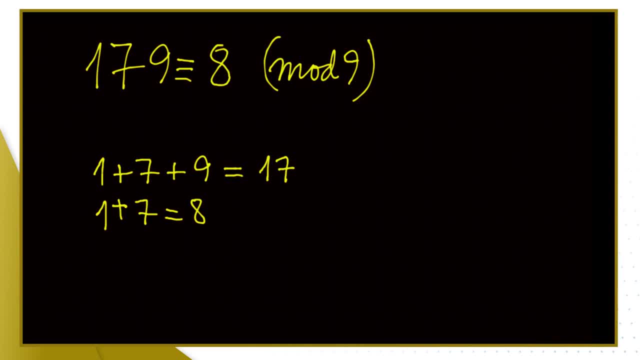 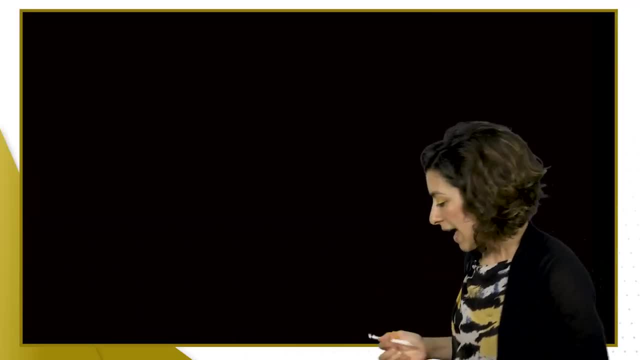 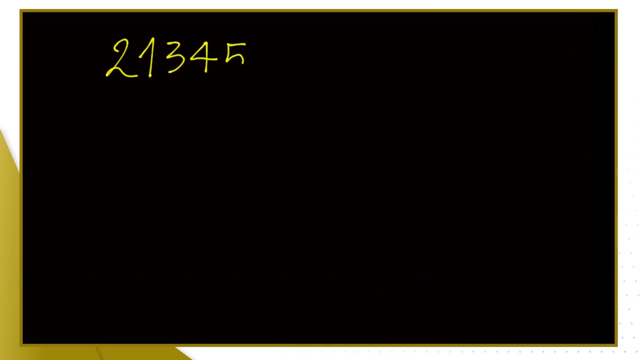 the mod straight away. It's a pretty cool property. This also works with a little variation, for mod 3.. And in mod 3, there's a special relationship between 9 and 3.. It is a- yeah, 3 is a. 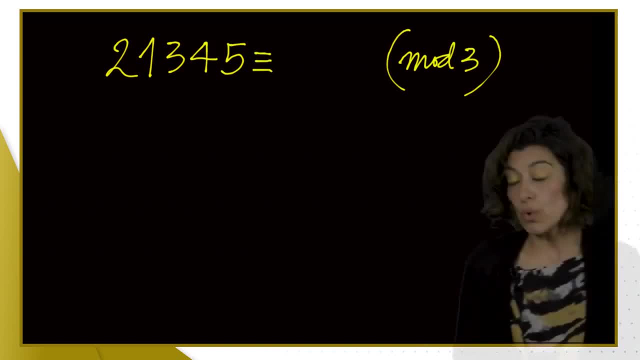 factor of 9.. So we can still do casting off 9s and then we do something else at the end. So let's do the casting off 9s. So add up the digits of this guy And we can shortcut this. 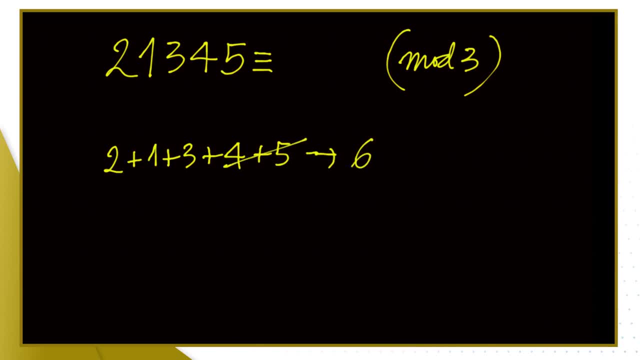 to 4 and 5 is 9, so I'll get rid of it And then I get 6.. 6 is a one-digit number. 6 would be the congruence mod 9, but we're not doing mod 9.. 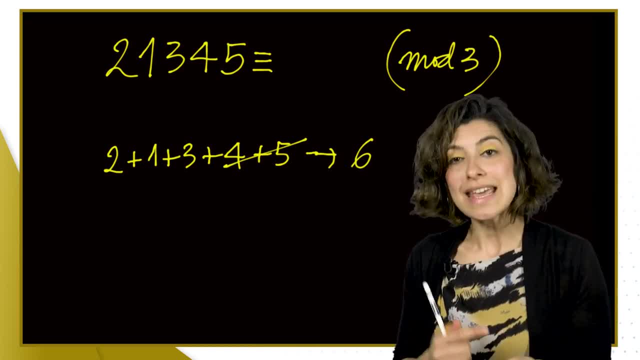 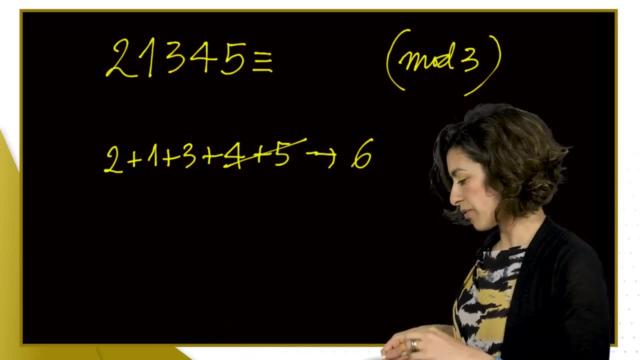 We're doing mod 3.. We just know that 6 is also a multiple of 3.. Therefore, the number we started with- 2,, 1,, 3,, 4,, 5, is going to be a multiple of 3 as well. 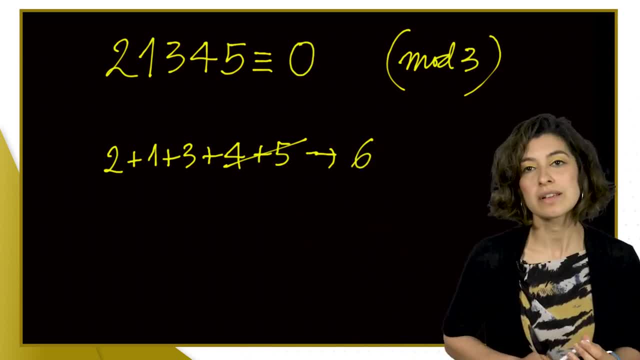 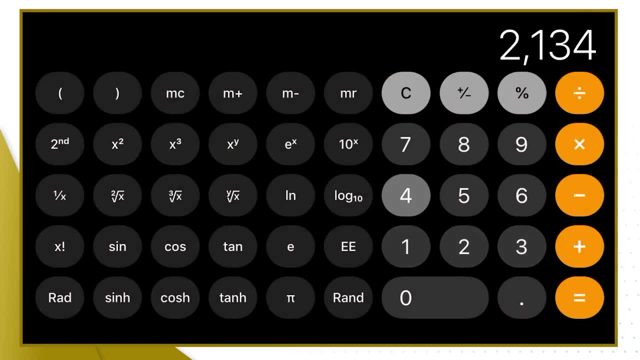 And therefore it has remainder 0 when divided by 3.. Do you want to check that? Let's look in the calculator. then 21,345 divided by 3.. Drum roll Pong: 7,115.. That means the division is whole. 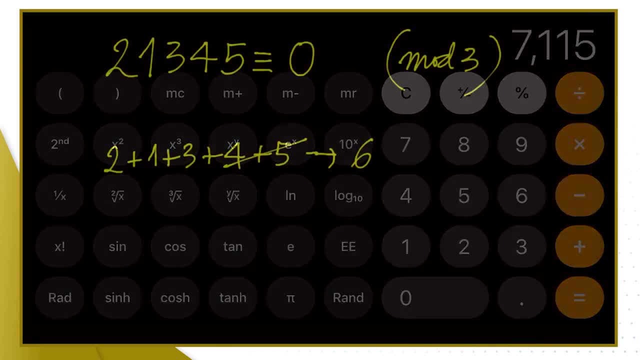 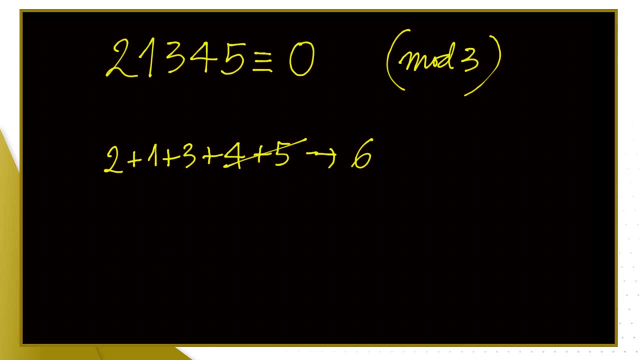 and you get 0 remainder. There we are For free. we get the numbers that come after and before this guy have the other remainders that are possible mod 3.. So 21,346 has remainder 1 when divided by 3.. 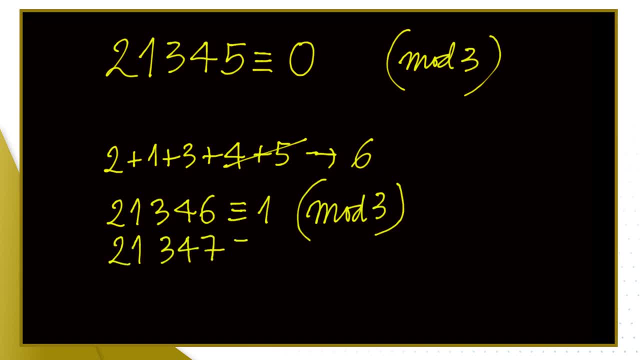 21,347 has remainder 2 when divided by 3.. And the next number, 21,348,. you say it is Yeah, Divisible by 3. And so remainder 0. If you were tempted to write 3 there, 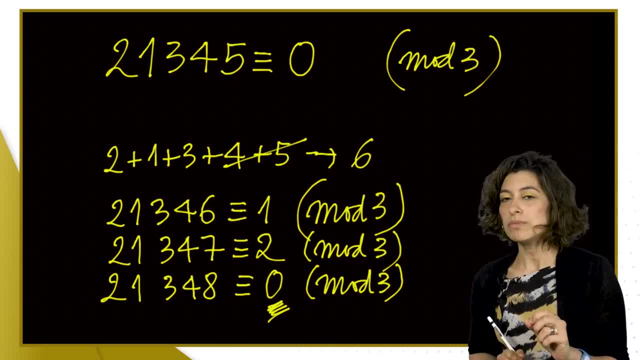 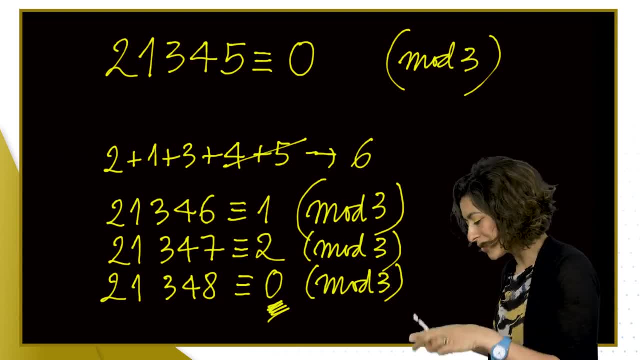 on the mod. it would be correct, but it wouldn't be totally correct, Because I want to boil it down to the smallest number. that is congruent with 21,348 mod 3. And the smallest is going to be either 0,1 or 2.. 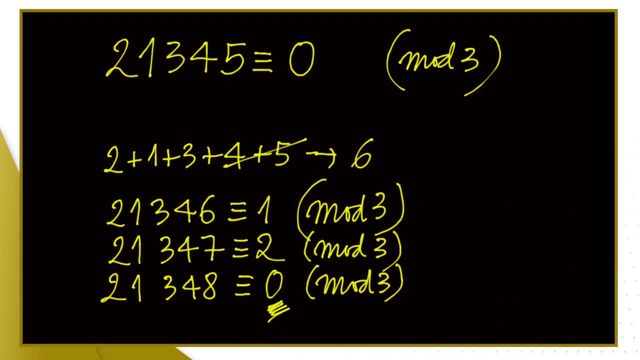 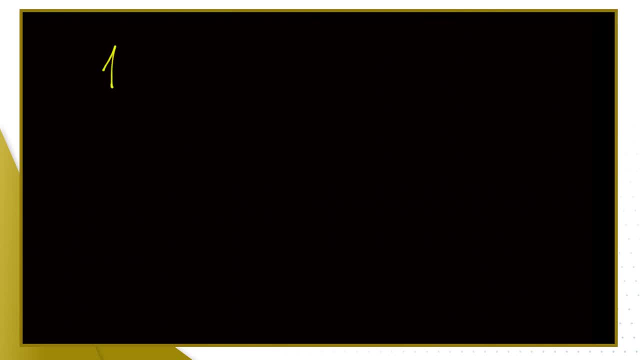 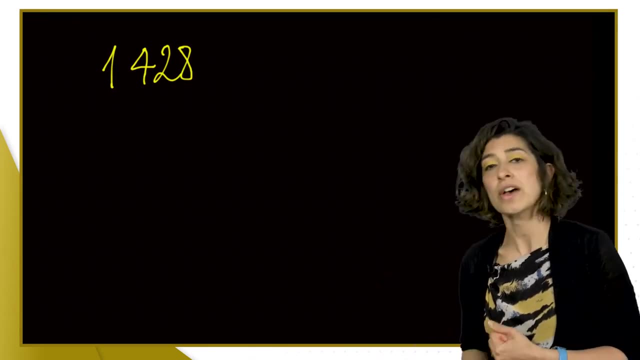 So we've got another multiple of 3 here, And so on, Mod 11.. Say, we've got 1,428. And again I'm asking you: what is the smallest positive number that's congruent with 1,428?? Mod 11.. 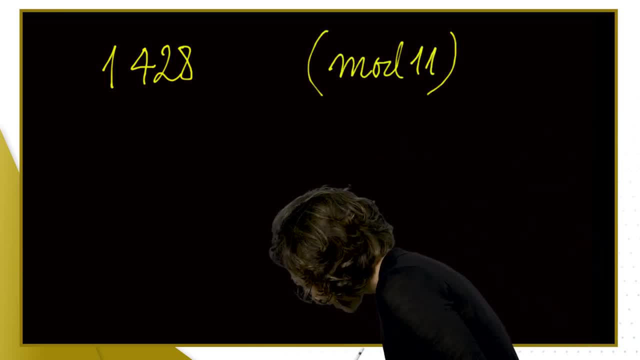 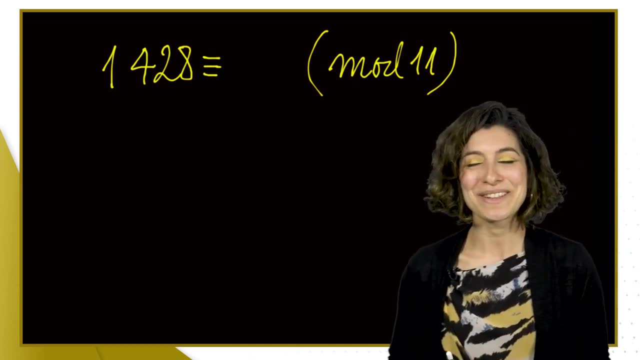 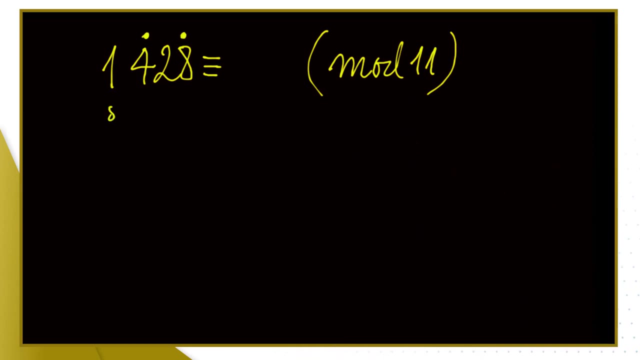 Mod 11.. 11 is pretty cool as well, because there is another shortcut for working out remainders of division by 11. And it goes this way: It's a trick with the digits, So we add up, So that's 8 plus 4. 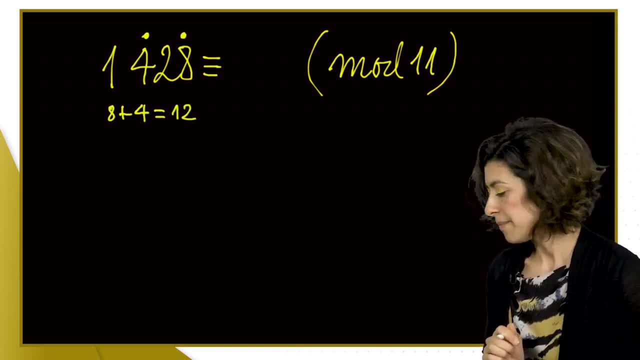 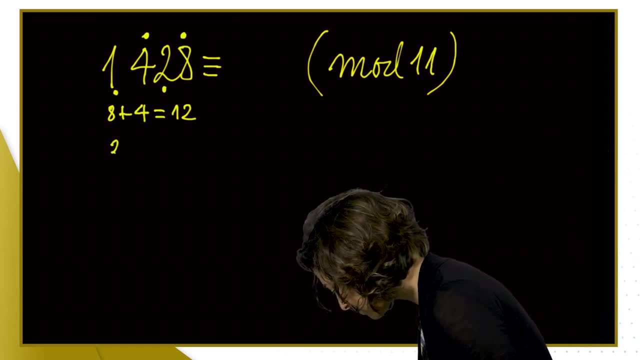 and that is 12.. Then we add up the second and the fourth digit, 2 and the 1.. So 2 plus 1 is 3.. And now here's the clever bit: You do 12, take away the 3.. 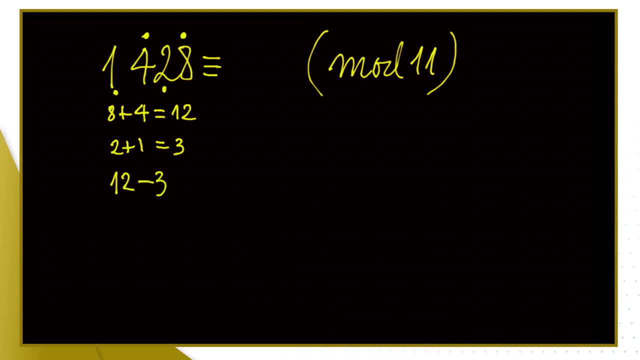 So you do the sum of the odd ordered digits. Take away the sum of the even ordered digits, So do the 12 minus the 3, and that gives us 9.. And 9 is going to be the remainder of division by 11.. 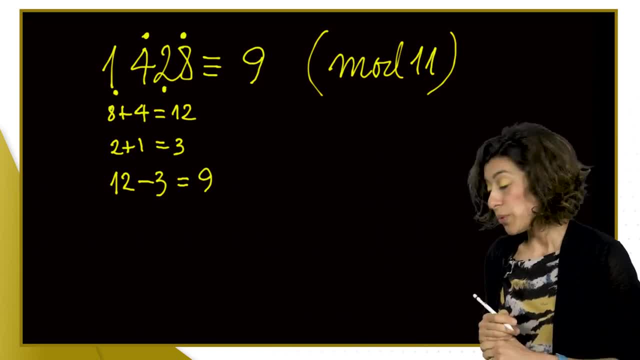 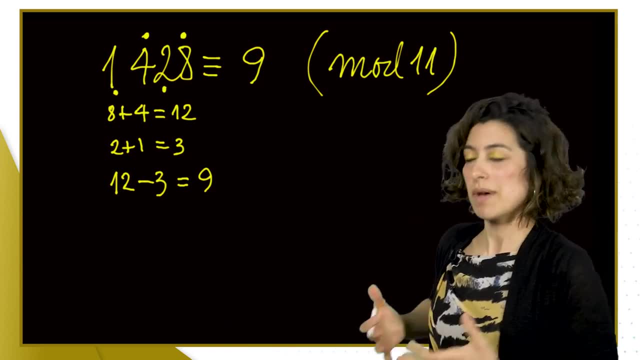 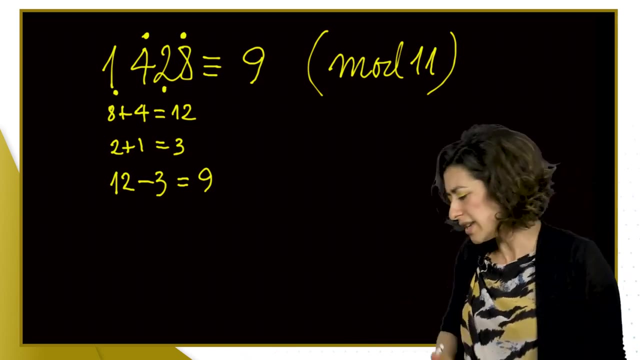 So that's going to be the mod. We can prove all these shortcuts I've shown you. We can prove them, But I just wanted to appreciate using them and see how much this helps you with your mental arithmetic and speeding up these calculations. It could be long and tedious. 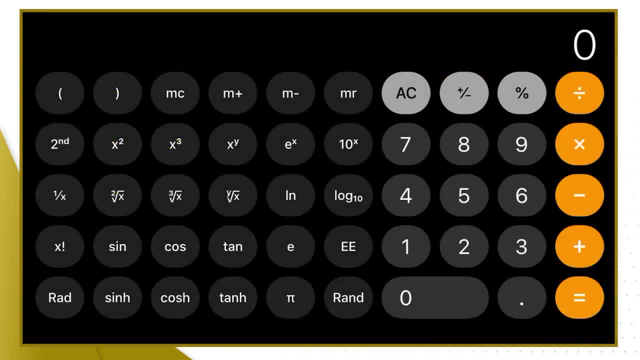 But let's look in the calculator. Is this true? Am I really talking the truth? You check? We're going to key this in in the calculator. So 1428 divide by 11. You get 129, blah, blah, blah, blah, blah. 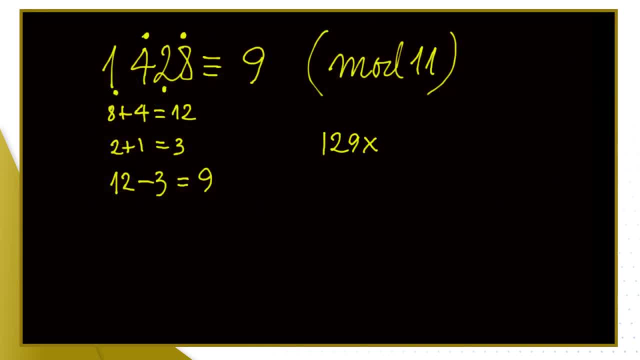 So you would do 129 times 11, which, by the way, we could do in the calculator, but it would be so much more fun if we do it by hand here. So I'll show you a trick of how we do multiplication by 11.. 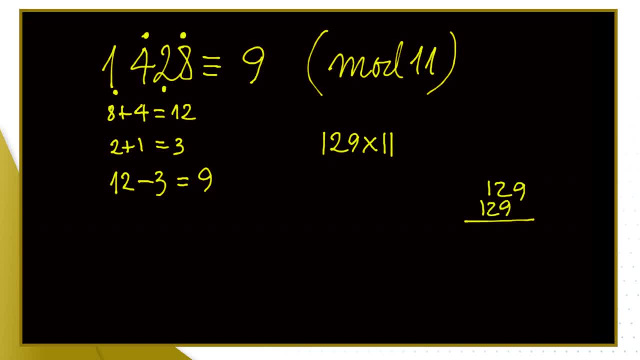 129, 129, a bit of sync, So 9, 11,, 4, 1.. There we are 1419.. And then you take the initial guy, 1428,. take away that product And what do you get? 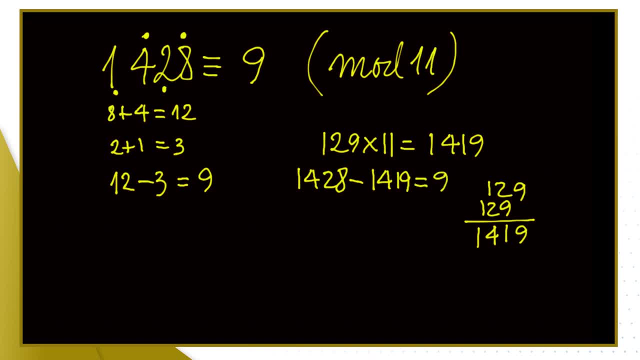 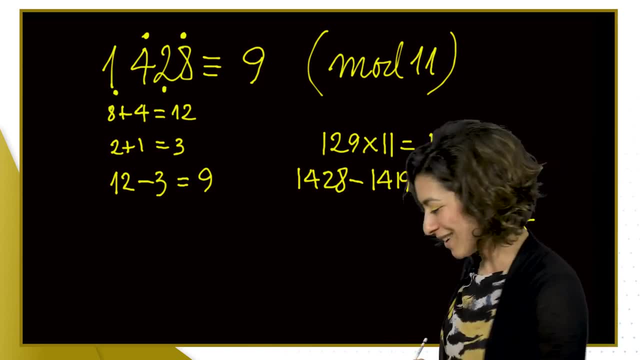 What do you get? You get 9,, as we said, And so that's the remainder. OK, You could do that in the calculator, but it's a lot more fun to multiply by 11 by hand. I know you would understand that. 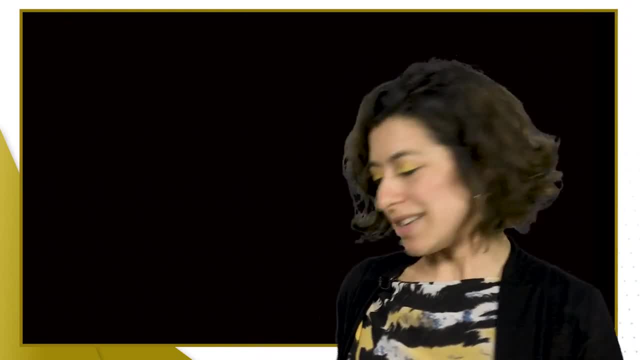 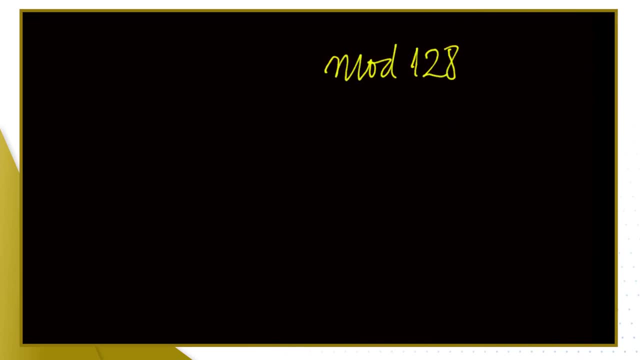 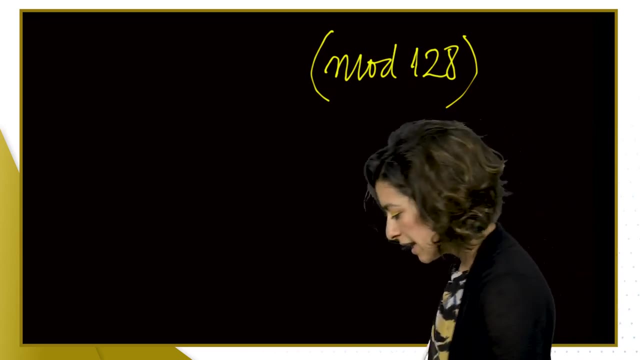 Right. So one more. Let's do mod 128. Big number. So in mod 128, how many remainders can we have when we divide by 128? 128. All the remainders from 0 to 127. If our number is bigger than that, 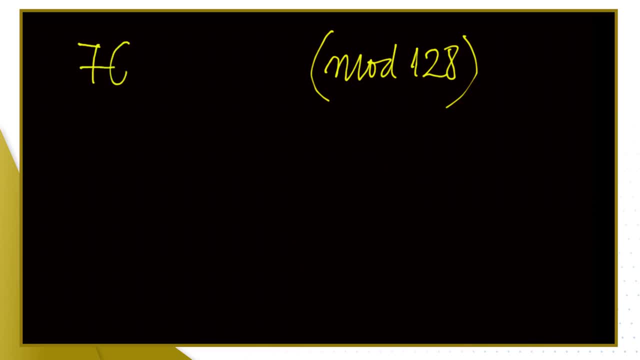 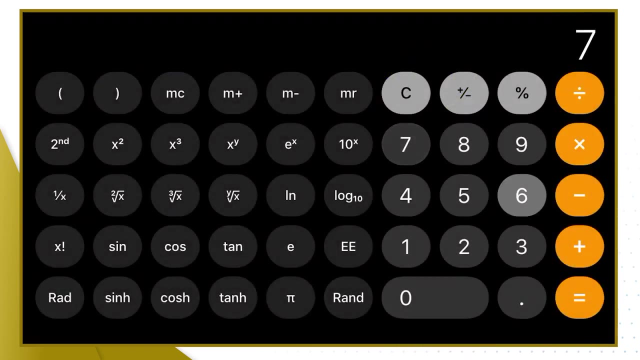 then we need to do some division. So let's look at 760.. What is the smallest positive number that is congruent to 760 mod 128? Let's do it. Calculator time Right. So we write 760 divided by 128.. 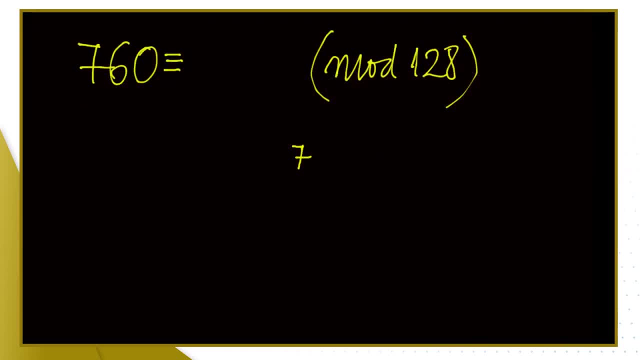 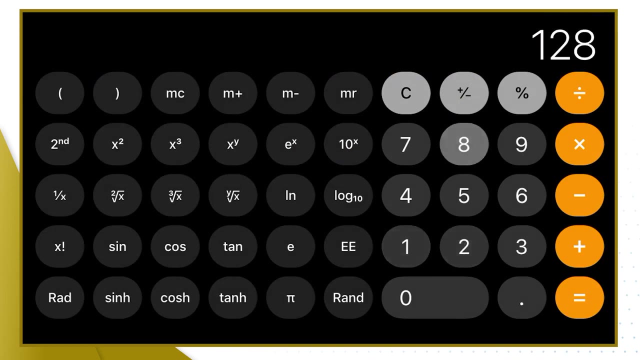 And there we are, So 760 divided by 128.. The whole part of this division is 5.. Let's work out the remainder. I'm going to back on my calculator just because I Yeah, 128 times 5.. Actually, this one we could do. 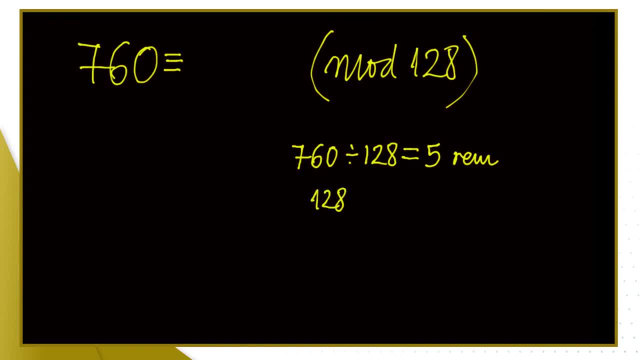 in our heads, couldn't we? 128 times 5, writing it down is 640. And then you would do 760, take away 640 and blah, blah, blah, You get 120.. Which is the remainder of this division. 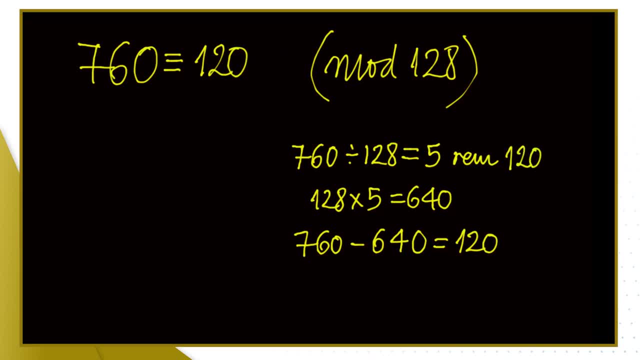 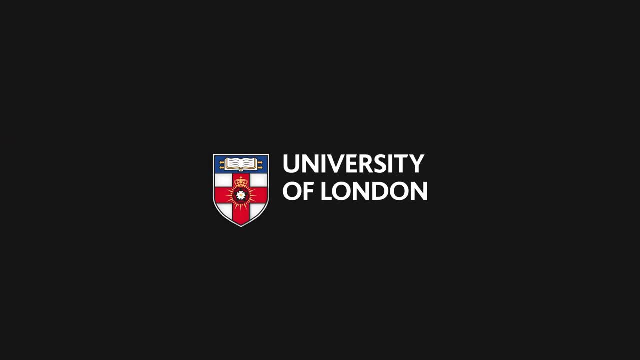 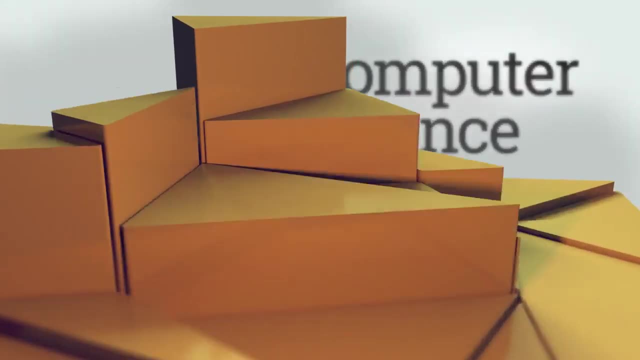 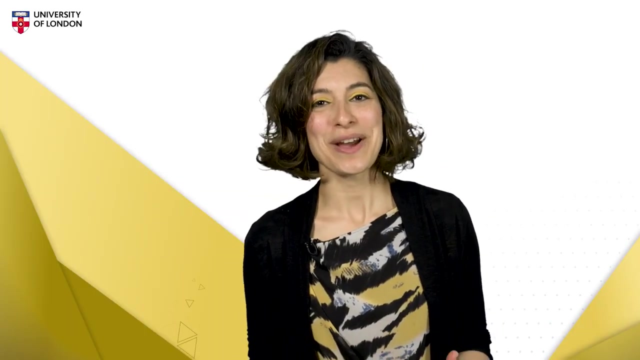 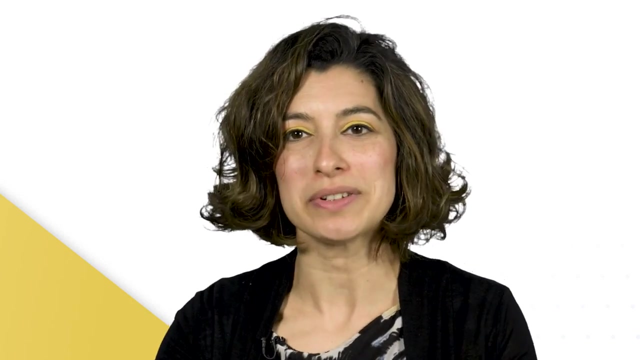 Okay, And therefore the number we're asking you on mod 128.. Hi there, Let's look at how to add up numbers in modular arithmetic. The key thing to bear in mind is the meaning behind all those symbols we use in modular arithmetic. 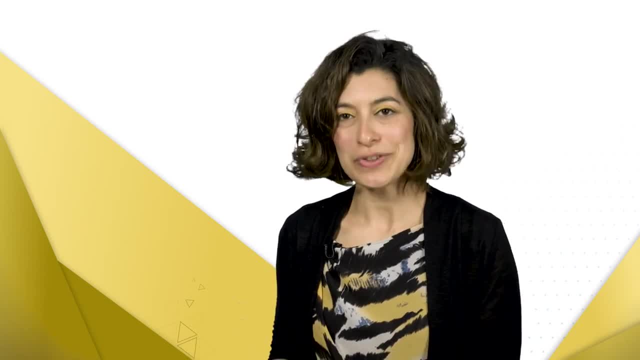 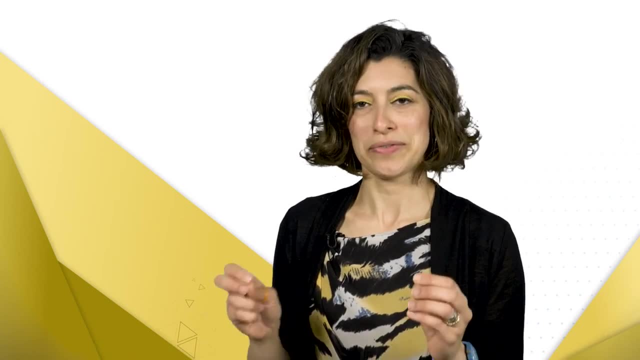 We are always using the remainders of division, And when we're adding numbers- mod, say, mod 5, we are adding the remainders of division by 5.. So I'm just going to show a different example, an example that apparently 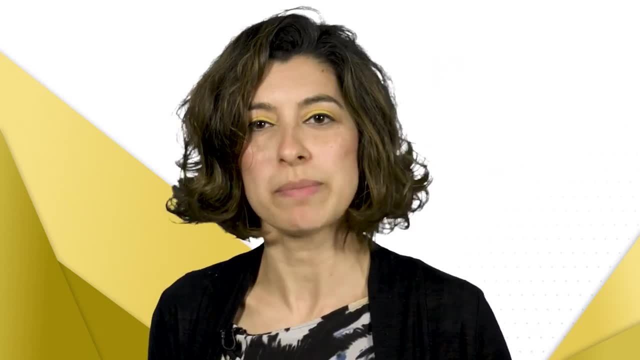 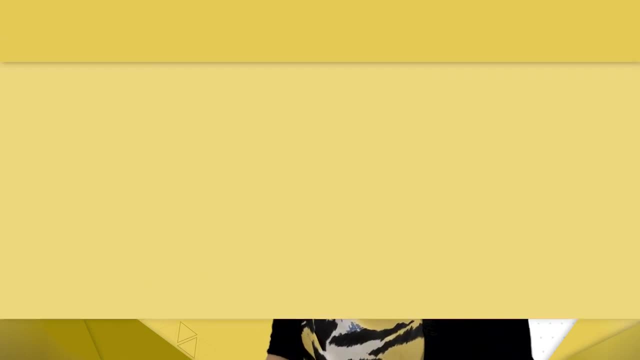 doesn't have anything to do with modular arithmetic, So bear with me in this Say I'm packing oranges in trays, Trays that take 12 oranges each. Okay, So I've got my happy oranges here in a tray of 12.. 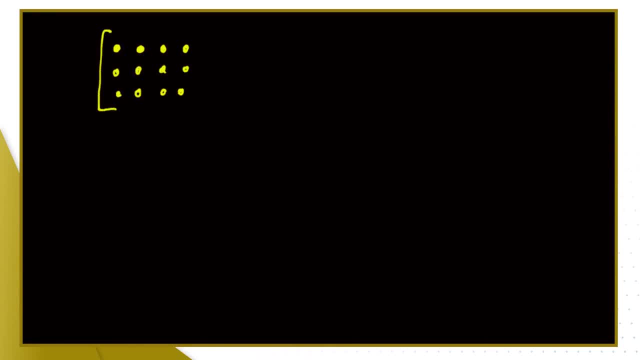 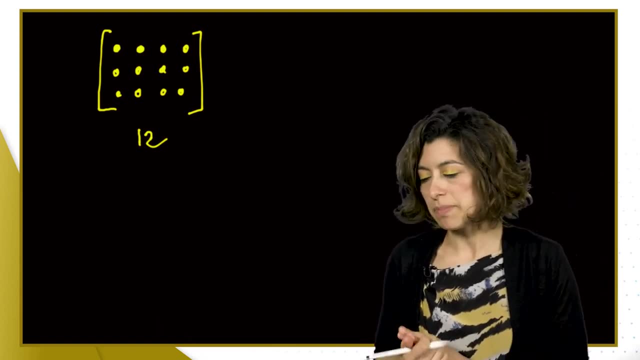 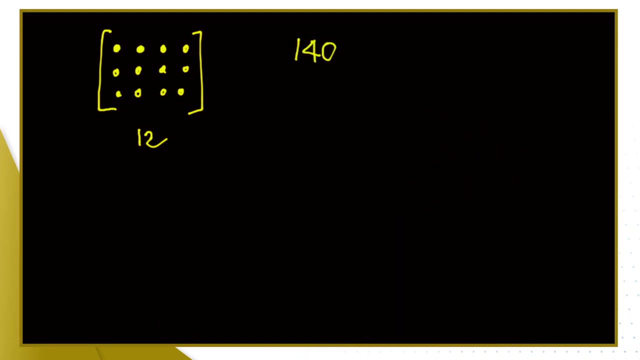 So 12 oranges, Really good. I got one tray with 12 oranges And I would give it a job that this week I'm going to be packing 140 oranges in trays of 12.. Okay, So I've got 140 oranges. 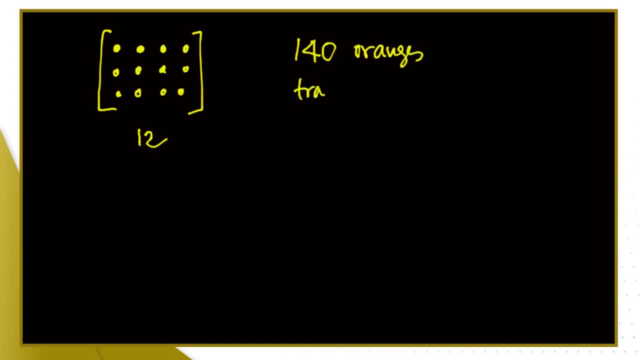 to pack in trays of 12.. How many trays do I get and how many oranges are left unpacked? Well, 140 oranges fills up 11 trays of 12.. So 140 can make 11 full trays of 12.. And that brings me to 132 oranges. 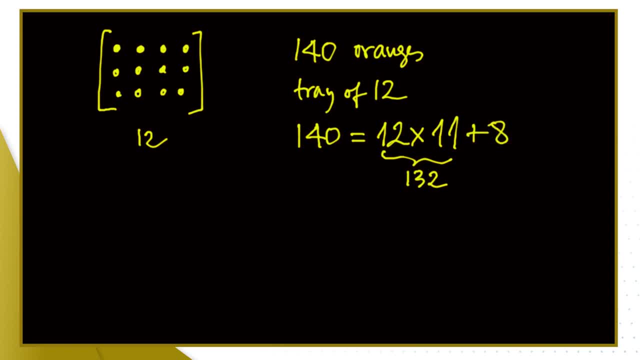 And then I've got 8 left. that aren't that? don't fill up the full tray. That 8 is the remainder of division of 140 by 12. 140 is 8 mod 12.. Okay, Say that now on the second week. 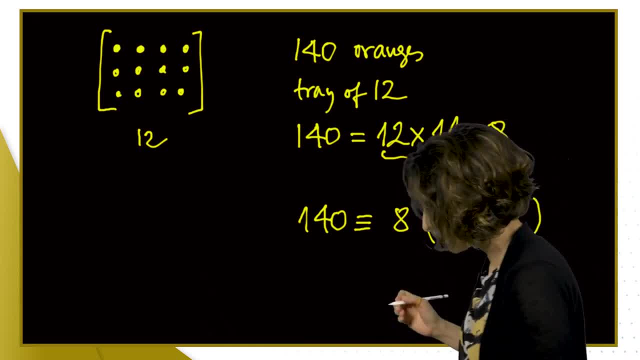 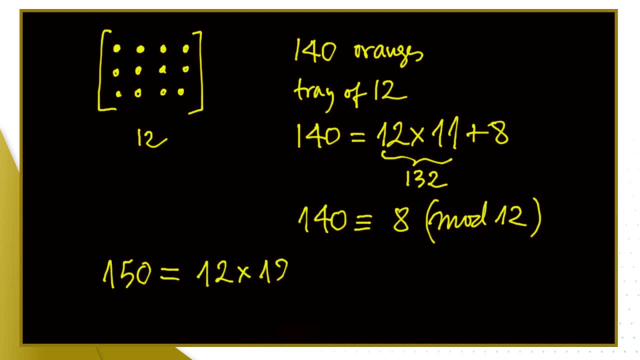 you know I've done such a great job packing oranges that I've got 150 to pack same size of tray. So 150, that's going to be. I can make 12 trays of 12. And that gives me 144 oranges. 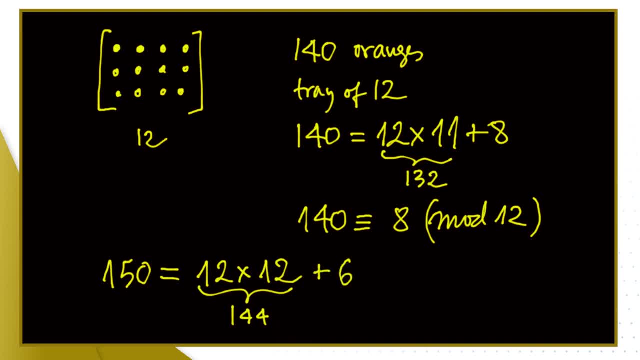 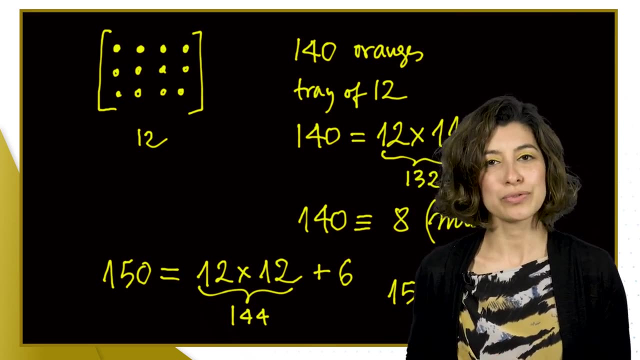 And then I've got 6 left that don't make a full tray. That's because 150 is going to put 6 mod 12.. Now the question is: over the two weeks, how many oranges are not in a full tray? 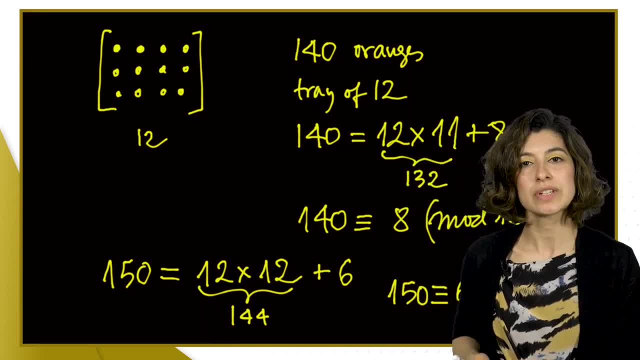 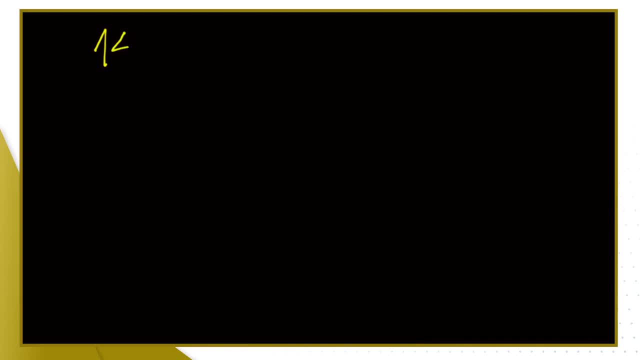 So you pack them all in trays of 12.. How many are left in a half filled tray? So it all boils down to 140 plus 150.. What's the remainder of division by 12?? We could add 140 plus 150. 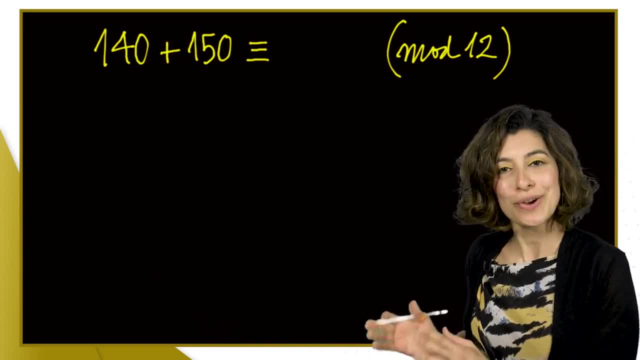 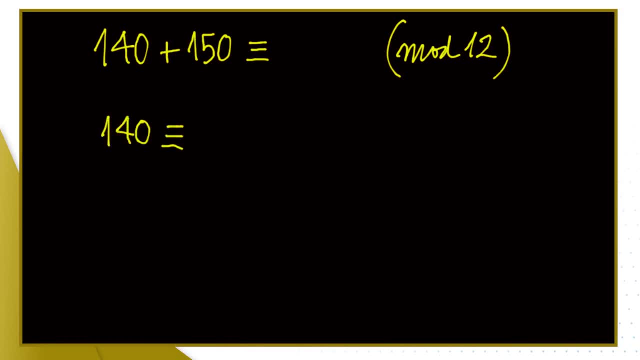 and then divide by 12 and find the remainder. But we have the remainders of 140 and 150 already calculated because we had that 140 had remainder. let's have a look. it was remainder 8 mod 12. And 150 has remainder. 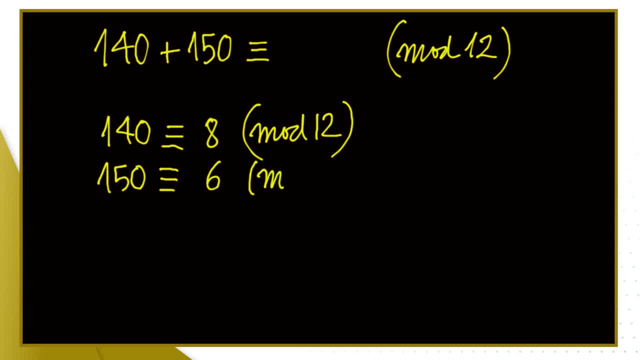 it was remainder 6 mod 12.. Therefore, when you add it up, the 140 add 150 is going to be congruent with 8 add 6, basically you're going to try to pack the 8 oranges left and the 6 oranges left. 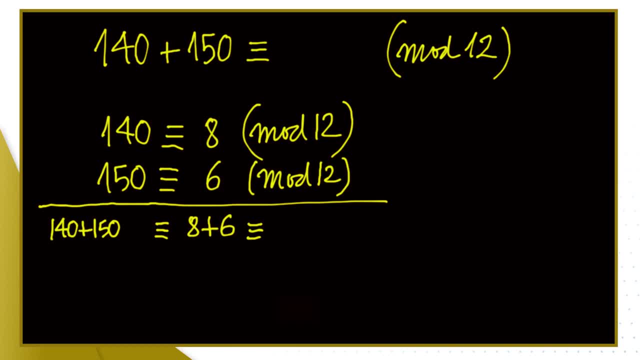 into another tray of 12. And that gives you 14 oranges. make one tray of 12 plus 2 leftovers, which means remainder 2 mod 12.. So we don't really need to add up the 140 with 150 and then do the division. 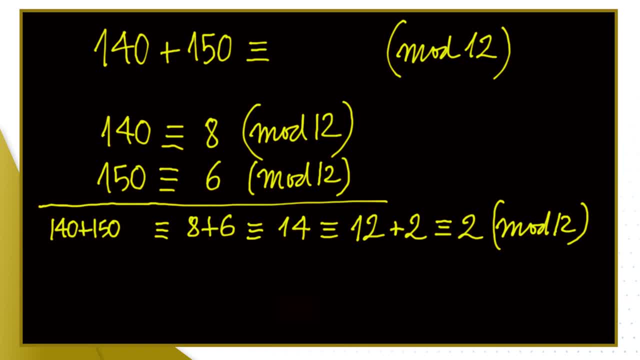 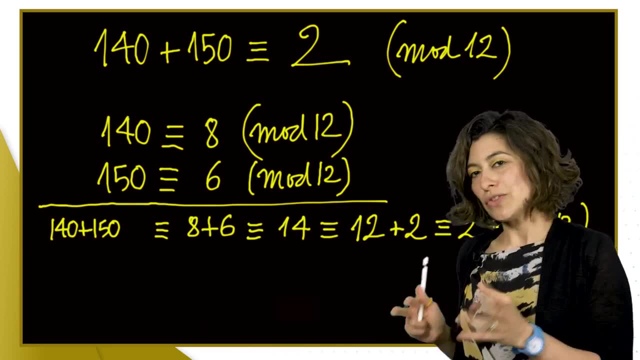 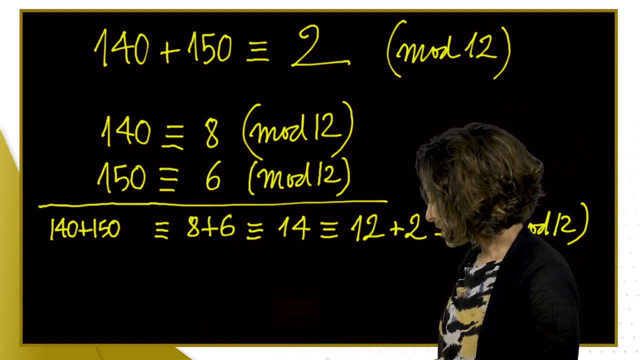 if we had the partials already done. So the answer over there is that you get remainder 2 mod 12.. Now that example just to illustrate the general rule that it's true in modular arithmetic: if you add up, if you have a number, 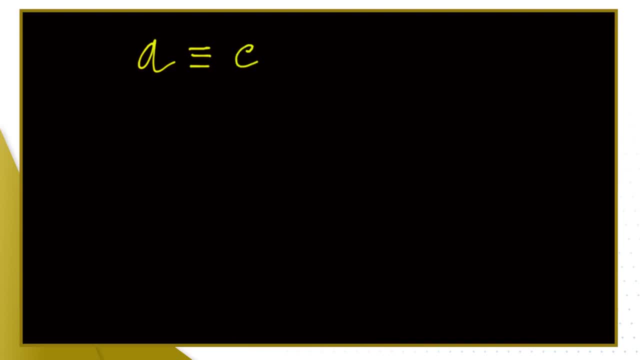 let's call it a, and we know that has remainder c when dividing by a number n. and you have another number, b, that has remainder d when dividing by the same n. it is true that the addition of the two numbers, a and b, 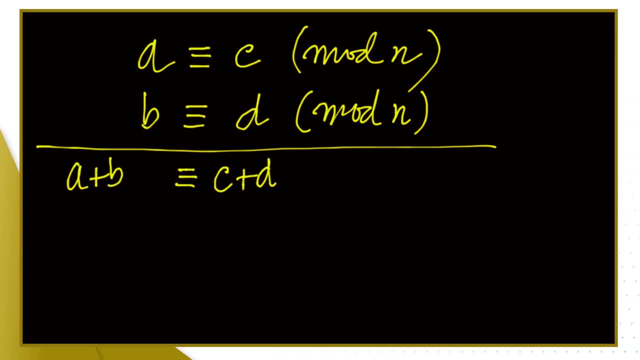 has the same remainder as the adding up the two remainders, Just like we did in the previous page, with a being 140 and b being 150.. Now, of course, this number here may not be a small enough number, but you can then find. 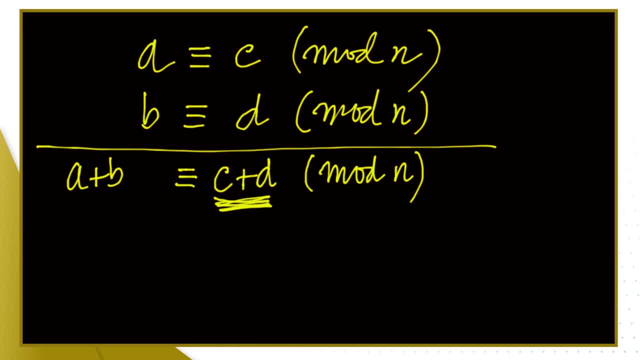 the remainder of this new number, that is, smaller, mod n. Let's have a look at how we use this. Just another example: We have 1456 and we want to find the remainder of this, mod 12, so how many? what's left after packing your oranges? 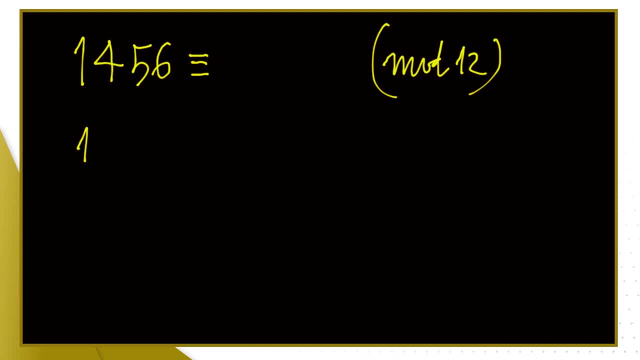 in trays of 12.. If you spot that this number can be written as a combination of a multiple of 12 plus something else, you can use that to shortcut the calculation. So I spot that this number is close to all: 1440,. 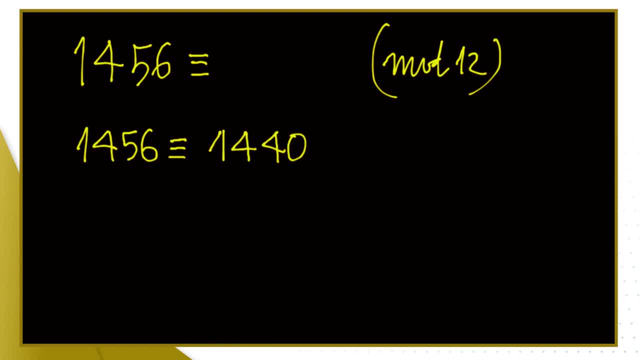 which I know is 120 times 12, because 12 times 12 is 144, and then I've got 16 there. I can use this breakdown to speed up the calculation: 1440 being a multiple of 12 is congruent with 0 mod 12.. 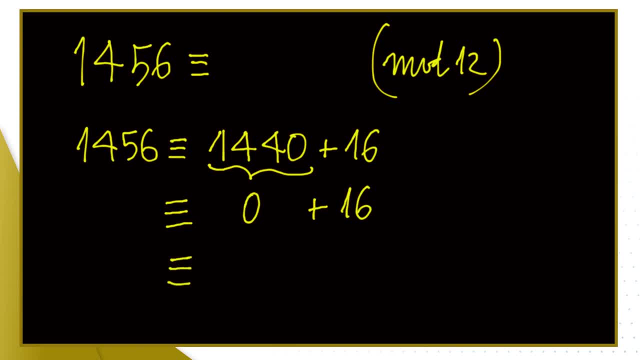 I'm now down to adding up these, and 16 is congruent with 4 mod 12.. So you can knock off multiples of the mod and take them away to speed up your modular arithmetic calculations. One more example, If you're explicitly asked. 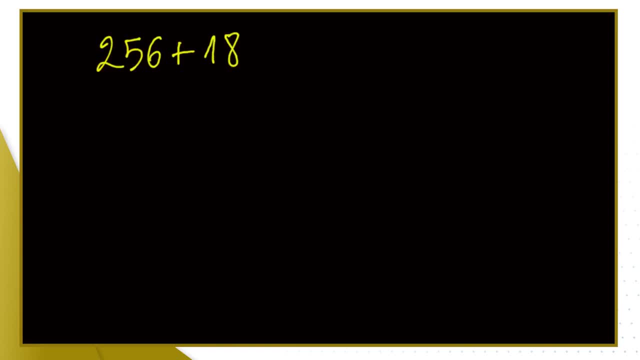 to calculate 256 at 18, still mod 12, we can do the partials again: 256, that is congruent with 4 mod 12.. You can check that out. And then 18 is 12 plus 6,. 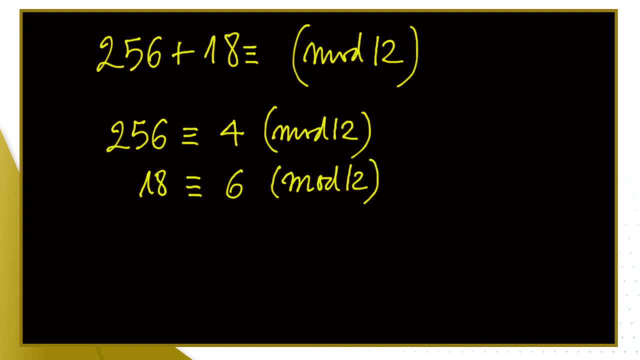 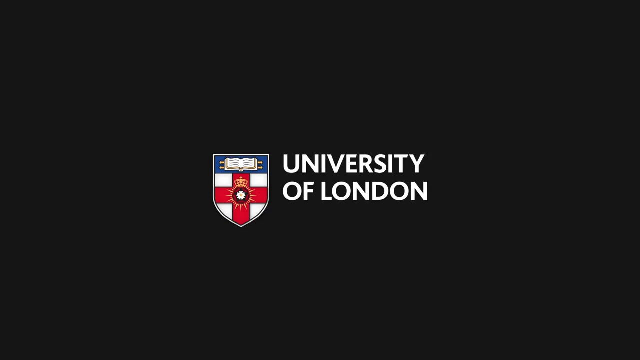 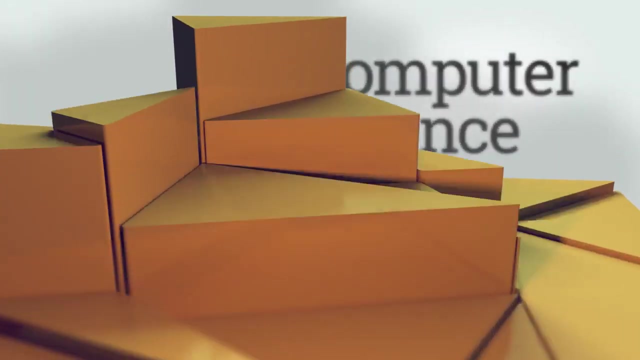 so 6 mod 12.. The addition of these guys is going to be congruent with 10 mod 12.. Okay, There you are, And we're right there: congruent with 10 mod 12.. We looked at adding up numbers. 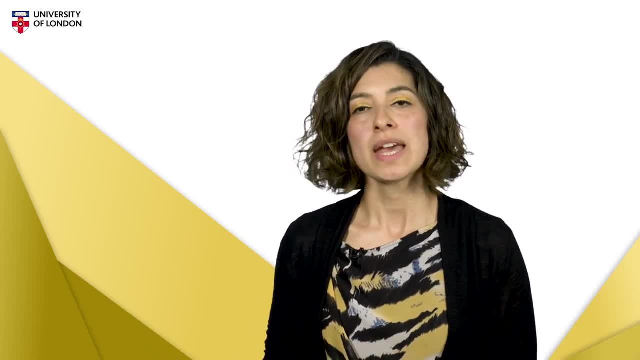 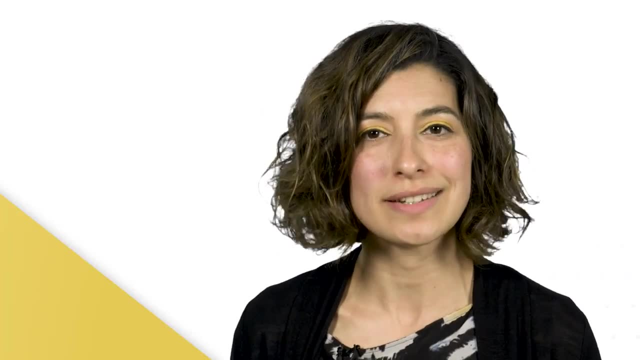 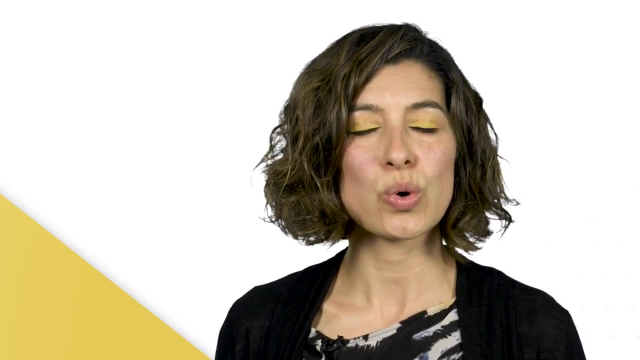 in modular arithmetic, for example, adding numbers mod 5.. Now, what number added to another changes nothing. That's going to be the additive identity And having that in mind, we will be able to understand what it means by having numbers that kind of cancel each other out. 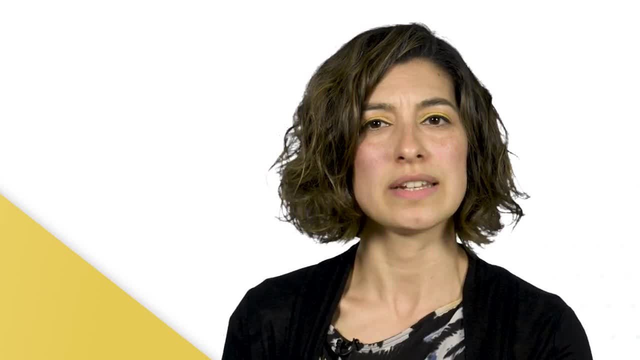 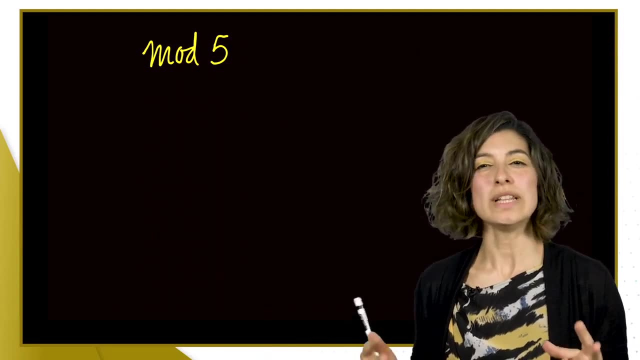 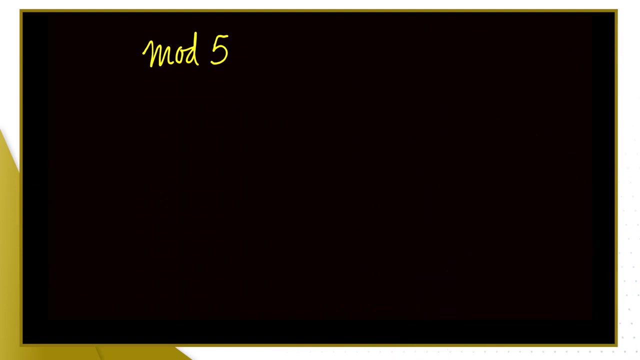 or add up to that additive identity Easier if I show you what I mean In mod 5, I'm really interested in working with numbers between 0 and 4, so the remainders of division by 5.. We'll look at the addition table. 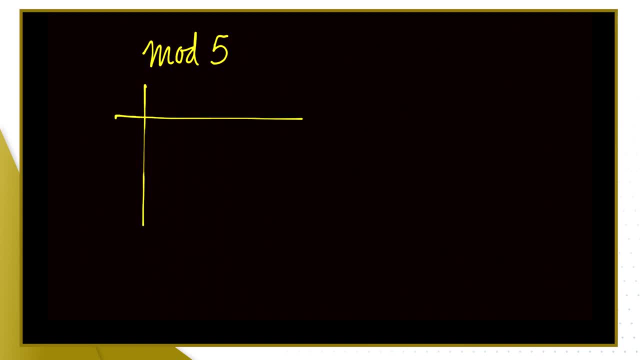 which I'll just write again here, The addition table mod 5.. We've got 0,, 1,, 2,, 3, and 4.. 0,, 1,, 2,, 3, and 4.. And I'm going to add up. 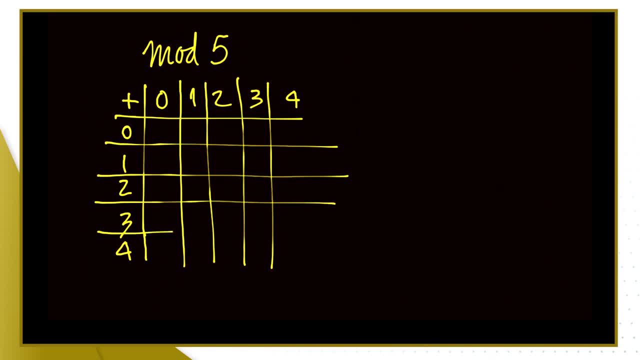 all those numbers, mod 5.. Okay, so 0,, 1,, 2,, 3, and 4.. 0,, 1,, 2,, 3, and 4.. 1,, 2,, 3,, 4.. 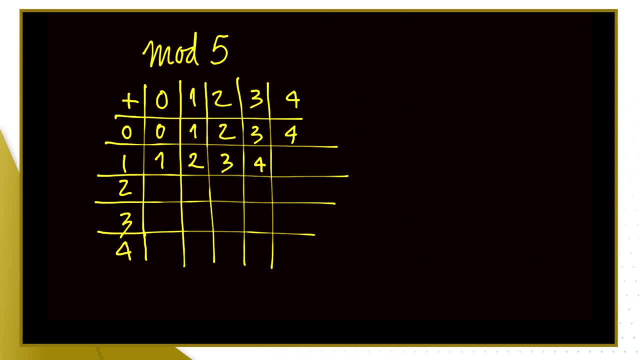 And then 4 plus 1 is 5,, which is 0 mod 5.. And then 2,, 3, 4.. 2 plus 3 is 5,, so that's 0 mod 5.. And 4 plus 2 is 6,. 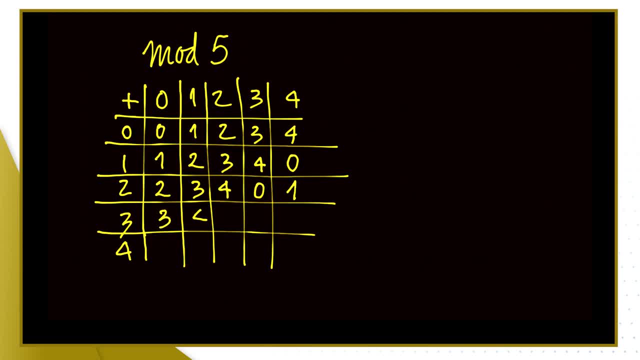 which is 1 mod 5.. And then 3,, 4,, 0,, 1,, 2,, for the same reason as before, And 4,, 0,, 1,, 2, and 3.. Right. 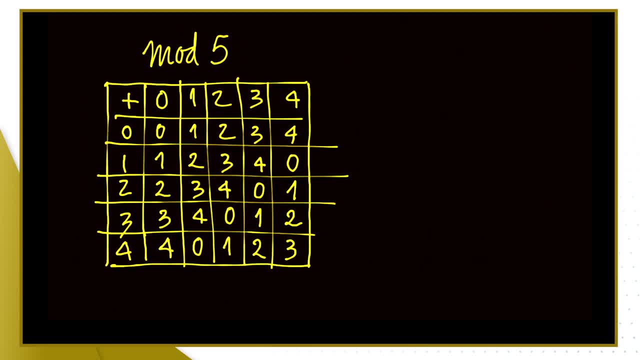 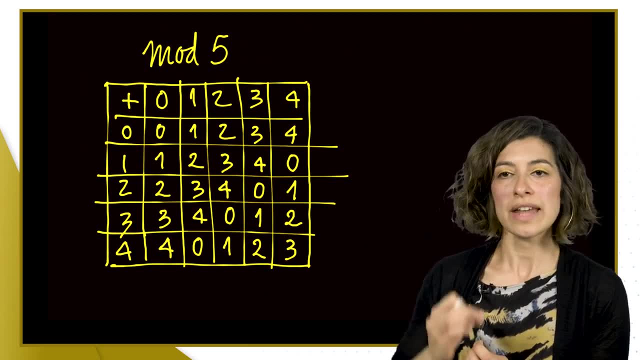 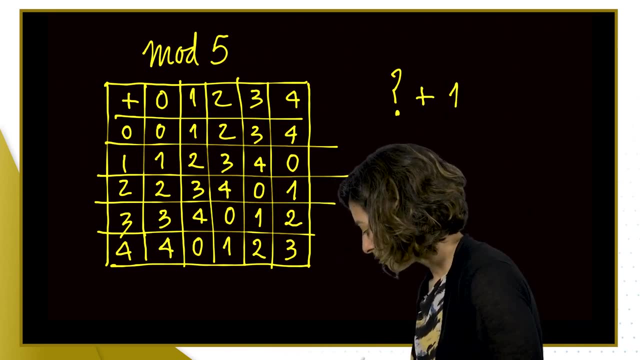 That's our addition table. Now we're looking for the additive identity. That is a number that added to any other doesn't change it, So it's a number that, added to 1, still gives 1 mod 5.. But instead of 1, I put 2.. 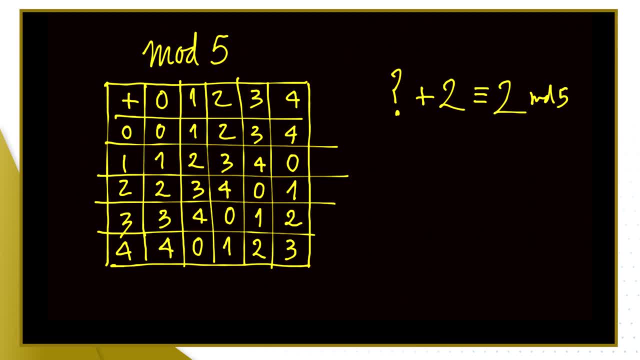 I want the result to be 2.. And so on, and so on, and so on. So it's adding nothing, isn't it? It's 0.. Now, does it still make sense in mod 5?? 0 plus 2 is just 2,. 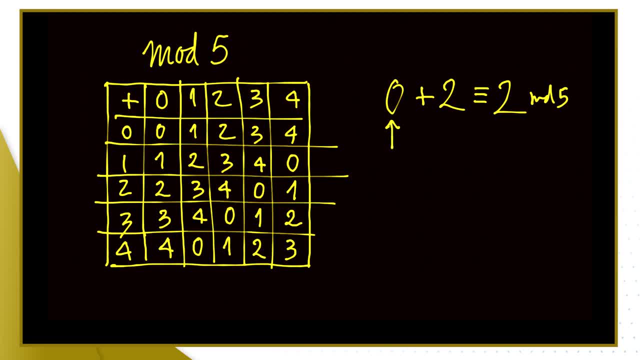 meaning 0 stands for any number that is a multiple of 5.. And 2 stands for any number that leaves remainder 2 when divided by 5.. If I add 2 of those numbers together, I still have remainder 2 mod 5.. 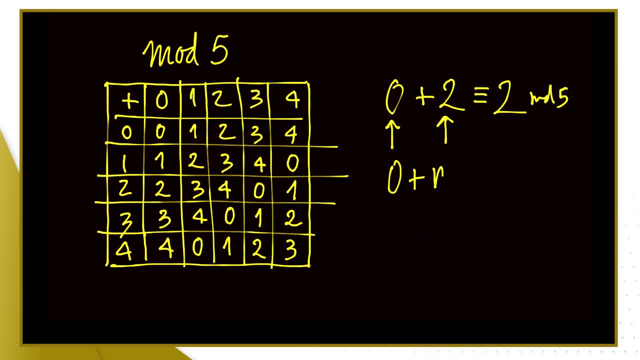 And 0 adds any number that is going to be the number itself, mod 5.. So the same 0 I have here. So 0 is our additive identity. So 0 mod 5 is the additive identity, Mod 5.. 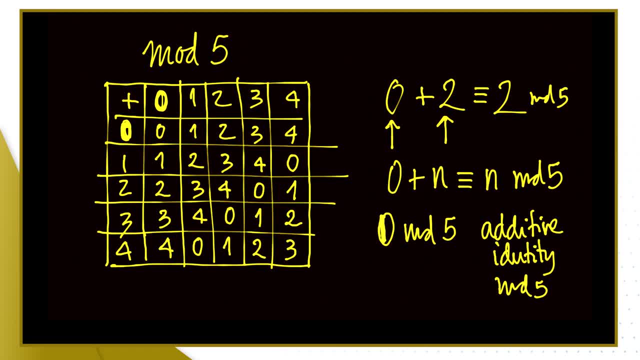 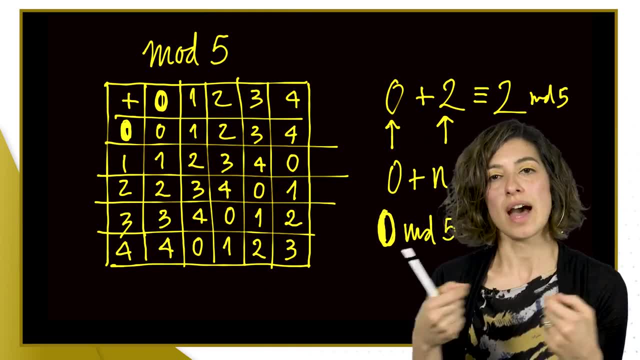 We could even write a special 0 for it, which sometimes we do, But we don't want to do it with 0.. Now where do I want to go with this? I want to look at pairs of numbers that add up to that 0. 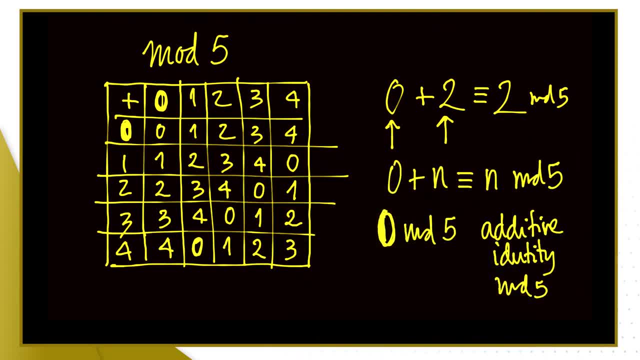 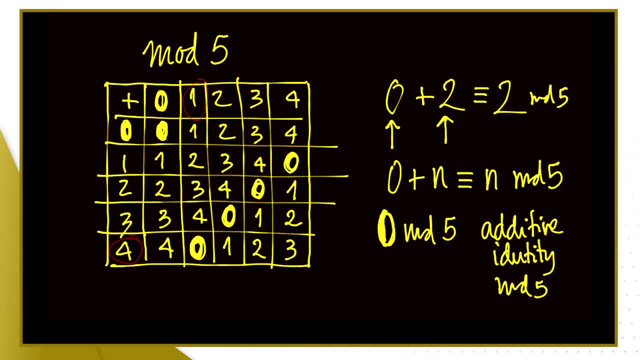 I've got the 4 and the 1.. 4 plus 1 adds up to 0. Mod 5.. That's not surprising. 4 plus 1 is 5.. 5 divided by 5 leaves remainder 0, mod 5.. 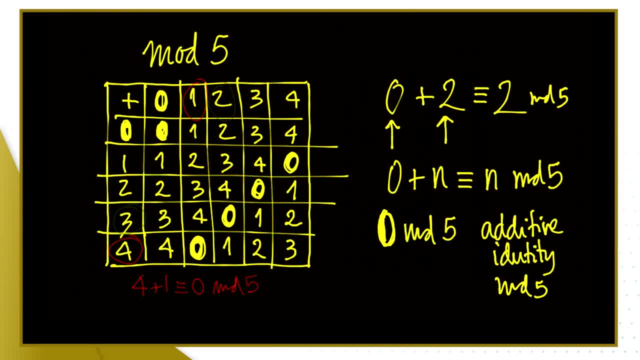 We've got the 3 and the 2, because 3 plus 2 leaves remainder 0, 1 divided by 5.. So, in fact, any pair of numbers that adds up to 5 in this table. So there we are. 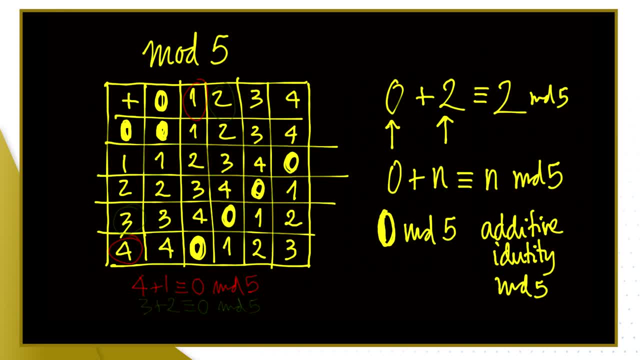 So 4 and 1,, 3 and 2,, 1 and 5,, 5 and 0,, 0 and 5.. So those pairs are additive inverses mod 5.. So I'll just write it there: 0 plus 0,. 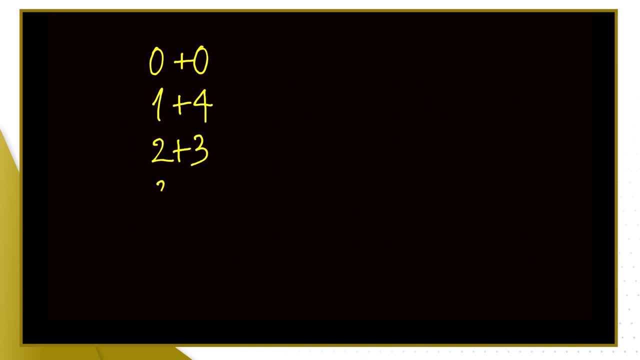 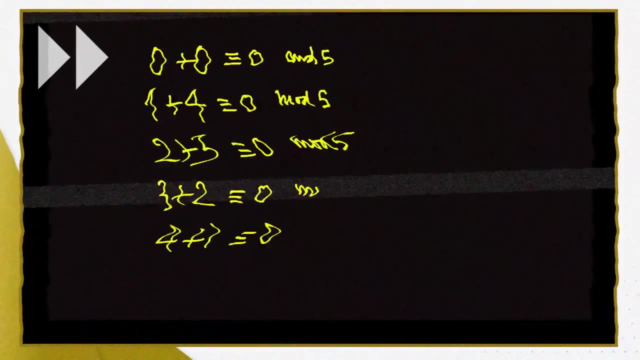 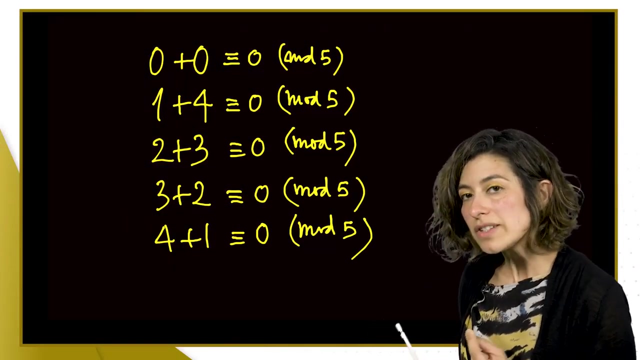 1 plus 4,, 2 plus 3,, 3 plus 2,, 4 plus 1.. They're all 0 in modular arithmetic with modulo 5.. That means each of these pairs are inverses of each other. Additive inverses, mod 5.. 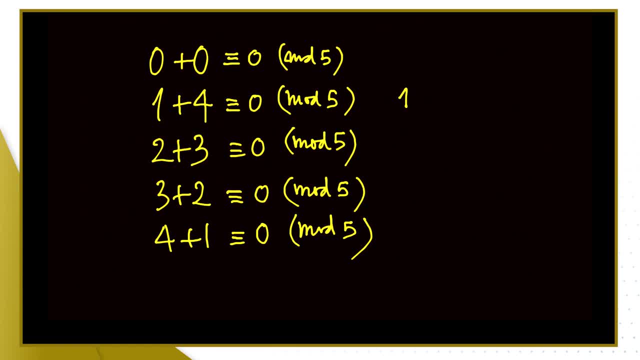 So that means 1 is the minus 4 mod 5, meaning 1 is the number that added to 4 gives 0 mod 5.. And also 4 is the minus 1 mod 5.. OK, so that comes from. 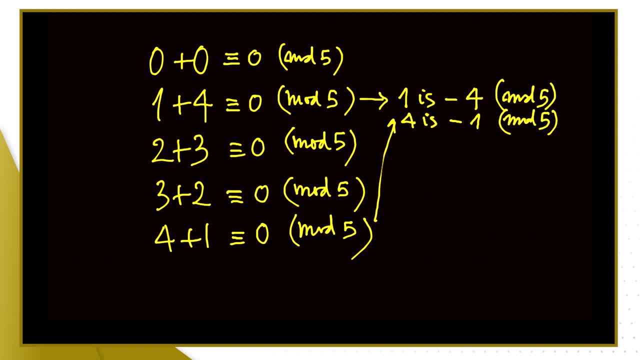 there and also from there, OK, From the other two, with 2 and 3 added to 0, that means 2 is the additive inverse of 3 and 3 is the additive inverse of 2.. So I write the minus for it. 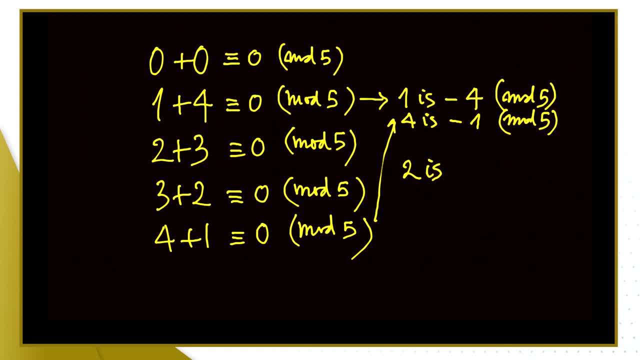 So 2 is the additive inverse of 3.. So I write: minus 3.. And 3 is the additive inverse of 2.. So 3 is the minus 2 mod 5. And 3 is minus 2 mod 5.. 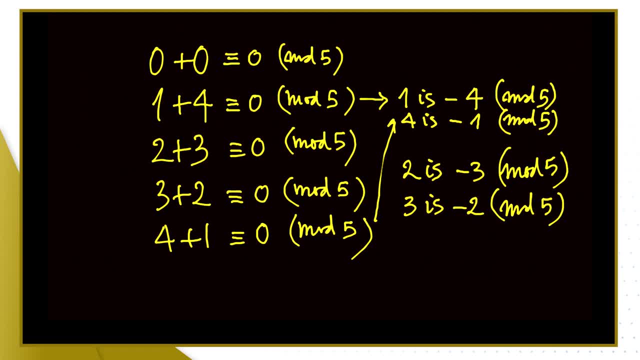 How do I write this in the middle of a calculation? I would simply write minus 4, and I use the symbol for congruence: minus 4 congruent with 1 mod 5.. And I would say as well that minus 1 congruent with 4 mod 5.. 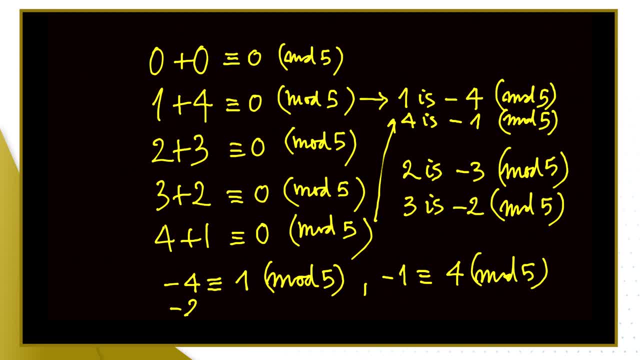 And similarly for the other numbers. So the minus 2 is 3 mod 5, and minus 3 is the 2 mod 5.. The key idea to bear in mind is which is numbers that, added together, give 0 mod 5.. 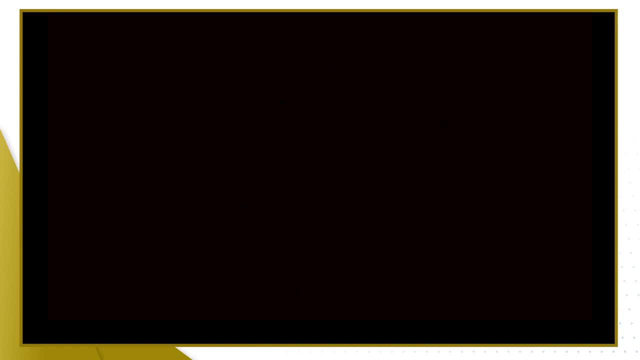 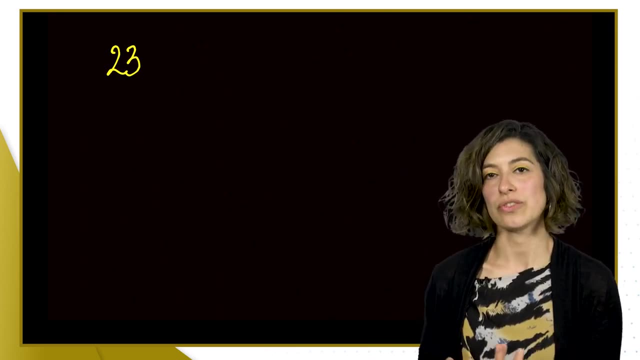 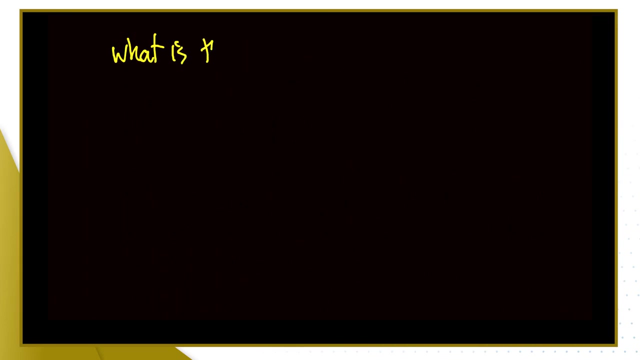 So let's look at this example. Say, I've got number 23. And I want to find what is the additive inverse of 23 mod 5.. So I would ask: what is the additive inverse of 23 mod 5.? The mathematical way of writing it. 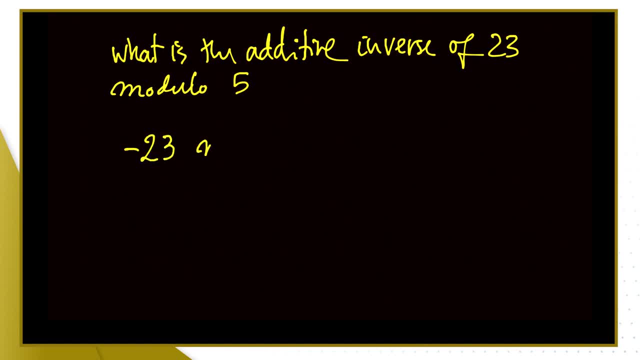 would be what is minus 23 mod 5.. We say what number added with 23 gives 0 mod 5.. Now, to start with, I wouldn't work with 23 because 23 is bigger than 5.. I would reduce 23 to: 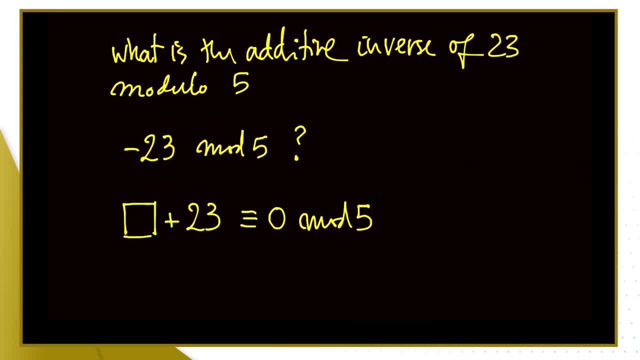 the remainder of division by 5.. So the smallest number I can. So 23 divided by 5. Well, 5 goes 4 times into 23.. So 23 is 4 times 5 plus 3. So the remainder is 3.. 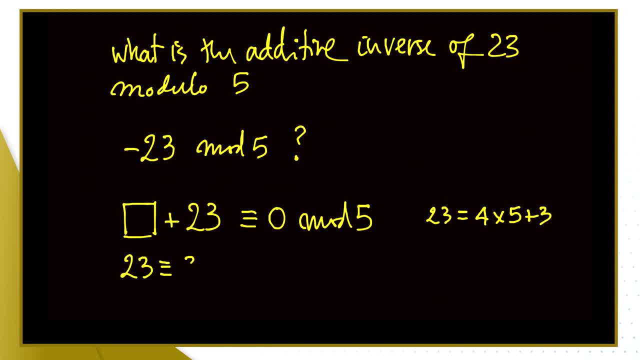 So to start with 23 is congruent with 3 mod 5.. So minus 23 is going to be minus 3, which we saw before. that the number that added with 3 that gives 0, is 2.. So the minus 3 is 2 mod 5.. 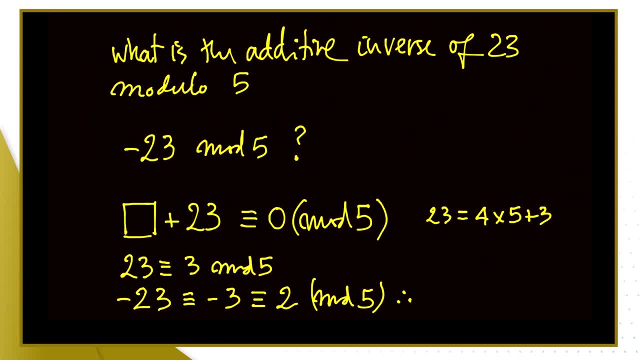 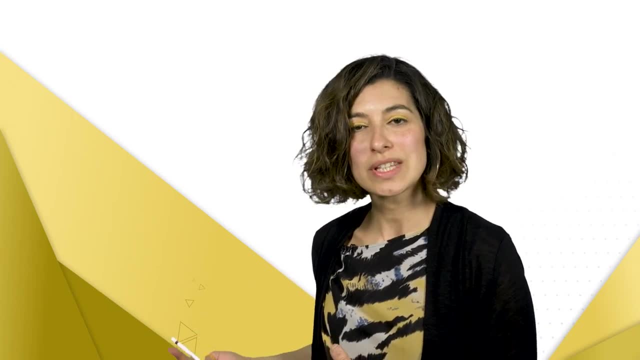 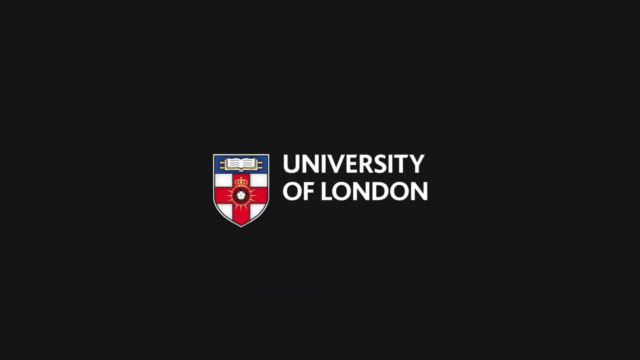 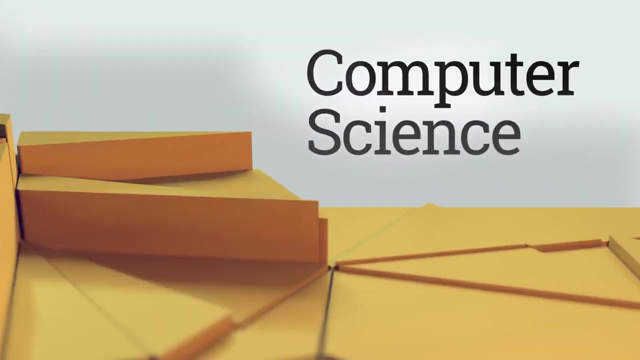 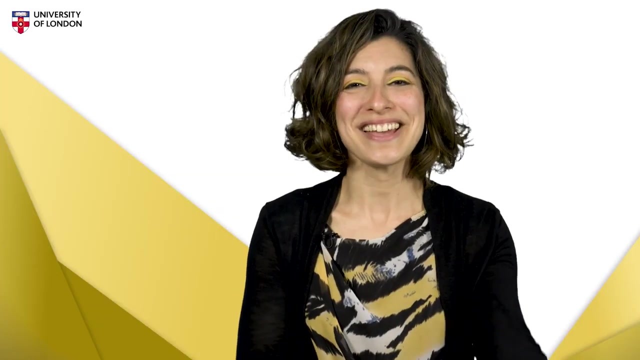 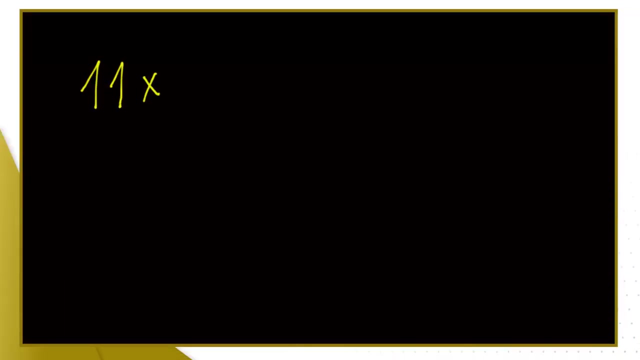 And therefore, and therefore, minus 23 is 2 mod 5.. And in this way we work out the additive inverse of any number in any module. So we have this: We've got 11 times 13 and we want to calculate this. 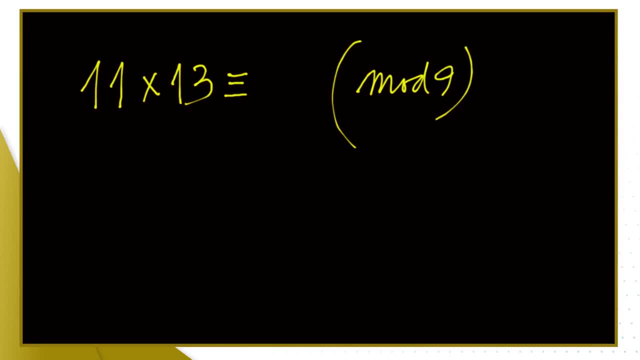 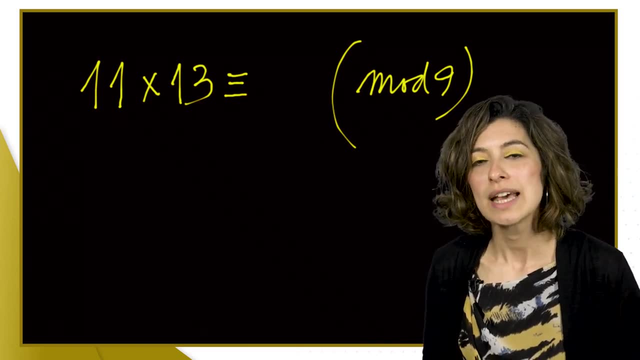 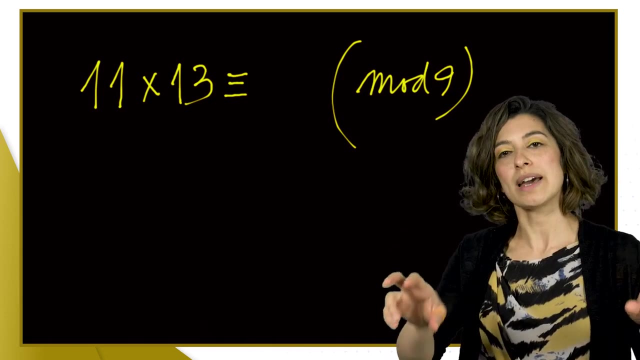 in mod 9.. Now, key thing to remember is: if you can avoid getting to big numbers, please avoid it. Keep the numbers as low as you can. In this case, 11 and 13,. the numbers we're trying to multiply. 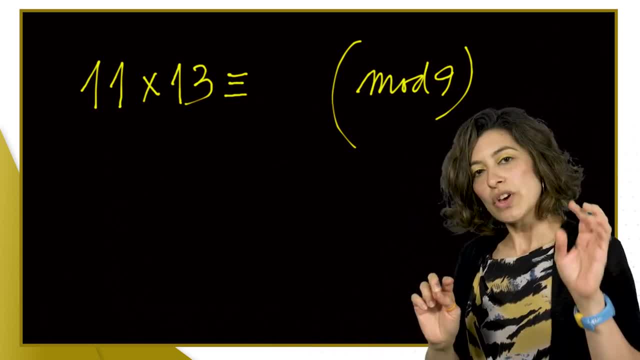 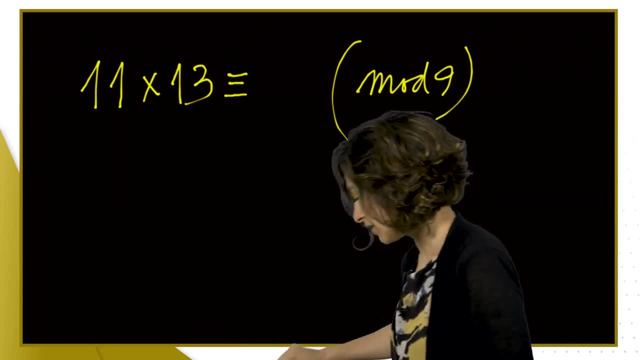 are a little bit bigger than the mod 9.. So we're going to calculate 11 mod 9 and 13 mod 9 and then multiply the remains together. That's what we're going to do. So 11 is congruent with 2 mod 9.. 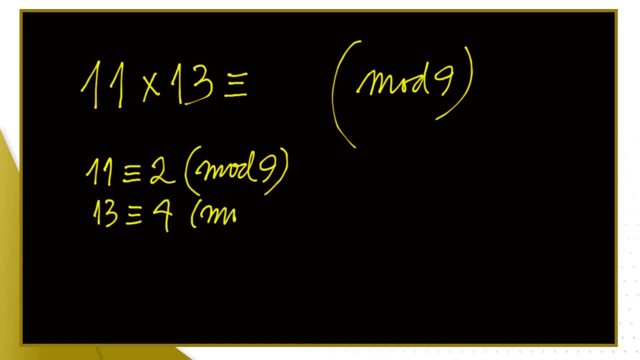 13 is congruent with 4 mod 9.. And the product 11 times 13- and no time avoiding doing the multiplication, because I don't have to- will be 2 times 4, which is 8 mod 9.. Okay, 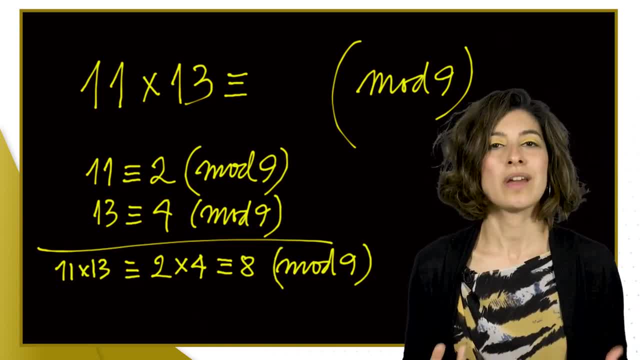 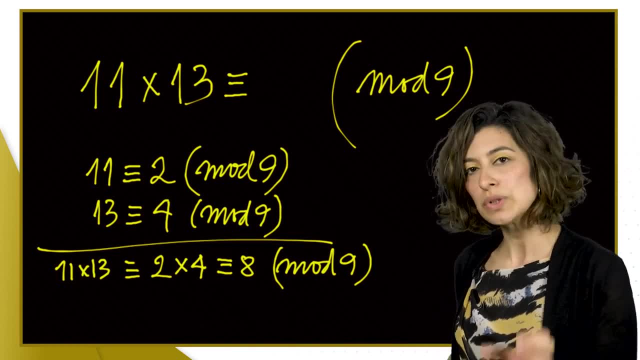 So this is what we're going to do every time we have multiplications to do in mod in modular arithmetic. We will just try to keep the numbers low and, when possible, calculate the remainders individually and then just do the multiplications together. 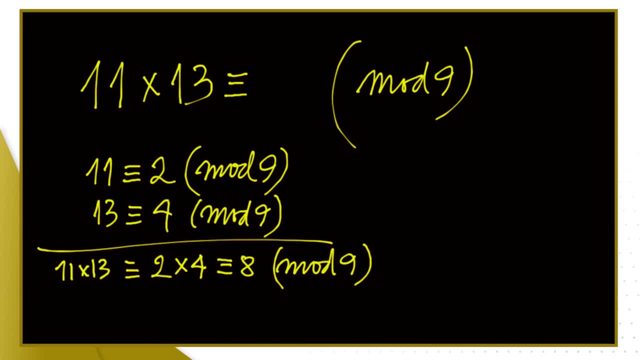 Right, I didn't quite tell you why we can do this. I'm not going to prove it, but I'll give an idea of why this works. The fact that 11 is congruent with 2 mod 9 means I can write 11. 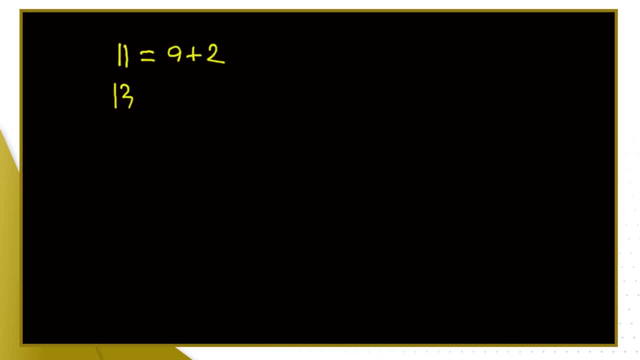 as 9 plus 2, and 13 is congruent with 4 mod 9.. So it's 9 plus 4 in this case, And multiplying 11 by 13,. I'm just going to do that carefully. here is the same as multiplying. 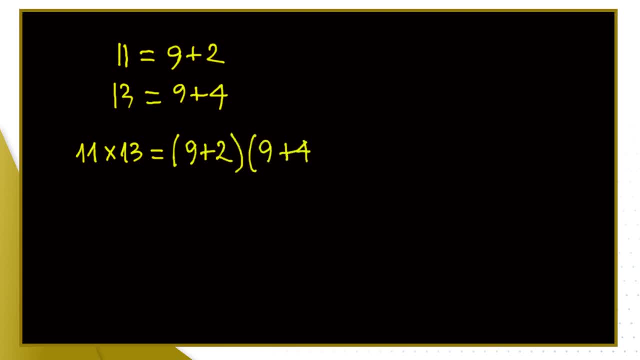 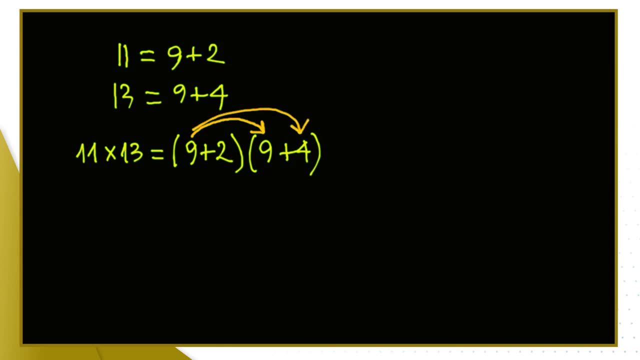 9 plus 2 times 9 plus 4.. And that means I would distribute 9 times that 9 and 9 times that 4.. And then do the 2 times that 9 and the 2 times that 4.. 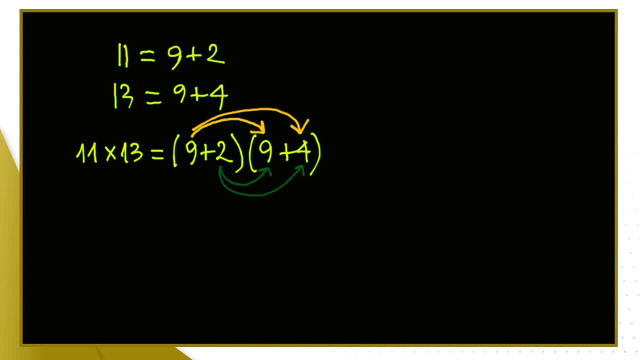 And that would give me- I'll just do all the terms bit by bit- 9 times 9.. Again, I'm avoiding doing the multiplications 9 times 9, I'll do plus 9 times 4, plus the 2 times the 9. 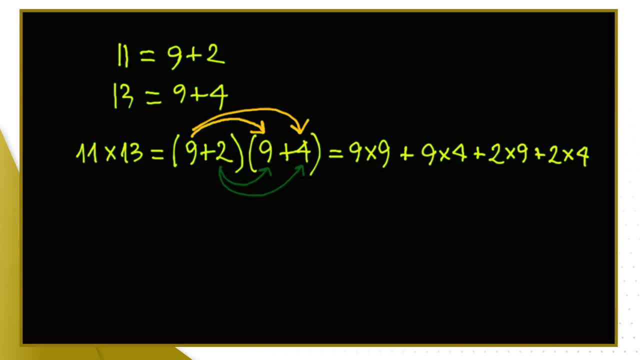 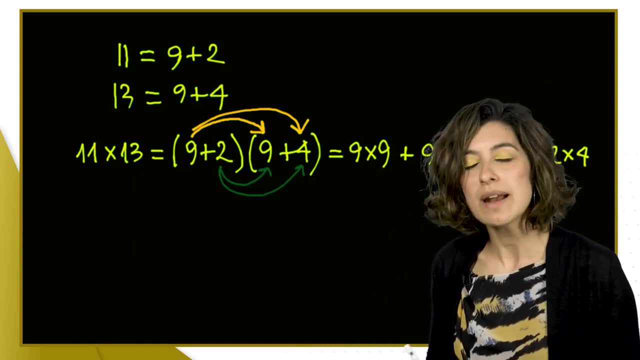 plus the 2 times the 4.. Now I didn't do the multiplications because I'm looking into mod 9.. That means I don't care about multiples of 9.. Multiples of 9 are going to get out of my way. 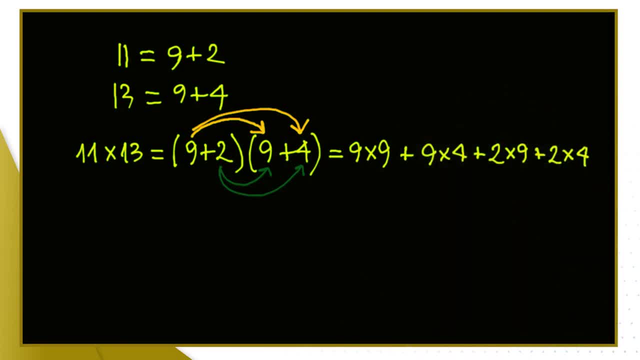 and all I'm going to concentrate is on the remainders. Now I've got here: 9 times 9 is a multiple of 9.. 9 times 4 is a multiple of 9.. 2 times 9 is another multiple of 9.. 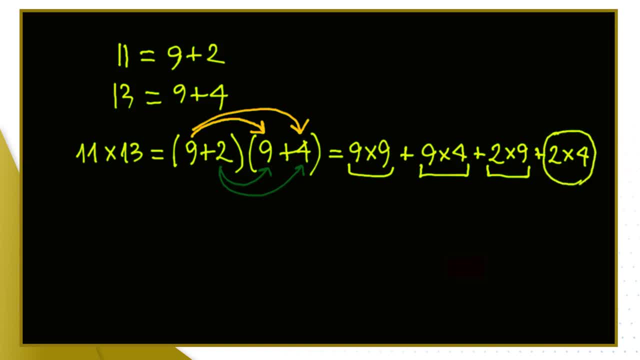 And the remainder is going to be this guy here 2 times 4.. So what I'm saying is that 11 times 13, because it is a multiple of 9 plus 2 times 4, so when we're calculating 11 times 13 mod 9,. 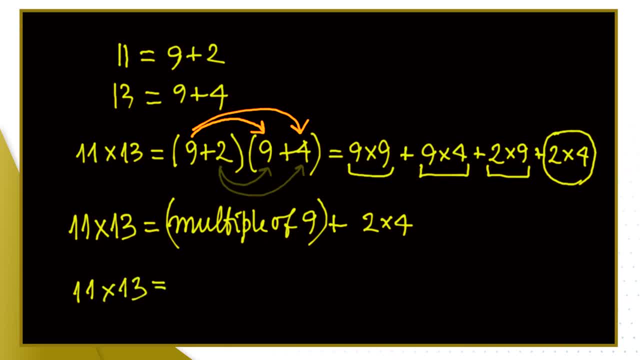 we have the same remainder as 2 times 4, which is 8 mod 9, because we threw away this multiple of 9 here in the calculation. So this is a generic example that gives an idea of how we prove this result. 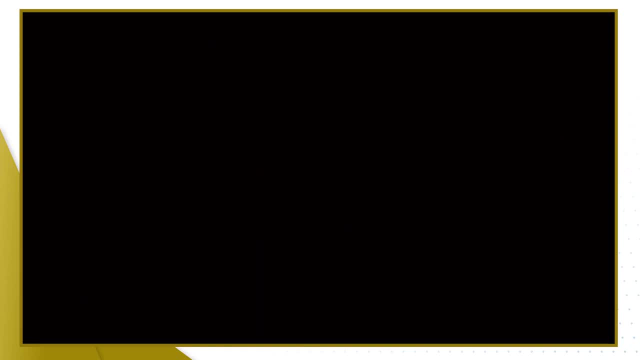 And this result. I'm just going to summarize it with variables. So if we have a that is congruent with c mod some n, and we have another number, b, that is congruent with d, for the same n, and I want the multiplication of a times b, 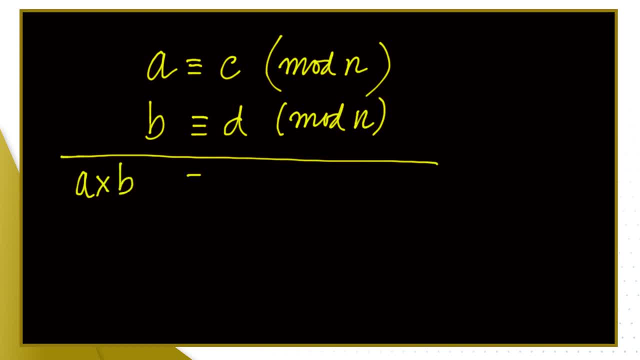 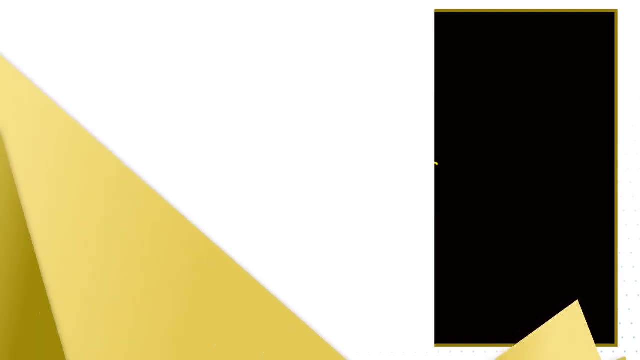 but I want the remainder of division by n, so all I have to do is multiply the remainders and then calculate that mod n. This is what I meant with the rule I applied in the last example. Let's look in more detail at mod 5,. 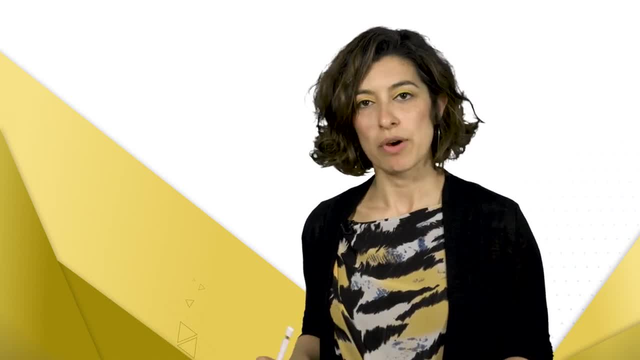 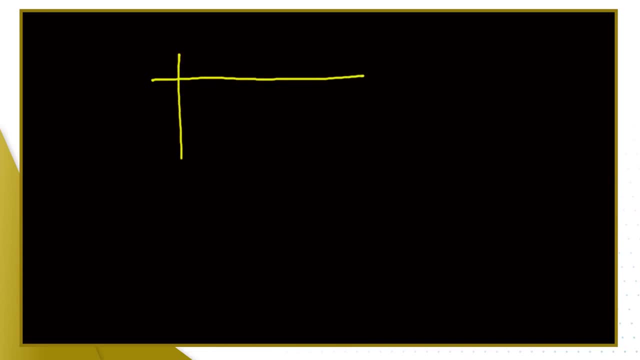 and we're going to write the multiplication table in mod 5.. The remainders of division by 5 are just numbers from 0 to 4.. That's all I need to write on my multiplication table And we are doing mod 5,. 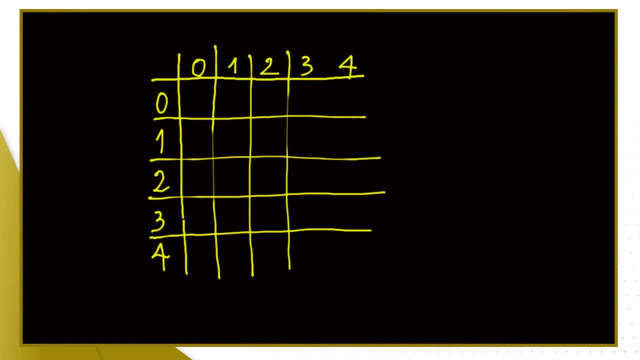 so we're going to multiply this out and write the remainders of the result. There we are. So 0 times all the other guys gives 0,, because every time you multiply a multiple of 5 by another number, you still have a multiple of 5.. 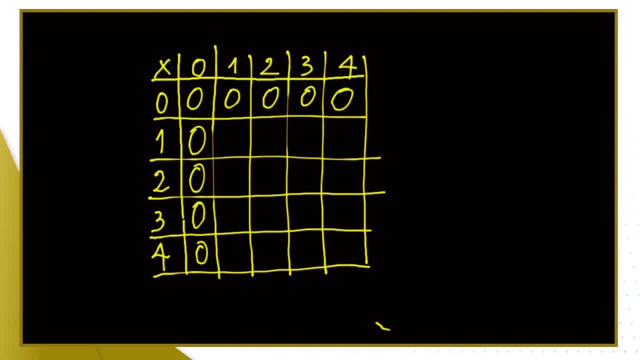 So all these bits here will be 0, and this is mod 5.. And then let's have a look. We're multiplying 1 by the other numbers. 1 times 1 is 1,, 1 times 2,. 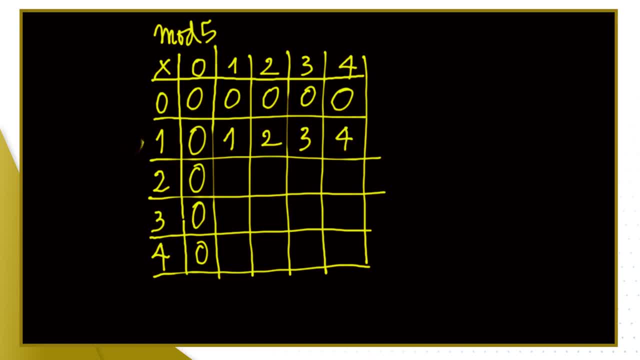 1 times 3, 1 times 4,. no surprises there. The same happens on the other, on the column of 1.. 1 times 1, 1 times 2 is 2,, 3,, 4,. 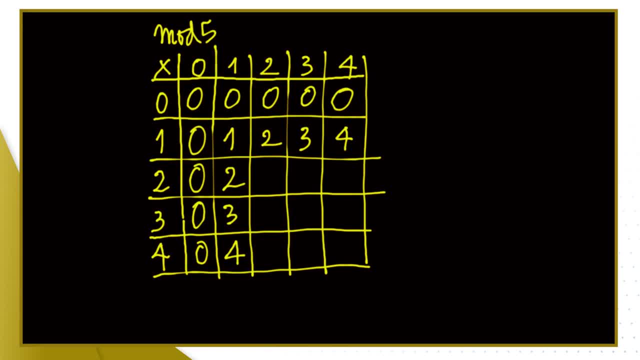 there we are Now for the row of 2,. 2 times 2 is 4,. 4 has a remainder of 4, mod 5.. 2 times 3 is 6,. 6 has a remainder of 1,. 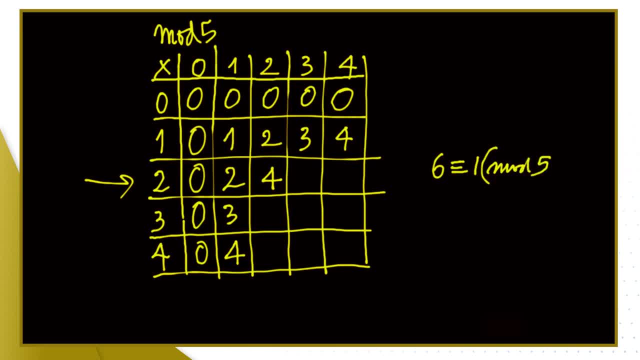 mod 5. So we write 1 there, And 2 times 4 is 8, 8 has a remainder of 3, mod 5.. So right there, And similarly on the column of 2, I've got 2 times 3,. 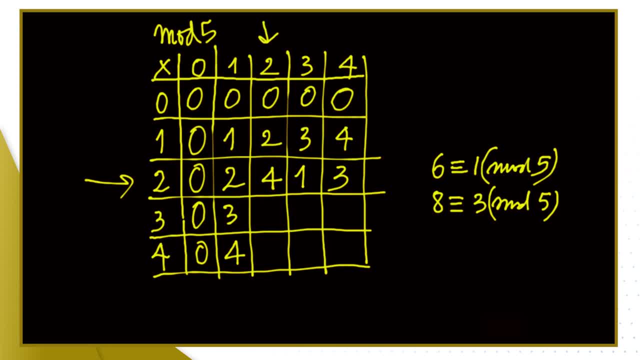 which is 6, is 1, mod 5.. And 2 times 4 is the same one as before is 3, mod 5.. So now mod 5.. On row 3, I've got 3 times 3,. 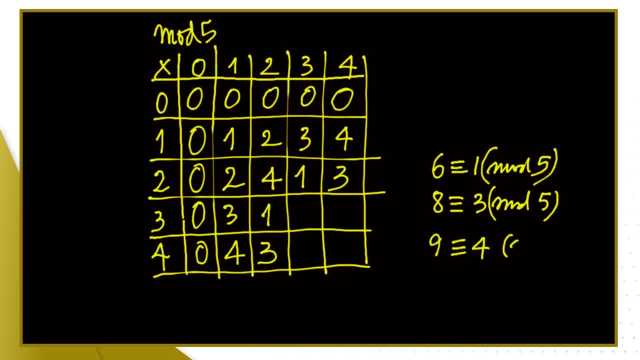 which is 9,. 9 is congruent with 4, mod 5.. And then 3 times 4 is 12,, 12 is 10 plus 2, so it's 2, mod 5.. And that means I've got a 2 there. 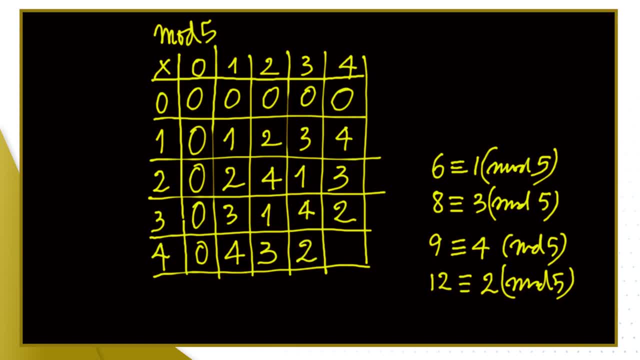 And similarly I've got a 2 on this 4 times 3.. And 4 times 4 is 16,. 16 is 15 plus 1,. therefore I get 1, mod 5.. And that's the complete multiplication table in mod 5.. 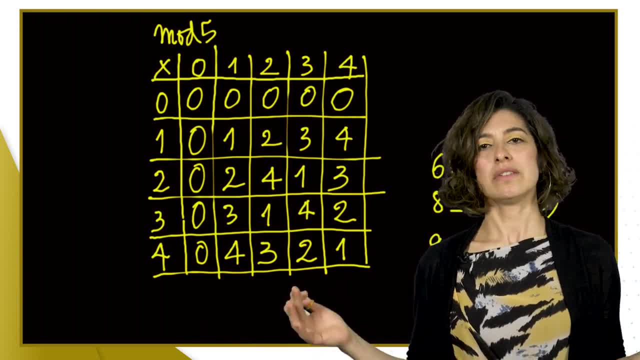 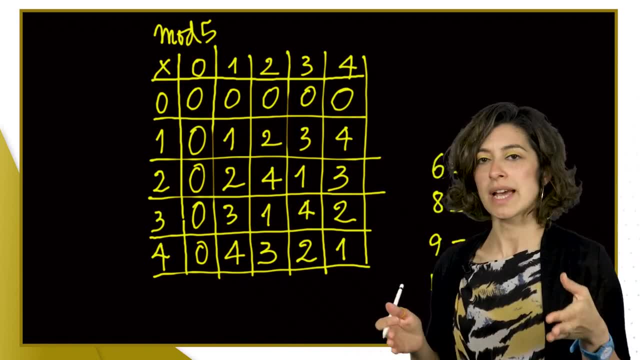 And you wonder: what if I've got bigger numbers than 4?? How do those numbers fit in the multiplication table? Remember, we boil the number down to the remainder of mod 5, and then there will be an answer in the multiplication table. 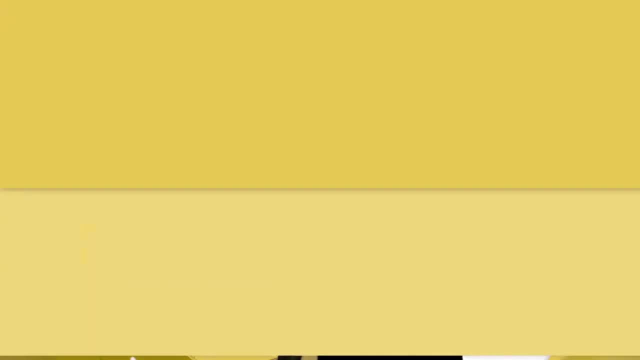 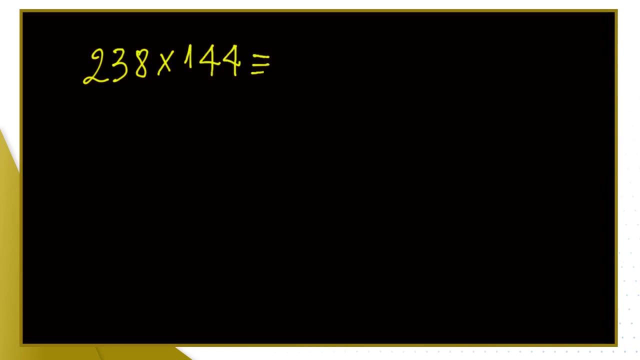 One final example on mod 256.. We're performing 238 times 144.. What is the smallest positive number that is congruent with this mod 256? Let's have a little think. In this case, both numbers 238 and 144,. 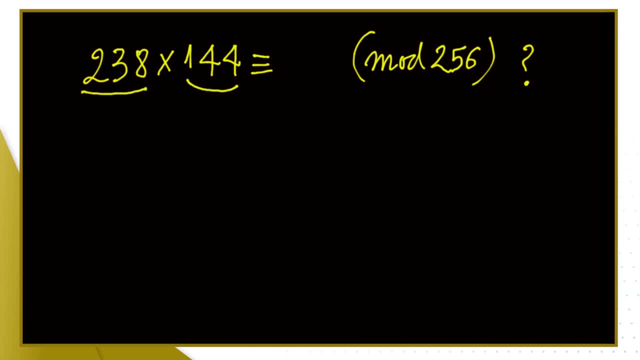 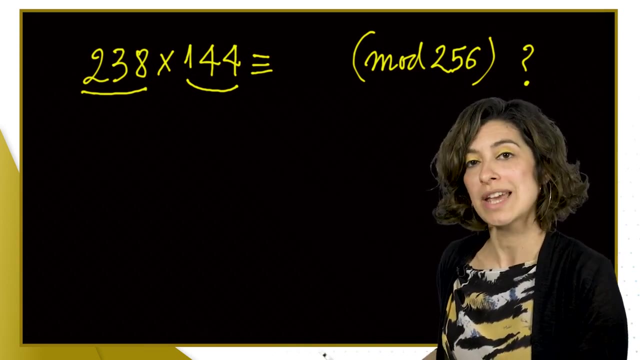 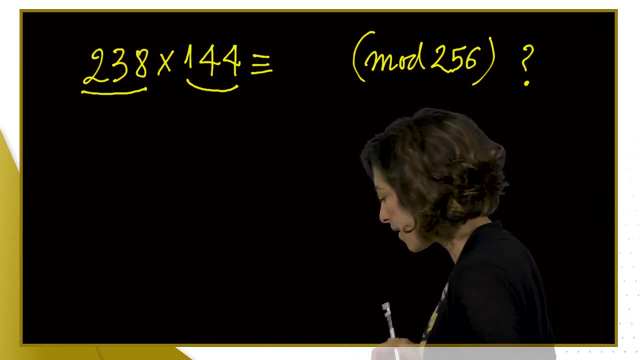 are congruent are smaller than 256. So these numbers are already remainders of division by 256. In this situation it might be easier to perform the multiplication and then work out the remainder, like we did before. So we're going to have a little help from our calculator now. 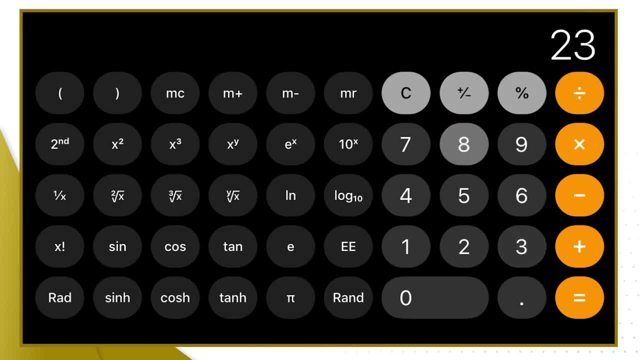 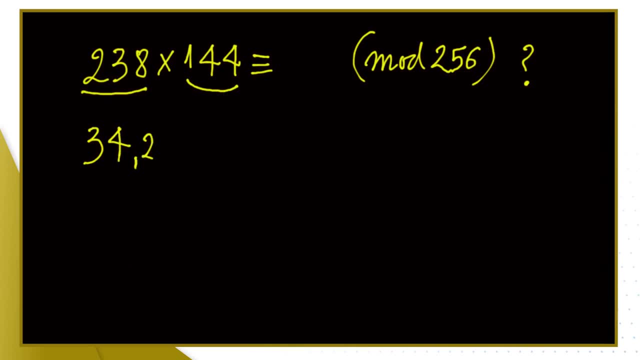 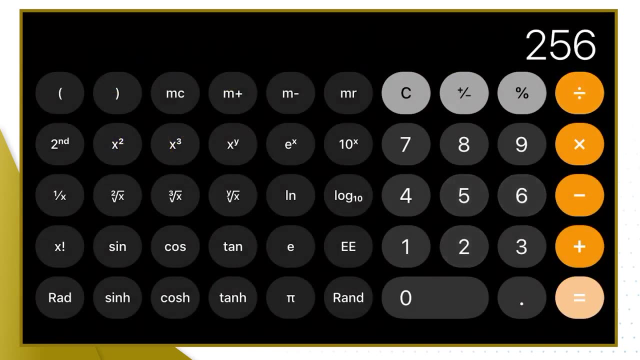 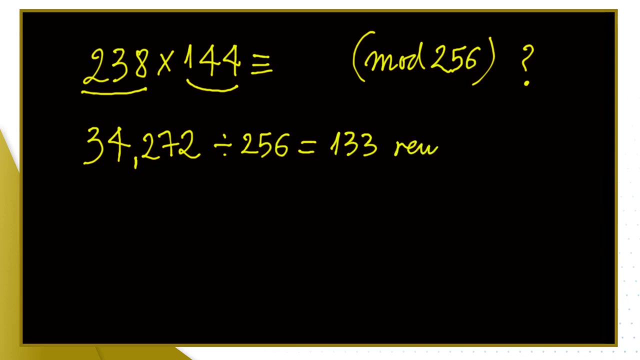 We're going to do the multiplication there, just to speed things up, And we multiply by 144.. That's, we get 34,272.. That number divided by 256, we have 133, and then let's work out the remainder. 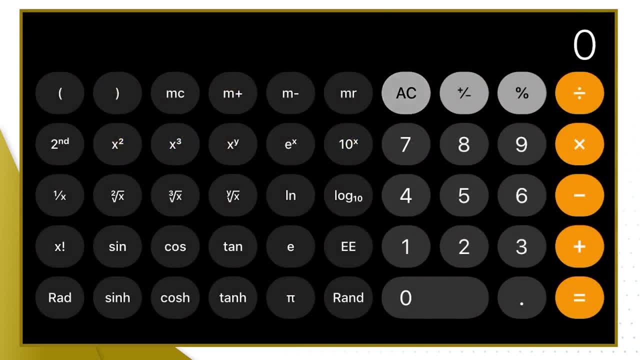 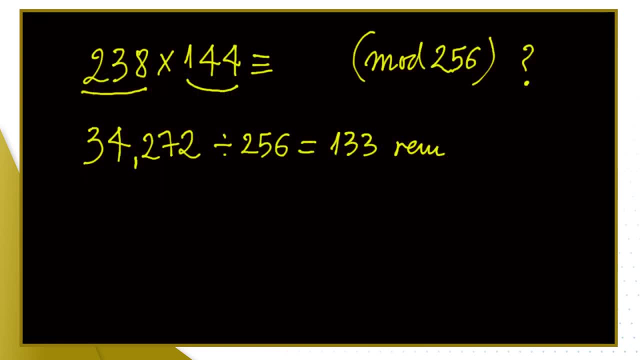 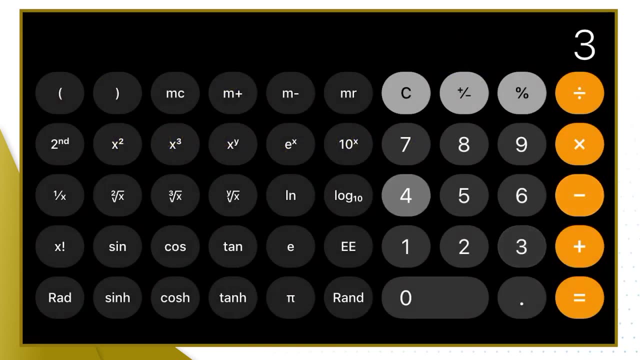 Once again, we take the integer part 133, multiply by 256, which is the mod, And we're going to take that away from the original number. So we're going to take that away from 34272.. And we have 224. 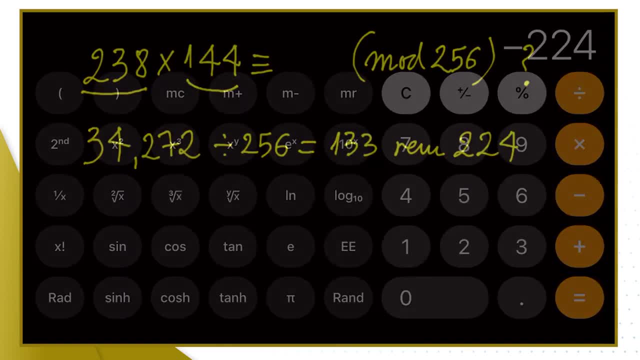 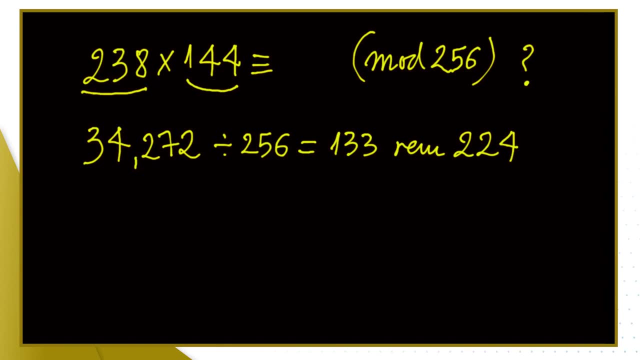 as a remainder. Don't worry about that minus there. I did 133 times 258, minus the original number, instead of the other way around. That's where the minus comes from. Okay, So the result is 224 mod 256.. 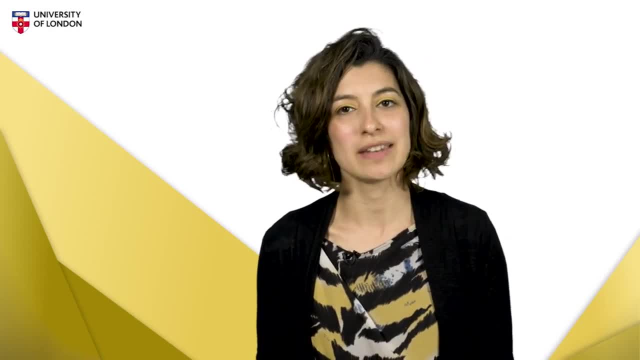 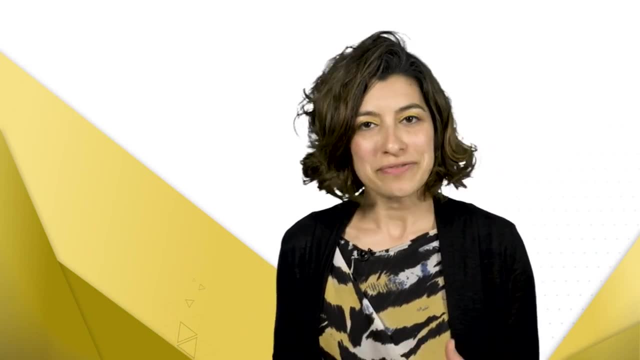 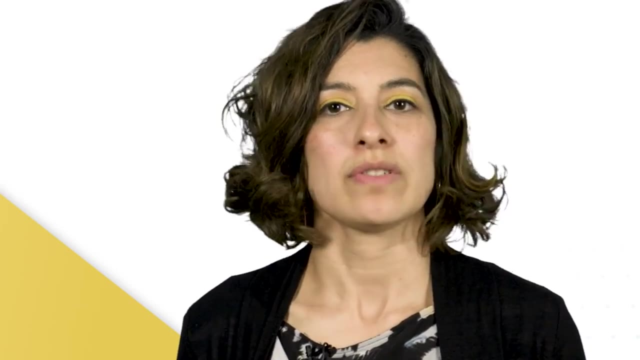 Hello, We're going to look at multiplication again. This time we're going to look at the multiplicative identity And multiplicative inverses in modular arithmetic. In normal numbers the number 1 has a special property When you multiply 1 by any other number. 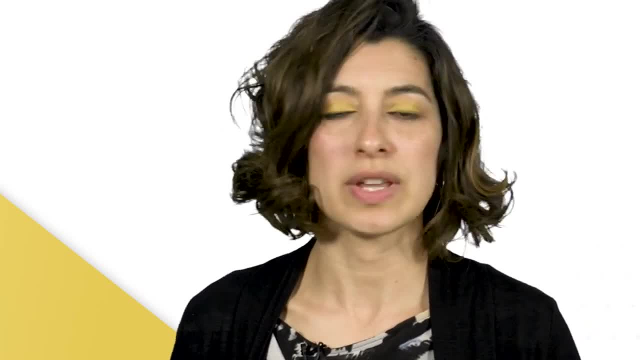 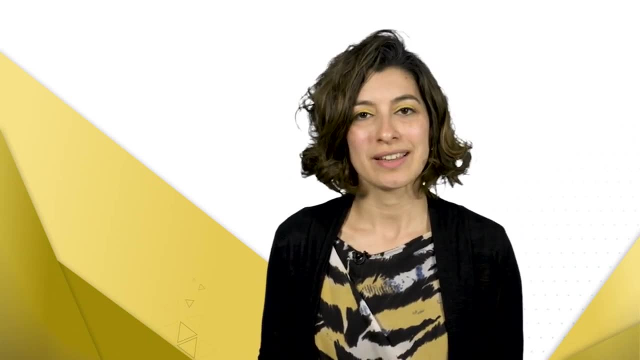 it doesn't change that number. So 1 times 3 is 3,, 1 times 10 is 10, and so on. 1 is the multiplicative identity for normal numbers, Because it's that number that we multiply by others. 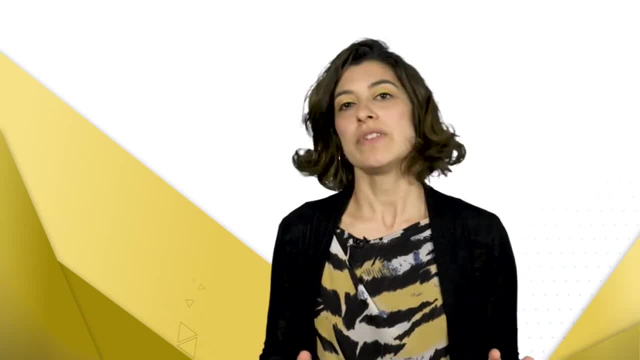 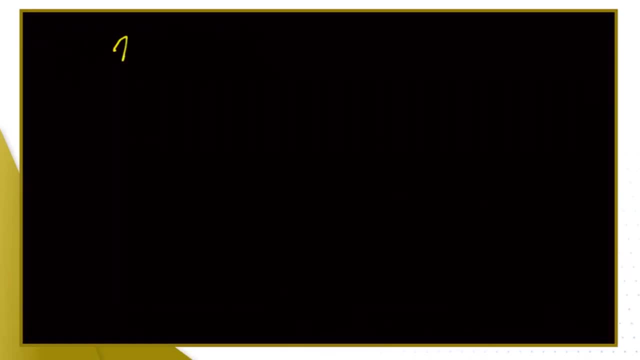 It doesn't change them. In modular arithmetic we want that property too. So we're looking at, say we're on mod 5. We're looking at a number that, multiplied by 2, still is 2 mod 5.. We're looking at a number 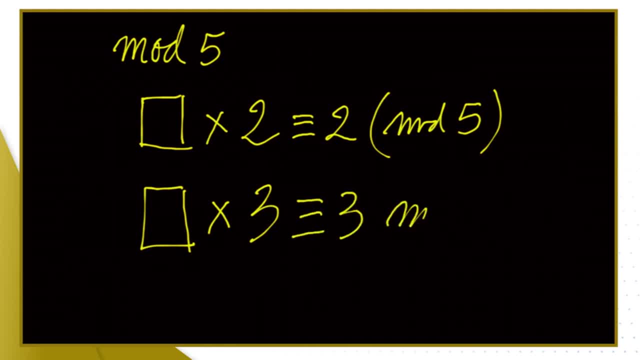 that when multiplied by 3 is still 3 mod 5.. Well, let's try: 1. Does 1 work? 1 times 2 is 2.. Yep, 1 times 3 is 3, and so on. 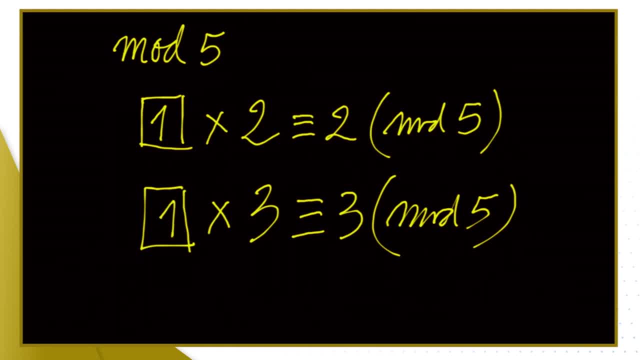 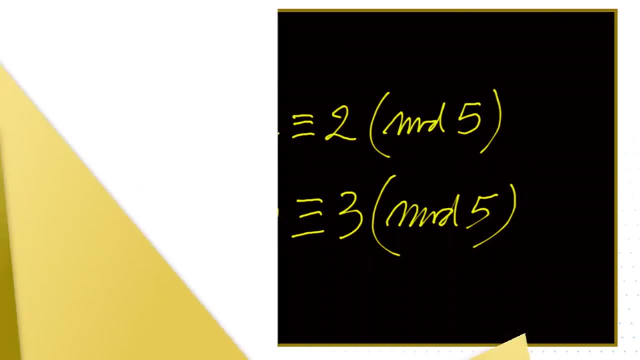 1 is the multiplicative identity in modular arithmetic for any mod we consider. So now that we know what the multiplicative identity is in modular arithmetic, let's look at inverses and what that means. Let's focus on mod 5 for now. 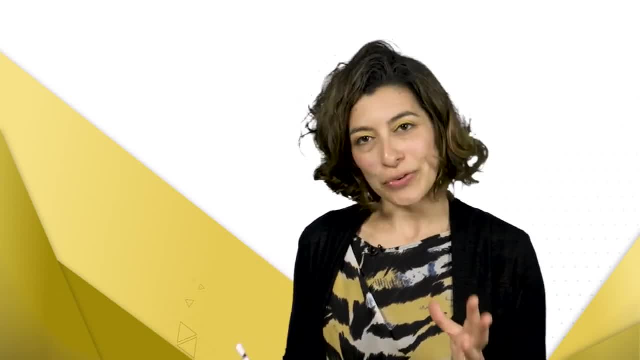 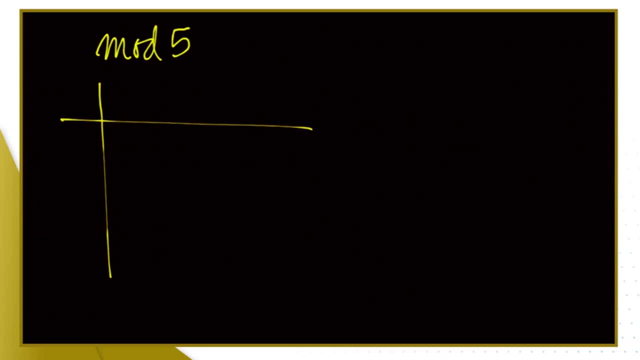 In mod 5, we have a number that is the multiplicative identity of any number. In mod 5, we already looked at the multiplication table. I'll just copy it here again. I didn't copy the 0 row and the column row. 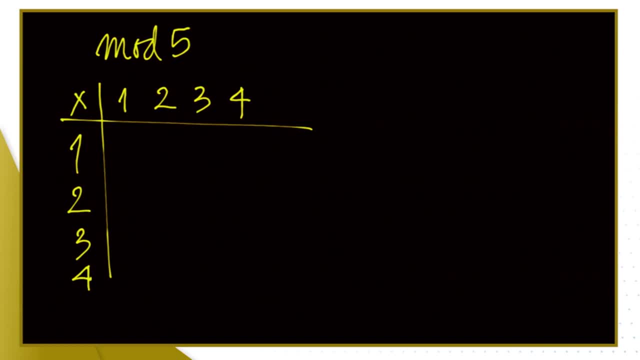 because that's not going to be of interest for now, So let's focus on these numbers. The multiplication table here it is: 2 times 2 is 4.. 2 times 3 is 6.. 4 times 3 is 6,. 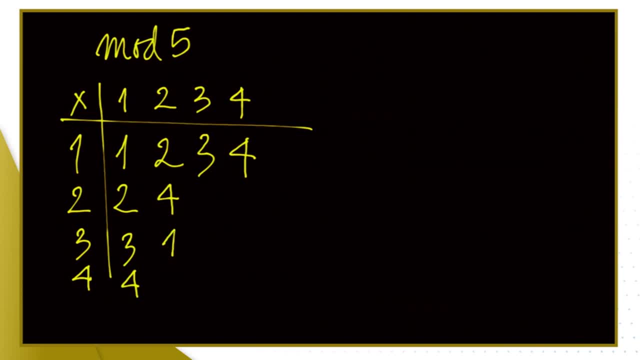 which is 1.. 4 times 2 is 8,, which is 3.. And now I've got: yeah, 3 times 3 is 9,, which is 4.. 12,, which is 2.. 2.. 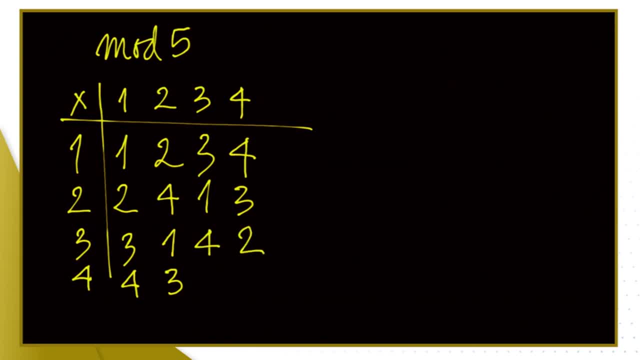 And 4 times 4 is 16, which is 1.. OK, So I've got the multiplication table for mod 5, and I have excluded the 0, because 0 times any of the other numbers gives me 0. So now I've got. 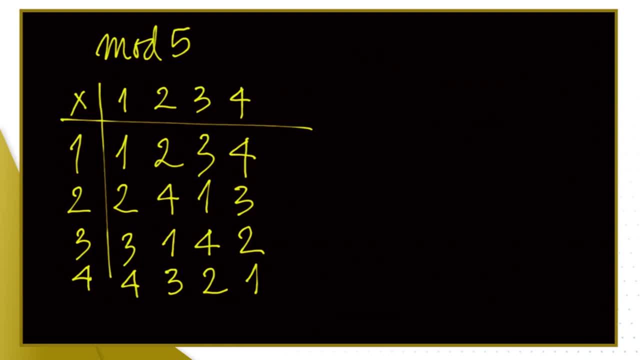 the multiplication table for mod 5, and I have excluded the 0 because 0 times any of the other numbers gives me 0. So that's not interesting for now And we're focusing on multiplicative identity, which is number 1.. 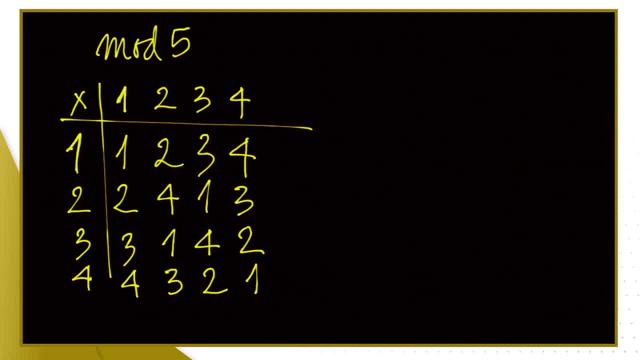 And we're looking for multiplicative inverses. Let's just remember for a second what happens with linear numbers. In linear numbers it makes sense to talk about inverses. That means, if I've got 2, what number times 2 gives me 1?? 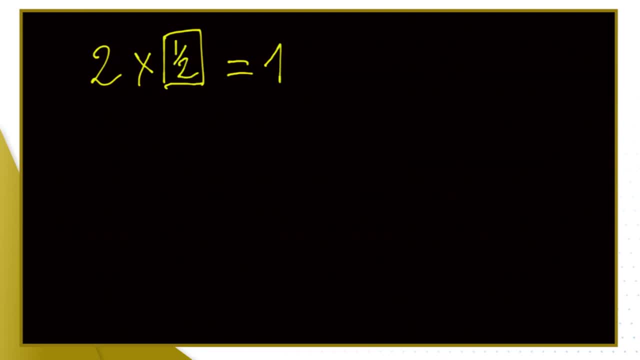 1 being the identity, And that is number 1 half. So 1 half is the inverse of 2, because when I multiply it together I get the identity. Similarly, for 3, the inverse is the number that multiplied by 3. 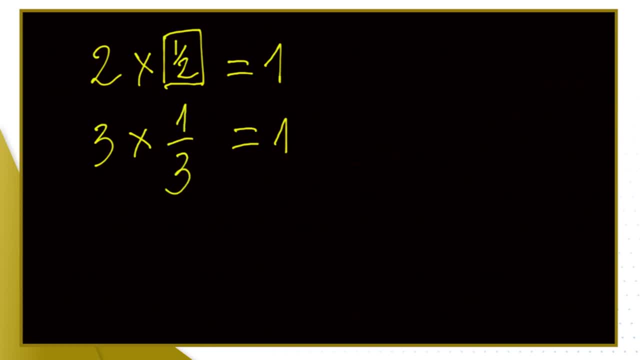 gives 1, which is 1 third, And at the same time 3 is the inverse of 1 third, because 3 times 1 third gives 1.. So that means 3 and 1 third are inverses, 2 and 1 half. 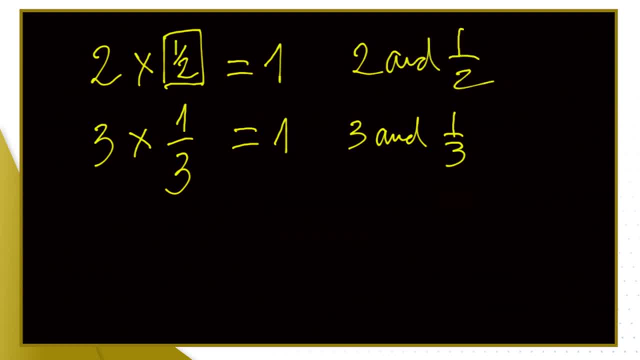 are inverses and so on. I'll just note that a half is sometimes written as a power, So a half can be written as 2 to the minus 1, and a third can be written as 3 to the minus 1.. 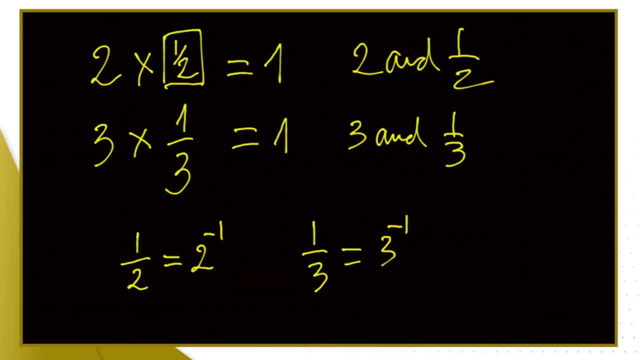 And that minus 1 in the power is an indication for inverse. You invert the fraction, but also in terms of multiplication it means it's an inverse. So we're going to grab the idea back to modular arithmetic. So on mod 5,. 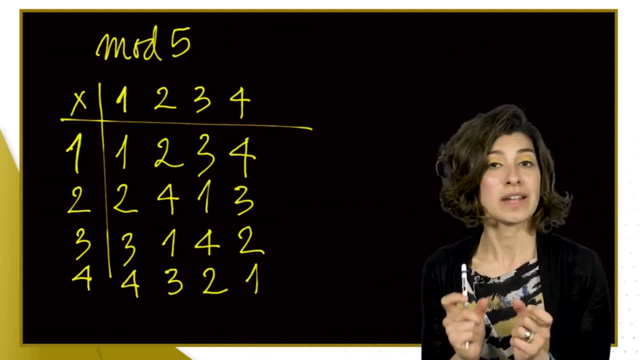 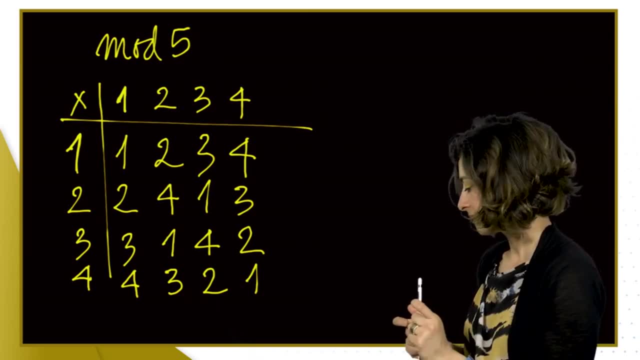 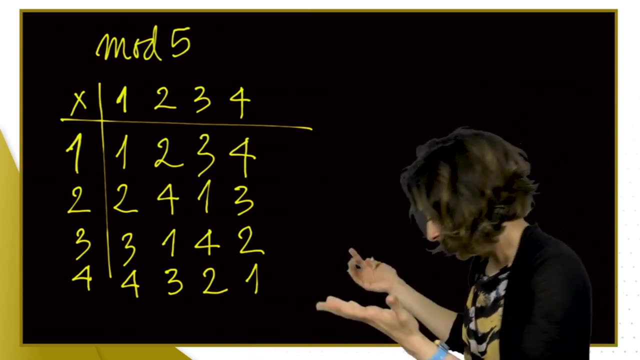 we want to know what are the pairs of numbers that are inverse for multiplication. What are the pairs of numbers that, multiplied out, give 1?? Well, look again at the table. What pairs of numbers multiply out to 1?? There we are. 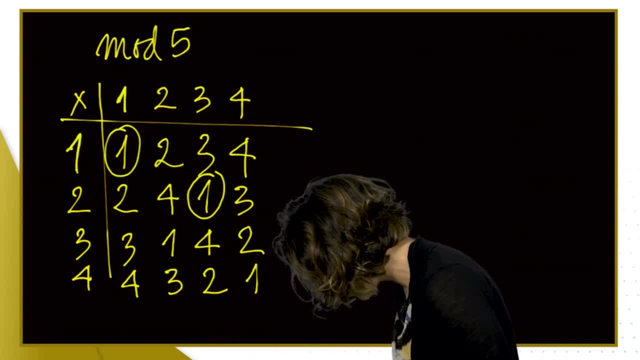 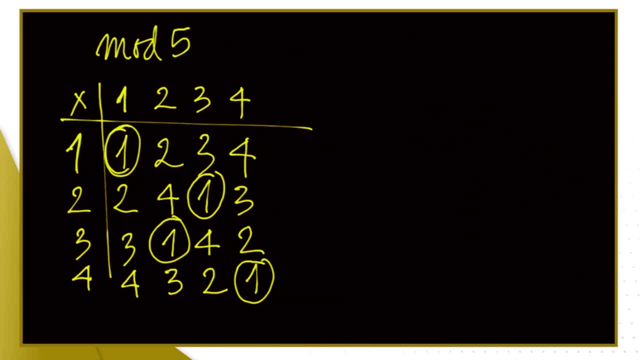 Everywhere in the table you find a 1.. That tells you what pairs multiply out to 1.. It tells you what are the pairs of inverses. Well, I've got a 1 that comes from 1 times 1, being 1 mod 5.. 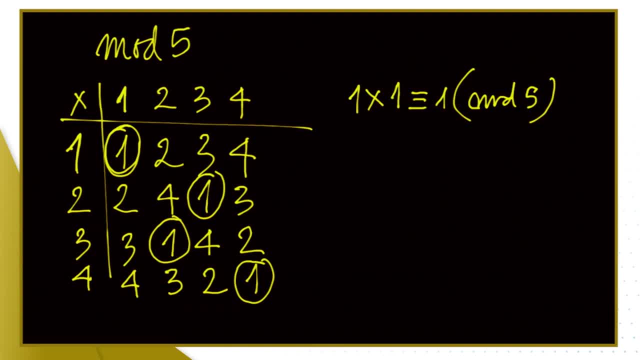 That's fine. We've got a 1 that comes from 2 times 3.. So 2 times 3 are inverses mod 5. And same with 3 times 2.. I'll just write it down. And 4 times 4. 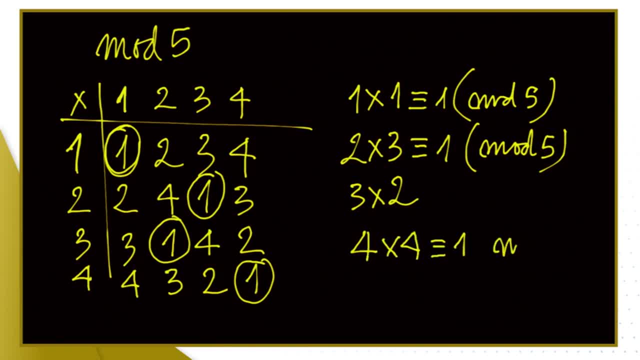 congruent to 1 mod 5.. So 2 and 3 are inverses, mod 5 and 4 is inverse of itself, mod 5.. I'll write that down: 2 inverse is 3 mod 5. That means the inverse. 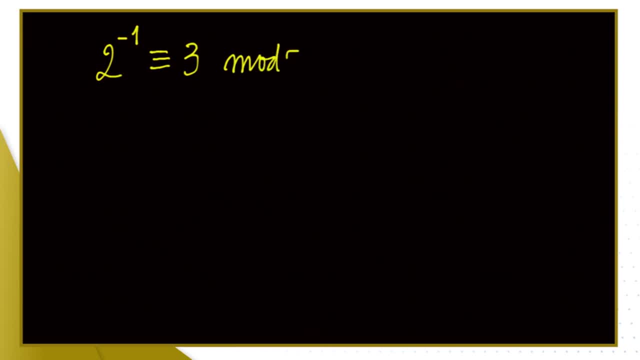 of 2 is 3.. 3 inverse is 2 mod 5.. That means that the inverse of 3 is 2 and 4 is an inverse of itself, mod 5.. So 3 is 2 mod 5.. That means 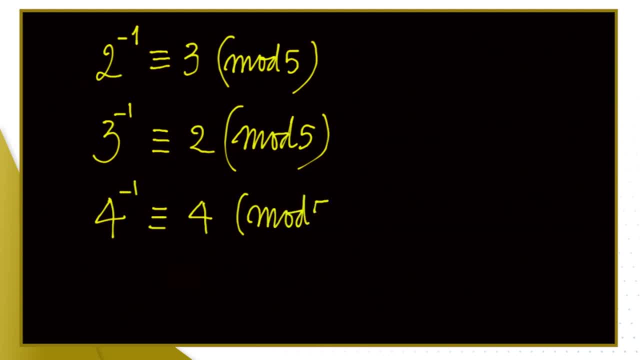 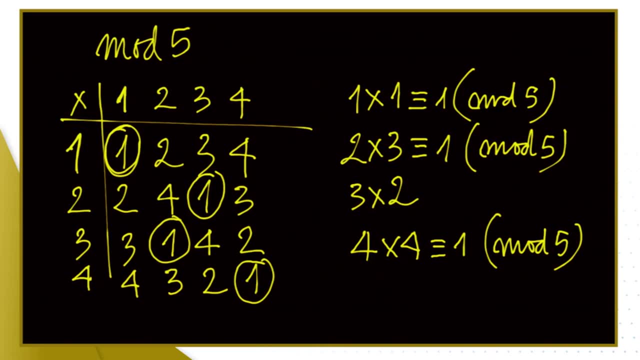 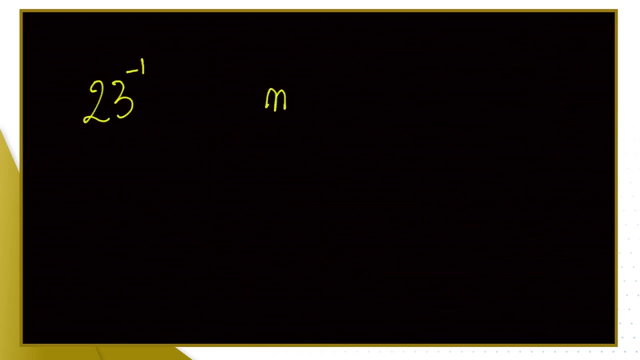 that the inverse of itself is 3.. And 2 is 3 and 4 is 3.. So I can write that down. So that's all for this video. Thanks and goodbye. 5.. What's that inverse? Not a problem, because, as before, 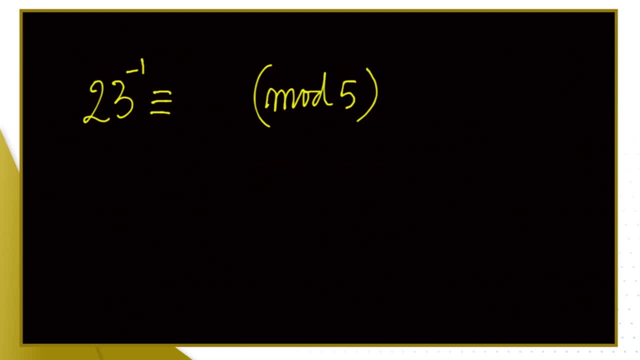 if the number we're working with is larger than the remainders you allowed, then we calculate the remainder: 23 is 3 mod 5 and therefore, when we're looking for the inverse of 23, we are looking for the inverse of 3.. 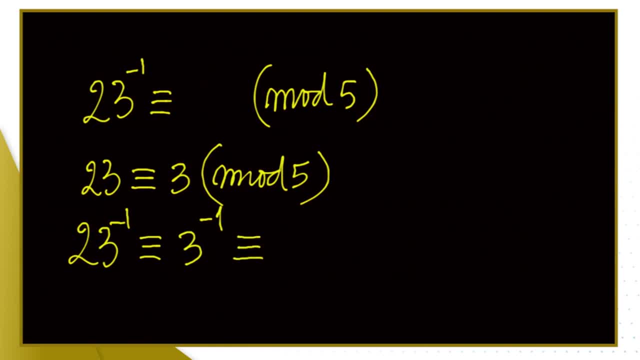 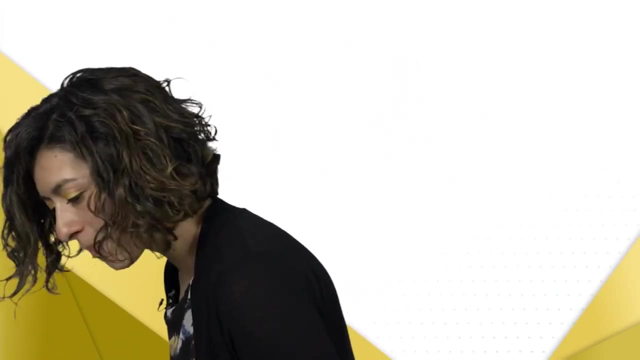 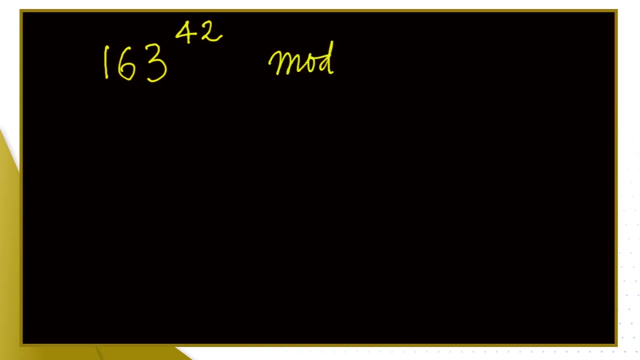 And we just saw that the inverse of 3 is 2 mod 5.. Let's look at another example. Say I wanted to calculate this big power. I've got 163 to the power of 42 mod 49. So that's the first thing I'm asking you to calculate. 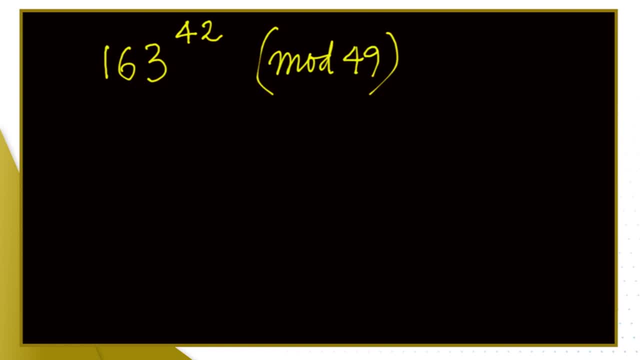 163 is a large number, and it's a large number in the sense that it's bigger than 49, the number in the mod. So the first step is to reduce that number to the smallest integer congruent with it, mod 49.. So we do 163. 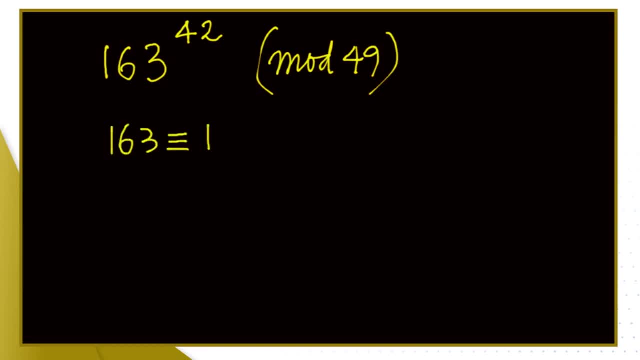 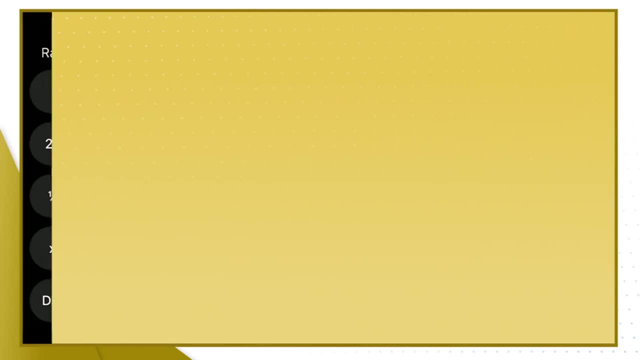 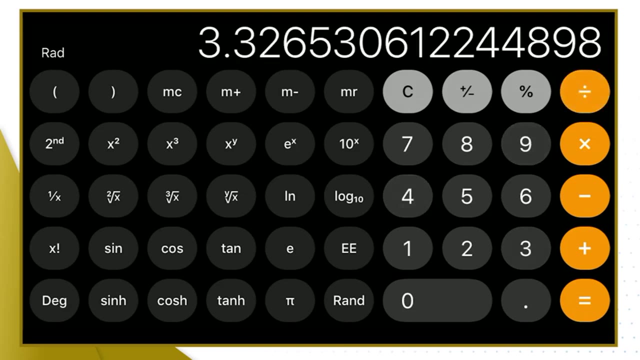 is congruent with 16 mod 49, and I'll show you in the calculator: 163 divided by 49, the whole part is 3, so I do 3 times 49 is 147, so I need to do 163. take away 147. 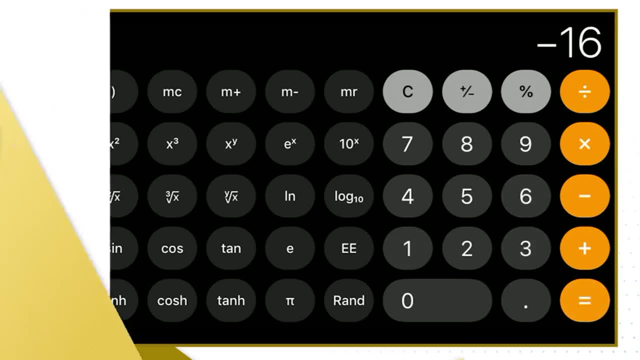 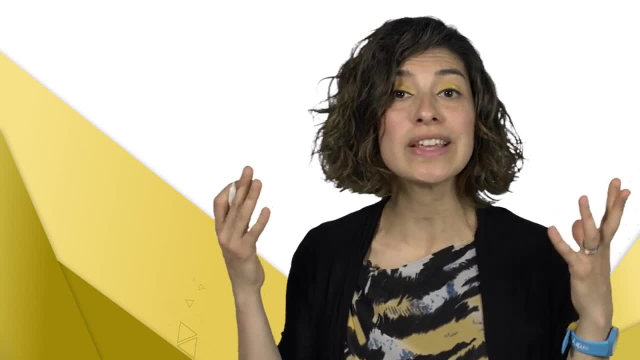 and that is 16.. That's how I got the remainder. Now, the clever bit here is that, instead of doing powers of 163, I'm gonna do powers of 16 and I'm going to build them up until I get to our big, big power, the power of 42.. 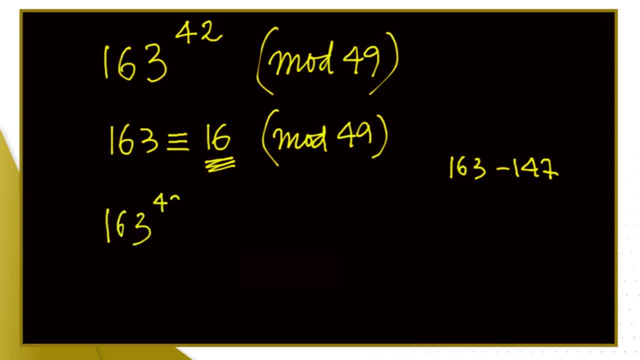 So I'm saying is that 163 to the power 42 is congruent with 16 to the power 42 mod 49. So I'm reducing the calculations to working with powers of 16.. Let's do it on a new sheet. So 16 squared is 256.. That is larger than 49.. 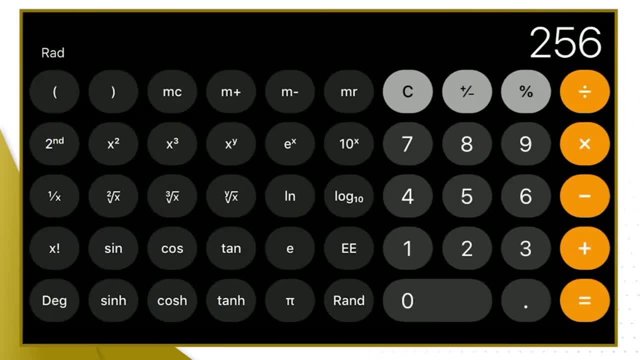 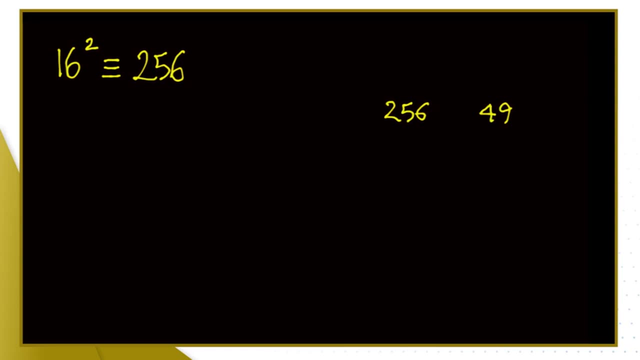 So let's do that on the calculator: 256 divided by 49.. I could do divided by 49,, but you're probably screaming that we know how much that is. Yeah, we could do 259.. How many, how many? multiples of 49, 15 to that. Look at that. 59 is almost 50. It's 50 minus 1.. 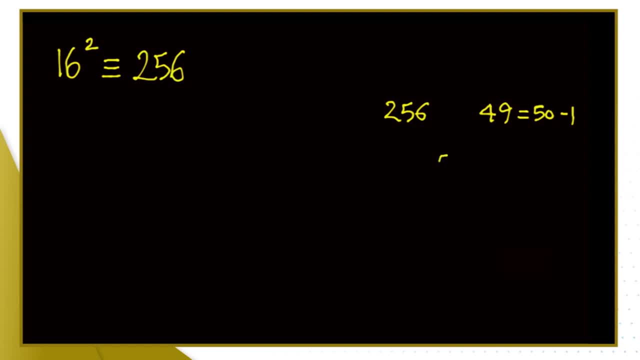 So we could do 5, 49,. 49 is going to be 5, 50s minus 5.. So it's going to be 250 minus 5.. So that's going to be 245. And so the remainder is going to be the same as taking away the 245 from it, which is 11.. 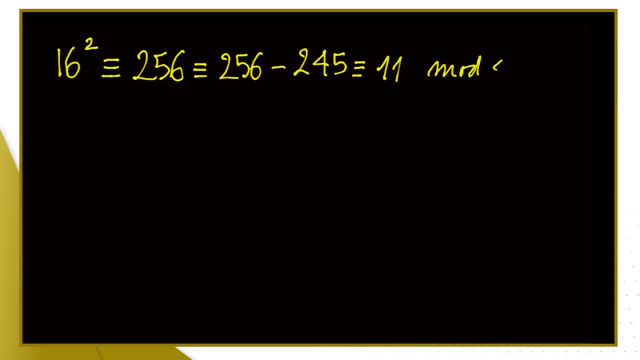 11.. Mod 49.. Now we're going to do the next power of 16.. We're going to do squares, of squares. So if I do 16 squared, squared again, I get a power of 4.. I'll just write here as a reminder of what we did. 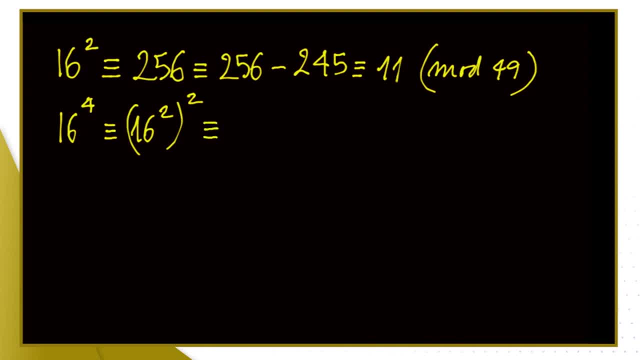 And the beauty of this is that now I do 16 squared was 11.. So this is 11 squared, which is 121.. And I had to do the first square. Okay, so I do that, So what I call 16 squared. 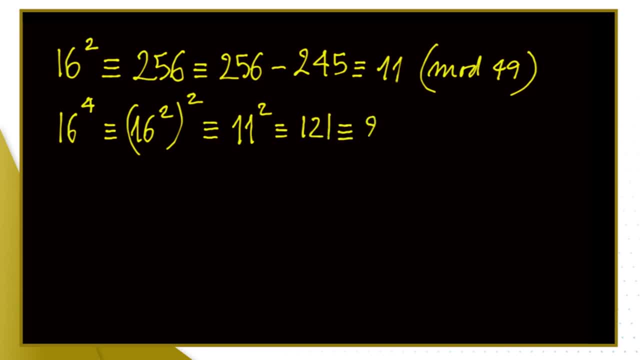 So how much is 3? Francisco roots on the 28th 3, which if you take away twice 49,, you get a remainder of 23.. And we keep going, we keep going. Let's do 16 to the power of h. 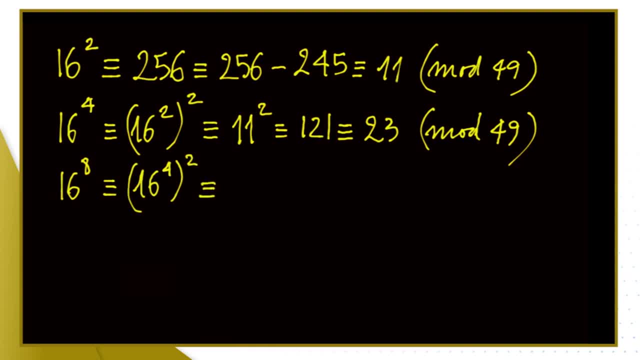 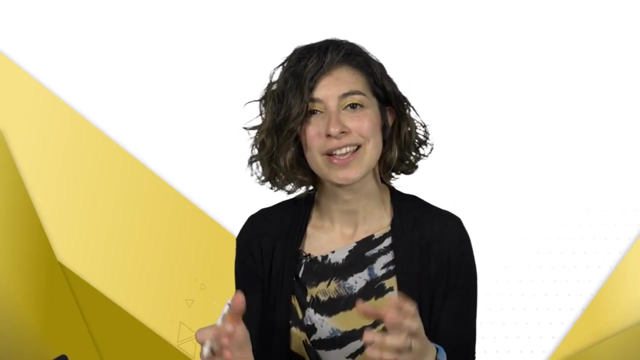 That is the square of the previous. just as a reminder, here is a square of the previous one, And that means I can replace…. and that gives us 529, which is the takeaway. multiples of 49 is remainder 39 mod 49. now 39 is quite close to 49. so instead of working with a positive remainder, I'm gonna work with 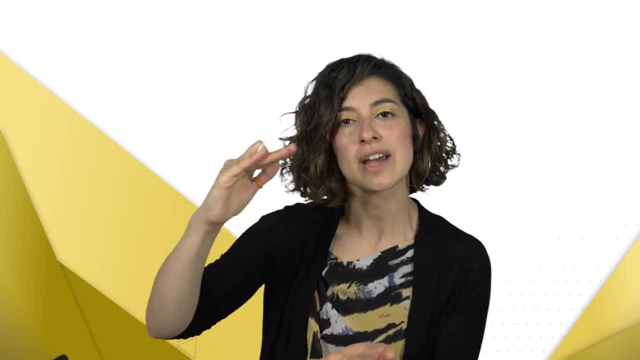 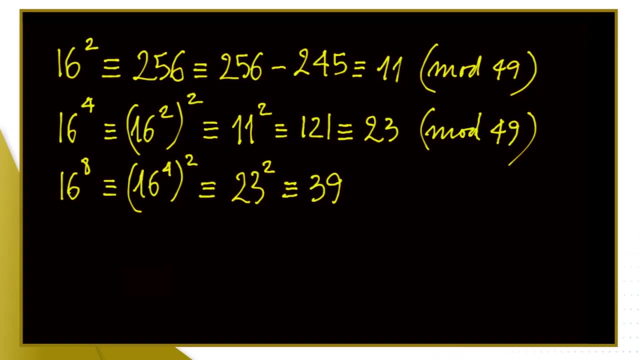 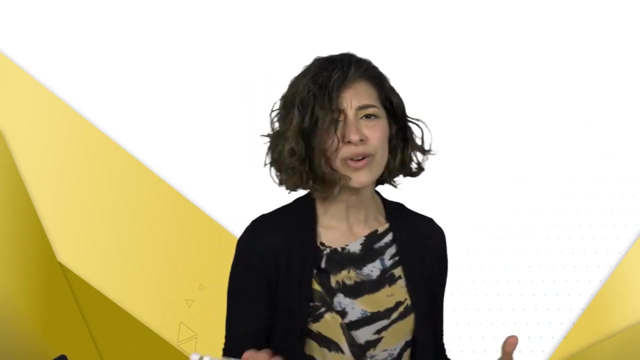 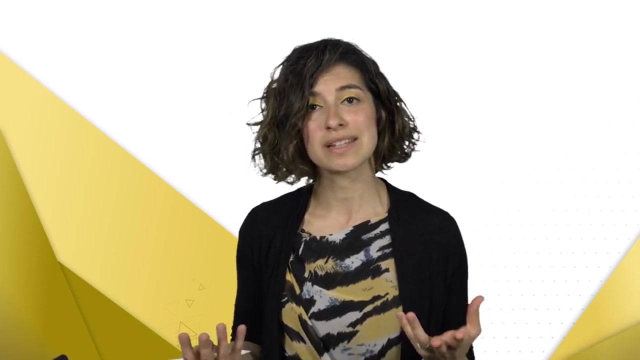 a negative remainder because although I've got a remainder of 39 over 49, it's 10 short from the next multiple of 49. so this is minus 10 mod 49. why on earth do I want a minus 10? 10 is very easy to the powers, isn't it? and I've got minus, so if I do a square of minus 10, I'm. 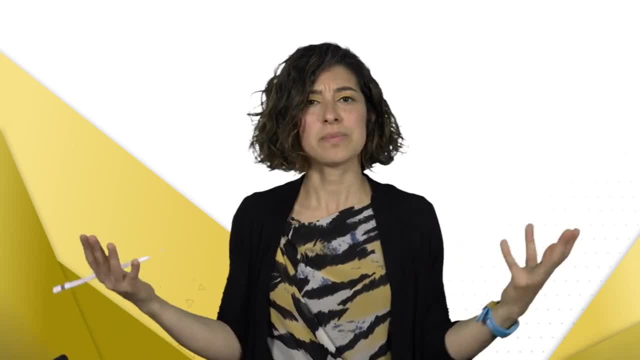 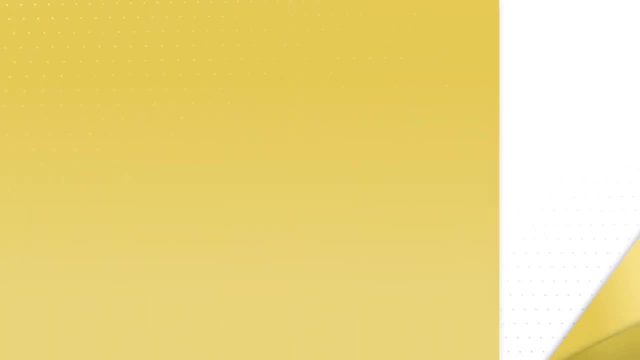 gonna have. the square of 10 is gonna be the same, it's gonna be a hundred, so you easy to work with and it's good to work with small numbers when you're doing big power. so let's, let's go with it. now we could do 16 to the 8 squared again, or we? 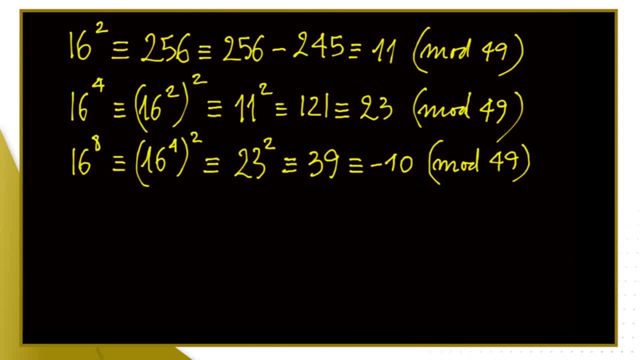 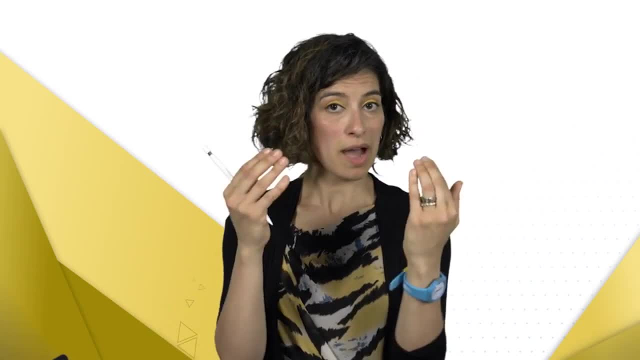 could do a different operation. let's keep in mind what's our goal. our goal is to get to power 42. we've got power 8. if we could get to power 10, then we would just raise it to the power 4 again. it would be very close to 42. so I'm gonna. 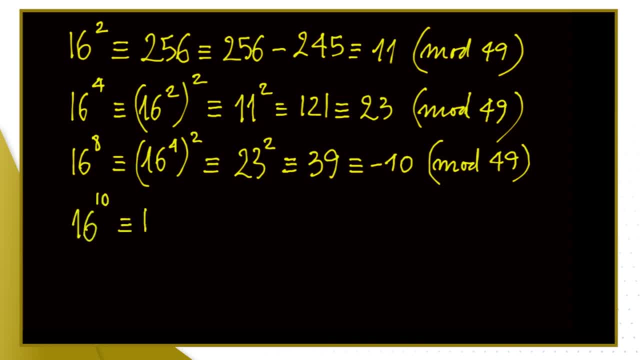 do 16 to the power of 10, 10, by noting that that's 16 to the 8 times 16 to the square, and we had calculated these numbers before. so 16 to the 8 is congruent with minus 10 and 16 squared is congruent with 11. 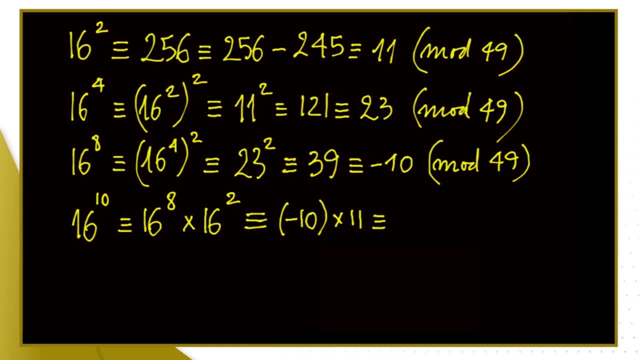 so that is going to be minus a hundred and ten. but again I want a remainder mod, which means we could just add twice 49 to it. so add 98 and that will give us minus 12 mod 49. if you add another 49 to it you get a positive remainder. but 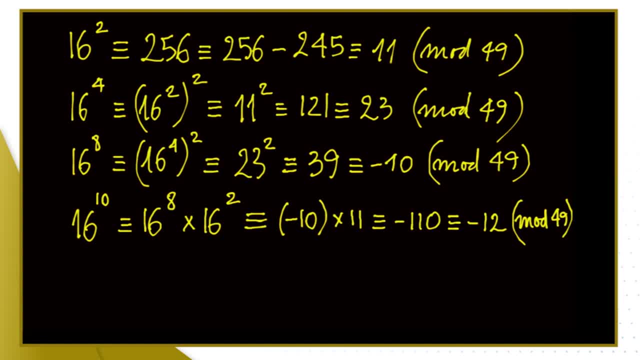 minus 12 is quite nice because it's still a small number in magnitude. now here's the magic bit: let's get to power 40 by doing 16 to the 10 to the power of 4. that's great, because a negative number to power 4 is going to be positive, and 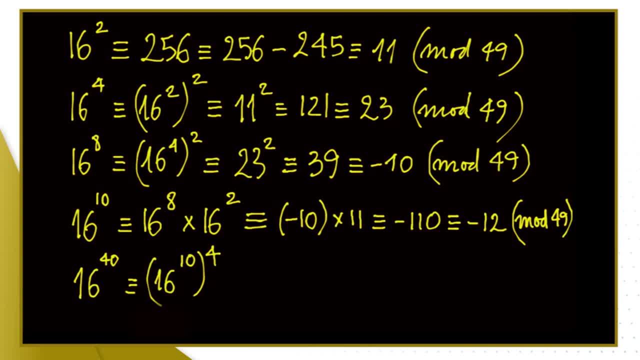 12 is quite small, so we're going to be able to handle this. so this is the same as doing minus 12 to the power of 4- don't forget the brackets- and that is the same as just doing minus 12 squared times minus 12 squared, and that boils. 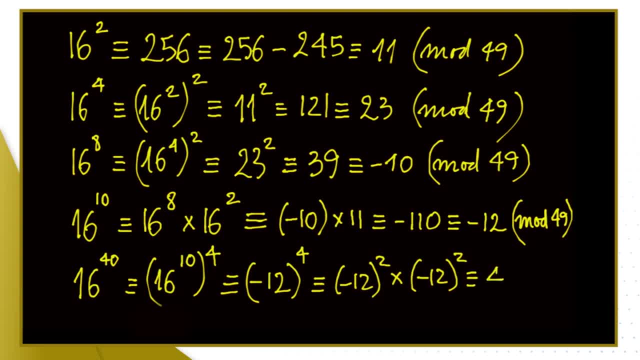 down to 46 on each side. so 46 squared, which is 46, is minus 3 mod 49. so that's going to be on the minus 3 squared, which is 9 mod 49. just recapping, we want to get 16 to the power of 42. we are on 16 to the power of. 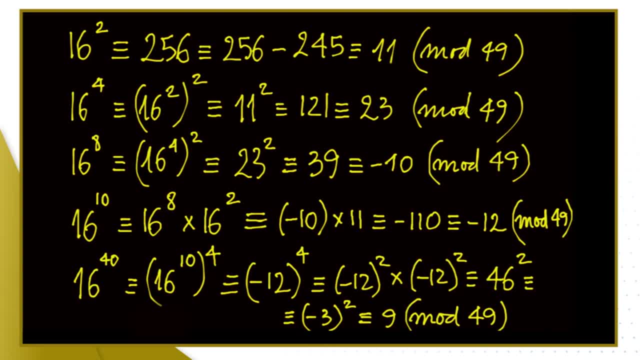 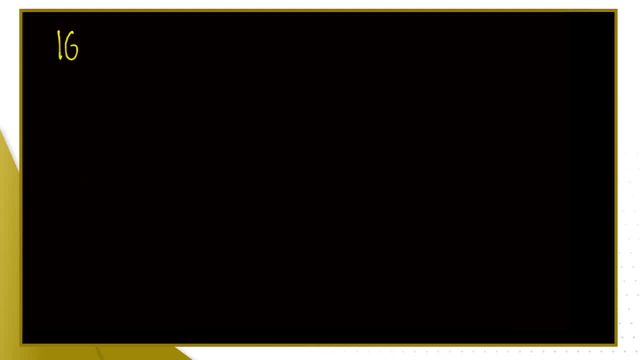 40. we just need to multiply this result 9 by 16 to the power of 2. let's do on the next page. so we've got 16 to the power of 40 is 9. we want to multiply by 16 squared. 16 to the 42 is 16 times 16 squared, which is the 9, and 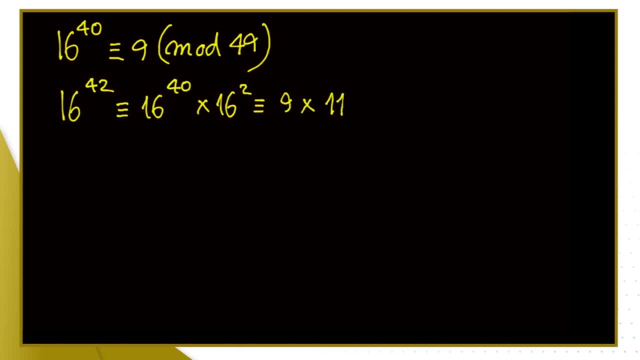 then 16 squared, we saw that it was 11 mod 49 and that gives us 99, which is just 1 more than twice 49. so it's remainder 1 mod 49. right back to the question we started with. 163 to the power. 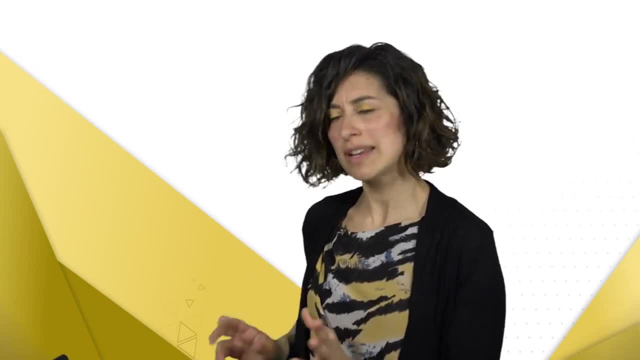 of 42 is 1 mod 49. I'm going to write this down. 163 to the power of 42 is 1 mod 49. 163 to the power of 42 is 1 mod 49. I'm going to write this down. 163 to the power of 42 is 1 mod 49. 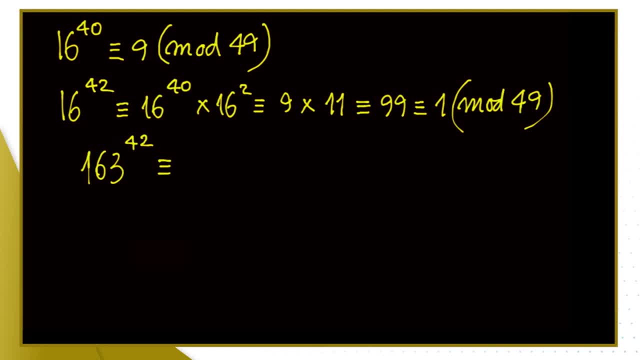 we said, because 63 is congruent with 16 mod 49. this is the same as 16 to the power of 42 mod 49 is what we said, and therefore this is all 1 in mod 49. the fact that this power is 1 means that we're very close to. 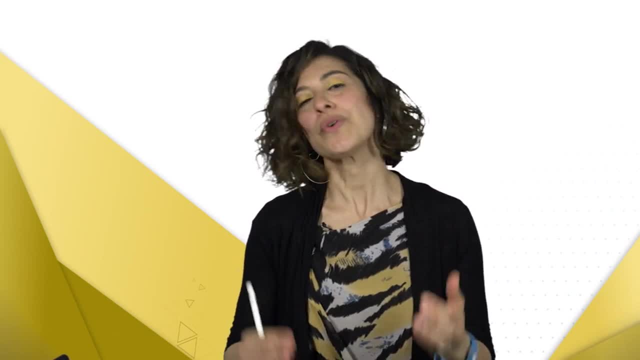 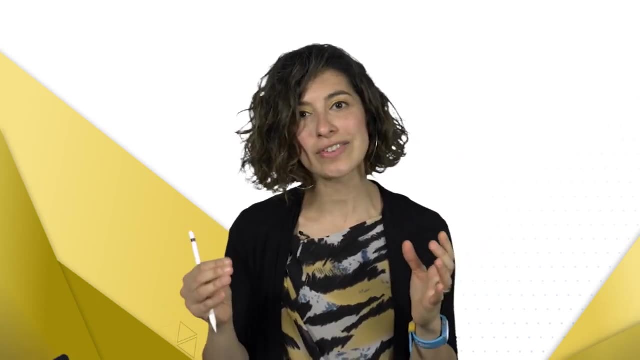 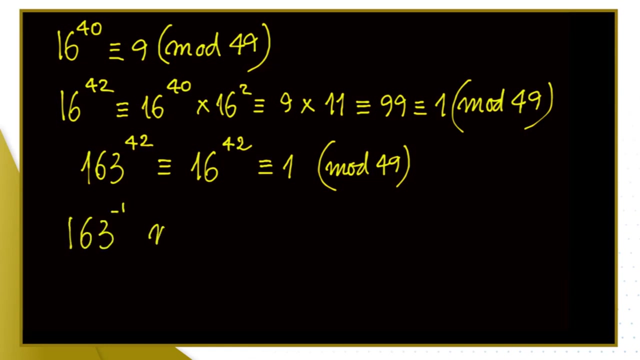 to knowing what the inverse of the number is. So a good follow-up question from here is asking: calculate the inverse of 163 mod 49.. So we are asked to calculate the inverse of 163 mod 49. That's a good follow-up question, and to do that we observe the following: 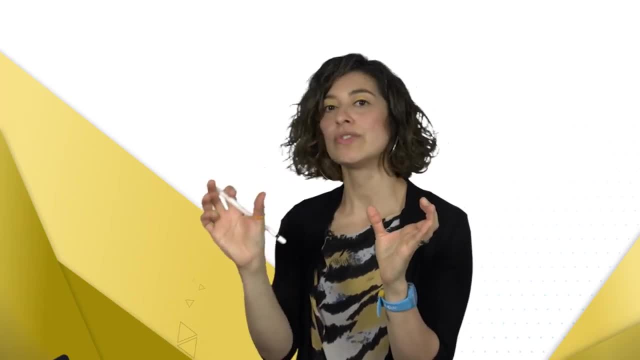 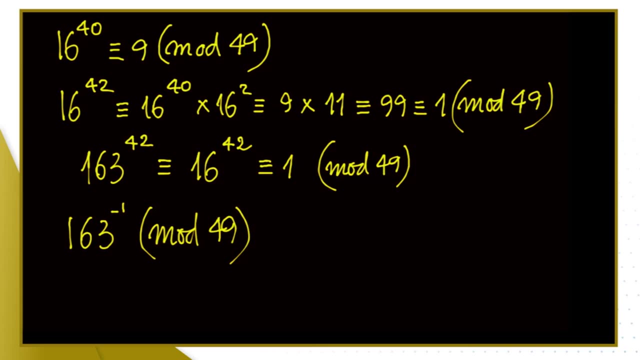 If you have a power that equals to 1,, the power before that is the inverse of the number. So 163 to the power 42 can be split as 163 to the power, 41 times 163.. If this product is 1,. 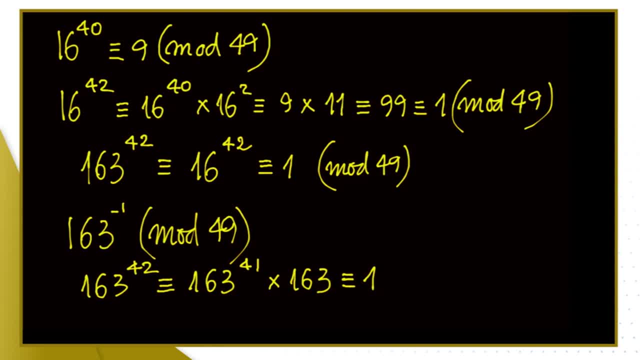 which we have calculated that it is. that means that is the definition of multiplicative inverse. It's a multiplicative inverse. What number times 163 gives 1?? Well, the number is this guy: It's 163 to the power of 41.. 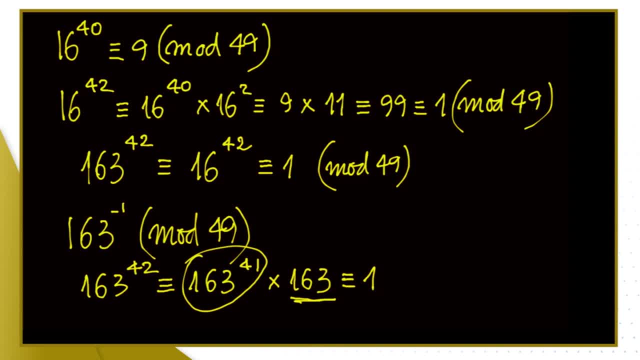 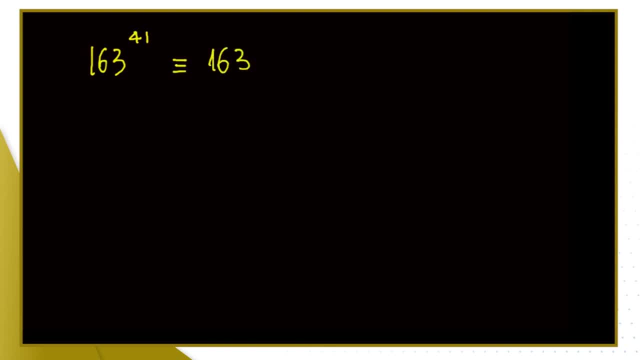 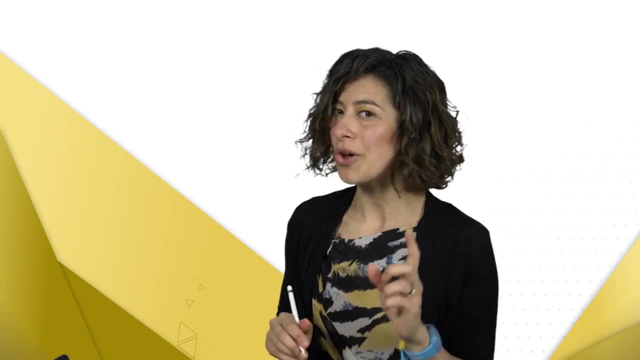 So that is the inverse. So 163 to the power of 41 is the inverse mod 49.. Do we have that number? Not yet, but we pretty much laid out all the foundations of the number. So we have that number Not yet, but we pretty much laid out all the. 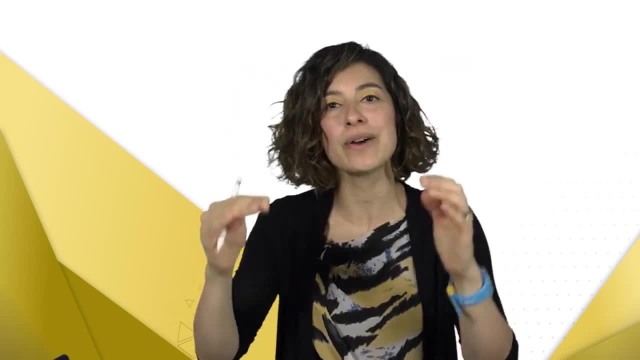 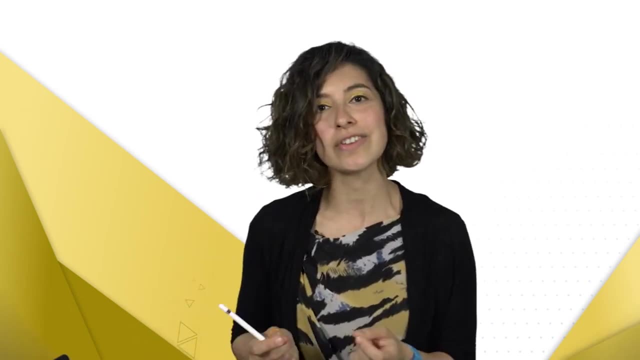 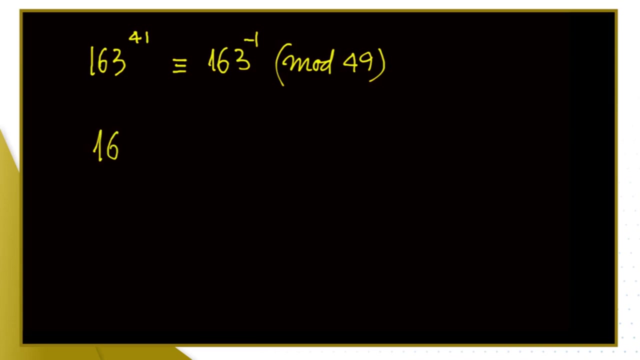 foundations to do this computation really quickly, because we've done a lot of powers of 16 to come to this one. And I'm still talking about powers of 16 because the inverse of 163 is going to be the same as the inverse of 16.. So to calculate the inverse we just go back to this. 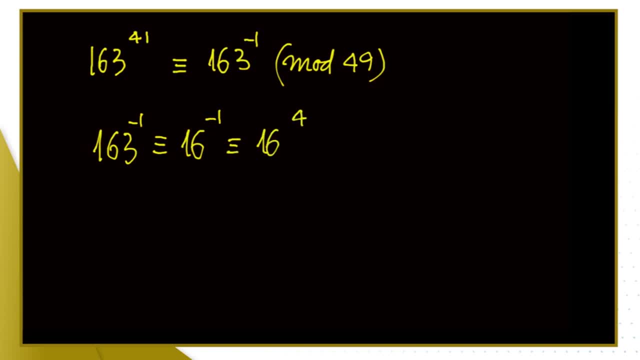 and this is also 16 to the power of 41, for the same reason that I explained above, And the power 41 is going to be made of 16 to the power of 41. So we're going to calculate the inverse of 16 to. 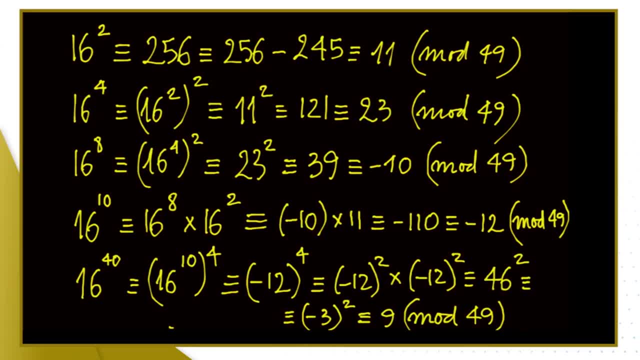 have lots of the other powers we calculated earlier. Let's have a look: The 41 I could make with the power of 40 and then just multiply by 16. The power of 40 was 9.. So 16 to the power of 40 was. 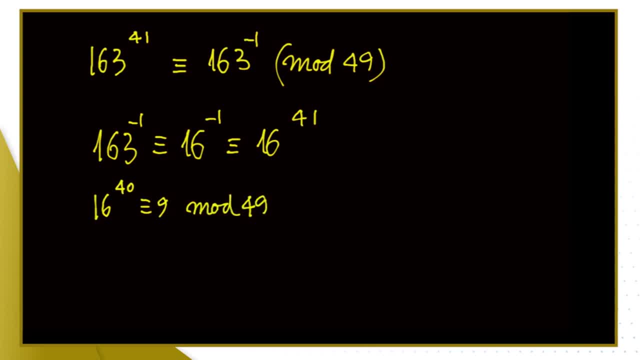 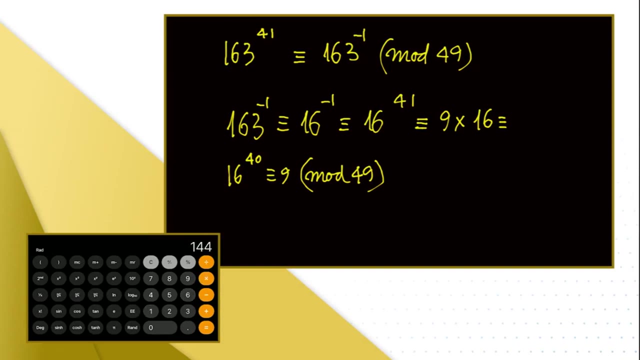 9.. And so all I have to do is do 16 to the power of 40 is 9 and then multiply by another 16.. Let's grab the calculator So that 9 times 16, we've got 144.. And that take away 98.. 98 is 2 times 49 minus 98.. That's our 46.. 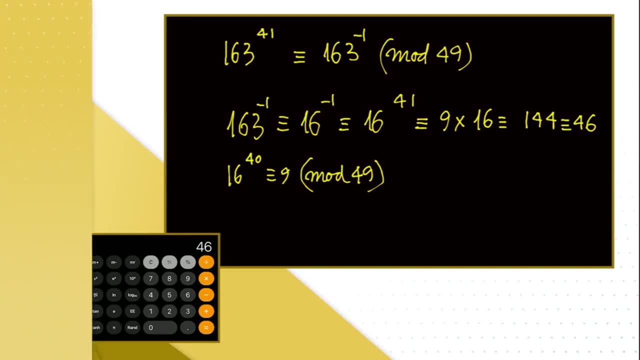 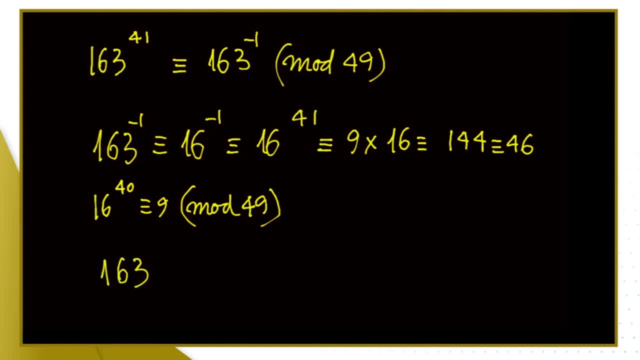 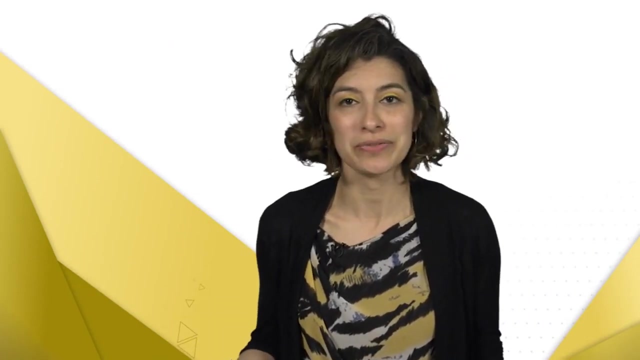 So that is 46 mod 49. That means that the inverse of 163 is 49. You could also say minus 3, because 46 plus 3 is 49.. We're going to look at exponentiation in modular arithmetic. That just means doing powers of numbers. 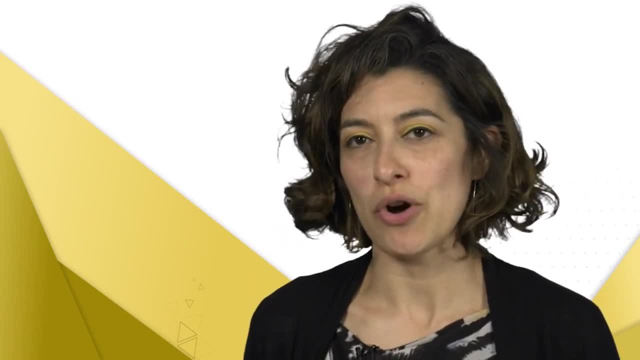 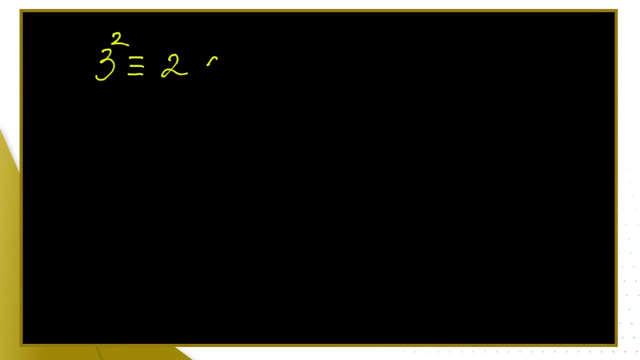 and taking the remainder, Let's look at powers of 3 in mod 7.. We're going to do: 3 squared, That's 9, which is 2 mod 7.. 3 cubed is 3 squared times 3- again, So 3 squared times 3.. And because 3 squared is 2 in mod 7,, 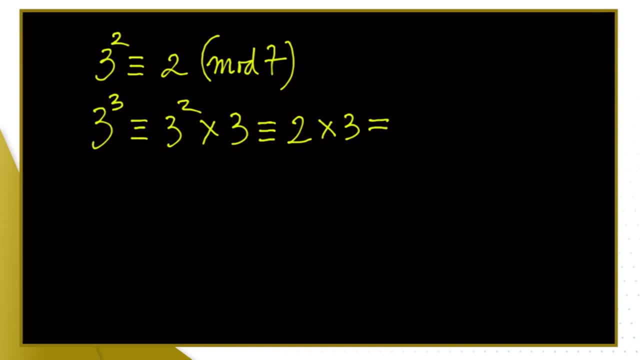 we just need to multiply this 2.. 2 with 3. And because 3 squared is 2,, we'll only need to multiply 2 by 3. And that gives 6 mod 7. square of the 3 squared. and that means we can square the 2, 2 squared, which is 4, and 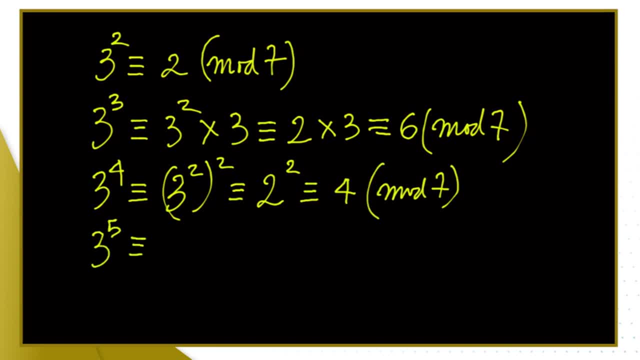 3 to the power of 5, we can do 3 to the 4 times 3, so that'll be 4 times 3, or we could do 3 cubed times 3 squared, for example, 3 cubed times 3 squared, because the power 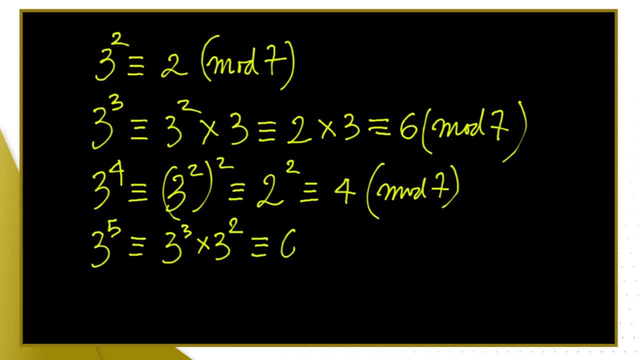 was add up to 5, and 3. cubed, we saw that it was 6, and 3 squared, we saw that it was 2, so that is 12,, which is 5 mod 7.. Whichever root you choose, you'll get the same number. 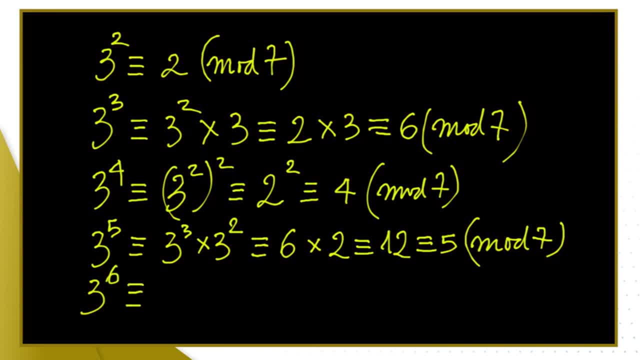 And one more 3 to the power of 6, it is, we can do 3 cubed squared or we could do 3 squared cubed. let's do that one: 3 squared cubed, 3 squared. we saw that it's 2, 2 cubed is 8, and 8 is 1 mod 7.. 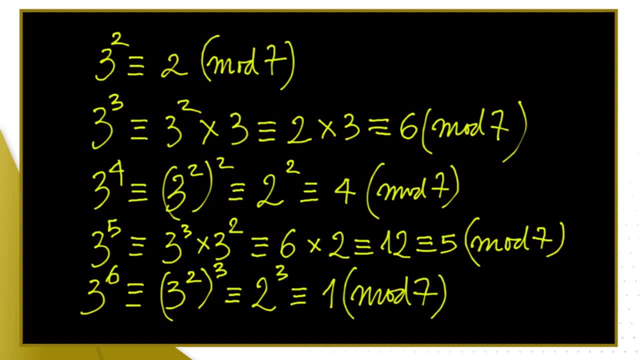 Now with that one. it's a good one because when you get 1 mod 7, you now can do powers and powers of powers of it and powers of 1 will always be 1 mod 7, so that means that. 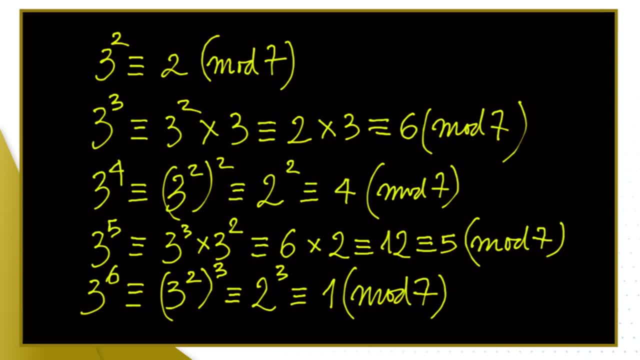 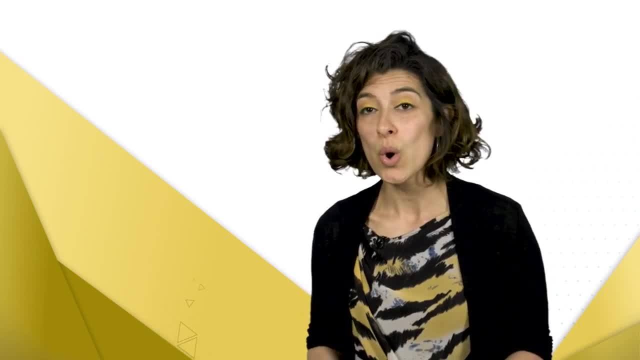 from here onwards, any power of 3 to the 6 is going to be 1 mod 7.. Why am I so excited about it? It's because we can do huge powers now with very little effort. I'll show you. 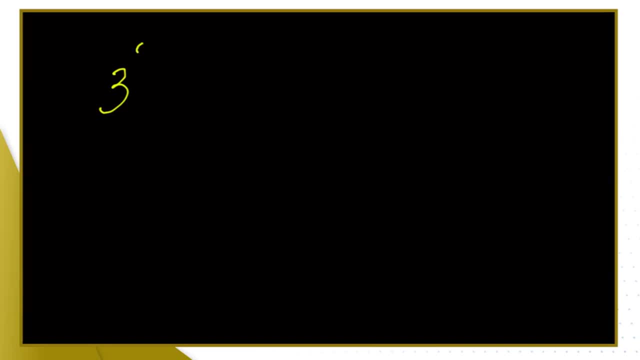 Say we want to do 3 to the power of 203 mod 7, pretty big and if you give it a go with the calculator, 3 to the power of 203 isn't going to fit in the screen, which means you. 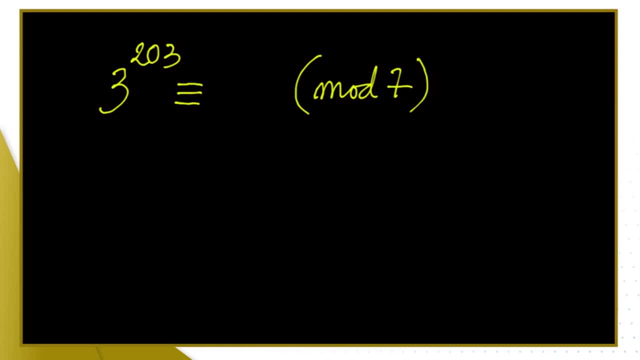 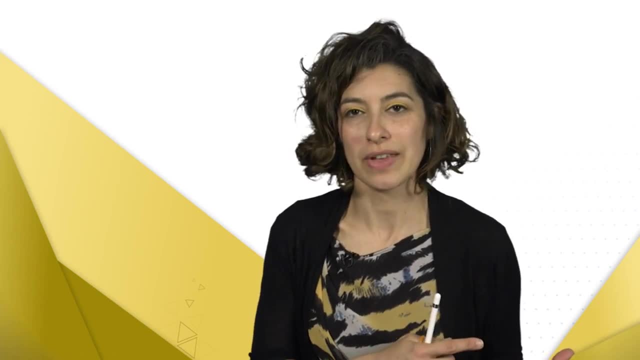 don't have a precise number, no point doing division by 7 and taking remainder, because it's not going to help. So instead we're going to take powers of 3, building from the previous results, and get as close as possible to 3, to the power of 203.. 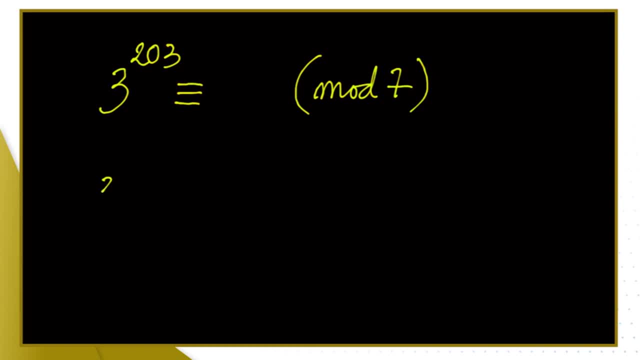 We've got 3 to the 6 is 1, so 3 to the 6 is 1, we're going to take powers of 3 to the 6 until we get very close to 3 to the 203, so let's do 3 to the 6 to the power of 33,. 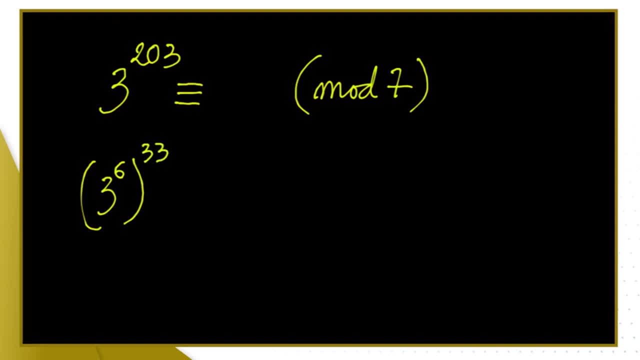 and you're wondering why 33?? Well, 3 to the 6 is 1.. Well, because 33 times 6 is 198, and that's the multiple of 6 closest to 203.. So that is 3 to the 6, we know it's 1, so now we do the power of 33,, which is still 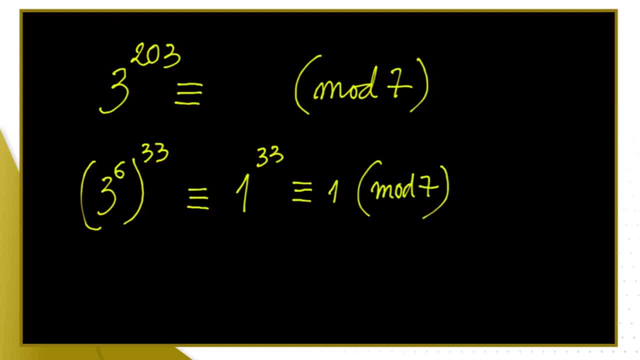 1. So 3 to the power of 203 is going to be 3 to the power of 198 times 3 to the power of 5.. And that 3 to the power of 198 comes from 3 to the power of 6 to the power of 33, because 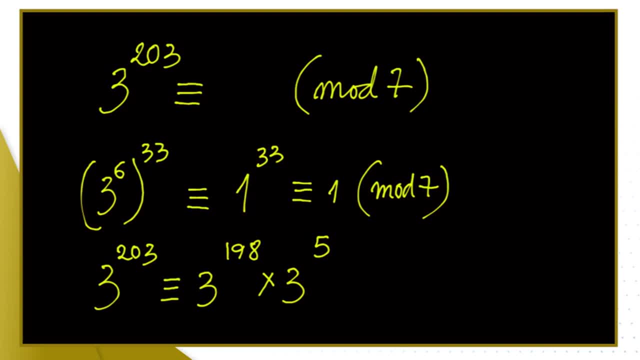 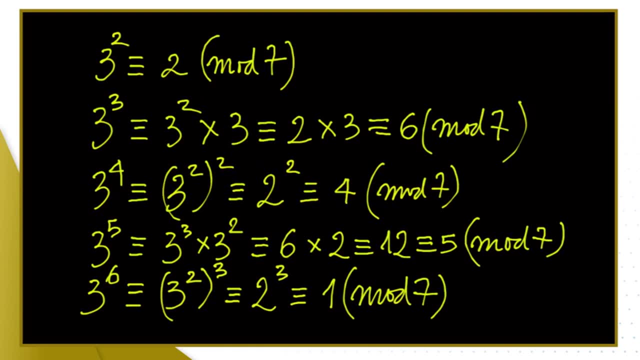 6 times 33 is 198. And so we've got 1 times 3 to the 5, and 3 to the 5 we worked out in the previous calculations, so it's 5.. So we've got 1 times 5, which is just 5 mod 7.. 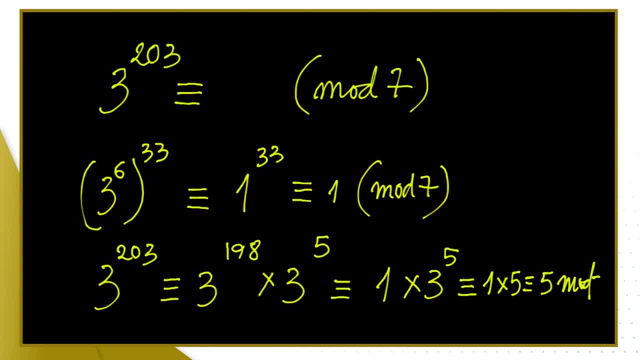 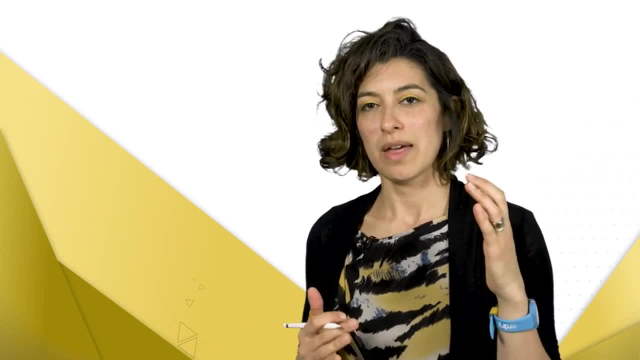 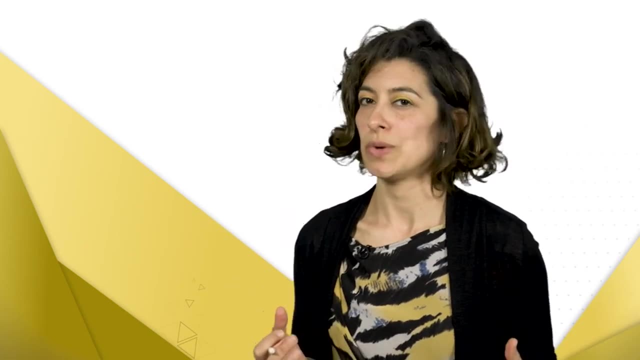 So we've got 1 times 5, which is just 5 mod 7.. OK, So this is an example of how we can use powers of a number in modular arithmetic to build up to a large power, but without having to work with very large numbers. 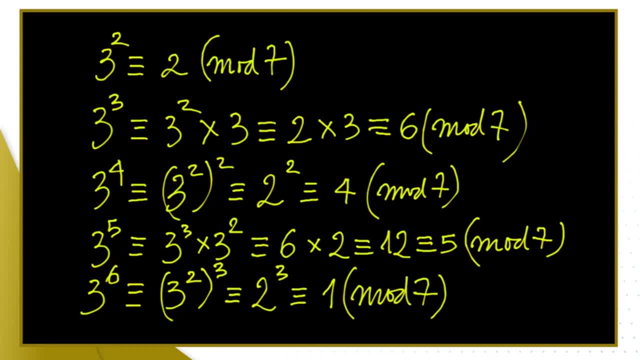 I thought it was interesting that in this initial calculation we work out all these powers of 3,, and 3 to the 6 is 1 mod 7.. Is that a coincidence, or does it always happen? Do we always get a power of number that is going to be 1?? 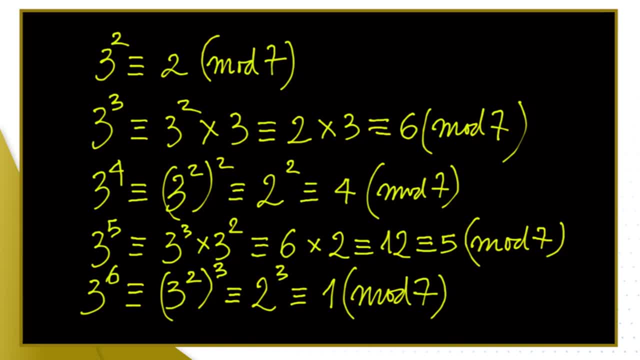 1 mod 7.. Does that always happen, And if so, can we work out that number? Is it always power 6?? Good question. The answer to that is summarised in what is called Fermat's Little Theorem, and it tells: 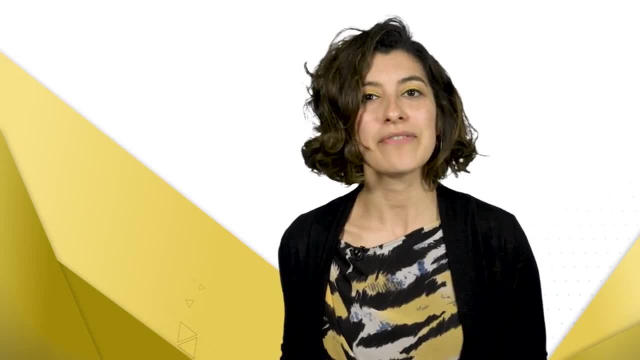 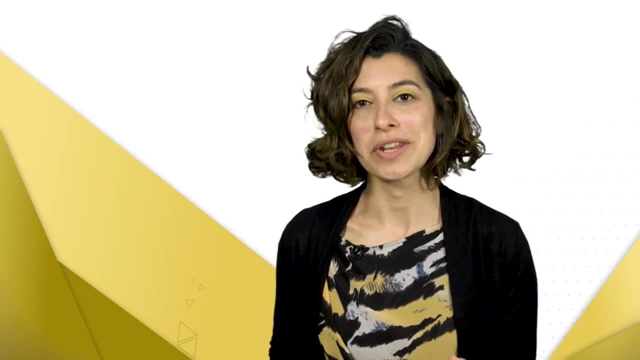 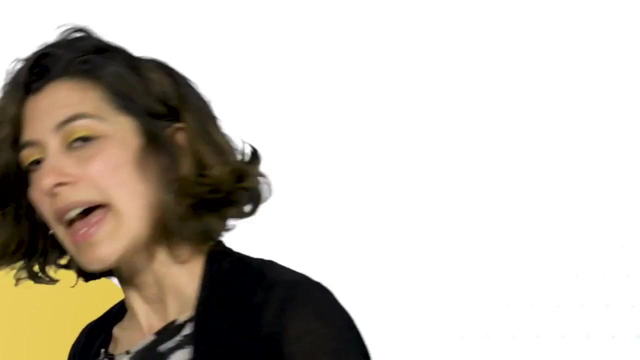 you how you get 1 mod a prime number. 7 is a prime number and in mod 7, power 6 is almost always going to give you 1. Fermat's Little Theorem. Fermat's Little Theorem says: let p be a prime number and let's work on mod p. 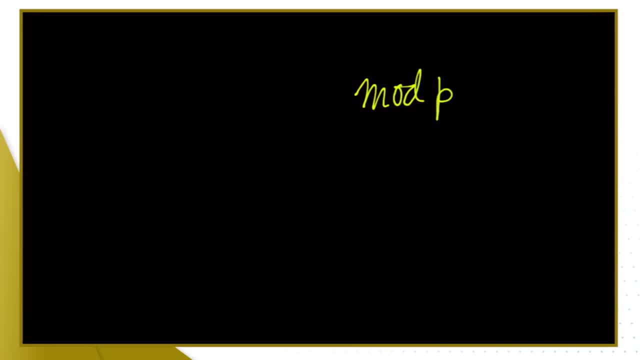 We're working on mod p, and on mod p the power p is very special, So any number to the power p is congruent with itself. mod p, provided p doesn't divide a. OK, So p does not divide a. 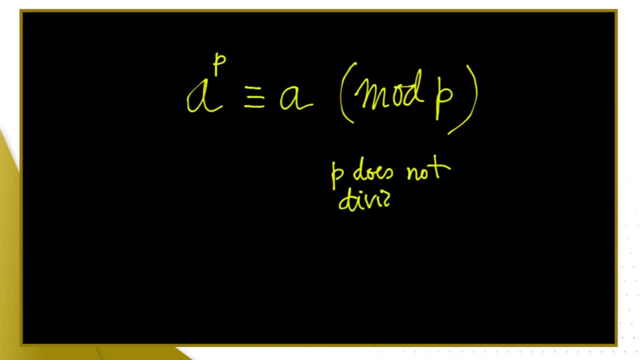 OK, So p does not divide a. Let's make sense of that. In our previous example we had powers of 3 mod 7. So our p is 7, and our a is 3.. Yes, 7 doesn't divide 3, so we're good to go. 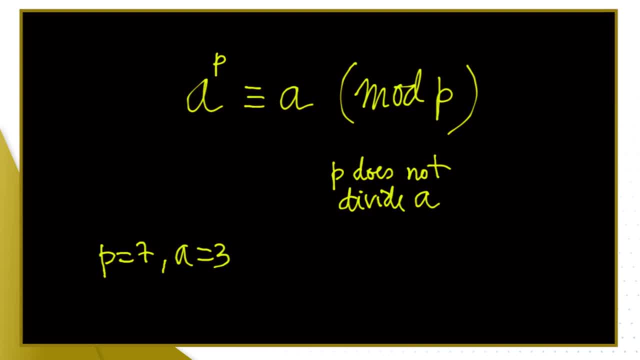 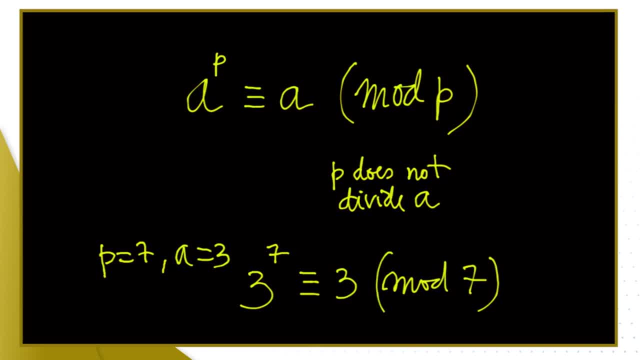 Now probably wondering. we don't have a 1 there, and I was promising that there is a power that gives result 1.. There is Just. let's look at this one again. It's 3 to the power of 7, it's 3 again. 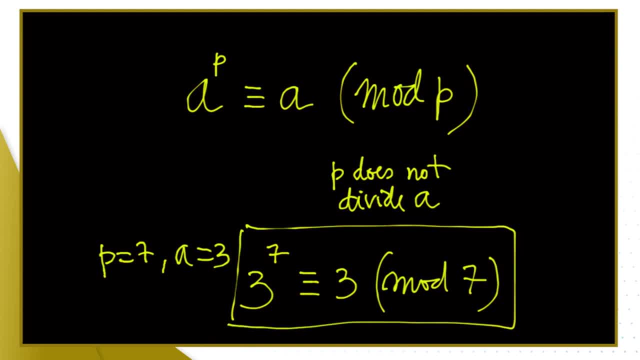 That means that the previous power- 3 to the power of 6, has to be 1.. I'll show you why. So 3 to the power of 7 is congruent with 3 mod 7.. So 3 to the power of 7 is congruent with 3 mod 7.. 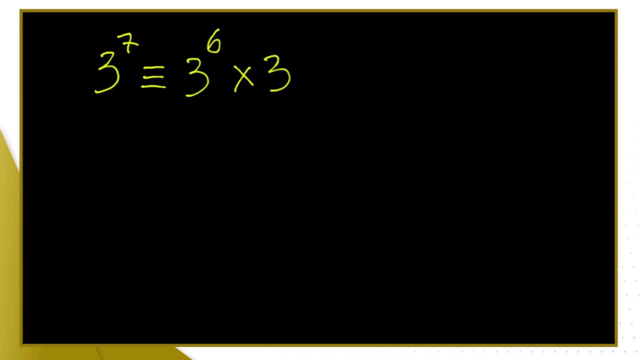 The previous sector has 3 to the 6 times 3.. And if this is 3 itself, then 3 to the 6 needs to be congruent with 1 mod 7.. So we can update Fermat's Leonor theorem to say not only that the power 7 returns the 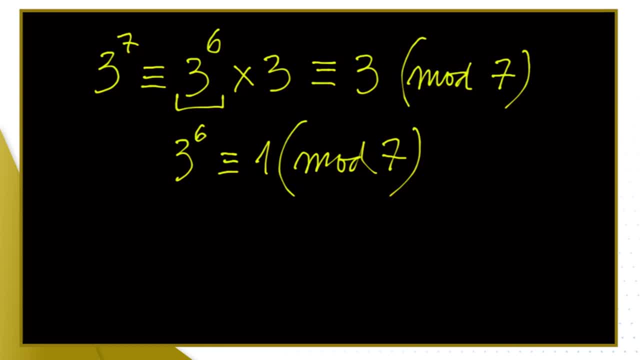 initial number, but that the power 6 is the identity 1.. So it says so. So we are going now with the final hypothesis. So a to the p minus 1 is the identity 1 mod p, provided p does not divide a. 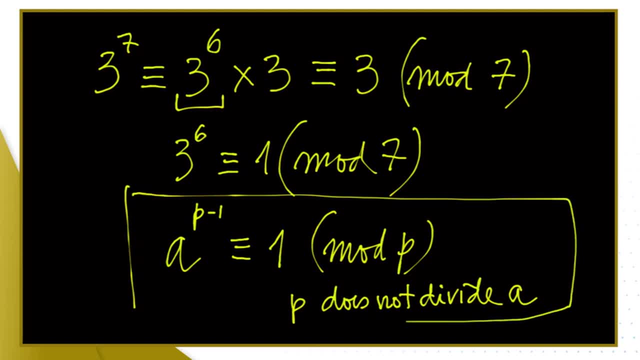 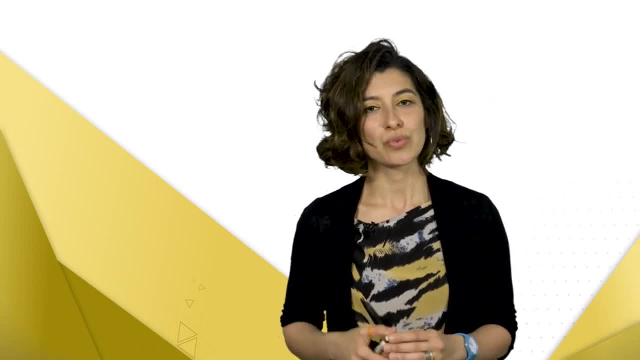 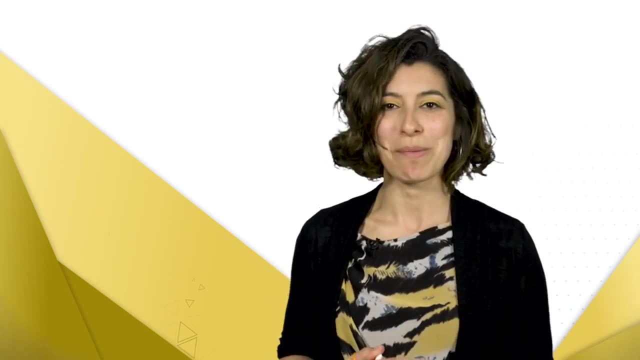 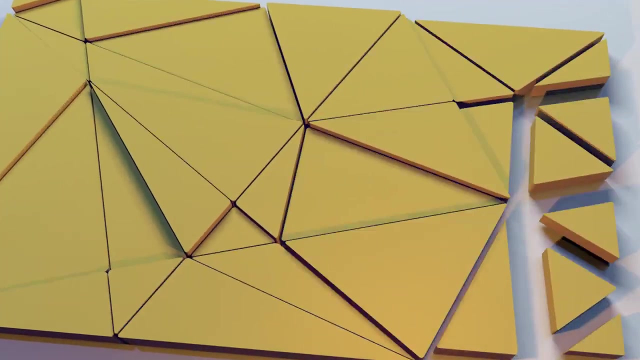 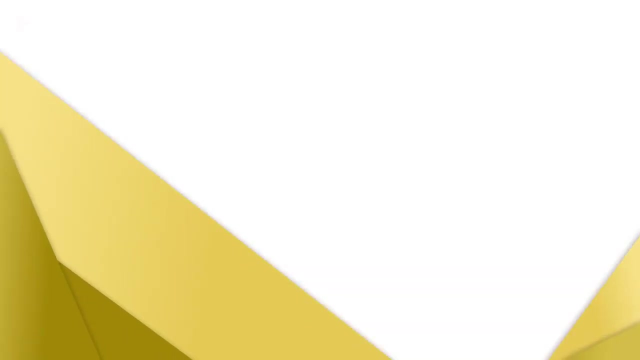 Okay, And that makes working in modular arithmetic with prime numbers a delight, And we will see later on an example of real-life application of prime numbers and modular arithmetic where we're going to capitalize on prime numbers. Earlier on in the course you wrote algorithms to convert a decimal number to binary. 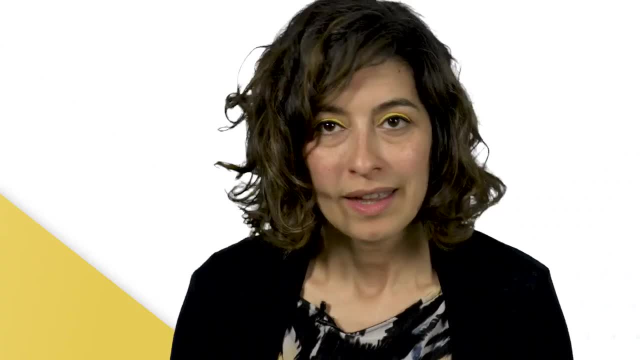 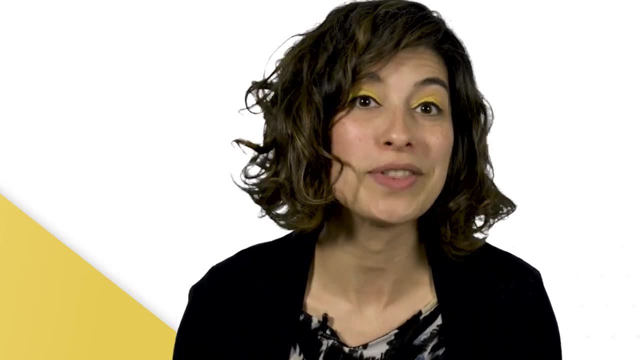 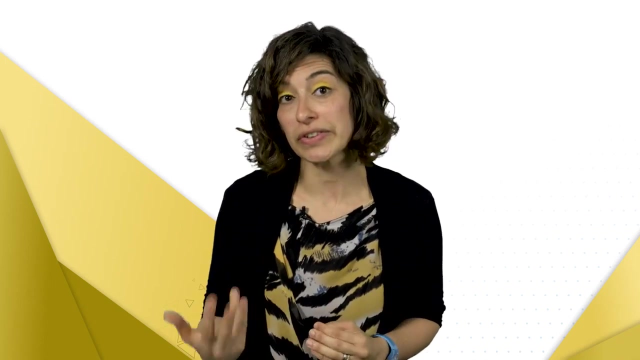 And you thought of the algorithms. In a programming language, you can use shortcuts to finding the remainders of integer division. Look out for the mod operator coming from modulus as we use it in modular arithmetic. For example, 56 mod 16 gives you the remainder of the integer division, which is 8.. 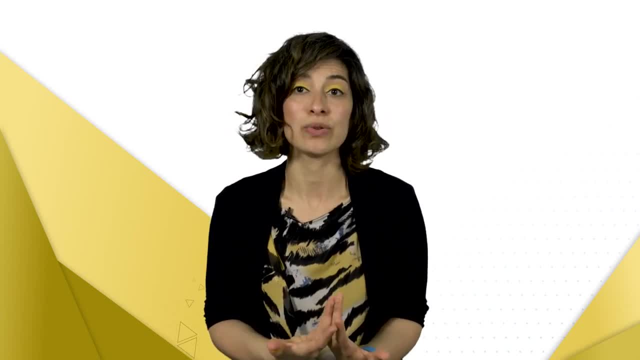 So you can implement modular arithmetic in a programming language using this operator: 56 mod 16 will return 8, giving you that 56 mod 16 will return 8.. 56 mod 16 will return 8, giving you that 56 mod 16 will return 8.. 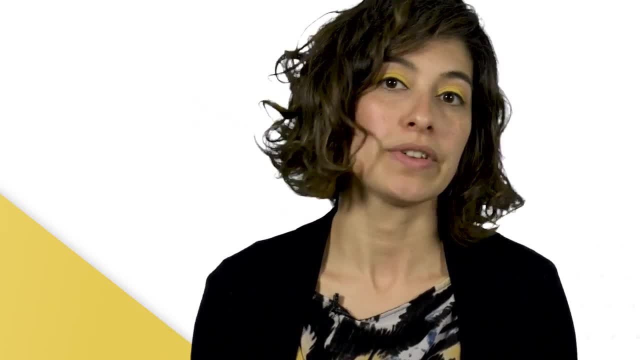 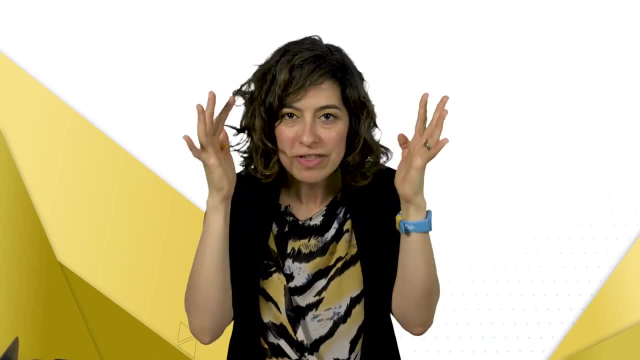 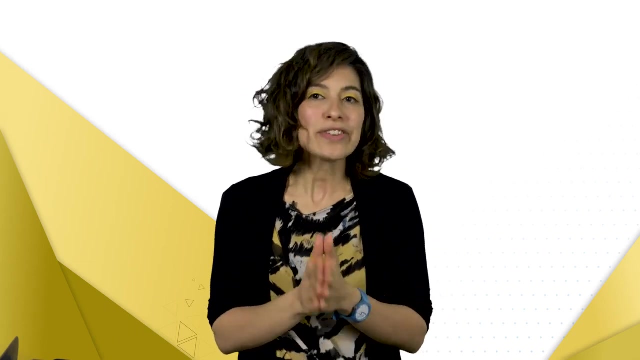 So 56 is congruent with 8 mod 16.. I've mentioned in earlier videos that we can use modular arithmetic to create mental arithmetic strategies to test for divisibility. And here's how we do it for casting off 9s: 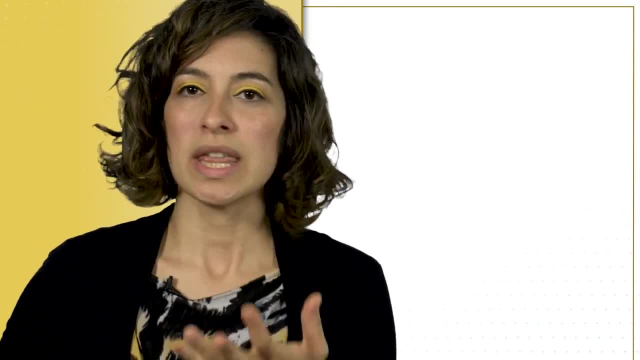 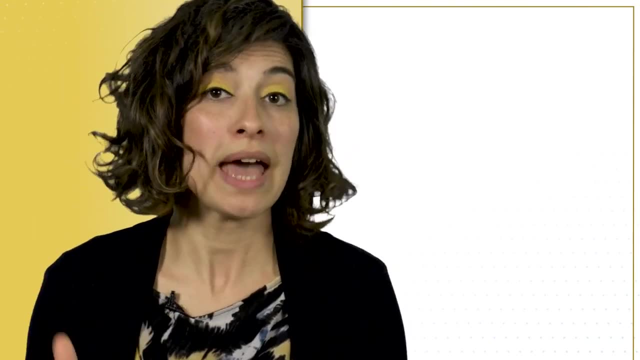 I'm going to write a generic number with digits from a n all the way to a 0. And I'm going to write this number in the expression- This is a spandered form using powers of 10.. And I want to check. 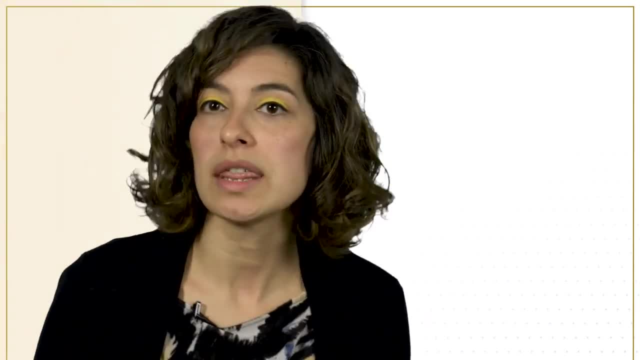 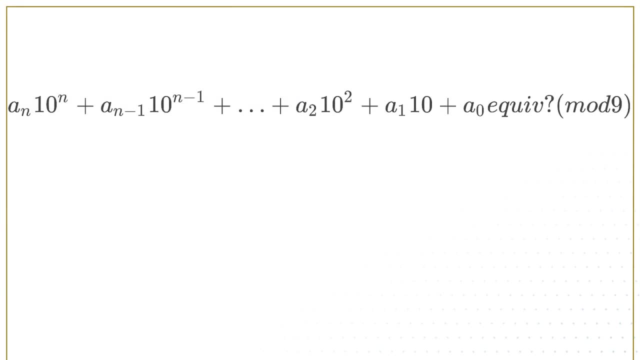 what is this number? congruent with mod 9.. So I'll write a n x 10 to the power of n plus a n minus 1 times 10 to the power of n minus 1, plus all these other terms, all the way to. 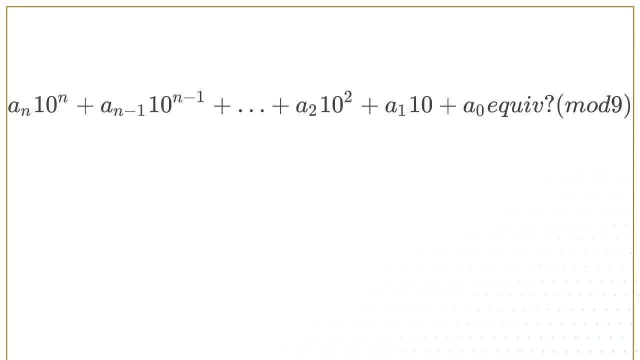 a 2 x 10 squared, plus a 1 times 10 plus a 0.. We want to check is congruent with mod 9.. Now this is what we do for divisibility by 9, because if the remainder is 0, the number is divisible by 9.. If the remainder is anything else, then 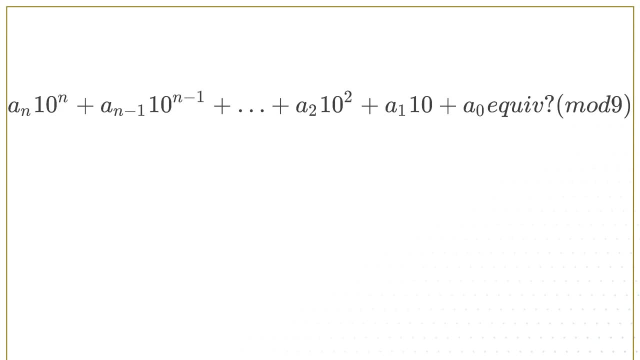 it is not. Let's break this down into each power of 10.. So 10 is congruent with 1 mod 9.. 10 squared is congruent with 1 squared, which is congruent with 1 mod 9.. And any power? 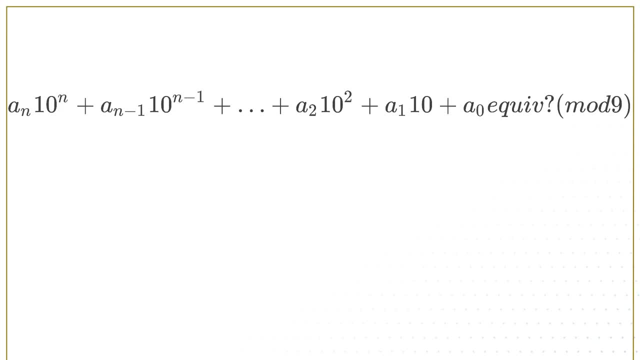 of 10 is congruent with 1 mod 9.. That means that this initial expression is congruent with a n times 1 plus a n minus 1 times 1, and all of them in the same fashion and so congruent. 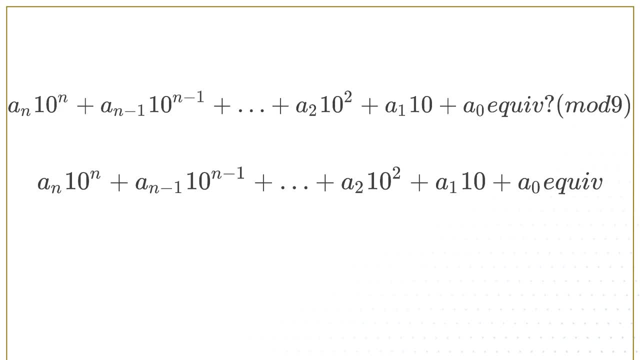 Adding a 2 times 1 and adding a 1 times 1 and a 0.. Now this is congruent. We're just eliminating all these 1s, because multiplying by 1 does nothing. a n plus a n minus 1 plus. 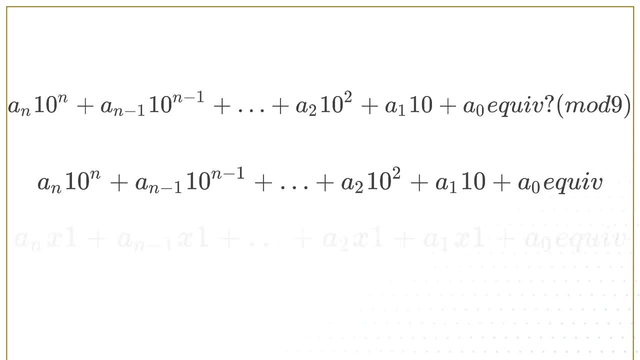 all the digits plus a 2, plus a 1, plus a 0 mod 9.. Now, let's just think about that. That means that the remainder of division by 9 only depends on the remainder of division by 9 of the sum of the digits. That's what. 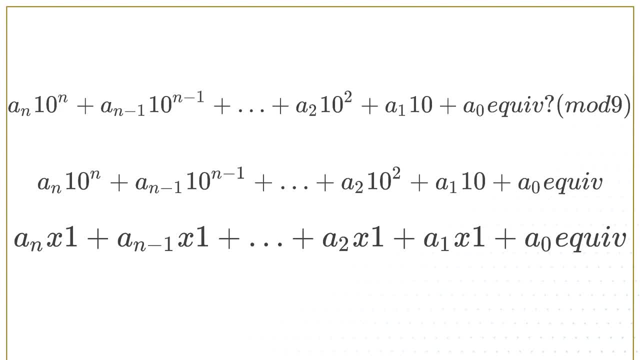 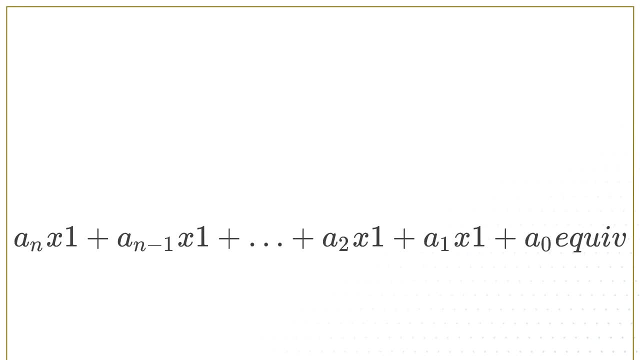 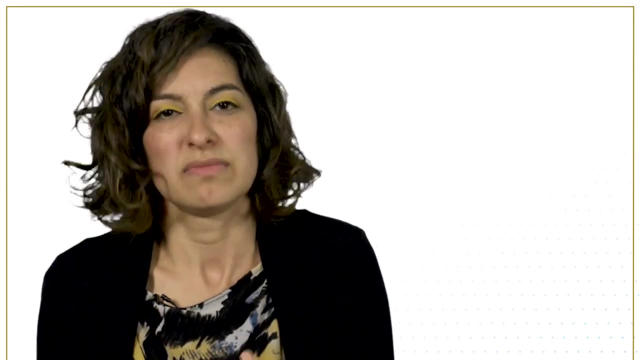 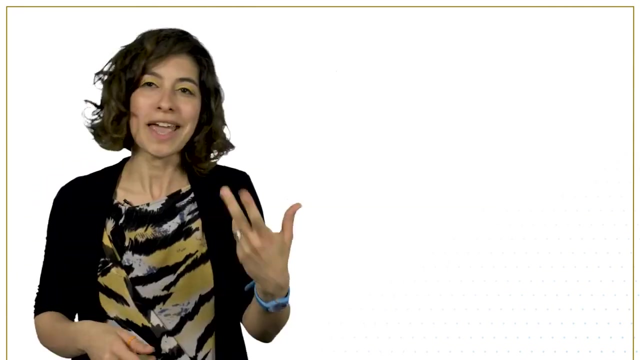 If mod 5,, what you get is that the remainder only depends on the units digit. If it's 0 or 5, then it is divisible by 5.. For divisibility by 4, mod 4, you get that the remainder only depends on the 1s and the units of the number a 1. 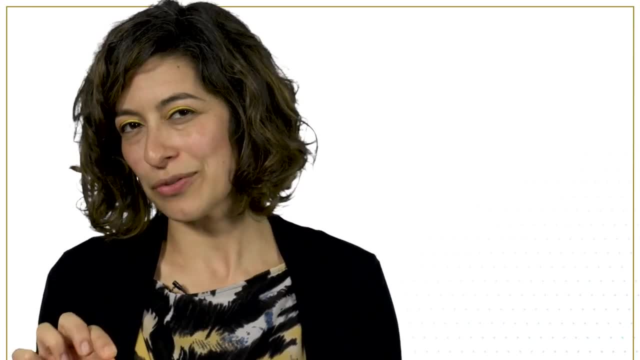 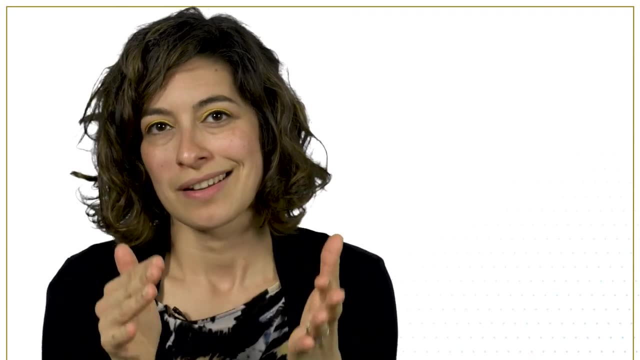 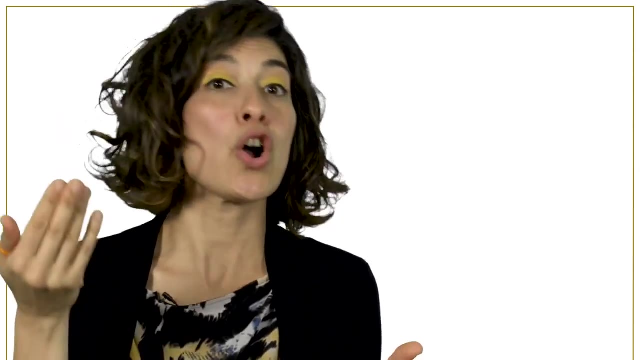 and a 0. For mod 11, this is a nice one, The one I mentioned in another video, Divisibility by 11, let's check each monster, The power of 10.. So 1 is congruent with 1 mod 11.. 10 is congruent with negative 1 mod 11.. 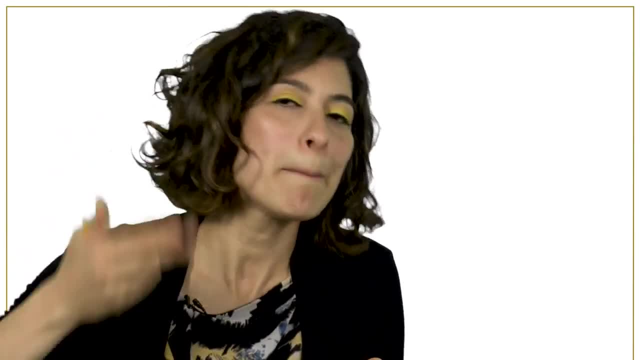 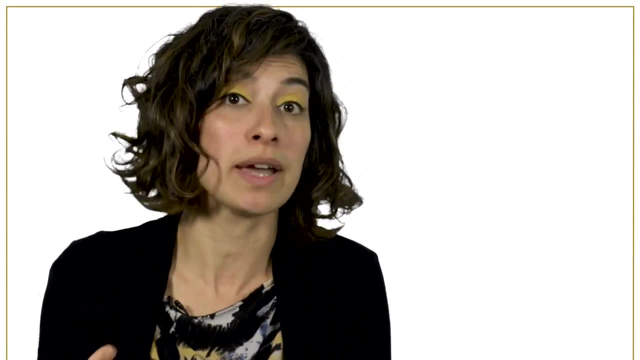 You would say: 10 is congruent with 10 mod 11, but it is also negative 1.. Now, 10 squared, let's use the minus 1, 10 squared is congruent with minus 1 squared, which is congruent with 1 mod 11.. 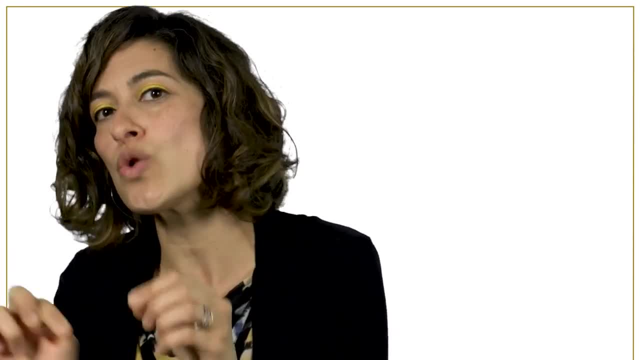 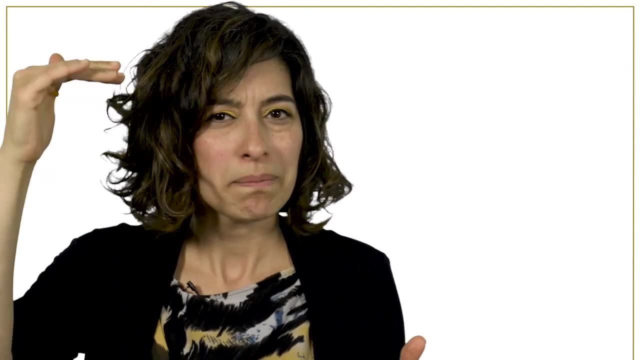 And 10 cubed is congruent with minus 1 cubed, which is congruent with negative 1 mod 11.. See the pattern. If the power is an odd power of 10,, we have congruence with minus 1.. 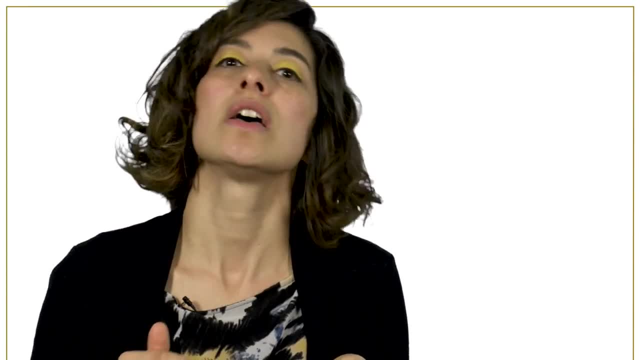 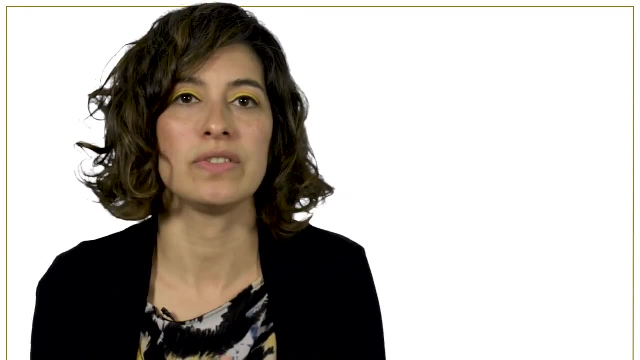 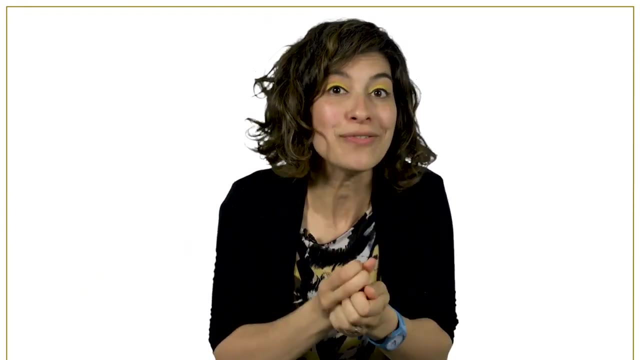 And if it's an even power of 10, we have congruence with 1 mod 11.. That means you can pair up the odd positions and the even positions, And so the sum of the odd positions, The sum of the odd position digits minus the sum of the even position digits, is congruent with the initial number mod 11.. 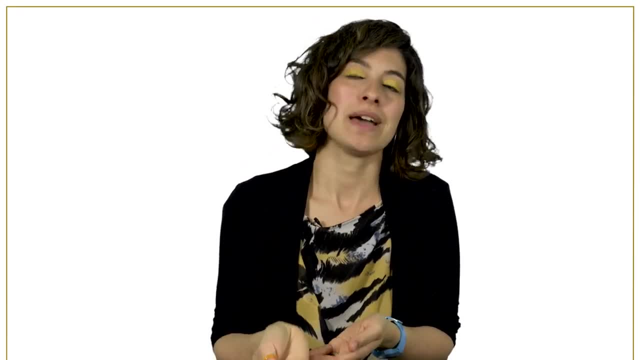 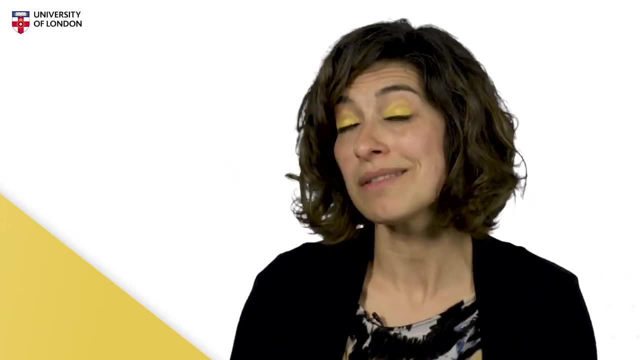 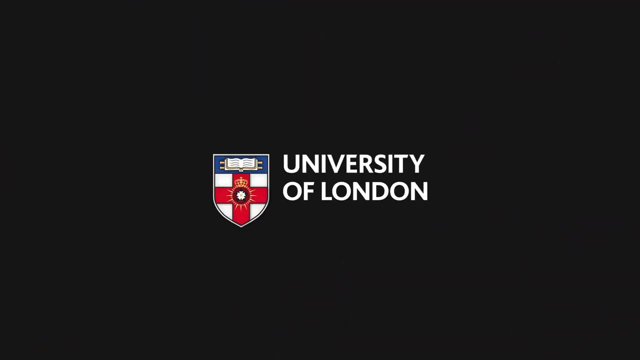 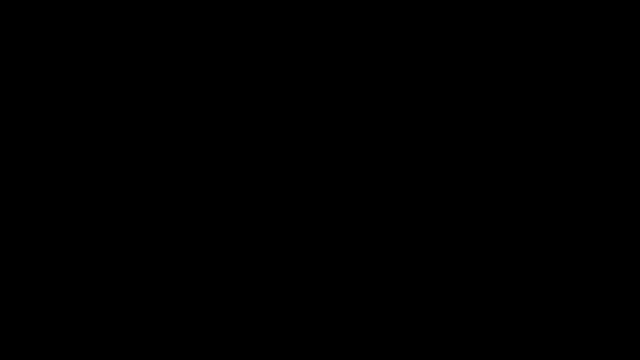 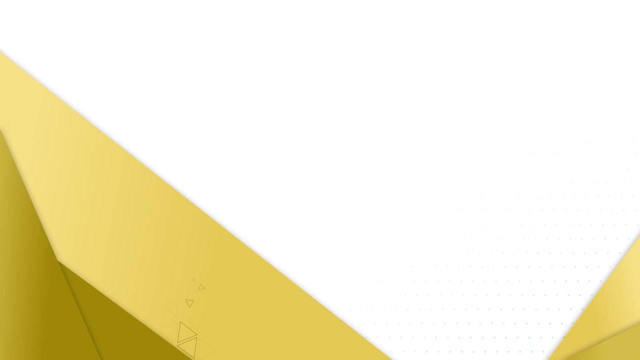 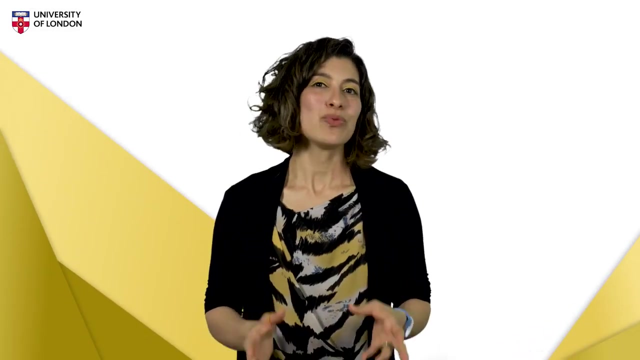 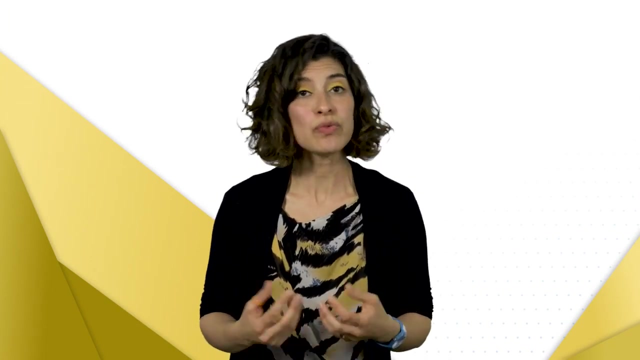 That means that is the key to divisibility by 11. You can have the reassurance that your mental arithmetic shortcuts always work, because you can prove them with modular arithmetic. Thank you. Let's recap what we've done so far. One aspect that came up over and over again in number systems was working with remainders. 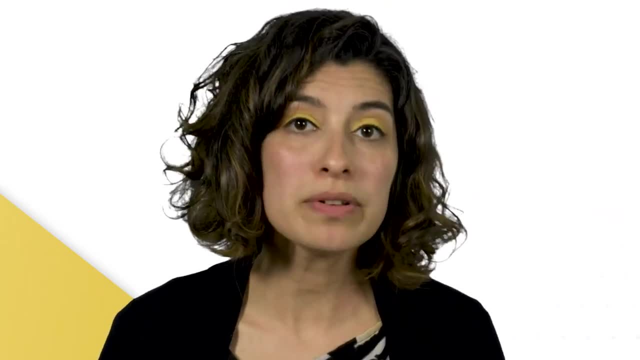 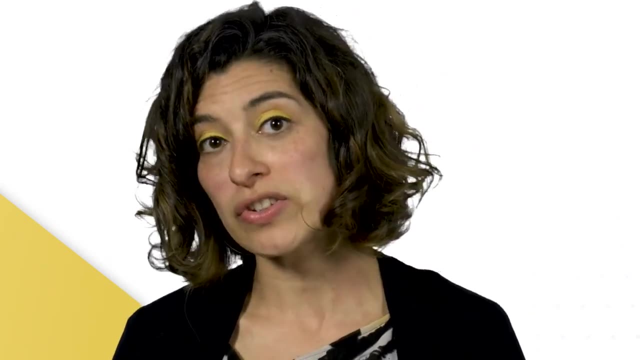 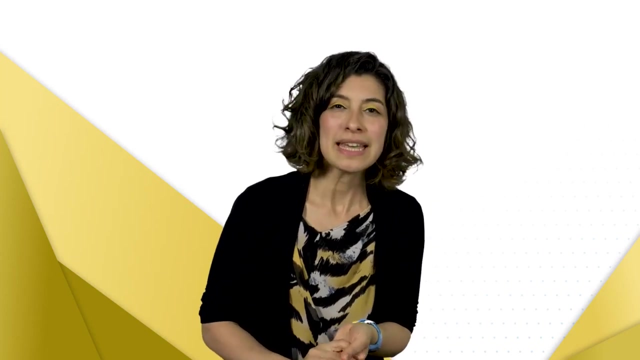 of division In modular arithmetic. we looked at the powerful mathematics that can be done with such remainders to create an environment with arithmetic operations similar to day-to-day numbers. When iterated over and over again, multiplications in modular arithmetic seem to have a random 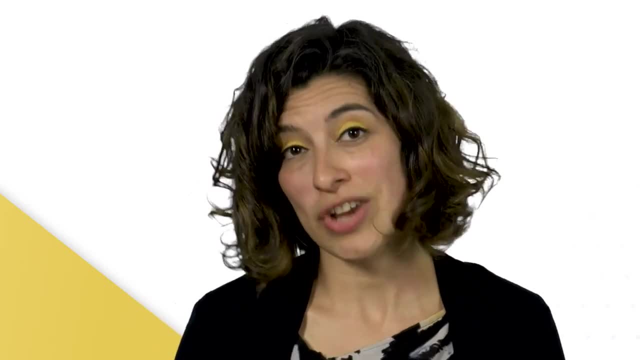 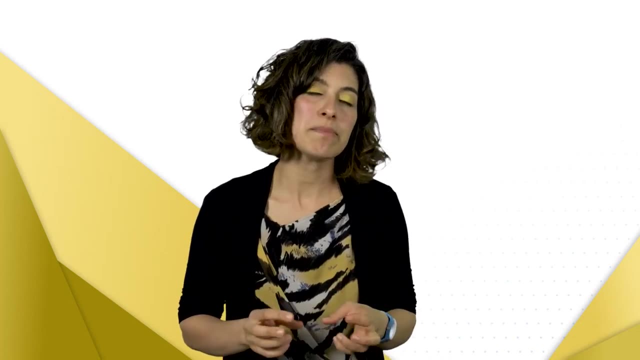 pattern That is tapped into in computing to generate pseudo-random numbers. The unpredictability also contributes to an encryption method, up to today the most powerful in classical computing. This method, RSA, taps into the fact that the arithmetic method is the most powerful. 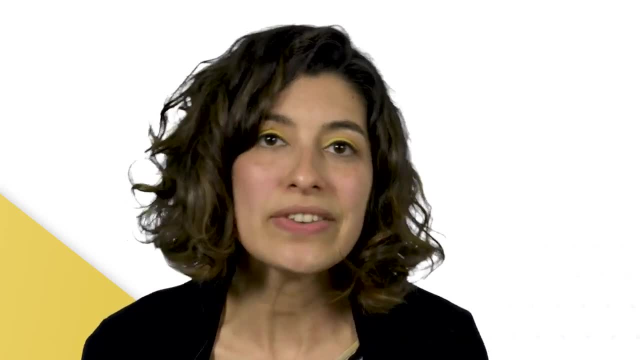 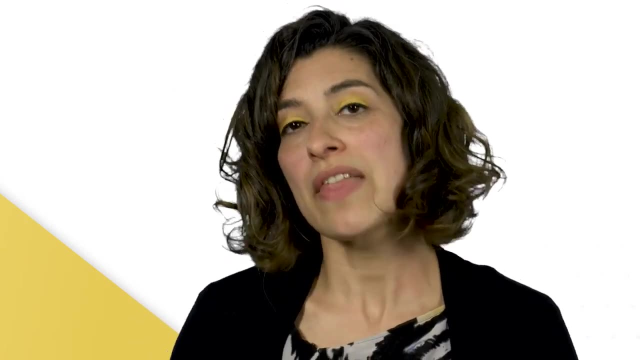 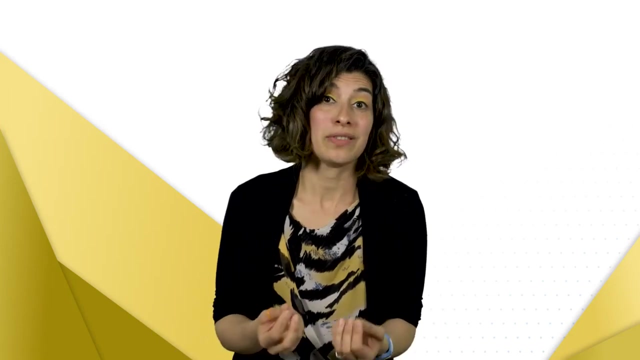 in classical computing. The RSA is the most powerful in classical computing. In fact. it is computationally hard to factorize numbers into primes and so exploits large prime numbers and their product to create a public key encryption method. You can share that huge, large number that is a product of two large primes and anybody 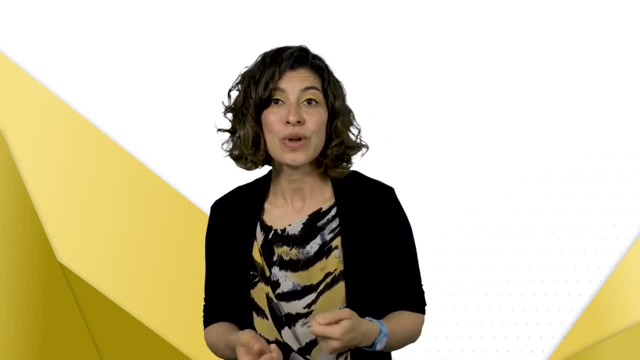 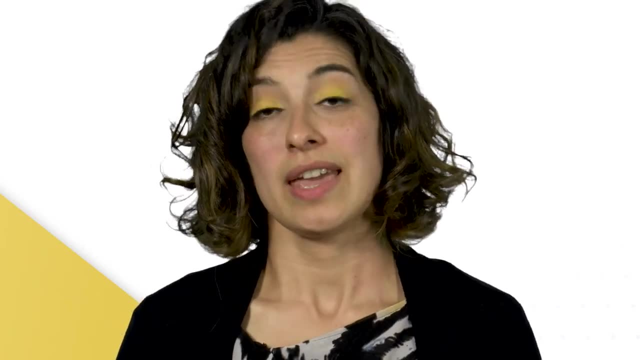 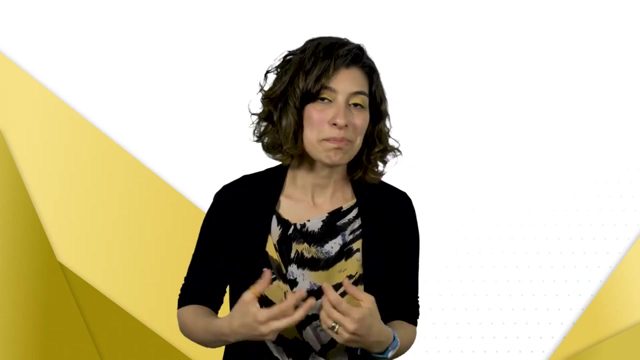 can send you secure messages with that key that only you can decrypt and redistribute. The tool we've learned to implement RSA encryption was SQL. The tool we've learned to implement RSA encryption was calculating multiplicative inverses in modular arithmetic. We calculated powers in modular arithmetic and we used a shortcut called Fermat's Last. 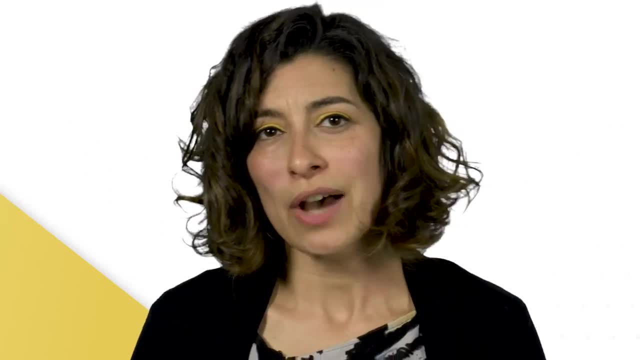 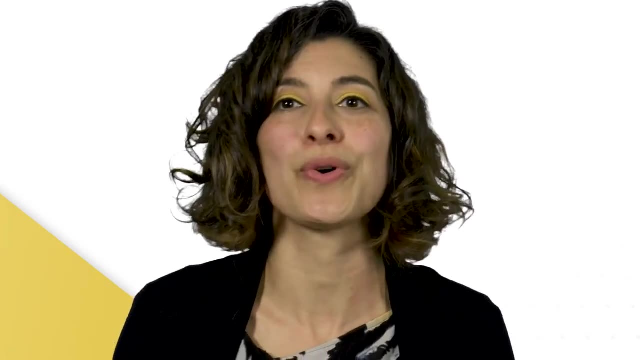 Theorem when the modulus was prime. You can go ahead and program your mini-implementation of RSA if you wish. you know it's outside the scope of the course and you can go and read about digital signatures and other tools we can use to communicate. 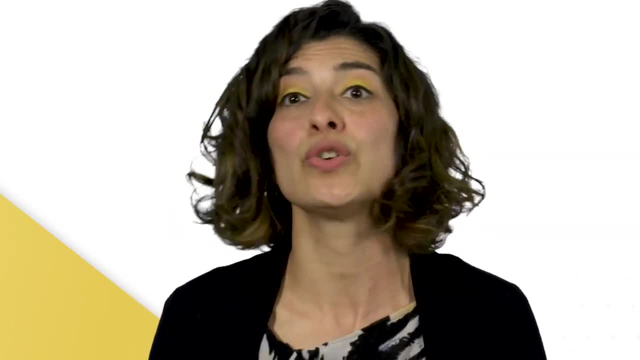 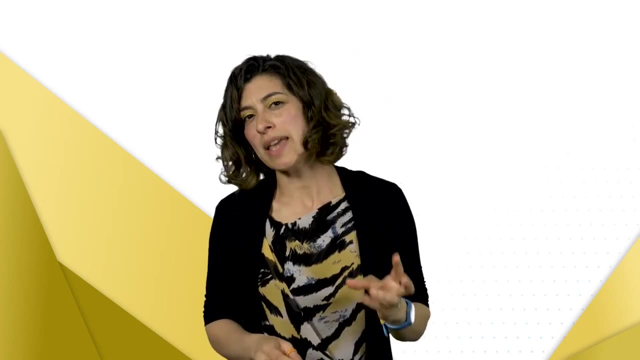 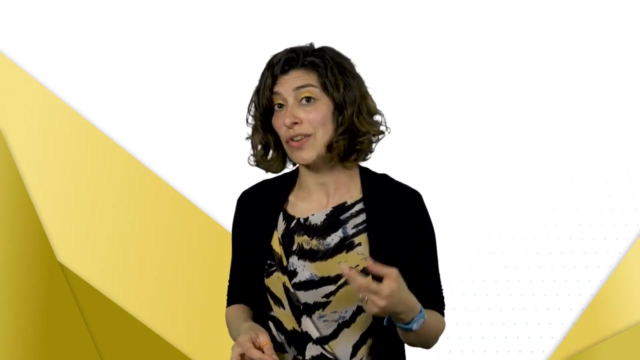 Thank you, And even exercise democracy in a secure way digitally. Next we will get started with sequences and series. To get ready, start paying attention to streams of numbers around you and see which ones. you can come up with a generating rule and make predictions on the behavior of those numbers. 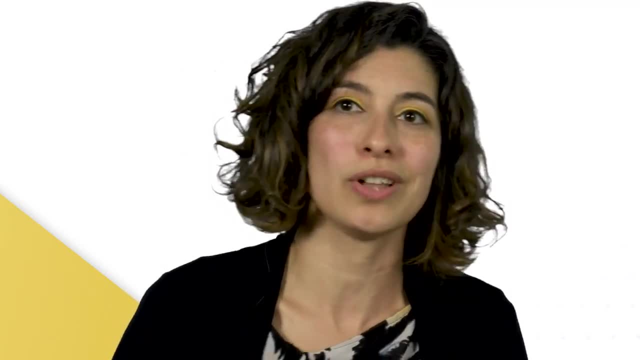 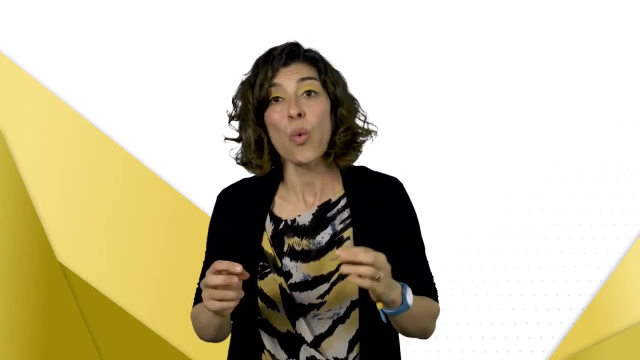 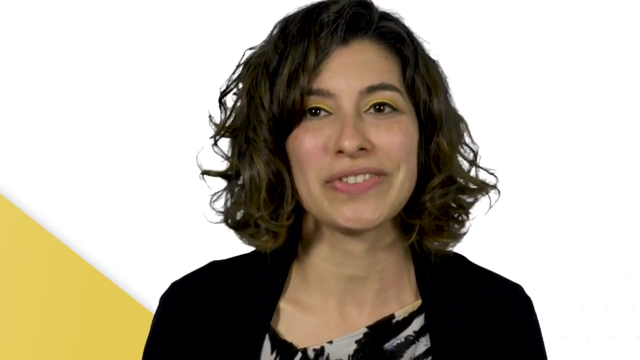 Mind you, we won't be cracking the secret rule behind stock market or the lottery- there's no such thing. but we will open the door to what tools are out there to understand what can be understood from streams of numbers. As always, we want to see it from the point of view of a computer scientist, so get your. 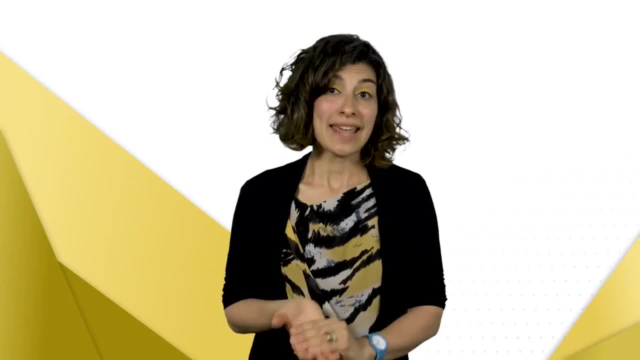 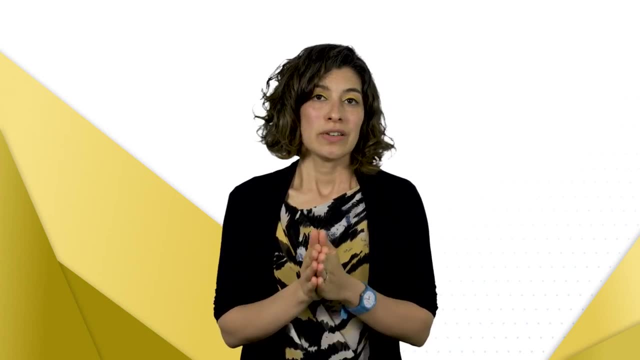 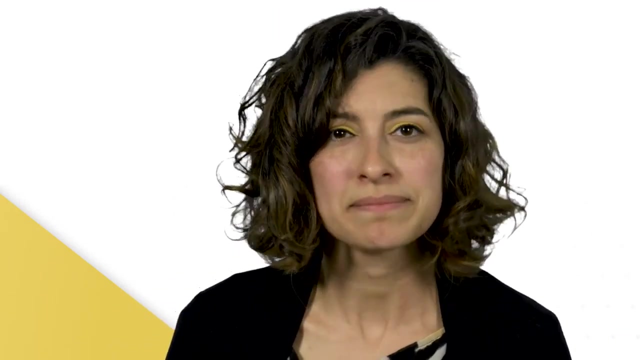 focus on that. I will leave you a puzzle. It dates back to the first century before Christ and it can be found in the literature. so, as true as books can be, Josephus was a commander in Galilee as the Roman army was invading. he had 40 soldiers. 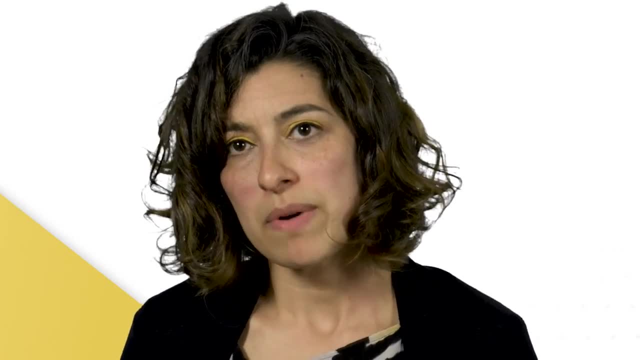 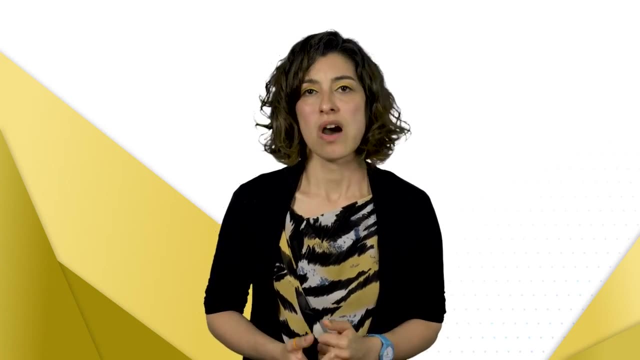 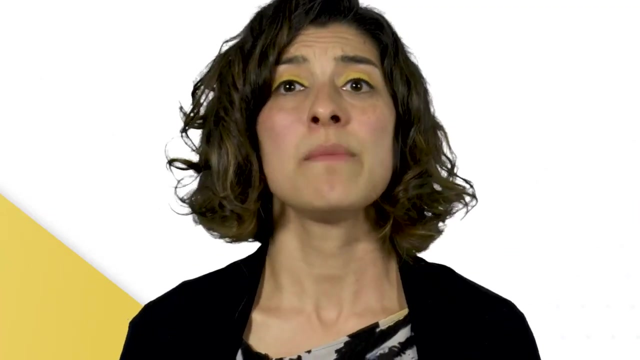 under his watch. He decided that, as their number was minute, they would not stand a chance against the Romans, So he looked for a randomized way of taking their lives that did not go against their moral and religious beliefs. Josephus and his army stood in a circle. 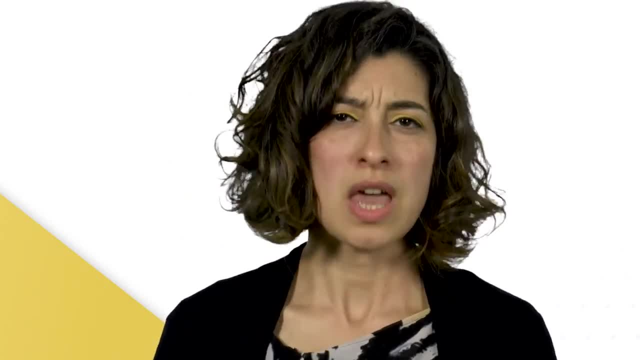 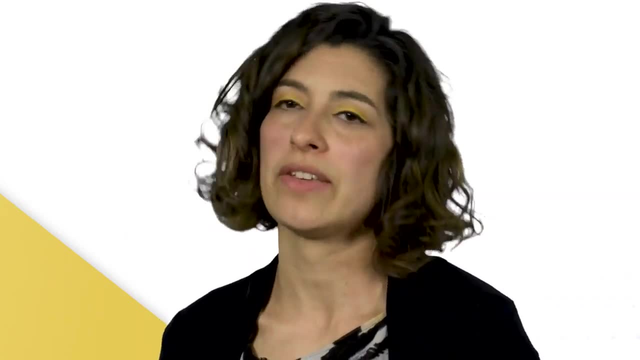 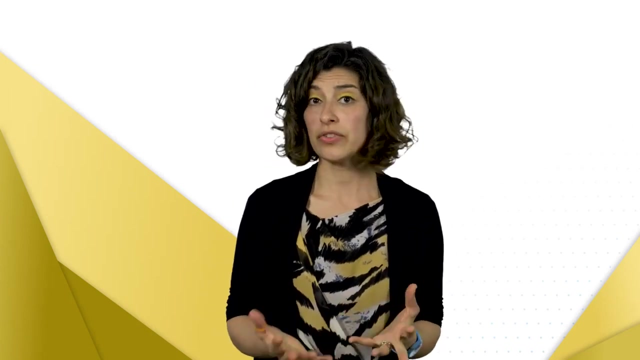 One sword is used. The first person in the circle kills the person to their left. Another sword is taken by the next person alive and the person kills the next person to their left. The process went on like this until there were only two people alive. 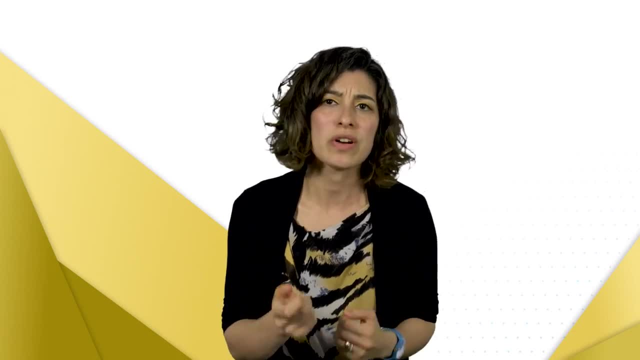 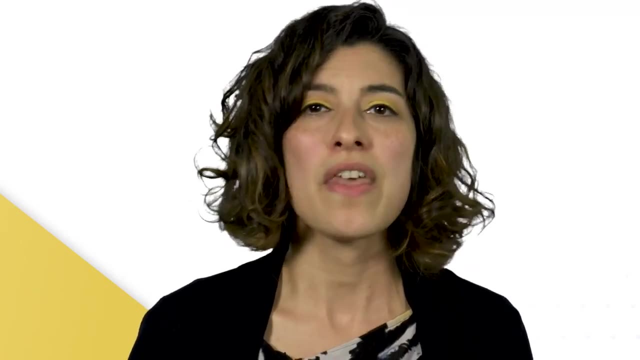 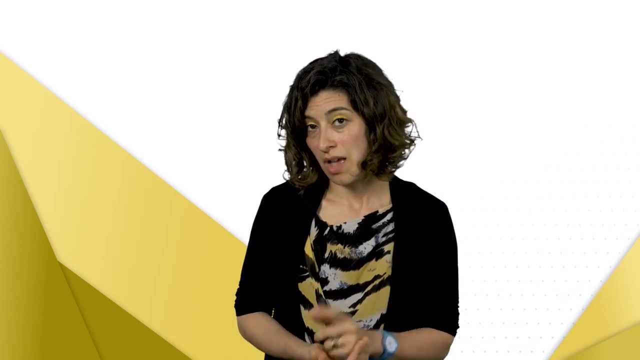 The instructions were so that the last two would stab each other at the same time. Only that Josephus was the last person holding the sword and convinced the other person that they could disguise themselves as Romans and survive. He lived to tell the tale. So where in the circle was he? 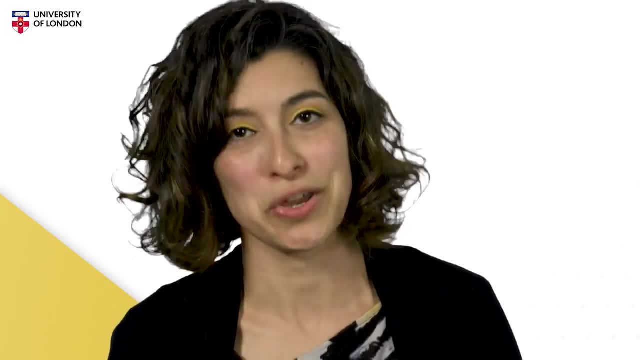 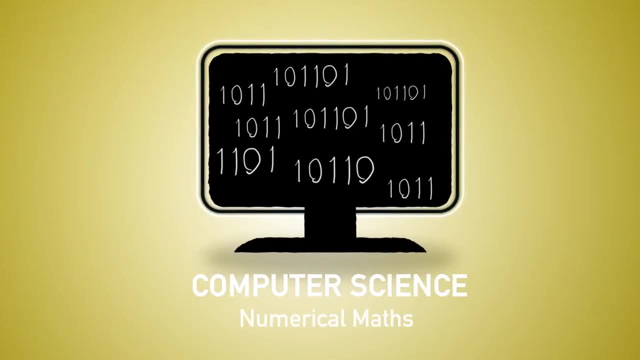 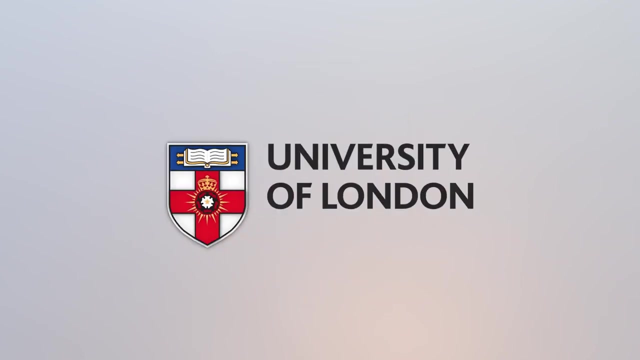 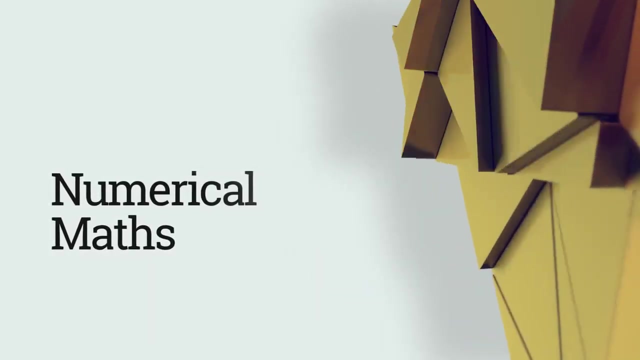 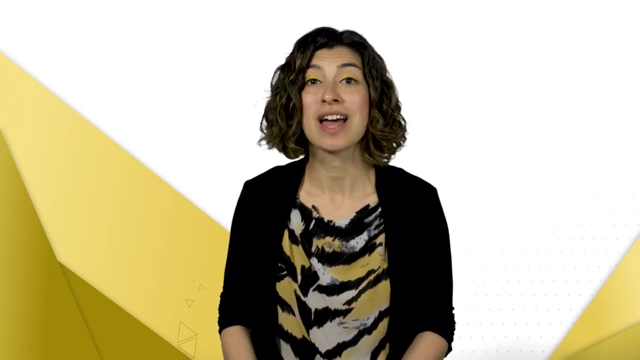 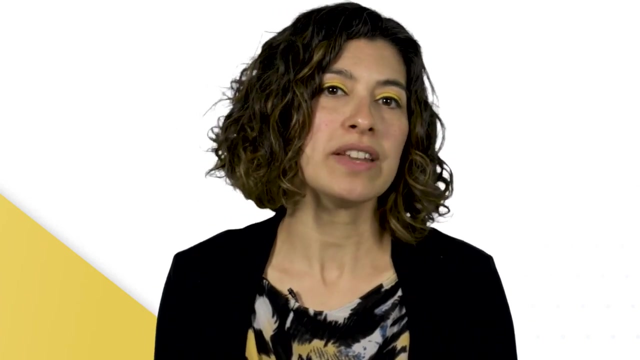 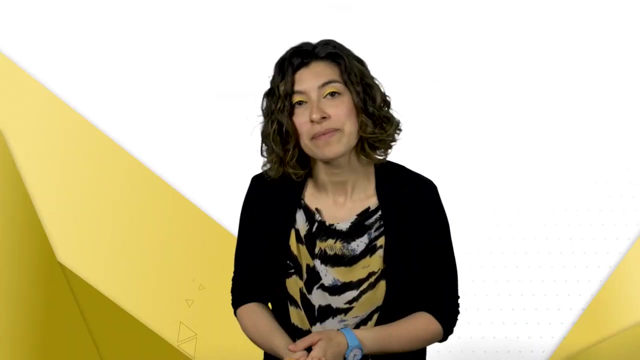 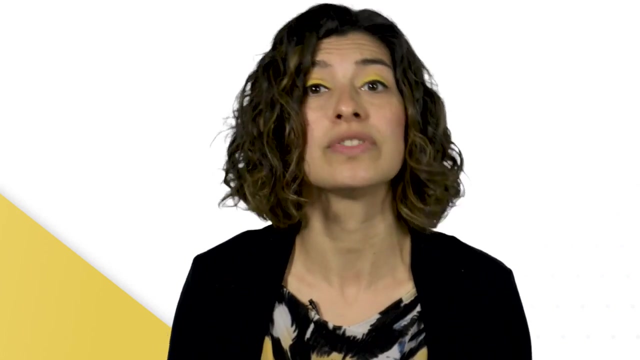 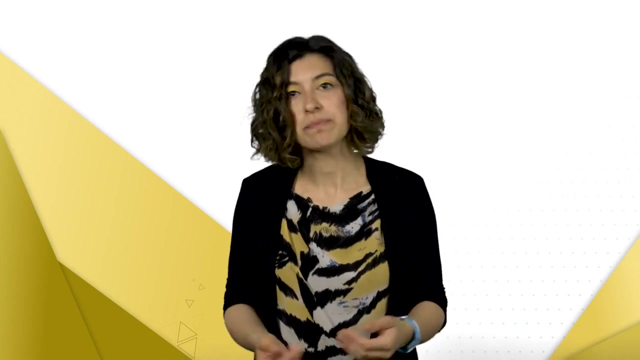 And how did he work out the correct position to guarantee he was to live? I no. Now the big question is about the answers. Is it real? Will he wear red? What does he look like? A Christchurch we're going to use is a public key cryptosystem as a scrambling key can be. 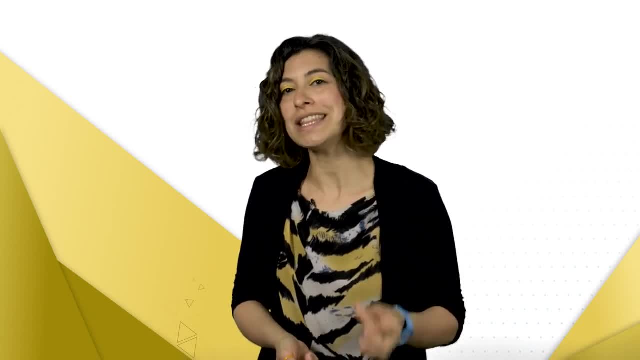 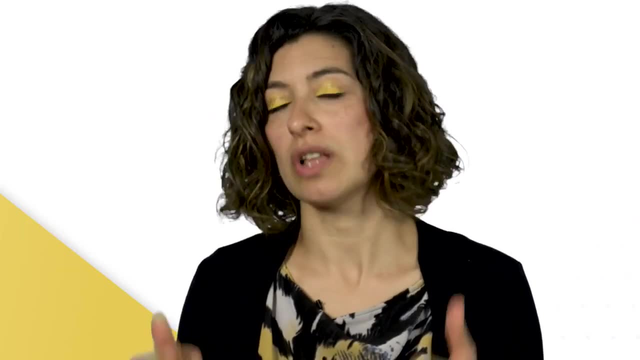 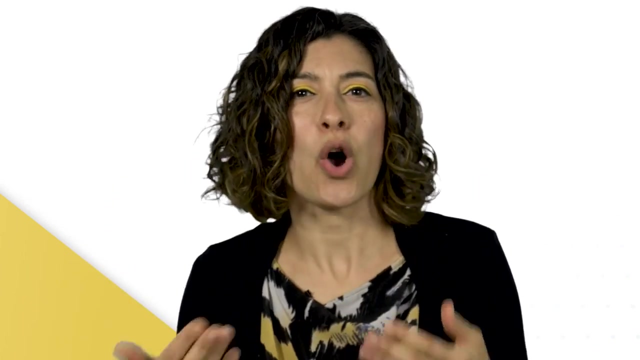 given to anyone to encrypt a message, but only the holder of the private key can unscramble it. Think of it as a post box with a special lock. The public key can only be used to put a message inside the post box, like the opening of a slot to. 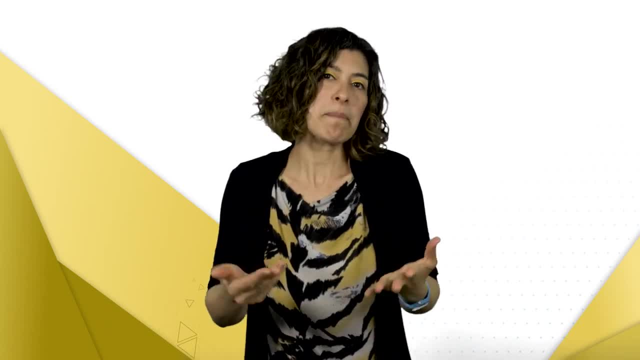 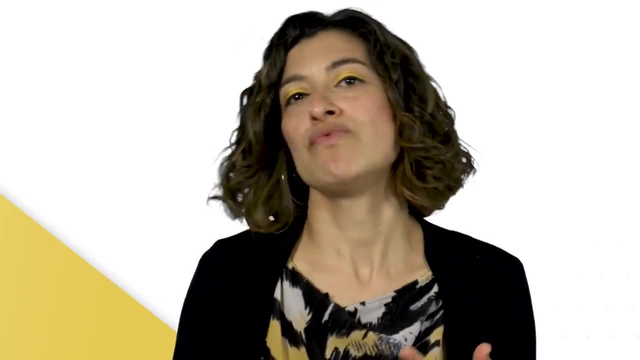 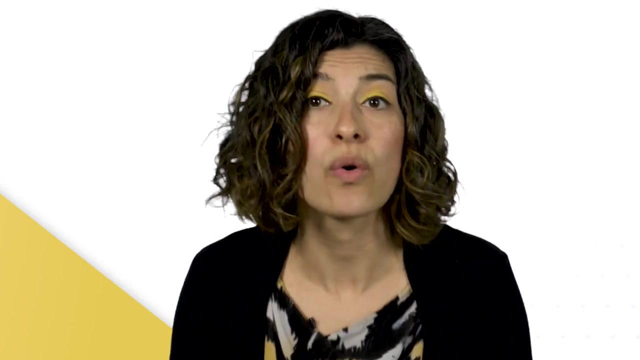 feed messages through and the private key is a sort of master key that opens the compartment where all messages are. The post box owner is the one that receives messages. They own all the keys and have given copies of the public key to anyone who wants to send the owner messages. If you want to learn more about 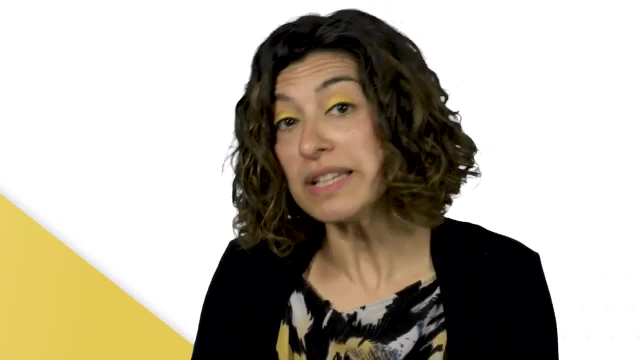 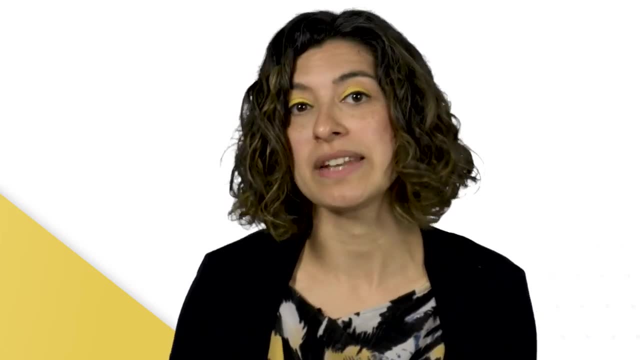 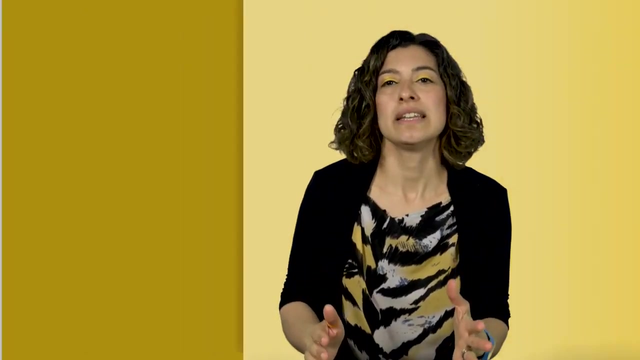 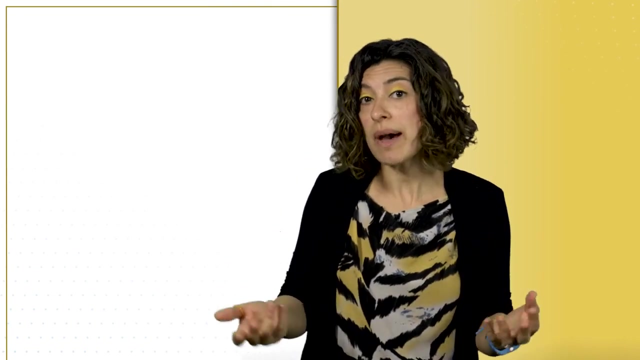 encryption: read the further reading section. but please note that encryption itself isn't a learning outcome for this module. but understanding the mathematics for this particular method exposes you to a new world. We said earlier in the module that everything is number, Letters and symbols in a written message can be converted into a number or several. 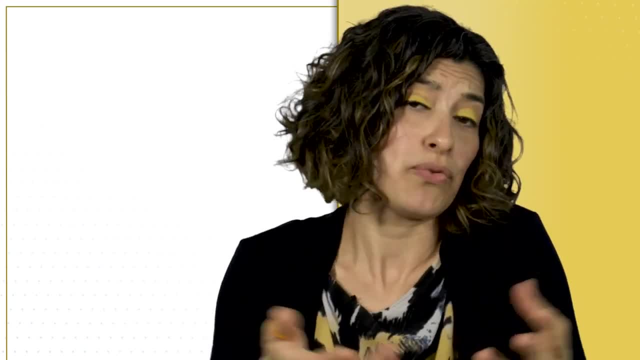 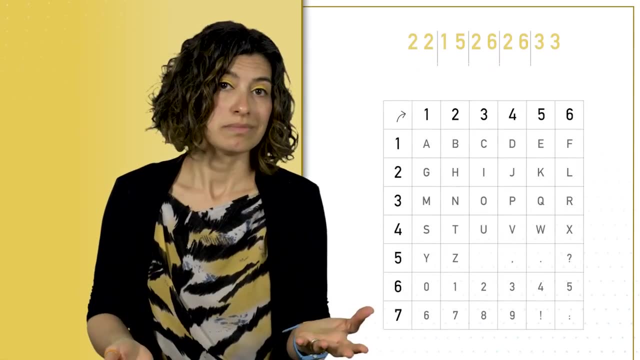 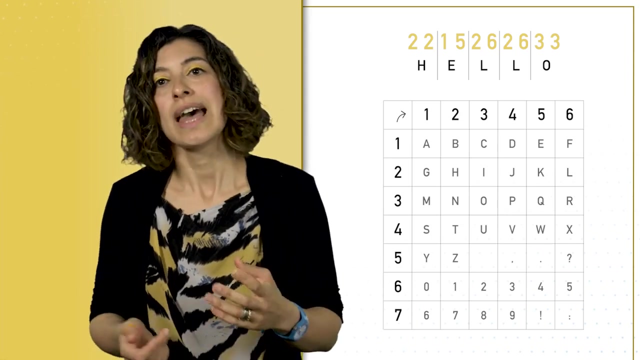 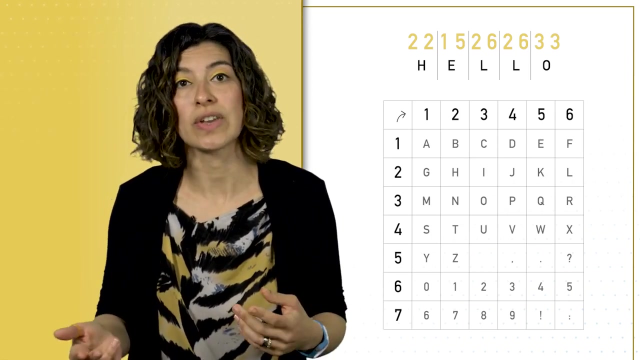 numbers. There are many ways of doing this. For example, we can use my table that we've seen earlier and the message hello could be 22 for H, 15 for E, 26 for L twice And 33 for O, And so we could have the number 2, 2, 1, 5, 2, 6, 2, 6, 3, 3, making up the 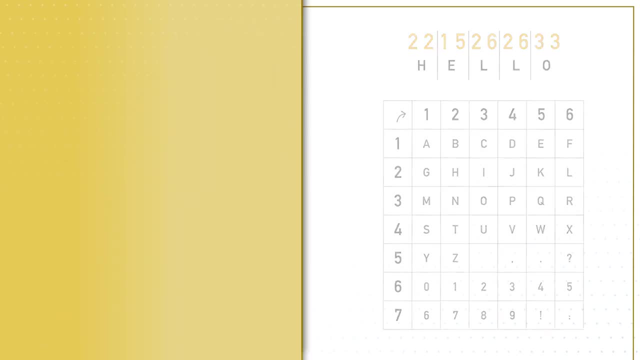 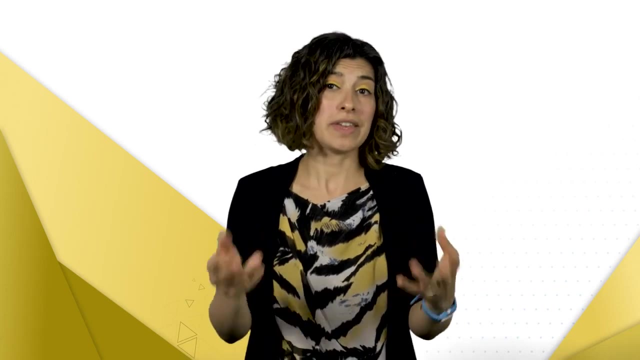 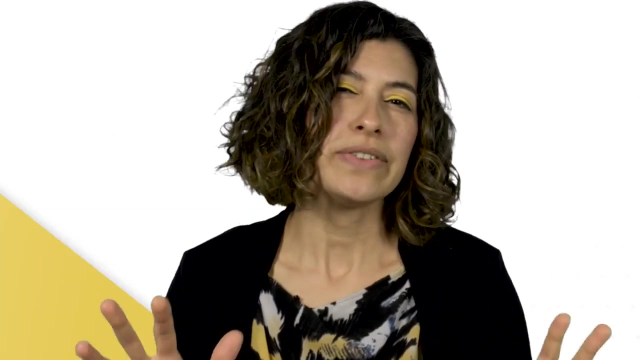 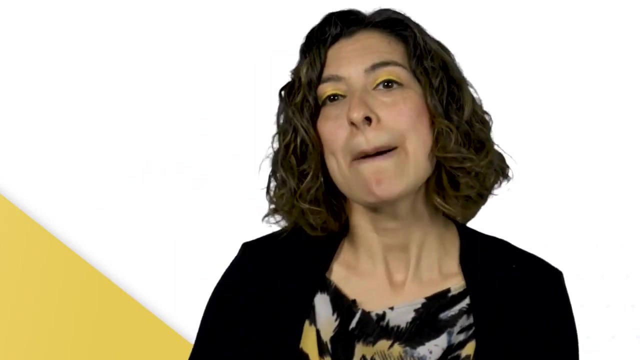 message. There are standard ways of encoding a message into a number, but we won't be exploring such methods here. So in this next task we will just assume that the messages are numbers. And here is the main idea: A secret message, remember. a number is encrypted by raising it to a certain power in modular. 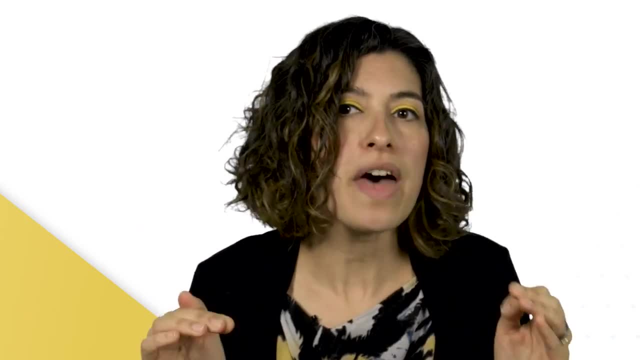 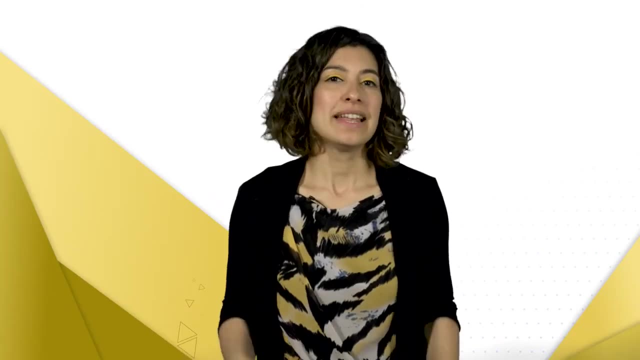 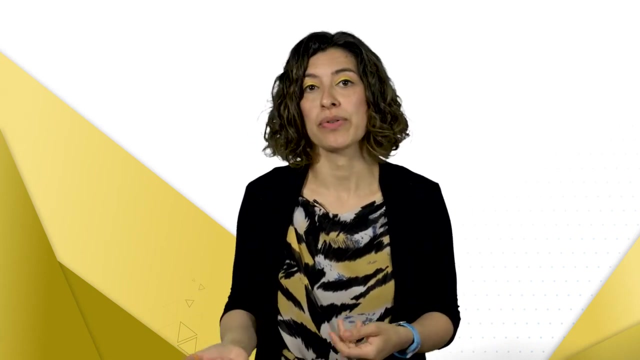 arithmetic. Then there is another power: you can raise the encrypted message to returning the message you started with. Let's imagine Bob is going to send messages to Alice. He has the public key and Alice has both. The keys are the powers? Follow me. 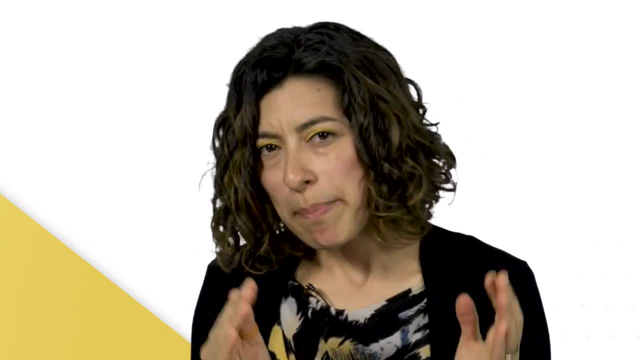 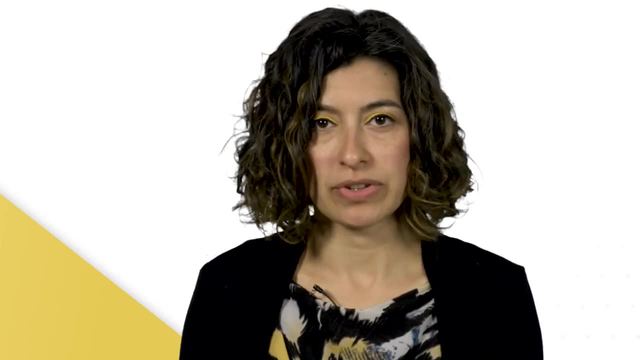 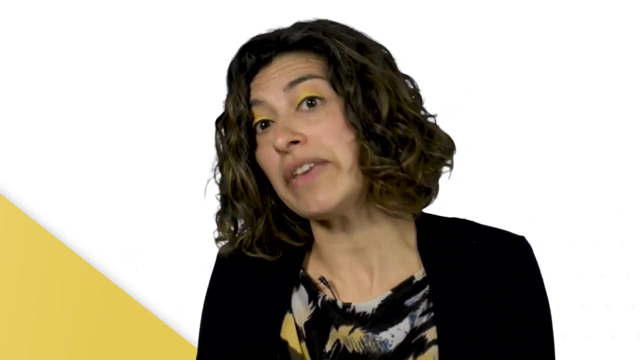 The whole process is like this: Say Bob raises the message to a power in modular arithmetic to encrypt the message And he sends Alice the encrypted message. Alice then raises this message to another power in the same modulus and that returns the message Bob wanted: Alice. 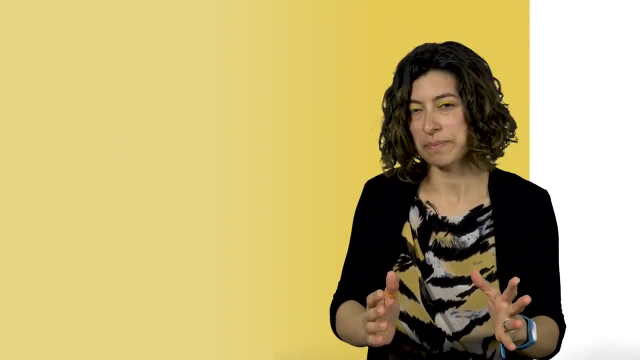 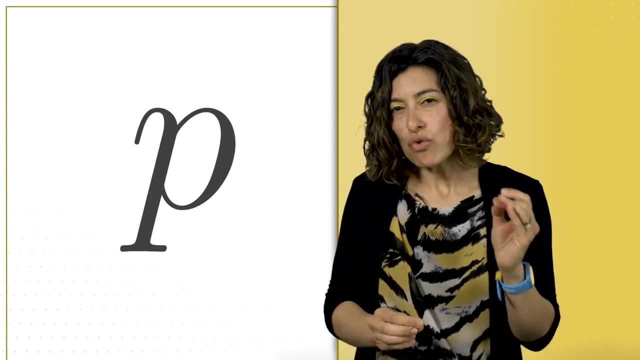 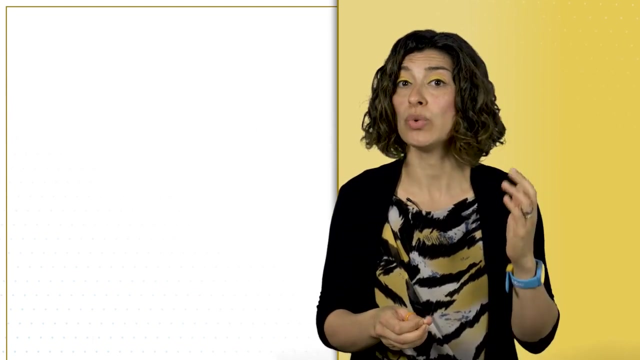 to read. And here is the set up: We're going to use a prime number and we're going to call it p. The original message to be kept secret will be called m, And m has to be a number between 1 and p minus 1 so that it survives the. 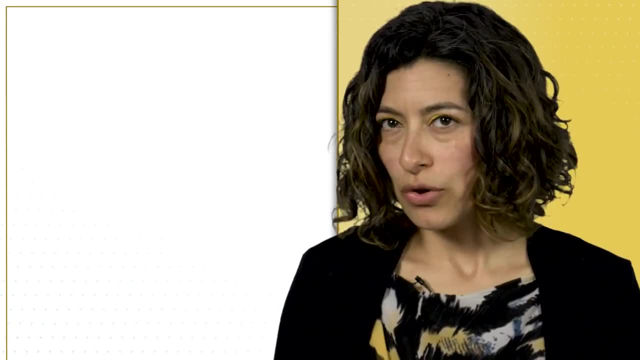 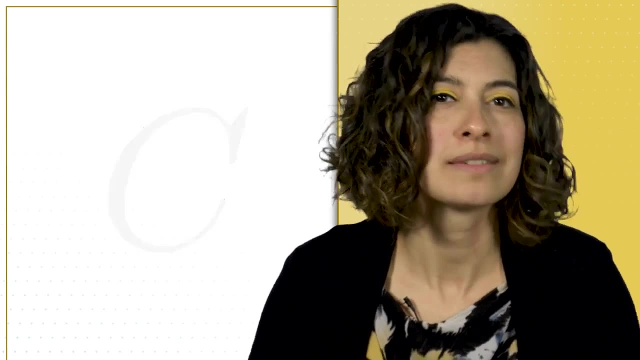 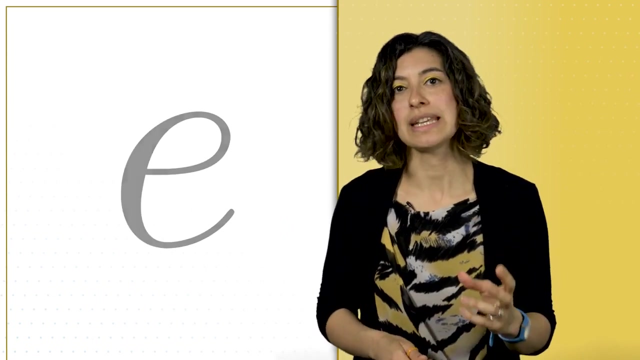 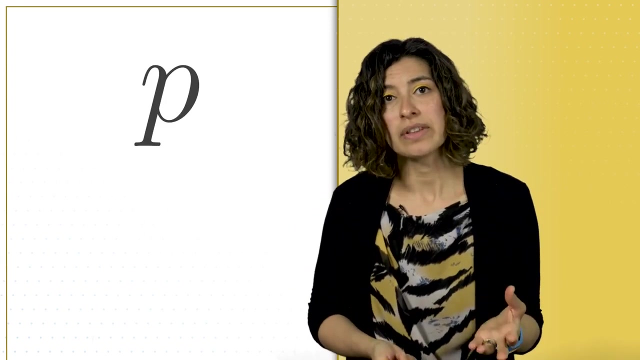 encryption and decryption process. When we encrypt the message m, the resulting scrambled message will be called c for cryptic, Two special numbers: An encryption key e and a decryption key d. The public keys will be the number p and the number e. The private key will be d. 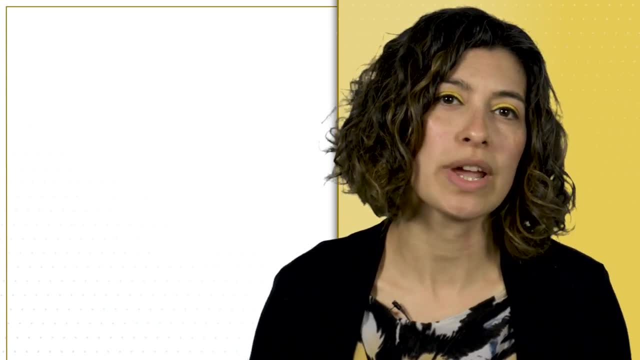 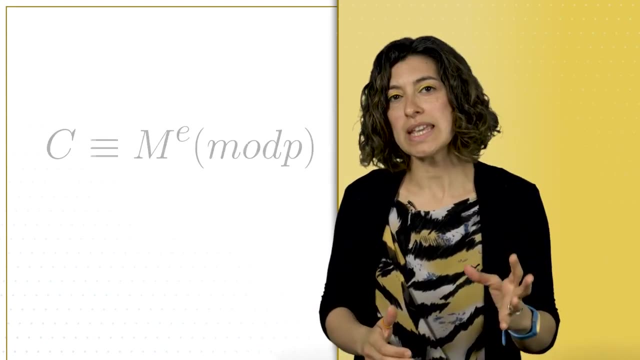 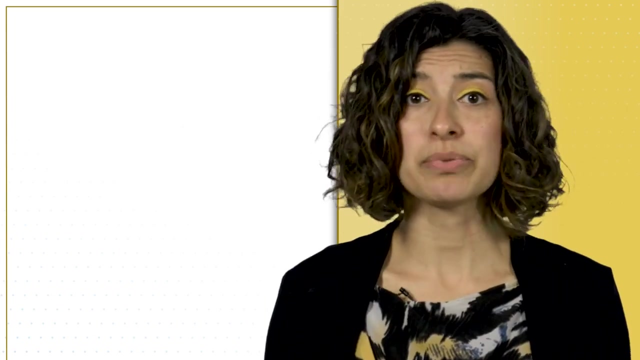 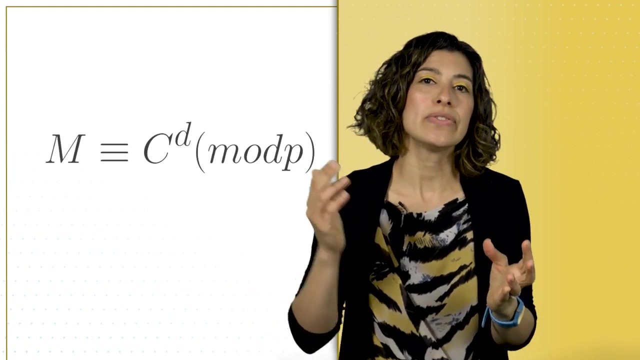 And here is the procedure for encryption. We are going to operate in modulus p. for the encryption and decryption process We do c. This is congruent with m to the power of e modulus p. And here is the procedure for decryption. We operate in modulus p. so m will be recovered by doing c to the power of d modulus p. 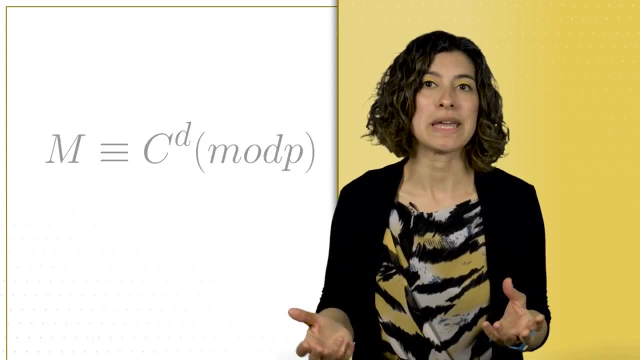 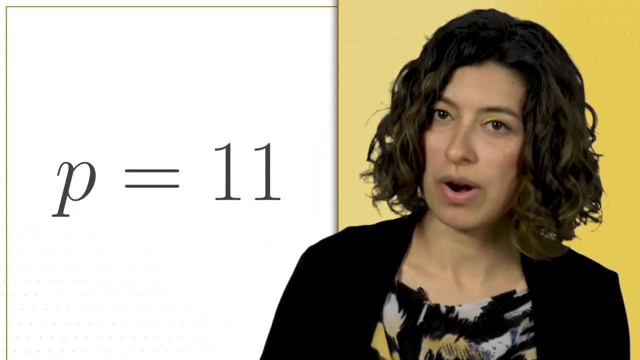 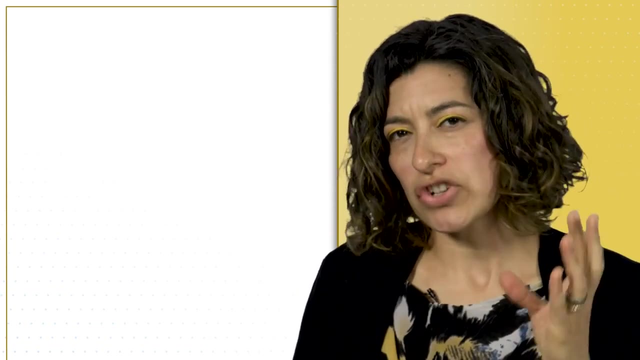 So m is congruent with c to the power of d mod p. This means that if Alice issues out public keys, p equals 11,, which is prime, and e equals 3, and it gives them to Bob. Bob wants to send the message: m equals 5, so Bob does the. 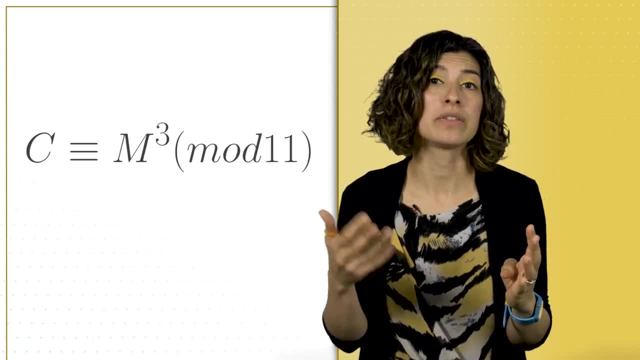 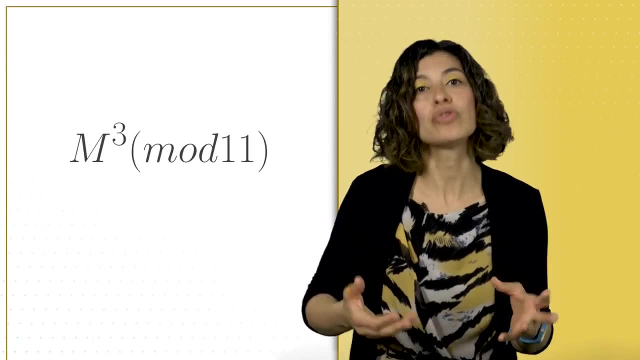 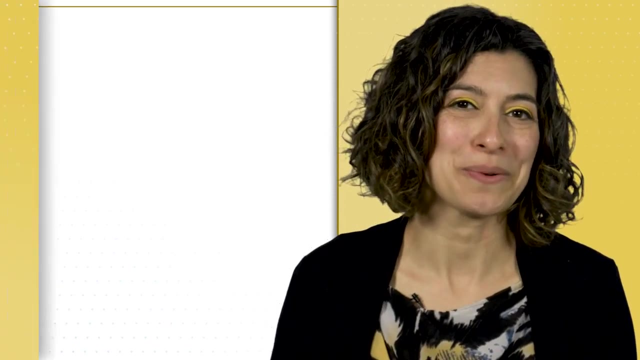 following: c is congruent with m to the power of 3 mod 11.. So he works out what m to the power of 3 mod 11 is and he calls the result c. That's the encrypted message. Work this out yourself before you continue watching the video. 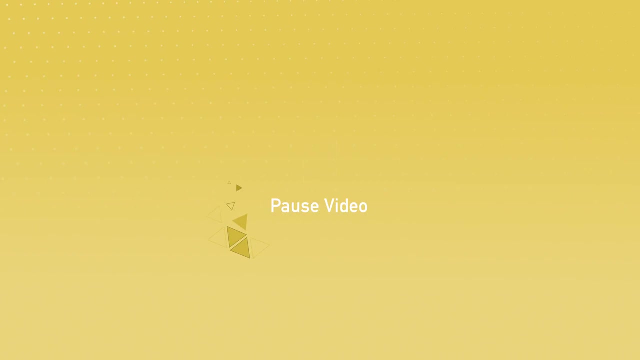 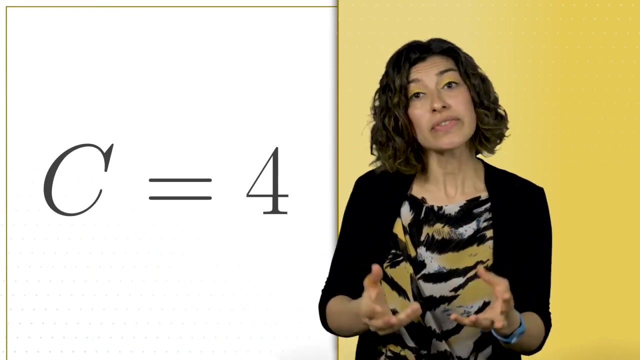 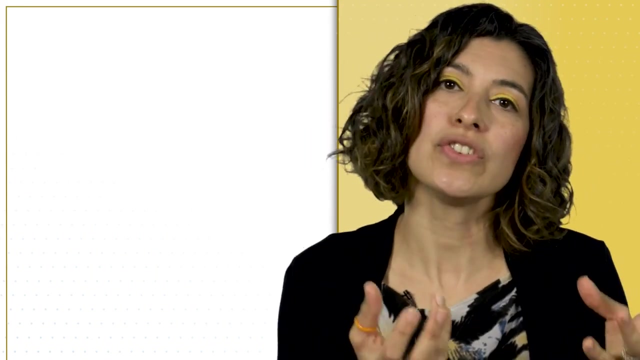 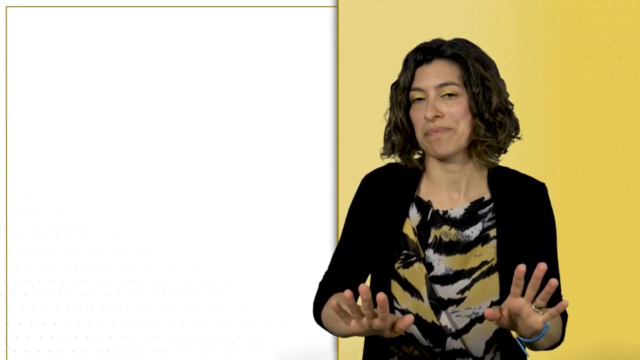 Yes, the result is that c equals 4.. So he sends c equals 4 to Alice the encrypted message. Now Alice wants to decipher this message, so she's going to use the private key: d equals 7.. For now, don't worry about where the private key comes from. 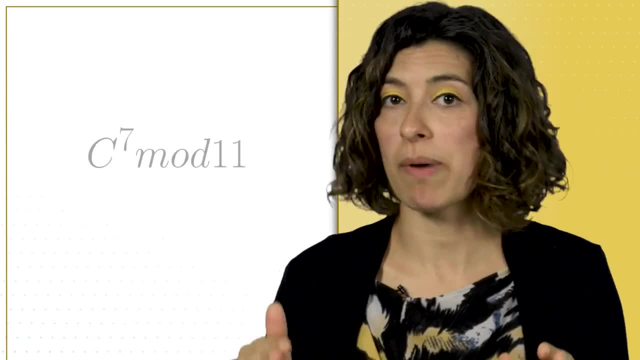 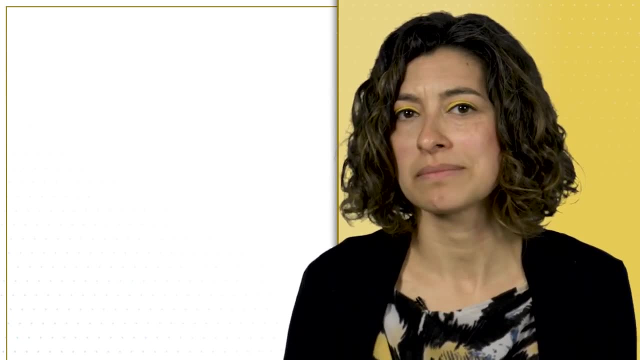 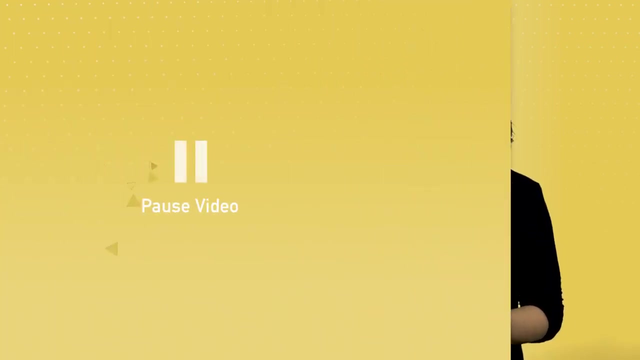 Just follow me. Alice calculates c to the power of 7 mod 11.. The result will be the same as the original value of m. Work out c to the power of 7 mod 11 yourself before continuing watching the video. Continuing the calculation: it gives that m is 5, as Bob intended. 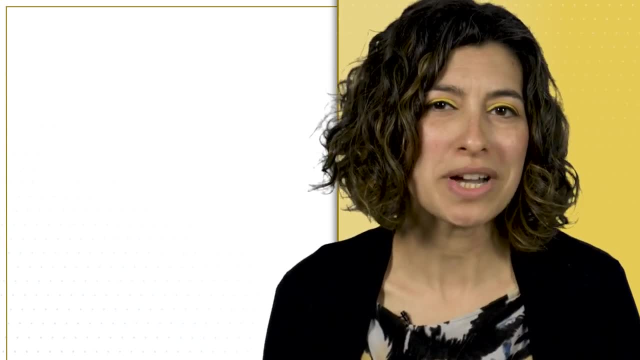 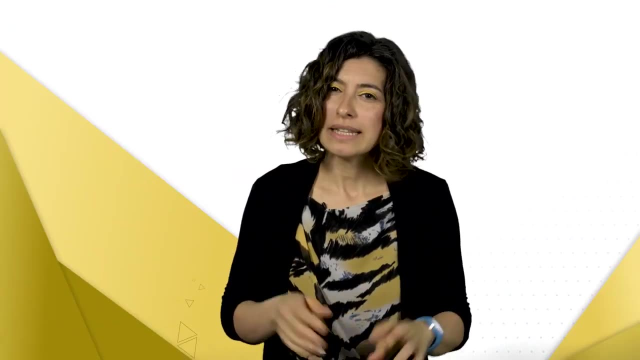 Are you asking yourself? why Are you asking yourself? why does it work? We will talk about it later, but you go ahead and discuss your thoughts in the discussion forum. In the discussion forum, you can follow the discussion prompt. post encrypted messages for others to decrypt. 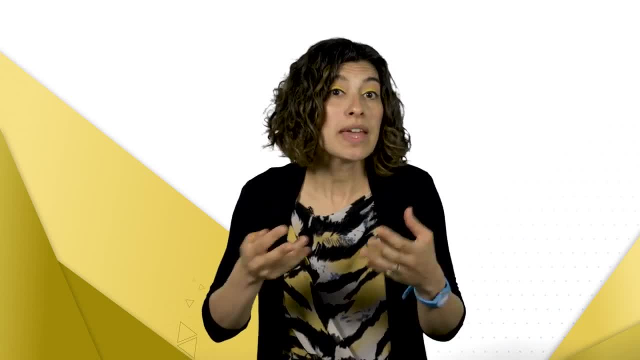 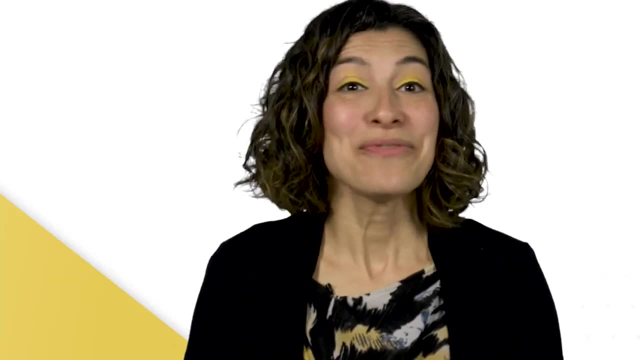 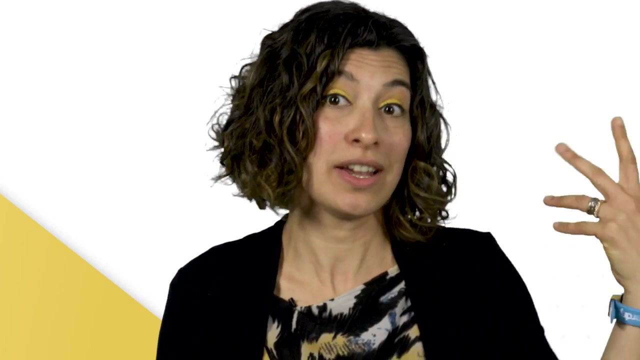 You need to post the message c and use the same keys as we used in this example, Then read the encrypted messages of other people and decrypt them If you want to up the game, actually write a message and convert it into a message, Convert it into numbers using the two-way table I just showed you. 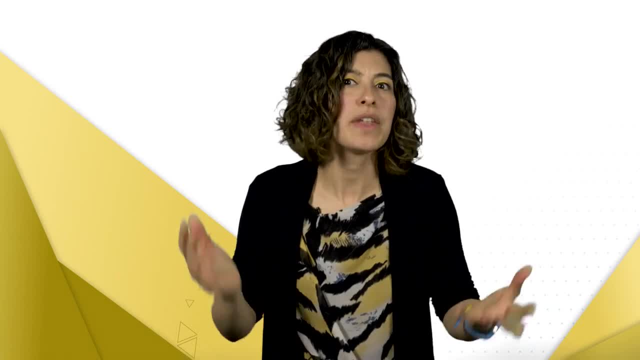 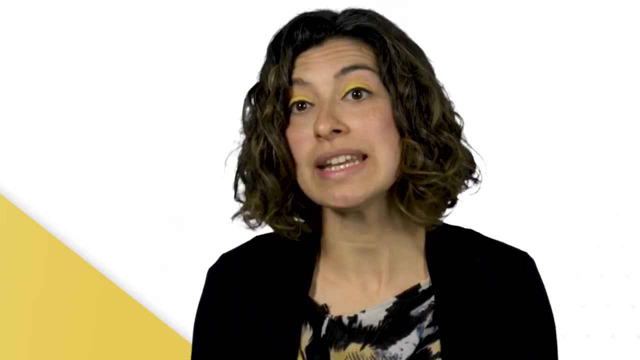 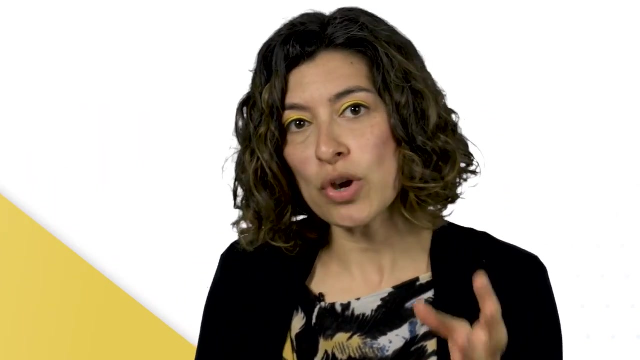 You can discuss with your peers how to use the numbers Now to make the game playable. do make it explicit that you are sending an encrypted message by saying c equals the number When you are decrypting. check with your peers if your result m equals. 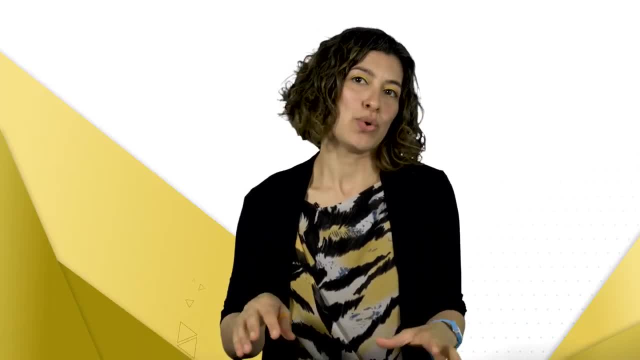 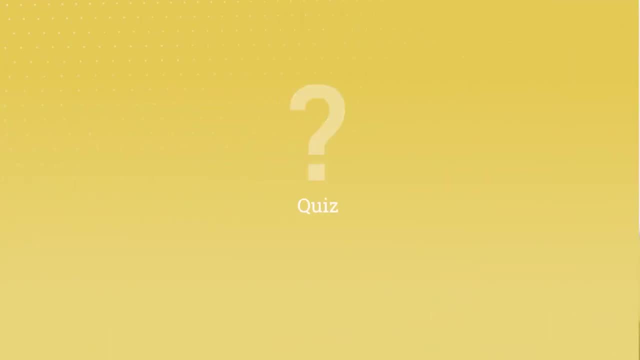 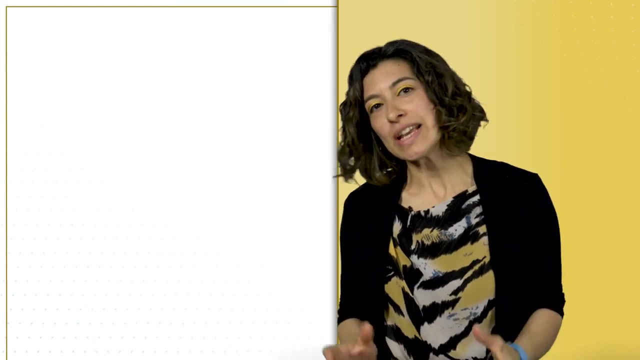 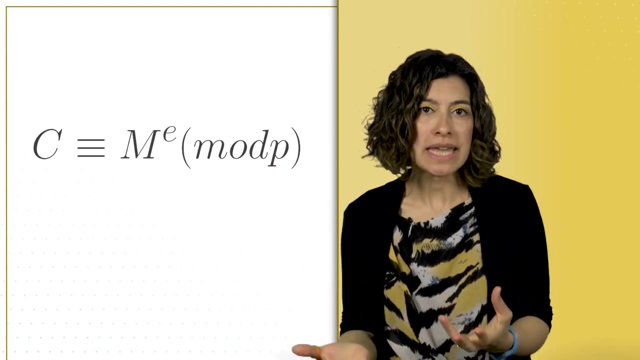 Your result is correct. Try this in-video quiz and replay the last part of the video and the modular arithmetic videos if you need. So why does it work? Why does encrypting m into c by doing c congruent with m to the power of e, mod p and then doing 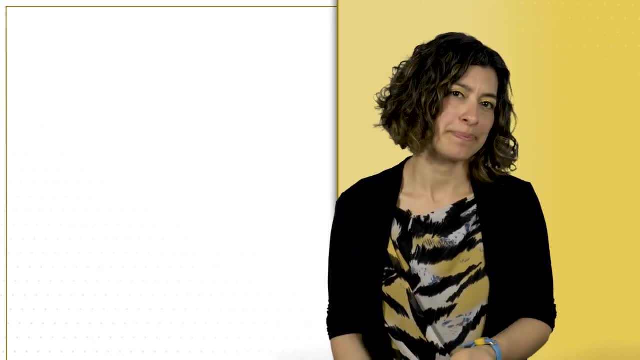 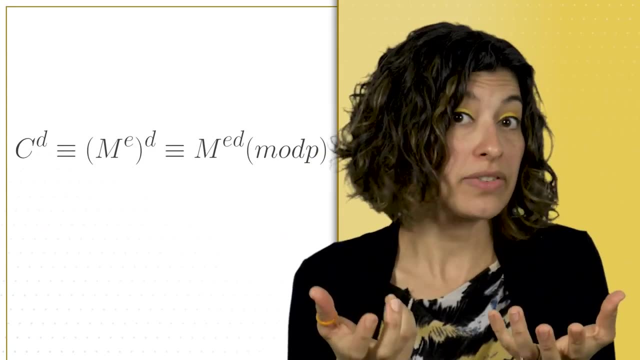 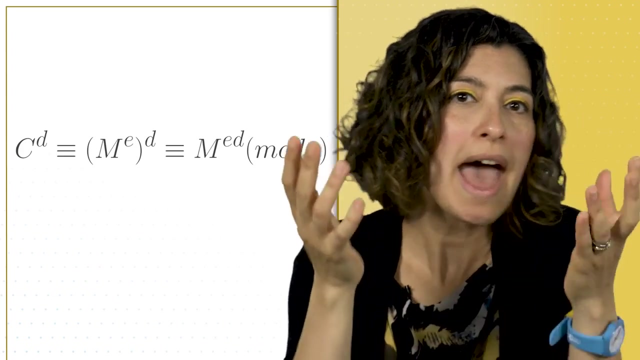 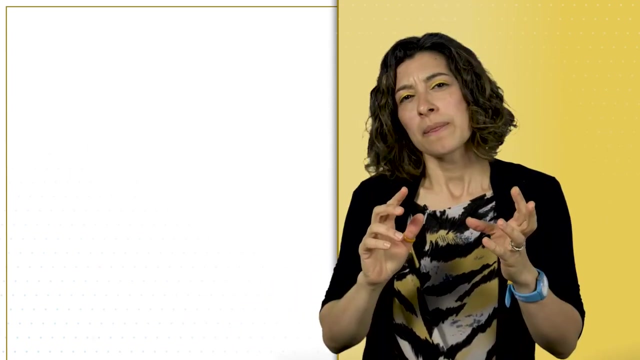 c to the power of d mod p, retrieve m. It is congruent with m. to the power of e, that's the c, and then to the power of d, And that is congruent with m to the power of the product of e, d in mod p. 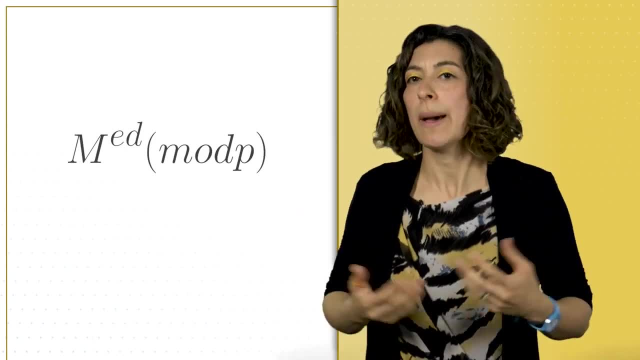 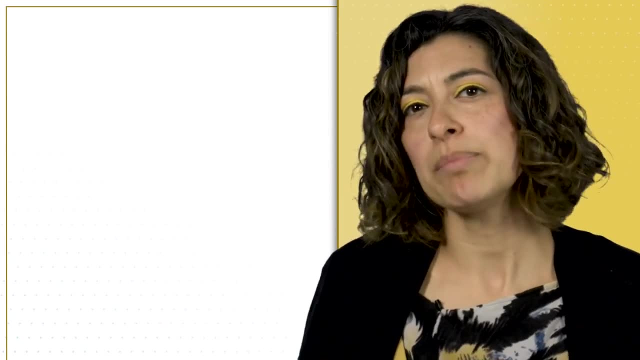 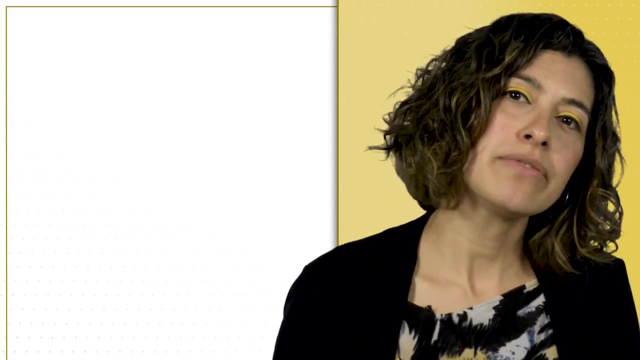 So what is m to the power of e d mod p? To start with, what is e d In the examples we saw in mod 11,? so p equals 11, e was 3 and the private key was d equals 7.. 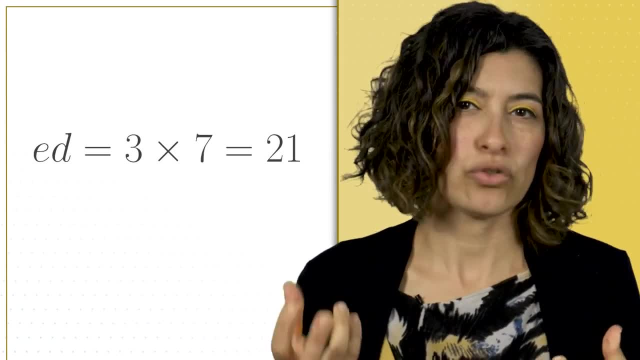 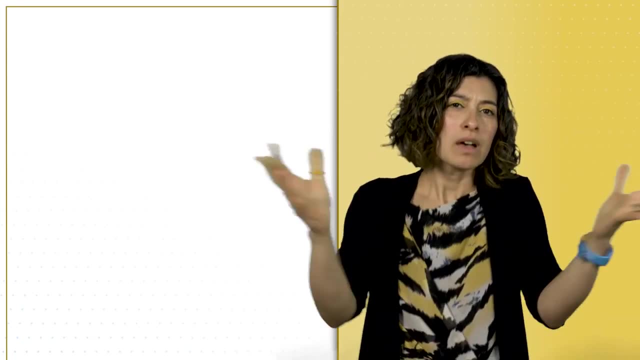 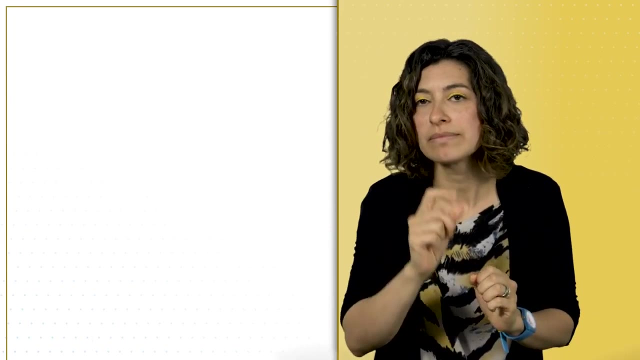 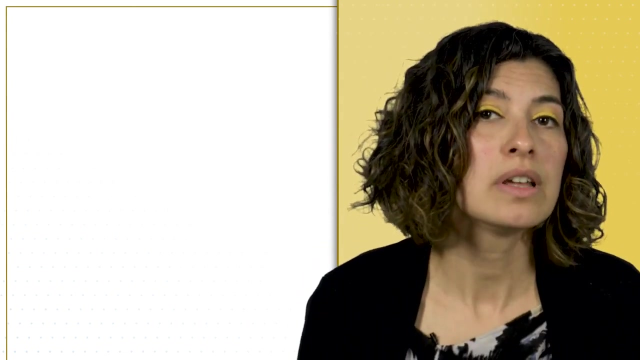 So e times d, 3 times 7, is 21.. But you wonder what is so special about 21?? Well, in mod 11, the special power that turns any number into 1 is power 10.. From Fermat's little theorem we have that a to the power of 11 is congruent with a itself. 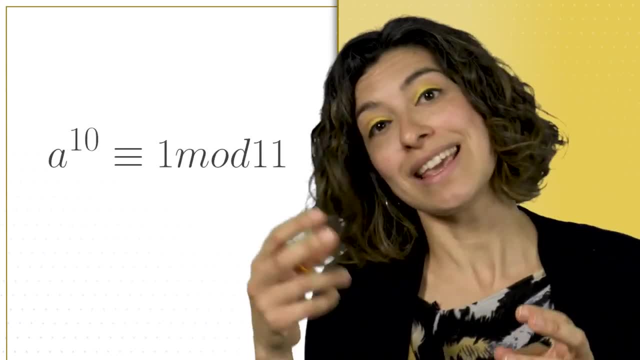 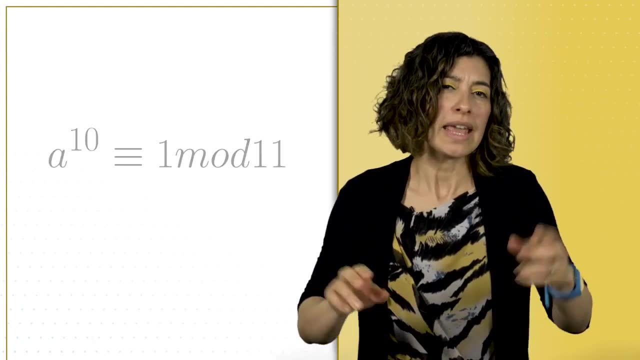 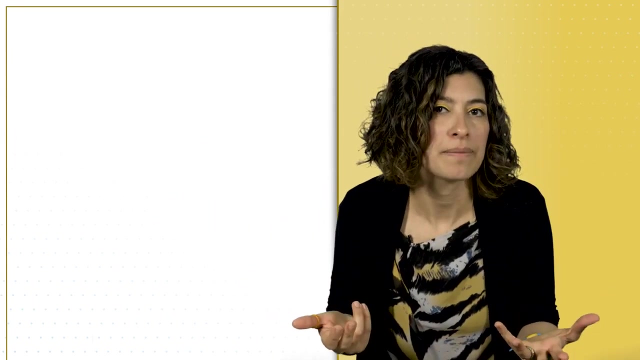 mod 11.. And that means that a to the power of 10 is congruent with 1 mod 11.. Now, what about 21?? Let's see: a to the power of 21 is congruent with a to the 10 times a to the 10 times a. 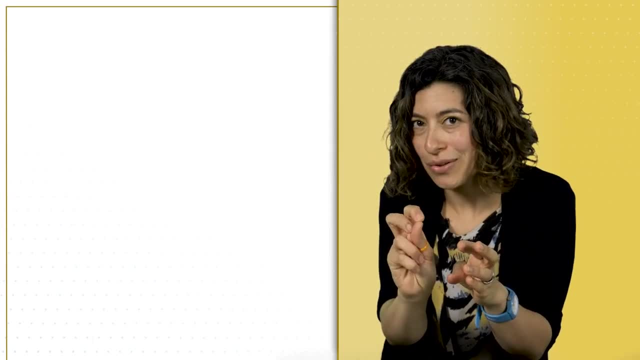 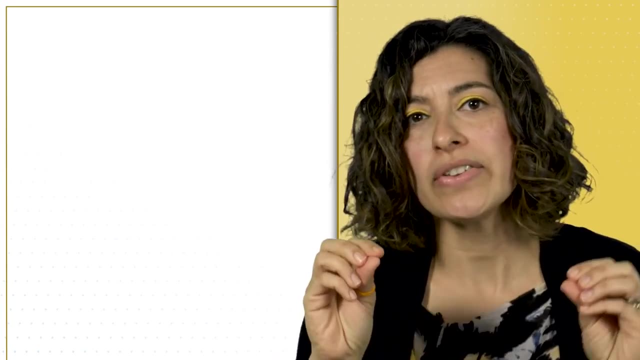 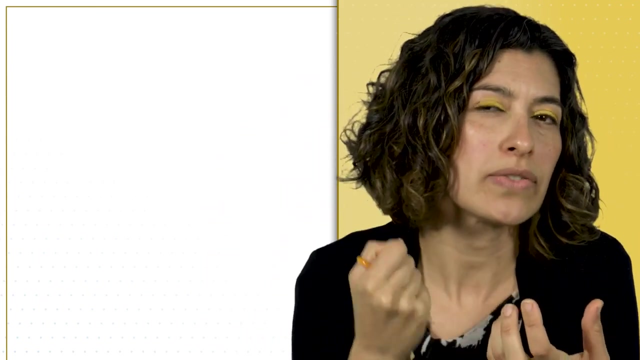 And that is congruent with a itself, Because a to the 10 is 1 in mod 11.. So 21 is special because it is a multiple of 10. 10 being 1 less than the modulus, 1 less than the 11.. 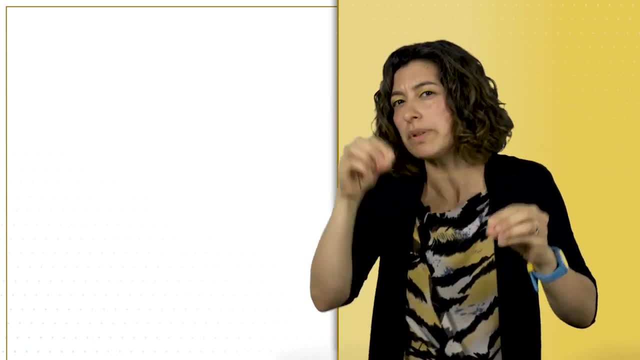 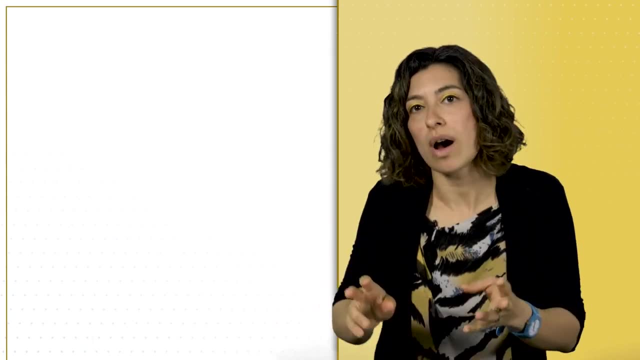 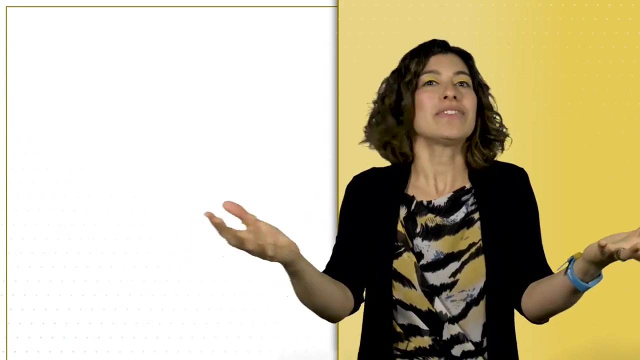 So 21 is a multiple of 10 plus 1, meaning that 21 is congruent with 1 mod 10.. Not mod 11.. OK, Mod 10.. What this means is that 3 and 7 are inverses, modulus 10.. 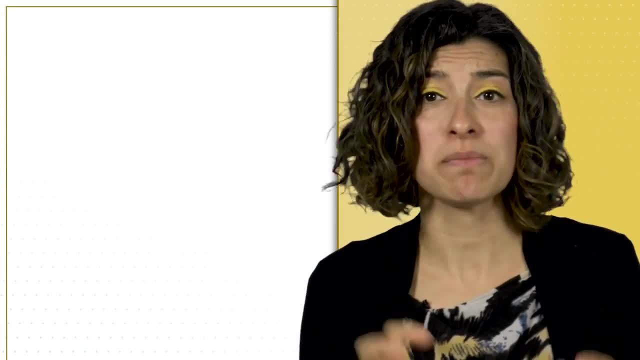 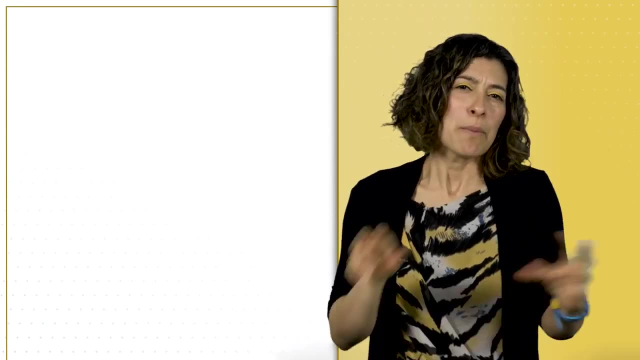 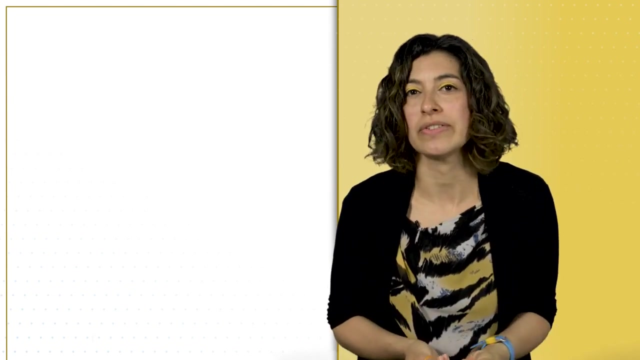 So this is the clever thing that Rivest, Shamir and Adelman saw in inverses in modular arithmetic to create this system. Now back to Alice. She concocts the private and public keys d and e by finding inverses mod p minus 1.. 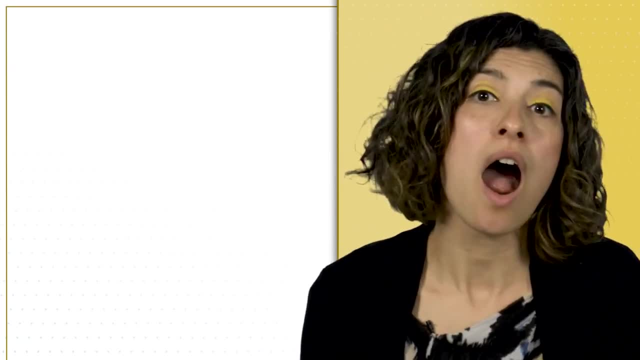 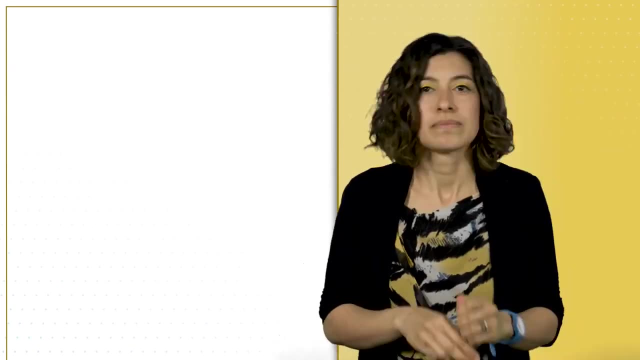 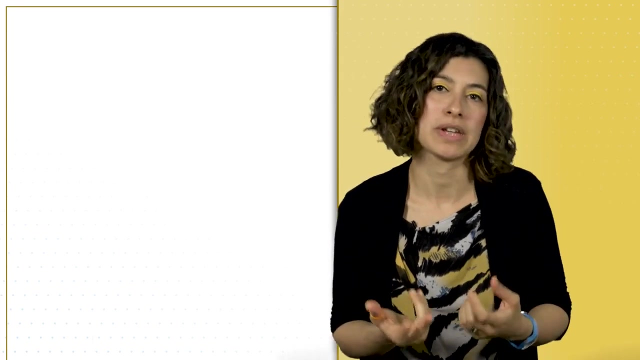 But she knows that the only numbers that can be used as keys are numbers e and d that have no factors in common with p minus 1.. I'm not proving this result here, but you may have worked this out in one of the quizzes on multiplicative inverses, mod n. 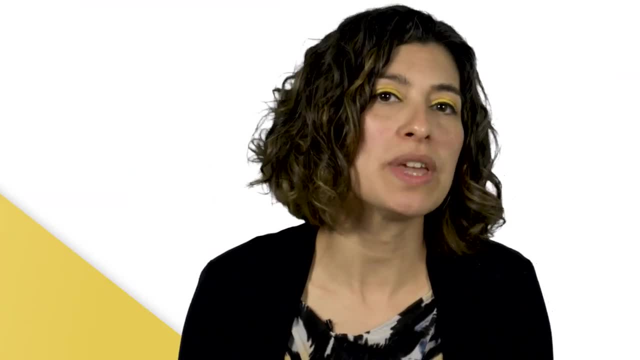 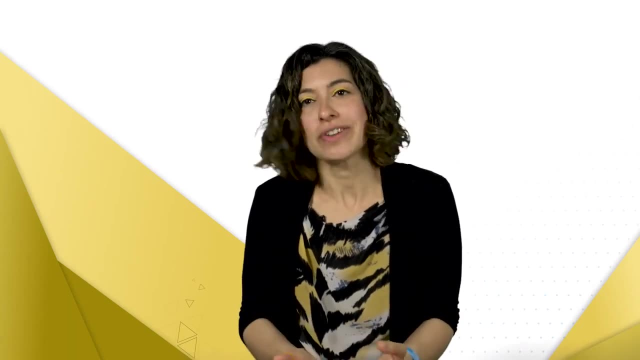 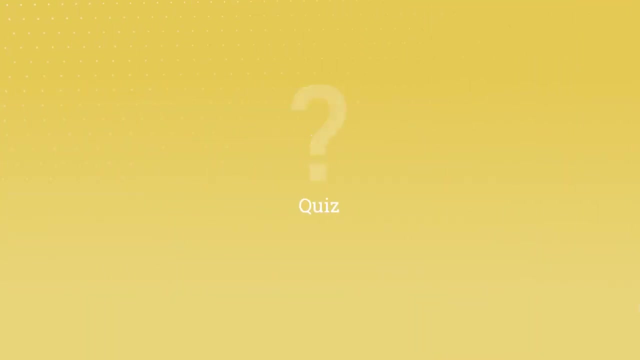 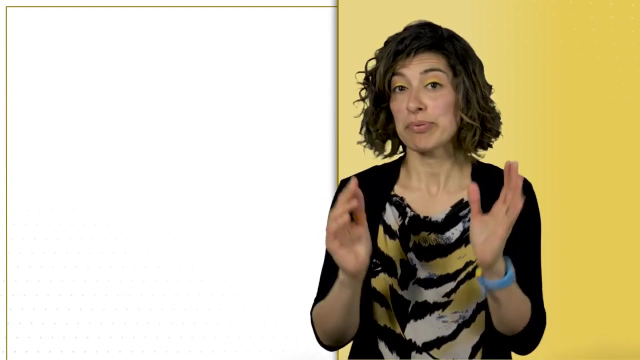 Now, are there any other numbers we can use as keys in encryption? mod 11? Meaning, are there other inverses mod 10? And how does one compute inverses mod 10?? We saw earlier that in mod a prime we use Fermat's Little Theorem to help. The strategy is to calculate the special power of a number that is equivalent to 1.. In mod a prime prime p, that special power is power p minus 1, as a to the power p is congruent with a mod p, meaning that a to the power p minus 1 is congruent with 1 mod p. 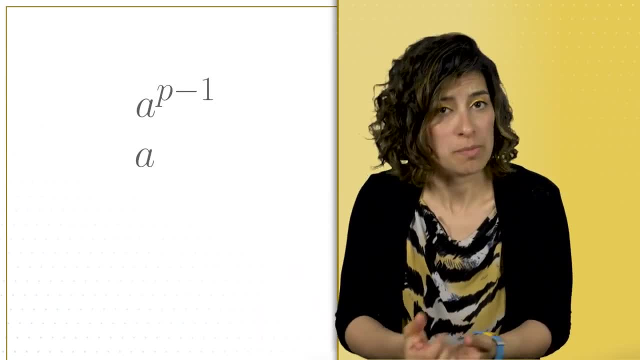 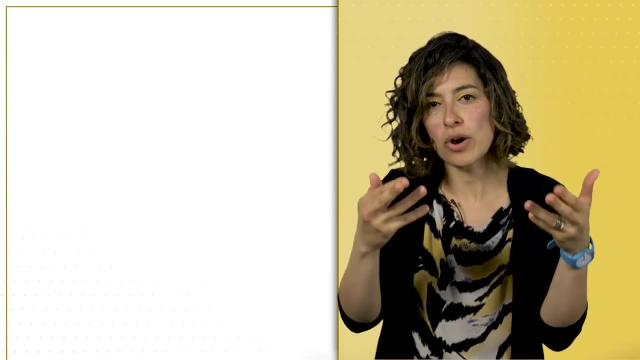 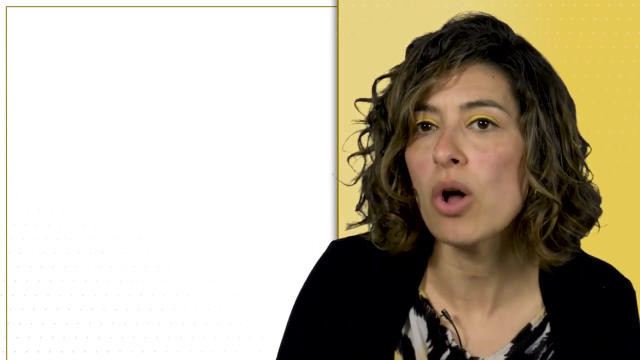 And so a to the power p minus 2, and a are inverses mod p. That means that the special power for mod p prime is power p minus 1.. It may happen that there was a smaller power giving 1, but the theorem says that if you don't know otherwise, 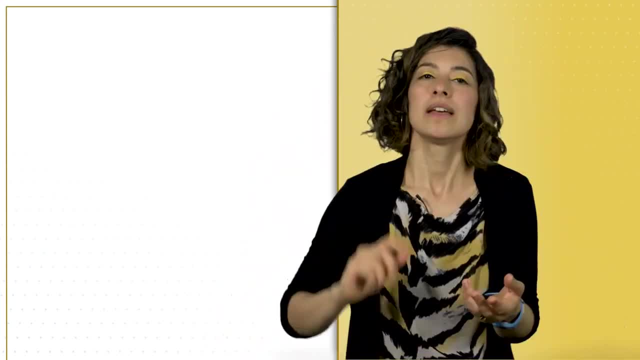 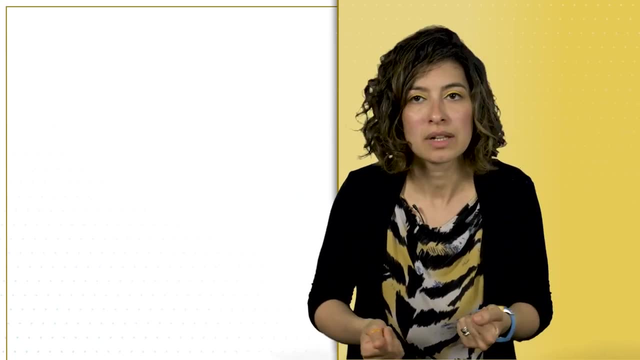 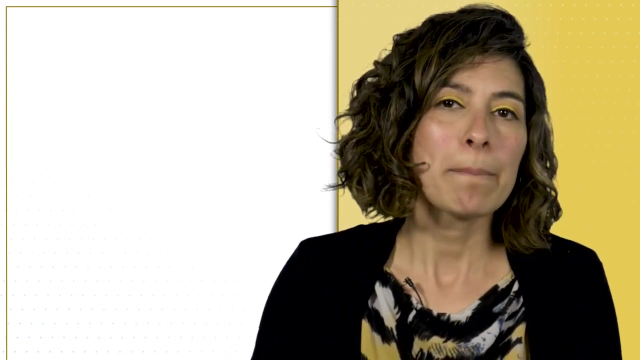 try this special power: p minus 1.. That's all good for primes. How about for composite numbers? Number n, say n, equals 10, meaning working in mod 10.. It turns out that the special number here is given by how many numbers, from 1 to n minus 1. 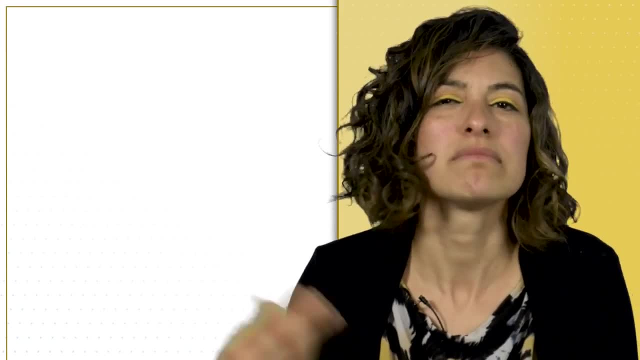 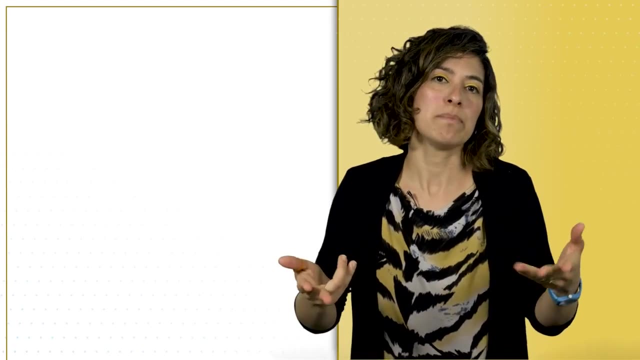 that have no factors in common with n. That means co-prime with n. In our example, n equals 10, and we're looking at numbers between 1 and 9 that are not divisible by 2 and also not divisible by 5,. which are the factors of 10.. In mod 10, we will only work with numbers 1,, 3,, 7 and 9,, as all other numbers- 2,, 4,, 5,, 6,, 8- are divisible by 2 or by 5 or by both. 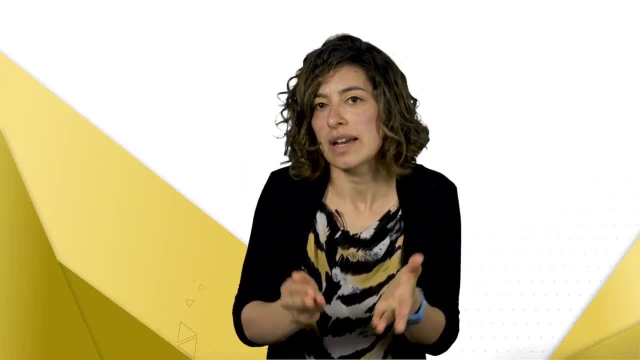 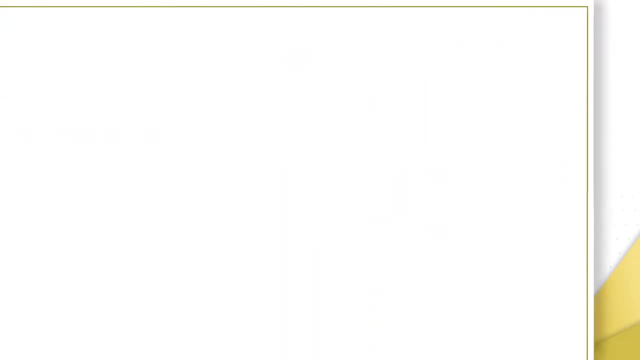 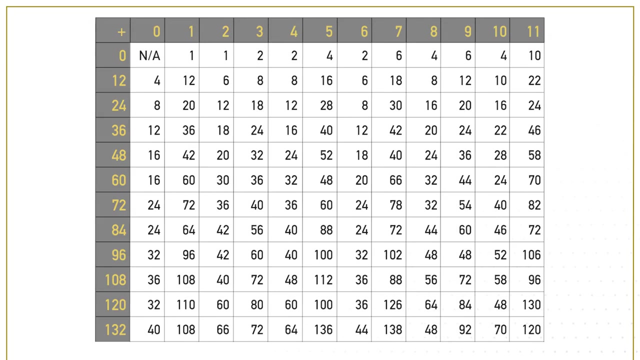 So 1,, 3,, 7 and 9 are 4 numbers and that 4 is the special power in mod 10.. For convenience, I'm including a table with the special power for several modeling. In this table you can find the power. 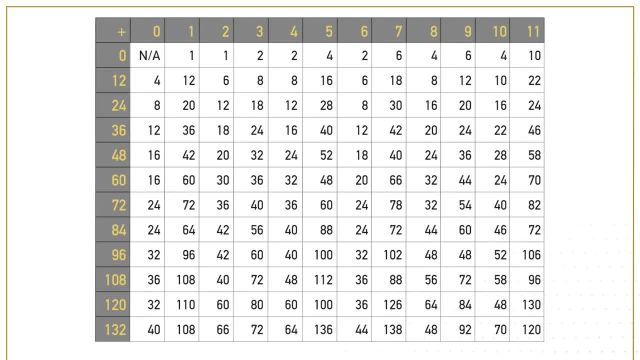 for mod 18 by looking on the row with 12 and the column with 6.. So 12 plus 6 is 18. And the special power is that number there, 6.. Again, there may be a smaller power that achieves the result. 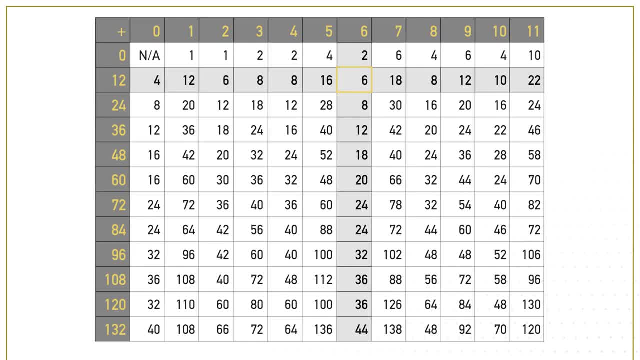 but we guarantee that the power on this table works. I haven't totally explained why this works, but you can work through the algebra if you fancy. The proof is outside the scope of the module. You can read the references in the further reading section. 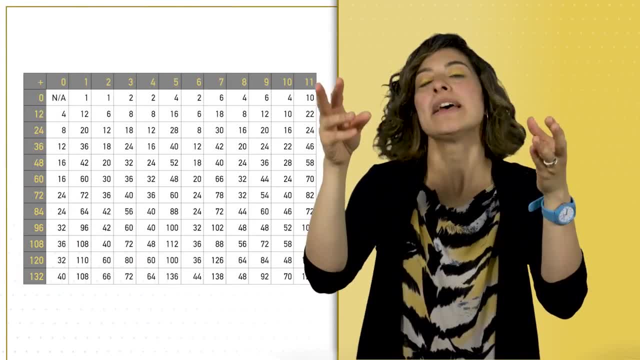 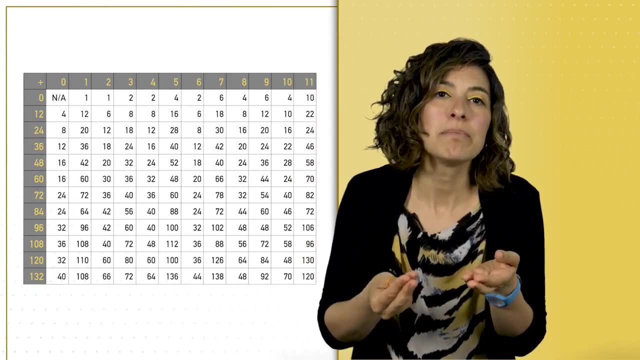 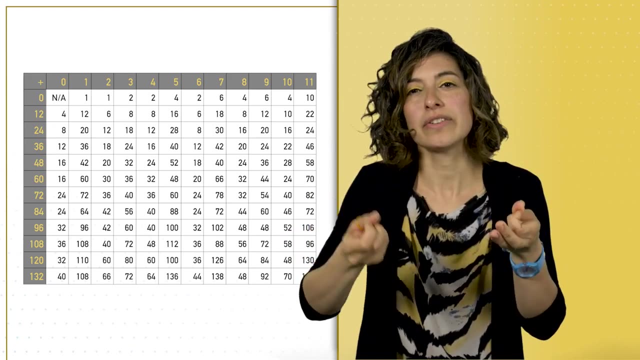 So how does this work? The special power for mod 10 is 4. And that means that all inverses are given by the lower power power, 4 minus 1, which is 3.. That means, to calculate inverses, we're going to take powers 3.. 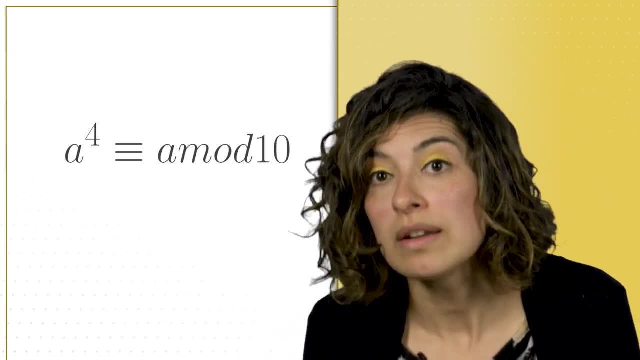 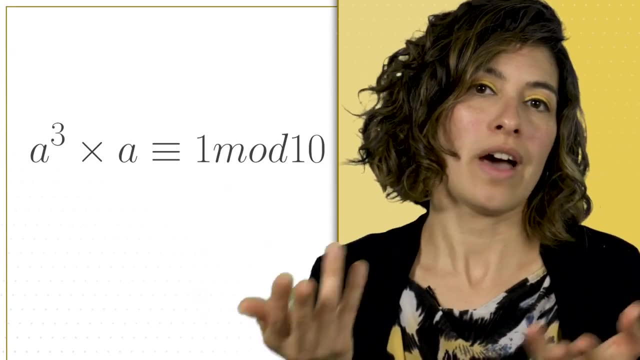 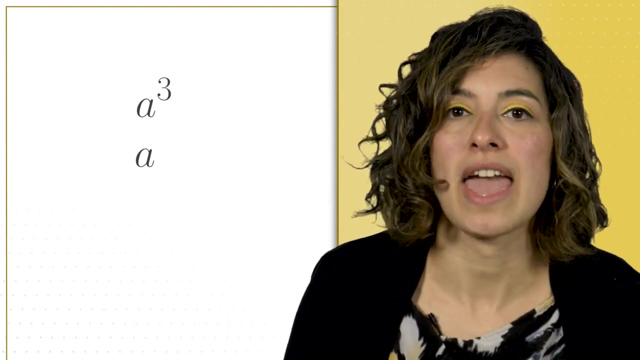 So a to the power of 4 is congruent with 1 mod 10.. That's using the number from the table And that means that a cubed times a is congruent with 1 mod 10.. And therefore a cubed is the inverse of a mod 10.. 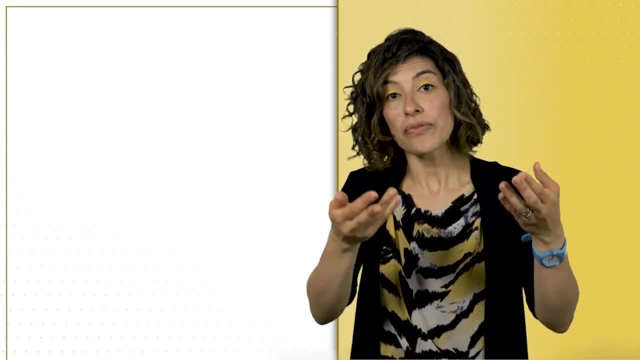 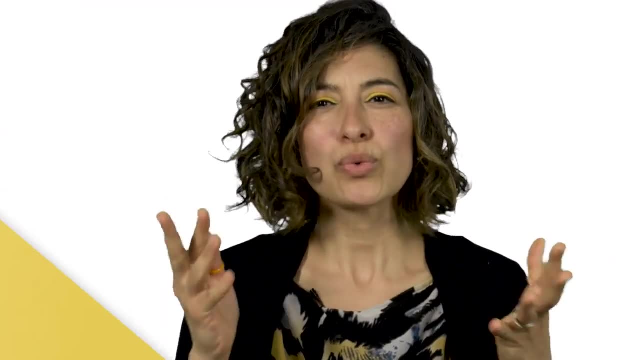 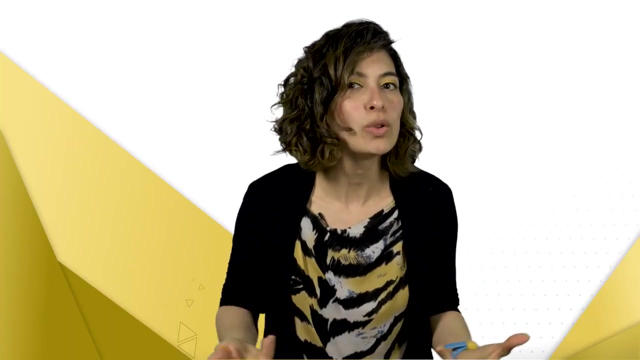 This technique is an extension or Fermat's literal theorem for when the modulus is not a prime number. Now, back to where we were. We're trying to calculate other inverses, mod 10. We can only consider numbers 1,, 3,, 7,, 9,. 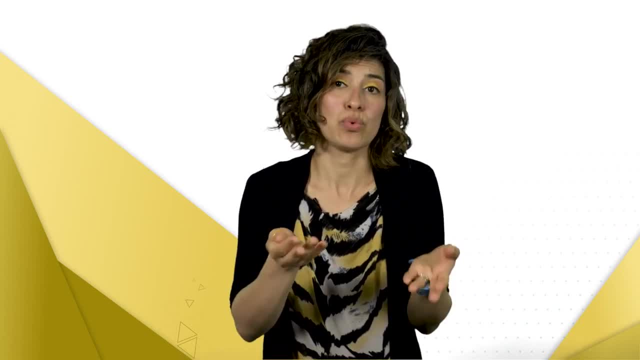 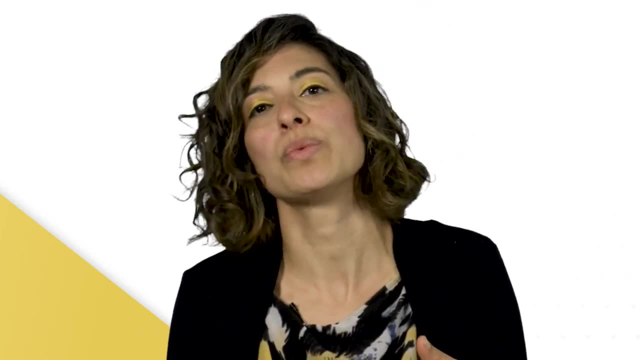 as these are the only co-prime with 10.. 3 and 7 are inverses, we saw earlier- because 3 times 7 is 21,, and that's congruent with 1 mod 10. And so we now got 9 and 1 left. 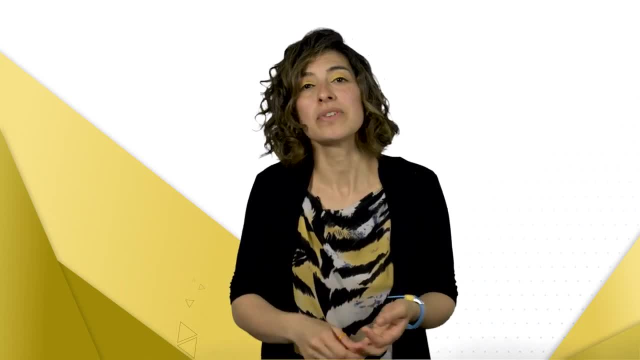 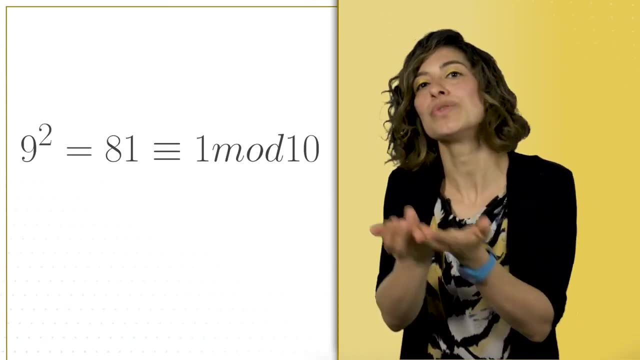 Now, 1 is the inverse of itself. so let's see what happens with 9.. 9 squared is 81.. 81 is congruent with 1 mod 10, so 9 is inverse of itself as well mod 10.. 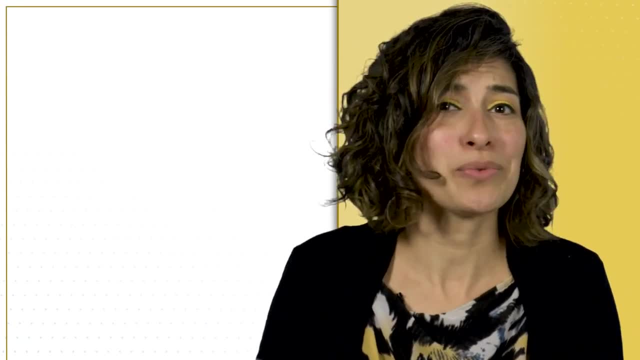 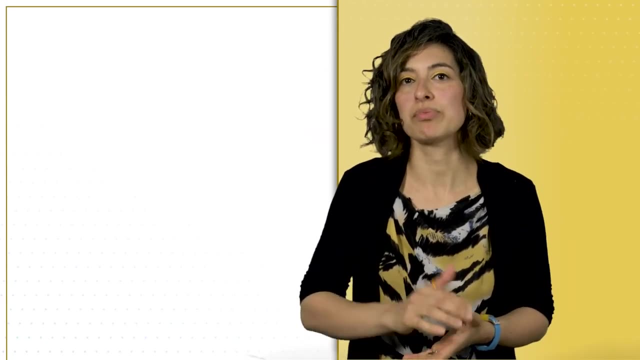 Now those are no good as keys. The only good keys are the ones where you've got two inverses that are not the same. Let's see what happens with p equals 17,. still prime: The keys have to be inverses mod 16,. 1 less than 17.. Now, 16 has many factors. Let's see which numbers up to 16 have no factors in common with 16.. We've got 1,, 3,, 5,, 7,, 9,, 11,, 13 and 15.. 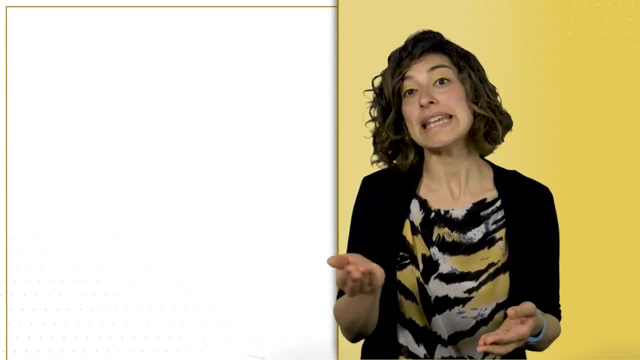 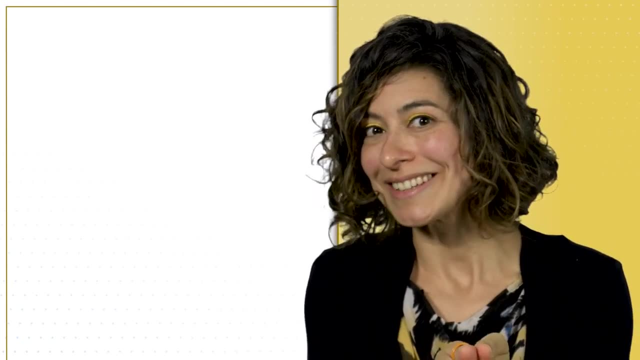 That's altogether 8 numbers. Let's find the inverse of 3 mod 16.. The special power for mod 16 is 8, you can use a table or you count the number of co-primes. So the power to give the inverse 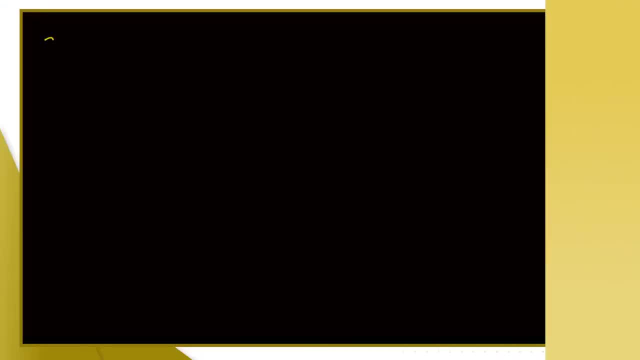 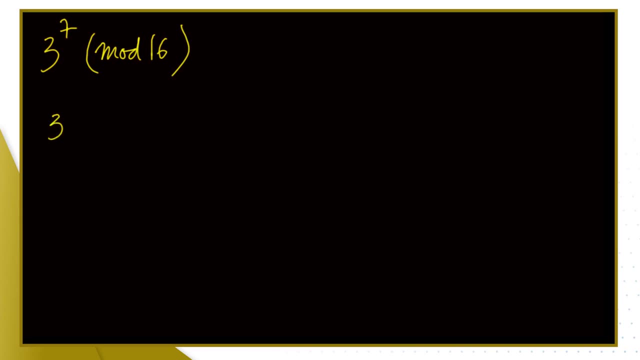 is going to be power 7.. So 3 to the power 7 mod 16, that's what we want to calculate. We do 3 cubed, which is 27,, and 27, take away 16, that's 11.. 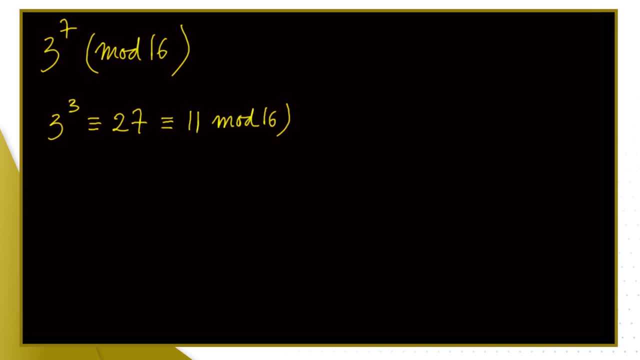 So it's congruent with 11 mod 16.. 3 to the power of 6 is going to be the square of 11. And so we've got 121, which is congruent with 9 mod 16.. Check that out. 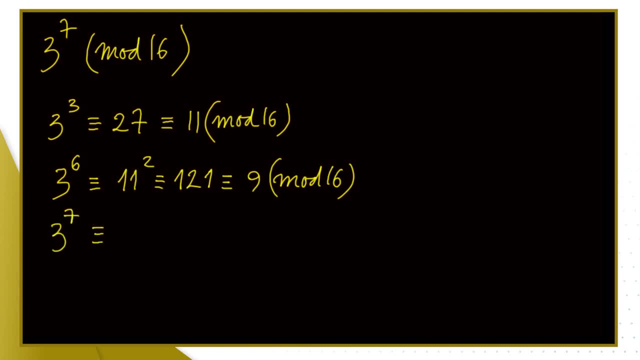 And so 3 to the power, 7 is congruent with that 9 times the 3, the 9, from 3 to the 6, and 3 to one more power, and that is congruent with 11 mod 16.. 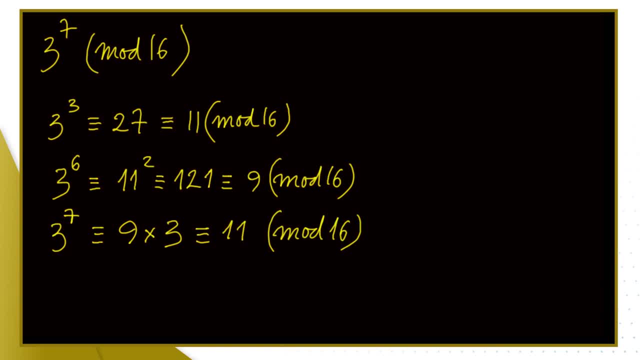 Now that means that because power 7 gives the inverse, we have that 3 to the 7 is the inverse, so 11 is the inverse, So 11 is the inverse of 3. mod 16.. That means that for encryption, 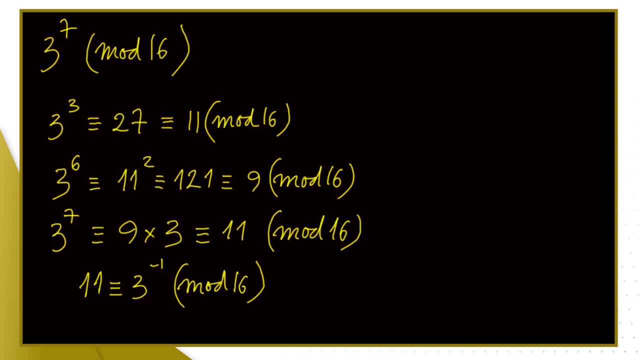 mod 17,. we can use keys 3 and 11, because they are inverses. 3 and 11 are inverses, mod 16, one less than the prime. Now you can compute for the other numbers. So, for example, 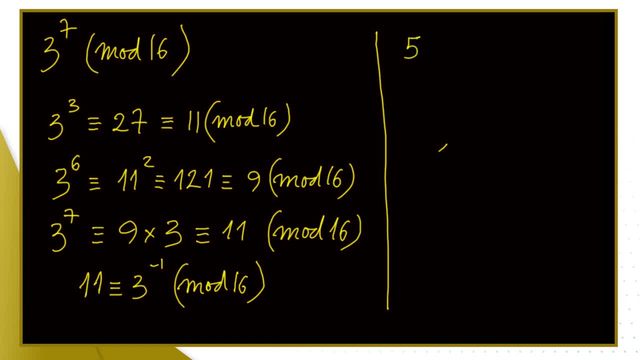 for 5,. what's the inverse of 5?? You do the same. It will be power 7 to find the inverse of mod 16.. That's the inverse of 5.. And working through the powers you do, 5 squared is 9,. 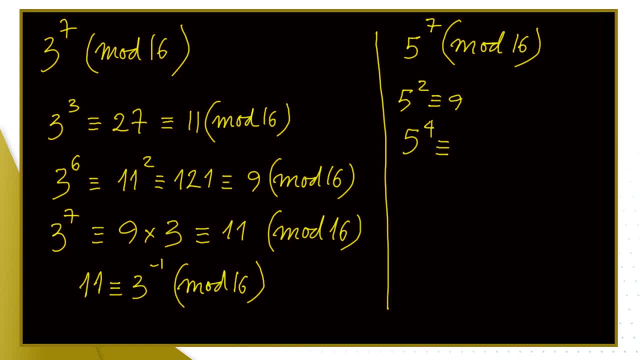 mod 16.. 5 to the power of 4 is 9 squared, which is 1, mod 16.. And that means we actually achieved a power that has the result 1 earlier than the power 7.. And that means if 5 to the 4 is 1,. 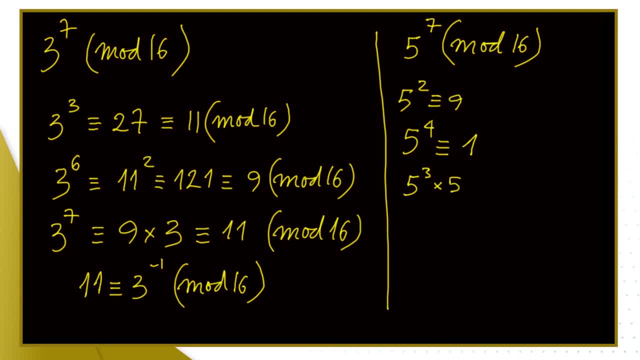 that means that 5 cubed times 5 is 1, and that means that 5 cubed is the inverse of 5.. So let's compute 5 to the 3.. 5 to the 3 is the 5 squared. 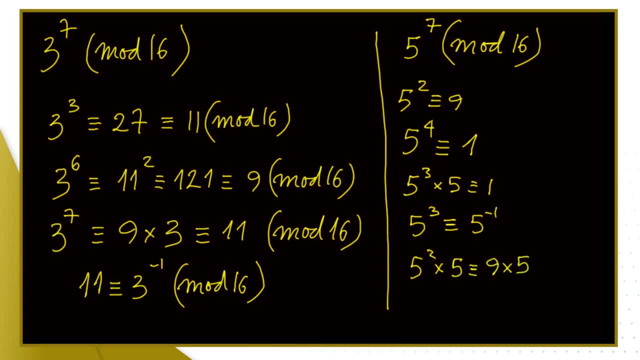 times the 5,, so 9 times 5,, which is 45, and 45 is congruent with 13. mod 16. So 5 and 13 are inverses. We've got 3 and 11,, we've got 5 and 13,. 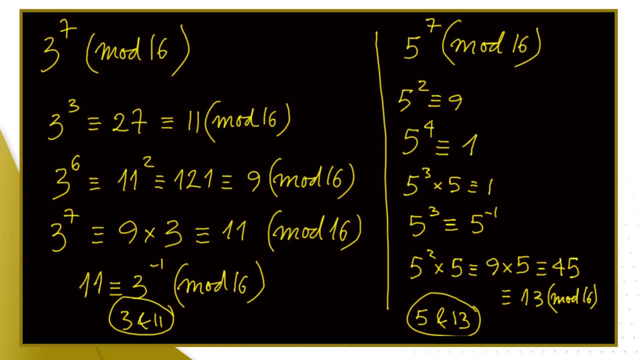 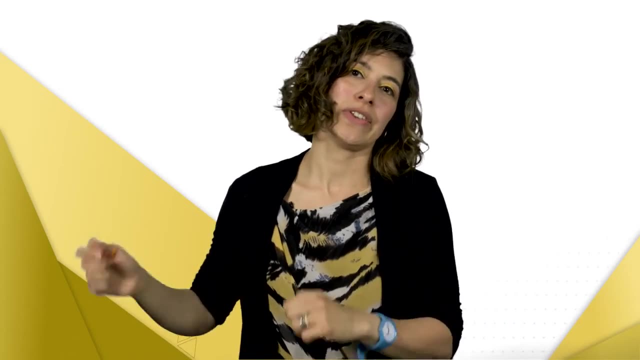 and you can carry on the calculations to find out all the other pairs of inverses in mod 16, so that you have all the other pairs of keys, mod 17.. That's the cool thing about modular arithmetic In real life. RSA encryption. 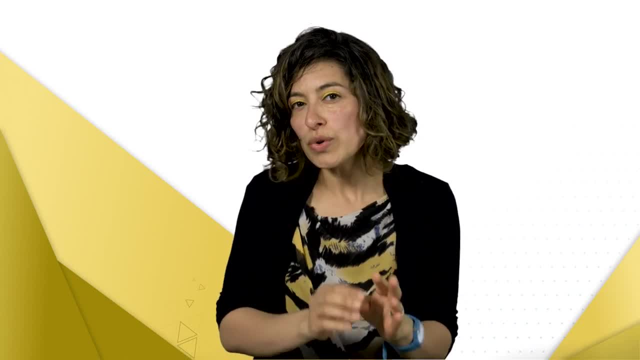 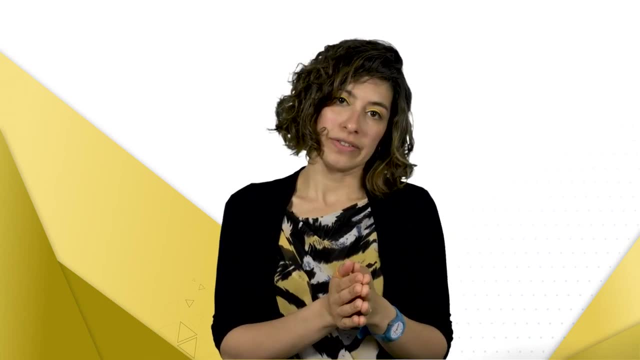 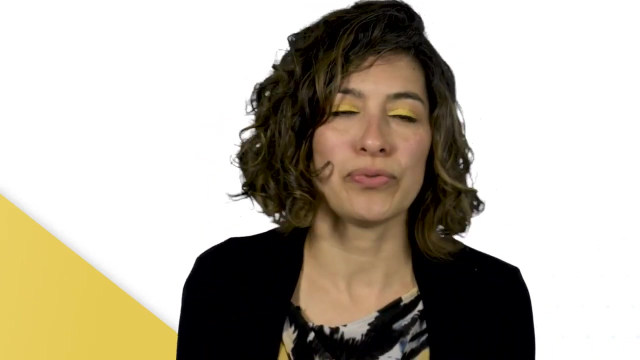 we don't use one prime number, We use a product of two prime numbers, making it difficult to calculate multiplicative inverses. I haven't explained it but take my word for it for now. But in this module I'm not asking you to work on the full RSA. 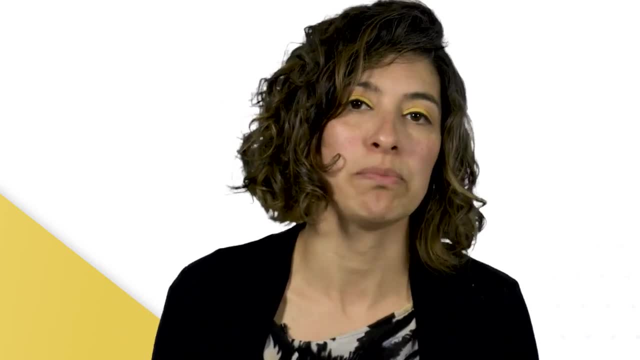 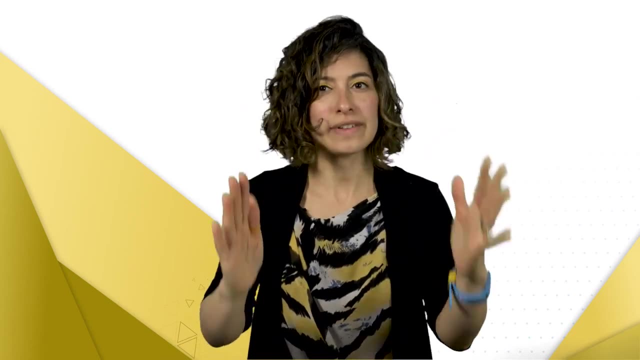 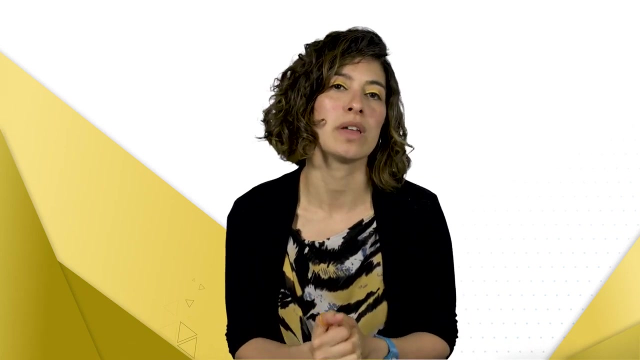 only in the simplified version, using a prime p as modulus and keys e and d that are inverses: mod p minus 1.. So just so we have it clear, we work in mod p for encryption and decryption and we work on mod p minus 1. 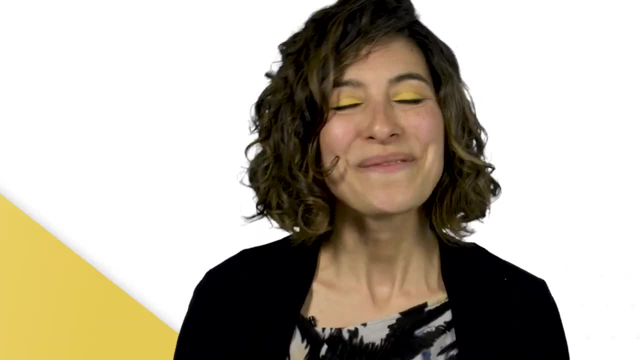 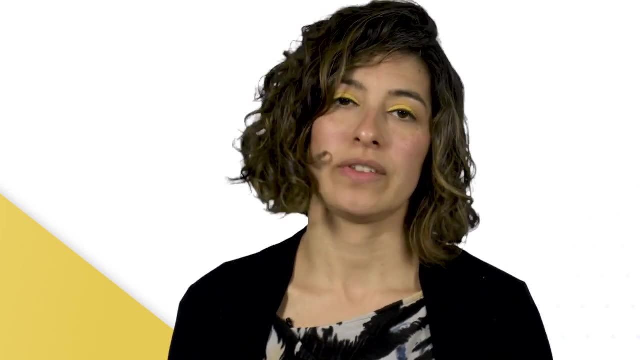 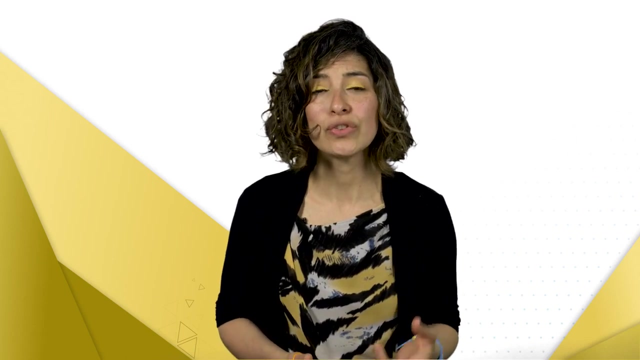 to find keys that are inverses. The next assessment task consists of you implementing by hand the methods I just explained. You are also asked to assess the security of the system by explaining the calculations you would need to perform with the public keys in order to decrypt the message. 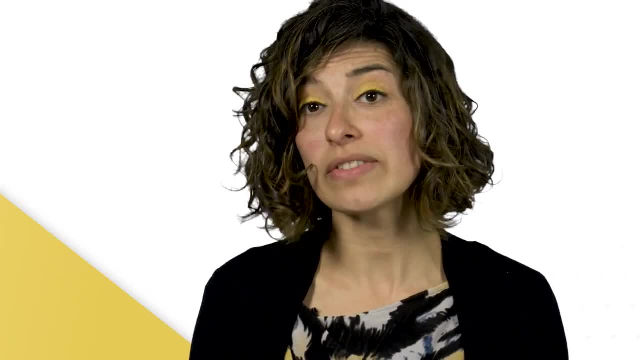 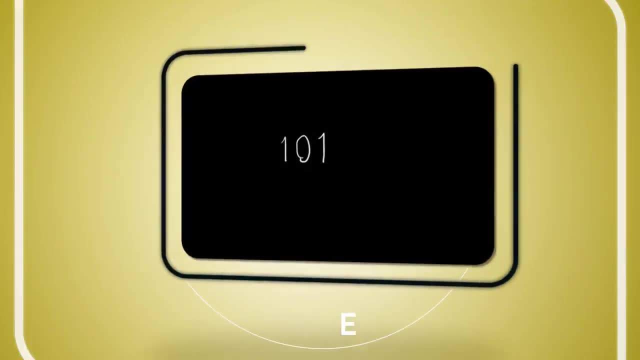 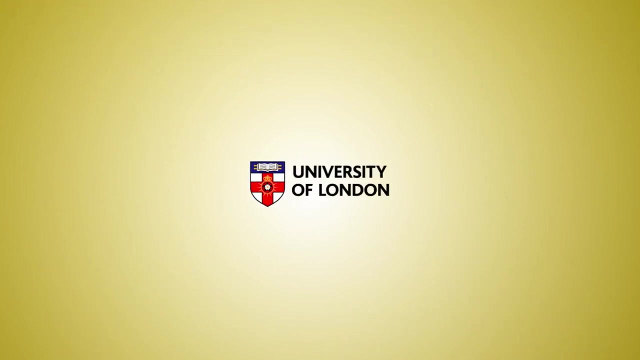 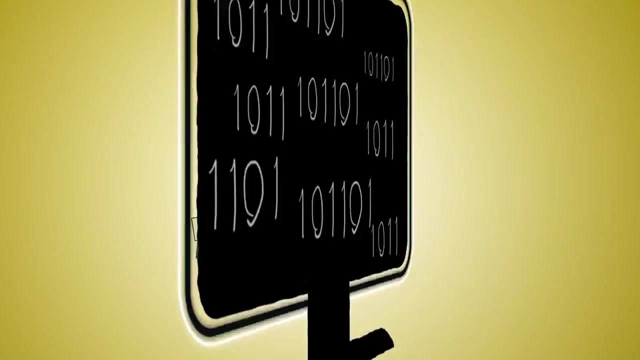 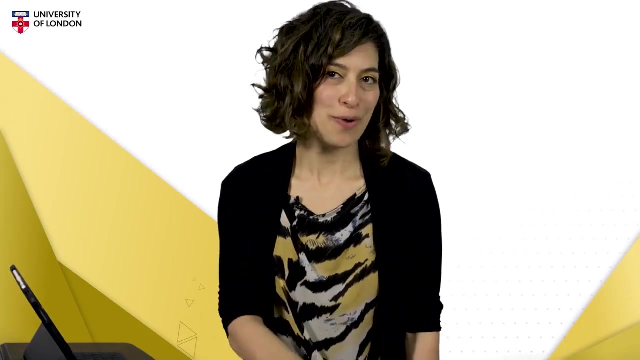 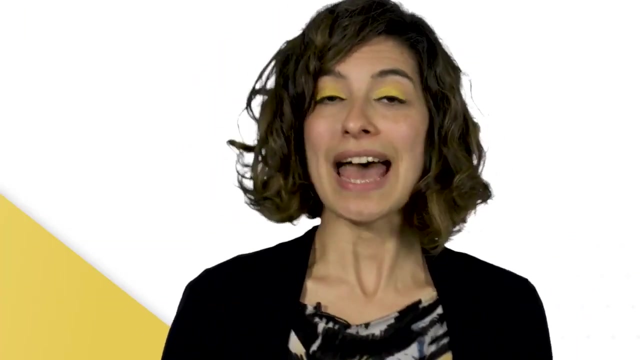 You will start by exchanging ideas in the discussion forum and then you will complete your own task individually. I've got a great job offer for you. You can even choose the salary plan. You can get £100 on the first day and each day you work. 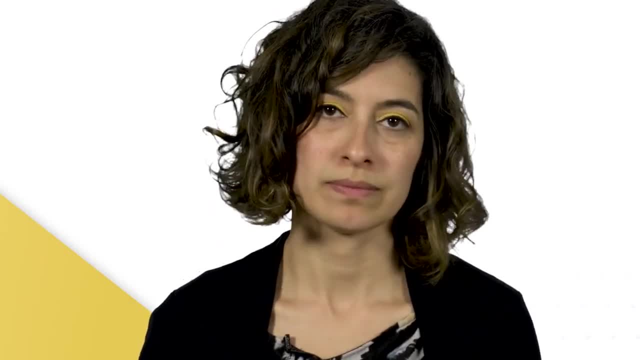 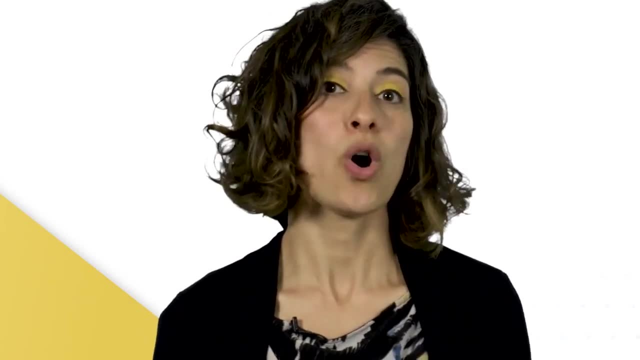 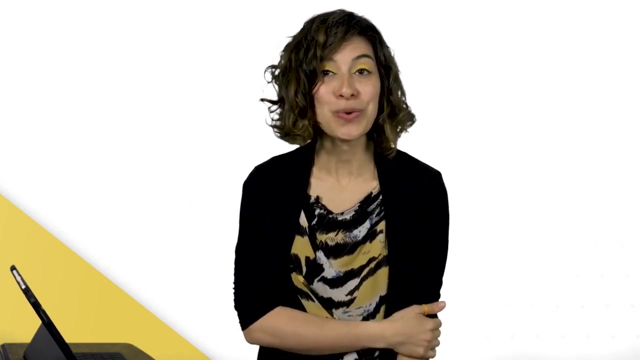 you get £50 more than the day before, Or a different plan. I double your salary every day, but you start on £1 on day one. The question is: how long do you want to work for us And what payment plan do you want? 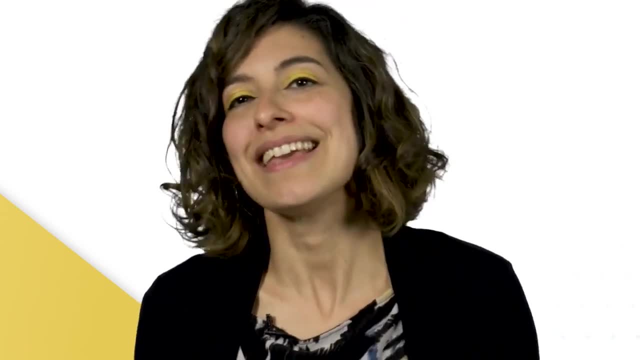 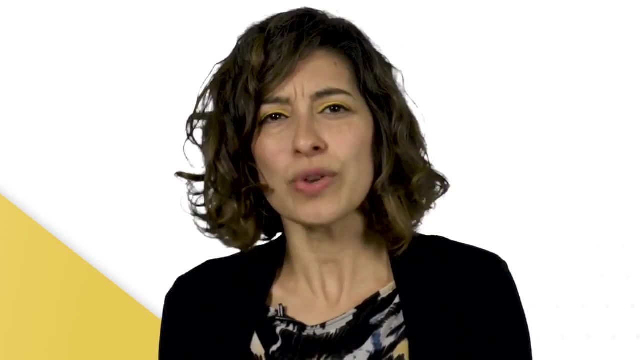 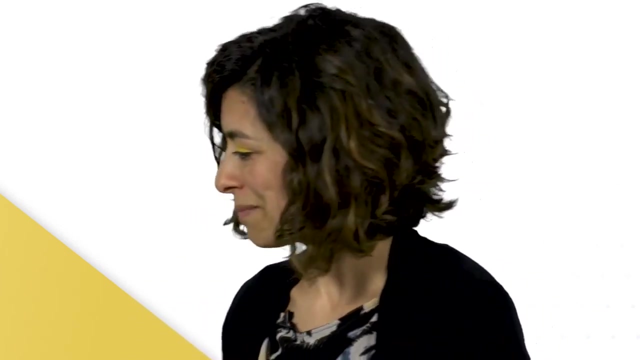 Is that too good to be true? OK, it's just a story, I know, but we can still look at the figures. Have you made a decision? How do we actually decide? You could get your spreadsheet out and try it. I'll get mine. 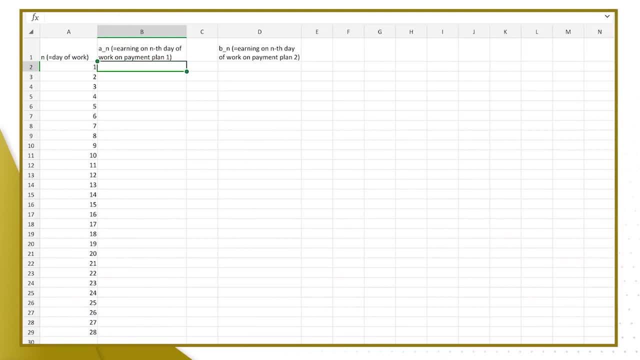 Let's put in all the data from these payment plans. So I've got a column here for the days of work and the first payment plan and the second payment plan. So the first payment plan: we start with £100 on day one. 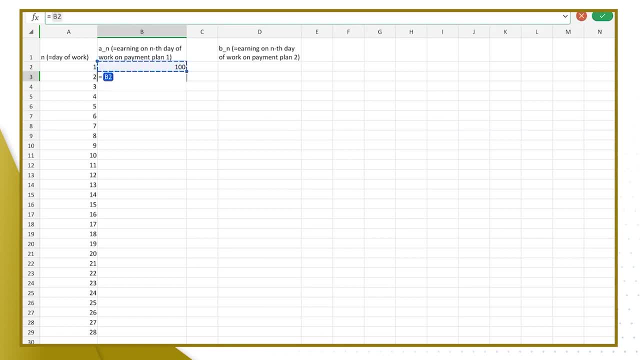 and on the second day is the payment we had on the previous day, with extra £50 on top. So that means we get £150 on day two, £200 on day three, £250 on day four and so on. So we get all of that. 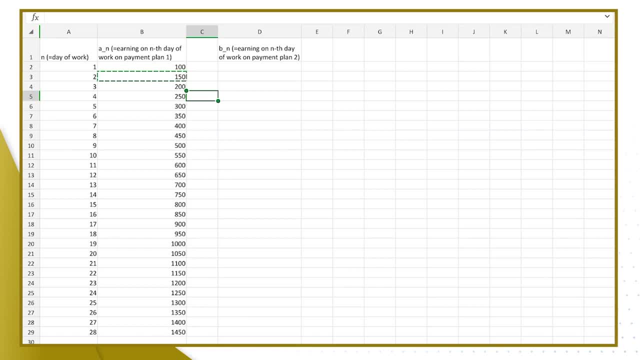 Let's see how many days we need, but we'll put 28 for now. Now on the second option: you start on £1.. So we start on £1, and on the second day we go with doubling what we earned on the previous day. 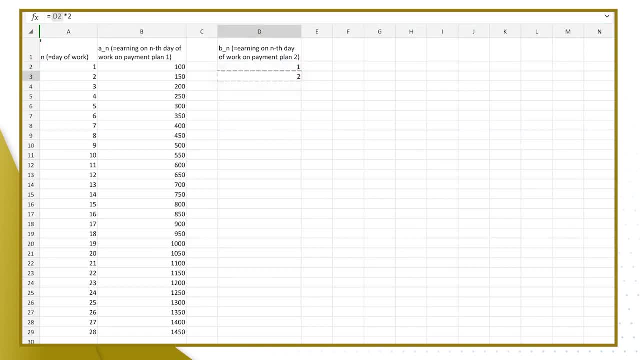 And we carry on in that fashion. so we're going to double. Now is that a good table to help us make a decision? Let's see We're earning a really low amount. on the second payment plan We go £1,, £2,, £4.. 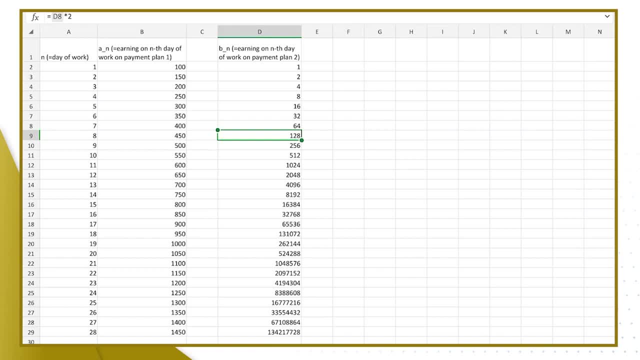 Day eight: we earn £128.. Not bad. And it keeps doubling, so we're just making really serious money. on day ten, And it looks like we're catching up with the £550 we get on the first payment plan Now. so how many days should I work? 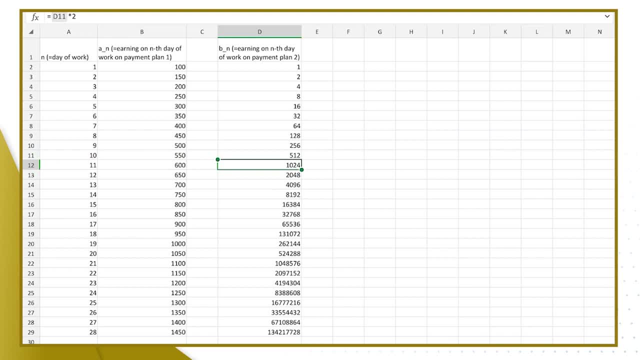 On day 11, I'm already earning more on the second plan than on the first. Is that how I should make my decision? Yeah, I can hear you screaming there. It's not enough just to compare that. We need to say: 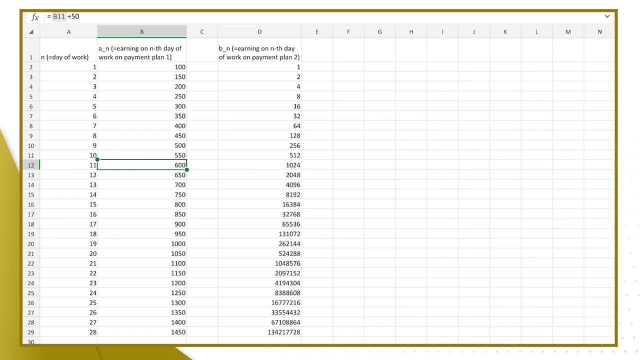 how much money do you make in total? We will need to tally up all of this. So let's do that. We have that value, and then the new one. Let's add up- And we're just adding up the money you've earned. 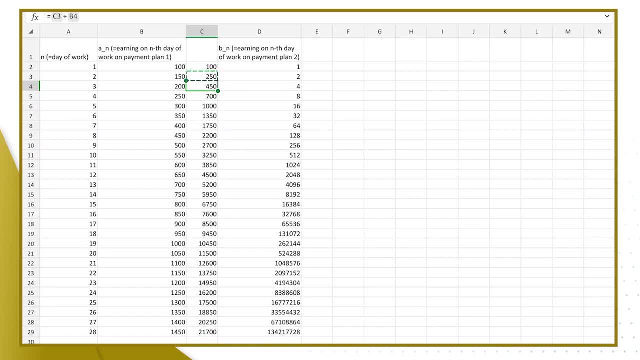 up to that day, All the payments you received up to that day. So there we are. And then let's do the same on this one And let's copy that formula: OK, big numbers. There we are. We're having the accumulation of salaries. 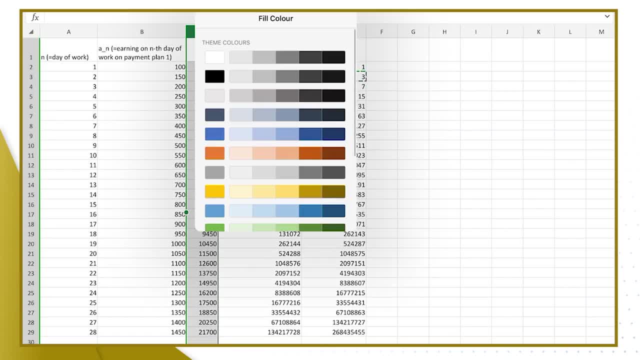 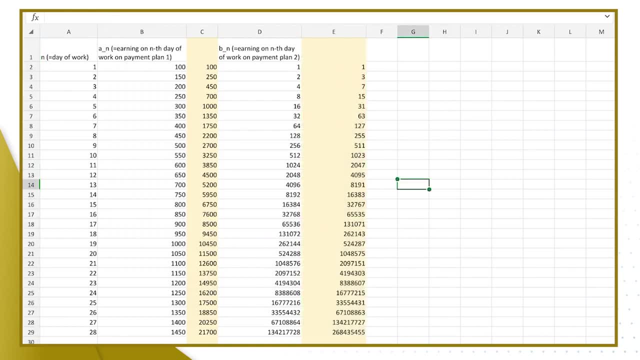 Let's highlight this column here. So we're actually comparing the sums of these And looking at that in detail. the first day the income of plan B overtakes plan A is when you earn 8,191 against 5,200 in total. 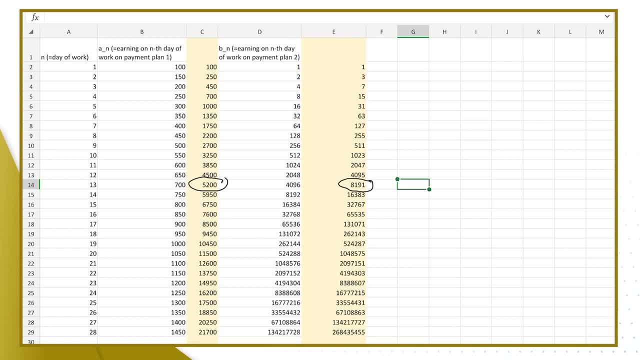 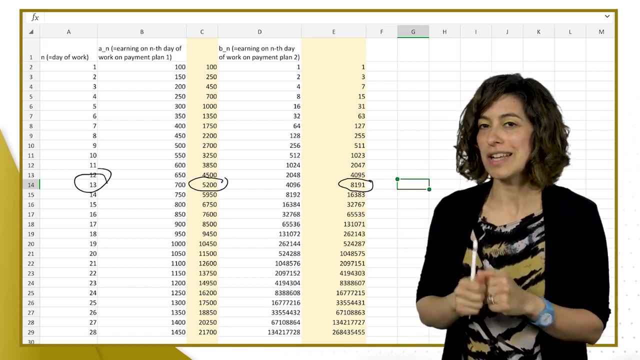 So the day before we're still making more money on the first payment plan, but we are ahead from the 13th day onwards. Why am I talking about that? We are going to pay attention to sequences of earnings and sums of earnings. 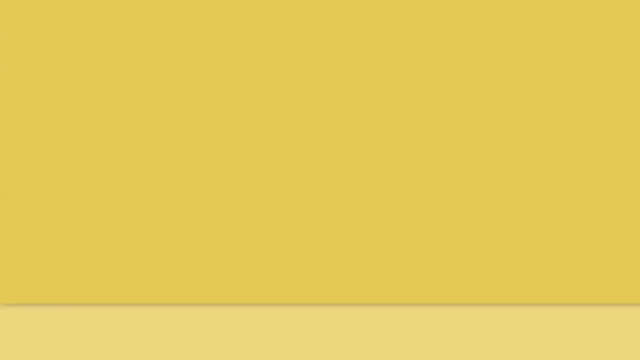 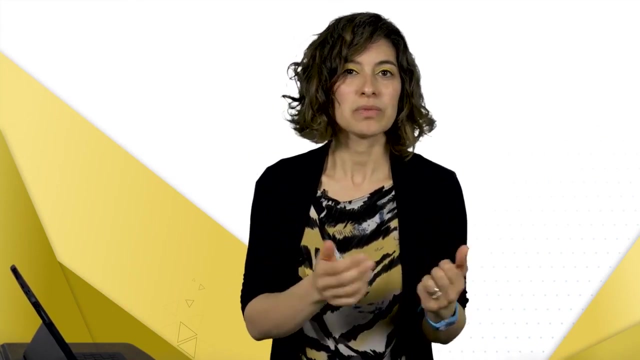 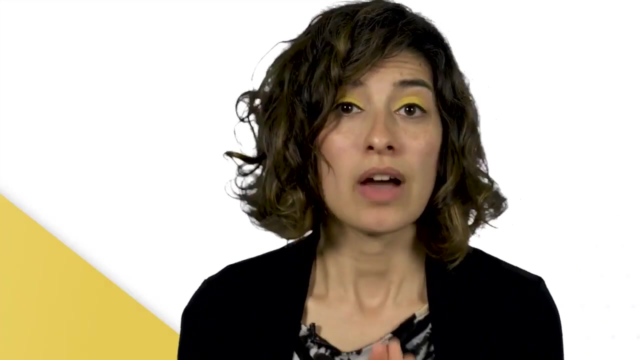 But let's look at another example. I've got another story for you. The inventor of the game of chess- this was before the 7th century in India- presented the game to the emperor. Now, having enjoyed the new game, the emperor praised the inventor. 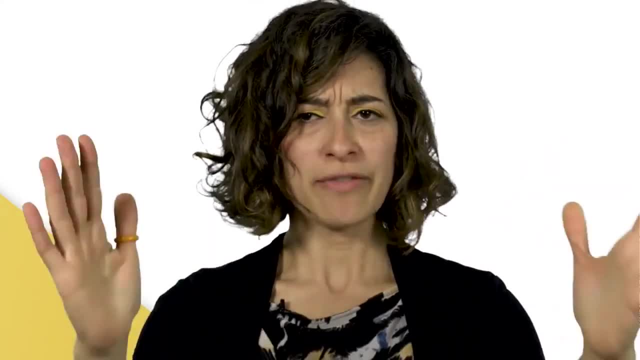 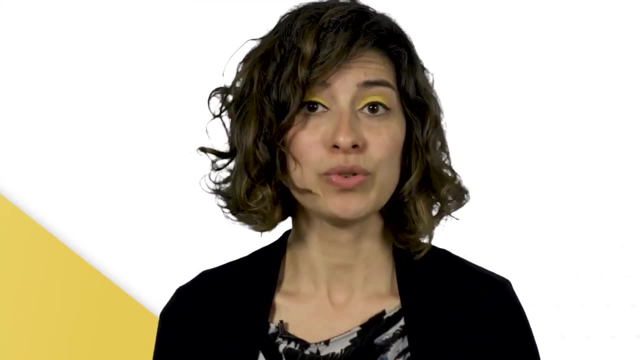 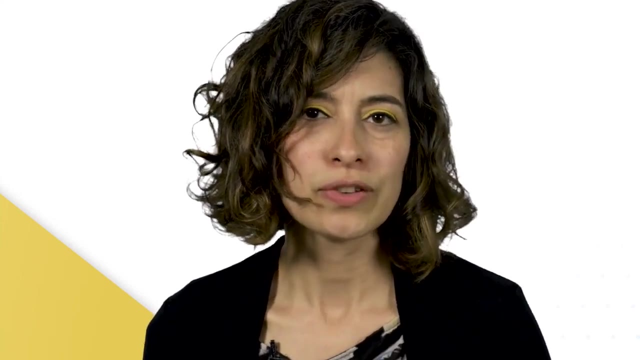 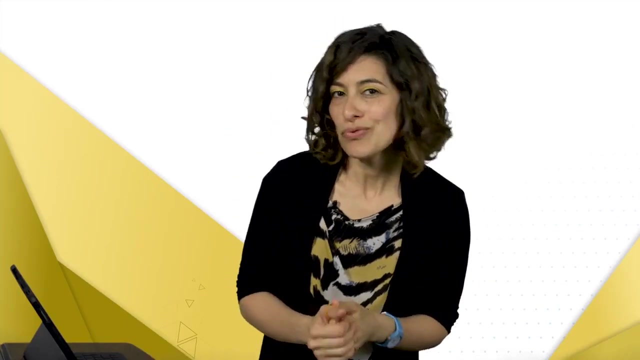 and offered a generous reward, Whatever you want. She asked for one grain of rice for the first square of the board, two for the second square, four grains of rice for the third square, eight for the next, and so on. The emperor approved the payment. 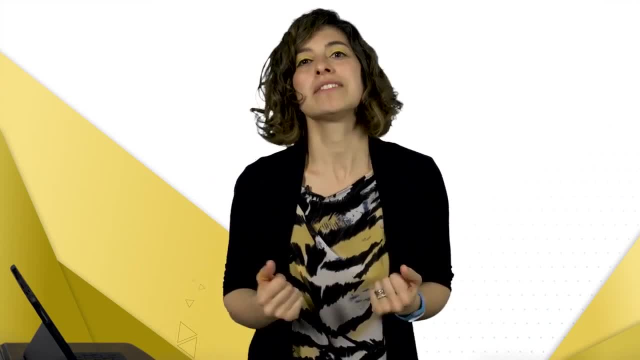 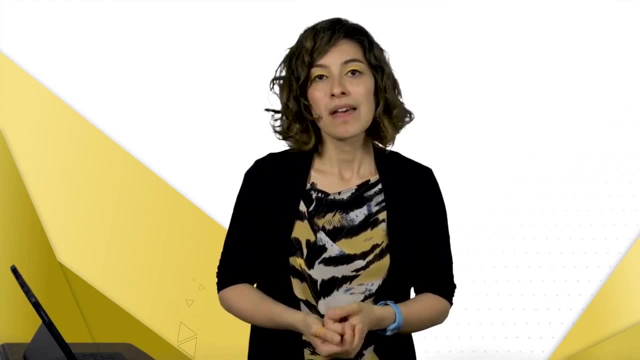 probably dismissing it as a humble request from this inventor and not giving it much more thought. Well, in the end it's just a few grains of rice for an emperor. The treasurer in charge of the transaction later returned to the emperor, informing them the reward. 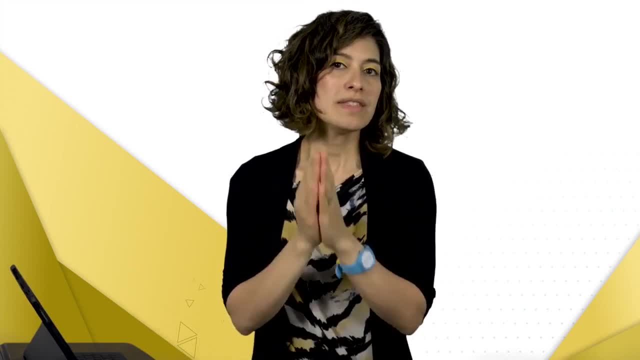 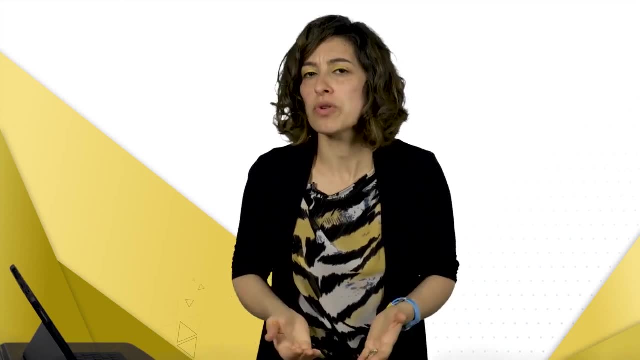 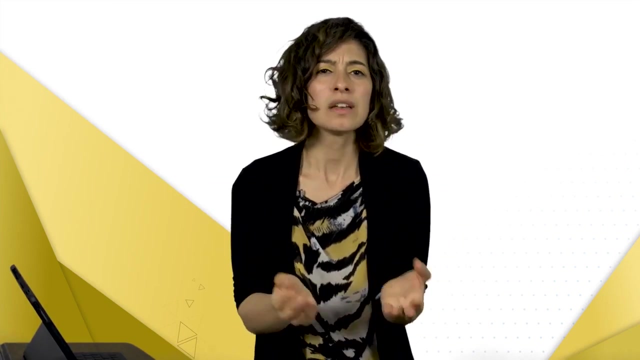 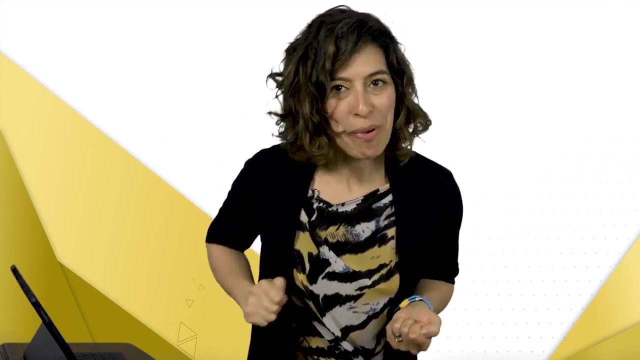 would add up to more rice than they could ever ever have grown. What is going on? You know the chessboard: It's an eight by eight, so we have 64 squares, Surely, adding one plus two plus four plus eight, all the way to two, to the power 63. 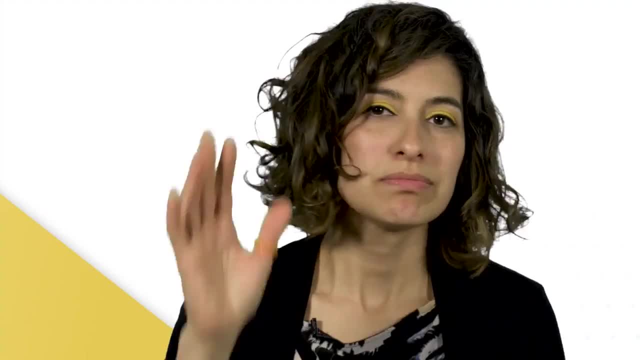 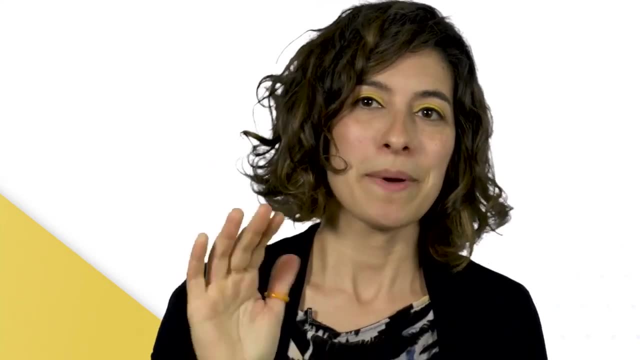 grains of rice. that can't be that much, can it? Now, if you want, you can go and find out how much do we produce in the world in rice in terms of grains. but I leave you to that, and I have another problem for you. 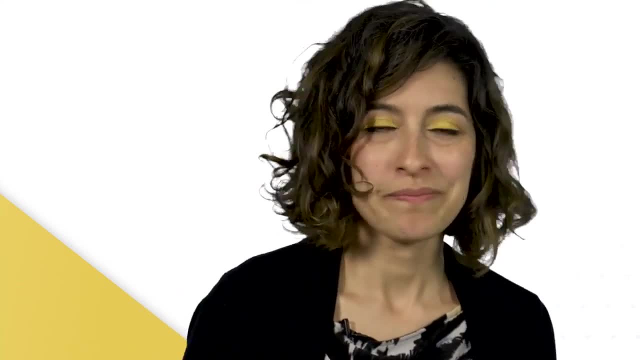 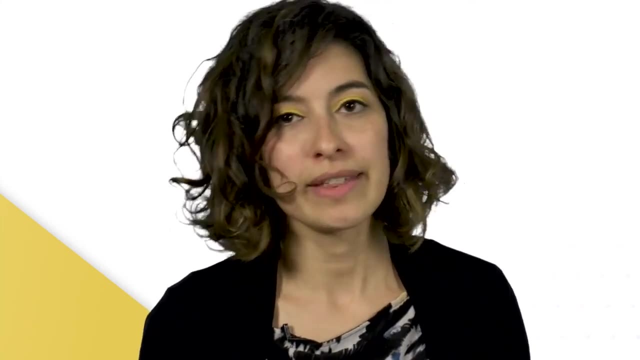 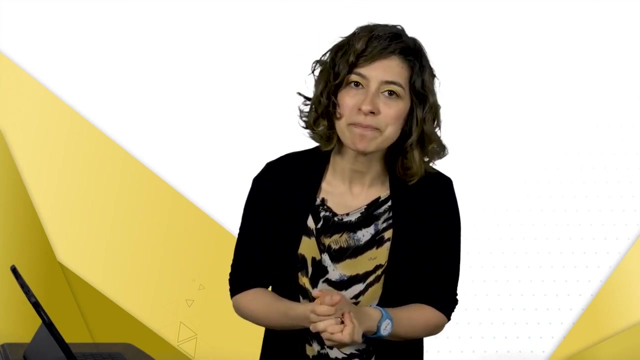 the travelling maths presenter problem. I'm taking bookings for touring with my new show and here is my schedule for the next summer, together with the travel costs. So initially I'm going to London, Manchester and Edinburgh and I need to travel. 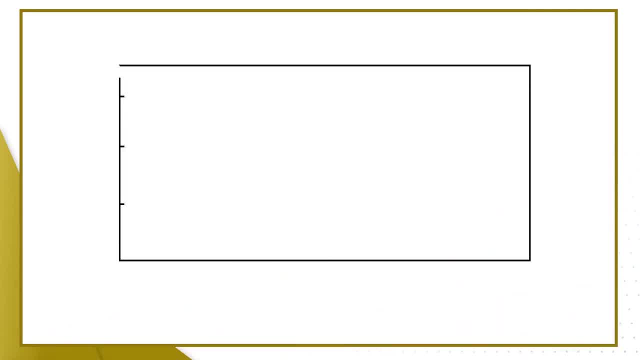 between all these cities and, yeah, London to Manchester. I'm seeing that there's a £100 fare London to Edinburgh, £150 fare Manchester to London. yes, trains in Britain It's a little bit more expensive, It's £120,. 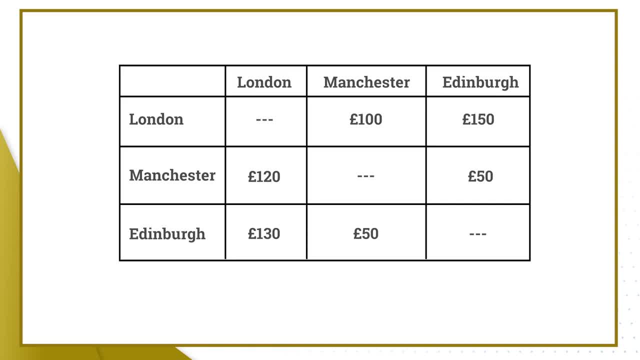 and Manchester to Edinburgh, a bargain £50.. Edinburgh to London: £130.. Edinburgh to Manchester: £50.. So this is what I'm expecting. I'm expecting to spend so far. now I have to visit all these cities and come back to the starting point. 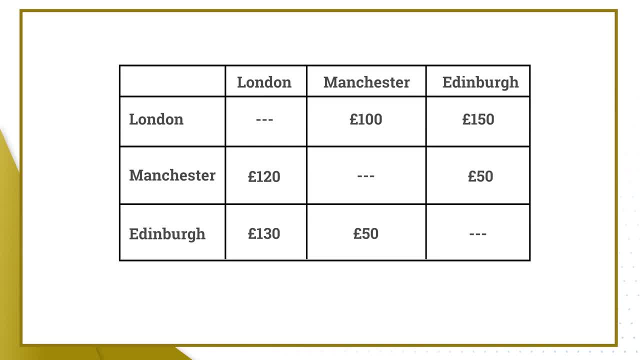 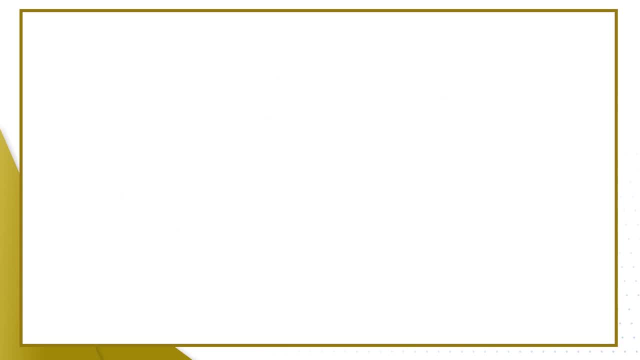 Of course, in the cheapest way possible. but no cities are to be repeated. apart from the start and end, I do want to end up at home. We can attack the problem by trying out all the possible trips. in my tour I could do London to Manchester. 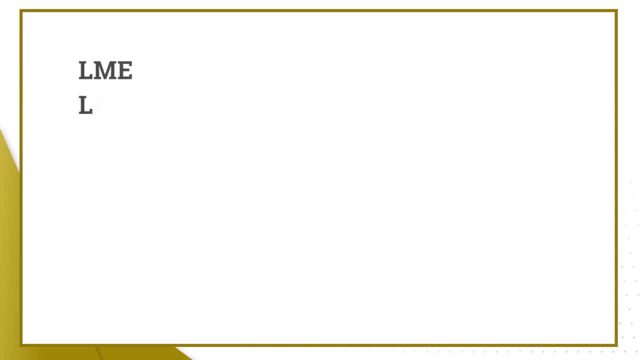 to Edinburgh, of course, back to London, London, Edinburgh, Manchester, back to London, Manchester, London, Edinburgh, and so on. These six trips to check, and surely we can add up the totals and calculate the cheapest trip, Doesn't sound difficult. 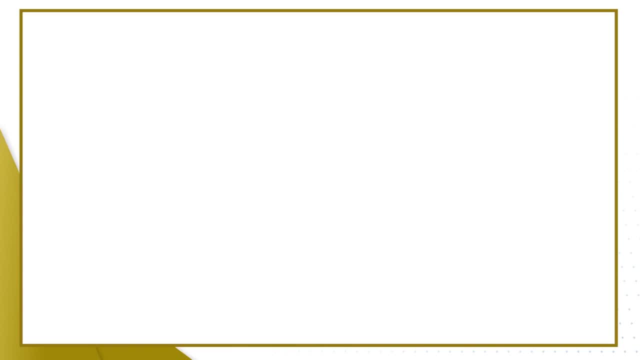 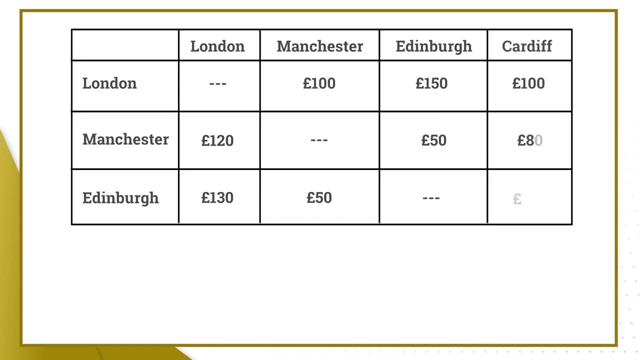 Oh, but it turns out I just got another booking coming in. I'm going to Cardiff, and here's my updated table with my costs. Now, with this extra city, the trips I'm to make, I'm to travel, I could do Cardiff, London, Manchester. 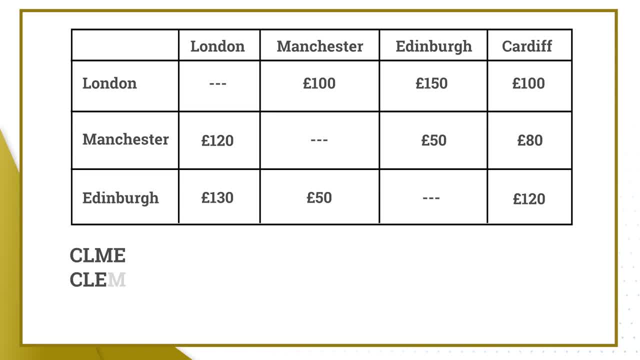 Edinburgh back to Cardiff, Cardiff, London, Edinburgh, Manchester back to Cardiff, and so on. So I could just put a Cardiff at the beginning of all the trips I've studied before. That gives me six of them, But I could go to Cardiff second. 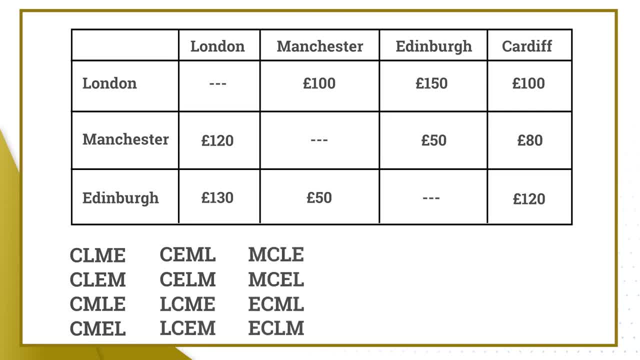 couldn't I- And here's the list- Or I could go to Cardiff in the third place, Or in the fourth place, and so on. How many trips do I have now with this extra city? It turns out there's 24.. 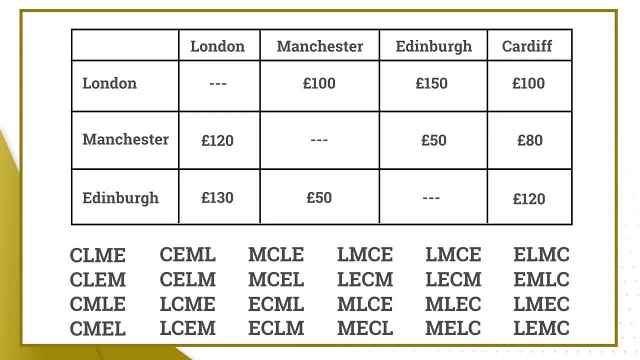 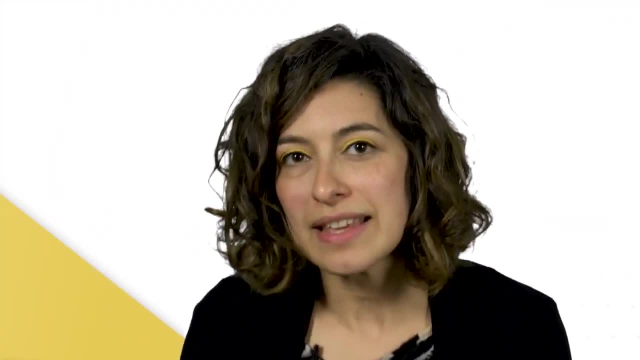 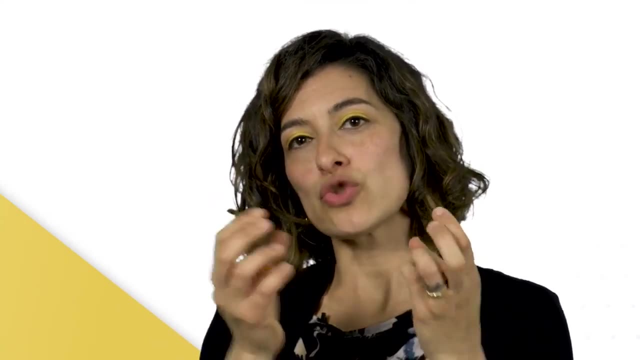 So, with three cities, six trips that I can consider. With four cities we now have 24 trips. How many trips for N cities? I'm expecting a big tour. The trips to consider with one more city is the same as the trips I had with. 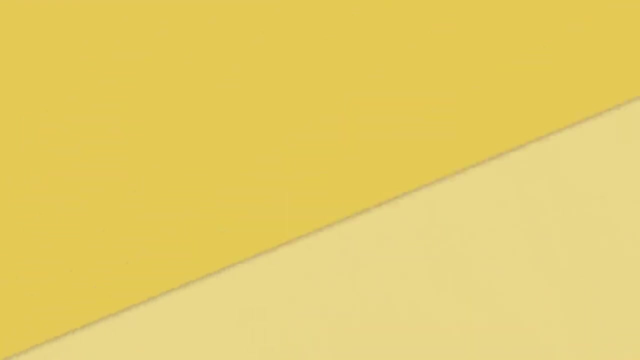 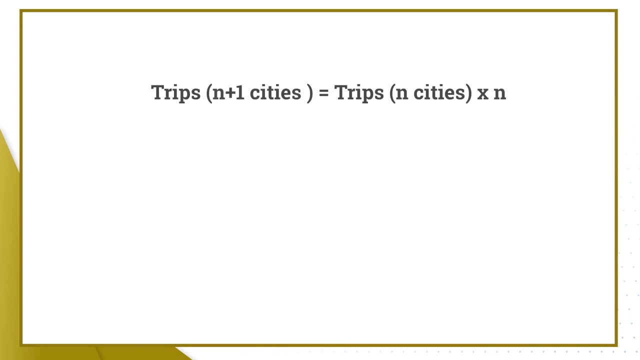 my old number of cities times the new number, So trips of N plus one cities is the same as N times the trips with N cities, So trips on three cities six. Trips on four cities is four times trips of three, which is four times six. 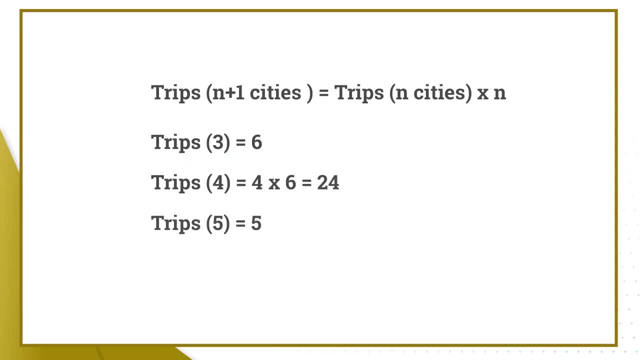 24.. Trips with five cities is five times the trips of four, which we've just done. It's five times 24, which is 120.. So I can expand this as the trips for N cities, as N times N minus one. 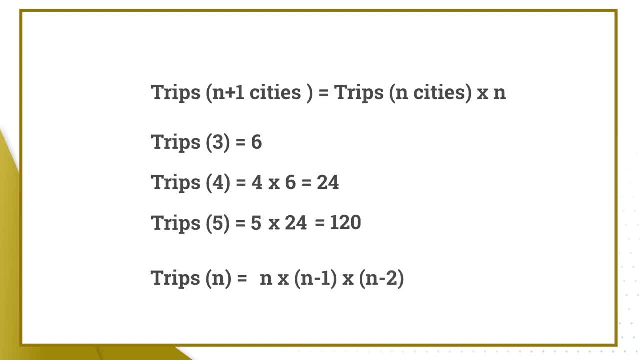 times N minus two times a smaller or smaller number, times three times two. We could analyze the costs of all these trips, couldn't we? But how long does it take to do that job, to cost and analyze all these possibilities as the number of cities increases? 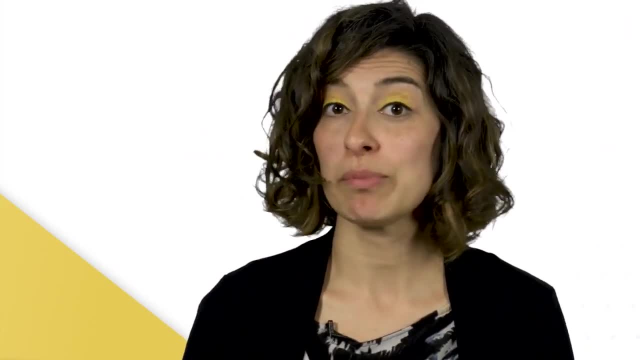 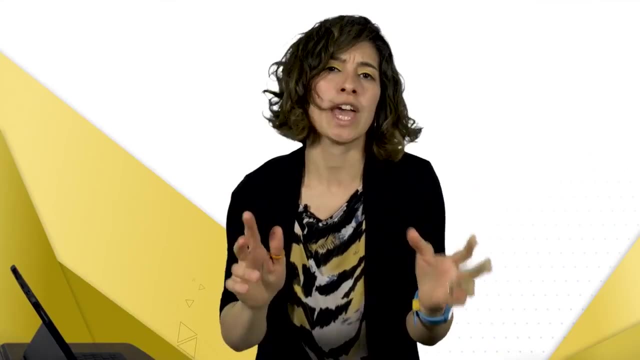 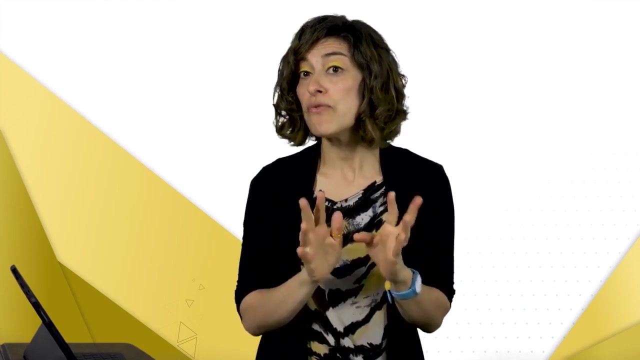 Yep. As I get more and more bookings, this approach to finding the cheapest tour becomes unmanageable. I hear you cry. Surely we can use computers. The number of options to look at grows very fast as we increase the number of cities to visit. 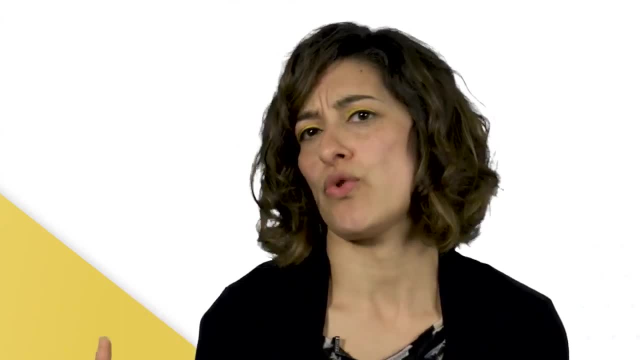 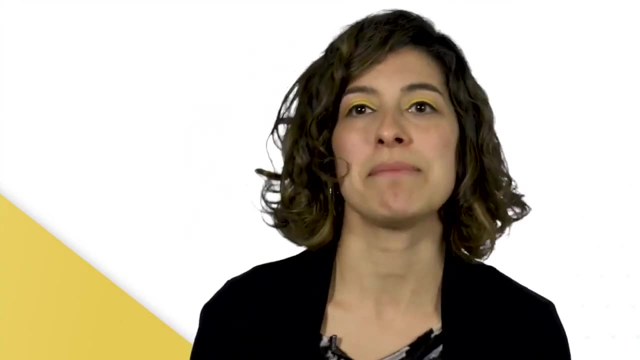 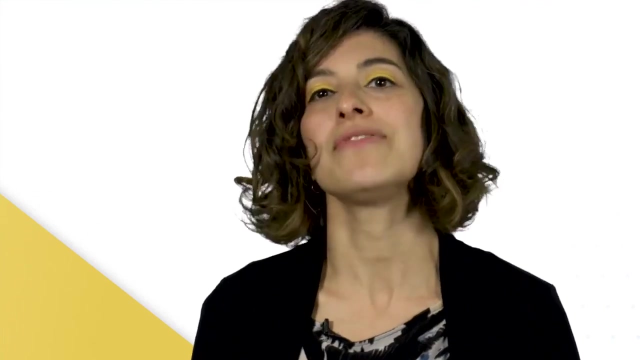 So fast that this brute force approach of checking every option is not okay, Not even with computers. And in the case of the traveling maths presenter problem, also known in the literature as the traveling salesperson problem, there is no known algorithm to give the optimal solution. Yep. This is why in a computing degree, you study problem solving, maths, algorithms, complexity and get to learn why some algorithms just do not accomplish the task within our lifetime, Not even with all computers in the world linked up working on the same task. 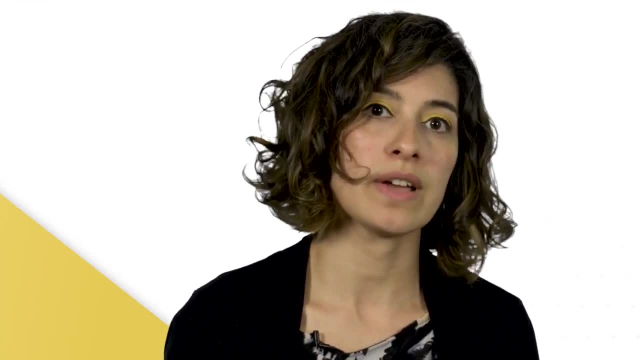 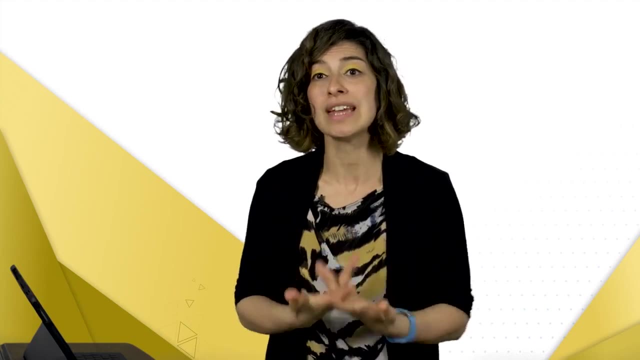 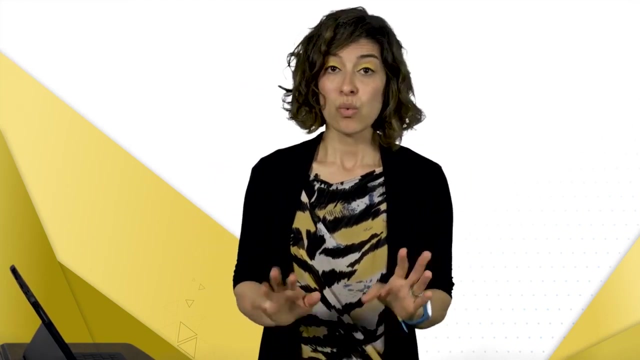 We touched on this before when we talked about factorizing large numbers and deciding of a number being prime. In this topic we will be looking at some tools for understanding sequences of numbers like the ones we saw earlier. their growth and summation We will not cover. 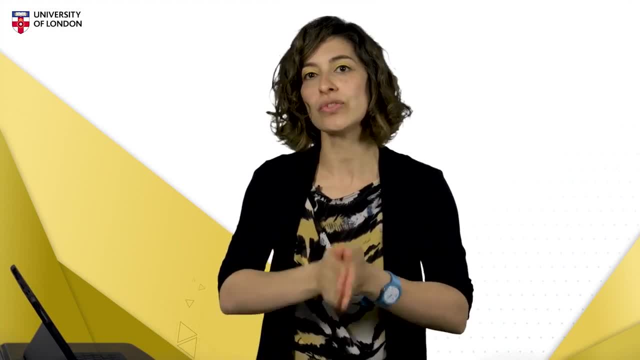 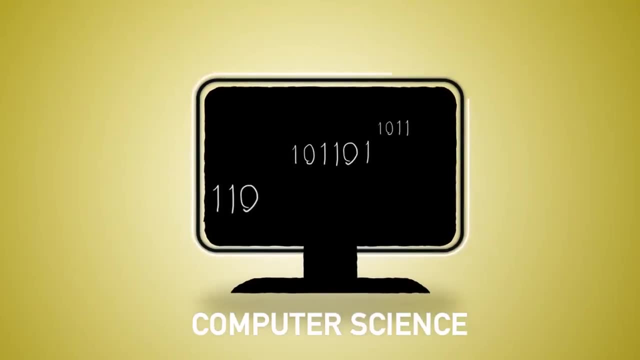 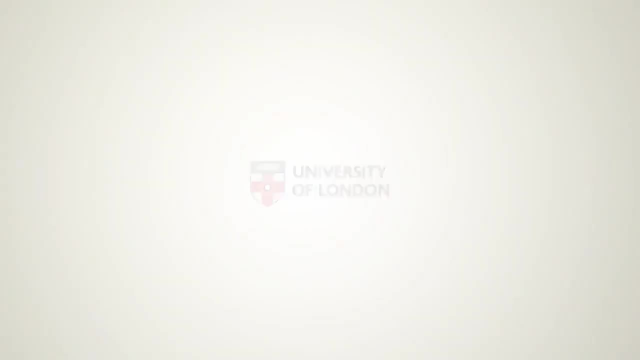 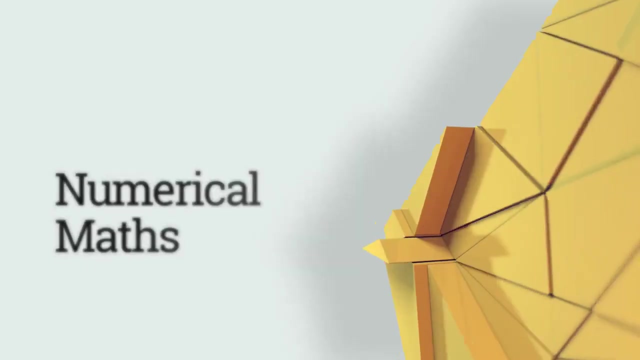 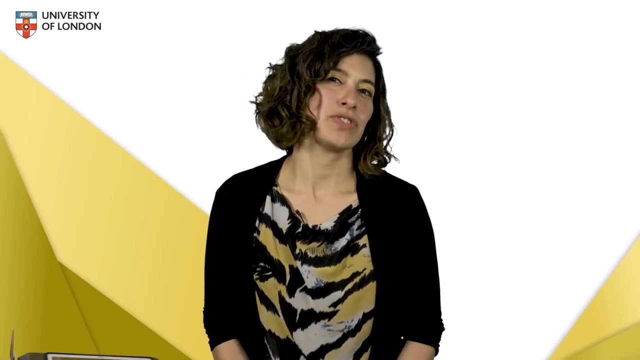 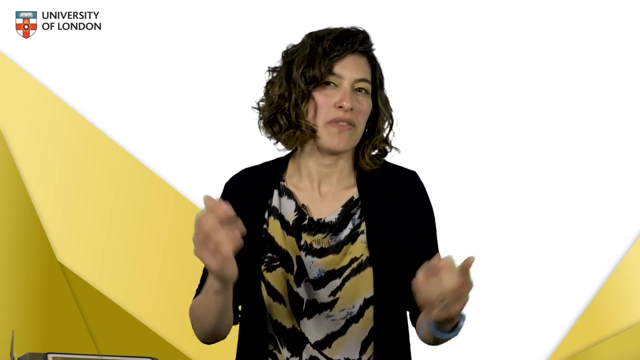 all possibilities, but we will introduce key tools that will allow you to make sense of the behavior of sequences. What makes a sequence more than a bunch of numbers Is the order the numbers feature. Think of it as a cloakroom of a bowling club. 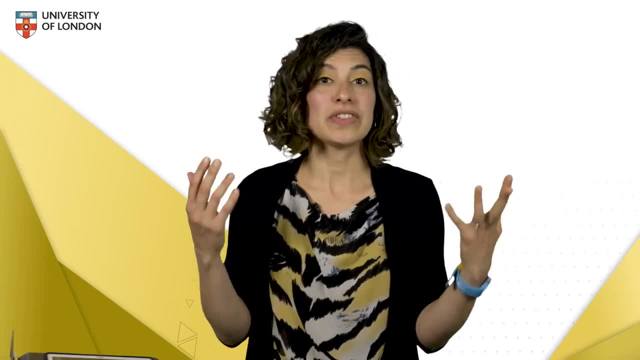 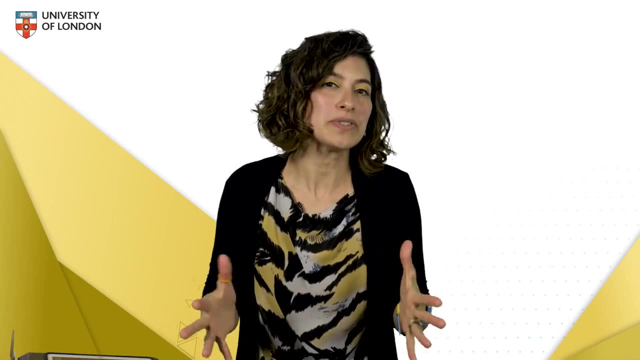 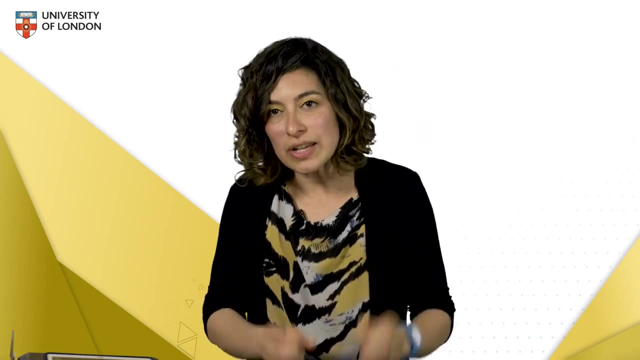 school play theater nightclub. There is a ticket with a number for each item. Well, the analogy breaks down as the items are all different, but two people could have the same coat or bag. The point is, the items in a sequence are labeled. 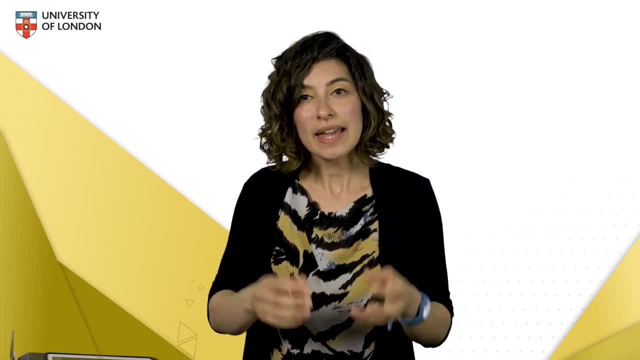 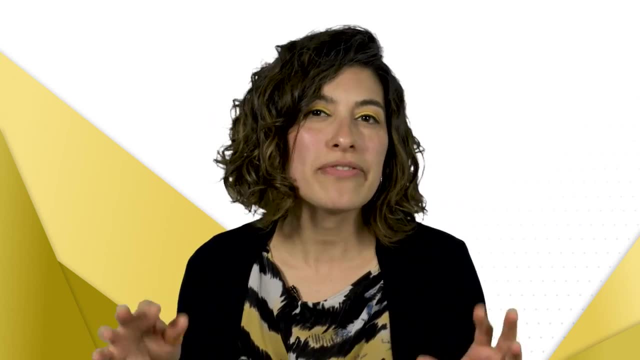 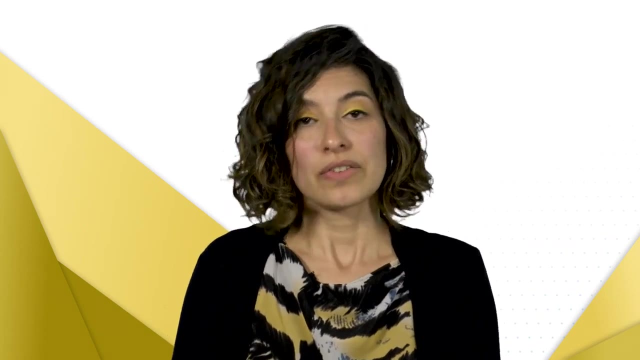 and so there is an order. In a different day we have a different sequence of things. When we deal with sequences of numbers we care about the variation of numbers as the labels, ticket numbers increase. So a sequence is an ordered list of numbers. 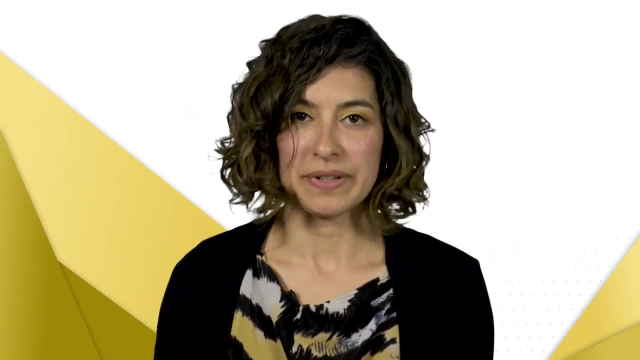 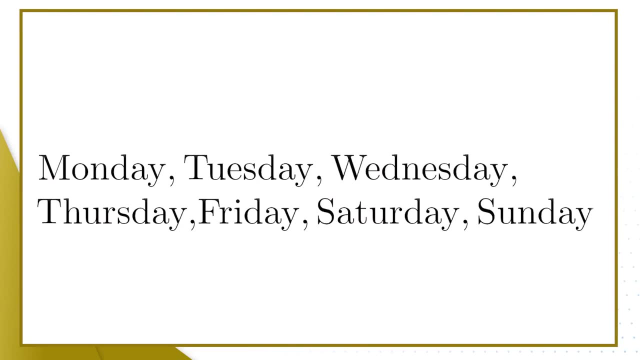 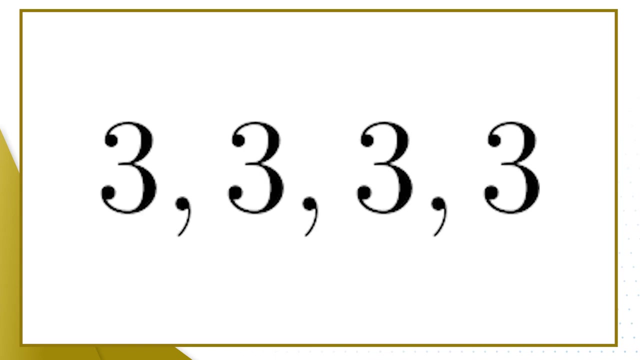 Here are some examples of sequences: Monday, Tuesday, Wednesday, Thursday, Friday, Saturday, Sunday, Ending there: One minus one, one minus one, one minus one, and so on. So three, three, three, three, three and carry on. 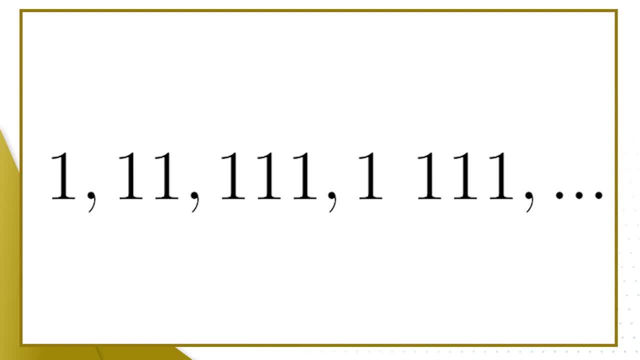 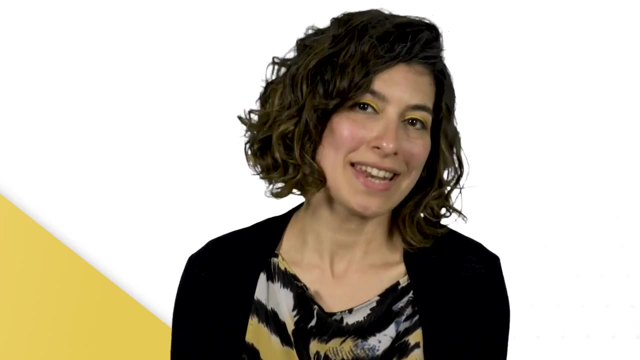 like that: One, eleven, a hundred and eleven, a thousand, a hundred and eleven and so on, Or five, four, three, two, one, zero, Ending there, As a computer scientist, one of the basic uses of sequences. 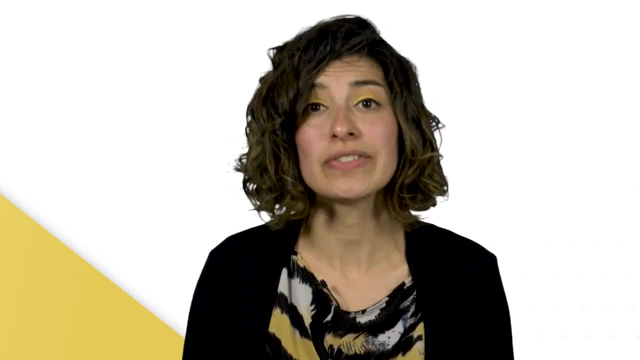 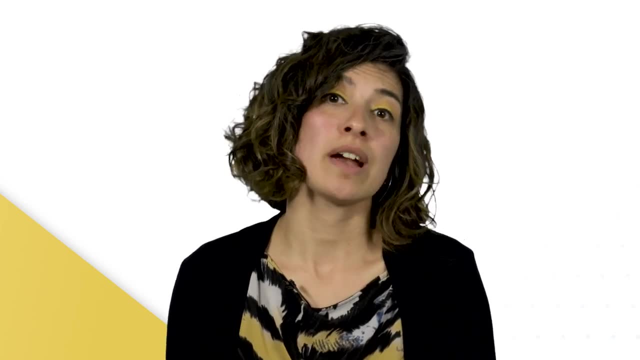 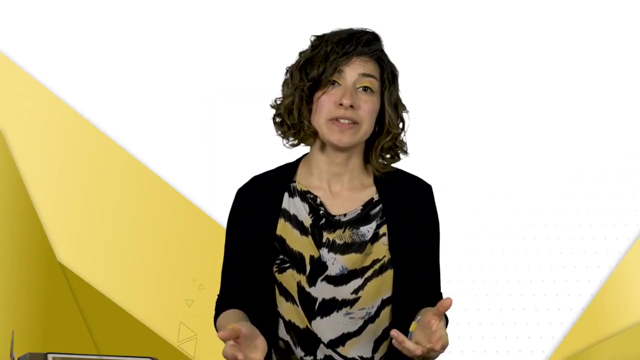 will be tapping into their patterns in order to be able to use them computationally, As I mentioned in the introduction. there are many other applications, but for this video let's be pattern hunters. So take a moment to go through the sequences presented, Make some notes. 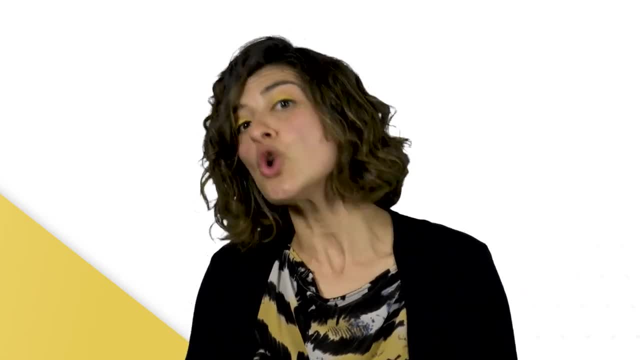 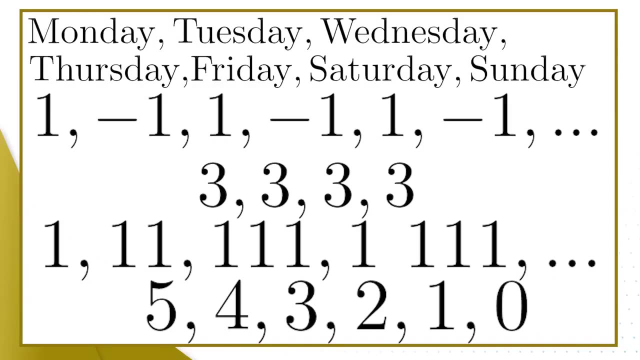 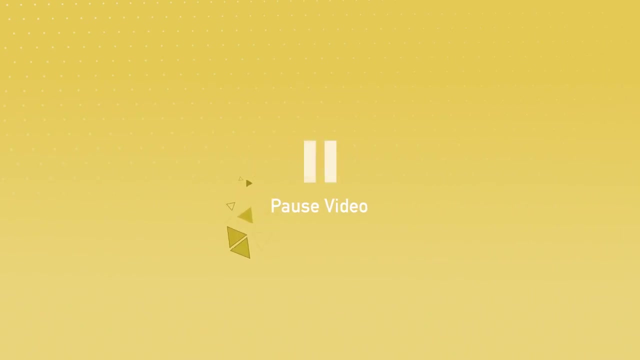 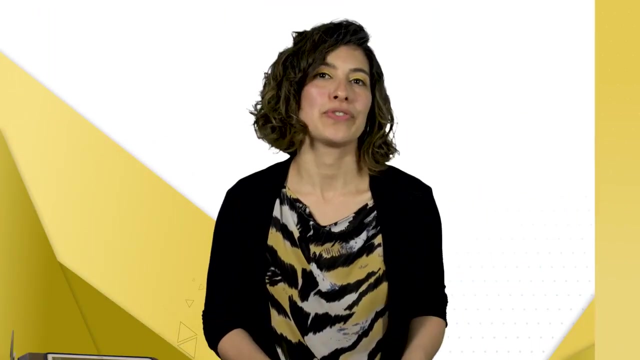 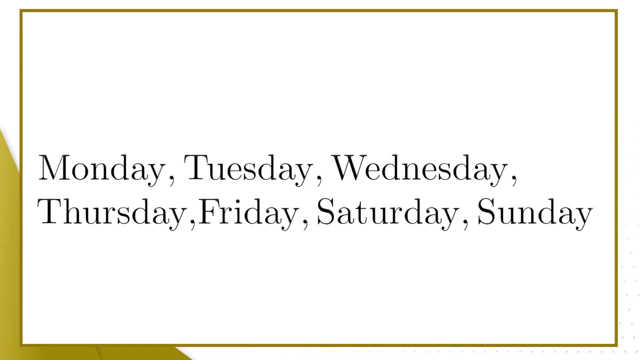 on the patterns found and your own way of describing each of these sequences in words. Let's gather our thoughts on this. The first is the sequence of weekdays starting on Monday. Note that it's a finite sequence. It only has seven terms. The second sequence: 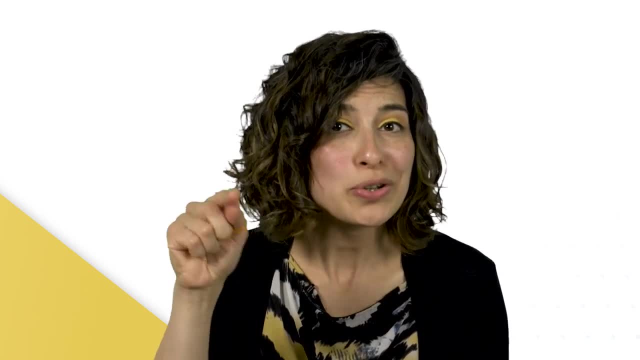 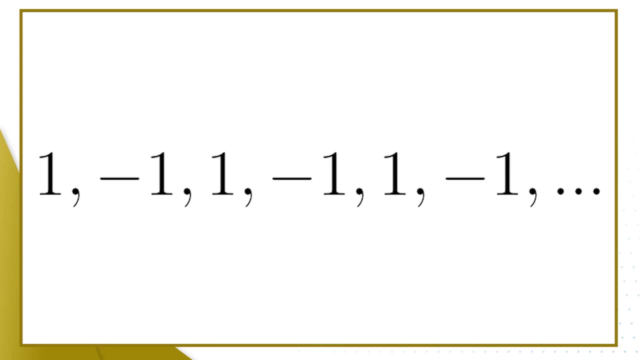 is infinite, as implied by the dot dot dot, which says continuing in the same pattern. So the pattern is alternating, Alternating between one and negative one. Or you could say: beginning in one subtract two, then add two, and so on, Another way of saying it. 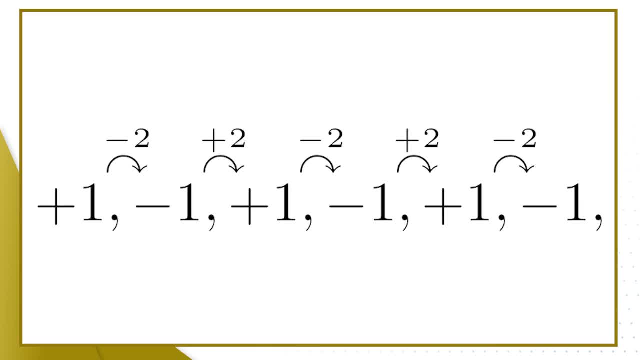 would be: you start in one and alternate between subtracting two and adding two. There is more than one way of describing it. The third sequence is described as begin with one, then write another one next to it and carry on like this. Or we could say: 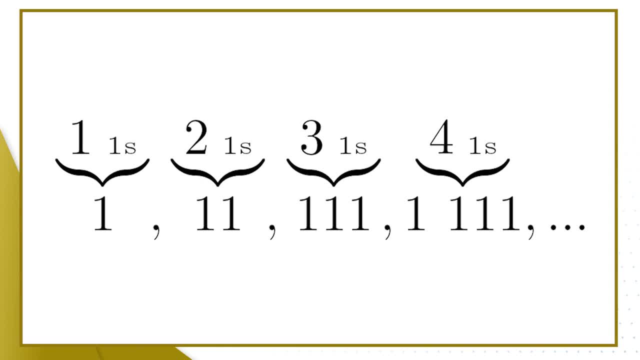 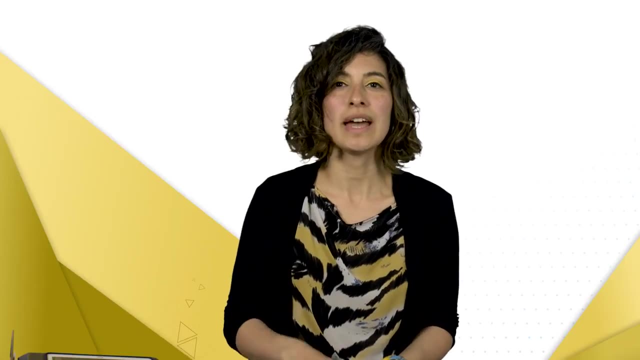 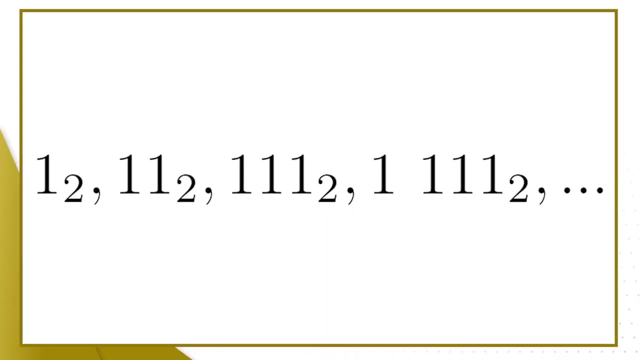 instead on each position write that many ones, So one one in the first position, two ones in the second position, three ones in the third position, and so on. Then add a hundred and so on, Or you could even be thinking of binary Anyway. 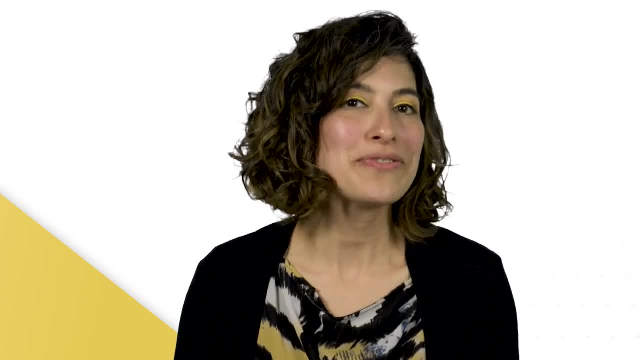 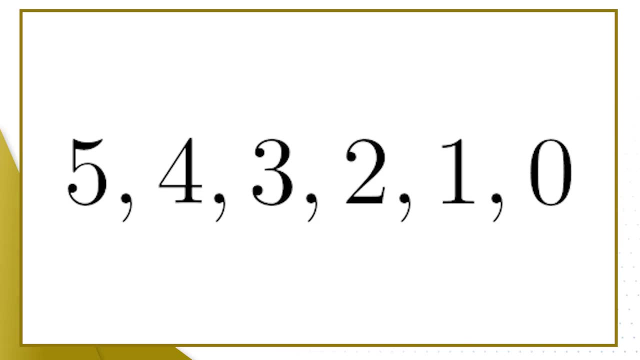 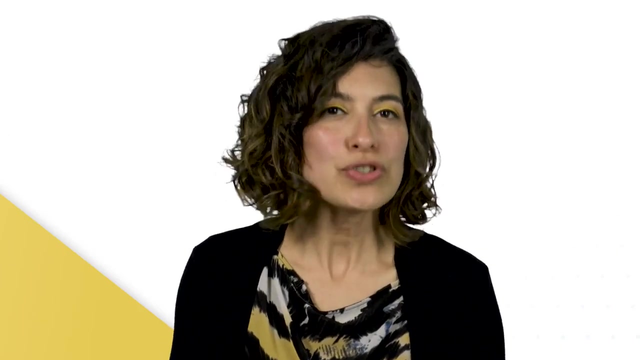 I let you think of how to express this pattern. The fifth is a finite sequence, a countdown from five, Or start in five and subtract one to get next stop at zero. Let's have another look at sequences. I want you to write down the patterns. 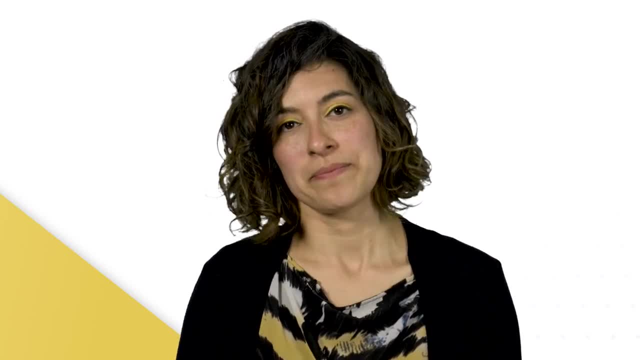 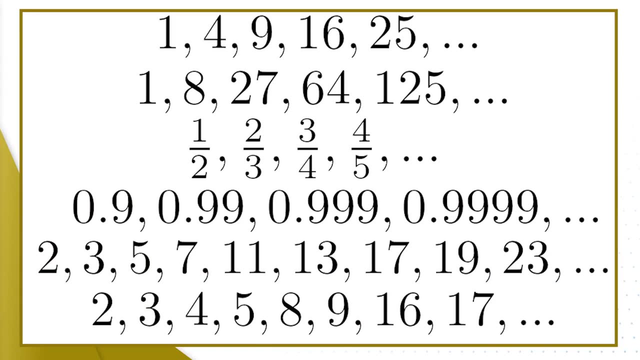 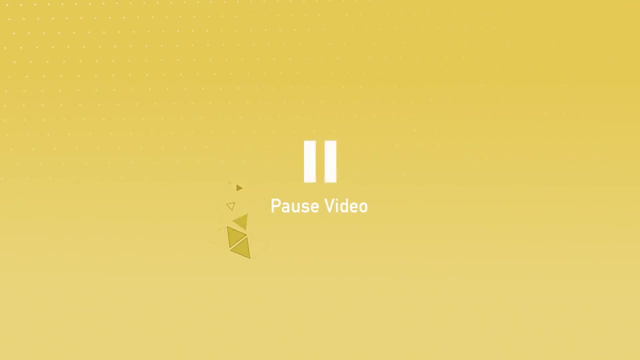 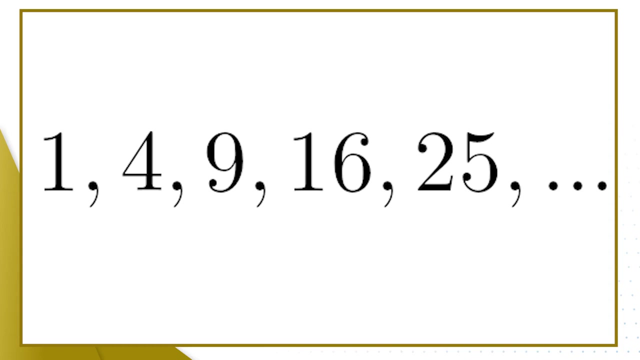 you find, so that you can relate them to another person. Here are the sequences. We're going to discuss them after the pause. Now, the first is a sequence of consecutive square numbers, starting from the square of one. The second is a sequence of consecutive: 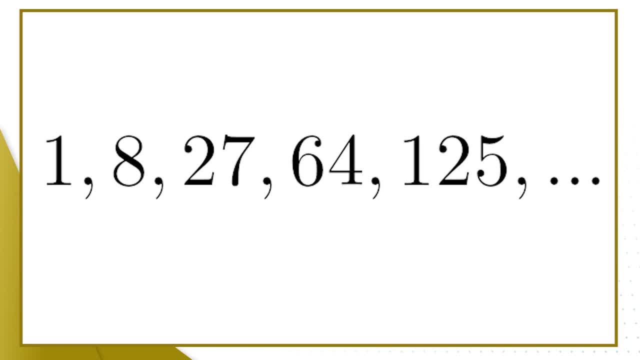 cube numbers, starting from the cube of one. The third is a sequence of fractions, of ratios, of consecutive numbers. The first term is one over two. The second term is the second number over the third. So two over three and so on. So the nth. 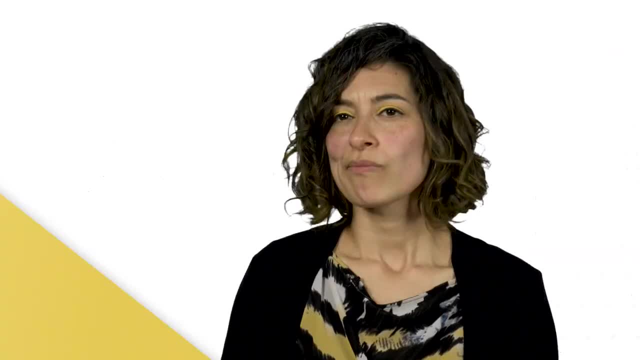 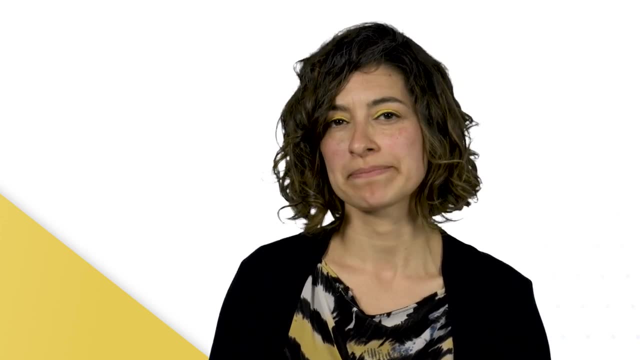 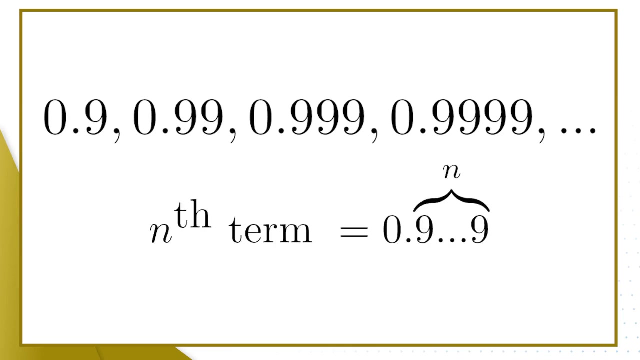 term is n plus one. We start needing formal mathematical language to define these sequences precisely Now. the fourth is zero point. as many nines as the order of the term? Does that sound complicated? The fifth could be the sequence of prime numbers. There is 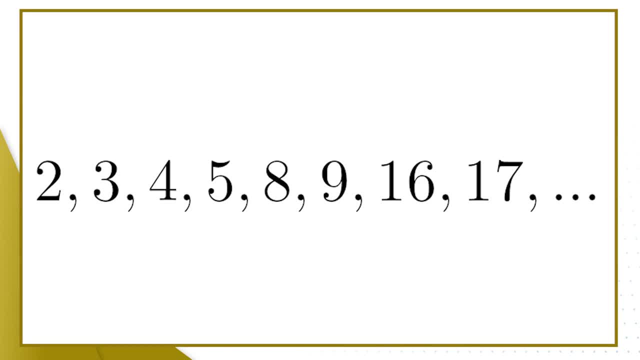 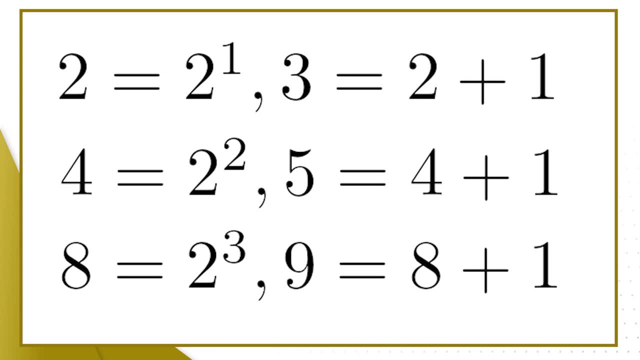 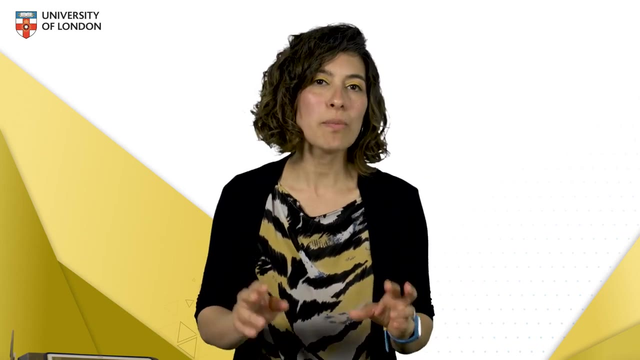 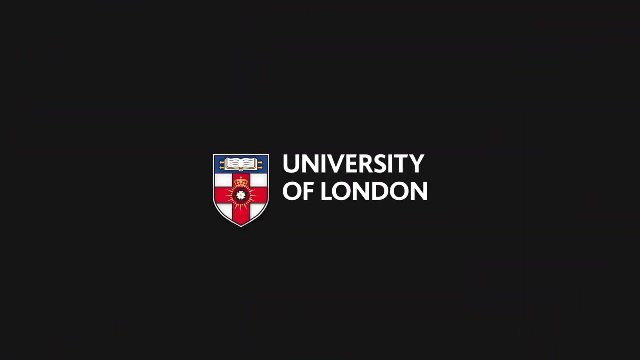 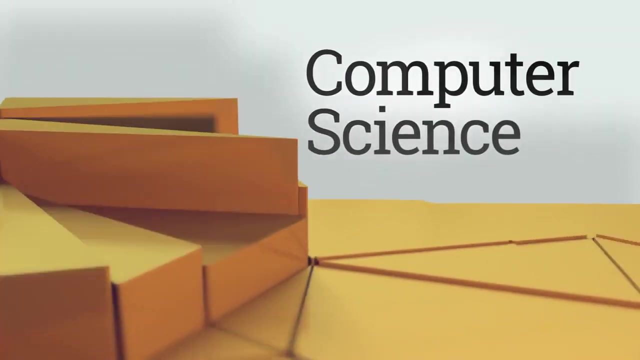 one over two and one over one. The sixth sequence seems to be a power of two and the number that comes next, Then the next power of two and the number one over it. You are probably with me. In the previous video we looked at patterns. 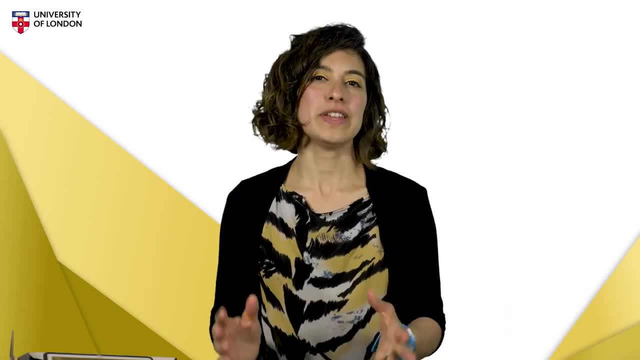 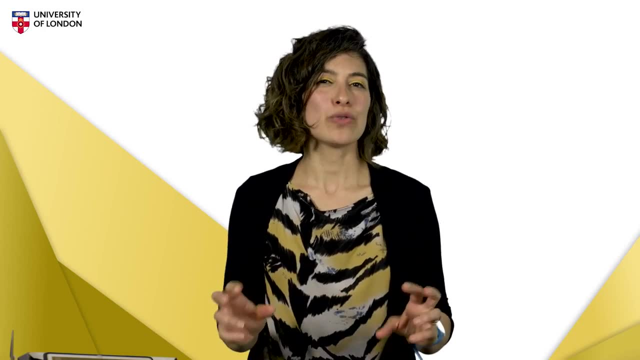 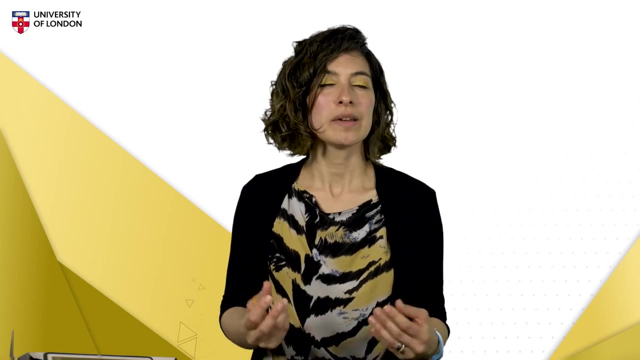 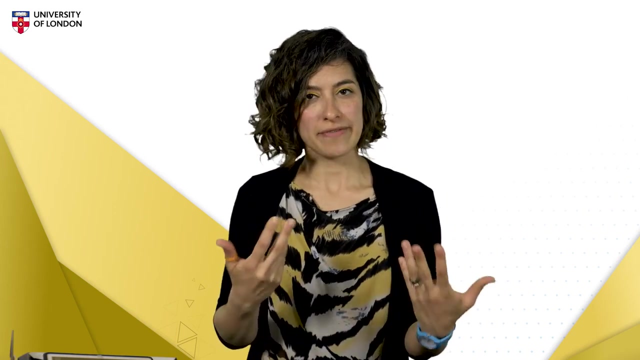 in sequences and I think you and I came to the conclusion that our way of describing them was a little bit ambiguous and sometimes hard to define precisely with words. Now we are going to define them more precisely here. Let's look at the sequence A1. 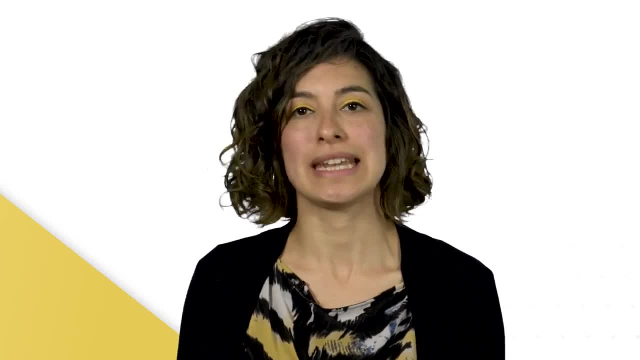 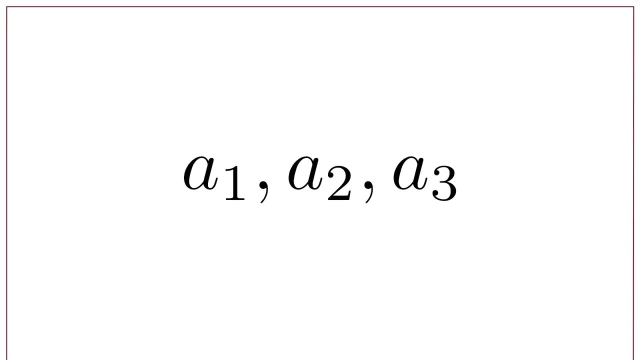 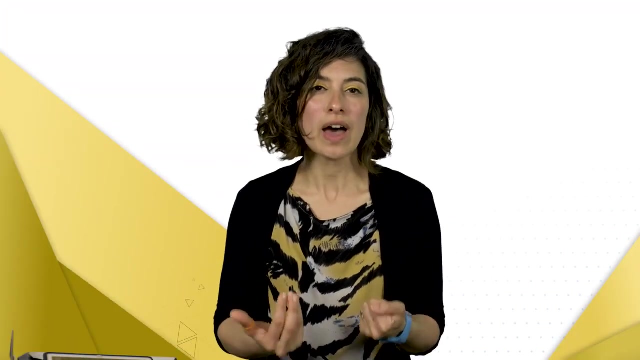 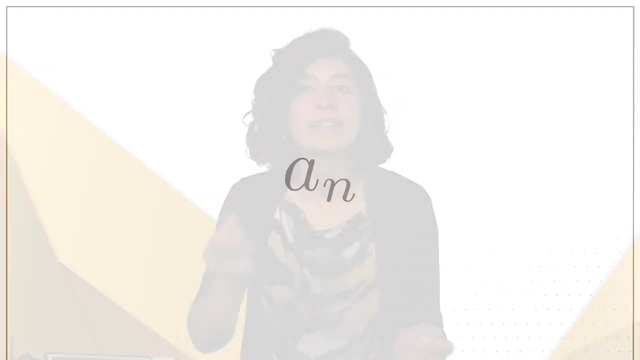 A2, A3 and so on. Each number in the sequence is labelled according to the order it appears. For example, in the sequence A there are terms such as N, and we write AN with the N in subscript as the general term of the sequence. 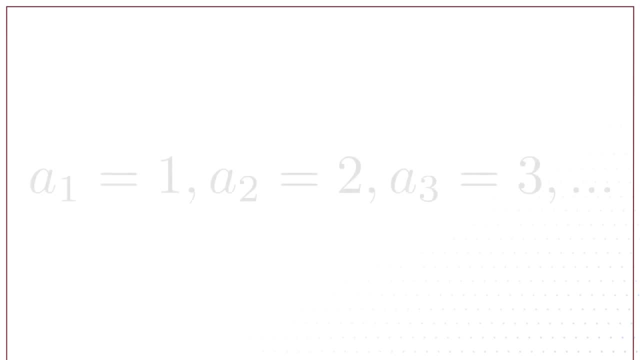 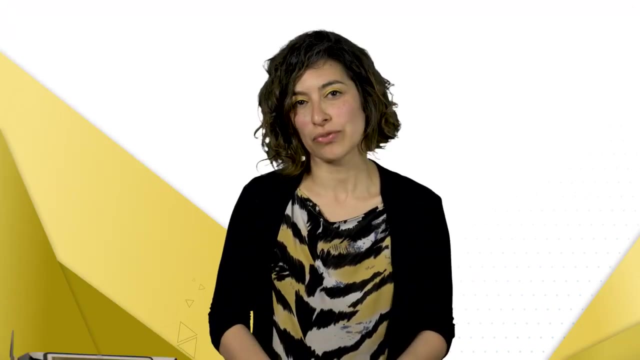 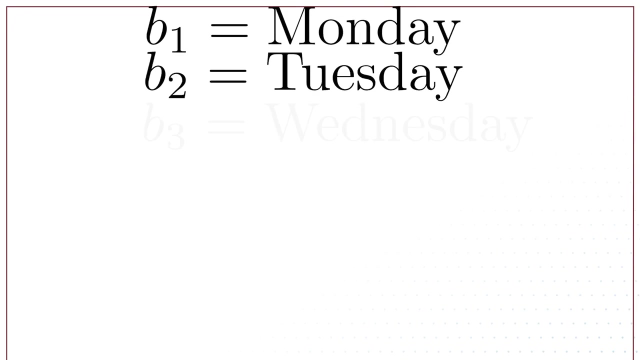 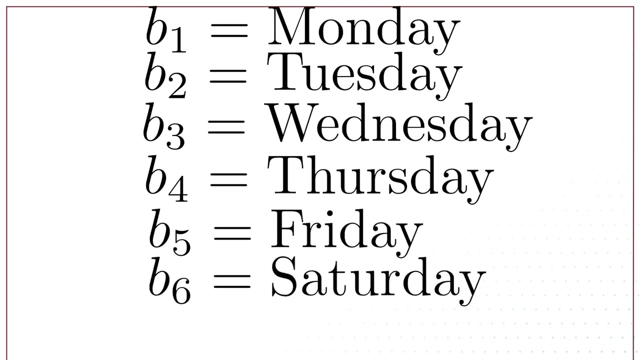 An example of such expression could be: AN equals N. This means that the sequence A will be term A1 is Tuesday, B2 is Tuesday, B3, Wednesday, B4 is Thursday, B5 equals Friday, B6 equals Saturday and B7. 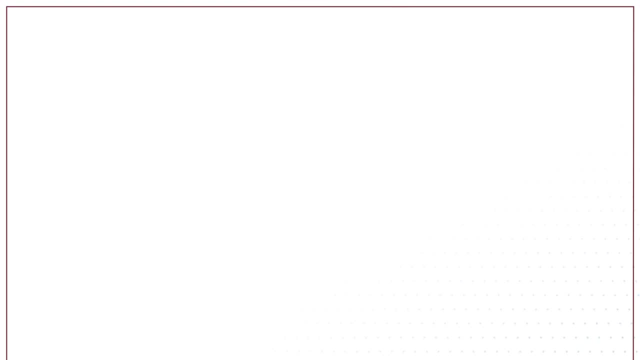 equals Sunday. The general term could be written as: BN equals the Nth day of the week, with N ranging between 1 and 1.. C1 is 1, C2 equals minus 1, C3 equals 1, C4 equals. 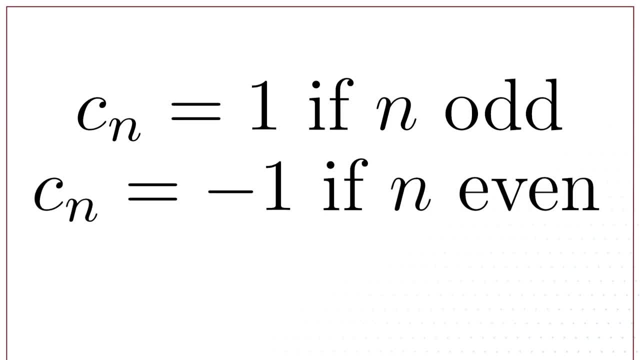 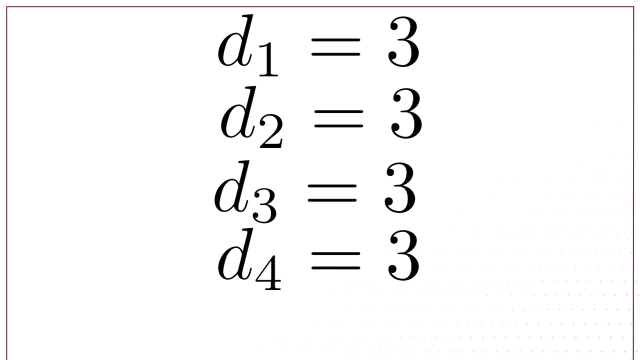 minus 1, and so on. The general term could be: CN is 1. when N is 1, CN equals minus 1 times minus 1 to the power of N. Check this out. The next sequence with constant 3s: D1. 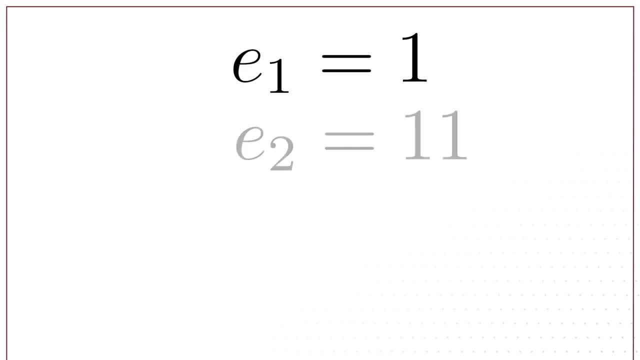 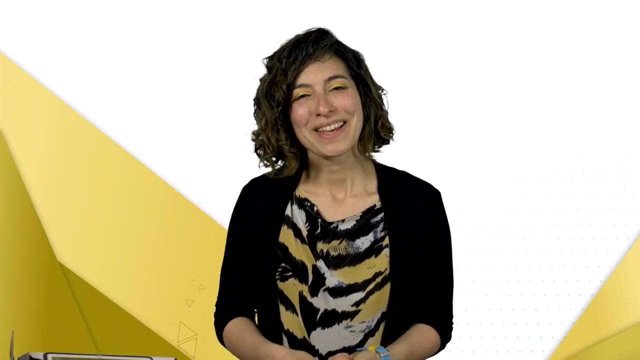 equals 3, D2 equals 3, D3 equals 3, E4 equals 1111, and so on. Or you may have read it as E1 equals 1, E2 equals 11, E3 equals 111,. 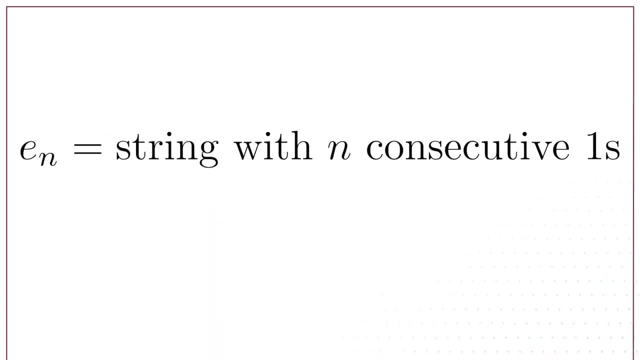 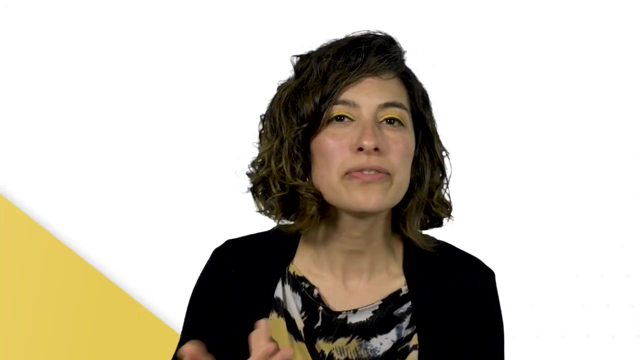 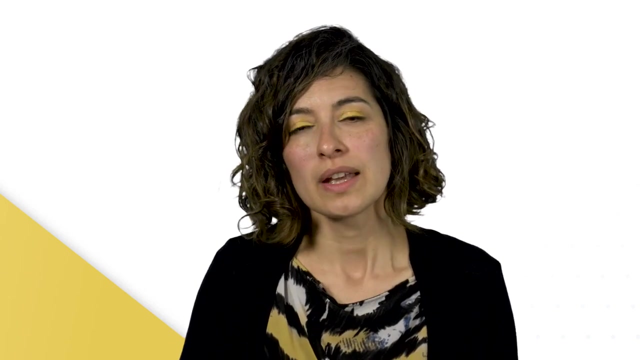 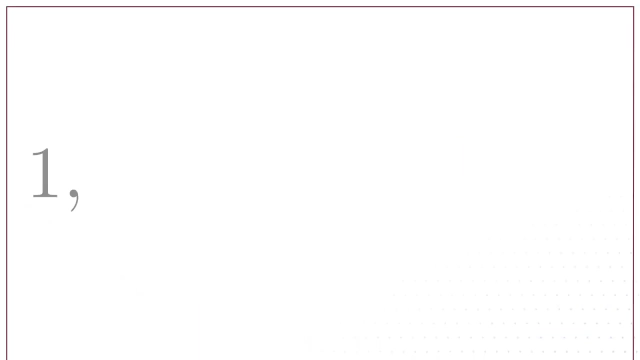 E4 equals 1111.. So the general term could be written as: 1 plus 10, plus dot, dot dot, the sum all the way to 10, to the power of N minus 1.. So we gave an expression to calculate the number of. 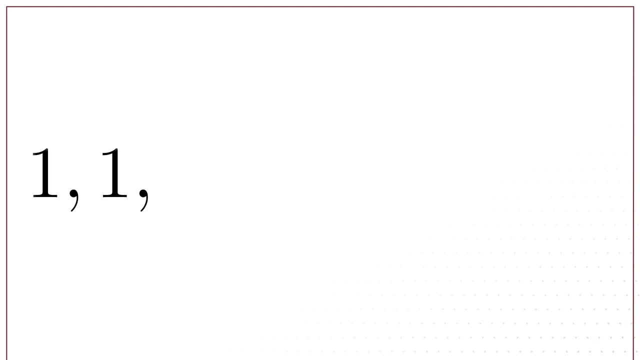 terms that are in the previous term. So we have 1, 1,, then 1 plus 1 is 2,, then 1 plus 2 is 3,, then 2 plus 3 is 5, 3 plus 5 is: 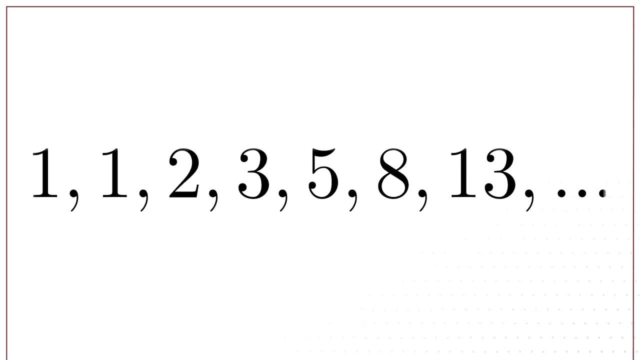 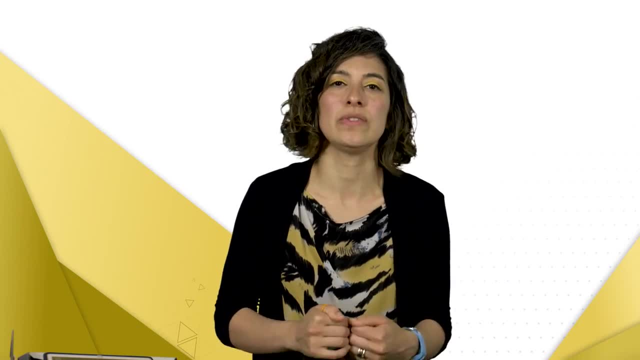 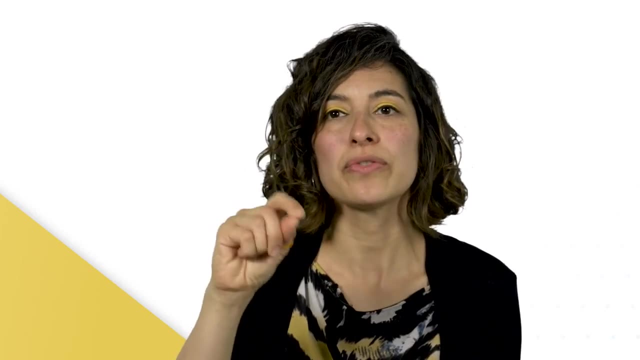 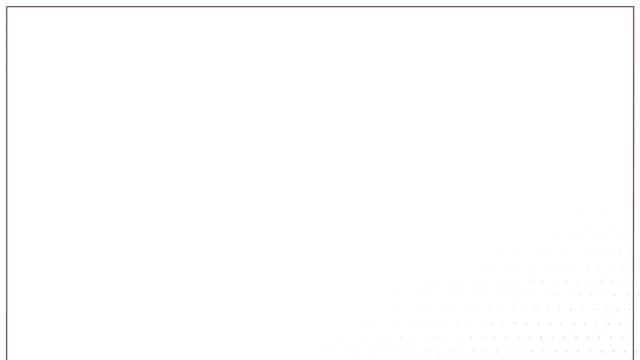 2 plus 3.. So this is a different way. This is called giving the recurrence relation. It is self referential, It refers to terms of the sequence to generate a number of terms. So we have f of n equals f of n. 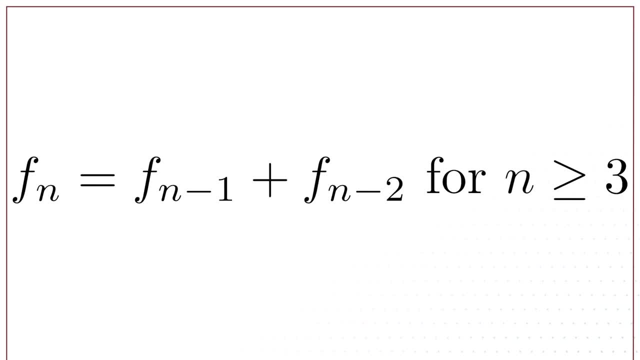 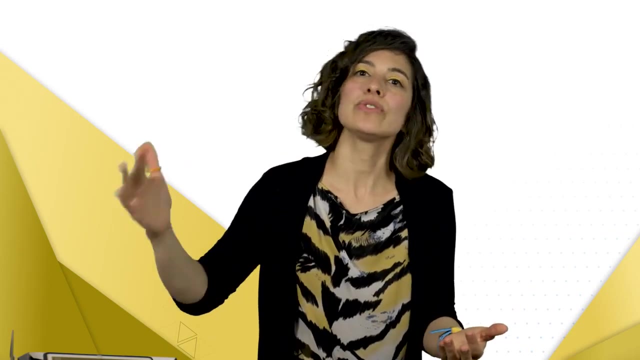 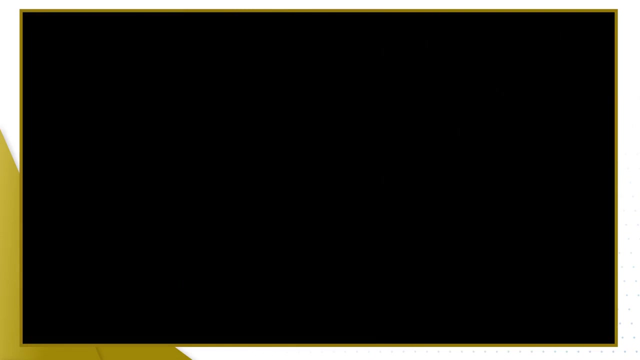 minus 1 plus f of n minus 2.. Those were the previous terms, the numbers before running from n equals 3 onwards and replace the value of n in the expressions. So I mean when n equals 1, we already have that f1. 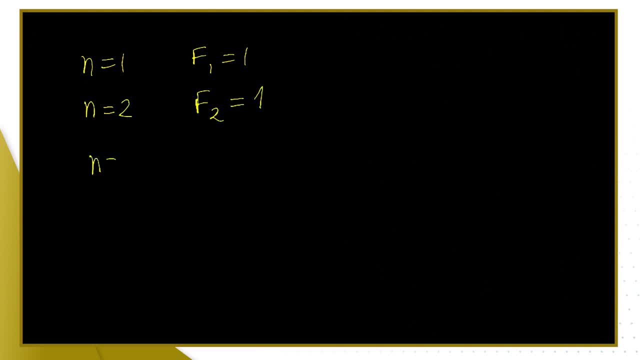 is 1.. That's stated explicitly. n equals 2, we have f of n minus 2.. We need to say when n is 3, in my expression I replace the n by 3. So f of 3 equals when. 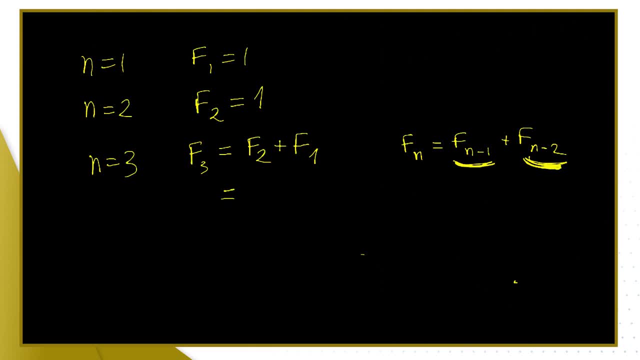 n is 3 plus f1.. Well, f2 is there, f1 is there. add them up, 1 plus 1, that is 2.. So I've got my f3.. And then for n equals 4,. 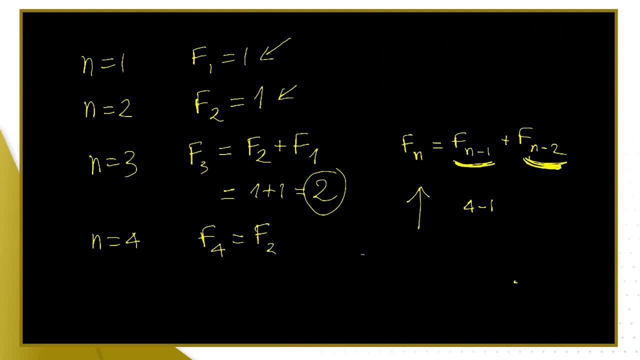 f of 4 equals- let's look at my expression over there- f of n minus 2.. So that's f of 4. take away 2, that is f of 2.. And that means the f of 3, which 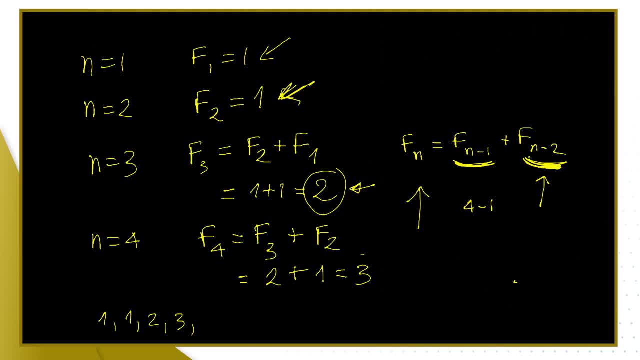 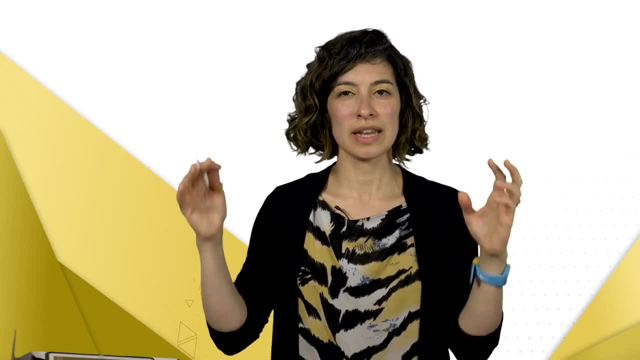 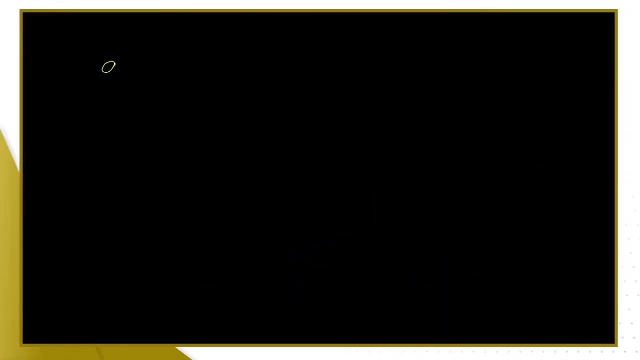 I got here, which is the value of n minus 1.. So that's the value of n minus 1.. And that is the value of n minus 1.. And that is for n greater or equal to n minus 1.. So 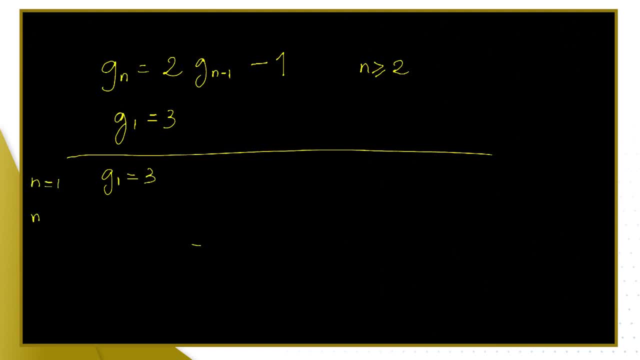 we start with 3.. So g 1 is 3. That's when n equals 1.. When n equals 2, we want g of 2. We'll replace g of 3 and then take away 1.. Watch bitmas. 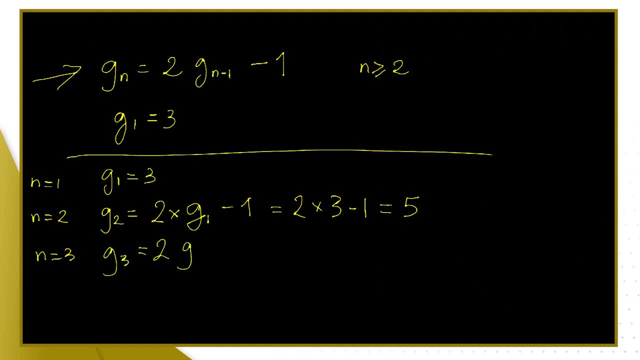 2 times 3 is 6.. 6 minus 1 is 5.. For n equals 3, g of 3 is twice g of 2, take away 1.. So that's 10 minus 1, that's. 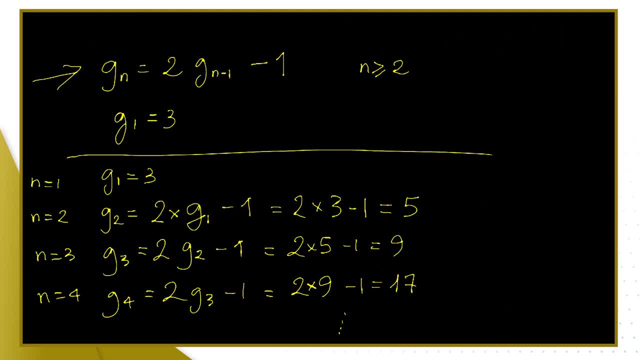 9. 10 minus 1 is 17,, and so on. So that sequence goes 3,, 5,, 9,, 17,, and so on. Now, if we look at the differences between consecutive terms, so the second from: 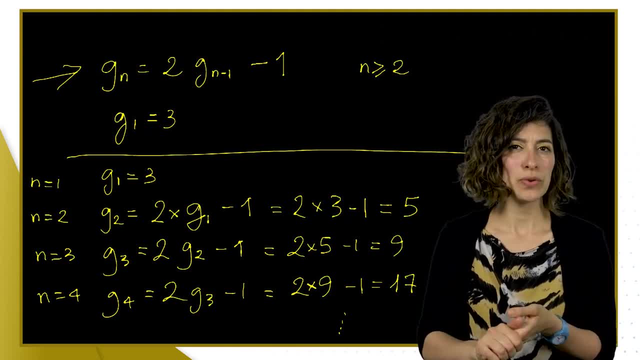 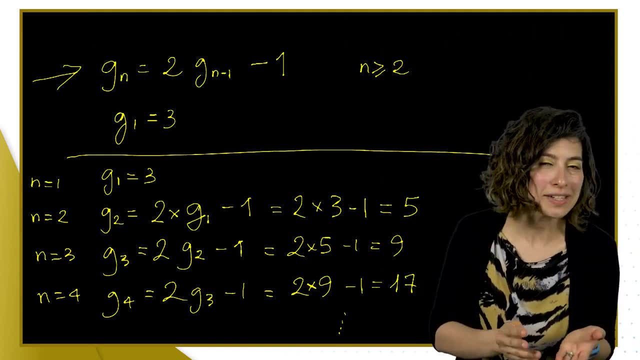 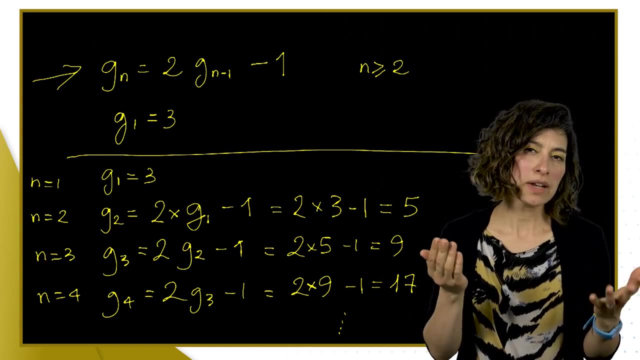 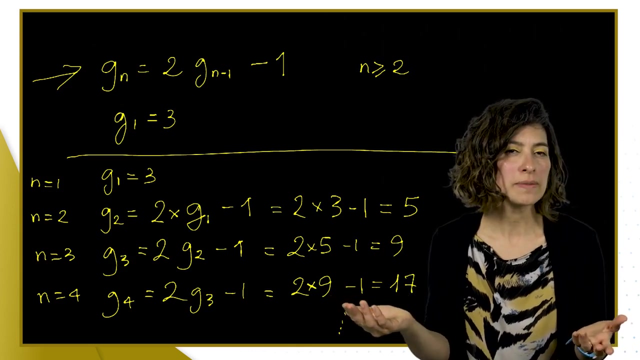 the third. so what happens with the second difference, meaning the differences between consecutive numbers in the differences sequence: 4 minus 2 is 2,, 8 minus 4 is 4,, 16 minus 8 is 8.. Does it? 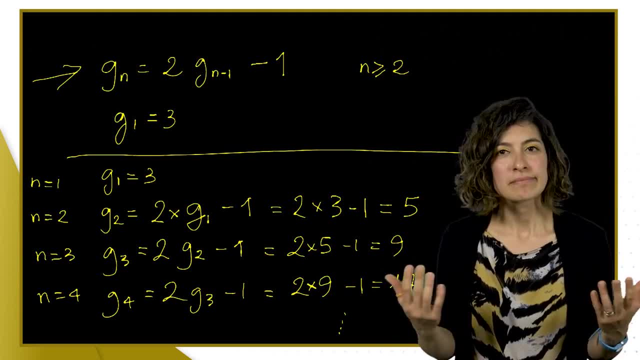 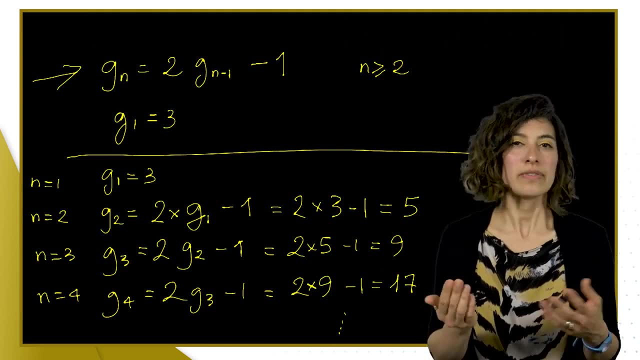 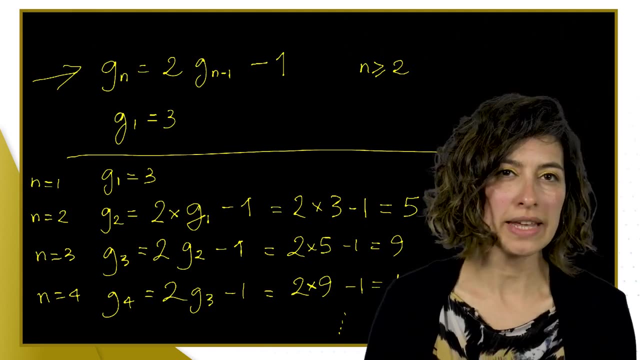 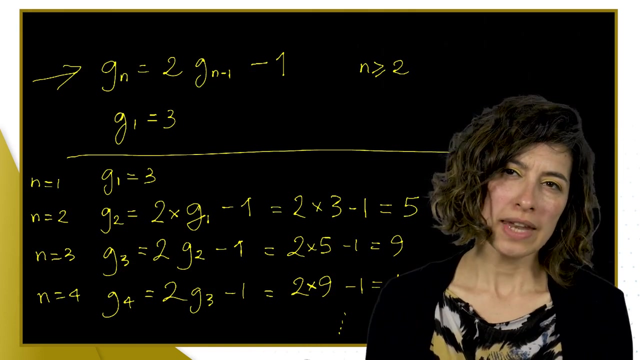 continue like this. Good question. Let's look at the ratio between consecutive numbers: 5 divided by 3, 9 divided by 5, 17 divided by 9.. Is there a pattern? Let's take the sequence as it is. 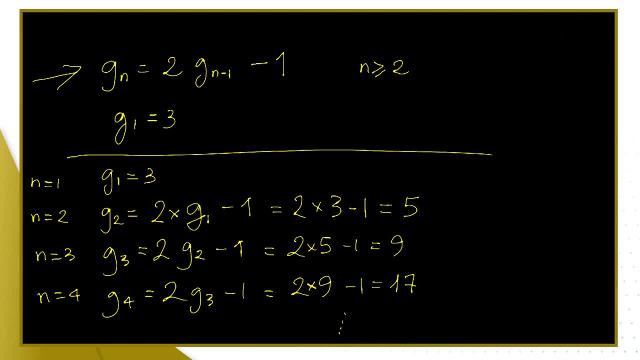 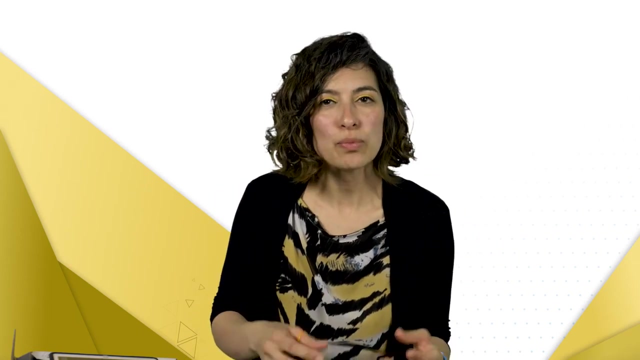 and subtract 1 from all the consecutive numbers In the new sequence 24816,, the ratios between consecutive numbers are always 2.. 4 over 2 is 2, 8 over 4 is 2,. 16 over 8 is. 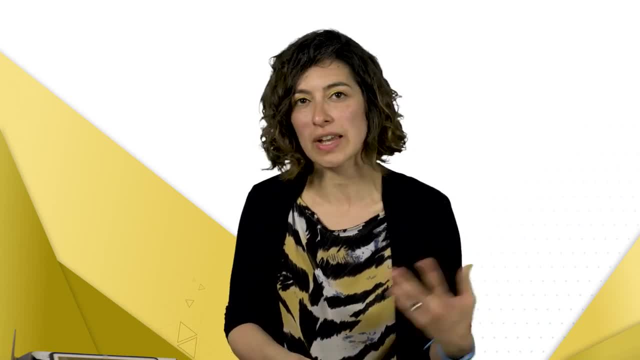 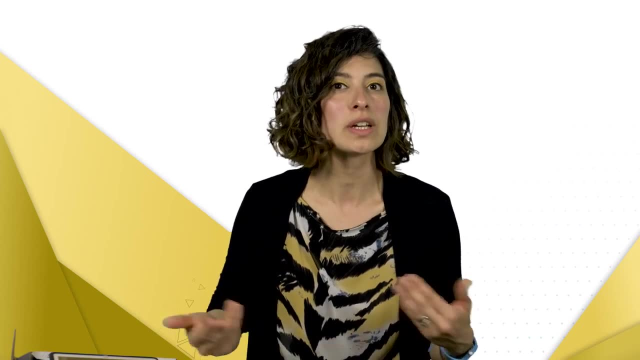 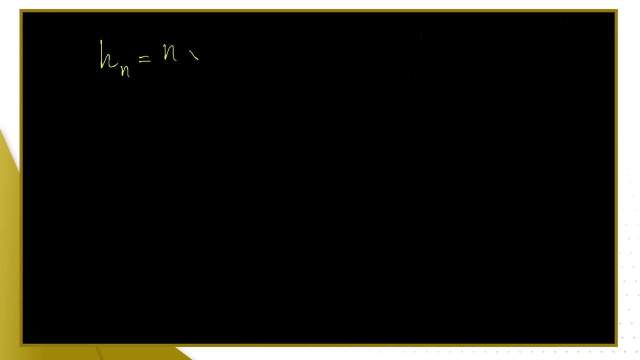 2.. That's interesting. I'm exploring the sequence and you might notice even other patterns. like we did, We subtracted 1 from the sequence and then took ratios. Let's look at another sequence. So the results for the new sequence are: 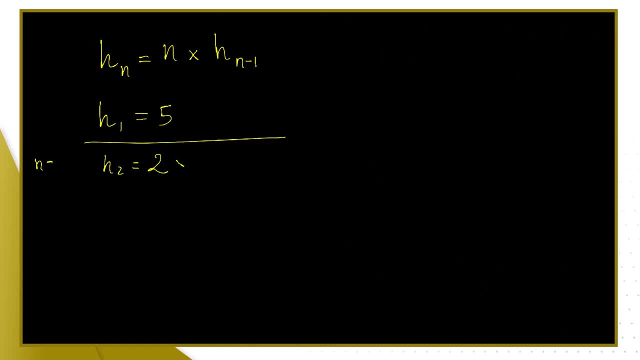 become 2.. We can make a pattern that is 2 times the 7. And we get 1 over 8. And we get 1 over that. n is 3, and here we have n minus 1, so we have 3 minus 1, which is 2.. 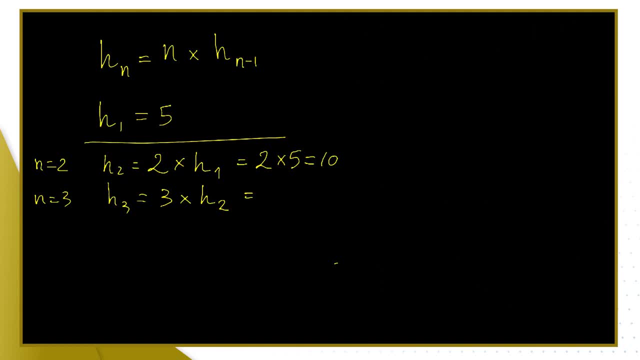 And that means 3 times the previous, so 3 times the 10,, which is 30.. When n is 4,, we have h4, so 4 times the previous guy, so 4 times the 30,, which is 120.. 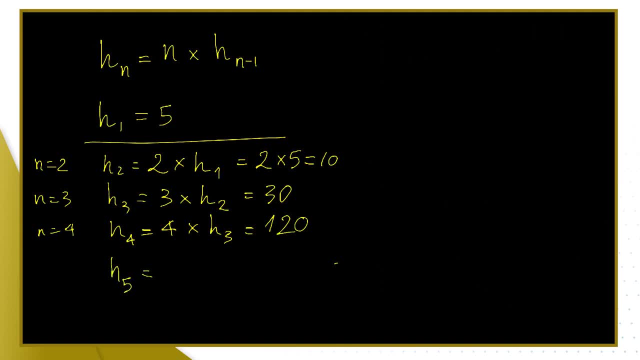 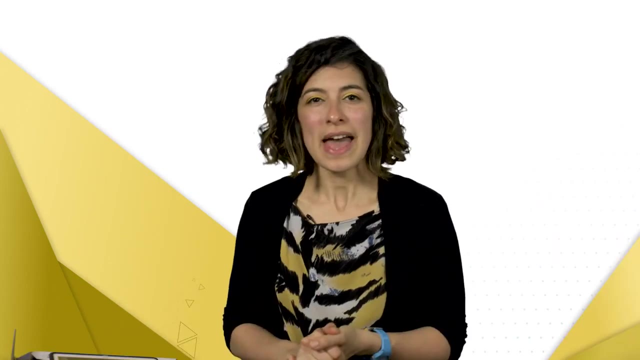 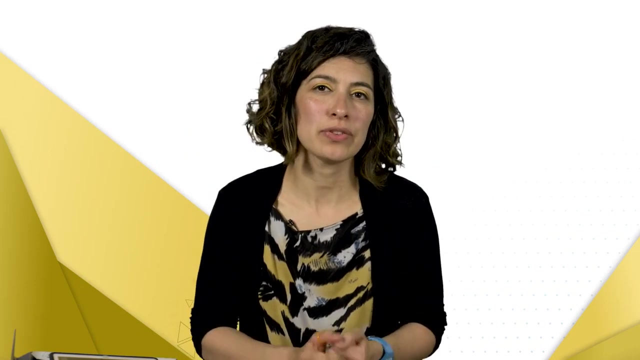 And for h5, we've got 5 times the h4, so 5 times 120, and that is 600.. And it carries on in that fashion. Let's see how we can describe this. one d of n is d of n minus 1 plus 2 times n minus 1, add 1.. 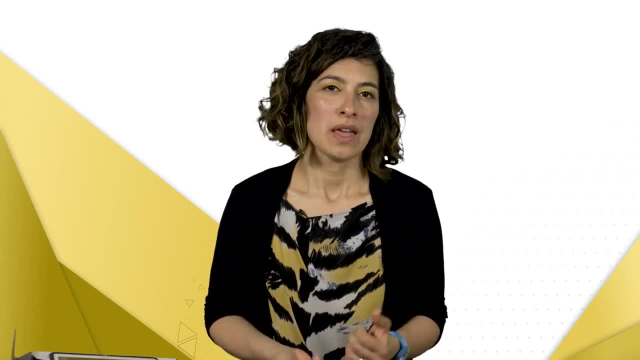 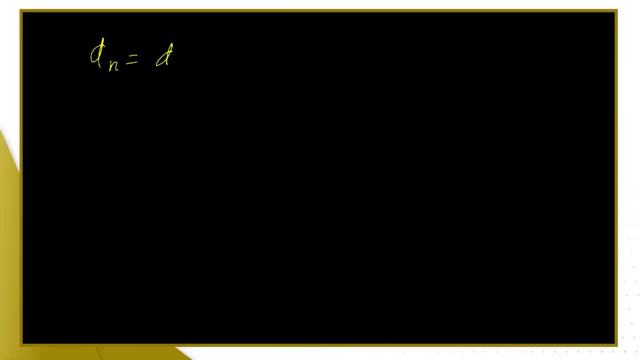 And the starting value- d1, is 1.. So how does this one go? Let's write it down. Okay, so that's for n greater or equal to 2.. So we've got: d1 is given. d2 is when n is 2,. 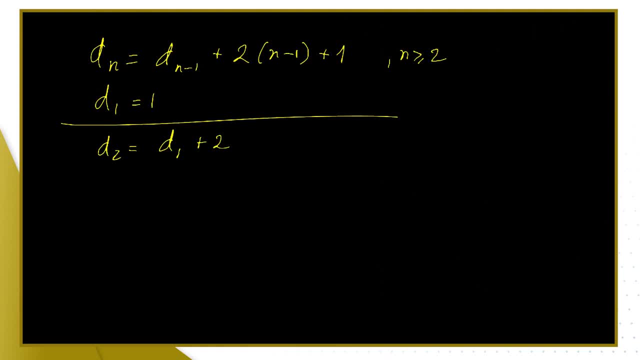 so we have d1 plus 2 times when n is 2, n minus 1 is 1.. And then like this: so d1 is 1, so 1 plus 2 plus 1, that's 4.. 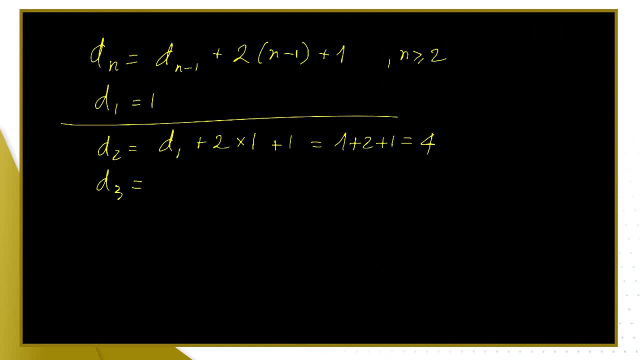 d3, this n is 3, so n minus 1 is 2, so I have d2 plus 2 times the n minus 1, so 2 times 2, add 1.. d2 was 4, so I got 4 plus 4 plus 1, that is 9.. 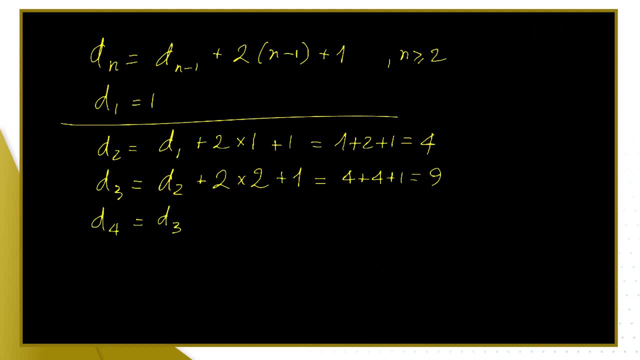 d4,, so n is 4.. That means I've got d3 plus 2 times 3 plus 1.. So that's 9 plus 6 plus 1, which makes 16.. And let's do one more. That's going to be d4 plus 2 times 4 plus 1.. 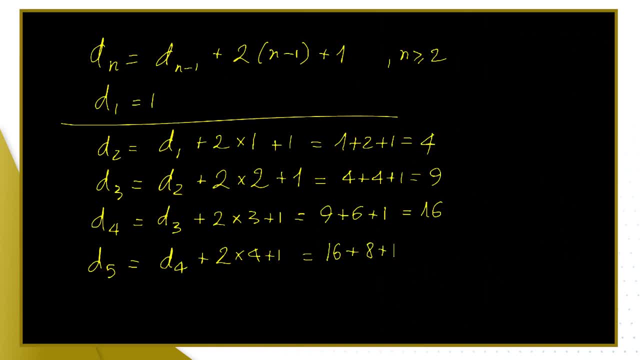 That is 16 plus 8 plus 1, and that makes 25, and so on. Now is there a pattern you can see there. It is described as a recurrence relation, but the numbers go as 1,, 4,, 9,, 16,, 25.. 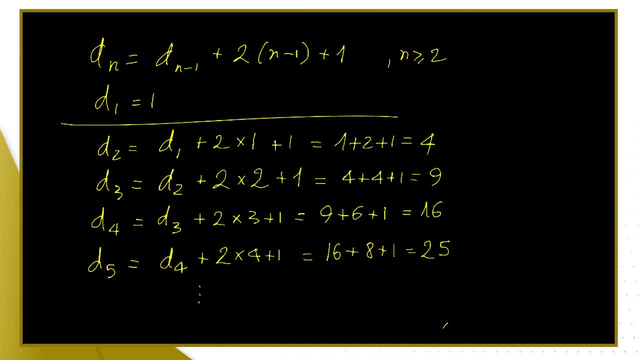 And you're probably thinking this is a square number sequence. It is, We could write it as a square number sequence. so we could write it as: dn equals n squared for every value of n And at the same time, that is the recurrence relation. 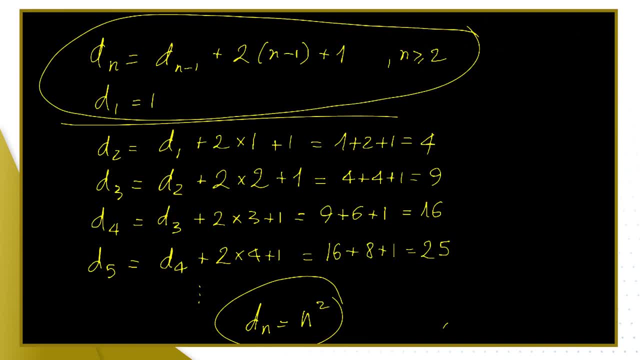 So you can have both. Can you always write a formula like a general term for a sequence that is given as a recurrence relation? That's a good question. We're not going to worry about that in this course, but I'll let you investigate that for your own satisfaction. 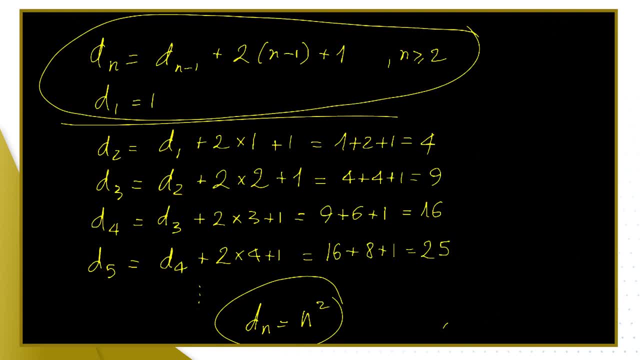 Now one more. Sorry, I said that wrong. The one more is not. Now still on this sequence, we can look at the differences Between consecutive terms: 4 minus 1 is 3,, 9 minus 4 is 5,, 16 minus 9 is 7, and so on. 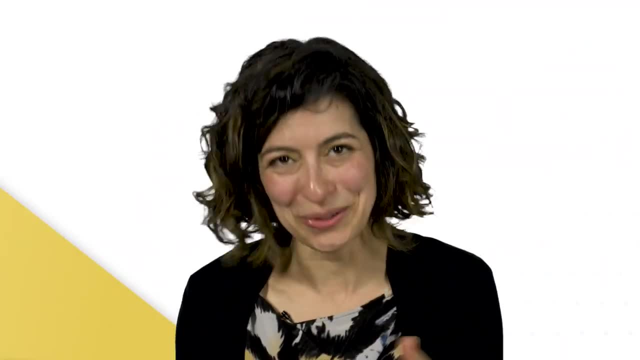 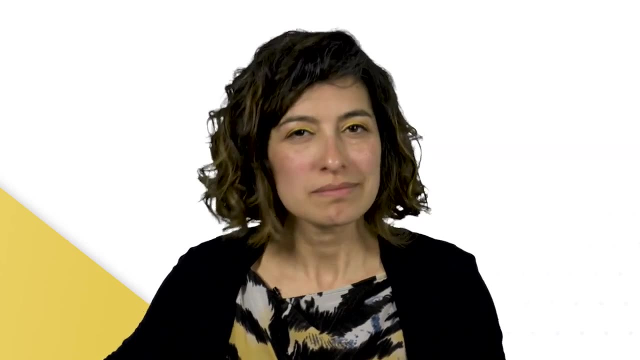 Is it the prime number sequence? No, we need to look at more terms. The next difference would be 9.. Actually, the odd numbers, Of course. there's the question: can we prove it? You can by looking at that sequence. 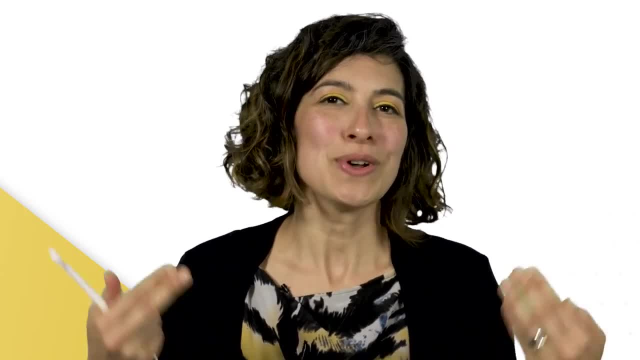 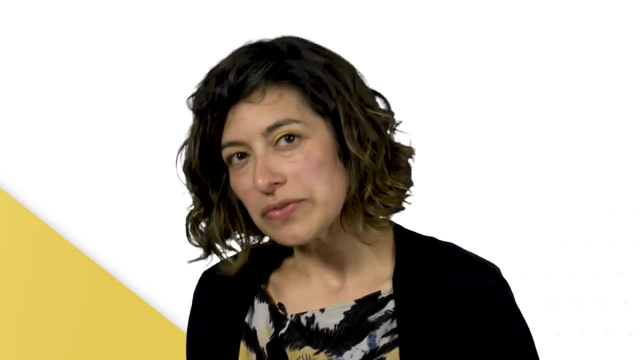 I'm not asking you to do so, But I was just wondering. I just want to get you to think about all these patterns. Now still on that, on the sequence of differences: if we do second differences, we get 2 every time. 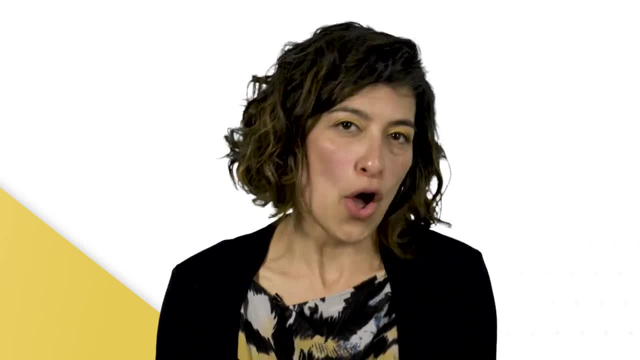 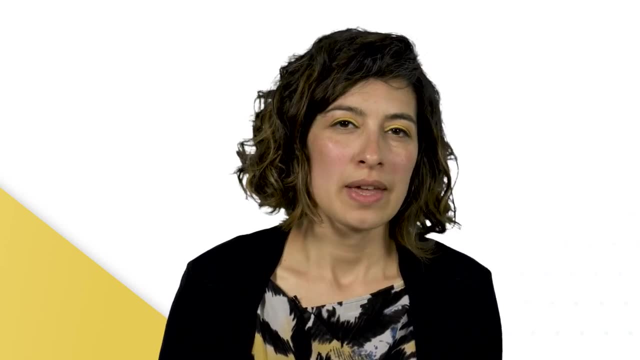 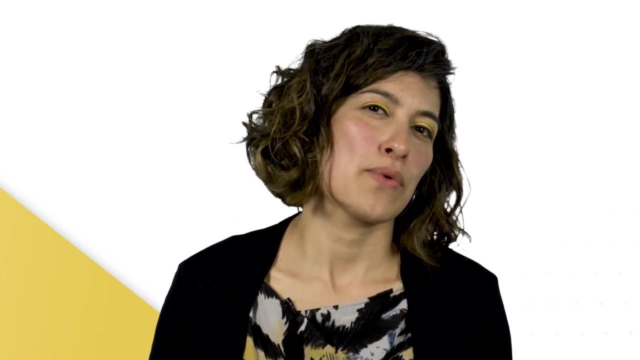 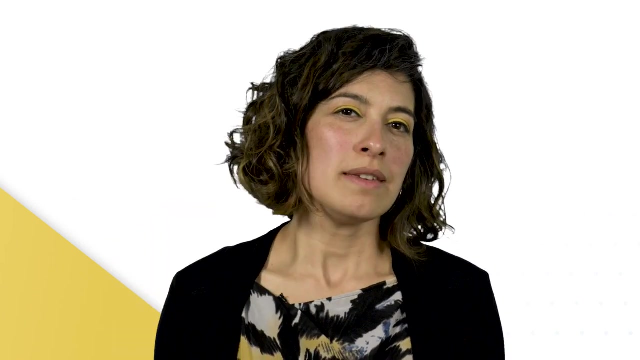 Is it a coincidence? No, it is not. If you look at the expression for dn, yes, it is a sequence of square numbers. No, dn is the sequence of square numbers, So being a sequence of square numbers, the second difference. 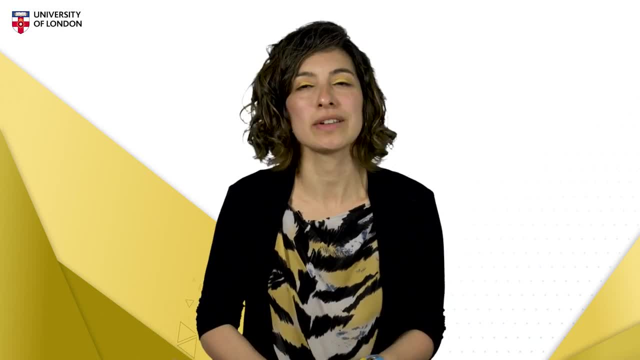 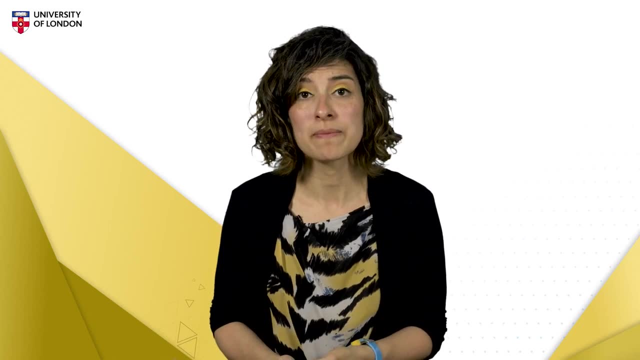 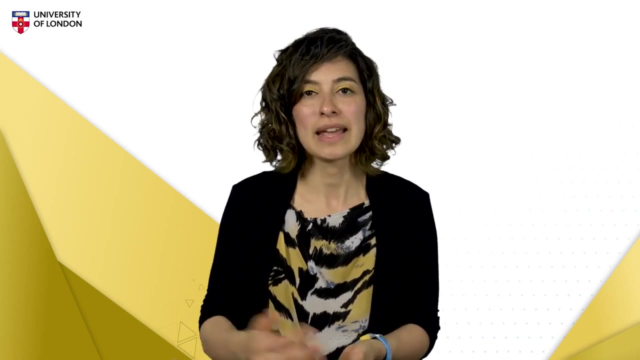 Well, it's not really a coincidence, dn being a sequence of square numbers, that squaring actually means that the second differences should be constant. There's no reason why you should know that, but I'm going to plant that in your brain for now. 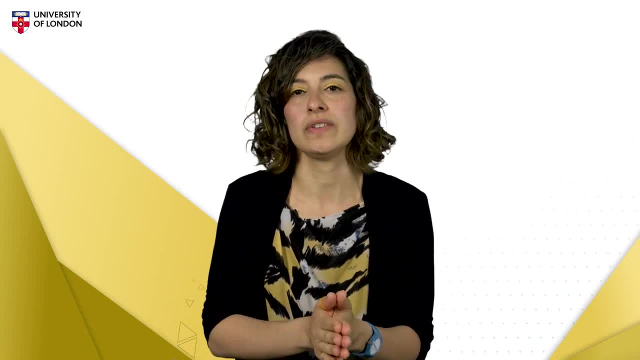 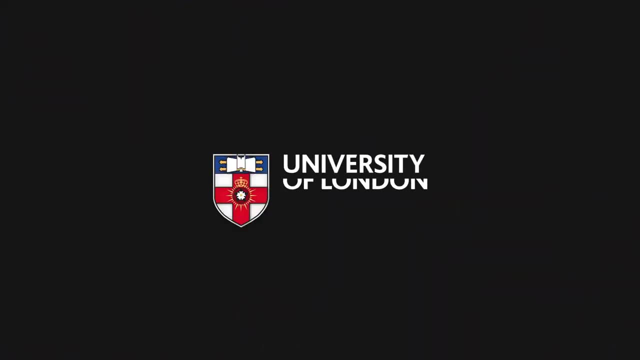 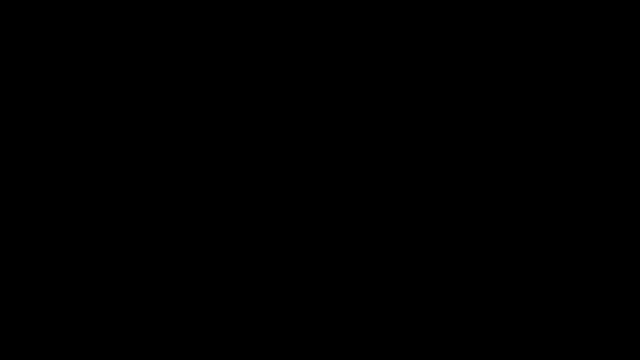 Now, when you work with data and are looking to find patterns, you can also use a spreadsheet to automate your pattern search. So, for example, let's do that. So if we take the first one, what we do is go through the first one. 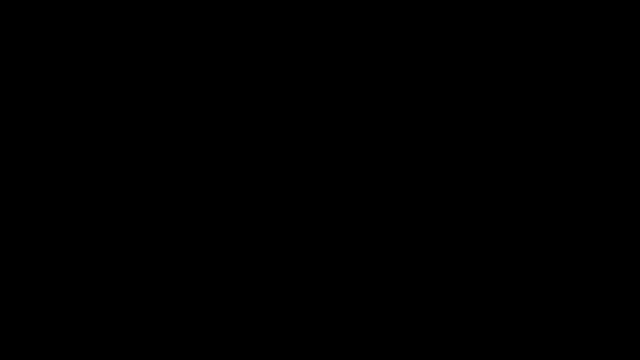 And we can use our first one to see what it looks like And we can use our second one to see how it looks like. And the reason we have the second one to see how it looks like is because the second one is aowed to us. 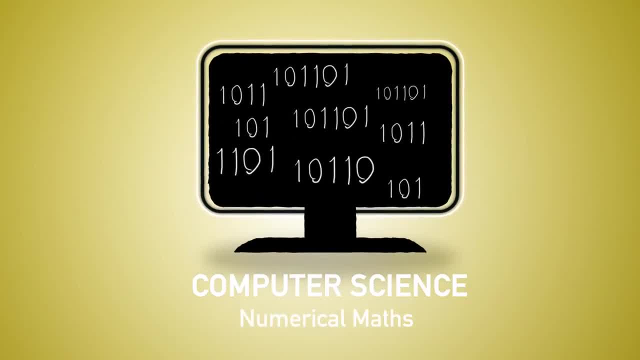 And so what we have is the first one, And the second one is not the first one, but the second one. So that's all we're going to see, And then the next one. let's put ourselves in your brain. Hello there. 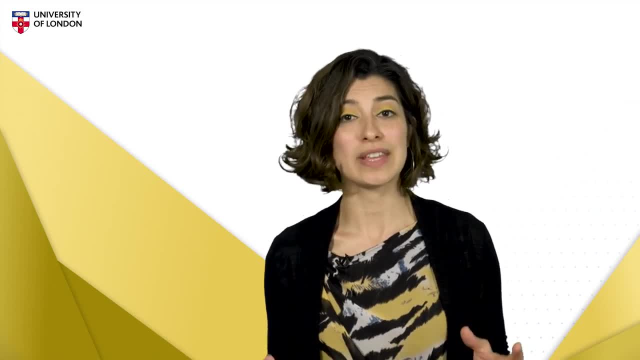 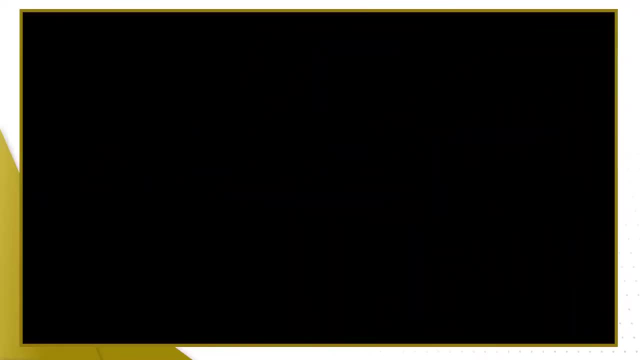 And we're going to look at special type of sequence called the arithmetic progression. Let's look at the sequence AN. that starts with 4 and it goes with 6,, 8,, 10,, 12 and so on in the same pattern. You probably notice what the pattern is. We're adding 2 every time to 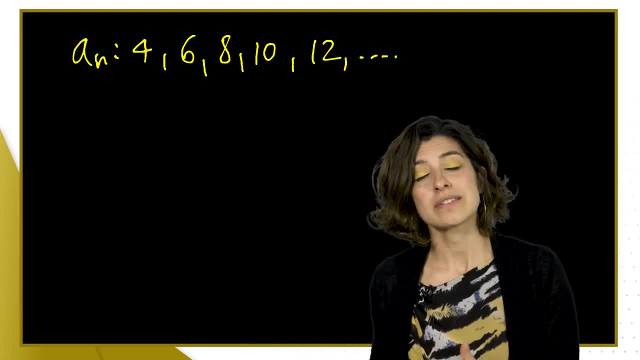 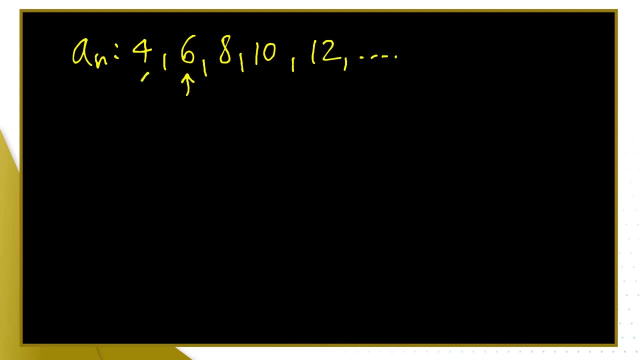 generate the next number and I can check that by doing the subtraction of two consecutive terms. So 6 minus the 4 is 2, 8 minus the 6 is 2, and so on. So I'll write that using the terms: so A2 minus. 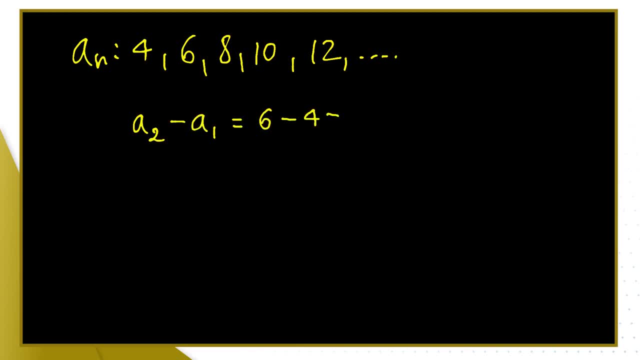 A1 is 6 minus 4, that's 2, A3 minus A2 is 8 minus 6, which is 2, and I will carry on doing consecutive subtractions and I will always get 2, because the law of 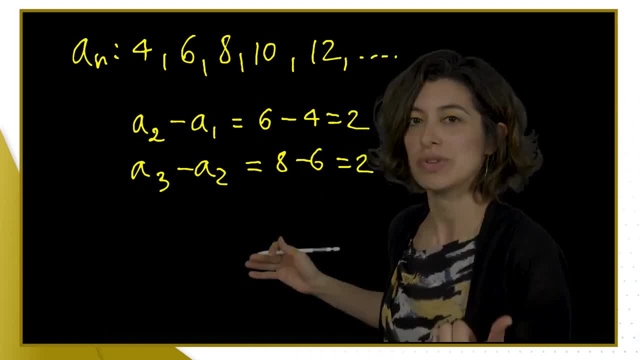 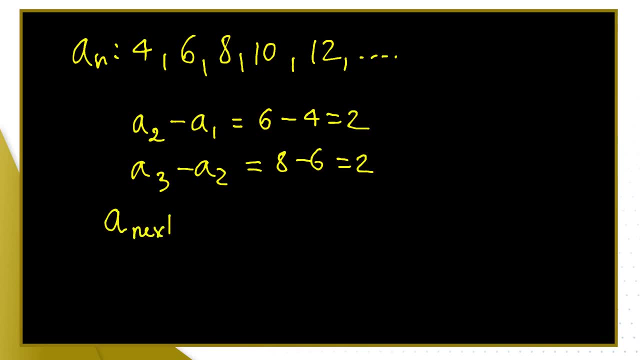 that motor does not operate. generating the next term is always adding 2 to the previous term. That means we can write it as a recurrence relation and that means that the a next is the a previous plus 2.. We're almost there, because it's not a very maths-y way of writing that expression. 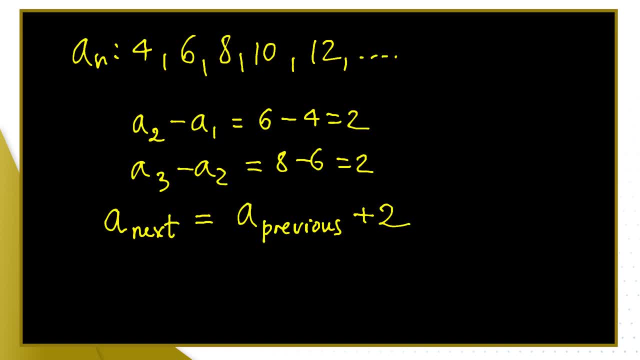 Let's write it properly with the variable in the label. So a of n plus 1 is the a of n add 2.. So I'm adding 2 to the term a n, just to make sure we're not adding 2 to the. 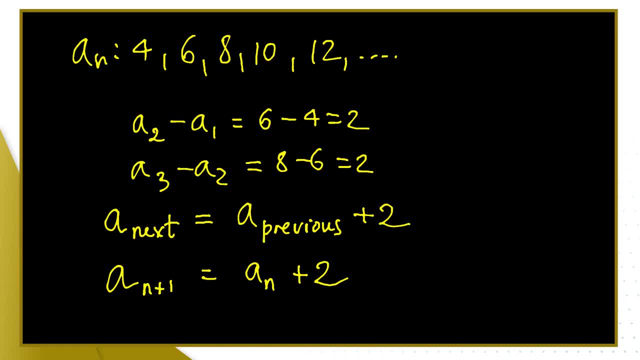 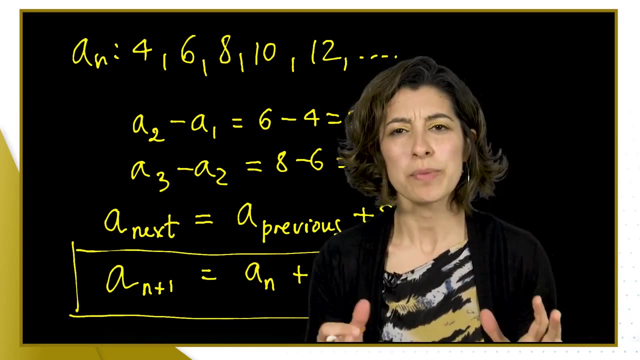 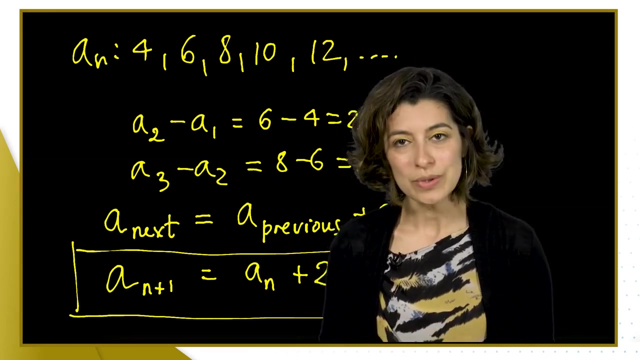 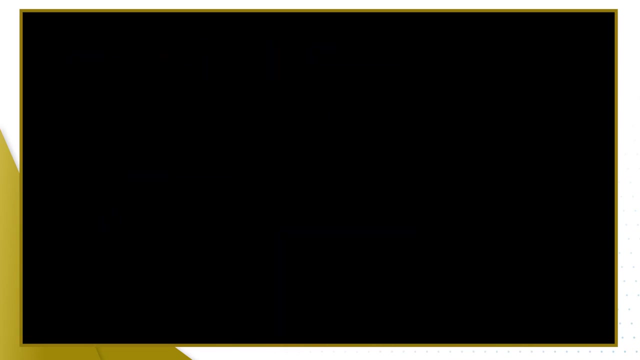 label, We're adding 2 to the value of the term And, as usual, we need to say what's the first term, and that is 4.. So that completely defines the sequence above. Subtitles by the Amaraorg community group at Amaraorg. 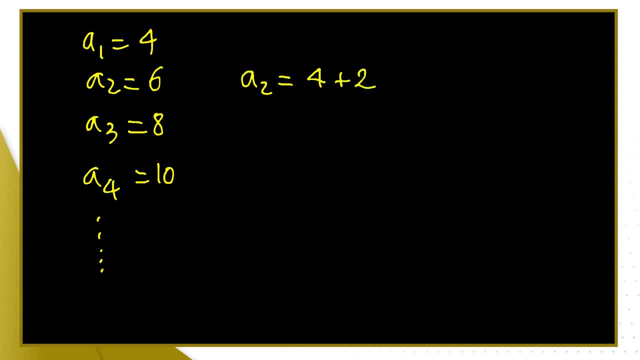 A2 is 4 plus the 2.. A3 is 4 plus the 2 and another 2.. And A4 is the 4 plus the 2 plus the 2 plus another 2.. I wrote all that detail because I wanted to see how the formula is. 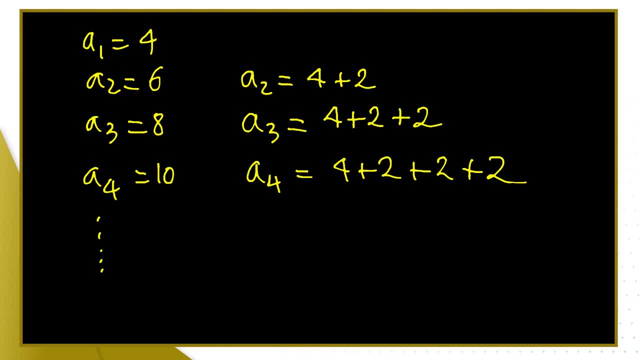 going to appear. I start with 4, and then I add a certain number of 2s. How many 2s do I add every time? For the first term, I add one 2.. For the third term, I add 2 2s. For the fourth term, I add: 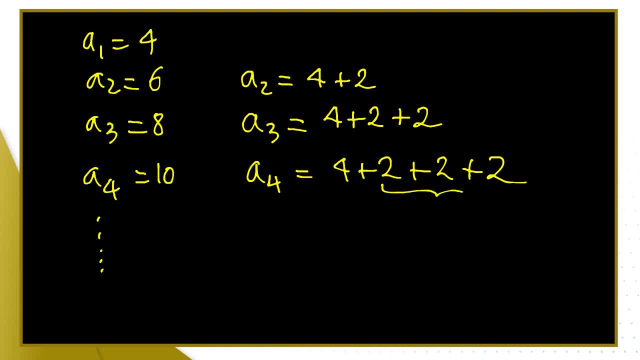 3, 2s. So for the nth term I'll start with 4 and I add 2s, but just one s, then the n, And that will be the expression for the sequence. that is an arithmetic progression with common difference 2 and first 2.. 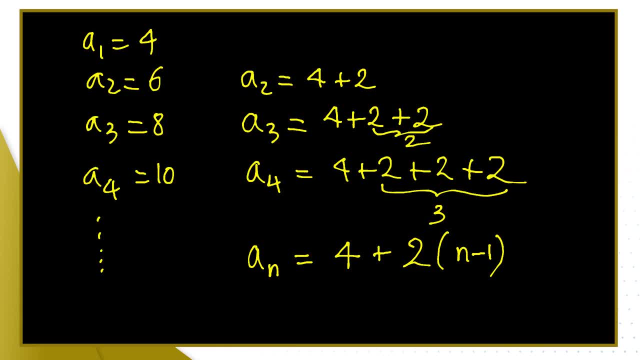 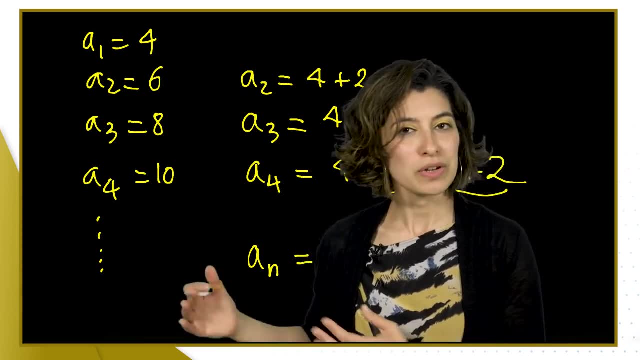 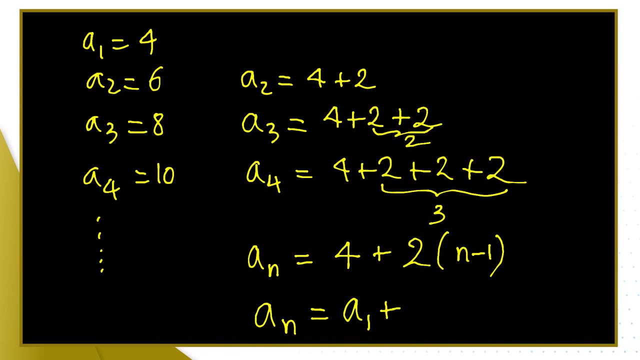 Subtitles by the Amaraorg community term 4.. Traditionally we write d for common difference and the first term is a1, so I'm going to rewrite this formula in that way. So an is the first term for added, the common. 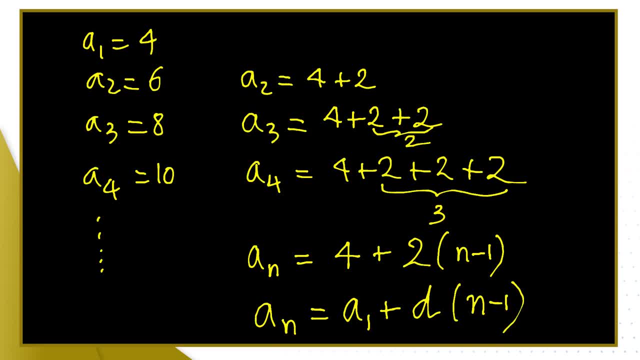 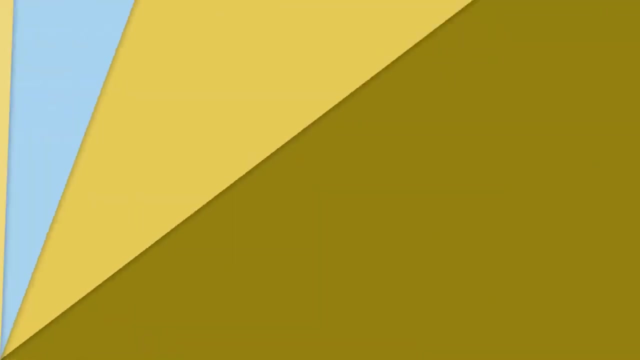 difference d n minus 1 times, And any arithmetic progression will obey this law. Any arithmetic progression will have a common difference d and will have a first term, a1, and the expression for the general term is given by this formula. Given any sequence, how do you? 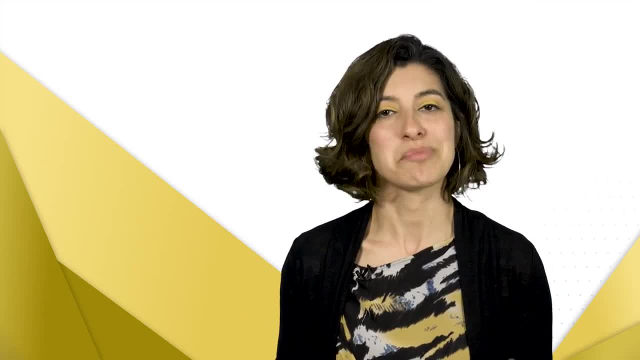 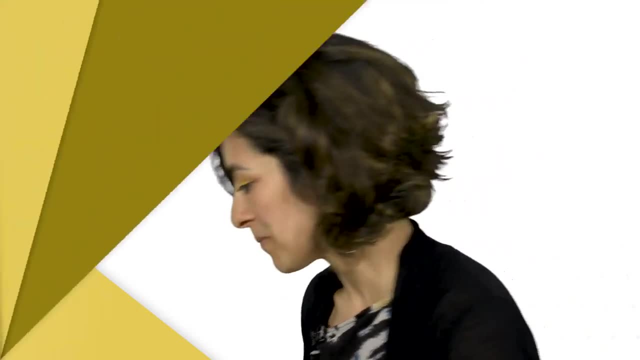 check if the sequence is an arithmetic progression. We need to check if there is or not a common difference. For example, if we have 1,, 3,, 5,, 7,, 8,, 9,, 10,, 11,, 12,, 13,, 14,, 15,, 16,, 17,. 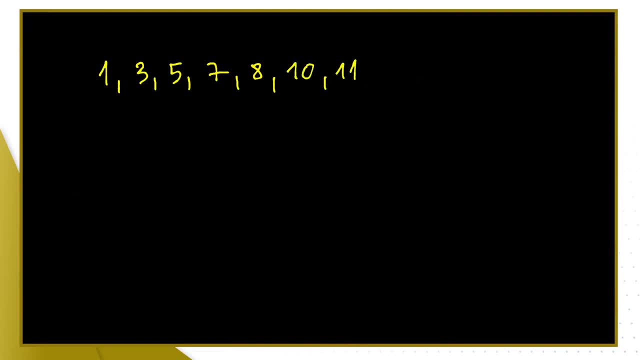 18,, 19,, 20,, 21,, 22,, 23,, 24,, 25,, 26,, 27,, 28,, 29,, 30,, 31,, 32,, 33,, 34,, 35,, 36,, 37,, 38,, 39,. 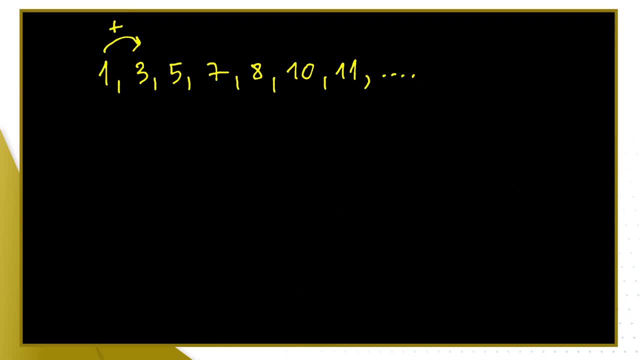 40,, 41,, 42,, 43,, 44,, 45,, 46,, 47,, 48,, 49,, 50,, 51,, 52,, 53,, 54,, 55,, 56,, 57,, 58,, 59,, 60,, 61,. 62,, 62,, 62,, 63,, 61,, 62,, 63,, 62,, 64,, 63,, 62,, 62,, 63,, 64,, 64,, 65,, 67,, 67,, 68,, 69,, 67, 68,. 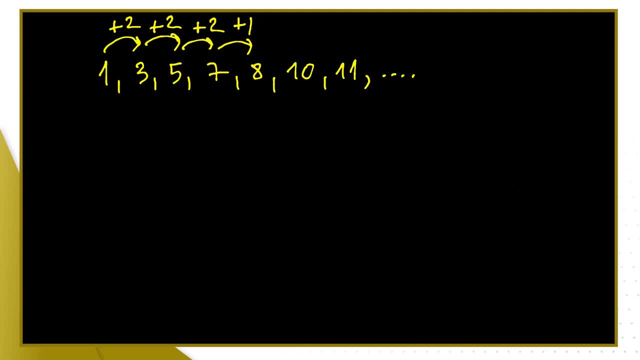 69,, 69,, 7,, 8,, 10,, 11, and so on. What do you think? Is this an arithmetic progression every time? so this isn't an arithmetic progression And you can prove it by just. 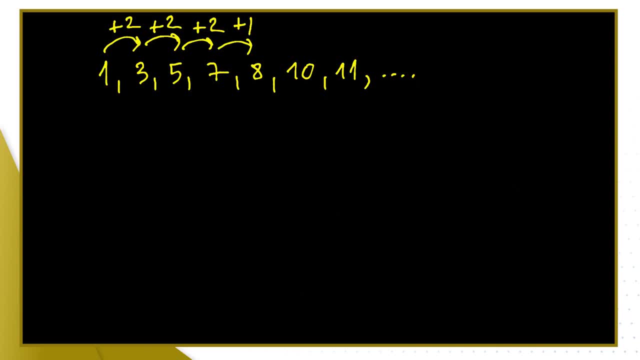 saying the common differences don't match. So you can say this is a1, a2, a3, a4, a5.. You can say a5 minus a4 is 1, but a2 minus 1 is 2.. These aren't the same. 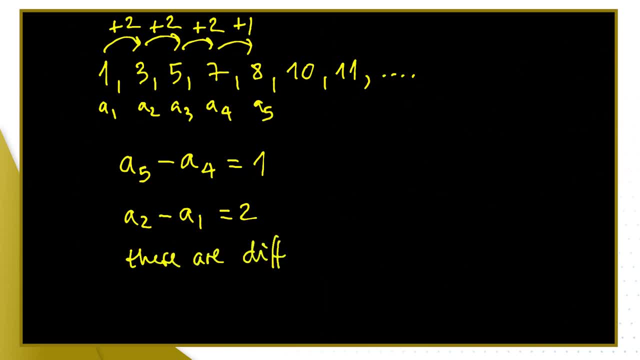 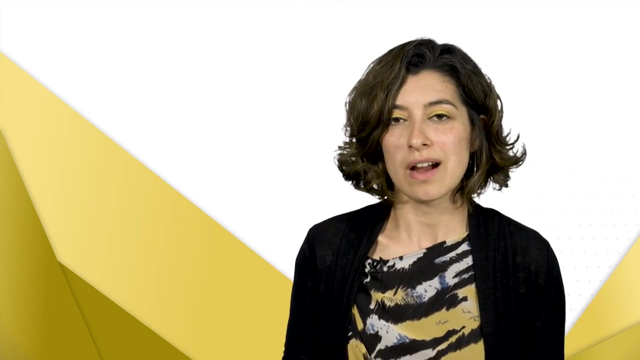 these are different. Therefore there isn't a common difference. And if there isn't a common difference, then we don't have an arithmetic progression. Now, the first example we saw was an increasing arithmetic progression. We can have Common differences that are negative. we can have 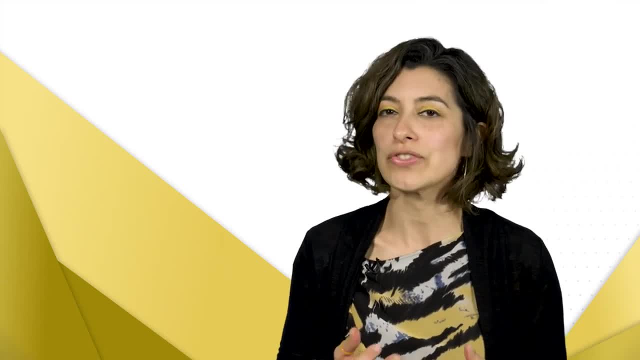 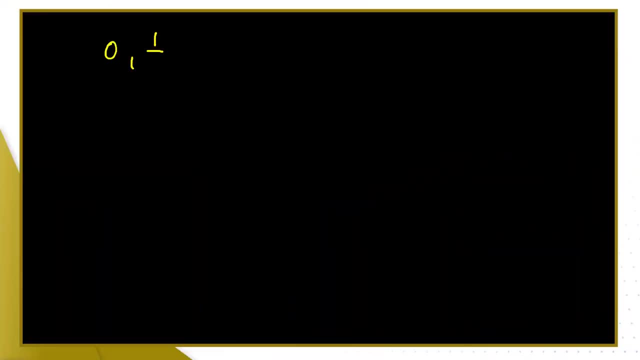 Common differences that are fractional. we can have Any common difference as such, as long it is the same difference over and over again. So 0, 1 half 1, 1 and a half 2, and so on. 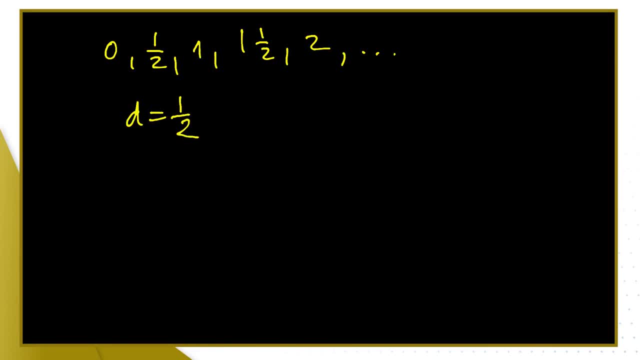 Common difference 1 half. That's an arithmetic progression. The expression would be: a n is 0 and n minus 1 times 1 half, which I can just tidy up as n minus 1 over 2.. That is an arithmetic progression. 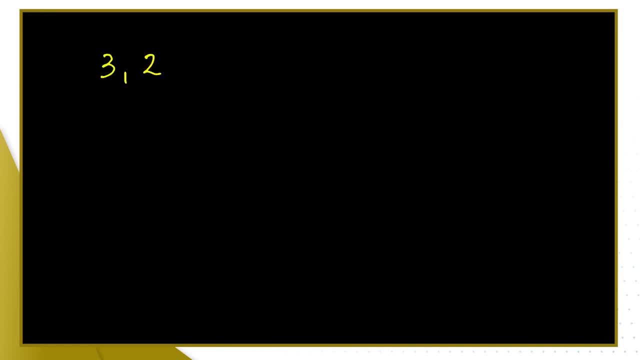 For example 3,, 2,, 1,, 0, minus 1, and so on. The common difference is minus 1.. So d is minus 1.. Because it is a2 minus a1 is 2, take away 3,, which is minus 1.. 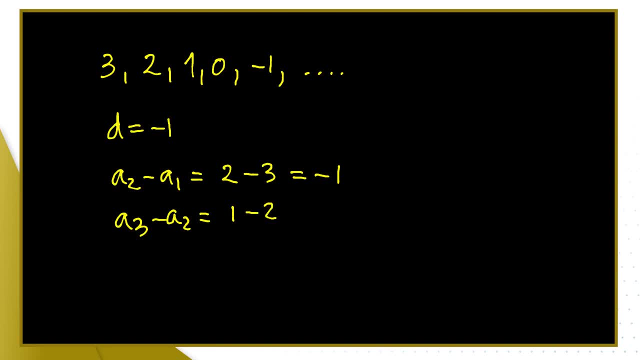 a3 minus a2 is 1 minus 2,, which is minus 1, and so on, And the first term is 3.. So the general term is: a n equals 3 plus minus 1, times n minus 1.. The common difference times n minus 1.. 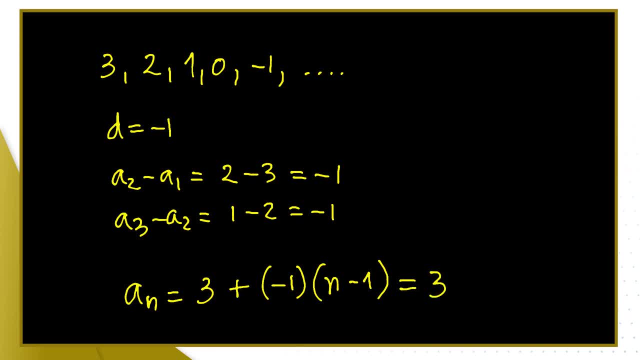 And this comes as 3. Minus n plus 1, which is just 4 minus n. You can check: Just replace n by 1,, 2,, 3,, 4,, 5, and so on and see the results. 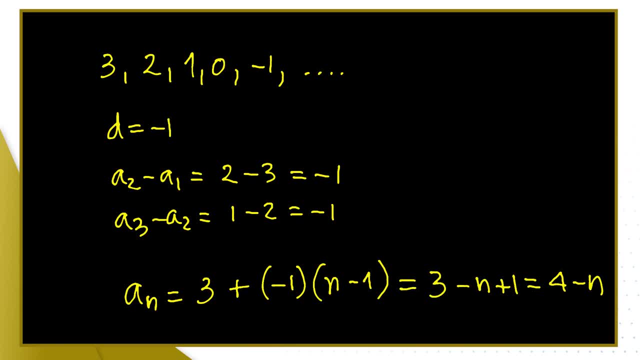 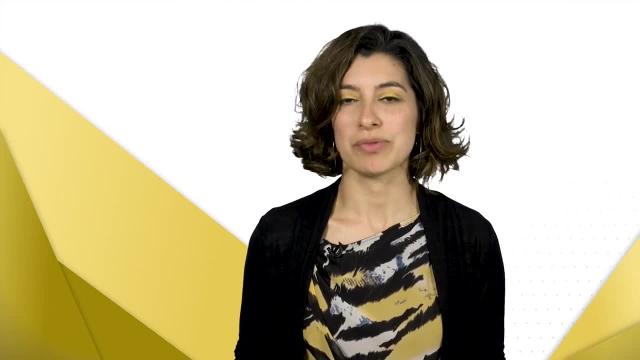 When n is 1,, you've got 4 minus 1, that's 3.. When n is 2,, you've got 4 minus 2, that's 2, and so on. In summary, there's two ways we can define arithmetic progressions. 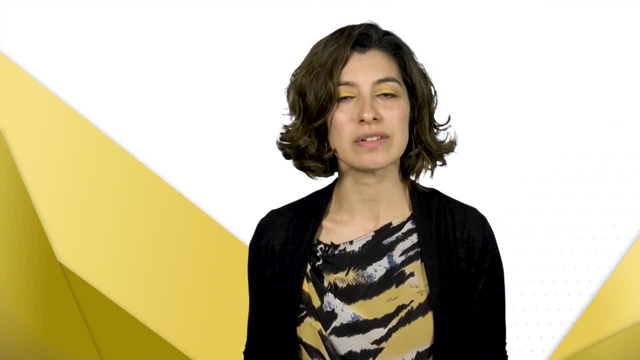 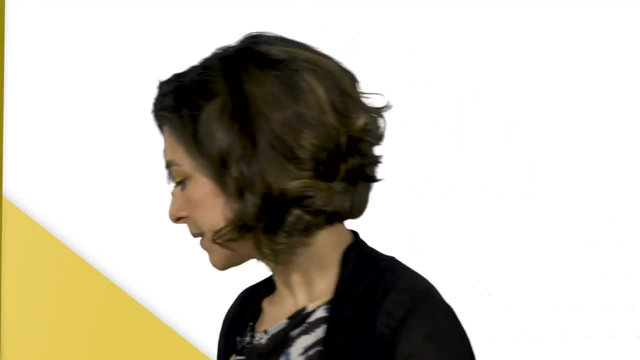 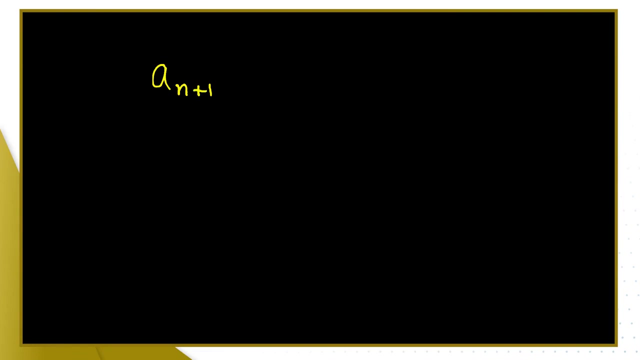 By writing out its recurrence relation or by giving the general term. They both need the knowledge of the common difference. I'll write them here. As a recurrence relation, it would be that a n plus 1, the next term is a n. add the common difference. 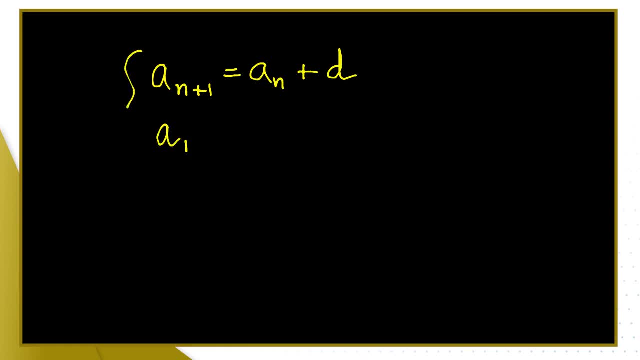 And we need to make explicit what the first term is. The general term is given as a, n being the first term, adding the common difference Not quite n times, but n minus 1 times. So you can either use this one or the other one. 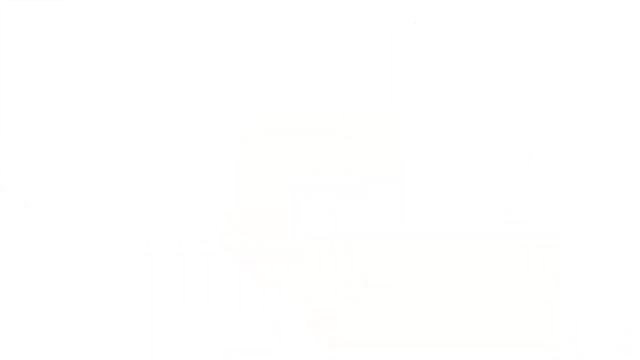 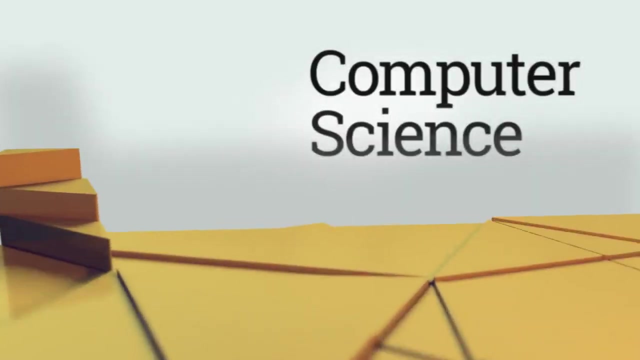 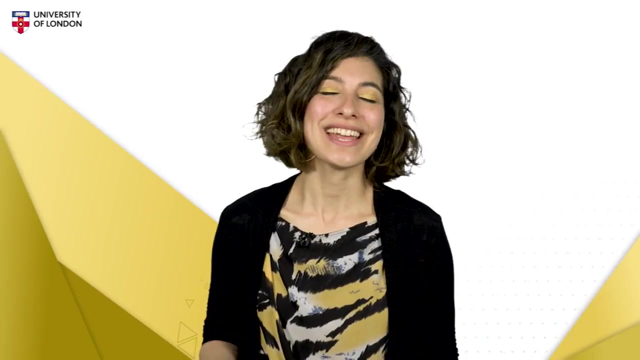 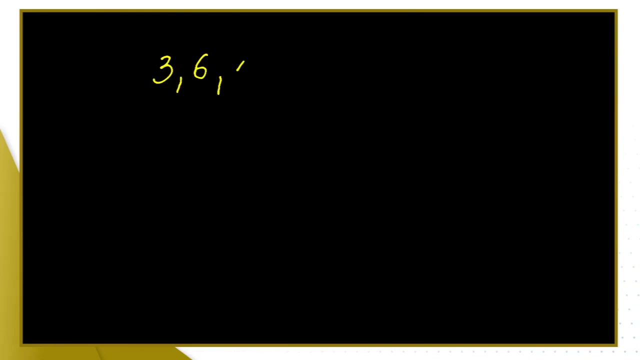 And that's arithmetic progressions. We're going to look at another special type of sequence. Say, we've got 3, 6, 12,, 24,, 48, and so on. I think that was enough to see the pattern. 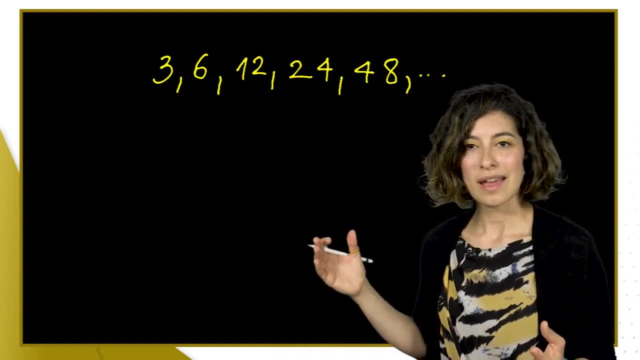 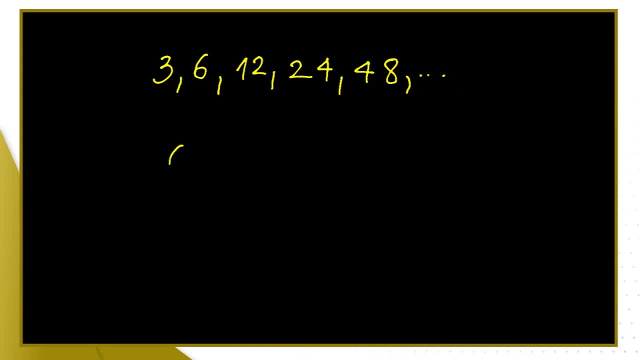 It is a doubling sequence And I mean that any new term can be computed from the previous term by multiplying by 2, by doubling That means that I can say that if my sequence is called a, a new term for a is twice the previous term. 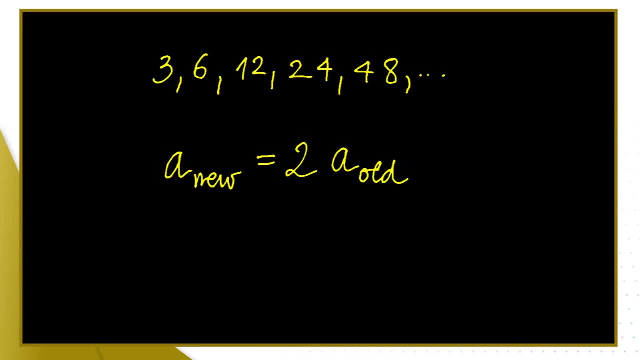 Let's say the old term. Let's write that more mathematically: The new term is the term of order n. The previous term is the term of order n minus 1.. And so the new term is computed by doubling the previous. 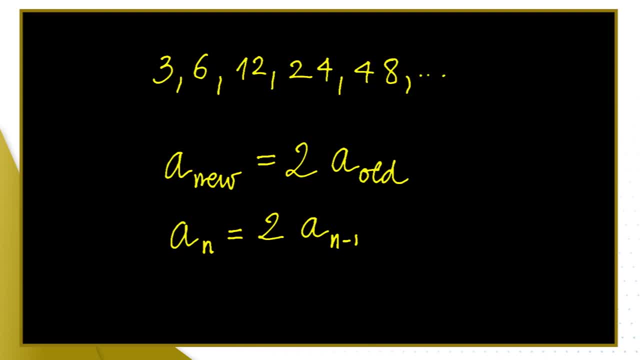 That expression isn't enough to totally define the sequence I've written. Any doubling sequence would be, So I need to define what's the first term. This is how we define sequences given by a recurrence relation, as we've seen earlier. So the first term in this case is 3.. 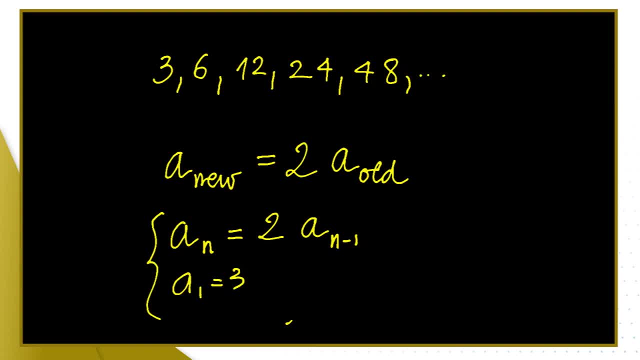 So these two together define this special sequence. So these two together define this special sequence. This is called a geometric progression, And it is so because any new term is computed by multiplying the previous by a common ratio. The common ratio for this one is 2.. 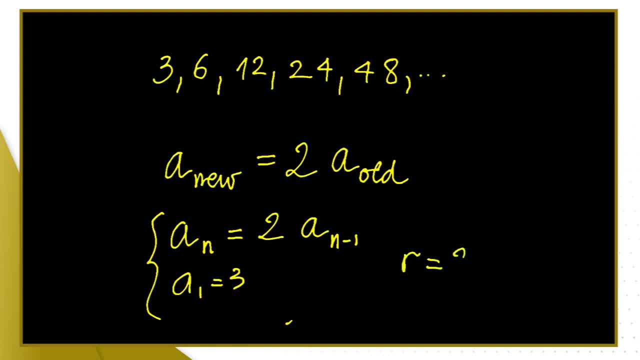 So I'll say: the common ratio, usually denoted as r, is 2 for this sequence. Now you might be wondering: can we do better than this? Can we write an explicit formula for the term a? n? Can we write an explicit formula for the term a? n? 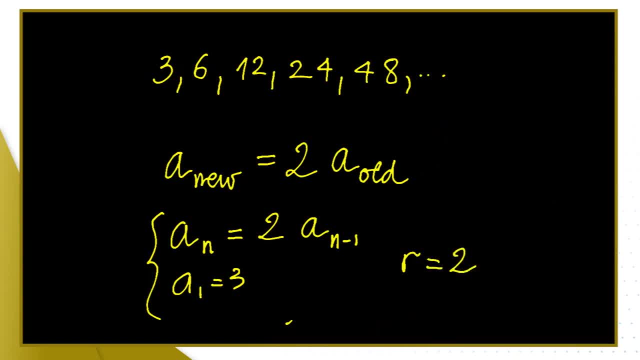 Yes, we can. Let's look at it. So the first term term of order 1, is 3.. The second term we said it is doubling the previous one, So it's 2 times the 3,, which is 2 times the a2, right? 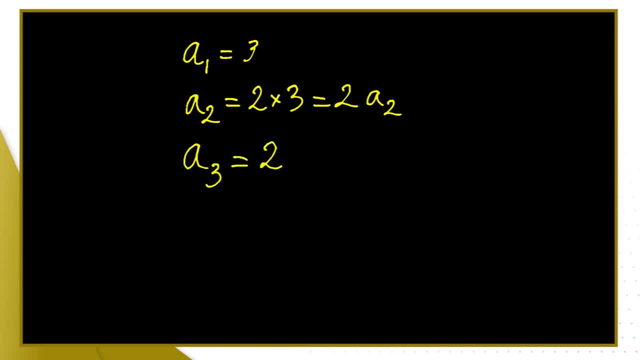 And then the next one is twice the previous, which is twice the 2 times 3.. And the next one will be twice the previous, so twice the 2 times 2 times 3.. And it carries on like that. You're probably spotting the pattern. 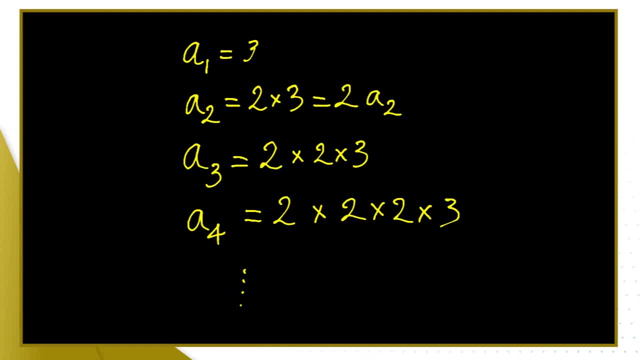 We have powers of 2 over and over again. So here on a4, I've got three 2s multiplying together, So that's 2 to the cube times 3.. The previous one, a3, I've got two 2s. 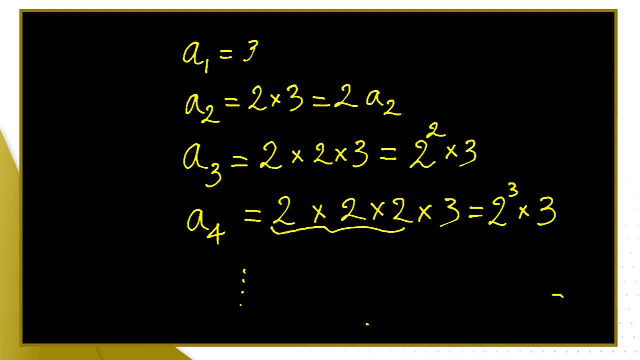 So I've got 2 squared Times 3.. And a2 is just 2 to the 1 times 3.. And if we want, we can write here that it's 2 to the 0 times 3.. Because 2 to the 0 is 1.. 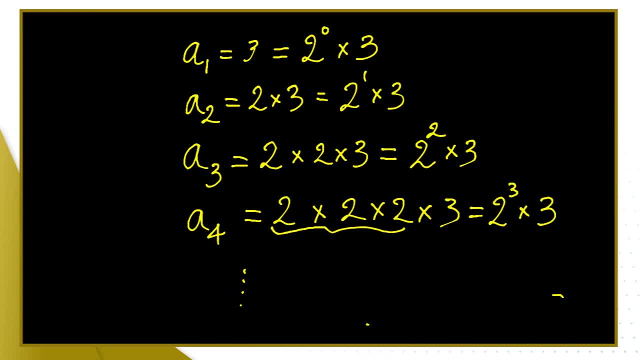 And this pattern can be extended to the general term. So I can say that term of order n is going to be a power of 2 times 3.. How many powers of 2?? Is it n or is it less? Let's look. 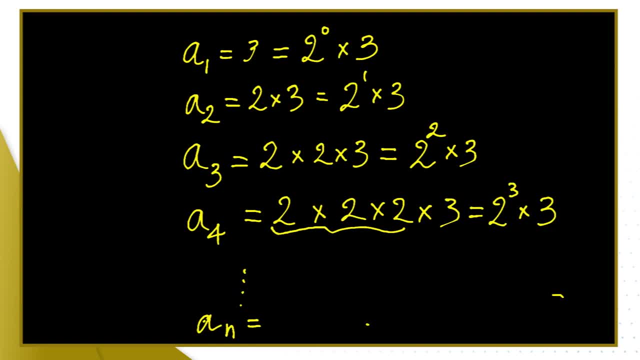 For a4, I've got 2 to the 3. So one less than the number 4. And therefore I have 2 to the n minus 1 times 3. Which might be a bit more elegant to write in this way. 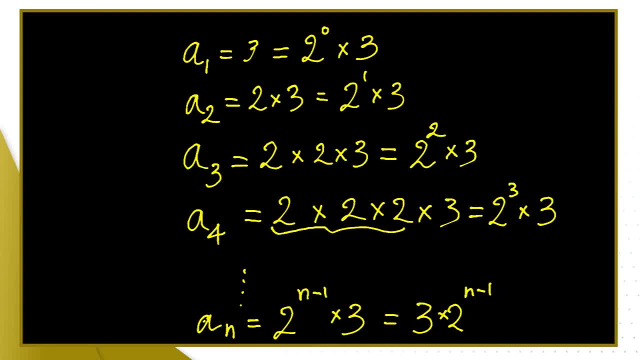 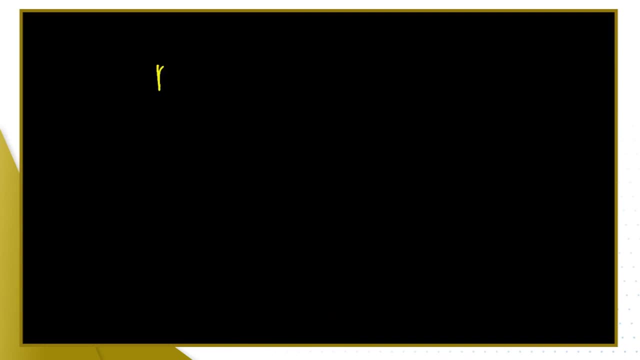 Okay, So n3 is the first term of the sequence, And then I times it by 2 to the power of n minus 1.. And that gives me the term of order, n For any ratio, r, So that's the common ratio. 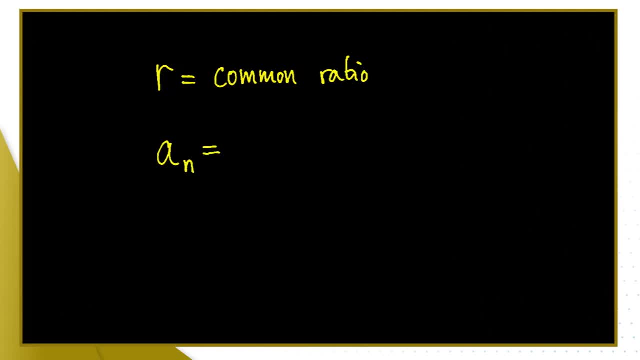 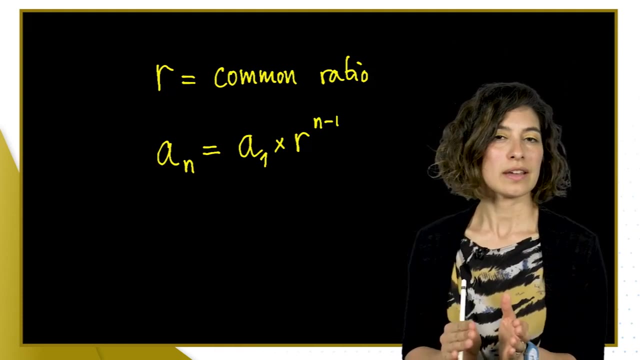 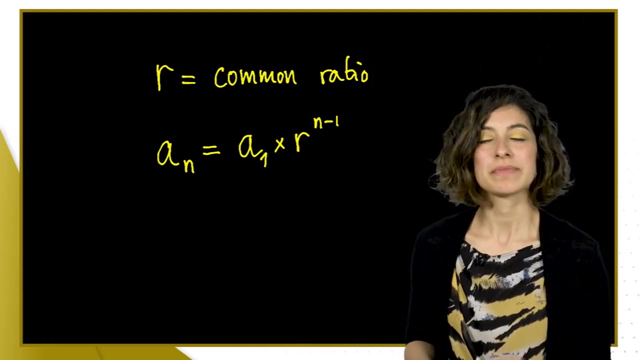 The general term of the geometric progression will be a1, the first term times r to a certain power. And remember, it is one less than the n, So n minus 1.. Just a little note to say: How do we check that? the sequence we have in front of us? it is really a geometric progression. 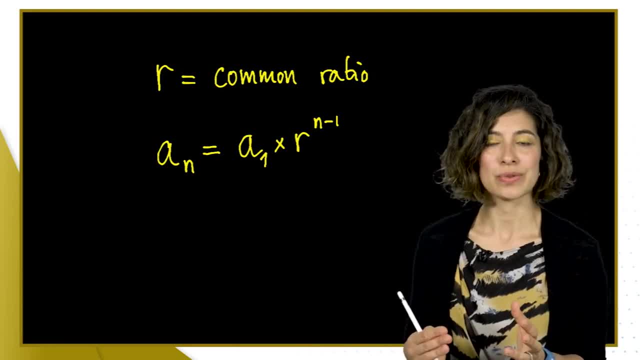 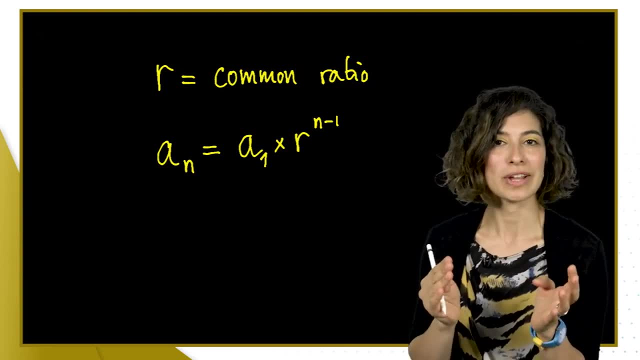 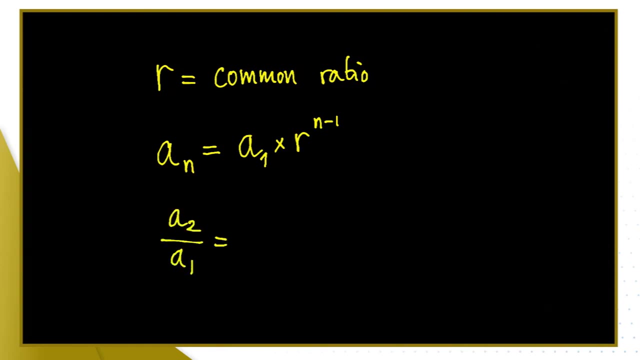 The key thing is that there is a common ratio And that means that the ratio between consecutive terms of the sequence is the same number over and over again. So I look at a2 over a1. Which was a2 was 6 and a1 was 3.. 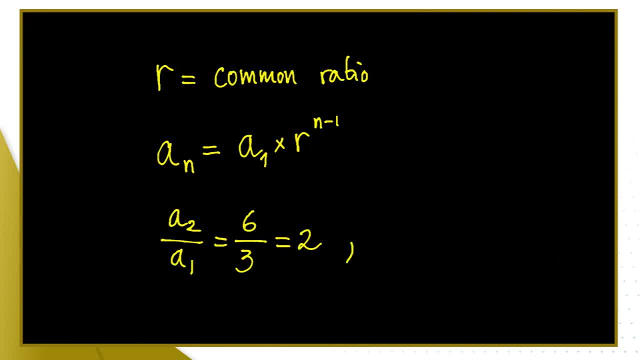 So that ratio is 2.. I also need to look at the next pair, So a3 and a2.. So a3 divided by a2. And that is 12 divided by 6. So that's 2.. And so on. 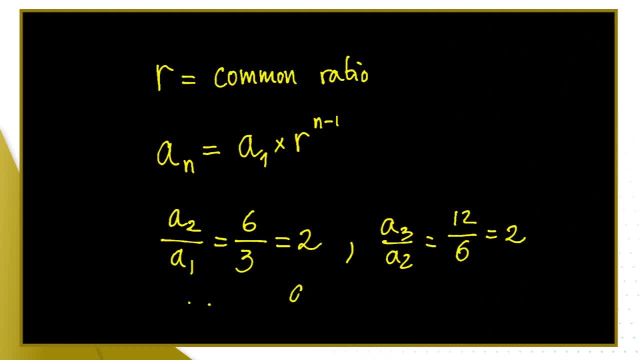 For this sequence, it is true that a to the n plus 1 over a to the n is always 2.. Which is the common ratio r. Let's look at another example, The sequence 1,, 3,, 9,, 18,, 27 and so on. 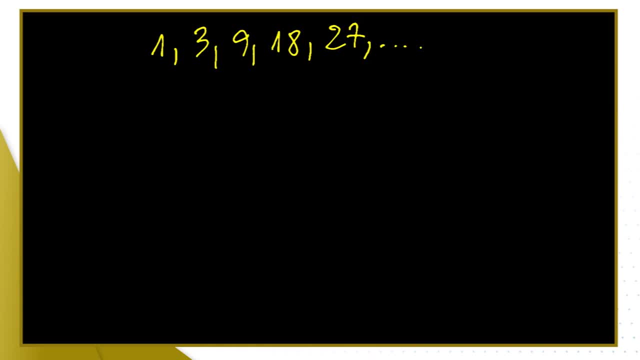 Is this a geometric progression? We're going to check if there is a common ratio. We're going to look at ratios of consecutive terms. We do the second term over the first, So we do 3 over 1.. That is 3.. 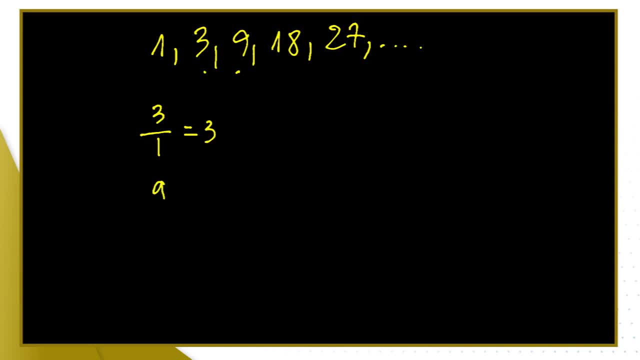 We now do the third over the second, So 9 over 3.. That is 3.. Now we look at 18 over 9.. 18 over 9.. That is 2.. This is not the same number. Therefore it's not a geometric progression. 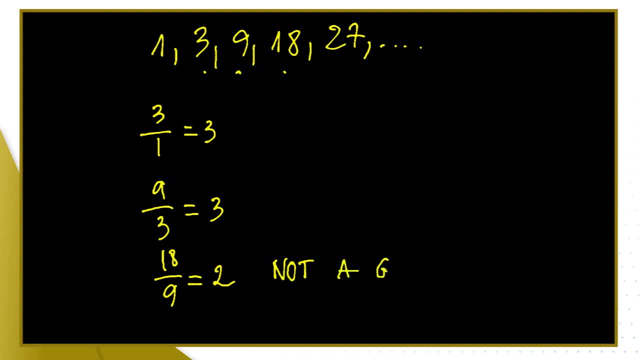 So not a geometric progression, Because the common ratio needs to be common. Let's look at another one. We have 9, 3, 1.. 3, 1, 1 third, 1, ninth, 1 over 27, and so on. 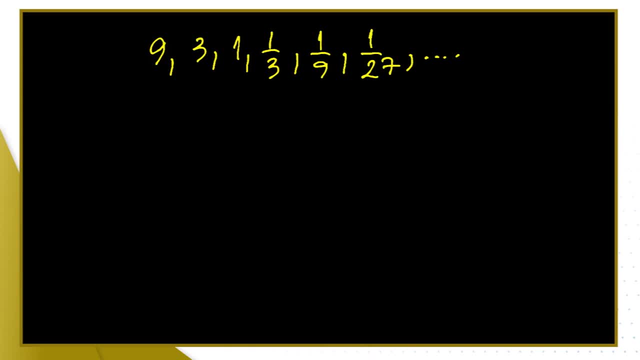 What is the pattern here? From one term to the next, I'm multiplying by a third, Or I'm dividing by 3, whatever you like to say, And so on. And that matches. Well, I wrote there that it's. 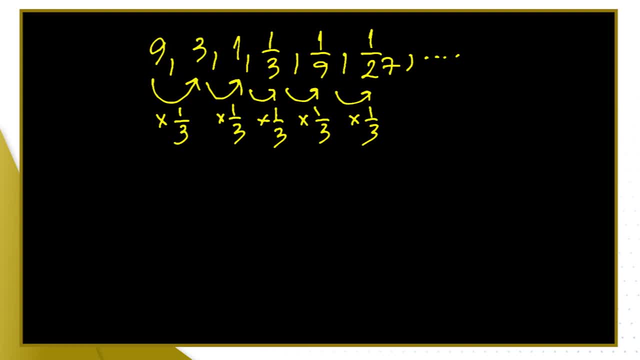 I multiply by a third every time. You could check once again by doing the ratio I explained earlier. So we would do: 3 over 9 is the same as 1 over 3.. It's the same as 1 third over 1.. 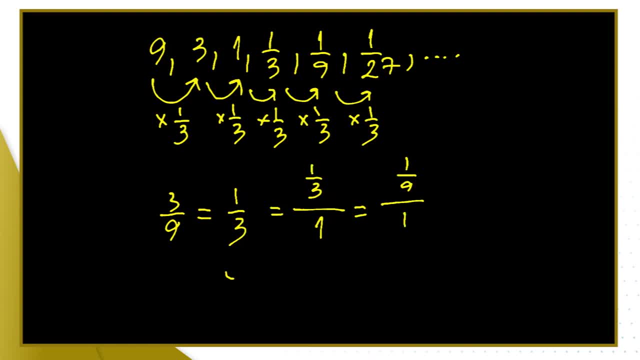 It's the same as 1 over 9 over 1 third, And so on. It's always 1 third And that's our common ratio. If you found the fraction over fraction a little bit confusing, I'll just do a quick recap on that. 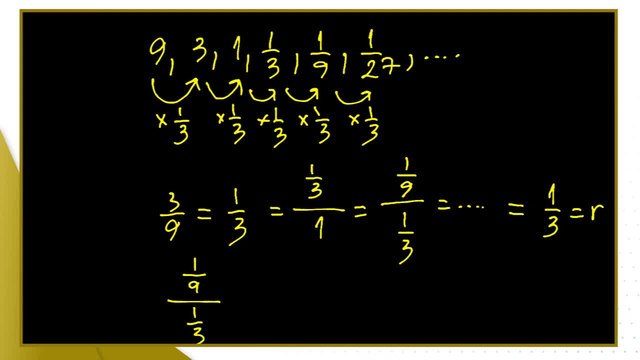 1 over 9 over 1 third is 1 over 9 divided by 1 third, which to divide fractions, we turn that into a multiplication of the reversed fraction, And so you do 3 over 9, which is 1 third. 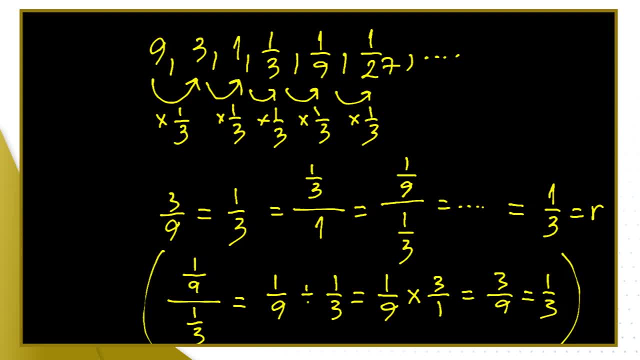 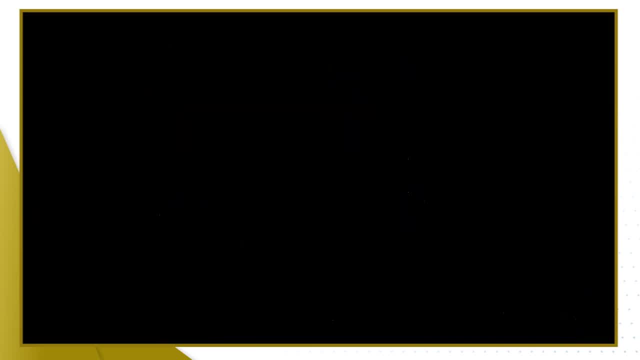 OK, Now we have a common ratio of a third. Let's write the expression for this geometric progression. So let's call that sequence b. So bn will be the first term, which was 9, times the common ratio, which is 1 third to the power of n minus 1.. 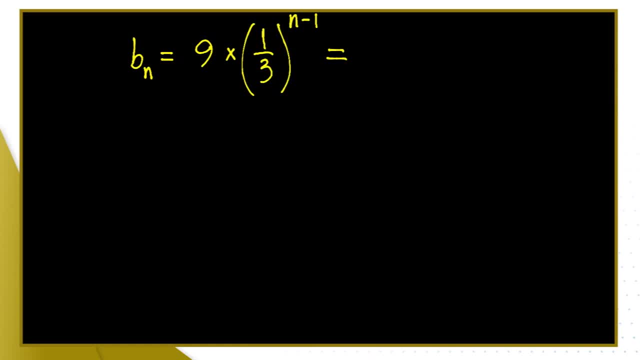 Now we can tidy this up a bit, because 9 is also a power of 3.. So this can be 3 squared from the 9 over 3 to the n minus 1.. And that comes from the fact that 1 third to the power of f minus 1. 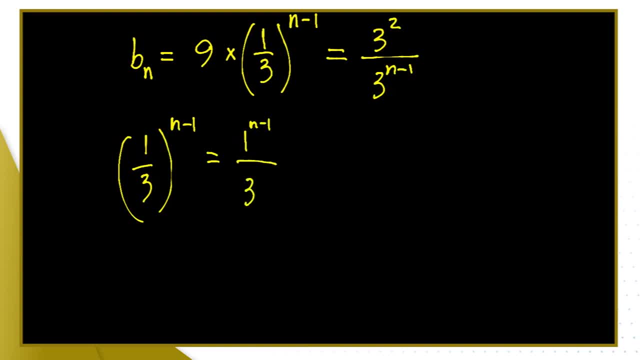 is 1 to the power of n minus 1 over 3 to the power of n minus 1.. And 1 to any power is just 1.. So this is 1 over 3 to the n minus 1.. OK, So just a little side comment for you, if you need that. 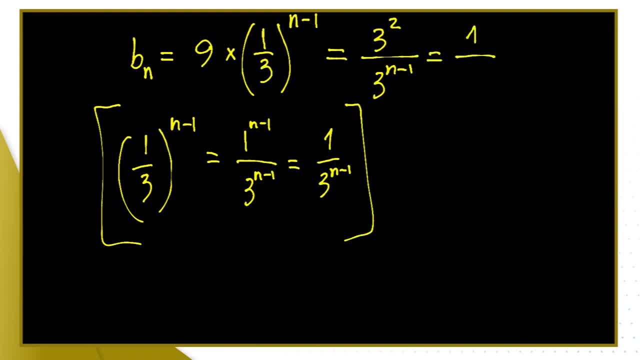 And now rules of powers. Just say that I will do 3 to the n minus 1.. Take away the 2 on the top, So n minus 3.. OK, And if I want, I can write in this way as well. 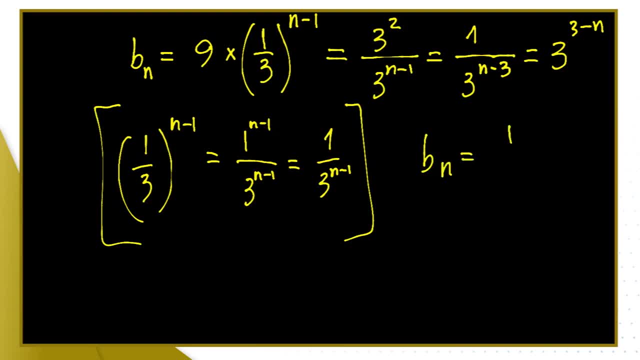 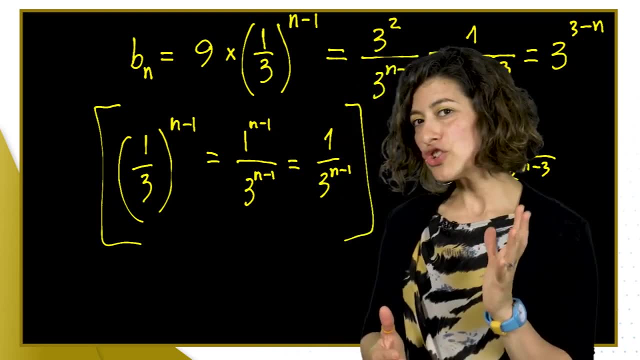 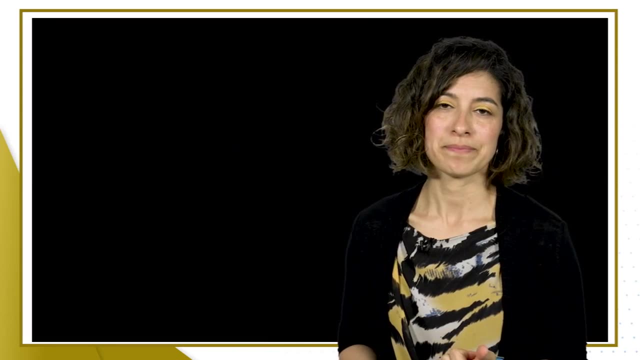 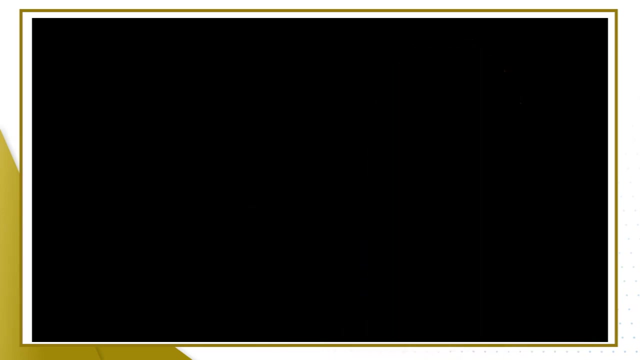 But I'll be really happy with a result written as that. I've got a question for you. Say we have a geometric progression with common ratio 4 and first term 1.. Is 1000 a term in this geometric progression? Let's check it. 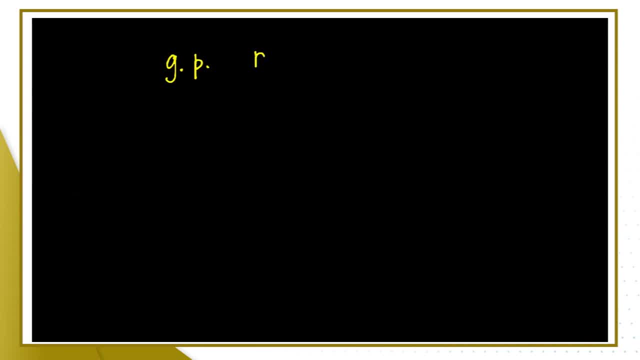 So I've got a geometric progression with ratio 4. And first term, so let me call it a1, 1. And I want to know if 1000 is a term in this sequence, Is there any n such that 1000 equals it? 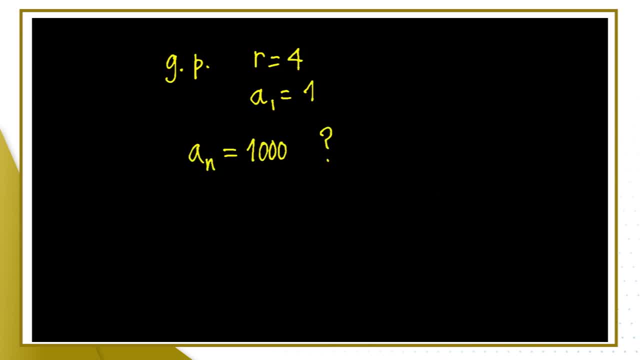 Is it possible? Let's solve the equation, The equation that involves the general term of the geometric progression. So from here I know that a n should be 1 times 4 to the power of n minus 1.. OK, So is there an n such that 4 to this power is 1000?? 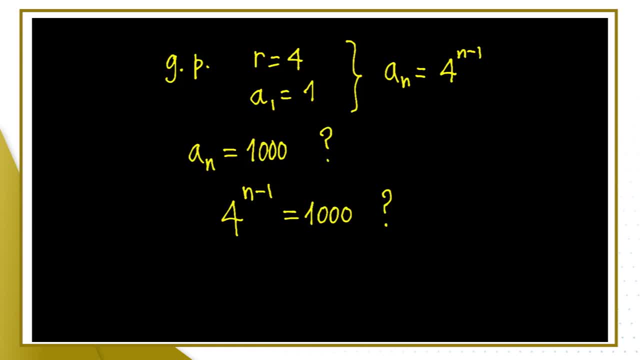 In other words, is 1000 a power of 4? It is not. You can check through the calculator. You can run all the first powers of 4. And 1000 isn't one of them. Run through the powers of 4.. 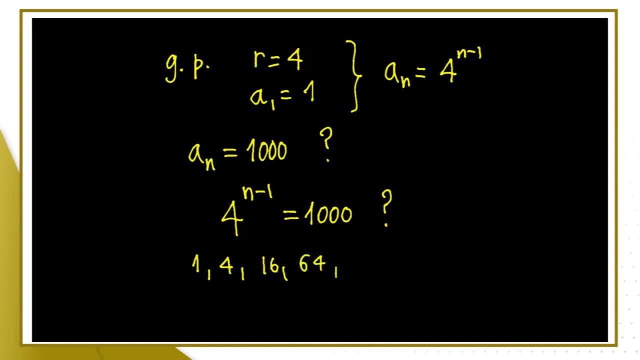 Get 1,, 4,, 16,, 64,, 128.. And you carry on multiplying by 4.. You will never get to 1000.. So there is no such n And therefore 1000 is not in this sequence. 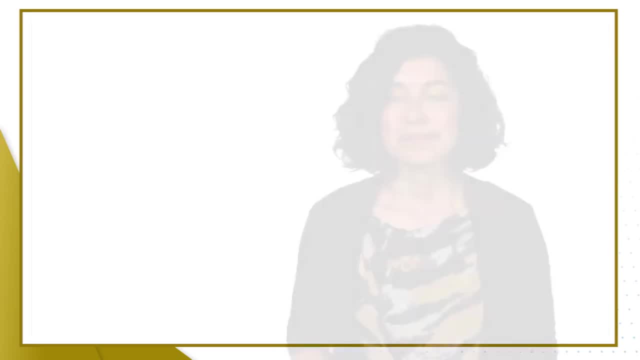 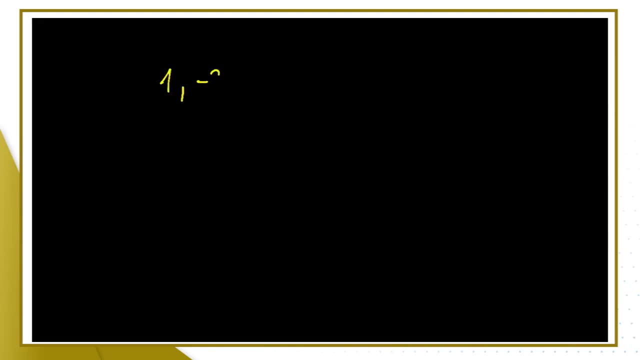 It's not in the sequence a- n. The ratio of a geometric progression can also be negative, For example the sequence 1, minus 2,, 4, minus 8,, 16, minus 32, and so on. The common ratio is negative 2.. 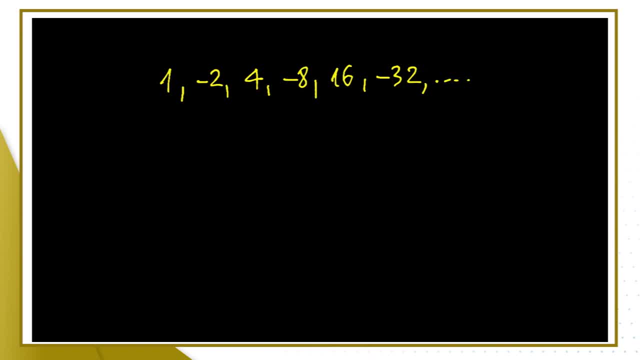 So the terms alternate between a positive and a negative number. A negative common ratio can also be a fraction, For example the sequence 1 third minus 1 over 9,, 1 over 27, minus 1 over 8, and so on. 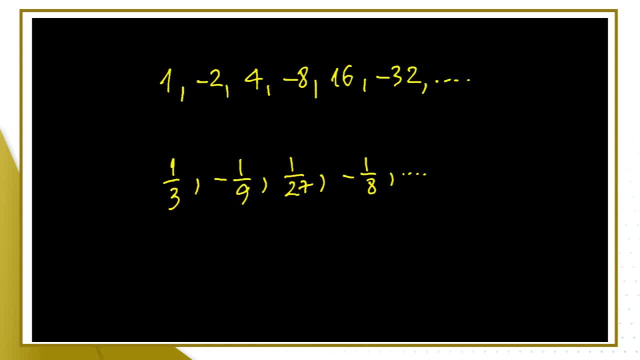 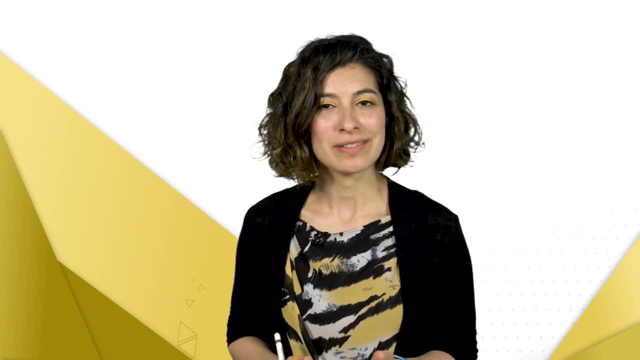 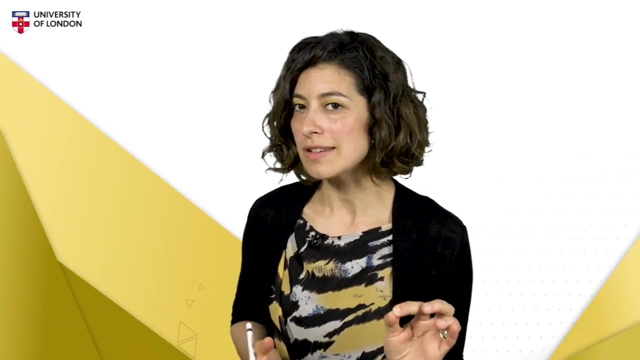 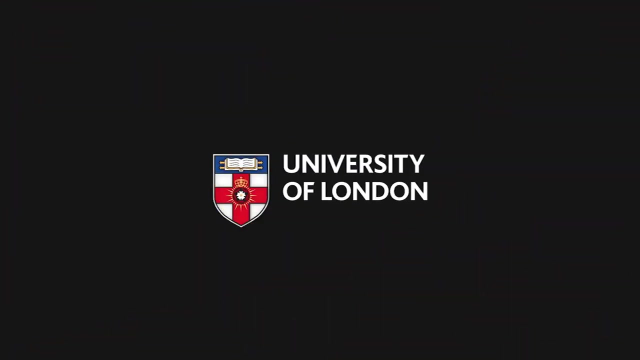 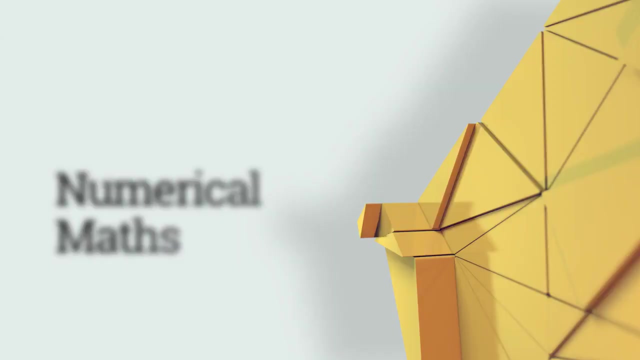 is a geometric progression of common ratio minus 1 third. I leave you with a question: How do you imagine geometric progressions behaving as n grows larger and larger? I give you a hint: It depends on the type of common ratio. Modular arithmetic is a tool used. 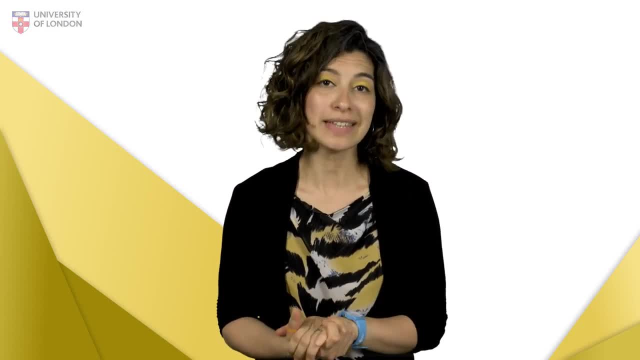 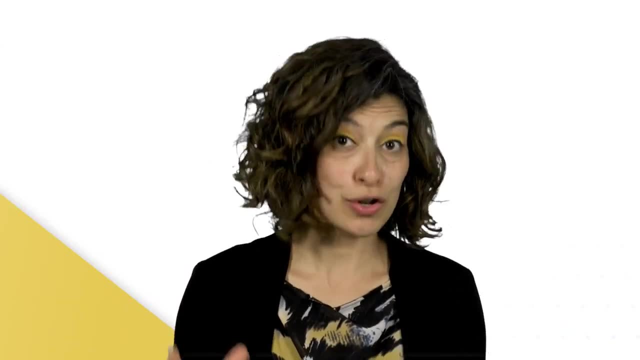 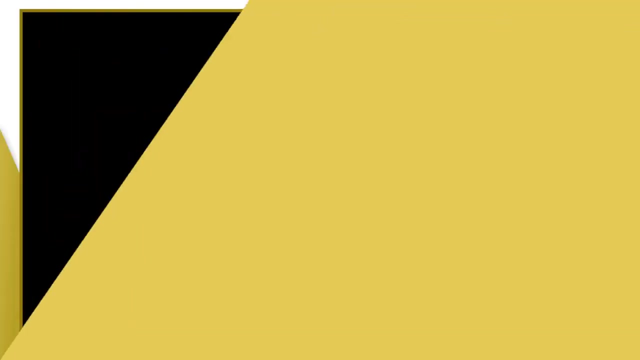 in one of the most popular methods for generating sequences of numbers that appear random. Here's the setup: We're going to use modular arithmetic And we're going to choose a modulus, a multiplier, an increment and a seed value. I'll show you. 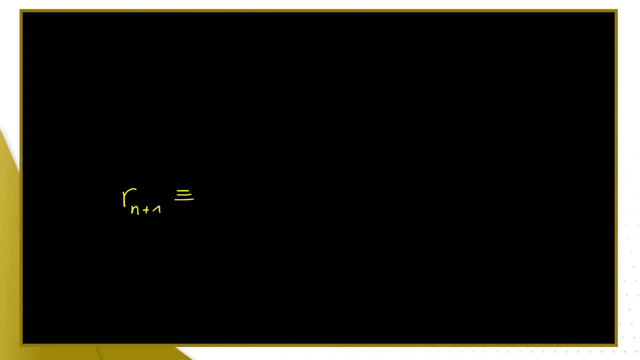 So we're going to use a recurrence relation. So I'm going to write that my next random number- r n plus 1, is congruent with m times r n, which is the previous number plus an increment i mod c. 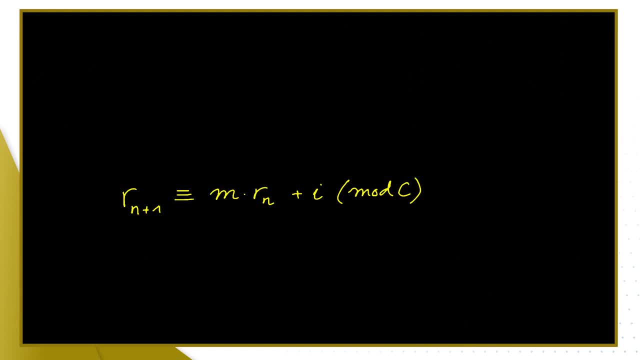 the modulus for this particular method. Now, c needs to be a positive number, That's the modulus. m is going to be the multiplier, i will be the increment, And our seed value, r zero has to be between zero and the modulus. 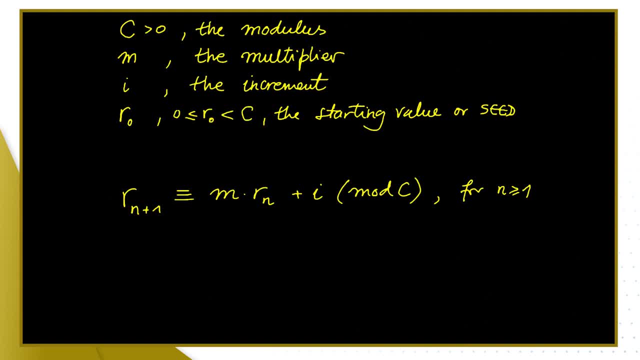 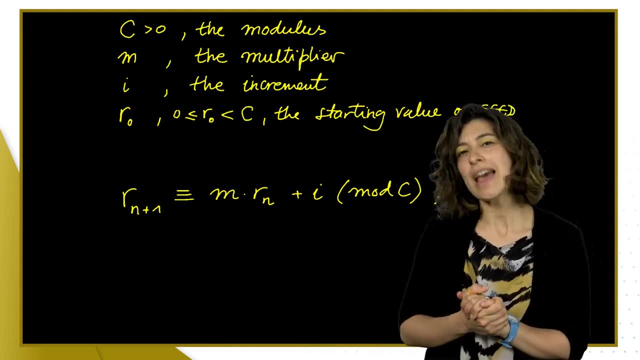 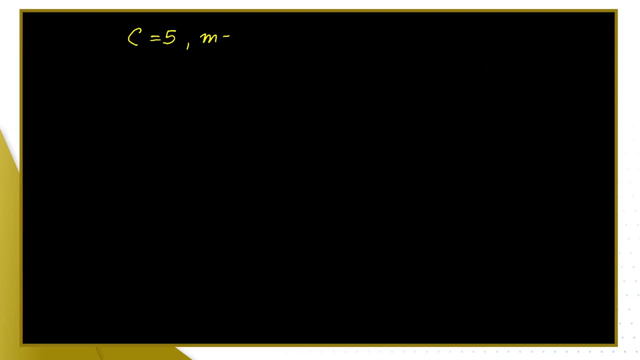 but less than the modulus. So this will be my formula for generating random numbers. But let's see how random they really are. In this example, I'm going to choose the modulus to be 5.. The multiplier will be 1.. The increment will be 1.. 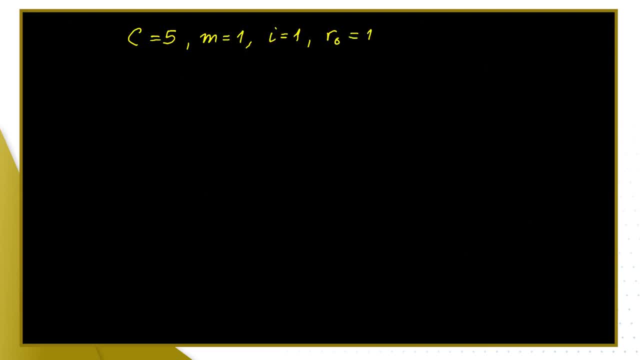 And we'll have a seed value of 1 as well, And so my expression boils down to the next random number: r n plus 1, will be congruent with r n add 1, mod 5.. So I'm going to add 1 to the previous value, mod 5.. 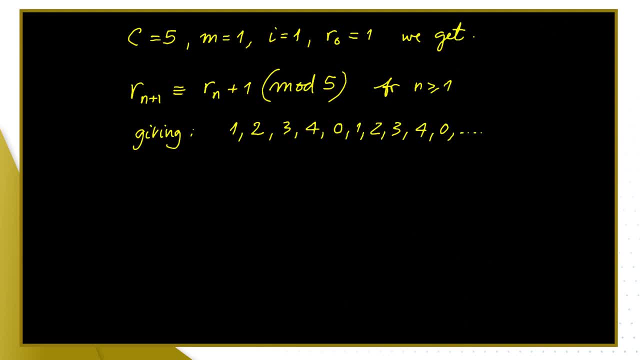 What do I get? Well, if I start with 1,, the next number will be 2,, then 3,, then 4, and then- haha, not 5,- 0,, then 1, and 2, and 3,. 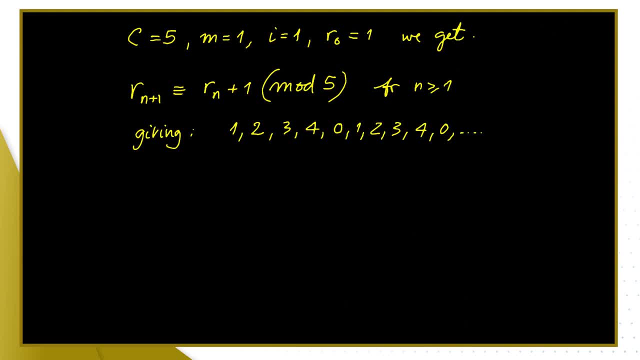 and 4, and 0, and so on. Yeah, it's not very random looking. Let's look at another instance. We keep the modulus 5.. We're going to up the multiplier to 2 and the increment to 2 as well. 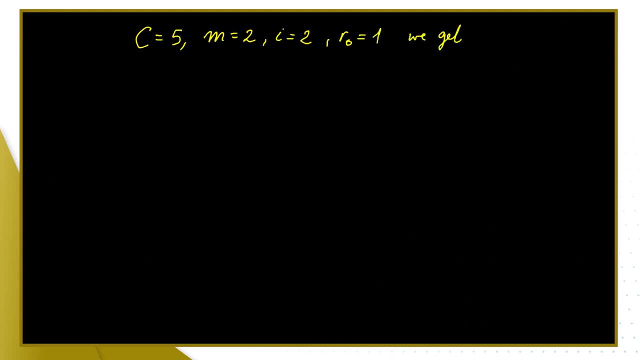 And let's have 1 as the seed value, So we're going to get my expression. So next random number will be twice the previous, add 2, mod 5.. Let's see what we get. We start with 1,. 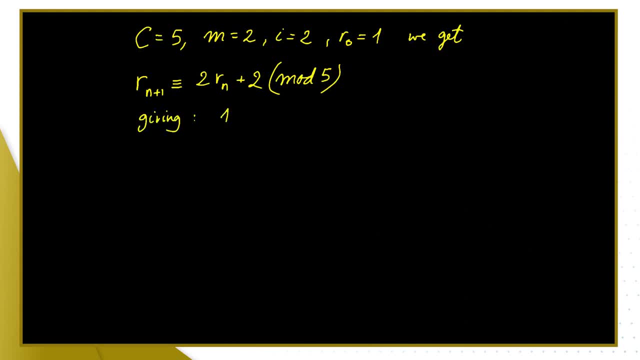 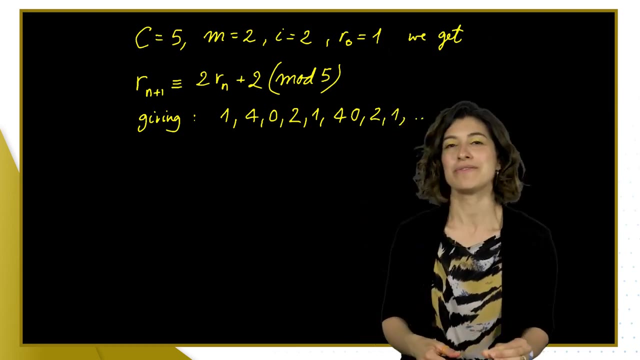 and then we get 4,, 0,, 2, then 1,, 4,, 0,, 2 again and 1, and we'll be repeating. It's a little bit better, but it's still not very random. 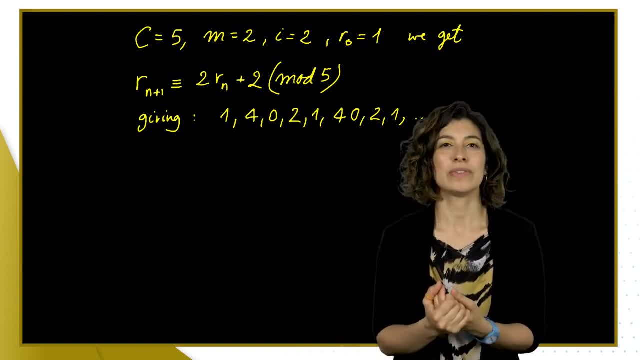 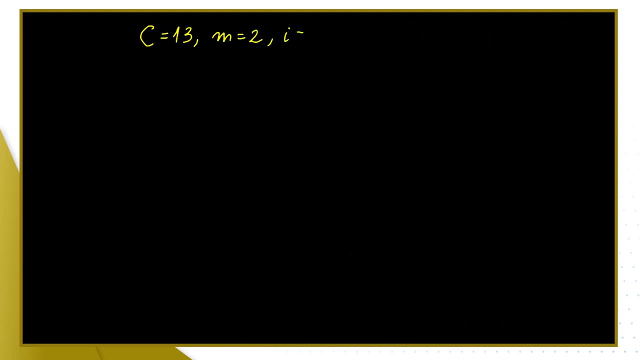 What should we do? How do we make these sequences more random? Well, let's try another example. You will play with it, but let's try with different modulus. Let's go for modulus 13.. Yeah, let's do doubling. 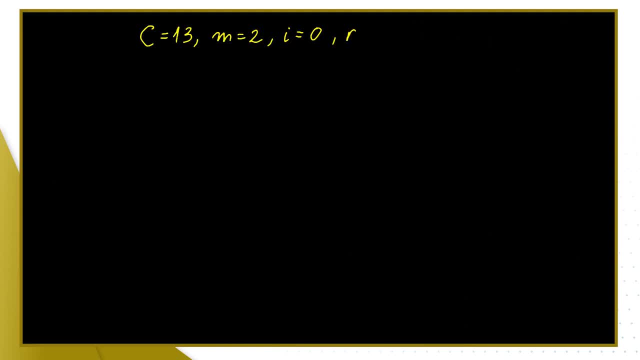 Let's have a multiplier of 2,, an increment of 0, and start with the seed of 1.. Now do this one. Do this one yourself. I'm going to write the expression. It will boil down to doubling mod 13,. 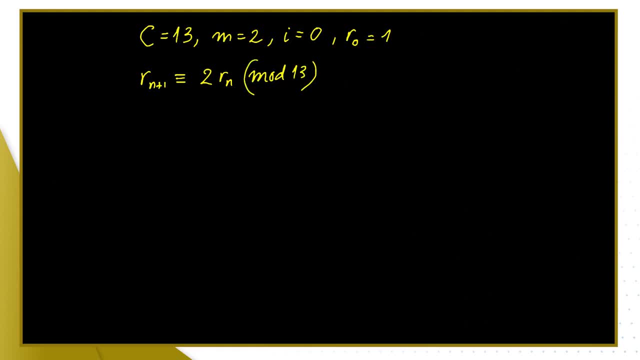 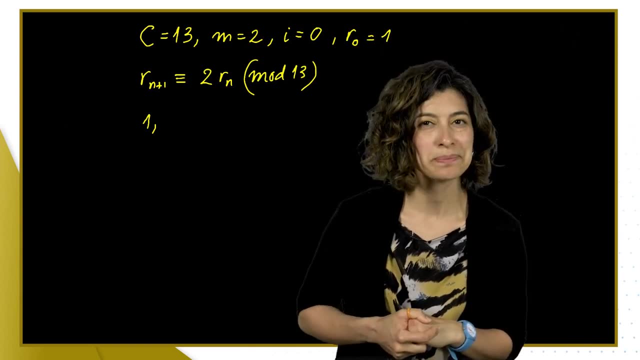 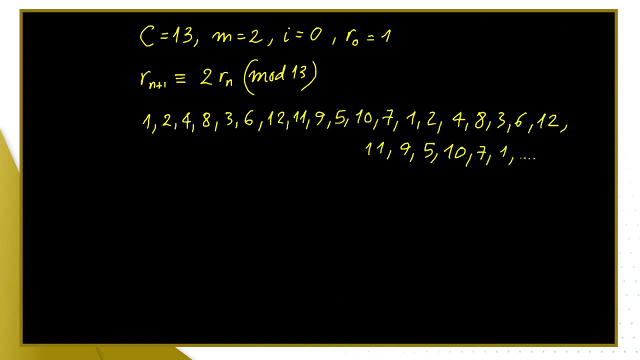 and we start with seed 1.. What do we get? Take your time, Do a few calculations, Write it down. Okay, let's have a look at the results. It takes a bit longer to repeat the pattern, doesn't it? 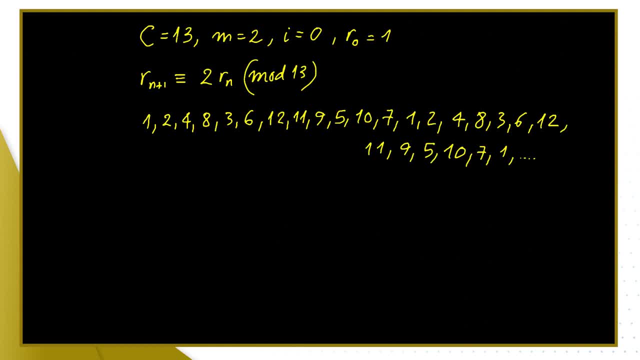 Does it look a little bit more random to you? We still go 1,, 2,, 4,, 8, clearly a doubling- and then 3,, 6,, 12,, 11.. I would like to know your comments. 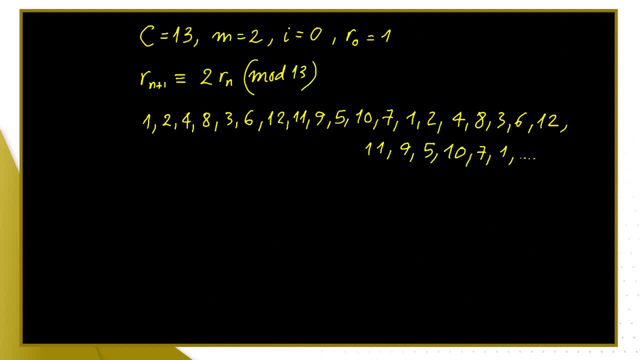 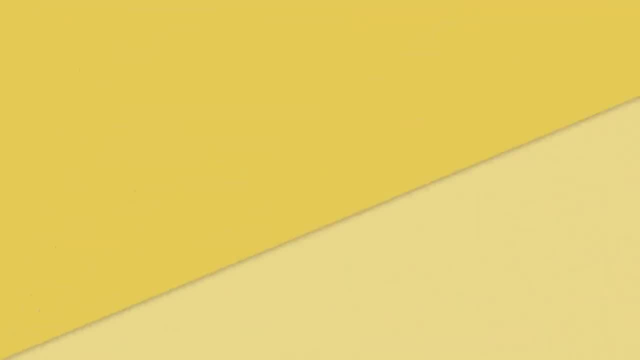 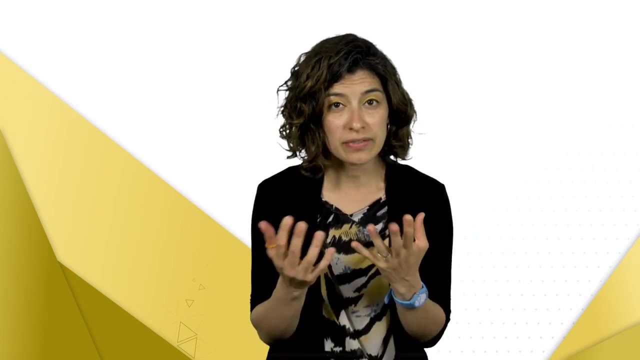 and do share your ideas in the discussion forum. Now, the task you will work on next is self-assessed, but the summative assessment will refer to things you can only understand if you have performed the task to a satisfactory level. So what will happen is: 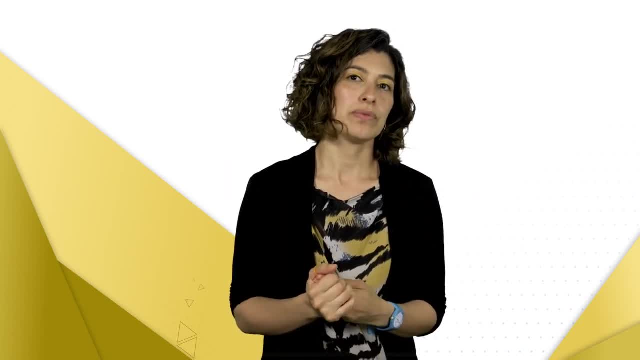 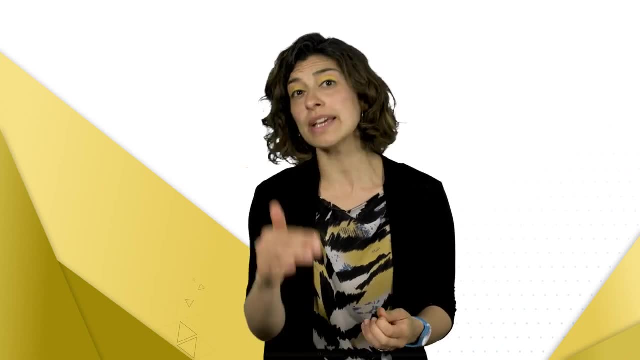 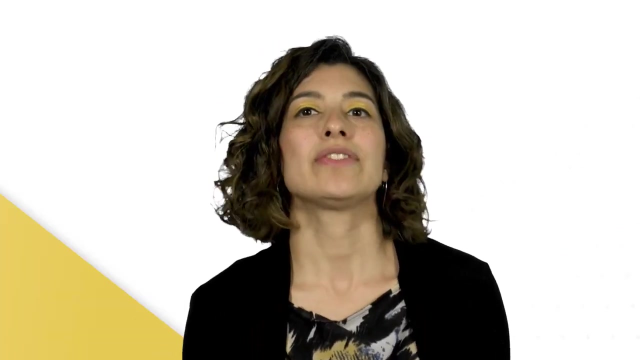 we will look at the examples. we've done before and I wanted to explain why the numbers repeat, why they are periodic, and I would like you to use as much of mathematical statements as you can. I also wanted to make it explicit what is the period of repetition. 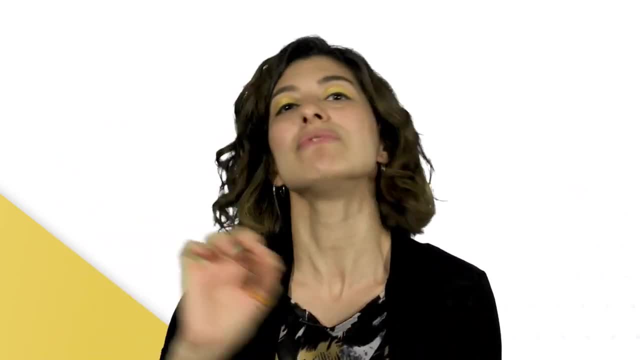 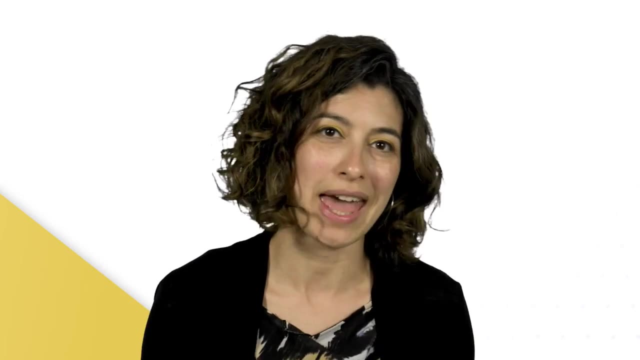 so the length in terms of the parameters. So I wanted to relate that to the values of the modulus, the multiplier, the increment, and do that as much as you can Now using the same formulae we've given you before. 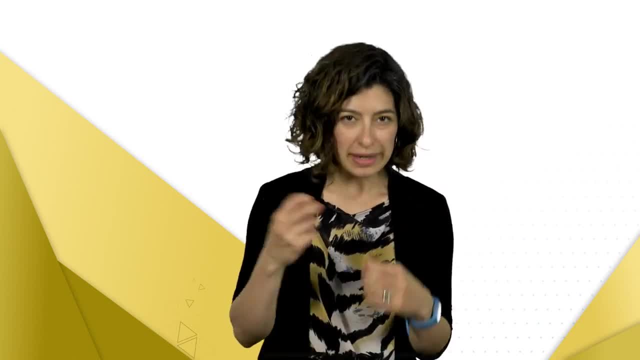 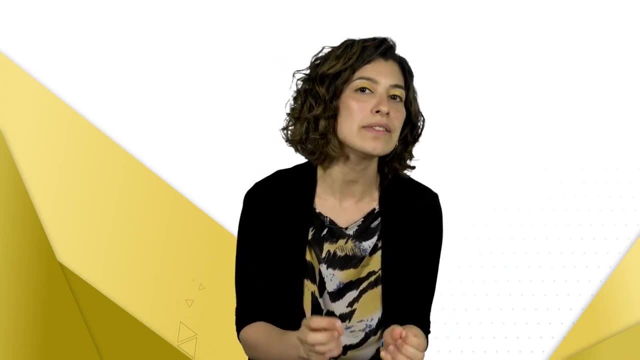 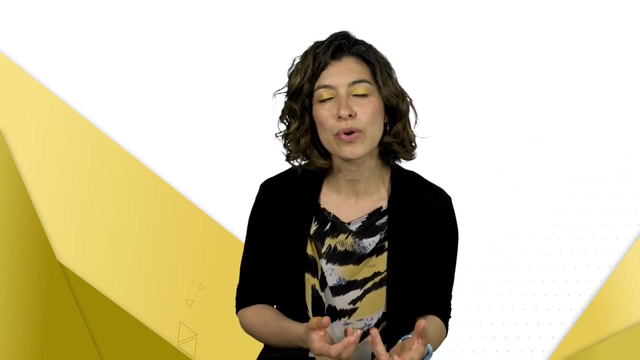 I'd like you to write sequences of numbers by changing the parameters. but I'll be a bit more specific. I'd like you to try at least 10 different sets of parameters, So do also work with the ones I've given you before. 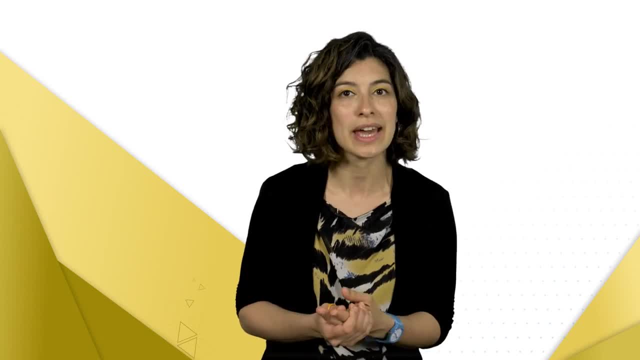 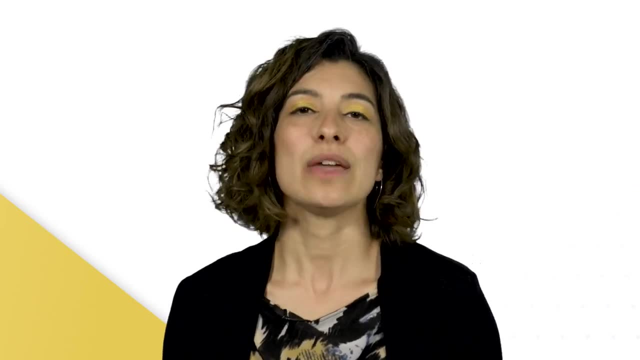 but those will not be included in this count of 10,. okay, And then, in terms of how long should you go for in calculating the terms of a sequence? it will be at least 2 times c terms, So for c equals 13,. 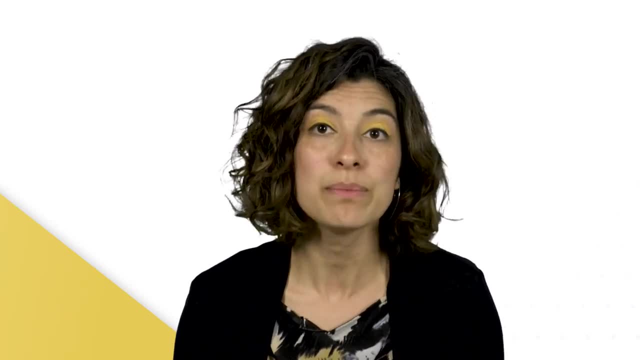 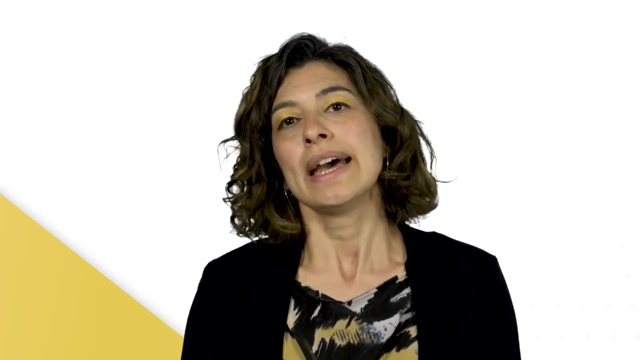 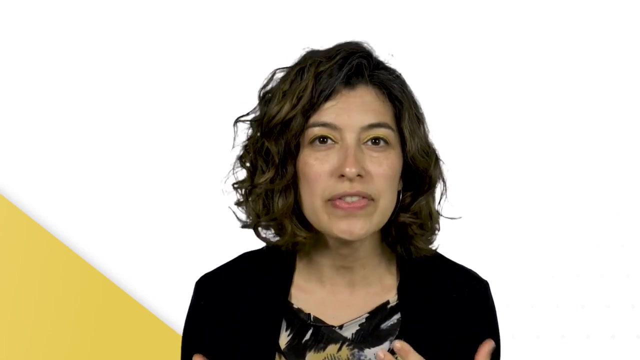 I wanted to do at least 26 terms of that sequence, But if you need to write more to make the pattern explicit, do okay. And here's a suggestion of the sets of numbers that I would like you to use. So I'll suggest these three: 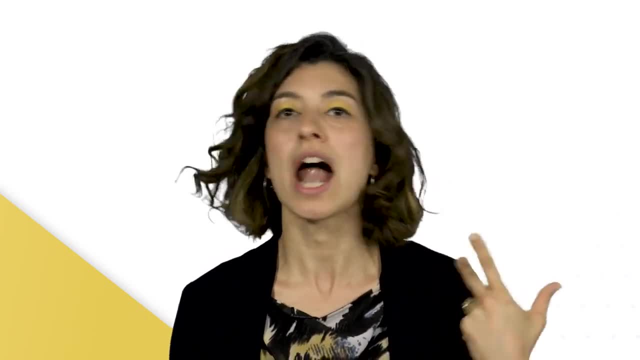 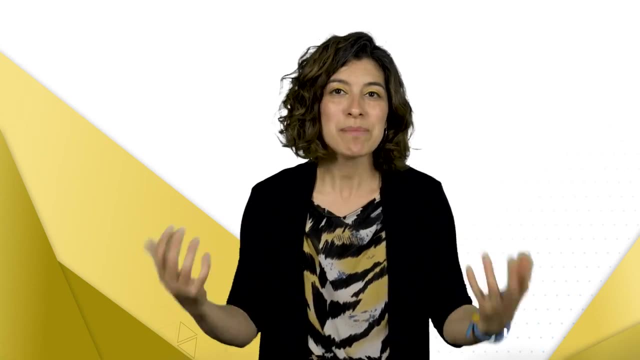 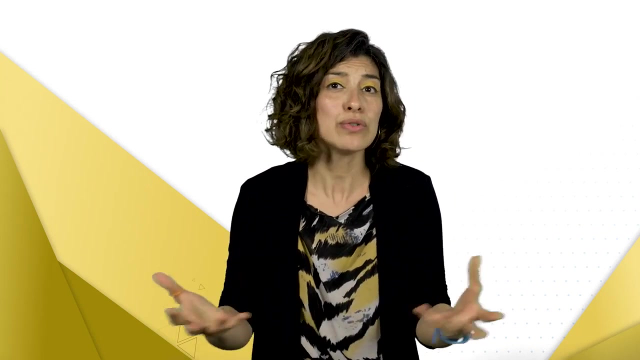 But you will need to come up with seven more that aren't the ones in the examples. And then, once you've done all these calculations, I'd like you to group parameters in families, according to the properties you're finding relevant, to decide how good these sequences. 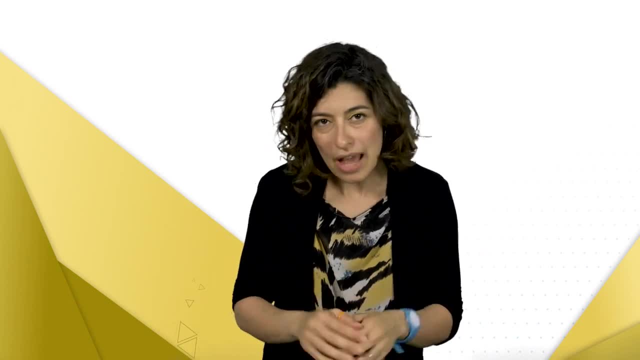 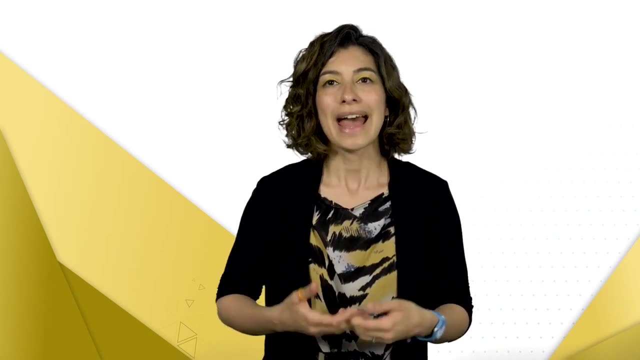 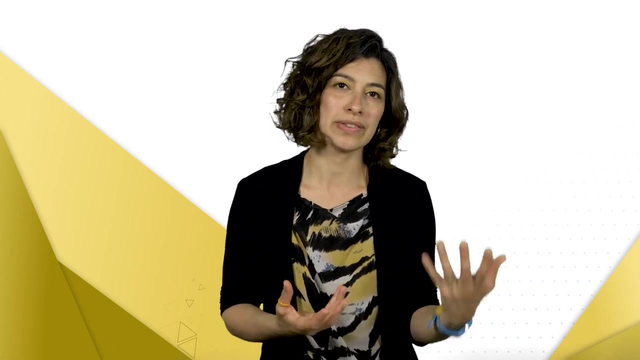 are at appearing random. Now, everything you say in your work, I would really want you to justify your observations and illustrate that with calculations And any predictions you make. I would like you to back it up, not just with the examples of the calculation. 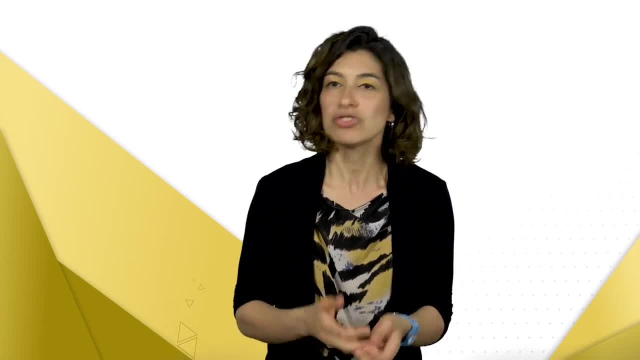 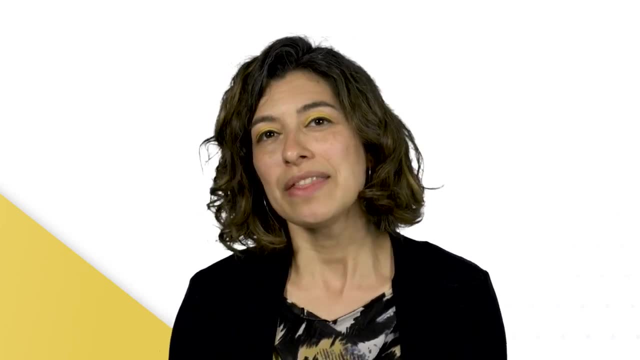 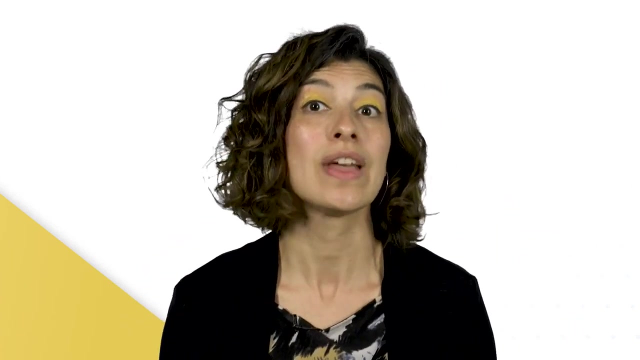 but the best mathematical explanation you can write. Just try your best. If you decide to use a spreadsheet to help with any of the calculations, then the patterns you find need to be explained in terms of how you would do those calculations by hand. It's also a very good idea. 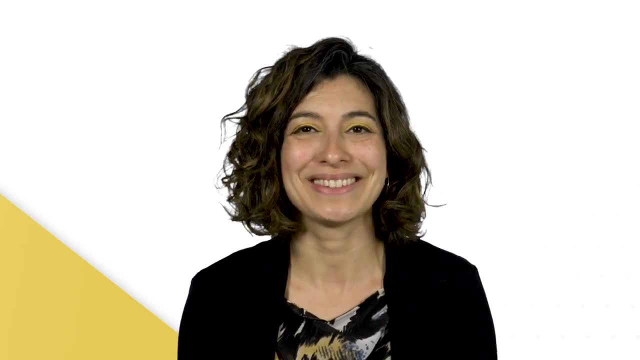 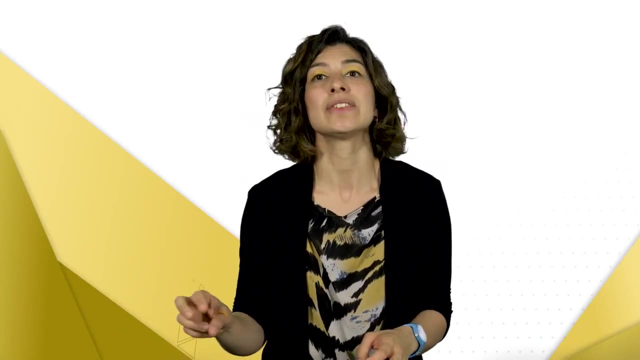 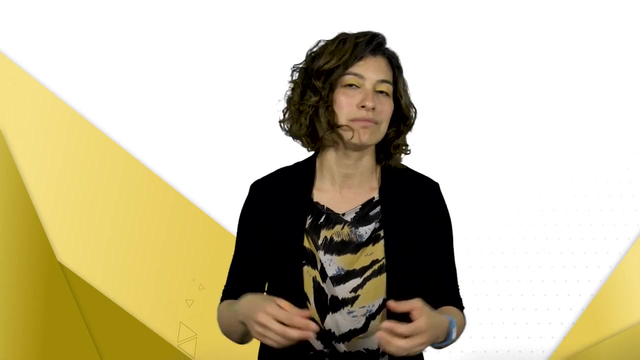 to double check that what you do in the spreadsheet is actually correct by doing it by hand. Now, if you calculate by hand, I want to see you're working for at least three examples that involve calculating something like a mod b, when a is larger than b. 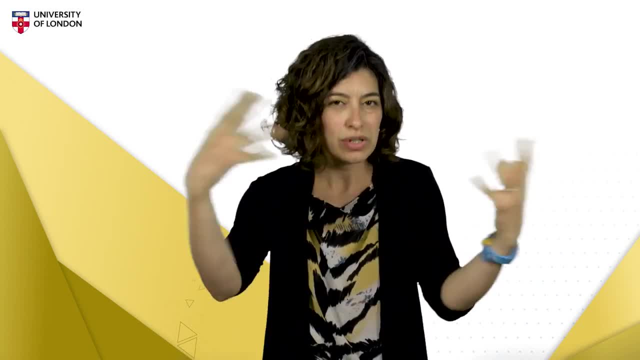 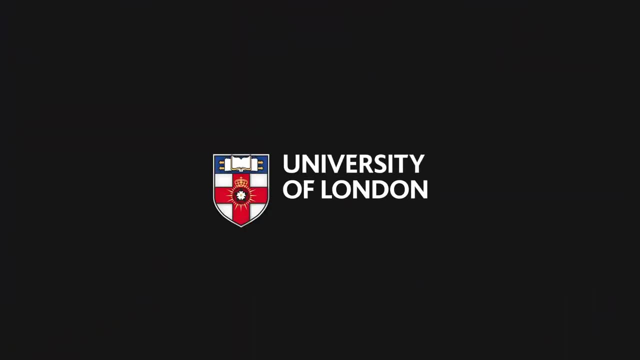 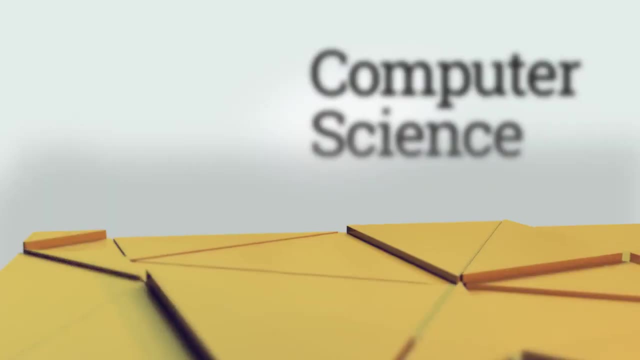 So not just the simple mods. I want you to go over the modulus at least three times and show it explicitly. We looked at how to formally define sequences of numbers by either giving an expression for the general term or by giving a recurrence relation between terms. 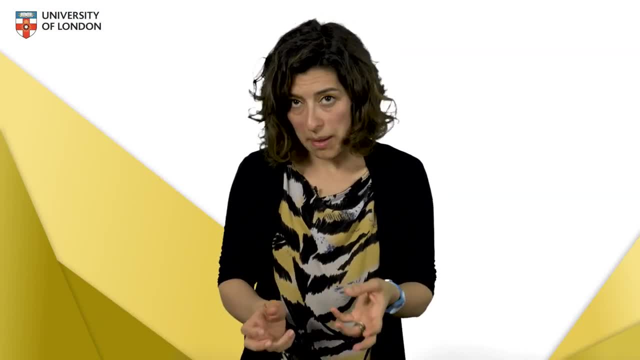 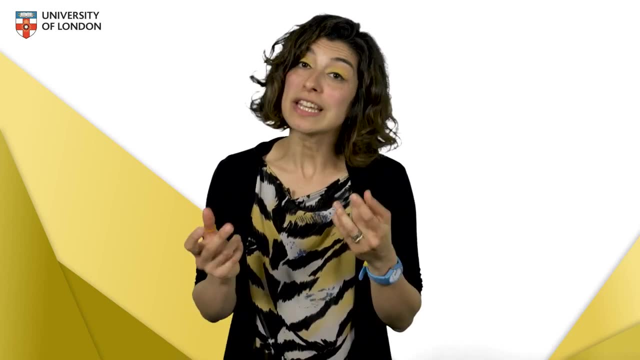 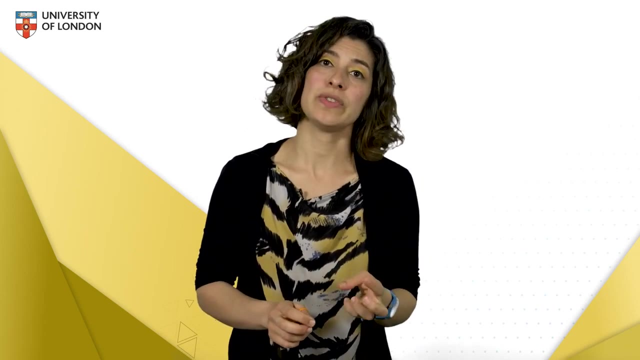 We looked in detail at two special types of sequences. The first one is called the general term and the second one is called the recurrence term. The second one is called the general term and the third one is called the geometric progression One with a constant increment. 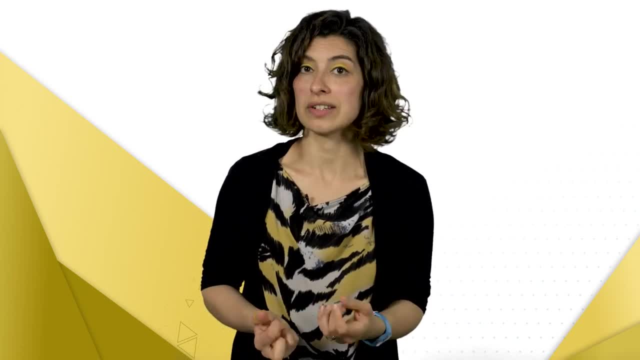 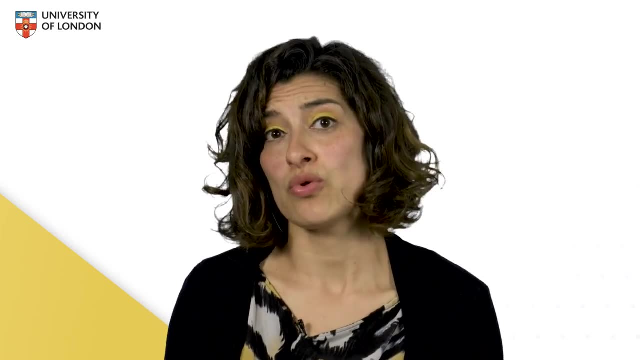 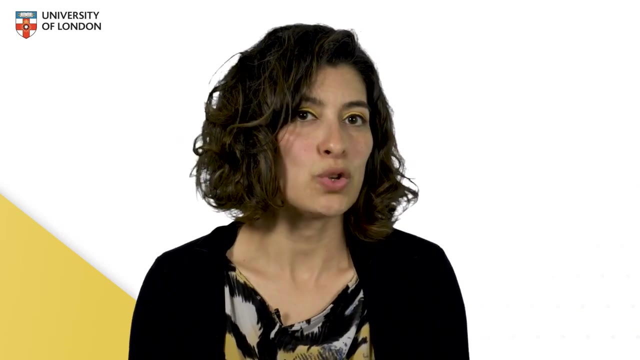 and another with a constant scaling factor. We are interested in the behaviour of a sequence as more and more terms are computed. We sometimes need to add up a certain number of terms. You wonder, are there any shortcuts to this? We will see in the next lesson. 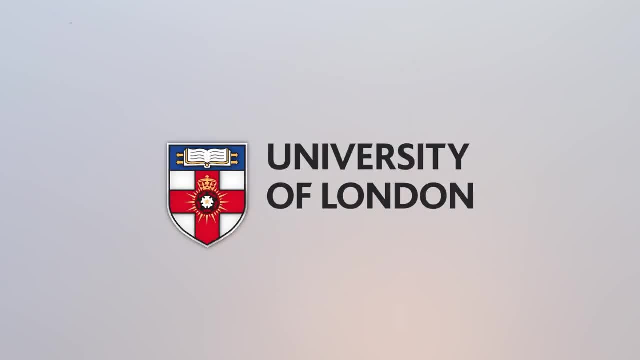 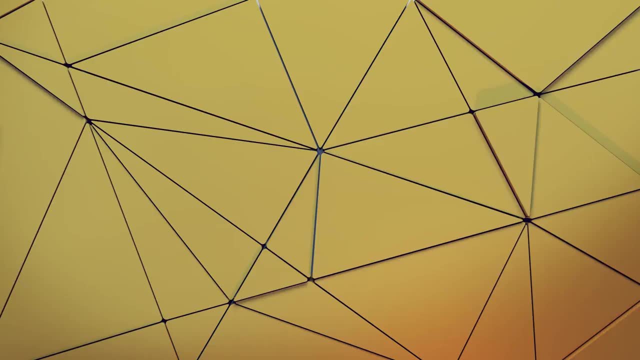 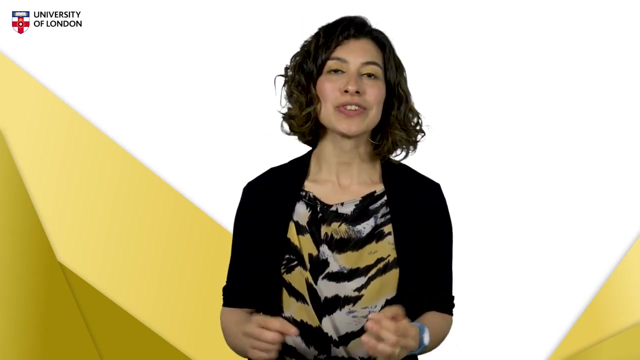 We are going to talk about series, and series is all about adding up terms of sequences. Now back to us humans. Most cultures have cumulative songs, Songs that have a structure that is changed in order to create a sequence. Now back to us humans. 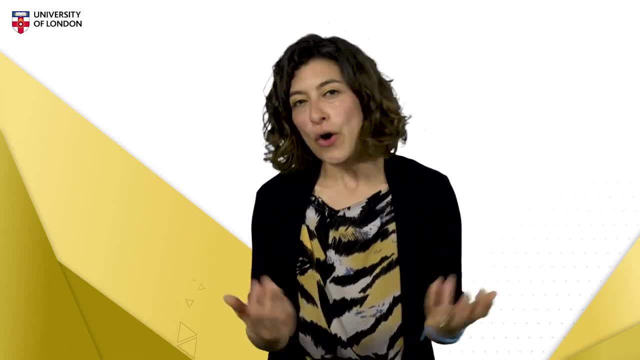 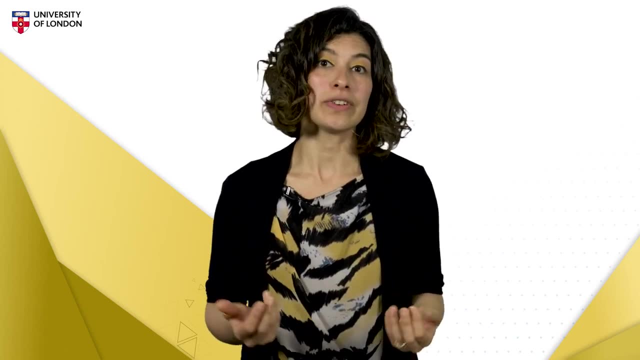 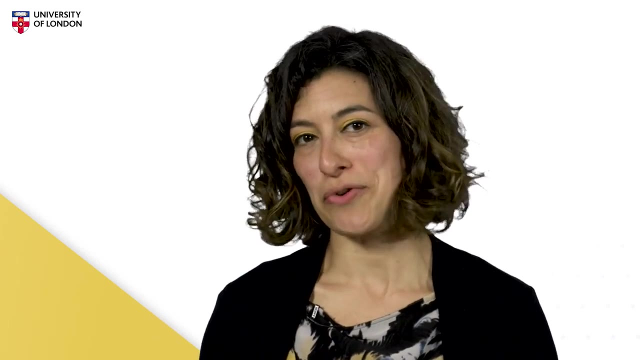 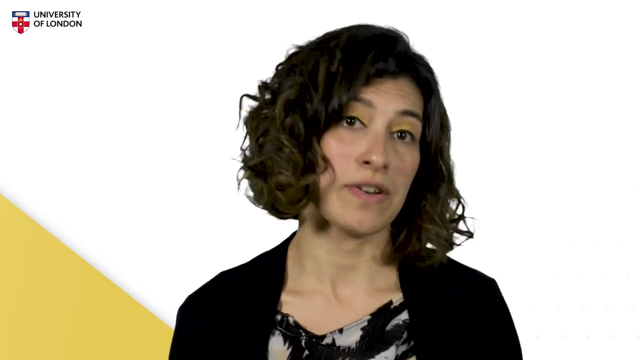 Most cultures have cumulative songs, Songs that have a structure that is changed using progressive addition, resulting on each verse being longer than the previous. Do share such examples with us in the discussion forum. An example of a cumulative song is the British song The Twelve Days of Christmas. 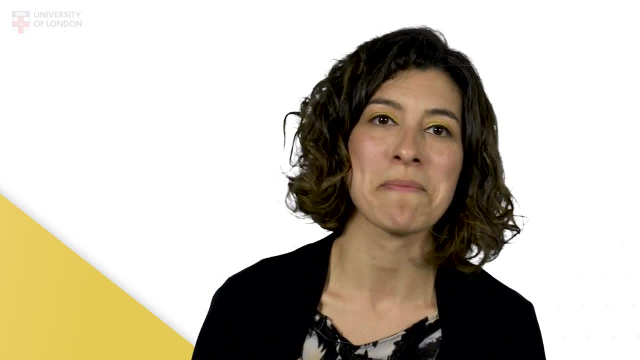 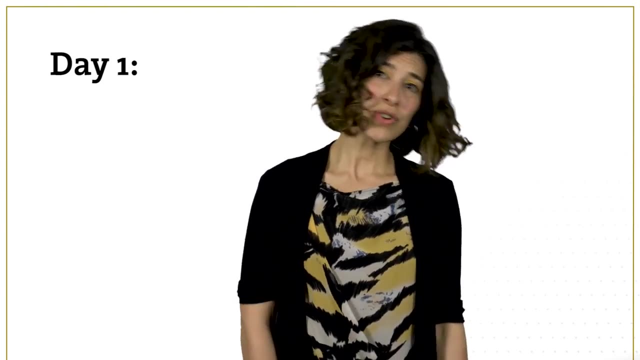 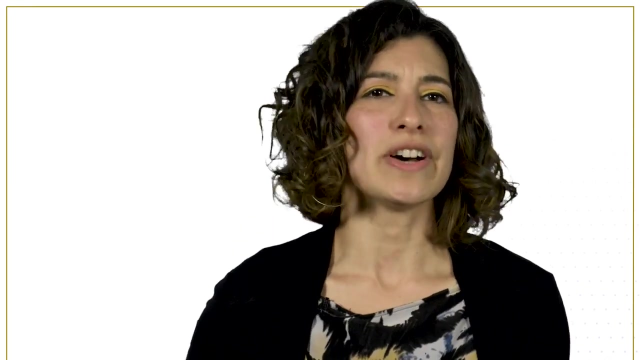 You may have heard it: in the middle of shopping for presents, On the first day of Christmas, my true love sent to me a partridge in a pear tree On the. Let's read the verse, And it goes like this: On the second day of Christmas, 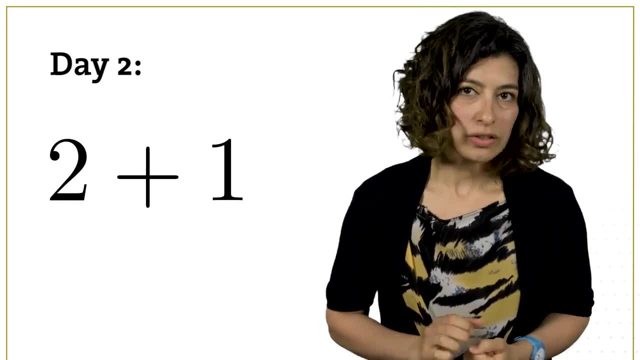 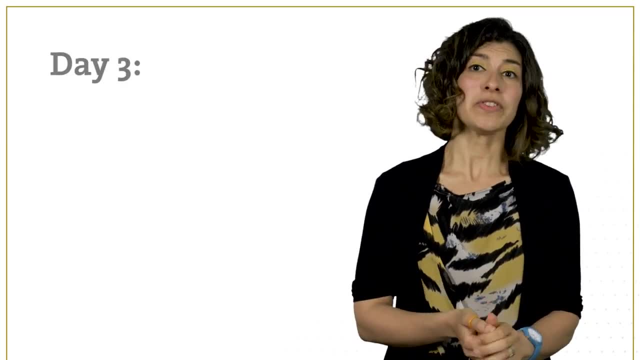 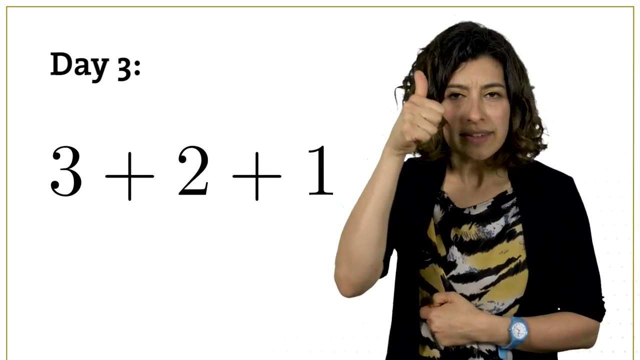 my true love sent to me two turtle doves and a partridge in a pear tree. On the third day of Christmas, my true love sent to me three French hens, two turtle doves and a partridge in a pear tree. And it carries on. 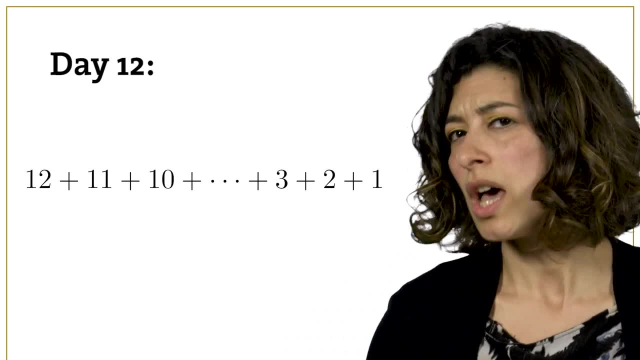 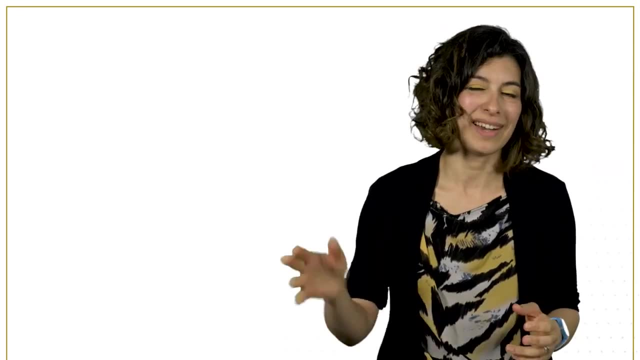 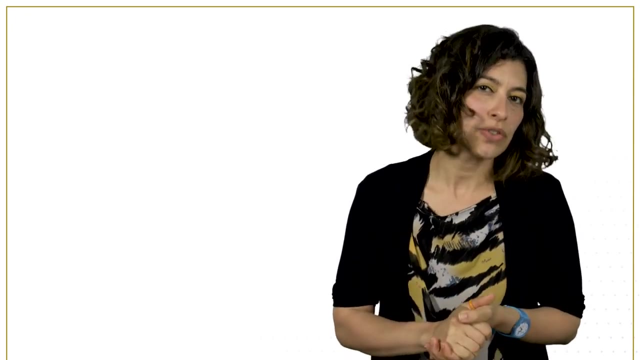 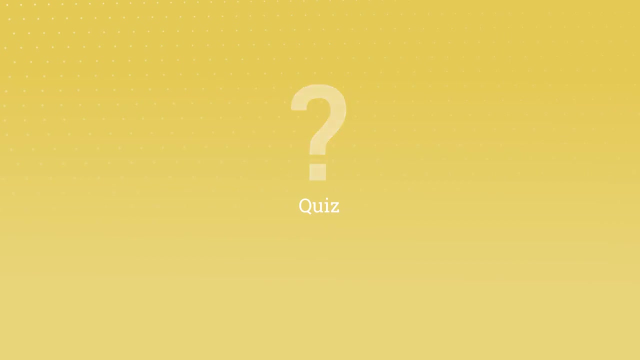 like this, with more gifts in this pattern until there are twelve drummers drumming on the last one. That's a lot of noise for sure. Yeah, yeah. well, How many gifts are there all the way to Christmas? Okay, so in the quiz. 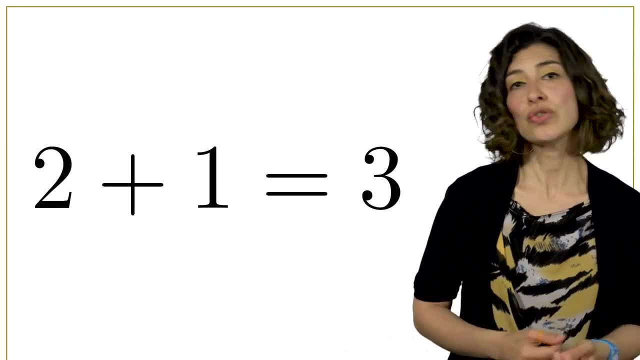 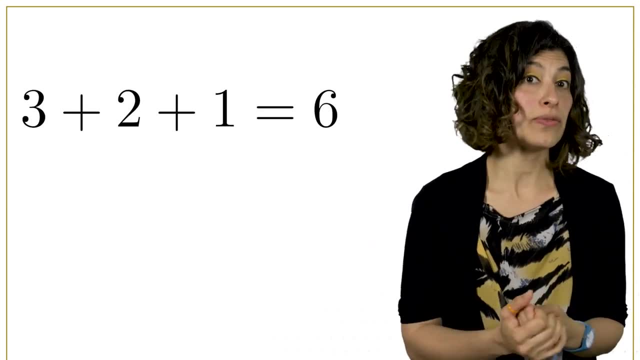 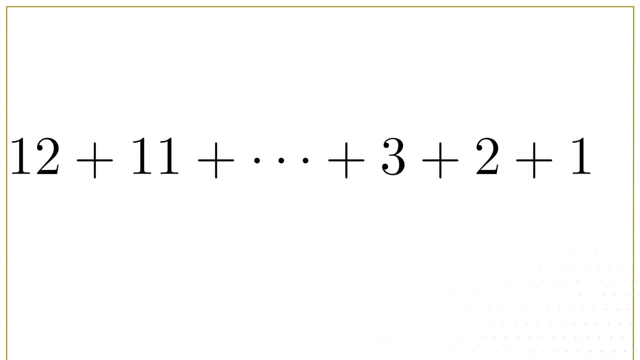 you've written day one, you've got one gift. day two is one plus two gifts, so there's three gifts. day three: one plus two plus three, so there's six gifts on day three, and it carries on like that. so by day twelve we are have one plus two plus three plus four. 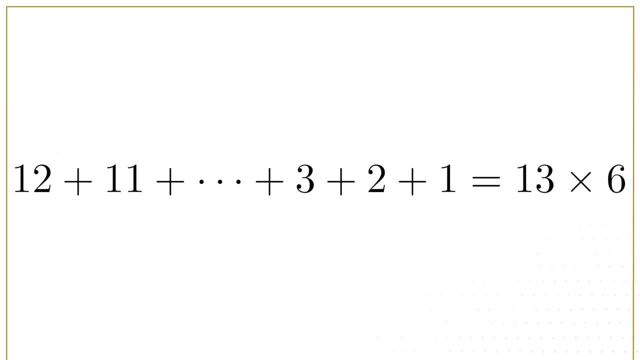 all the way to twelve, which is thirteen times six gifts on day twelve. So what we want to know, the total sum of gifts all the way to Christmas, is this: addition of that one plus the three, plus the six, added with seventy-eight, The way we write. 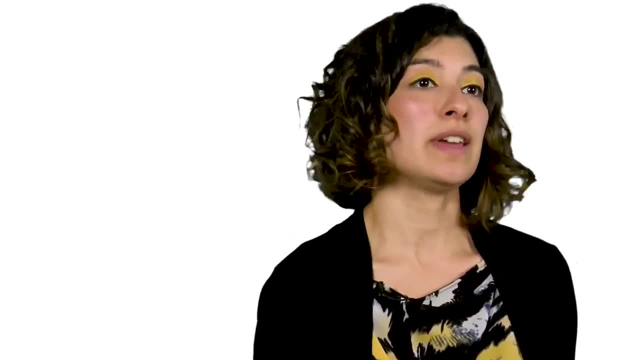 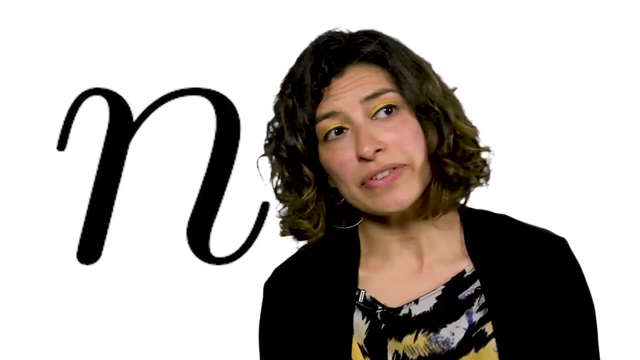 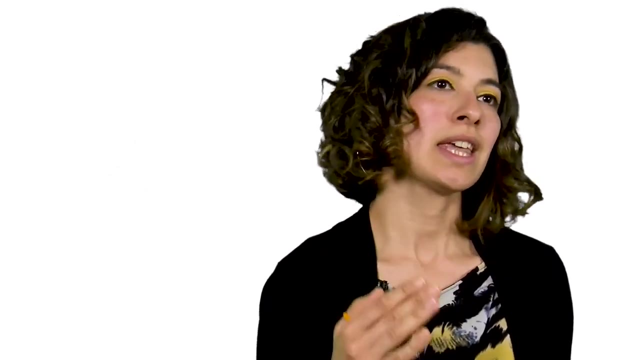 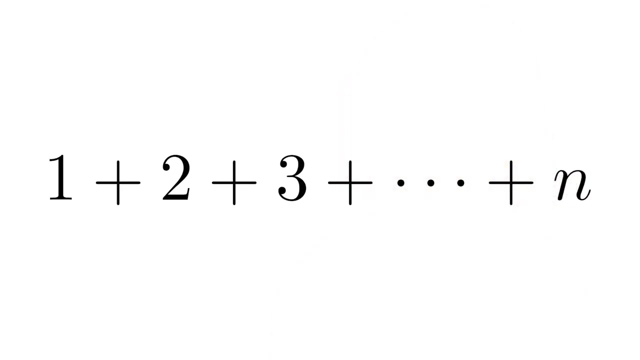 the pattern of presents in one specific day is related to an arithmetic progression. On day N we have the sum of the first N terms of the arithmetic progression, with first term one and common difference one. so one plus two plus three, all the way to N. 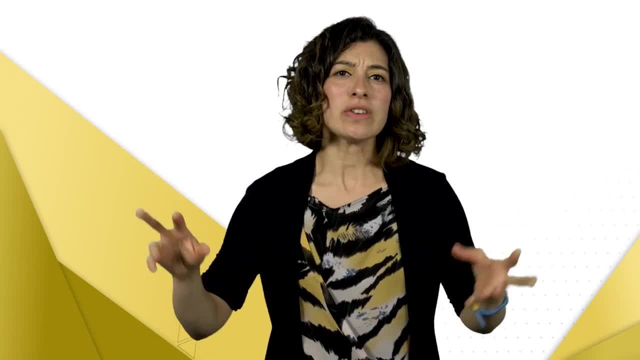 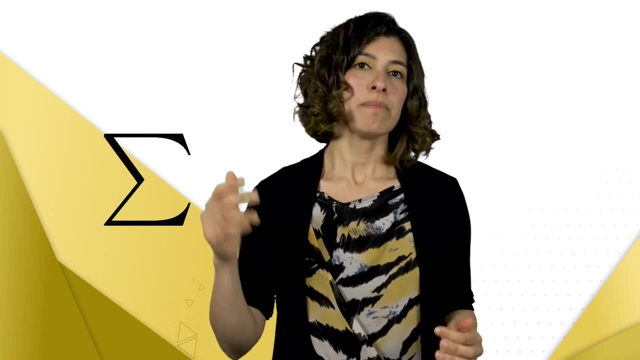 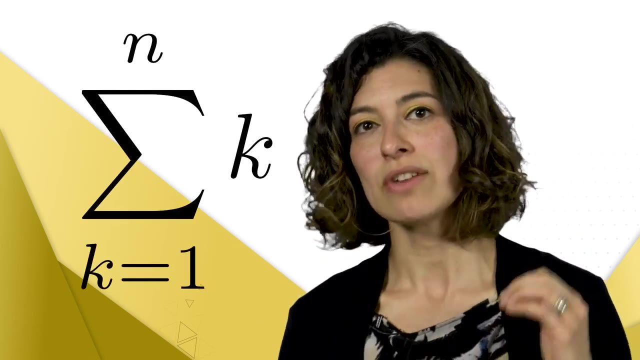 So we write this using a summation symbol, which is the Greek letter sigma, and it looks like this: sum from K, from one to N, of K, We're adding K as K ranges from one to N. That's what that means. The symbol sigma means the sum. 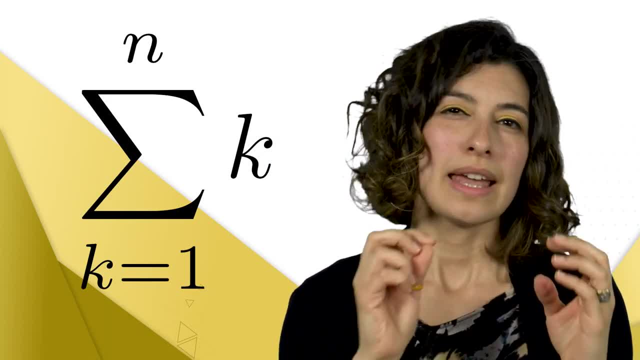 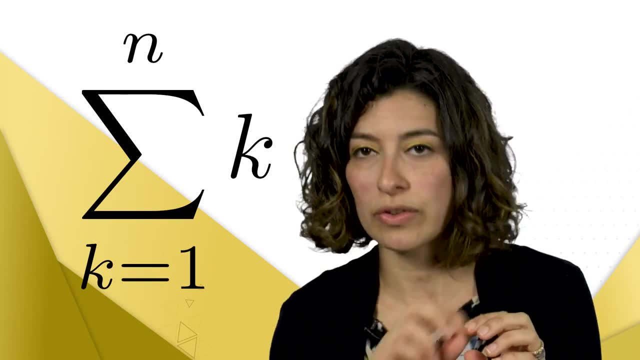 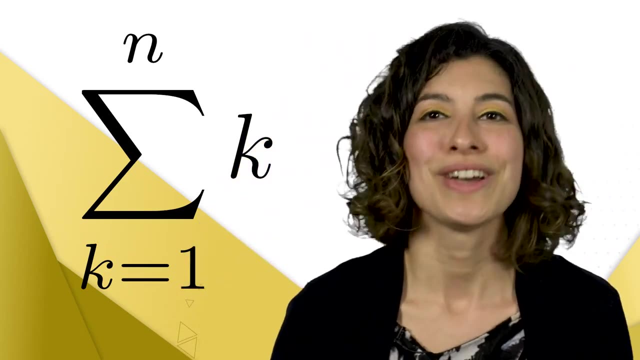 and then the K equals one means that the index of summation, so the variable of the sequence, is K and we start with value one. so we say K equals one and the N on top is the last limit, is the last value that we replace K. 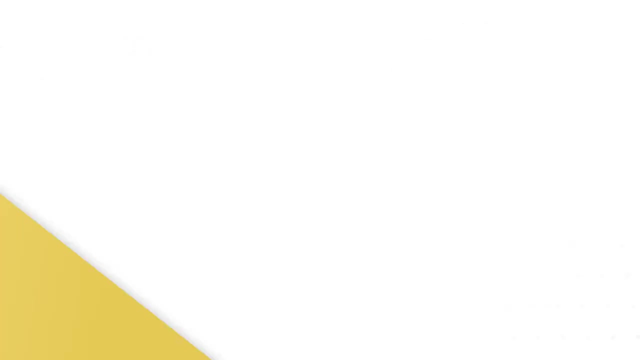 by. So let's look at what happens as I replace N by different values. So when N is one, we get the sum from one to one of K, which is just one. When N is two, I'm adding two terms. I'm adding the term when. 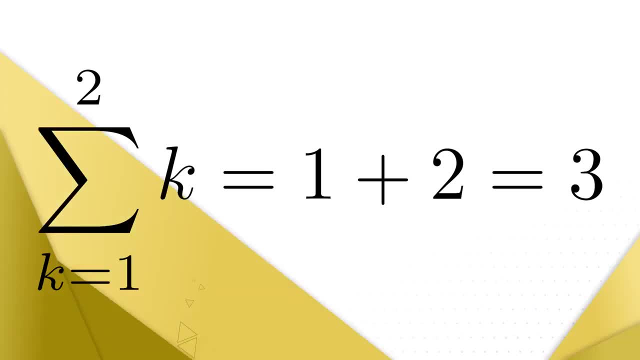 K is one and when K is two, So one plus two, which is three. When N is three, I write: the sum from K equals one to three, which is one plus two, plus three, which is six, and so on. So this is what the summation symbol. 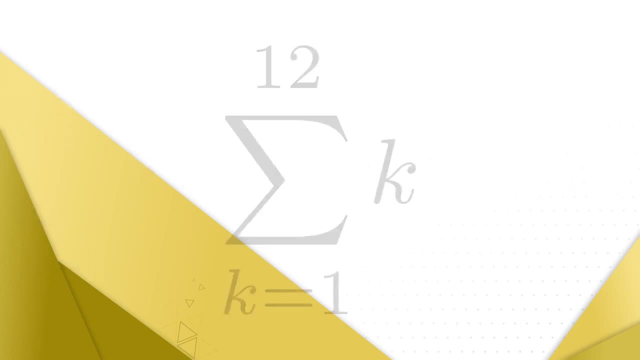 and the series notation looks like and how we use it. So when N equals twelve, I've got the sum from K equals one to twelve of the term K, and so, as I replace K by all those values, I get one plus two plus three all the way. 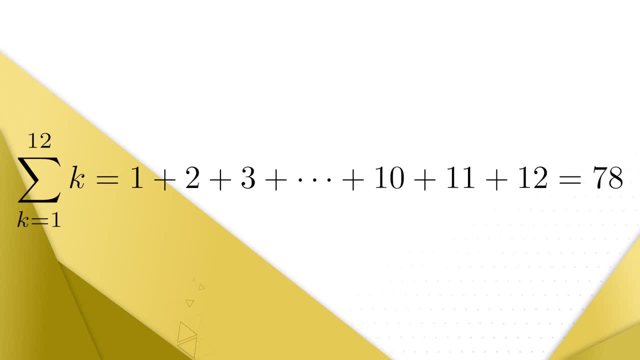 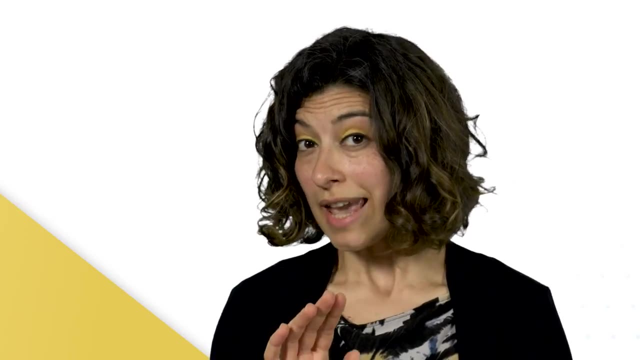 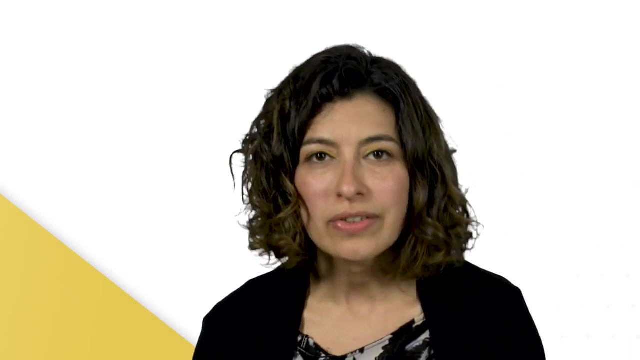 plus twelve, So that's the extended form of this summation and that totals seventy-eight Now. in total, it turns out that there are three hundred and sixty-four presents in the whole of the twelve days of Christmas song, And actually I'm here adding: 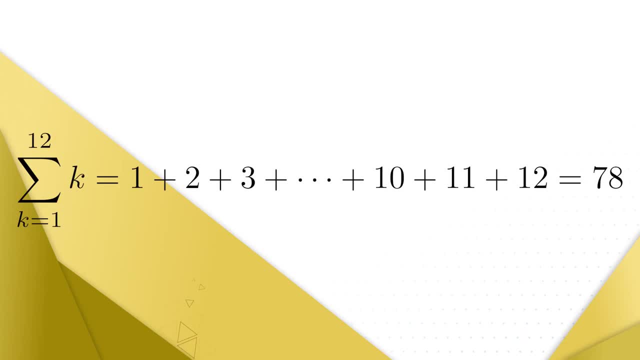 the sums. So it's another use of sums. But just for us to complete the exercise for Christmas, I'll translate this as the sum from K equals one to twelve of the total presents on day N. So I'm adding one plus three plus six, all the 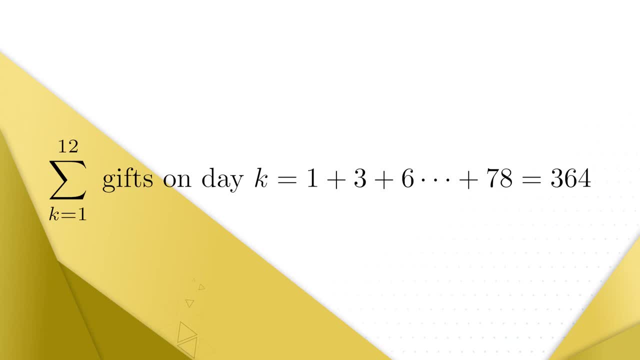 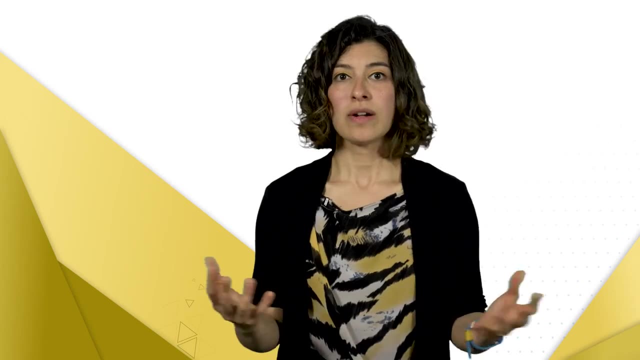 way to plus seventy-eight, which I've done. the calculations have you is three hundred and sixty-four. Now it is a long sum to do, twelve numbers to add up plus. you have to work out all of these in between you and I are probably wondering. 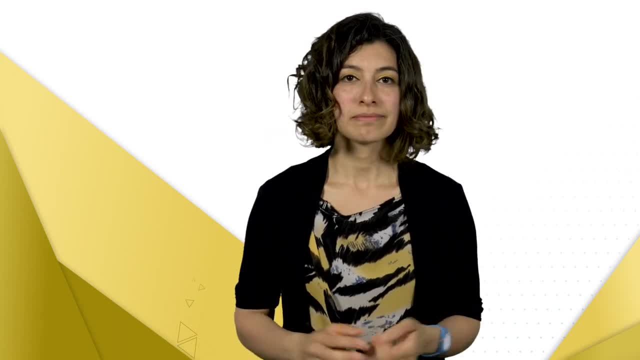 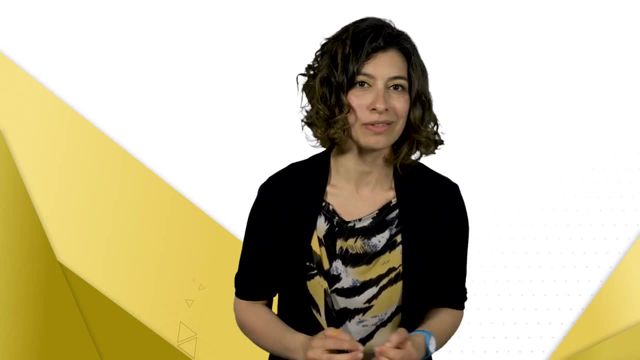 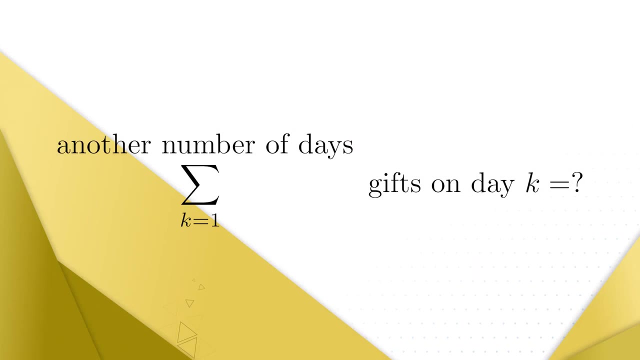 is there a shortcut to work this out? I mean, if the song went on and on for another few days instead of just twelve? in the same fashion and in the terms of wanting to budget for this expense, is there a way of working out this result? 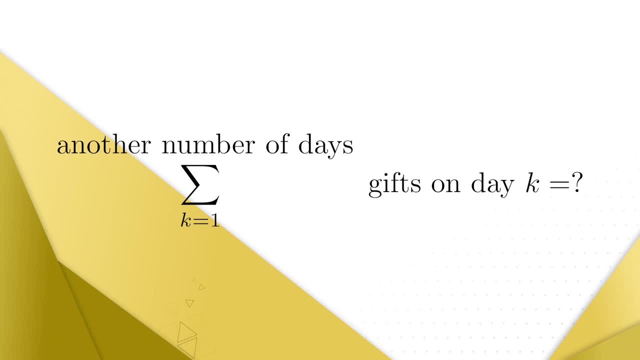 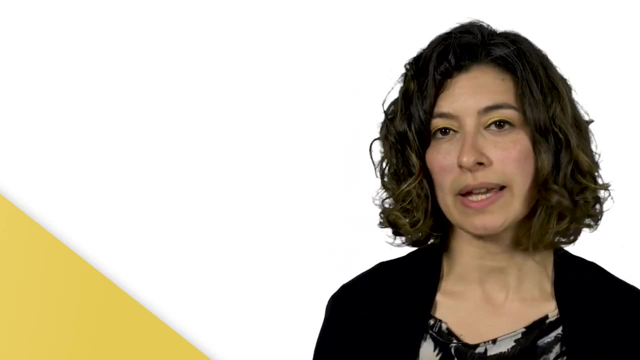 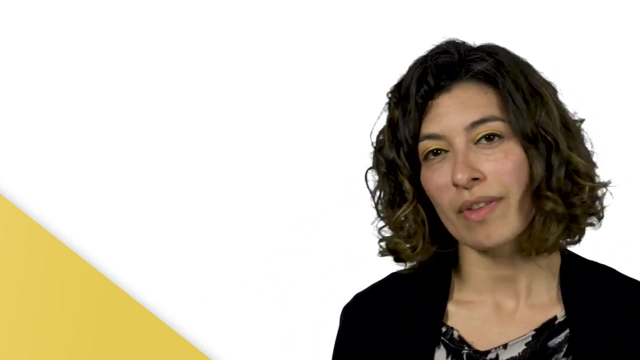 Yes, there is. You will find out as we go along with this lesson. Now back to the sequences we saw in the introduction to this topic. Let's rewrite the rise reward as sequences and series: The amount of grains that arise for square of the chessboard. 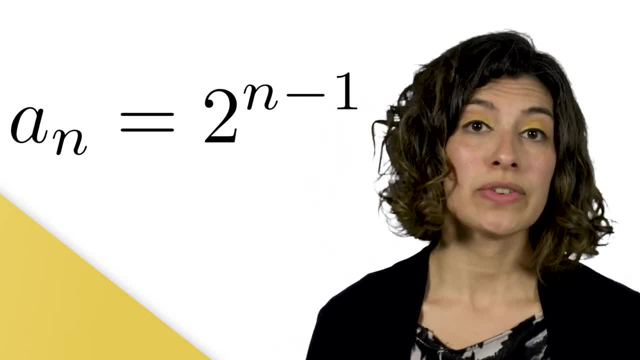 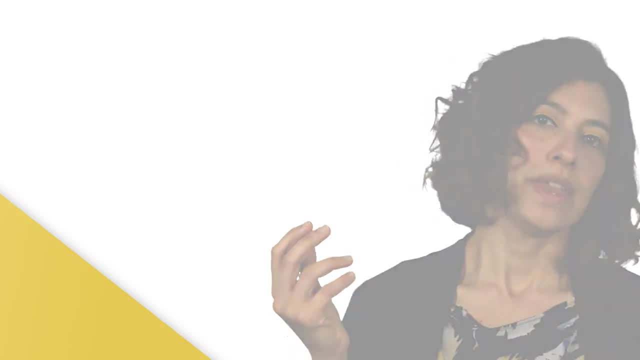 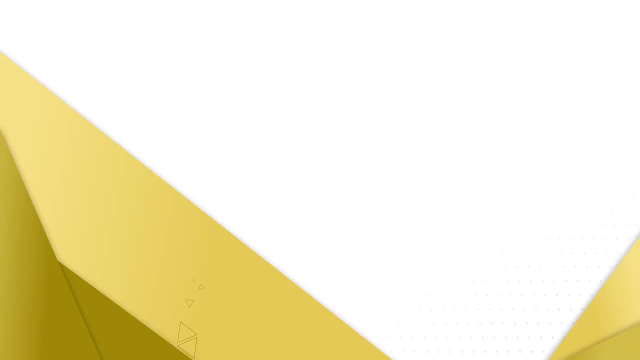 for square n is given by the sequence: a n equals two to the power n minus one, with n ranging from one to sixty-four. The total reward is the sum of all these terms. So the total reward is the sum of the series, the sum of a n. 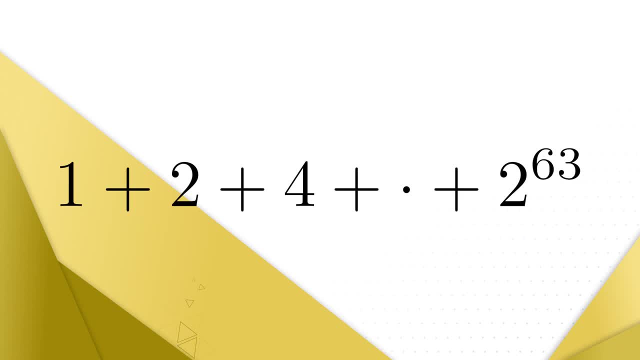 now we need to work out what's the first and last value for the index of summation. We want to have one plus two plus four plus eight plus sixteen, all the way to adding two to the sixty-three, not sixty-four, There's sixty-four squares. 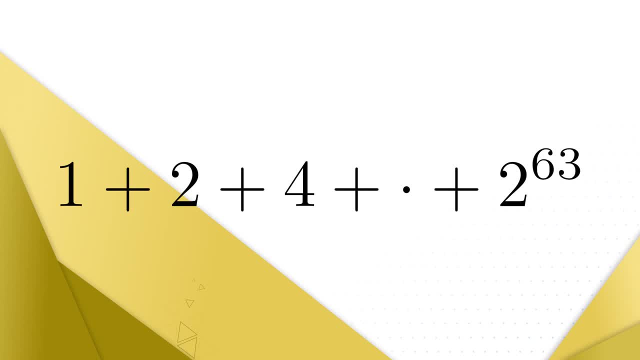 but we start in one. So we write: one plus two plus four, plus eight plus sixteen, dot, dot, dot all the way to two to the sixty-four, and that is written as: the sum of n equals one to sixty-four, of two to the power of n minus one. So this is how we. 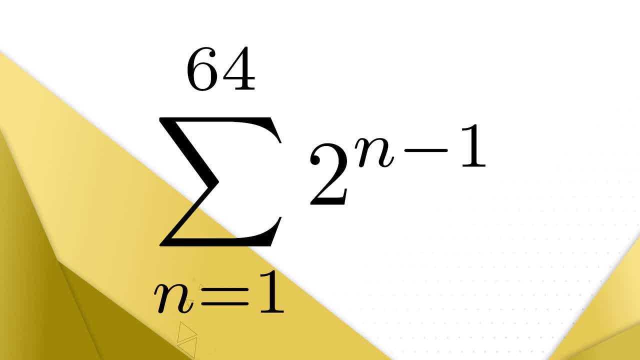 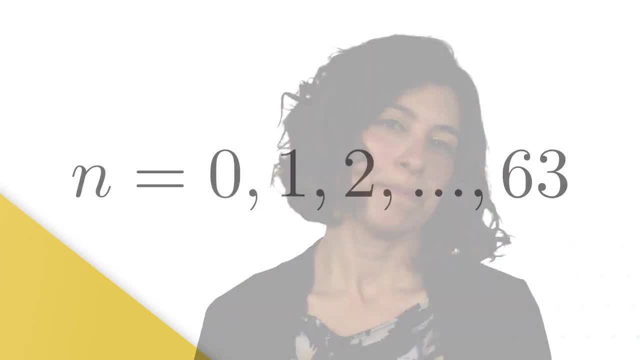 transform this sum into a summation symbol. Now notice that we could change the limits in the sum and have it written as: the sum from n equals zero to sixty-three of two to the power of n. It's just a cosmetic change. they're exactly the same sums. 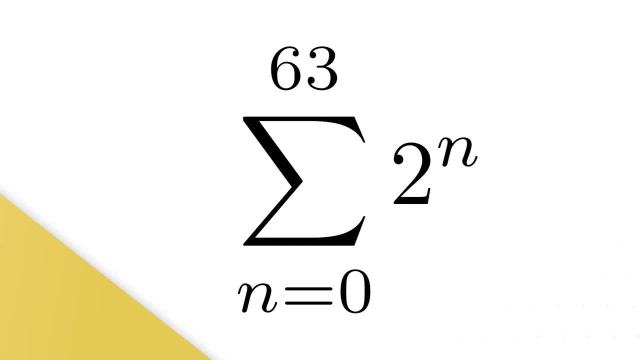 but they're presented slightly different. All I've done is that, because I've got n minus one in the other series and I've got the range from one to sixty-four, if instead of n minus one I have n, then I'm starting at zero and ending at sixty-three. 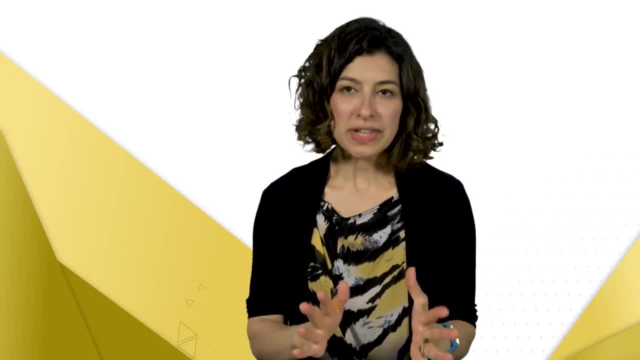 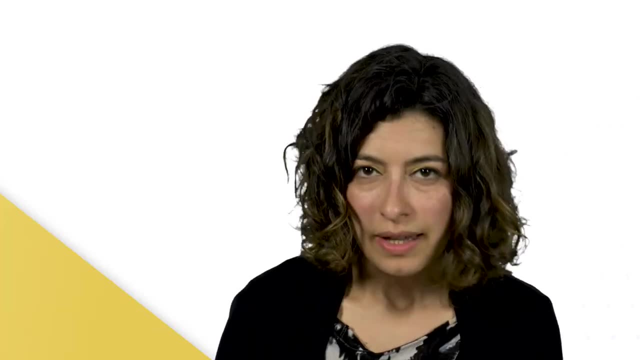 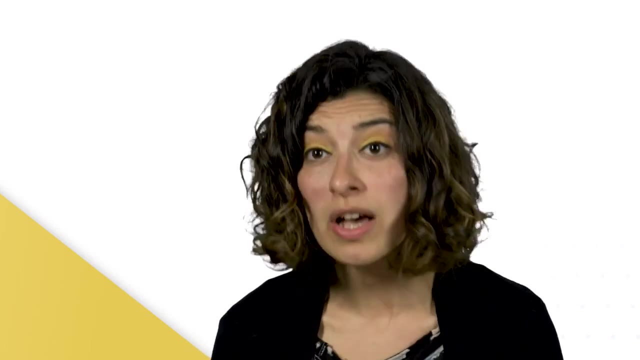 So the idea here is that when we add up sequences incrementally, we are creating a new sequence, the sequence of partial sums. But because this sequence is specifically generated by adding a consecutive number of terms of a sequence, we call it a series. So that's what a series is. 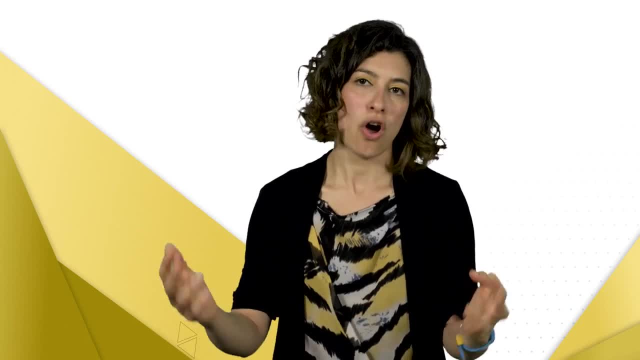 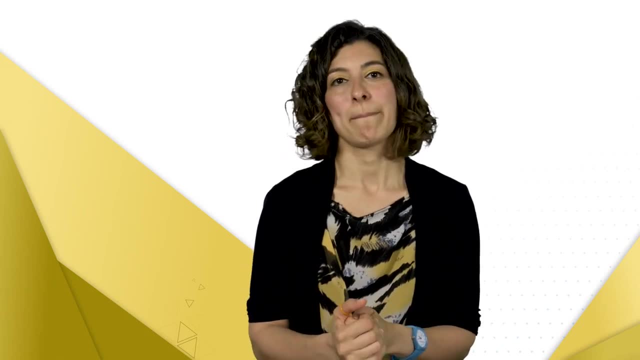 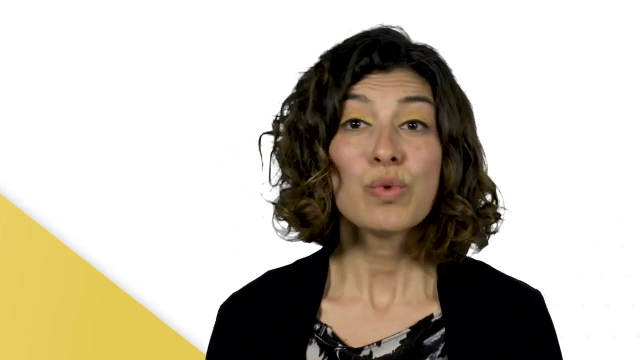 is the sum of consecutive terms of a sequence, And in some cases we have shortcuts to find this sum. At the start of this topic we talked about a job offer with two payment plans. We wrote the sequences for those and we did the sums in our spreadsheet. 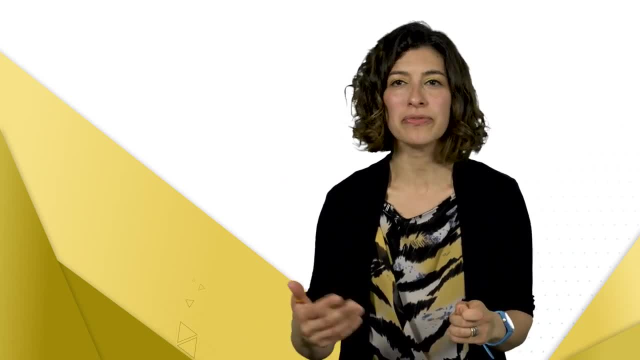 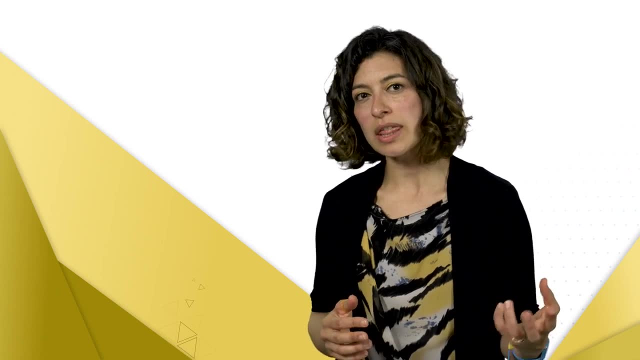 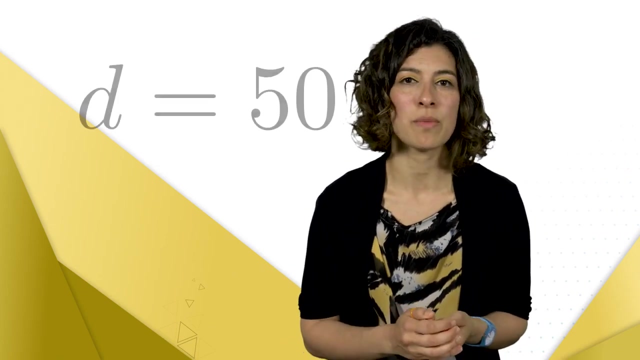 Option one was we had £100 in the first day and then £50 extra than the day before in any new day. And option two was a pound to start with and then the pay was doubled every day. So we saw option one is an arithmetic progression. 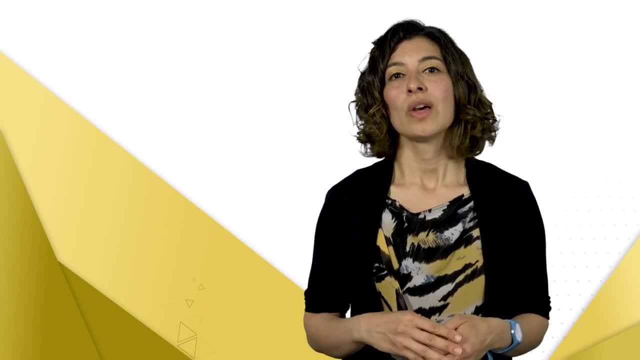 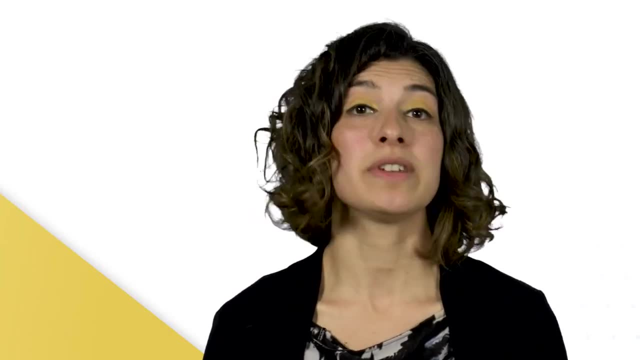 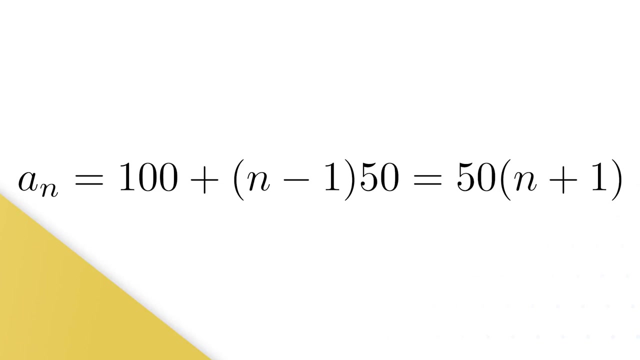 of common difference 50 and first term 100. and option two is a geometric progression of common and common ratio 2.. Now, in terms of the arithmetic progression, the general term is: an is 50 times n plus 1. you can work it out from the formulae we worked. 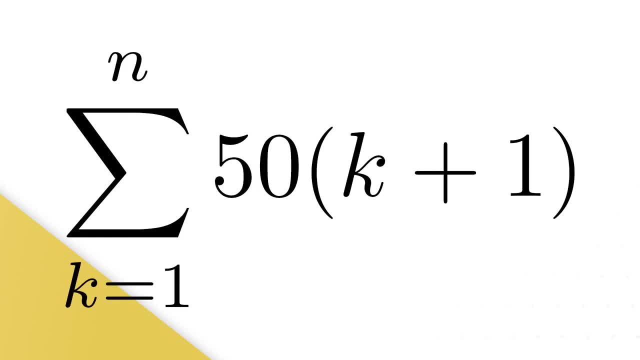 and the sum up to day n is the sum from k equals 1 to n, of 50 times n plus 1, which is, in the expanded form, 100 plus 150 plus 200 plus all the way to 50 times n plus 1.. 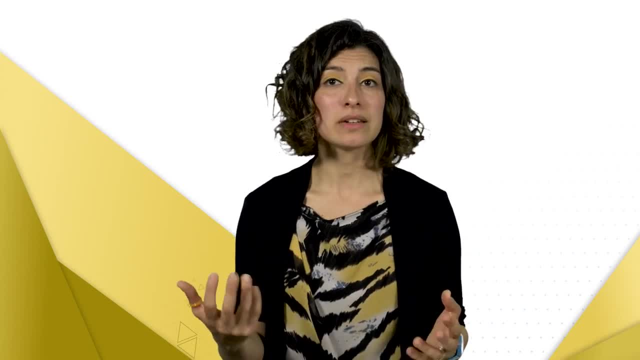 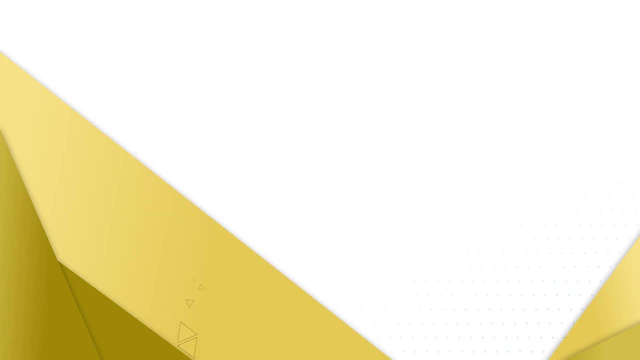 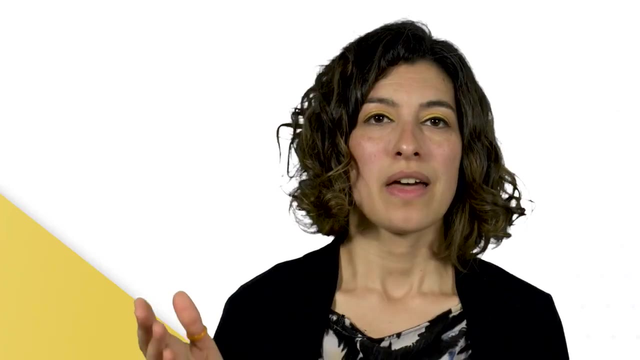 For the geometric progression on payment plan 2, the general term is: bn equals 2 to the power of n minus 1, or just 2 to the n divided by 2.. So the sum up to day n is the sum from k equals 1. 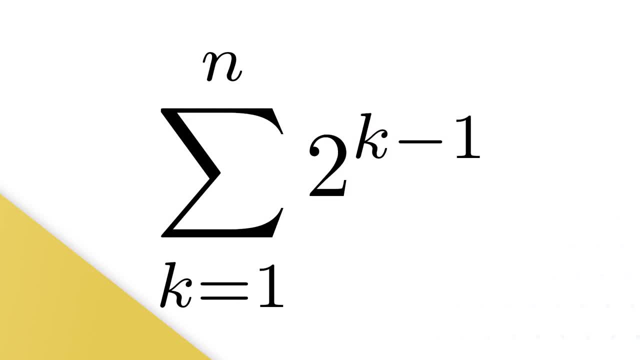 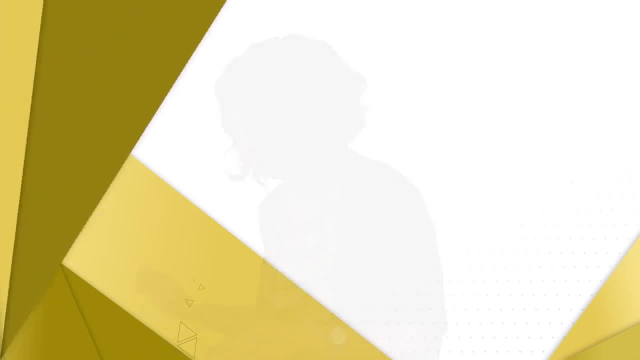 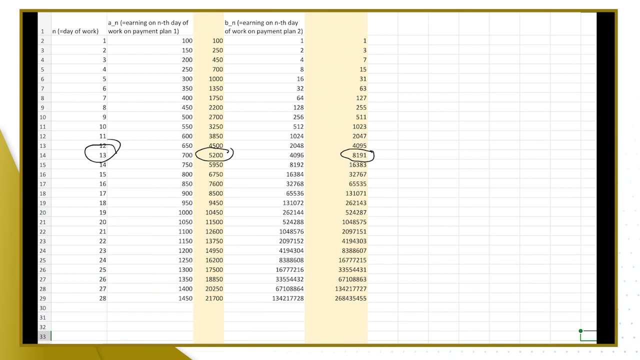 to n of 2 to the power of n minus 1.. So when we looked at the spreadsheet which I actually show you, we had results for the sums. So we can actually write that the sum on the 13th day which I calculated and highlighted last time. 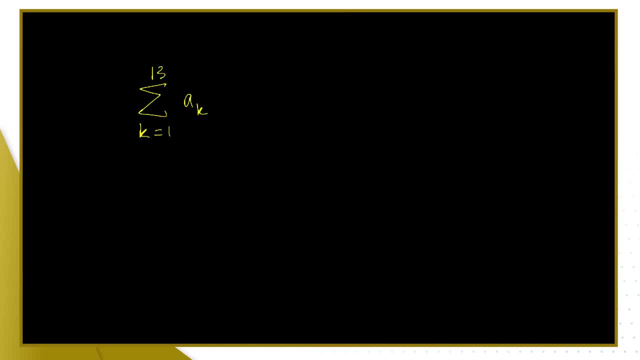 the sum of k from 1 to 13 of a k from our spreadsheet was 5200 and the sum on the second payment plan from 1 to 13 was 8191. So we can say the sum of the first payment plan over 13 days. 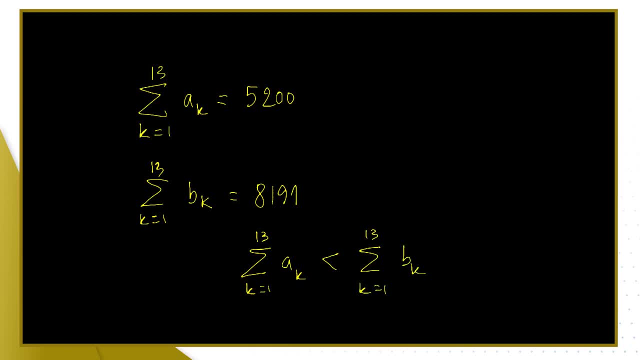 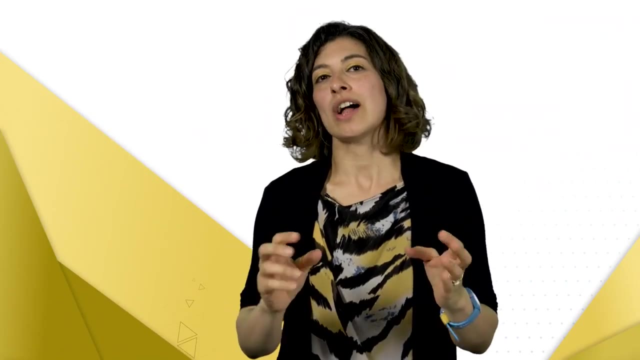 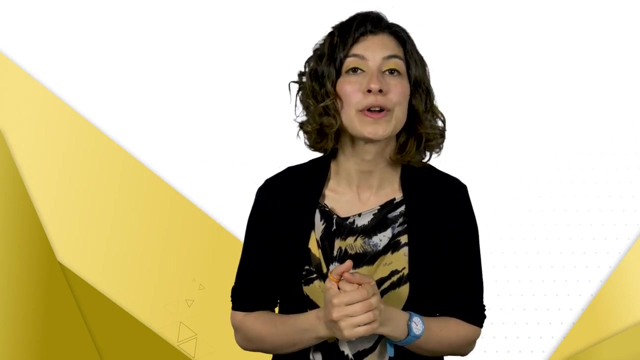 is less than the sum of the second. So that means that we would choose payment plan 2 if we were planning to work for 13 days or more. Now, when we were calculating the presents on a particular day in the Christmas song, we have a special type of 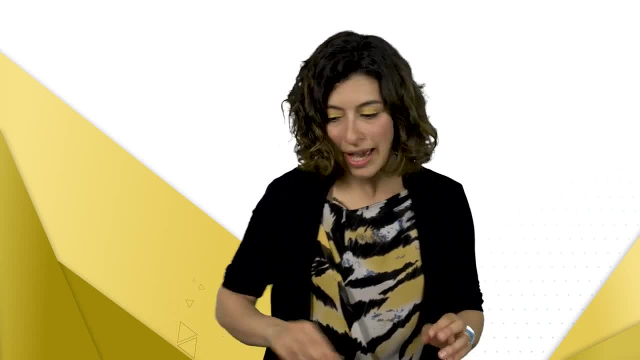 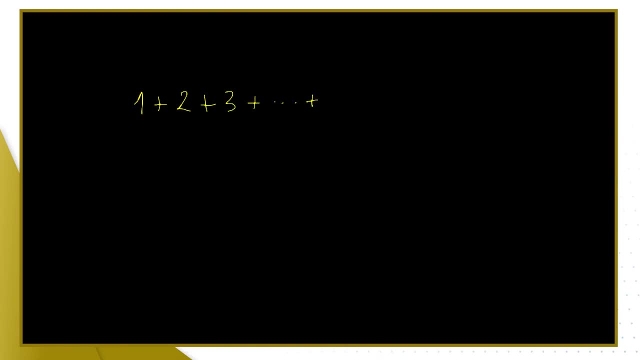 number coming up and I really need to talk to you about that. So we had numbers, we had the sum 1 plus 2 plus 3, all the way- if it was day 7, it would be all the way there- And this sum, which is the sum of a very particular 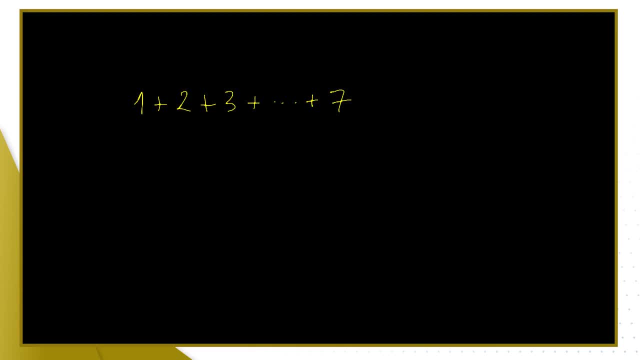 arithmetic progression. when the common difference is 1, the result of these sums is called a triangular number. What I mean is we have number 1, that's a triangular number. number 1 plus 2, being 3, is also a triangular number: the 1 plus 2 plus 3. 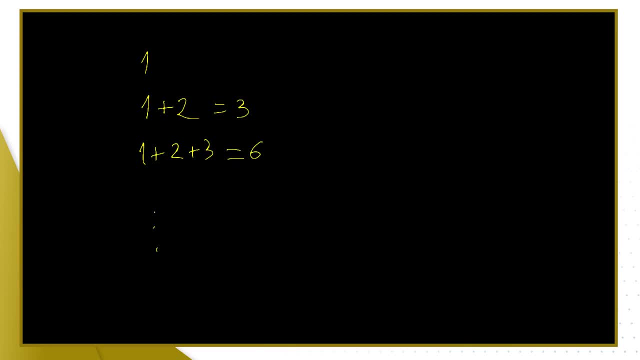 which is 6, is also a triangular number, and so on, all the numbers written in this fashion, and that's because that many dots can be arranged in a triangular pattern. So 1 is just a very simple triangle. 3 can be written as 1. 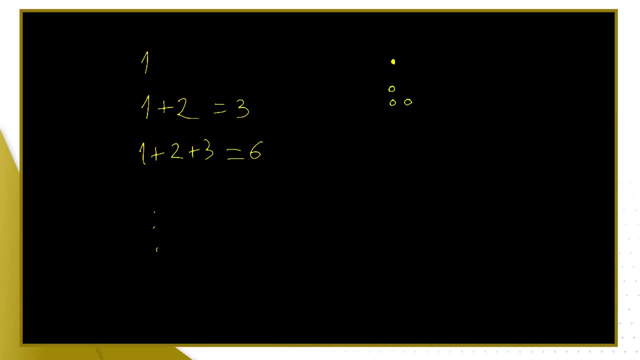 and then 2. underneath that's a triangular pattern. and then we have a new row- triangles- how beautiful. and it carries on. the next triangle number will have 4 rows. so we have a 1 with a 2 with a 3 with a 4. 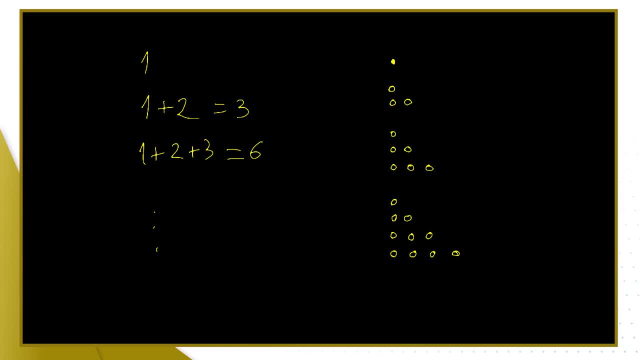 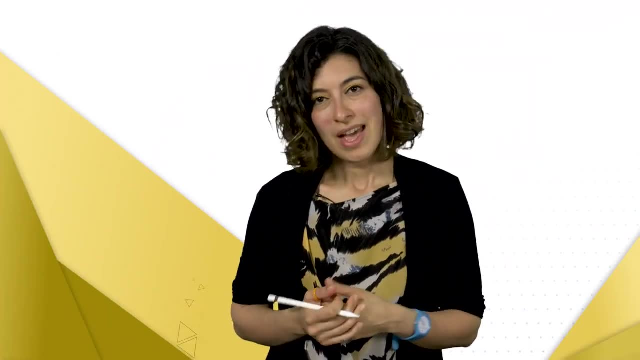 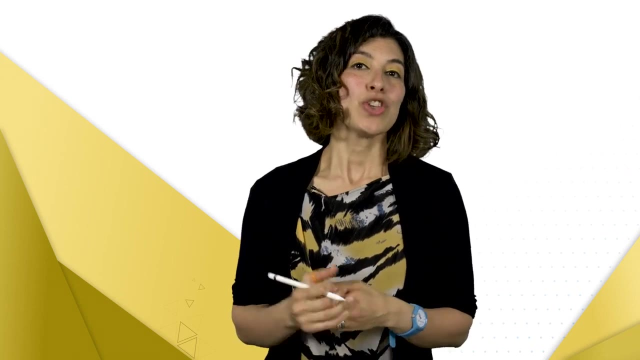 so that's 6 plus 4, so that's 10. so all of these are triangular numbers and they will come up again and again in your. So when we look at the sum of the arithmetic series, you will get a formula for triangular numbers. 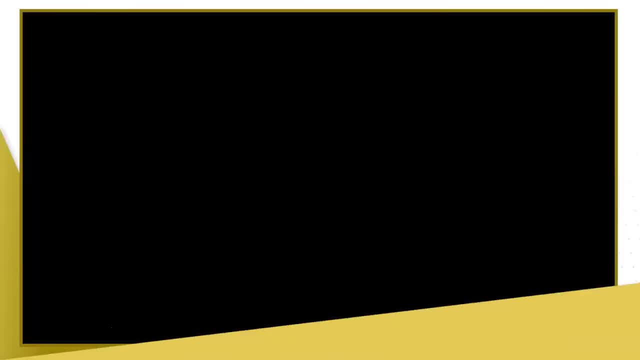 So let's expand the following series. We have: the sum from n equals 3 to 7 of the expression n, plus 1 over n. Let's write this in the expanded form. That means we're going to replace n by the first value and then carry on until I get to the last value. 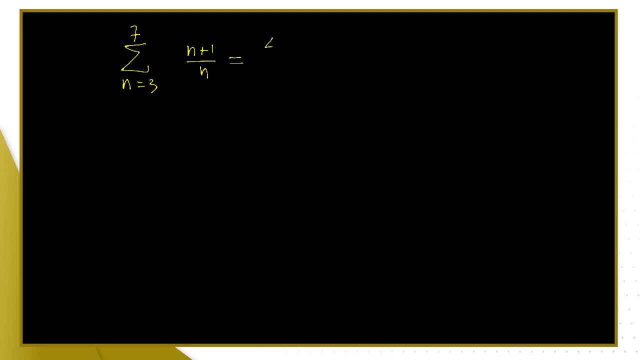 So when n is 3, I have 3 plus 1, which is 4 over 3.. Plus, when n is 4, I have 4 plus 1 on top, so it's 5 over 4.. 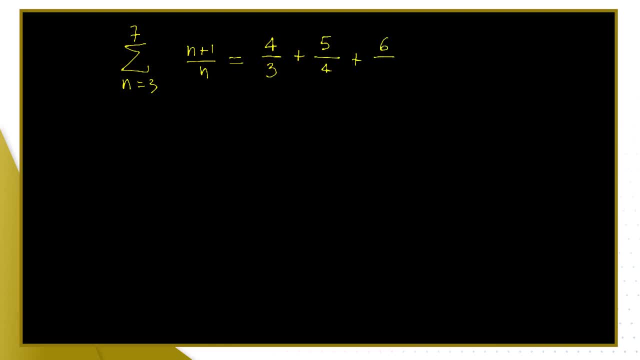 When n is 5,, I get 6 over 5.. When n is 6,, I get 7 over 6.. When n is 7,, which is the last one, I get 8 over 7.. So this is the expanded form. 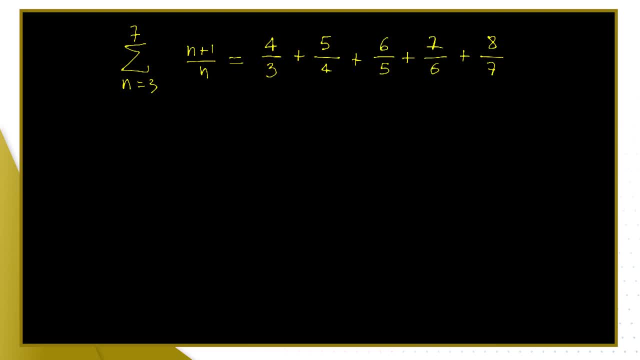 And to find the result you just add up those values And this equals 6.09285714 recurring. I mean it's going to be a fraction, so it should be either finite or recurring. So this is the value. 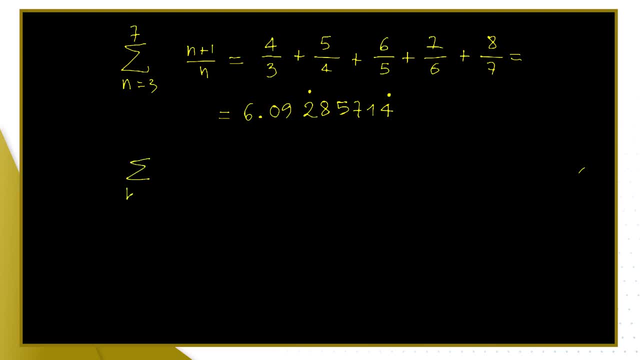 So let's look at another one. So we've had a sum From k equals 2 to 5 of k cubed. it's important that the index of summation, which in this case is k, because that's what k equals 2, is the same as the variable used in the sequence. 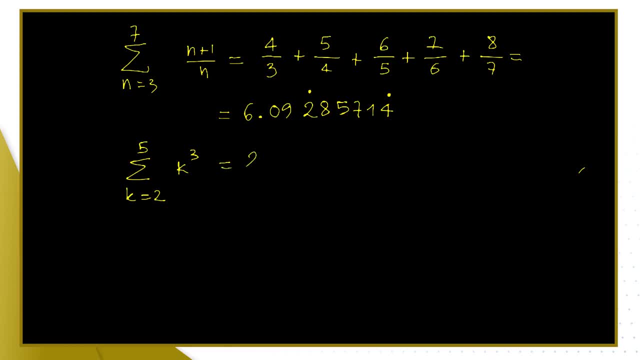 So I've got k cubed, So I've got 2 cubed plus 3 cubed plus 4 cubed plus 5 cubed, And you can work out what that is. Another one Sum from i equals 1 to 4 of the number 10.. 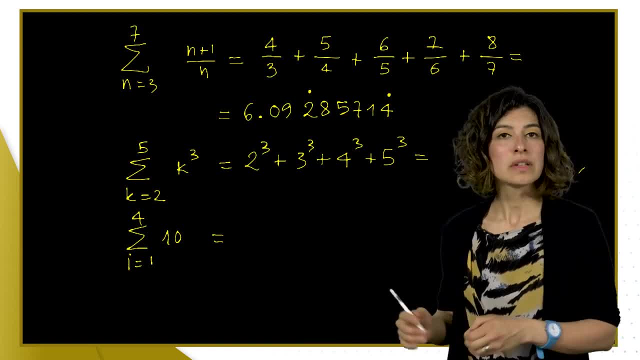 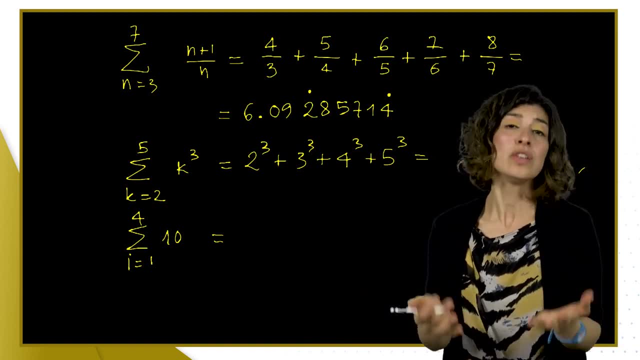 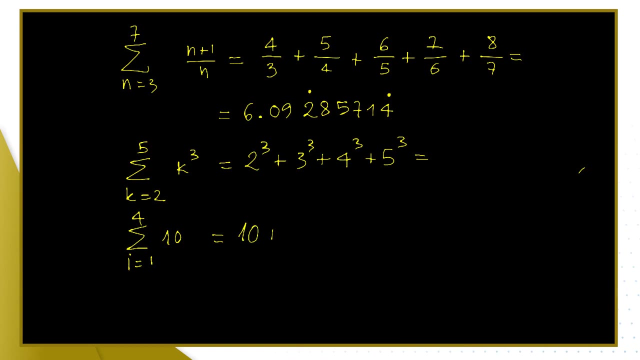 Now i is the index of summation. The number you're adding every time does not change with i. So you're adding 10 to itself as many times as i goes from 1 to 4.. So 10 when i is 1.. 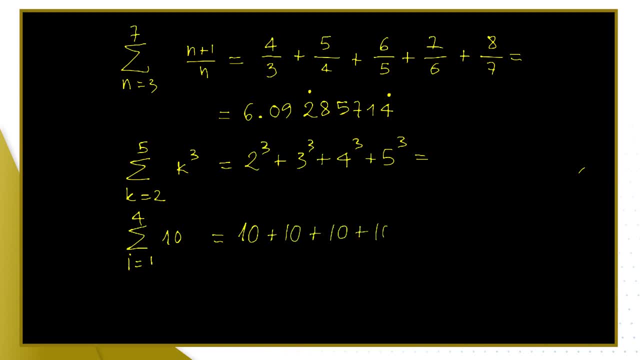 10 when i is 2.. 10 when i is 3.. 10 when i is 4.. Four times Four times 10 is 40. So in general, if you have a constant number added between, i equals 1 to 4,. i equals 1 to 20, it's that many times the constant number. 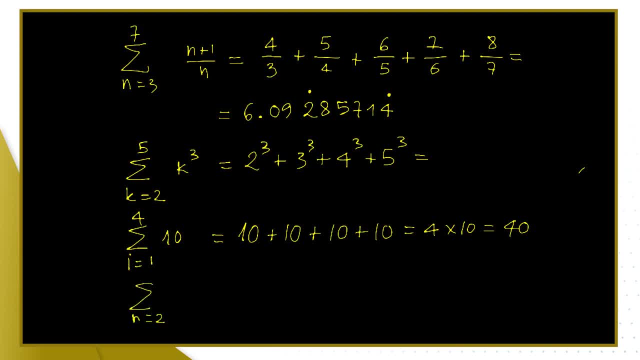 And the sum from n equals 2 to 6, of 2 to the power of 6 minus n, 6 minus n in the power. When n is 2, I've got 2. to the 4. When n is 3, I've got 2 cubed. 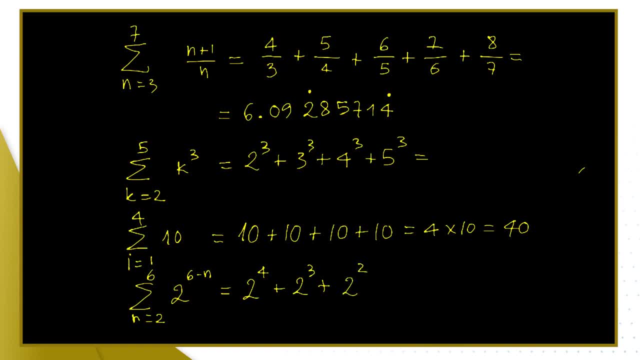 When n is 4,, I've got 2 squared. When n is 5,, I've got 2 to the 1.. And when n is 6,, I've got 2 to the 0, which is 1.. 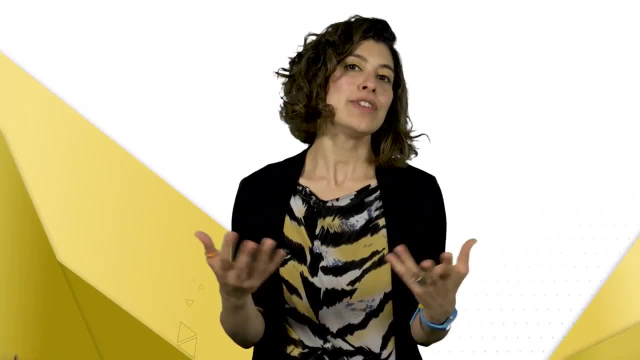 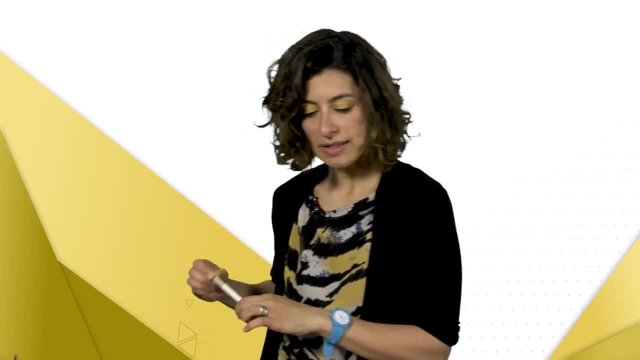 And then you can work that out as well. Let's now do the other way around. Let's start with sums and write it with a summation symbol. So if we're adding the odd numbers from 1 to 13.. 1 plus 3.. 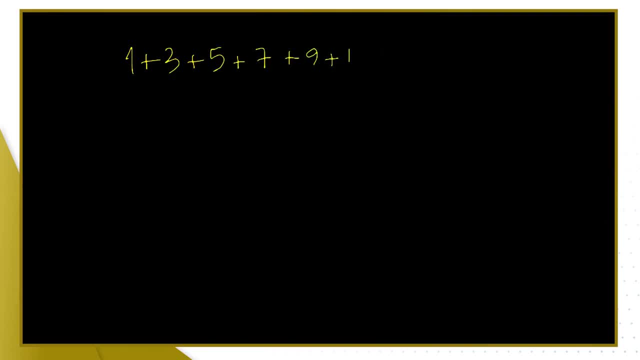 Plus 5. Plus 7. Plus 9. Plus 11. Plus 13.. This can be written as the sum, And now I need an expression that is going to generate all these odd numbers. Well, we start in 1 and then add 2 every time. 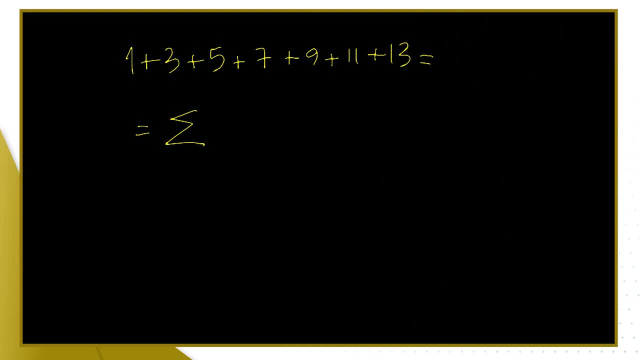 So that's an arithmetic progression with first term and common difference 2. It will be 2n minus 1 will do the trick, From n equals 1.. And now, how many terms? 1,, 2,, 3,, 4,, 5,, 6,, 7.. 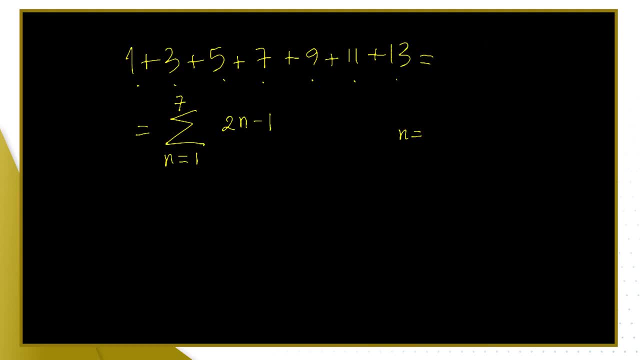 Let's check that. when n is 1,, we get the first term. When n is 1,, we get 2n minus 1 is 2 times 1, which is 2.. Take away 1, that's 1.. 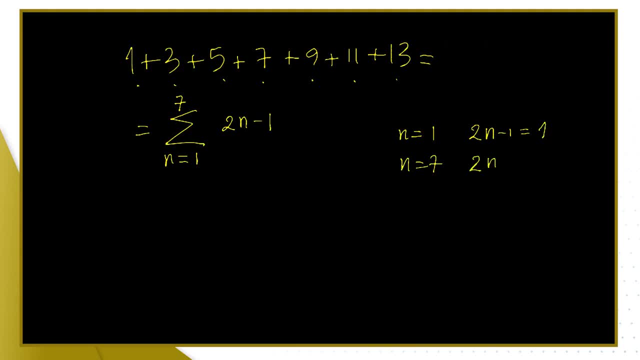 And when n is 7, we have 2n minus 1 is 2 times 7,, which is 14. Minus 1,, which is 13.. So, yes, those are correct, And I'll put brackets to make sure that the 2n minus 1 is all being added up in the series. 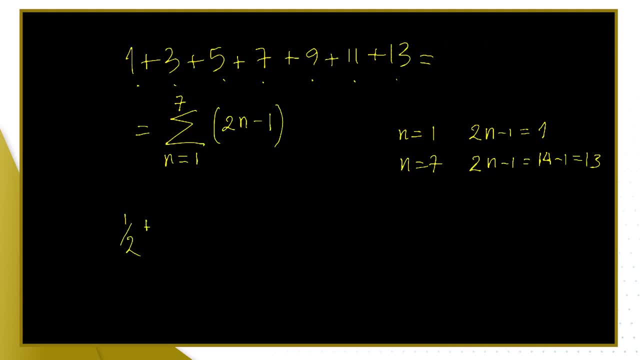 So let's now do a half added with a quarter added with an eighth, and so on all the way to 1 over 64.. So this is a geometric progression with common ratio: 1 half, with first term 1 half. So this will be: 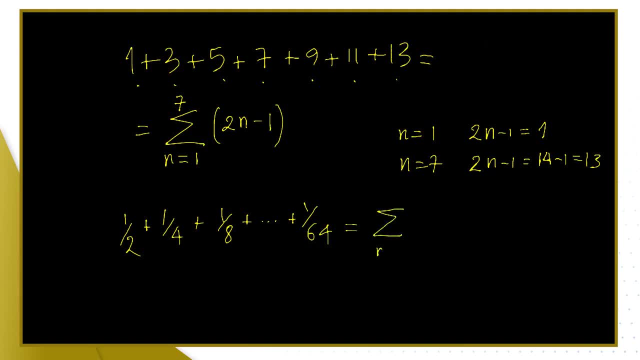 So this will be The sum. let's have a variable n, and we need a half to a certain power. Now we can simplify things by choosing a value of n that will give us a half on the first instance. So when n is 1, we get a half, and then we've got how many terms. 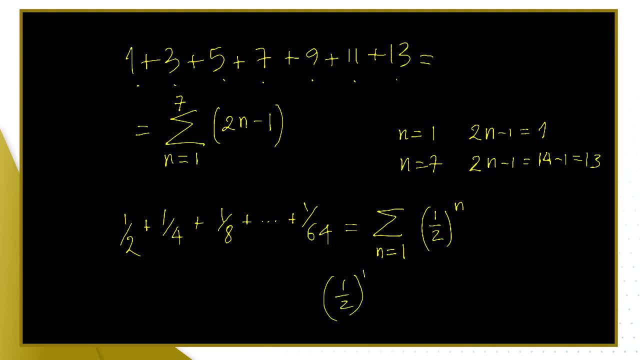 Well, we need to do: a half to the power of n equals 1.. So we just need to work out, when 2 to the n, what n makes, 2 to the n being 64. So 64, we've got 2,, 4,, 8,, 16,, 32,, 64. 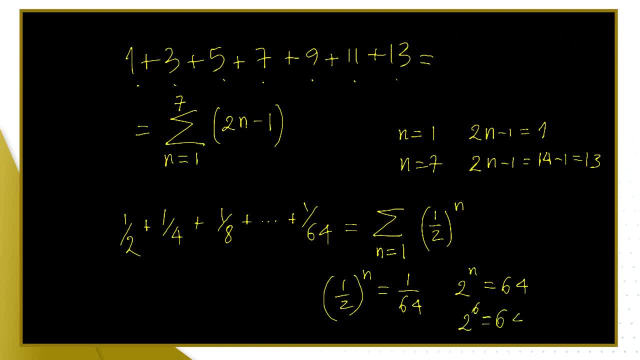 That's power 6.. So 2 to the 6 is 64.. So n is 6.. And there we are. So we wrote that sum of a geometric sequence, So a geometric series, So a geometric series with a summation symbol. 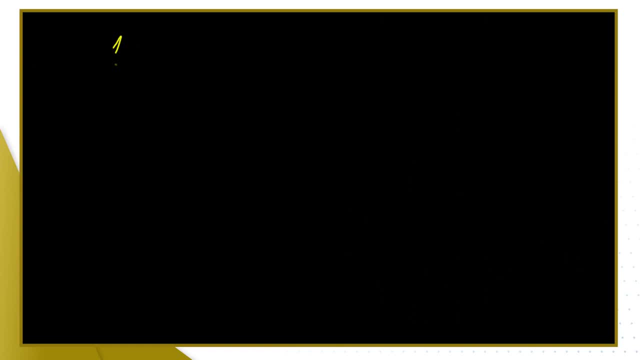 Let's do another one with alternating terms, as in positive, negative, positive, negative and so on. Okay, we've got this one That looks like a geometric progression. We're doubling every time, but not quite So. we're multiplying by negative 2 every time. 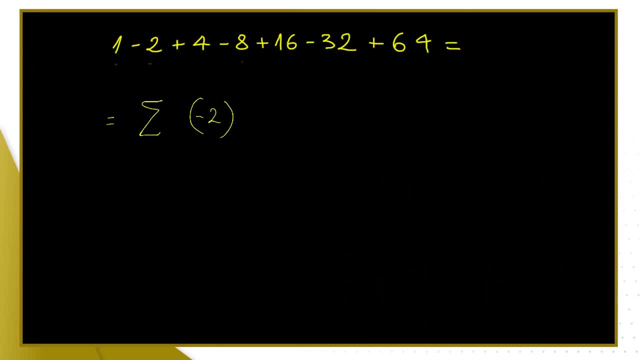 So we will have Minus 2 to some power. Let's put it n And then let's work out what will be the value of n, to give us 1 to start with, and then minus 2 next. So if n is 0, minus 2 to the 0,, it's 1.. 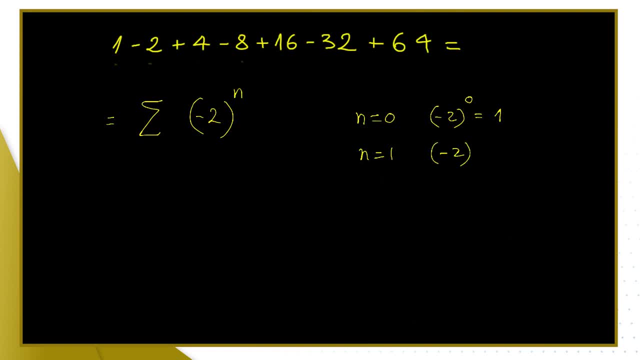 So that works. And then when n is 1, minus 2 to the 1 is negative 2.. So that's fine. So n equals 0, we'll give that guy. Then n equals 1. And all the way to 64.. 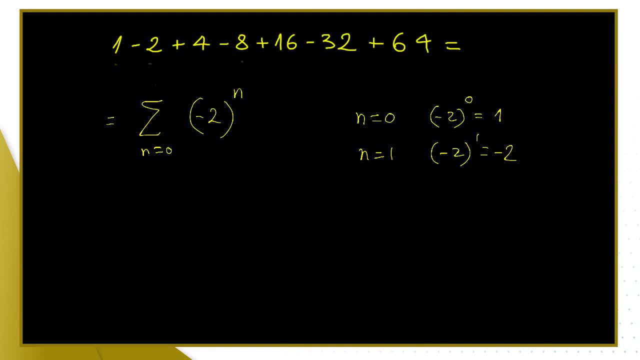 But we can just count the numbers, So 0, 1,, 2,, 3,, 4,, 5,, 6.. Okay, Or we could use the same technique- we're using the other one- to work out the power of 2.. 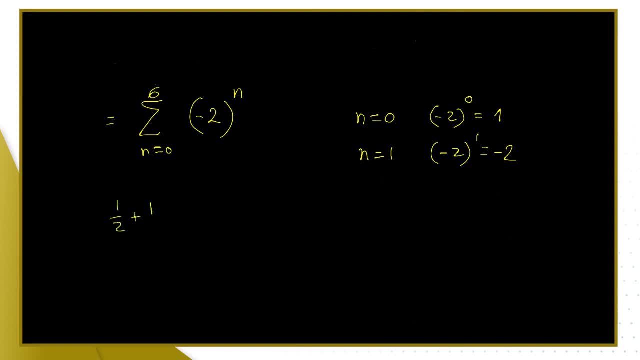 Another one: 1 half plus 1 third plus 1 quarter plus 1 fifth plus 1 over 6.. That one It's actually called harmonic series. We're having 1 over a number that is increasing. that denominator is increasing. 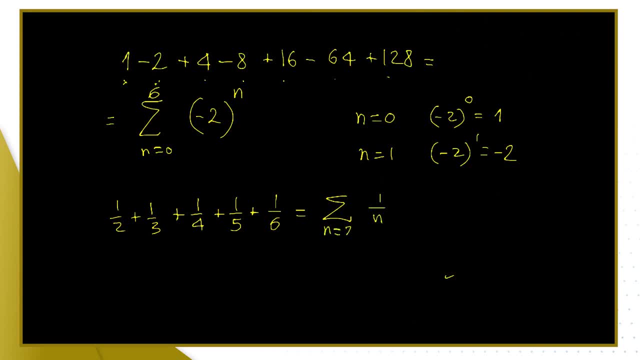 So we have 1 over n and n begins in 2 and ends in 6.. Now be very careful of division by 0. They'll make n equal 0 in that one. And one more Say we're adding 4 plus 9 plus 16 plus 25 plus 36.. 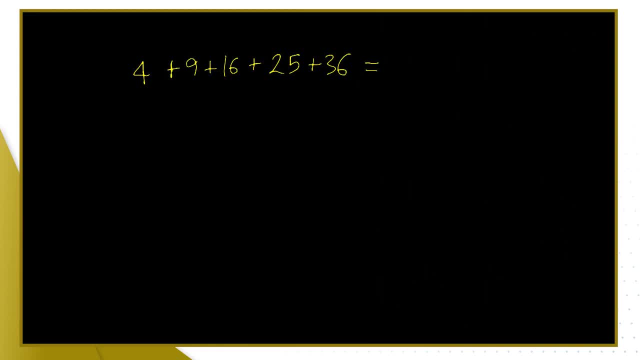 And those you'll probably recognise. there are square numbers: 4 is the square of 2.. 9 is the square of 3.. 16 is the square of 4.. 25 is the square of 5.. 36 is the square of 6.. 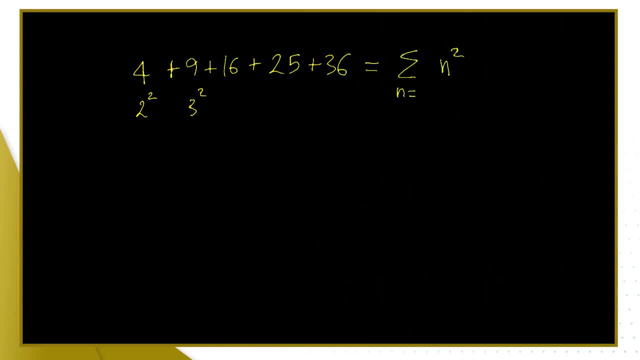 So we're doing squares of numbers, And the first square is the square of 2.. And the last square is the square of 6.. Because the summation symbol has behind it a sum. we can add and subtract and multiply by a constant these sums. 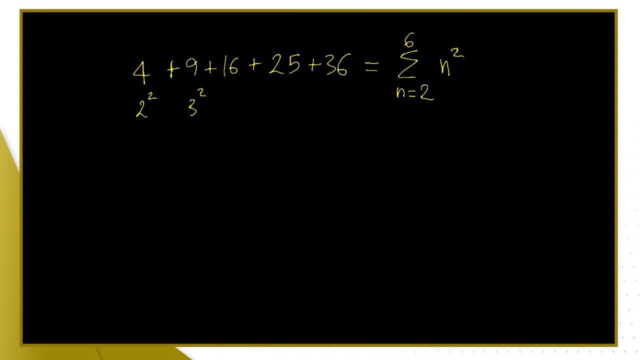 So we can do things like if I have the sum of n plus 2 to the n and my n is ranging from 1 to 4, I can, because I'm adding the n and the 2 to the n inside the bracket. 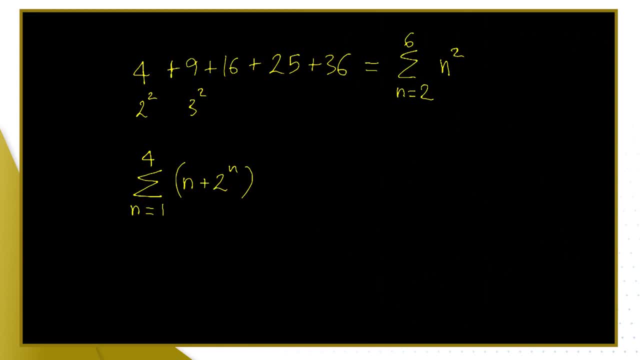 I can separate the sums. I can say I can add the n and I can add the 2 to the n. but I need to be careful with the variable. It's from 1 to 4, and it's from 1 to 4 on both. 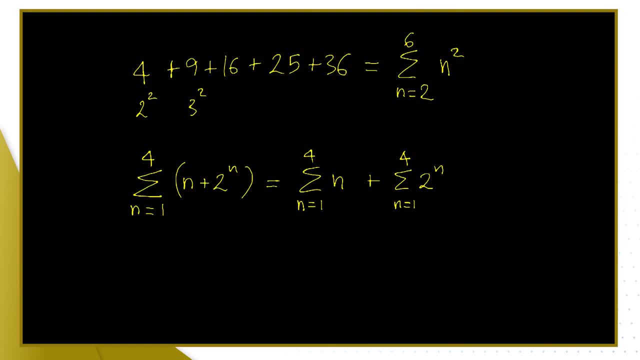 So basically what I'm saying is that if I'm adding 1 plus 2, when n is 1, and then 2 plus 2 squared plus 3 plus 2 cubed, plus 4 plus 2 to the 4,, 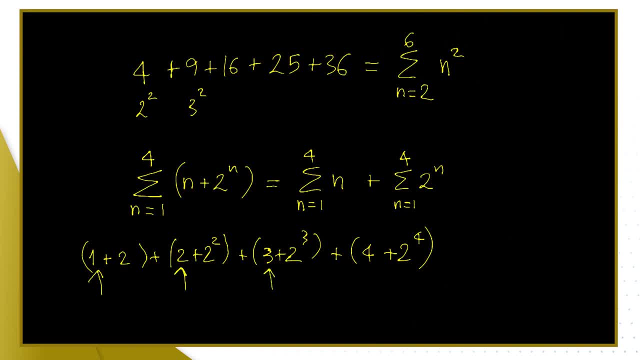 I can choose. I can choose to add the 1 with the 2, with the 3, with the 4 in one summation and the 2, 2 squared, 2 cubed, 2 to the 4 in another summation. 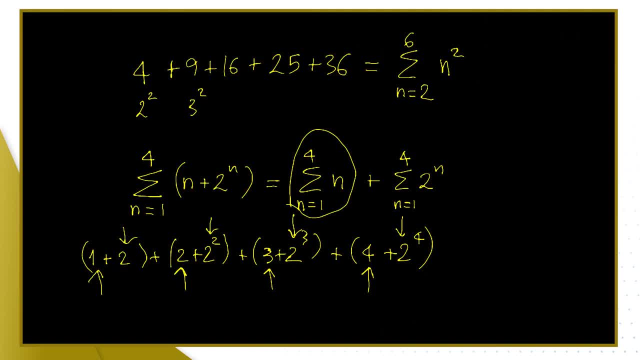 And that's why I did one summation for the 1,, 2,, 3,, 4, and another summation for the powers of 2.. We can do that, and we can also do the subtraction of two summations. 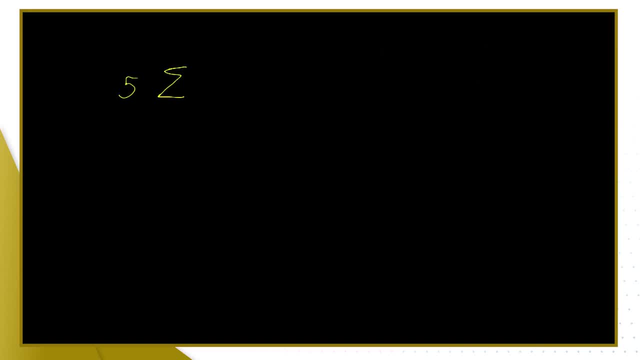 We can also do 5 times a sum. Let's say we have n plus plus 2 to the power of n and my n could be ranging from 2 to 4.. If I multiply everything by 5, that is the same as saying I have the sum of multiplying the number inside. 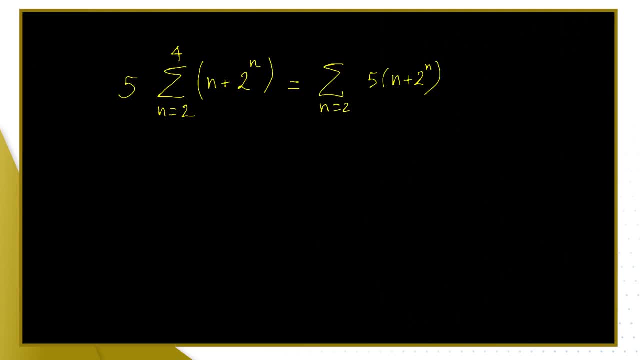 the expression inside by 5.. Okay, So that is saying, if I've got 5 times the sum, that it's 2 plus 2 squared, which is the first one. n is 2, plus 3 plus 2 cubed. 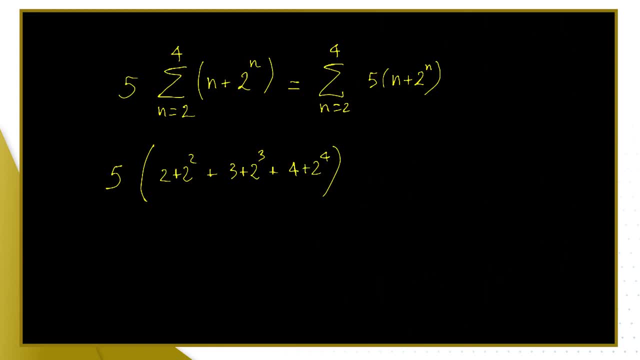 plus 4 plus 2 to the 4,, along with these little brackets here, is the same as doing the sum of every single term multiplied by 5.. I'm just saying I can do 5, 2 plus 2 squared. 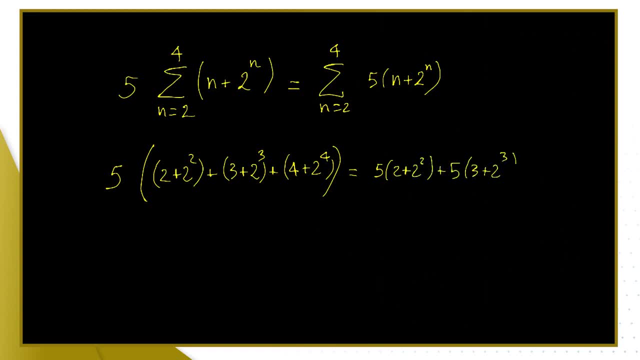 plus 5, 3 plus 2, cubed plus 5, 4 plus 2 to the 4.. So that's what that means: putting the constant inside the summation or outside the summation. Now, what's really important is that when we multiply two sequences inside the summation symbol, 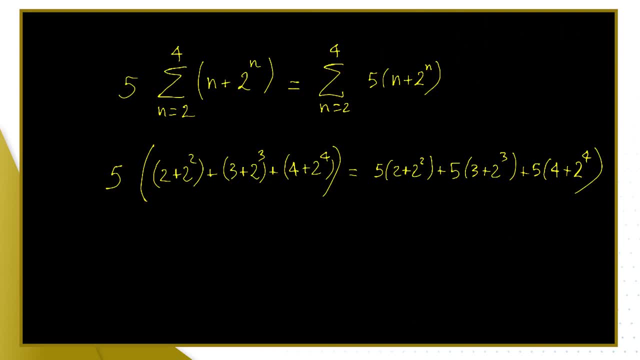 that is not the same as multiplying the summations. It is not So. what I'm saying is that if you have n times 2 to the n and you're doing this sum, this is not the same as multiplying the summations. 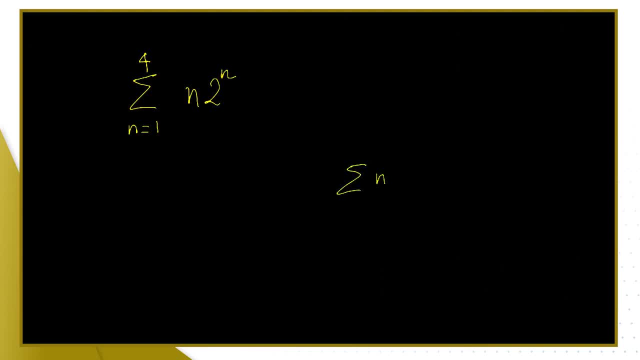 It is not, not the sum of n times the sum of 2 to the n. It is not the same. okay, And the way you can look at that, expand this sum, expand this sum and then multiply the results together. 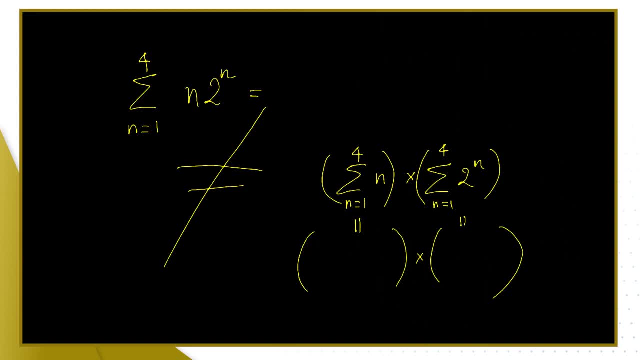 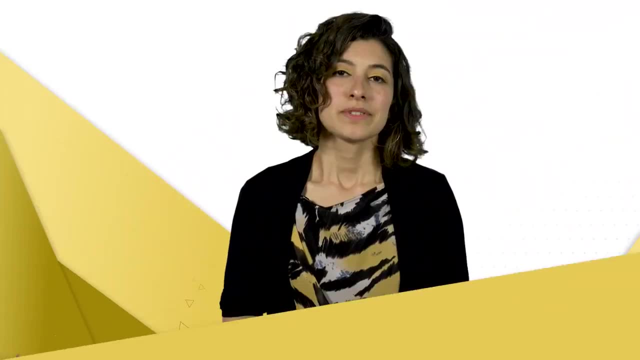 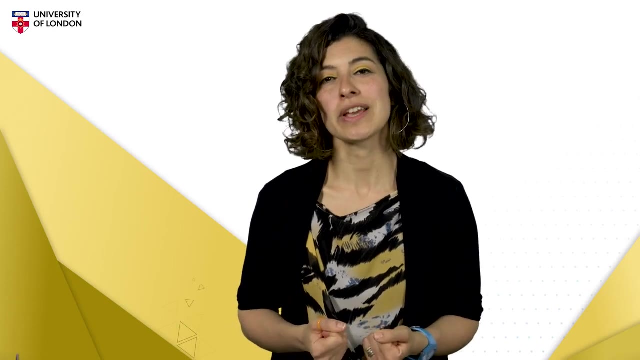 and you'll see it is not the same. You may find one or two examples where they are, but in general they are not. So now join me in exploring all these concepts in more detail and answers to some of the questions raised in the next videos. 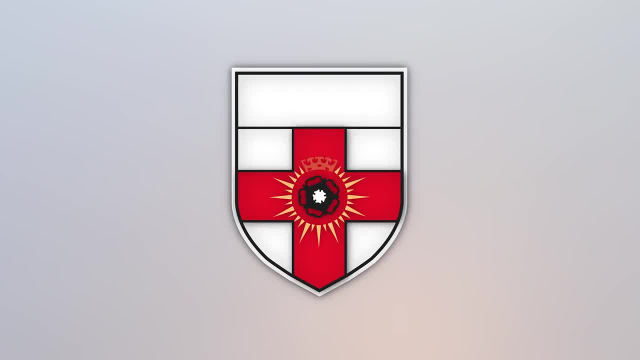 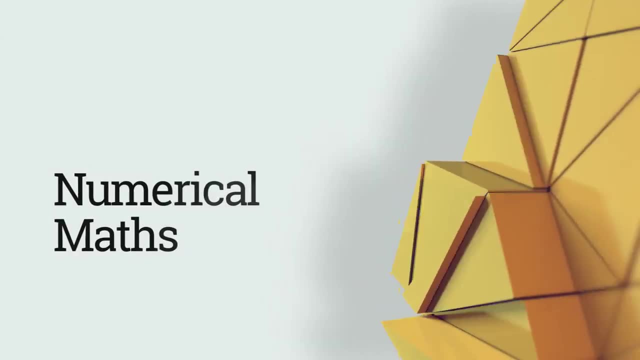 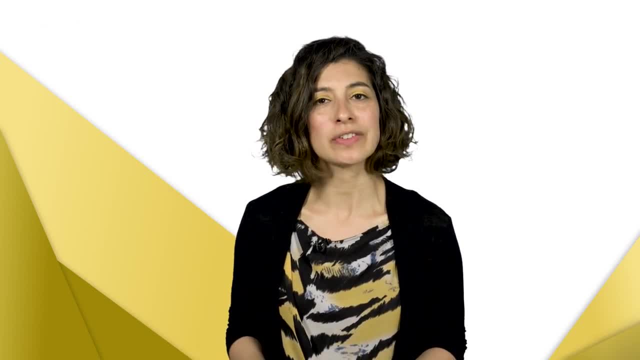 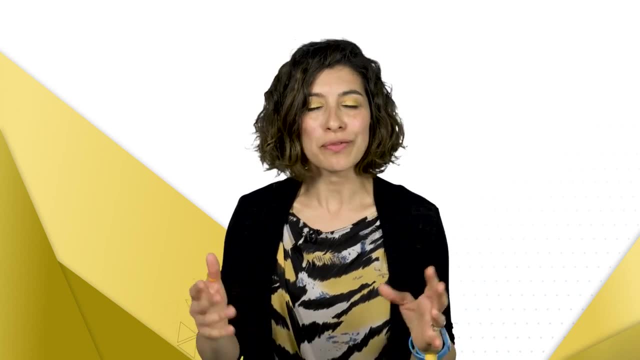 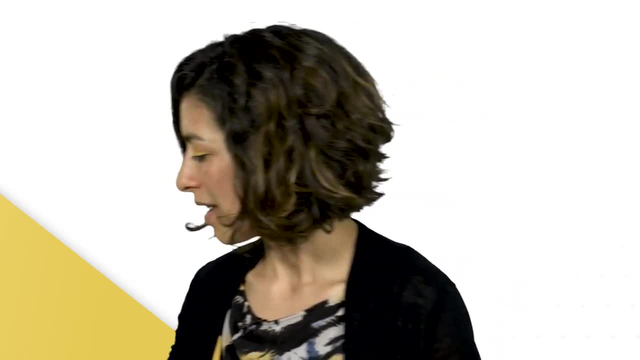 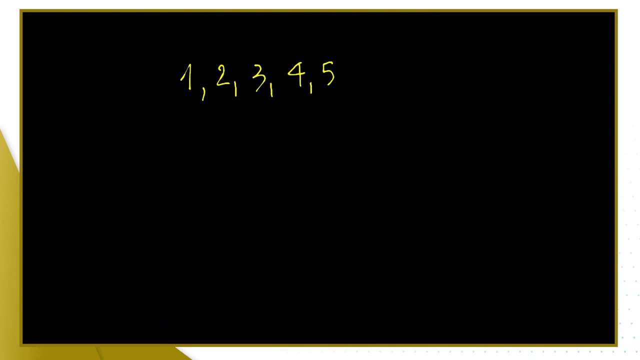 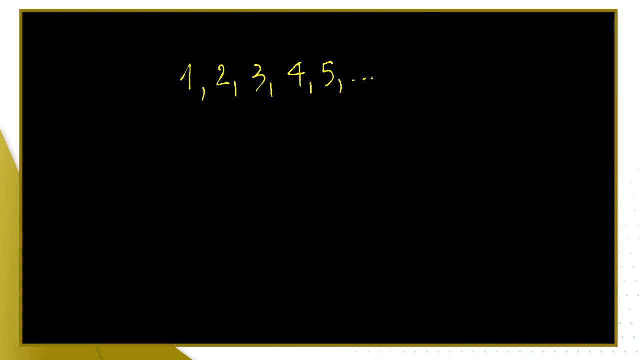 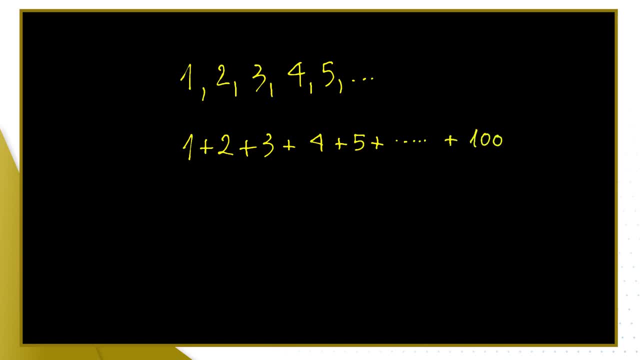 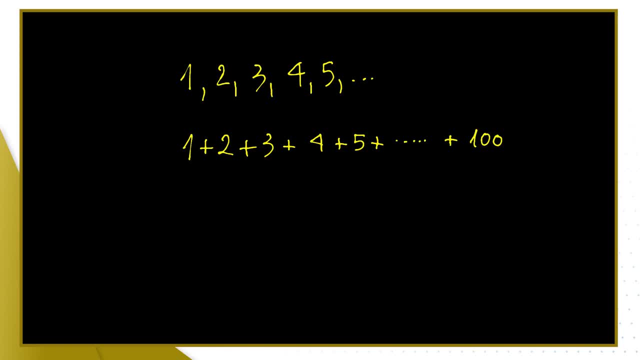 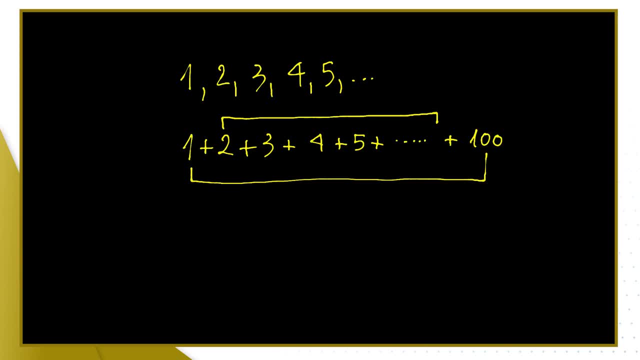 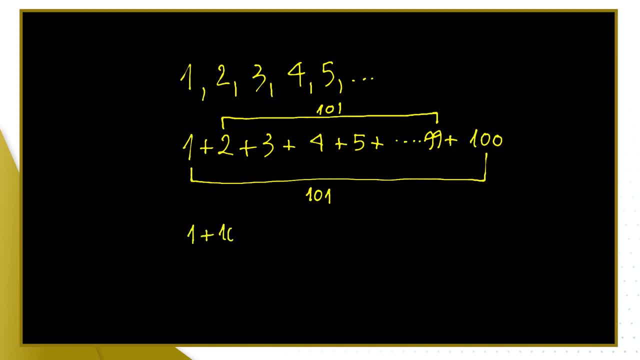 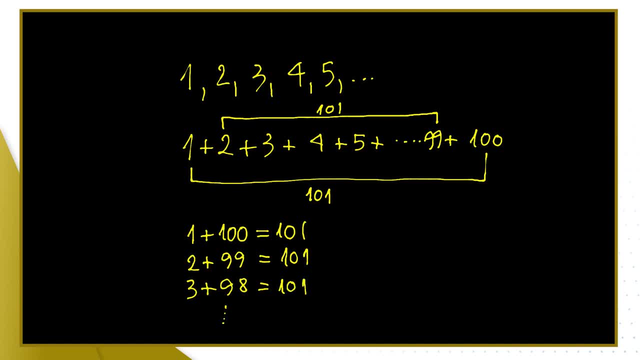 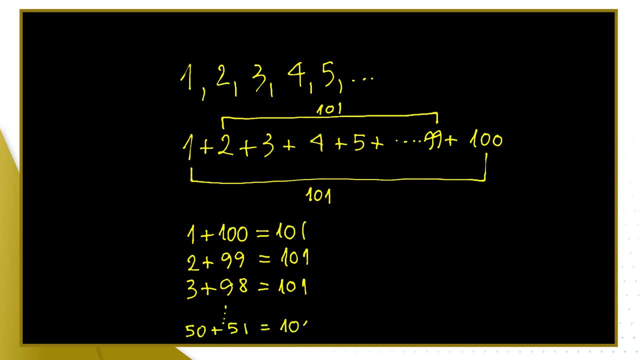 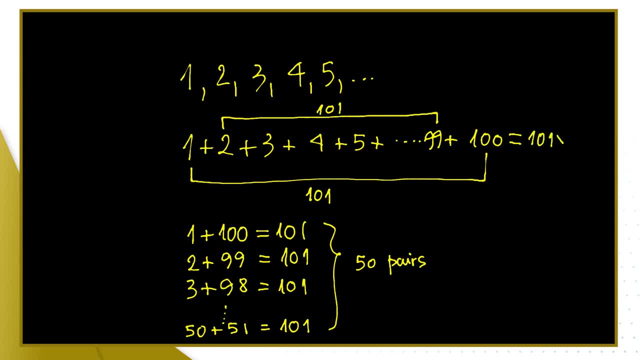 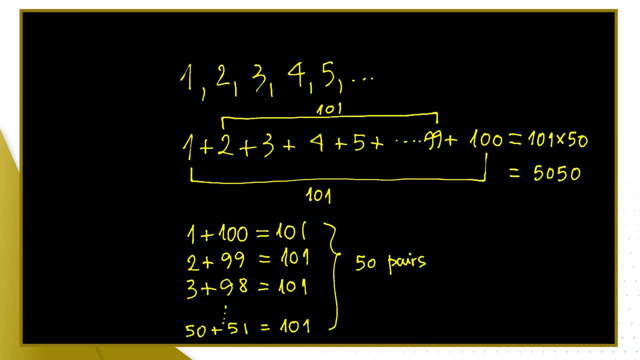 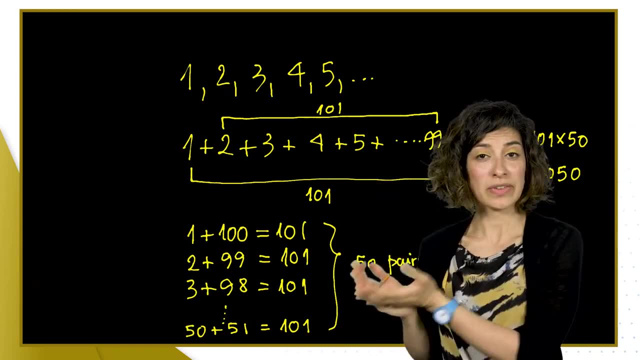 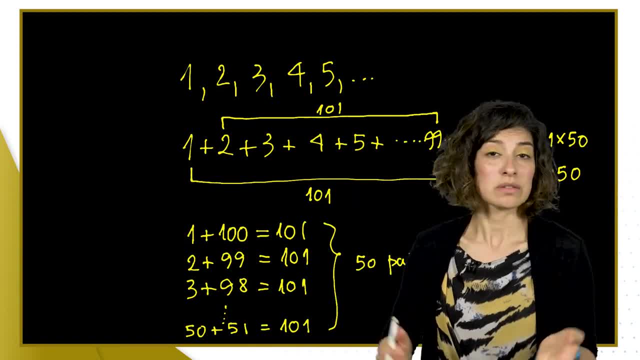 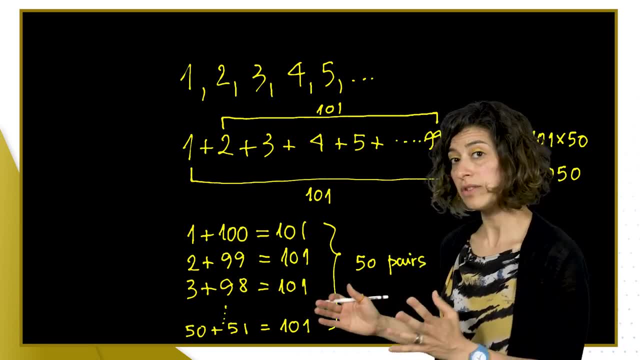 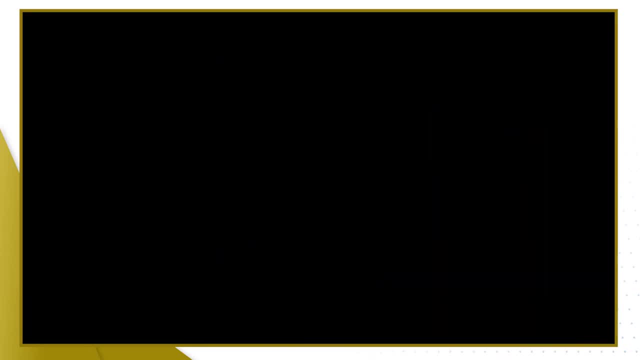 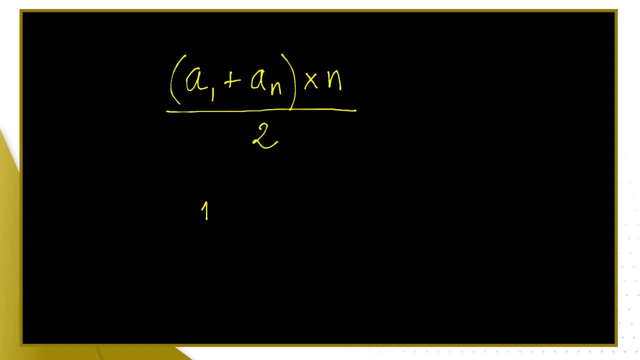 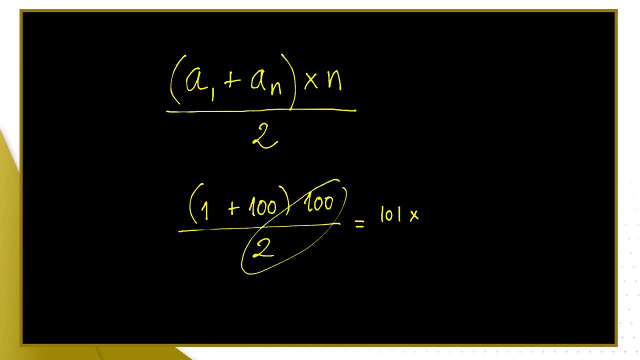 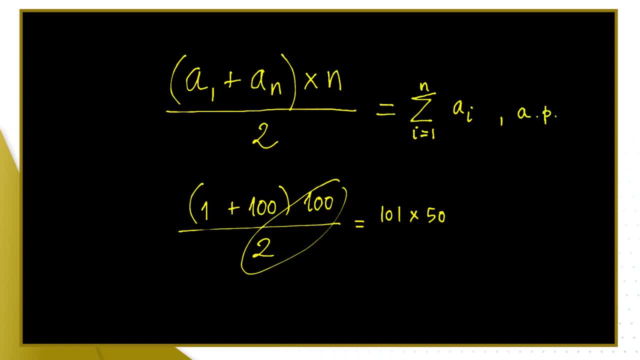 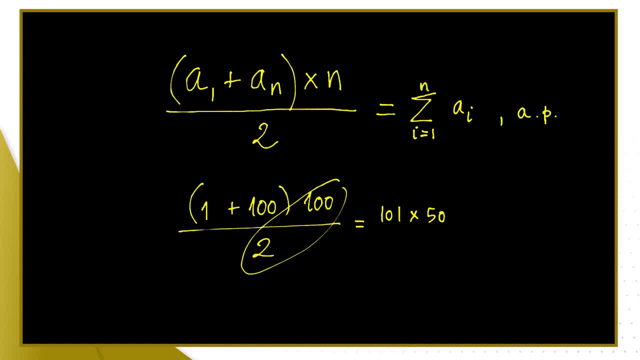 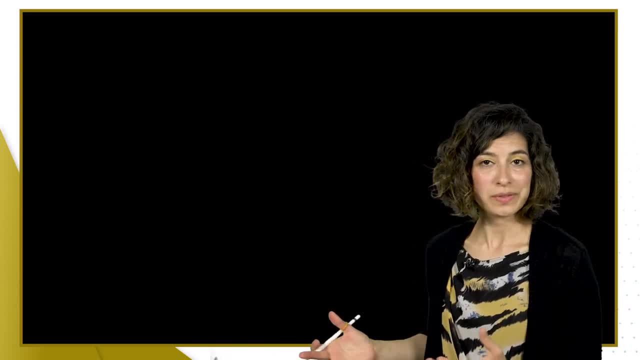 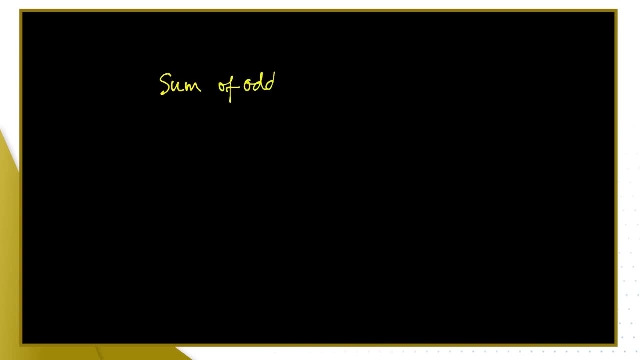 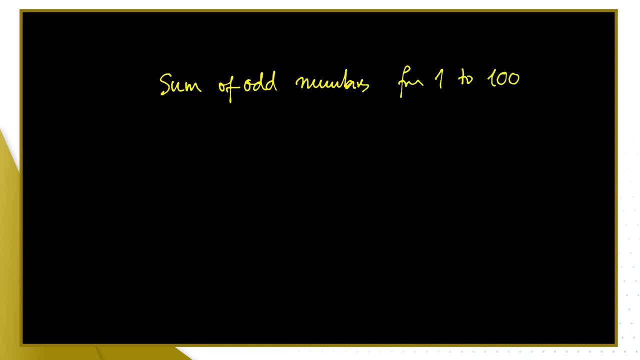 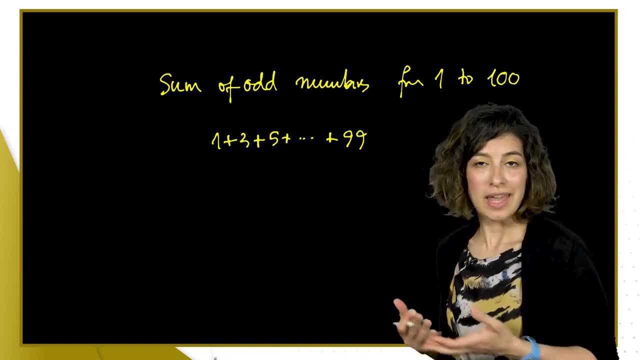 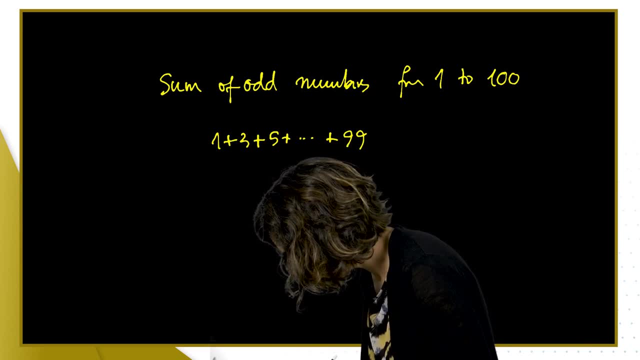 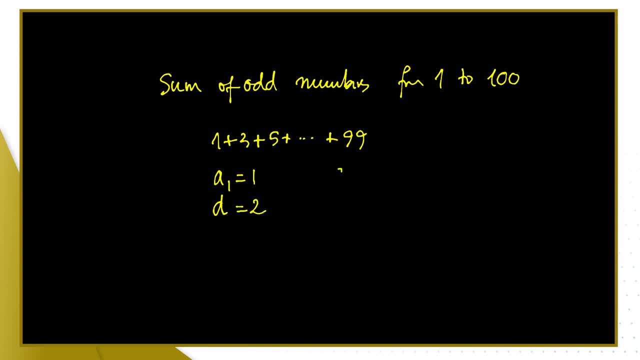 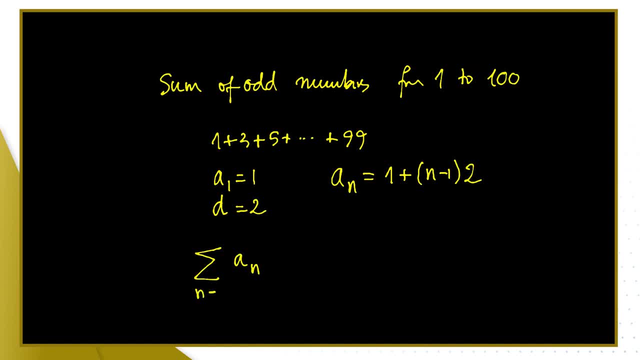 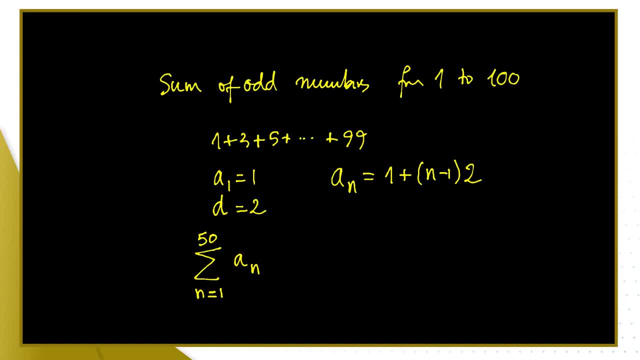 Subtitles by the Amaraorg community: 2 plus 1, and that gets us 99,. okay, So this is given by the first term plus the last times, 50,, which is the number of terms divided by 2.. So that means I do 1 plus 99,, which is 100,. 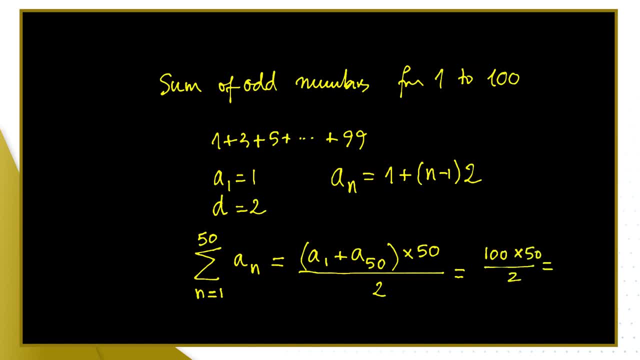 times 50, divided by 2, that's 50 times 50,, which is 2,500.. Pretty neat. If I wanted the sum of even numbers from 1 to 100, I'm looking at adding 2 plus 4, and so on. 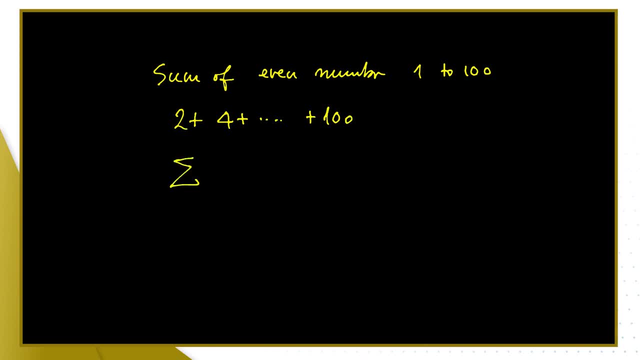 all the way to 100.. I want to write it as a sum of an arithmetic. and I want to write it as a sum of an arithmetic and I want to write it as a sum of an arithmetic progression. and let's write what's bn, and bn is going to be 2 plus n minus 1 times the common. 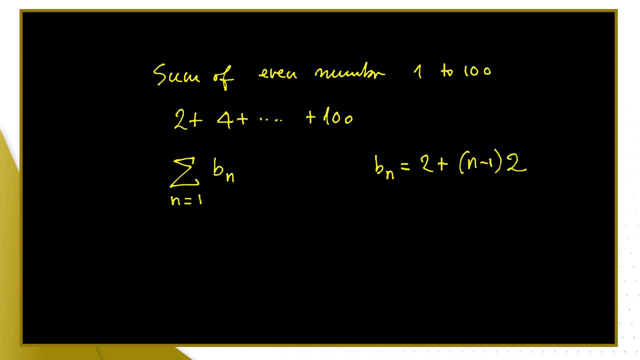 difference, which is still 2 in this case, and the last term is 100, and I achieve that when n is 50, because I start with 2 and I add 49 2s to it to get 100, so it's also the sum to 50,. 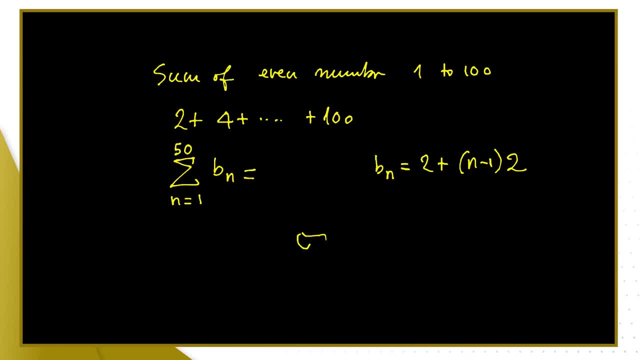 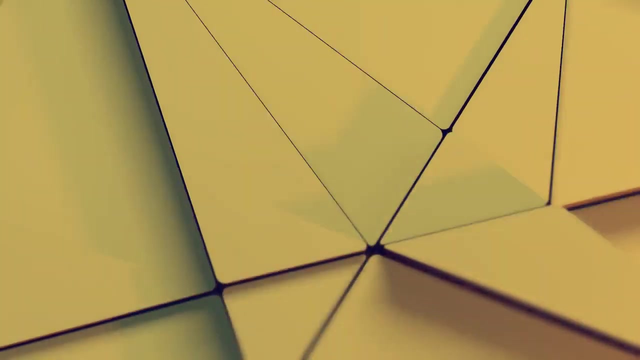 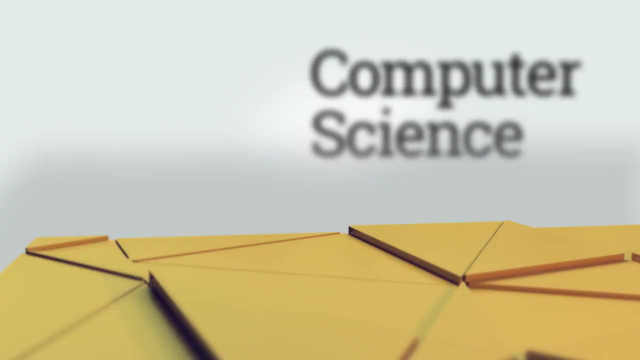 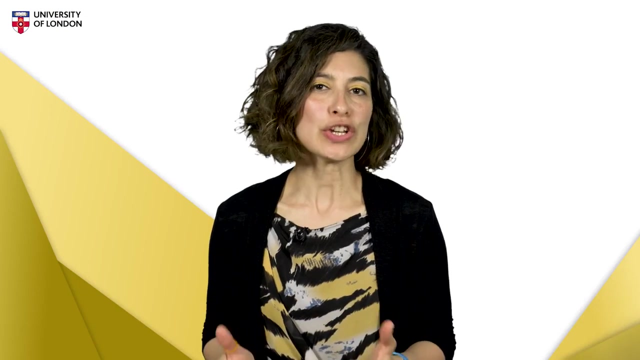 and therefore this result is the first term plus the last, that's 102, times 50,, divided by 2, and that turns out to be 51 times 50,, which is 2,550.. Let's now look at the sum of a geometric series. 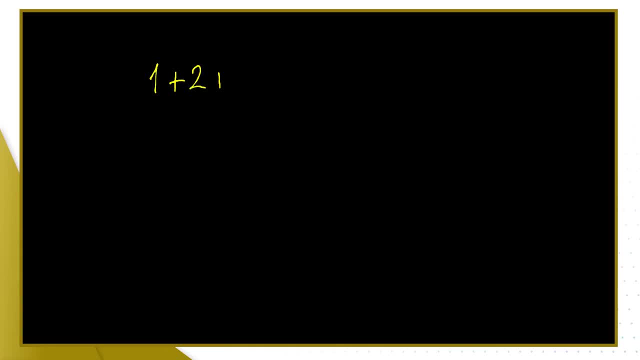 Let's say we have 1 plus 2 plus 4 plus 8, and so on, all the way to 1024. to add up The sequence we are adding in this series. it is a geometric progression. it begins in 1,. 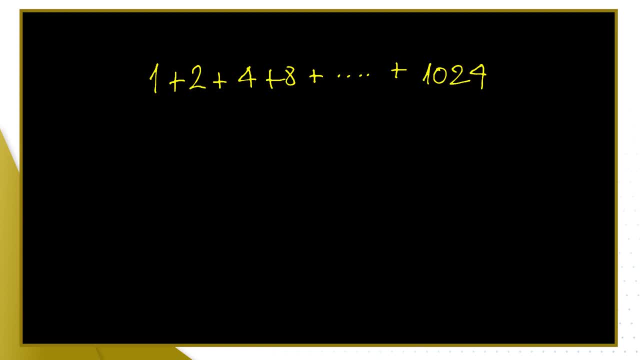 and the common ratio is 2, it is a doubling sequence. The general term is bn, which is 2 to the power of n minus 1, and we want to add all the terms all the way to 1024.. We need to work out how many terms that is to start with. 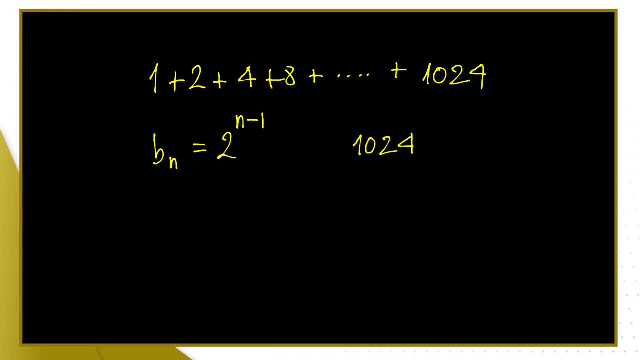 So 1024 is 2 to the power of 10.. We are adding 2 to the 0,, 2 to the 1,, 2 to the power of 10, that's 11 terms. So we want to add bn from n being 1 all the way to n being 11, so it's 11 terms. 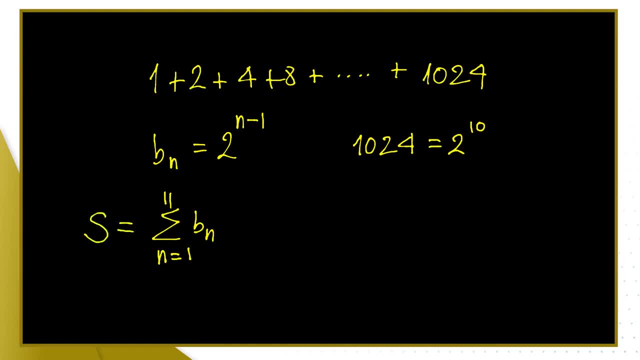 So let's say for now, we're going to call this sum big S And I'm going to write it on top as well. So that is our sum. It's kind of a clever little trick to work out this sum. We want to multiply the sum itself by the common ratio by 2, because this is a doubling geometric progression. 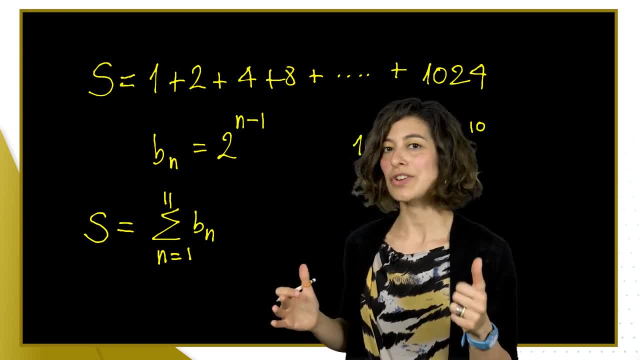 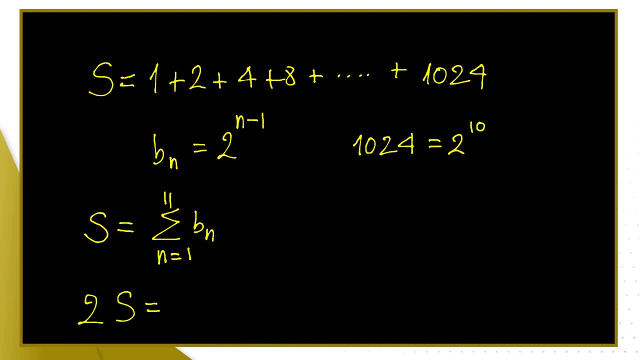 So we're going to multiply that sum by 2, and that's going to help us. Let's see So 2s. and for us to appreciate the pattern, let's use the sum at the very top Twice. the sum is going to be twice every term. 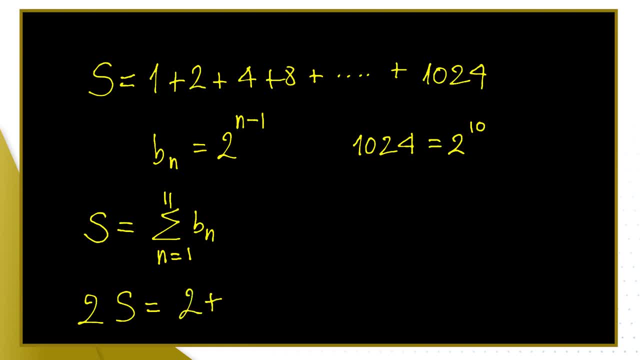 So I'm going to add 2, which is twice over the sum, which is twice of 1, I'm gonna add 4, which is twice of 2, twice of 4, twice of 8, all the way to twice of 1024.. And now let's compare the two, let's compare the. 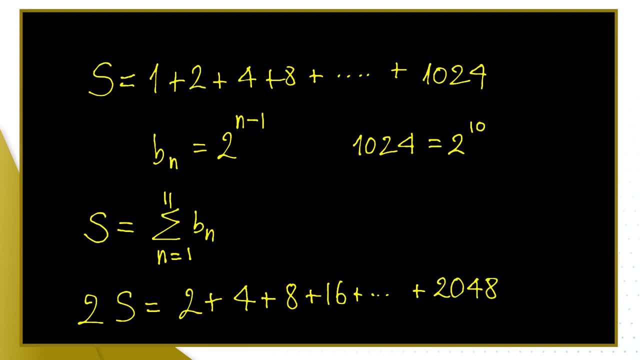 sum and twice the sum. Most numbers are the same as in. I've got numbers from 1 to 4, all the way to 1024, and 2s goes from 2 to 4 and so on, and here there's a 1024 as. 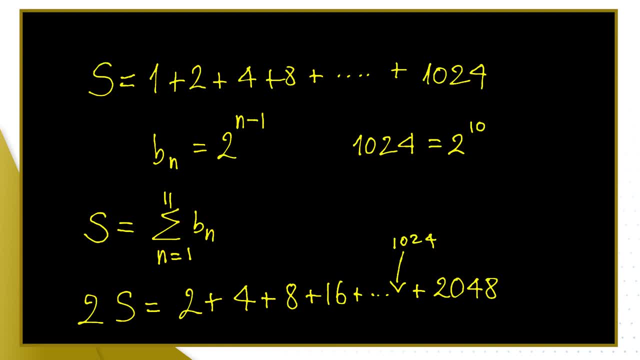 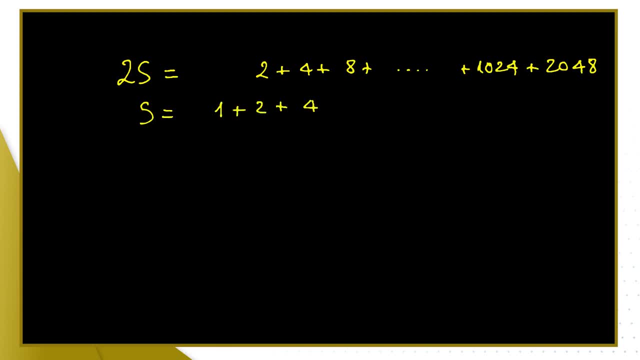 s is 1 plus 2 plus 4, and so on all the way to 1024,. and now, if I subtract s from 2s, I'm gonna subtract 1,024 from that 1024.. I'm gonna subtract all these numbers here in the middle and these: 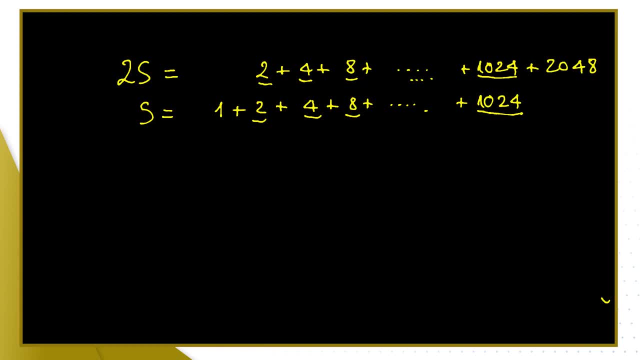 two and these two and these two. So those are all gonna cancel out and I'm gonna end up with 2048 minus the 1.. So 2s minus the s is gonna end up being 2048, take away 1.. But all we did was to 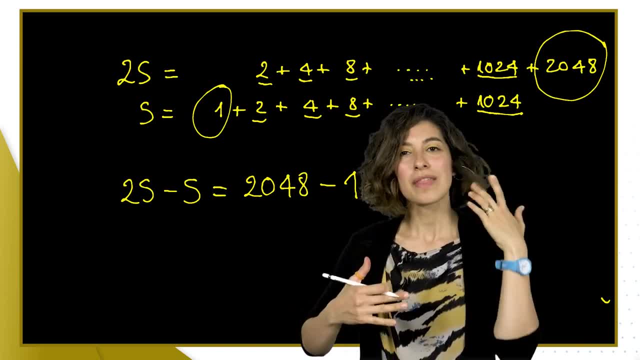 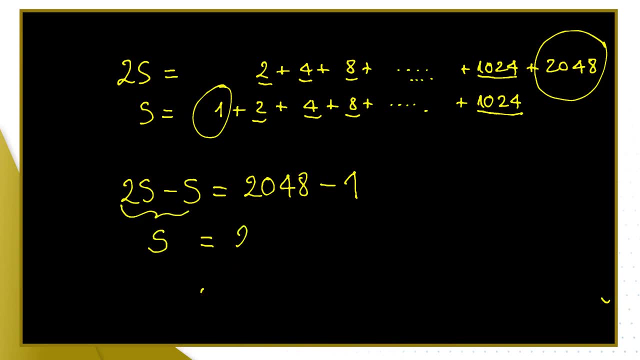 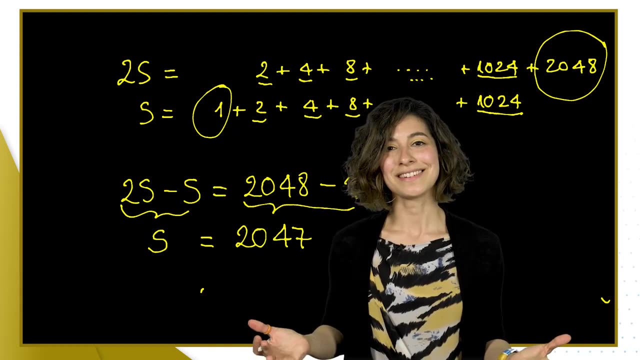 start with twice the sum and subtract the sum. that means I just got one sum here, So this is the value of the sum and that is going to be 2047 from here. And it's done. We didn't have to add up all those numbers. This is the shortcut. 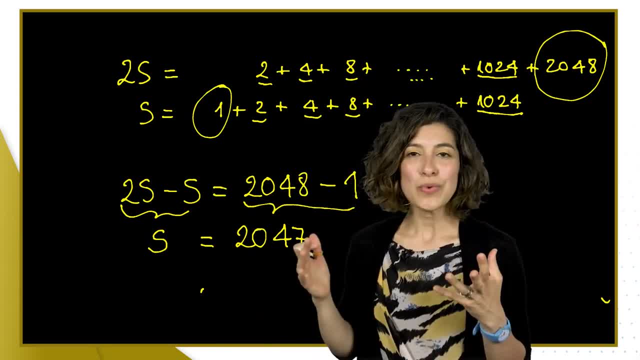 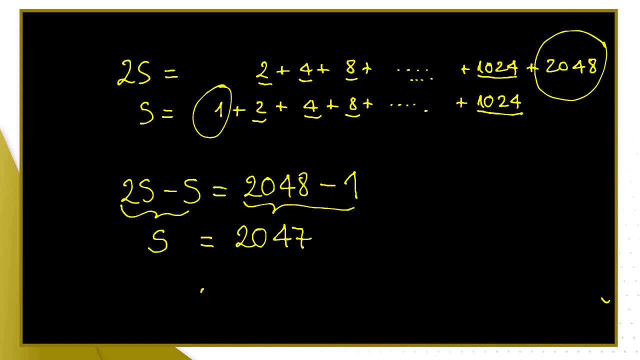 The good news is that this also applies to any geometric progression, not just to the one we saw, And the same method is done. I'm going to write down the general case. So, if we are doing the sum of a geometric progression that starts in 1,, 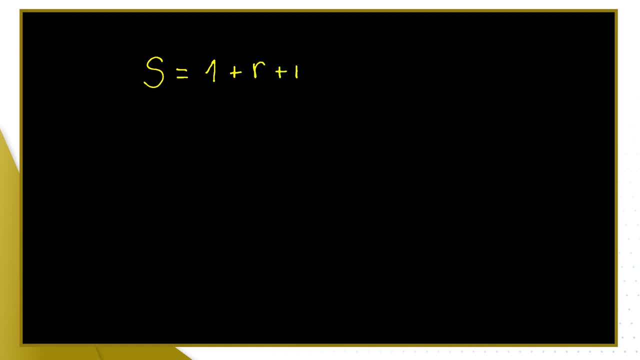 and then there's ratio r. these are going to be the terms and I'm going to add n terms of this series. so the last term is r to the n-1.. The trick I did was to multiply the sum by the sum of all the terms, and then I'm going to write down. 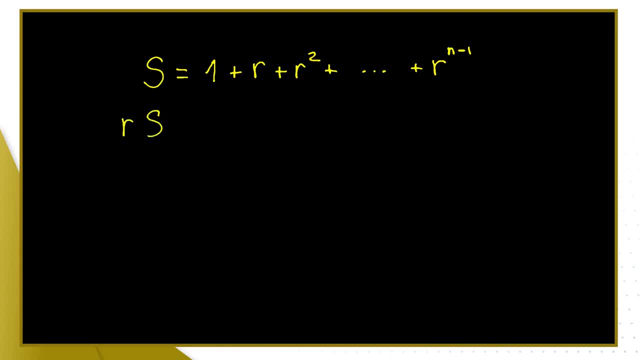 by the common ratio. So I'm going to do r times s And as I do that, I have the one on the sum times r. so I'm going to have r. The r of the sum times r is going to be r squared, and so on. Every term above is going to be multiplied by r. But I have as 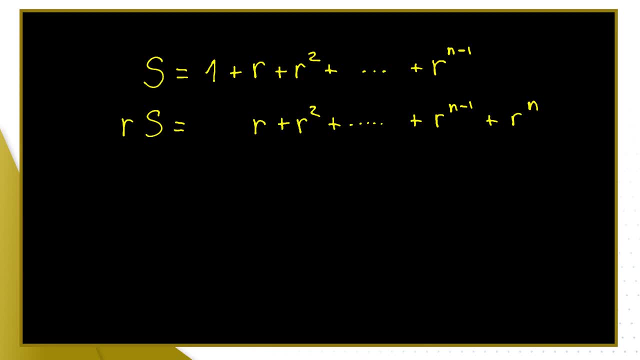 many terms in one or the other. So the last one is r to the power of n, And now I'm going to subtract. I'm going to do rs take away s, And that means these here will cancel out, so they'll subtract to zero. The same with everything in the middle. 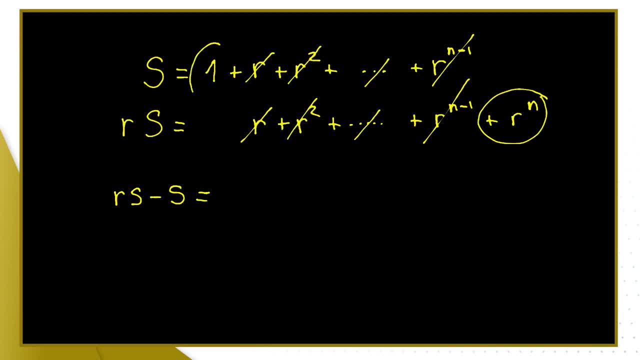 And I'm left with r to the n. take away the 1.. Now let's look at the left-hand side. This is r times s minus s. so that is r. take away 1 multiplied by the sum and the right hand side. I've got r to the n minus 1.. I can divide both sides of the equation by r minus 1, and. 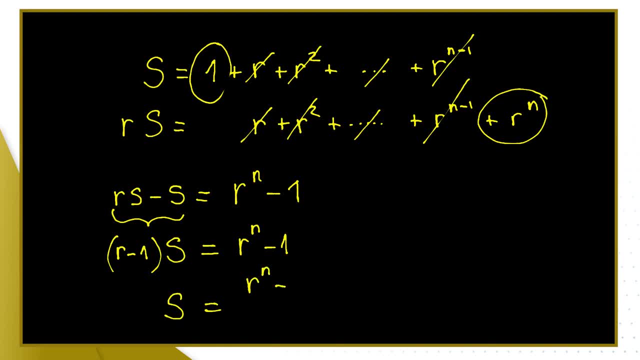 so I have that s is r to the n minus 1 divided by r minus 1.. Of course, if r isn't 1.. If r was 1, we didn't need this formula to add it up. It wouldn't be an interesting geometric. 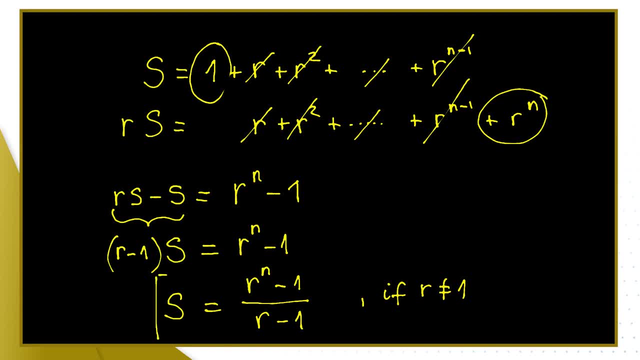 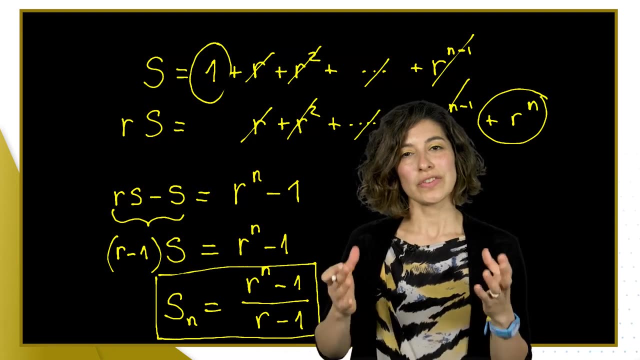 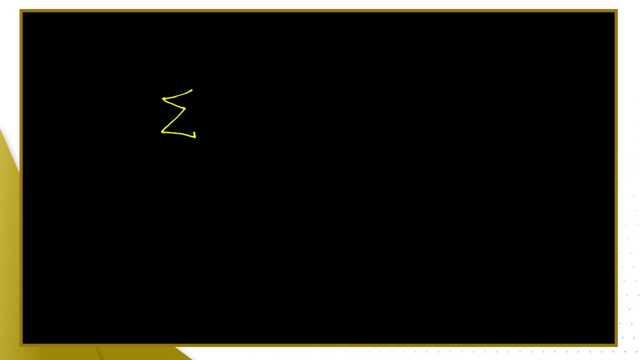 progression. So this is the sum of n terms of a geometric progression. I'm going to write s with a little n underneath. Of course we are using the series notation, so the series notation will have the big sigma. so I'm going to rewrite that as the sum of the powers of 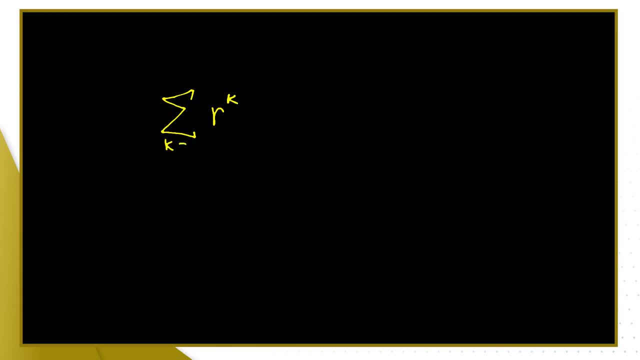 r All the way from 0 to n minus 1.. Remember we were doing 1 plus r plus all the way to r to the n minus 1, so those are the limits of my sum. This is given by the formula we. 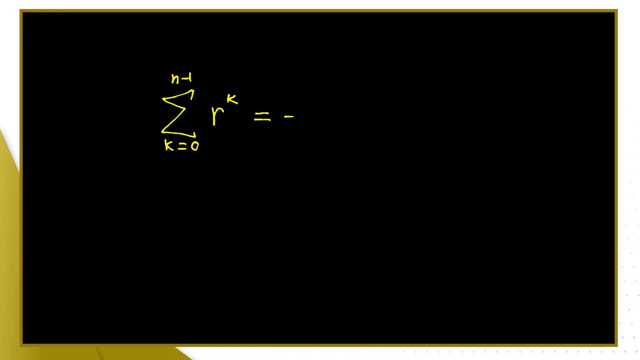 just wrote, which is r to the power of n. take away 1 over r. take away 1, provided r isn't 1.. So that is the sum of a geometric series. Let's just see that formula applied to the sequence we just added up When r was 2, the sum of 2 to the k, k running from 0. 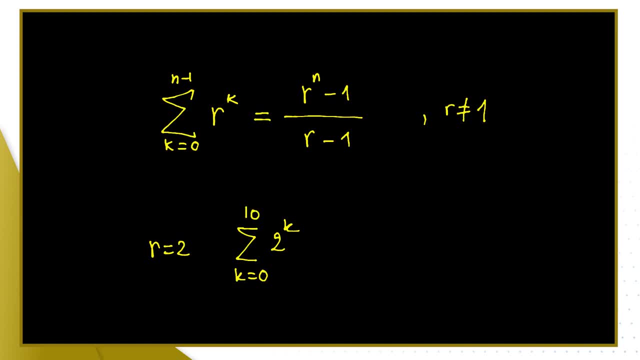 to 10.. I know we wrote k going from 1 to 11 on the other example, but we are using the expression of 2 to the k, So this is the same value. This is using the formula 2 to the n. n here is 11, minus 1,. 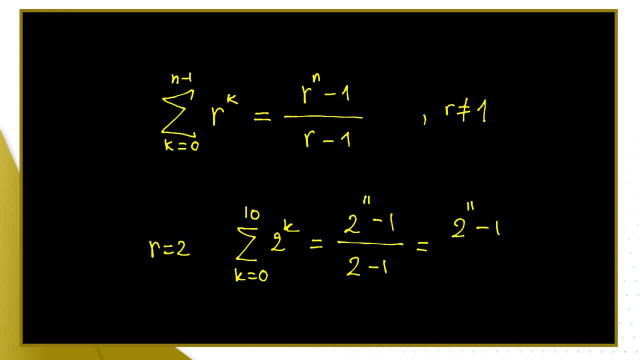 2 minus 1, and that is 2 to the 11. take away r1, because the denominator is 1, and that is our 2048. take away 1, as we had calculated before. Let's look at another couple of examples. 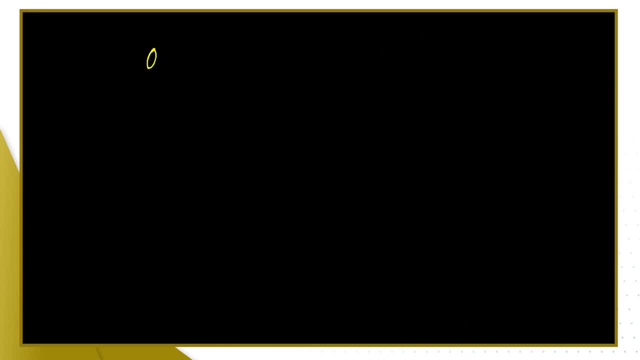 Say, we've got the sequence 0.3, 0.06, 0.012, and so on. It is a geometric progression, The common ratio is 0.2, and we you would verify that by doing 0.06 divided by 0.3.. And that is 0.2.. And we'll be back, And we'll be back 0.6, 0.12, 0.12, 0.3.. We're going to verify that. We're going to verify that by 0.03.. 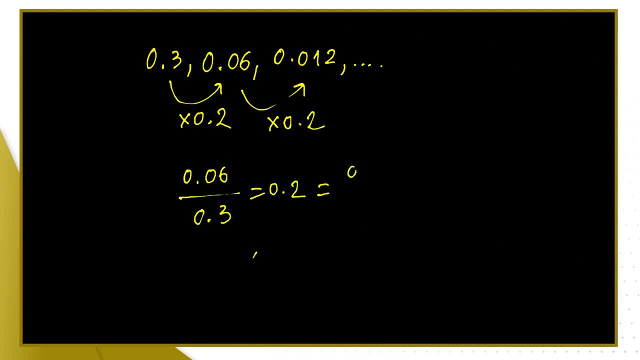 We're going to verify that. We're going to verify that by 0.03.. We are going to verify that by 0.03.. 0.2 and it's the same as 0.012 divided by 0.06,. okay, So it is a geometric. 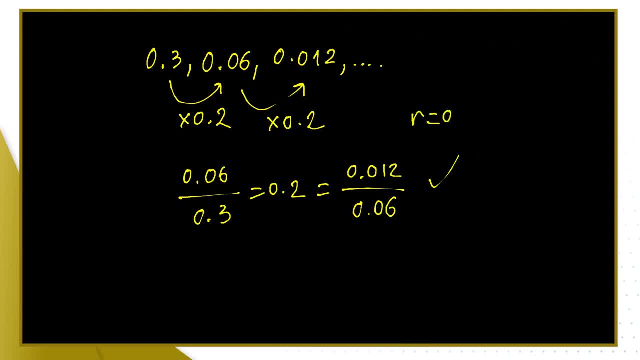 progression with ratio 0.2.. Let's add the first five terms of that series. So we want to add a n when n goes from 1 to 5.. And here what we do is we note that this series is not exactly powers of the ratio, But the ratio is 0.2.. The 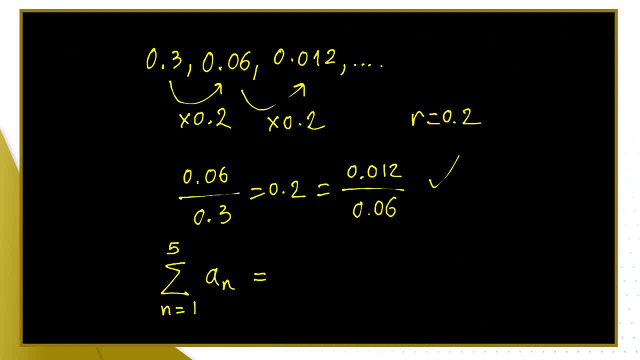 general term of the sequence. we're going to write it up here. The general term for the sequence is an equals 0.3 times 0.2 to some power. Well, when n is 1, I'm not multiplying by 0.2,, it's only when n is 2, so I'm going to do. 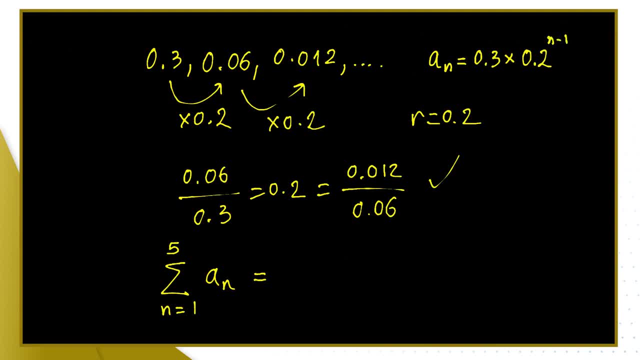 n minus 1.. And so the sum I've got here, the series I've got here, is 0.3 times the sum of 0.2 to the n minus 1.. So that is 0.3 times 0.2 to the power of 5,. take away 1, over 0.2, take away 1.. 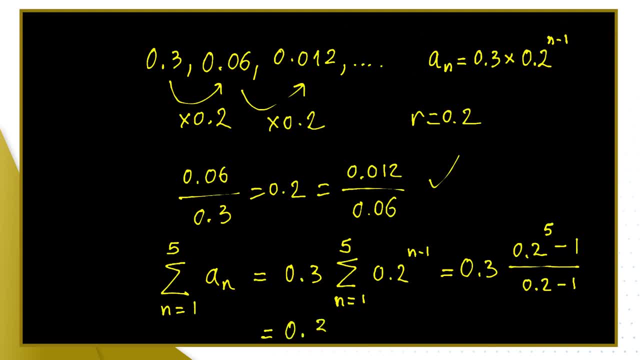 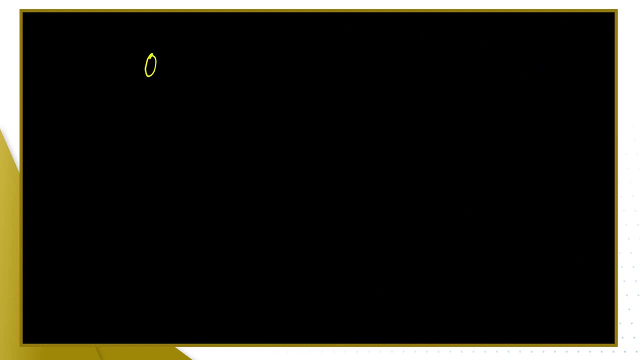 Which equals to 0.37488.. So that is the sum of the first 5 terms of that geometric progression. One more example: let's do 0.1 minus 0.05 plus 0.025, and so on. This is the series we want to. 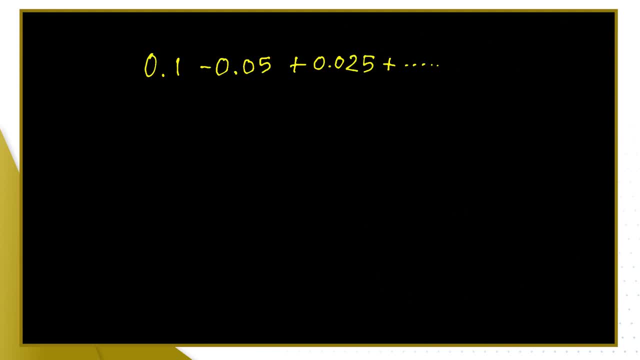 add up. Now I want to add up the first 5 terms of that geometric progression. So I'm going to add up the first 5 terms of that geometric progression. Let's check that it is a geometric progression. So the terms are 0.1 minus 0.05, 0.025, so let's do the ratios minus 0.05,. 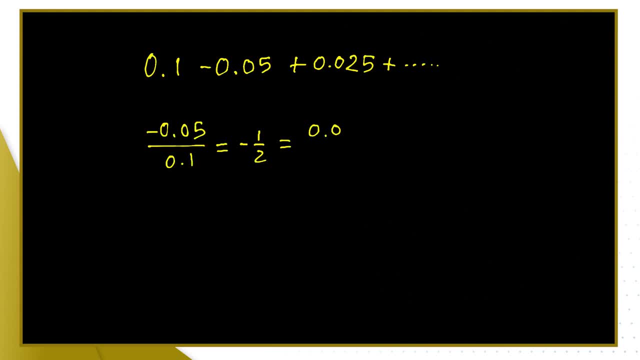 this is minus a half, and that is the same as 0.025 divided by minus 0.05.. So we want r to be minus 1 half, and so the sum we're calculating is 0.1 times the sum of powers of minus 1 half. 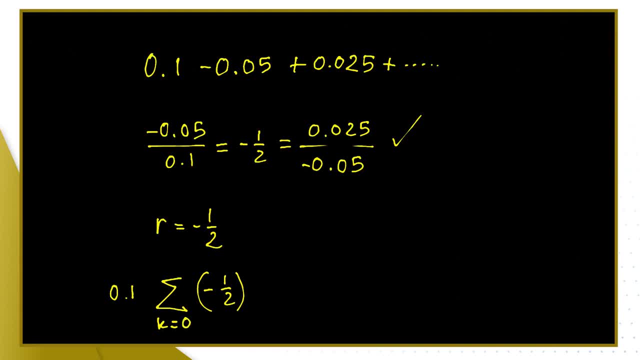 And we're running this from 0 to 4, that's 5 terms. and now this is going to be 0.1 times the formula for the sum, which is minus 1 half to the power of 5, that's 5 terms. take: 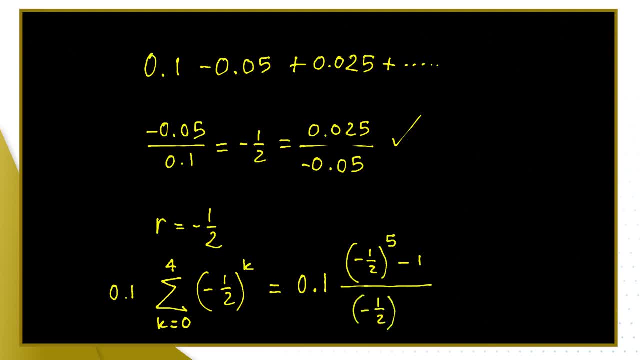 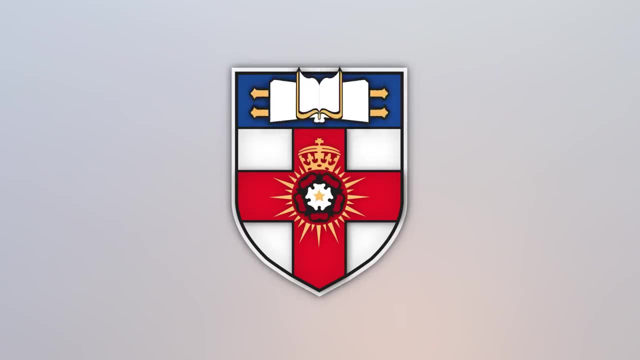 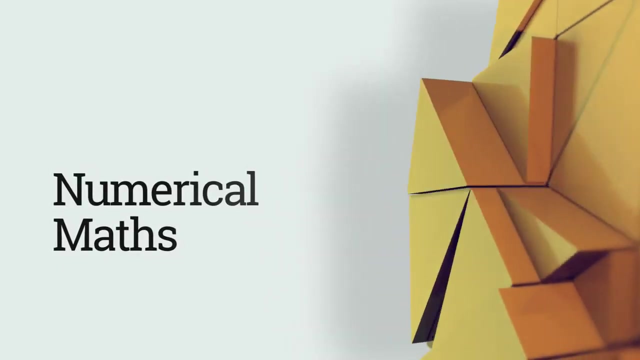 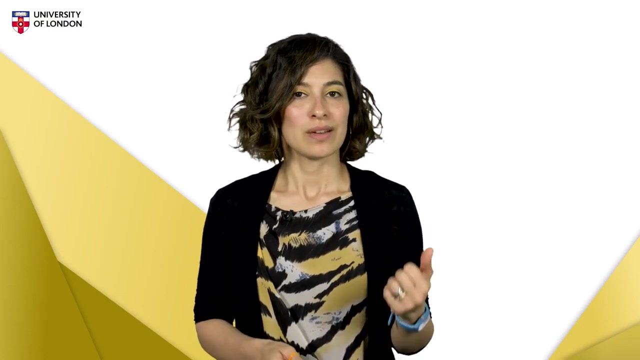 away 1, divide by minus 1, half, take away 1. And that is 0.06. 875.. We looked at two formulae for finite series. We saw the sum of an arithmetic progression and the sum of a geometric progression. 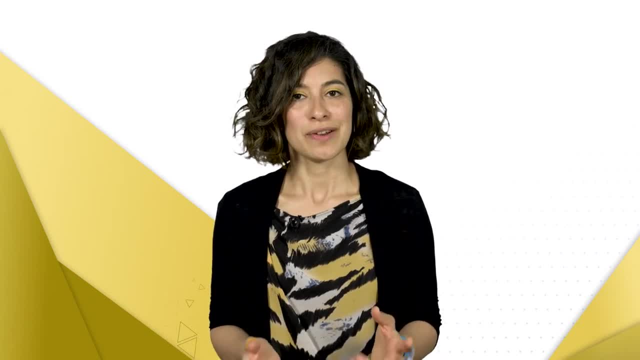 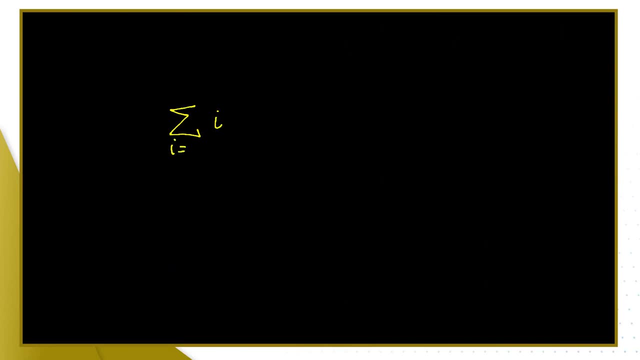 So we're going to look at the sum of a geometric progression and the sum of a geometric progression. Let's look at three more formulae for series. The sum of i, i between 1 and n. that means just adding up 1 plus 2 plus 3, all the way. 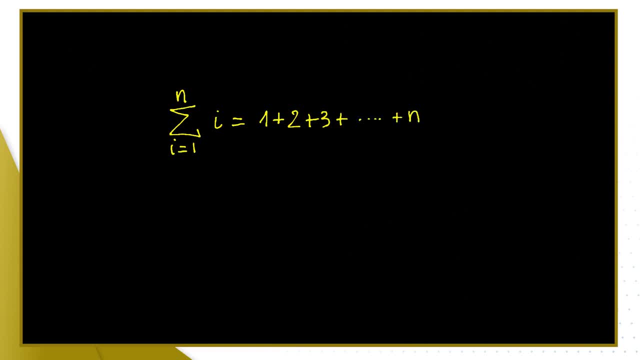 to number n. The formula for this one comes from the sum of an arithmetic progression of common difference, 1, and beginning in 1.. And this is written as n times n plus 1 divided by 2.. Check for yourself that this formula matches the formula we've learned for the arithmetic. 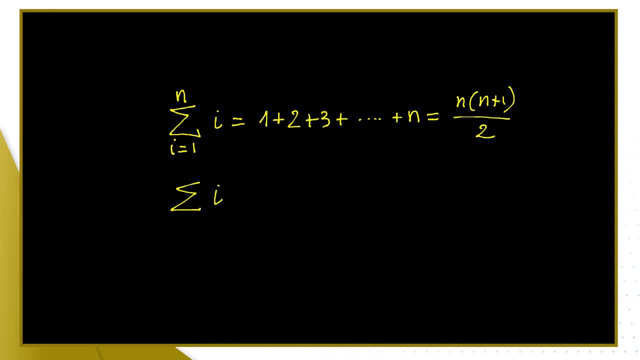 series. Now, more interestingly, the sum of squares, the sum of consecutive squares from 1 to n, that is doing 1 to n, 1 squared plus 2 squared plus 3 squared, all the way to the square of n. 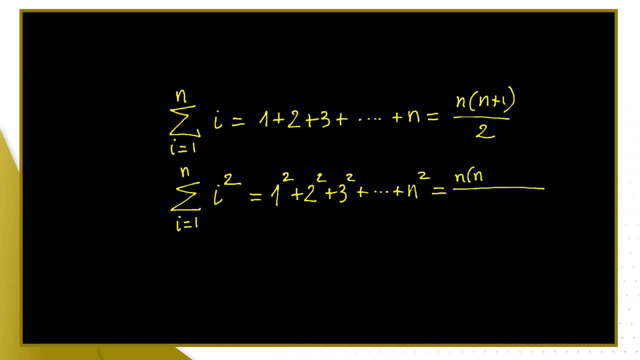 That boils down to n times n plus 1 times 2n plus 1 divided by 6.. And finally, the sum of cubes, The sum of i cubed between 1 and n. This means 1 cubed plus 2 cubed. 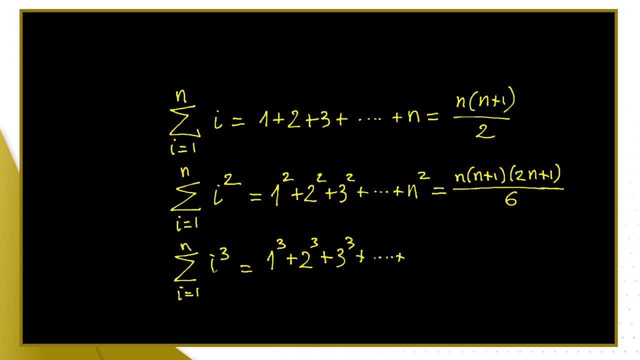 Plus 3, cubed plus, all the way to the cube of n, This one, surprisingly or not, it is the square of the first formula we have there. It is the square of n times n plus 1 over 2.. So it's n squared n plus 1 squared over 4.. 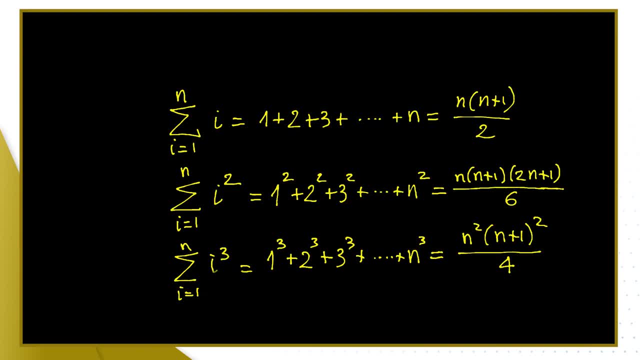 Let's just look at a couple of examples. Let's just look at a couple of examples of these formulae in action. The sum of i, when i goes from 1 to 10, that is, we're going to use the formula we've learned. 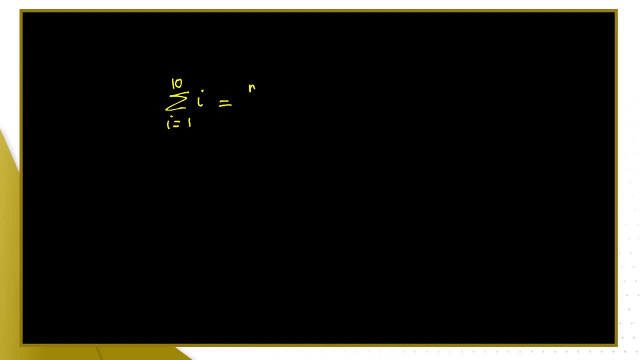 before with n equals 10,, so that it's n times n plus 1 over 2.. We replace n equals 10 in here, So we've got 10 times 11 over 2,, which is 5 times 11,, which is 55.. We've got 10 times 11 over 2,, which is 16.. We've got 10 times 11 over 2,, which is 55.. We've got 10 times 11 over 2,, which is 55.. 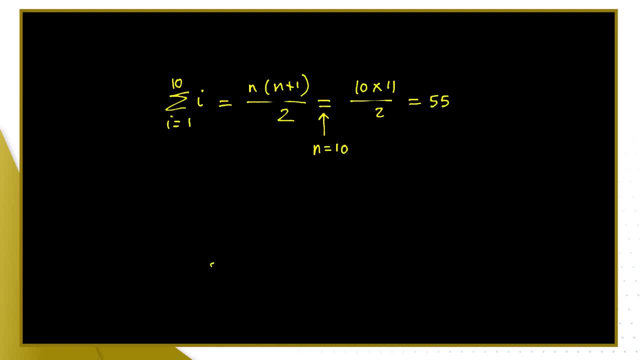 55.. The sum of squares. let's do that. let's do the sum of the first seven squares. so i, from 1 to 7.. The formula for this one was n times n plus 1 times 2n plus 1, divided by 6, and so we need to make n equal 7 in this one, and so it's. 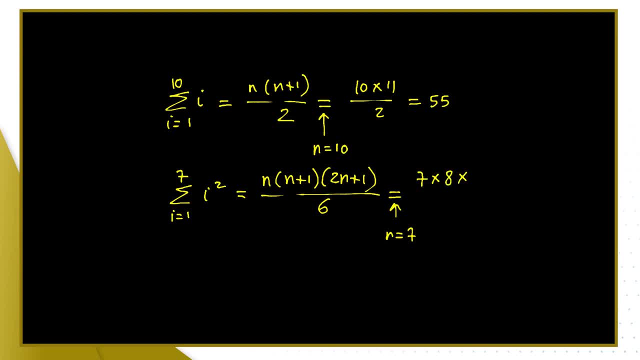 7 times 8 times 15, divide by 6, equals 140.. Let's do the sum of cubes, let's do the first five cubes. So that is the square of the first formula. so n squared n plus 1 squared over 4, we're gonna make n equal 5 in there. so we got. 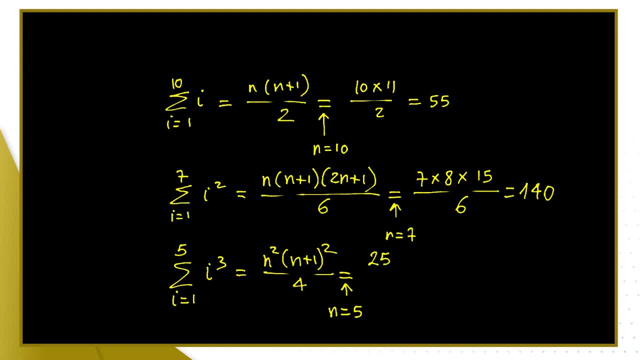 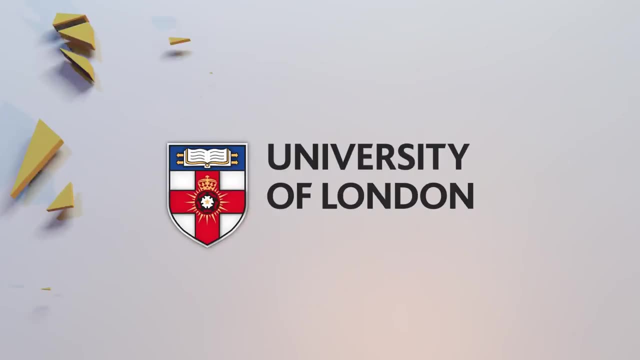 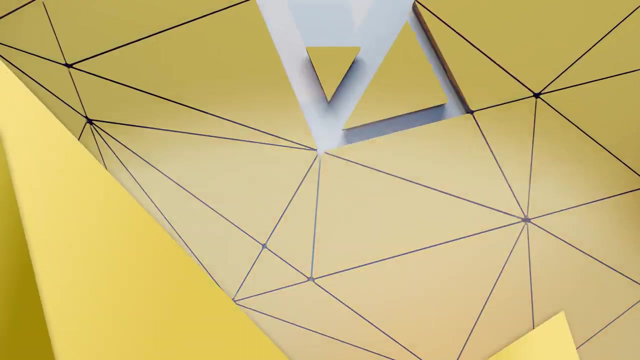 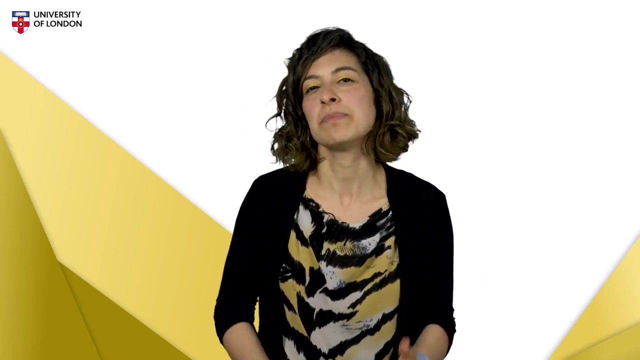 5 squared, which is 25,. angels on the board: 225 times 6 squared, which is 36, divided by 4, 225.. In this lesson we looked at adding up terms of sequences. We called these sums series and we used the summation symbol, sigma, to write them. 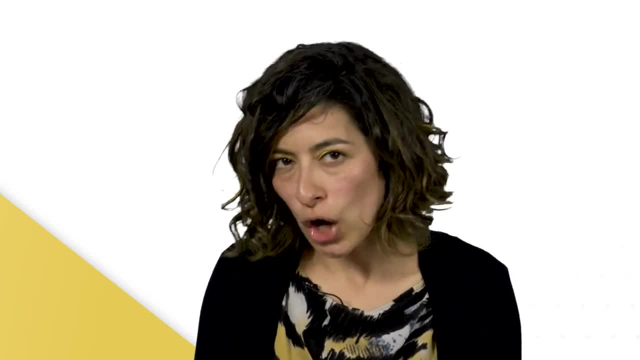 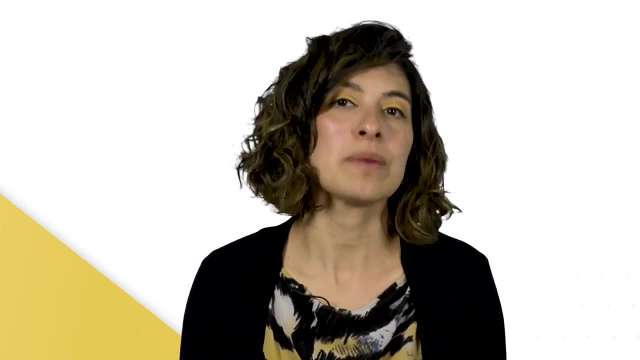 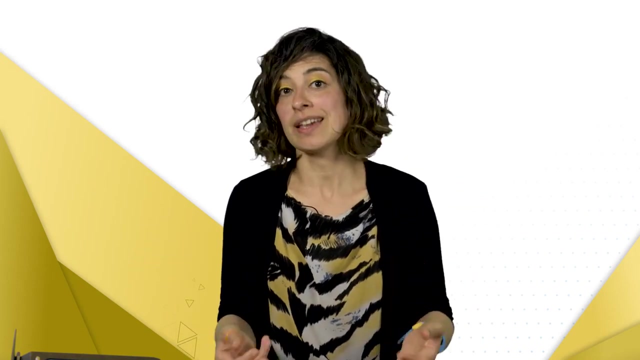 We added sums and multiplied a sum by a constant. We also used formulae for the sums of consecutive numbers and the sums of consecutive squares. We even saw the special cases of sums of arithmetic and geometric progressions. We saw formulae for these. 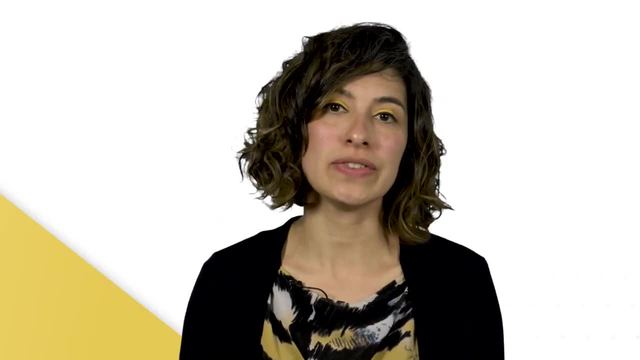 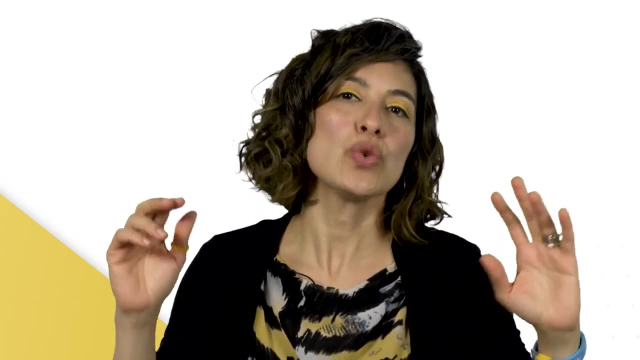 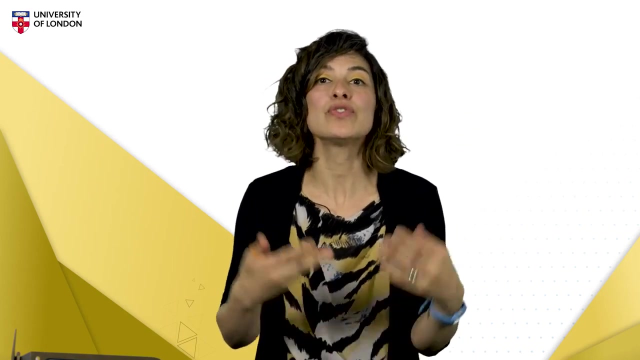 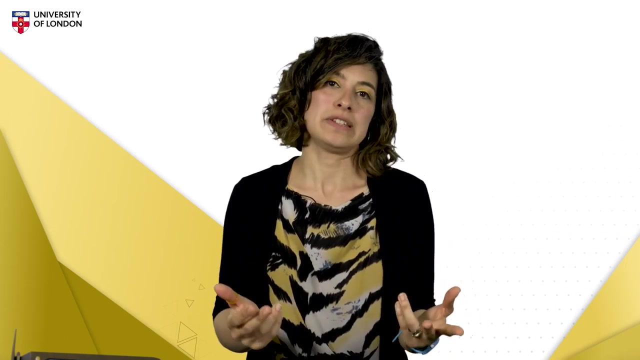 Next we will look at the behaviour of sequences and series as n grows unbounded, in other words, as n tends to infinity. To get ready for the next lesson, I invite you to observe what happens to arithmetic and geometric sequences and series as n tends to infinity. 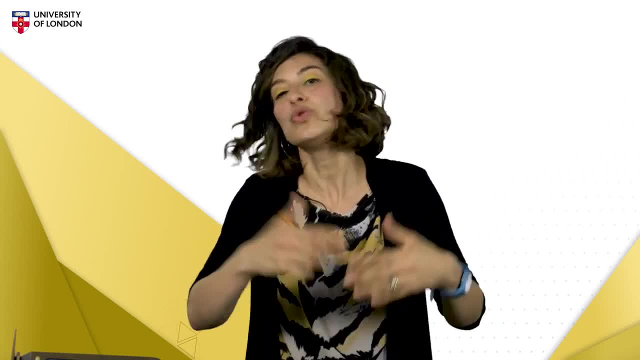 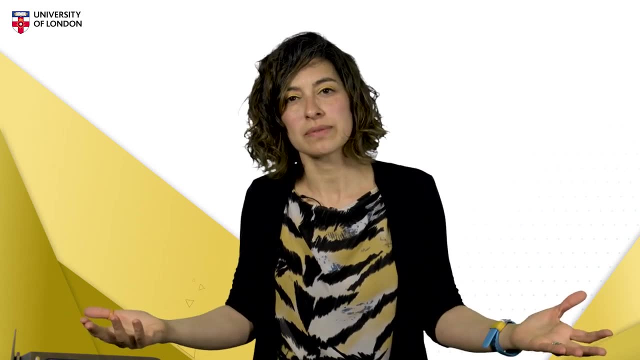 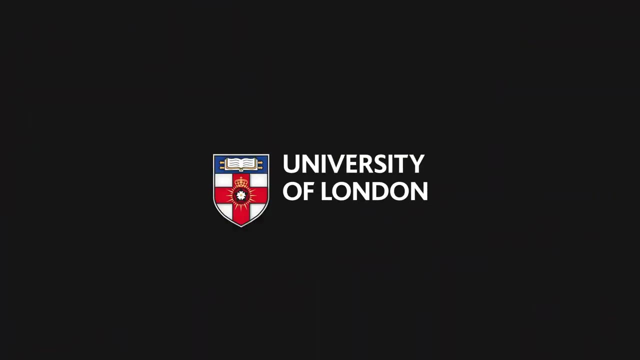 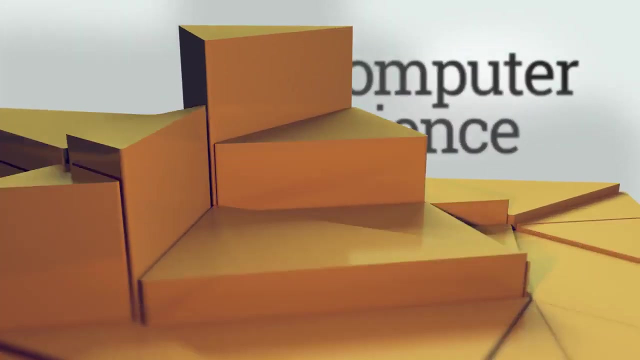 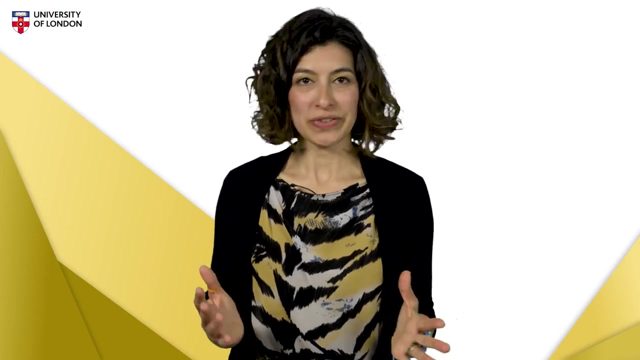 Do the terms stay bounded? Do the sums sums stay bounded? Do the terms grow unbounded? What about the sums? Bring your thoughts with you to the next lesson. Hello and welcome back. We worked with several sequences and series and by now you're fully. 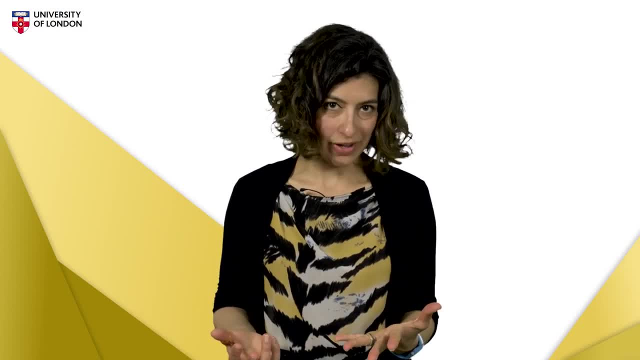 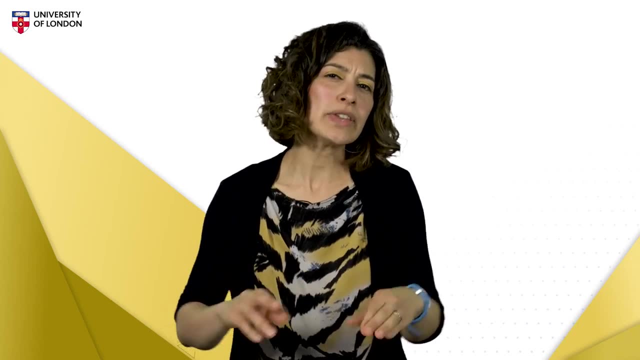 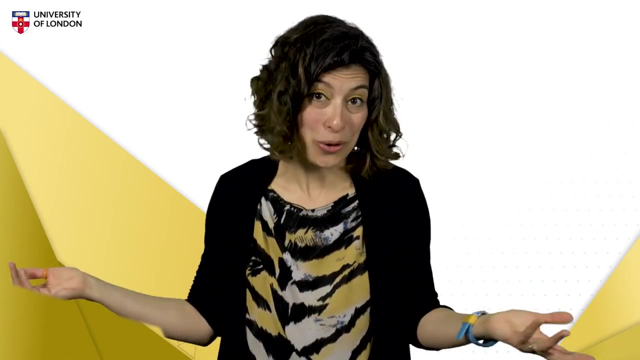 familiar with computing terms of sequences and their sums. We are now going to look at the behaviour of sequences. That means that we want to analyse the long term pattern as more and more terms are computed, without having to compute all of them. We're going to look. 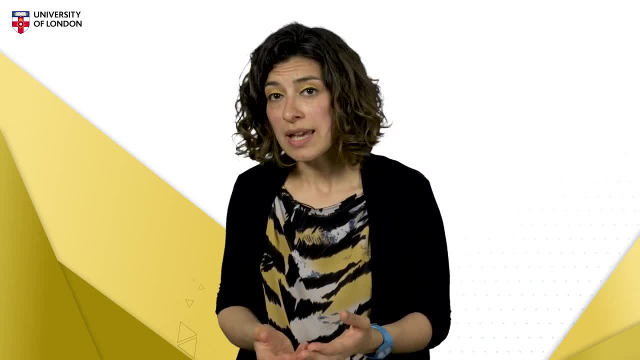 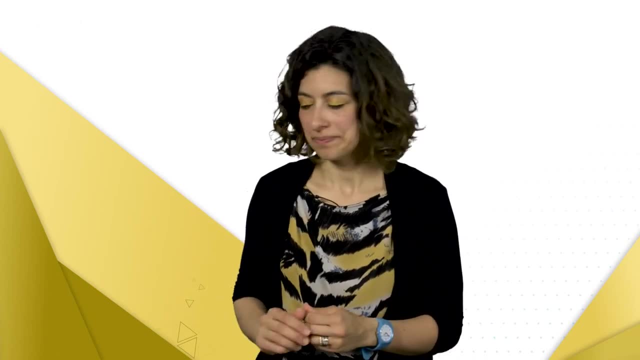 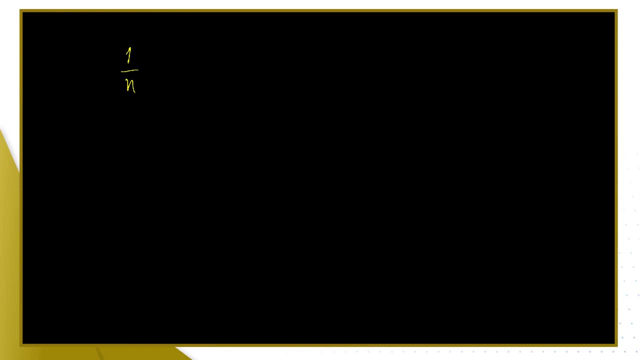 at a few examples of sequences. I wanted to join me in trying to predict what happens as n grows unbounded. I'm going to list a few sequences here. you can get thinking of them. 1 over n: 0.1 to the power of n. 10 to the power of n minus 0.1 to the power of n minus. 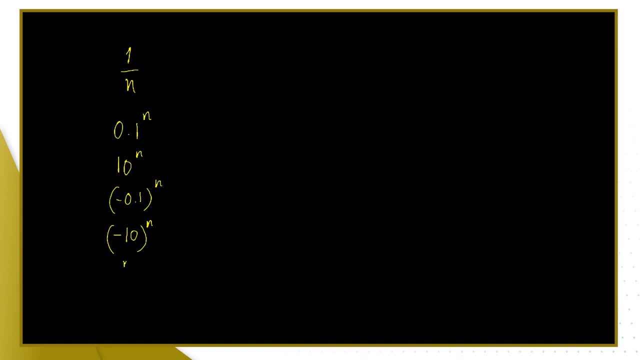 10 to the power of n, and then n over n plus 1 and n plus 1 over n, All these sequences. here We're going to run our n from 1 onwards. So we've got n is 1 in 1, 1 half, 1 third, 1 quarter, and so on. 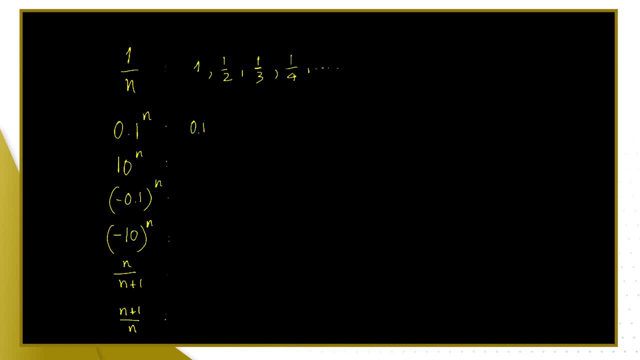 0.1 to the power of n is 0.1, then squared is 0.01, cubed 0.001 to the power of 4.. There's one more four decimal places, and so on: 10 to the power of n. start with 10 to the 1, 10. 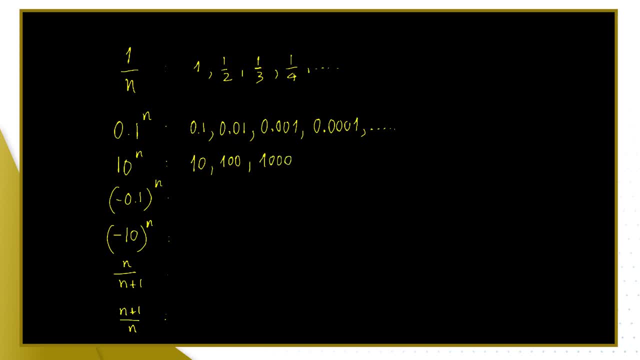 squared 10, cubed 10 to the power of 4, and so on. Now 0 point minus 0.1 to the power of n sounds very similar to the other one, but remember, we've got the brackets. we're going to have to do powers of the negative 0.1, so the first one is: 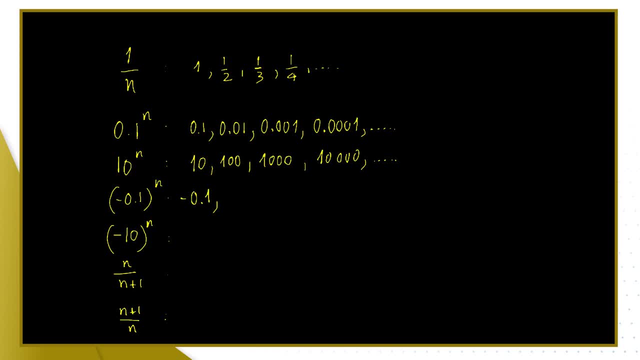 minus 0.1, the second is a square, so it's going to be positive 0.01, the third is going to be negative. so it looks very similar to the 0.1 to the n, but it alternates in sine, the odd powers being negative and the even powers being 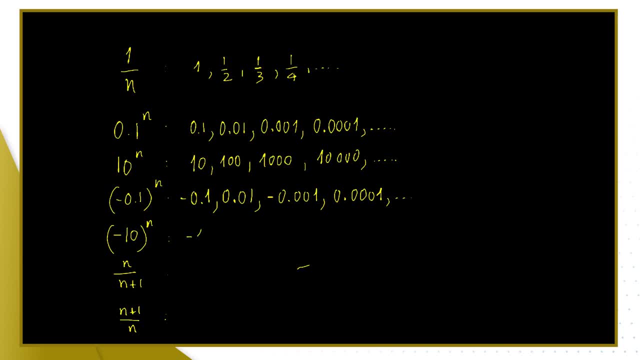 positive. Next similar stuff. so negative 10,, positive 100, negative 1,000,, positive 10,000, and again odd powers negative and even powers positive. Now for n over n plus 1, starting with n equals 1, we've got 1 on top, 2 below, so 1 over 2, and then 2. 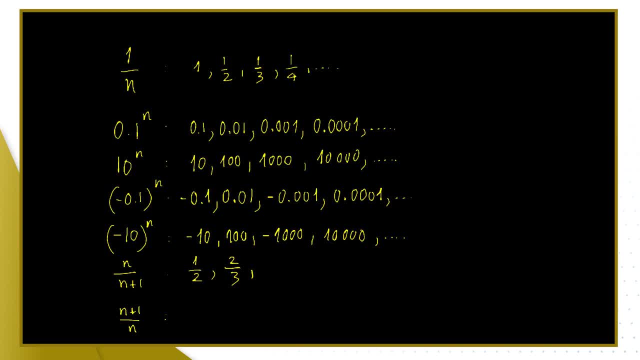 over 3, and so on. So it's a number over the next one, so 3 over 4,, 4 over 5, and so on. And the very last sequence is the other way around. when n is 1, we've got 2 on top, 1 underneath, so just 2.. Then we 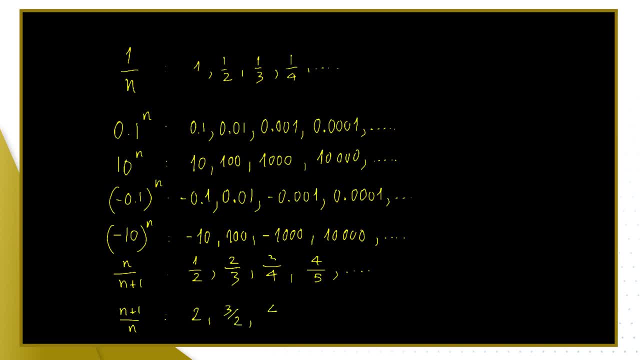 have 3 over 2,, 4 over 3,, 5 over 4, and so on. Now I know that it's very tempting sometimes to write all these numbers as digital expansions rather than fractions. I would like to do that as well, and I wanted to see how useful is one or the other. It's. 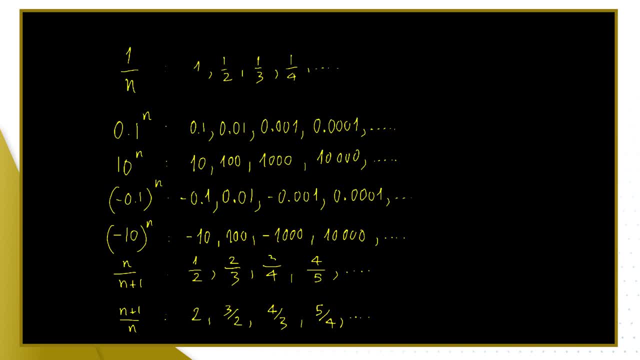 good to bear in mind that, in some cases, one expansion might be more useful than the fraction, or the other way around. Now what I want us to focus on is what happens to these sequences as I compute more and more terms, As n is growing, as n goes. 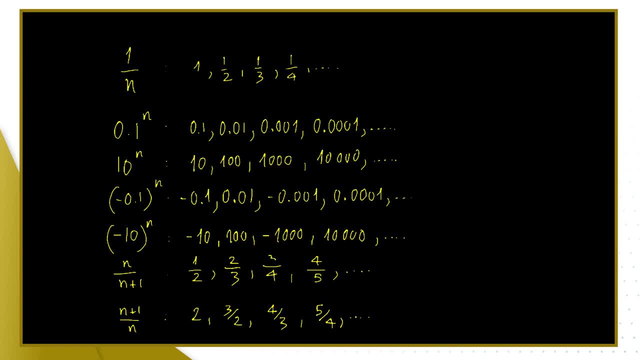 to infinity. Saying as n goes to infinity is a way of saying as n grows, n bounded larger and larger. So I want to capture that behaviour to infinity. So what do you think happens? How do you explain what happens with the 1 over n? What would be the behaviour expected after a quarter? 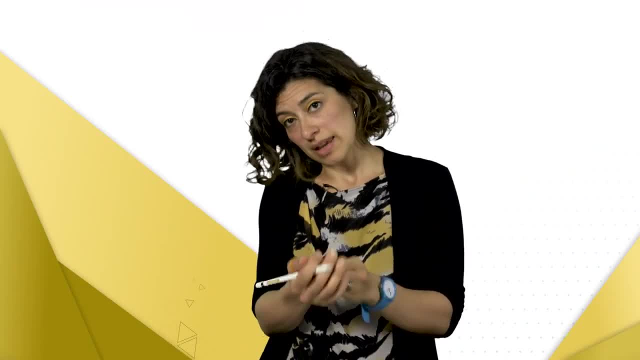 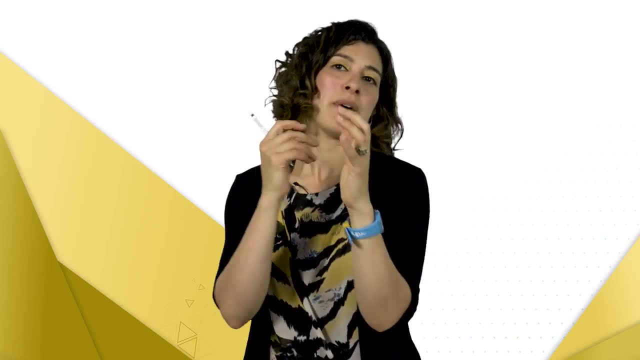 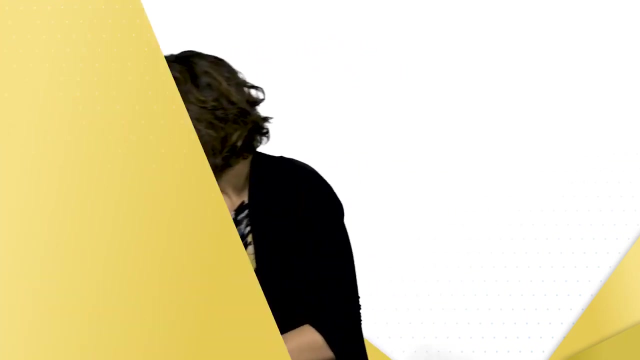 a fifth and six and so on. You'll probably join me in saying that that number gets a and smaller and smaller in magnitude. I'm dividing 1 by 4, 1 by 5, 1 by 6, 1 by a thousand a million, it's getting really, really small in magnitude. so I say that. 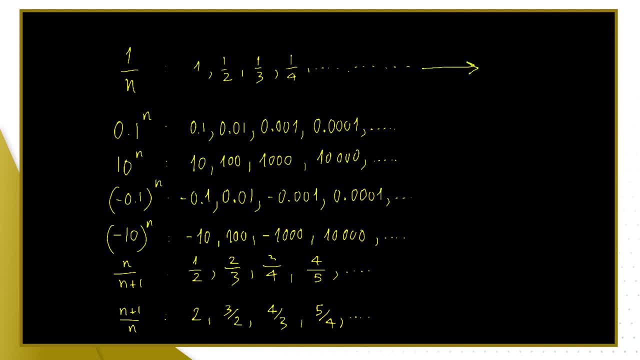 the limit, and I put this arrow here. it's 0, meaning what I expect these values to converge to 0, to get smaller and smaller and closer and closer to 0. it doesn't matter whether or not 0 is attained. it's not attained, but the values are going to. 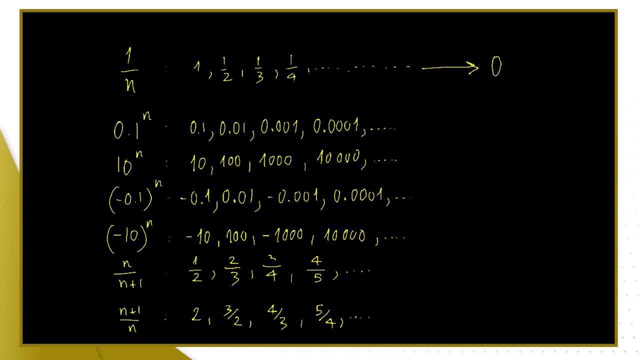 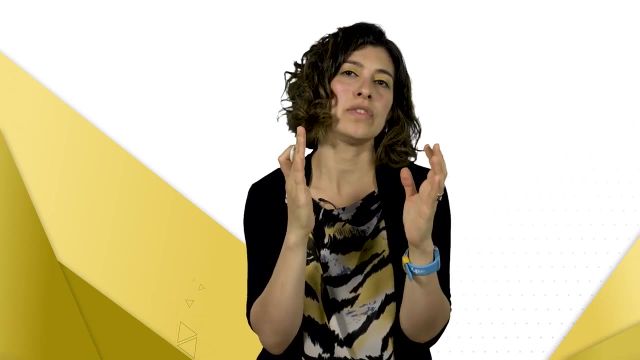 be closer and closer. if I say: can I get to 0 with a certain error bound within, say, 0.001, yes, there will be a number after which all the numbers in this sequence are going to be within 0.001 of the limit 0, but I can make that error. 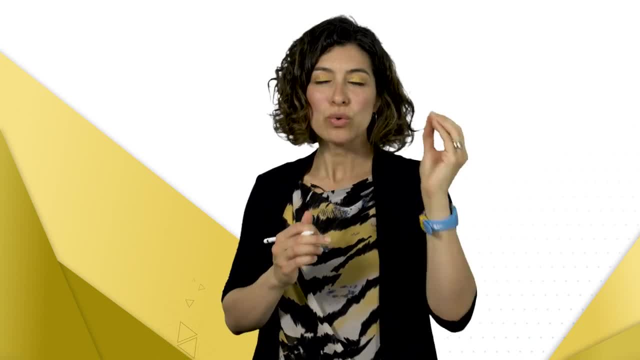 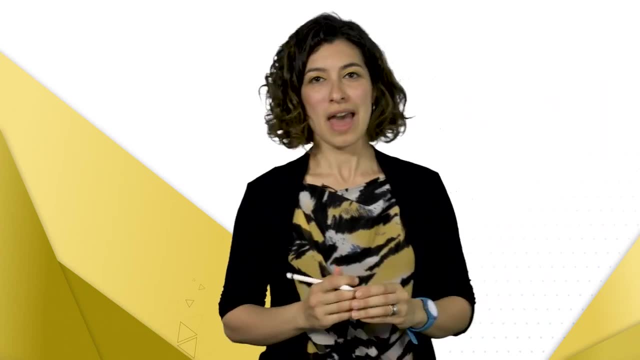 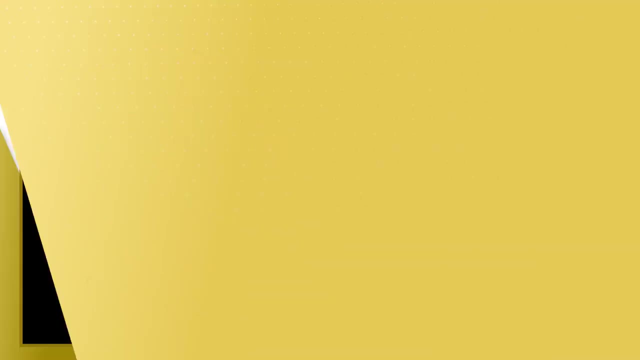 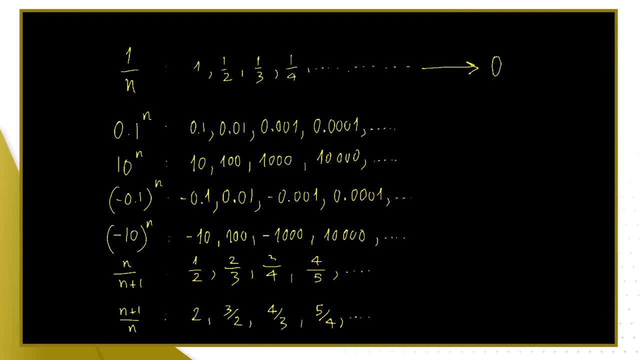 the, yet the next one. so we got 0.1, 0.01, 0.001. it's getting really, really, really, really small and that is also converging to 0, has a limit of 0. now, when we have 10 to the power of n, that is growing rapidly. 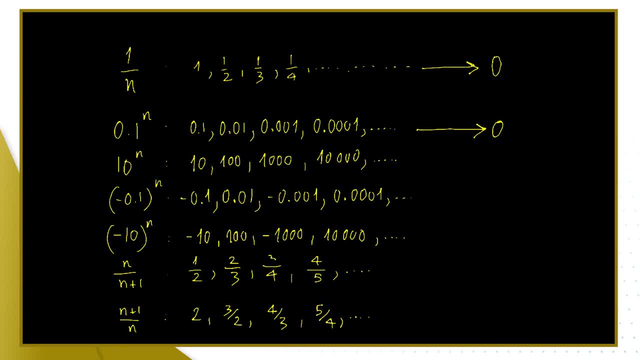 look, the number of zeros is increasing. so I call numbers larger and larger and larger and that it's. there are many ways of saying that, but one: what? in this particular case, the numbers are growing and boundedly and they're getting larger and larger and positive, so it's pretty clear that it's just blowing up as a 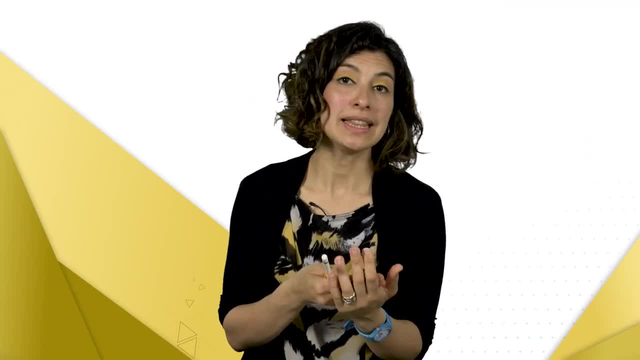 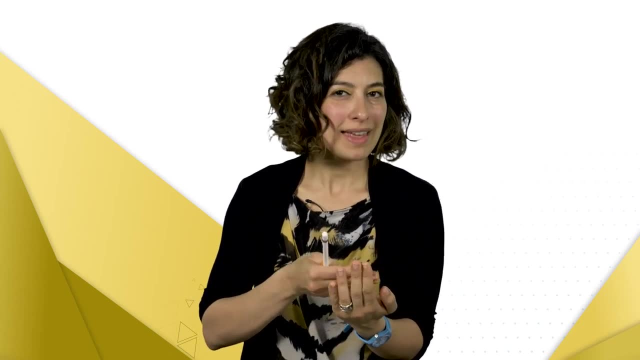 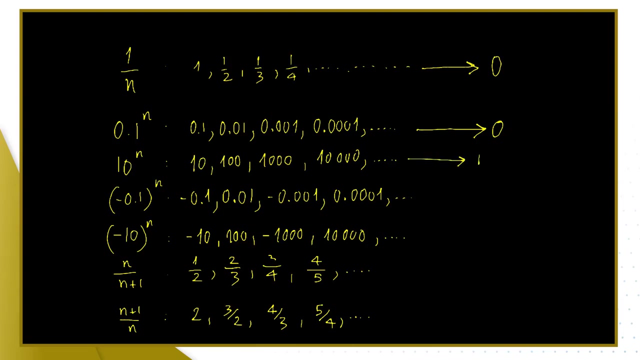 positive number, we can say that it has an infinite limit, but is also correct to say that it's divergent. but it's. I will tell you more about divergent sequences. so this one: here I'll say limit plus infinity, because it's getting larger and larger and larger, is growing and bounded. now what does that mean? it means that I 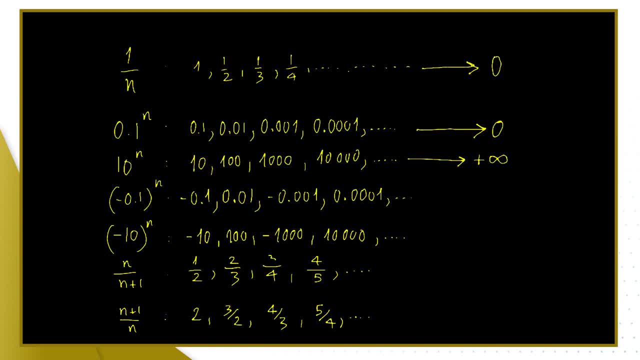 say: let me see if I can contain these numbers within this size. you know I've got a bound. say: let's see if I can contain these numbers up to a million. will this sequence ever grow beyond a million? yes, it will, because a million has six zeros. it's only a matter of time. ten to the. 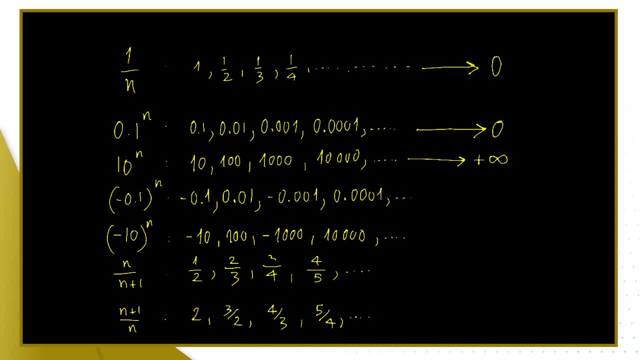 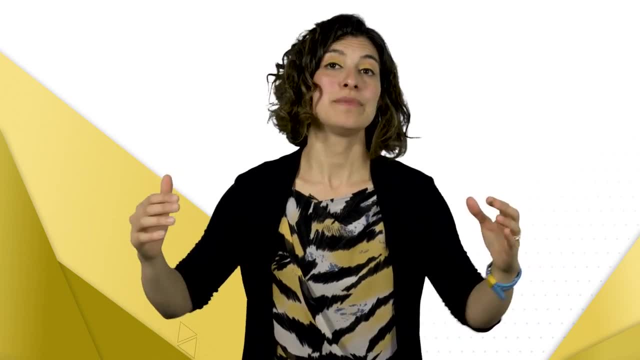 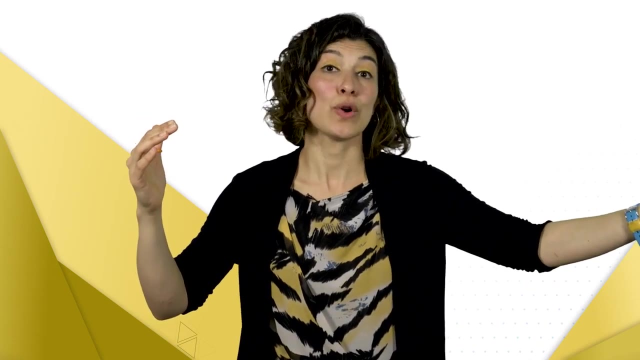 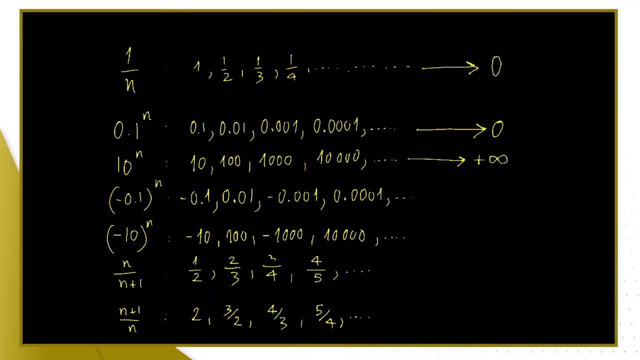 power of seven has seven zeros. so after seven terms, the sequence is beyond my bound. so every time I attempt to put a boundary on the size of the terms, there's always a number that goes over the boundary. so that is infinite limit in this case, yes. so for the next one, minus 0.1 to the power of n is very. 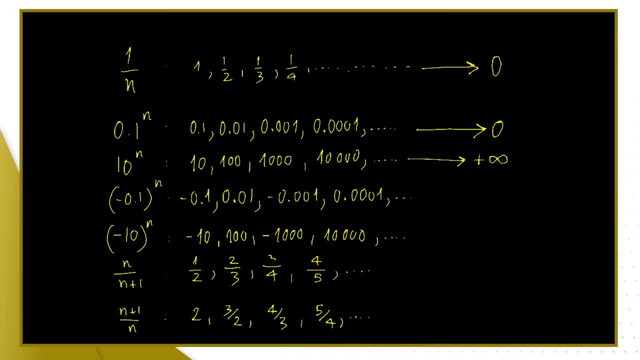 similar to the one we had before, but this one alternates between being positive or negative, but they're still in magnitude really small and we've seen with the yüz mycket before. so sometimes above, sometimes below, this one still converges with limit zero, the next one minus ten to. 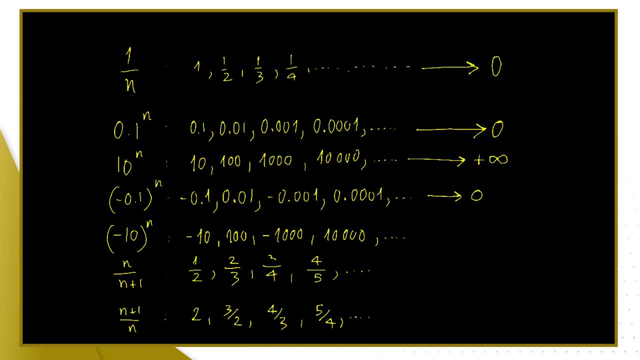 the power of n, the numbers keep blowing up, but in both directions they get infinitely negative and infinitely positive. so this one, I'll say: no limit, so divergent. okay, down to our fractions. you may have written down the values of these terms as a decimal. 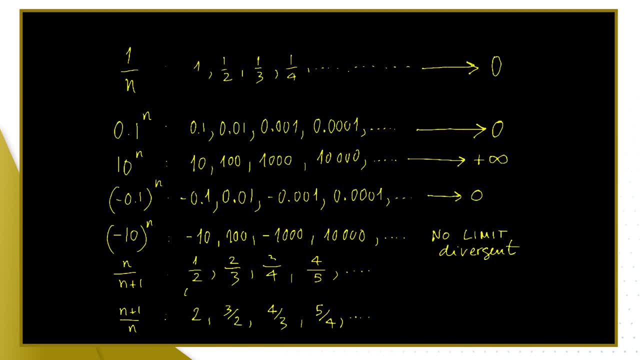 as a digital expansion, That would have been 0.5 for a half, 0.6, recurring for two-thirds, 0.75, 0.8 and so on. The pattern isn't so clear when I write it as a digital expansion. 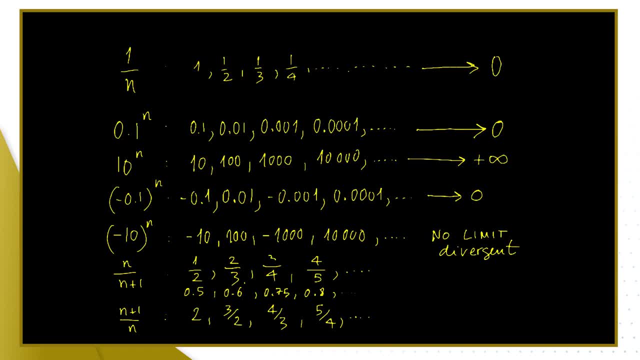 but with a fraction it's a lot clearer to me That what we get. we get a fraction when the numerator and the denominator are close and the larger they are. just a difference of one between top and bottom isn't going to make much of a difference in terms of the magnitude of the 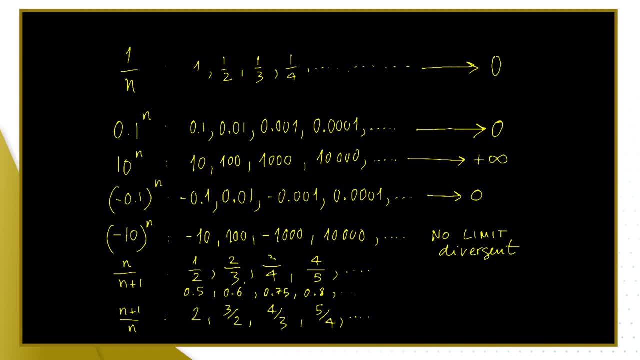 number. It seems to me that they're approximating to one. The numbers are getting larger and larger, approximating to one. Now you may wonder: can we prove that? I'll show you in a second. So that'll be a limit of one, The bottom one, two, three-halves, four-thirds, five-quarters, and so on. 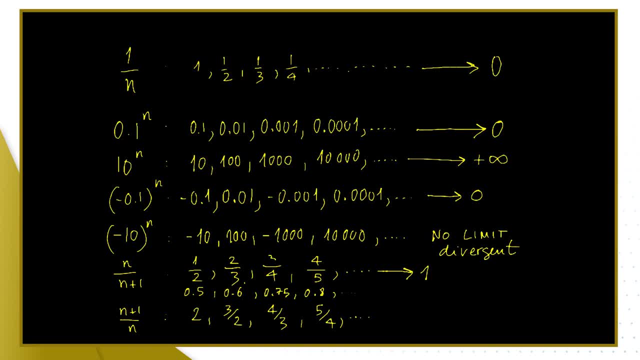 there's just a tiny bit. the numerator is a tiny bit larger than the denominator, so the numbers are larger than one, but just a little bit larger than one, And you can write the decimal expansion yourself. the limit of this one is one as well, And I've used a notation there. I've used the arrow. 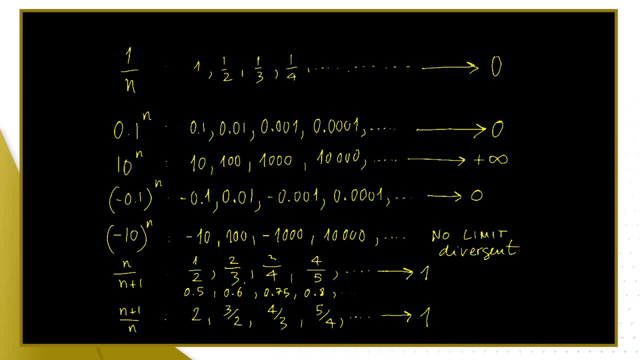 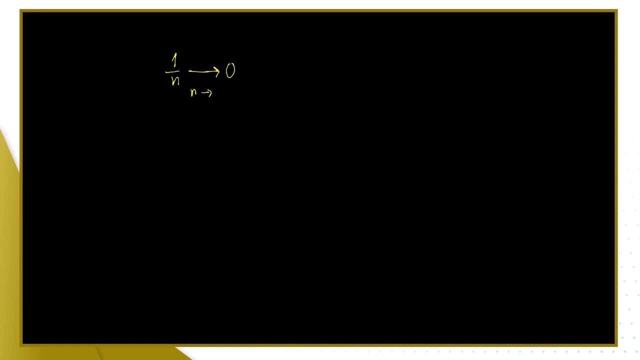 I'm just going to formalize that. The way I would write this without this long diagram, would be one over n converges, that's the arrow to zero, as n goes to plus infinity. That is one way of writing it. The other way of writing it is with lim from limit The limit, and underneath I say the variable. 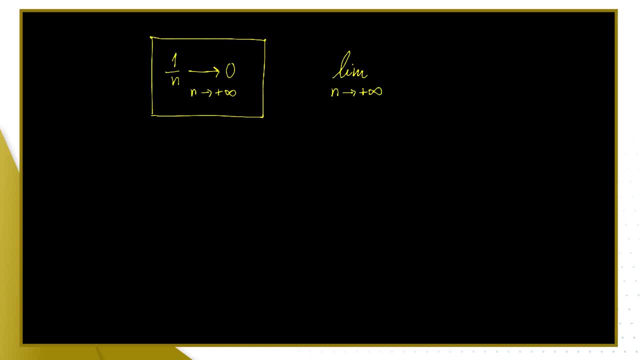 is n as increases to plus infinity, the limit of what, and I'll write the of what is here: the limit of one over n. as n tends to plus infinity, that limit is zero And is is the equals. OK, so that's another way of. 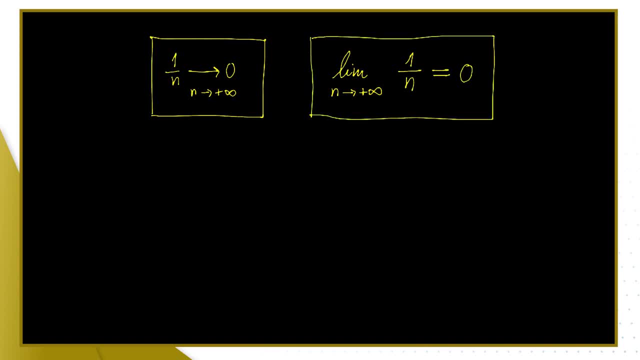 writing it And so applying it to the other examples. we have that n over n plus one converges to one, as n tends to plus infinity. we can say the limit, as n tends to plus infinity, of n over n plus 1 is zero. 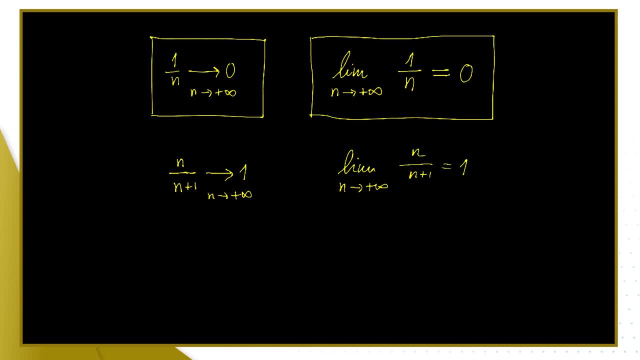 1, and similar to the other examples. Now can I show you that this limit is really 1?? Here's a little trick: n over n plus 1.. Well, we can do fractions, and so here I can say: 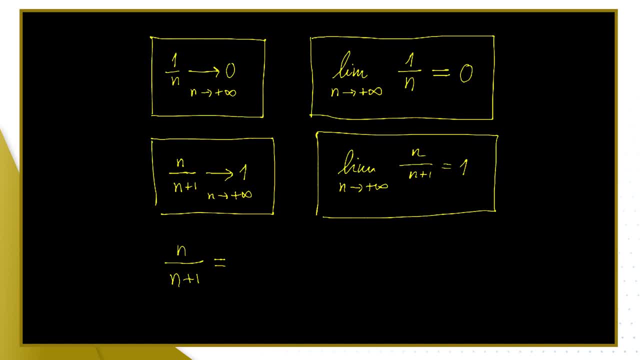 well, the denominator and the numerator are very close, so I'm gonna write the numerator as n plus 1 and then take away 1.. You'll agree that that totals up It's still n. I just artificially added and subtracted a 1 to make it look a little bit more like the denominator. And now 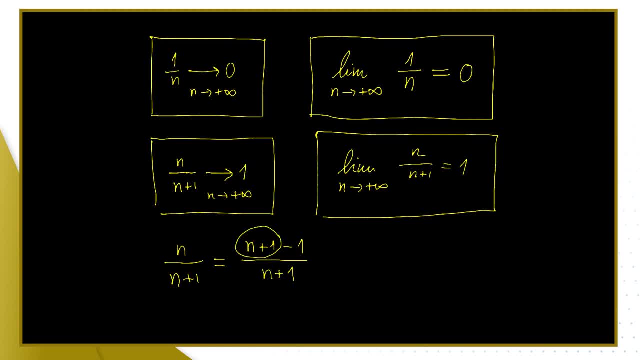 I'm gonna split the fraction into this bit minus this bit, So it's gonna be n plus 1 over n plus 1 minus 1 over n plus 1.. And now this is the cool bit. this is 1, because top. 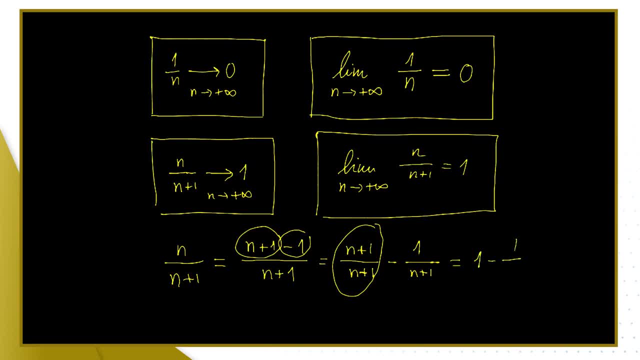 and bottom are the same. So I've got 1 minus 1 over n plus 1.. Now this bit here: 1 over n plus 1, it's very much like that sequence there: 1 over n, So that one has a limit of 0. That means I. 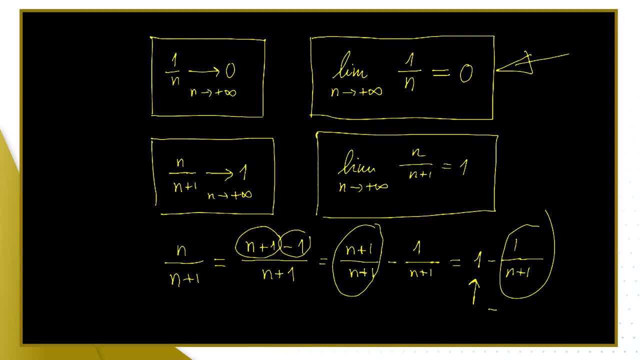 have terms that look like 1 minus something that tends to 0. So the limit is going to be 1.. So n over n plus 1 is the same as 1 minus 1 over n plus 1.. And in the limit it's going to be 1. 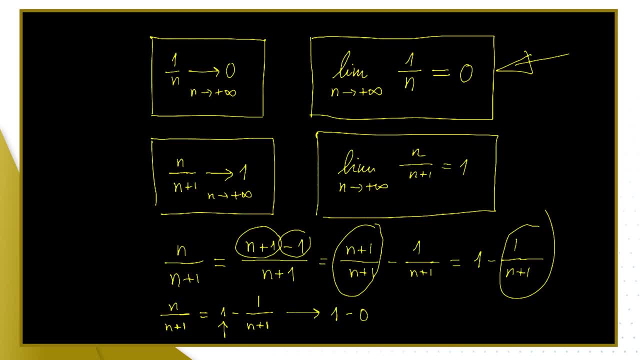 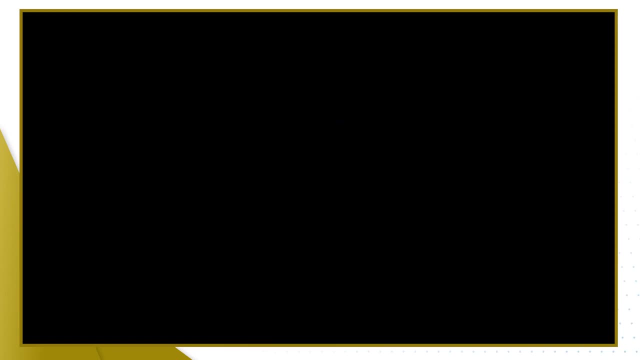 from this one and take away 0 from this bit. So the limit is just 1.. And you can do the same to prove that n plus 1 over n has a limit of 1 as well, Just how we write the other limit. 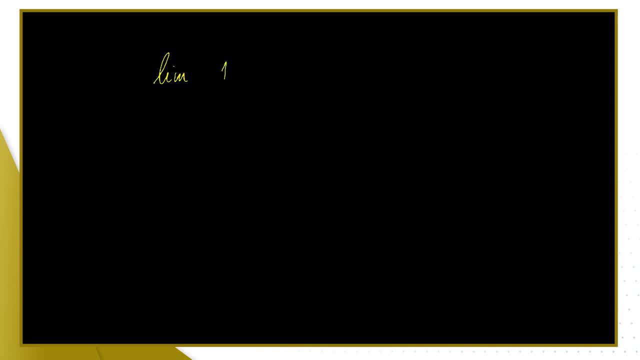 so we had a limit of 10 to the n. When n tends to plus infinity, we saw that that was infinite. It's a divergent sequence, but it's a special type. We can still say: the limit here is plus infinity. 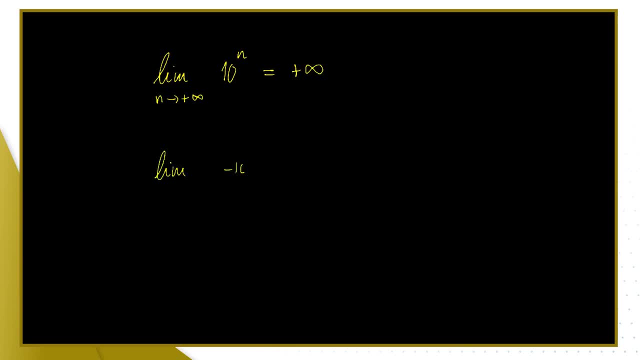 Whereas minus 10 to the power of n, because it alternates between positive and negative, this one has no limit. So they're both divergent, but the first one has an infinite limit and the second one does not have a limit at all. 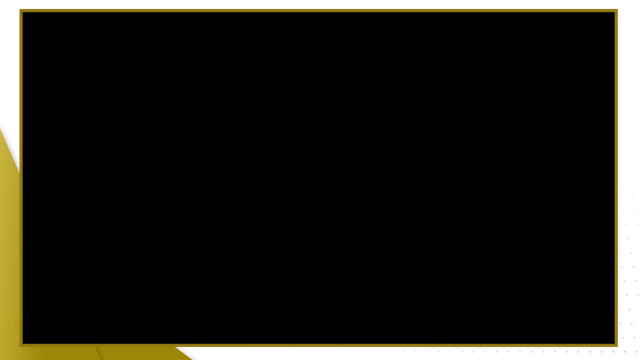 We're going to look at a couple of examples. Say, we've got a. n is 2 to the n, b, n is 5 plus 2 over n squared c. n equals a half to the power of n and d? n equals 2 plus n. 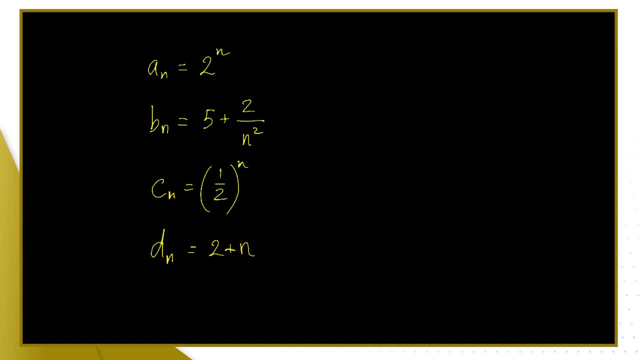 What are the limits of these sequences? So let's have a look at the other terms. The first one: we got 2,, 4,, 8,, 16, and it keeps doubling. What do you think it happens? Well, it's going to grow unbounded. 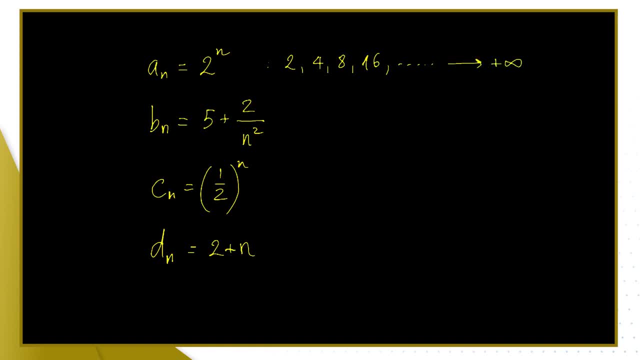 The limit here is going to be plus infinity. This one here starts with: when n is 1, I've got 5 plus 2, that's 7.. When n is 2, I've got- let's do the calculation- 5 plus 2 over 4, so 5 plus half. 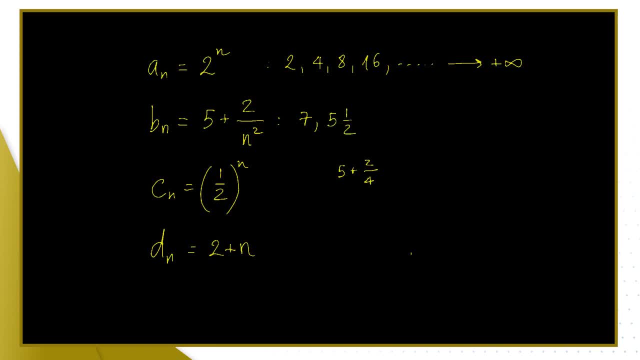 So 5 and a half. Then, for n equals 3, I've got 5 plus 1.. So 5 plus 1.. 2 over 3, squared, that's over 9, so 5 and 2 ninths. What do you think is going to happen? 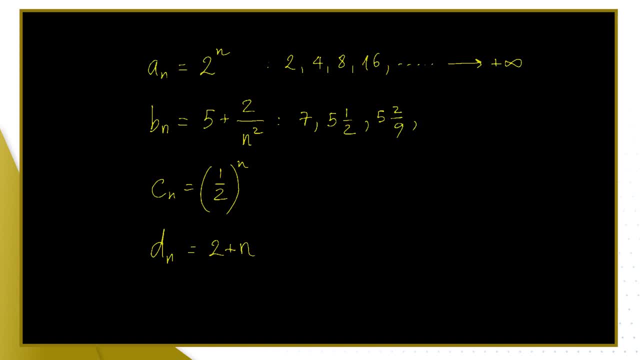 here as we increase the n. Let's try a couple more examples. So 5 plus 2 over 4 squared 16, so 5, 2 over 16 is 1 eighth 5 and 1 eighths. What's happening here? 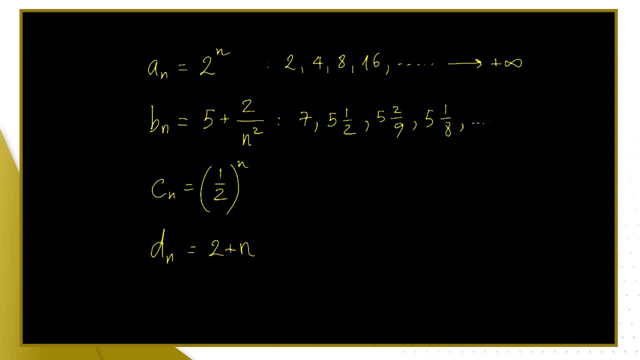 It seems very close to 5.. It seems that I've got 5 and a little bit, and that little bit it's smaller and smaller and smaller. So is it limit 5?? Can we prove? Yes, we can prove So. 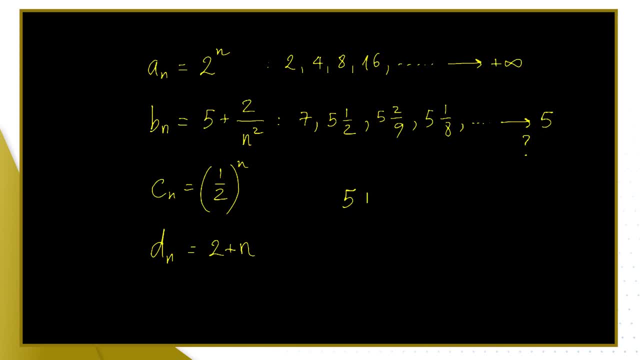 let's have a look What we can do. we can argue that it's 5 plus 2 over n squared. Now this 2 over n squared is very much like 1 over n. 1 over n has limit 0, so if I square it, I'm going to square that limit. 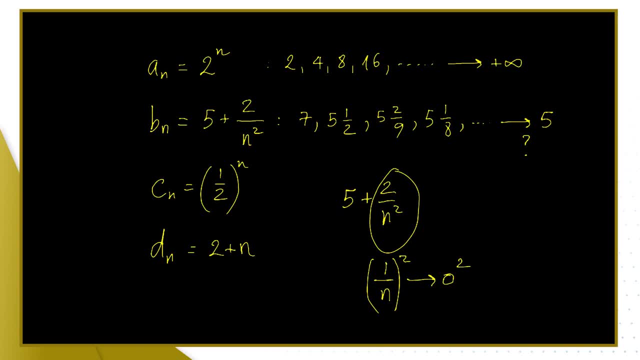 it's going to be 0 as well. And now, if I double it, multiply by 2, I'm going to multiply the sequence and the limit By 2, well, 0 times 2 is just 0, and this is the same as 2 over n squared. So what I'm saying is: 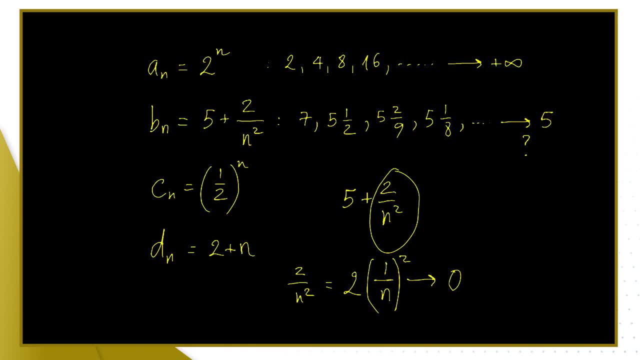 that that sequence there that I circled has limit 0, therefore the limit of 5 plus it has a limit of 5.. Okay, so how would you write this down? You will say the reasoning I explained is that the reasoning I explained there in steps of starting with 1 over n has limit 0, then, square, it has. 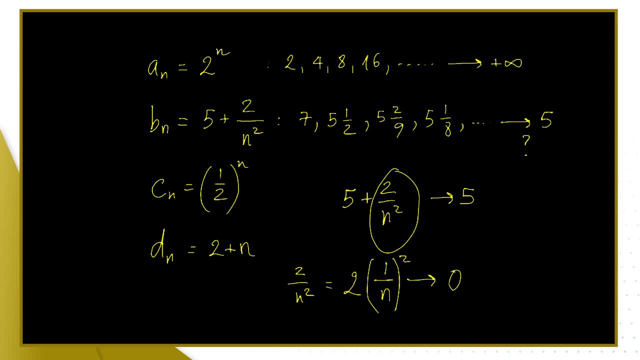 limit 0 squared, which is 0, then double, it has limit twice 0,, which is still 0, and then add 5, the limit will be 5 plus 0,. the limit is 5.. Okay, so that's the argument you'd use for that. 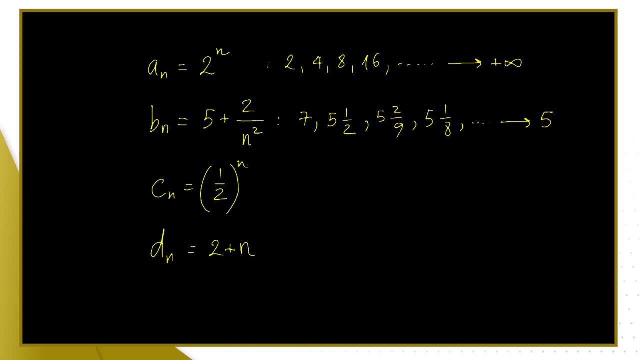 So yes, we proved that that limit is 5.. This one here we have a half a quarter, one eighth, and so on, Smaller and smaller, the limit is 0. And this one here I have 2 plus 1,, which is 3,, 2 plus 2,, which is 4, I just add one more every time. 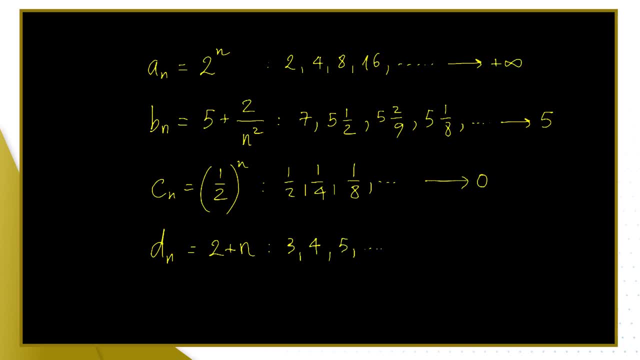 It's an arithmetic progression with common difference 1 and first term 3.. That is going to grow unbounded, slowly but unbounded. So from here I just want us to recognize a few examples. So bn, it's similar to the 1 over n sequence we saw earlier, So we can do operations with the limits. 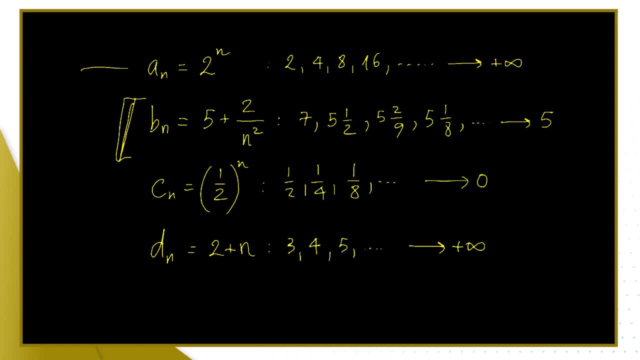 to get to the limit of that one. The top one, an, and this one, cn, are geometric progressions. an has a common ratio of 2,. cn has a common ratio of a half. And look what happens With a common difference of 2,, which is large. 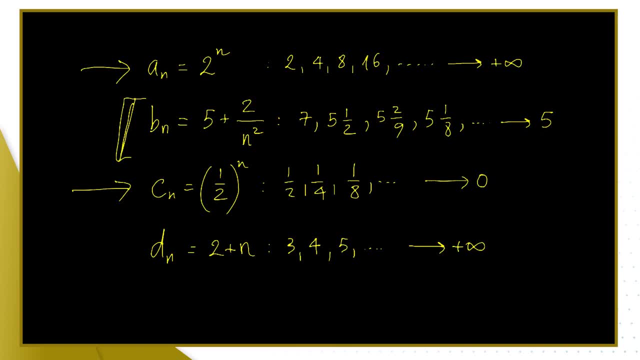 it's making the number grow. the geometric progression will have a limit of plus infinity or no limit. With cn, where the common ratio is a half, it makes the number shrink. The limit will be 0.. The fourth one being an arithmetic progression. 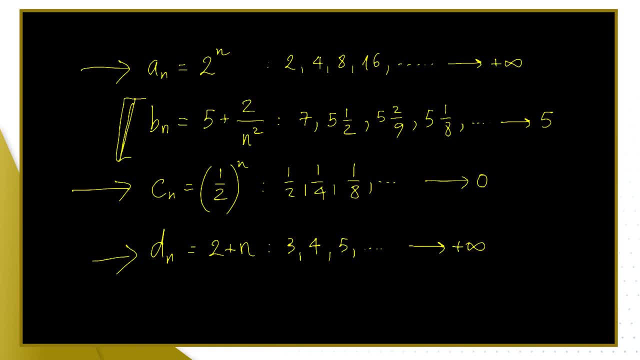 I'm adding a constant number every time. Even if I subtract the constant number every time, the sequence is either going to go to plus infinity or to minus infinity. So the only that is convergent to a finite limit is the geometric progression where the common ratio is small. 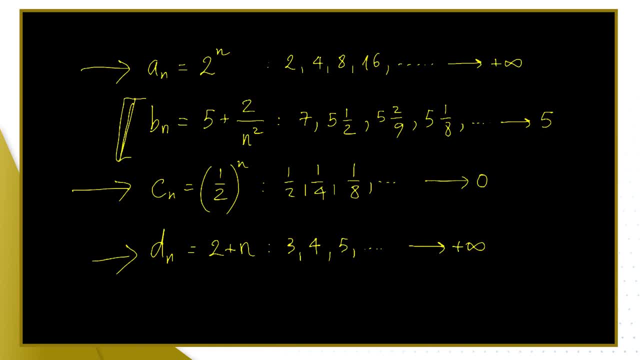 We're going to make precise what I mean by small. If it's a shrinking ratio, that means it has to be a number between minus 1 and 1.. If it's negative, it will alternate sign, but it's still going to. 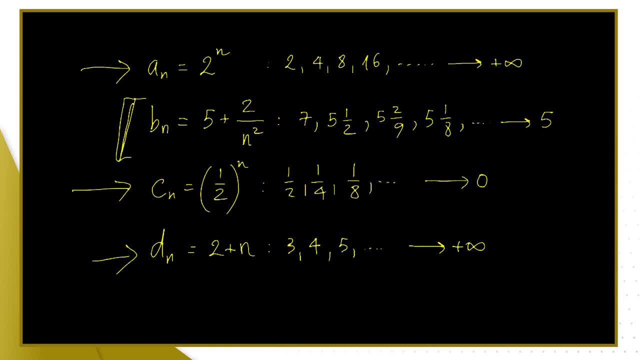 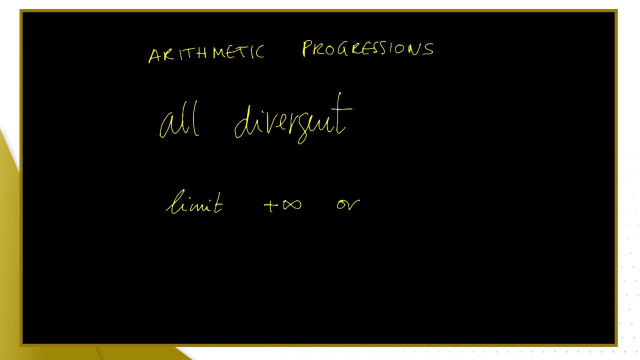 shrink the sequence value, the terms of the sequence in magnitude. So let's summarize that For arithmetic progressions, they are all divergent And the limit will be plus infinity or minus infinity, depending on whether you adding a positive common difference that you 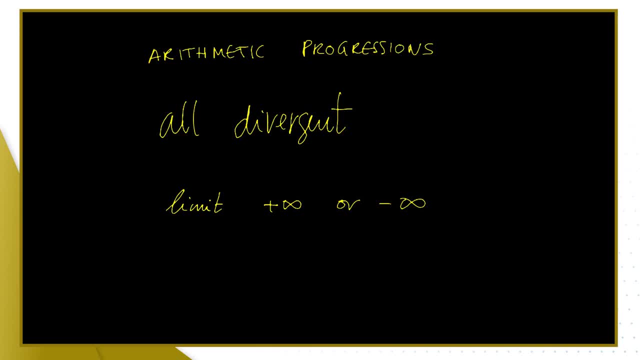 get a plus infinity limit If you're adding a negative common difference. you get a minus infinity limit For geometric progressions. if the common ratio, if it's greater than one, I will have a limit that it's plus infinity or minus infinity, depending on what your starting value is. If you start with a positive, 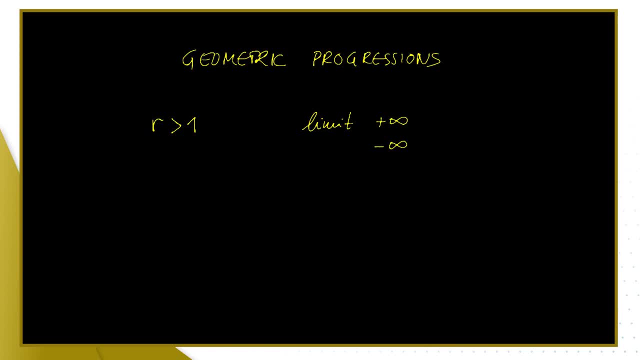 number like two and you multiply by three every time you're going to get a positive infinity limit. It's divergent. but with plus infinity limit, If you start with a negative number and keep multiplying, say minus two- and keep multiplying by three, you're gonna make it more and more. 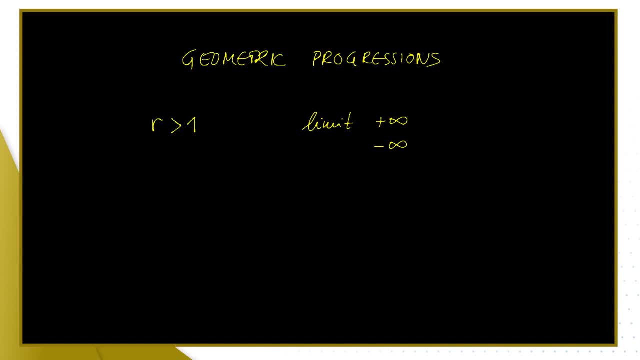 negative and really large. so negative infinity in the limit When the ratio is less than negative one. if you start with a positive value, so you start with two and then keep multiplying by minus three. you're going to have sometimes negative, sometimes positive values, but it's still going to be large in magnitude, so it's 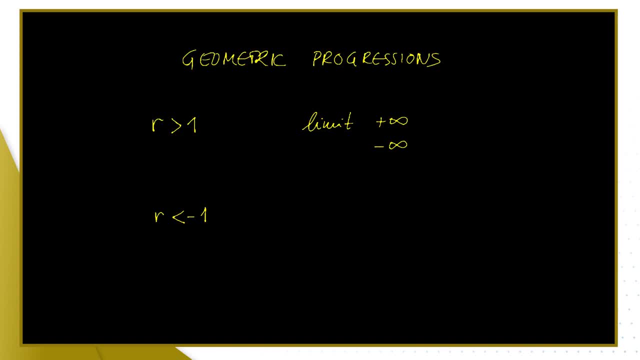 going to be divergent, but the limit will not be plus infinity or minus infinity. there will be a difference. no limit, okay, So no limit. And if you started with a negative value and keep multiplying by a negative number, you'll still have the same situation. The sweet spot of convergence is 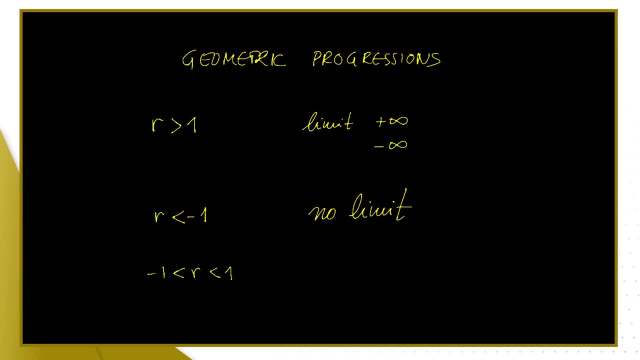 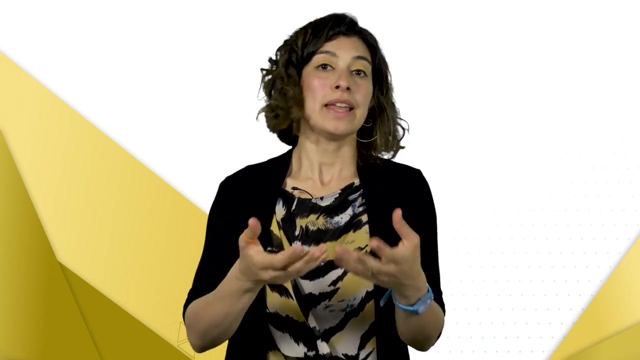 between minus one and one. If the ratio is between minus one and one, you are shrinking the numbers in magnitude, sometimes alternating if the ratio is negative, but it will shrink down to a value, So we'll have convergent. Okay, Now it's up to you to go and practice these skills. 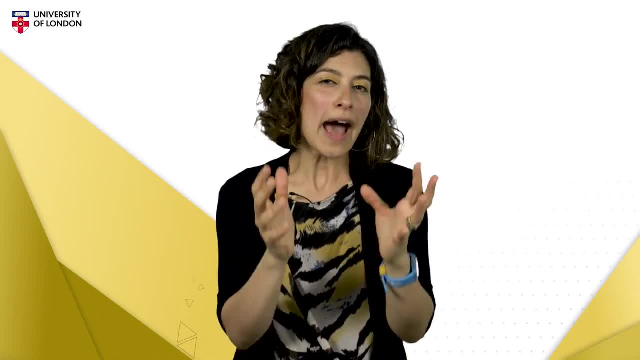 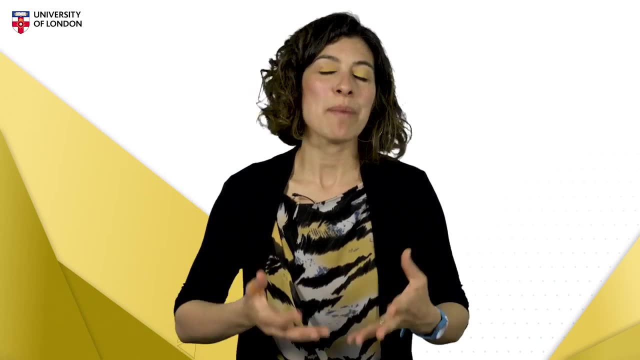 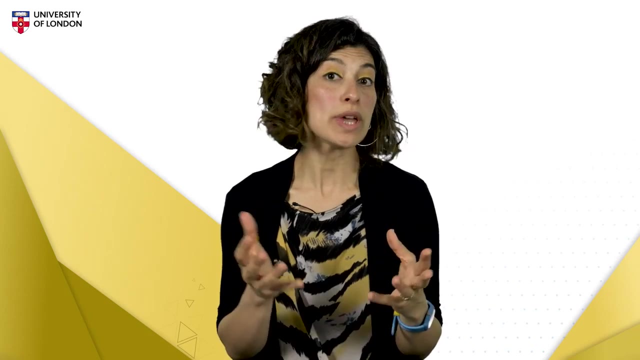 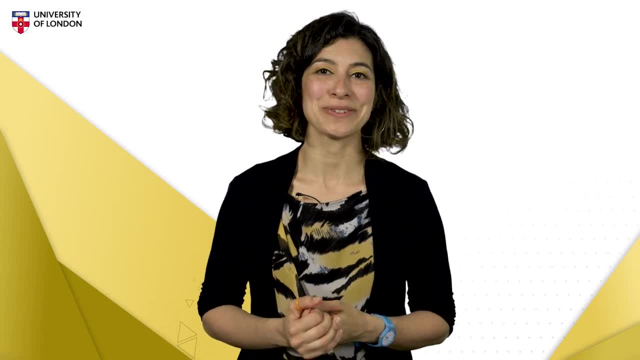 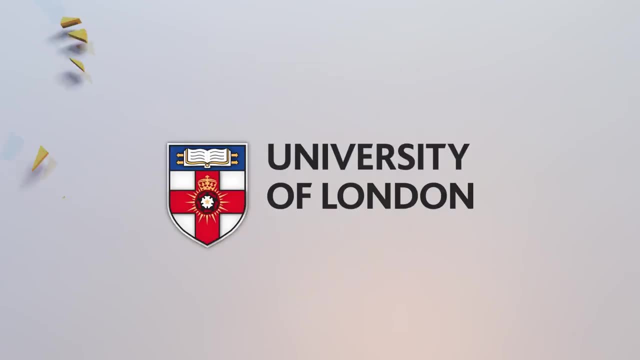 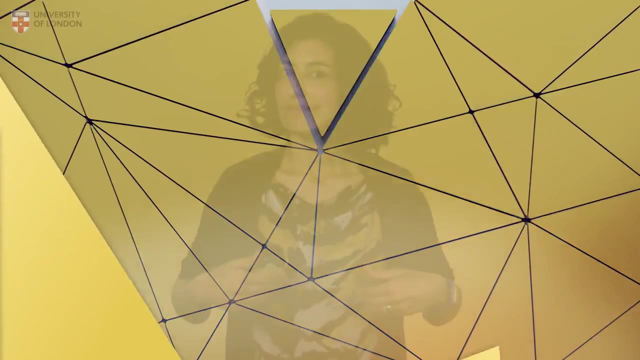 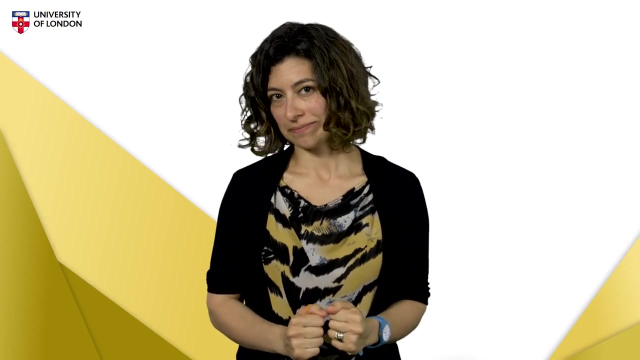 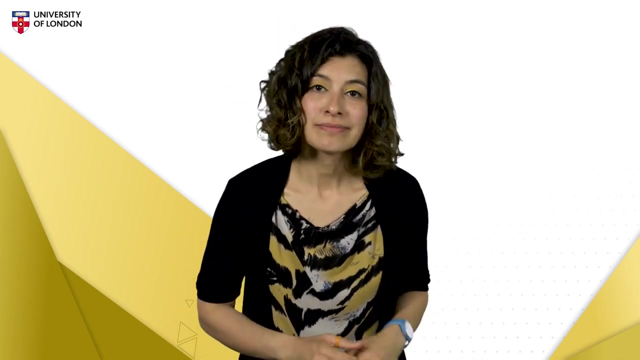 a finite limit? We'll find out next. Can the sum of an infinite number of terms of a sequence be a finite limit? Can the sum of an infinite number of numbers ever be finite? This is what this video is about. The answer is sometimes yes. It goes without saying that. 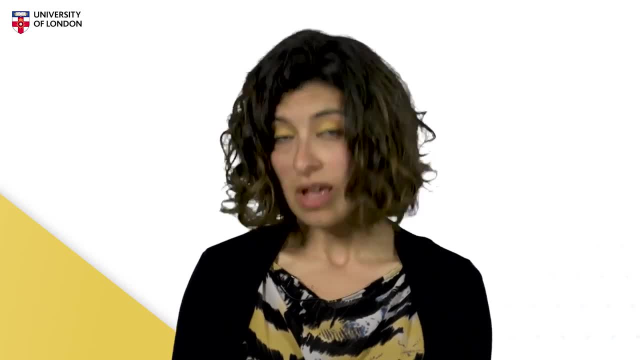 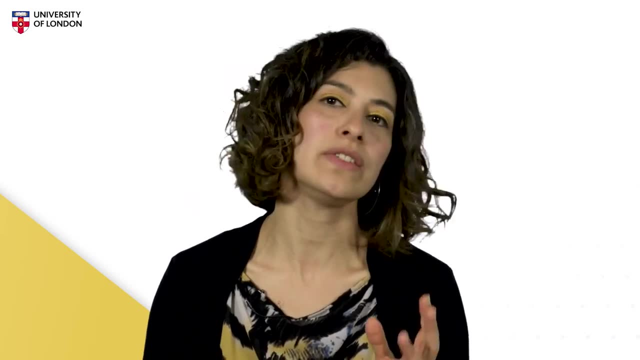 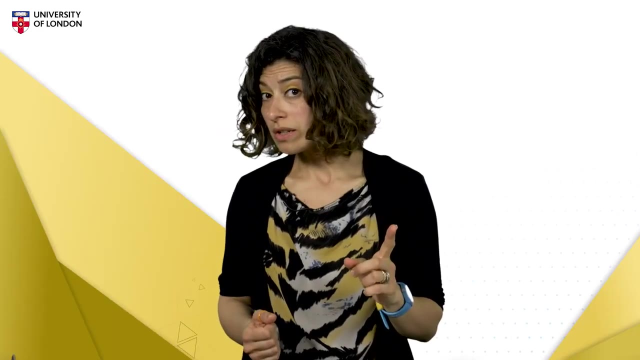 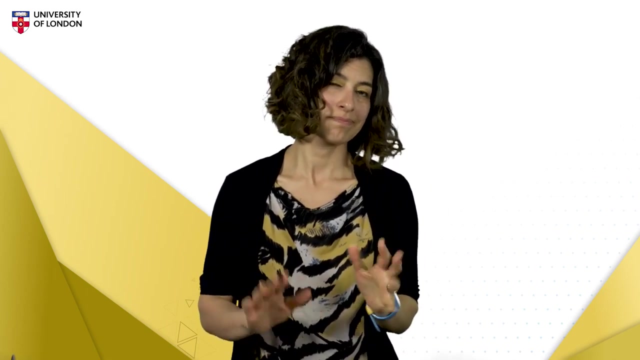 the numbers we are adding up cannot be very large. In fact, the starting point is: the sequence we are adding up has to be convergent to zero if we are even going to consider the infinite sum. But not all sequences with zero limit will have a finite sum. Let's get this in writing. 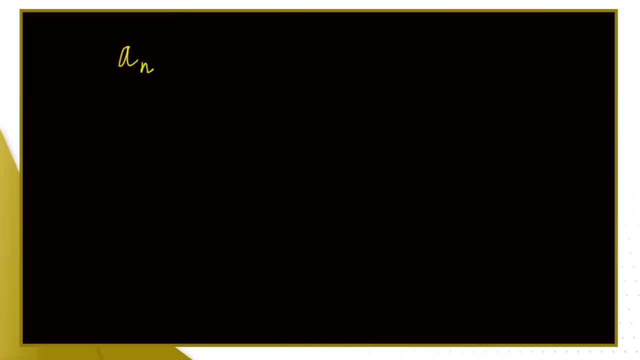 So I'm looking to adding a sequence, sequence a- n and adding the sequence a- n We've seen earlier. we will have a summation symbol. We're adding the sequence, I'm going to change the variable. as for k, and I'll say I'm going to start from the first term, I'm going to add it all the way. 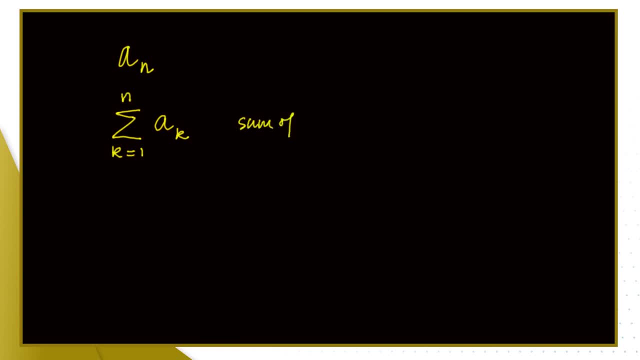 to n. So this is the sum. I'm adding up the sequence. I'm adding up the two numbers of the first n terms And the expanded form is a1 plus a2 plus all the way to a n. I'm adding that sequence, That's. 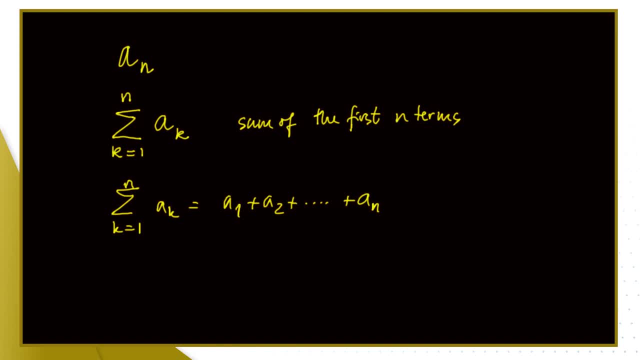 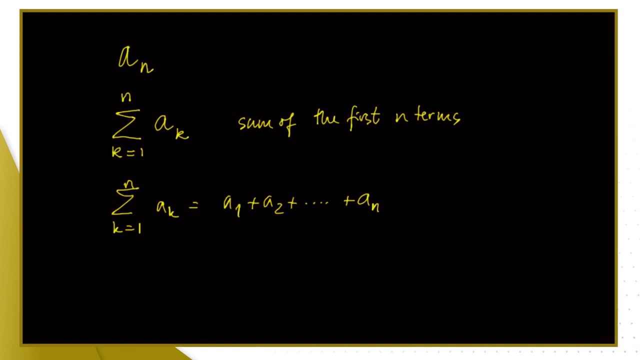 the series, The first n terms. What I'm asking here about an infinite sum is: as n goes to infinity, what is the limit of this sum? So I'm actually asking you to consider this sum as a sequence itself. So for each value of n, I've got a sum up to value n. 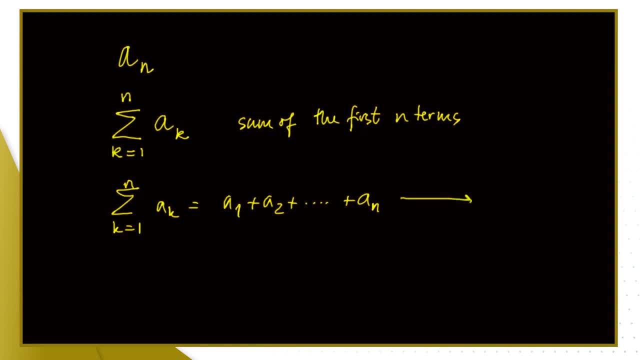 And as n tends to infinity, is there a limit? So, in other words, I'm still adding up the same sequence. My label runs from 1 to n, as n tends to infinity, So I'm going to write all the way to infinity there at the top. 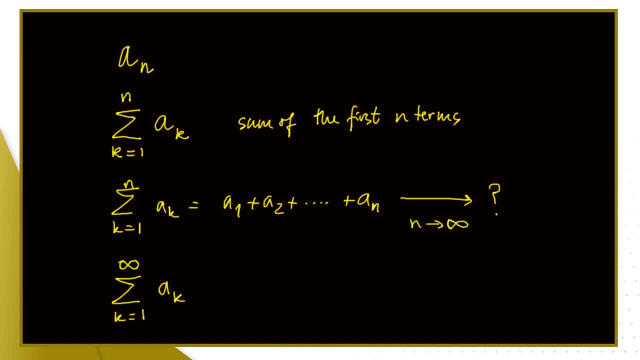 This is the sum of all the terms of that sequence. So this is the series we're interested in in this video. So I said that the starting point is: don't even bother trying to add up sequences that are too large, Meaning If the sequence I have here doesn't converge to 0,. 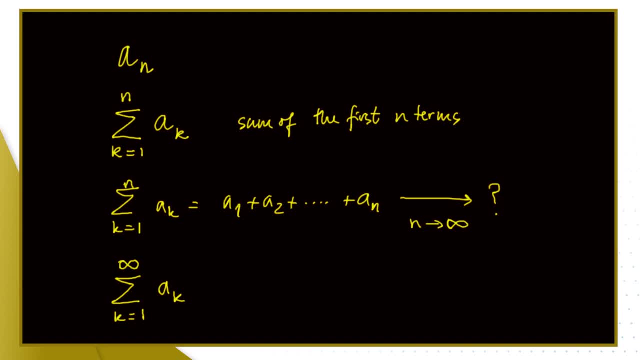 then there's no point looking at the series, because the series will have an infinite value or it will be divergent. So I'm going to write that down, saying a series, an infinite series like this, can only converge if the sequence itself is convergent to 0.. 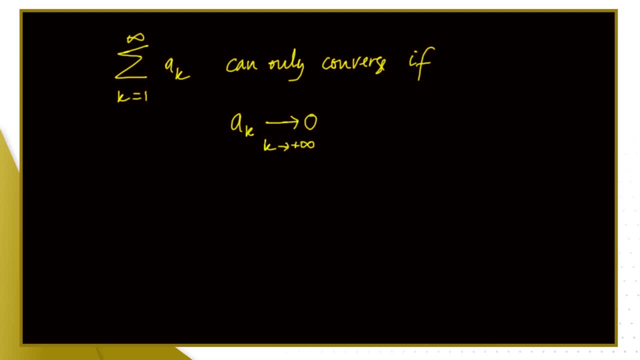 So this means this is a necessary condition for the series to converge. It's a necessary condition. It's not a sufficient condition. The sequence converging to 0 does not guarantee that the sum does, So I'm going to show you both situations. 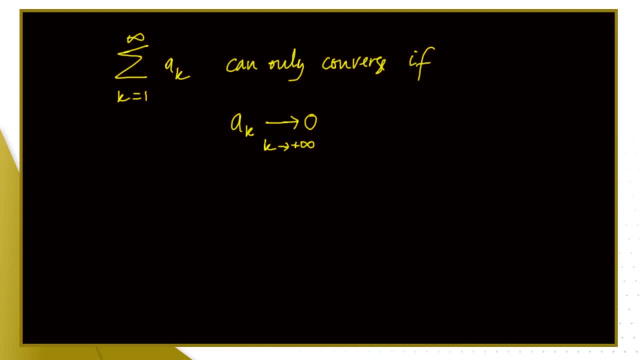 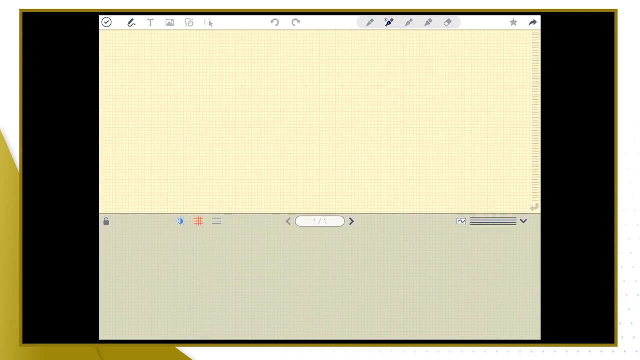 So, to start with, I'm going to show you a series, an infinite series that converges. So I'm going to draw a picture. Just follow me in this. So I'm going to start with drawing a rectangle here. So there's a rectangle. 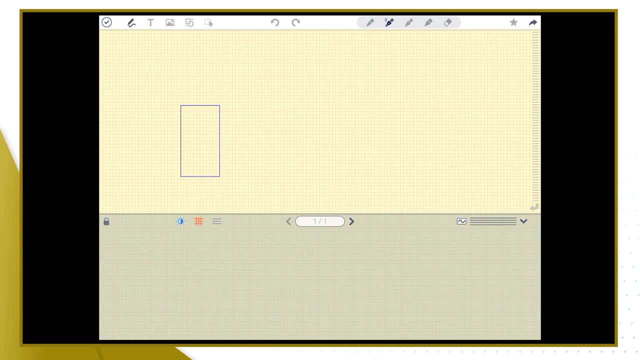 And now I'm looking at the area of rectangle. So I'm considering that area and then I'm going to add half the rectangle to it. So Same width but half the height. So I've got the first rectangle, then half of it, and now I'm going to half. 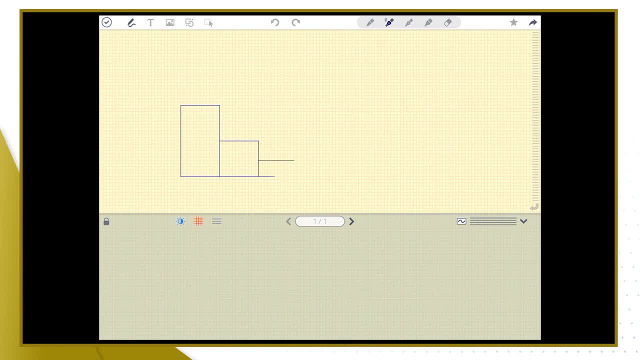 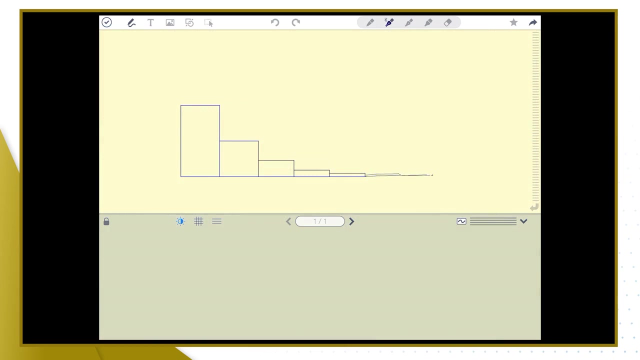 that again and half that again roughly, and so on and so on, And thinner and thinner. So the question is: this area, Okay, Okay, Added with this area, with this area and that area, and so on, and so on, and so on. 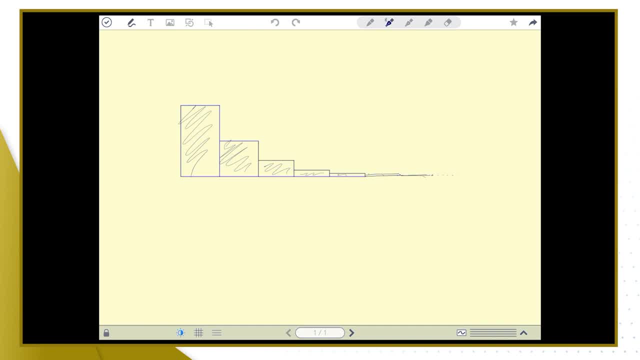 What is the total if we keep adding? Well, we're adding, say, we're adding an area of one rectangle plus half of that area, plus a quarter of the initial area, plus an eighth, halving every time, and we keep adding all the way to infinity. Is this a finite area? 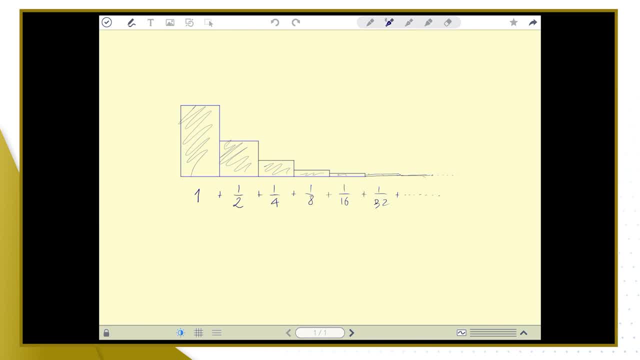 The answer is yes. Now I can convince you of this by showing you the detail on the diagram. So what I'm going to do is I'm going to shift this rectangle here over there, Because that's a quarter of the total, it's a half of the half. it fits there, So I'm going to remove that one. 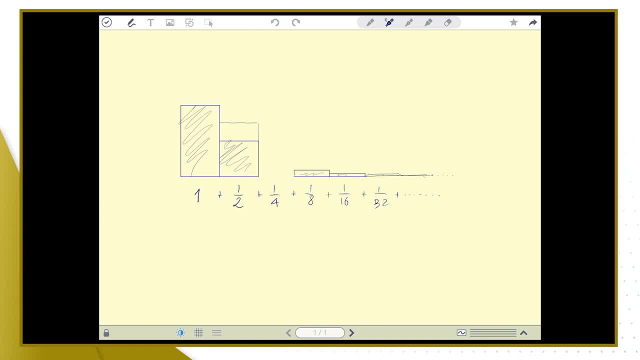 And now this one here is going to fit, Okay Okay. And now this one here is going to fit over there, So I can remove it. So this part is going to fit there. It's actually half that space, So I'm going to put it in there And 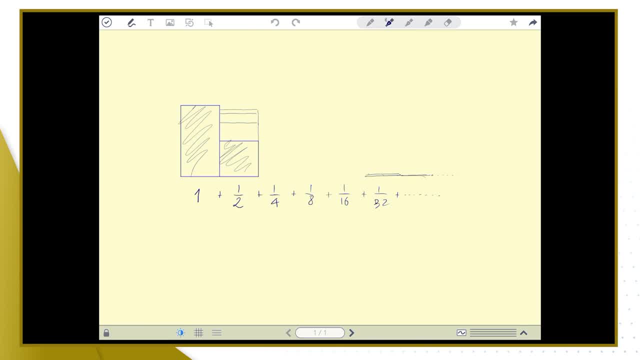 I just carry on in this fashion, All these next halves of halves of halves of halves are going to fit in the space. So in total, if I add all the way to infinity, I'm going to fill in the rest of the space. Well, theoretically, if I could physically add up all these infinite. 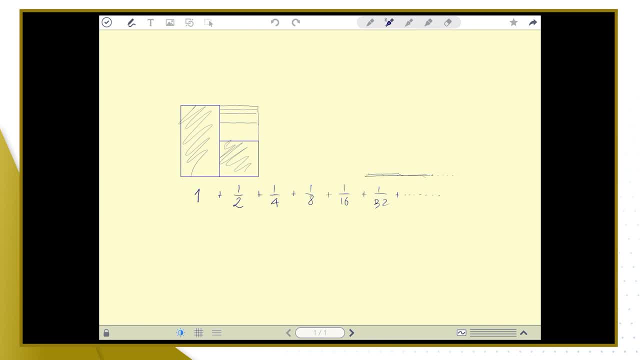 quantities, I would get the whole space filled in. So if this part is one as well and that's another one, this sum should be two. So I'm adding an infinite number of halves, of halves, Number of numbers, And I'm getting, as a result, two. Now, if this is a little bit hard to 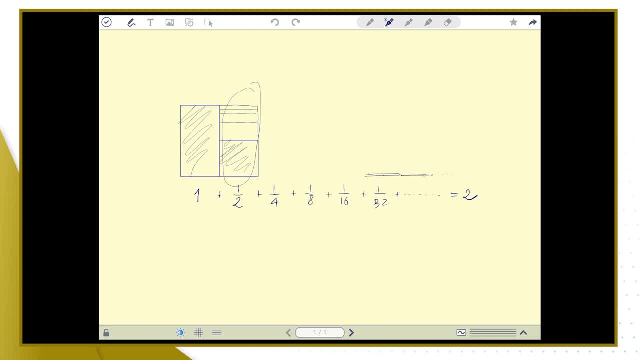 stomach. I'm with you. We can't actually physically add up an infinite number of numbers, But it's the concept of limit, like we used earlier in limits of sequences. So what we're getting is that, as I add more and more terms of this sequence, so partial. 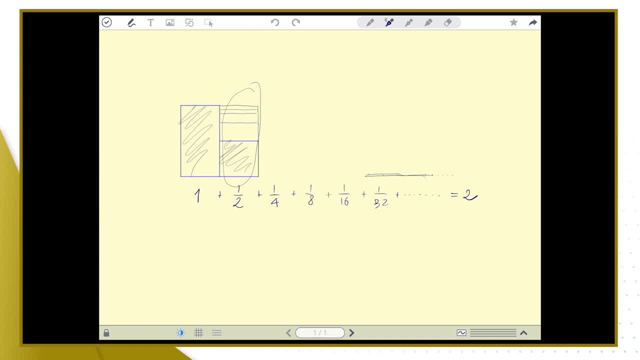 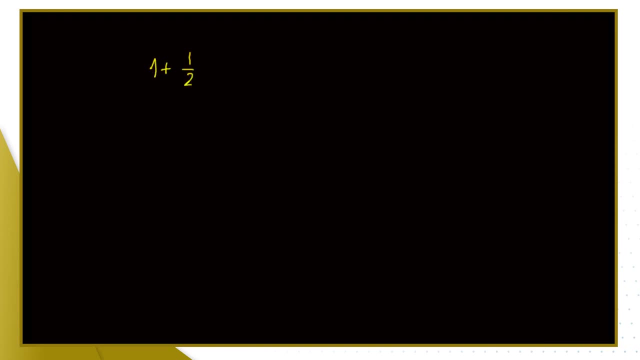 sum, So the finite series, And as I increase the number of terms in the limit, I approximate two. I can get as close as I want to two. So I'm going to write this down. We looked at the series one plus one, half plus one quarter, plus one eighth, and so on all the way to 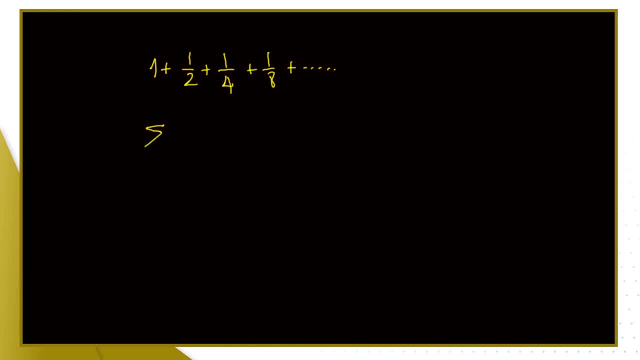 infinity. That is written as the sum of the sequence one over two to the power of infinity, When n runs from zero all the way to infinity. Let's check: When n is zero, I have one half to the power of zero, and that is one. When n is one, I have one half to the one which 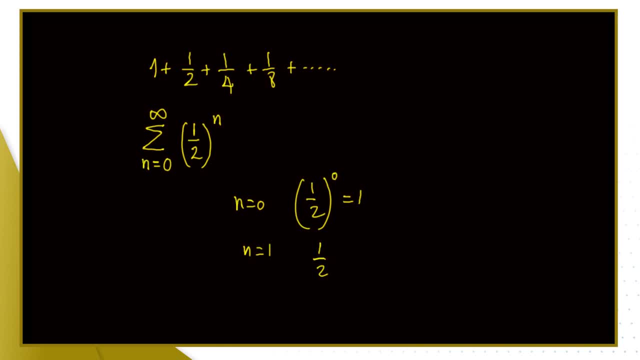 is one half and so on. So because I want all the terms, I am adding them up from zero to infinity. So this is the sum I want And what I'm saying is I consider partial sums, so finite series, I can do k from zero to some value, n. Actually I'm going to put 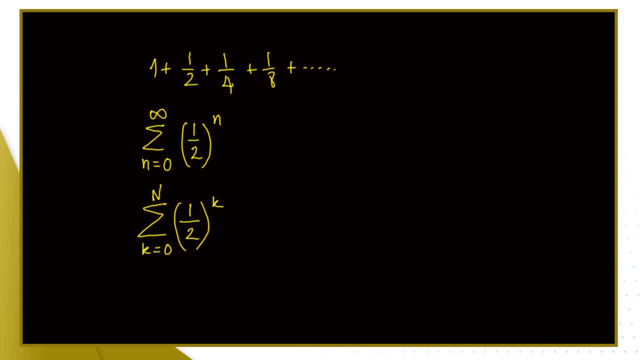 large n there, so there's no confusion. So for n, that could be 1,, 2,, 3, you know any number. And then let's see what that means. That means that when n is one, I'm doing the. 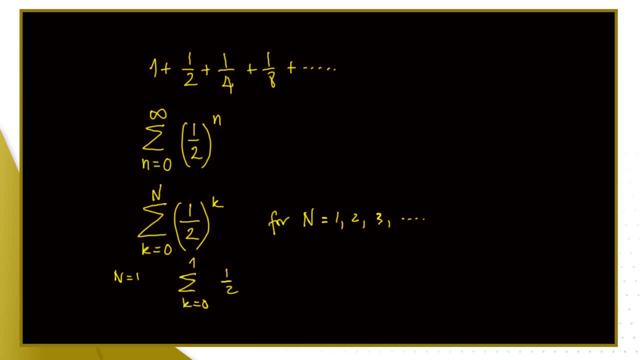 sum from k equals zero to infinity. So I'm going to multiply this by one, and this is exactly the same thing that I did in the first case, And now I'm going to multiply this zero to one of a half to the k, and that's the sum of one plus one half When n is two. 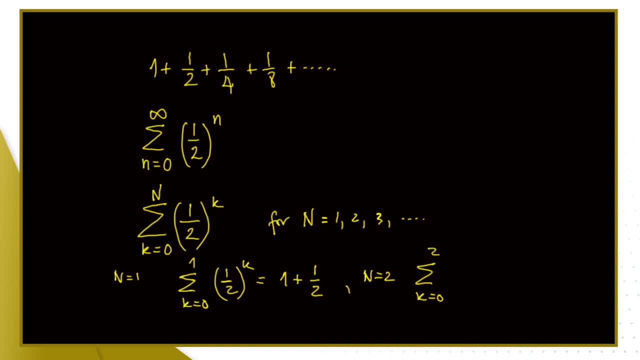 I'm doing the sum from zero to two and that's going to be one plus a half plus one quarter. The sequence is the sequence of these partial sums. This series has a limit because the sum k from zero to n, of one half to the power of k, has limit two, when n tends to infinity. 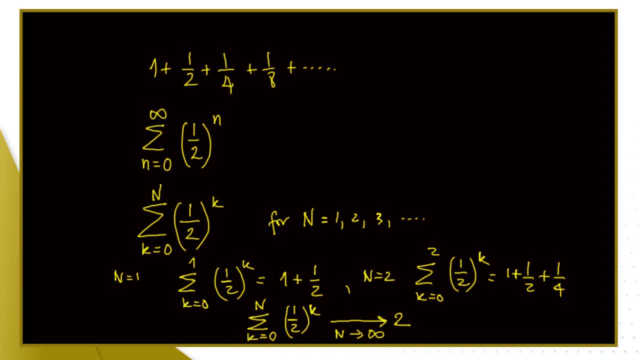 We have looked at that geometrically and I gave you a nice argument for why that is. two: You may want an analytical or an algebraic method of proof that is a bit more reliable than my drawing. I'm with you. We are doing maths and computer science, so we need to do that. 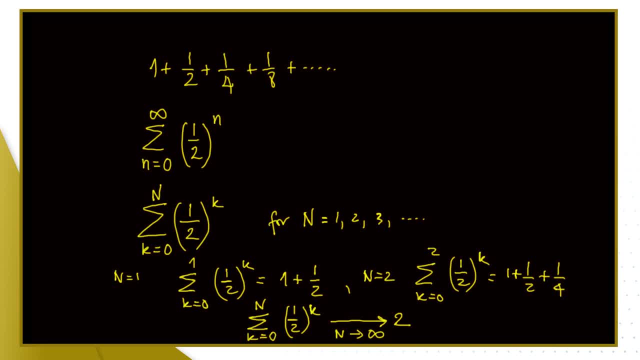 I'll go into that. So what's going on here? I've shown you this example to give you an example of a series that has a finite sum. So, in short, the sum of a half to the power of k and k, from zero to infinity, that sum is two. Now I said that, the sequence itself converging to zero. 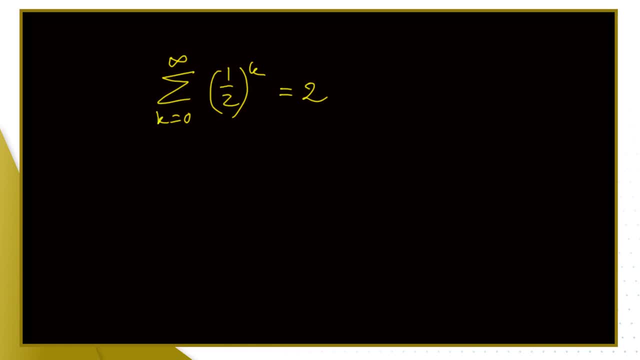 was not sufficient for the series converge. I'm going to show an example of that. So if I have the sequence 1 over n and I'm going to add the sequence, so I'm going to do the series when n goes from 1 to infinity. Now the sequence. 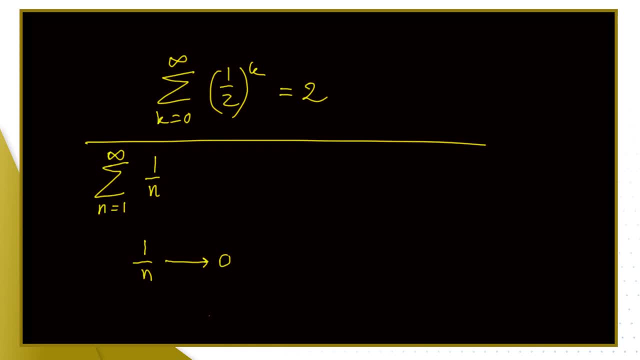 itself. so the 1 over n part that converges to 0, as we saw earlier in another video That converges to 0, so it satisfies the necessary condition. but this sum is not finite, So meaning that when we add 1 plus a half, plus a third, plus a quarter and so on, this sum is going to blow up, Even though 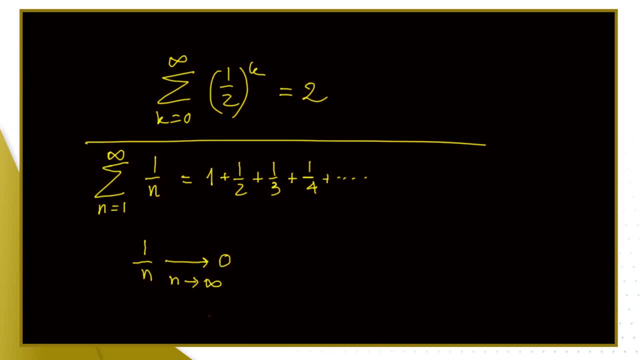 the terms you're adding are smaller and smaller. they're not small enough. They will still compound to a root. So if I have the sequence 1 over n and I'm going to do the series when n goes from 1 to infinity, this is going to be a really large number. So this is going to be divergent. I am not. 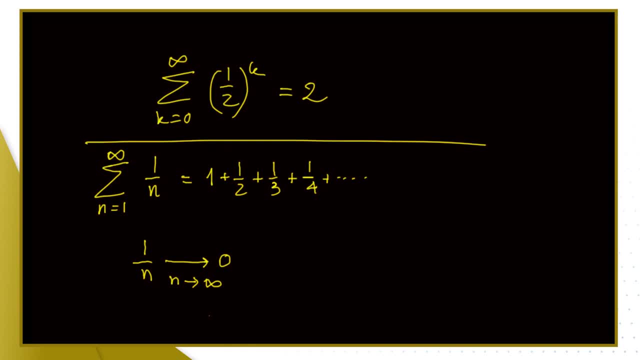 going to prove it to you. There are plenty of proofs you can find in references. I do encourage you to go and find that out because it's quite intriguing. This is not slow enough. it's not small enough to add up to a finite number. Now, this is called the harmonic series, If you want. 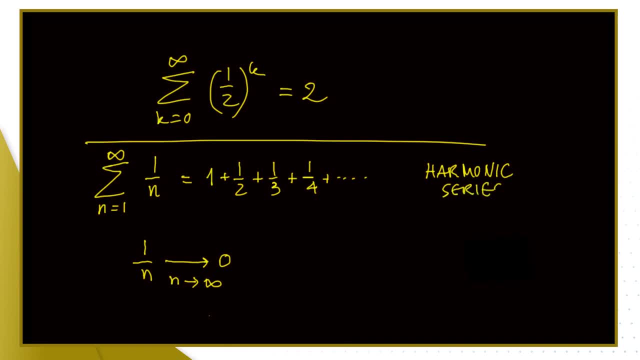 to look it up. that's the harmonic series and the example we saw earlier. you've probably probably spotted that it was a geometric series and it's a geometric series as we saw earlier. So in this module we're going to look at convergent series, we're going to look at geometric series. 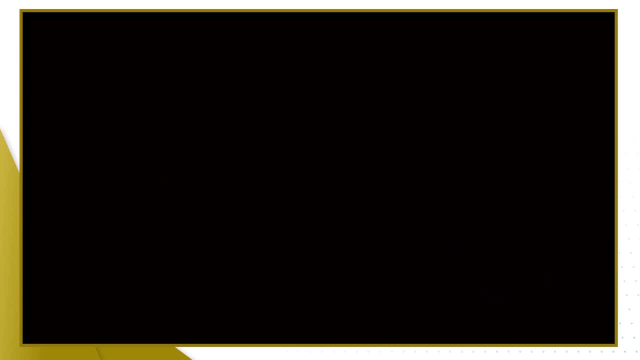 and there's one type that converges. We saw earlier in the course that the finite sum of a geometric progression of common ratio, r, that finite sum has a formula that is r to the n minus 1, over r minus 1.. And now we need that r isn't 1, and that is a finite. 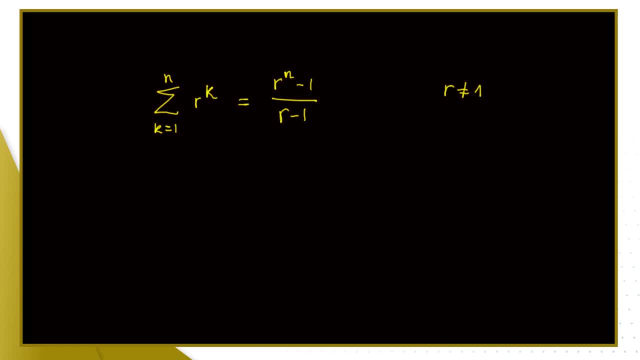 sum. Now, if we look at that, looking for the infinite series- we're spoken about r minus 1, plus r minus 1, and assume the Supremacy после n going to infinity. Now, as n goes to infinity, we need to look at what happens there. We've got 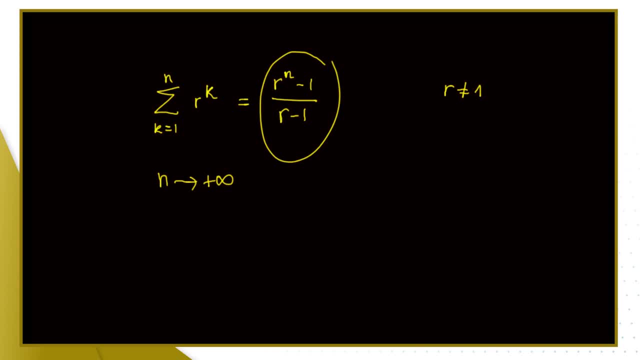 a geometric sequence there with r to the n. Yeah, I know it's subtracting 1, dividing by r minus 1, but it's essentially that is comparable to r to the n or r to the n minus 1.. It's comparable to that. So this kind of sequence only converges when r is small, when r is between minus 1 and 1. 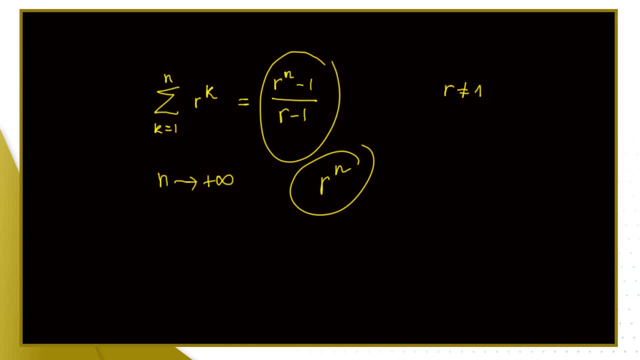 and when r is between minus 1 and 1 is exactly when the geometric series with infinite items, with infinite terms, will converge. So r to n minus 1 over r minus 1 has a finite limit when n tends to infinity If, and only if, r is between minus 1 and 1.. Okay, and that limit is well if r is between minus 1 and 1. 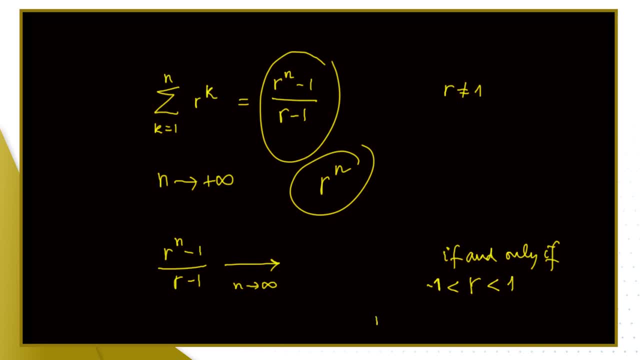 r to the n converges to 0.. So r to the n converges to 0 and it converges really fast, exponentially fast, and that means that guy goes to 0. that means this limit is minus 1 over r minus 1, which if we rearrange would be 1 over 1 minus r. 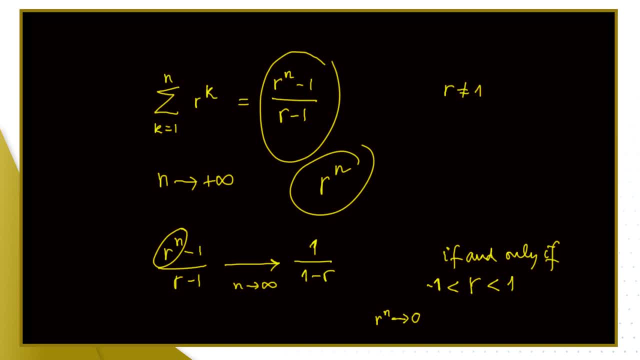 Right. so what I just said is that the infinite sum, the infinite sum is 1 over 1, minus r, if, and only if, r to the n converges to 0. That was the series of infinite terms, that r is between minus 1 and 1.. 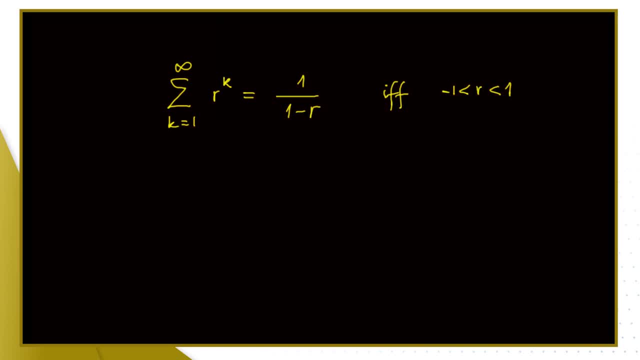 r is between minus 1 and 1.. So that is the series with the finite infinite sum that we will use in this module. Okay, so let's look back at our example. we had one plus a half, plus a quarter, plus an eight, and so on. 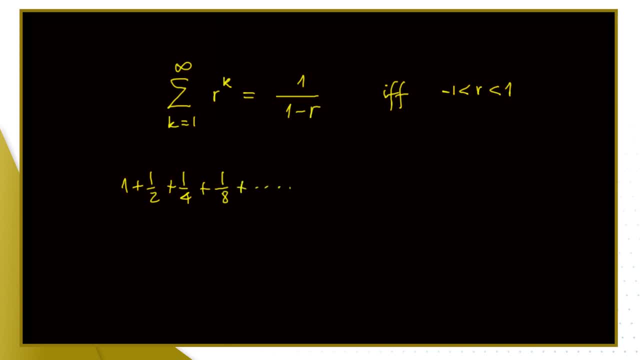 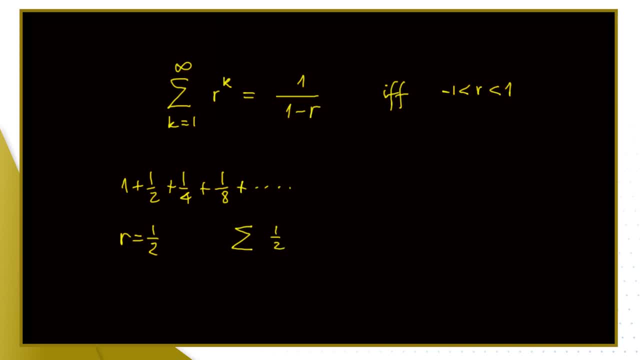 let's carry on: The sum of a half to okay, from one to infinity. that's going to be one over one minus r, r is a half. okay. That means I've got one over one half, which is two. Okay, so that one is convergent and that type of geometric series is convergent. 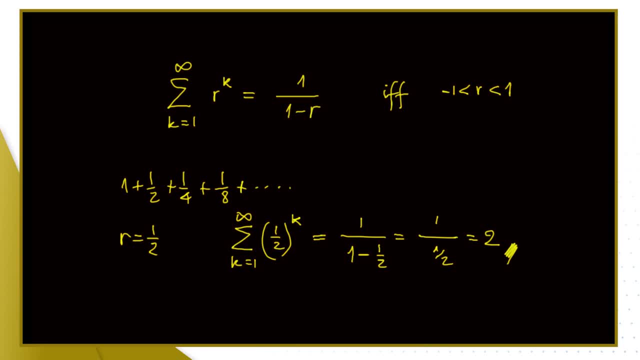 We have a formula for the sum- brilliant. I'm just going to recap that. all the others we've seen aren't convergent. So things like sum of two to the k, when k goes from one to infinity, this is divergent. 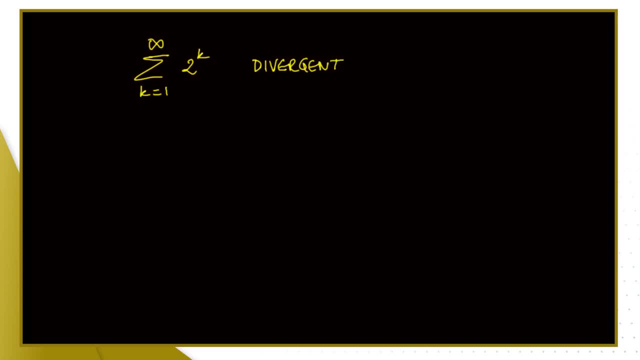 It has an infinite sum. okay, And in fact, if you've got that sum of a geometric series, when r is greater than one, then the sum is also divergent. It's also true that if r is less than negative one, that sum is also divergent. Now, when the common ratio is less than negative, 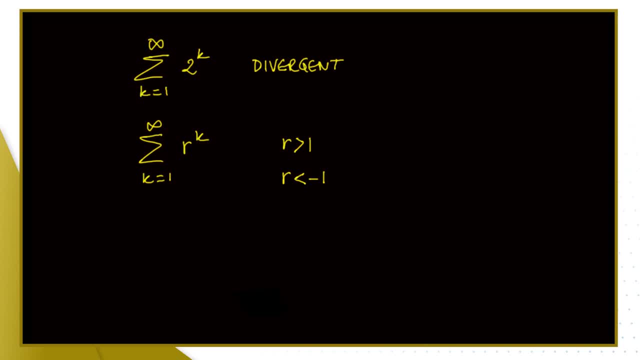 one. one might think: well, some terms will be positive and other terms will be negative, So maybe the sum of the positives and the sum of the negatives kind of cancels out and we have something with a finite sum. It's a good idea, but let's see what happens. 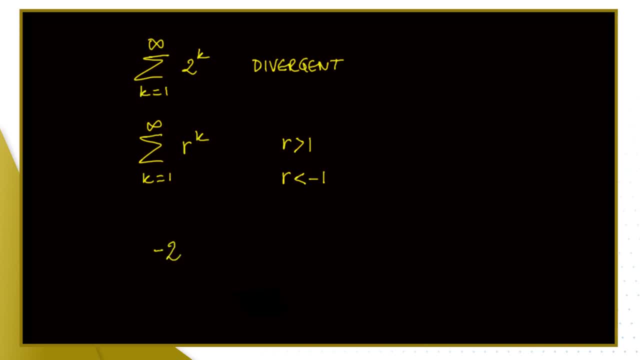 Say: the example is: I've got ratio minus two and I'm adding powers of that, I would have minus two at four, minus eight at 16,, minus 32 at 64, and so on. okay, The next term being negative, the other one positive, and so on. Now, if we pair up numbers, 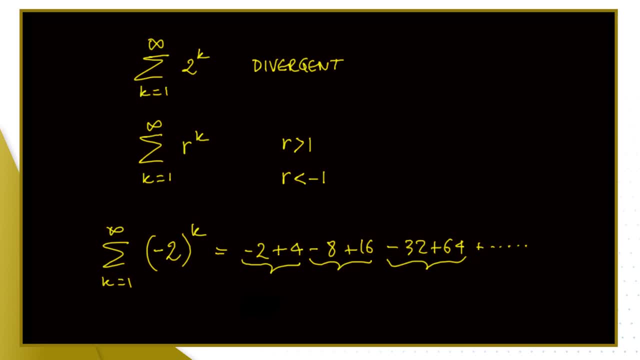 like this: the sum is two here, it's eight there and it's 32 there. We're still adding up a sequence that doesn't converge to zero. So let's look at another example of using the sum of a geometric series. 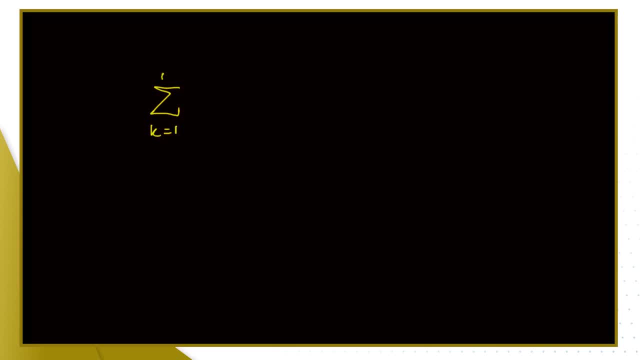 Let's do the infinite sum of three times 0.1 to the power of k Infinite sum. How do we use our series formula? So I'm multiplying the geometric series here by a factor of three, so I can take that three out. 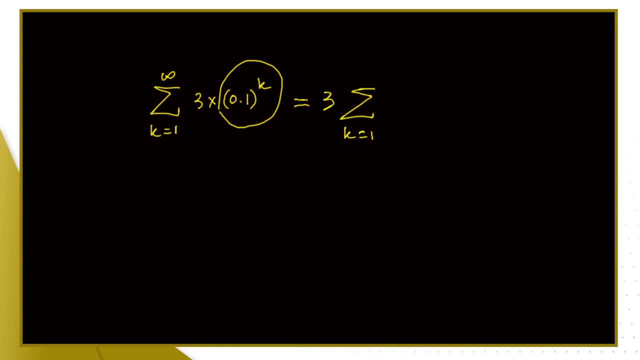 and multiply by the whole sum. That's still possible with infinite series, okay. So that's all I'm doing. and now I've got pure geometric series to add up and the common ratio is 0.1.. So I replace the series by the formula. so 1 over 1 minus the ratio, okay. 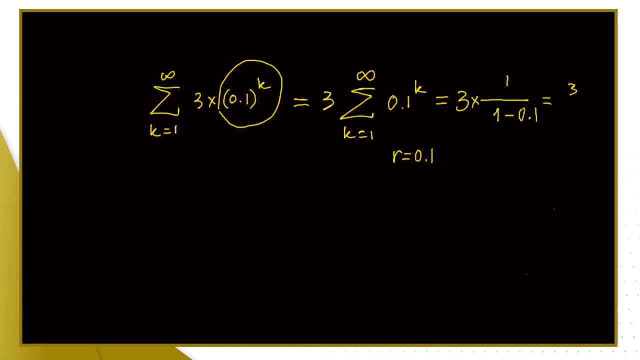 So I have 3 over 0.9,, that's 27 over 0.1, so that's 270,. okay, So the sum of three times 0.1 to the k totals 270.. Okay, So there's another example. 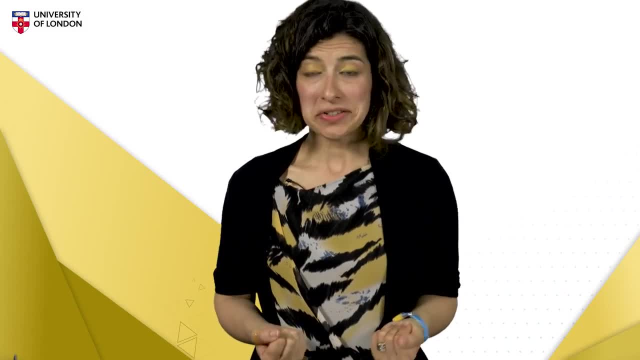 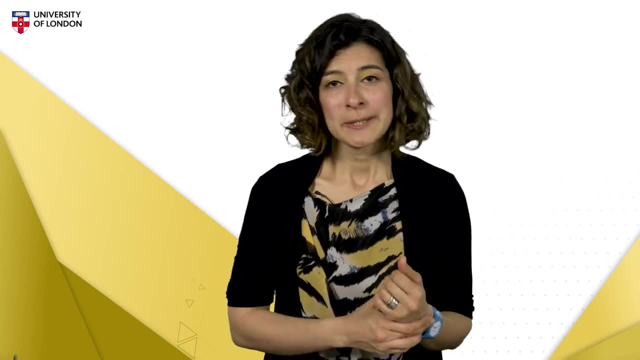 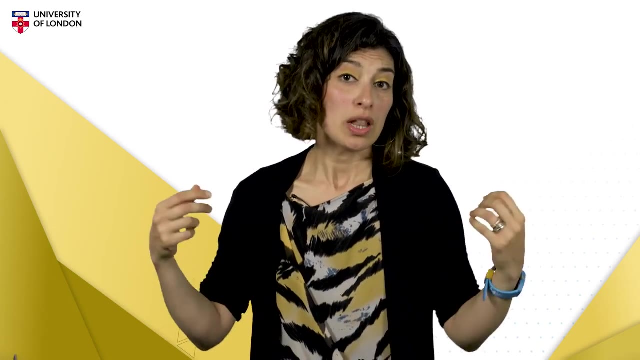 Now, why would you care about this as a computer scientist? Surely you're not going around adding areas of crazy rectangles that go all the way to infinity. Yes, true, you are not going to do that, But as a computer scientist, you will compute loops. 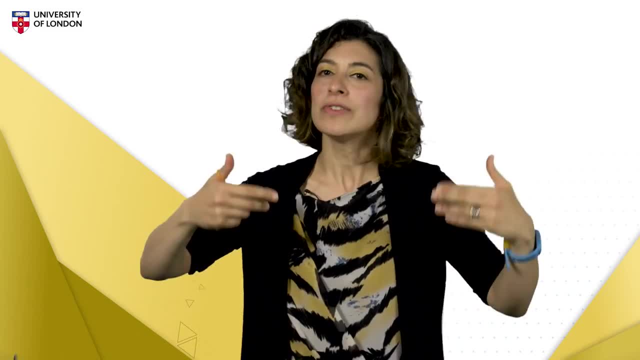 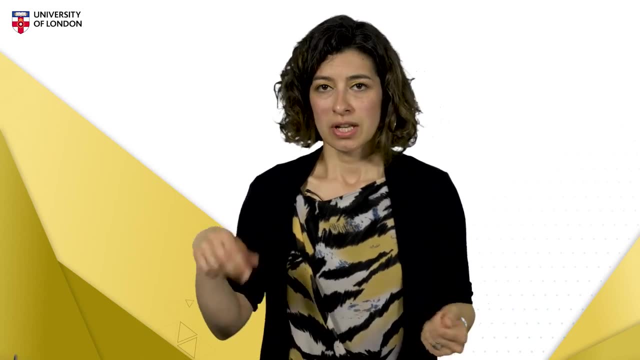 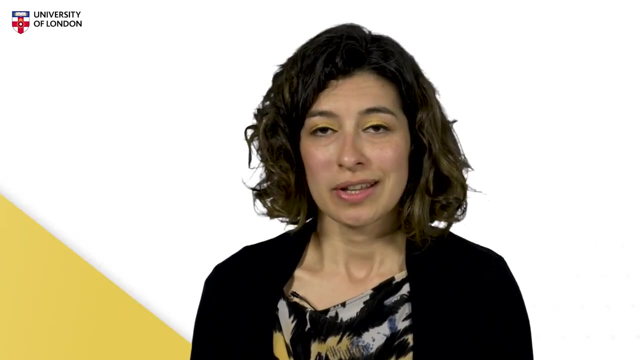 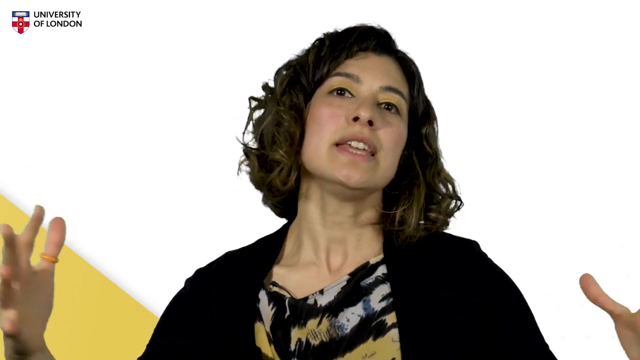 You will compute sums of consecutive terms on the loop, So you'll have something like 4k from one to a thousand. add this term to this existing sum. You've got to be careful about sums that will overflow, sums that will become really large, so large that you run out of memory to do the computation. 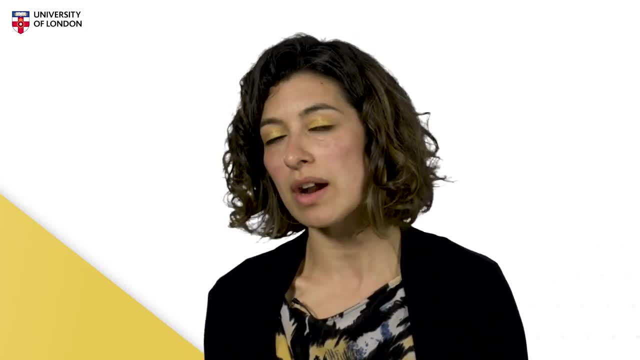 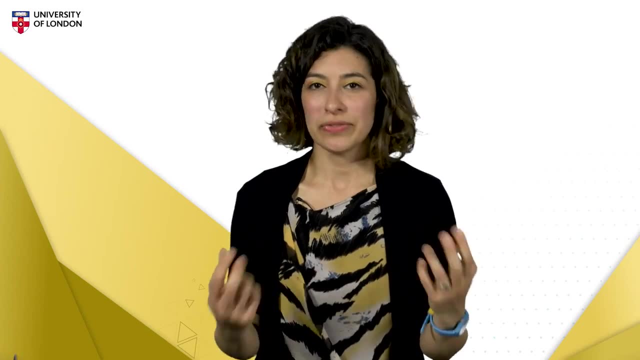 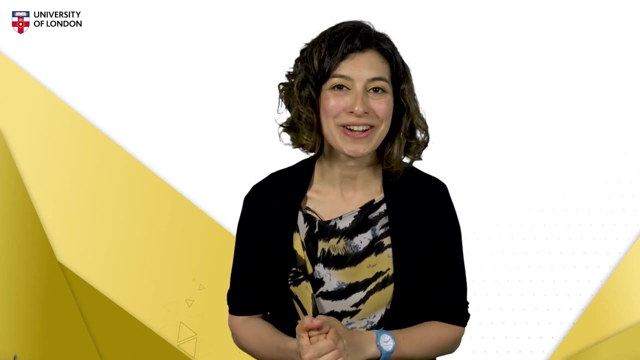 or you will lack precision, So you need to be aware of how far you can add up such things. Also, any numerical analysis of sequences and series that may come across in terms of performance or complexity. this is part of your numeracy and your literacy in mathematics. 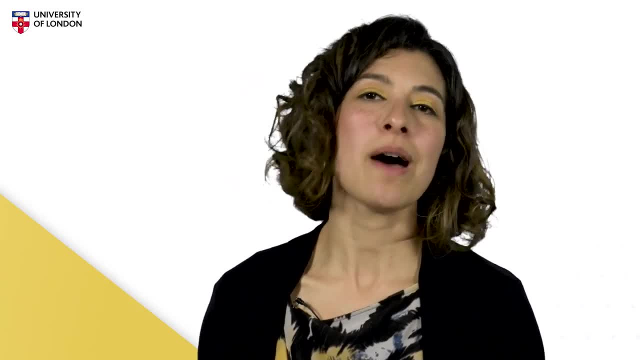 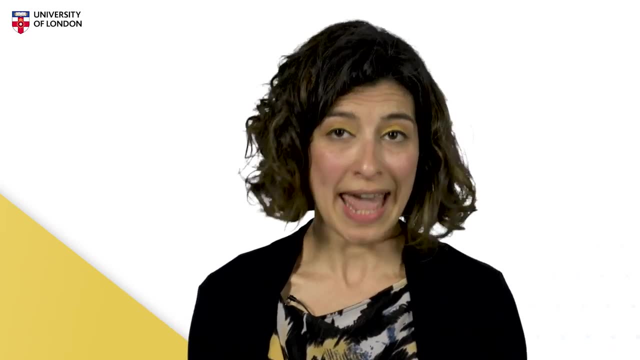 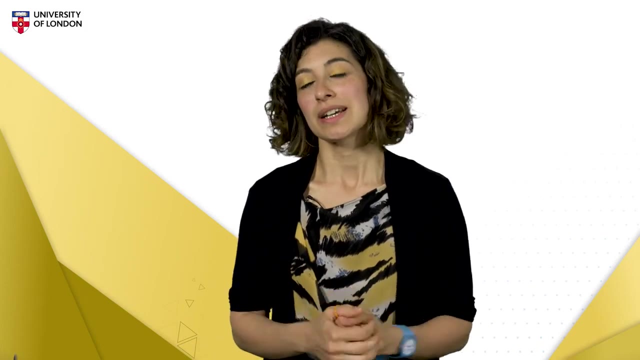 I leave you as an exercise to apply the sum of the geometric series to the place values in binary or the place values in any any base. One connection with the real world. and I do love paper. I use the A format paper a lot. A4 is my favourite printing format. 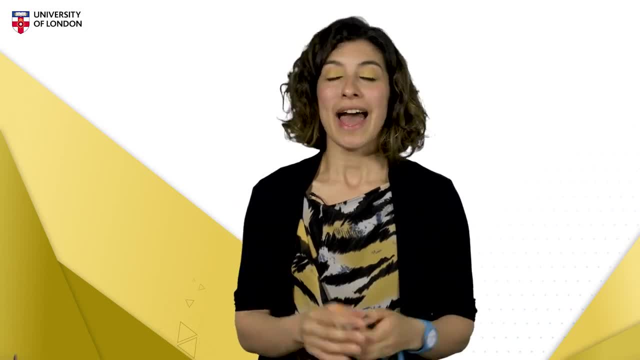 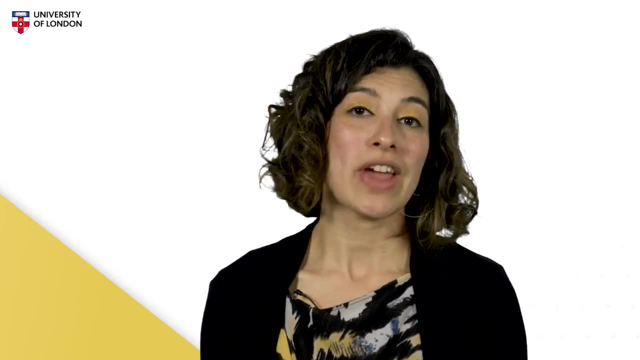 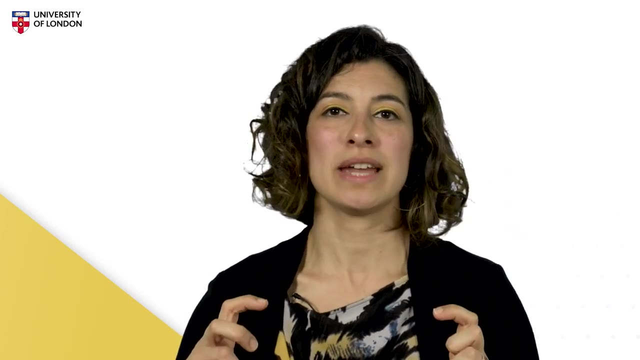 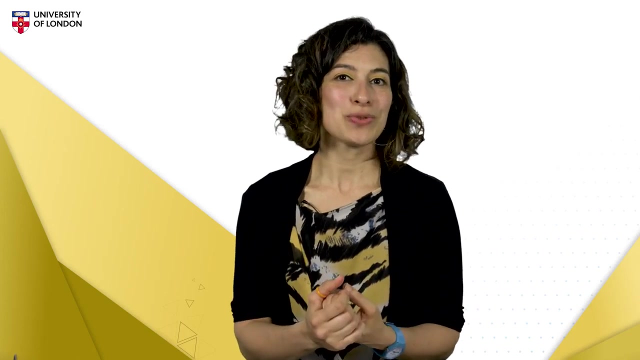 and the format A for paper has a very specific property. When you half a page, the smaller page has the same proportions as the bigger sheet of paper. So as you fold you keep the same format but the sizes shrink down And it's a particularly nice paper format to explore geometric sequences. 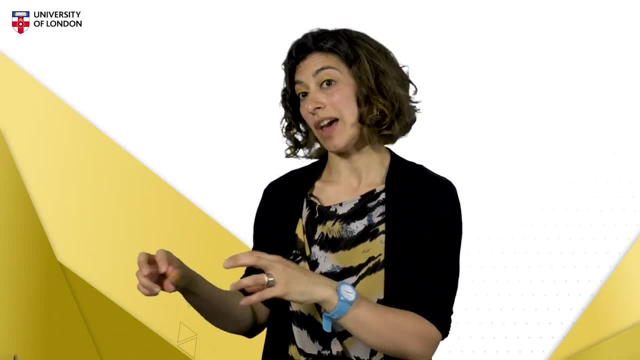 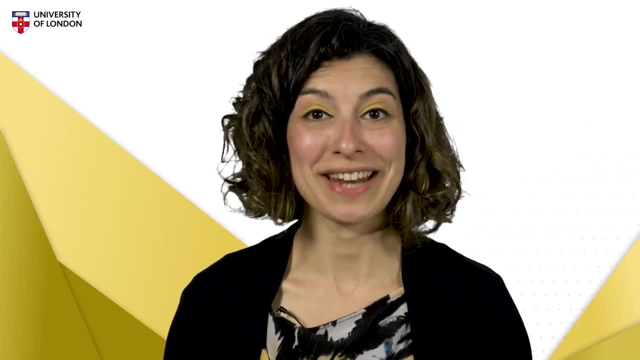 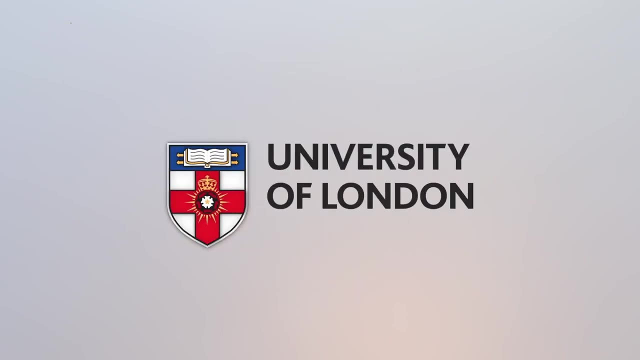 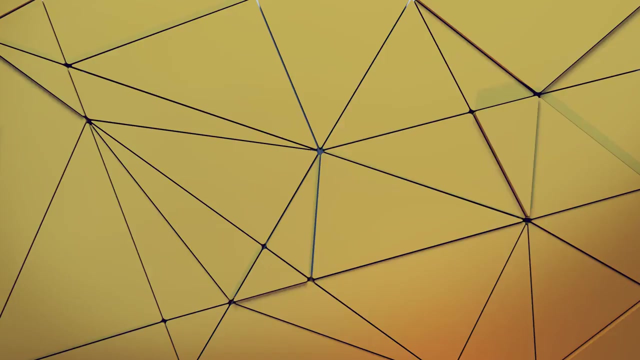 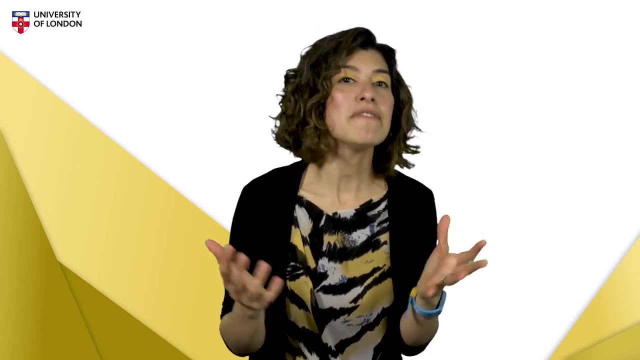 and if you want to add up the area of the sizes of paper, you'll be looking at the geometric series too. So go ahead and practice economy. Wow, You have a great deal of information now about limits of sequences. You saw the convergent sequences 1 over N. geometric progressions with: 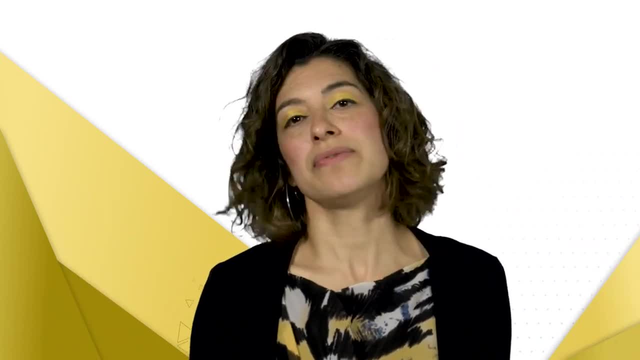 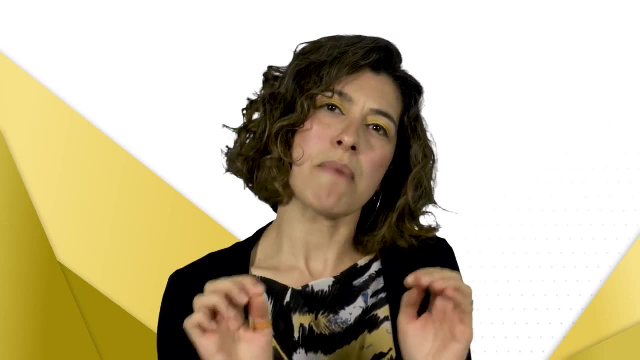 ratio between minus-one and one. We intuitively used the following idea: If two sequences come descending from the top of the table- they're Canon's curves- What is the sequences are convergent. then adding them up gives a new sequence that is convergent. 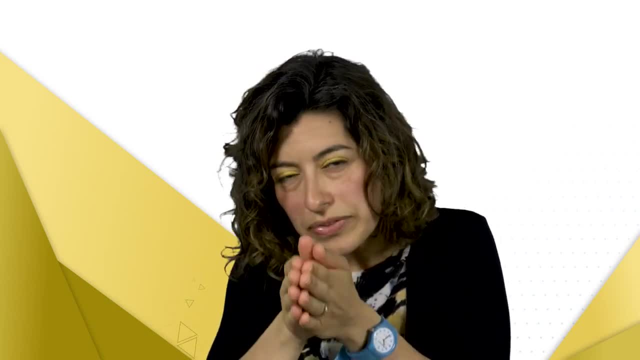 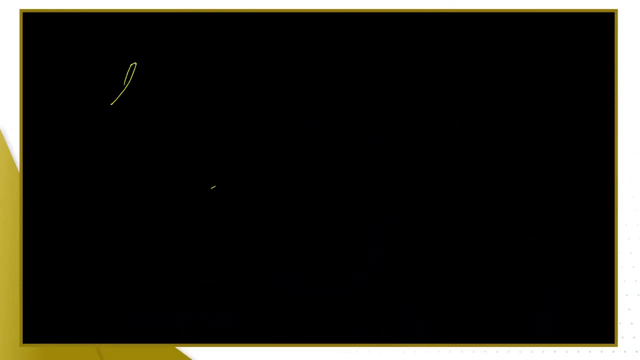 to, and the limit is the sum of the limits of the two sequences. I can write that as the limit of a sum of sequences is the sum of one limit with the other limit, Of course if a, n and b? n are both convergent. 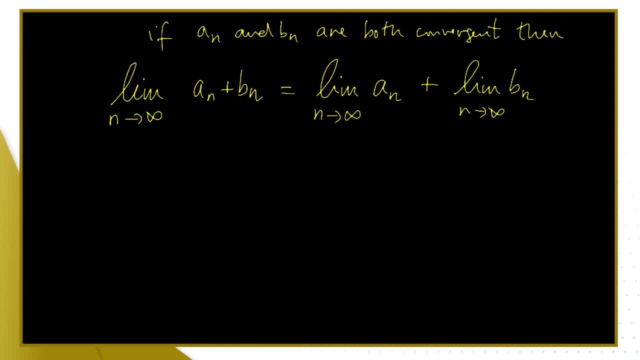 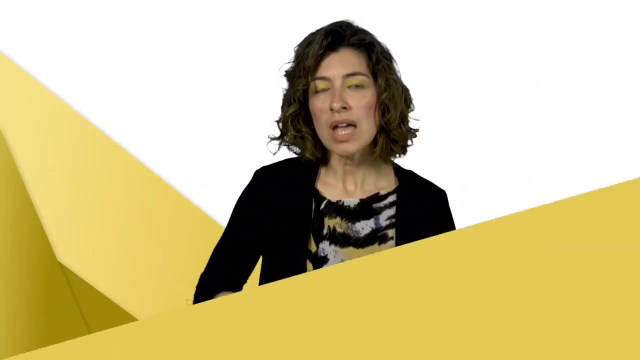 Meaning that a n plus b? n is also convergent. I mean, we're not only saying that the sum is convergent, we actually tell you exactly what the limit is. Now here's another case. We also used intuitively the fact that multiplying 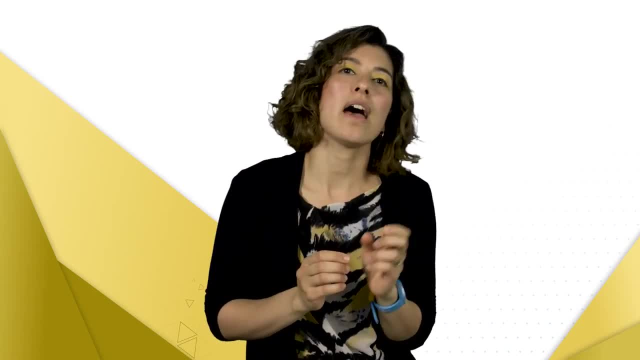 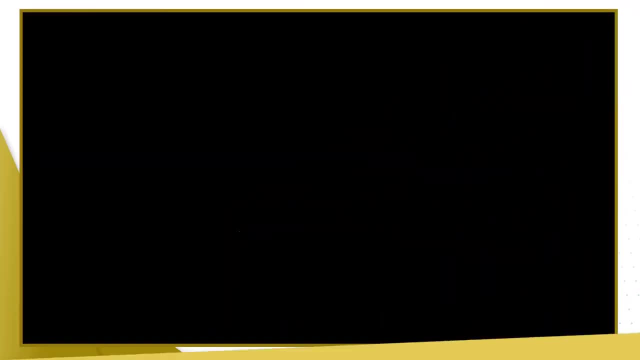 a convergent series by a constant still results in a convergent sequence. And we can write that in this way: If a, n is our convergent sequence and c is a constant, then I'm saying that multiplying the sequence by a constant, just we take the limit of the sequence itself. 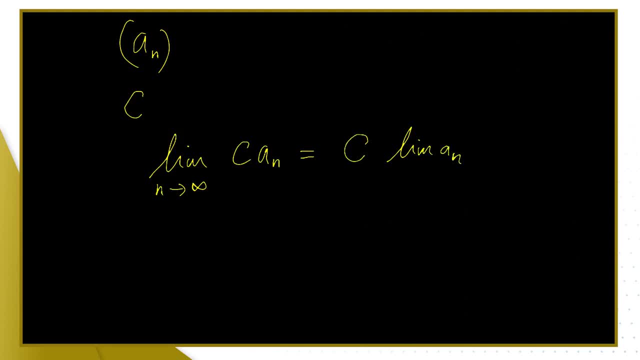 and whatever that is, we multiply by that constant. So that means because we know that 1 over n is convergent, 3 over n is convergent, that is, 1 over n multiplied by 3, and 1 over 4n is also convergent, because the constant there 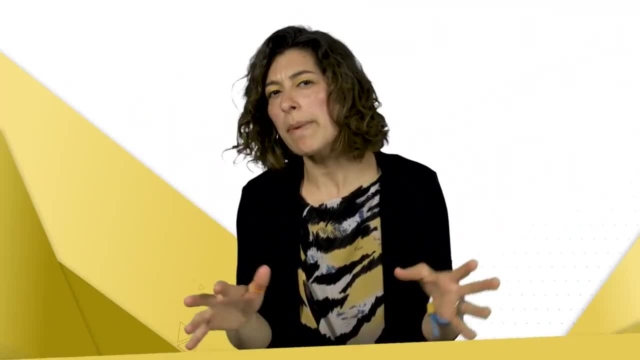 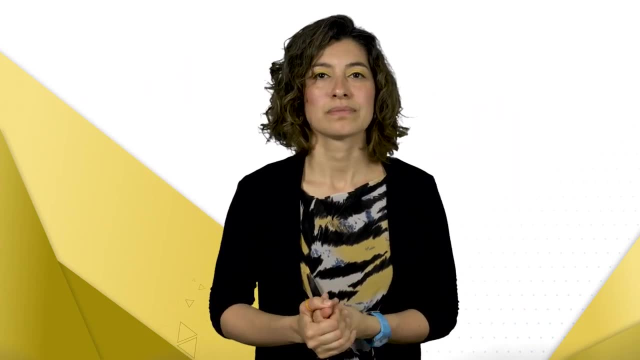 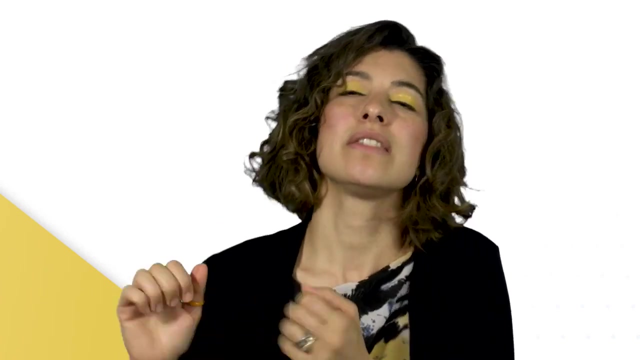 is a quarter and so on. But what about all the other sequences? you know the ones that we can't just use? these two rules Convergent, Convergent, Convergence is all about being bounded and narrowing down the variation of terms as n. 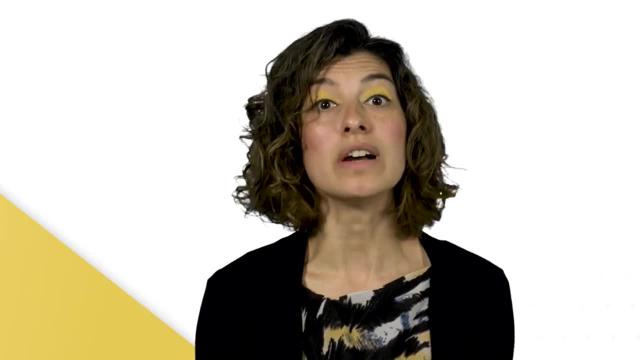 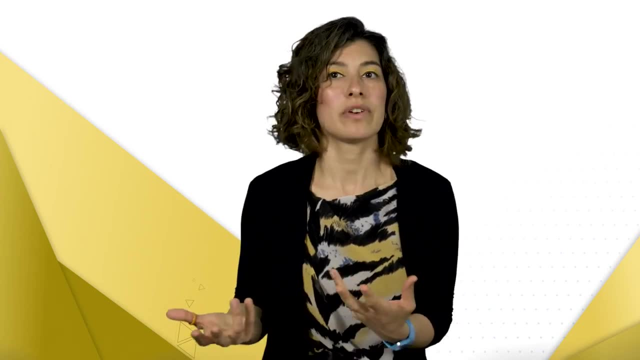 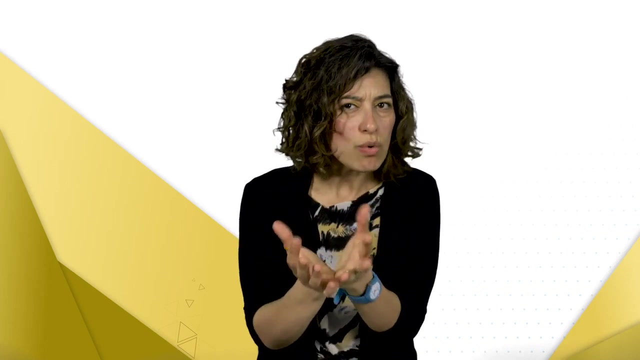 increases. That's my mental picture of convergence. Say, we're looking at 1 over n squared. That is a bit similar to 1 over n And 1 over n is convergent. Now you're probably thinking 1 over n squared is smaller than 1 over n. 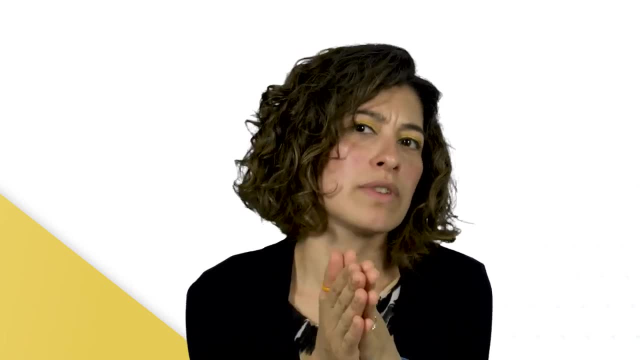 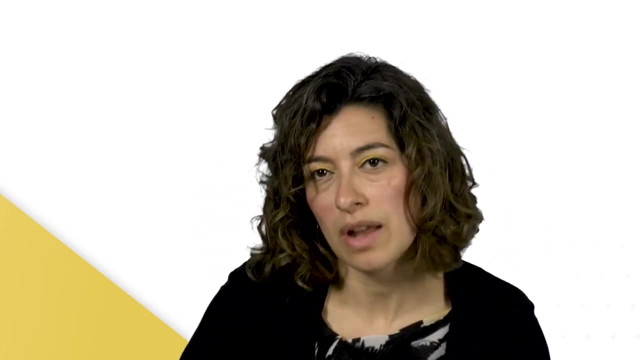 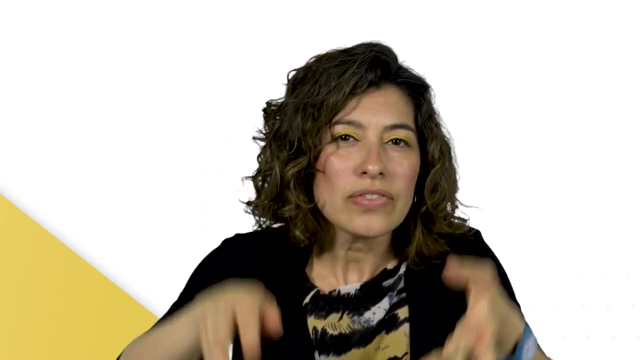 So surely that should guarantee that 1 over n squared is convergent. And you're right If we're talking about magnitudes of the numbers, if we're comparing the magnitude of the numbers in the sequence and the sequence you're working with. 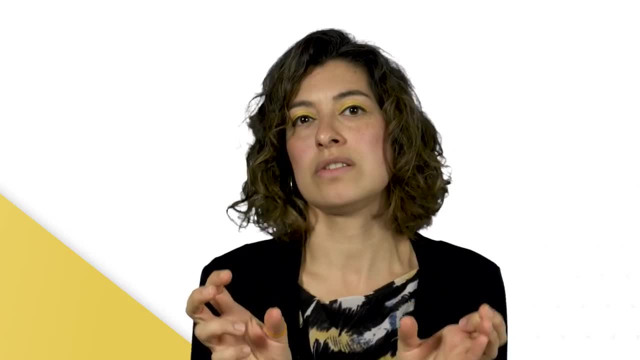 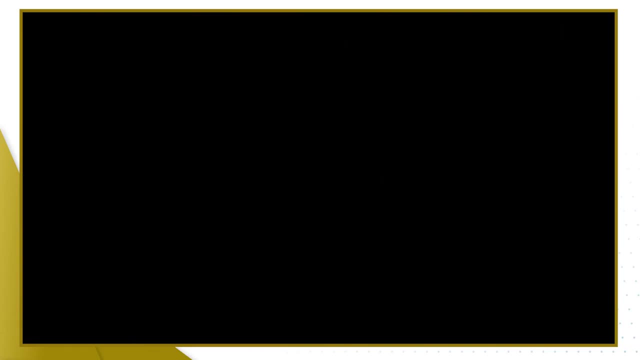 is sandwiched between two sequences that converge, then the one in the middle is also convergent. So what I write there is: if we have a sequence- bn that is convergent and cn that is convergent- and I'm wondering about the convergence of an 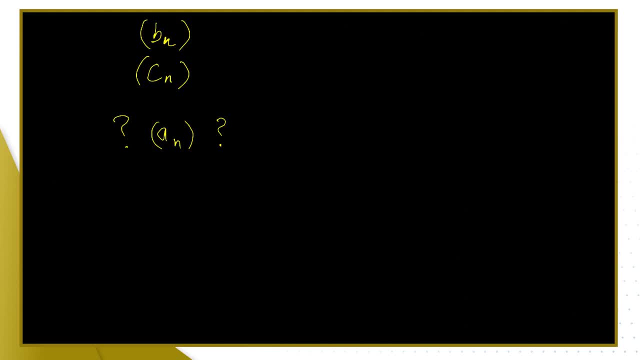 wondering about that. but I realize that actually an is sandwiched between the other two because the other two have limits. these have limits, then that one in the middle is going to have a limit too and the limit is going to be in between. 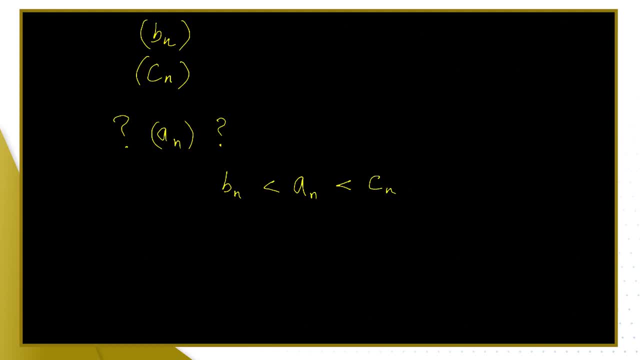 So that means that if this happens for all n, in fact for all n after a certain number, but let's say for all n- then then the limit of a n exists, and the limit of a n is in between the limits of the. 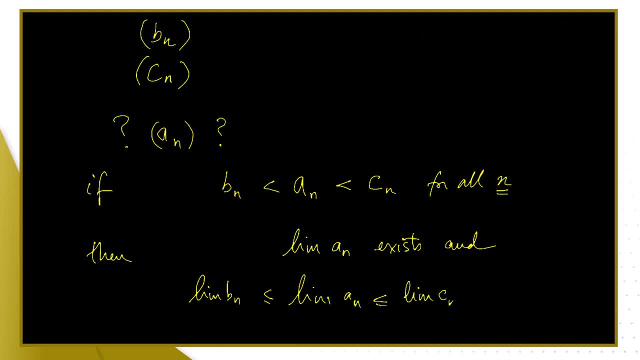 others. And now just notice that I used strict inequalities for the sequences. I used bn less than an, less than cn, but when I came to the limit I wrote less or equal to, because in the limit you can actually have those numbers being equal. 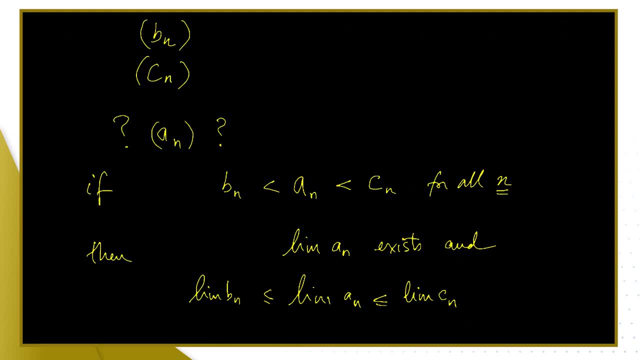 In the same way that 1 over n is never 0, but the limit is 0. So if this exists, So what we take home is that if bn is convergent and cn is convergent and an is a sequence in between those two, then an is also convergent and the limit is in. 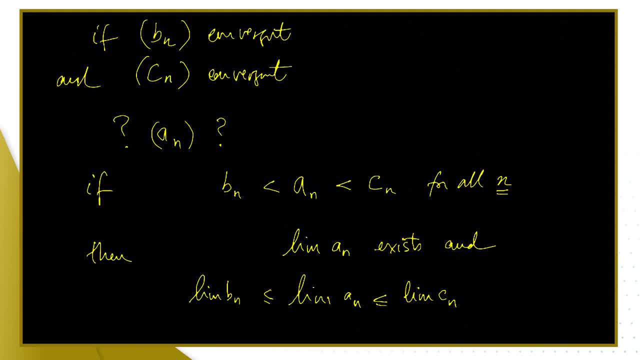 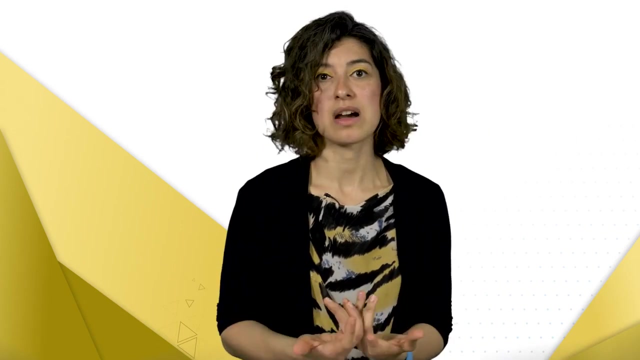 between the limits of the other two. Now, this does not give the limit. This is a rule that doesn't give you the value of the limit, but it guarantees it exists and gives you bounds for the limit of a- n. This is of use as you analyse sequences and functions in practical life. 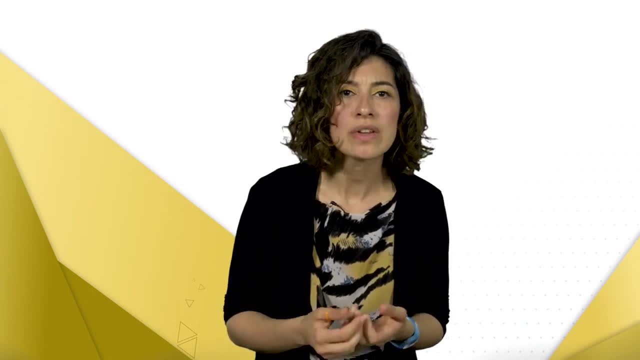 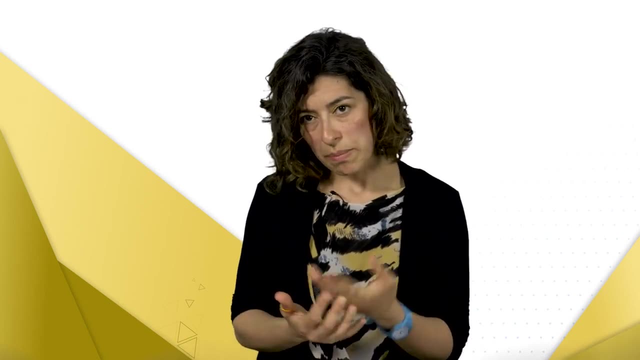 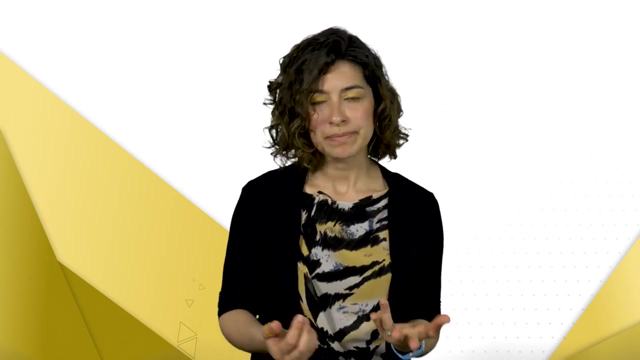 You want to have a sense of convergence and have bounds for limits, but you don't necessarily need the precise value of the limit. So back to my example of 1 over n squared. That is between 0 and 1 over n, So 1 over n squared. 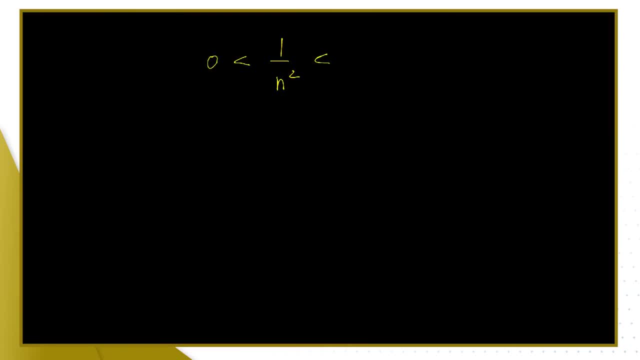 is between 0 and 1 over n. In fact, if you make that n is greater or equal to 2, because we only need it to happen after a certain number- and if your sequences in the beginning are very different and the pattern only happens, 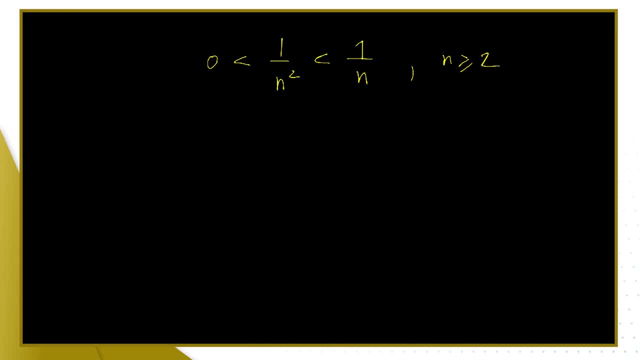 after a while. just take that number for your analysis. So in this case, for n greater or equal to 2, this works. Therefore, the limit of 1 over n squared is going to be in between the limit of 1 over n and the. 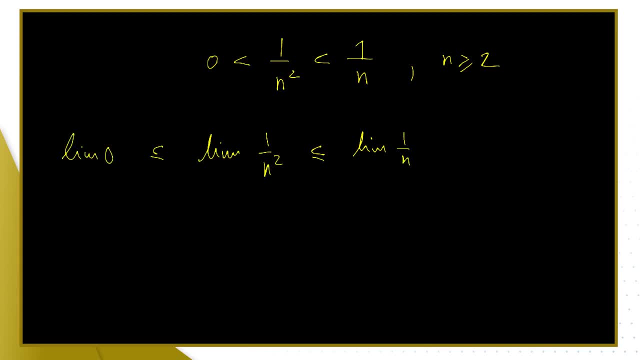 limit of 0.. Now, this is quite a nice one, because the limit of 1 over n is 0 and the limit of 0 is 0, so therefore the limit of 1 over n squared has to be 0 as well. So that part is 0, that part is 0, and therefore the limit of 1 over n. 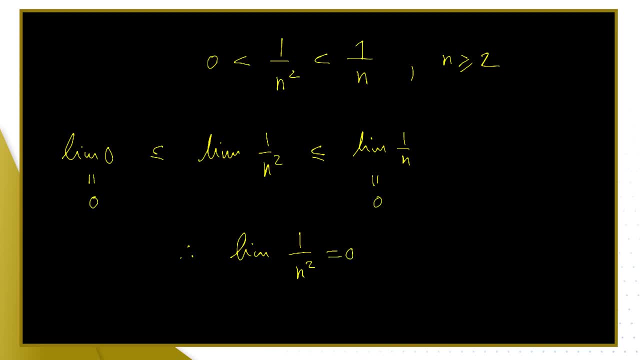 squared is 0 as well. Again, we cannot guarantee strict inequalities in the limit, since a limit can be smaller than all the terms of a sequence, or larger than all the terms of the sequence. Now for series. we can use comparison too, But let's recap what we. 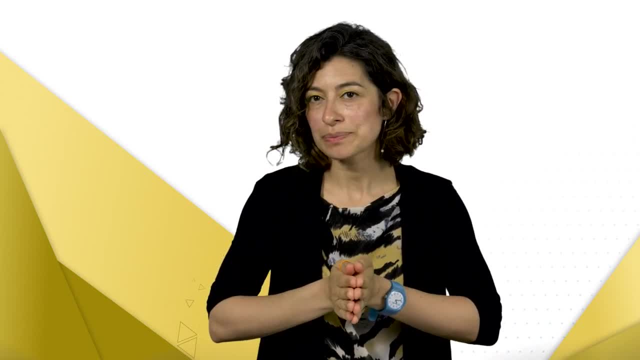 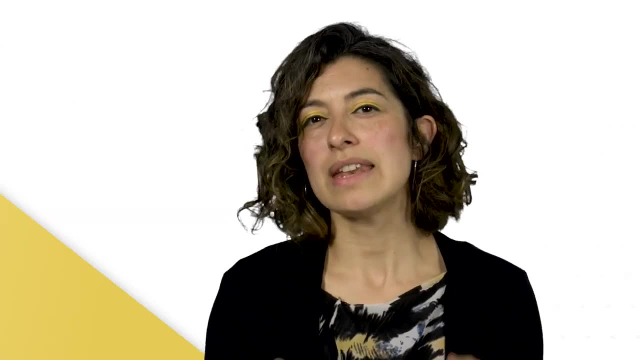 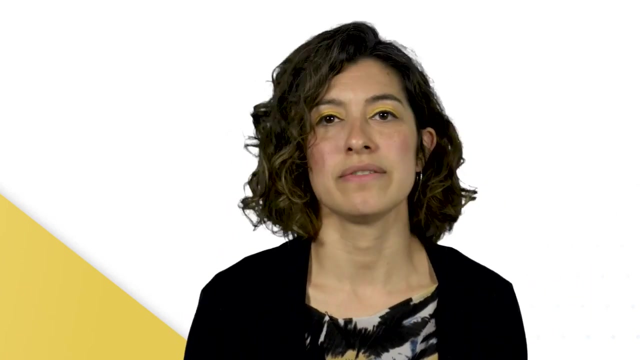 said about the sequences we're adding up in a series. If we're looking at a series that is a summation of a? n, we said that if a- n is not convergent or the limit is not 0, then the series cannot converge. This gives a necessary condition for convergence. that is not a. 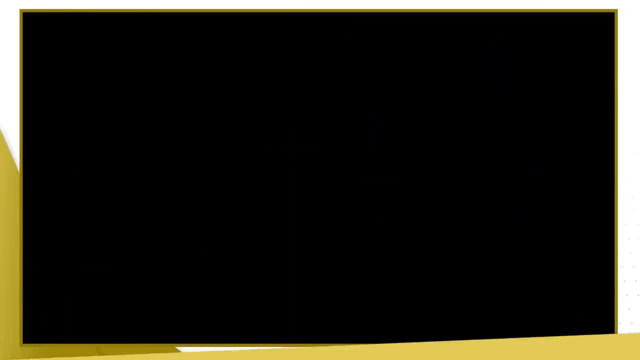 sufficient condition. So what I said was that when we're looking at a series- a, n- and this is implied that the limit is from a number 1 to infinity- in fact I can put here any finite number- the necessary condition for convergence is: 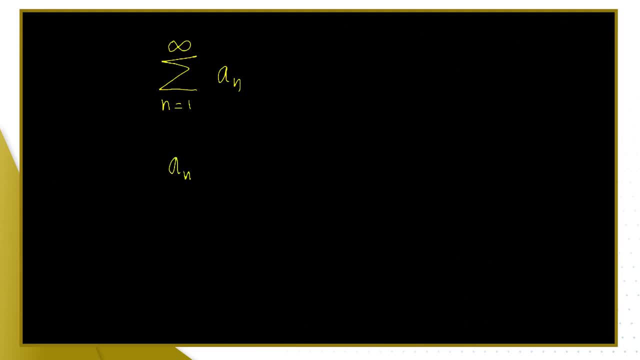 that a, n converges and the limit exists and it is 0. So this limit existing is a necessary condition for the sum to converge. converge. that is not sufficient. Now that means it will be handy to have some sufficient conditions. It will be handy to have some tests that could guarantee convergence. Now 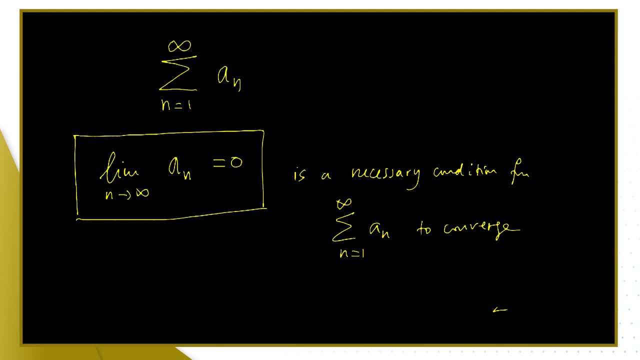 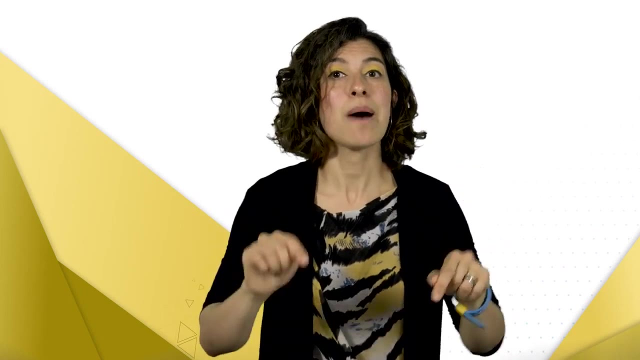 there's some good news. If the sequence is almost a geometric progression with ratio r that is between minus 1 and 1, then the series converges. Unfortunately, I don't have a formula for you, because we saw a formula for the sum of the geometric progression with. 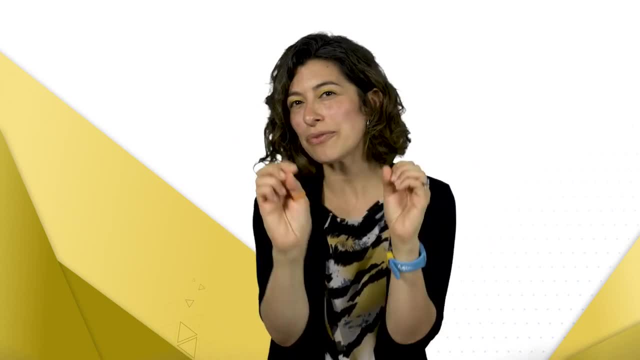 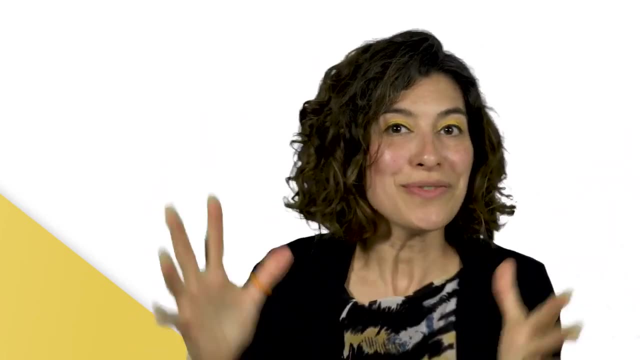 ratio r between minus 1 and 1, we saw that formula, but if the sequence is almost like that, we still guarantee convergence. OK, so the series I'm wondering about is the sum of a- n. OK, so the series I'm wondering about is the sum of a- n. 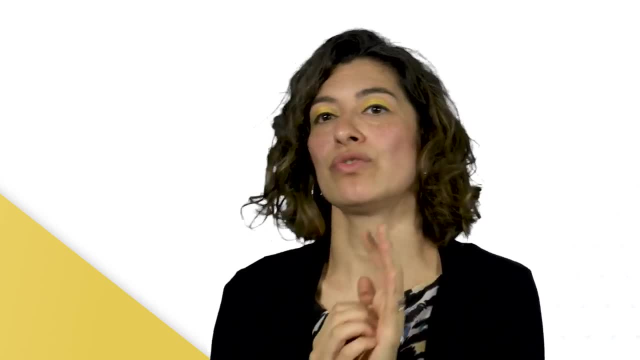 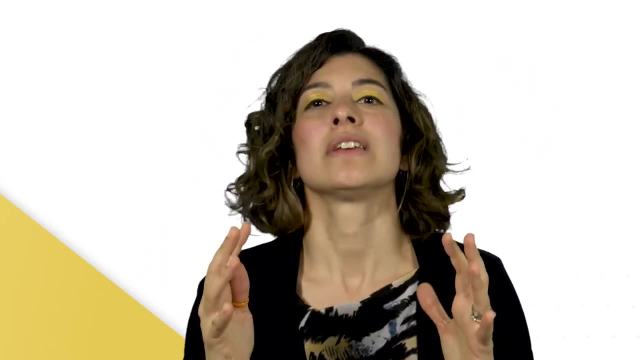 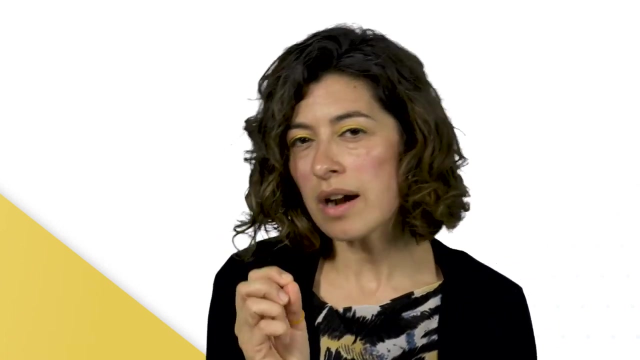 OK, so the series I'm wondering about is the sum of a- n. If we take the magnitude of a n plus 1 divided by a n, and the absolute value of this ratio in the limit gives a value r, then if r is between 0 and 1, then the sum converges. So 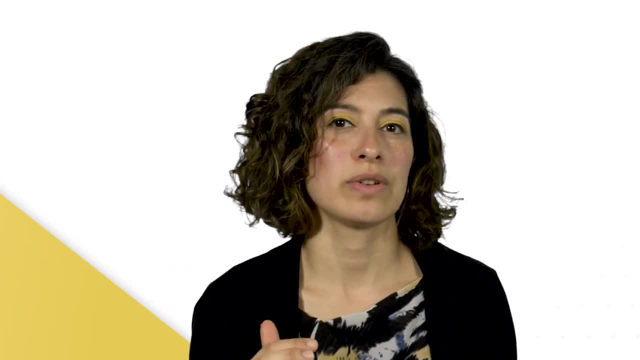 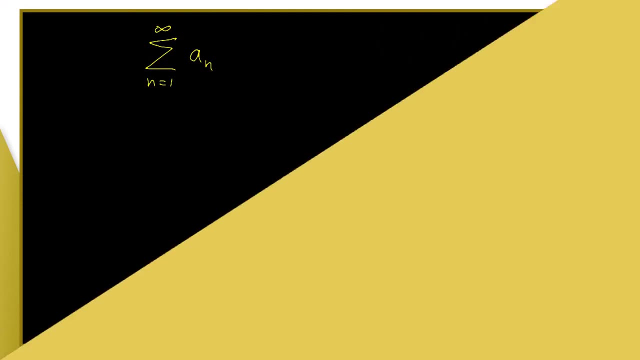 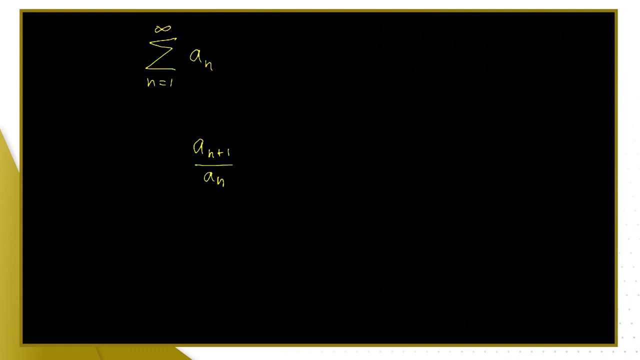 basically, we're saying: if this looks very much like a geometric progression, then the sum converges. if the ratio is a contradiction, If there's negative points to the value of r and we have negative points, then the sum converges、. we don't want a tiller either. we don't want a tipping. 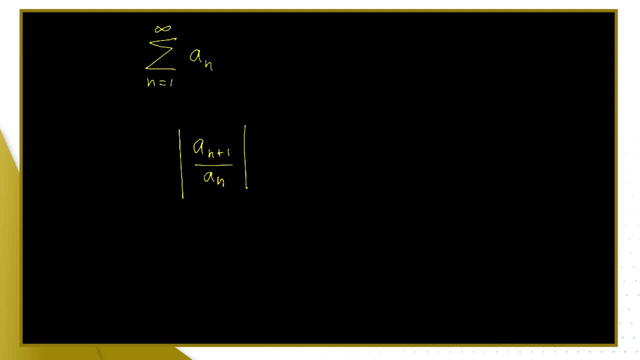 We want a наконецrocket. So this image again: yaş bidder. That means I write an plus 1 over an, and it's the magnitude of this number that I want. So I want the absolute value, which is usually denoted with two bars around it. So that means: 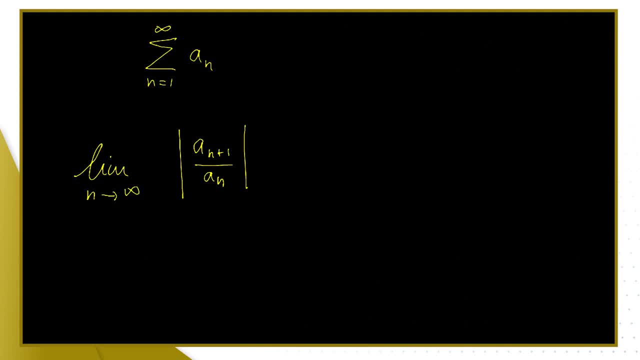 If this in the limit is an r and that value is going to have to be 0 or more, if that limit is r and r is between 0 and 1, but not 1, then the series converges. We don't know the value, but we know it converges. Now, if r is greater than 1, it will diverge. 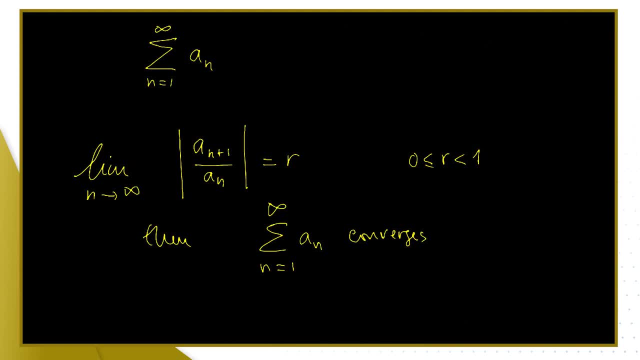 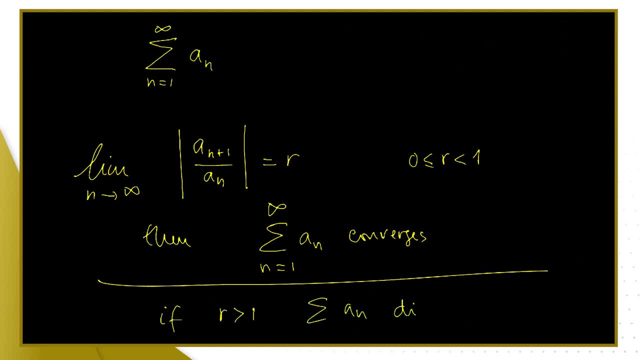 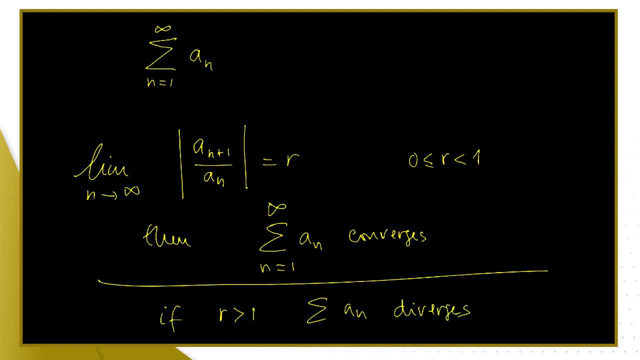 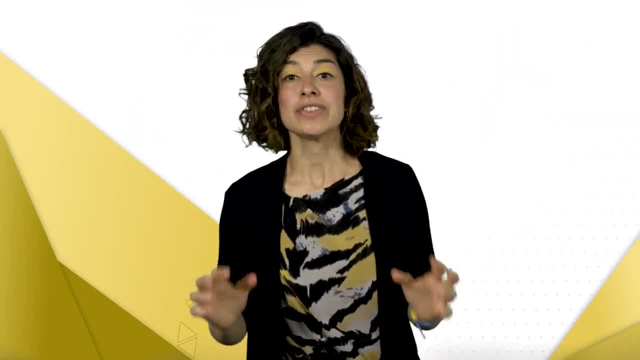 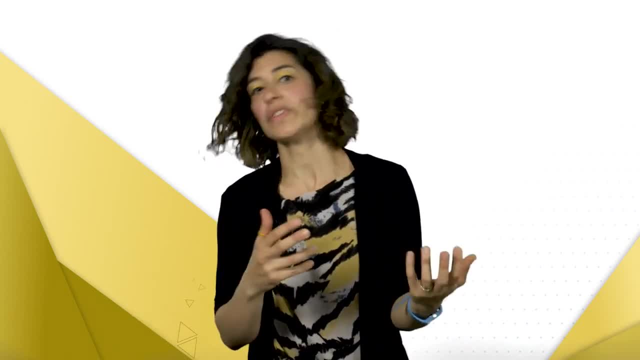 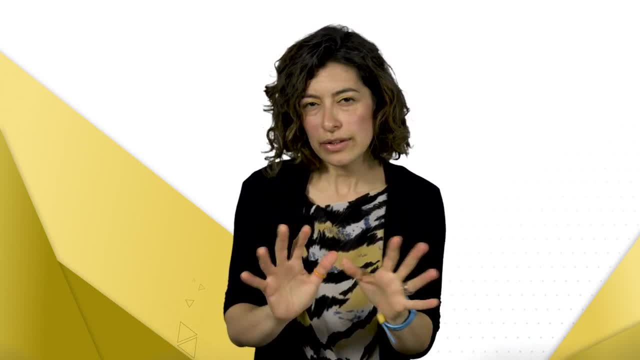 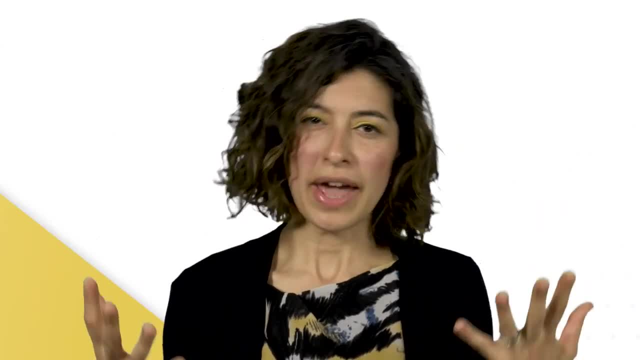 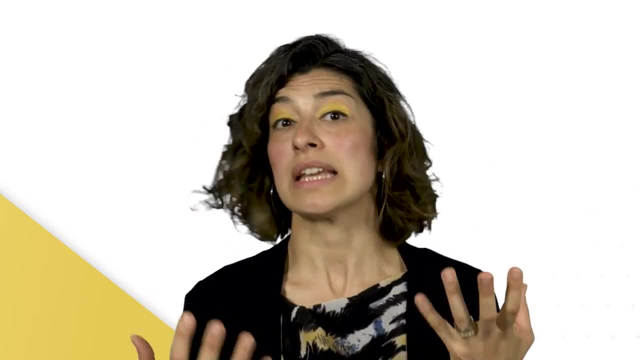 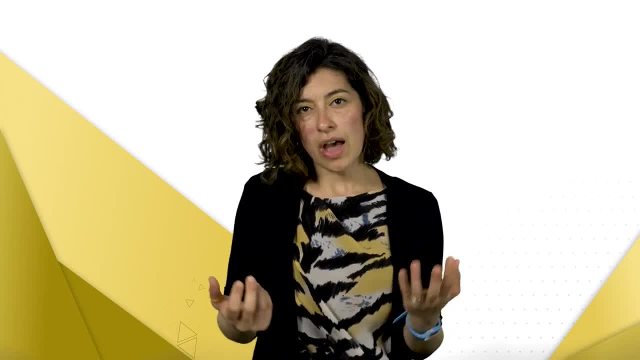 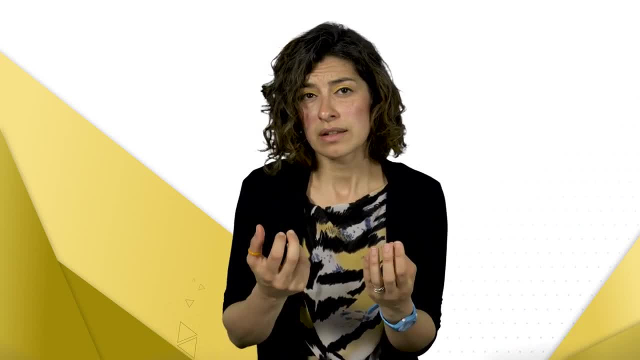 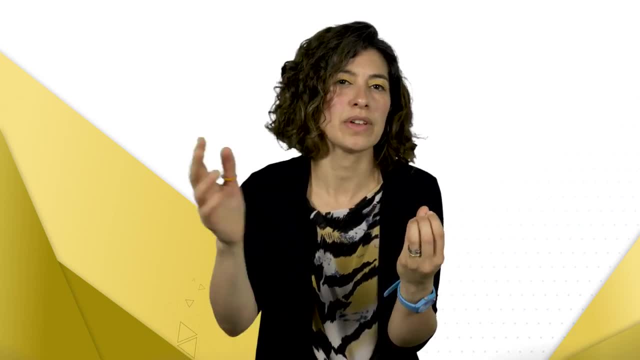 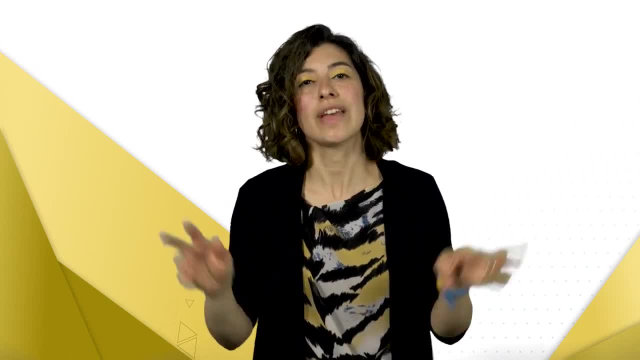 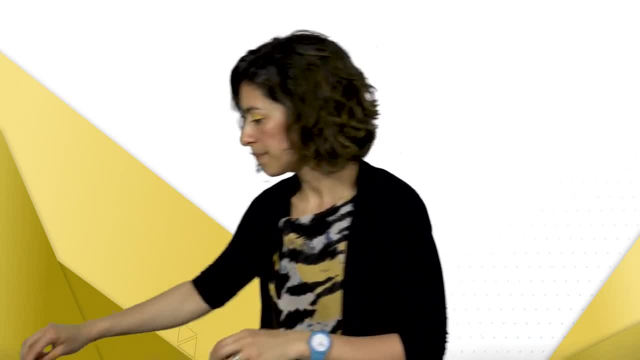 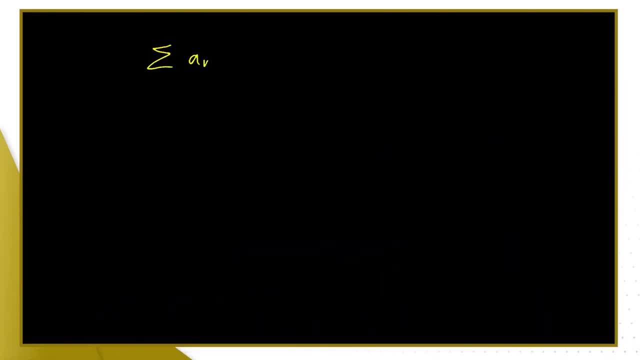 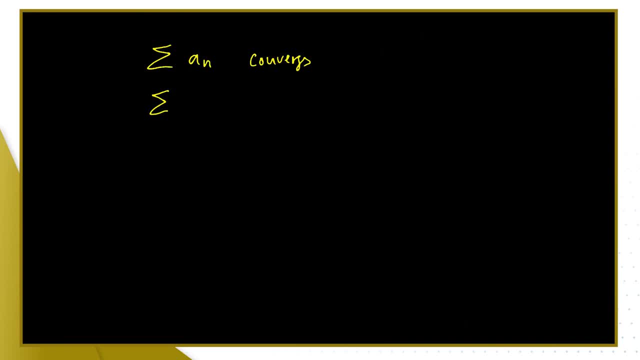 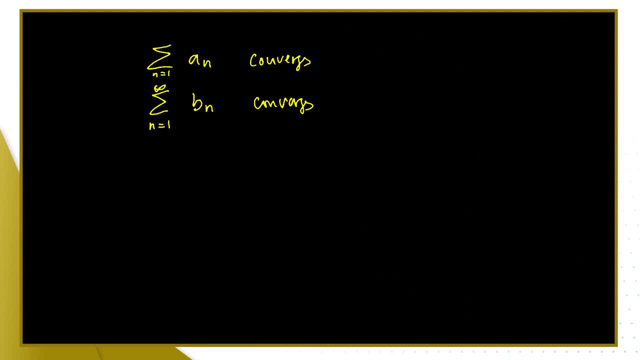 the values here, and if we have that the terms of the sequence C? n are sandwiched between the terms of the other sequences, then the sum of the series is also gonna be convergent. Then the sum of C? n will be convergent, Convergent. 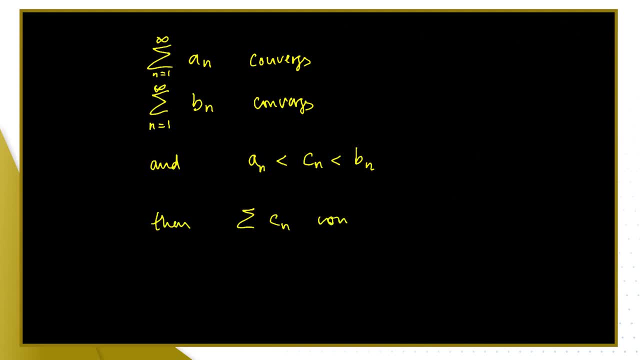 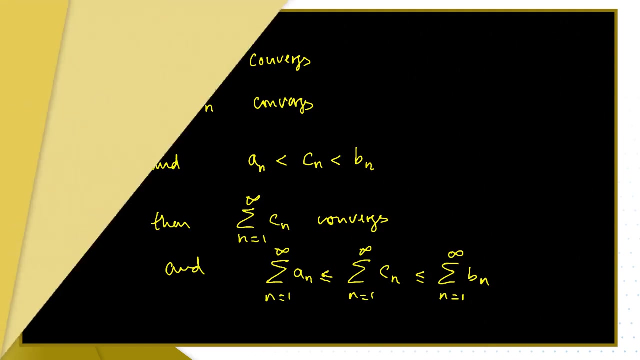 Convergent converges and we have bounds for that value. And again, I use less or equal to in the limit, even if I have a strict inequality between the sequence terms. There are more criteria that have been studied and proved and you will be able to use them in your professional life. I encourage. 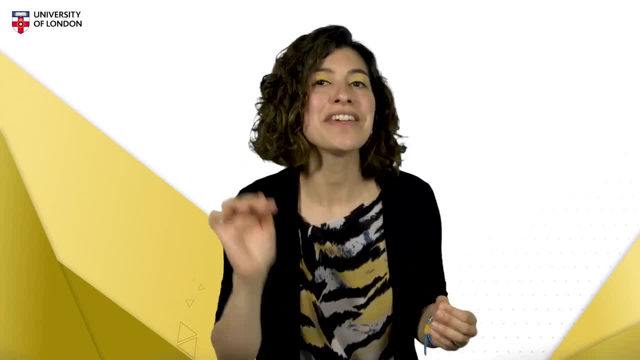 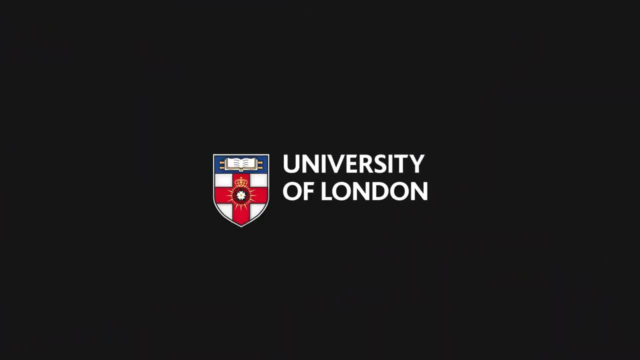 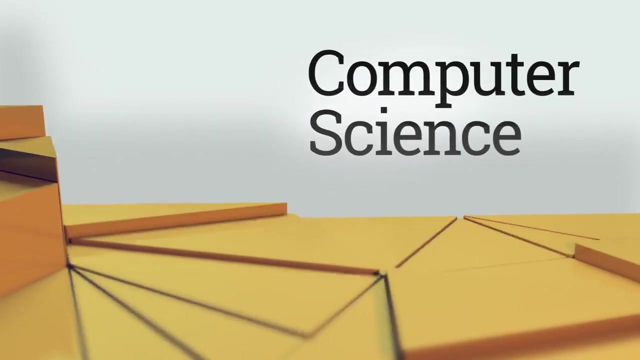 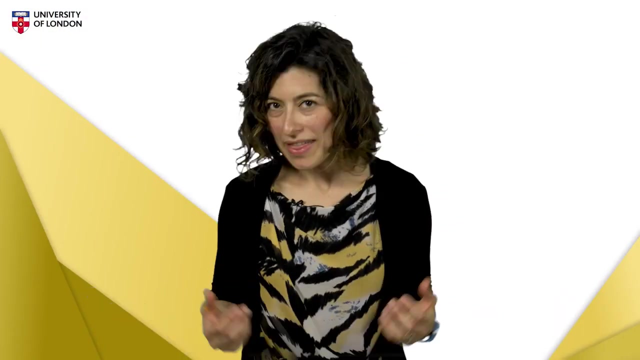 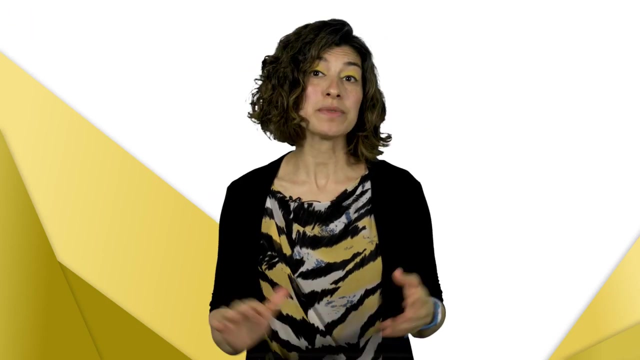 you to go and learn about those, but be aware that any other criteria not stated here is outside the scope of this module. Sex off limits. In this lesson we looked at the behavior of infinite sequences and infinite series. We introduced the concept of Limit, calculated limits of sequences and 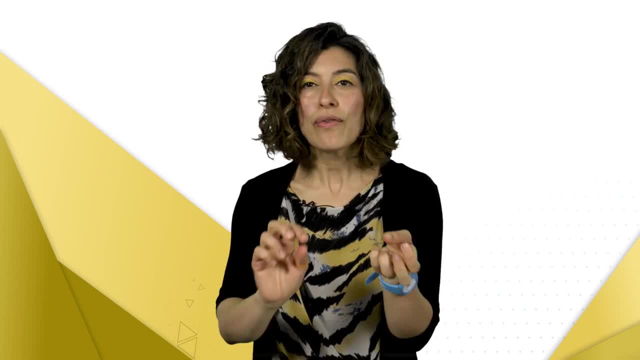 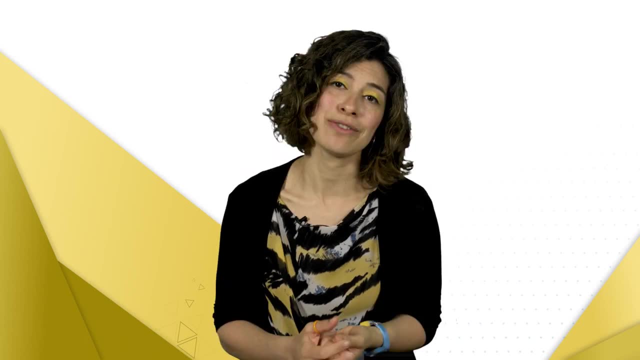 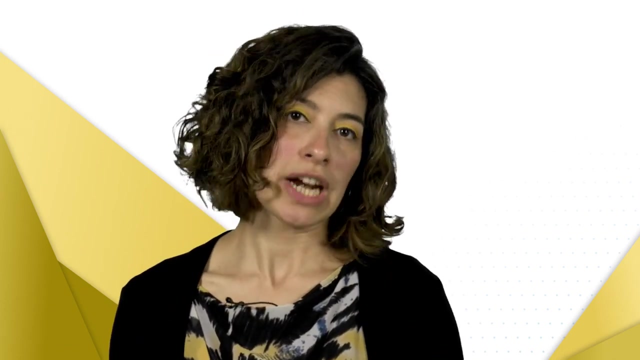 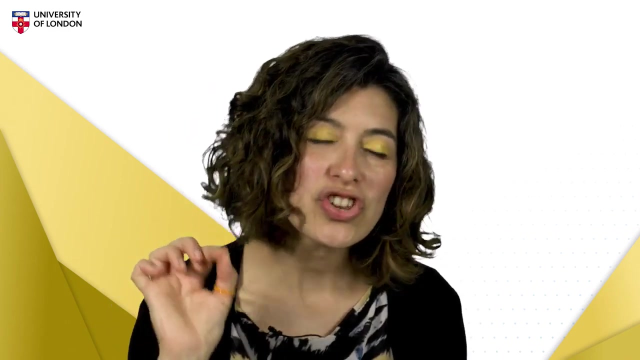 series. In particular, we saw formulae for limits of geometric sequences and series for when the Ratio is a shrinking ratio, meaning that it is between minus 1 and 1.. We formalized our intuition and gave criteria to decide if a sequence or a series are convergent, by inspecting the general term or comparing. 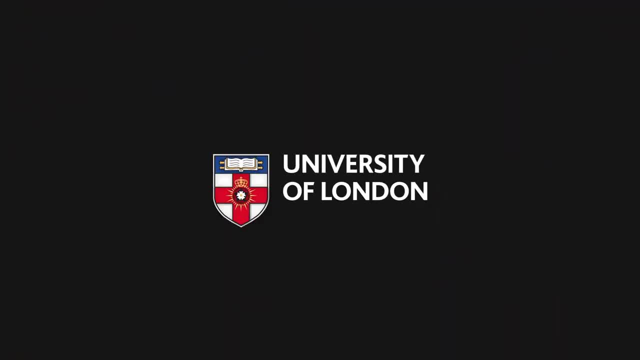 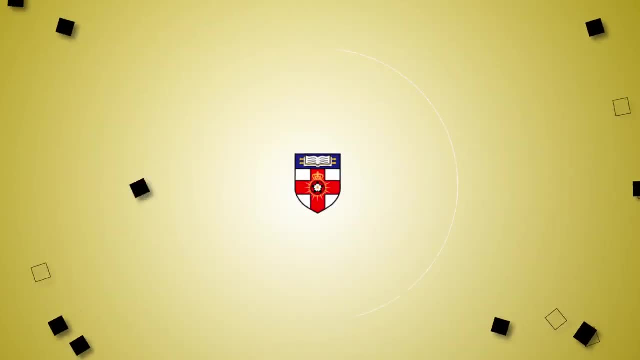 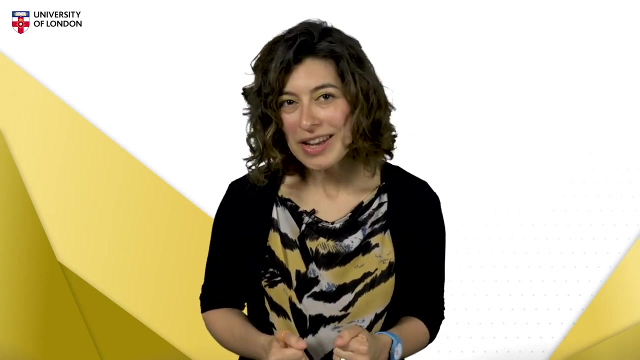 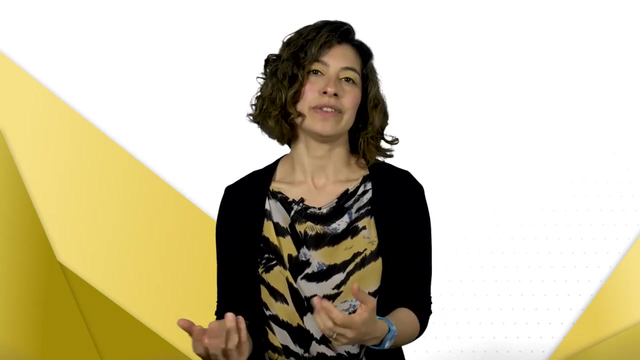 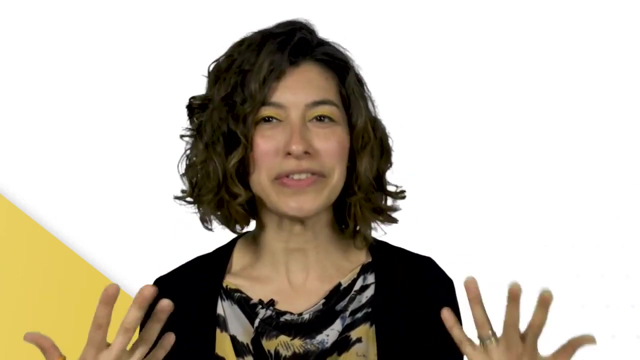 it to others In this topic. you've been on a journey through ordered lists of numbers and their sums. These are called sequences and series respectively. Our emphasis is on you using critical thinking when dealing with sequences and series you've been working on. 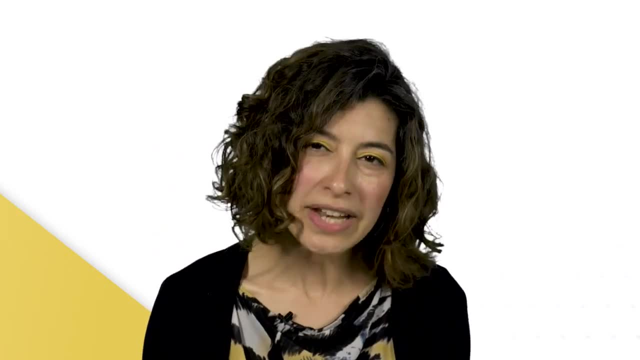 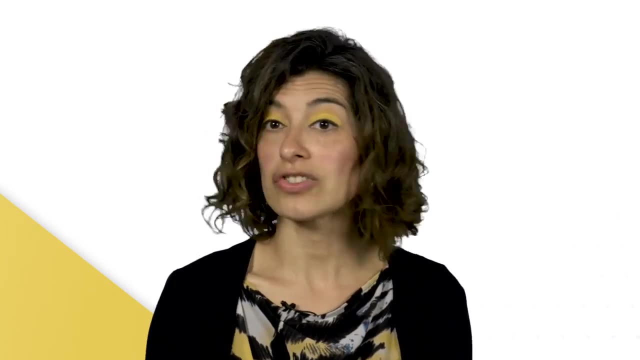 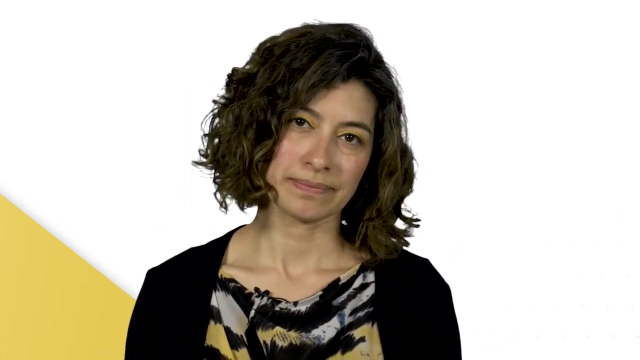 So we got you to make sense of patterns and then see the need to formalize such patterns in a precise definition, such as the general term of the sequence, basically an expression or formula or a recurrence relation. The main difference between these two ways of defining a sequence is that the recurrence 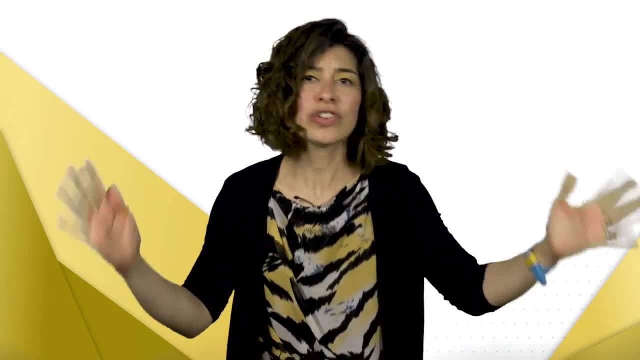 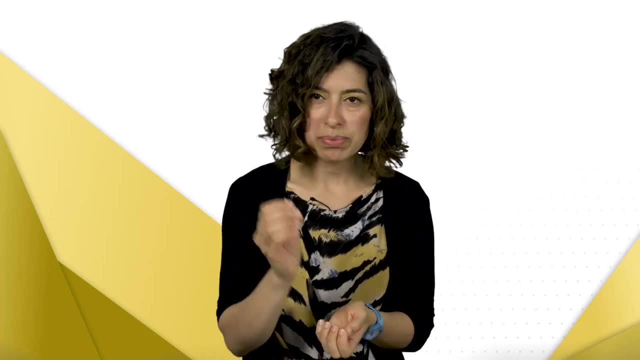 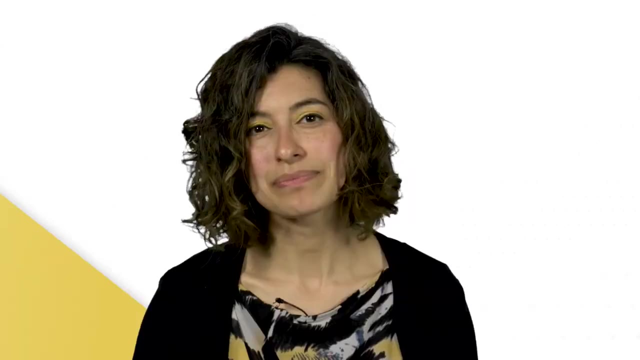 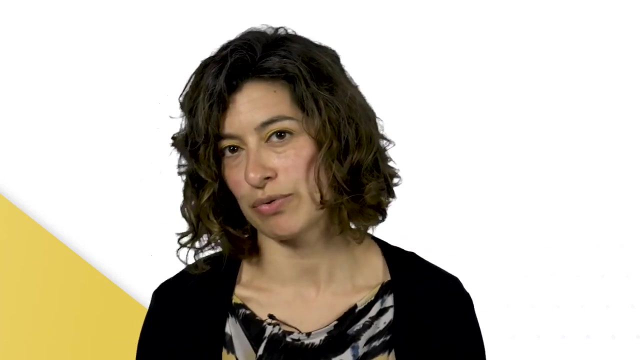 relation requires you to calculate all terms before the term you are interested in, Whereas the general term allows you to just replace the index variable by the value you want to get the term you need. We looked at two special families of sequences: arithmetic progressions and geometric progressions. 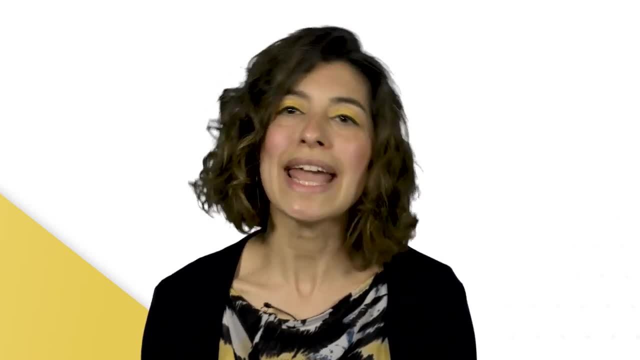 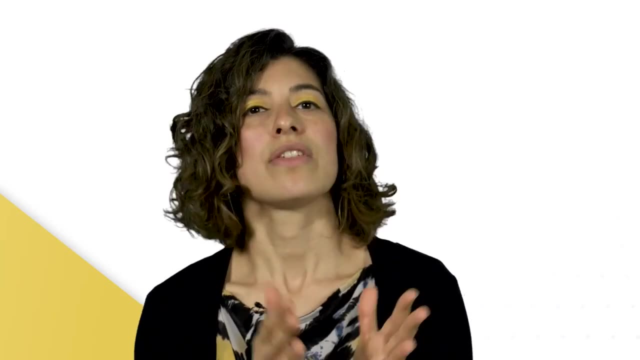 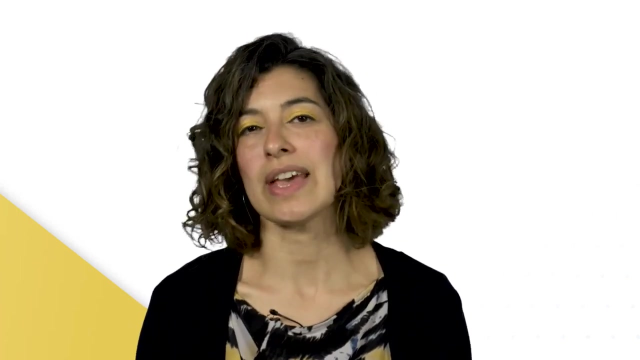 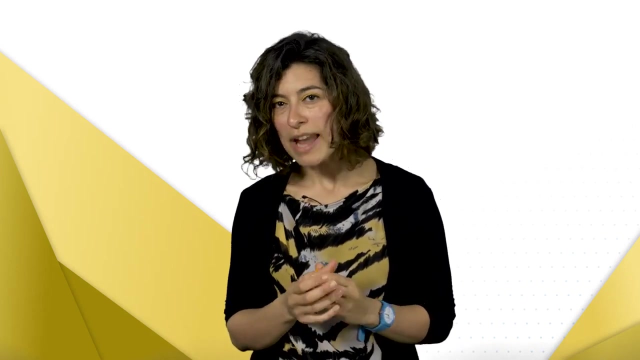 The first consists of sequences where any two consecutive terms differ of the same value. The second the regular term. the ratio between two consecutive values is the same. We also looked at limits and said: when a sequence converges, We saw that arithmetic progressions do not converge, but geometric can if it's a scaling. 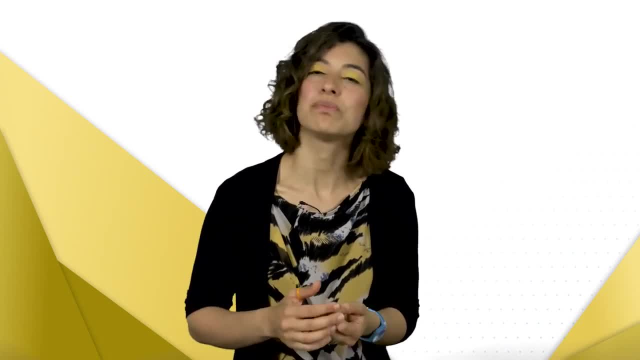 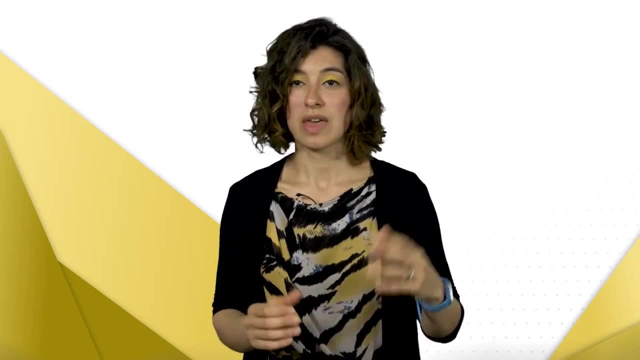 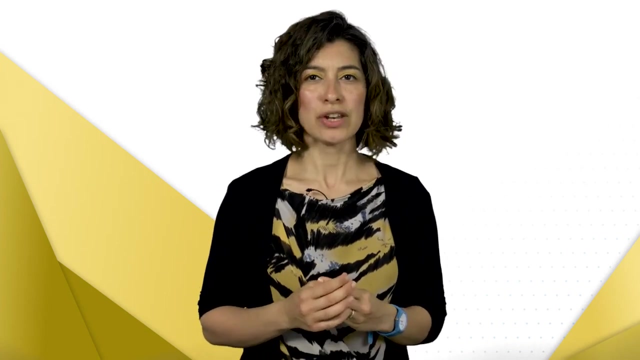 down progression, meaning that the common ratio is between minus one and one. We then looked at adding up consecutive terms of a sequence. These sums are called series. We have formulae for such sums for arithmetic and geometric progressions for a finite number. 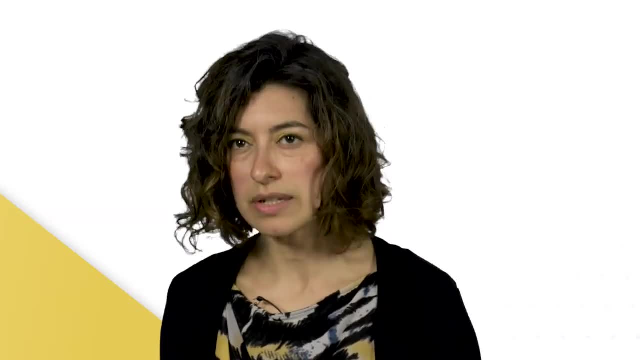 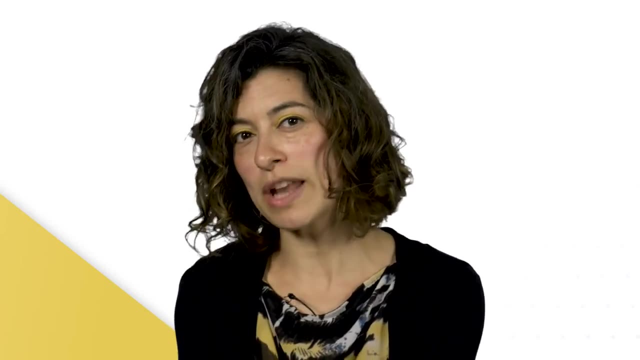 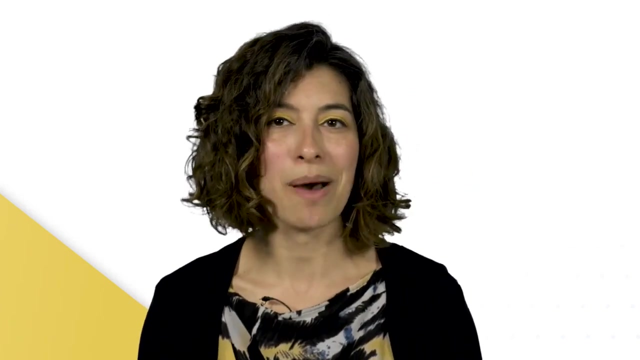 of terms. Now, taking series to the limit, these sums do not often converge. We saw criteria for convergence and, in the case of geometric progressions of ratio r between minus one and one, we have an explicit formula for the sum of all terms. 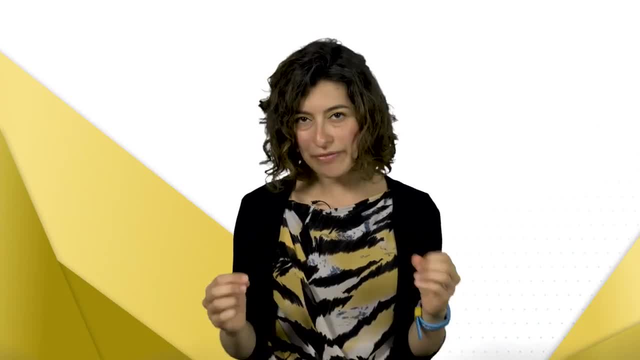 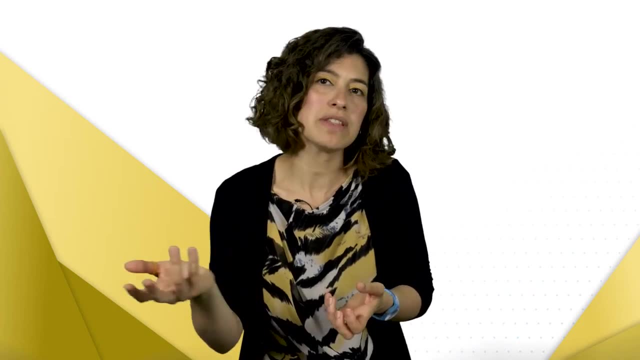 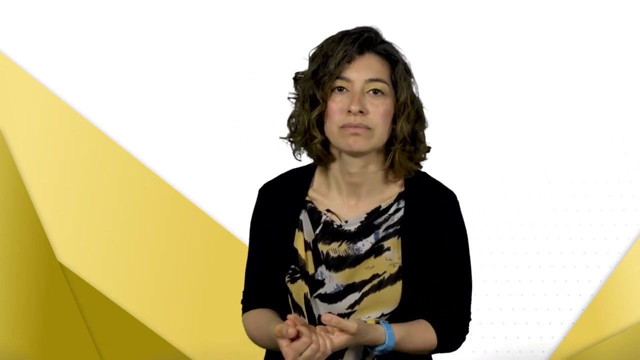 To understand where this all fits with computing, have a go at adding up numbers in a loop and looking at numbers of comparisons an algorithm requires to perform and the performance of different algorithms that solve the same problem. Or design computer graphics where you need to access resolution limits of how much of. 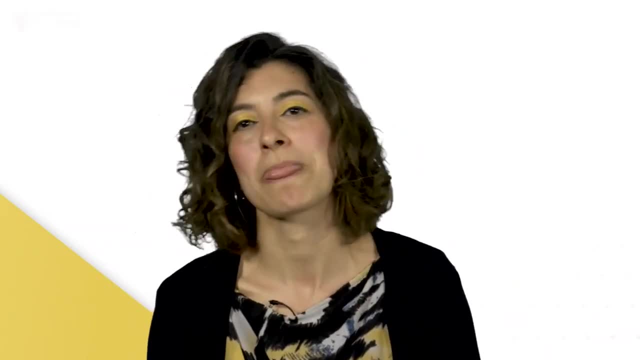 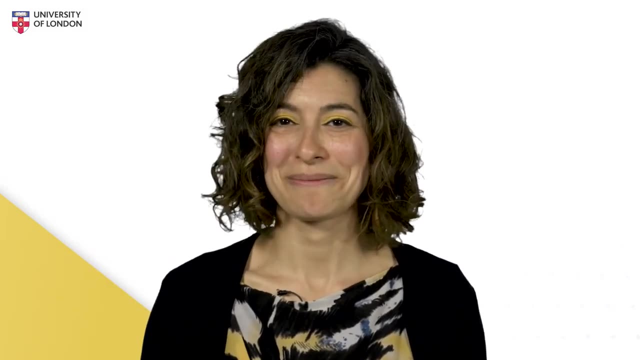 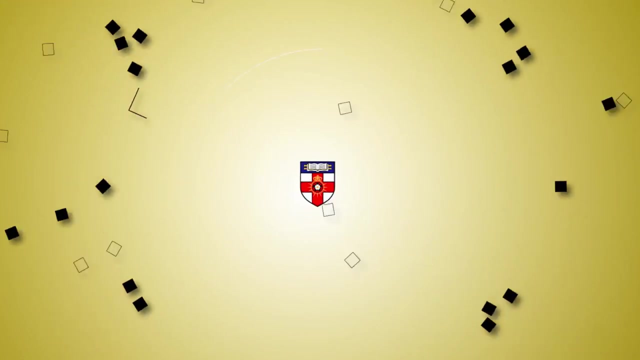 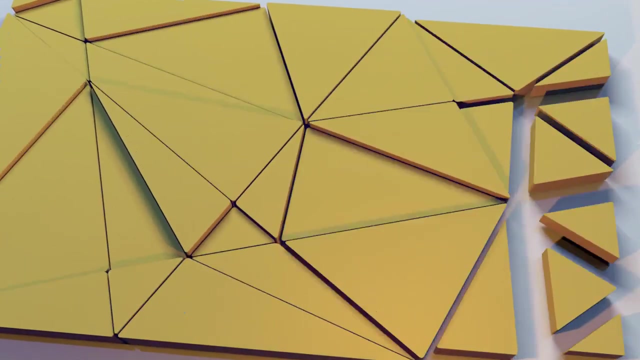 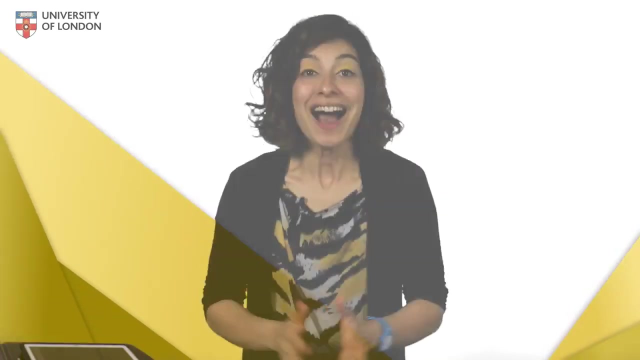 your design shows up when we zoom in and out of the image. This is outside of the scope of the module, But part of the professional development of a computer scientist. I love maths. Look, I love maths. 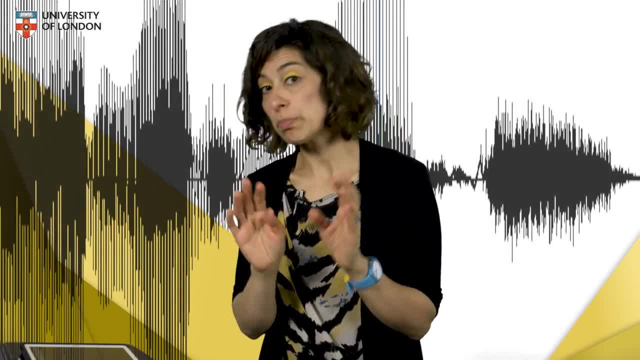 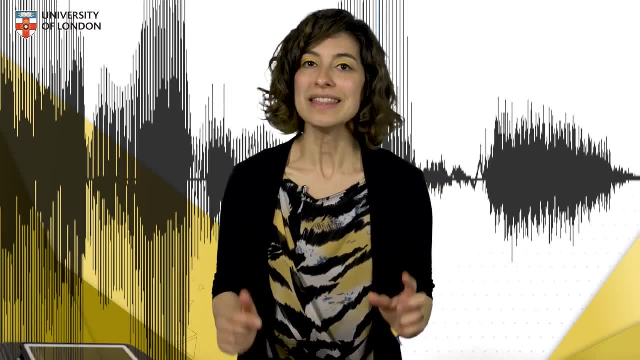 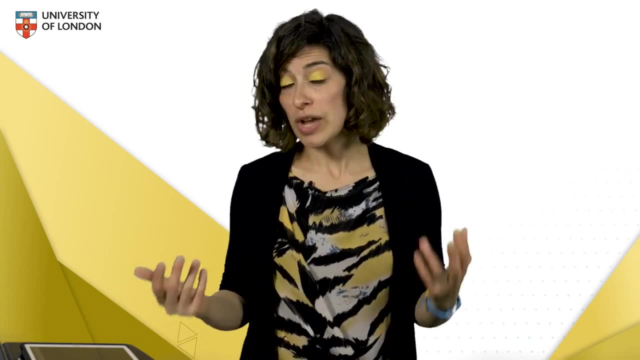 Let's take a look at some examples. How is this done? The sound waves were plotted as a graph. We have sound as function of time. In this topic, we will have look at tools required to represent information as images, From designing a computer game to creating digital art or simply understanding how images 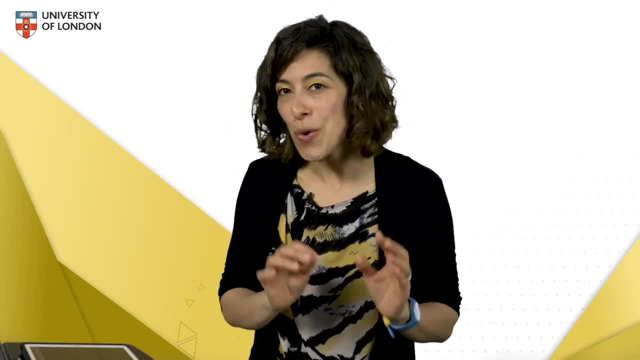 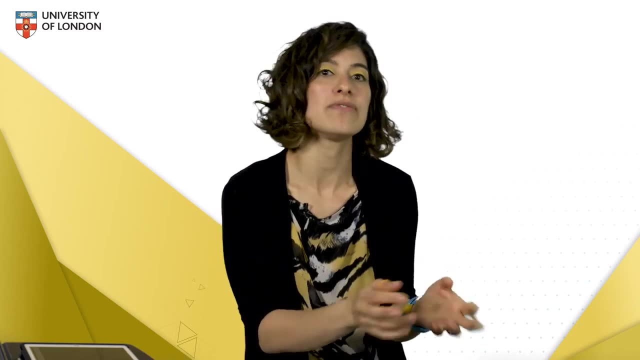 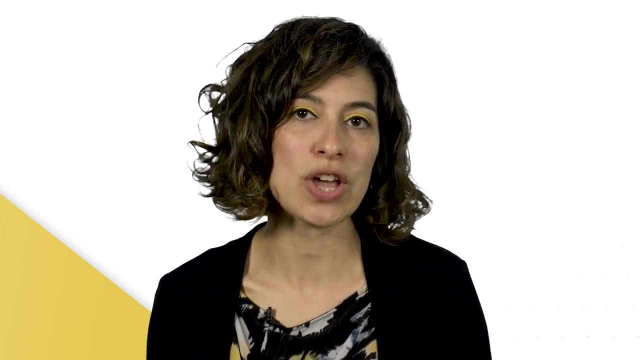 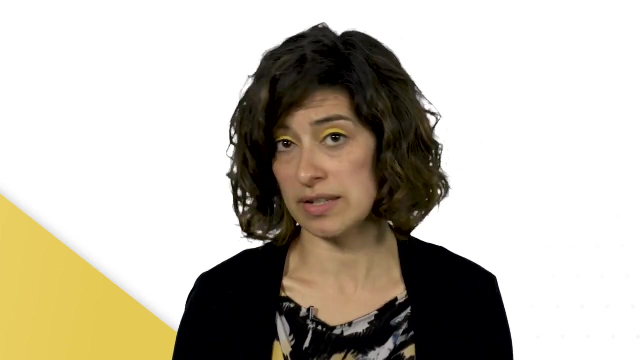 fit on screens. we used the basic knowledge of coordinates to represent functions, as a graph encodes the variation and behavior of that function. We will illustrate one application in modeling motion in the kinematic equations for simple straight-line motion with constant acceleration, also known as Suvat. 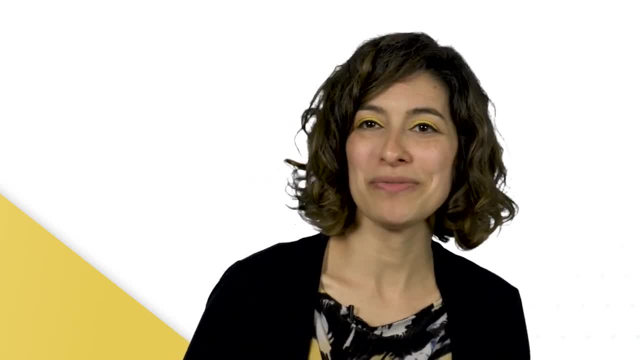 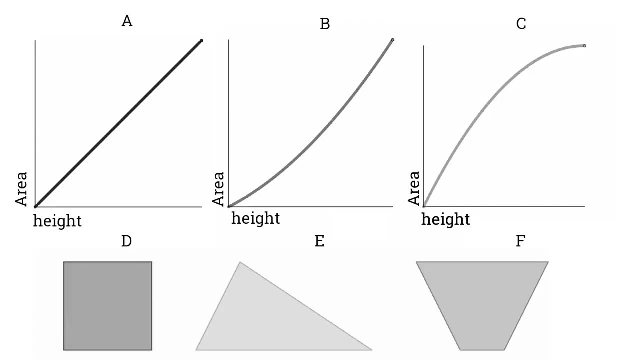 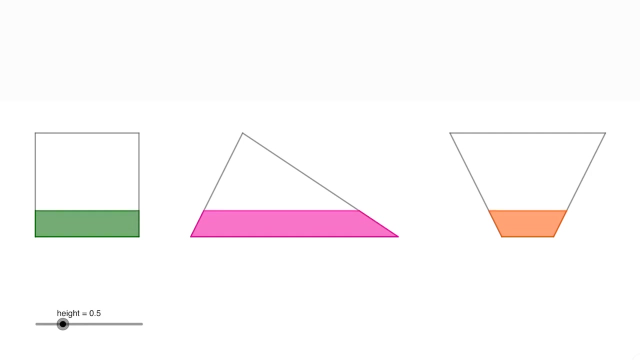 equations Handy if you want to design a simple video game throwing balls in the air, or simple race cars colliding. Here are some examples: We have volumes of containers plotted against height as you fill them up. Which graph corresponds to which container? You can answer in the in-video quiz. 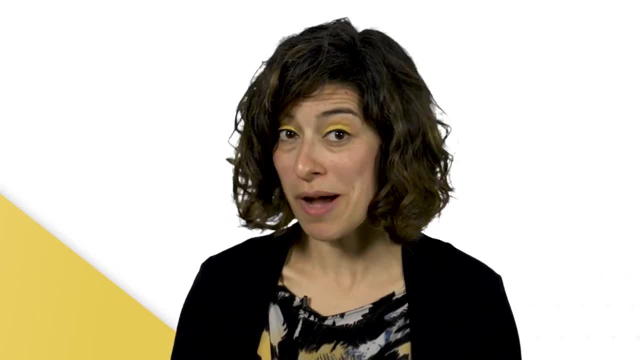 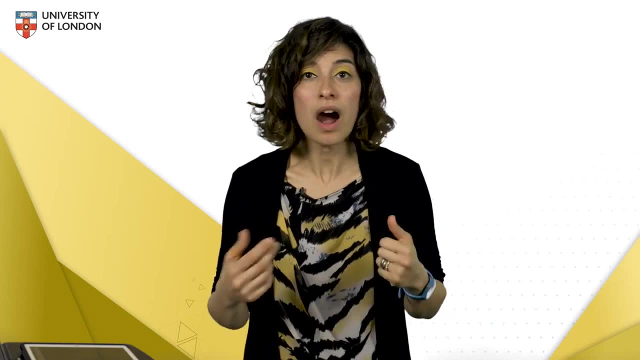 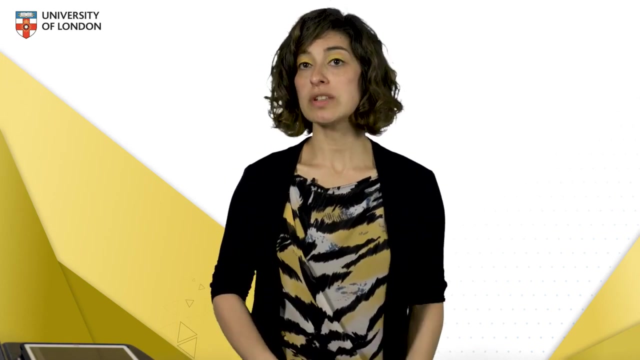 Now then, how hard was it for you to match them up? It probably varies on how familiar you are with analyzing these things. Some containers are harder to figure out and need closer study. Experiment with the information you have, Experiments run, data collected and graphs plotted. rigorously, Of course. 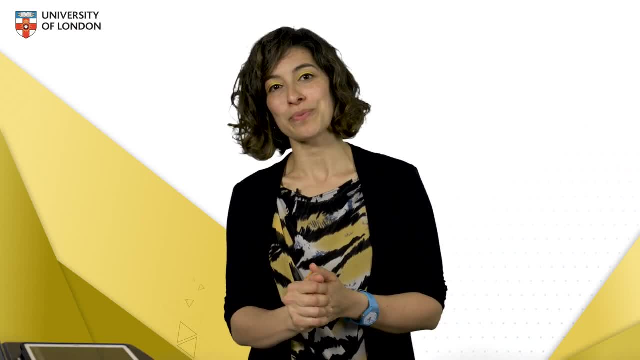 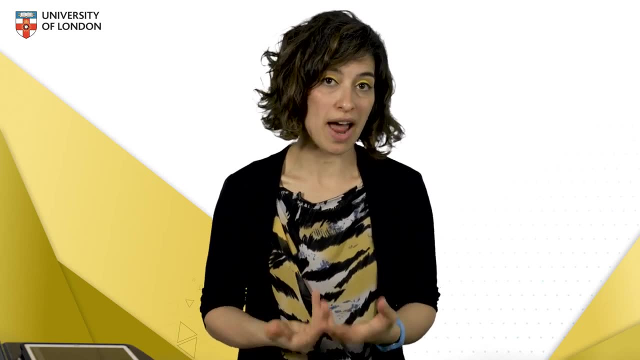 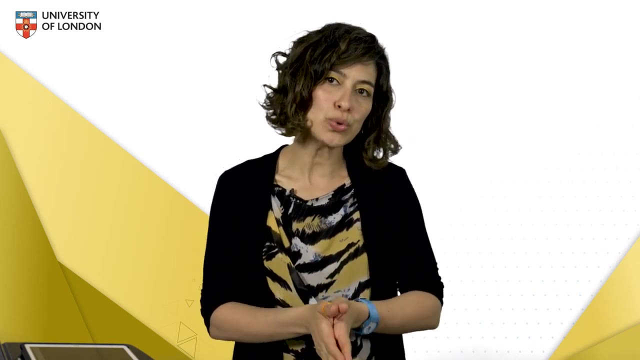 computers and some calculators can plot graphs for you. In this module, we are focusing on the thinking skills of deciding how to plot a graph, how to represent it, how to interpret it. We will use a digital graph plotting tool to gain intuition on how functions work and to get to know types of 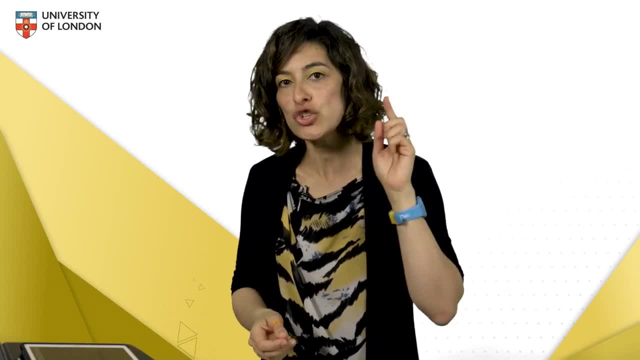 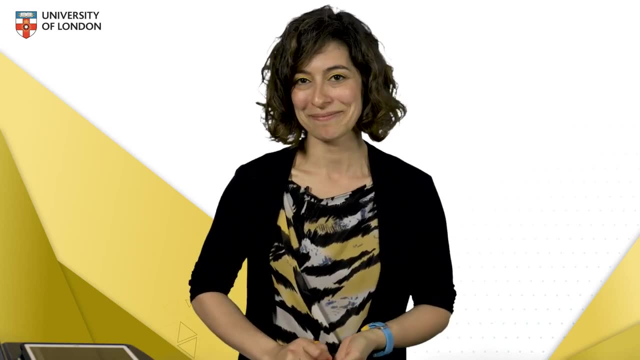 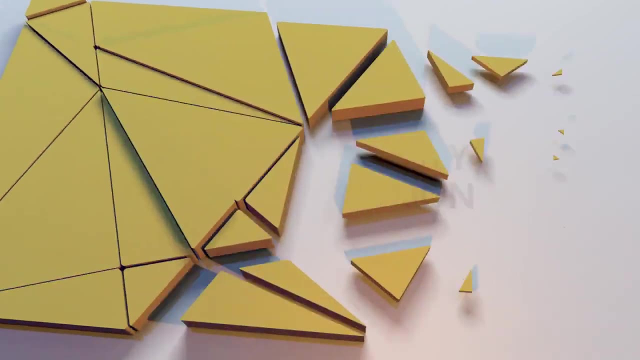 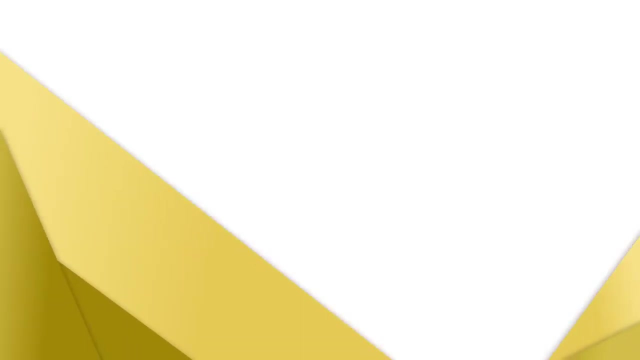 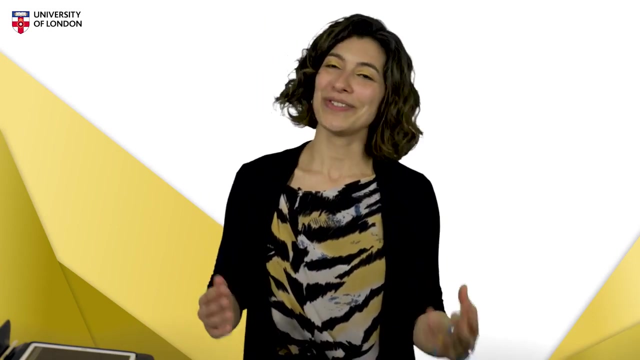 graphs without having to plot everything by hand, But you will be asked to submit hand-drawn graphs, so get your graph paper and geometry set ready. Where are you? The answer being two numbers, Your coordinates, whatever system you want to use: latitude, longitude- two numbers that describe your position on the planet. 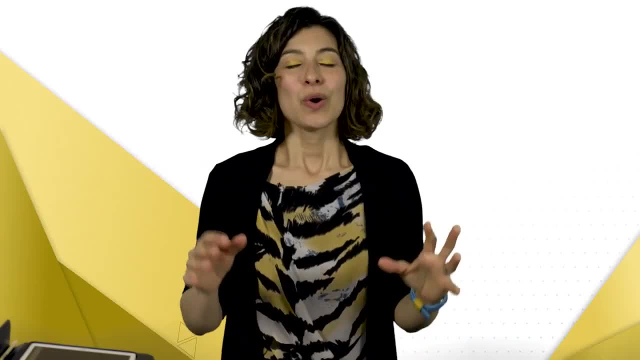 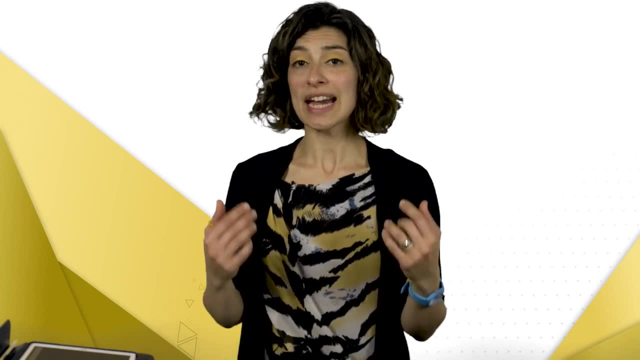 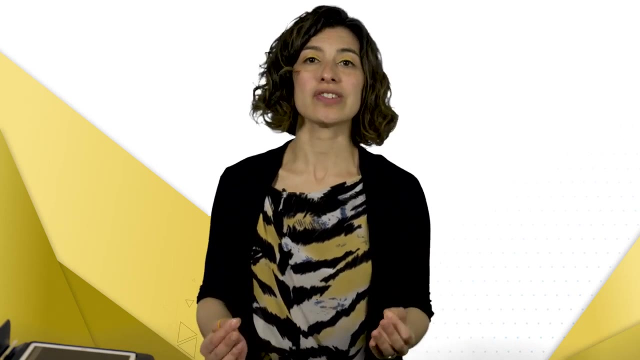 Well, three, if you want to tell me how far up you are. We're going to look at functions and graphs, and for that we need to be able to represent points in the plane. We're going to use Cartesian coordinates, and that just means we're going to have two numbers to give me the precise location of a point in a plane. 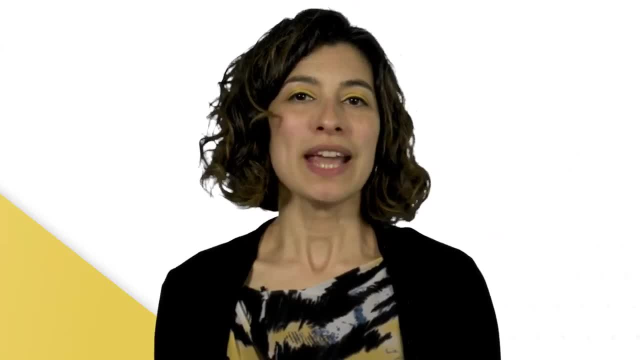 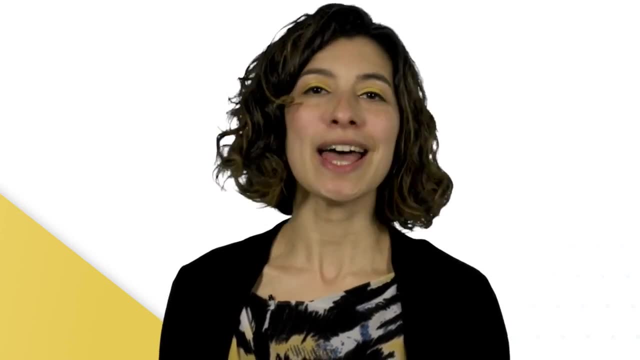 In, say, an infinite piece of paper To make those instructions precise. we need a reference. We need a reference point that's going to be our origin, and we need two axes, two lines that are going to be our frame of work. 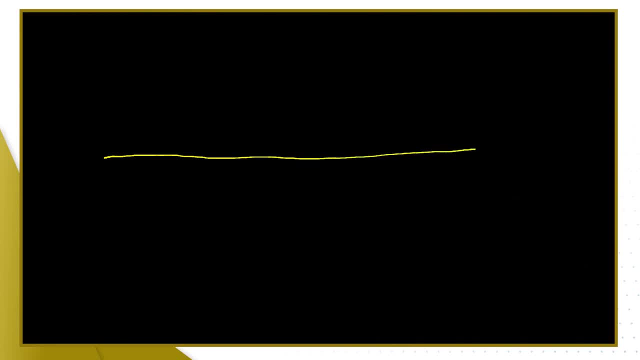 That means we're going to have a horizontal axis- and notice that I'm labeling it X as our tradition and our convention, and a vertical axis That we're labeling Y and notice that it is important to put the arrow at the end of that line in both of the axes and the letter that it refers to. 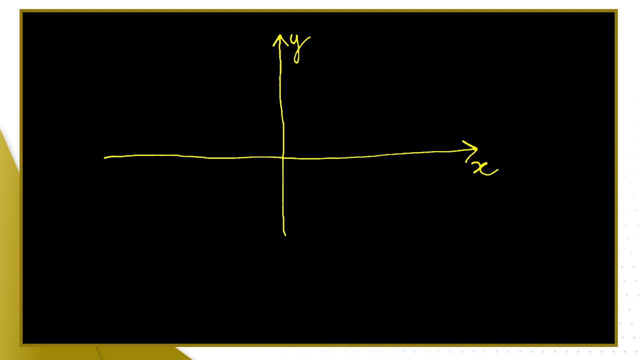 We're using handwritten lowercase letters X and Y. The other important thing is these axes have to be orthogonal, meaning perpendicular, meaning that the angle is 90 degrees. The point where they cross is called the origin, and it's where everything starts. 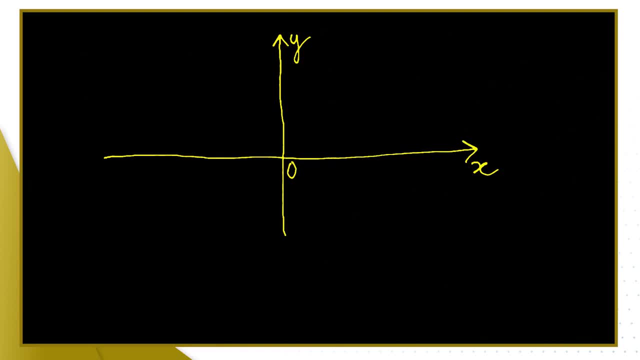 Now our convention is going to be: we are assigning two numbers. that tells you in which direction you're walking to get to that point. You start at the origin and if you go, 2 and then 3, we are using 2 in the X direction and we're using 1,, 2 and 3 in the Y direction. 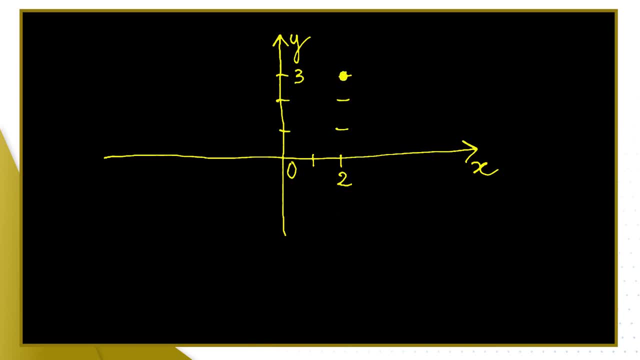 And our point is going to be the X direction. The point is there. The way I write that point, you can label it. say that is point A and A has coordinates 2, 3.. I did use a dot on that point, but it's important that when you locate a point you use the cross and then you can embellish it with a point if you want. 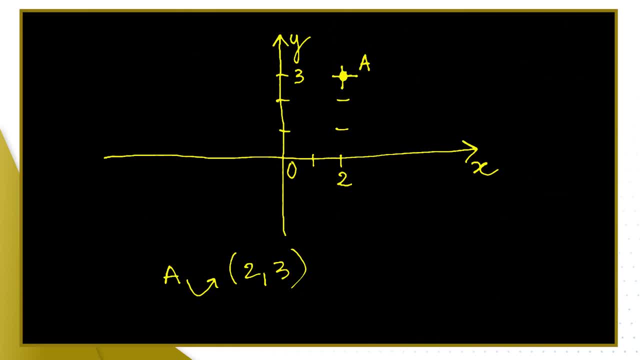 Now let's see what happens with other points. Let's make three more points. Let's start here And we'll do say point B has coordinates minus 1, 2. That means I will use minus 1 steps in the X direction from the origin. 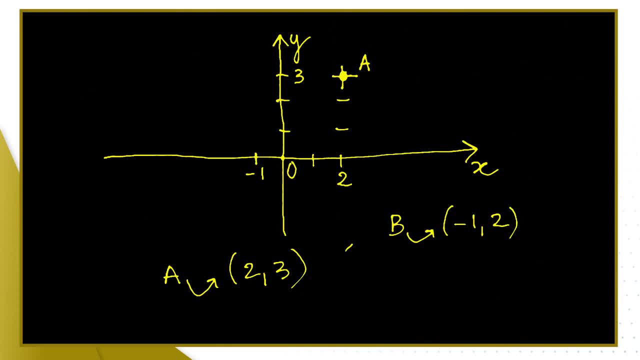 So from the origin I go negative 1 there, and then I do 2 in the Y direction. That means 2 upwards from where I was. So 2 upwards from here, 1 and 2.. So here's my point B. 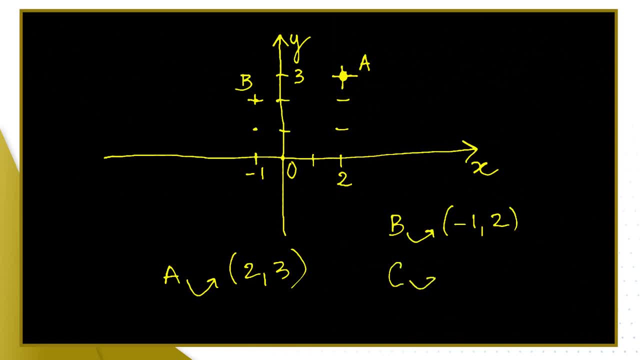 There we are. So I've got C with coordinates: negative 2, negative 1.. I start at the origin. I go 2 steps on the negative direction of X, So negative 2, and now negative 1 on the Y, so 1 down. 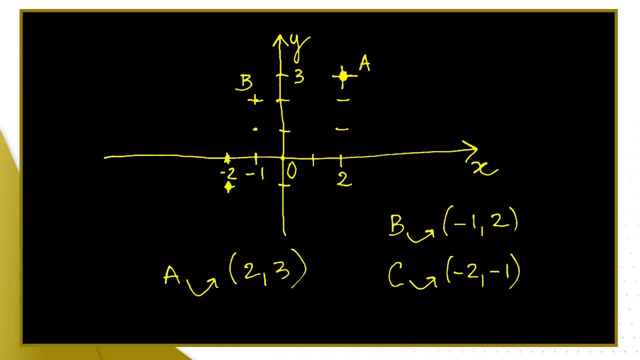 1 down from here. So I've got point C And for point D you're probably guessing I'm going to use a positive X And a negative Y. yes, I'll have 1 and negative 2.. That means 1 in the X direction here and then 2 down. 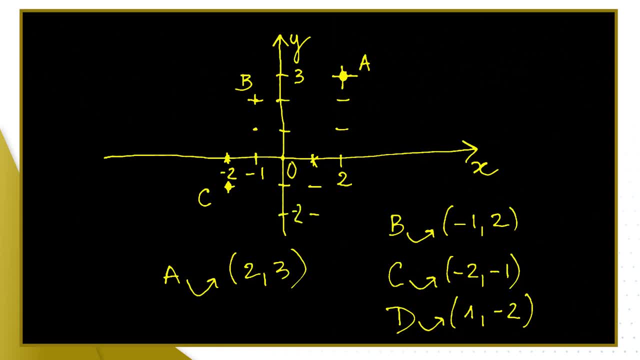 That's negative 2.. And so it's my point D. Okay, So I've got four points there, one in each quadrant, And the quadrants are the four parts of the plane that were split by the axis. So we have the A is in the first quadrant. 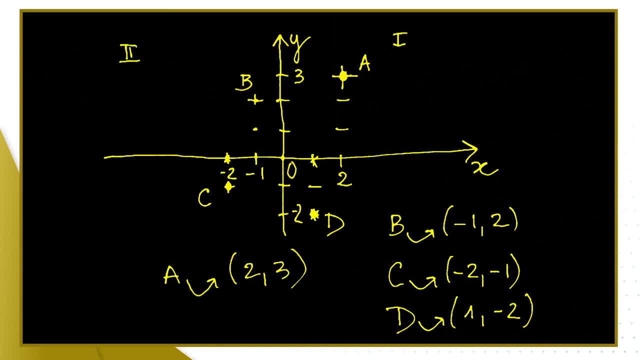 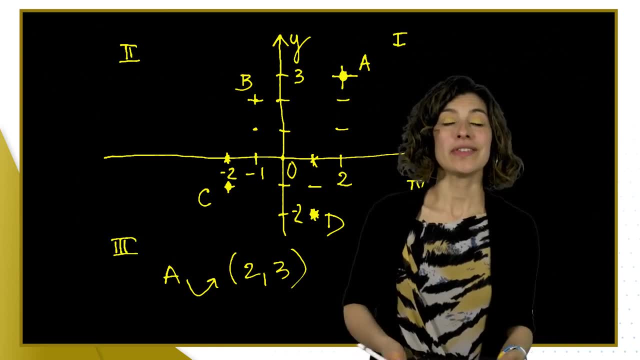 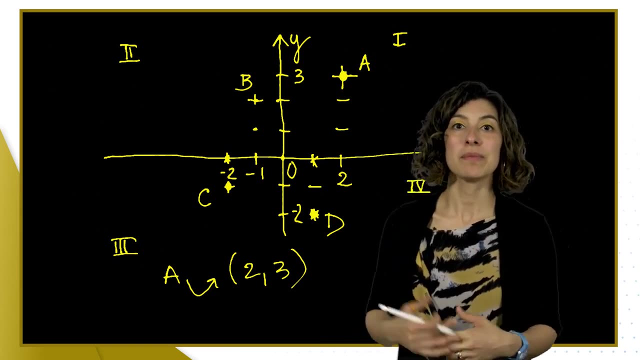 The point B is on the second quadrant, Point C is on the third quadrant And point D is on the fourth quadrant. Coordinates of points can be added and subtracted And you can scale up a picture by multiplying the coordinates of a point by a number. 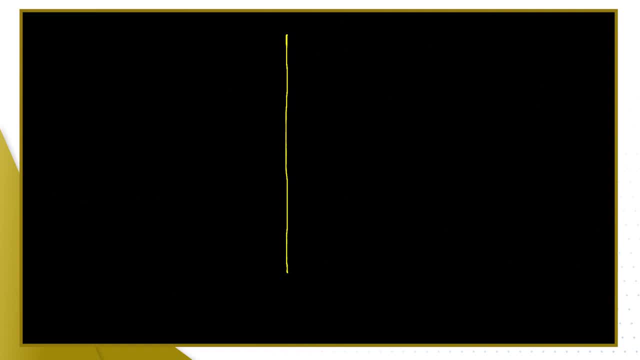 So, on a new graph, my X, my Y, I have points P with coordinates 1, 2, and Q with coordinates minus 2, 3.. We're going to use a different scale this time. I'm going to represent 1 and then 2.. 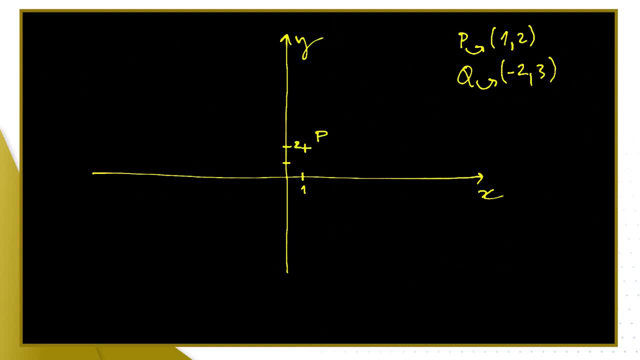 So my point P is there, Then Q is on minus 1, minus 2.. And then 3,, 1,, 2, and 3. there, That's where Q is. Let's use a little colour. So I've got P and Q. 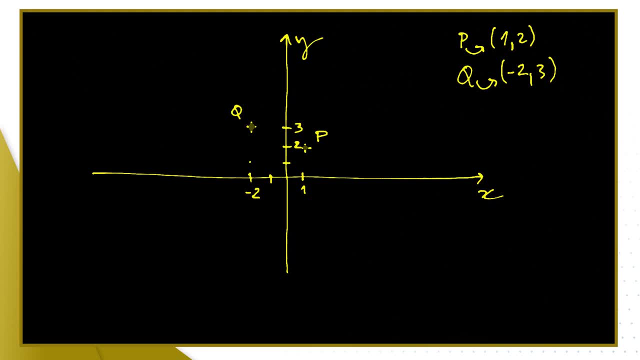 Okay, We can write what P plus Q makes sense to do. What we do is just add the coordinates: 1 plus minus 2 is minus 1.. 2 plus 3 is 5. And, geometrically speaking, P plus Q has also a meaning. 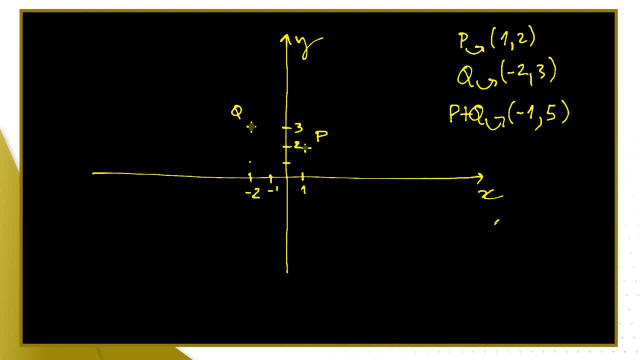 Let's just plot the coordinates: Negative 1, it's there, And then 5,, 4,, 5.. There we are. Here's the point. That is P plus Q. Let's put that a little green. That's P plus Q. 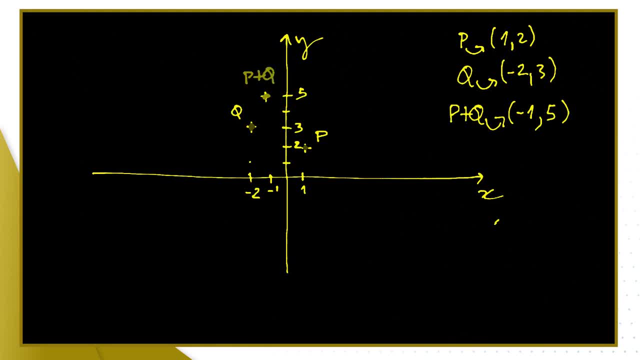 And if you've done vectors, you may have seen this before. If not, I'll just look at that. If I look at the arrow that goes from the origin to P and the arrow that goes from the origin to Q, that adding of P plus Q is the vertex of the parallelogram. 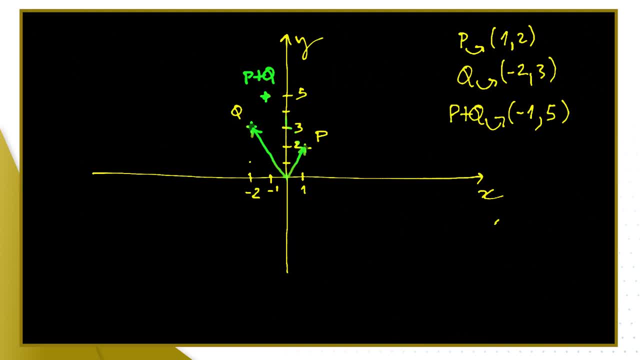 made by those two lines. What I mean is I take the arrow for P and I put it there, And I take the arrow for Q and put it here, And that P plus Q is the other corner of that parallelogram. Just the sides are all parallel here. 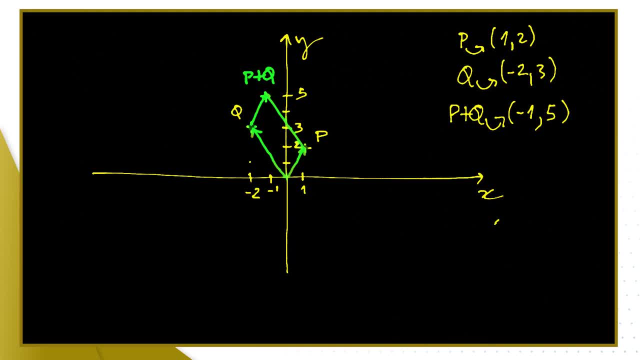 You can subtract as well the coordinates one by one. So, for example, if we do Q minus P, that would be the coordinates of Q. take away the coordinates of P, So that would be minus 2, take away 1, which is minus 3.. 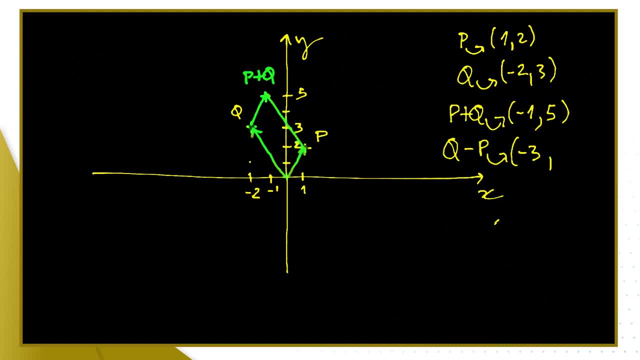 And then 3, take away 2,, which is 1.. And so the subtraction of that will be minus 3 and 1, which is here Q minus P, And I will leave you to work out what that might mean geometrically. 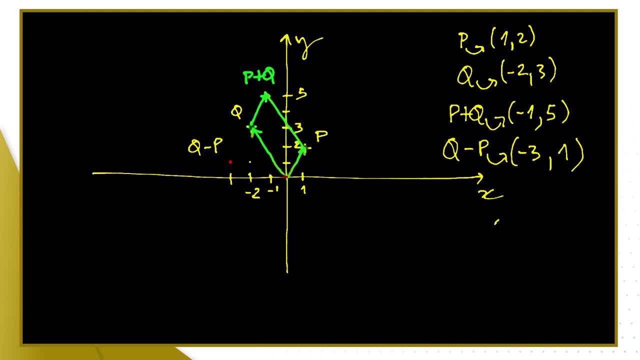 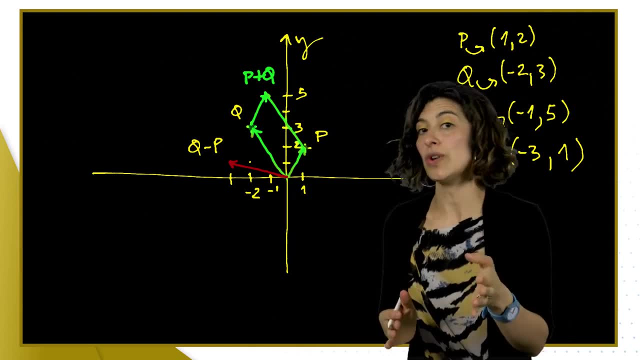 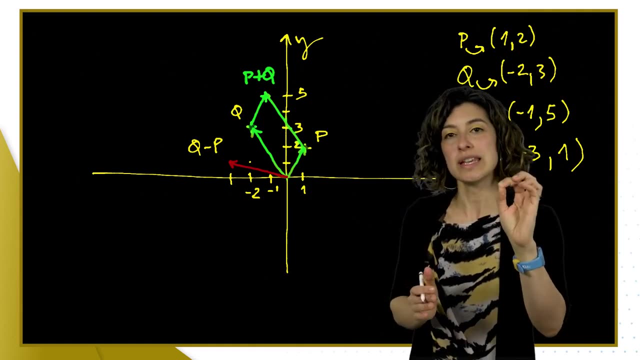 Just telling you that we can do those sums. So the arrow is there Now. just to clarify, we are not talking about the arrows just now In Cartesian coordinates in points. we are looking at the dot where the point is. I'm talking about the arrows. 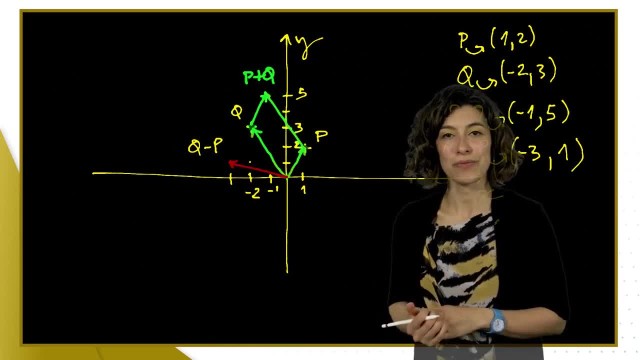 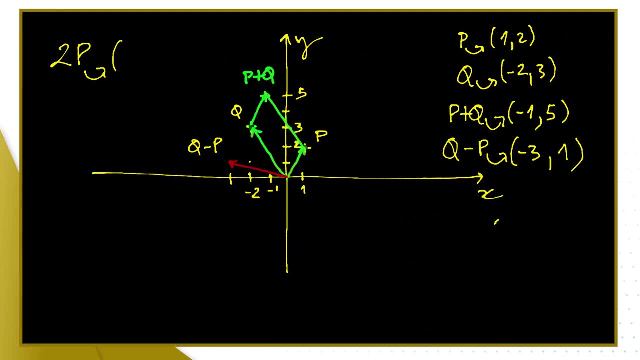 So you can build on any knowledge you might have had from before. As to scaling up, let's just see what 2P might mean. 2P would be doubling every coordinate in P, So P is 1, 2.. So we double the 1,, which is 2.. 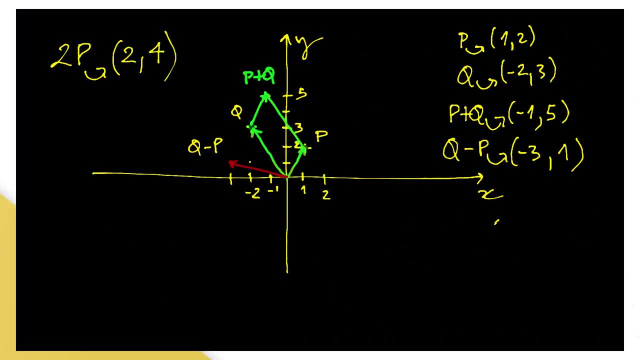 We double the 2,, which is 4.. And so 2P will be 2 and 4 there. So 2P is there And in terms of arrows, 2P would be the double arrow, an arrow that goes from the origin. 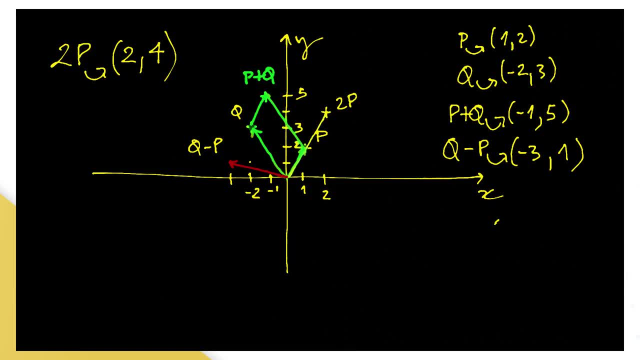 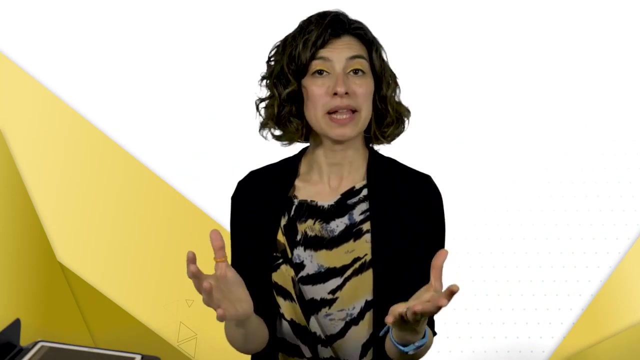 goes through P and goes over there. OK, Right, so we can add, we can subtract coordinates. We can also multiply coordinates by one number. We do not multiply coordinates of two points. We are not going to do that. We're using coordinates to describe parts of the plane. 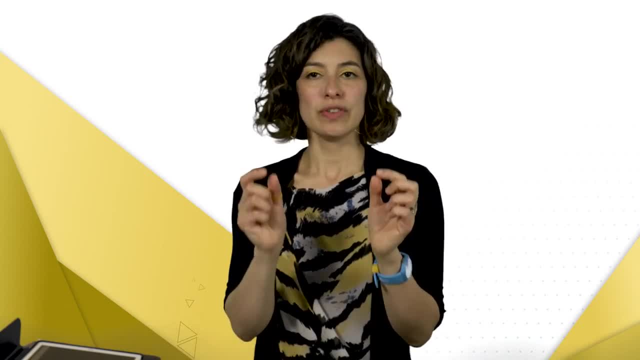 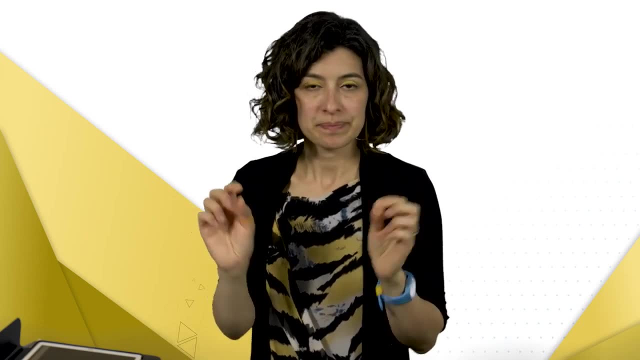 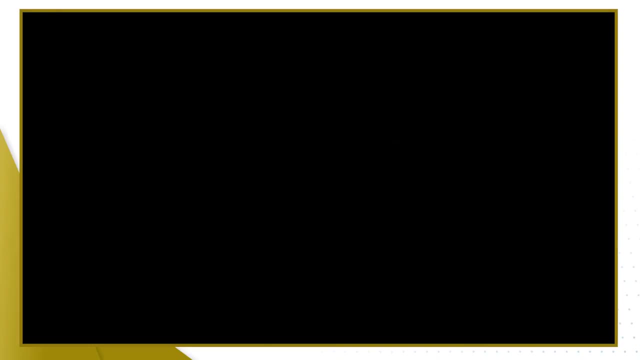 but we are also going to need language to describe language and notation, language and symbols to describe points within a line. So we're going to look at interval notation and simply say I want the point values of x between 1 and 2.. 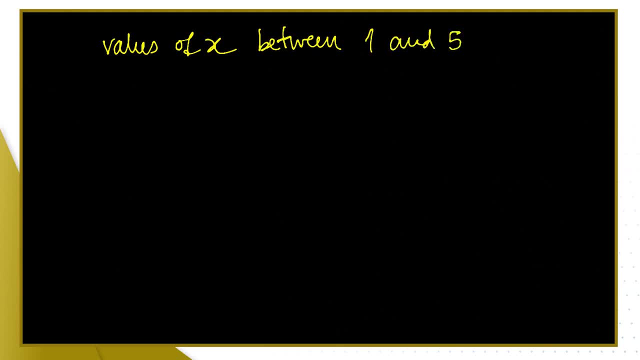 1 and 2.. 1 and 2 and 5.. That was a long sentence to write. We can summarize that in mathematical notation in the following way: x is greater than 1 and is less than 5.. But some of you may be thinking: could we have? 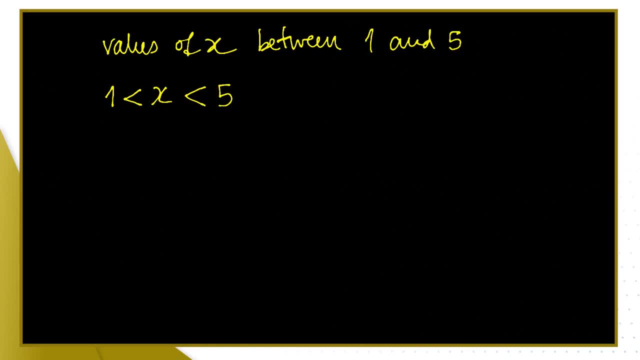 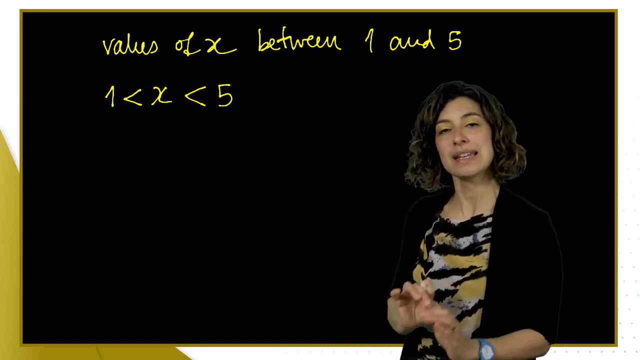 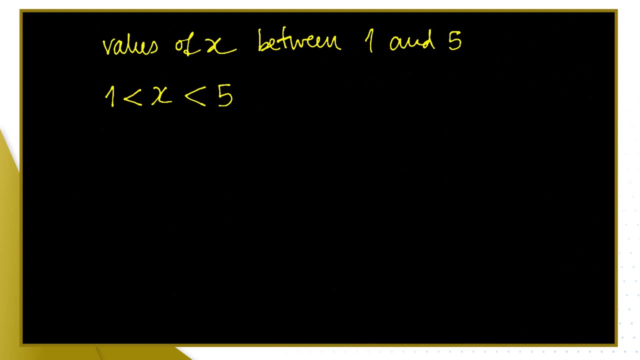 one less or equal to x, or could have x less or equal to 5 instead of just strictly less. written language wasn't clear enough, was ambiguous, so in mathematics we're going to make it absolutely clear whether we want to include the 1 and the 5 or not. So I want to. 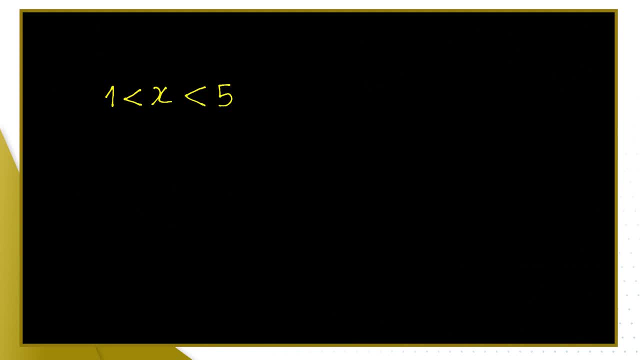 script that 1 less than x, less than 5 means in a line. I have the x line there, I've got the origin there with a 0, I've got a 1 and 2, 3, 4, 5, I mean all these points here, but not the 1,, not the 5,. 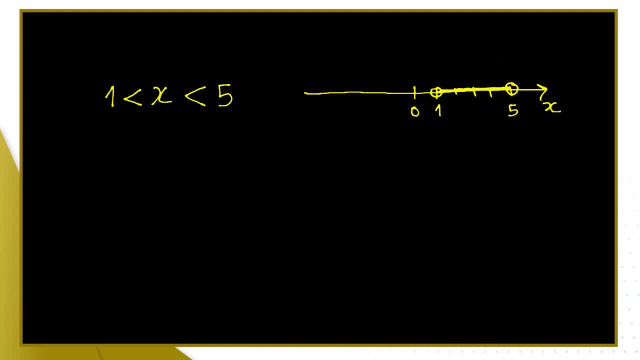 so I'm excluding that. and when we're drawing points and graphs, if we want to exclude a point, we draw a circle that is left empty inside. if we want to include the point, we fill in that little circle. So if we wanted to include the point, we would have to fill in that little circle. 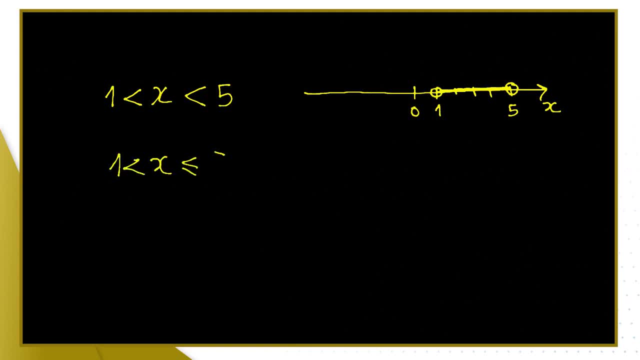 if we wanted to exclude the point, we would have to fill in that little circle, the five. we would write it with that symbol and, in terms of representing it on the line, we would make the ball open in one, the ball closed and filled in five, and we are thickening that line in between. so that will be our. 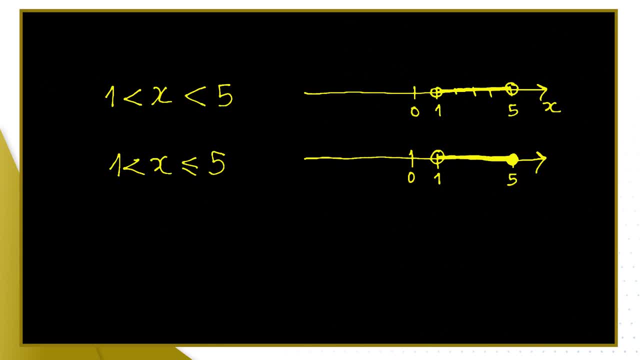 representation. now, this notation is still long, so there is a shorter way of writing it. that is the interval notation. gonna make some space here for it. alright, the first condition as one comma five, and that is an interval, and here 1 comma 5 with a rectangular brackets. that means close, that means include the 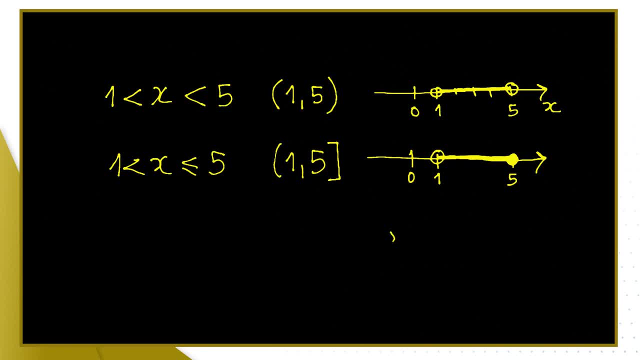 five. if I want to include both, I would write 15, and the condition that goes with it is: one less or equal to x less or equal to five. we can also have closed on one- that's the one that is missing- and open on five, so that will be that condition. 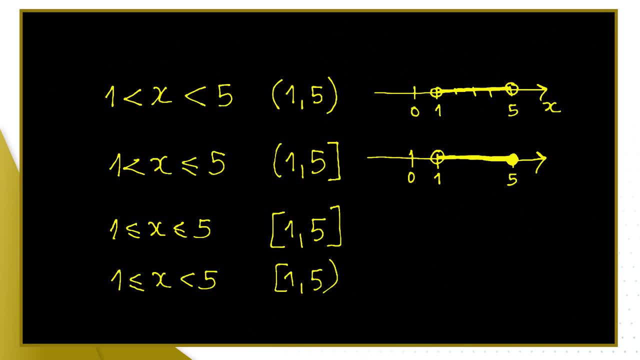 ok, there are times we want to include infinity, but just saying, you know, I want all the points after two, all the points after two. excluding two will be x is greater than two. that, on the line, means here's two at the end. I haven't plotted, is it the known infinity? and I want all. 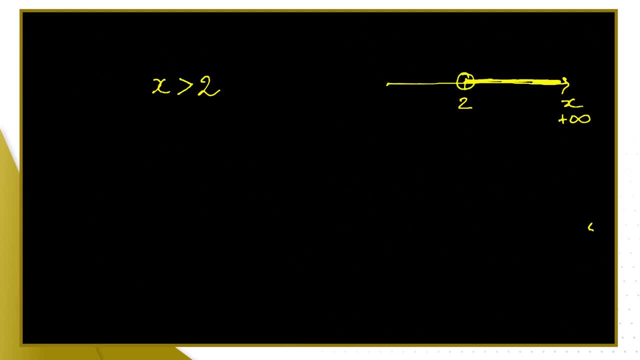 of those guys and I don't want to so open ball. or I could have x greater or equal to 2 and therefore I would include the ball and the interval notation would be 2, 2 plus infinity, and it's always open on the infinity and this one will be. 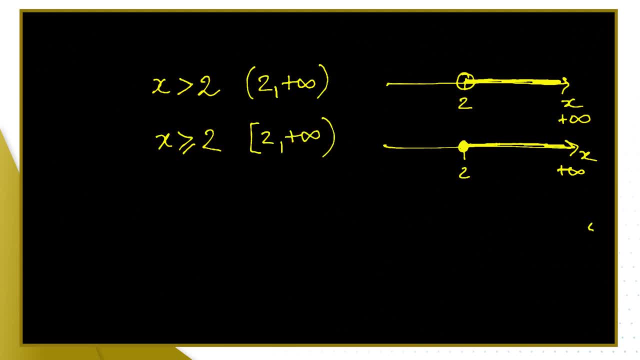 closed on 2 to infinity. and what's missing now? just doing the minus infinity intervals. so X less than 3 will be minus infinity to 3 open. X less or equal to 3 will be minus infinity to 3 closed. and that means the points on the number line, those ones closed with minus. 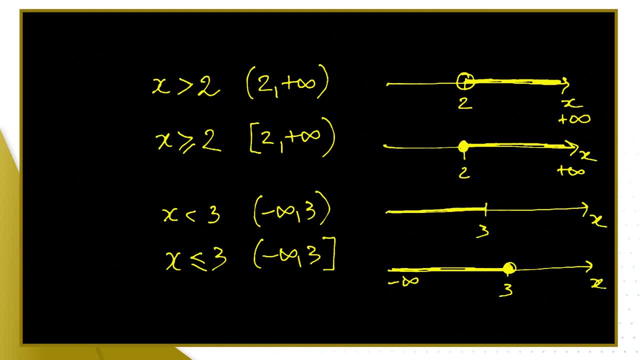 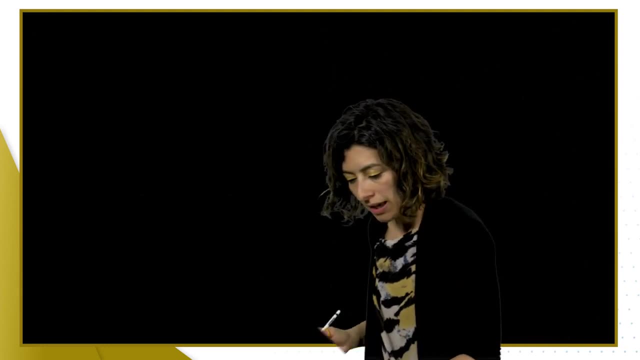 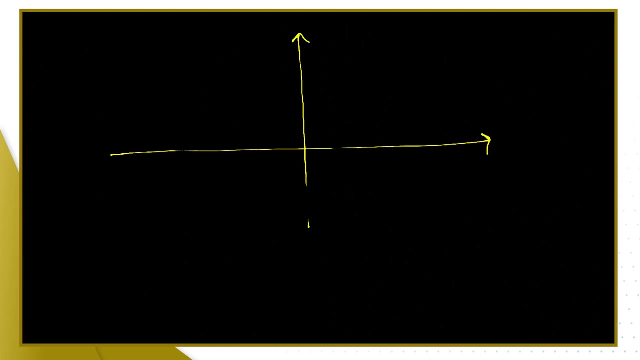 infinity and those open with minus infinity. there, how do we use this? we want a condition in the plane that we're going to use coordinates to describe and we might need to use these conditions or these intervals so say: I have got to that, so this is X. that's why that's the origin and I want all these. 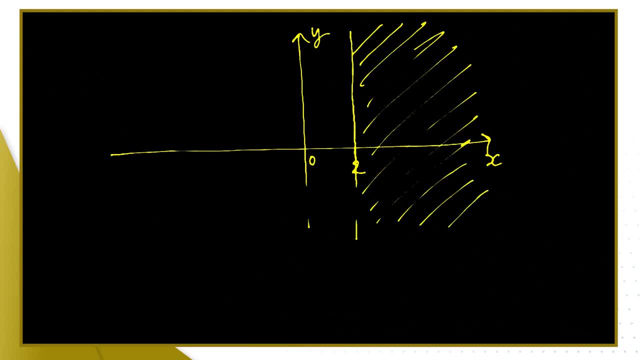 points. how do we describe them? looking at them, I see that it is everything that is to the right of two, everything's to the right of two, including two. that means that the points will have coordinates, X and Y, there will be coordinates, and the X itself is going to be greater or equal to 2, that's it. 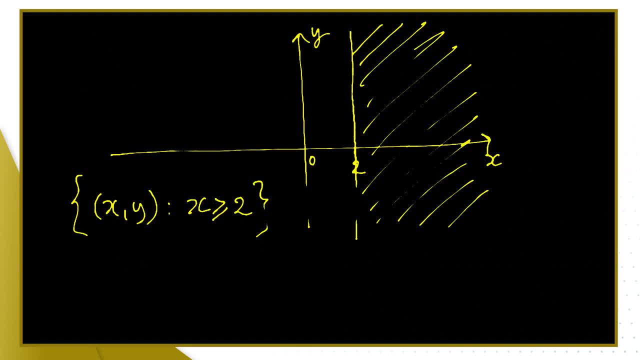 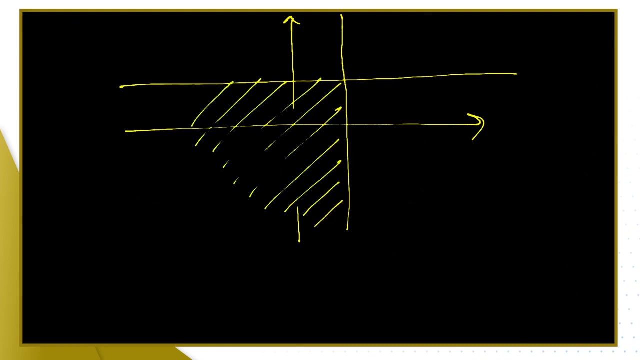 Y can be anything. those curly brackets around it just mean it's a set, is a set of all the points that have coordinates X and Y, and X is greater or equal to 2. another example could be that I wanted this is one and that is three. I want that region there. so this is X, this is Y. 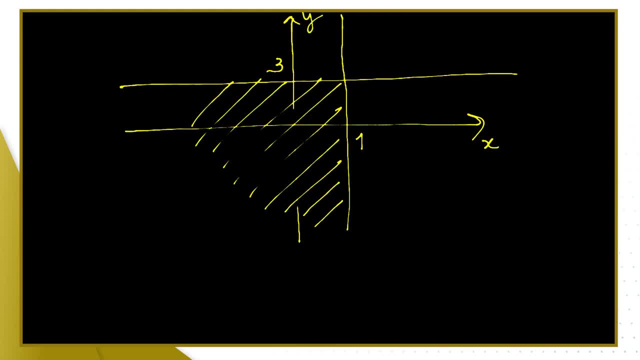 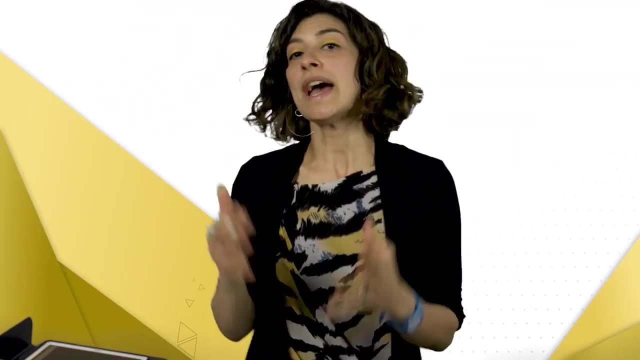 and I'll say I want the points with coordinates X and Y, and X has to be less or equal to 1 and at the same time Y has to be less or equal to 3. just an idea now. you might not write this formally like this when you're in. 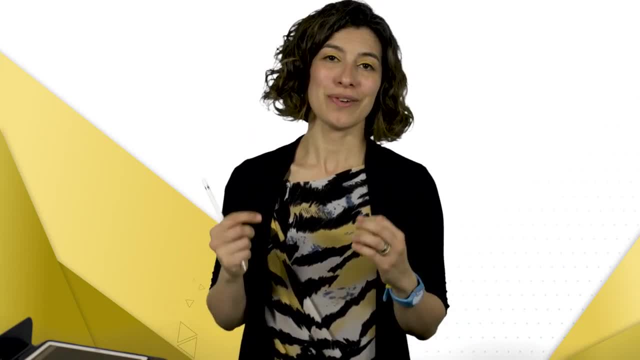 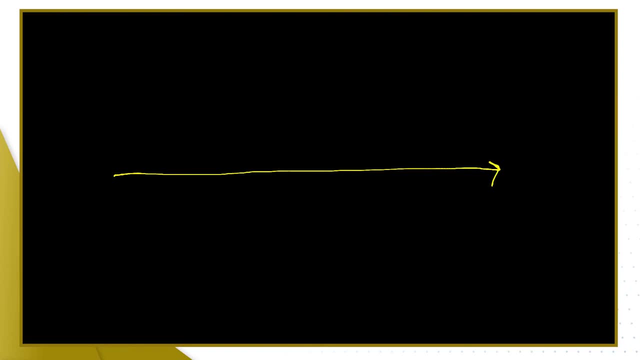 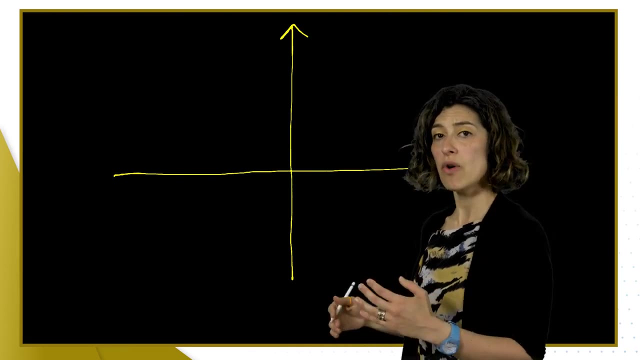 computing, but you will need to be able to make sense of the of of regions, and these are some of the ideas. you need to do that. the idea for graphs of functions will be that as X changes, we will have a value of Y that may or may not change. 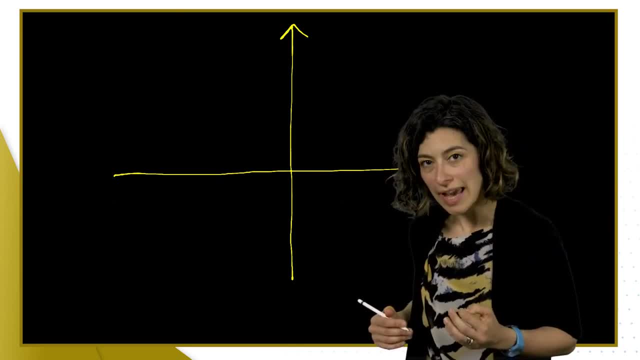 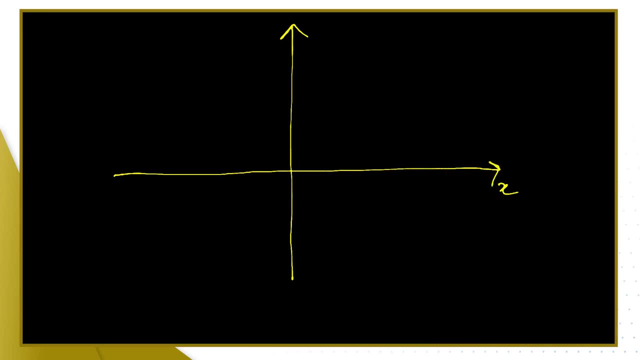 but it will be written as a function- will be dependent on the X. so the X, the horizontal, is the independent value, the independent factor, the independent variable, and the Y, the vertical, will be dependable one the one that is written as a function of the other. so a line like that is a line of a function, that's. 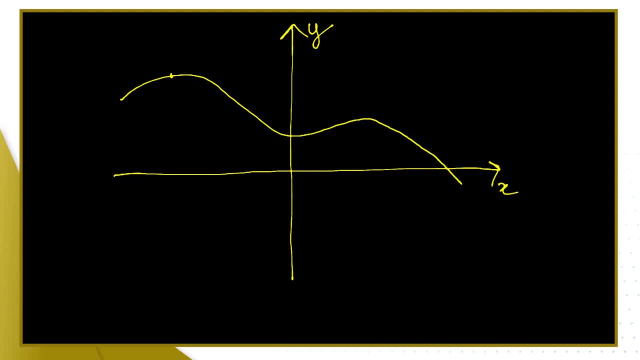 because each point on the graph has, of course it has- coordinates, X and Y, but you will never find one X value with two Y's, never. if you draw a vertical line, you will only cross the graph in one point, only in one point, and that's the Y value corresponding to the X. the opposite isn't true. you may have one Y. 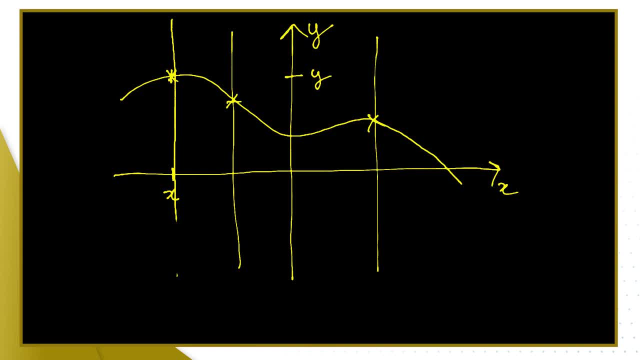 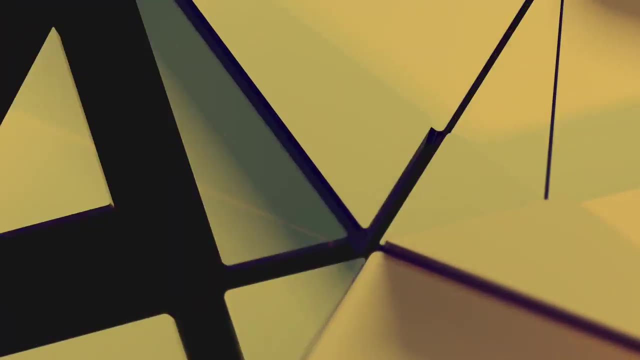 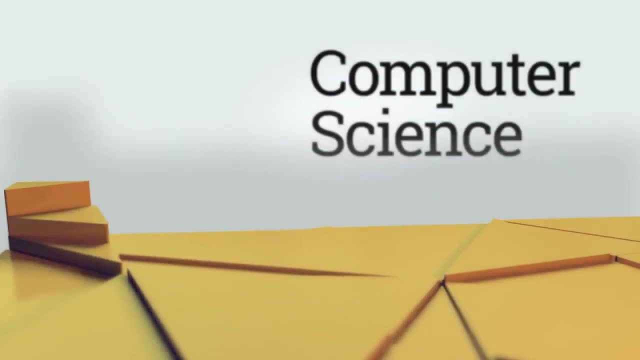 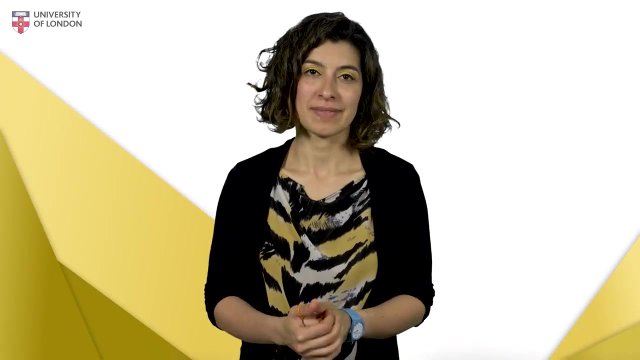 value that is the result of different X's. so in this case of this graph of sketch here, I will say that each value of Y is a function of X and usually written as F brackets X. in this lesson we use coordinates to represent the behavior of functions. 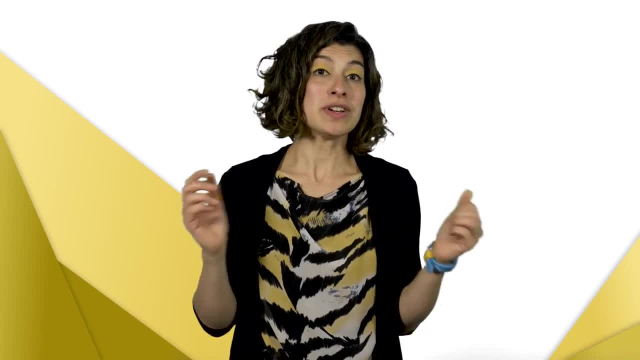 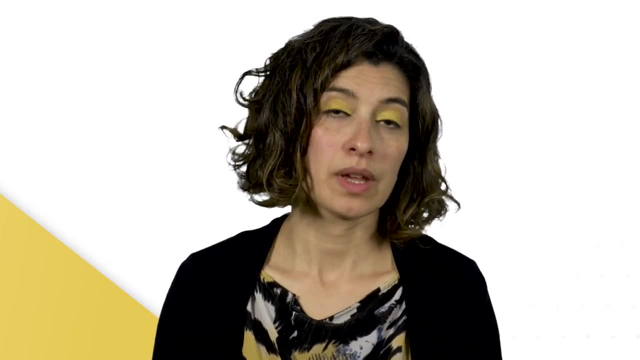 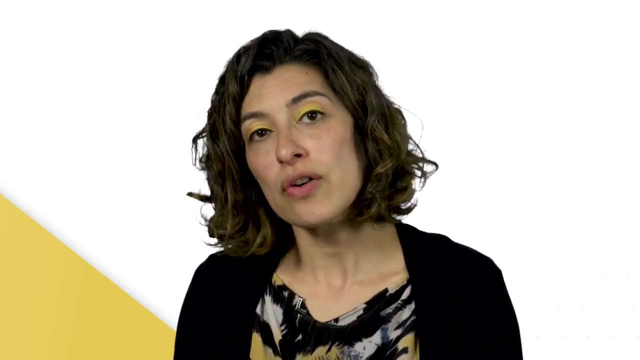 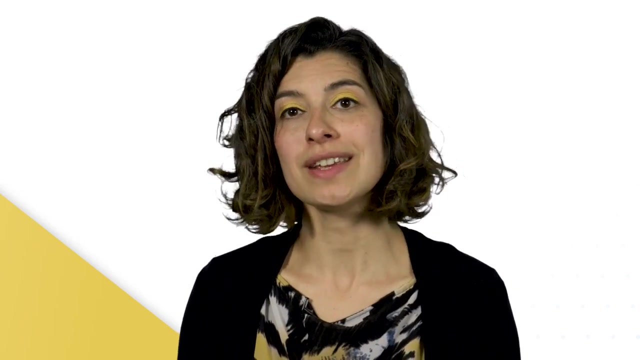 graphically. a picture is worth a thousand words. someone said once again: why do it by hand when machines can do it for you? you will need to make choices, to request a machine to highlight the features of the function that are of interest for a specific purpose. within the module, we will focus on you demonstrating that you. 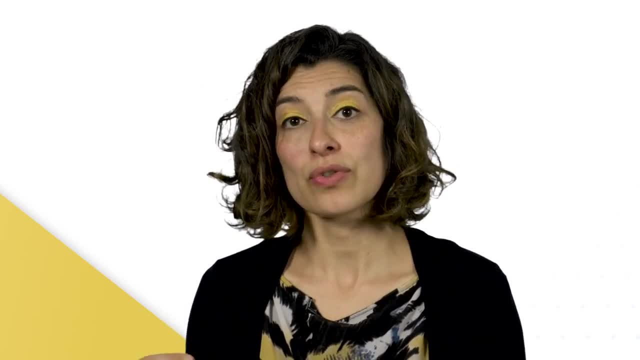 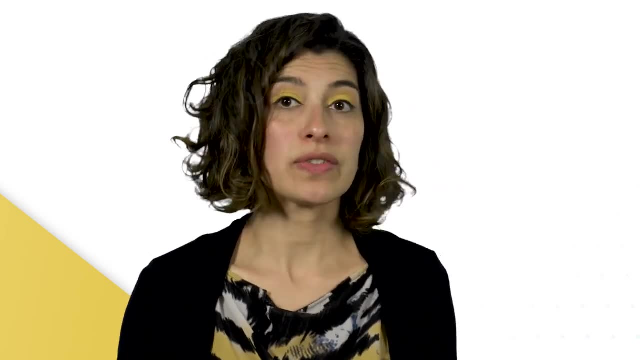 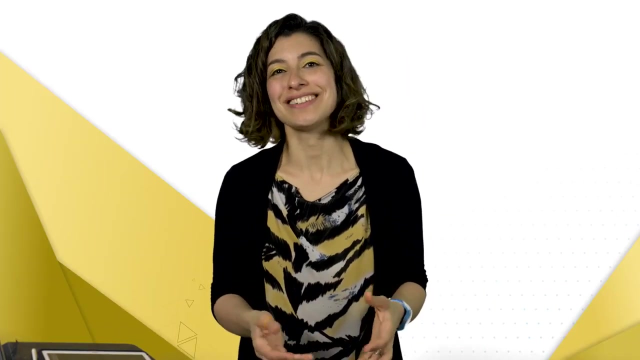 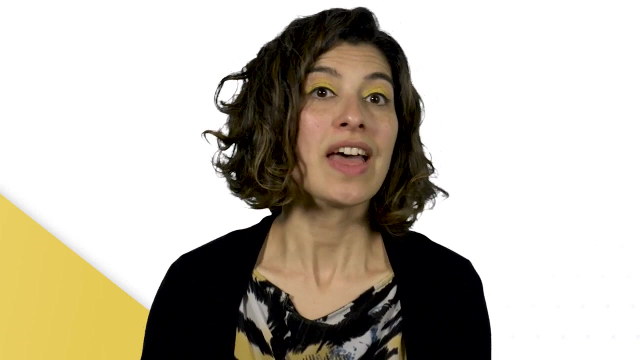 know what to expect from a given function in terms of growth and function, if it has repeating patterns, symmetry, if there are gaps in the graph, points of interest, and choose how to plot the graph to show such features. traditionally, the horizontal axis marks values of the variable, usually X that is independent, and the vertical axis the 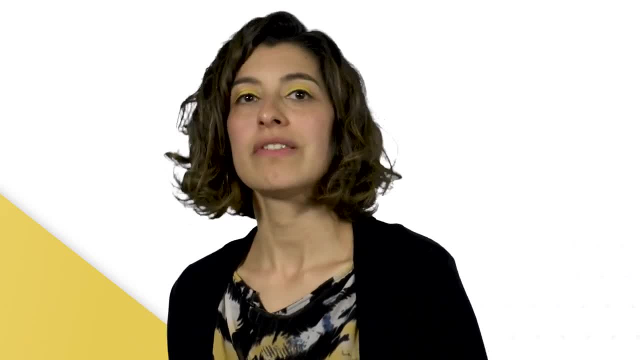 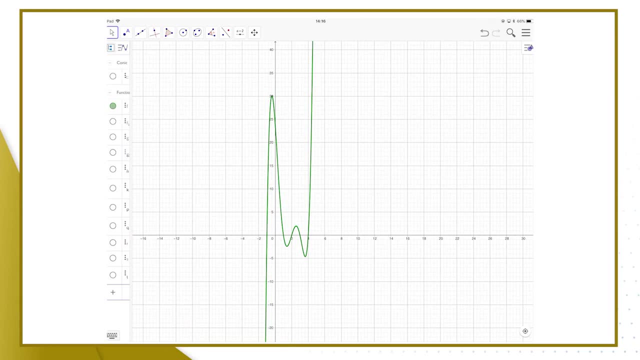 value Y of the function for each value of X. for example, this graph shows a function of X, meaning that the Y values are dependent on the value of X. there is only one Y value for each X value and that means that if we draw any vertical line, the line only cuts the graph once. 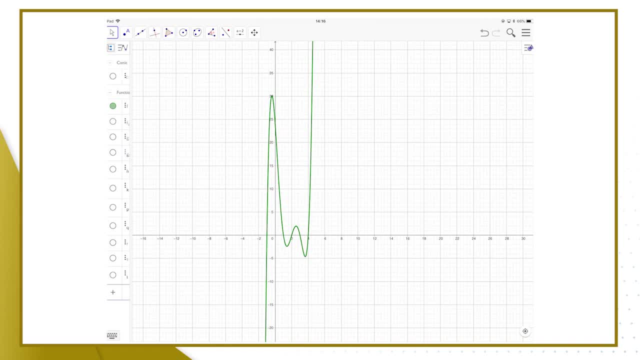 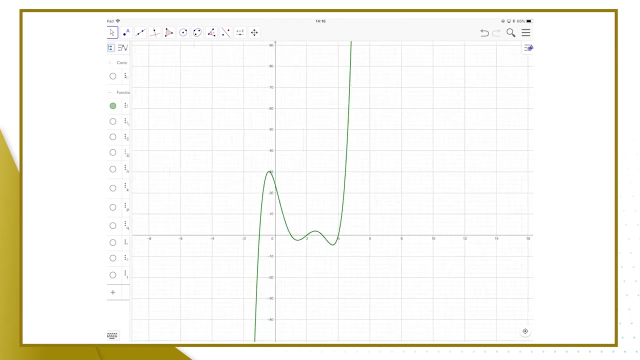 at most. now to show you this graph. I've already started making choices on how to highlight the interesting behavior. now I'm going to make some more choices here to see what is happening. near X equals zero. that's better. already. near zero, we now can see that actually in the window. 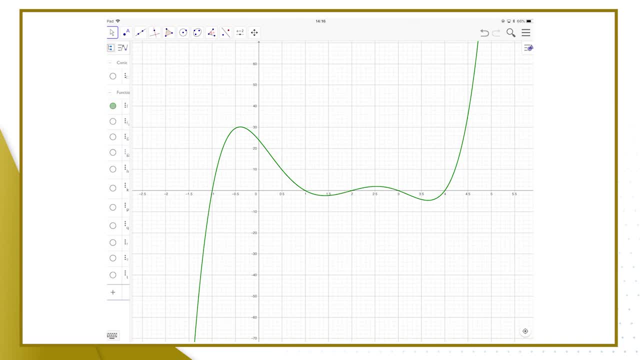 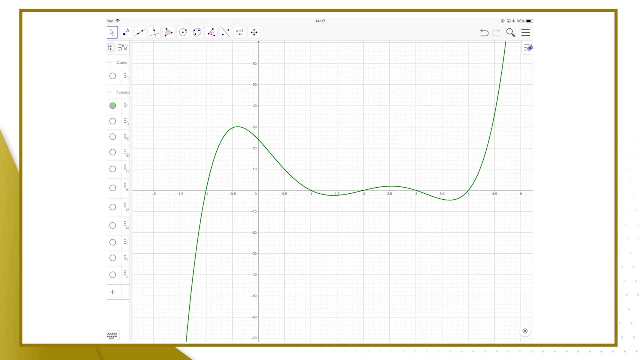 between minus 1 and 4. there's quite a lot of interesting behavior. there's a lot of variation in the graph. we now can tell that the values of Y increase for X up to about negative 0.4, where Y reaches about 30. see over there round about. 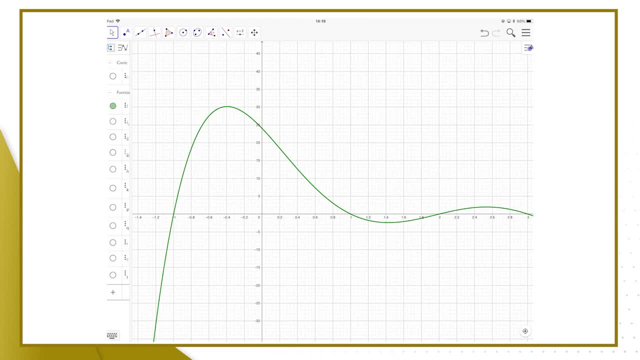 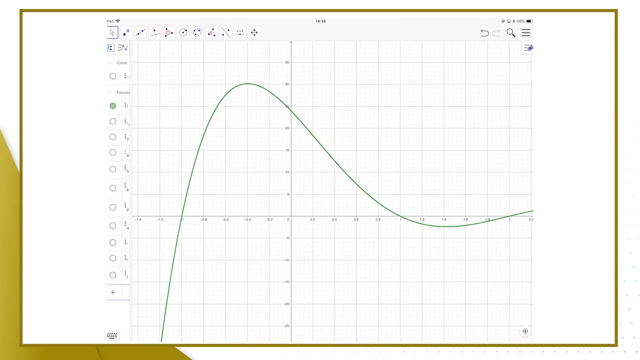 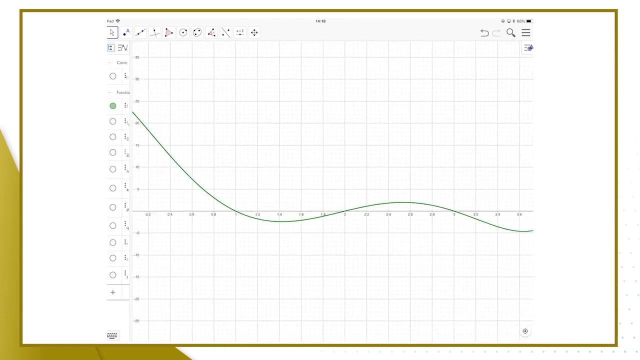 minus 0.4, Y is 30. now between X equals minus 0.4 to 1.4, the values of Y decrease animals andtest red, just so they come from 30 to around minus two and a half. then between X equals minus 0.5 will form positive y. so this is: 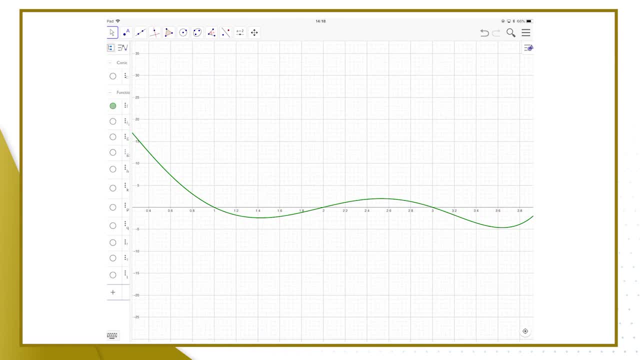 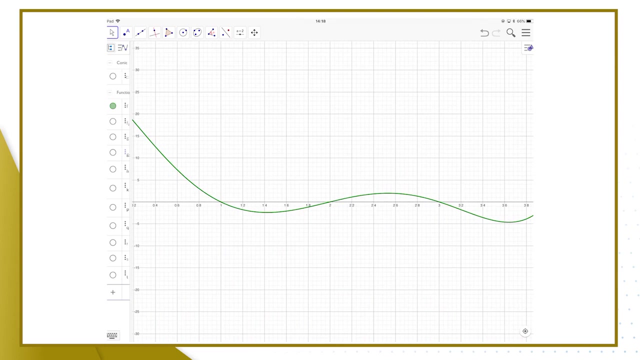 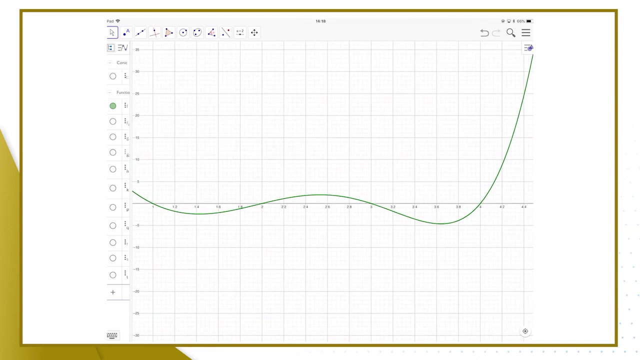 1.4 and about 2.5, y increases again to a maximum of about 2.. Just need to make sure that we're reading the scale right. Yeah, about 2.. And again, y decreases when x goes from 2.5 to about 3.65, give or take From that point, from x equals 3.65 onwards y. 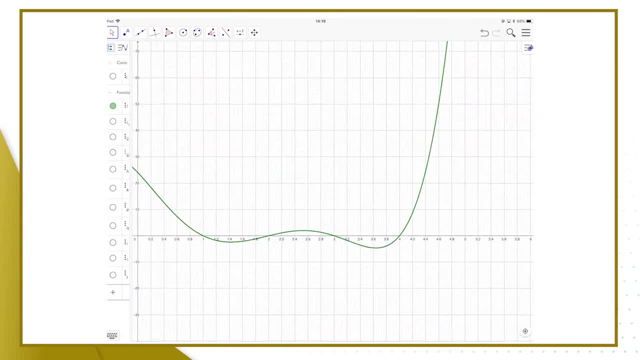 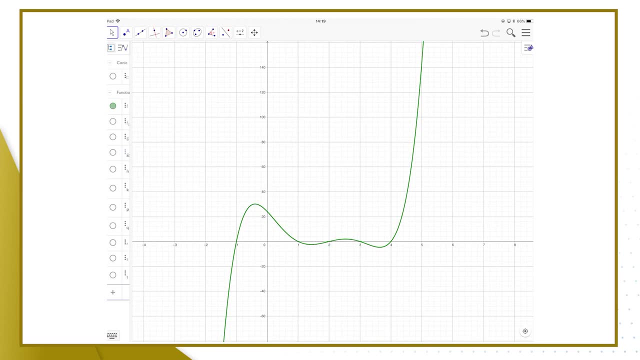 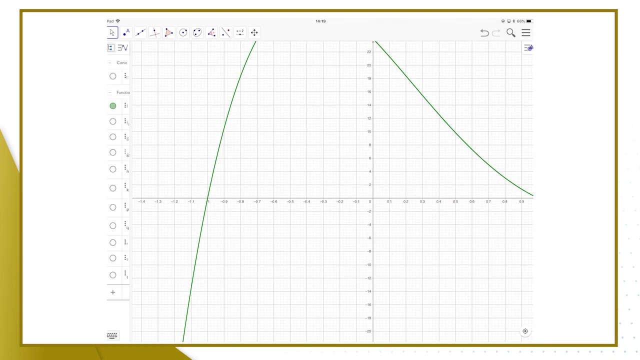 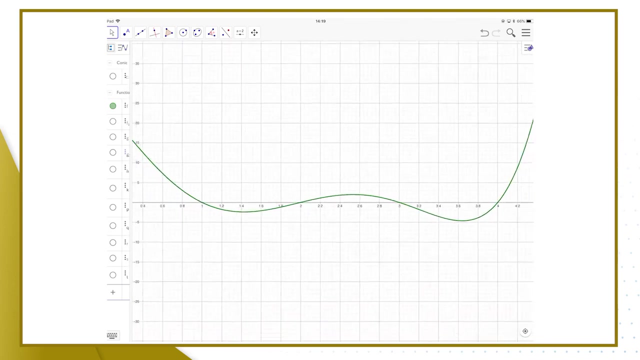 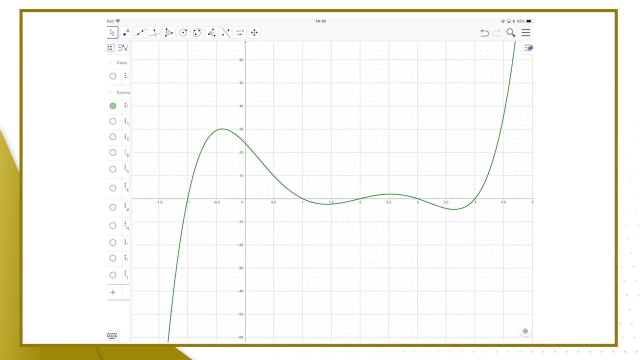 increases rapidly And we can see that zooming out again, We can also see that the graph cuts the x-axis several times. Let's look at the point. x equals minus 1.. Is it precisely minus 1?? Good question. At 1,, at 2,, at 3, and at 4.. We can check whether or not that is precise. We can check. 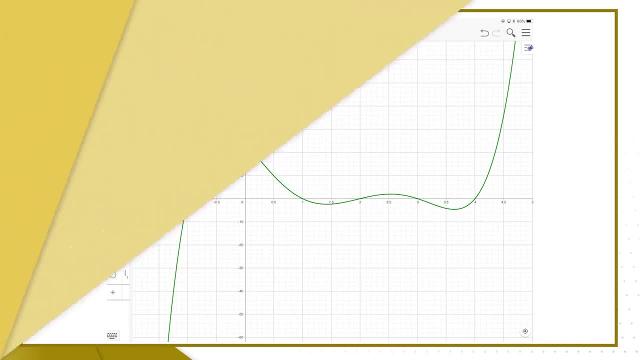 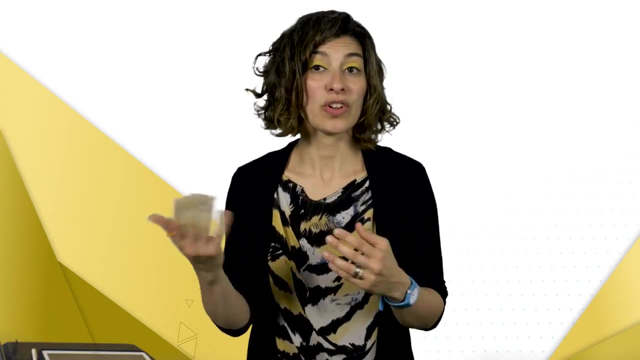 algebraically We can do calculations. We're going to find those precise values where the line crosses the axis. Those are called the zeros. But can we always find that out? Sometimes we can, sometimes we can't. We will look at the x-axis. 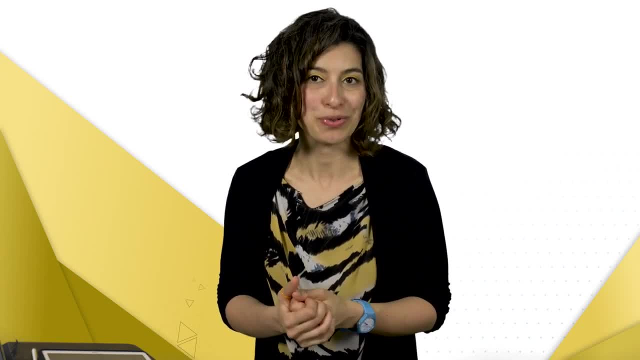 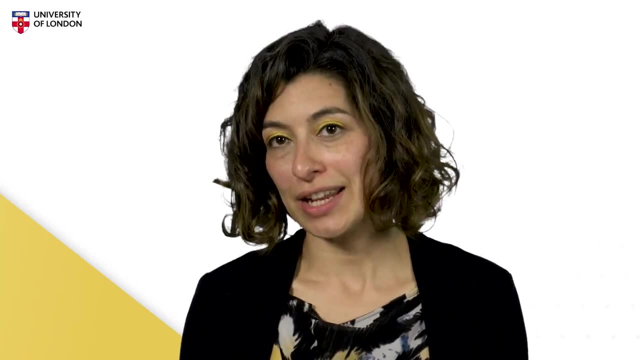 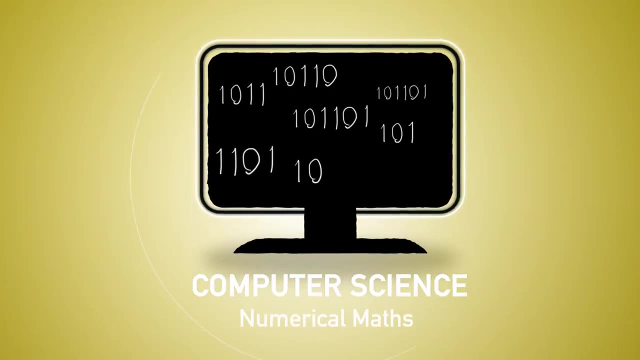 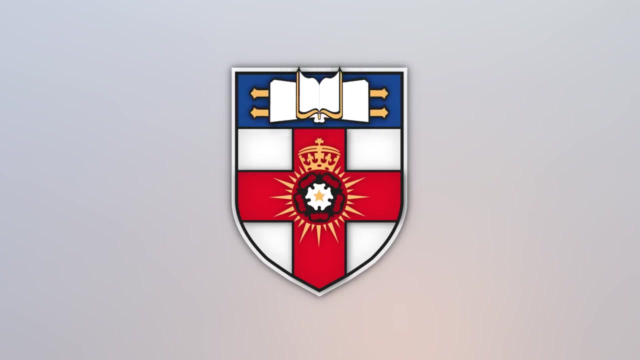 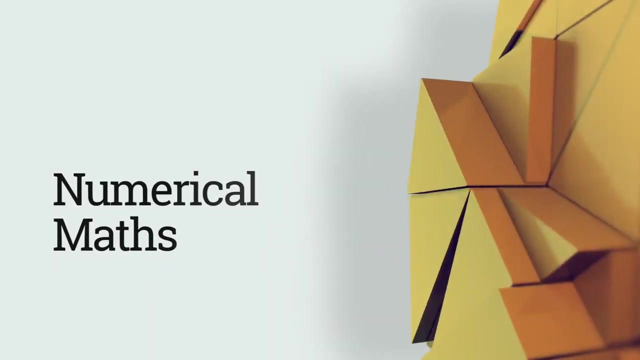 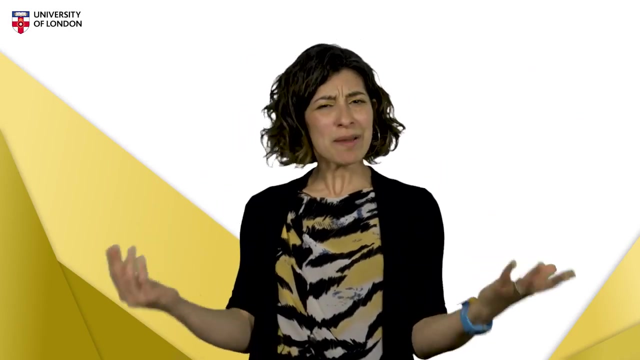 We will look into these questions so we know how much is possible to do with precision. We will get some of the tools needed in this topic. We will learn more tools with limits and calculus later on. in this module You're going to plot and sketch graphs by hand. And you wonder, but I'm a computer scientist. 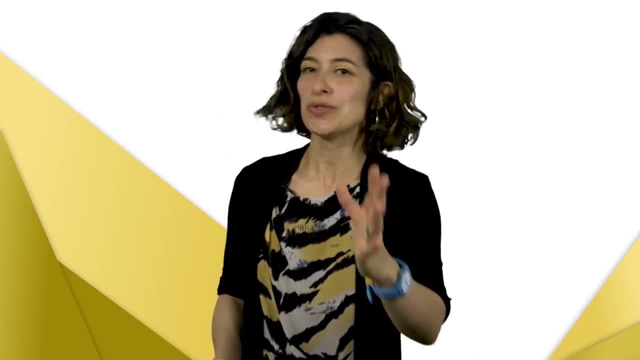 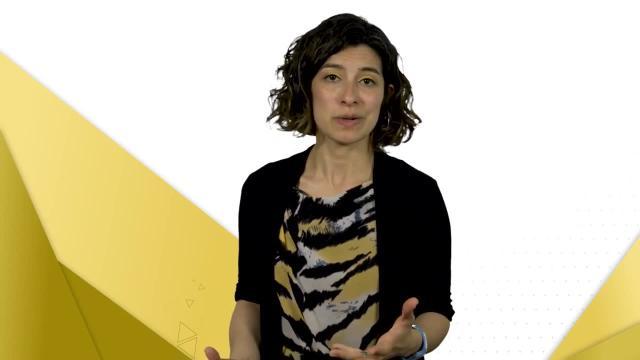 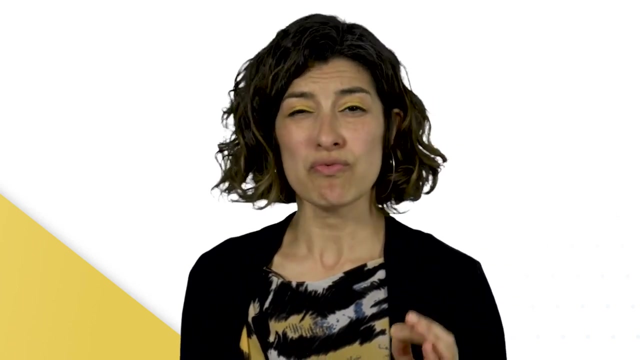 Why do I have to do this by hand? We want you to understand functions so that you are able to implement functions in your programming appropriately. So in this module I want to prepare you to do all the work, to do a really good graph that. 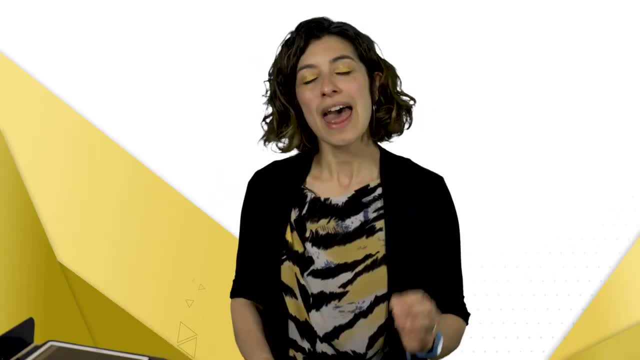 captures the graph. So I want you to do all the work to do a really good graph that captures the graph. So in this module, I want to prepare you to do all the work to do a really good graph that captures the graph, Because it represents the essence of the behaviour of the function. 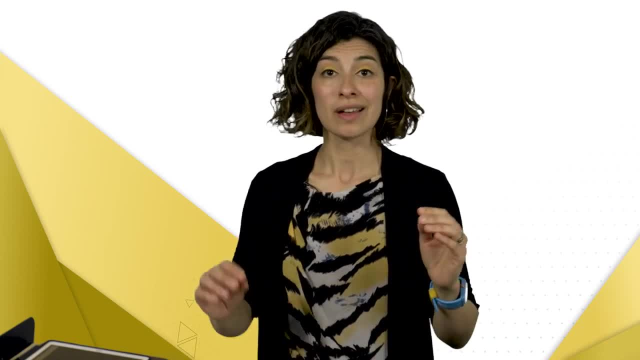 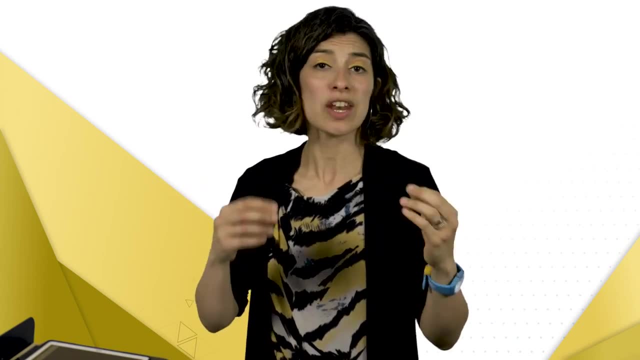 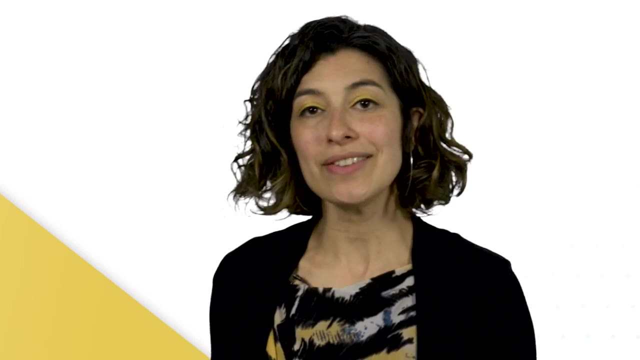 And that's what we're looking for. We're not looking for you to replace a plotting machine. We wanted to give the impression of that behaviour, the impression of change and all the points that are noteworthy in the function. The first thing we need is to have a table of values. 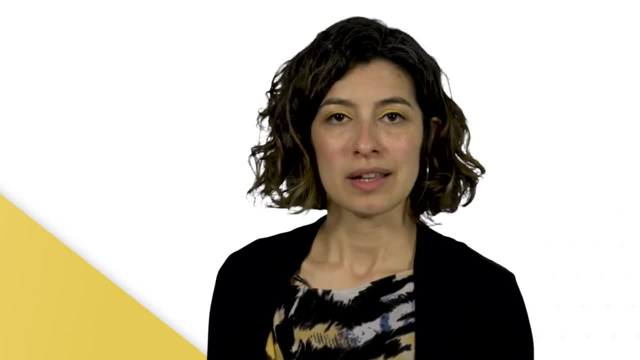 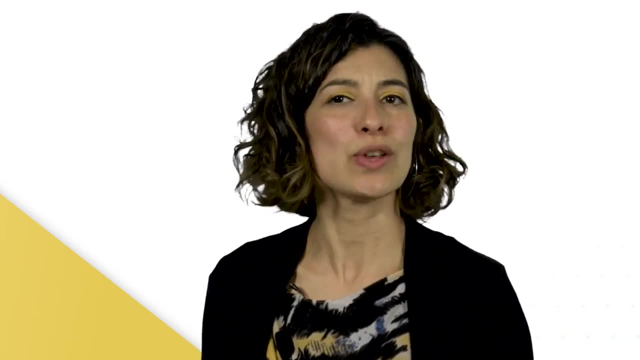 I mean, the first thing we need is to have a table of values. You need a table of values before you start drawing, And the table of values is not something just do blindly. we're going to think about what points, what values, are good to represent in this. 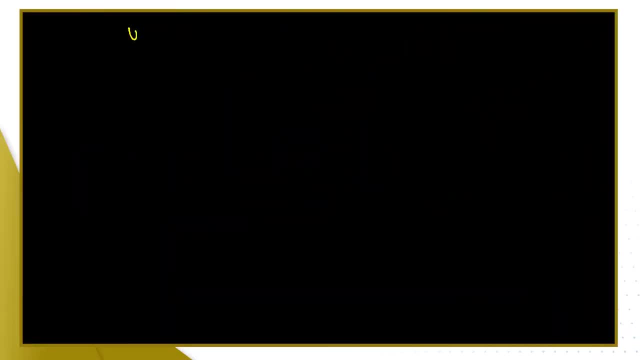 table. Say, we've got the function: y equals x squared minus 2.. We're going to prepare a table of values for this. If you know nothing about the function, you just start with a few values to help you. So we do. values of x are going to run over there and the corresponding value of y. 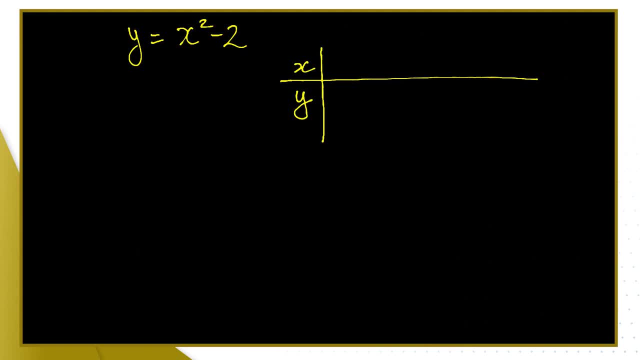 Now I write y there, but I really want you to think that, instead of just y, what you need to calculate in that line is x squared minus 2 for each value of x that appears on the top row. So really, what we have here is x squared minus 2.. Let's put it in a few values. 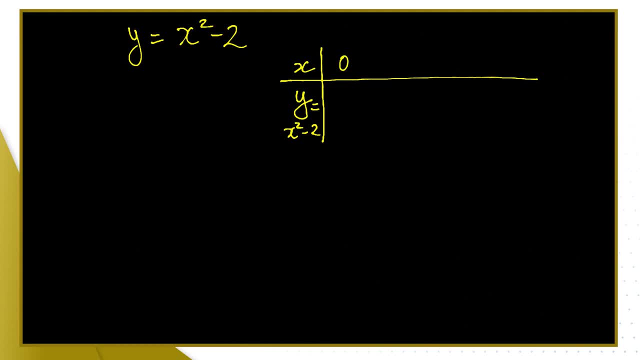 Let's try what happens if we put a value of 0.. 0 squared is 0, take away: 2 is minus 2.. Let's do 1.. 1 squared is 1.. 1 minus 2 is minus 1.. So minus 1.. Let's try the value of 2.. 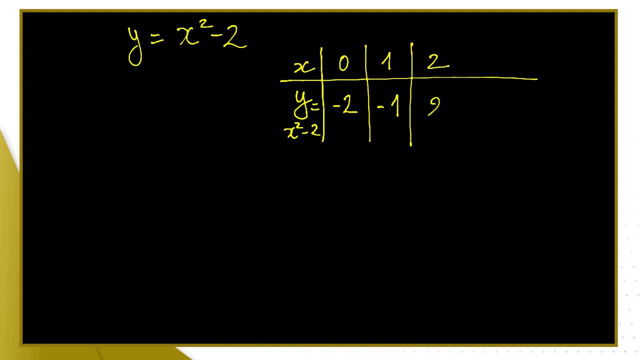 2 squared is 4,, 4 take away 2 is 2.. Are 3 points enough? Well, if you know nothing about the function, then I suggest you do the following: If you know nothing about the function, then I suggest: 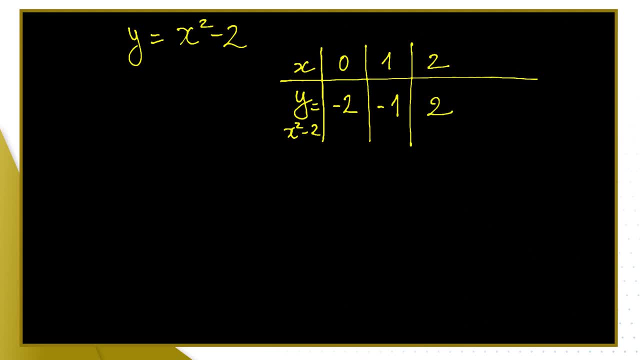 you start drawing the graph from the points you have. If you know something about the function, you will know that this is not a good choice of values, But let's do it So: x-axis, y-axis- we're going to have our origin there. We need to choose a scale for now. 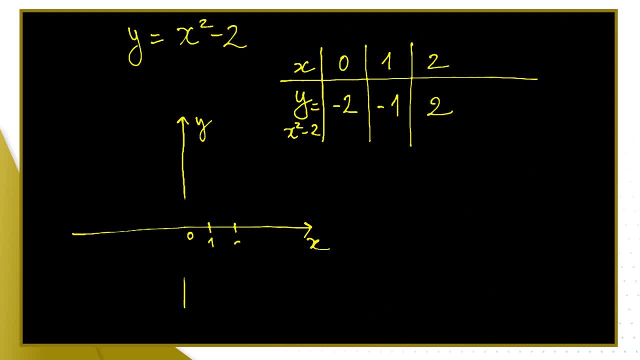 Let's see 1 there and 2.. And for the y-direction, we don't have to use a scale. We don't have to use the same scale for y as we use for x, but we just have to have a scale on each. 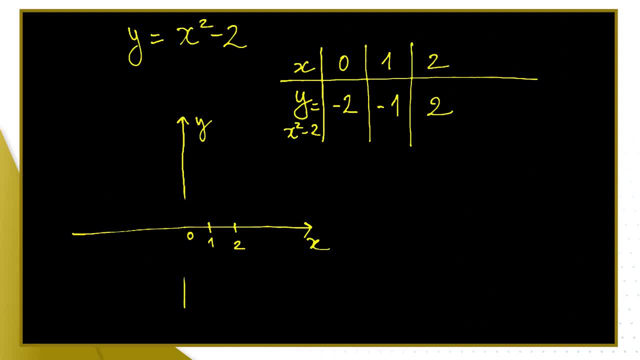 and have consistent representation. Now for now, 0 will have a value of y minus 2.. So 1, 2, so minus 1, minus 2.. So I've got that point there In 1, I've got negative 1, so I'm there. 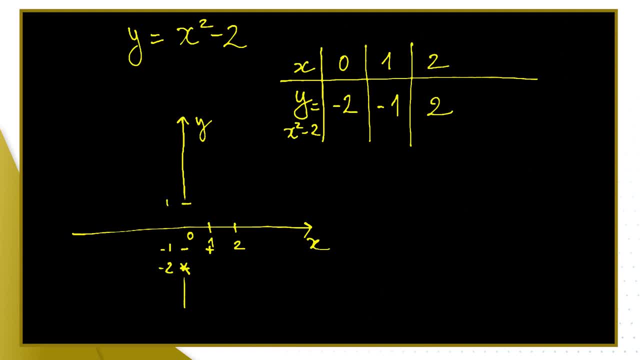 And on 2, I'm on 2.. Wow, 1 and 2,. what happened there, you wonder? All right, so I've got three points which I'm going to mark with a different color. I've got that point, that point and that point. 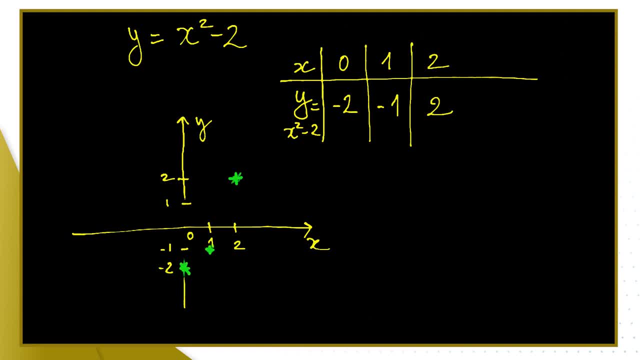 Okay, tempted to just draw the line there. Now, if you know nothing about it, you could be tempted to do this. That is terrible. What I wanted to do is you go through a few of these functions on a plotting software like what I've shown you in the previous video. 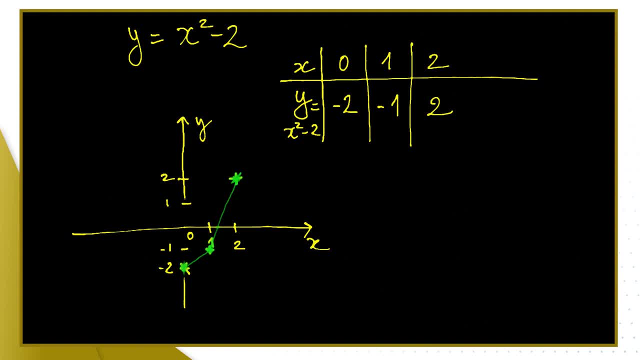 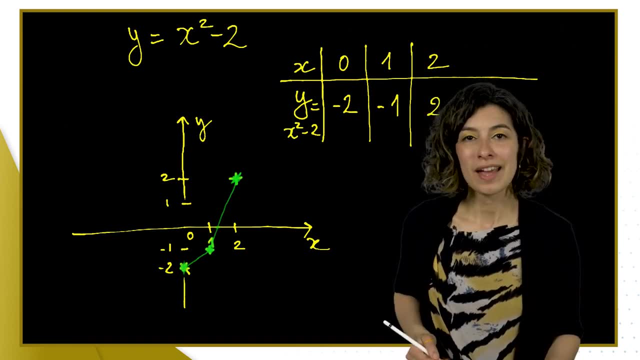 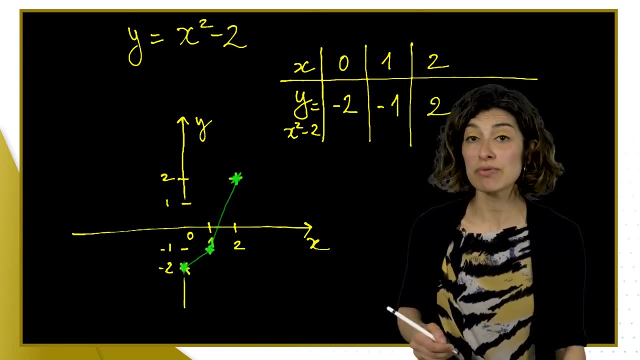 You build an intuition of what the graph should look like. That is awful. This graph is not going to be straight lines. This is a quadratic function And if this is new to you, just go and plot a few until you get a sense of what they look like. It has to look like a parabola And a parabola. 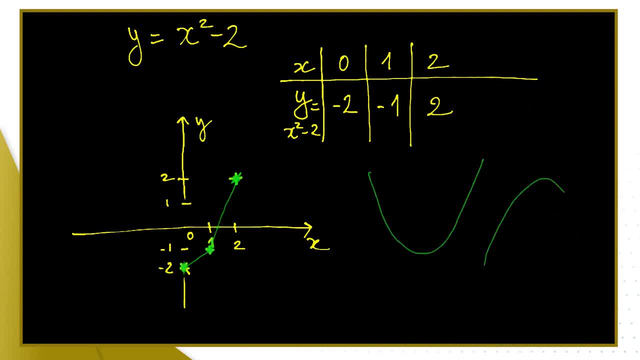 looks like this or like this: It's smooth, it's round and it's got a vertex. It's got a minimal point there or it's got a top point, a maximum point. That's the vertex, And although my sketch in green isn't that great, 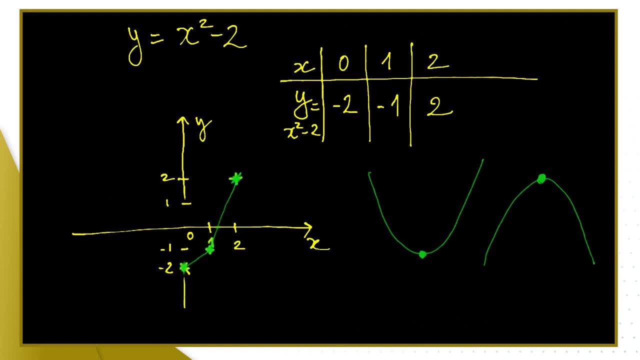 the idea I wanted to give there is that they are symmetrical. The two sides, the two arcs on each side of the vertex, look pretty much the same as a mirror image of each other. So the drawing I have there. it's really not good when you take that into account. To start with, we need a little. 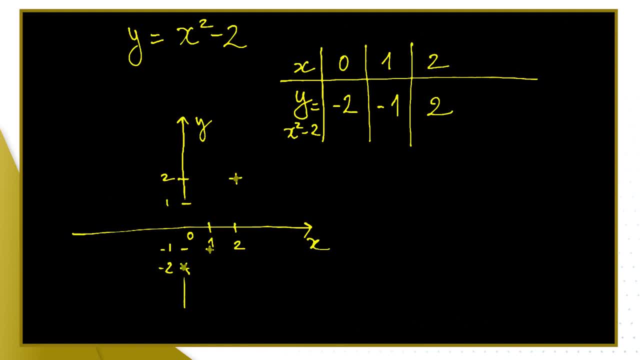 bit more points And now that we see what it looks like, we know we should expect something on this side. So let's give our table of values a few more points. So negative one, Negative one, squared is one. Take away two is still minus one. And negative two for the x Minus two, squared is: 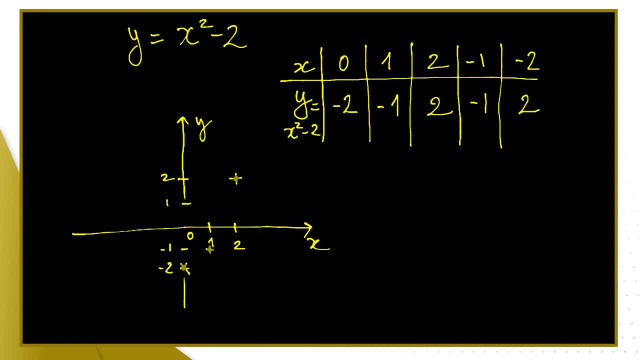 four, Take away two is still two, So marking these points on the graph. So on minus one, I got minus one, And on negative two I've got two. And so to sketch this, I've got a line that goes through all the points And I can adjust to give the impression of: 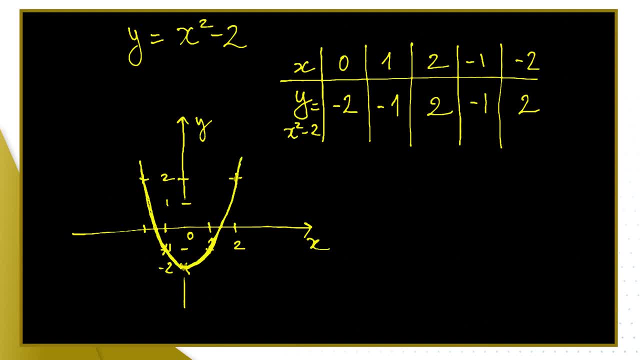 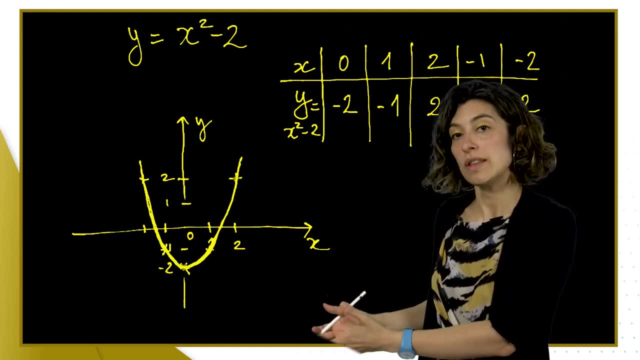 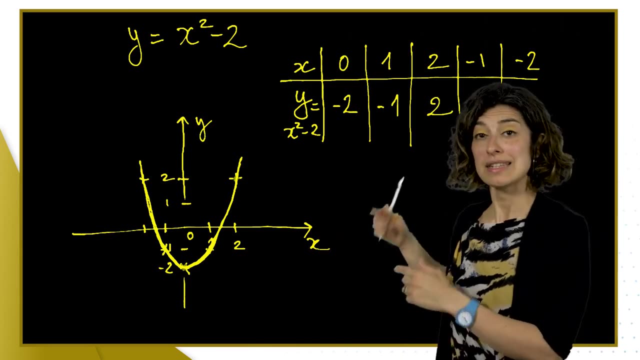 symmetry. Okay, And that is a sketch. It is a plot of the graphs. What's the difference between plot and sketch? I've actually calculated points And the line goes through those points. So that's a plot. A sketch would just give an impression of it, like I did. the earlier drawing of the two. 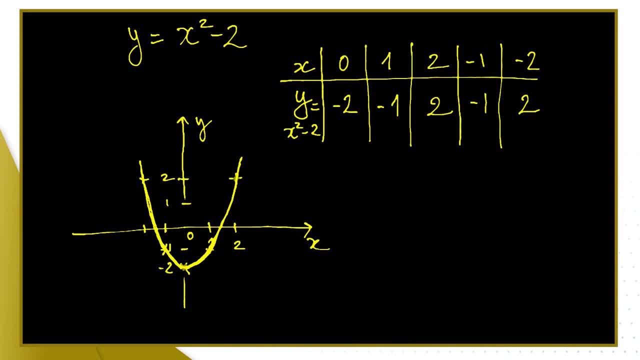 parabolae in green. So that's a plot And that's a sketch. And that's a plot And that's a sketch. Let's look at another one. Y equals two x cubed minus x. Let's have a table of values. Let's try x. 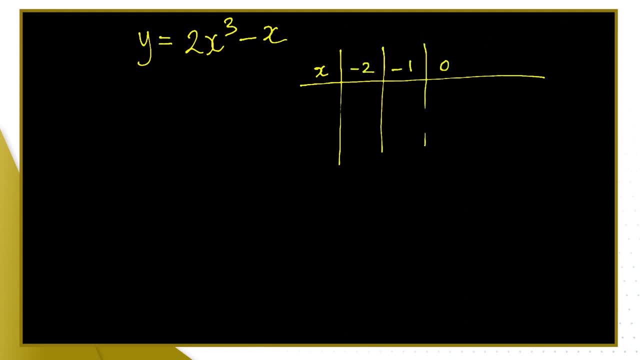 to be minus two minus one, zero one and two. The y value will be calculated using the formula So minus. So let's do two times minus Two cubed. take away negative two, That is minus two. cubed is minus eight times two is minus 16.. 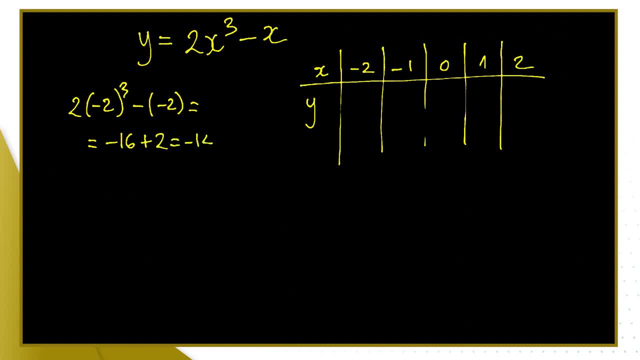 Minus minus two is plus two, So I've got minus 14.. Negative 14 there. Minus one. Two minus one. cubed minus minus one. I've got minus two plus one. That's negative. one For zero. I got zero. 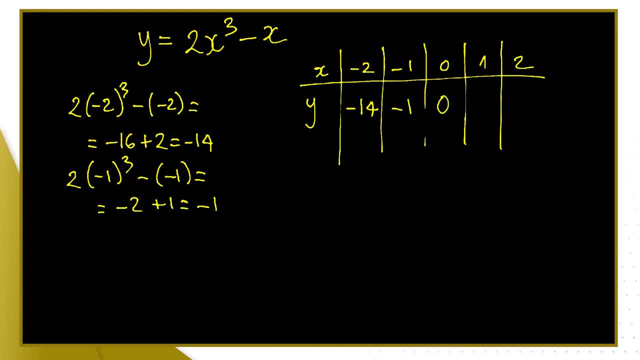 cubed, which is zero. Twice that is zero Minus two plus one. That's negative. one For zero minus zero, That's zero. And the value of one one cubed is one times two is two, Two minus one. 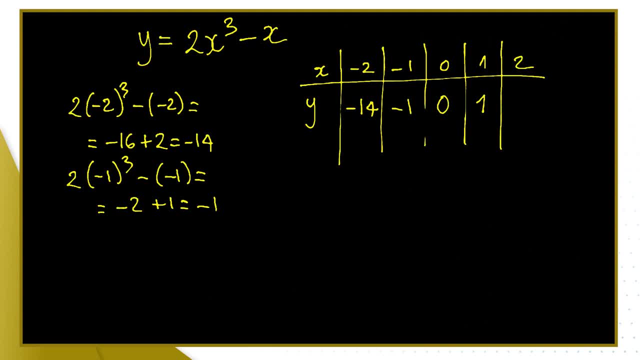 is going to be one And for two. I have two cubed, which is eight Doubled that is sixteen, Sixteen. take away two, That's going to be fourteen. OK, And this graph? it's going to look different from the quadratic. This is a cubic and we can pull it out here Roughly. 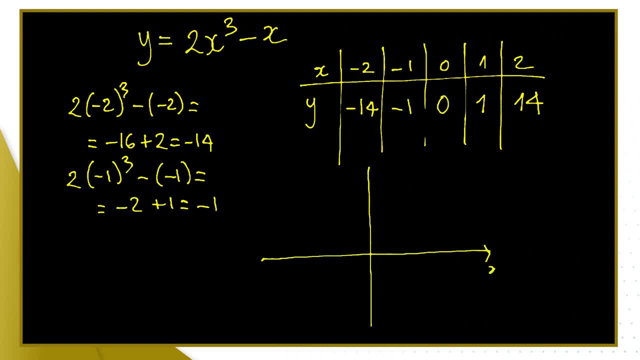 OK, And this graph? It's gonna look different from the quadratic. This is a cubic And we can pull up it here Roughly, it here, roughly it is. I need to pay attention to this scale because, look, I've got values from. 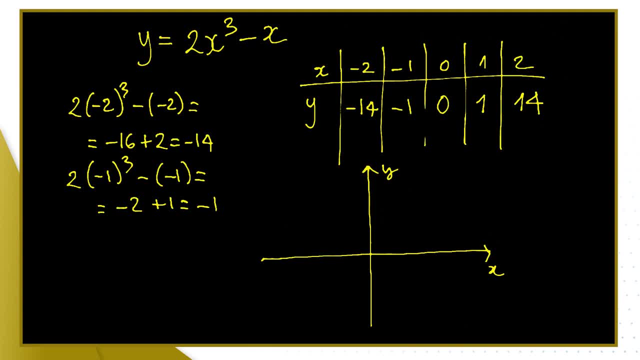 minus 14 to 14 on the y. so I'm going to do that's going to be my minus 14, that's going to be my 14, the same distance, and I've got points 1 and 2 on the x and minus 1 and minus 2 on the x. 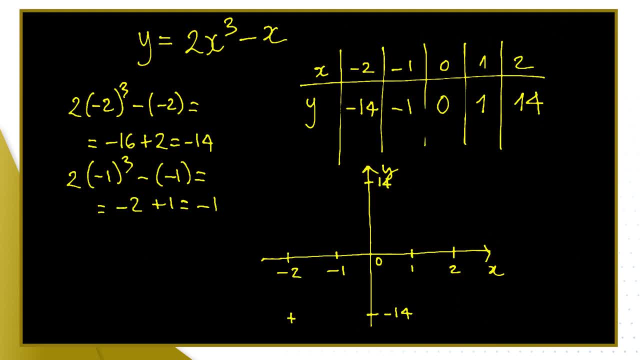 on minus 2, I got minus 14. on minus 1, I got minus 1. divide that vertical space into 14 parts roughly. it's going to be a tiny amount. that's a very mathematical way of saying it, isn't it, I know? and then that's going to be another tiny amount and it's going to be a zero there. 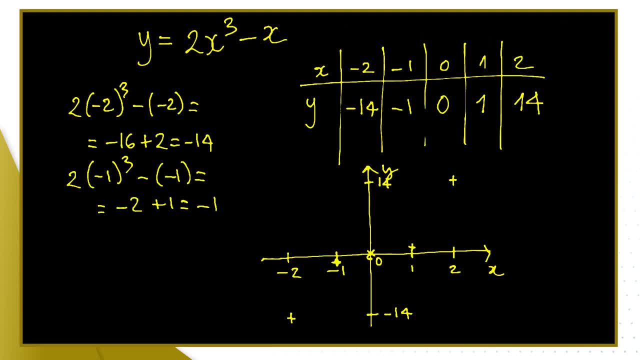 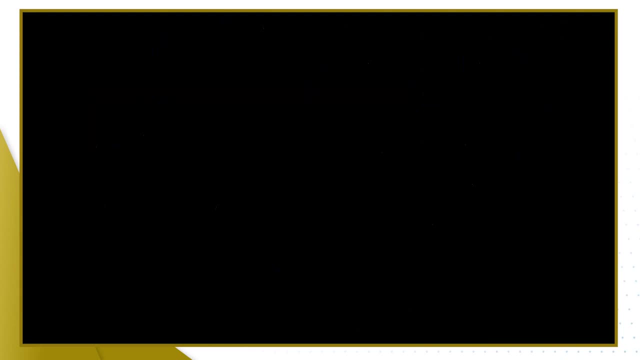 tiny amount and huge amount there and our cubic right that. okay, so that is the curve. y equals 2x cubed minus x. a couple more examples. so y equals minus 2 over x. we'll do a similar job as we did before. we're going to have a table of values and 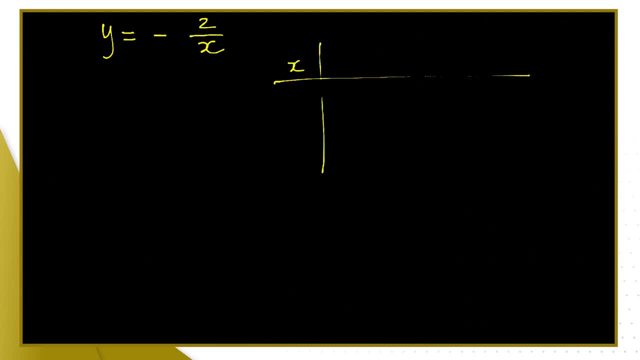 we could start by using: say you have minus 2, minus 1, are you tempted to put a zero there? why is that problem? we cannot do 2 over 0, so we cannot. I'm going to put the zero there. we're going to say it's not possible, it's not defined- okay, it's not defined. and then 1 and 2 and the. 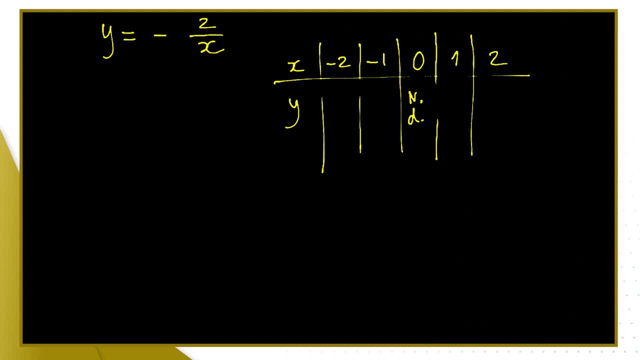 values for that: the y minus 2 over minus 2, that is 1. minus 2 over minus 1, that is 2, and here minus 2 and here minus 1, and undefined. now that doesn't give me enough information to do a decent plot. I'll show you why. 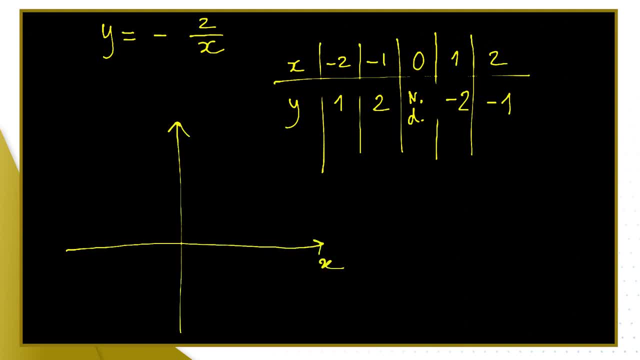 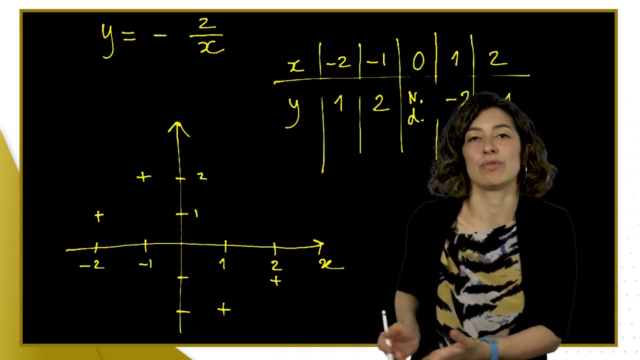 we've got minus 2, minus 1. I've got the value of 1 there and the value of 2 there. so 1, 2 and then that's mine. so that is 1 and 2 and I've got this value, this value. we've got all of those two points. what's going on? what happens near 0? near 0, because it's. 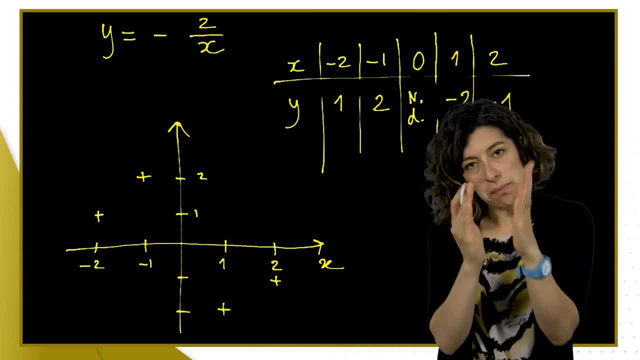 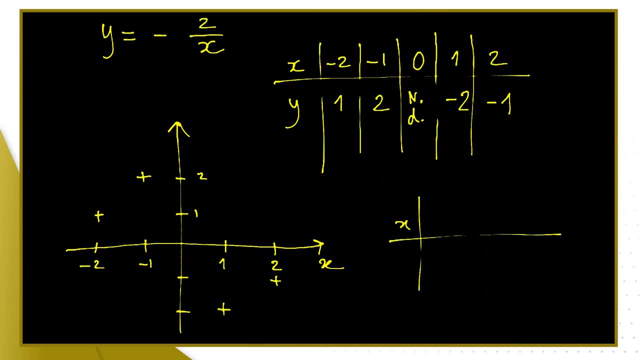 undefined. we need to have more values between the minus 1 and the 0 and between the 0 and the 1, so we actually need to have a decent approach there. between minus 1 and 0, let's say we do minus 3 quarters a half and minus a quarter, minus 3 quarters, minus a half, minus a quarter. 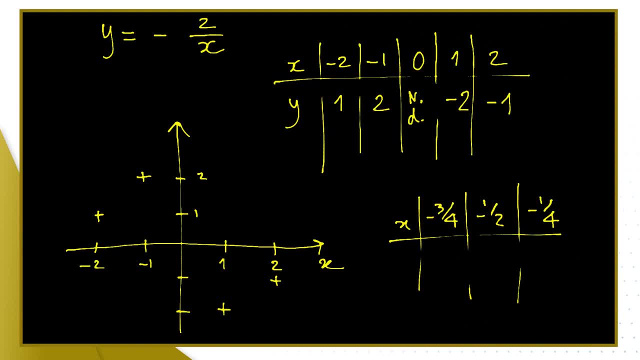 if we do minus 2 over that, let's do the sums here on the side: minus 2 over minus 3 quarters is positive 4 over 6, which is just 2 over 3. so that's two-thirds minus 2 over minus a half is going to be 4 and minus 2 over minus a quarter is going to be 8. 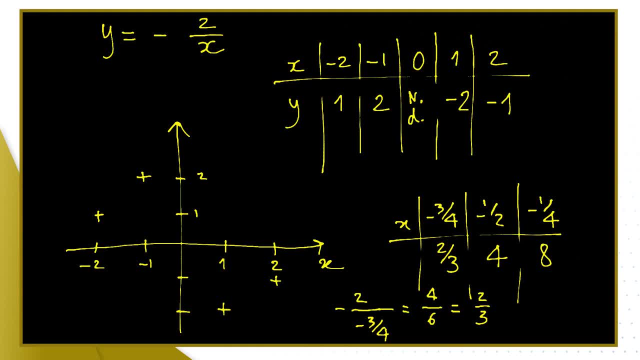 and then take the same times. that way, so 1, 5 divided by 3 times 2, over 7 és 10. so yet again, when we can, students or friends and others askЗ the the vertical axis, So the table of values. it's really important because it 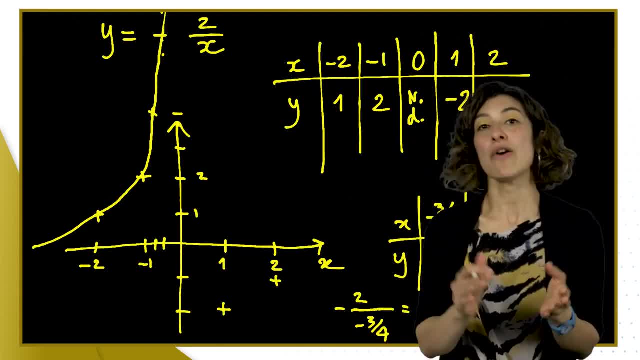 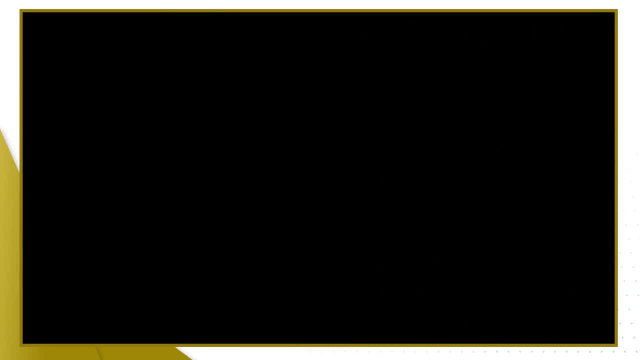 helps you plan what the graph should look like. So you can now fill in the gaps and put more values between minus 1 and 1 and you'll see the behavior. I'll just sketch it on the other page. What you should expect is to have a curve. 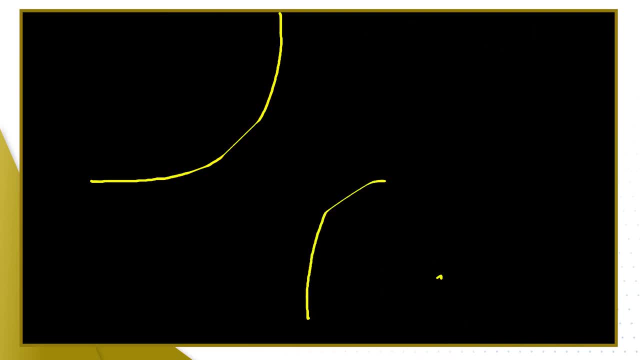 like this, that looks like this curve, is called a hyperbola. You don't have to know this, but this is a hyperbola and the x-axis goes over there and the y-axis goes over there, and this bit here isn't looking very good because you. 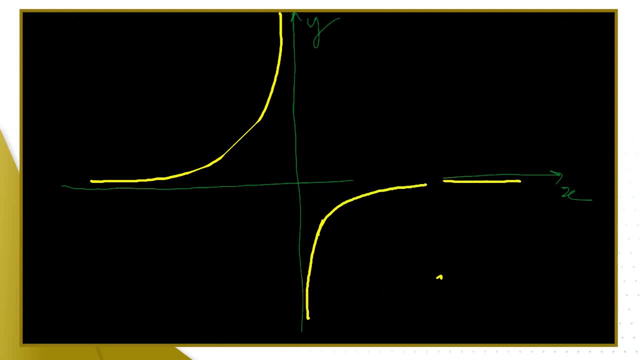 shouldn't really ever cross the x-axis, You shouldn't even touch. So the graph should look like that, with nothing happening on there, On the vertical line, through the origin. Now that brings us to another concept that we need to cover, which is the domain of a function, This function, 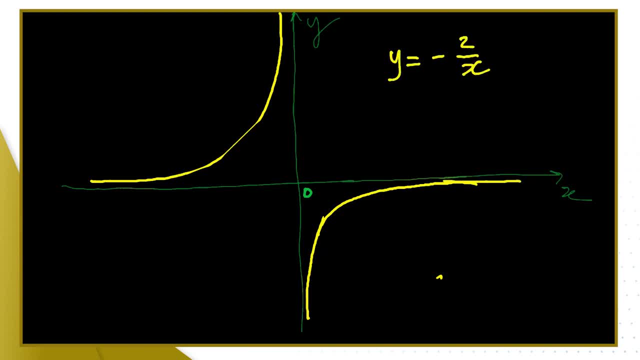 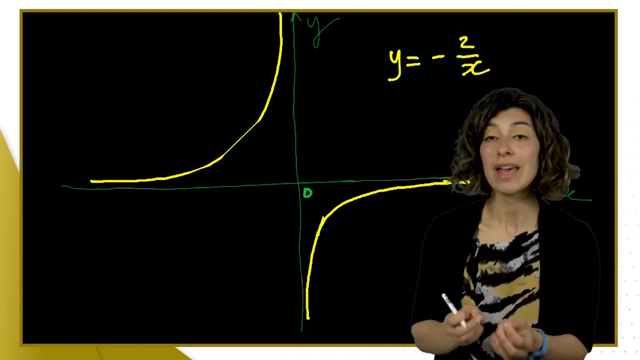 y equals minus 2 over x. this function cannot be calculated when x is 0. So x equals 0 cannot be part of the values we use. The domain of the function are all the values of x that we can actually use, and x isn't one of them. 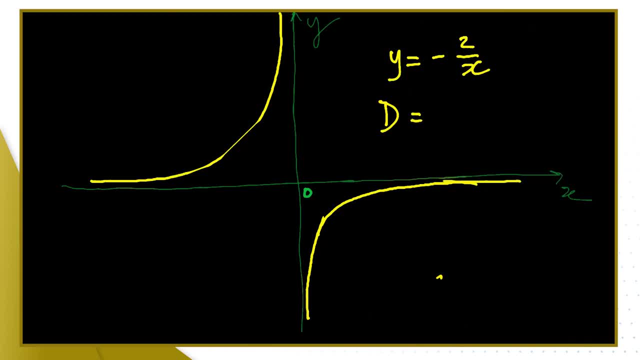 So I'll say that the domain is going to be everything except for number 0. So that's going to be minus infinity to 0, union with 0 to infinity, or you can call it r, as in all the real numbers, except for the point 0. So that's the. 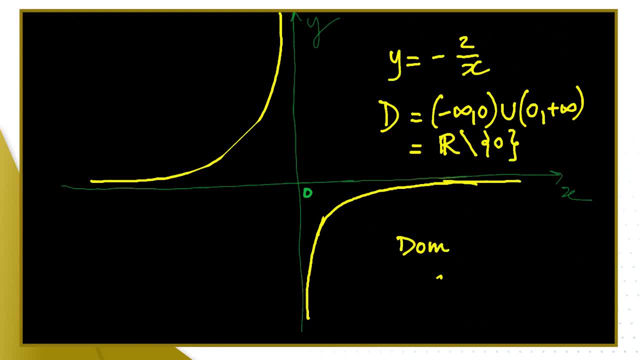 domain of this function. How do we calculate? Well, we look at the expression and we think: what values can I not put in x And you take those out of your domain? Say, we've got y equals square root of x, which I will introduce it to the function notation as well. I can write it. 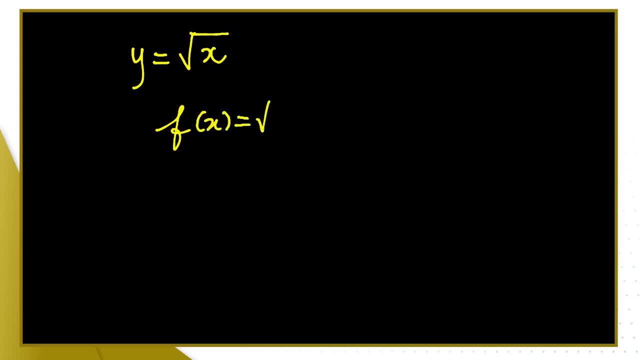 instead of that saying f of x equals root of x, and I say that y is a function of x, So y equals that function of x, So this is a function of x. Over here I'm telling you what the expression is. Here's another way of. 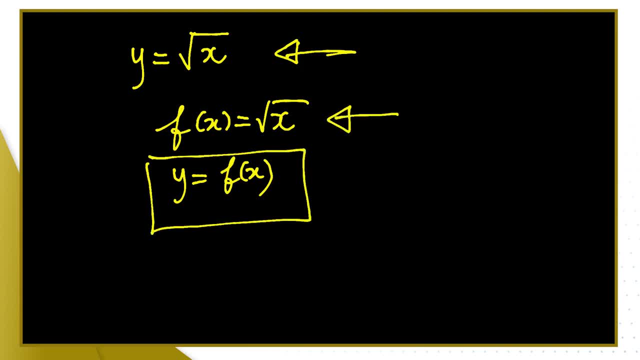 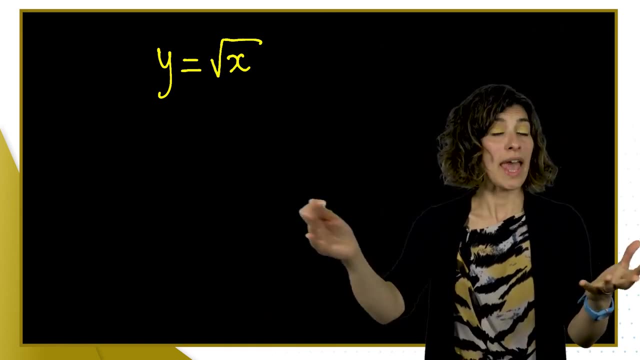 doing the expression, and here I'm just saying y is going to be calculated as a function of x. Now, so with y equals root of x, where are the values of x that cause a problem? Well, what values of x can you calculate? the square root of Any value that is? 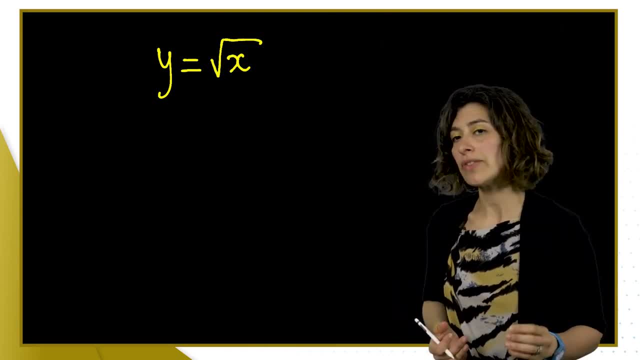 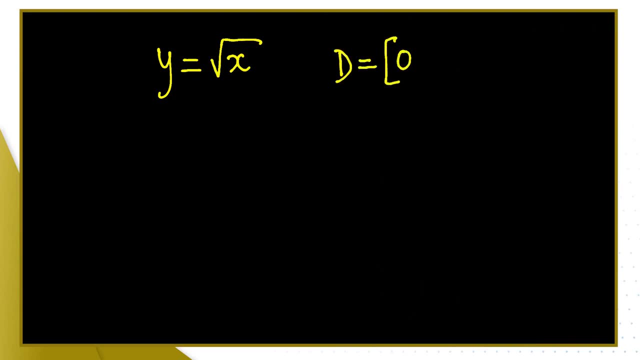 positive and 0. So negative values of x cannot be in the domain. So the domain is going to be just the positive numbers and 0. You can write it that way or you can write it as the real numbers, the positives and 0.. So positive and 0. 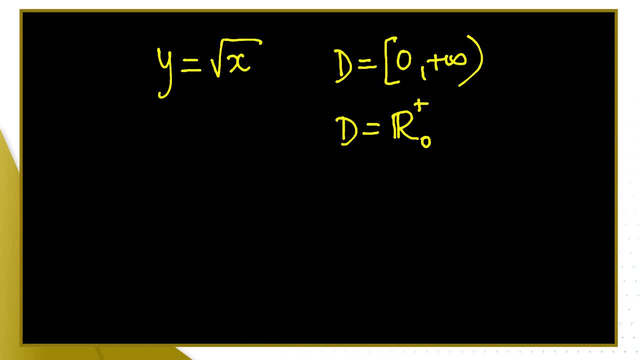 real numbers. That's the domain And this function. that means your table of values would incorporate positive values and 0, and I'll give you a sketch. That way, And the value for 1 is 1.. Okay, and nothing on the left hand side. 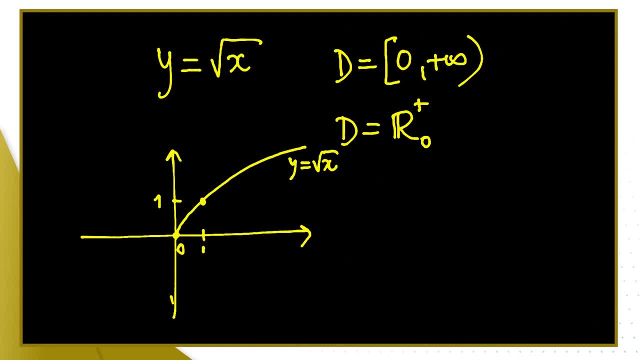 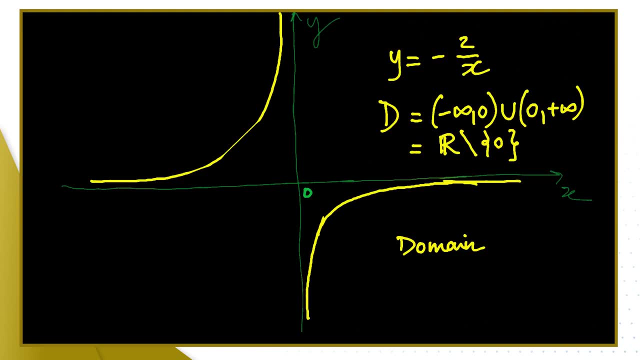 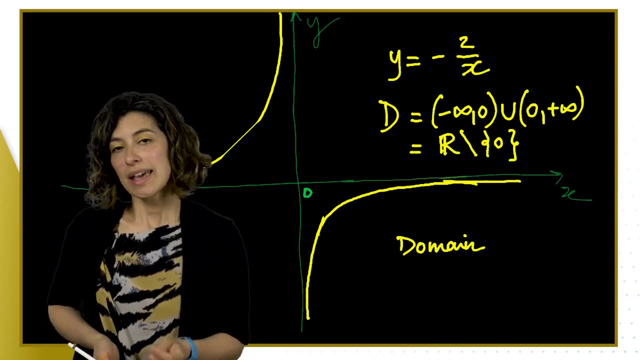 because there's no negative numbers in the domain. I want to go back to the function we saw earlier, this one here, That line that I said, that the vertical line for the origin where there's no graph, that is called an asymptote, Not a. 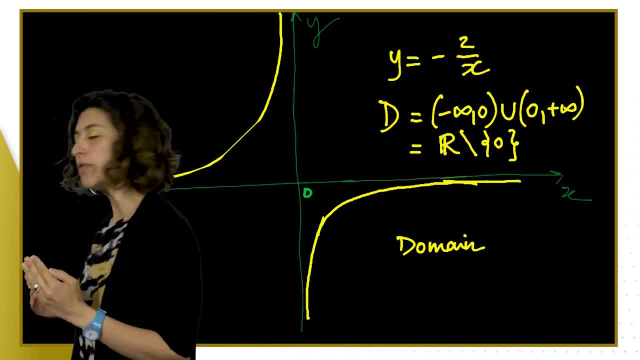 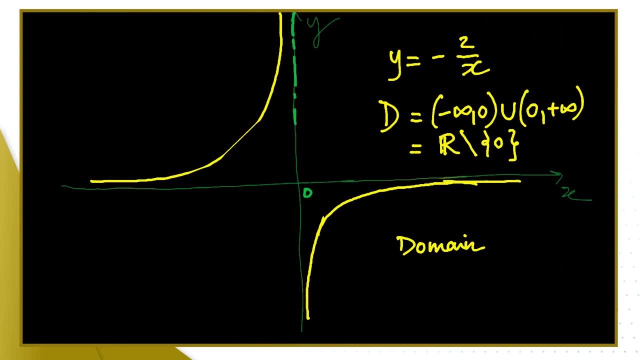 graph, not because there's no graph, but because the curves of the graph really, really want to touch that line. So this line here is the vertical asymptote for this graph, Because the two branches want to approximate it, One on the left and one on the right. 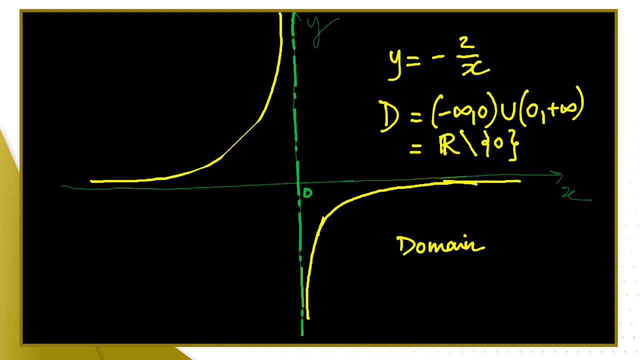 This graph has even another asymptote. It has a horizontal asymptote where the axis is: Because, again, as you make values of x larger and larger, or larger and larger, but negative, the values of y are going to approximate 0. And so they're. 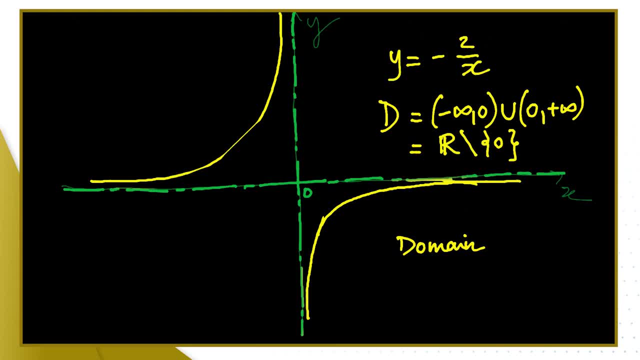 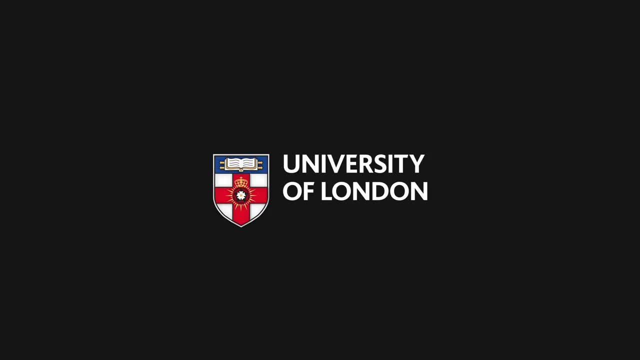 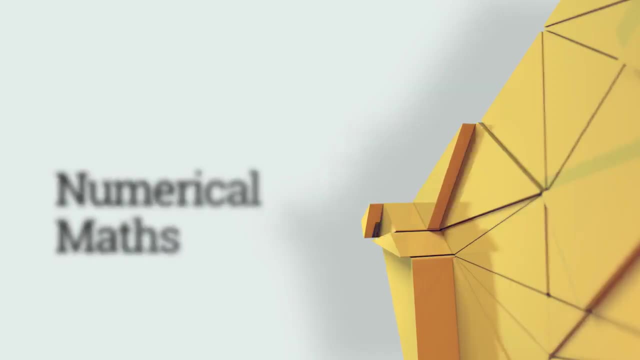 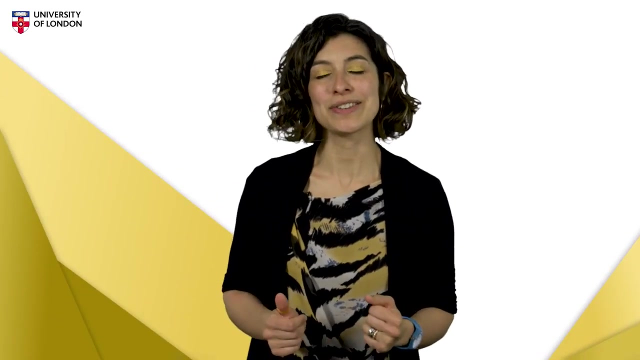 going to, they're trying to, they're trying to lie down on the axis, but they're just not getting there ever. So that's an asymptote. We've got a look at a series of examples of plotting graphs by hand. Let's bear in. 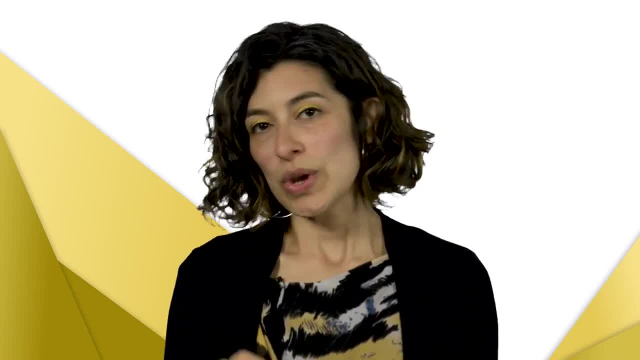 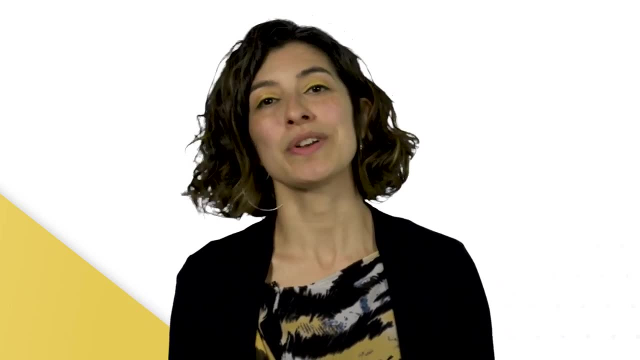 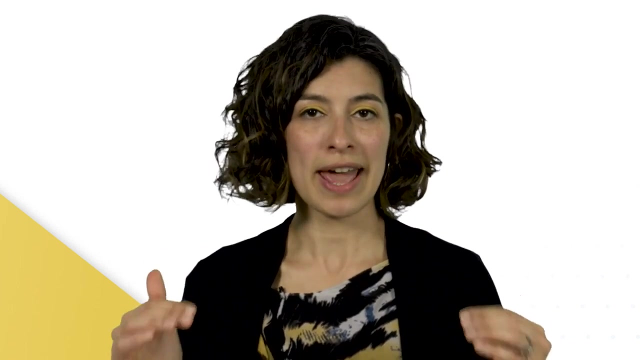 mind a few key principles. We need to have correct labelling of the axis. We need to have correct labelling of any points we want to highlight. The scale needs to be consistent. You can have a different scale for x, for the x-axis and for the y-axis, but you also need to have 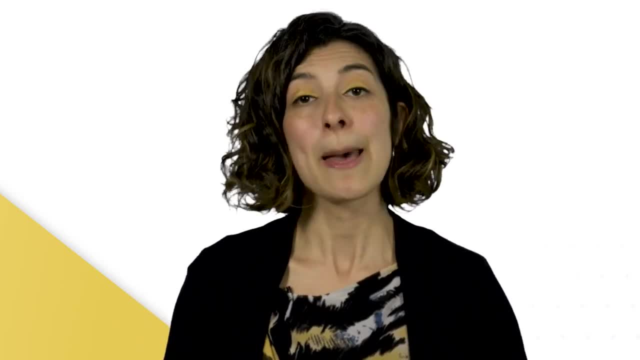 a different scale for the y-axis and for the x-axis. You need to have a different scale for the x-axis and for the y-axis, So the scale needs to be consistent. You can have axis that it's fine, but the scale you use in one axis need to be consistent across the whole drawing. 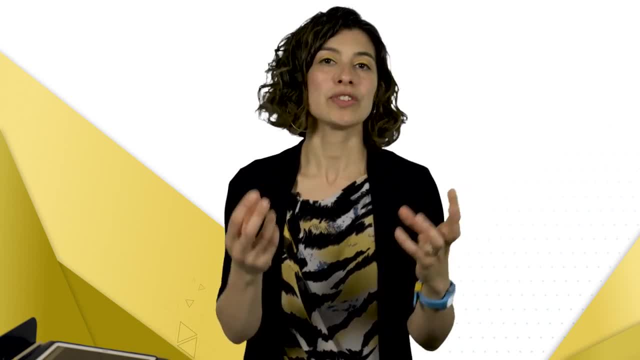 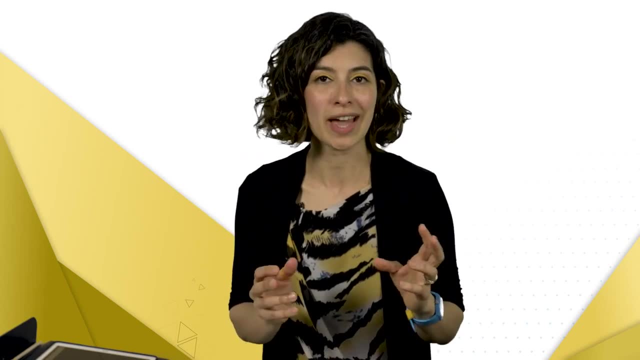 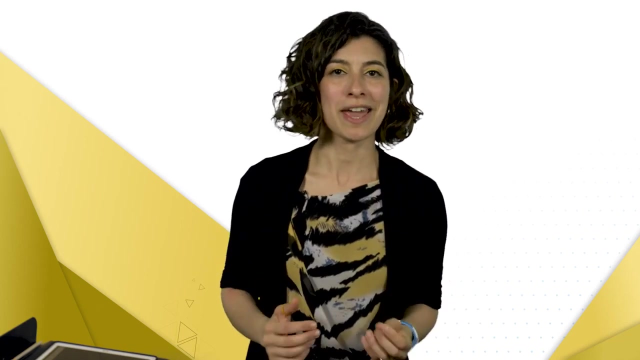 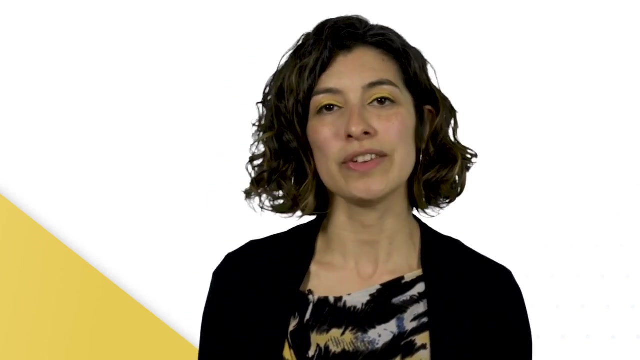 if the function has symmetry, you are to highlight that symmetry. even if your values aren't absolutely accurate, it's important that you highlight that you understand that the function has that symmetric behavior, or that it has an increasing or decreasing or a flat behavior. any other key features you can be aware of of a function are to be highlighted in all these. 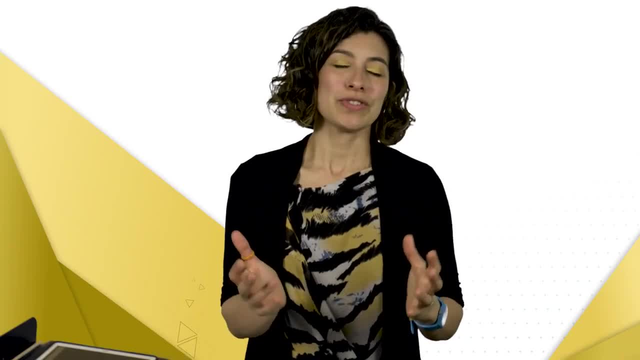 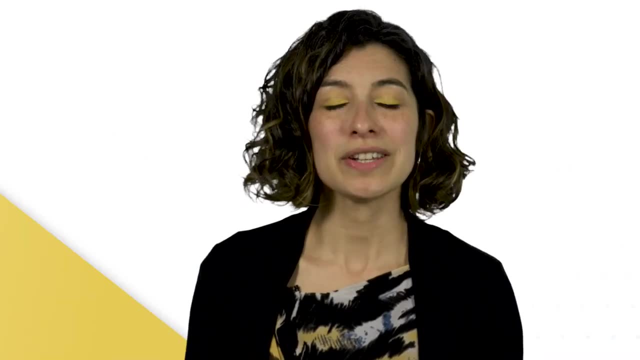 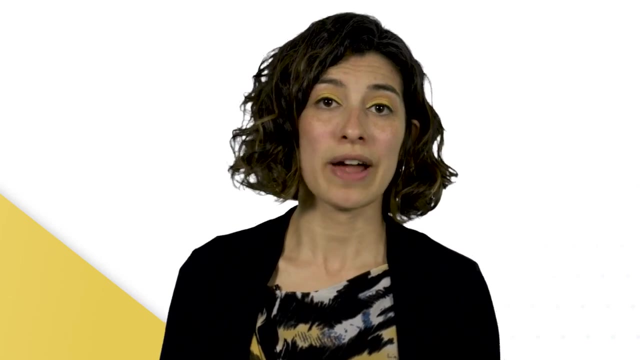 plots and sketches you do by hand. i would like you to plot graphs by hand once you've looked at a few examples of them plotted in a plotting software. further to that, do build tables of values to make accurate plots of graphs by hand, and then you'll build intuition and experience to 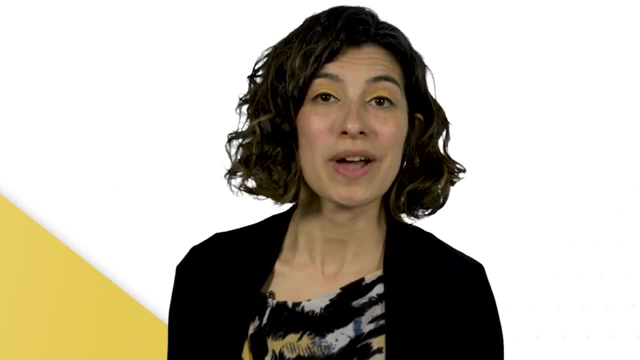 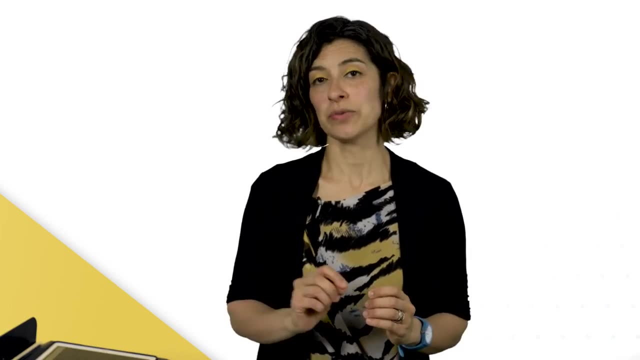 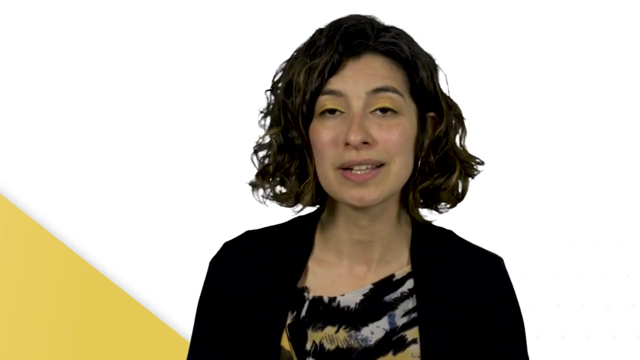 choose values for your table in a much more efficient way and sketch graphs with very little information. bear in mind that not all functions have one expression. some functions have expressions are broken into branches. those are piecewise functions. we'll look into those as well, but in the end, all these pieces are going to be built from types of graphs that you're. 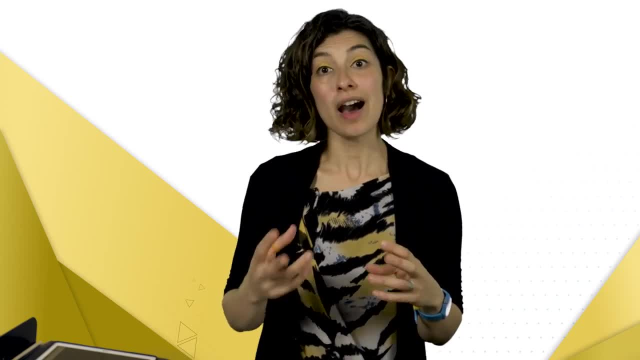 going to study individually. in computing, you may have other special functions like absolute values and other special functions, and that's why you take the best part of this video to the next one that you're going to study individually. in computing, you may have other special functions like absolute values. 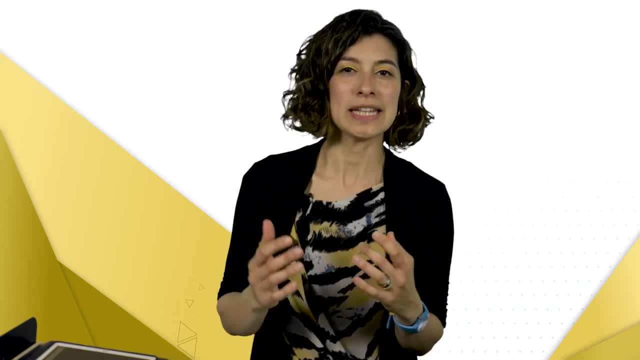 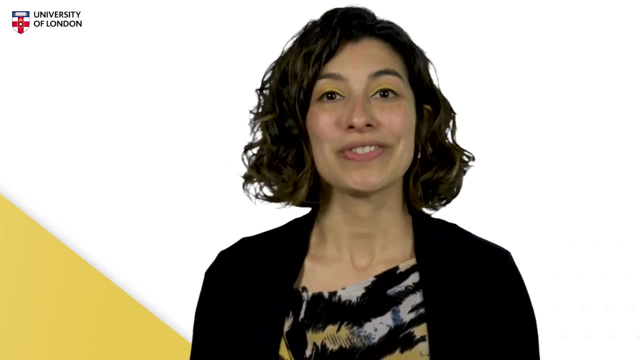 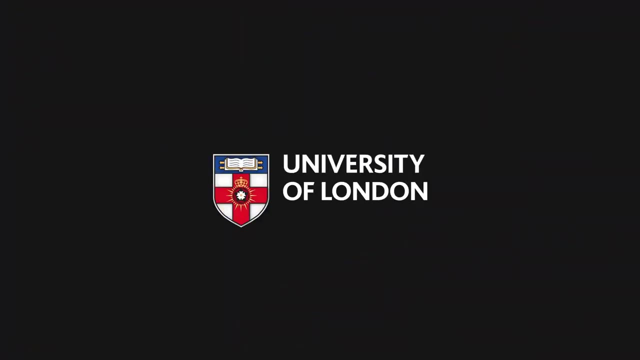 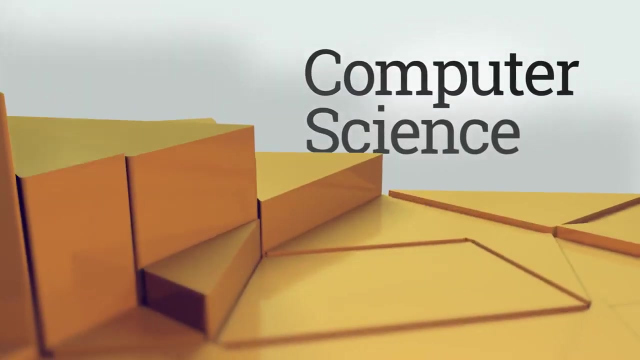 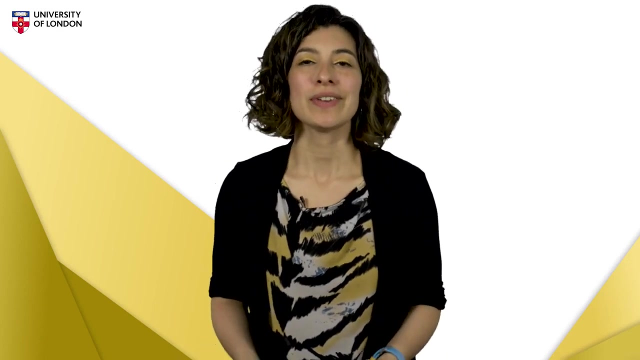 and step functions like ceiling or floor functions. I invite you to explore those as well. The skills you need for those are the same skills we're going to study with all the other functions we'll look at now To plot straight lines, we can start with the expression. we can look at what the slope 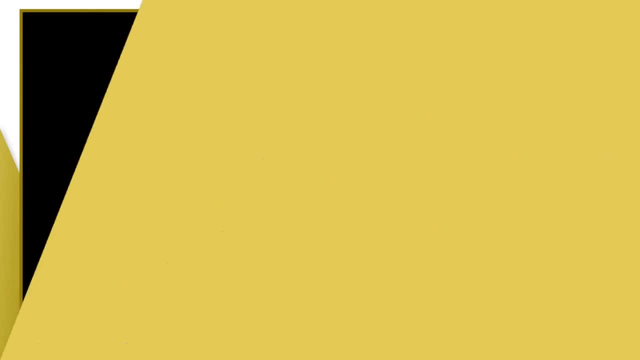 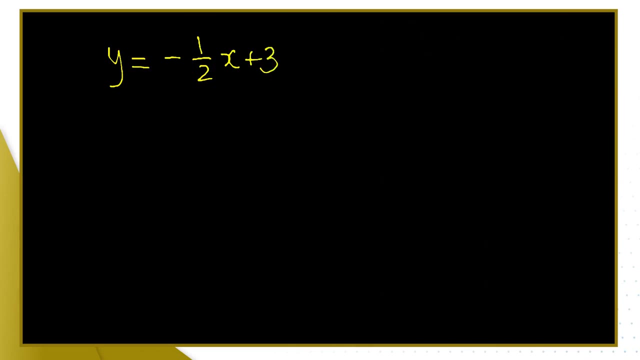 might be, and the intercept Say: we have y equals minus a half of x plus 3.. We will write a table of values but before we go into the table of values from the numbers in front of us, we have the slope, this minus a half, and we have the y-intercept which 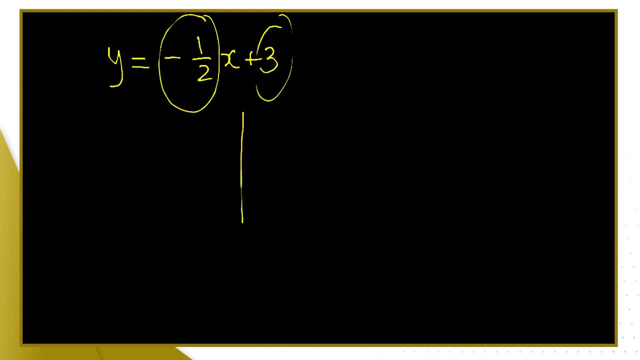 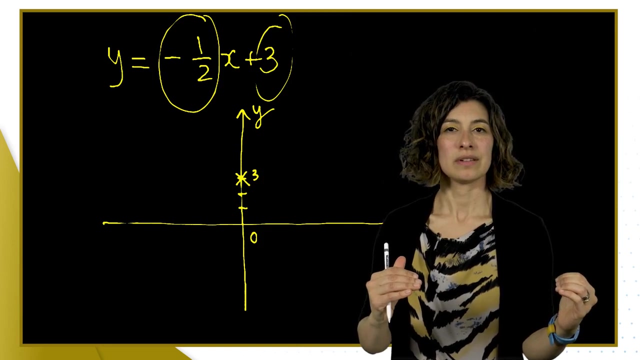 is 3.. That means we know a little bit more about our function. We know that the graph cuts the y-axis in that point and we also know that the slope is negative 1 half. I move 1 in the x-direction. I move minus a half down in the y-direction. Easier if we 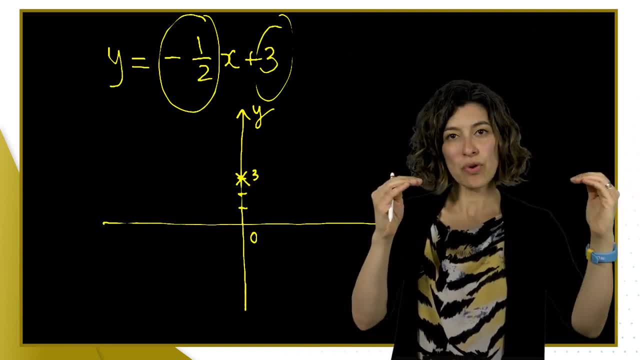 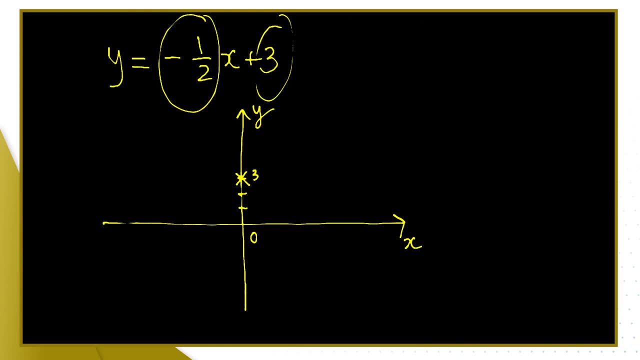 think of: if I move 2 in the x-direction, I move 1 down in the y. So from that point of coordinate, 0,, 3,, the intercept: if I move 1, to move 2 down, I move. 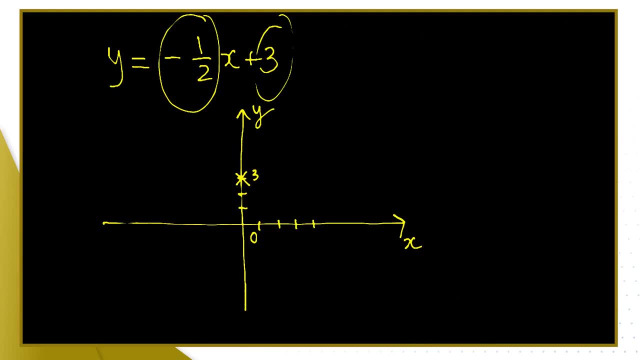 2 up to move 3 down. I move 6 down, So I should expect that point to be the point in the straight line. Let's check if that is true. Table of values. when x is 0, we've got. 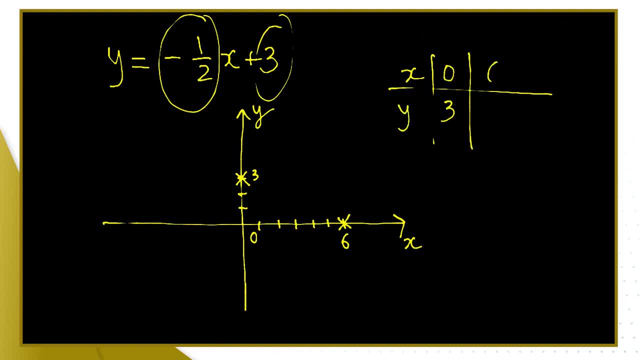 3 to y, set when x equals 6, I've got. I've got minus half of 6 plus 6 in the x-direction and I move a straight line down and I track my difference. for me that's 6, so yourself. 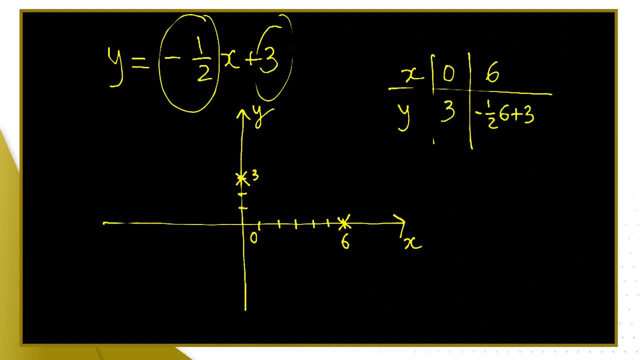 2, 2 declare 2.. Minus half of 6 is minus 3.. Minus 3 plus 3, it is 0. So our geometric thinking paid off And the straight line will be just a straight line that joins those points. 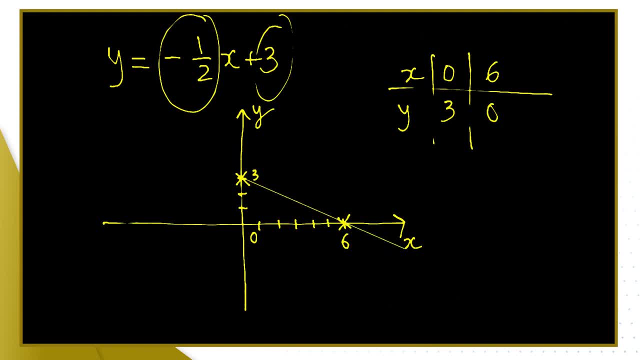 And we have: y equals minus half x plus 3.. So here's an example where you can use the geometrical information to speed up your plotting and choosing your values for the table. Now, we had a special number, a special value there. 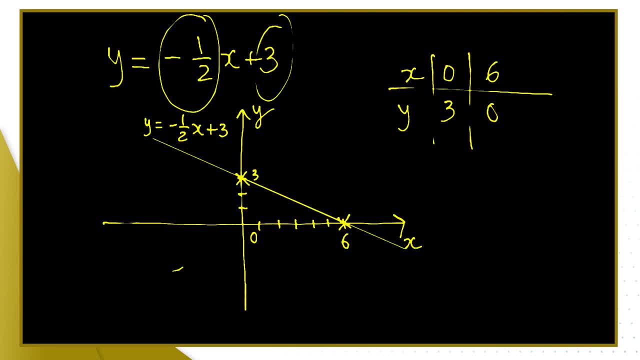 We had on that graph a point where the straight line crossed the x-axis. That is called a zero. A zero is a value of x that gives 0y. That's why we call it a zero. So it's a point where we cross the x-axis. 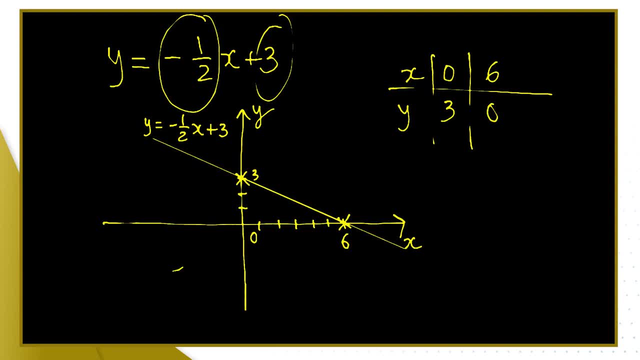 Now what if the geometric information didn't allow us to calculate that point? It's not a problem. We have algebra. So in this example, to calculate that point, that x equals 6, I could have just said: I want to know when y is 0.. 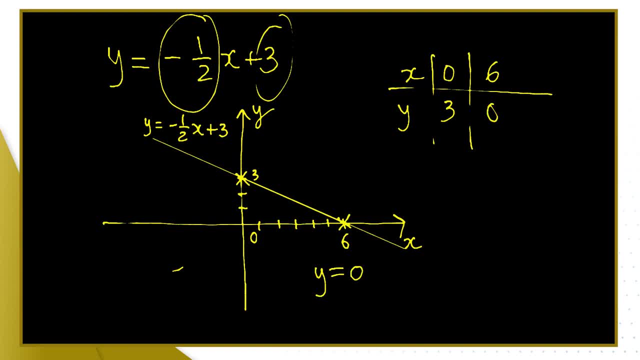 When y is 0 in that expression That means that I want minus one half of x plus 3 to be 0. That means I'm just going to run a bit of algebra on here to solve the equation for x. So I subtract 3 to both sides. 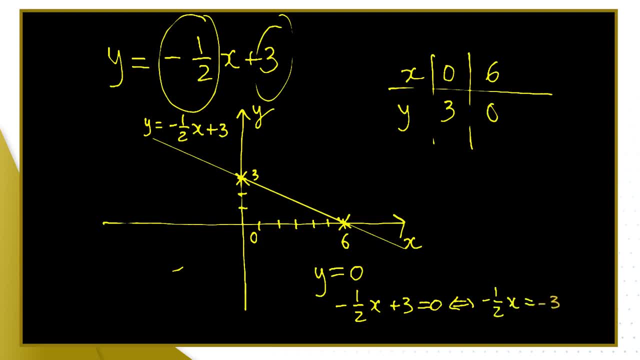 I get minus a half of x equals minus 3.. I now multiply both sides by minus 2. And I get x on this side and 6 on the other. Done, That was the value of the zero, The value of that point there in the graph. 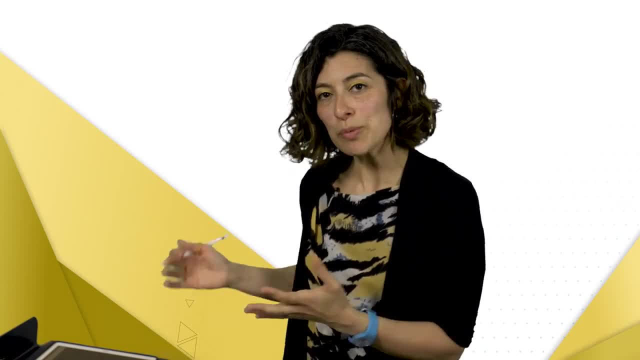 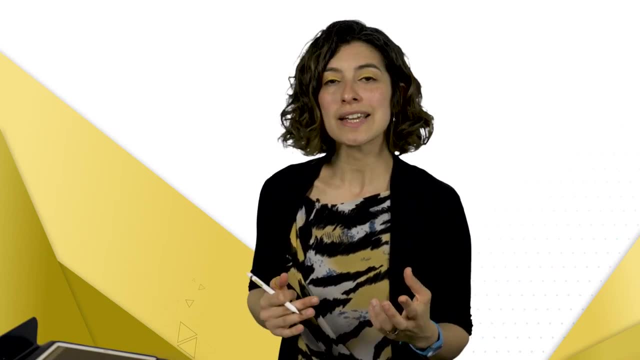 So, in summary, you can use geometrical information to help you draw the graph and speed up the choice of values for the table and what the graph is going to look like. But you can also use algebraic tools like solving an equation And to find the zeros. 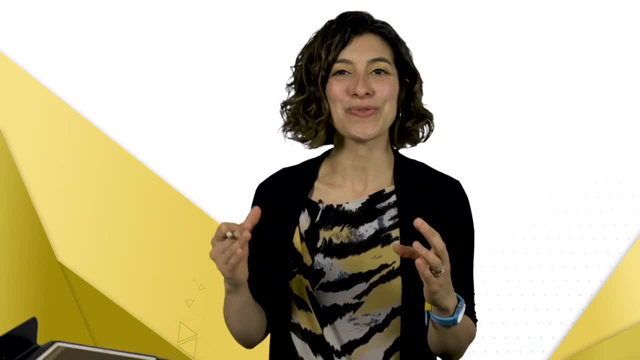 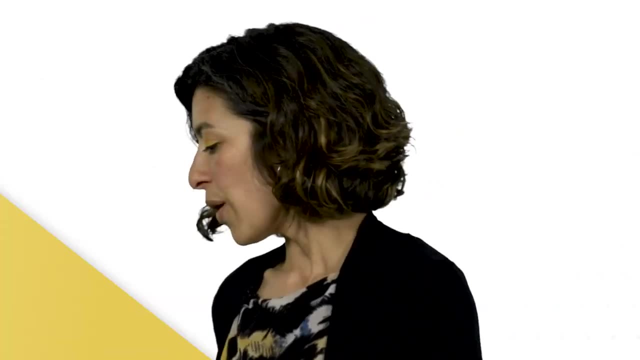 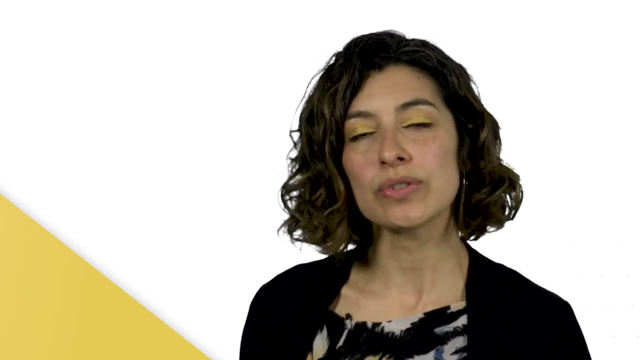 Or in this case The 1, 0. You solve the expression of the function equal to 0 and solve it for x. Now we have the y-intercept, We have the 3 on the y-axis. Could we have solved that one algebraically? 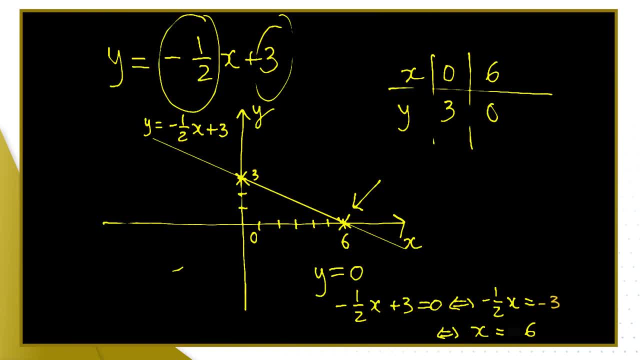 Of course, In that case we're not looking at y equals 0. We are looking at x being 0. So that point there has coordinates 0, 3. The x is 0. So we want to know in that expression, when is x equals 0.? 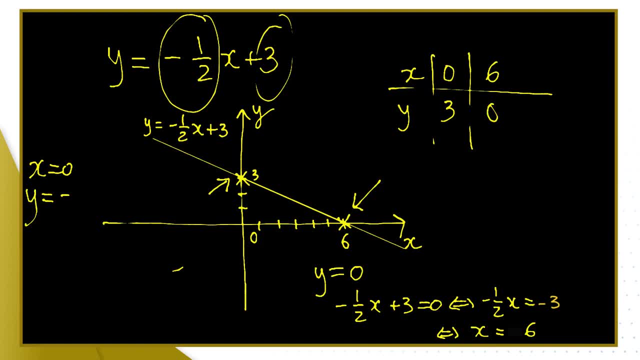 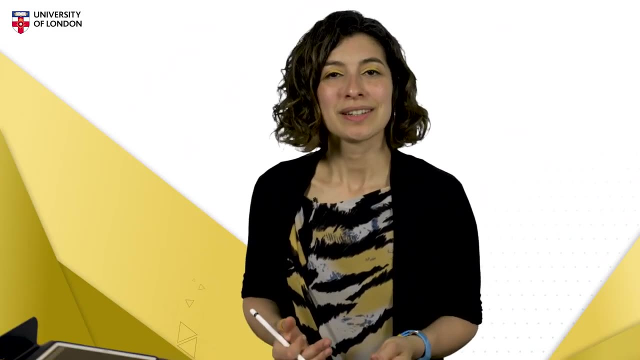 Well, we substitute x equals 0 into the expression, So minus a half times 0 plus 3.. And it gives us the value 3, as we knew already, As we knew already there on that table of values. So both those points are obtainable by algebraic methods. 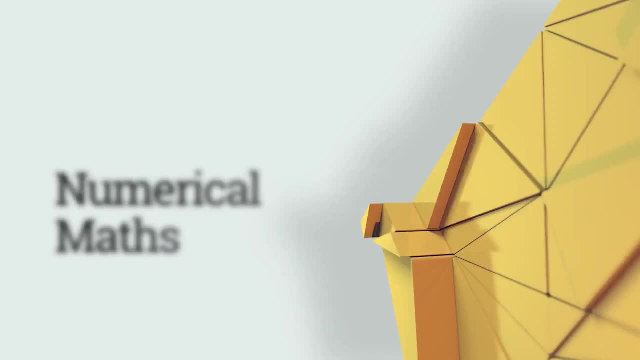 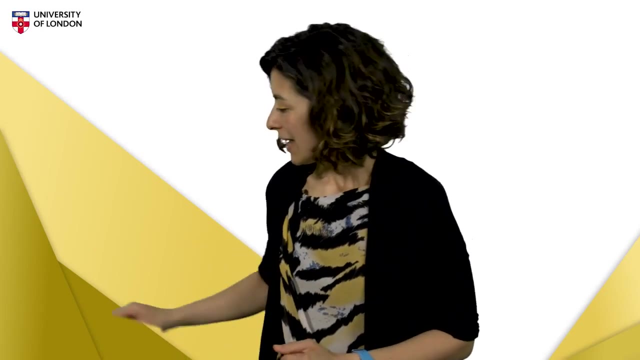 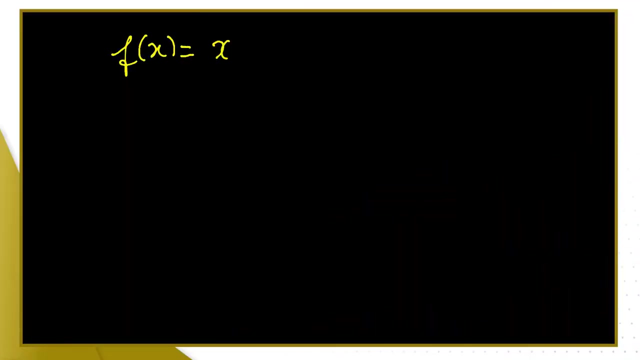 We're going to plot quadratics. Here's one We have: f of x equals x squared plus 3x. That just means that y is going to be x squared plus 3x. Okay, We're going to plot the graph of y as a function of x. 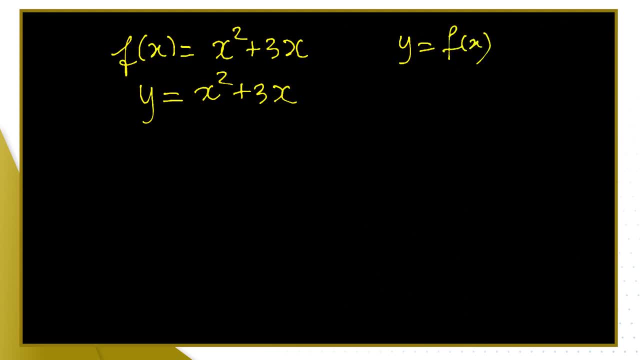 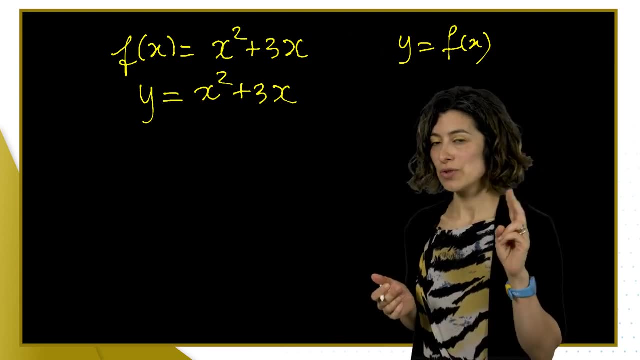 Given that, Given by that expression, Now it is a quadratic, because the largest, the highest power of x is x squared, So that's power 2. That's a quadratic Inspecting the function things we can look for straight away. 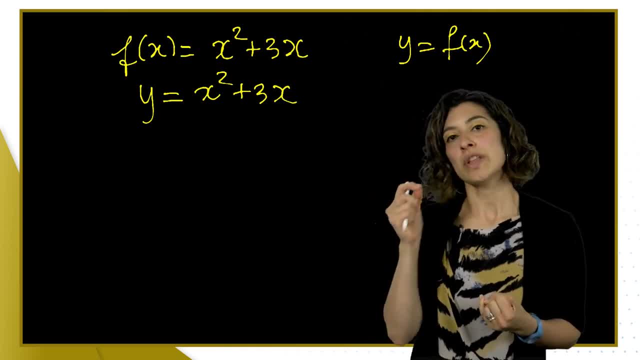 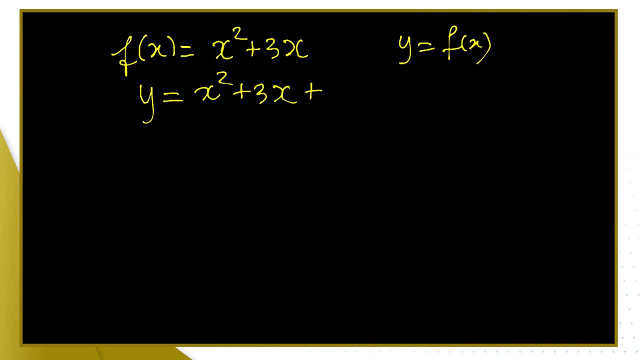 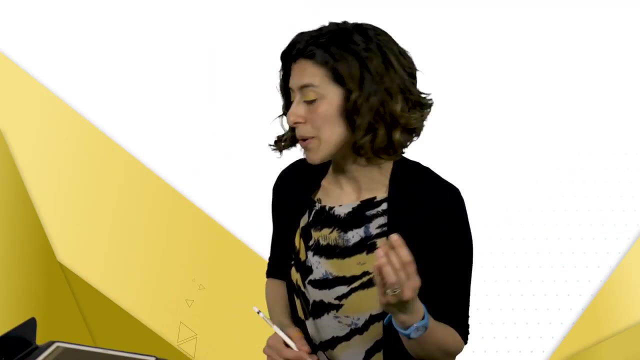 What's the y-intercept? What is the individual number? This function has a plus 0. there The independent term is 0. So that means the intercept is 0. That means it crosses the y-axis at value y equals 0.. 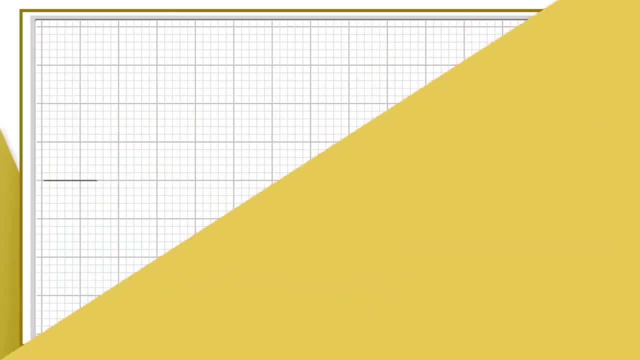 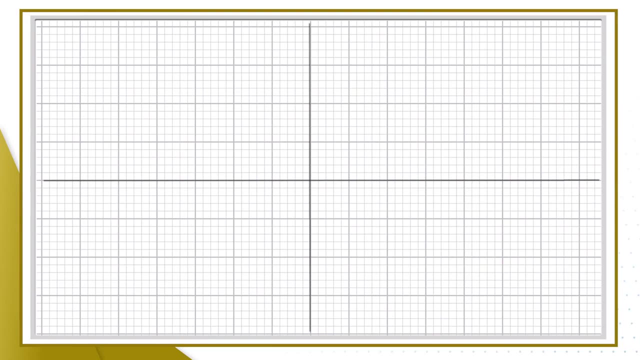 That means you're not on the graph which I'm going to draw here. I'm going to draw my axis, That's my x and my y. That means that it's going to go through the origin: When x is 0, y is going to be 0.. 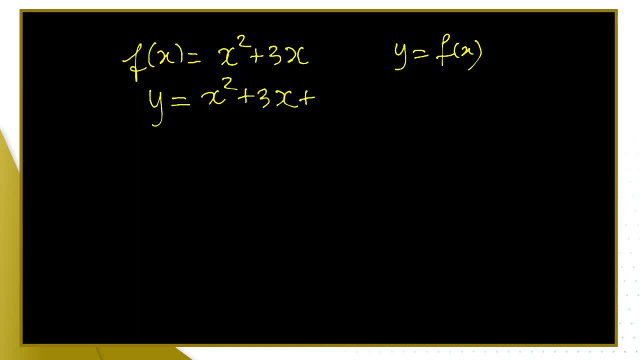 So that's the intercept That we got from the fact That there is no independent term here. So there is a plus 0. So we got that. Now what else can we take from there? Well, we need to understand what the shape is. 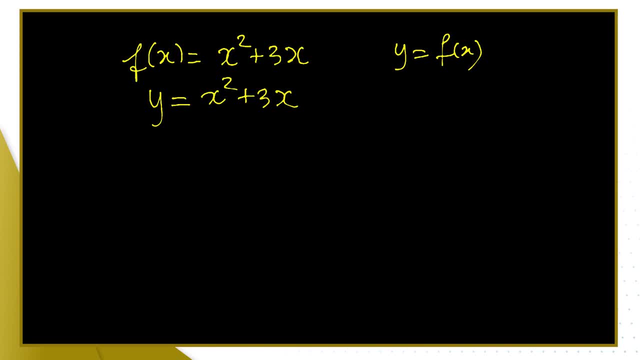 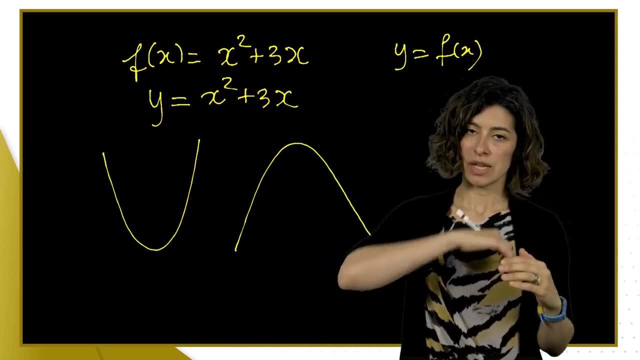 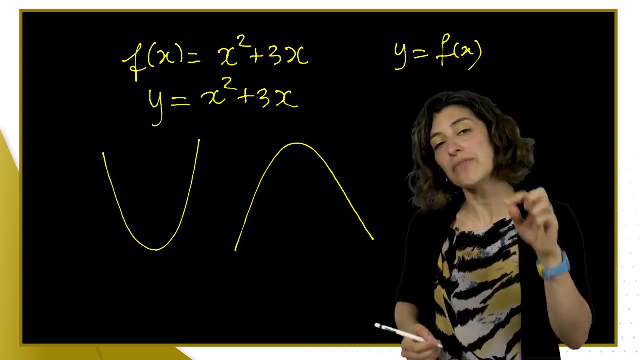 And we know from experience that it's going to be a graph like that or like that. Now, the happy parabola or the sad parabola, is all to do with the sign of the coefficient of x squared. That means the sign of the number multiplying by x squared. 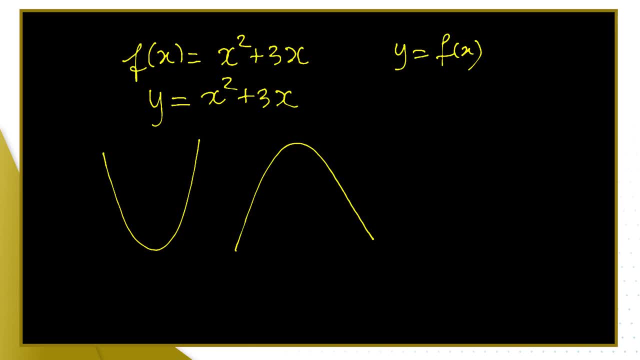 In this case we got x. squared is the leading term And x squared has a 1, an invisible 1, multiplying there That's a positive number. So this is the type of parabola we expect to have. That parabola has a vertex: the lowest point. 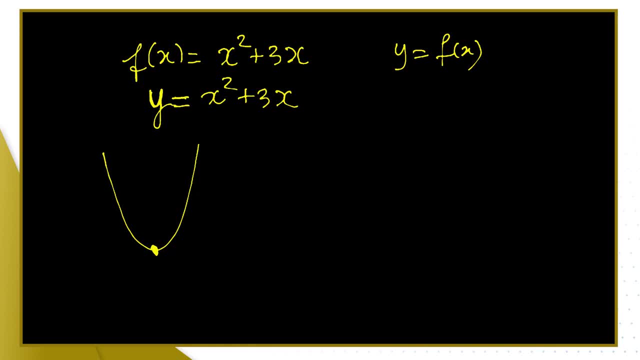 So we'll be looking to finding that point And this graph may or may not cross the x-axis, may or may not have zeros. Let's start with the zeros, Looking at that expression to find the zeros we'll be looking at. solving y equals 0.. 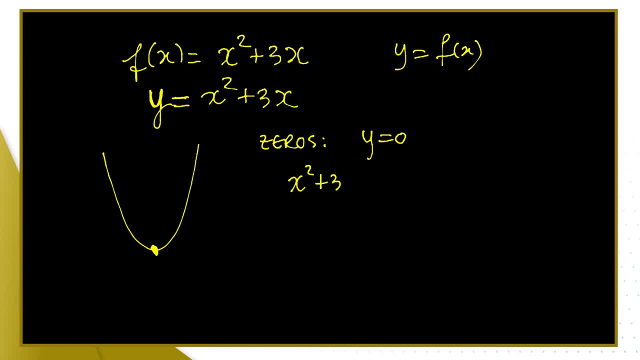 That means we need to do: x squared plus 3x, which is the expression for y, equals 0.. Can we solve this? Yes, we can. There's many ways you can do that. One can be by factorizing, if it's possible. 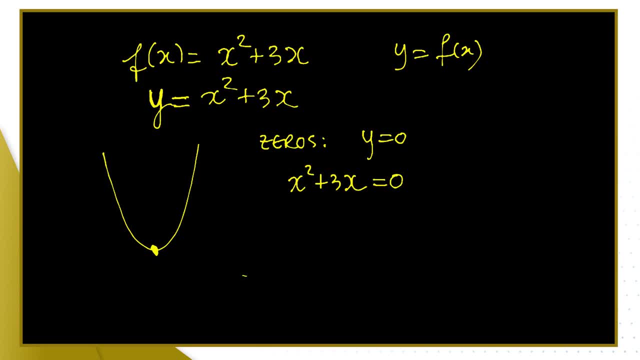 Or you can use the quadratic formula. The quadratic formula applies when you have a quadratic with coefficients, as I'm writing here. so a- the coefficient of x squared, b the coefficient of x and c the independent term, And solving that to 0 means. 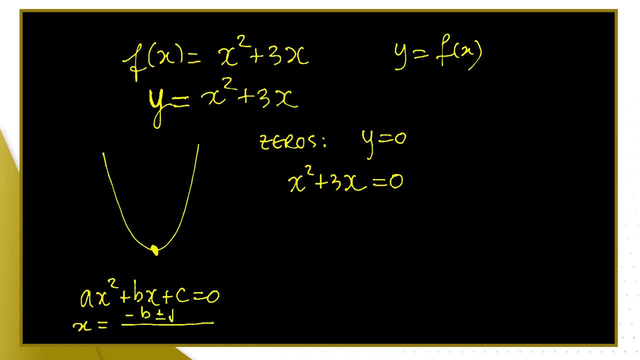 we use this formula: minus b, plus or minus the square root of b squared minus 4ac, all inside the root divided by 2a. In this case, a is 1,, b is 3, and c is 0.. 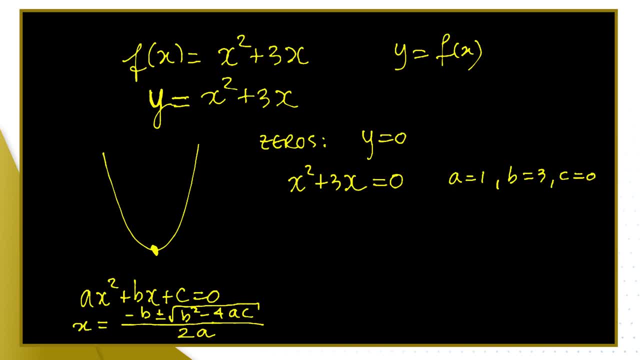 The independent term is 0. We had a y-intercept of 0. Now we can do that and apply it to the formula. So we could do: x equals minus b, which is minus 3, plus or minus root of b squared. 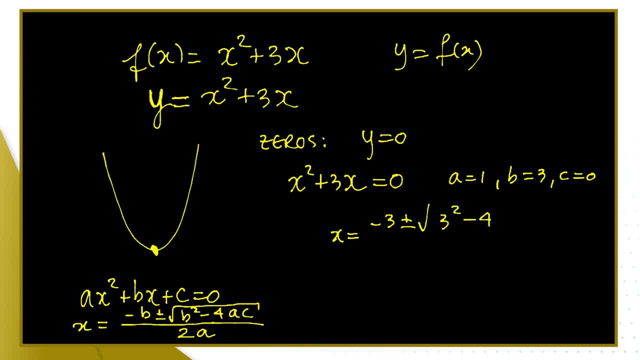 so 3 squared minus 4, times a, which is 1, times c, which is 0. So this bit disappears as 0, over 2a, which is just 2.. And we could solve and simplify that. 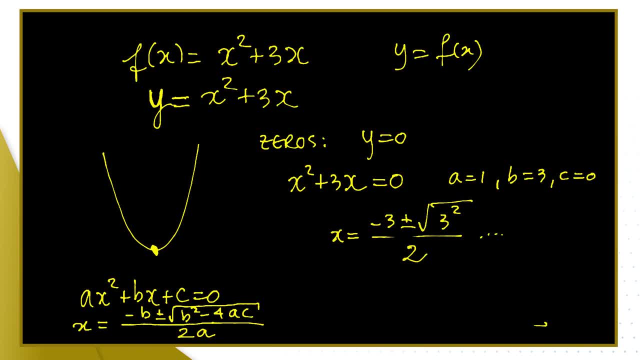 Now we can do that, but I'm going to show you another way that works for this particular example. So I'm going to rub all of this off and leave the quadratic formula for a more complicated example. In this particular case, I can factorise. 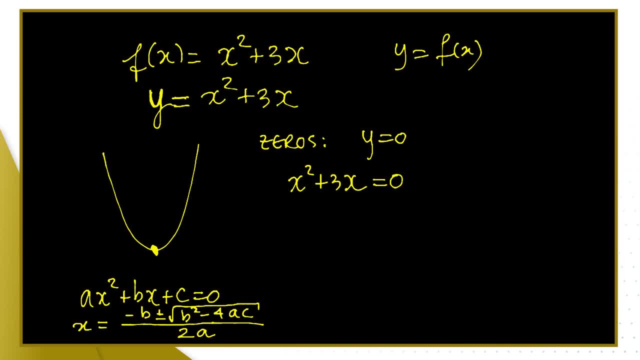 because there's no independent term, so there's a common factor of x. So I do x times x plus 3, all equals 0, and I have to do the equivalence, And that is equivalent to say: well, two numbers multiplied. 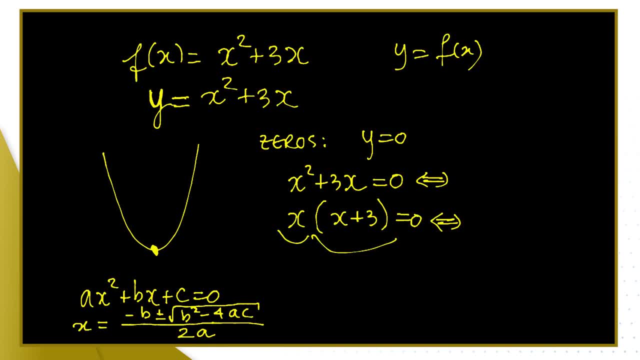 this and this multiply out to 0. The only way we can have that, if it's one of the numbers is 0. So I say x is 0, or x plus 3 is 0, which means that x is 0,. 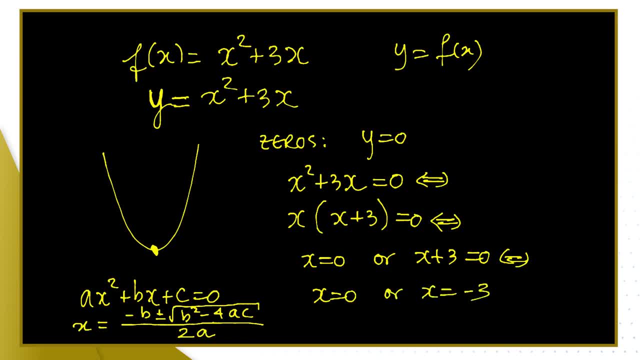 or x is negative 3.. So the zeros of my function, the points where it crosses the x-axis, are minus 3 and 0.. So on my graph, I'm going to choose a scale and I'm going to say: 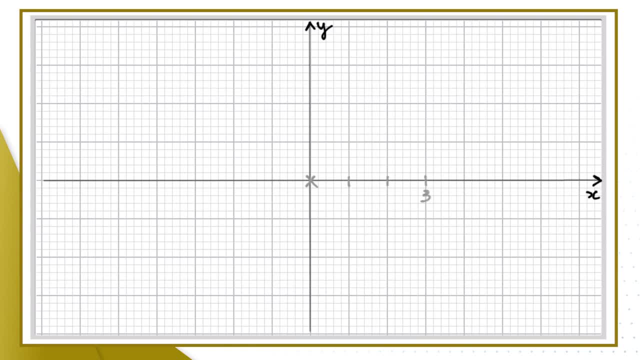 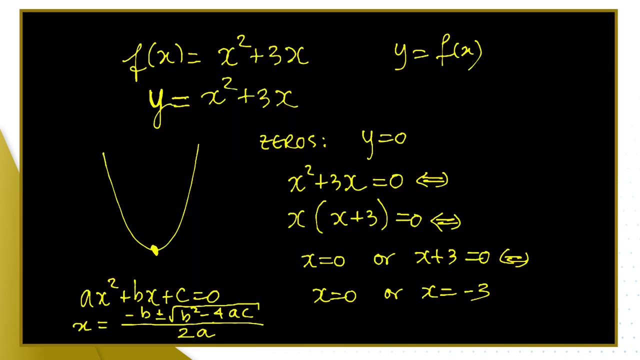 this is going to be the scale 1, 2 and 3.. Okay, Minus 3 and 0 are the points where the graph crosses the x-axis, So I've got those there. Now, what else other than the zeros? 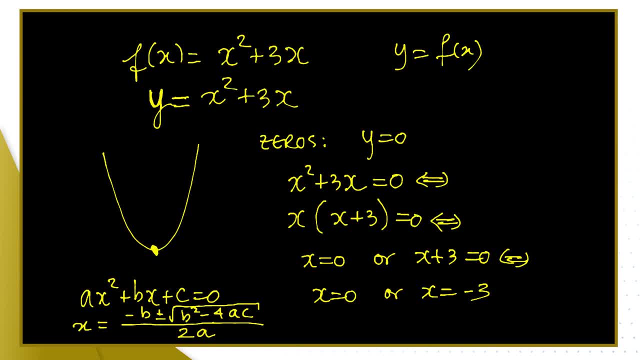 I mentioned the vertex. Where is the vertex? It's on that point there. but because we have two zeros, the x-axis is somewhat above the vertex. So we know we've got a minus 3 there and we've got a 0 there. 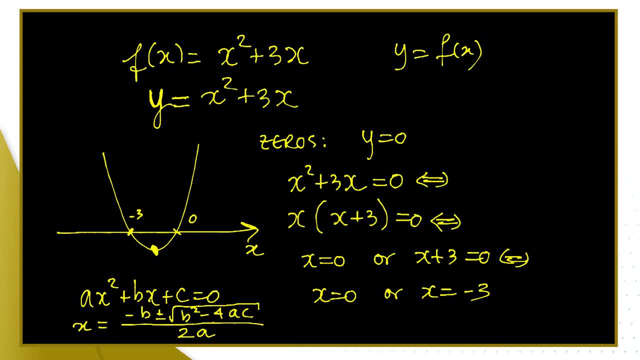 The vertex is always in the middle, in the middle of the two zeros. So we should expect the vertex to have coordinate x minus 3 halves. It's bang in the middle. But we don't know what the y-value is yet. 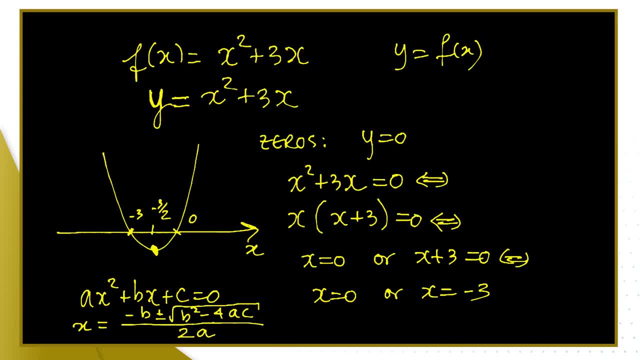 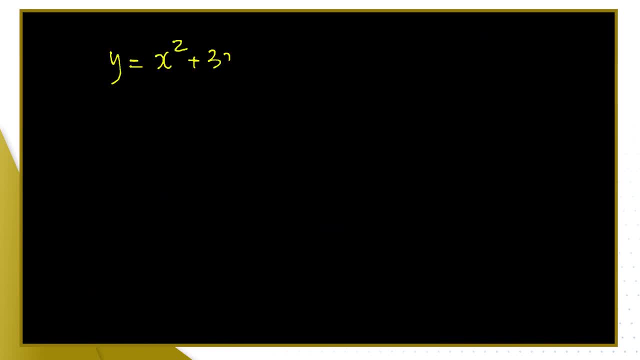 because what we do is we replace x equals minus 3 halves in the expression and we get the value of y, So y is x squared plus 3x. We're going to do x equals minus 3 halves because we said it's in between the zeros. 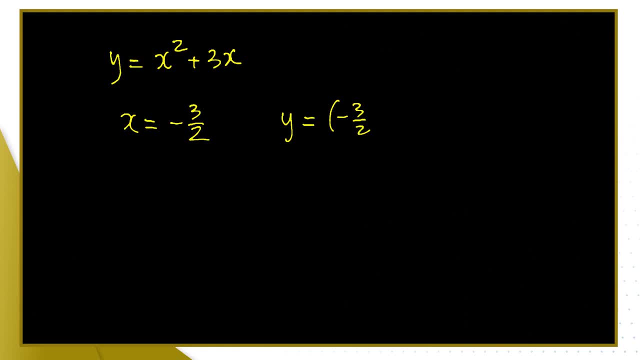 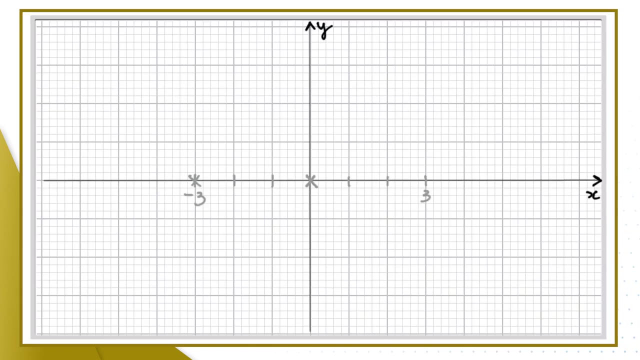 and that means that y equals minus 3 halves, all squared, plus 3 times minus 3 halves and that gives us boil down all the numbers to minus 9 quarters. So in our graph we can do minus 9 quarters, That is, minus 2 minus a quarter. 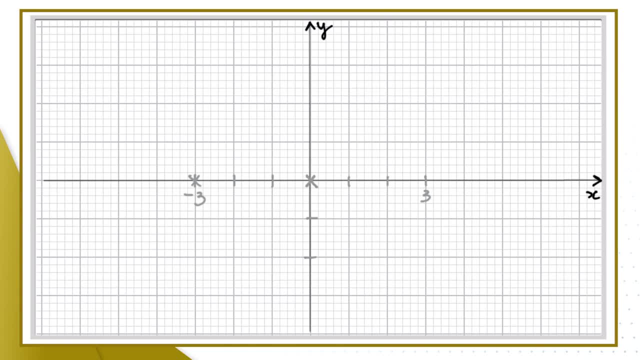 On that scale, if that's minus 1, minus 2, a quarter is around there. So minus 9 quarters is there and that is the value of y for the point minus 3 halves, which is here minus 3 halves. 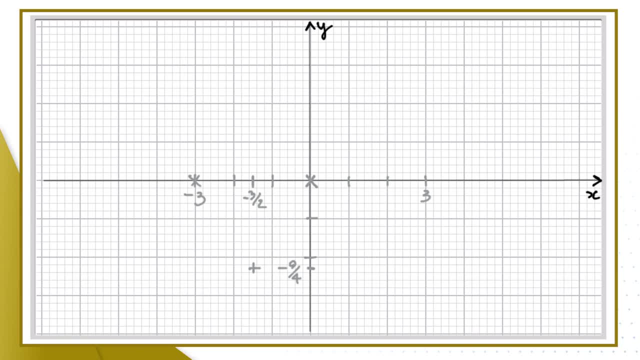 And so this is the other point I've got. That's the vertex. I'm going to call it z for vertex, that point there. Okay, so far I've got 3 points for my parabola. We could add a few more. 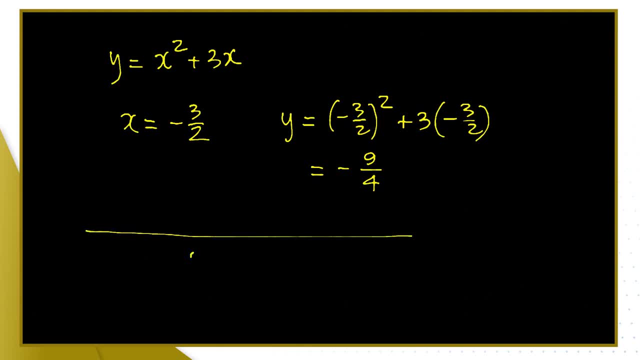 to do a nice plot So we could complete our table of values. Let's say I've got minus 4, which is before the 0, minus 3, that is, the 0, minus 3 halves which is on the vertex. 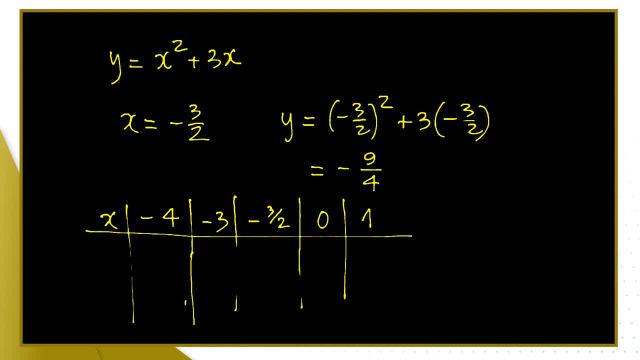 the 0, and then let's do another value of 1.. So we've got 0s here. we've got minus 9 quarters here, and now let's calculate the others. Minus 4 squared is 16,. 16 plus 3 times minus 4 is minus 12,. 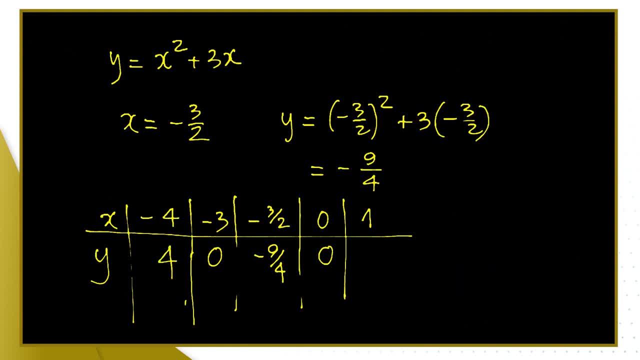 so I've got 4, and then I've got 1 plus 3,, which is 4.. Okay, and then now on the table we see the symmetry. The values are the same distance from the vertex. have the same values of y. 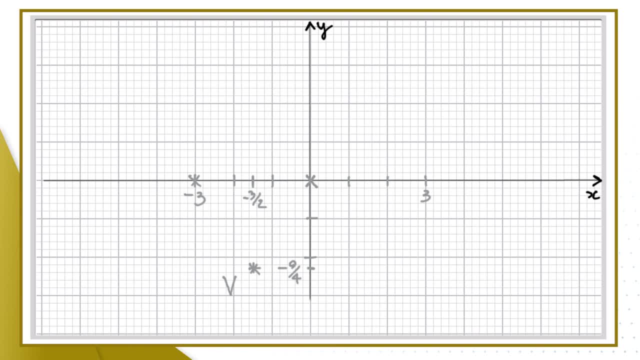 So on my graph I've got 4, so 1,, 2,, 3,, 4, at the very top of my, at the very top of the page. So for my there's 4 and 4, 1,. 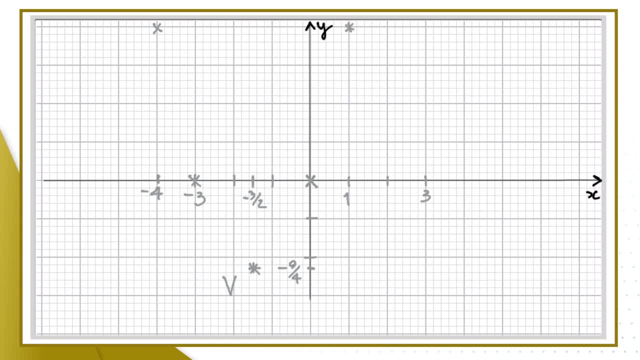 I've got those points there and now the sketch. Let's have a look. Really trying to capture the symmetry of my drawing- and you can always readjust. It's best to use a thicker line to make sure I cross the points I need. 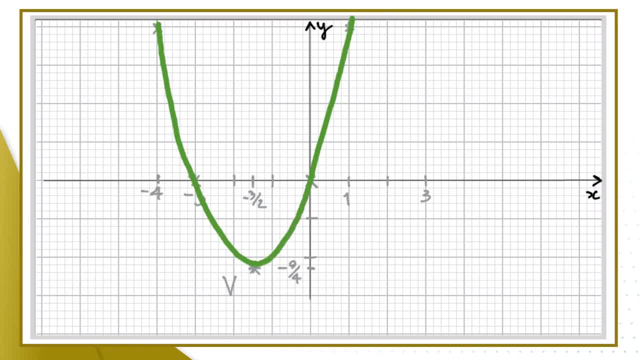 Now, if you're submitting hand-drawn work, it doesn't hurt to make a comment saying it is supposed to be symmetrical and you explain more about that. if you haven't achieved that with your drawing Now, questions you may be asking. 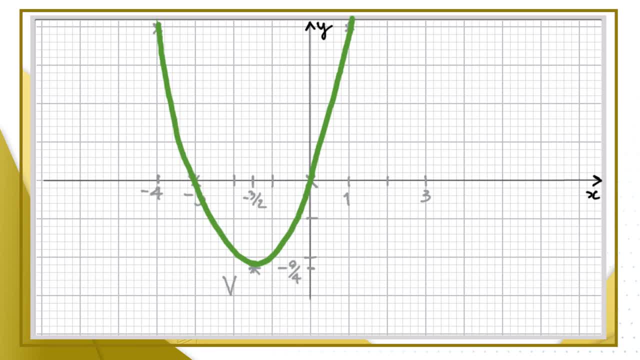 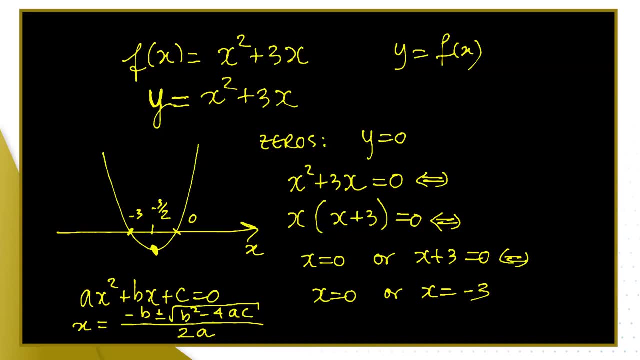 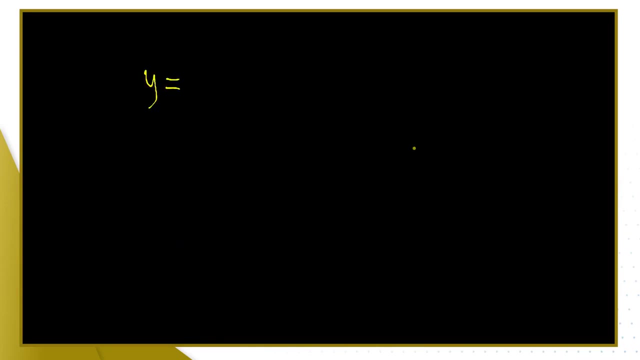 what if we hadn't worked out the zeros of the graph? Could we still work out the vertex? Yes, we could. To do that, we can complete the square. To complete the square, I start with my: y equals x squared plus 3x. 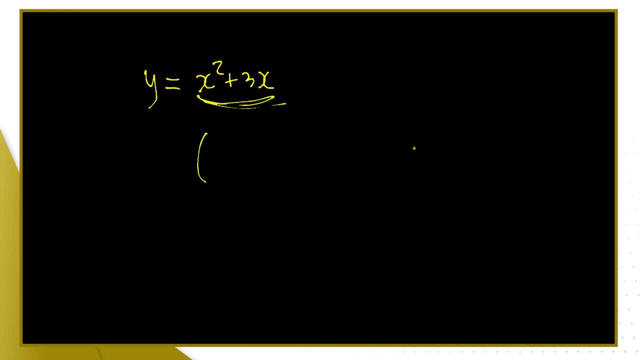 that's my function, and this part here I'm going to write as an x plus something all squared. So the way we do that, I need to put a number here, so I do the half of the three, so three halves, and then I have to take away. 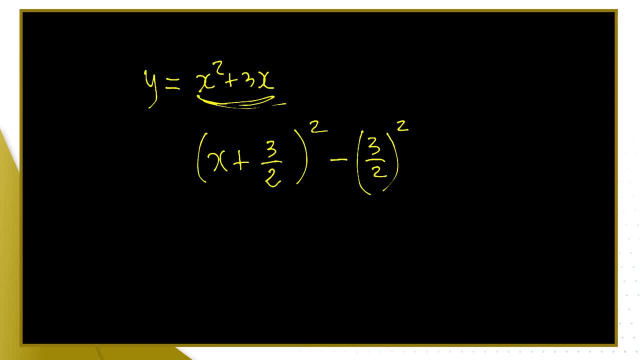 the square of that three halves, And this gives me I won't expand, because if I expand I get what I started with and I just work out what this is: Three squared is nine and two squared is four. So that is the expression. 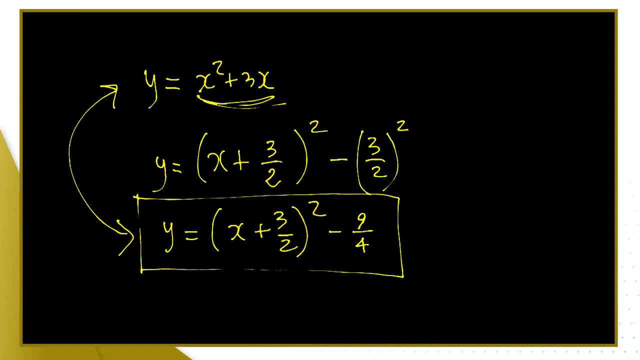 which is the same. it's the same function as there. they're equivalent. but this one, the bottom one, reveals the vertex. These are the coordinates of the vertex. So the vertex has coordinates. there's a three halves there, so we do minus that. 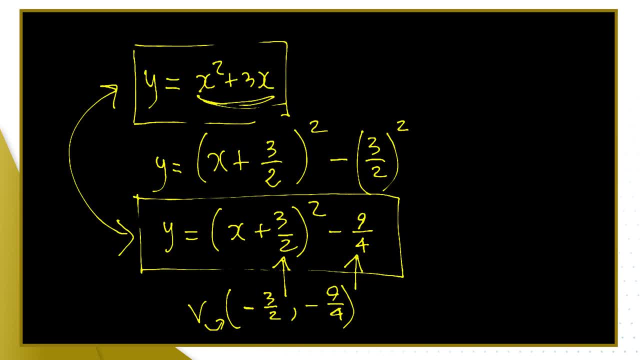 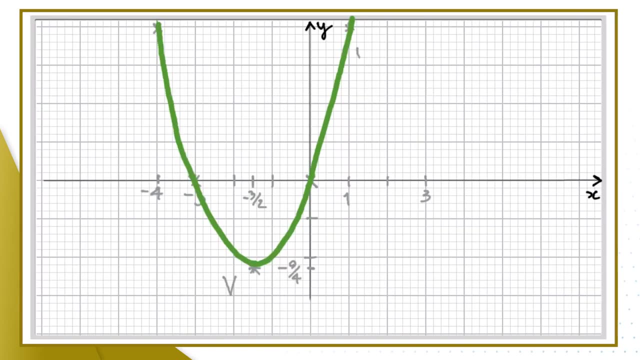 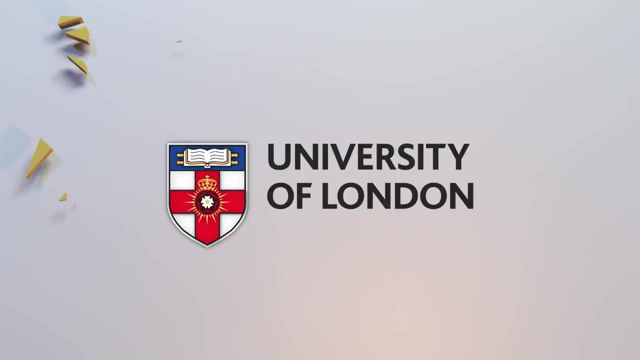 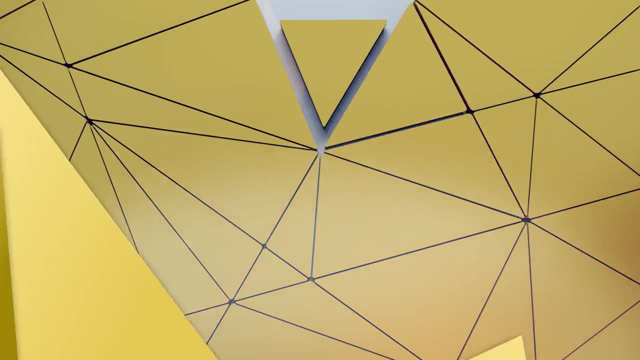 and then minus. so in other words, if you have x minus a number, the number is b, the vertex is ab. Okay, Which is our lovely graph there. so y equals x squared plus three x Sketched. We're looking at cubics now. 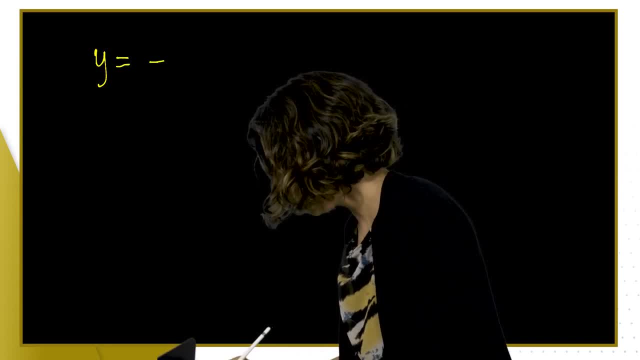 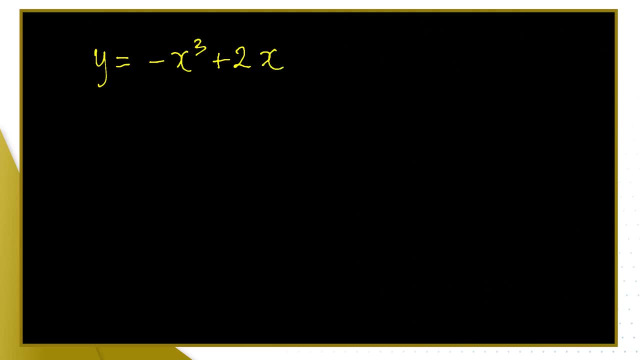 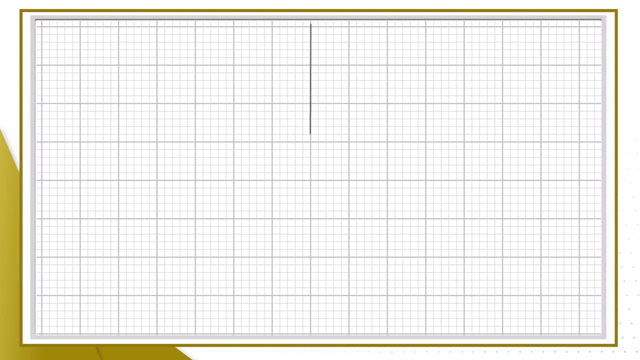 Say we have: y equals minus x, cubed plus two x. Looking at the expression, the independent term is zero. That means we have a y intercept of zero. So we can already put one point on the graph. So let's draw our graph. 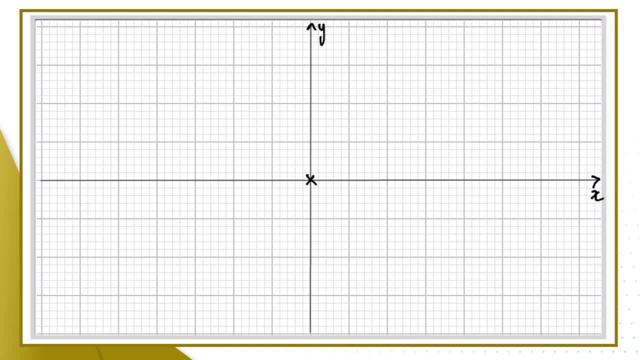 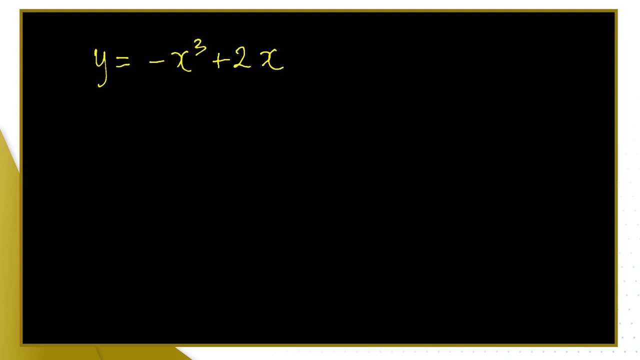 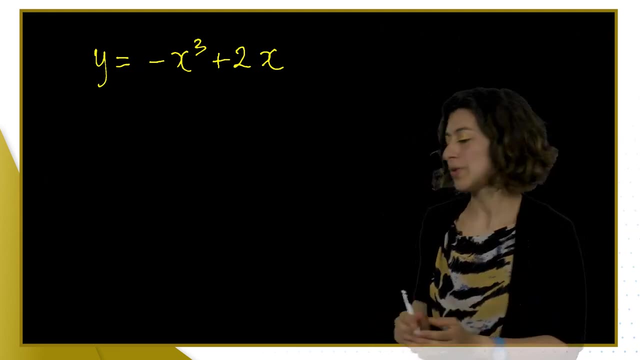 And we already have. the intercept is at the origin. What else can we know? It's a cubic, so we have less tools than with quadratics, but in this particular case we can look for the zeros. We can solve with y equals zero. 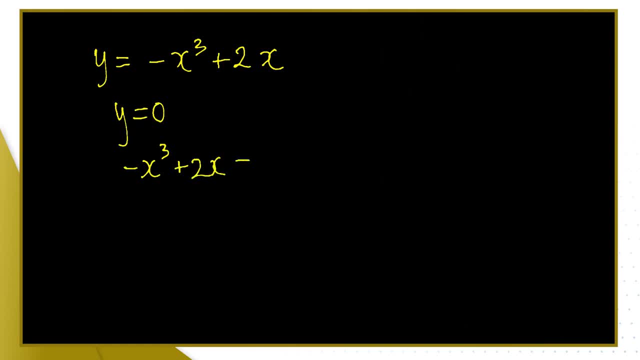 So we can solve minus x, cubed plus two x equals zero. We can do that not only because we have no independent term, we also have no term in x, So it will be possible to factorize and solve this equation. So that means I've got an x factor. 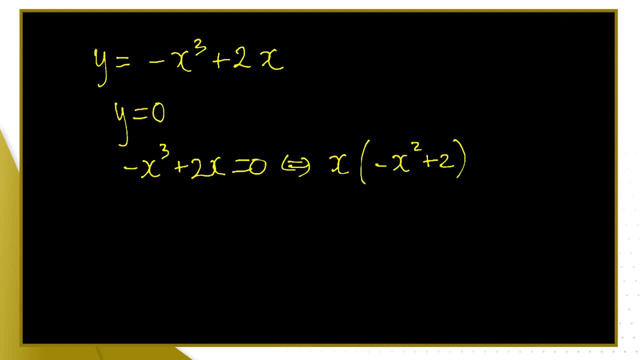 minus x squared plus two, that equals zero. Again, a product that gives zero. That means each of the numbers could be zero. Okay, And now we solve these. So we've got: x is zero or x squared minus x squared equals minus two. 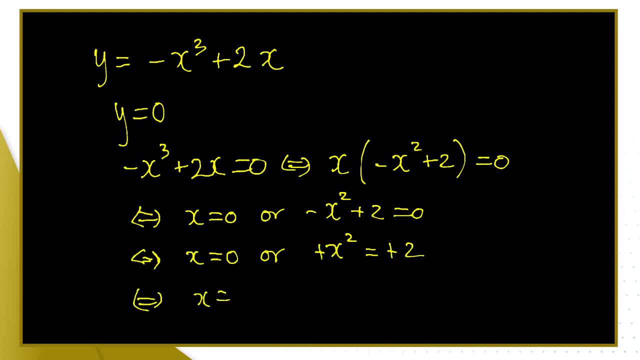 So x squared equals two And that means that x is root of two or x can be the minus root of two. So in this case we can find the zeros of the function, But note that in general with a cubic it will be beyond the scope. 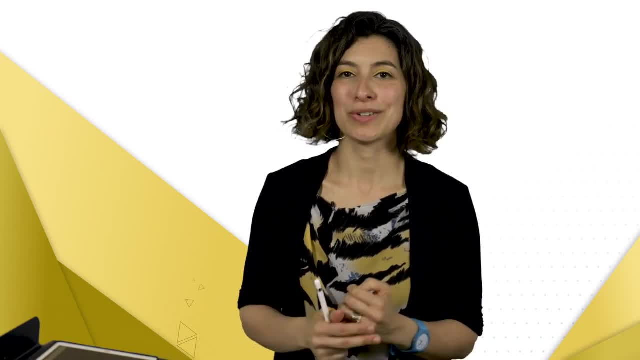 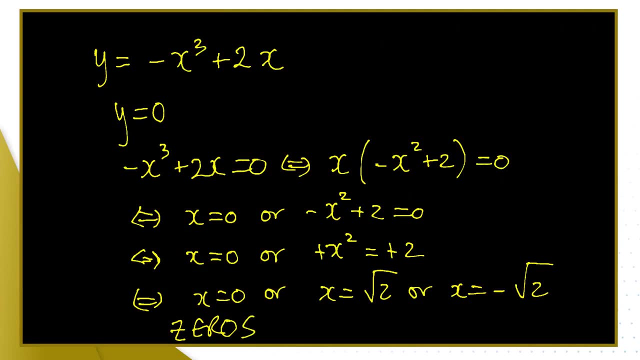 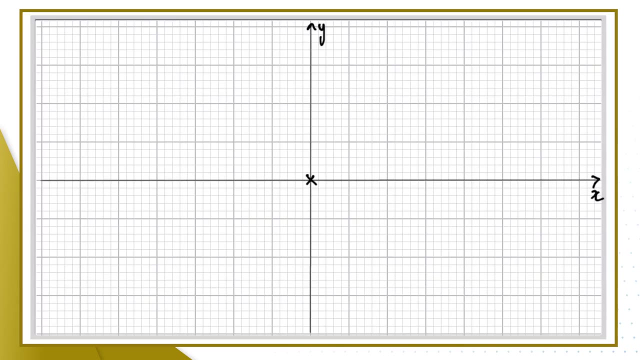 of this course and many undergraduate courses, to find the zeros of a cubic. Now we got the zeros here. There's three of them, So we're going to mark it on the graph. So root two is around 1.4.. So we've got a scale. 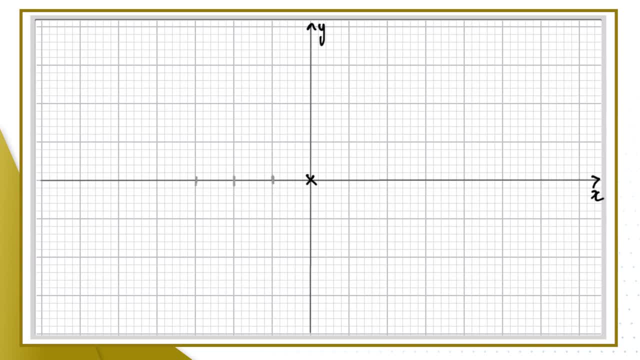 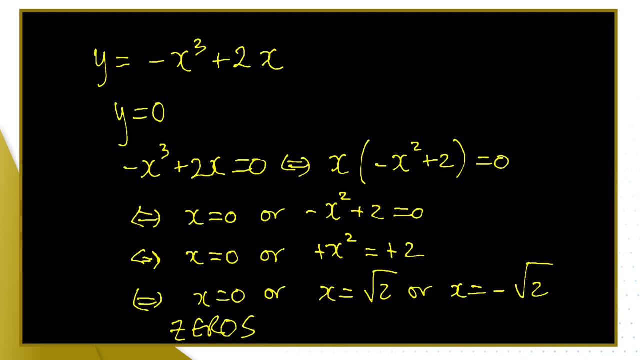 If that's our scale- one, two, three- Is that a good scale? We could be a bit more generous. Let's do minus one and this, minus two And this one and this two. Okay, So our zeros minus root two. 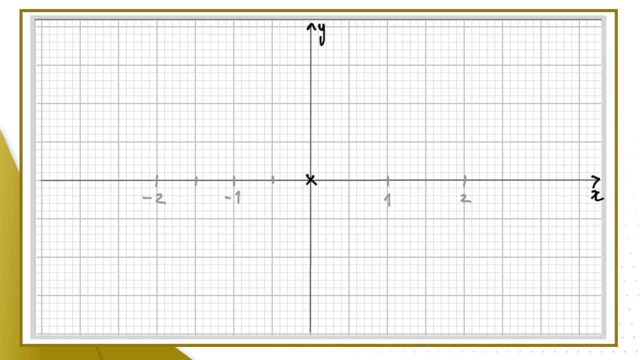 root two or zero. Root two is about 1.4.. So we have, minus root two over there, a zero, and root two around there And we have a zero. that is a zero. Okay, We've got those three points. 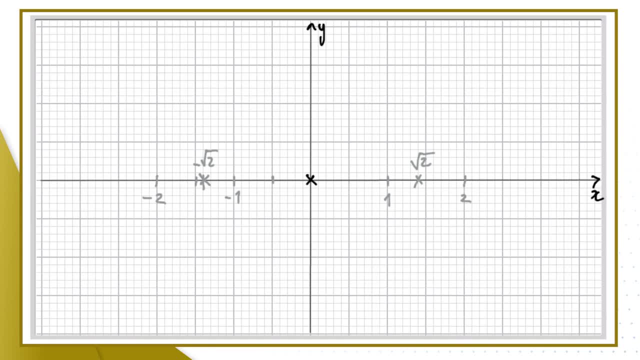 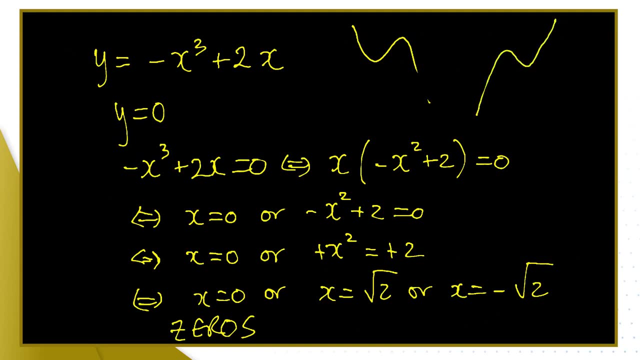 Now what does the graph look like? It's a cubic, So a cubic. it's either like this or like that, Or you don't have the wiggly bit in the middle. It could be just like that or like that. 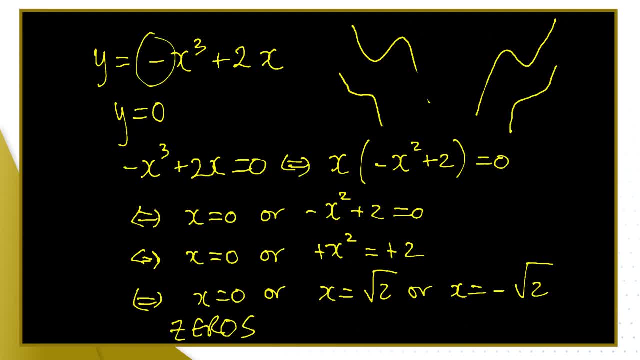 Now this is the coefficient of x. cubed is negative one, So it is a descending cubic. So it's one of these, Either the top one or the bottom one. Finding the middle bit will depend on the zeros. But look, we've got three zeros. 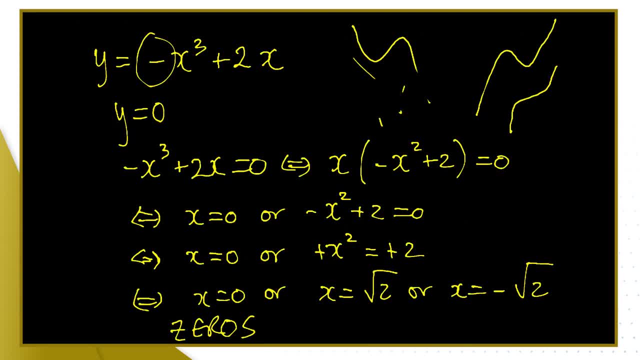 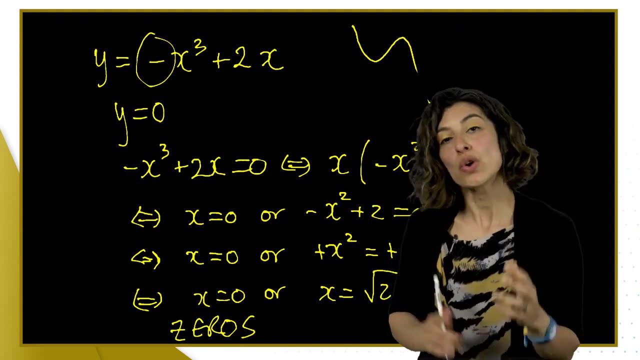 It has to be the wiggly type. We're going to delete all the others, So we expect the graph to look like that one. Let's find a few more values. So what values to choose for our table Now? we calculated vertices on quadratics. 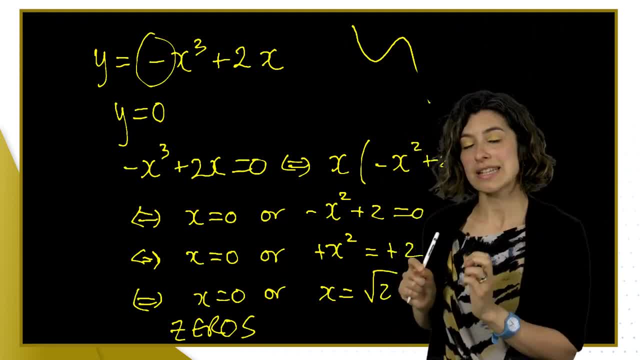 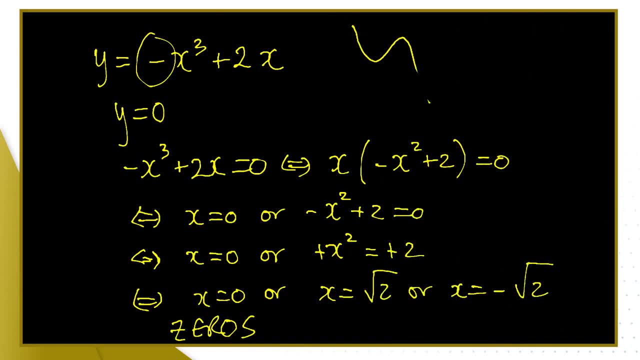 We don't have tools at this stage to calculate anymore Those kinky points on the graph. we don't have the tools now to find them. Okay, So we're going to estimate them. We're just going to find a value in between the zeros. 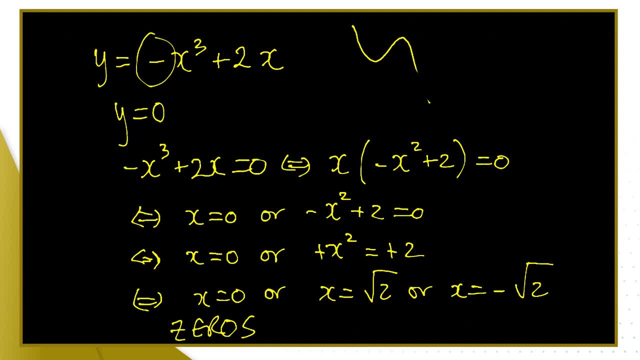 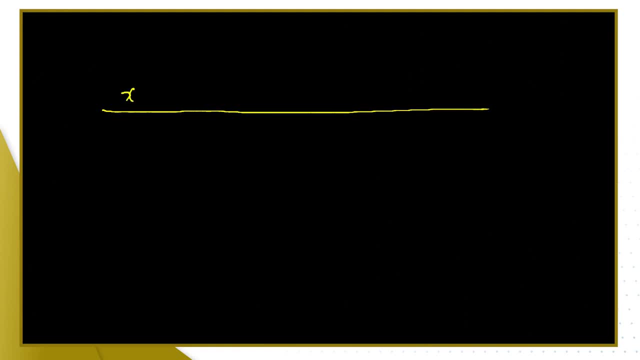 values in between the zeros, to make the best judgment we can about this graph. So our table of values: the values we want, minus two. we've got the minus root two, which is about minus 1.4, minus one. 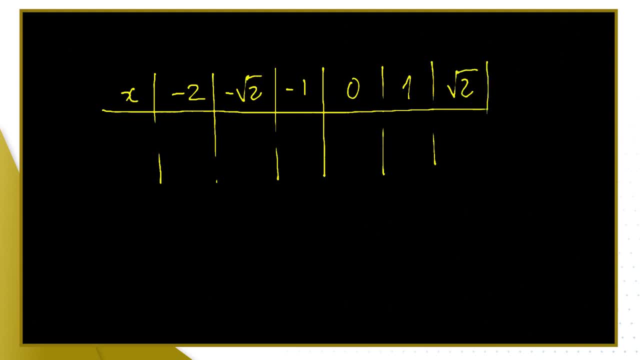 the zero, the one, the root, two and the two. So we've got the zeros, we've got values in the middle and we've got a little bit outside the zeros, So values of y, and we've got just remind ourselves what the expression is. 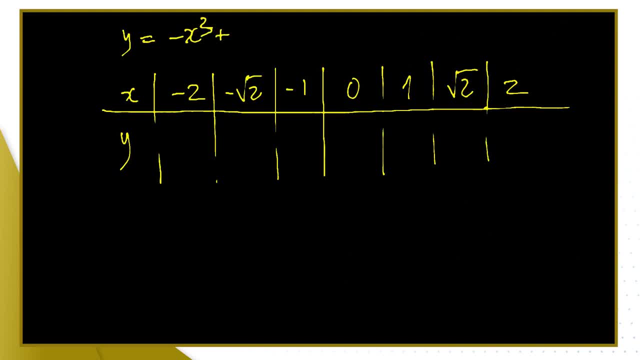 minus x cubed plus two x. So minus minus two cubed plus two times minus two. That is minus eight times minus. so it's eight minus four. That gives us four. Okay, Got that value. We should have the same value on the two. 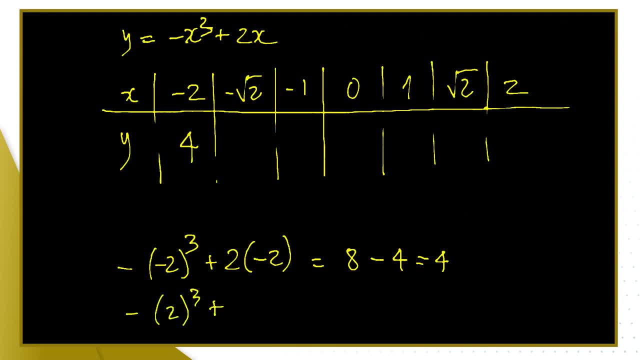 Let's check: Minus two cubed plus two times two, That's going to be minus eight plus four, That is negative four On minus one, we have minus, minus, minus one cubed plus two times minus one. That gives us: 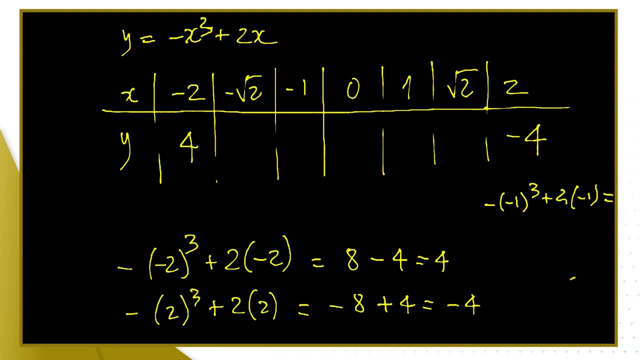 uh, one minus two, so that's minus one, And on one minus one, cubed plus two times one, we have minus one plus two, which is one, And on all the other values we had zero. Let's see if that makes sense in our graph. 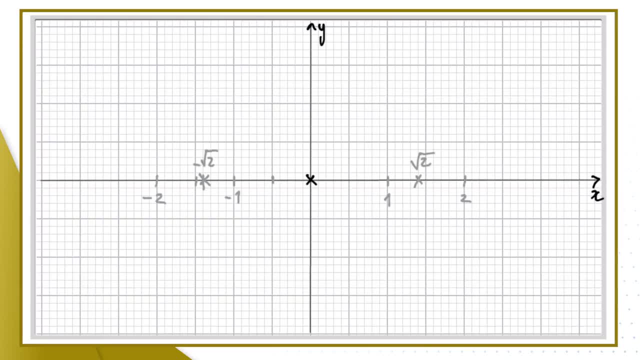 Got four and minus one, So I need an appropriate scale. That's minus two, That's minus four, That's two, That's four, And let's have a look On minus two. I've got four On my on two. 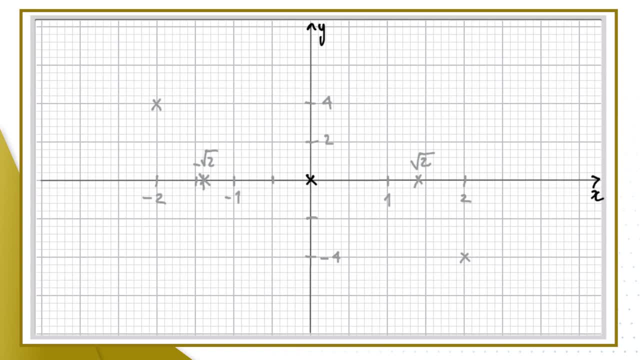 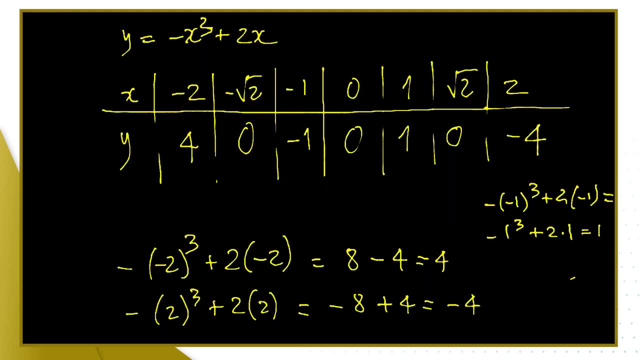 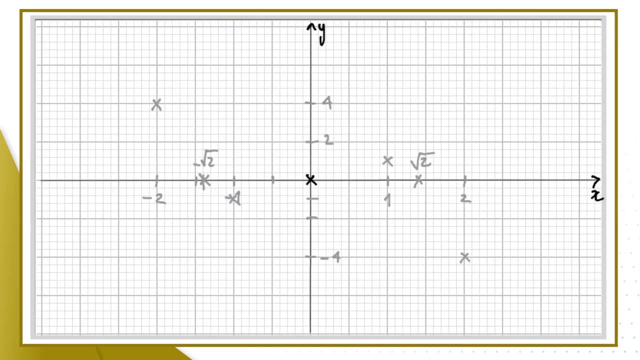 I've got minus four. On minus one, I've got minus one, which is here, And then on one I've got one around there And I've got zero. Okay, Let's see how this works. Let's try and draw that graph. 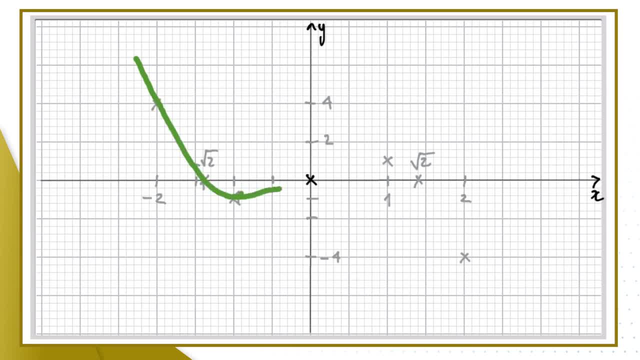 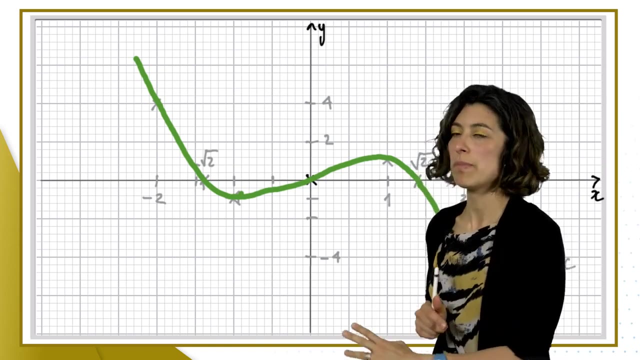 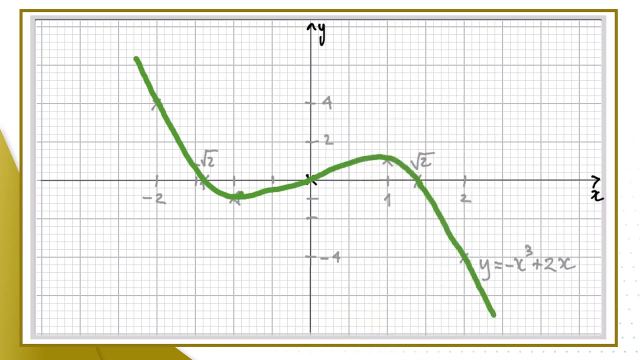 Not bad. Y equals minus x, cubed plus two x. Looking at that graph I know there's one part there that isn't really accurate: The behavior between the zeros. I don't know if it's as shallow as that or not. 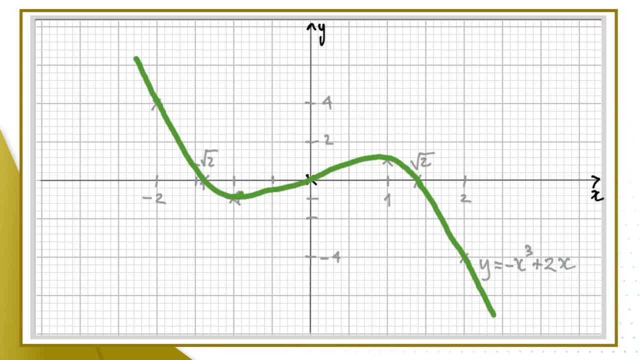 What to do. What I mean is I've drawn that green line But going through the points, here's another alternative. This orange line is a totally plausible line and it fits the data. We need to add more values to the table. 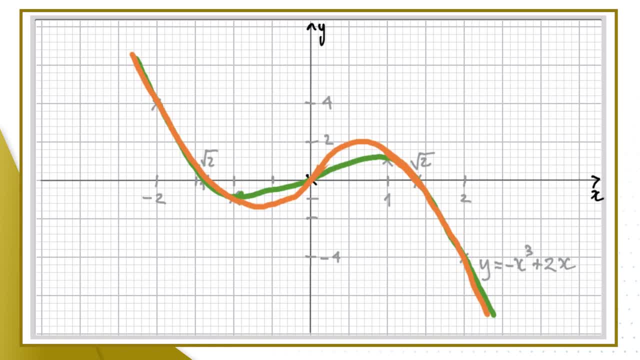 So you're going to do that, You're going to find, you're going to find more values of x in between here, So that you can figure out how the graph looks like, If it looks more like my orange or my green curve. 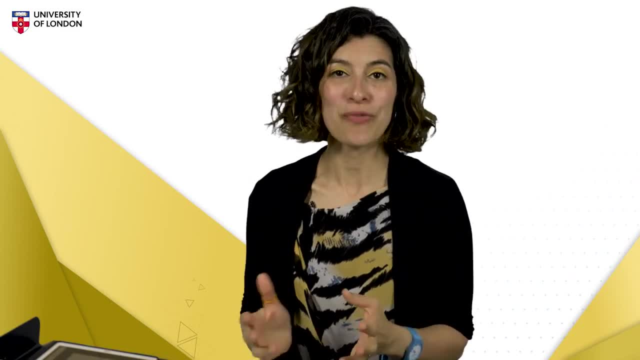 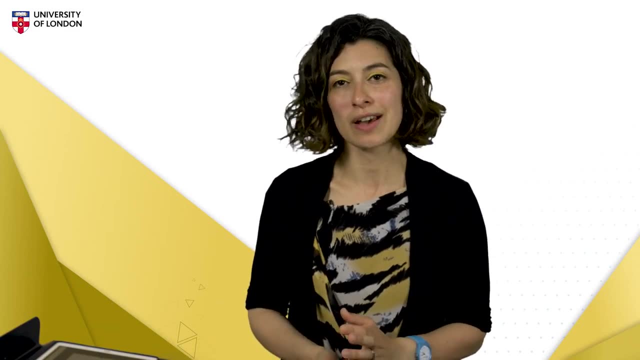 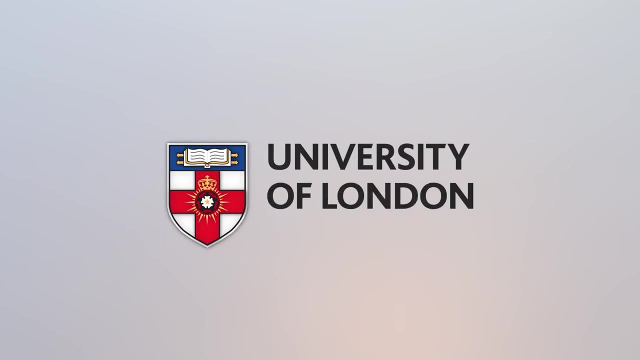 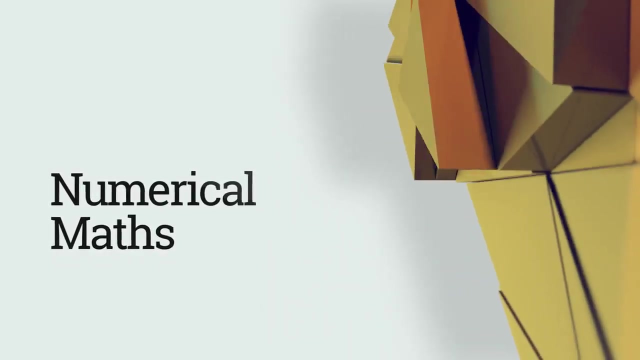 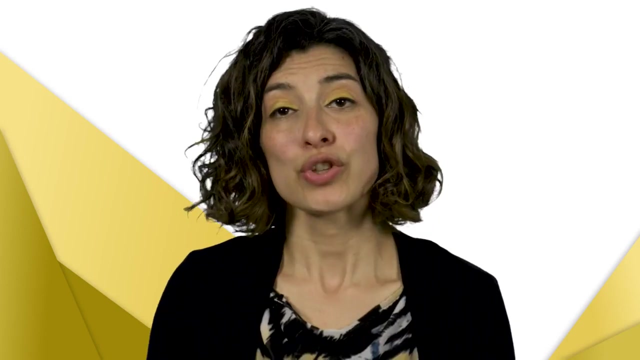 So you're going to go away and calculate more values of x and the respective values of y in those regions to clarify exactly what the behavior of the curve is like. So far, we've plotted graphs of quadratics and cubics. Quadratics and cubics. 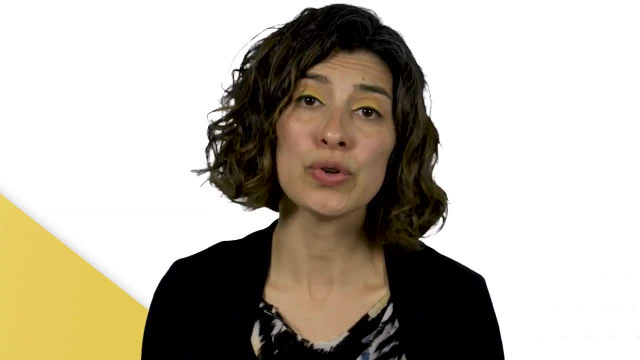 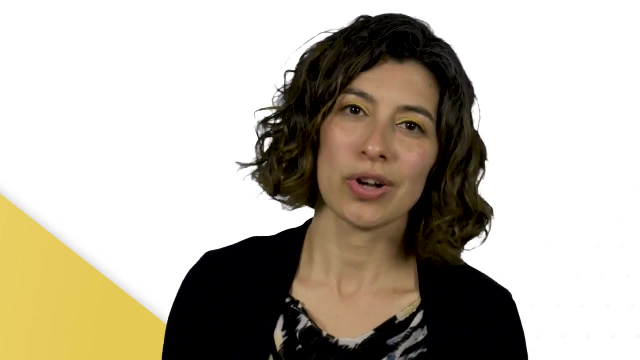 are special types of polynomials: Polynomials of degree 2 for quadratics and degree 3 for cubics. Any power larger than 3 on a polynomial. we're going to call them higher order polynomials, And there is a very limited 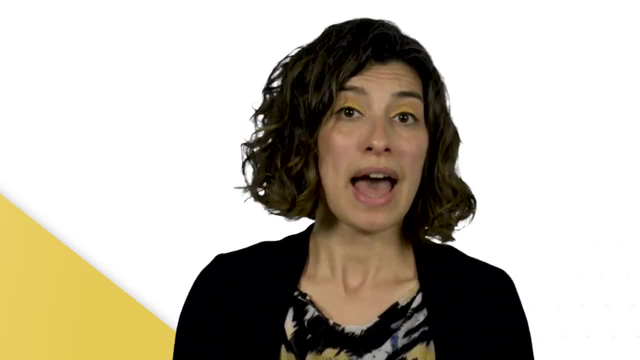 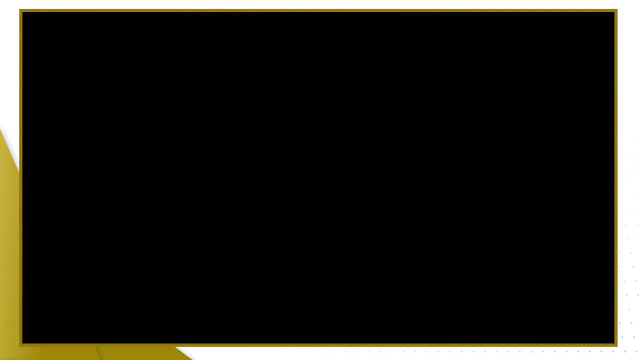 amount of mathematics you can do with them at this stage. So what can you expect If I give you a function that looks like this: y equals a really large number of multiplications: x minus 4 times x minus 3 times x minus 2. 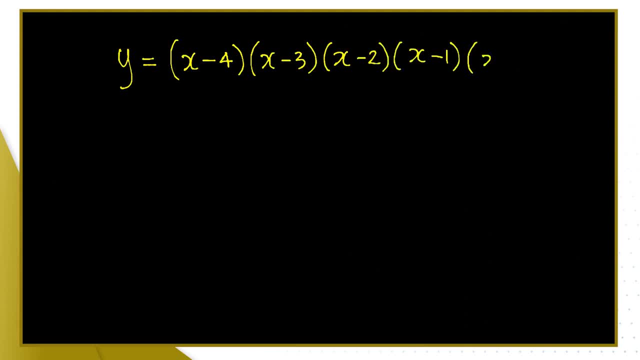 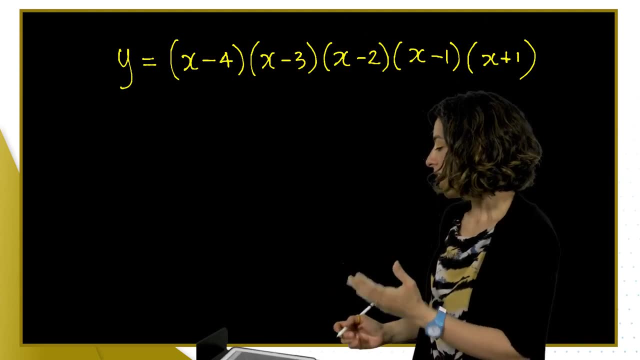 times x minus 1. times x plus 1.. If you were to multiply out all these brackets, the largest power of x you'll get will be 1, 2, 3, 4, 5.. x to the power of 5.. 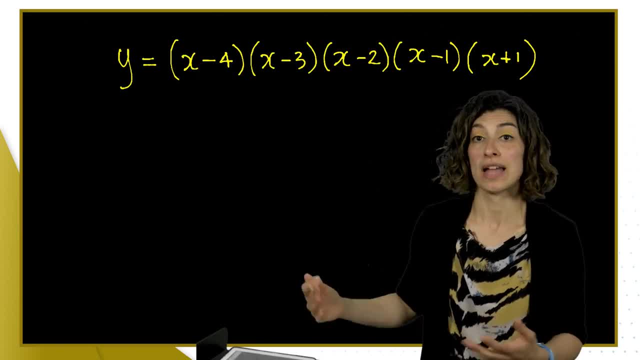 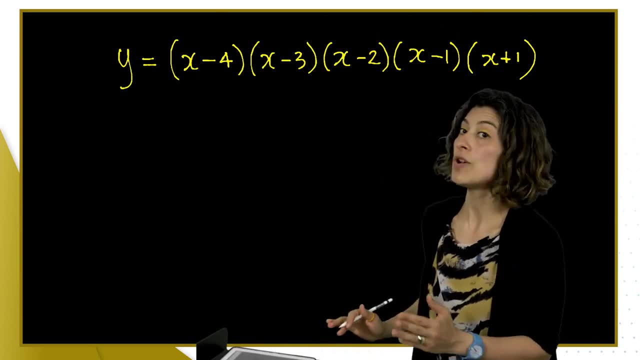 And then you have some terms in x to the 4,, x to the cube and so on. That will be a larger, higher order polynomial. It will be a polynomial of degree 5. Now there's no advantage in multiplying out. 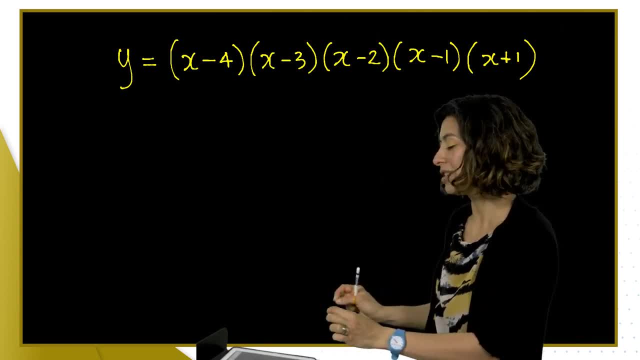 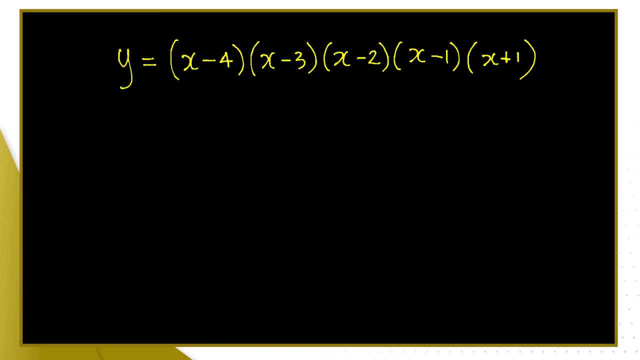 these brackets because we have a little bit of information in this polynomial, as it is The fact that it's written as x minus a number times x minus another number, and so on. that gives you the information of the zeros. So this polynomial we know. 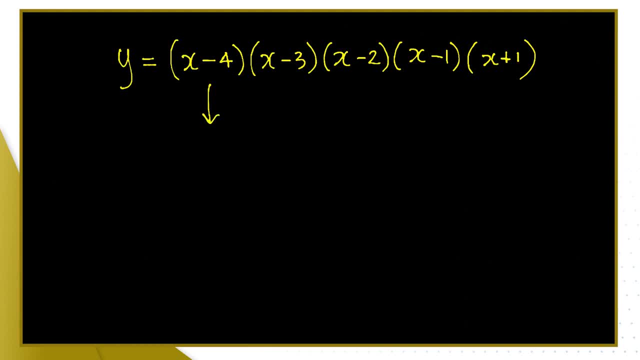 has to cross the x-axis when x is 4.. Because when you make x equals 4, that term becomes 0.. When x is 3, when x is 2,, when x is 1, and here, when x is negative 1,. 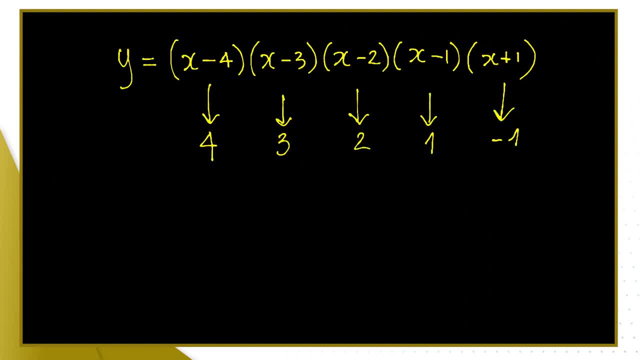 if you replace x by negative 1, everywhere you get numbers and this last term will be 0.. So each of the numbers I wrote there- 4,, 3, 2, 1, minus 1, are zeros of this function. 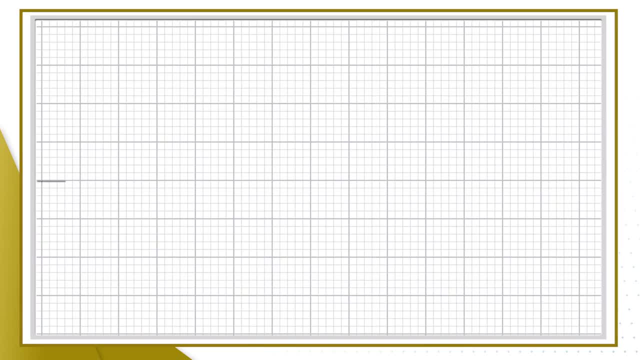 So we're going to draw that on the graph. Okay, we've got our y-axis and our x-axis and the zeros go from minus 1 to 4, minus 1,, 1,, 2,, 3, and 4.. 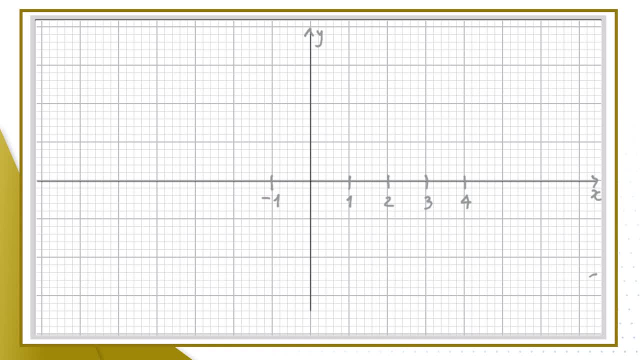 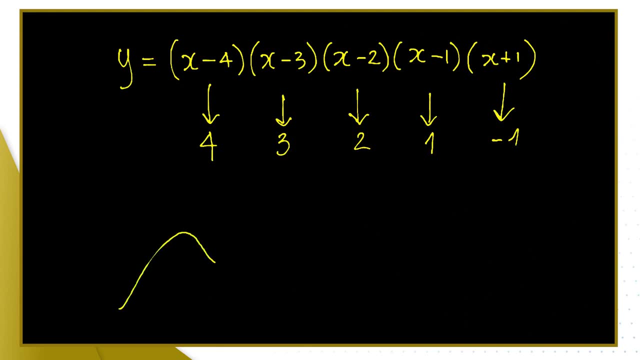 So those are the points where the graph crosses the axis, the x-axis. This graph, what it looks like, is a degree 5 polynomial. It's going to look like this with the x-axis crossing that way. So 1, 2,. 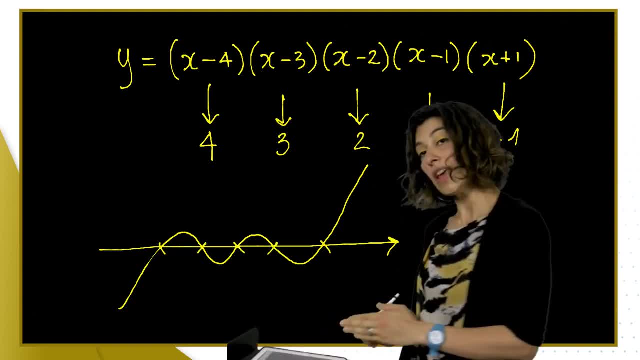 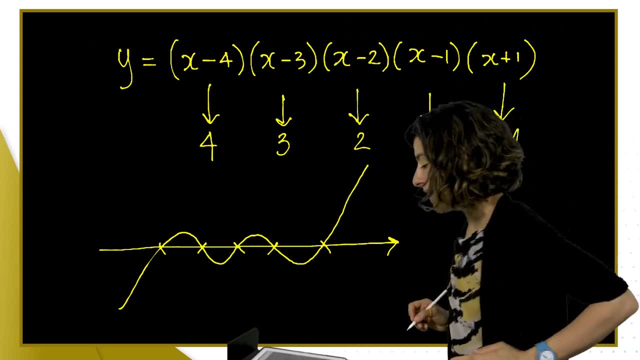 3,, 4,, 5 zeros. And I know there's an ascending one because when I multiply out all the x's it will have a positive coefficient. So it is an ascending graph in the sense that it goes from a lower value here. 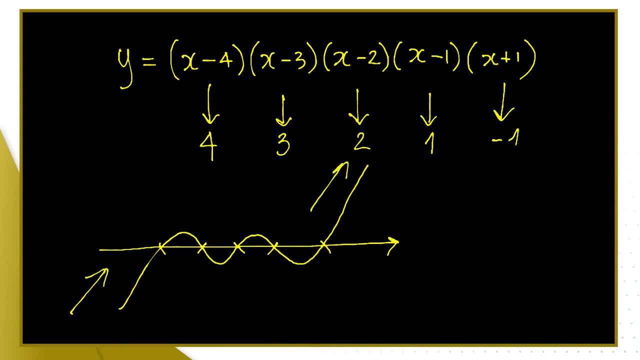 to a higher value there. To complete the graph, all you need to do is make a table of values that incorporates all the zeros and puts numbers in between, So it would be a nice thing to do. minus 2,, minus 1,. 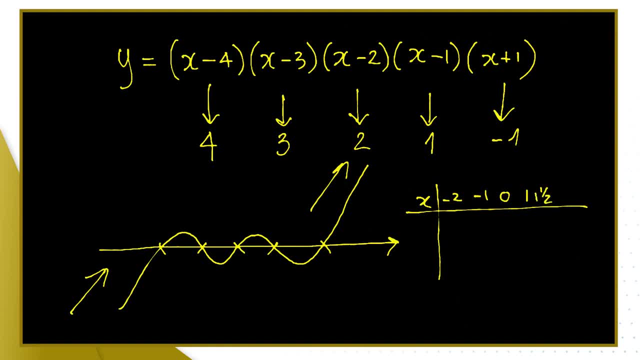 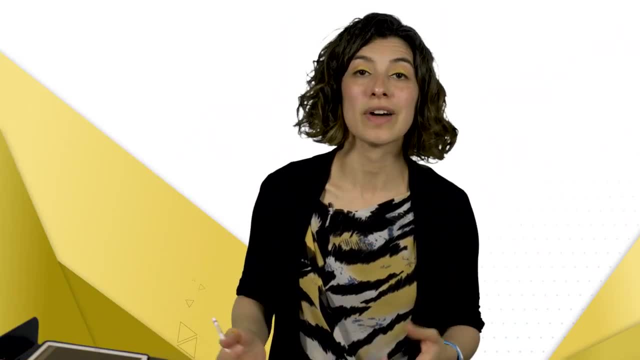 0,, 1,, then a half, one and a half, and 2,, 2 and a half, and 3,, 3 and a half, and 4, and 5. And you can complete that table of values. 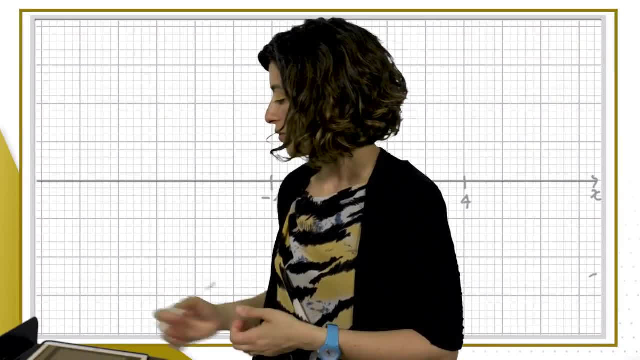 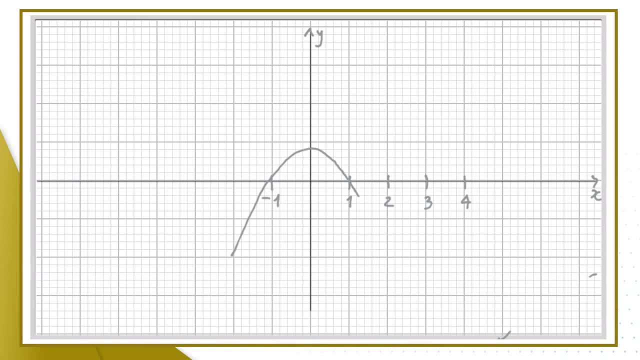 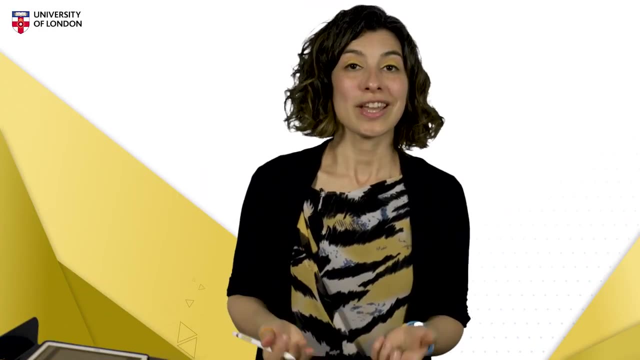 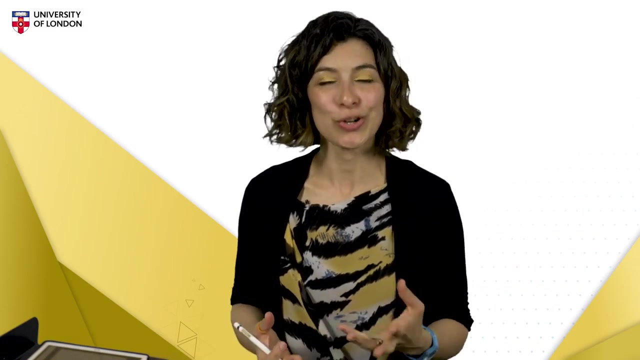 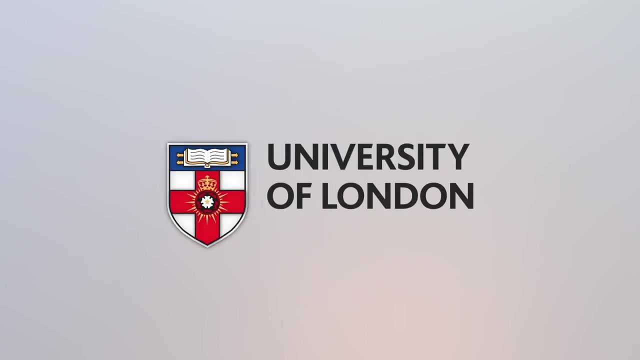 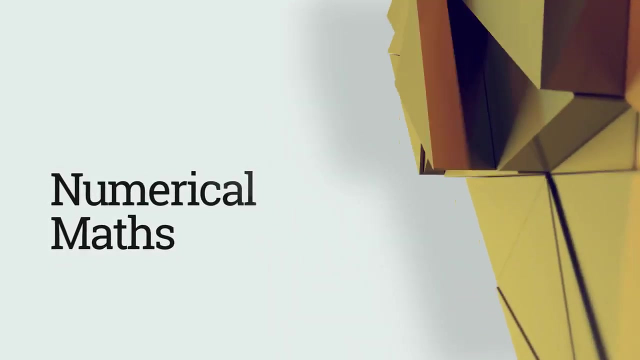 with corresponding values of y. plot it in the graph and you'll get a curve roughly like this: You can then check your answer by plotting the graph against graphing software and see how well and how accurate your own graph was. Let's look now. 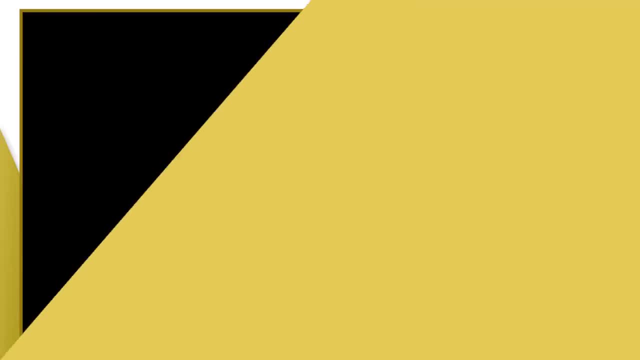 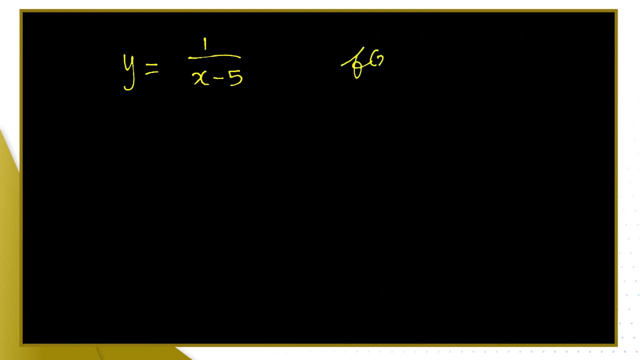 at plotting reciprocal functions. One example of that is: y equals 1 over x minus 5. Meaning that the function of x is 1 over x minus 5.. It is a reciprocal because we have 1 over an expression in x, In this case. 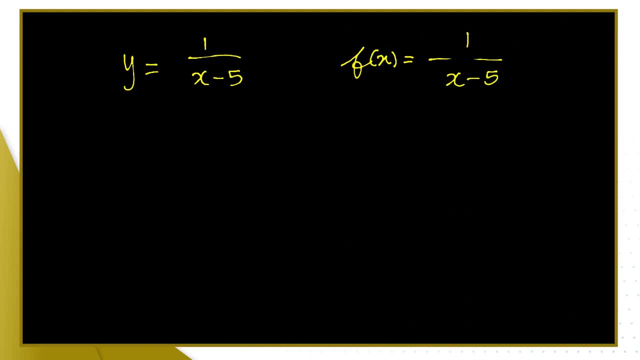 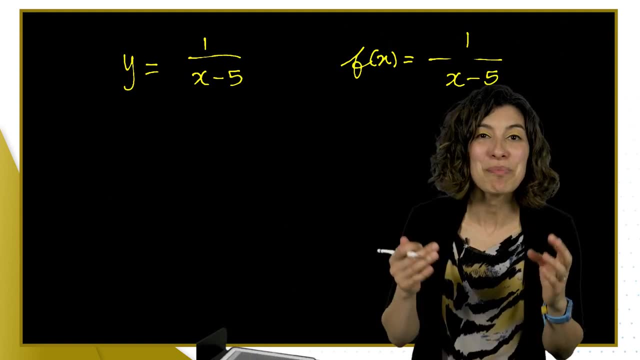 1 over x minus 5.. With reciprocals, the main thing to watch out for is the domain or, in fact, the points that aren't in the domain. So, in this case, the problematic value, the value that will give you. 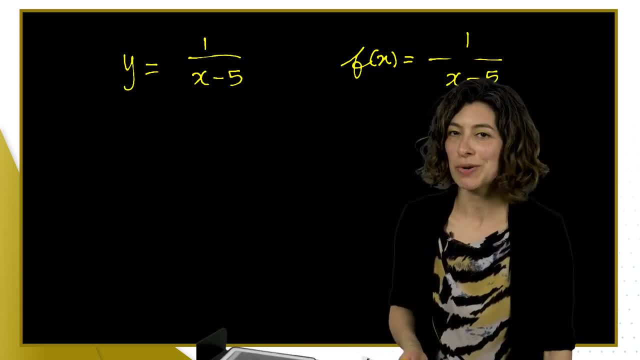 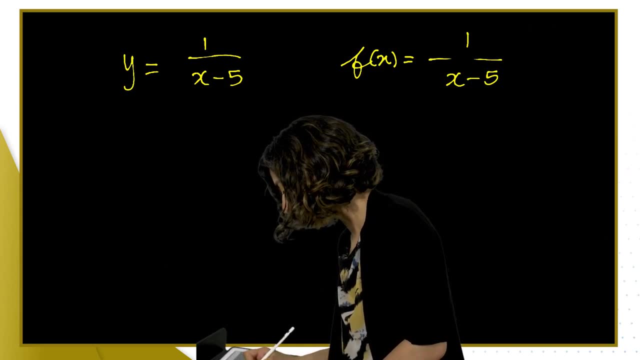 a division by 0 in computer is when x equals 5.. So x equals 5 is not in the domain. so the domain of this function is the whole of r, except for the value of 5. And that's 5 because if x 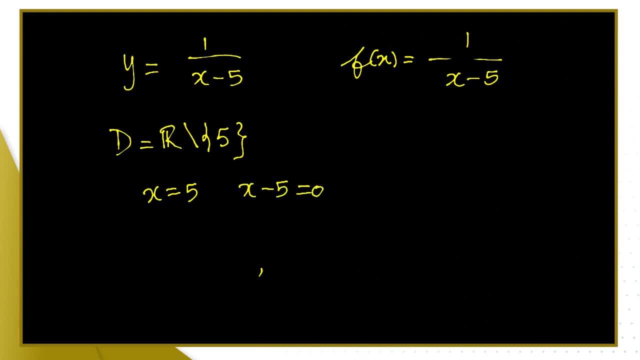 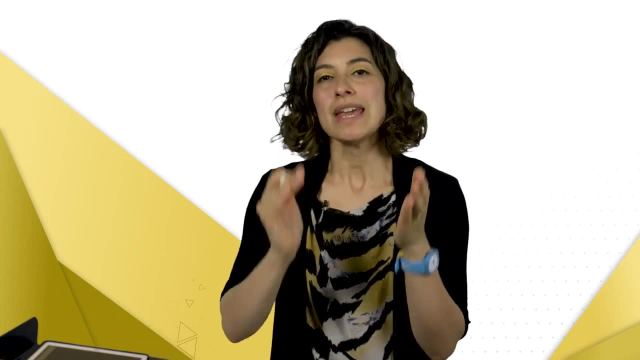 equals 5, then x minus 5 is 0 and we cannot perform division by 0.. Why do we care about the domain of this stage? It's because it's a very sensitive part of this graph When x approaches 5 by lower. 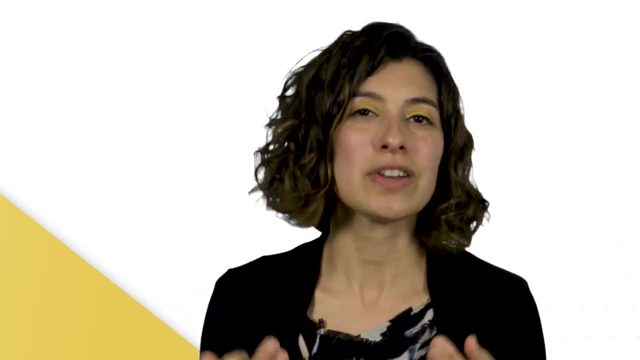 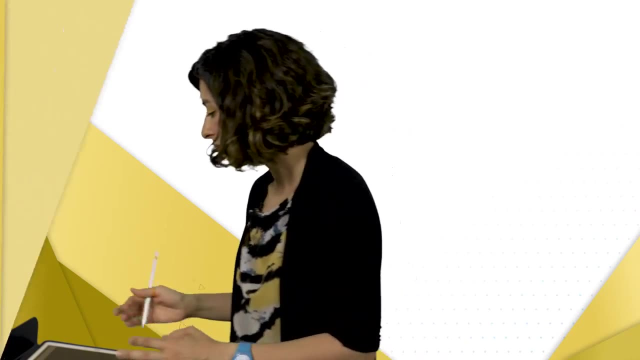 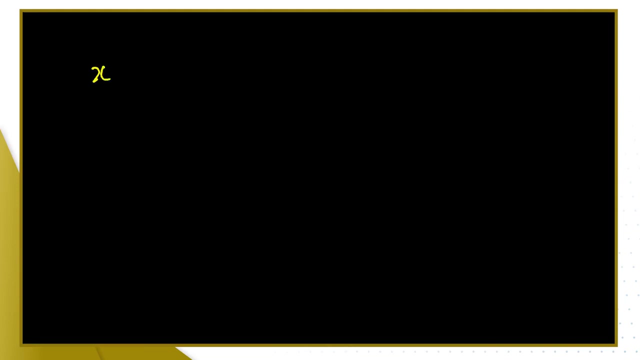 or upper values. the function is going to behave in a highly sensitive manner. The values of y are going to get huge, So we're going to prepare our table of values taking this into account. So 5 is our sensitive value. that the 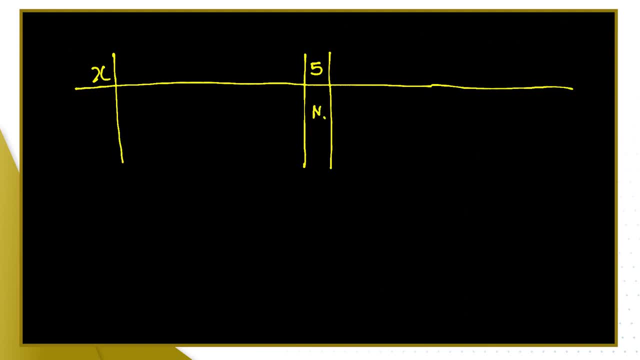 function isn't defined on, So we're going to have lots of values of x around 5.. So we're going to do 5 and a quarter. We'll do 5 and a half, 5 and 3 quarters. 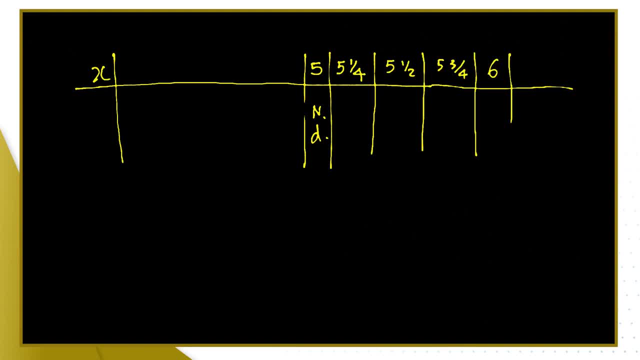 and 6 and so on. We'll see what if we need more, And on the other side we're going to take a quarter away of 4 and a quarter the value of 4, and then we'll see what else we need. 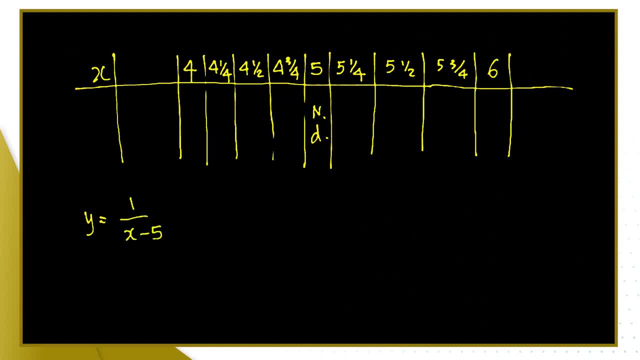 We're going to calculate those. So let's remind ourselves that it's 1 over x minus 5.. So for 4, we have 4 minus 5, which is minus 1.. So 1 over minus 1. 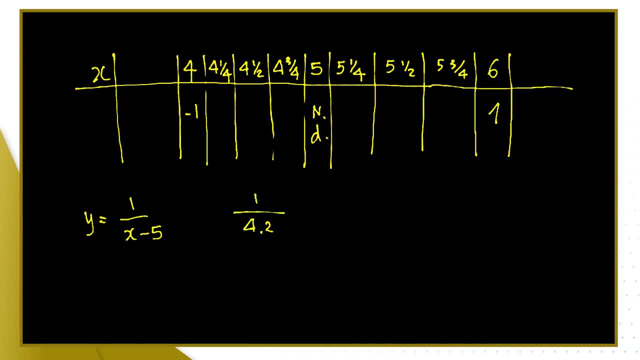 is minus 1.. For 6, we have 0.25 minus 5.. That is the denominator. We have 0.75.. That is 3 quarters of the bottom. So that makes 4 thirds. That's the. 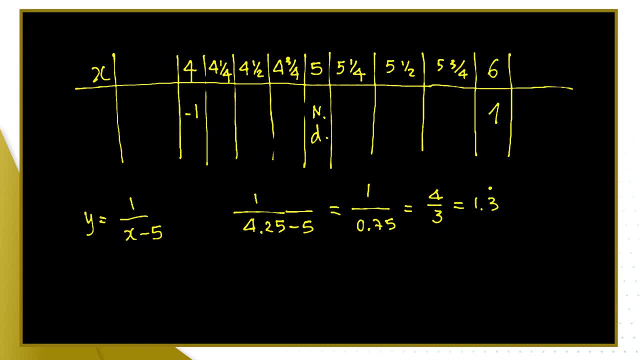 value and that's 1.3 recurring. or you can just write 4 thirds, 4 and a quarter. we have 4 thirds as the minus And in 5 and 3 quarters it's going to be 4 thirds. 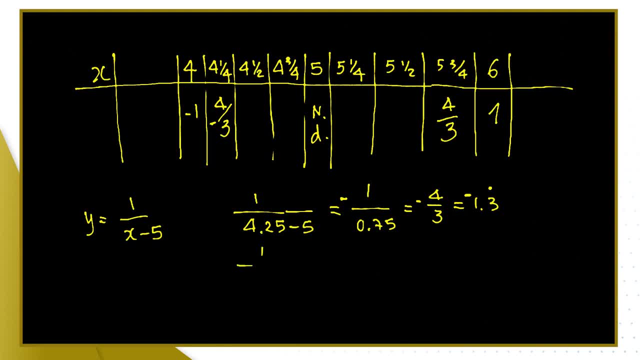 You can check that by yourself. On 4 and a half, 1 over 4.5 minus 5, that's going to be 1 over 0.5.. So 1 over negative 0.5, that's. 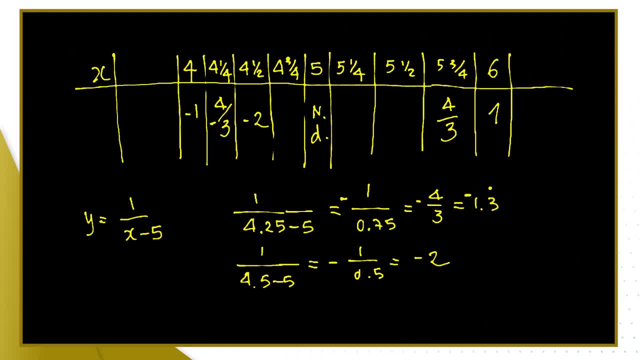 going to be minus 2.. And on 4 and 3 quarters it's 1 over 4.75 minus 5.. This will give us minus 1 over 0.25.. 0.25 is a quarter. 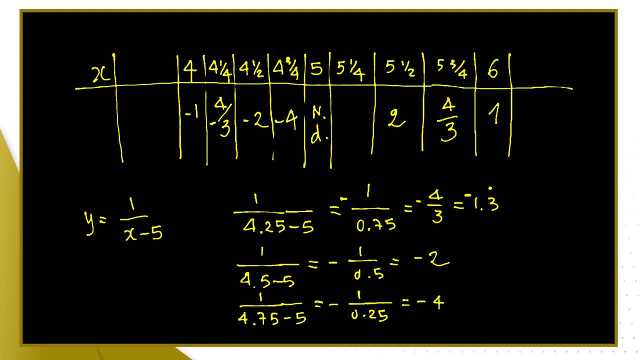 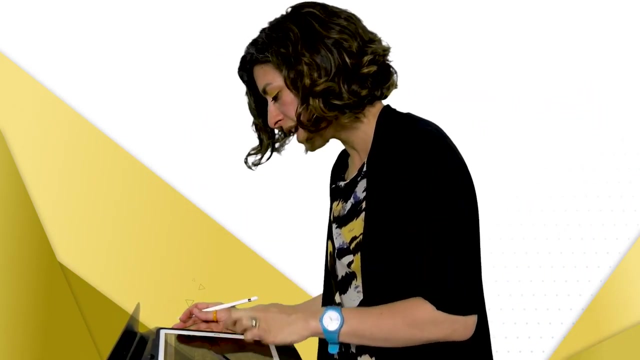 so this is negative 4.. So the values are increasing, And if we wanted to have a quarter inside, it will get you a value of 4.. You can check that Now. this should be enough for us to have a good. 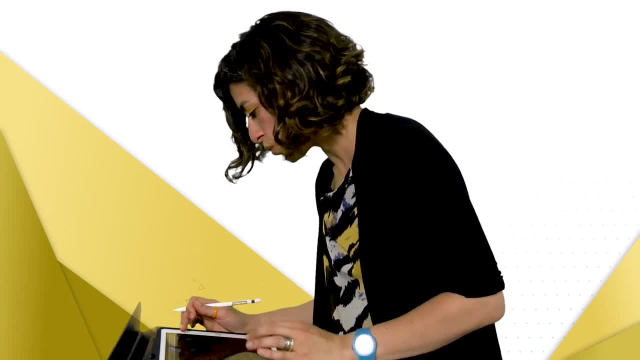 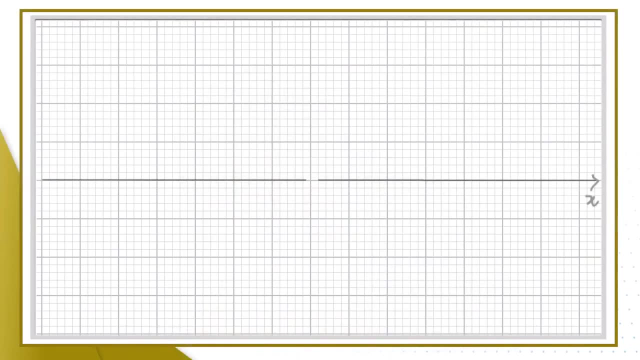 picture On our graph. we need a range, a vertical range from minus 4 to 4.. And we need x values from minus 4 to 4.. So we need a range from minus 4 to 4.. 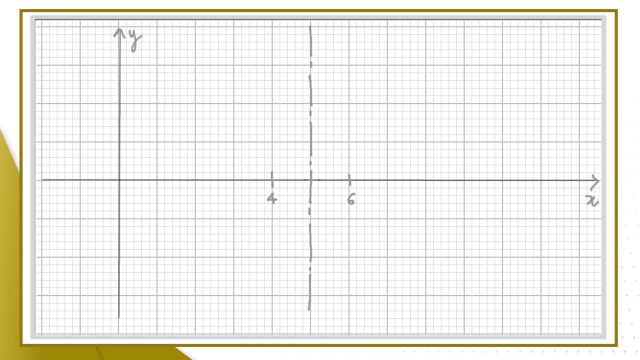 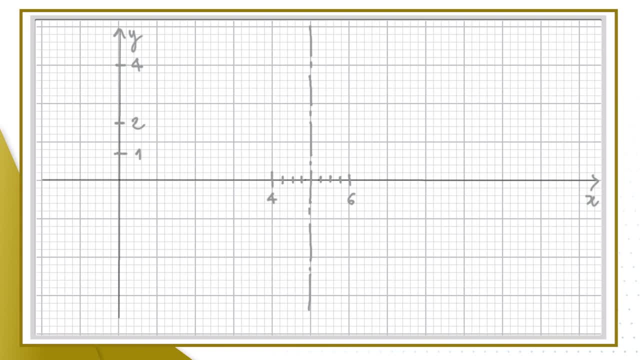 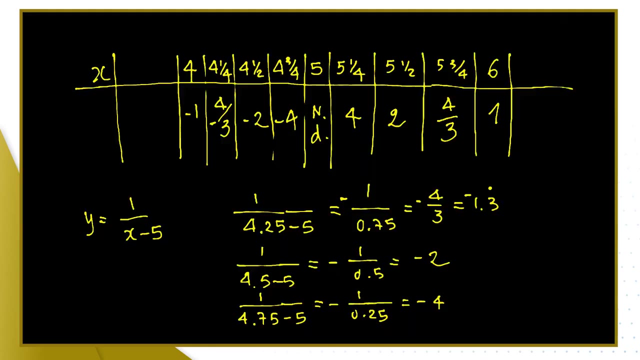 will be here and let's work with it. So with 4 we got minus 1, let's do it again minus 4, so minus 2, minus 1, so I've got 4 minus 1, on 4 and a quarter, I got minus 4 thirds. 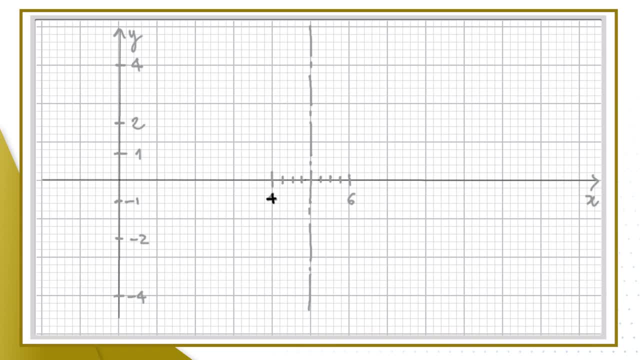 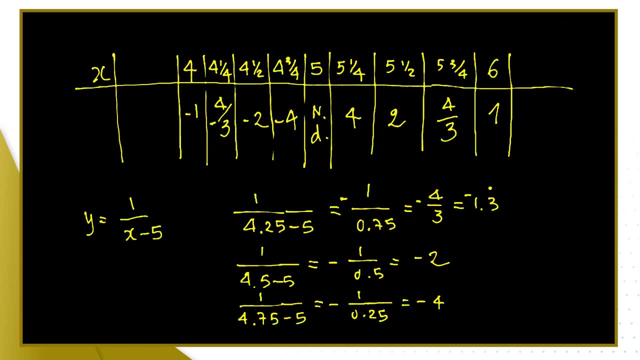 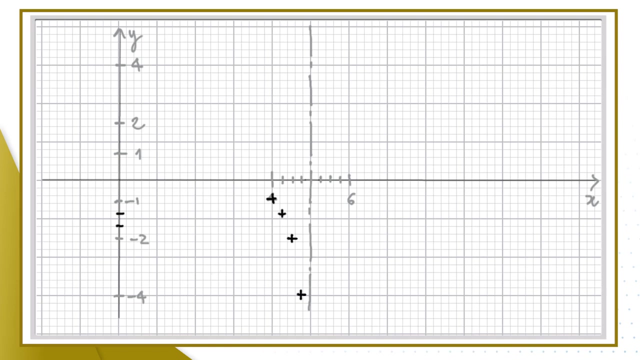 4 and a quarter is there, minus 4 thirds. let's do a third of that that's going to be around here, and then minus 2 on 4 and a half. minus 2 is here and minus 4 on the other one. okay, and on the other side I'll have a similar behavior. 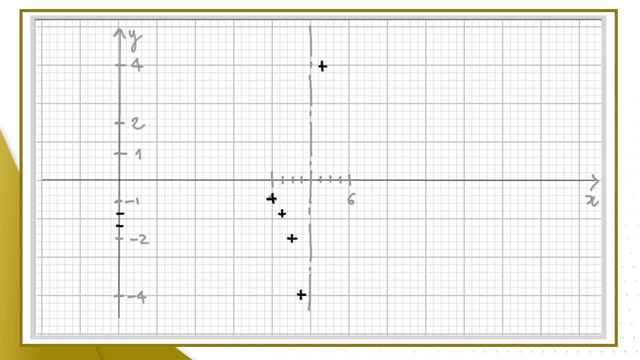 so I've got 4 around here. I've got 2 in the middle, so that's one there, and then I've got the 4 thirds, which is 1 and a third. that is going to be the value for that one. 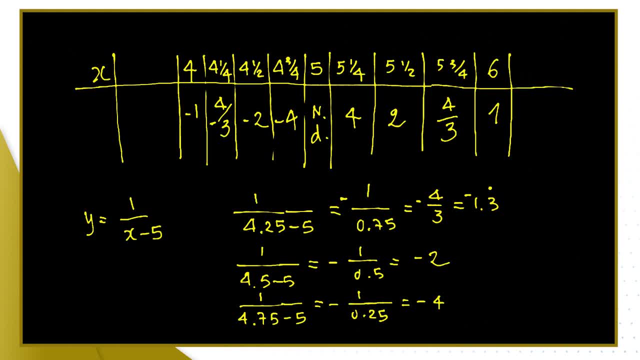 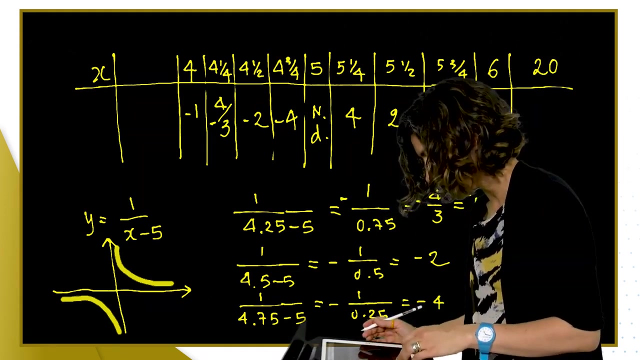 Now, what graph do we expect? We expect a graph like that, with axes going that way. so we have almost. so what happens as values of x increase? Let's try a big one, let's try in our calculator. so if we do what's big, so we try. let's try 20, if x is 20, we have 1 over 15, so 20 minus 1,. 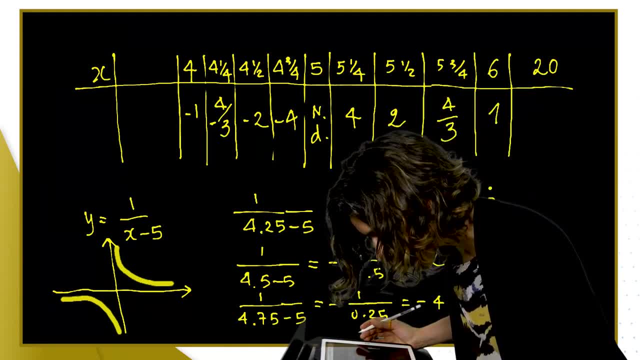 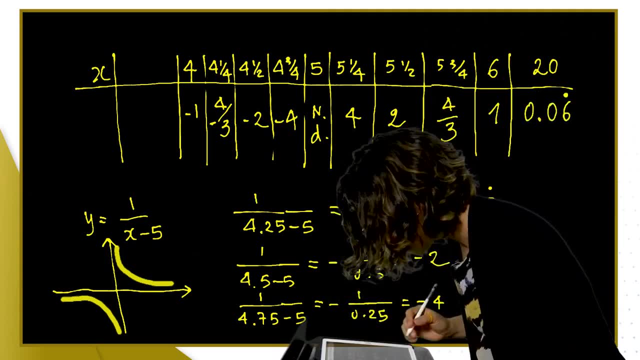 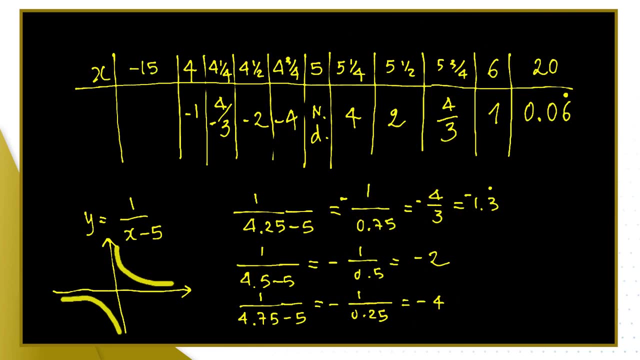 5 over 15,, 1 over 15,, 1 divided by 15, that is 0.6 recurring, 0.06 recurring. thank you, pardon. and then if I try the value of minus 15 on the other side, or let's try minus 10 on the other, 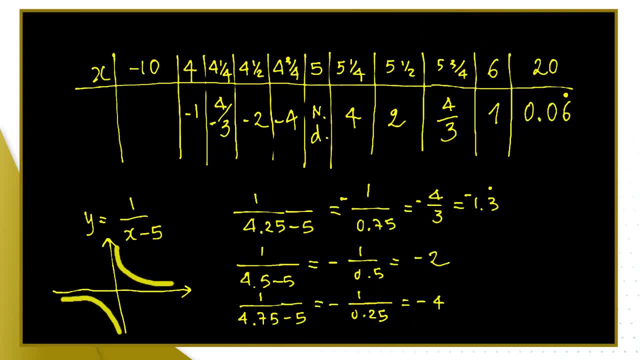 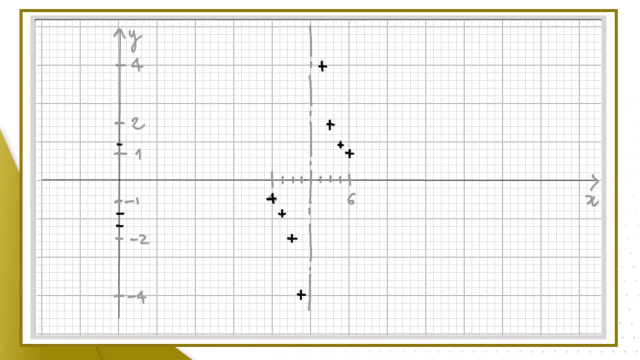 side minus 10 on the other side. that should be the equivalent value. minus 10 minus 5 is minus 15, so it should be minus 0.06, recurring so under 0.01, so very, very close to the x-axis. so on minus 10 and on 20, so really large. 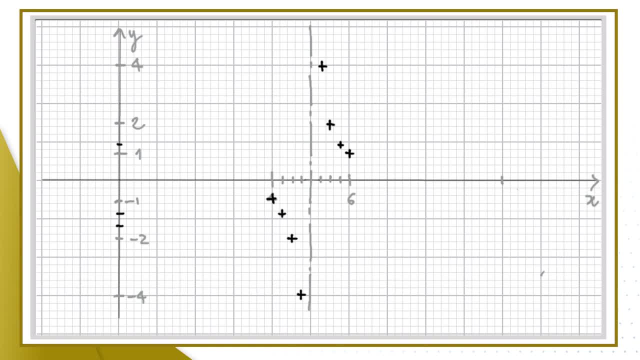 so we expect the graph to behave like this, this sort of behavior, and I'm implying that we're not touching the x-axis and we are not touching the asymptote, but we are approximating it. what to highlight? this line here is asymptote. it's a vertical line through 5,. 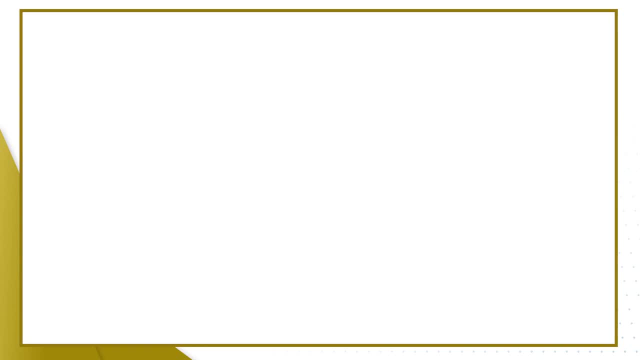 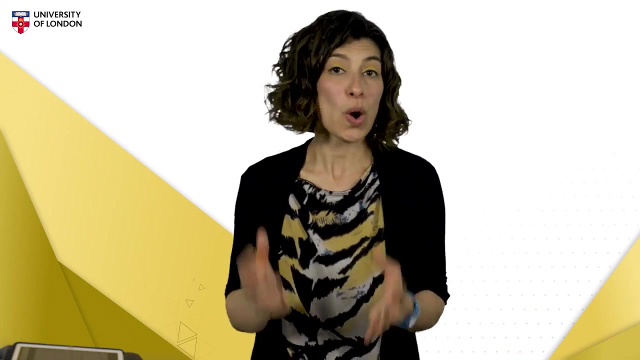 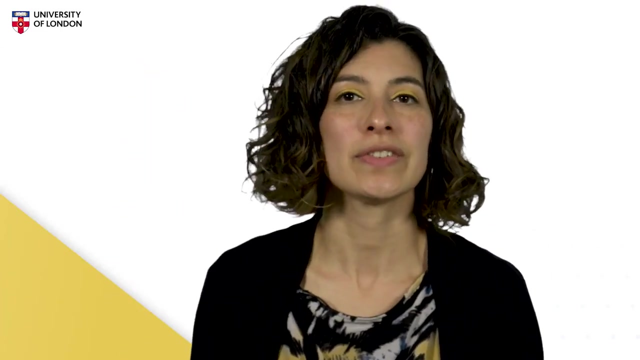 so it's the line of x equals 5, that's the symmetry line, and somewhere under that we humanly string this line abraire. if your graph doesn't look quite symmetrical- and it should be- then you can always leave a note saying that the two branches of the graph should be symmetrical. 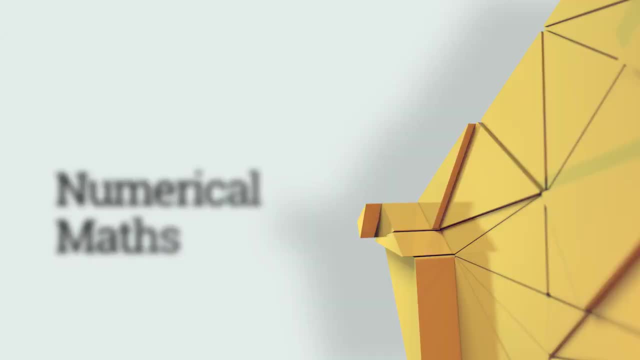 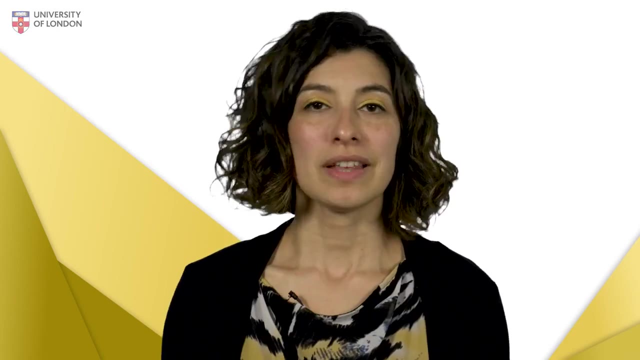 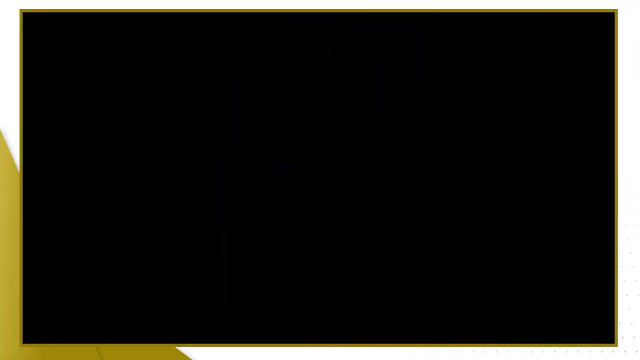 you, we just looked at reciprocal functions because we only have the linear functions. so we take Q1, communicate between the phases. there's another type that also has a ratio and it's a rational function. For example, the function with expression y equals x over x squared minus 1.. 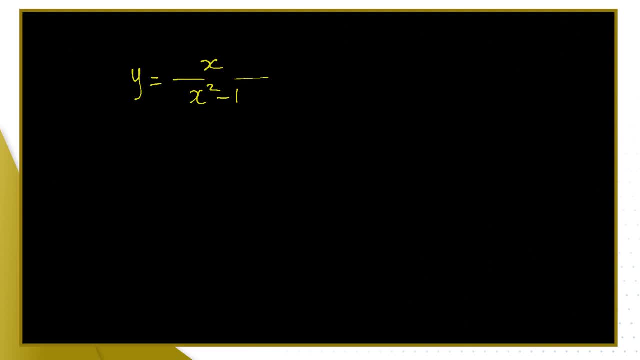 The denominator of this function, when calculated in x equals 1 and x equals minus 1, will be 0. Again, division by 0, which we can't have. So the domain will be r, except the values that make the denominator be 0, which is negative. 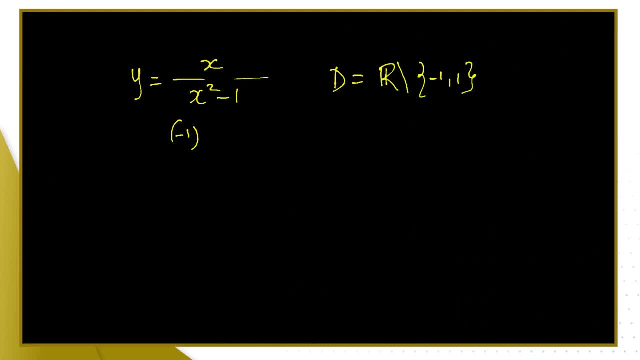 1 and 1.. That's because minus 1 squared minus 1 is 0, and 1 squared minus 1 is 0. So we expect to have two vertical asymptotes, one in negative 1 and the other one on 1.. 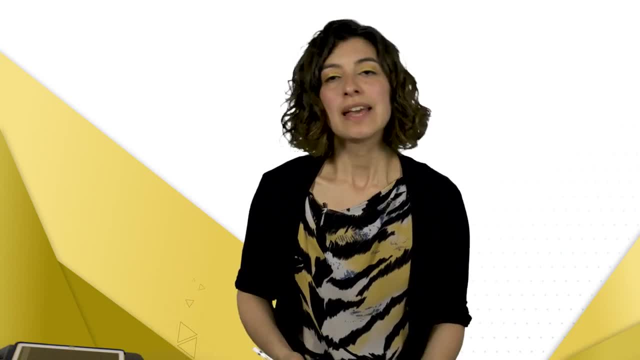 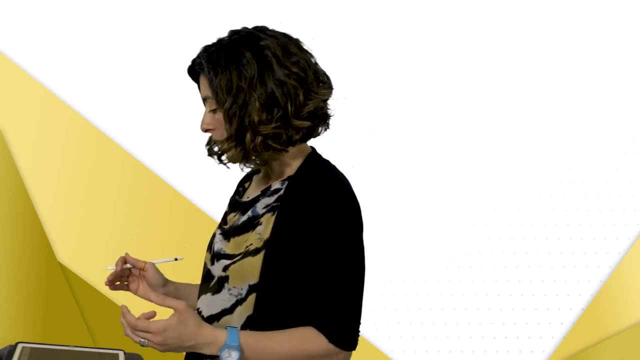 But what will the graph look like and how do we prepare for this? Well, the method is similar to what we've done for reciprocals, So I'm going to show you the graph plotted in graphing software. So this is the graph. 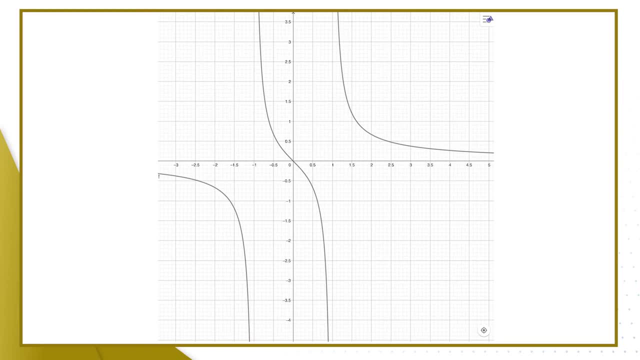 And we have. I'm just going to zoom in here and on negative 1 and 1, we have vertical asymptotes as in: we have no graph there and the function, the rest of the graph, is approximated to that line. 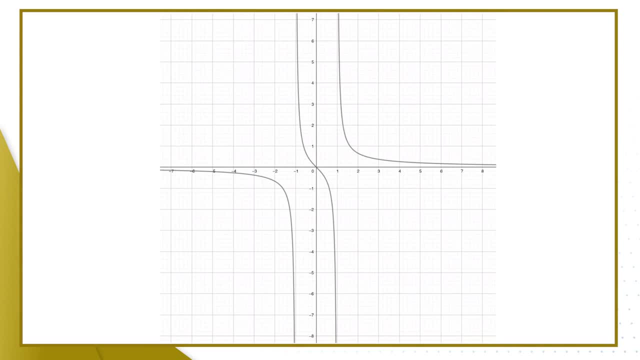 We grab the graph, we have it here, so let's just make some notes on top of it. So the asymptotes, That's with equation x equals negative 1, and the other asymptote over there, Equation x equals 1.. 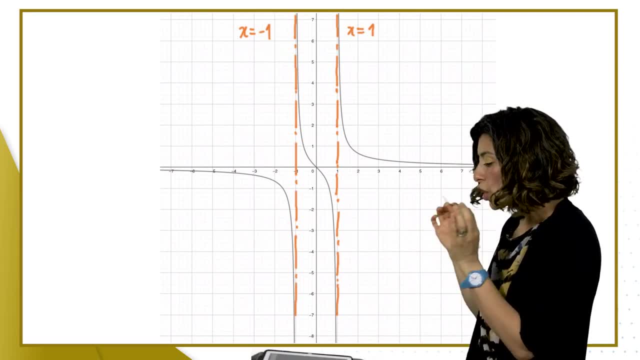 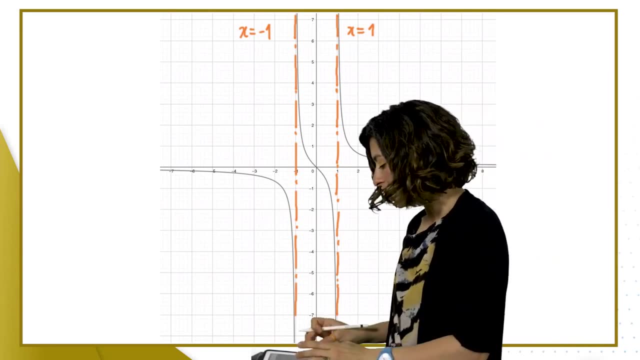 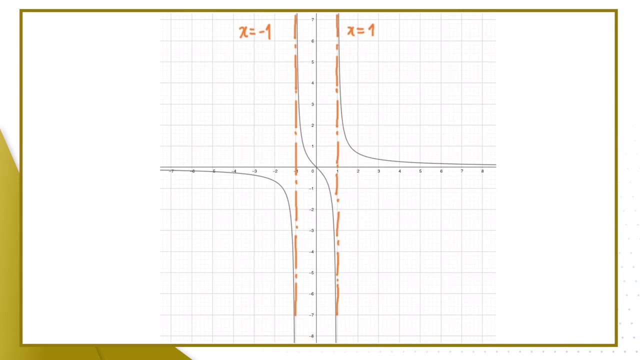 And in terms of table of values, we're going to choose values close to these asymptotes. OK, And enough detail in the middle to account for this really nice wiggly behavior around 0.. So I would suggest that we will use a number that's far away from the asymptote. 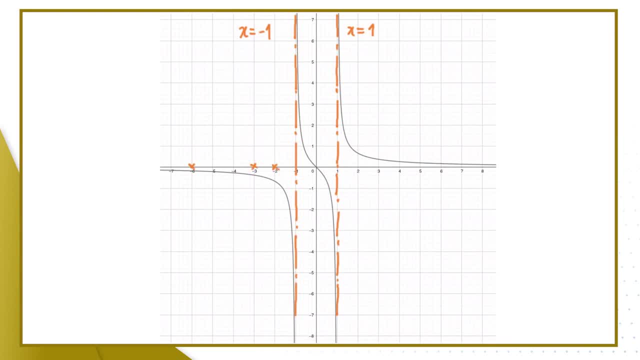 And then, as we get close, we want detail. So, in between minus 2 and minus 1, I suggest at least four points. The closer to minus 1, the better. So I'll recommend that we'll use values of there. 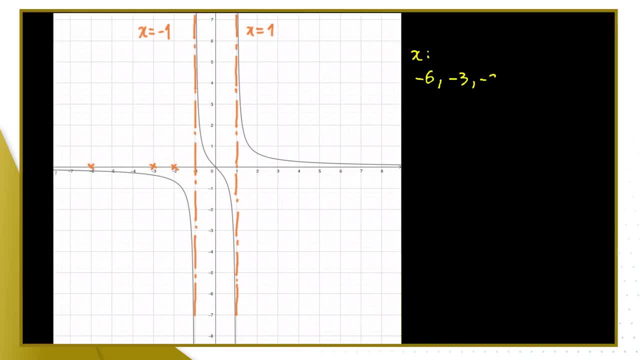 So x minus 6,, minus 3,, minus 2, and then between minus 2 and minus 1,, at least minus 1 and 3 quarters, minus 1 and a half, minus 1 and a quarter and, if needed, a little bit. 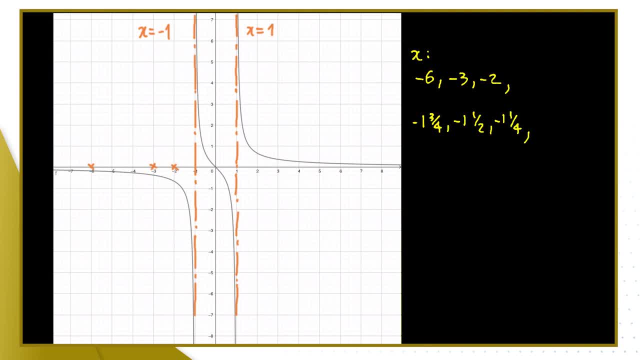 of finer detail. Then we skip the minus 1 because it's not defined there, And then we'll do minus 3 quarters, minus a half, minus a quarter the value in 0, and then the symmetrical values. So that's why I recommend you start with. 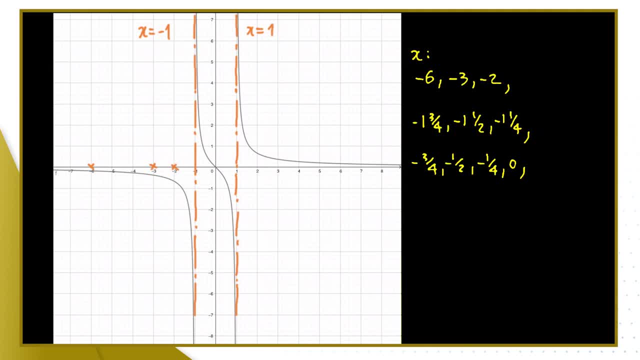 How would you know that without the graph? Well, we based it all around the asymptotes. So we chose a value far away from the asymptote, And then, as we get close to the asymptote, finer and finer detail, at least quarters. 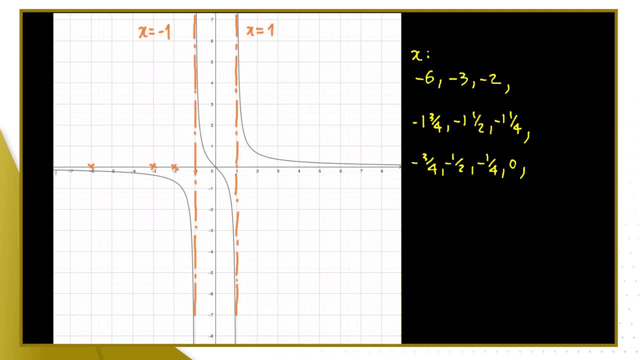 of interval between the values, That then between the asymptotes, between minus 1 and 1, again, fine detail. and repeat the same pattern symmetrically, If you choose the values of x symmetrically, take into account where the asymptotes are. 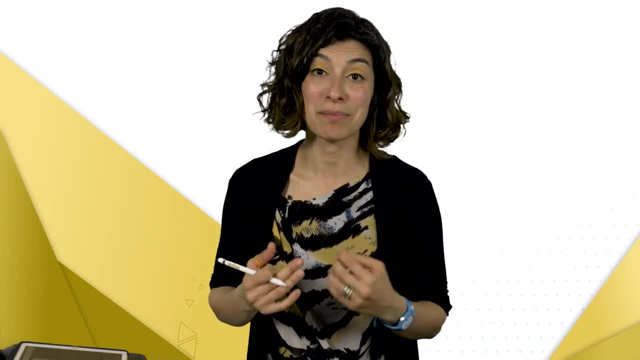 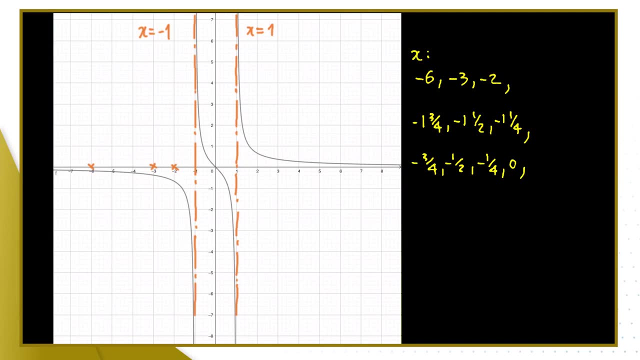 then the symmetry of the graph will be sorted out automatically by that choice of values, As before. this function also has a horizontal asymptote That's highlighted here in green, And it is the x-axis. once again, You might wonder: Do we have horizontal asymptotes that are not the x-axis? 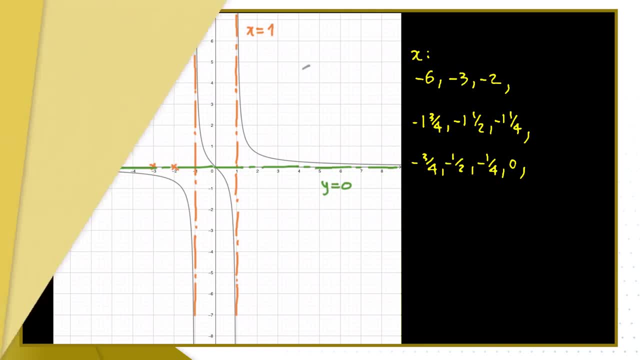 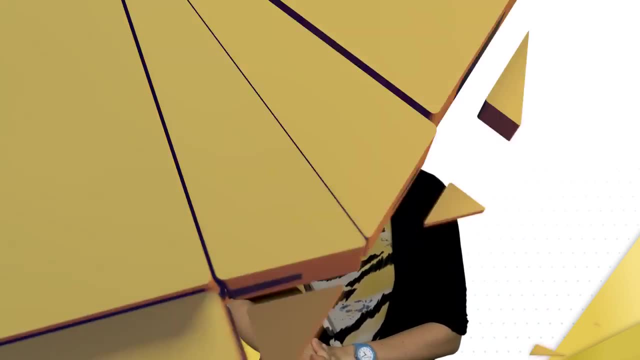 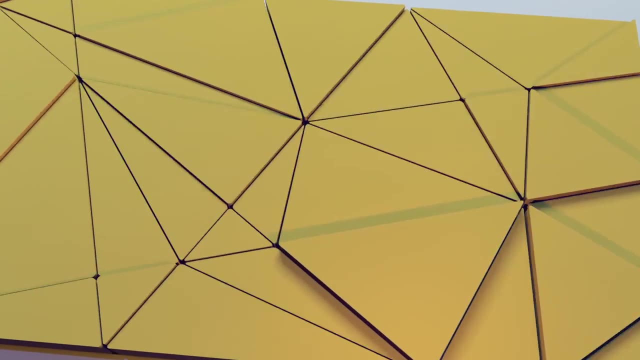 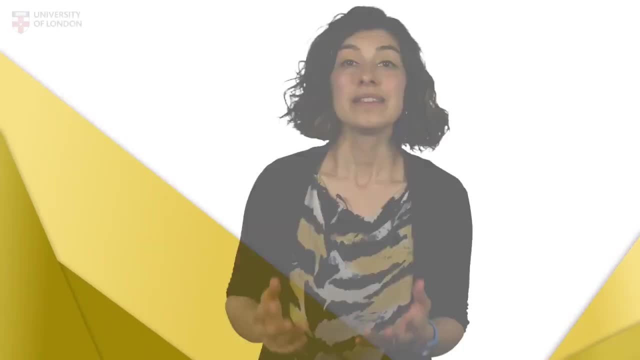 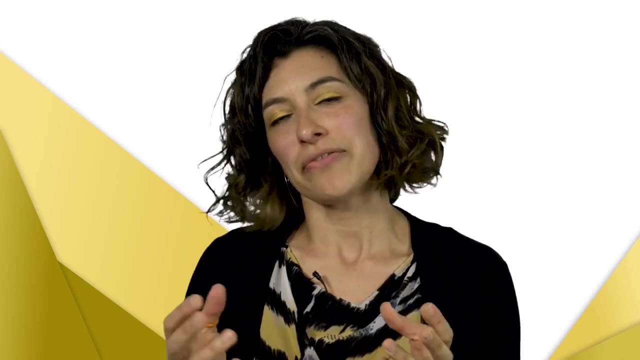 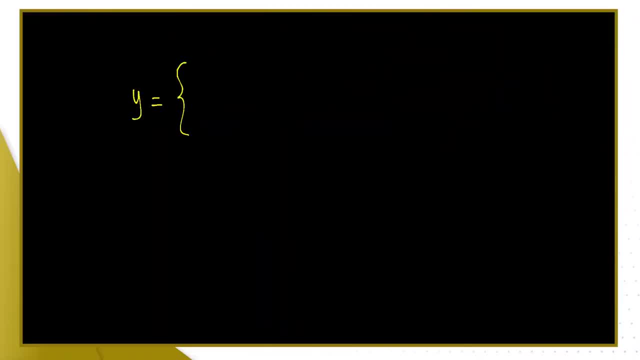 OK, OK, That's all I got. That's all I've got. OK, OK, OK, Thanks, Bye, Bye, Bye. two expressions. We have y equals x, and that's whenever x is less or equal to 5. 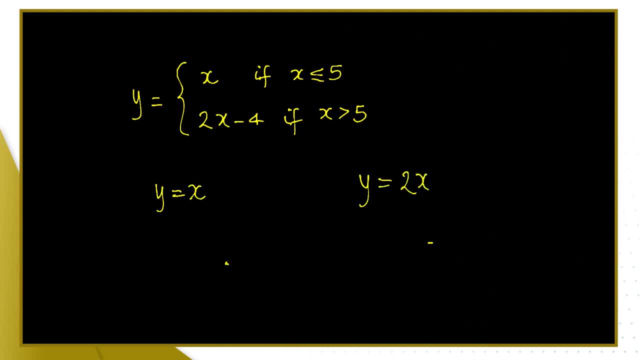 and we also have y equals 2x minus 4 for values of x greater than 5.. We're basically plotting two graphs: y equals x is a straight line with gradient 1 going through the origin, and y equals 2x minus 4 is a line with gradient 2 with minus. 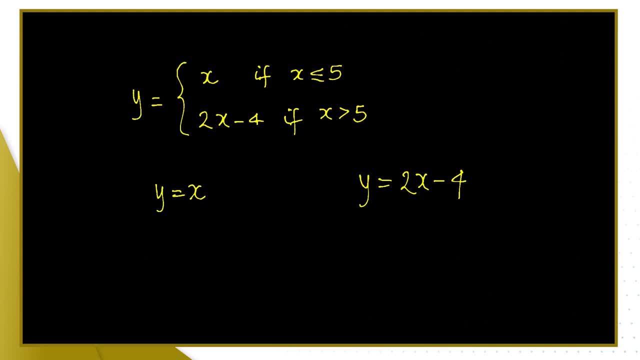 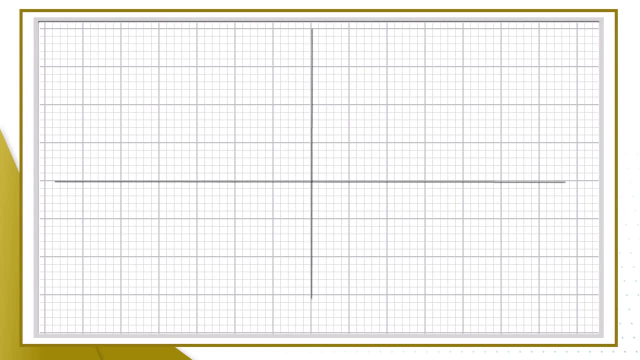 4 as the y-intercept, So we could sketch those to start with and then make sense of the branches later on. So let's plot the lines: y equals x. we need a scale here. we had a 1 to 1, but we're gonna choose. I'm gonna choose this value here. 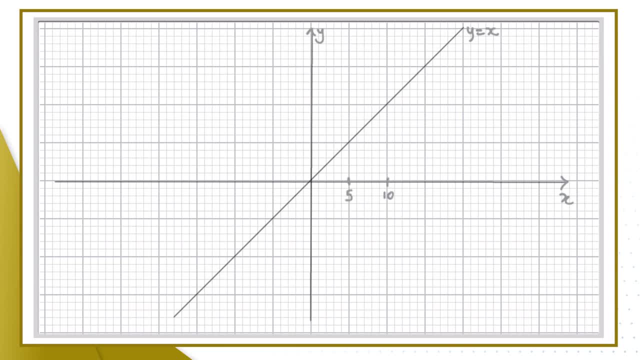 to be 5.. 10 and so on and so on. and on the vertical axis, the same scale. We already commit to it because we already drew: y equals x in 1 to 1.. Okay, and now y equals 2x minus 4, minus 4 and a slope of 2.. So that point, and that point, and that point. 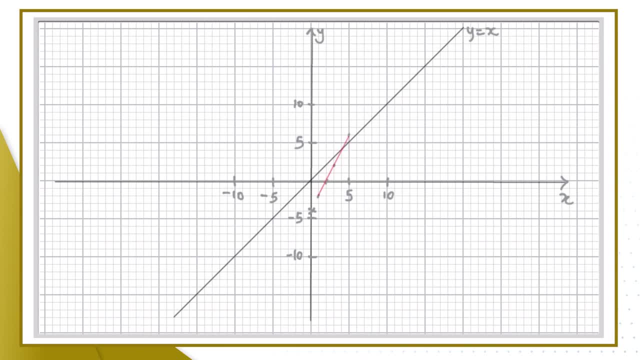 So let's get a line through all of this. So that is y equals 2x minus 4.. Now how do I know how to draw this graph? So let's look at the expression again. It's y equals x for x up to 5, including 5.. So up to x equals 5. we have the first graph. So I'm 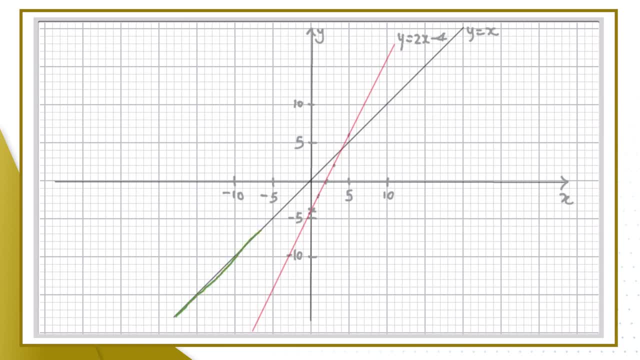 gonna use the green pen. so we have this graph, right, And then I'll will put it died in graph in green up to 5, including 5, and then we have the other one. So I want to include this point and I want to exclude that point. The branch of y equals x. 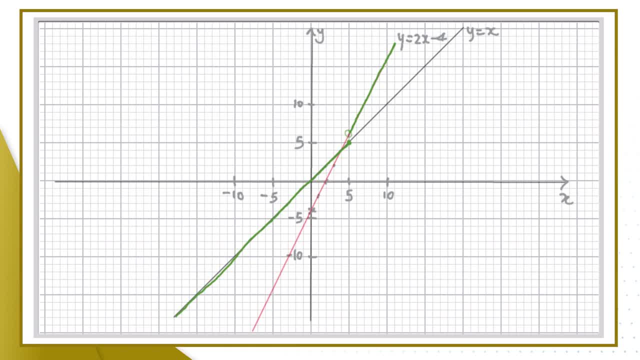 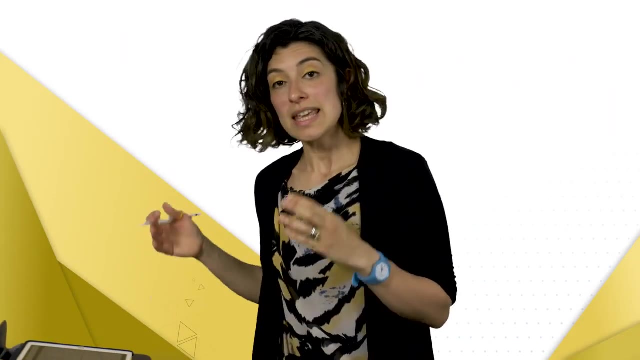 includes the point and the branch y equals 2x minus 4, has an open dot on the point of coordinates and then is full line from then onwards. So that's the graph of a piecewise function. The functions we're going to have in the 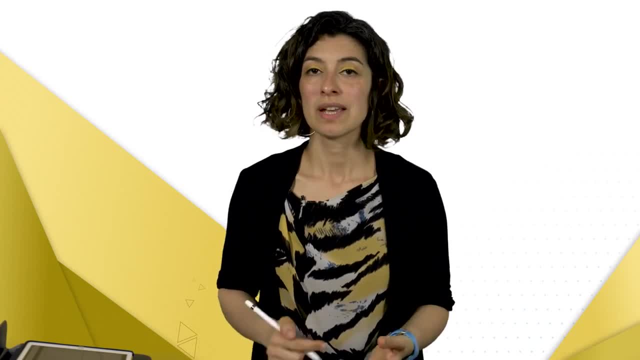 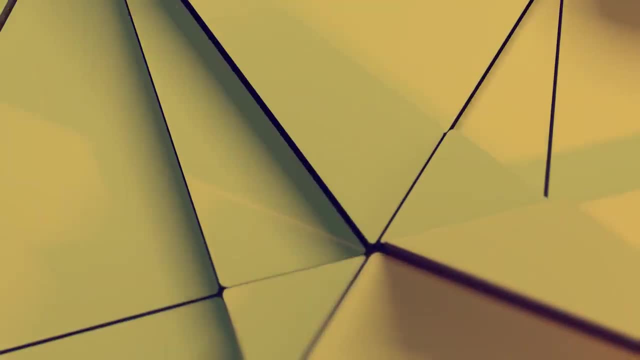 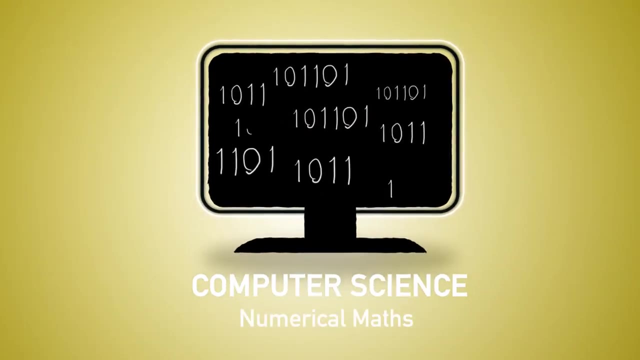 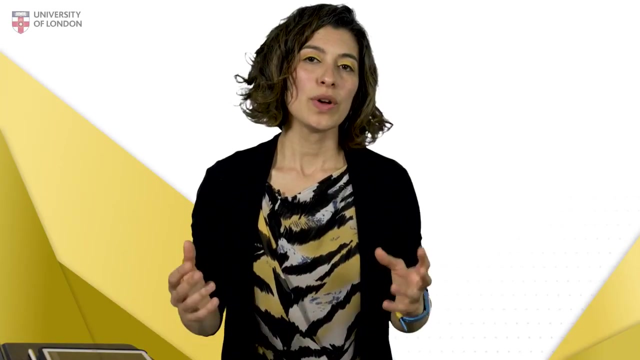 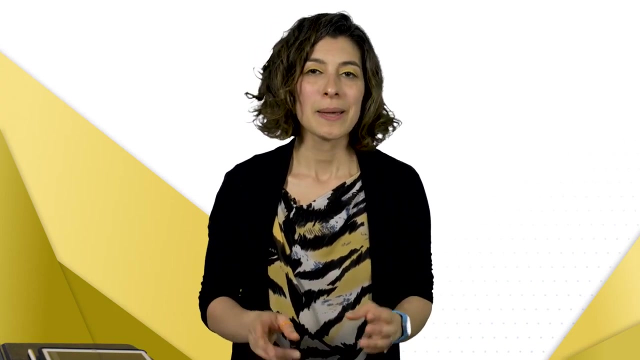 branches are going to be of the type we saw earlier: Straight lines, quadratics, cubics, reciprocals, rational functions. When you played with graphs of functions earlier, you may have noticed that some graphs looked pretty much alike, but their expressions were different. We're. 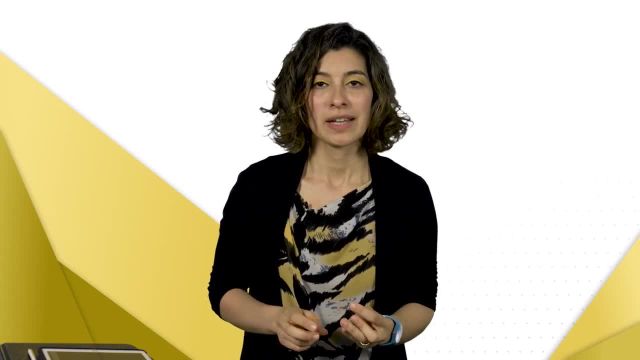 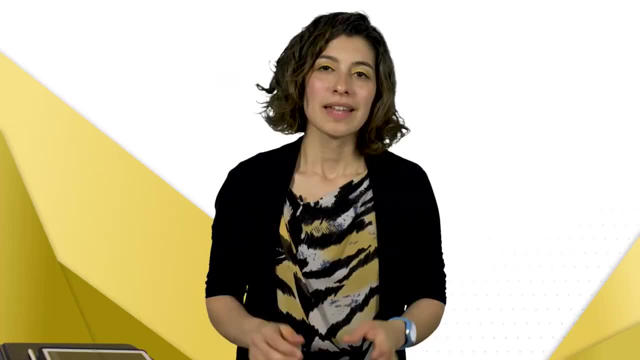 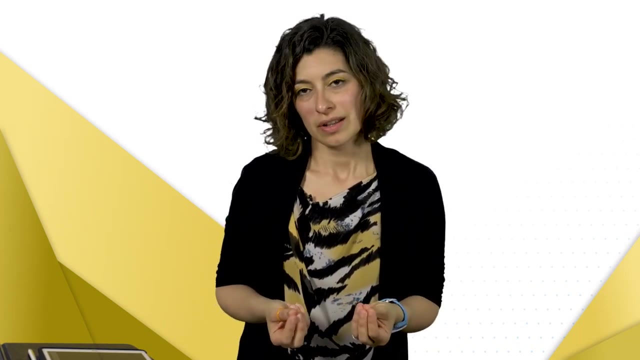 going to look at these cases and what is the mathematical reason for that? We're going to look at transformations of graphs, such as scaling, translations and reflections. Now, to make the most of the section, I wanted to bear in mind the key identifiers of a function. What I mean. 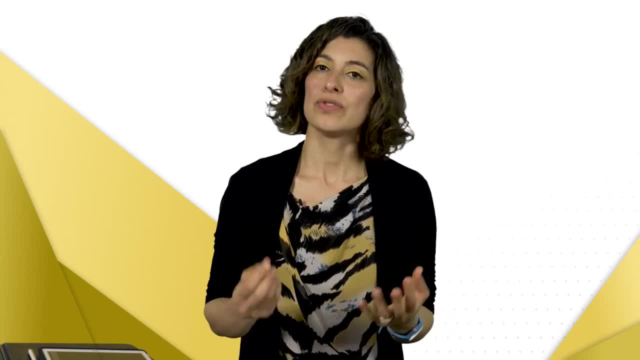 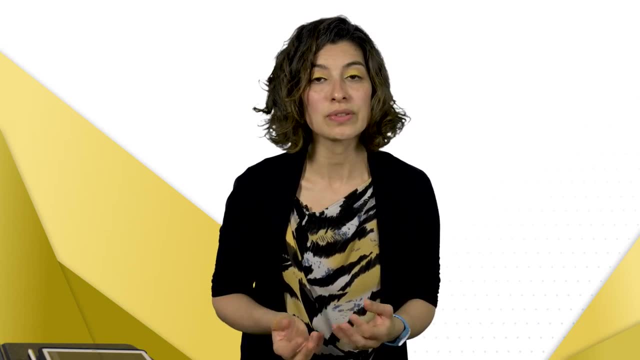 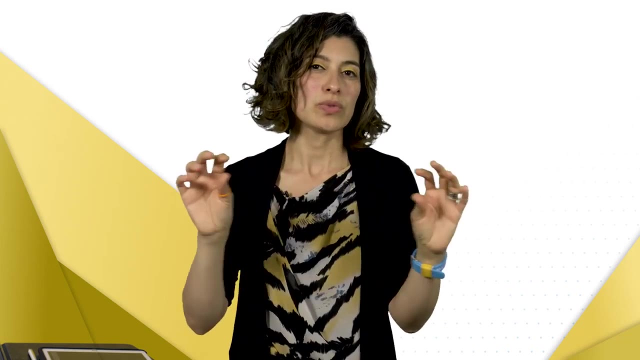 is that when you look at a graph or you study a function and if you notice details about the domain, whether there is there is a gap or a discontinuity, or there is a vertical asymptote or maybe more than one vertical asymptote- I wanted to bear in mind those bits of information about the domain and the 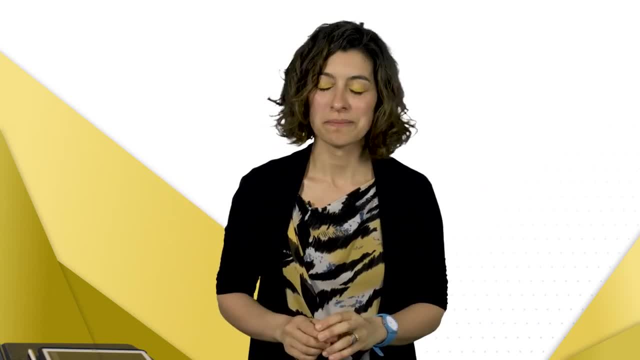 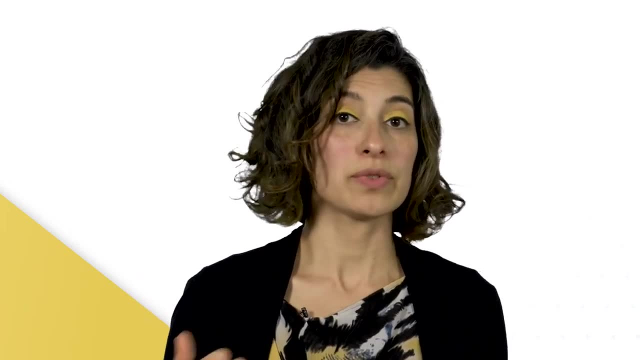 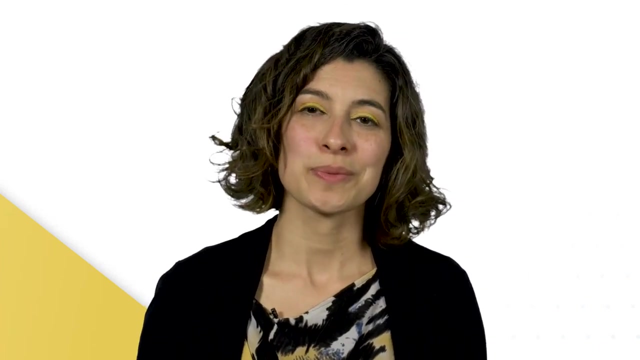 behavior on the x direction of the function. Thank you. Other things like zeros, meaning where the graph cuts the x-axis, or even intercepts, where the graph cuts the y-axis. Also, if they are horizontal asymptotes and where they are located, 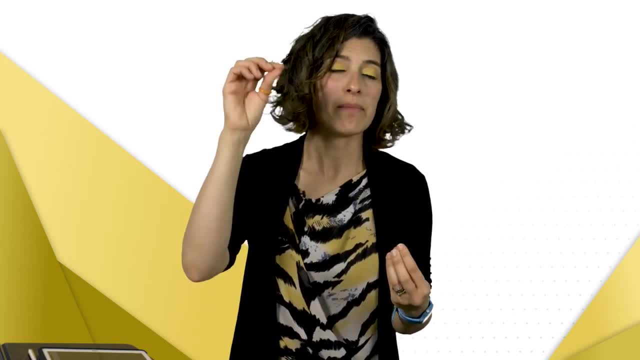 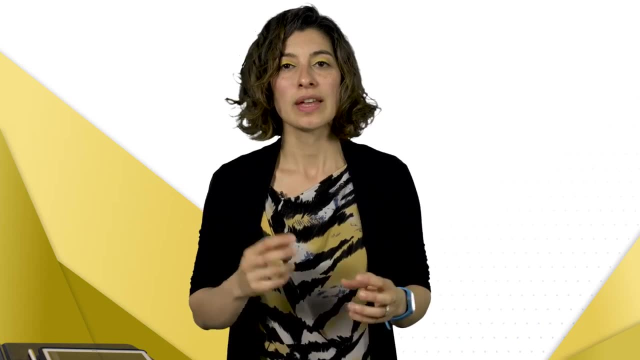 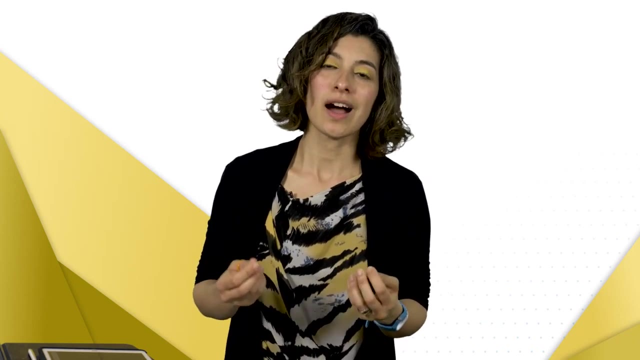 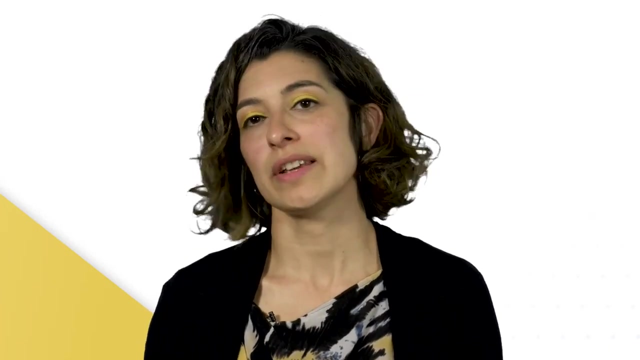 Other features, like extreme points, so where we have a maximum or a minimum of a function, where the function changes growth or decelerates growth, All these elements will be important to help you make sense of which transformations are happening to a graph. In some cases, like the quadratic function, we can even attend to details such as the vertex or the opening of the parabola. 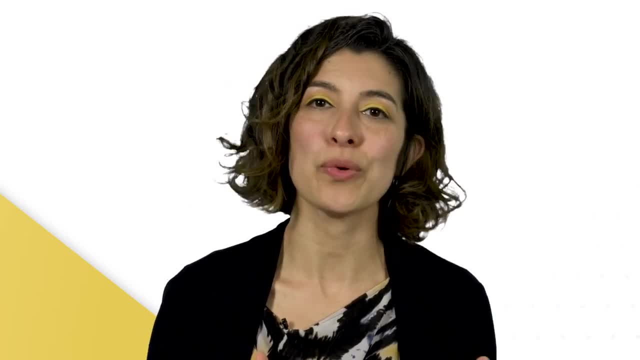 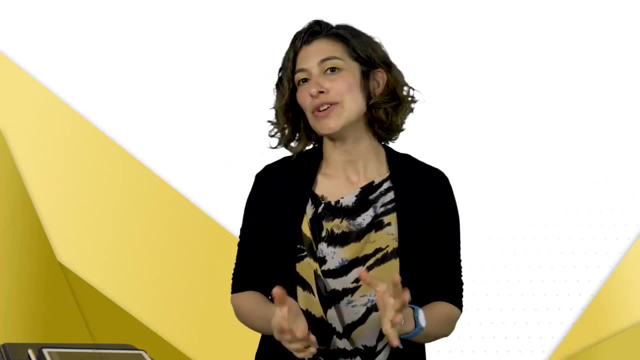 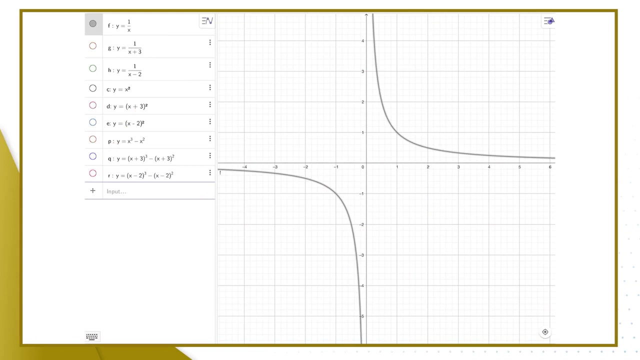 With straight line graphs, we'll be paying attention to the slope and whether it is ascending or descending, and what happens to transformations of that function. So join me, What do I mean by looking at these graphs? I'm going to picture here the graph of 1 over x. 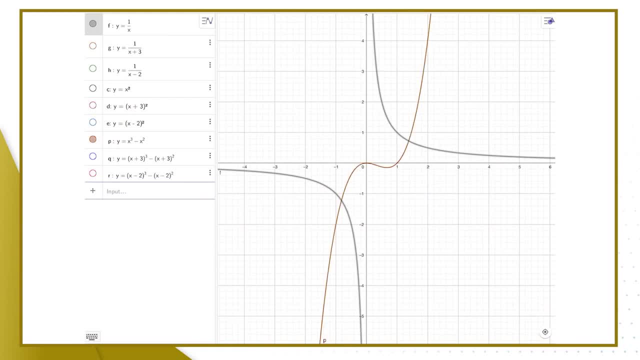 And I want us to think of the graph of: y equals x cubed minus x squared. So we're looking at those two And we're going to look at transformations of each of them. So let's focus first on the reciprocal: y equals 1 over x. 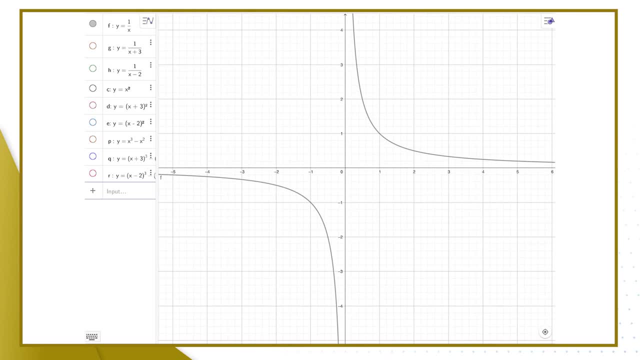 Now, in this function, one of the key features is that it has an interrupted domain. The 0 does not belong to the domain, and it has a vertical asymptote at x equals 0.. It also has a horizontal asymptote: at y equals 0,. the horizontal axis 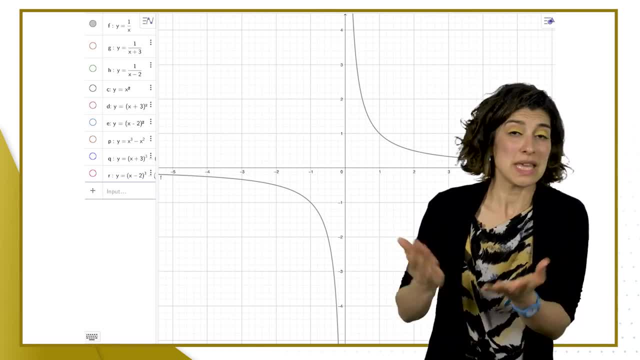 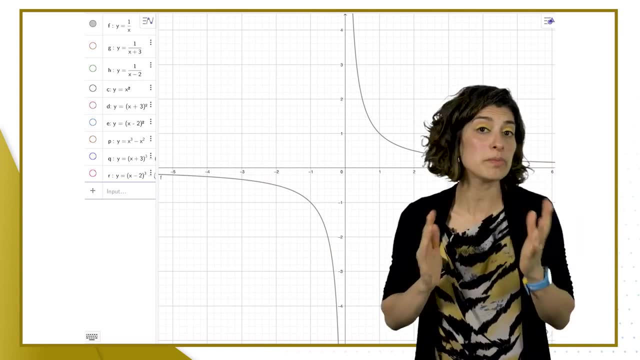 What would a transformation of this graph look like? Well, it will be this graph shifted somewhere else, either by a horizontal translation or a vertical translation, or a combination of both. We can reflect the graph on the y-axis or in the x-axis. 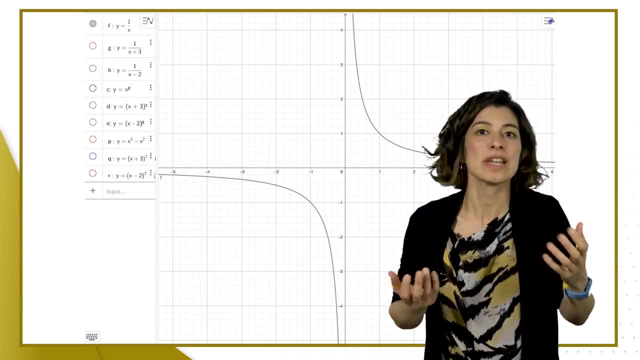 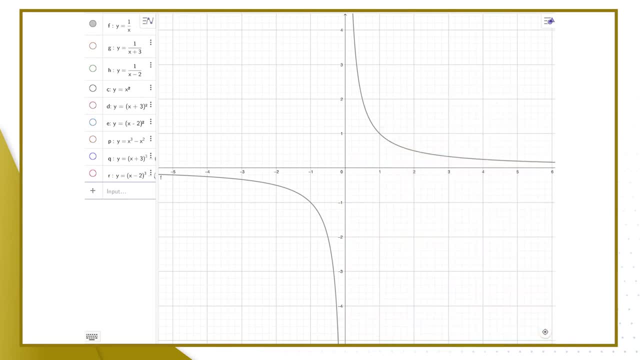 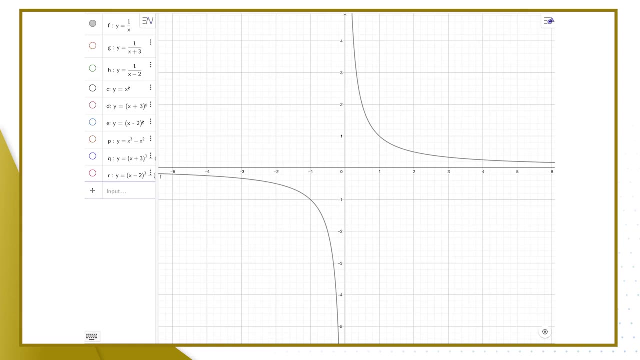 And we can also scale it up or shrink it, either in this direction or in the other direction. I don't mean by that to change the window like doing what I'm doing here. The scale there has changed, but the proportions of the graph are still the same. with respect to the scale. 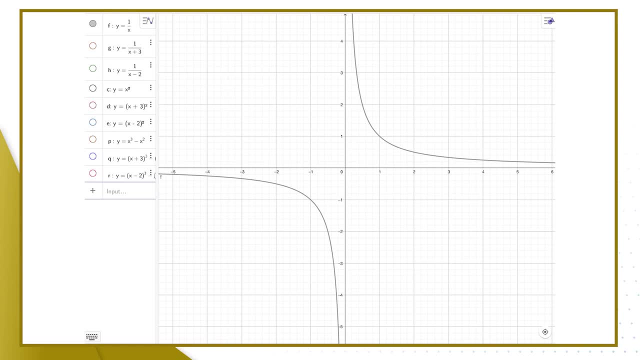 What I mean is absolutely having a different graph that stems from this one. So let's look at this one. Let's look at what the brown graph looks like compared to the grey one. So I started with a grey graph, which was the reciprocal. 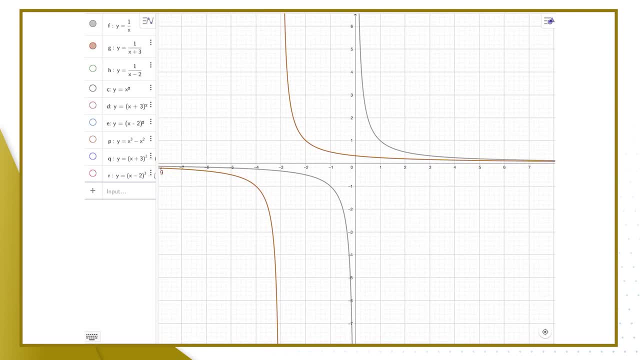 And the brown one. OK, yes, you can see the expression on my sidebar, But let's focus on the drawing at the moment. How would you describe? How do you get the brown graph? How do you get the brown graph from the grey one? 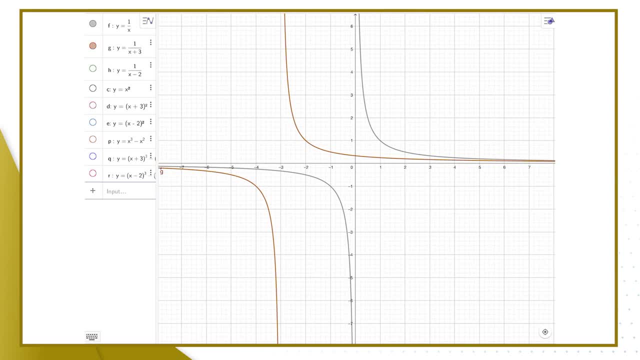 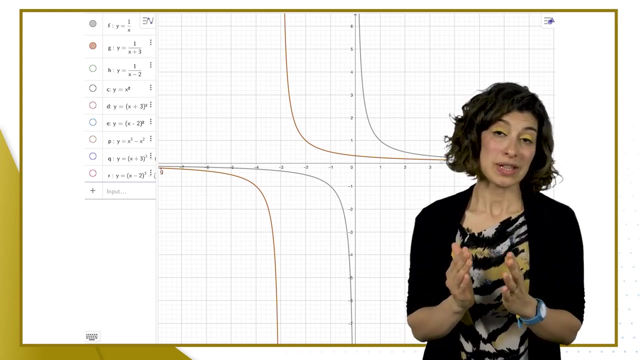 If we look at the discontinuity in the domain, the grey graph has an asymptote at x equals 0, whereas the brown one will have the same asymptote but at x equals minus 3.. So I shifted the graph 3 units to the left, so minus 3 units in the x direction. 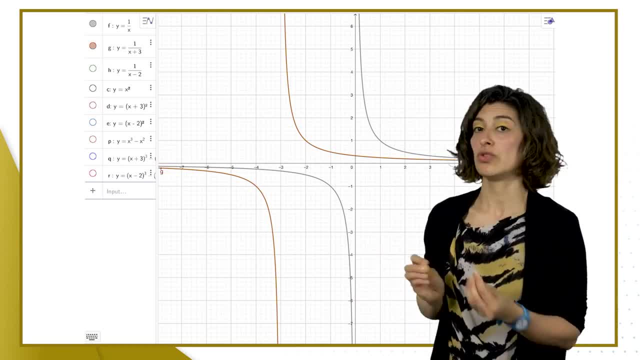 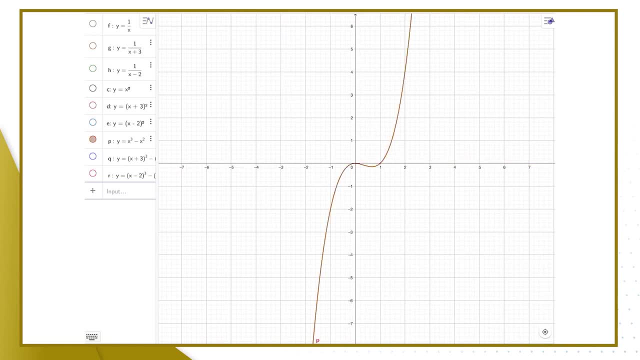 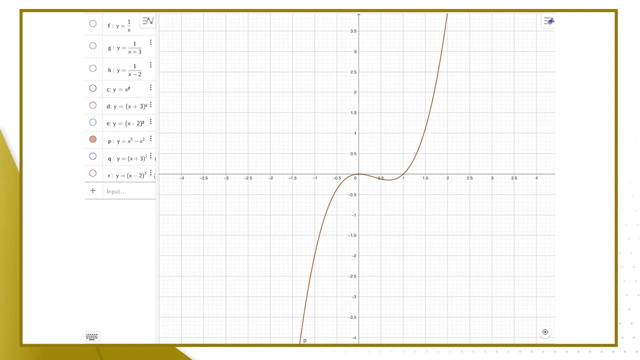 So that is a translation that brings the grey graph to the brown graph In the same way. the other example I had was the cubic. So now we're looking at a brown graph as our base graph, If I apply the same transformation of translating, meaning shifting this graph 3 units to the left. 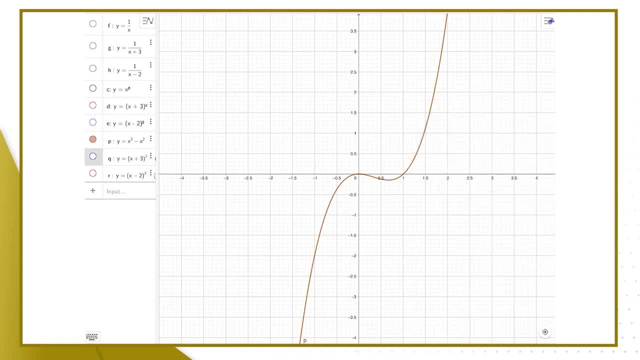 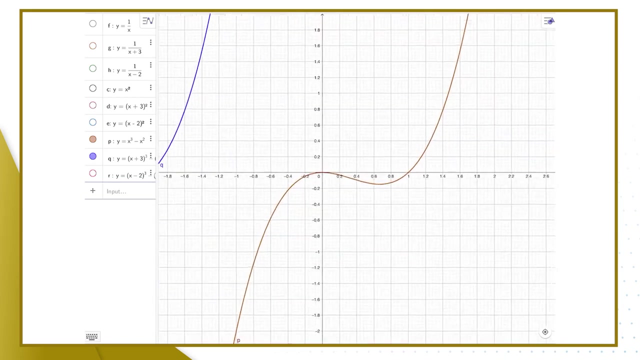 so minus 3 units in the x direction, I get that blue one And again, look that the point at the origin of the brown graph. it's now at a point when x equals minus 3.. The other zero of the graph of the brown graph, which was at 1,. 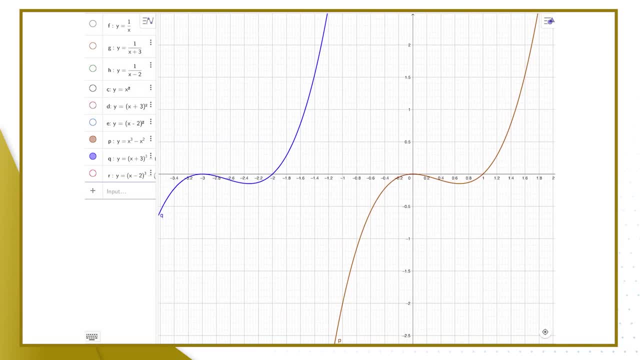 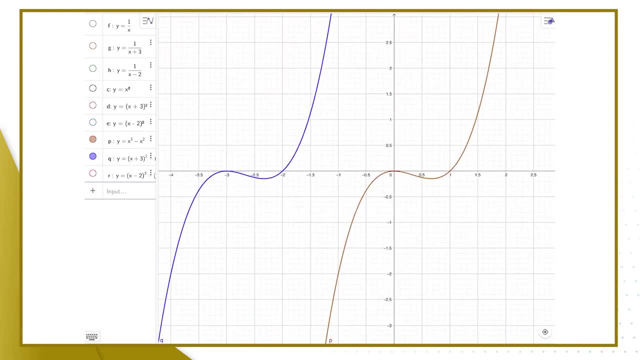 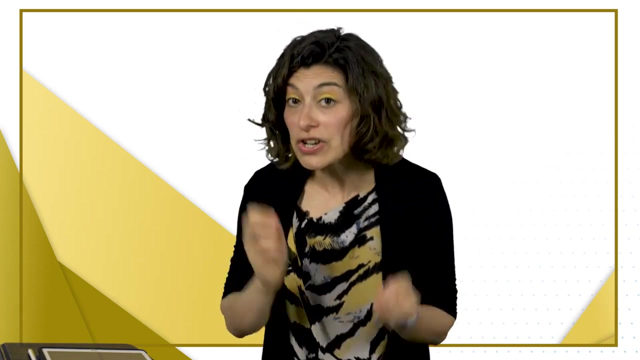 is now shifted to negative 2.. Again, 3 units to the left, so 1 minus 3, giving minus 2.. So this is what I mean by focusing on these key features of the graph to identify the transformation. Now, how does the expression of the function change when I do the translation? 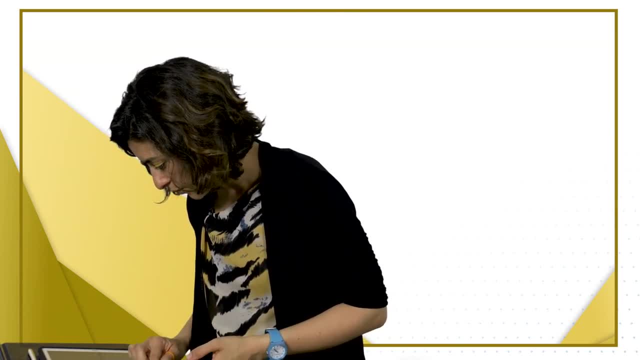 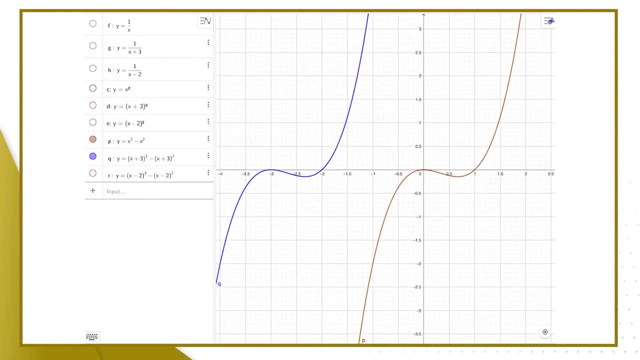 Well, let's focus then now on my toolbar. here on my sidebar, The brown graph has expression: y equals x cubed minus x squared. That's highlighted as my function p in this graph, The blue one, q is x plus 3 cubed minus x plus 3 squared. 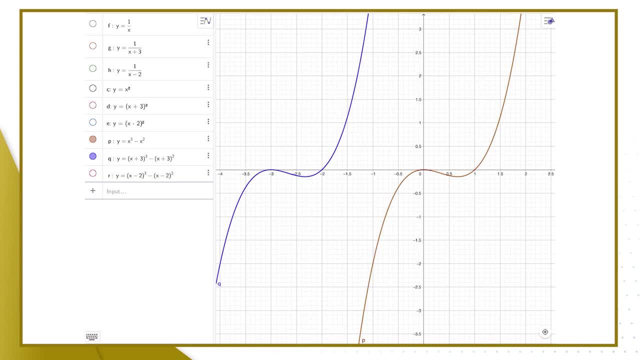 Just take a moment to think of what is happening between the two. The cube bit and the square bit look pretty much the same on both functions- p and q, but the q function is like the p, with the x replaced by x plus 3.. 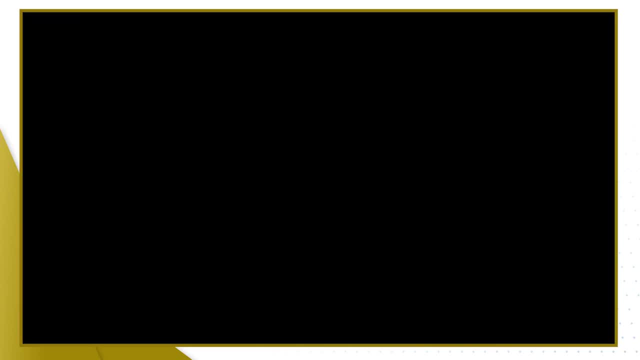 So I'll write that down, making sure we see that. So p is y equals x cubed, minus x squared. and then q is y equals x plus 3 cubed, minus x plus 3 squared. And I'm just going to take a moment to clarify the notation. 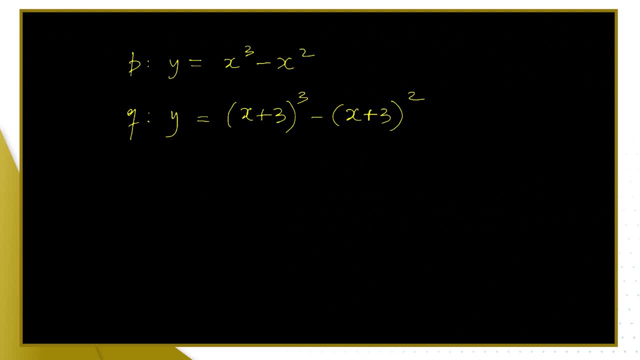 When I say p, such that y equals x cubed minus x squared, I mean that y is a function of x and the function is called p. And that means I could also write that p of x equals x cubed minus x squared. 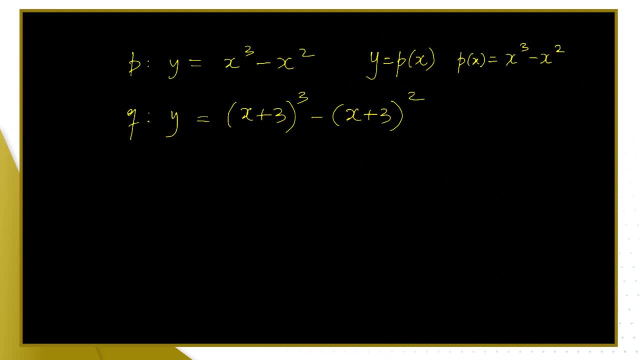 And that means I could also write that p of x equals x cubed minus x squared, And that means I could also write that p of x equals x cubed minus x squared. So these are ways of writing the same thing. So, in the same fashion, q of x is x plus 3 cubed minus x plus 3 squared. 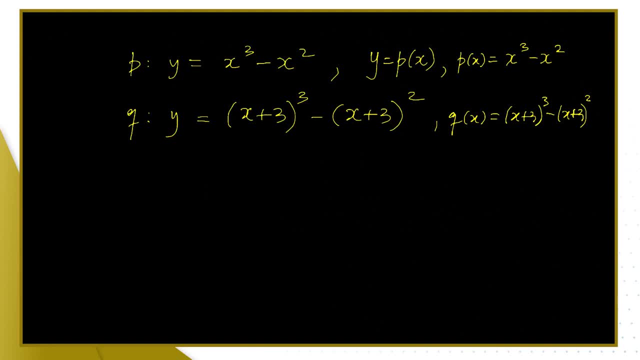 So, notation out of the way, The similarity between the two functions is that I'm doing a cube minus a square and I'm using the same thing- cubed minus the same thing squared. and I'm using the same thing, cubed minus the same thing squared. 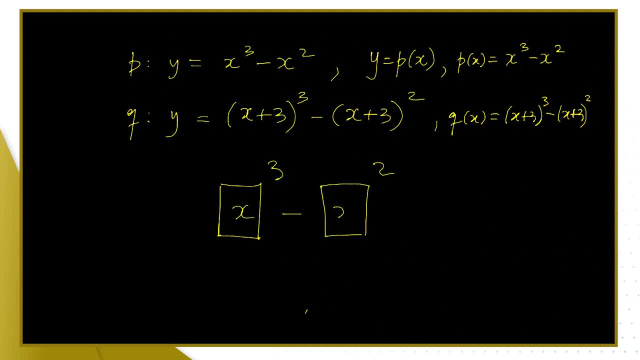 same thing squared, whereas in p I have an x, but in q I have an x plus 3, and obviously I need to put brackets when I'm cubing and squaring, but I've got the same, So that x plus 3 is responsible. 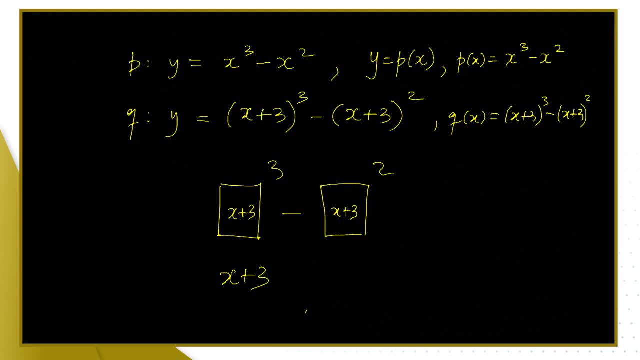 for translating the graph minus 3 units in the x direction. So how do I write this down? I'll say that the graph of q of x is a translation of the graph of p of x minus 3 units in the x direction. Now some of you may be wondering. 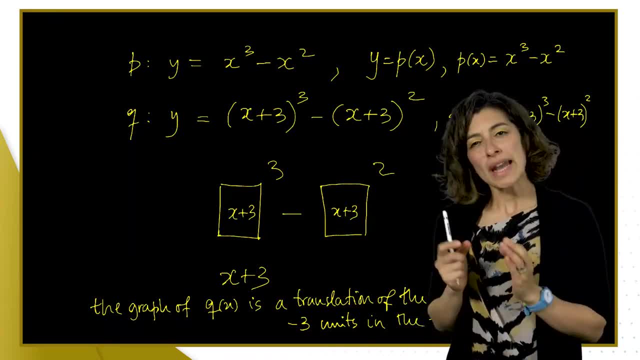 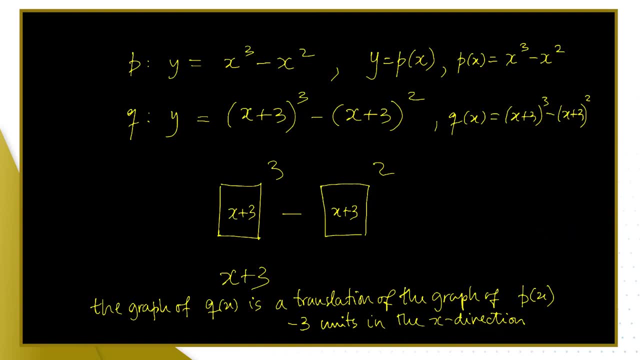 what does this mean? Well, it means that the graph of q of x is a translation of the graph of p of x minus 3 units in the x direction. Why minus 3 when I have x plus 3?? Good question. It can be confusing. This is where I think it's. 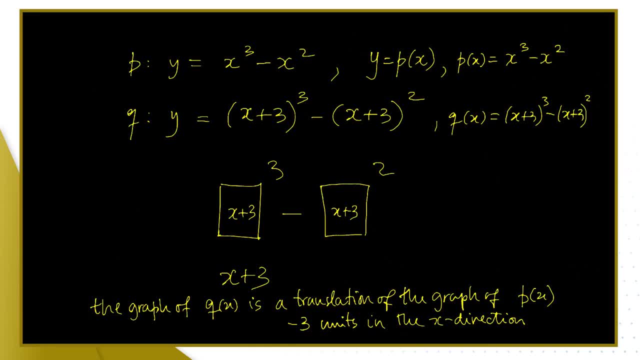 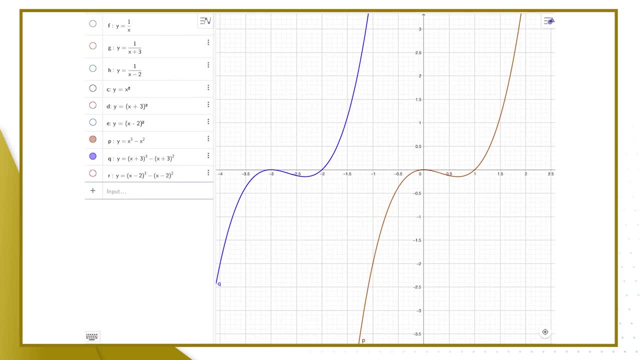 important to focus on the key identifiers of the graph. So let's look again at the graph we had, And the brown function is p. If I use as key identifiers the point when x is 0 and when x is 1,, what did I have to do to the? 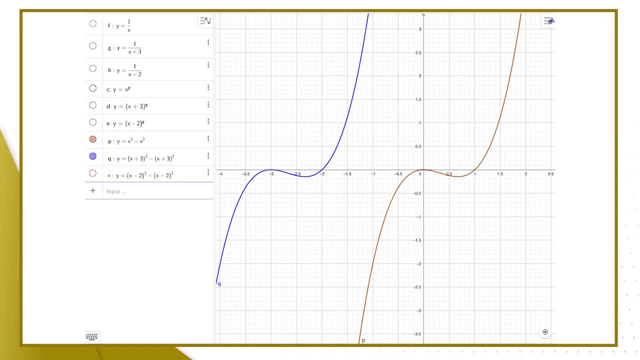 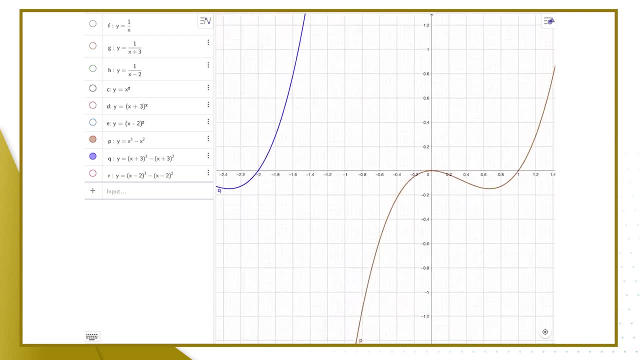 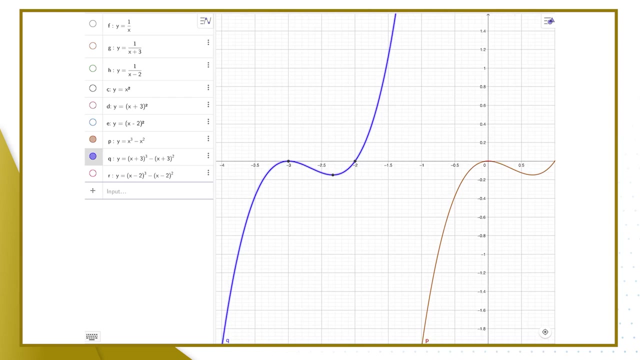 x values to end up in the same important points of the blue graph. This point here at 0 became the point here at minus 3.. So from 0 to minus 3, I had to do minus 3. And the same works from. 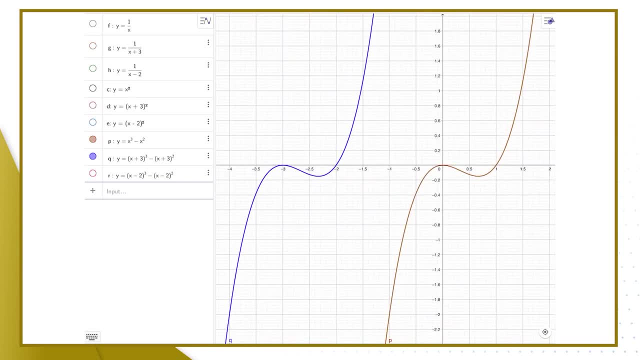 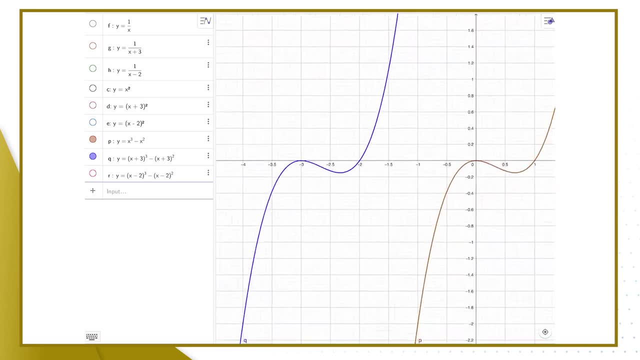 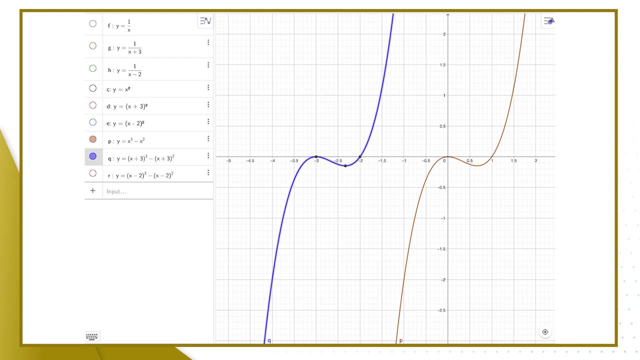 that point 1 on the brown function. What do I have to do to have minus 2?? Well, I do minus 3 again. So that tells me it is minus 3 units on the x direction. Let's see if that makes sense with. 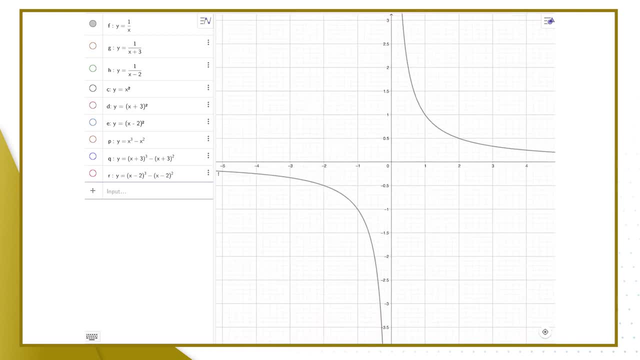 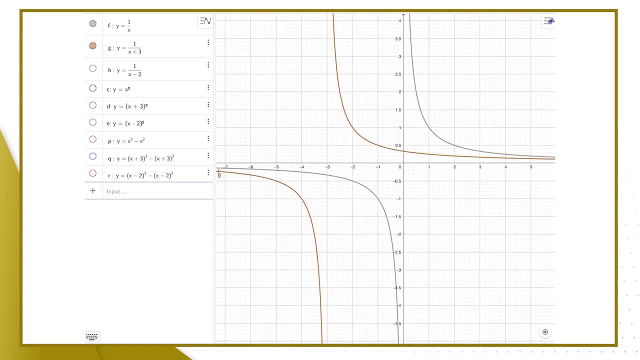 the other function. We had the reciprocal and the other function is there In terms of the expression I had, y equals 1 over x and the translated by minus 3 units in the x direction is 1 over x plus 4.. So I have minus 3 units on the x direction And the translated by minus 3 units in the x direction is 1 over x plus 4.. 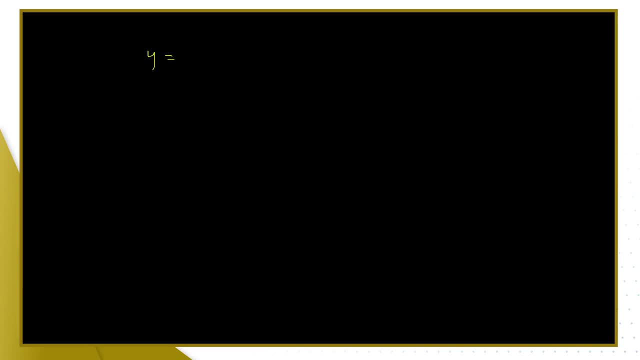 I'll just write that down. So on, y equals 1 over x. when we translate in the x direction by minus 3, we get y equals 1 over x plus 3.. You can think of it as we're doing: 1 over x minus. 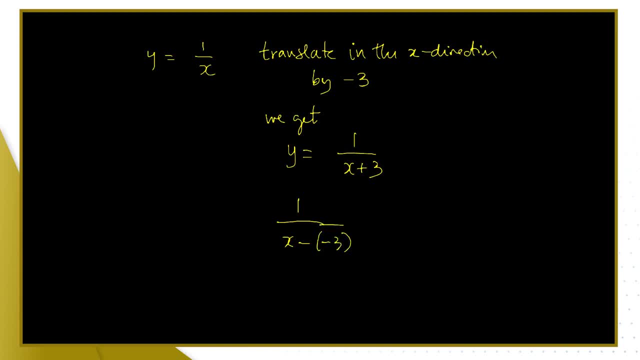 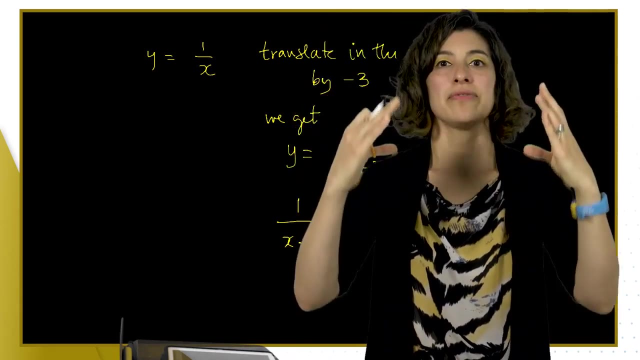 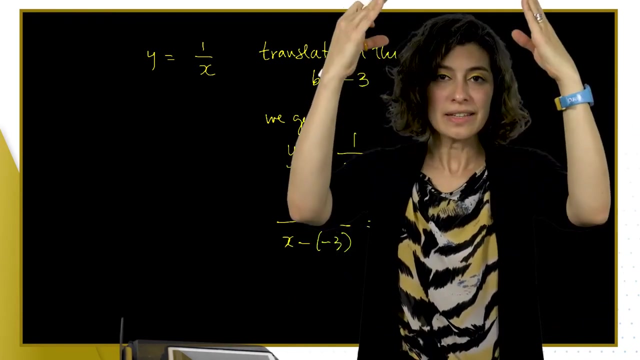 the translation part, Because the translation is minus 3, is 1 over x minus minus 3,, which is plus 3.. We can also translate vertically and that means we're going to move the graph up or down. That means we are changing the values of y by adding or subtracting a constant value. So if we start, with y equals 1 over x minus y and then multiply it by 1 over x minus y by adding or subtracting a constant value. So if we start with y equals 1 over x minus y and then multiply it by 2 over x, we get: 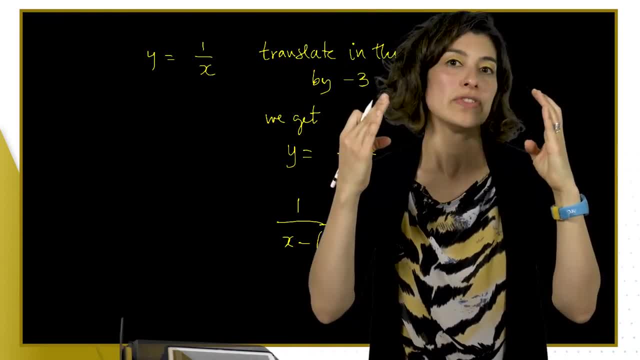 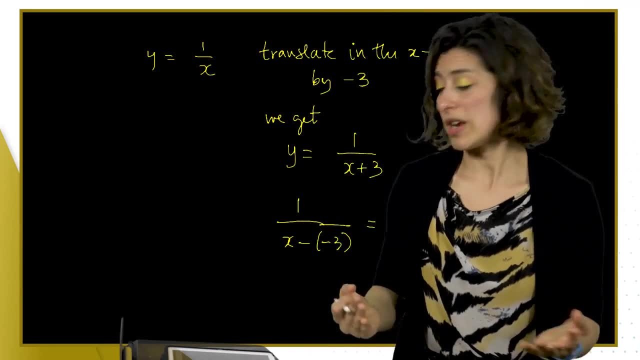 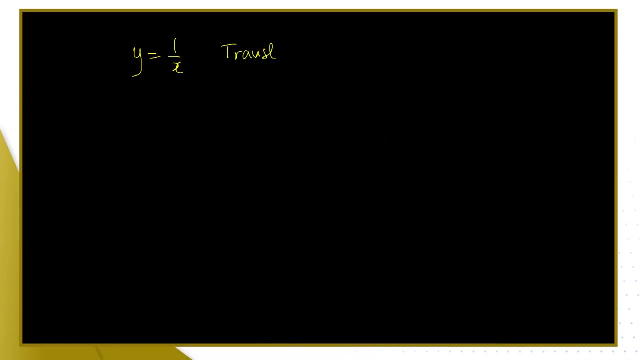 1 over x. if we want to translate it upwards by 5 units, all I have to do is add 5 to the expression. So, as simple as y equals 1 over x. when I translate by 5 units in the y direction, that means I'm adding 5 to everything. so I'm doing. 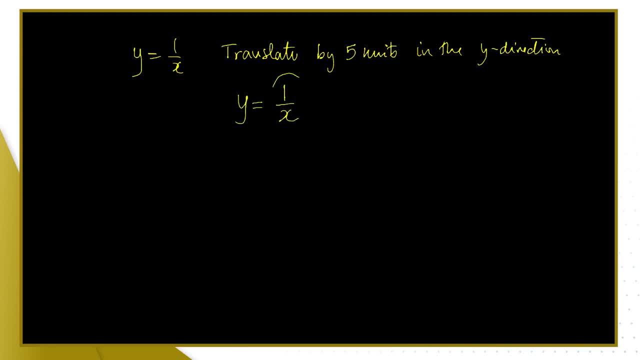 y is what I had before as y, which was 1 over x, and now add 5 to it. If I wanted to translate down 3 units, I would do: y equals 1 over x minus 3, so this function has. 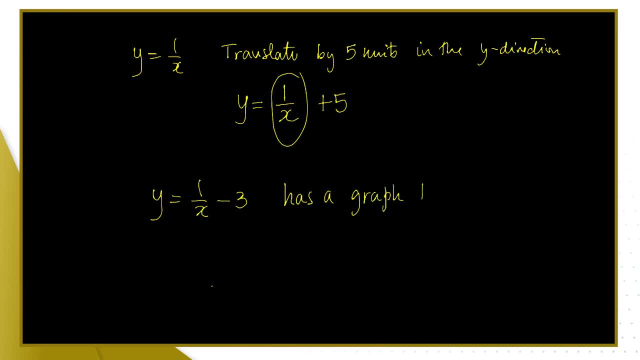 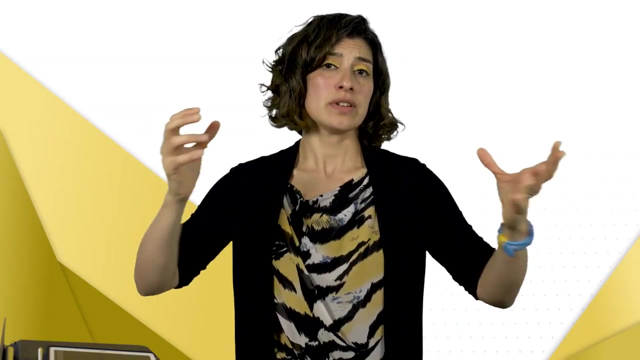 a graph- that is the translation of the graph- y equals 1 over x minus 3 units. in the y direction We're also looking at scaling and we're going to scale graphs in the x direction. We can scale them up or down. We're always going to take it from. 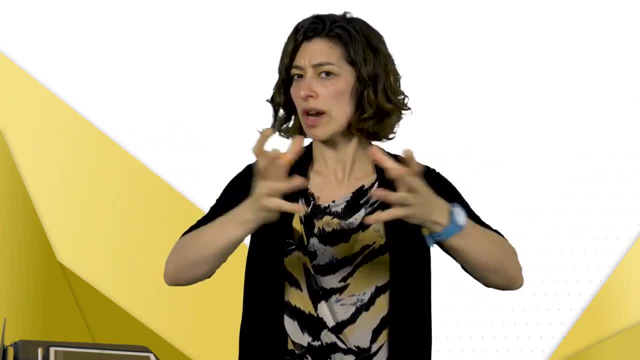 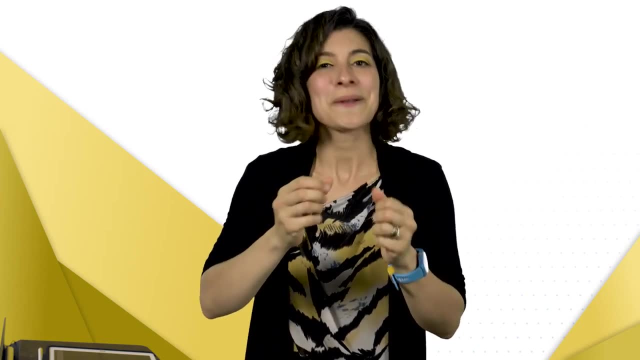 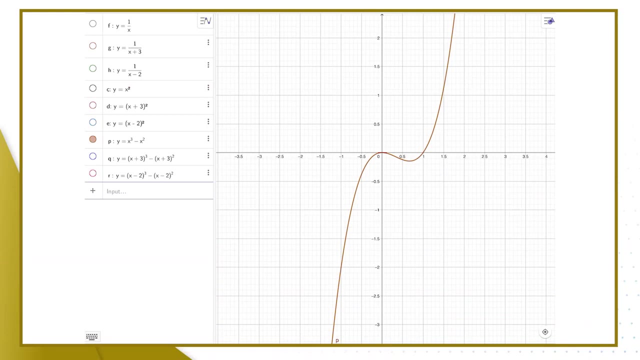 the point of view of scaling up. so if we scale up by a factor of 2, we are doubling. If we're scaling up by a factor of half, we're going to shrink it, And we can do that in the y direction as well. So back to our cubic function p. this y equals x cubed minus x squared. 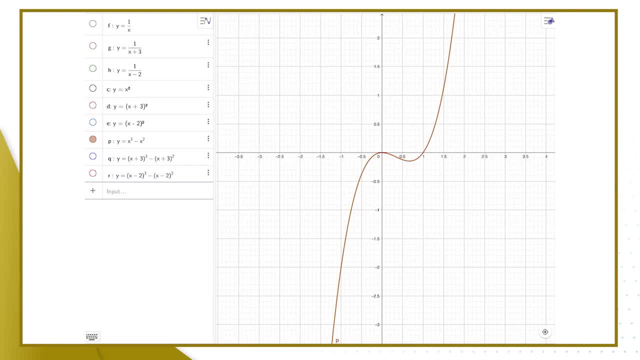 let's do some scaling. I'm going to create another function. I'm going to multiply everything by 2.. So I'm going to multiply, I'm going to do 2, and I had x cubed, so I'm going to do 2x cubed. 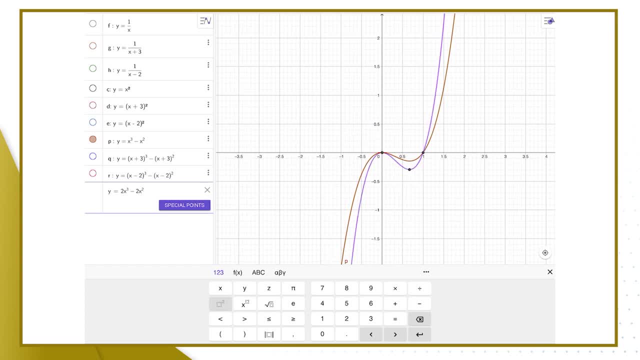 minus 2x squared. Now I've got a purple graph. that is a scaling of the brown graph by a factor of 2 in the y direction. multiplied everything by 2, I'm doubling all the y values. Now does it look like? 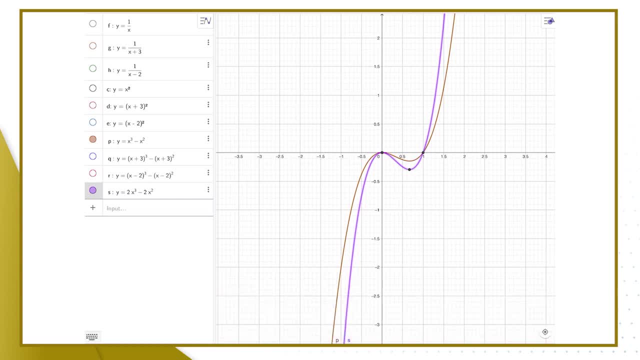 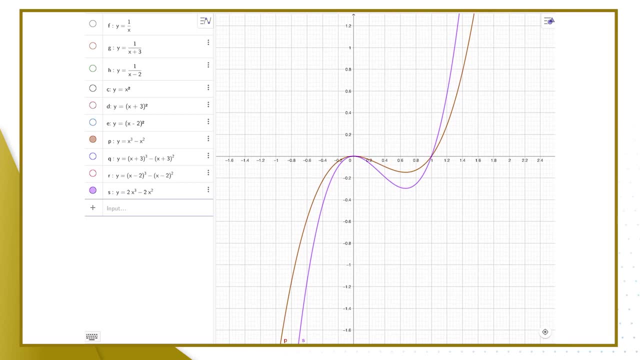 I've doubled it. Let's look into detail at what those two graphs look like. So the brown one is our base function. it's the function we started with and then we doubled everything. So when x equals 0, we have a y value of 0, so doubling that. 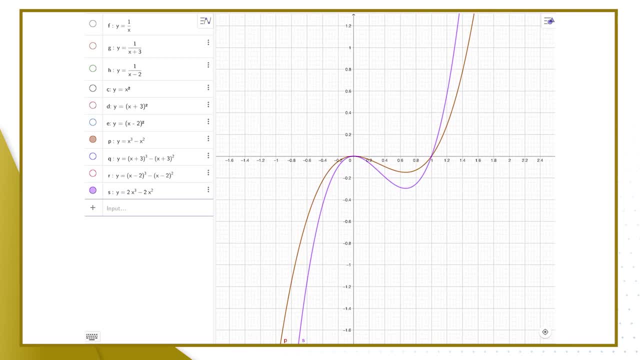 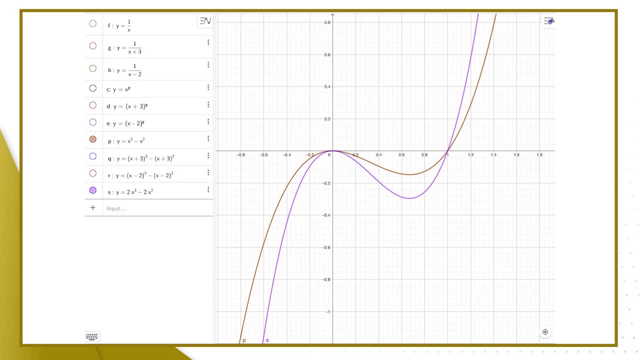 is just going to be 0, and the same happens in 1, and then look at the other values On the same vertical line. so if we look at around, x equals 0.6,, the brown line is just below the minus 0.2, and then the 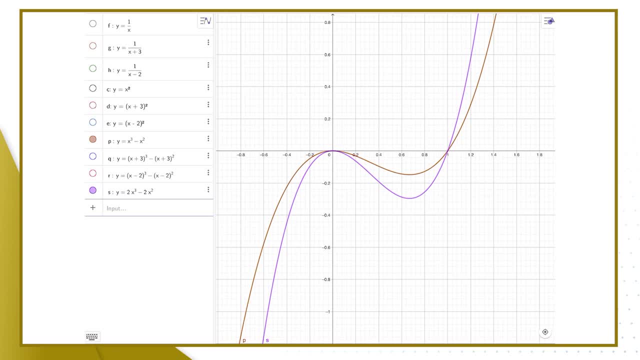 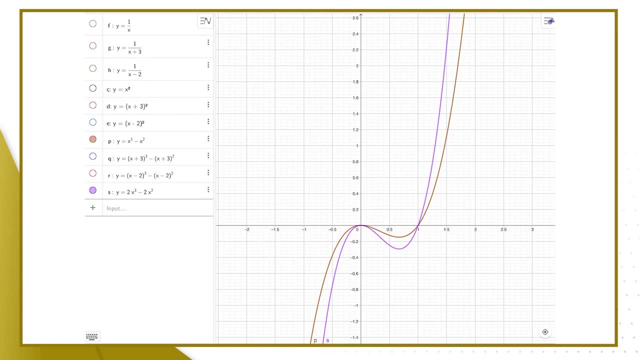 purple looks like the double of that downwards And looking at the positive side, here it's harder to tell If you focus on looking on a vertical line. say, the line that goes through x equals 1.4,. we have the brown graph with the y value around 1.1 and the purple of 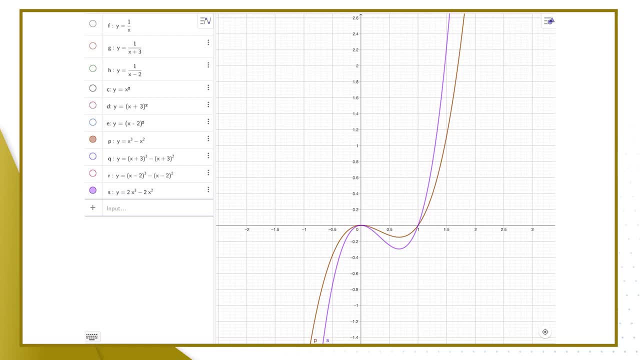 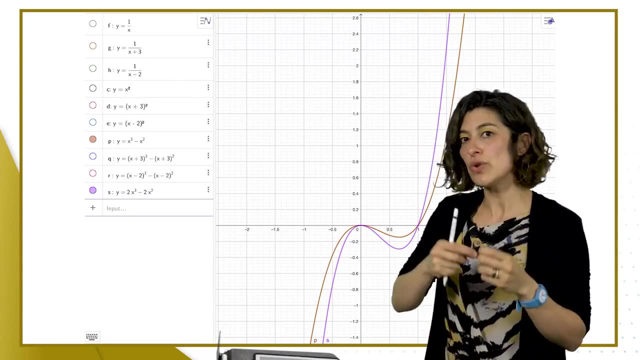 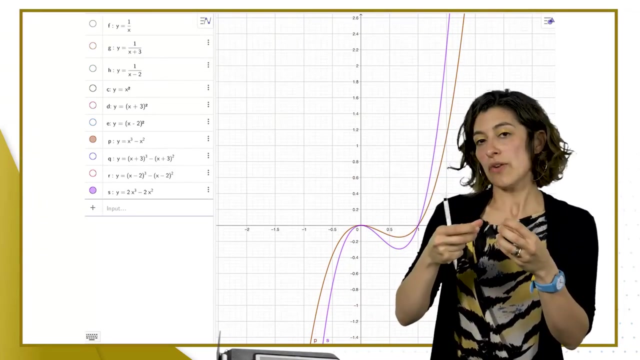 about 2.2.. It's the doubles. This is what is happening. Notice that there was no shift in the x direction on what happens to the graph, so it's purely a scaling a factor of 2 vertically on the y direction. Now, what would a scaling a? 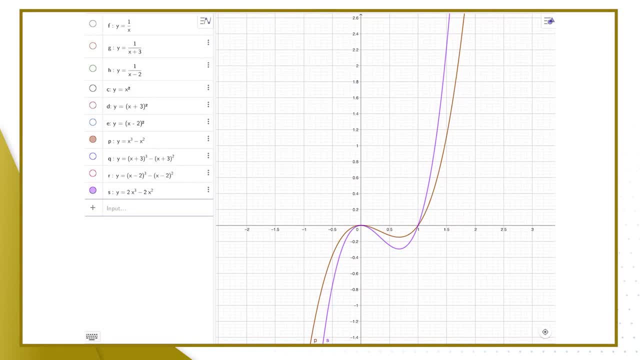 factor of 2. look like in the x direction. Some of you might be thinking: should we just double the x-direction x? We're going to double the x. I'm going to see what happens. We're going to double the x. 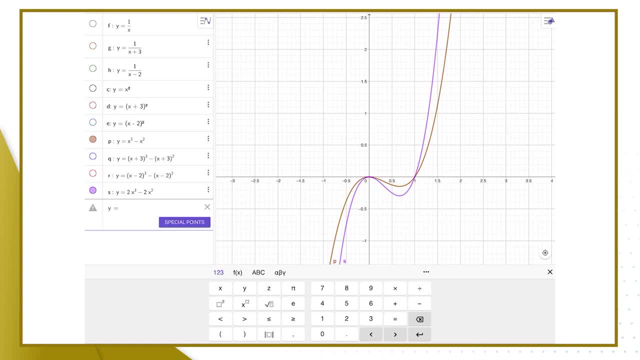 see what happens. You can take bets. Well, you don't. because you're mathematicians, computer scientists, You know that betting isn't a good idea unless you know how the odds work. But let's move on from there. So, x, I'm going to double the x, I'm going to 2x, inside the bracket. 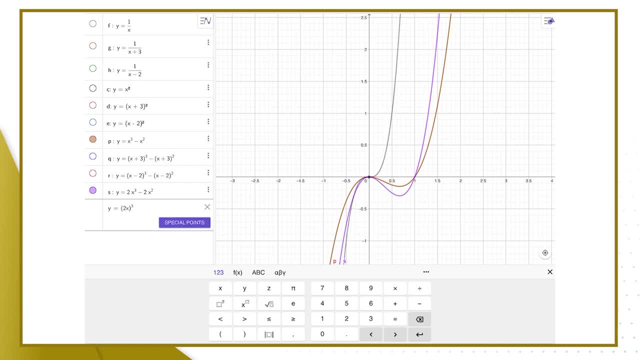 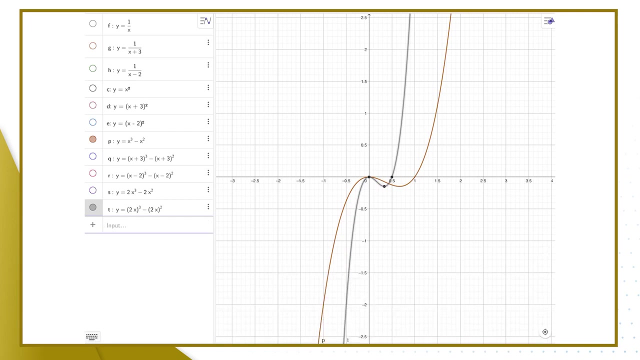 I need to cube it and then do minus the bracket And instead of x squared I'm going to do the 2x and now square it, And that is a grey graph. We're going to remove our purple one. So now the grey graph is what happens if you double inside the x. 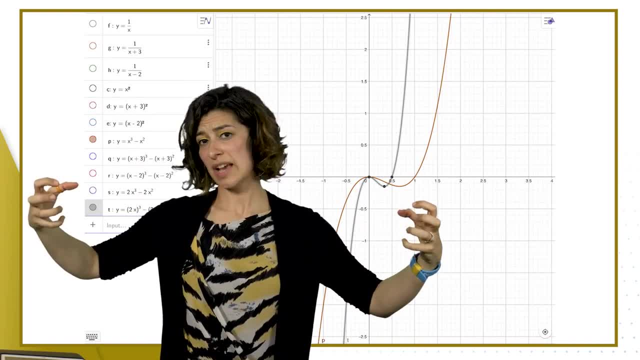 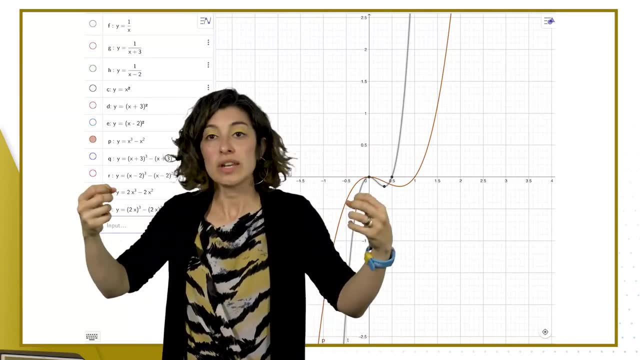 Does that look like We dilated by a factor of two in the x direction? It doesn't look to me. It looks like we've done the opposite. It looks like we shrunk it by a factor of two, In other words, that we dilated it. 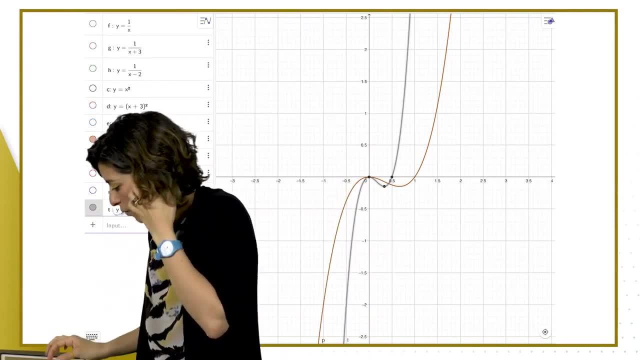 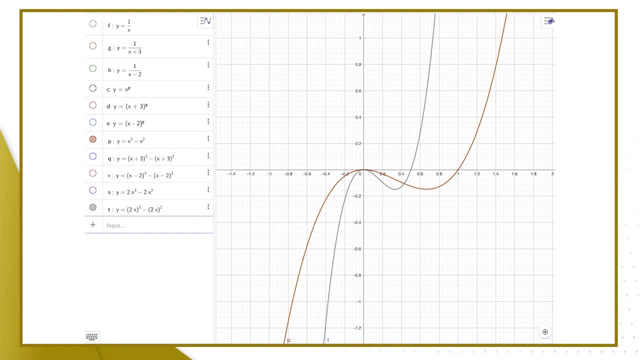 we scaled it by a factor of half. So it looks like again: things that happen in the x direction work in the opposite way of the numbers we put in there. So we multiply the x by two, we get a shrinking. So if we 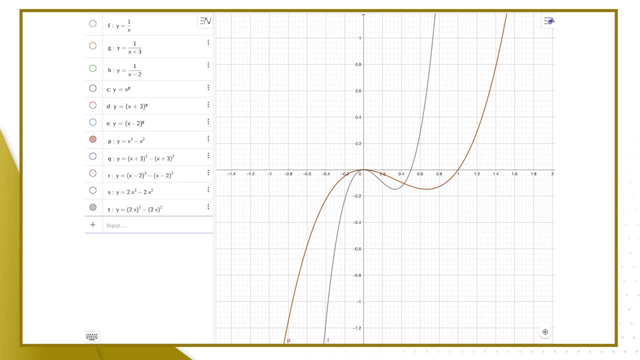 want to dilate the graph in the x direction by a factor of two, we need to divide the x by two. So let's do that one here. So y equals, so the bracket, and do x divided by two and then cube it and then do minus bracket x divided by two and square it, And that in black. 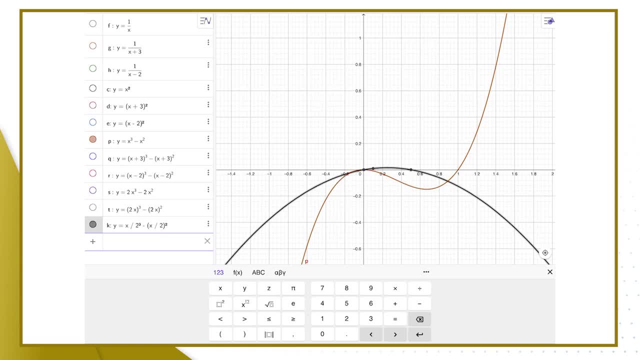 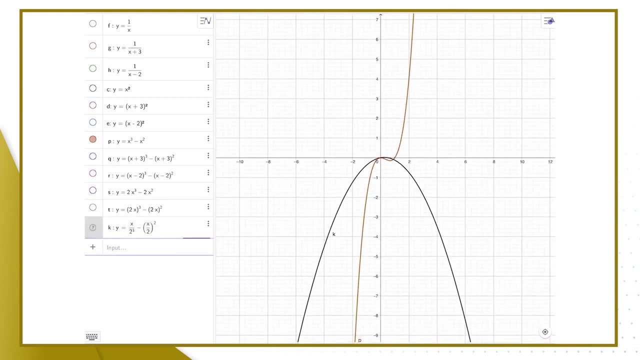 just let's look at black against the brown. I think I forgot. Oh, yes, I forgot something here. No problem, We're going to put some brackets there. It's good to have this mistake, so we know what could go wrong. So we put a bracket x divided. 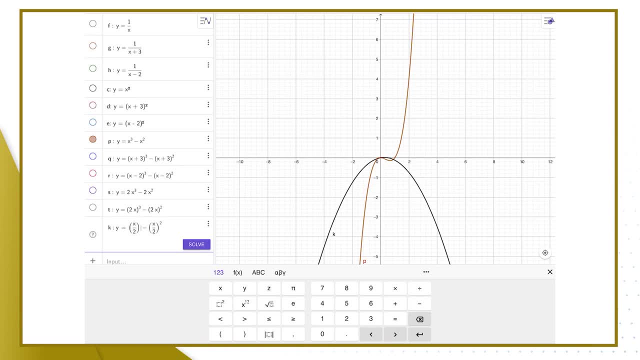 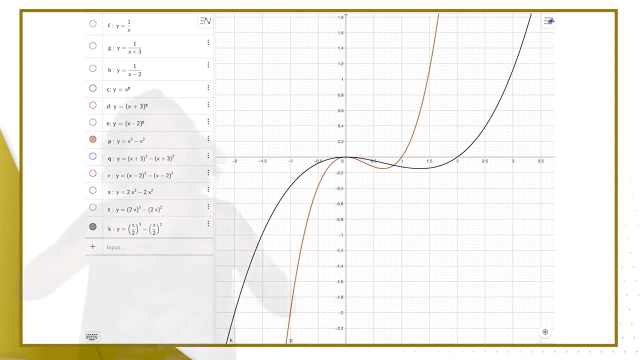 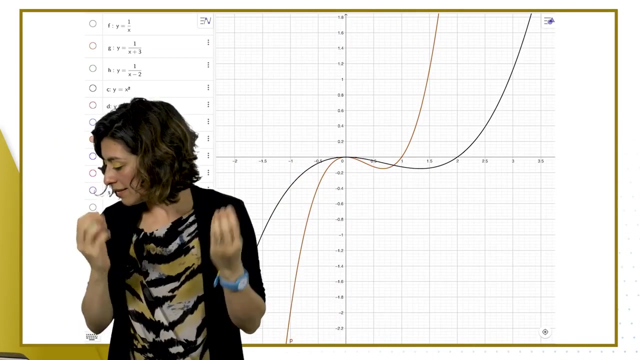 by two and then cube it Ha. black function against the brown function- That is more like it That it is the brown one is scaled by a factor of two in the x direction as the key points, the markers, the zeros at zero and one are now at zero and two. 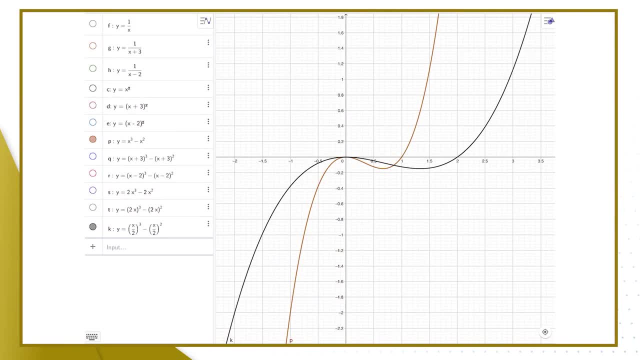 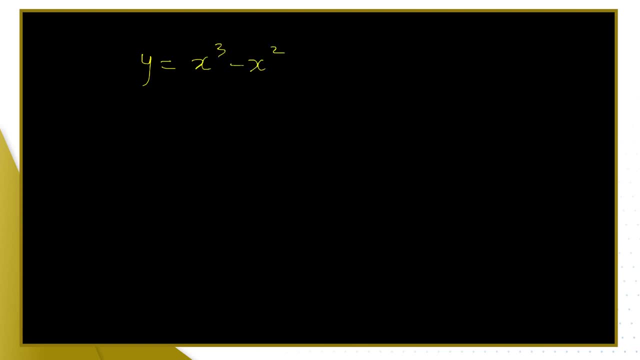 So let's write this down, Make sense of it as a pattern. So when we work with y equals five, y equals x cubed minus x squared, the expression where we double inside the bracket. we do this- This results in a scaling by a factor of one half in the x-direction. 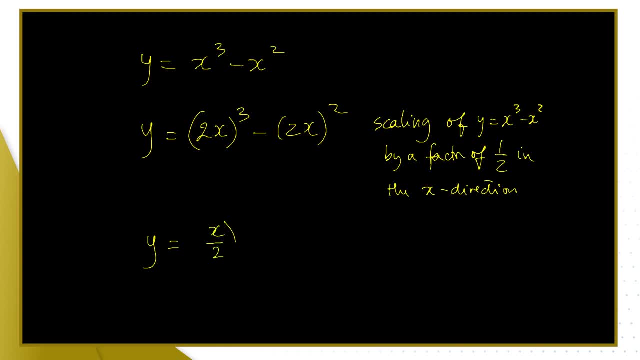 whereas when we divide inside the bracket we do this, This results in a scaling by a factor of one half in the x-direction, whereas when we divide inside the x, we have a scaling of the initial graph by a factor of two in the x-direction. 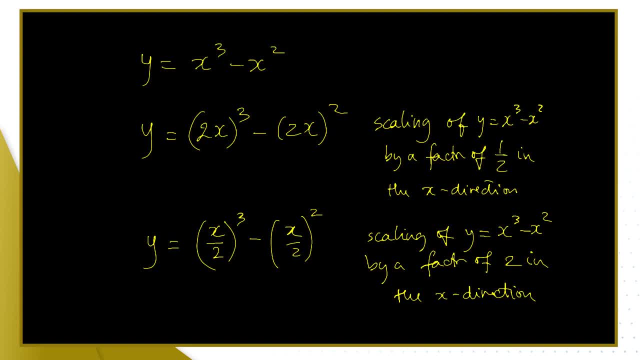 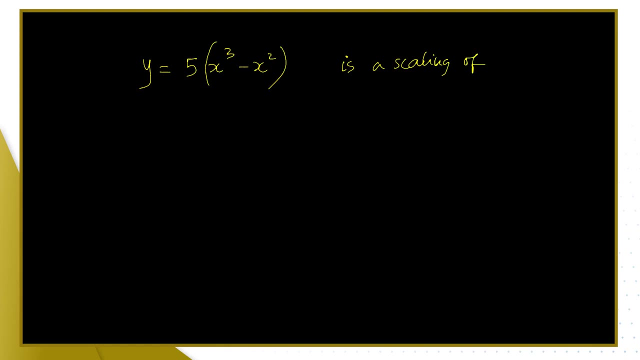 And we also looked at the scalars in the y-direction so I'll write that information down. So y equals: if we do 5x cubed multiply, everything is a scaling of y equals x cubed minus x squared by a factor of 5 in the y direction. 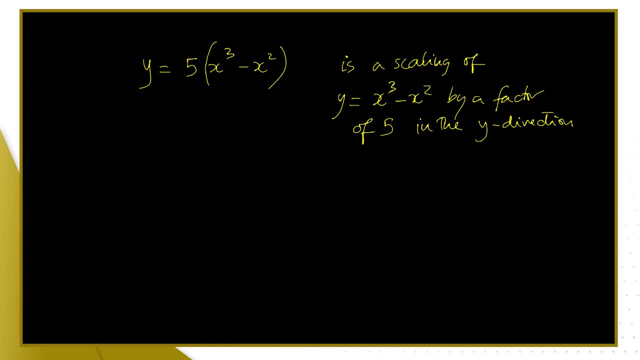 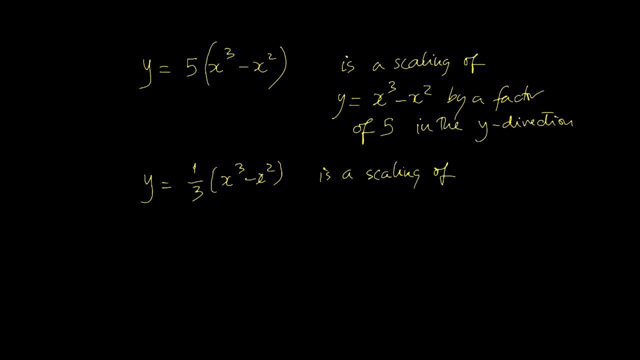 To shrink. we can do y equals, say 1 third of x cubed minus x squared, is a scaling of y equals x cubed minus x squared by a factor of 1 third in the y direction. That's the sort of answer we would like to see from you that summarizes this sort of transformation. 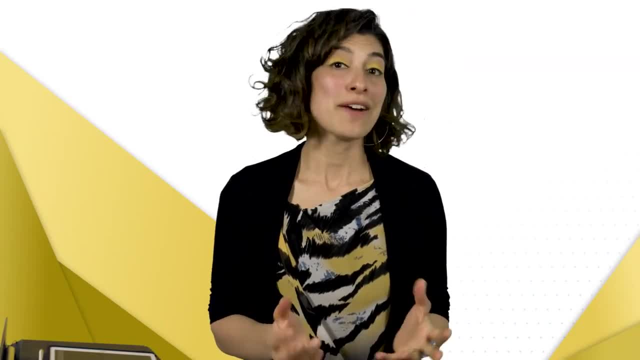 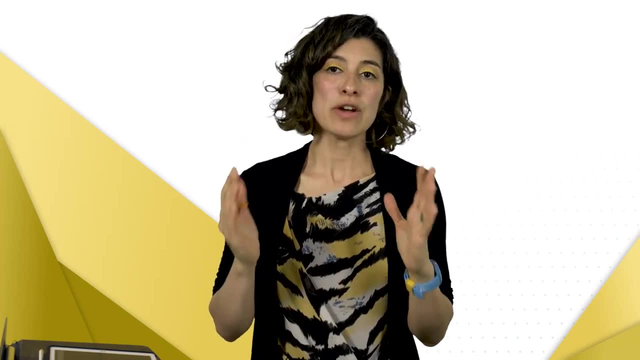 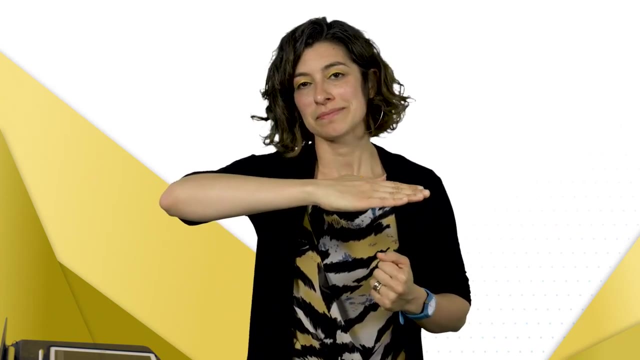 Finally, but not least importantly, we have reflections. Reflections are all about mirror images, so we're going to look at mirroring the graph in a vertical mirror- the y-axis- or a horizontal mirror- the x-axis. All we need to do is to change a sign. 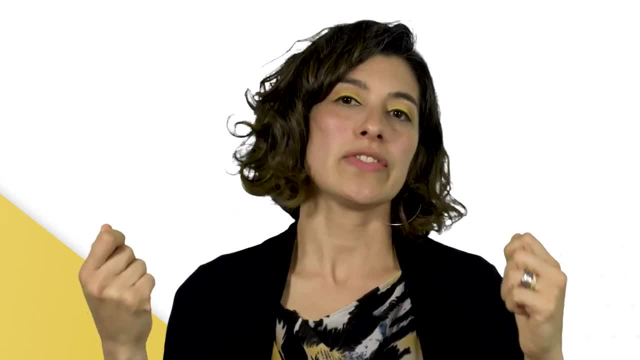 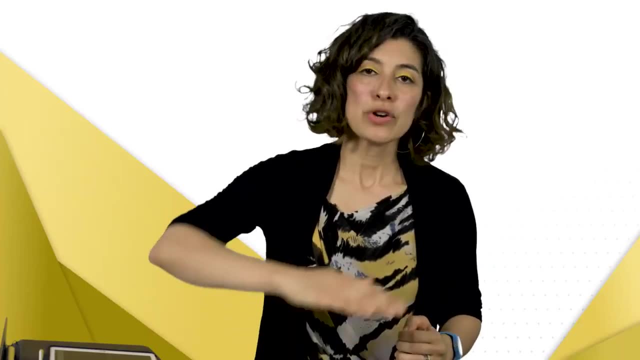 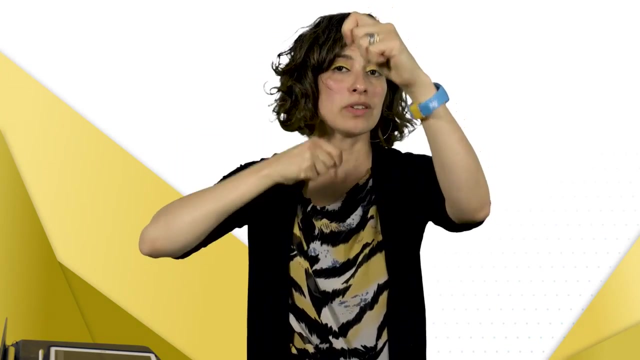 Mirroring in the y-axis means I'm going to change the signs of x. I'm going to swap positive x's with negative x's. Mirroring on a horizontal axis means I'm going to change the sign of the y's. I'm going to swap positive y's and negative y's. 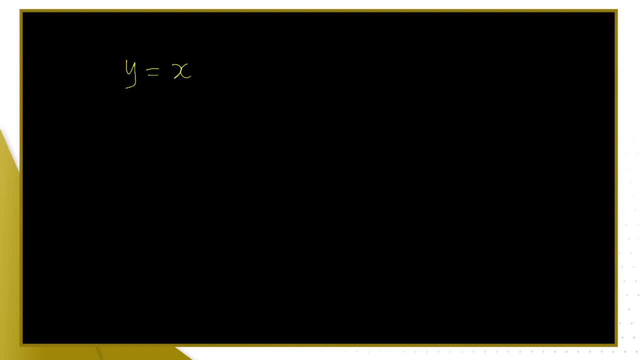 If I have the function y equals x, cubed minus x, squared, our beloved cubic. if I multiply everything by minus 1, meaning I do y equals minus the whole business, which does simplify into this, I obtain a function that has a graph that is a reflection on the x-axis of the initial one. 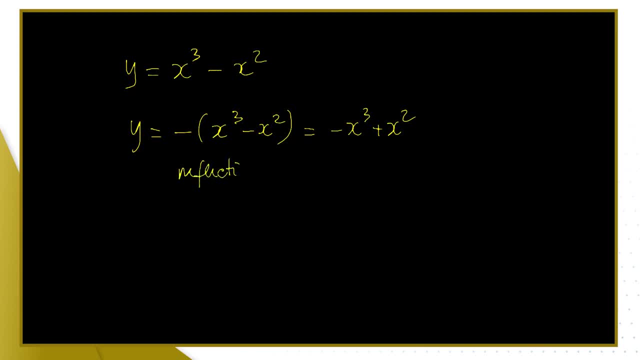 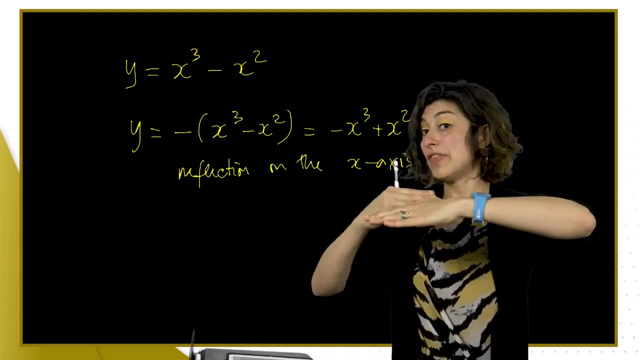 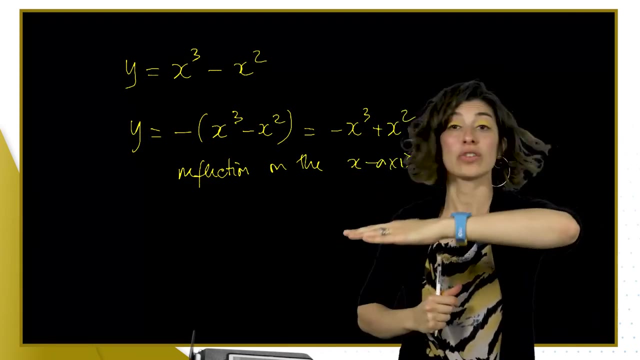 So I have a reflection. Reflection on the x-axis doesn't change the x, it changes the y's. Reflection to change the y's needs to be a reflection on the x-axis and I'm just changing the sign of the y's. 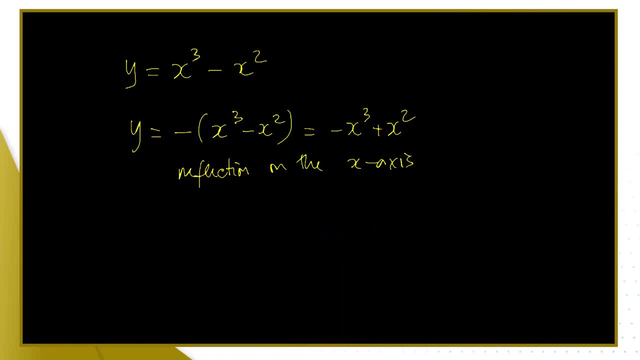 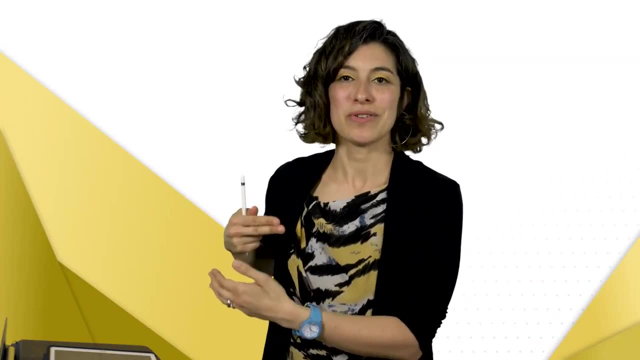 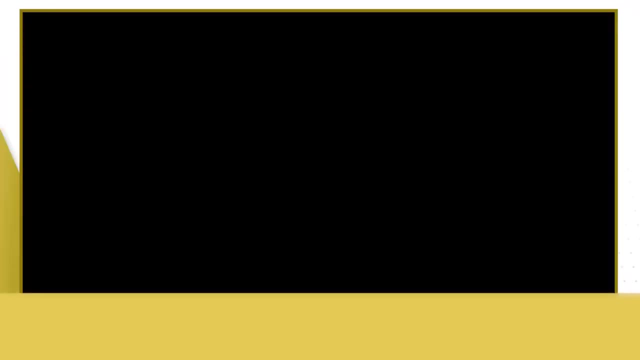 You start with the Brown function and you can use your plotting software to check that the graph is going to look like a mirror image. Just multiply everything by minus 1, like we did on writing. Finally, reflection on the x-axis. For a reflection on the y-axis, we start with our function again. 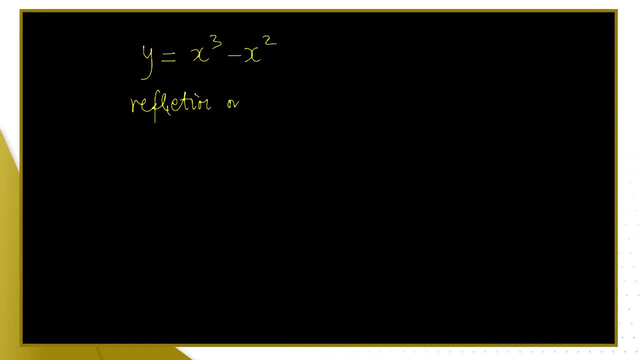 So for a reflection on the y-axis, I'm going to change the signs of the x's, So I'm going to replace x by negative x, So I get minus x, then cubed and minus minus x inside the bracket and then squared. 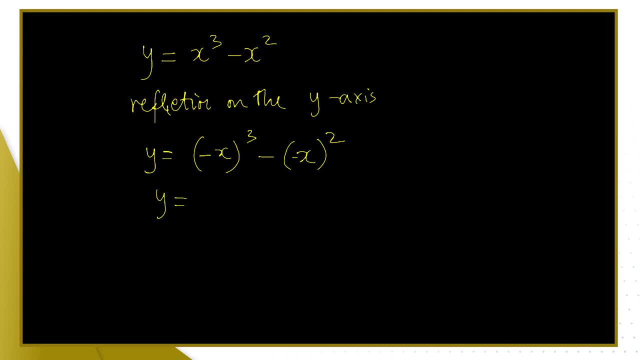 We can simplify that and it is minus 1 cubed, it's still minus 1, so that minus there and the x will be cubed And then I have a minus and then minus x squared. that is just x squared with the other minus. that was already there. 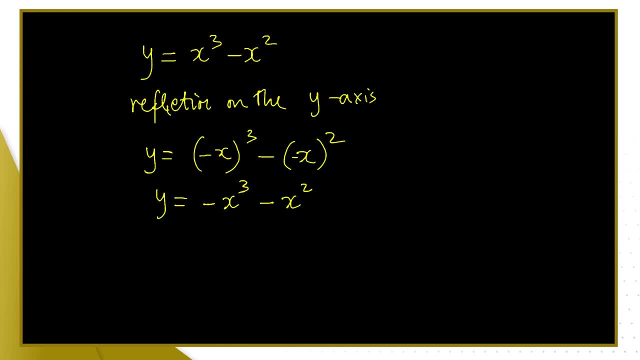 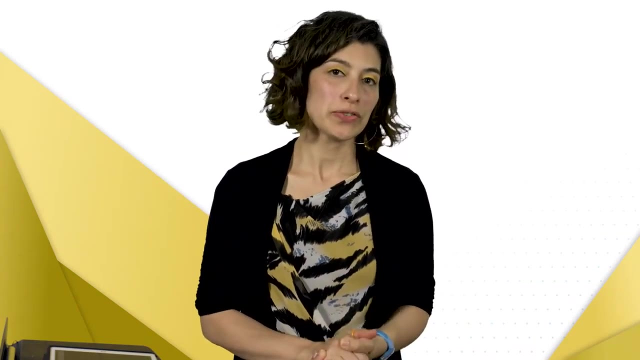 And see for yourself. plot that graph next to the original one and you'll see that it is a reflection on the y-axis, meaning that the left and the right sides are the same. The right side are swapped around. Of course, you can have fun mixing and matching all these transformations. 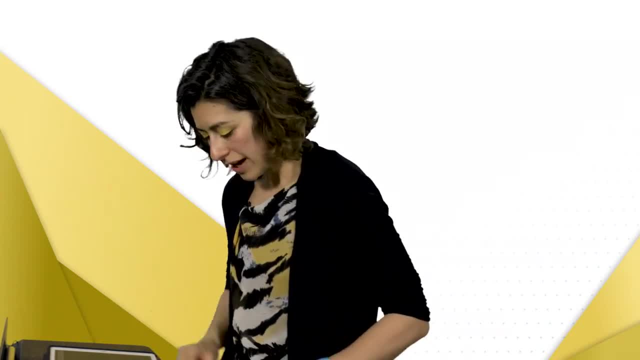 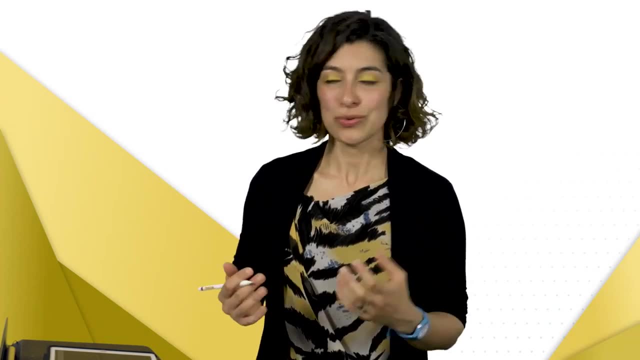 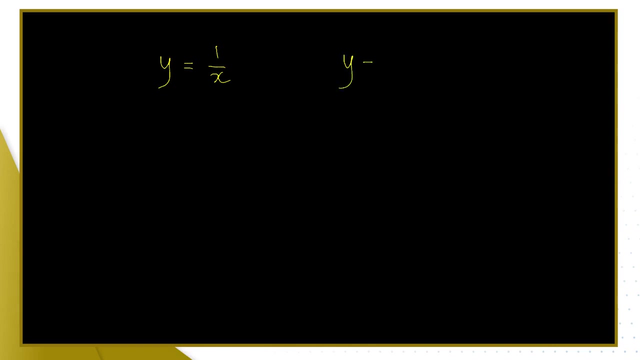 So we just look at one example to give you a taste of that. Remember, you can always plot the functions in your graphing tool to investigate what is happening. So if I have 1 over x and I have another function that is 5 over x minus 1,. 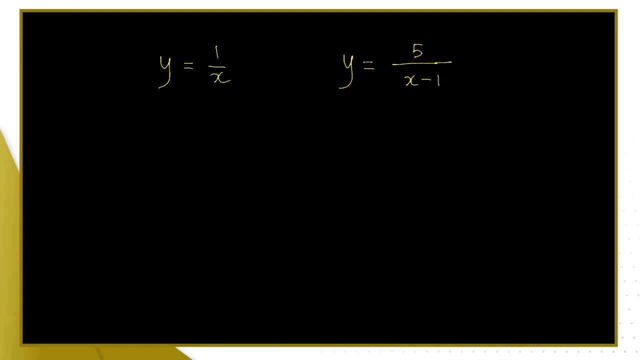 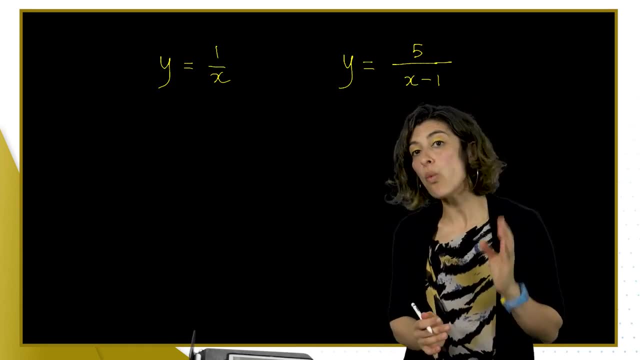 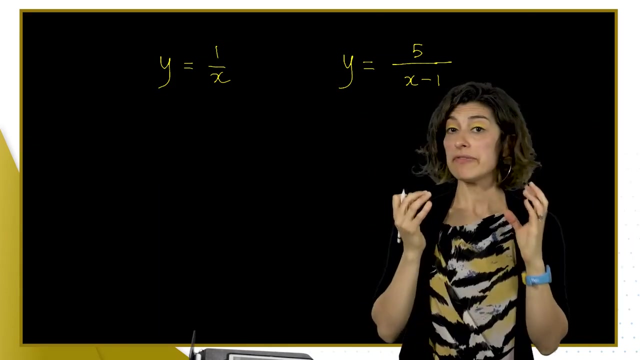 what are the transformations applied? The x minus 1 bit tells me that it's a translation in the x direction by 1 unit. The 5 part, because it is the same as multiplying everything by 5, it's a scaling of factor 5 in the y direction. 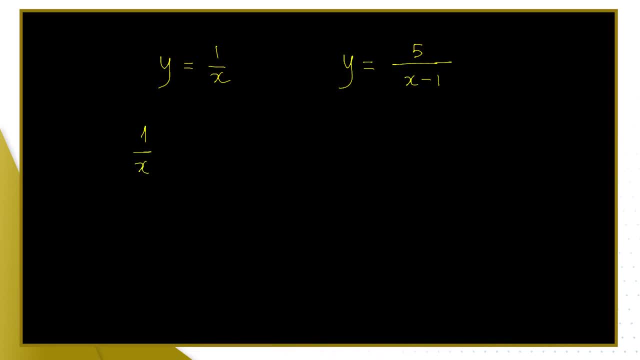 So I can break it down into steps. So I do a translation From 1 over x to 1 over x minus 1.. And then I'll multiply everything by 5.. Which is just the expression we have on top. The transformation is this, in this precise order: 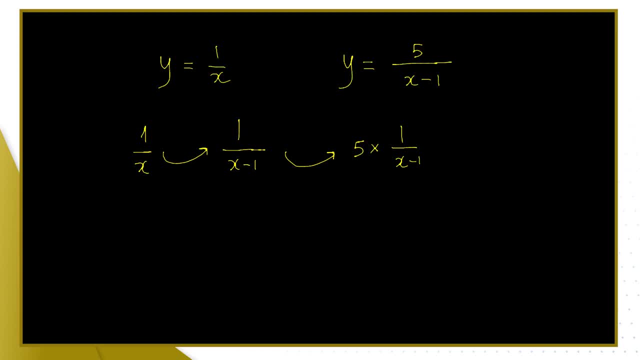 It is a translation of 1 unit in the x direction, followed by a scaling of a factor of 5 in the y direction. If we had y equals x cubed and we did the same transformations, let's see if reversing the order would make any difference. 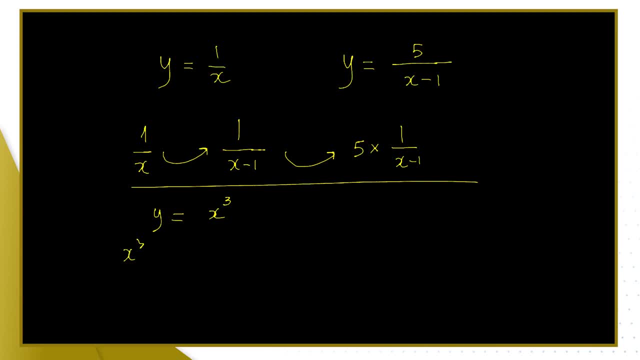 Say we do x cubed, do the translation by 1, and then multiply by 5.. That's what I get. What if I change the order? What if I did the multiplication by 5 first, x cubed, multiply by 5,. 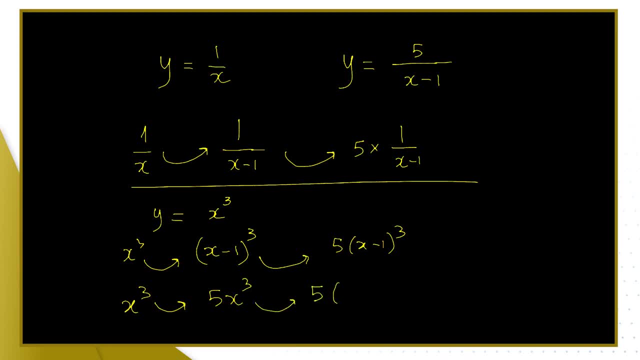 and then do a translation. We get the same in this case. Now, could we get a different result? Yes, if the transformations were happening in the same direction. So if I had still y equals x cubed and I do translation in the y axis. 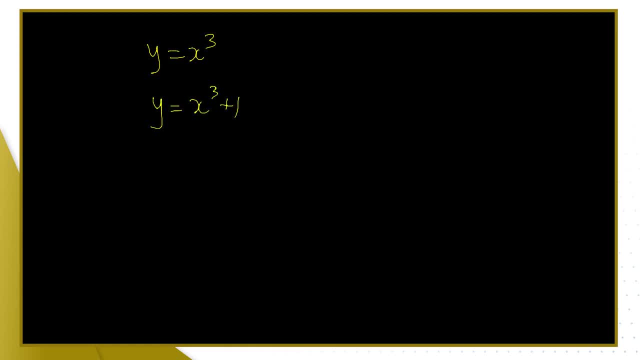 and then I scale it by a factor of 5 in the y direction as well. Now, if I do the other way around, I start still with the cubic and then do a scaling of a factor of 5 in the y direction. 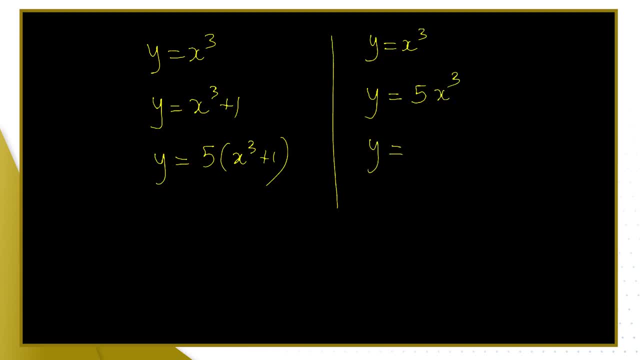 I will have this. And now, if I do a translation of 1 in the y direction, I need to add 1 to everything, And these two functions aren't the same. Don't take my word for it. Check, You can check algebraically. 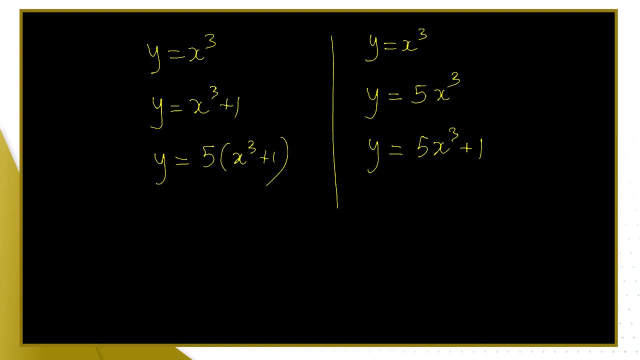 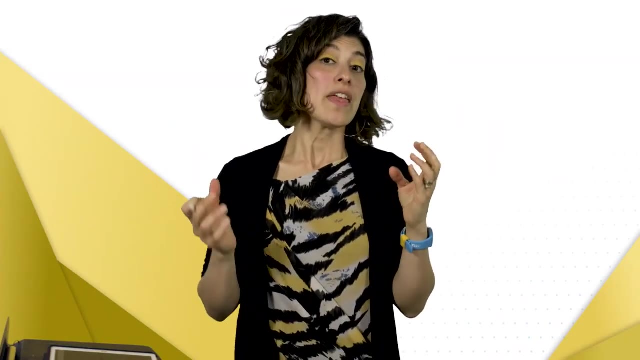 You also can plot the graph with a graphing tool or by hand. This side here we can expand the brackets, And that is totally not the same as the other expression. So the order of the transformations can matter, And I would like you to gain intuition on that. 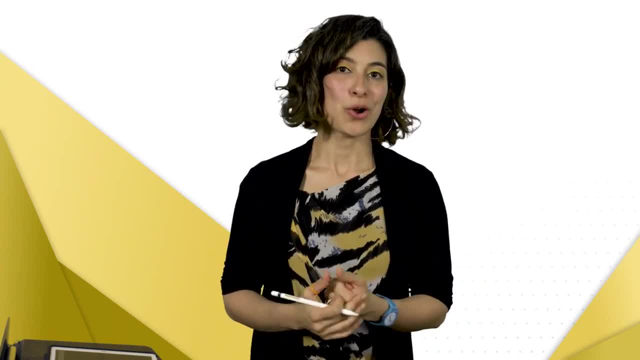 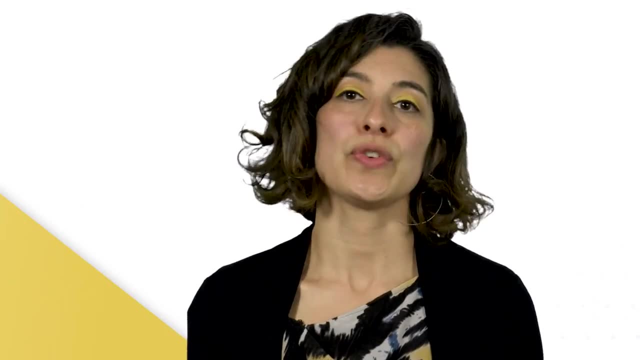 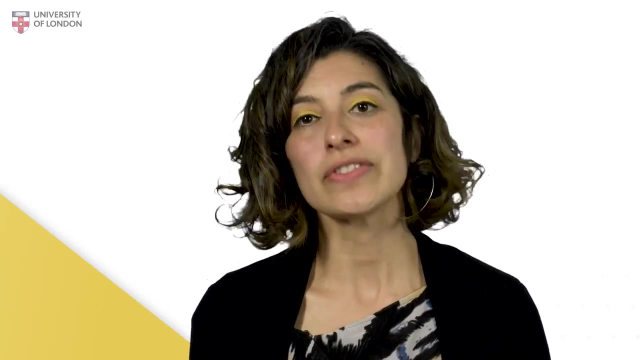 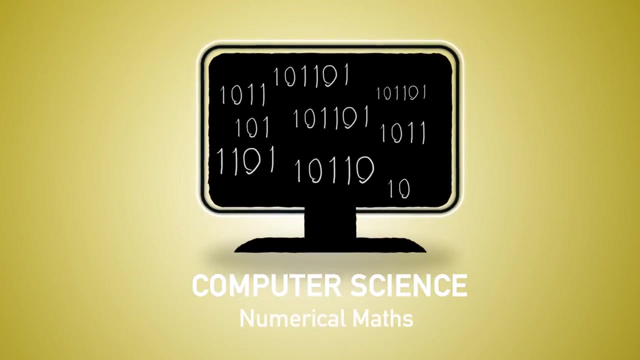 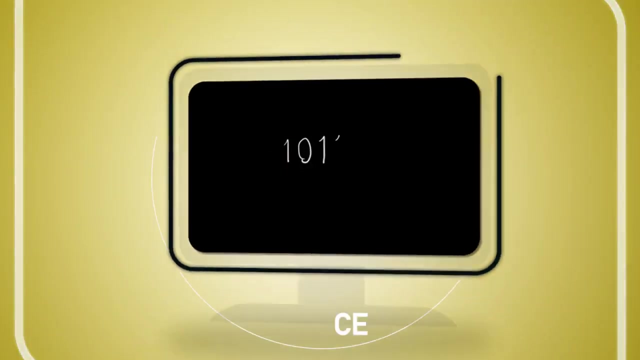 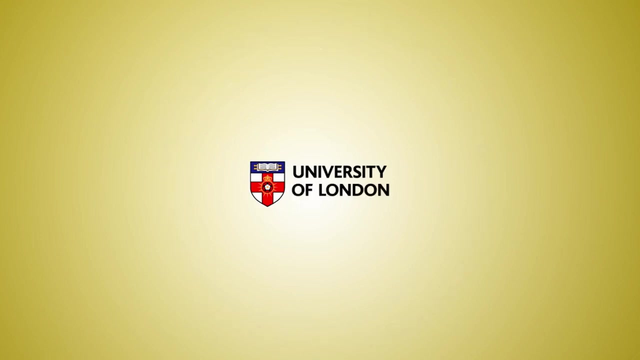 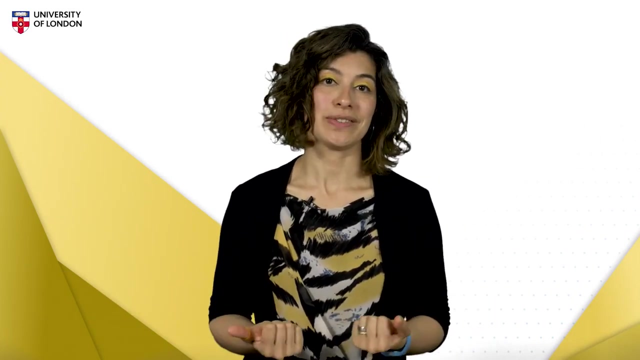 by trying several examples and finding your own pattern. So now you're free to go and play with all these transformations, Use your graphing tool and also practice doing these transformations by hand and describing what the results are and also what the transformation is. We looked at representing locations, points, in two dimensions using two coordinates. 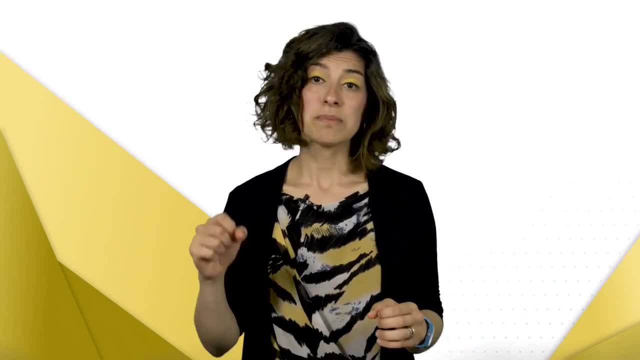 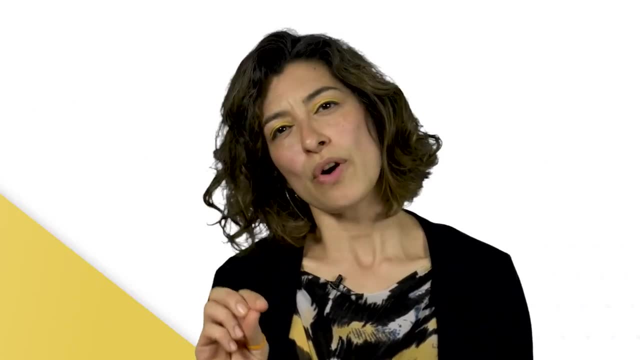 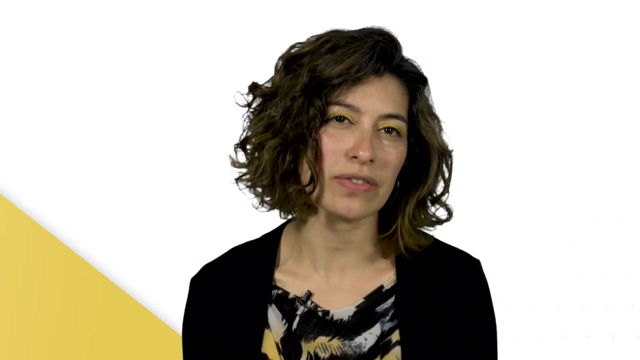 We worked with several types of functions to build tables of values suitable to plot the graph. We focused on two things. We focused on the suitability of these values, as the main idea of plotting by hand is to capture the key features of the behaviour on that plot. 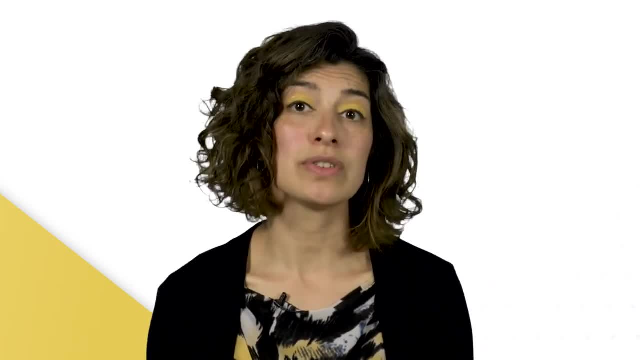 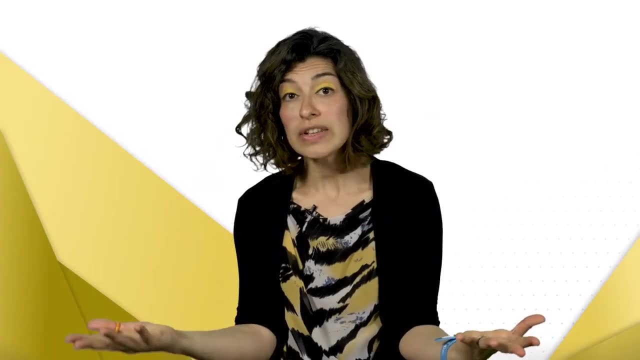 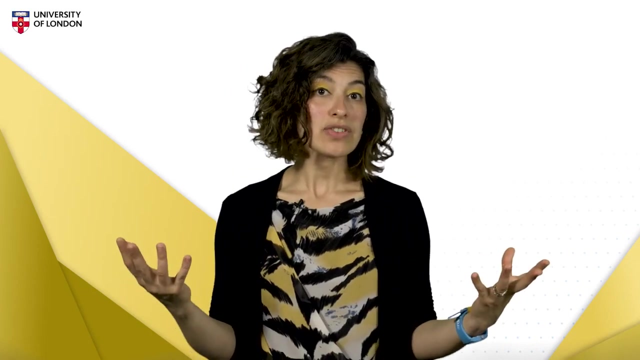 We then looked at geometrical transformations of graphs and how they correspond to changes in the presentation of the expression of the function. We looked at translations in the x and y direction, reflections in both axes and scaling in both directions. These skills are of use with any type of functions. 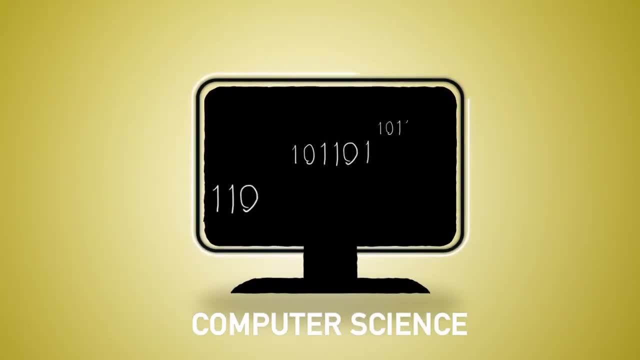 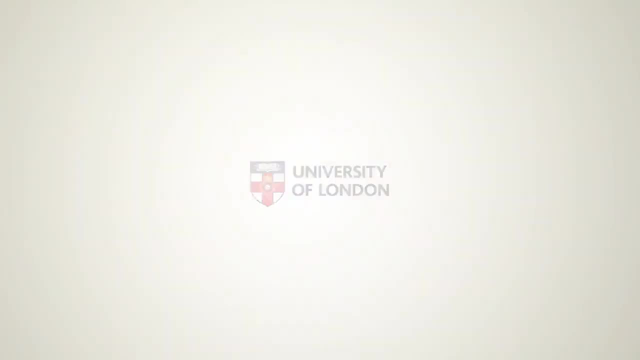 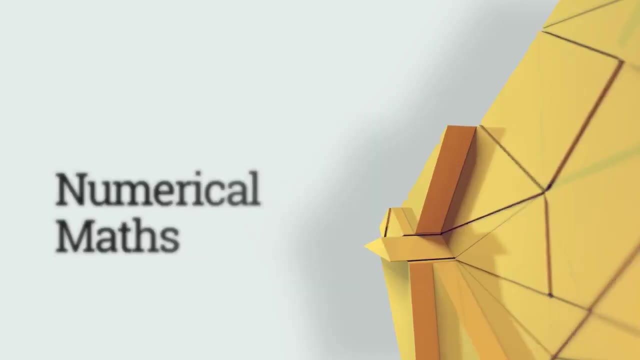 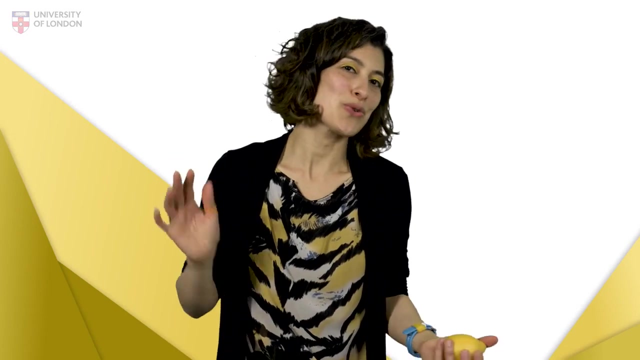 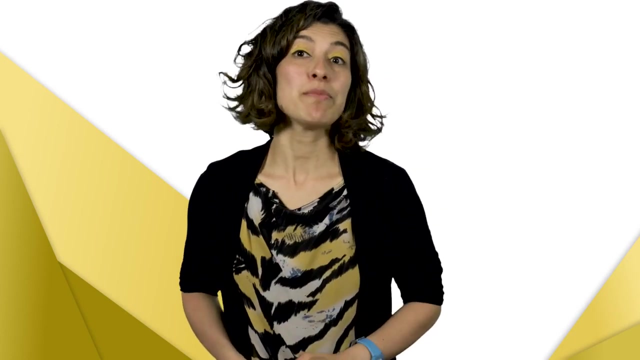 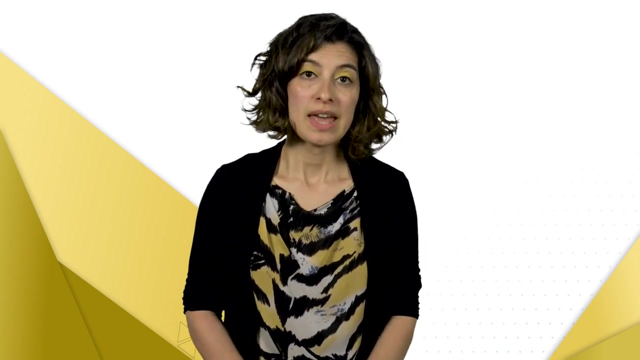 I promised computer games, Well sort of. You will learn the maths you need to design them. Let's get the ball rolling. We consider the motion of a particle moving in a straight line with constant acceleration as a function of time. The variables considered will be displacement. 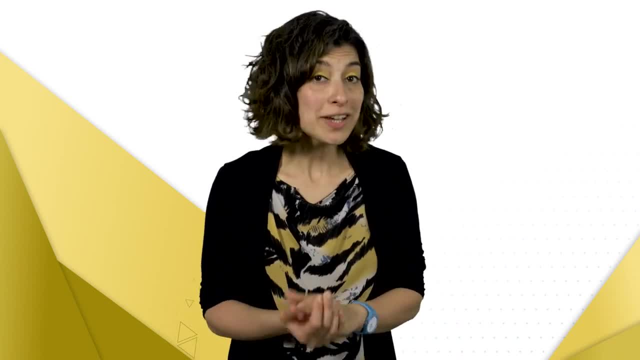 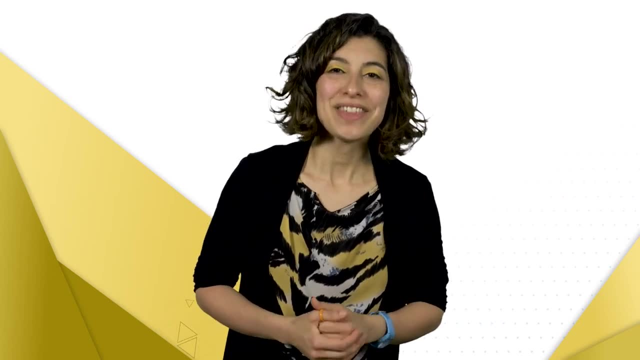 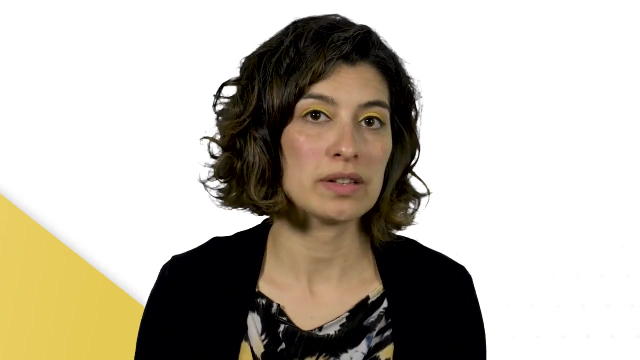 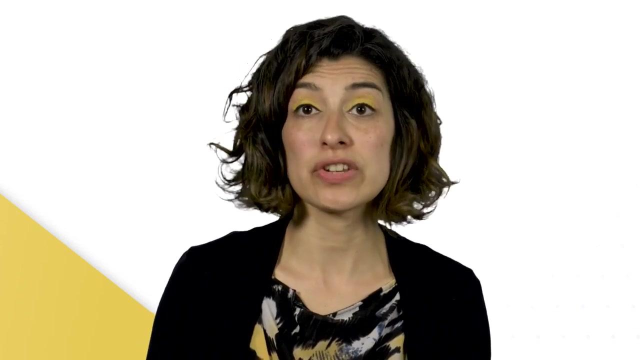 initial velocity, final velocity, acceleration and time. These equations are often known as Suvat equations. This means that the motion is in a straight line, with acceleration being the same direction of motion. So all calculations show variation from the initial position. So we're going to consider that the initial position has displacement s equals zero. 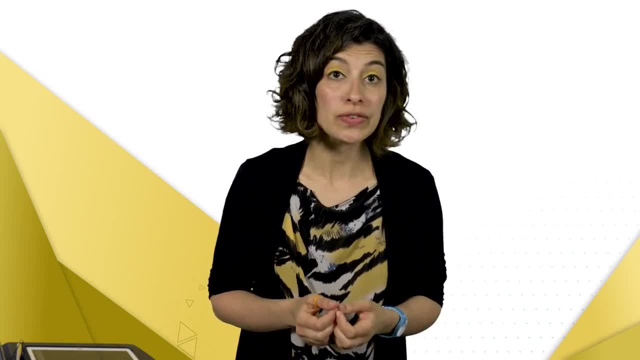 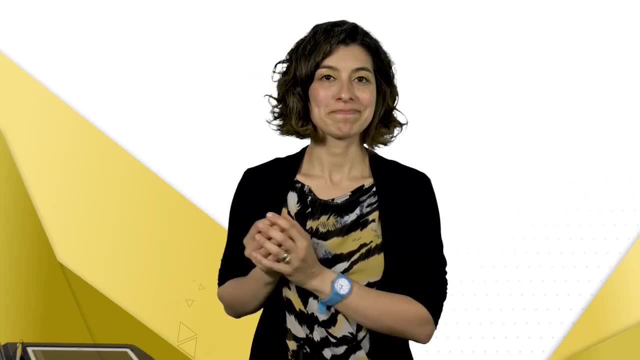 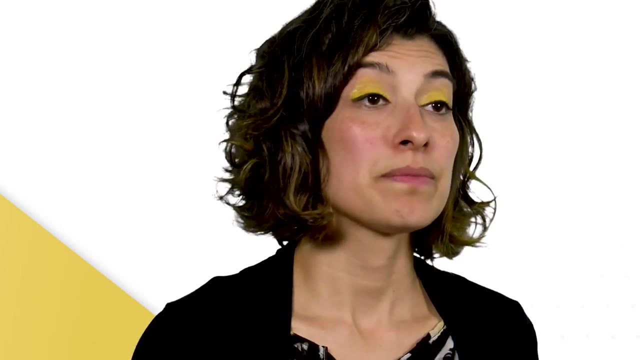 We're going to look at when the particle moves at constant speed, when the particle moves with constant acceleration, We studied the change of position, That means how far and in which direction it moved, And also the change of speed. We're going to look at some graphs. 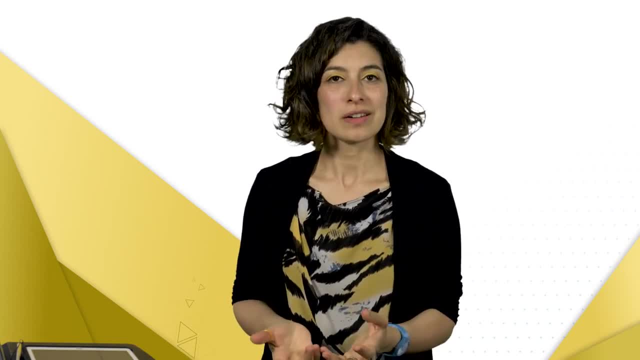 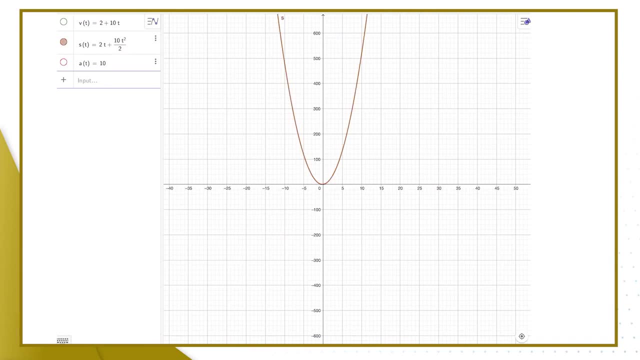 I know I haven't told you yet what the equations are, but we're going to look at some examples and we're going to make sense of them from there. So here I've got an equation for position. So I've got s of t is a function of t. 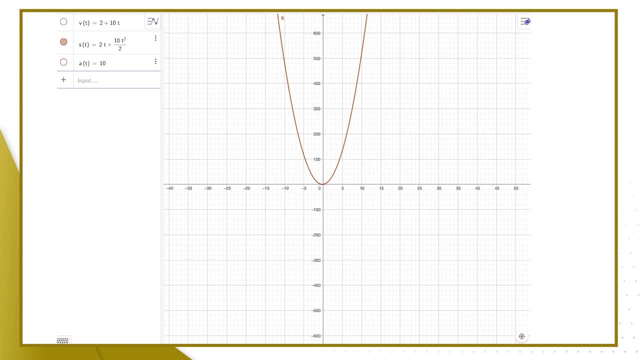 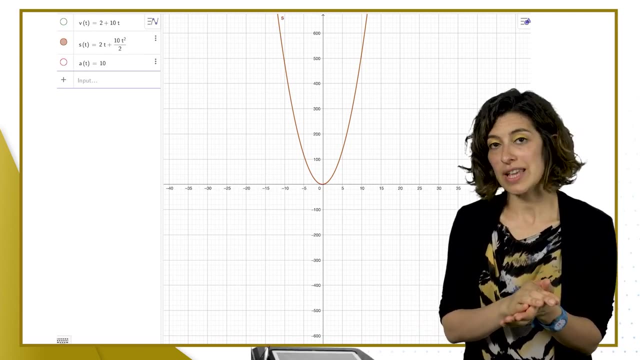 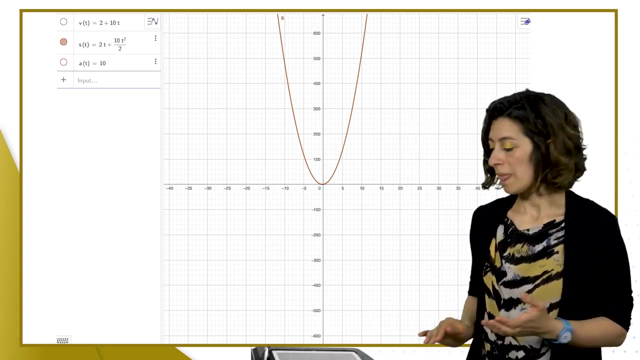 s being 2t plus 10, 10 squared divided by 2.. In this case, I've got an acceleration of 10 and I've got an initial velocity of 2. And I can tell that the acceleration is helping moving. 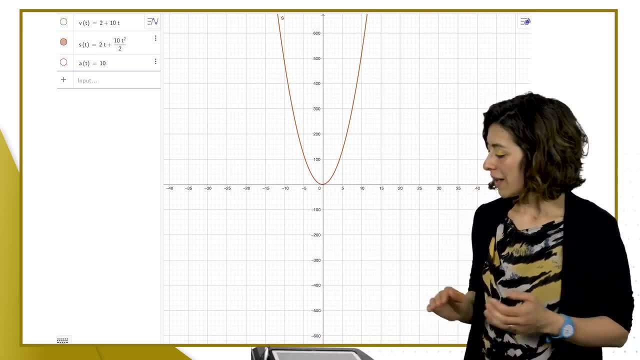 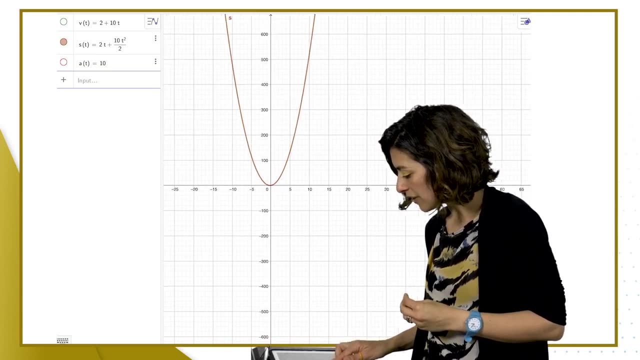 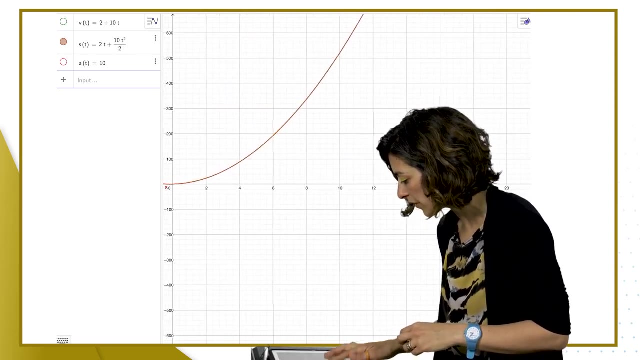 It's helping increasing the displacement And it's a positive acceleration, so it's a plus 10.. Now, how do we read this graph? This graph is position measured in the vertical axis against time time on the horizontal axis, And let's just focus here on the initial seconds of motion. 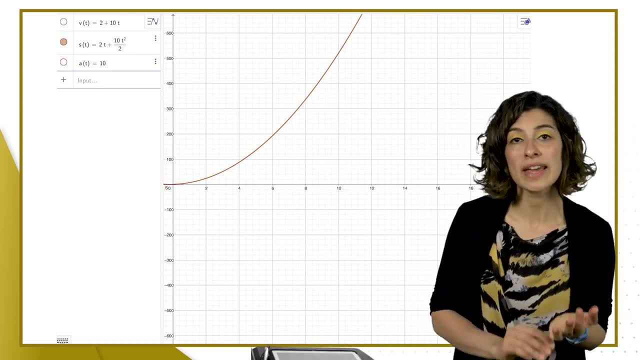 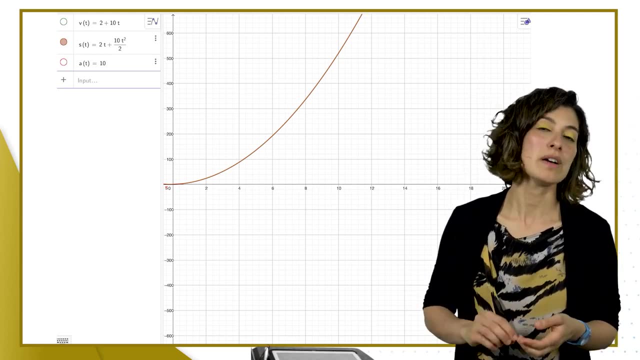 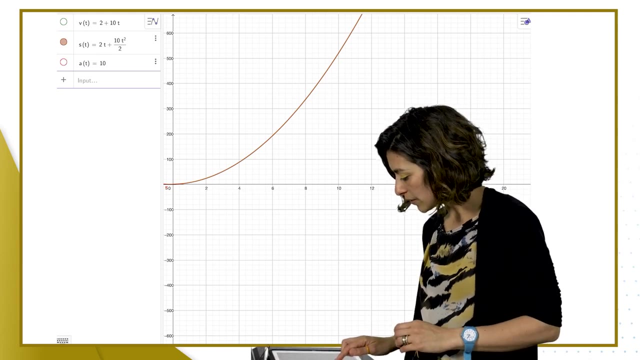 So the units, by the way, time is measured in seconds, velocity in meters per second and acceleration in meters per second squared. So we've got from t equals 0 to t equals around 6 seconds. we see, we've got a reading of position. 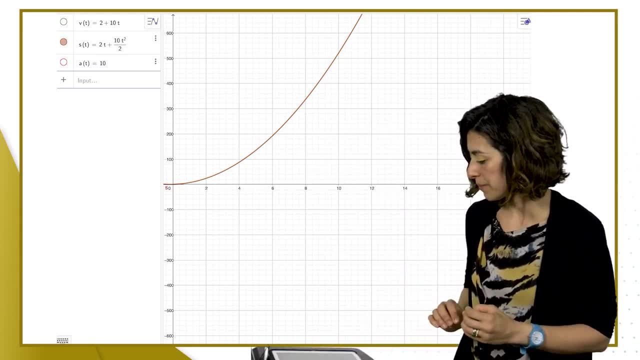 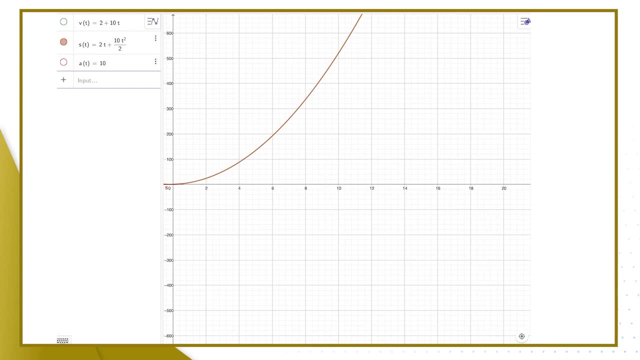 about just below 200 meters, The corresponding expression for velocity. it's on my, it's here as well, it's highlighted on green and the graph is showing as a green line as well. So that is showing the speed is increasing linearly with time. 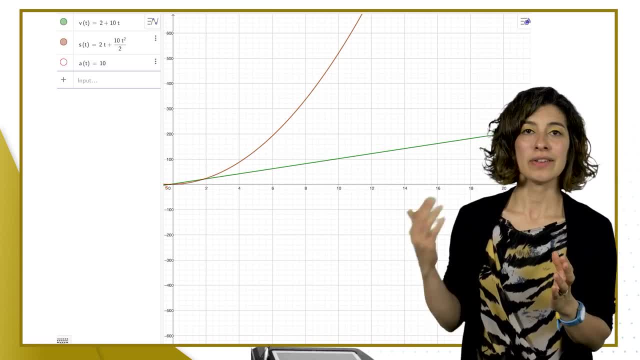 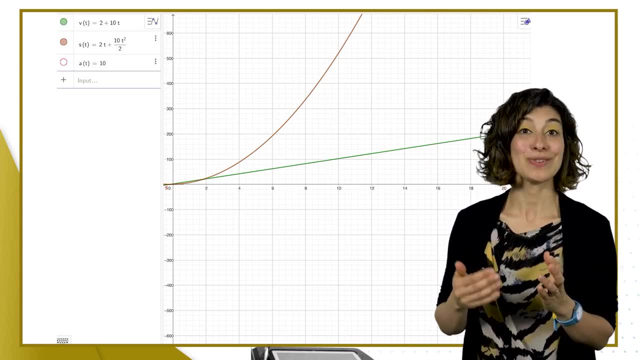 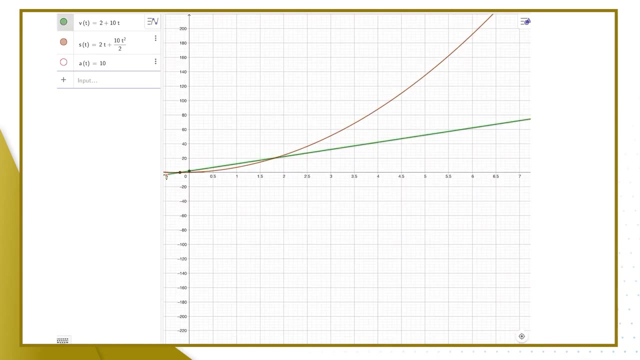 That's because my acceleration is constant. I'm just saying, as every second elapses, we are adding 10 meters per second to the speed. So we can see on this graph that we start with a 2, a speed of 2.. 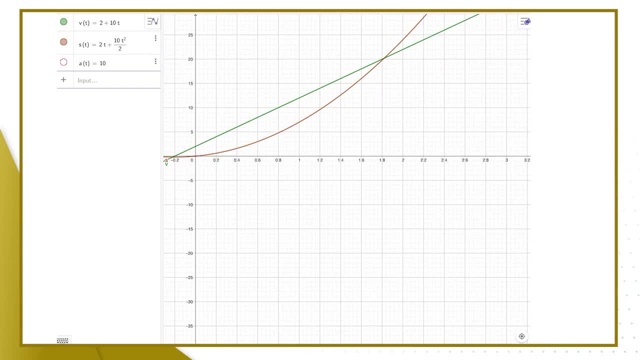 When t is 0, the green graph is having a reading of 2, because that's the initial velocity is 2.. And then every second elapsed, because my acceleration is 10 meters per second. squared for each second, the velocity is going to increase 10 meters per second. 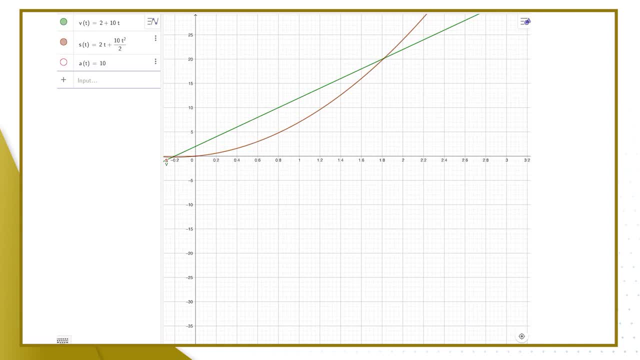 And look after one second. I have a reading of 12 meters per second on the green line When t equals 1,. I have a reading of velocity of 12 meters per second on my green line. I said that the acceleration is constant. 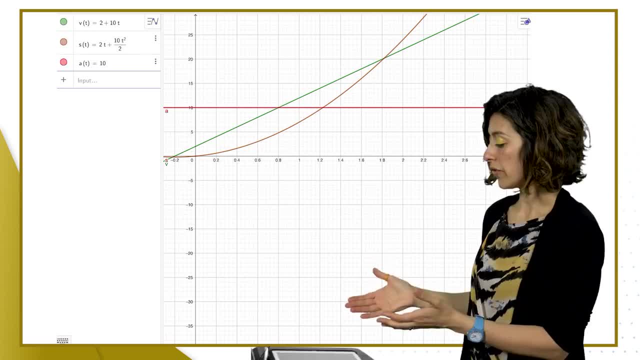 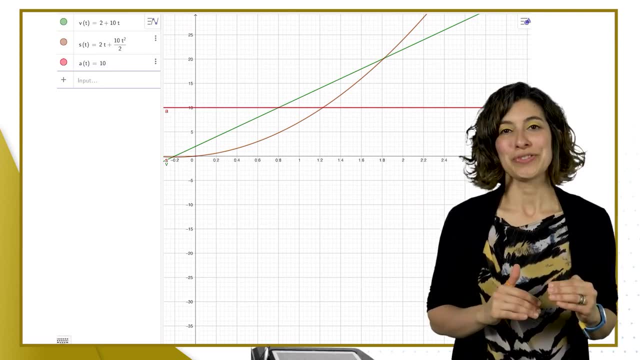 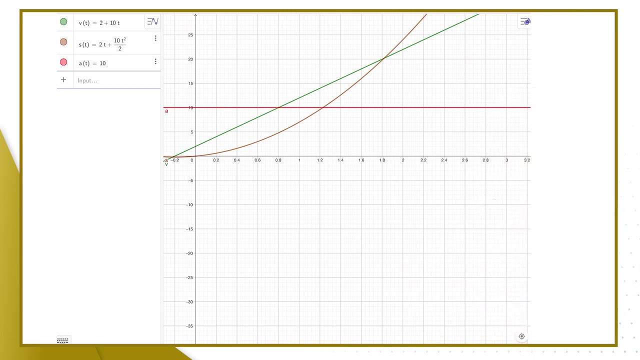 so the graph for the acceleration in this case is a horizontal line going through 10, 10 meters per second squared. It will always be a horizontal line because it will always be constant. Let's see what happens when I change the acceleration to be negative. 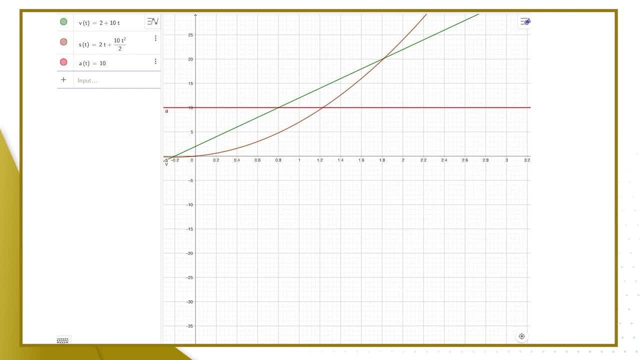 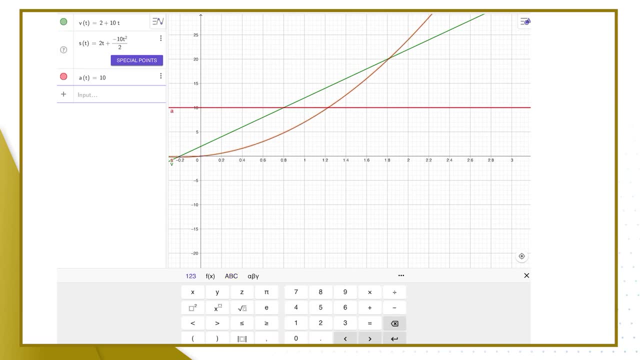 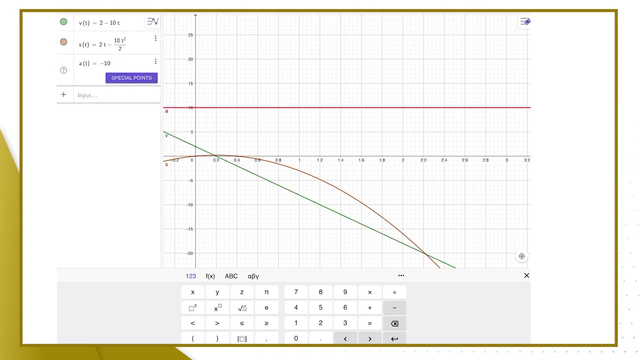 Let's just put it to minus 10 meters per second squared. So I'm going to change all my equations of motion here. Put a minus, a minus on that one, and acceleration here being Okay, Let's see the results. And there we are. 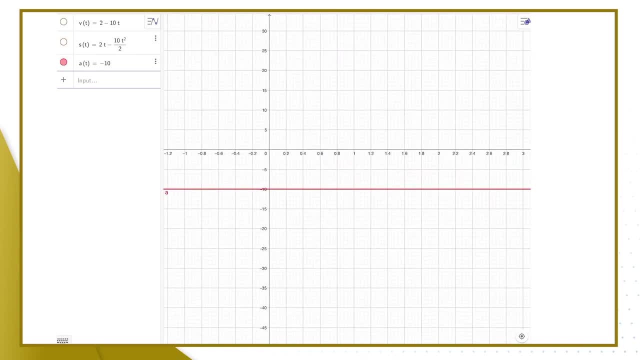 Let's isolate them. Acceleration is constant at minus 10 meters per second squared, The velocity is going to be decreasing because I have an acceleration that is negative. That means it's stopping motion. It's stopping, so it's decelerating. 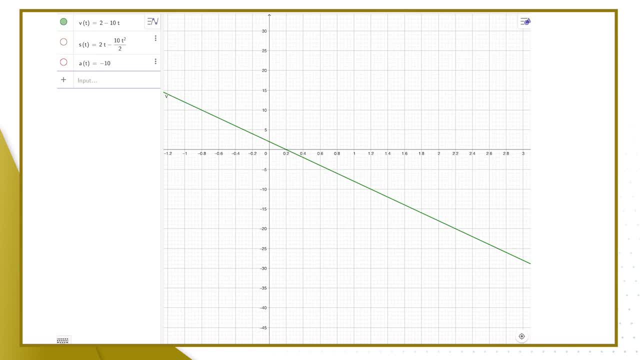 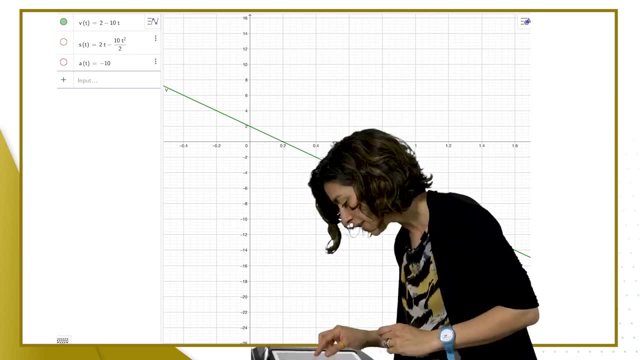 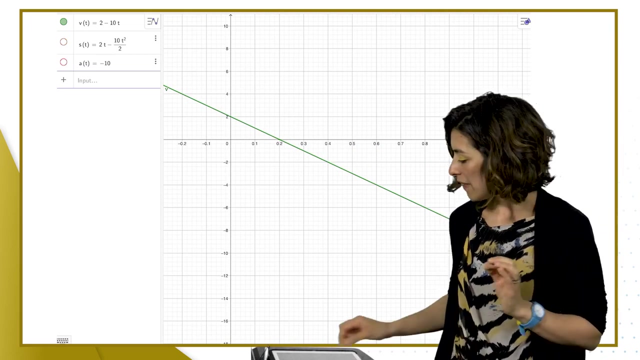 The velocity is going to decrease. It decreases from 2 meters per second. at time equals 0 seconds, And at 0.2 of the second the velocity is 0. And then it will be negative. So it's starting to move backwards. 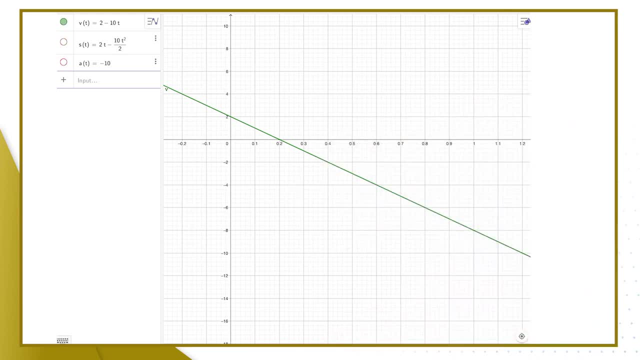 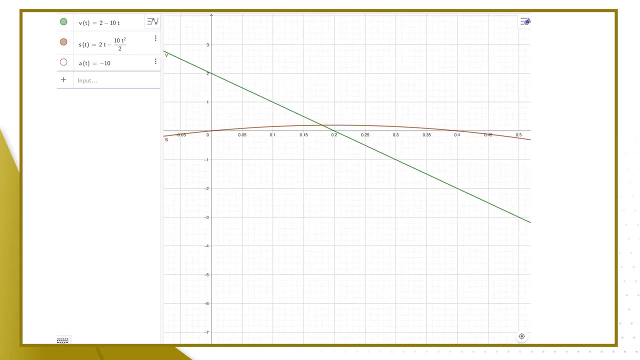 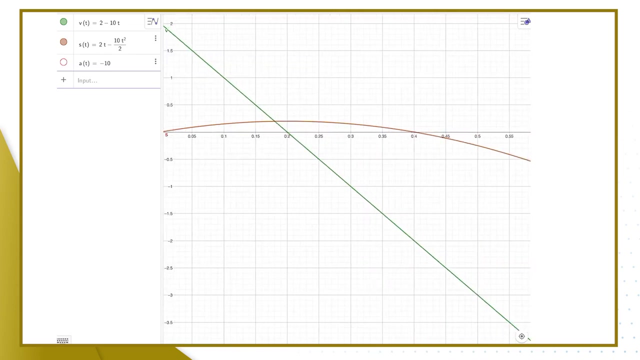 with the negative velocity. Let's see what happens with the position. With the position, we start at the origin. So displacement is 0.. And as time increases, when I get to that point, when time is 0.2 seconds, 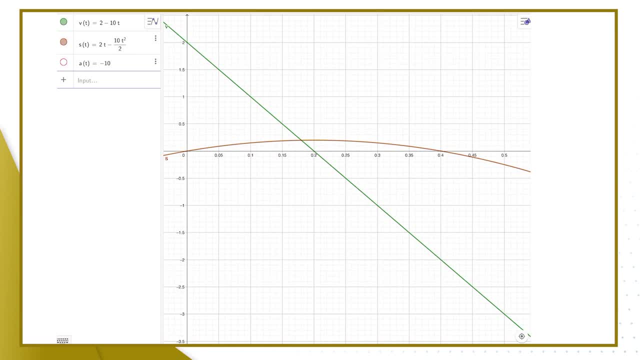 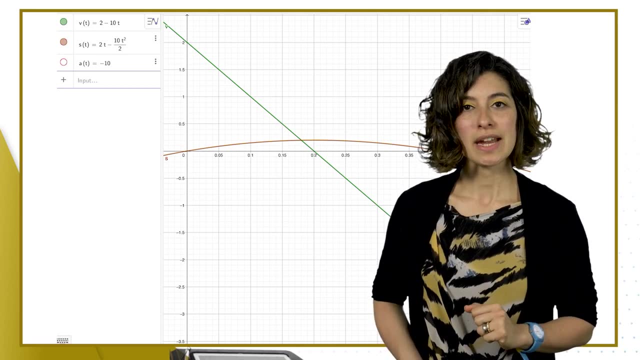 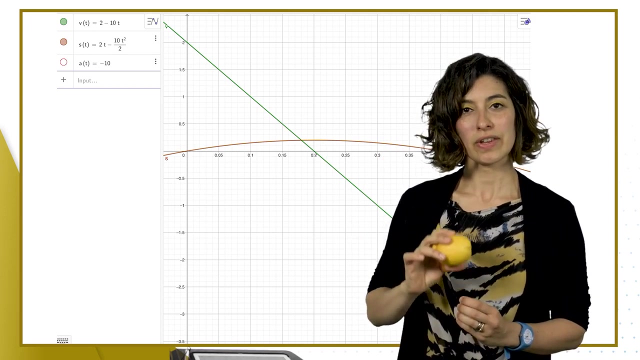 this is when the velocity hits 0, the position hits the maximum value. This is what happens when you've got a ball going up in the air. You go up, It stops and it comes down. The position has. The distance has increased, increased, increased. 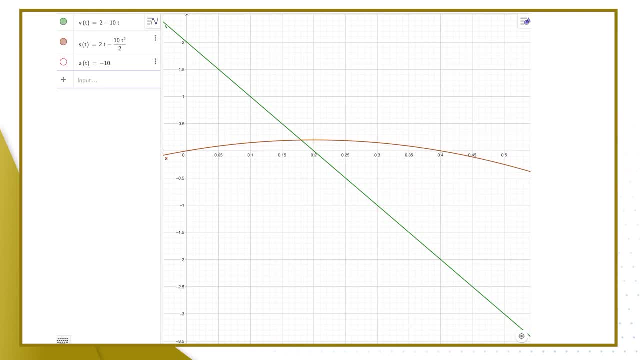 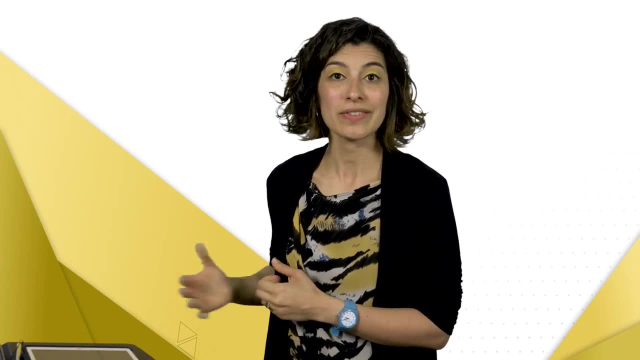 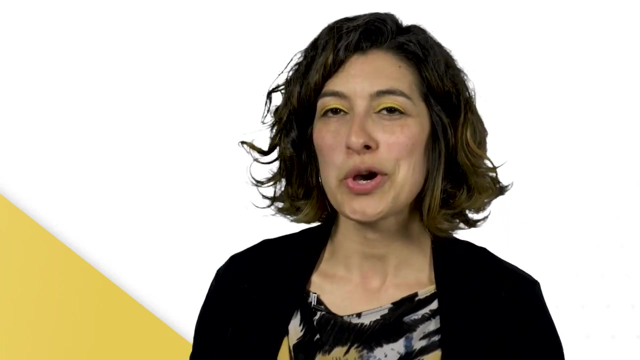 And then it starts decreasing again. That's what is happening with our brown graph there. Feel free to play with these equations on a graphing tool to make sense of how the graphs behave as you change the initial conditions. Now the equations. We're going to look at the equations. 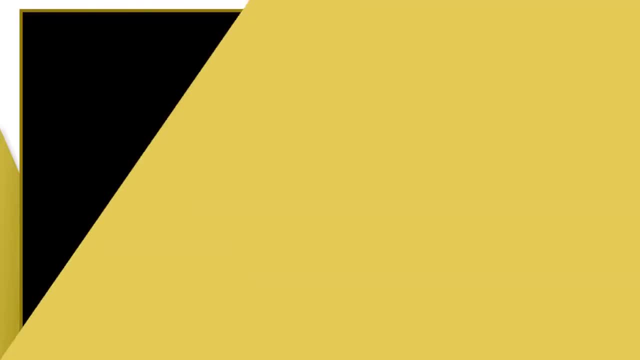 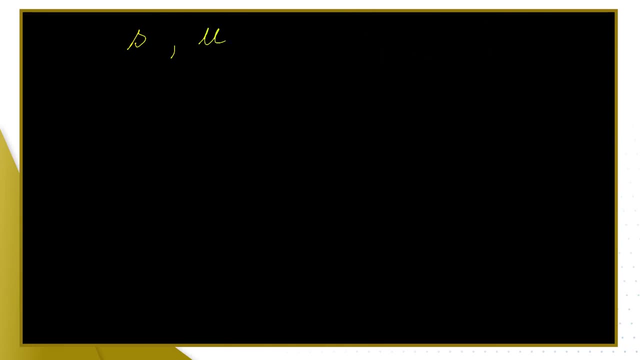 similar to the ones we saw and a couple more. So we write, just bearing in mind that S is a position, a long time, u, the initial velocity, v the final velocity and acceleration is constant and time elapsed The equation for position. 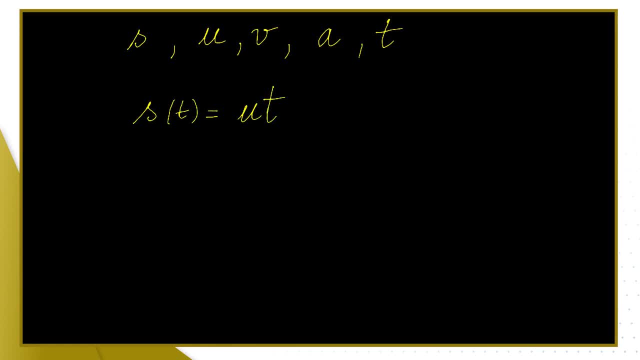 is initial velocity times, time plus a half of the acceleration times, the square of time. Sometimes we write this equation without the T after the S, Sometimes we write it just like this, But I quite like to write with the T to remind us that it's a function of time. 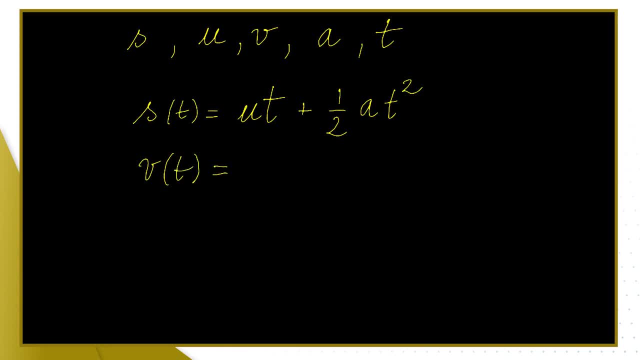 As to velocity, it is the initial velocity plus the acceleration times, the time elapsed. We can use these equations to derive others, So S can also be described as some sort of average of speed over time. The square of the velocity is also the square of the initial velocity. 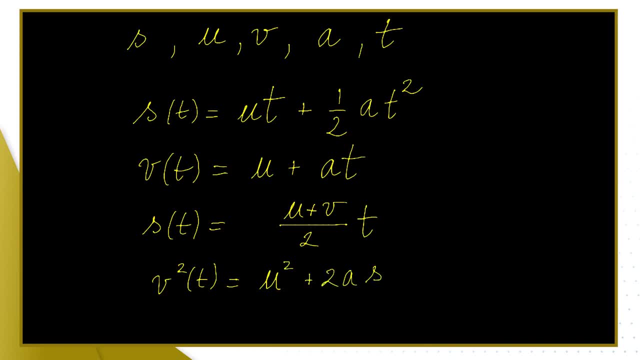 plus two times the acceleration times, the displacement, One more. We'll start with the final velocity times. T minus a half of A squared T squared. I'm going to remove the Ts there so we have a more traditional look of the Souvat equations. 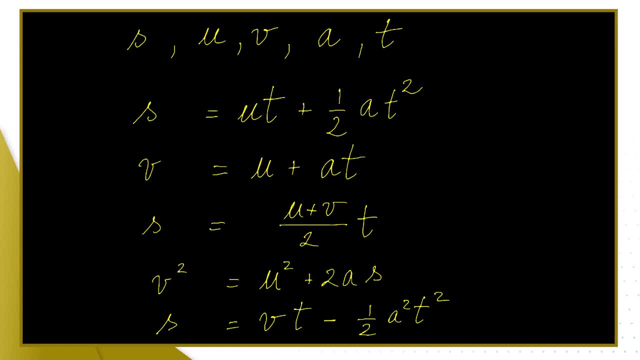 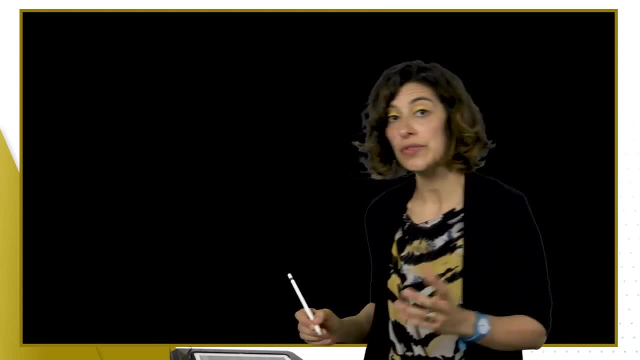 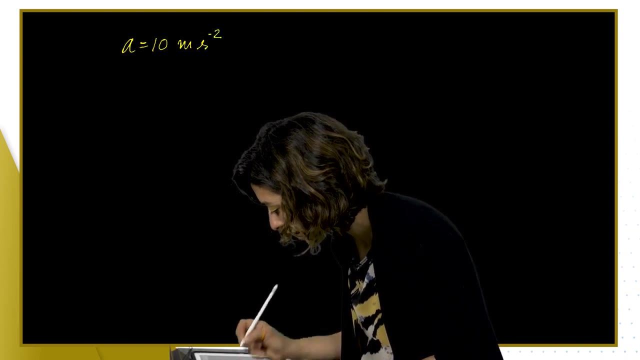 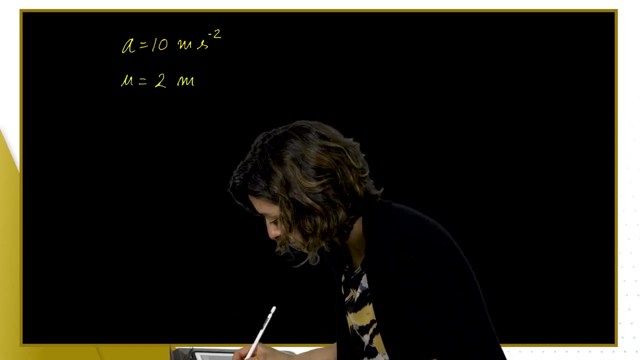 And let's look at a couple examples of how we use them. Say, we have an example. like we saw in the initial graphs, We had acceleration of 10 meters per second squared. So I'm going to do S to the minus two. The initial velocity was two meters per second. 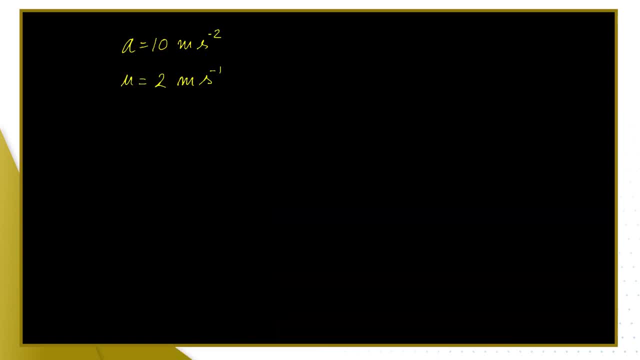 so second to the minus one, And I want to know how long it takes to move 600 meters. So we have S equals U T plus a half of A T squared. We have the initial velocity, We have the acceleration, We have the final position. 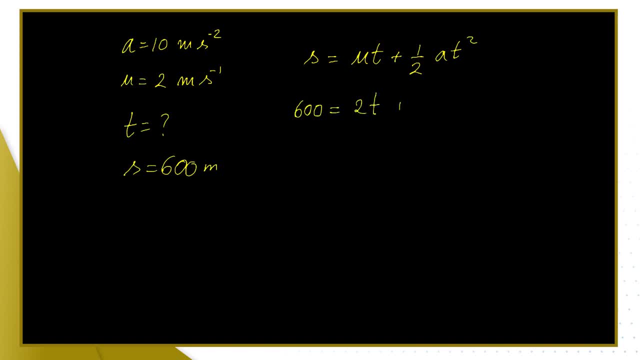 So the final position is two times T plus a half of 10 T squared. So 600 is two T plus five T squared And we're basically solving a quadratic equation And we can use the quadratic formula or factorize. Let's use quadratic formula. 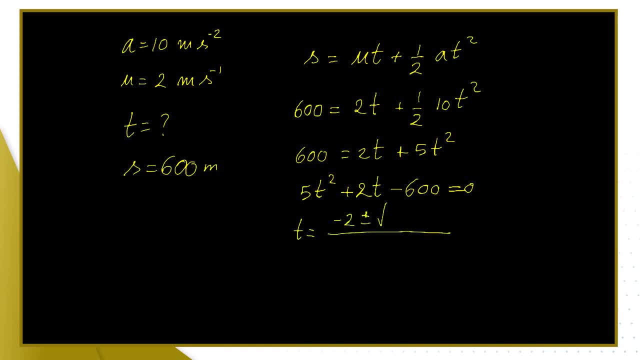 T equals minus B, so minus two plus or minus square root Of B squared, which is four minus four times A, which is five times C, which is minus 600 over two A, So two times five. This gives us minus two, plus or minus. 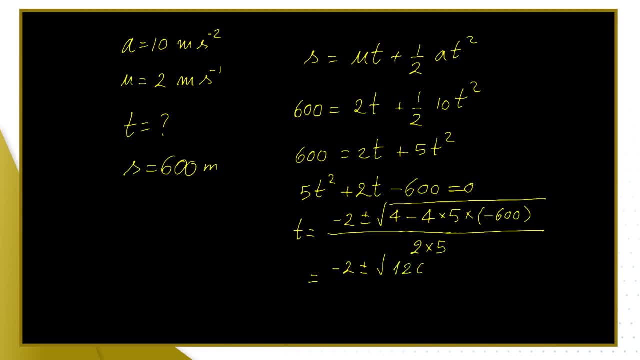 root of 1,204 divide by 10.. So minus two plus the root of 1,200.. 12,004 over 10. Or minus two, minus root of 1,2004 over 10. And that gives us 10.8 seconds. 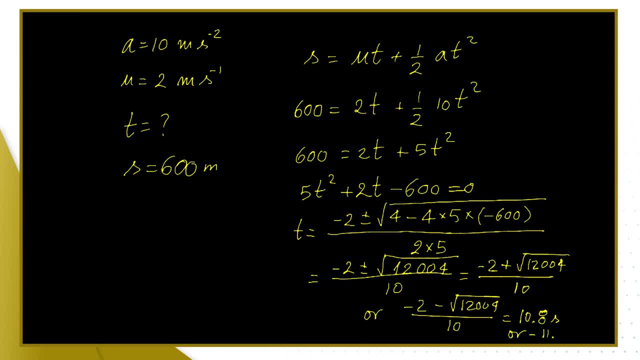 or minus 11.2 seconds. Now we're not going back in time, So the solution we want is: time equals 10.8 seconds over one decimal place. So after 10.8 seconds we achieve a position of 600 meters. 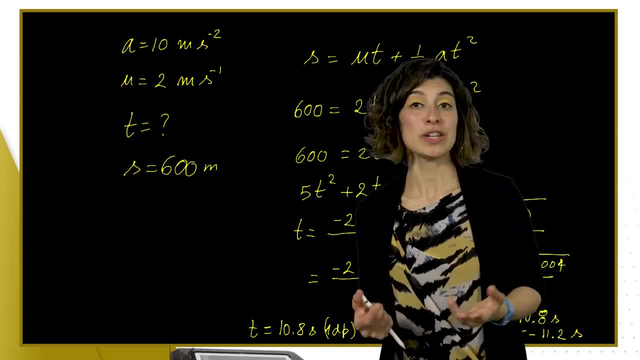 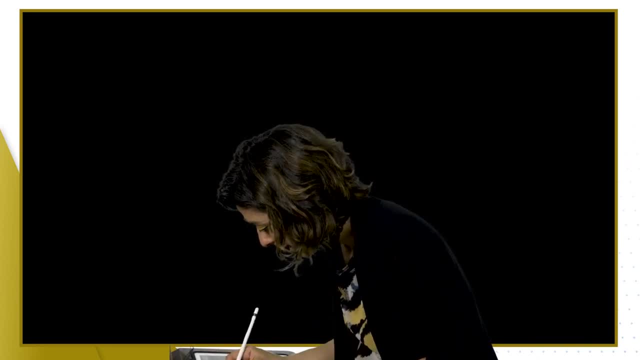 Another question could be how long it takes to get a speed of 400 meters per second. So we have the same data: A is 10 meters, second to the minus two, U is two meters to the minus one, And we want a speed. 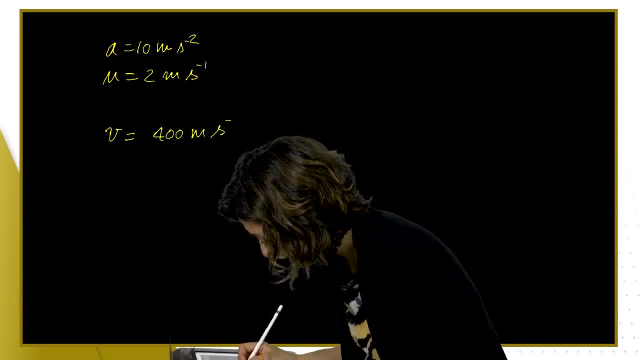 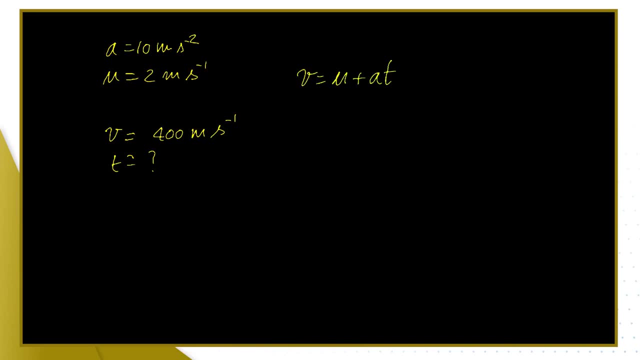 of 400 meters per second. How long does that take? We have that. V is U plus 80. We want 400 meters per second. We start at two. It accelerates 10 per second. So let's just solve that. 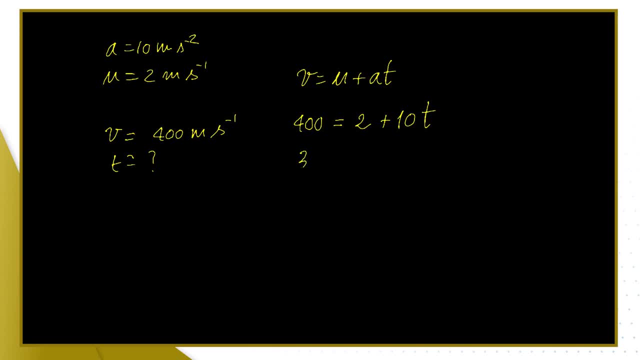 So we've got three. So 400 take away two. 398 equals 10T. That means that T equals 39.8 seconds. It takes 39.8 seconds to achieve the desired speed, So we use the velocity equation here. 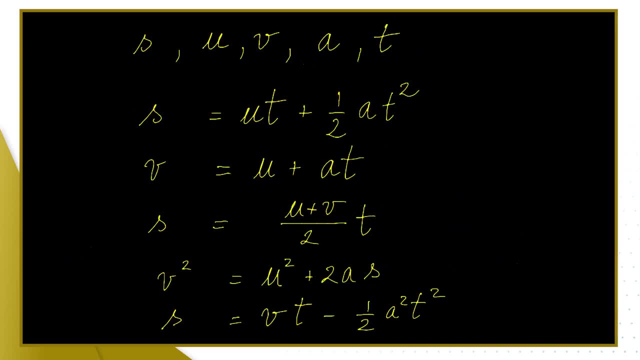 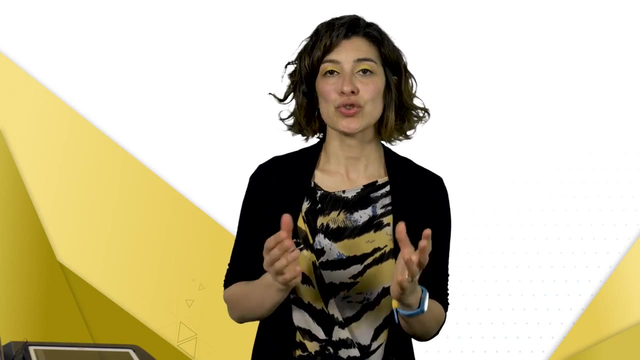 On the previous example, we used the position equation And then, depending on the problem, depending on the quantities you have, you choose the right relationship to obtain the quantity you want. Just one more note on graphs: The position graph against time should be a parabola. 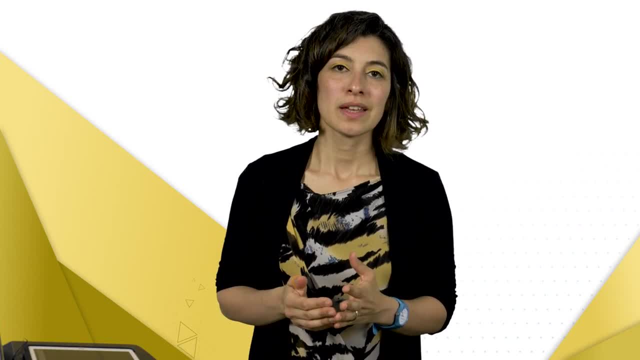 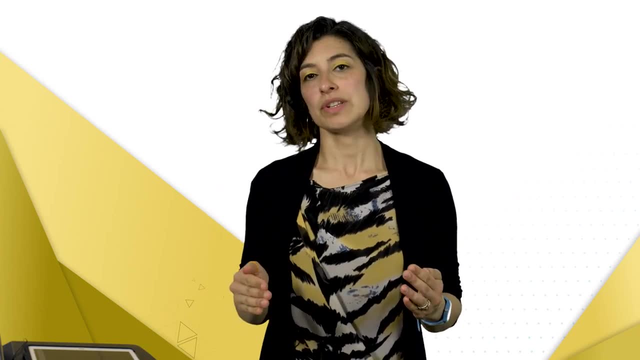 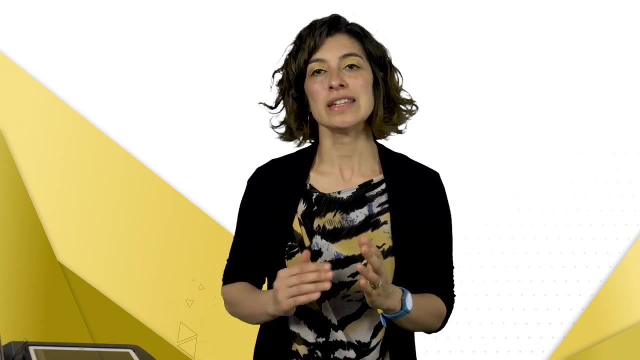 either upwards or downwards, depending on the acceleration. If the acceleration is positive, we have an upwards parabola. If it's negative, you have it pointing downwards. The velocity is always a straight line and is an ascending straight line if the acceleration is positive. 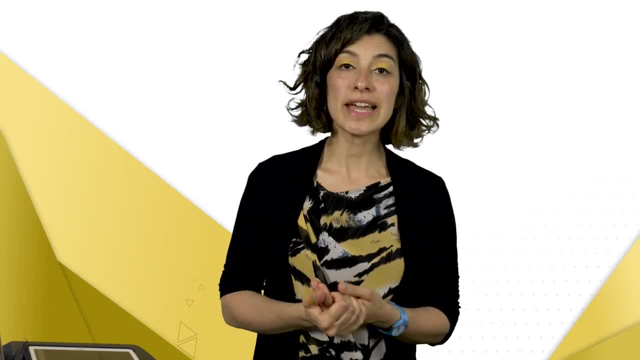 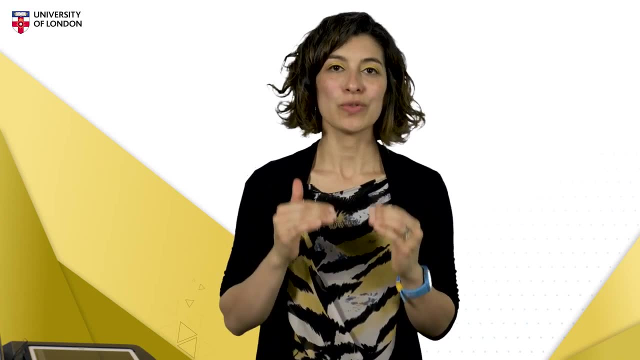 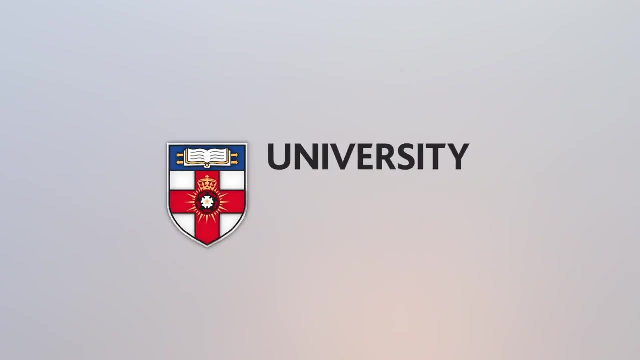 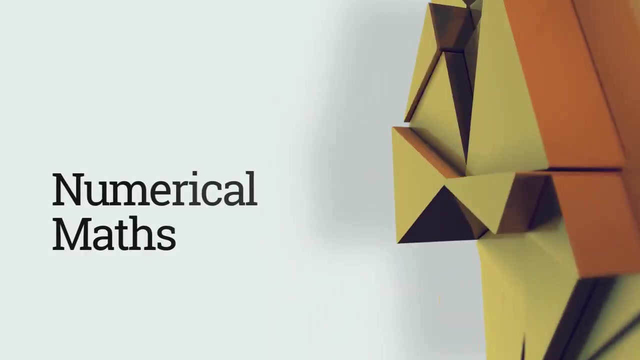 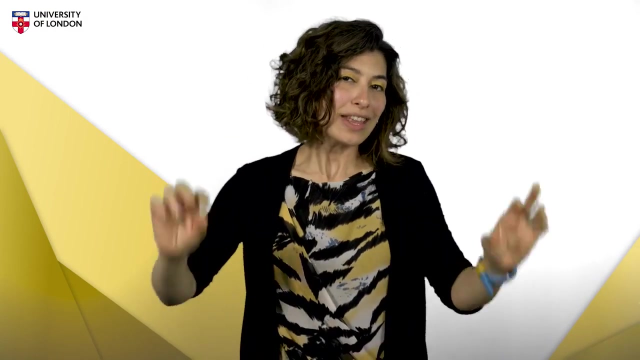 and is a descending straight line. if the acceleration is negative, The acceleration is always constant. therefore, it will always be a horizontal graph, Kinematic equations model, a very simple motion. It's so simple that we don't need to keep track of coordinates of the body that moves. We only need to track how far it moved from the starting point. This is because the movement is just on one straight line. That could be horizontal inclined or vertical. The trick is that the acceleration is constant, so the velocity changes linearly over time. 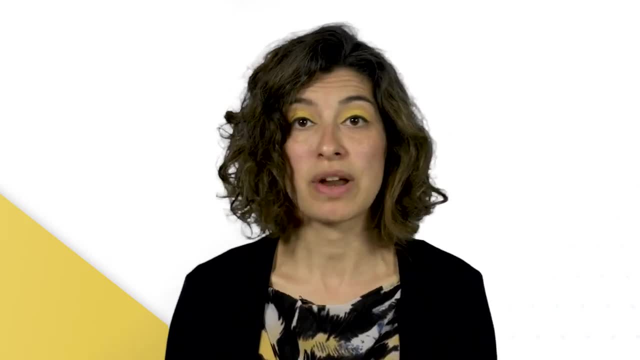 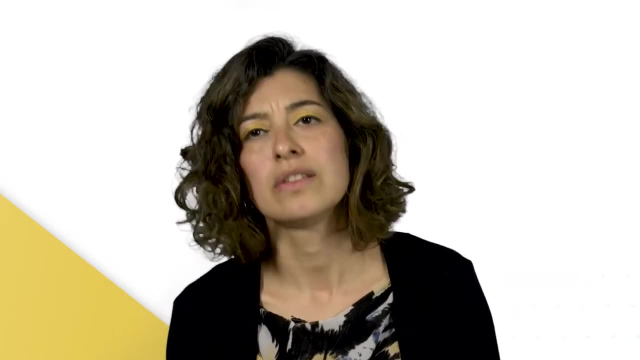 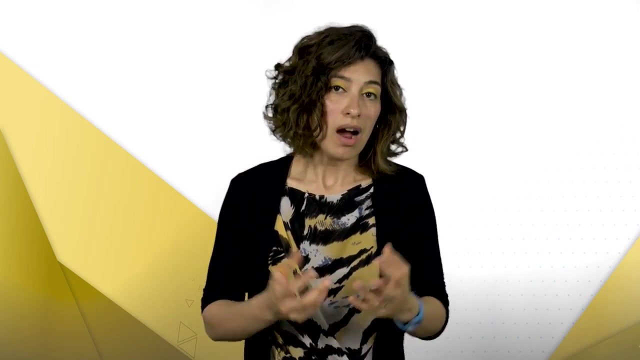 so only appearing t and numbers in the expression. and the position varies quadratically over time, So it features t, squared t and constants. This means that the graphs of these functions are quite simple too. Acceleration against time is a horizontal straight line. 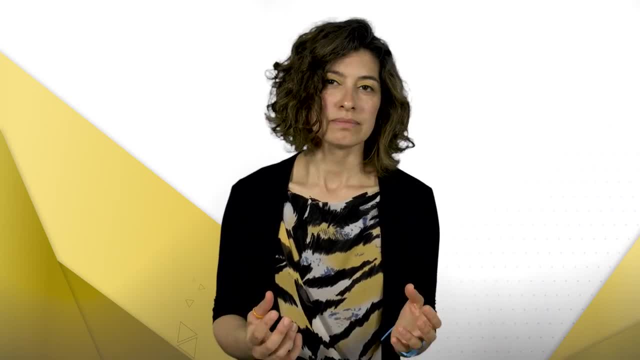 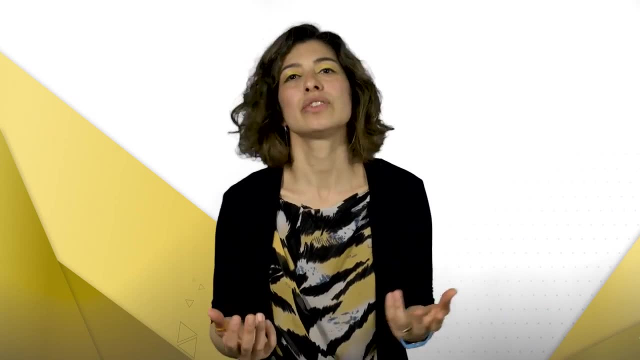 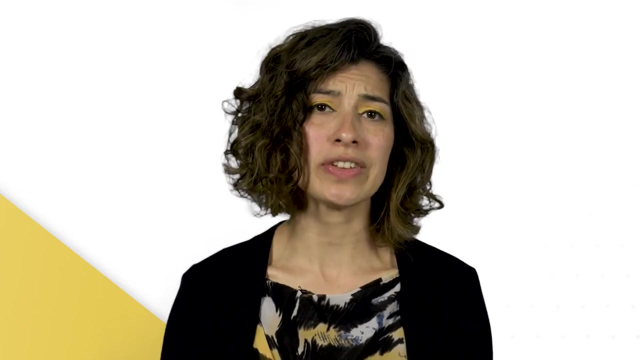 Velocity against time is a straight line and position against time is a parabola or a straight line, depending on whether the acceleration is not zero or zero respectively. The kinematic equations are often presented as SUVAT equations because of the S-U-V-A-T variables. 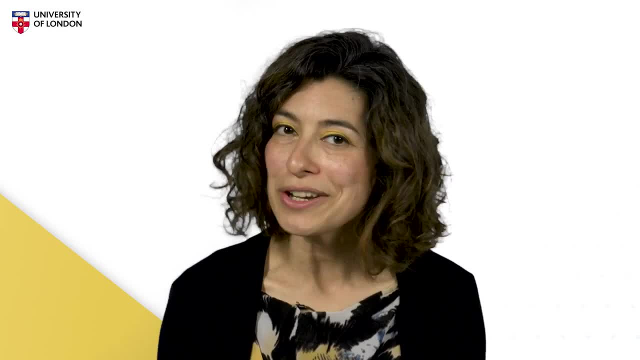 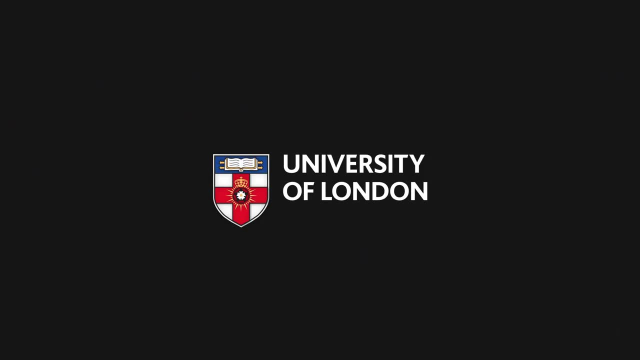 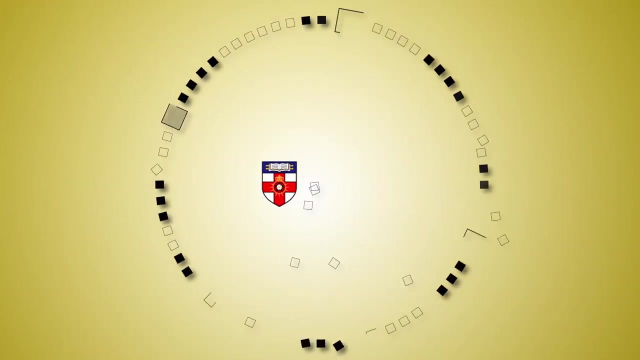 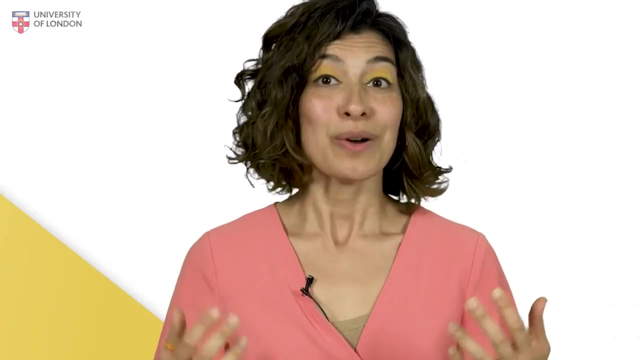 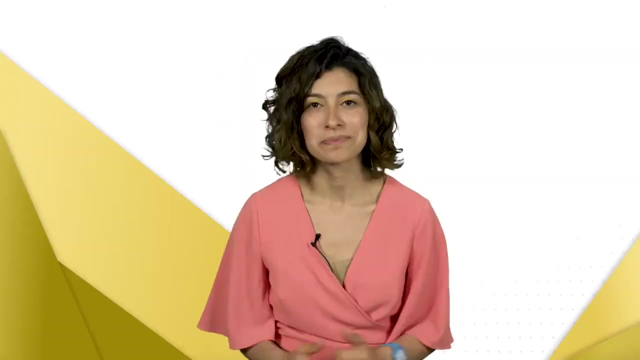 for position, initial velocity, final velocity, acceleration and time. And here you are at the end of the module. We looked at some mathematical tools that are a foundation for the numerical needs of a computer scientist. We looked at number basis and modular arithmetic.